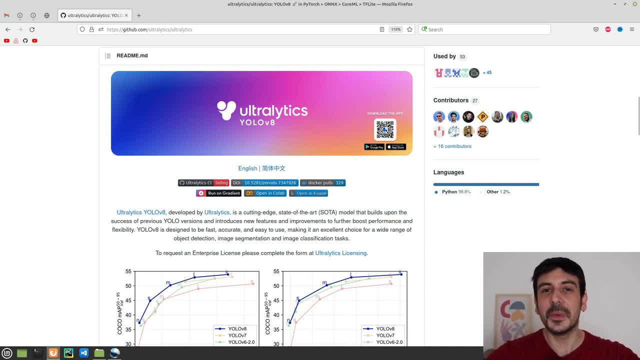 model you trained. So this is going to be a super comprehensive, step-by-step guide of everything you need to know in order to train an object detector using YOLOv8 on your own custom dataset. So let's get started. So let's start with today's tutorial. Let's start with this process And the first thing. 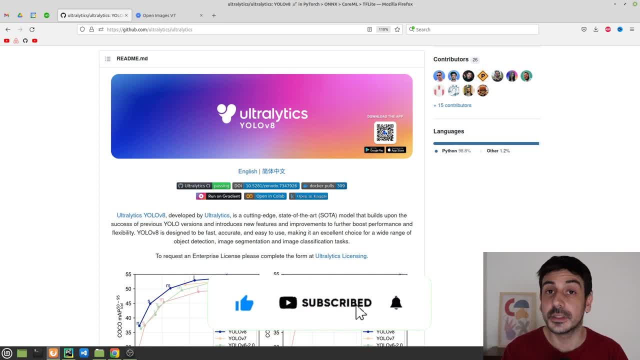 we need to do is to collect data. The data collection is the first step in this process. Remember that if you want to train an object detector or any type of machine learning model, you definitely need data, The algorithm, the specific algorithm you're going to use. 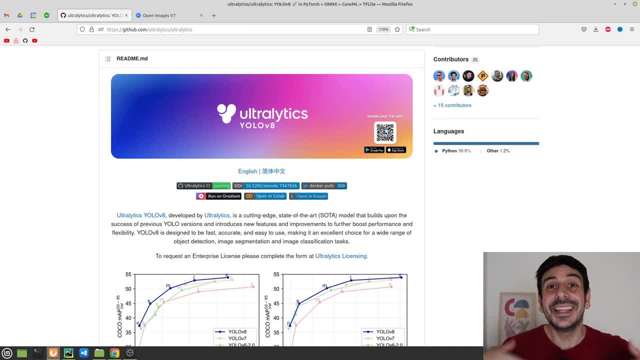 in this case YOLOv8, is very, very important, but the data is as important as the algorithm. If you don't have data, you cannot train any machine learning model. That's very important, So let me show you the data I am going to use in this process. These are some images. I am going to 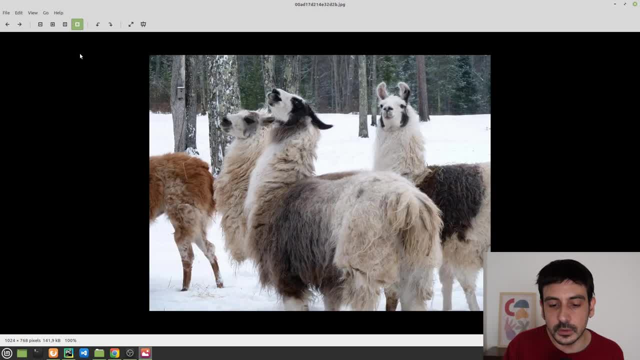 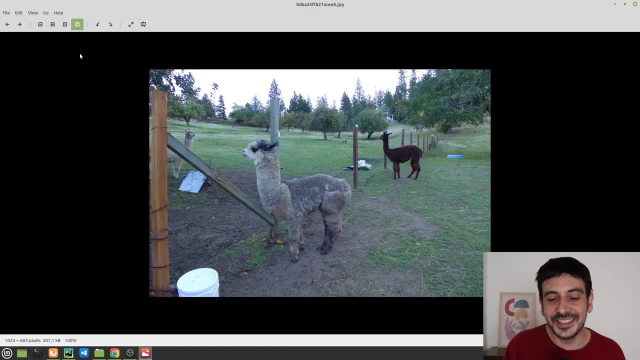 these are some images I have downloaded and which I'm going to use in this process. So let me show you, in order to train this object detector, And let me show you a few of them. These are some images of alpacas. This is an alpaca dataset I have downloaded for today's tutorial And you can see. 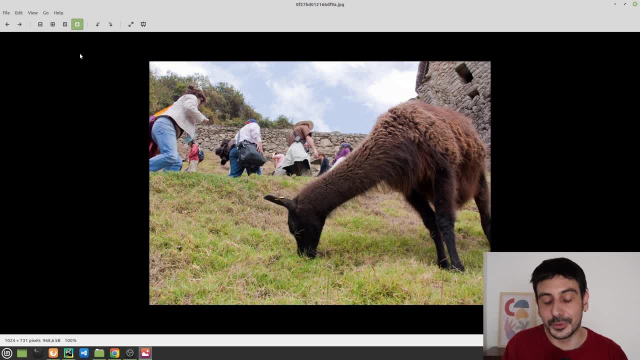 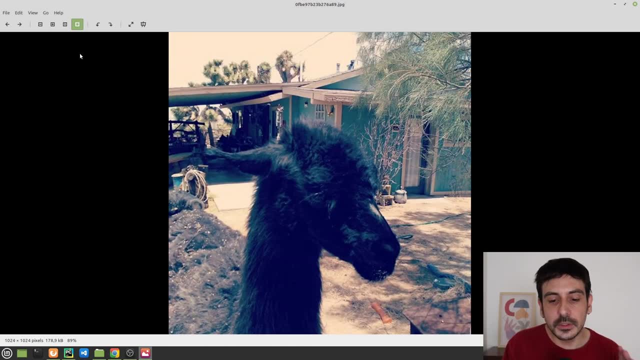 these are all images containing alpacas in different postures and in different situations. right, So this is exactly the data I am going to use in this process, but obviously you could use whatever dataset you want. You could use exactly the same dataset I am going to use, or you can. 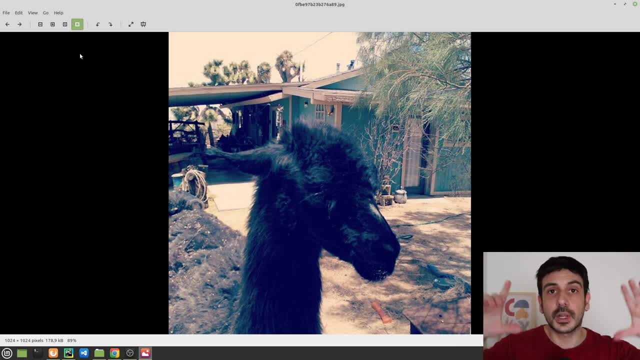 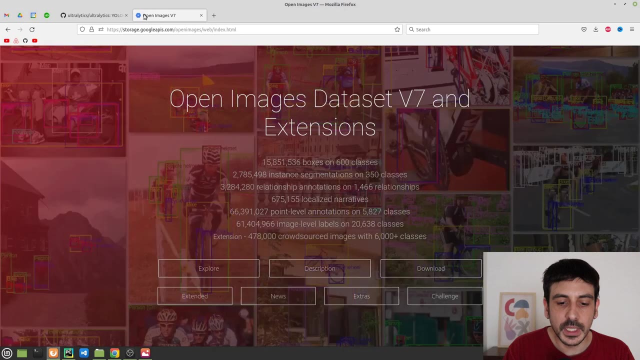 just take your cell phone or your camera or whatever, and you can just take the pictures, the photos, the images you are going to use. You can just do your own data collection, or something else you could do is to just use an available, a publicly available dataset. So let me show you. 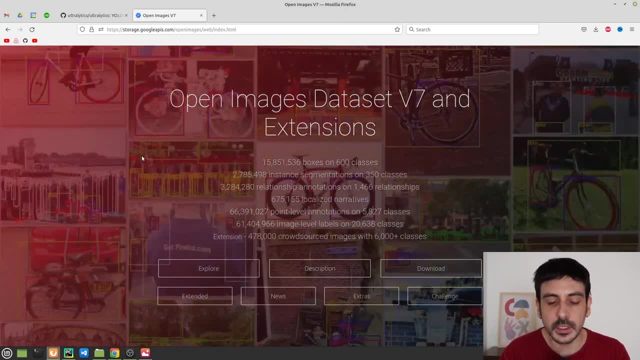 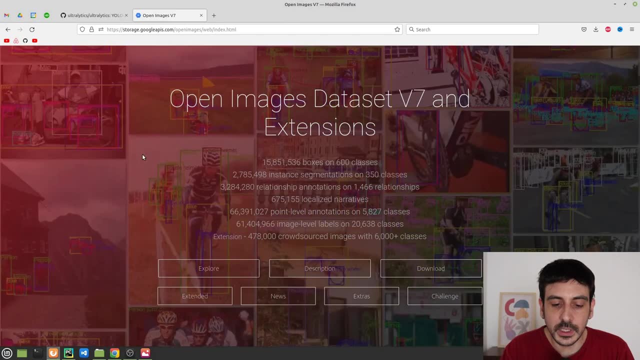 this dataset, This is the OpenImages dataset version 7, and this is a dataset which is publicly available and you can definitely use it in order to work on today's tutorial, in order to train the object detector which I am going to use in this process. 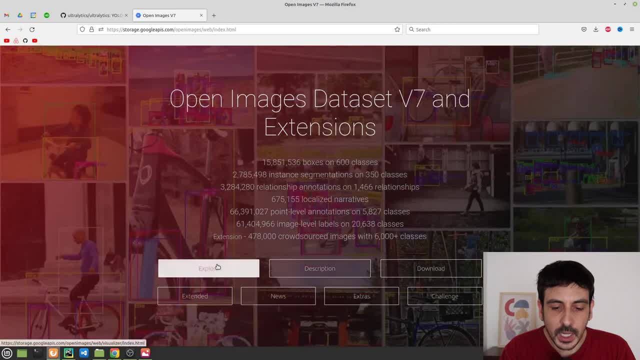 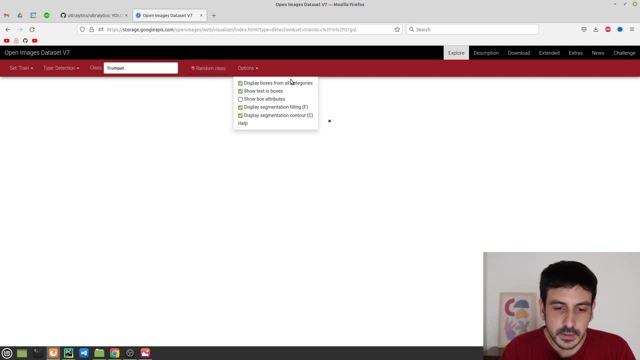 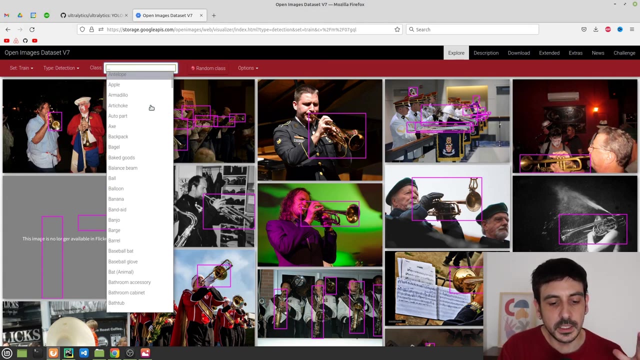 are going to train on today's tutorial, So let me show you how it looks like. If I go to explore and I select detection, you can see that I'm going to unselect all these options. You can see that this is a huge dataset containing many, many, many, many, many many categories. I 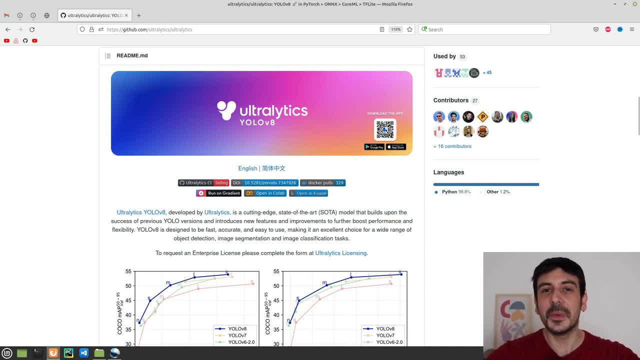 model you trained. So this is going to be a super comprehensive, step by step guide of everything you need to know in order to train an object detector using YOLOv8 on your own custom data set. So let's get started. So let's start with today's tutorial. Let's start with this process, And the first thing. 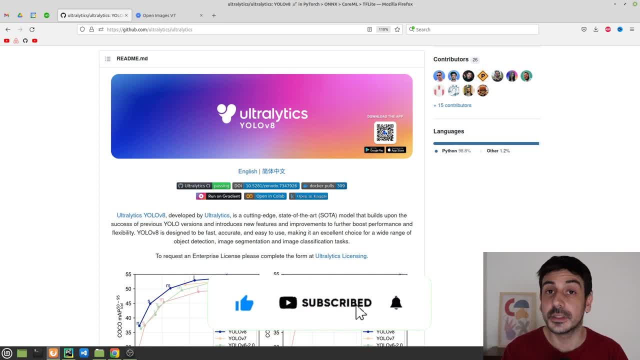 we need to do is to collect data. The data collection is the first step in this process. Remember that if you want to train an object detector or any type of machine learning model, you definitely need data, The algorithm, the specific algorithm you're going to use. 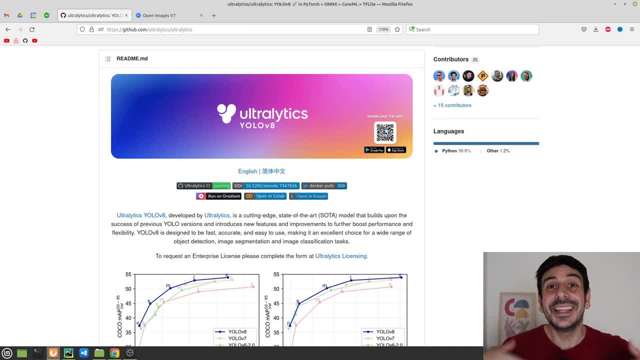 in this case, YOLOv8 is very, very important, but the data is as important as the algorithm. If you don't have data, you cannot train any machine learning model. That's very important, So let me show you the data I am going to use in this process. These are some images. I am going to 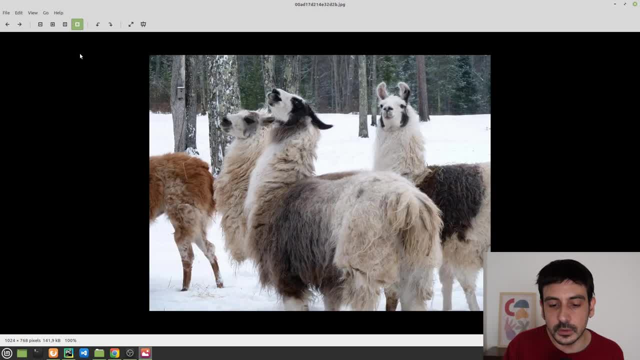 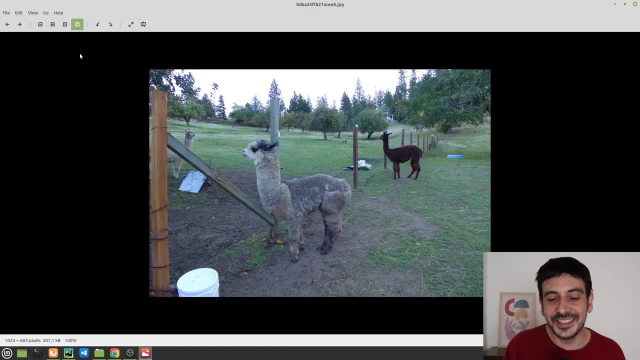 these are some images I have downloaded and which I'm going to use in this process in order to train this object detector, And let me show you a few of them. These are some images of alpacas. This is an alpaca data set I have downloaded for today's tutorial And you can see. 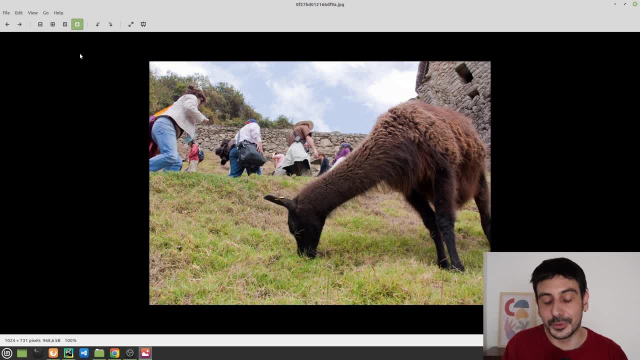 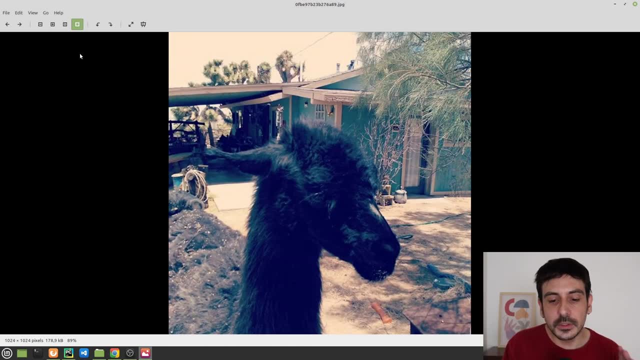 these are all images containing alpacas in different postures and in different situations. right, So this is exactly the data I am going to use in this process, but obviously you could use whatever data set you want. You could use exactly the same data set I am going to use, or you can. 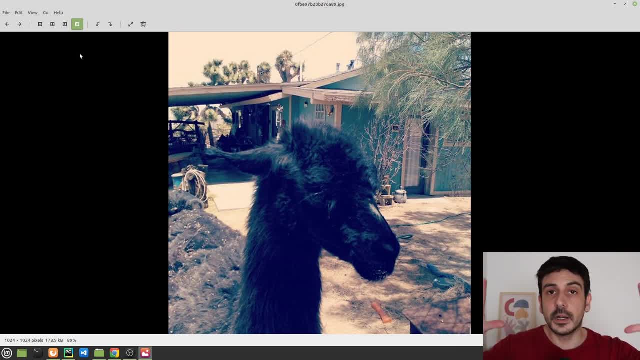 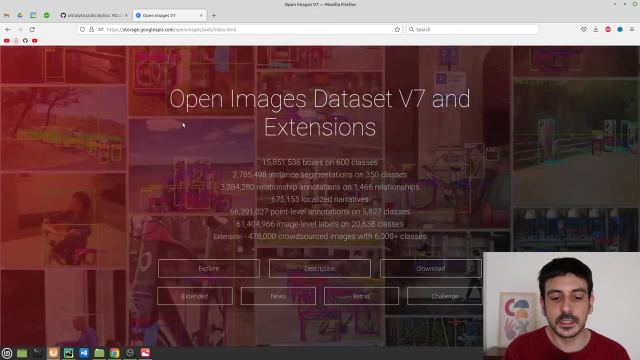 yourself. you could just take your cell phone or your camera or whatever, and you can just take the pictures, the photos, the images you are going to use. You can just do your own data collection, or something else you could do is to just use an available, a publicly available, data set. 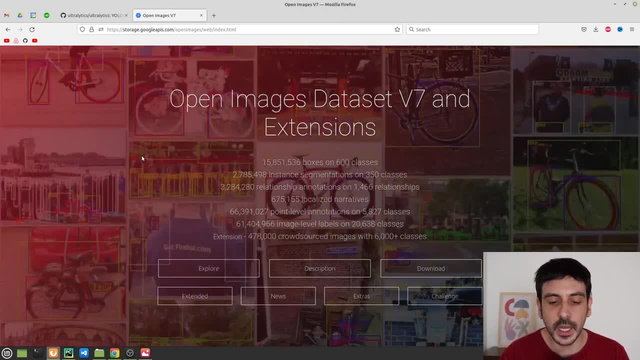 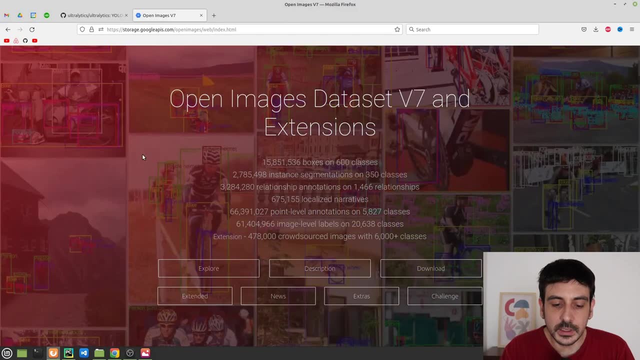 So let me show you this data set, This is the open images data set, version seven, and this is a data set which is publicly available and you can definitely use it in order to work on today's tutorial, in order to train the object detector. 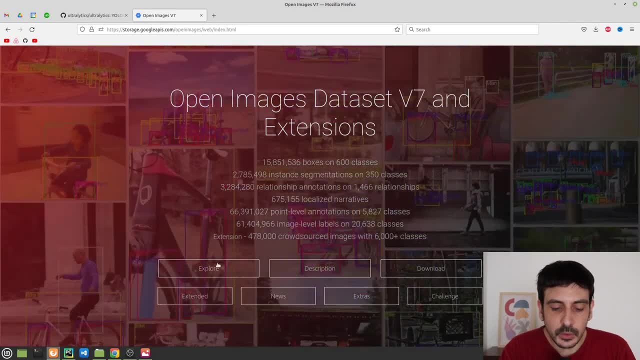 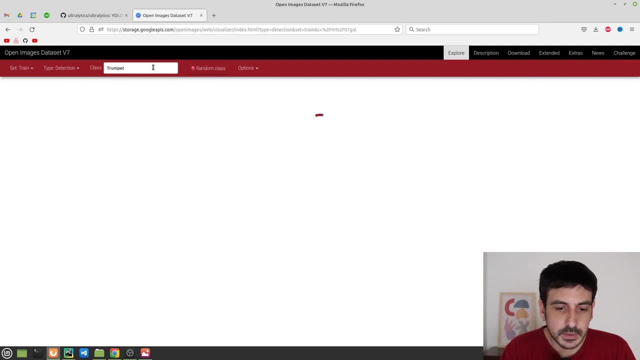 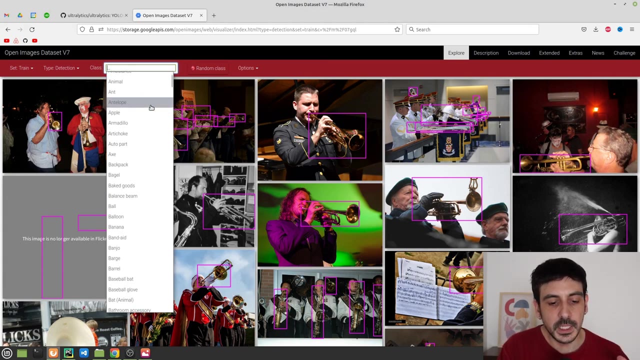 we are going to train on today's tutorial, So let me show you how it looks like. If I go to explore and I select detection, you can see that I'm going to unselect all these options. You can see that this is a huge data set containing many, many, many, many, many many. 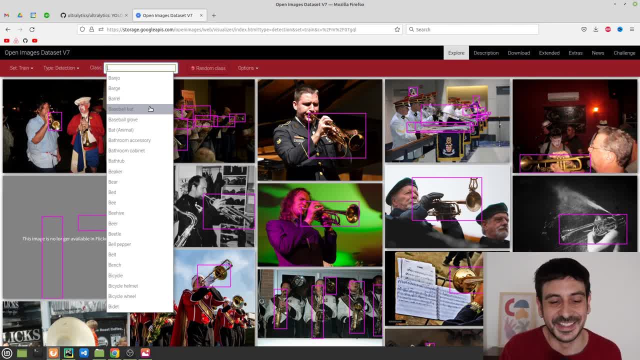 categories. I don't know how many, but they are many. This is a huge data set. It contains millions of images, hundreds of thousands, if not millions, of annotations, thousands of categories. This is a super, super, super huge data set And you can see that you have many. 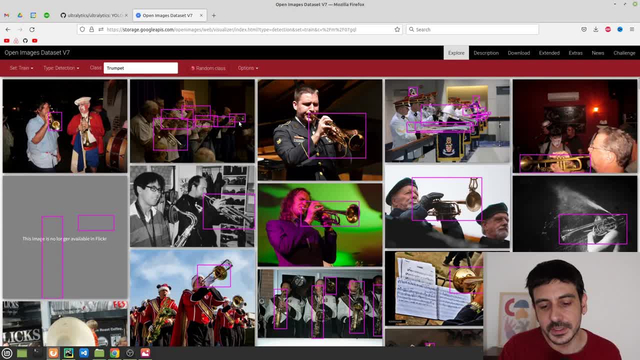 many different categories. Now we are looking at trumpet And you can see these are different images with trumpets And from each one of these images we have a bounding box around the trumpet. And if I show you another one, for example, we also have a beetle And in this category 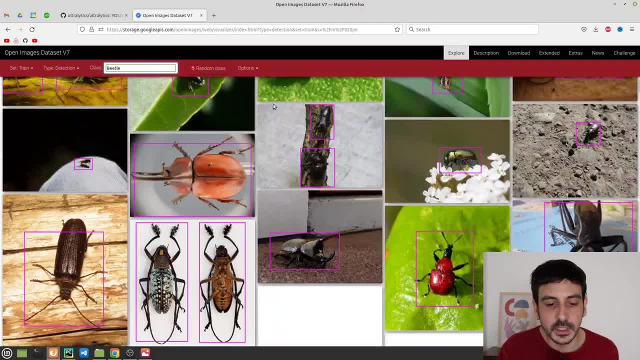 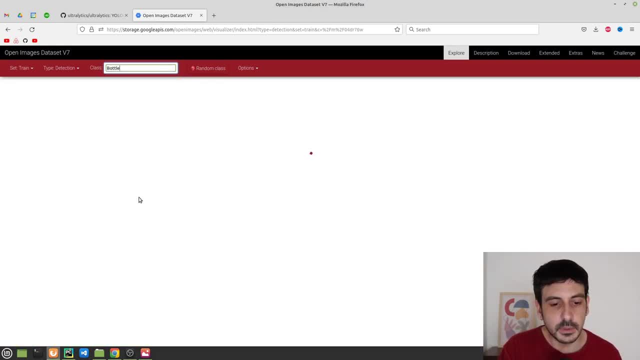 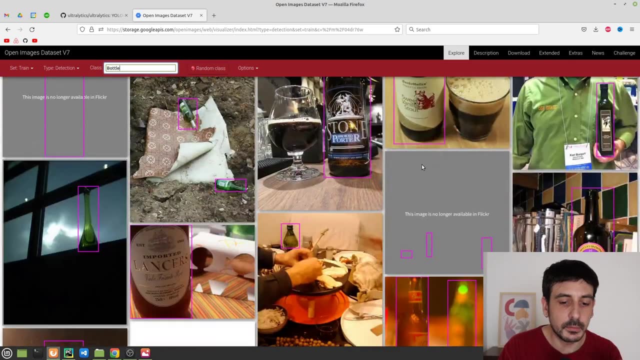 you can see, we have many different images from many different types of beetles. so this is another example. or, if I show you this one, which is bottle, and we have many different images containing bottles, for example, there you can see many different type of bottles and in all cases we have a bounding box around the bottle, and I could show you. I don't know how. 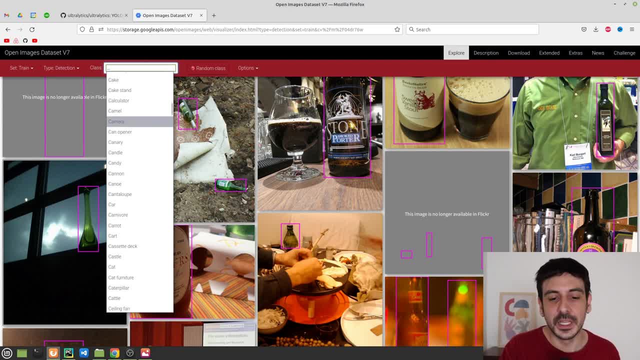 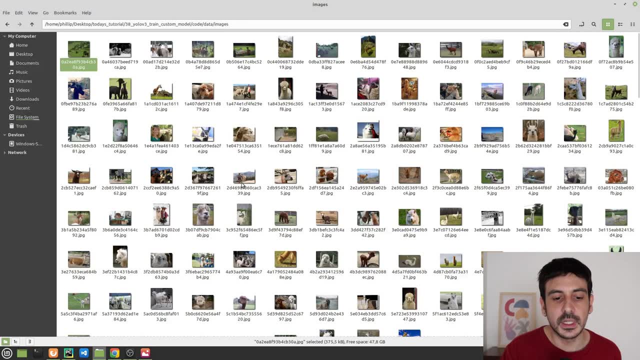 many examples because there are many, many, many different categories. so, remember, the first step in this process is the data collection. this is the data I am going to use in this project, which is a dataset of alpacas, and you can use the exact same data I am using if you want to. you can use. 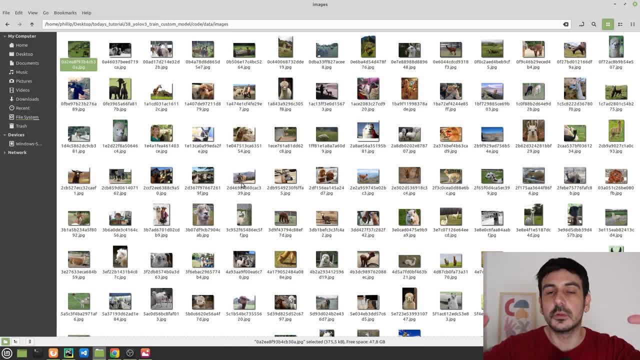 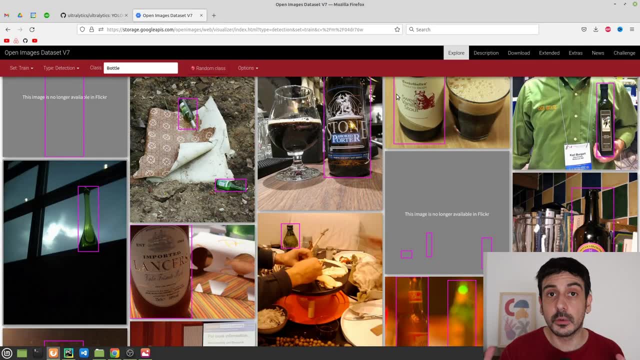 the same dataset of alpacas, or you can just collect your own dataset by using your cell phone, your camera or something like that, or you can also download the images from a publicly available dataset, for example open images dataset version 7. if you decide to use open images dataset version 7. 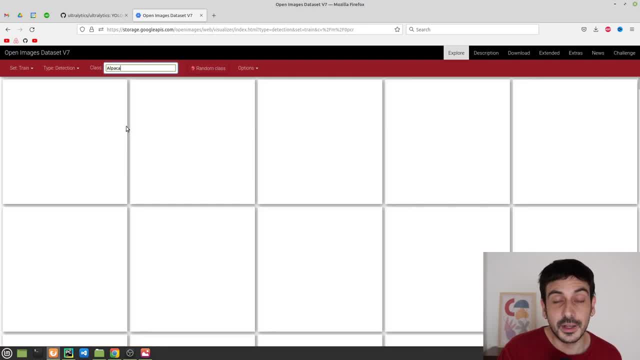 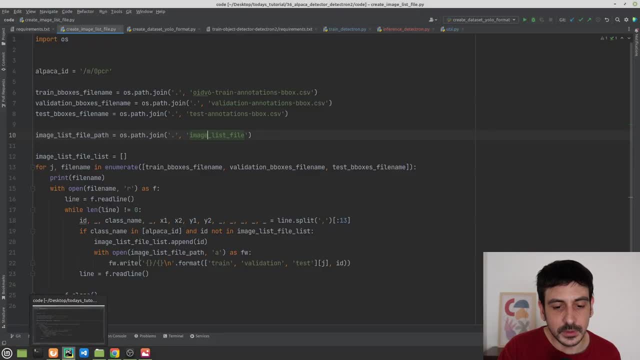 let me show you another category, which is alpaca. this is exactly from where I have downloaded all the images of alpacas. so if, in case, you decide to use this publicly available dataset, i can provide you with a couple of scripts i have used in order to download all this data. 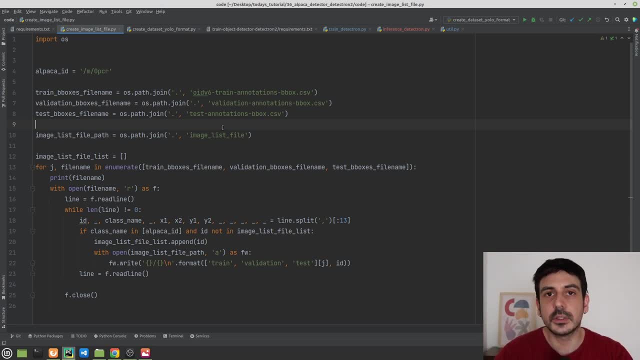 and in order to parse through all the different annotations and through to format this data in exact the exact format we need in order to work on today's tutorial. so, in case you decide to use open image data set, i am going to give you a couple of scripts which are going to be super. 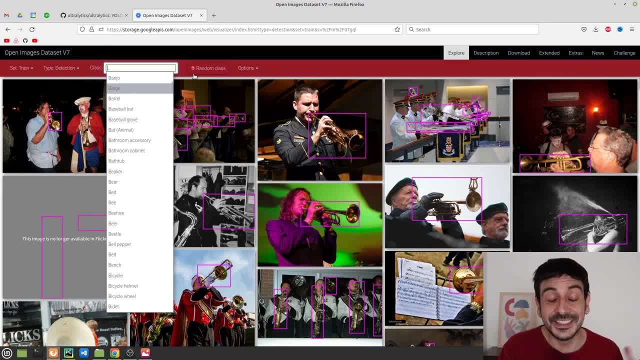 don't know how many, but there are many. This is a huge dataset. It contains millions of images, thousands, if not millions, of annotations, thousands of categories. This is a super, super, super huge dataset and you can see that you have many, many different categories Now. 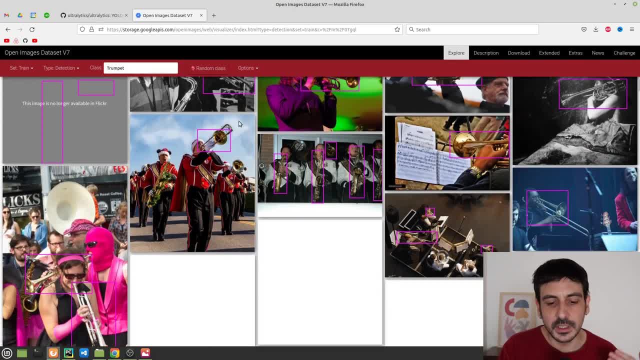 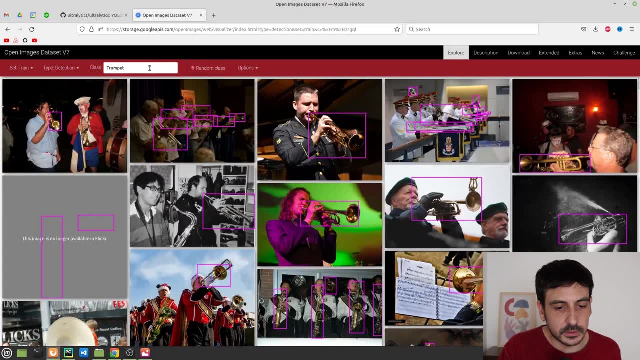 we are looking at trumpet and you can see these are different images with trumpets and from each one of these images we have a bounding box around the trumpet. And if I show you another one, for example, we also have a beetle and in this category you 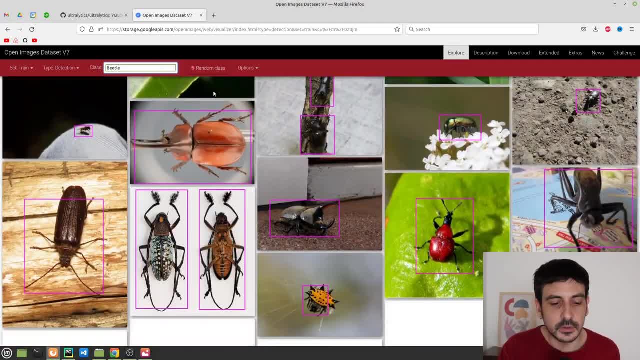 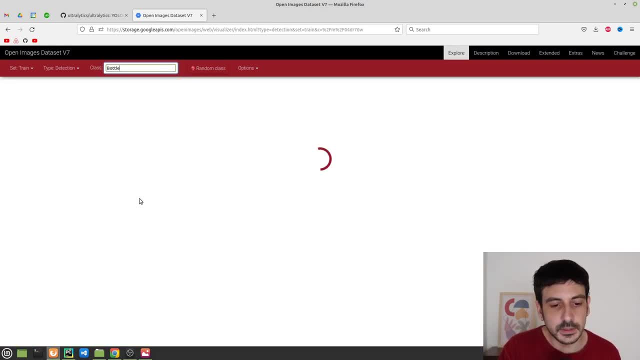 can see, we have many different images from many different types of beetles. So this is another example. Or, if I show you this one which is a bottle, and we have many different images containing bottles, For example, there you can see many different types of bottles and in all cases we 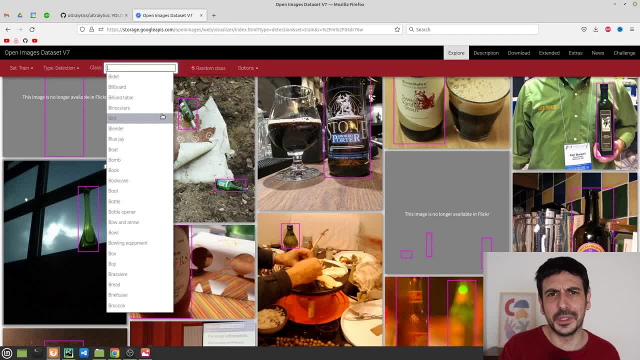 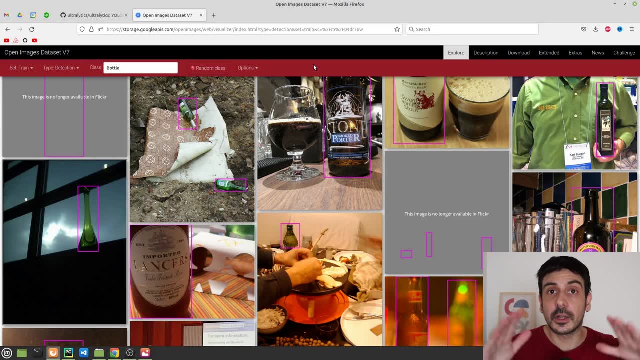 have a bounding box around the bottle, And I could show you I don't know how many examples, because there are many, many, many different categories. So remember: the first step in this process is the data collection. This is the data I am going to use in this project, which is a dataset of alpacas. 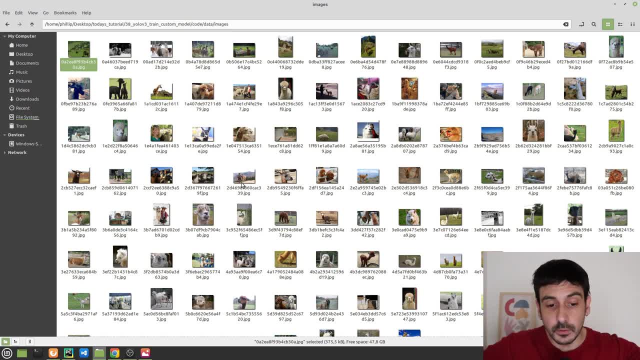 and you can use the exact same data that I am going to use in this project, which is a dataset of alpacas. If you want to, you can use the same dataset of alpacas, or you can just collect your own dataset by using your cell phone, your camera or something like that, Or you can also download. 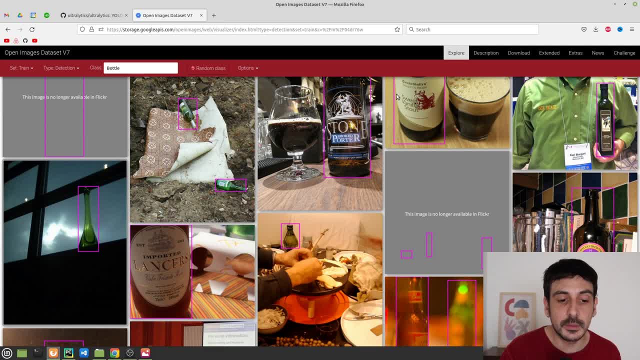 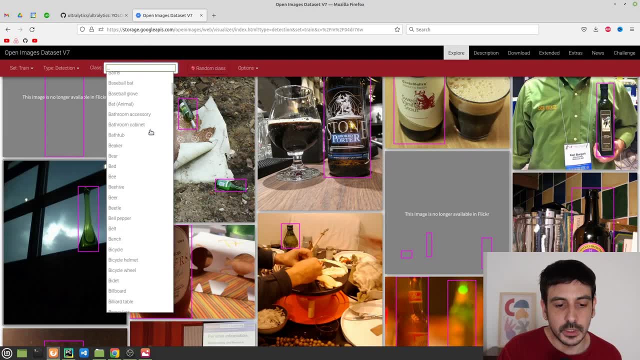 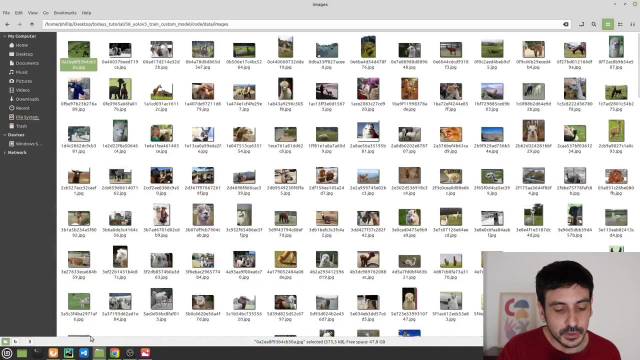 the images from a publicly available dataset, for example OpenImages dataset version 7.. If you decide to use OpenImages dataset version 7, let me show you another category, which is alpaca. This is exactly from where I have downloaded all the images of alpacas. So if 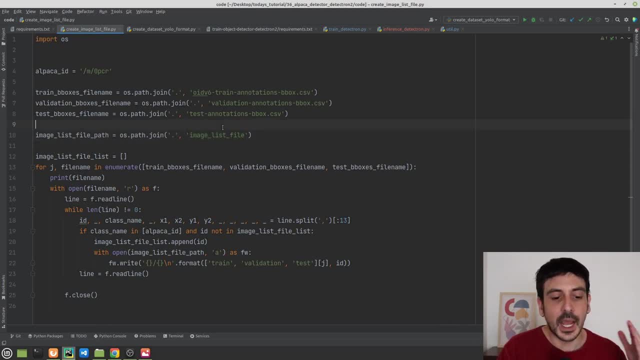 in case you decide to use this publicly available dataset, I can provide you with a couple of scripts I have used in order to download all this data and in order to parse through all the different annotations and to format this data in the exact format we need in order to 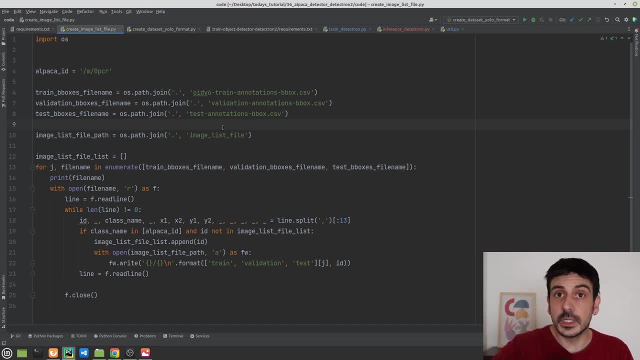 work on today's tutorial. So, in case you decide to use OpenImages dataset, I am going to give you a couple of scripts which are going to be super, super useful for you. So that's all I can say about the data collection. Remember, you need to collect data if you want to train an object. 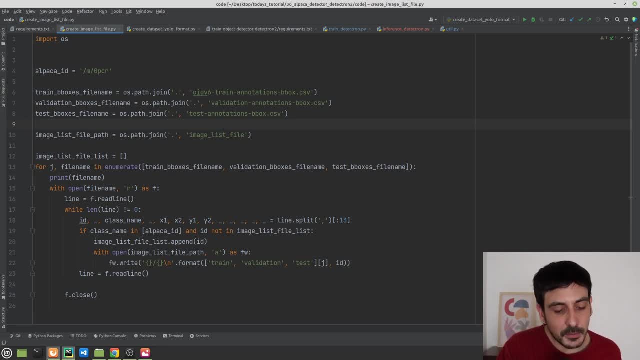 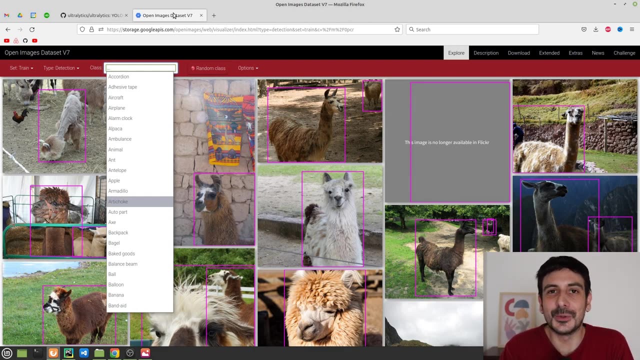 super useful for you. so that's, that's all i can say about the data collection. remember, you need to collect data if you want to train an option detector, and you have all those different ways to do it and all these different categories and all these different options. so now let's move on. 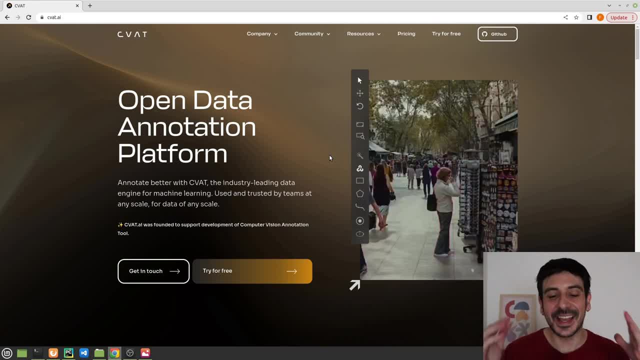 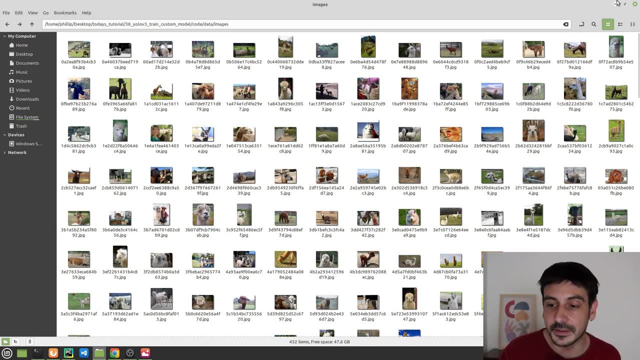 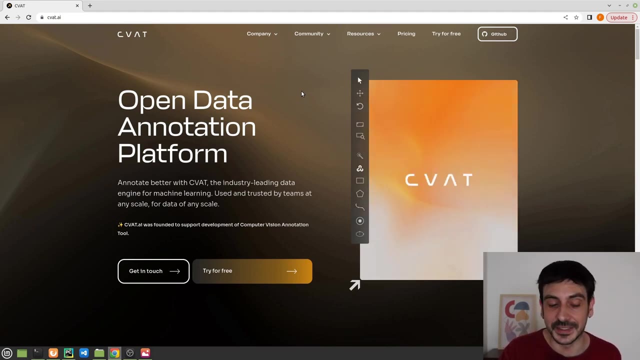 to the next step, and now let's continue with the data annotation. you have collected a lot of images, as i have over here. you have a lot of images which you have collected yourself, or maybe you have downloaded this data from a publicly available data set, and now it's the time to annotate this data set. maybe you were lucky enough when you were. 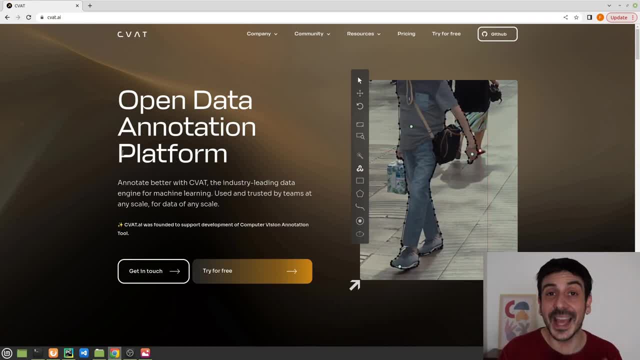 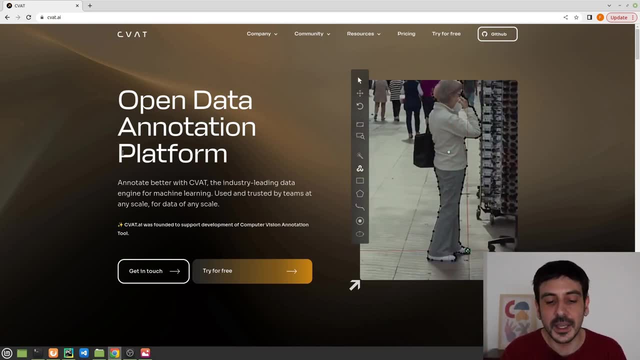 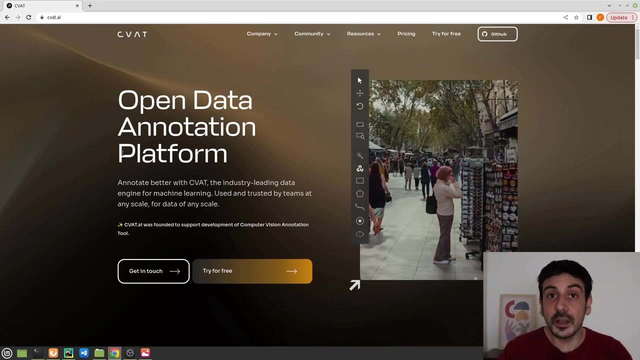 creating the asset and maybe this data set you are using is already annotated. maybe you already have all the bounding boxes from all of your objects, from all your categories. maybe that's the case, so you don't really need to annotate your data. but in any other case, for example, if you were using a 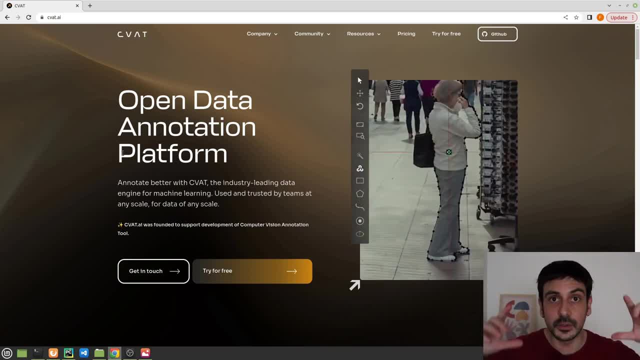 custom data set, a data set you have collected yourself with your own cell phone, your camera and so on, something you have collected. in that case, you definitely need to annotate your data. so, in order to make this process more comprehensive, in order to show you like the entire process, let me show. 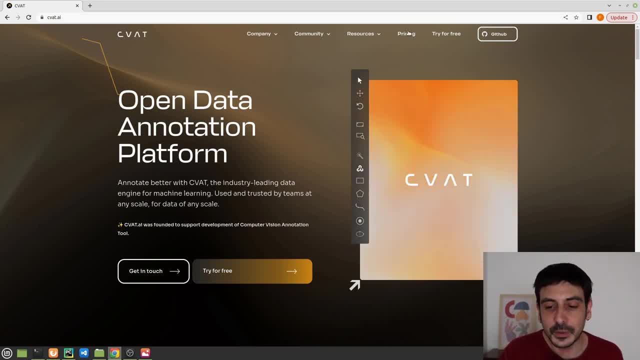 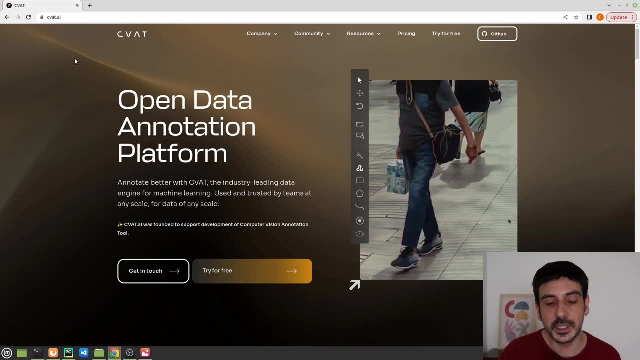 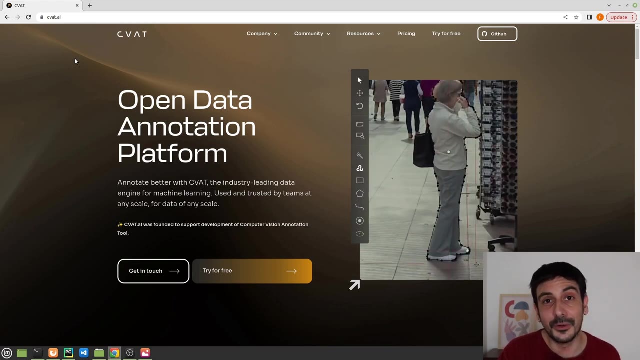 you as well how to annotate data, so we are going to use this tool, which is cbat. this is a labeling tool. i have used it many, many times in many projects. i would say it's one of my favorite tools. i have used pretty much absolutely all the object detection, computer vision related. 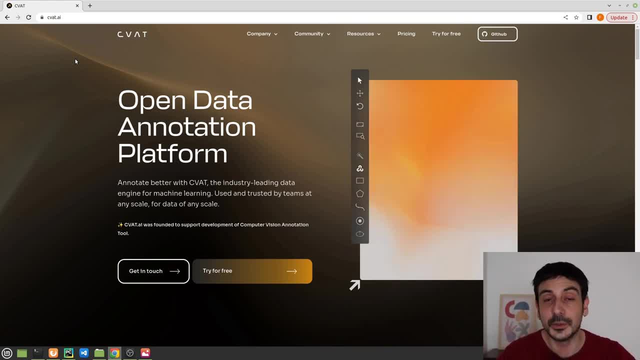 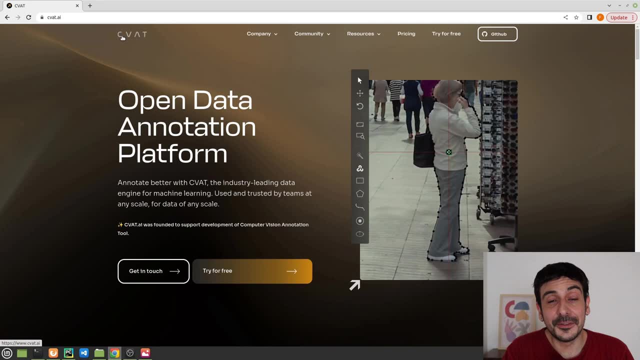 annotation tools i have used. maybe i haven't used them all, but i have used many, many, many of them and if you are familiar with annotation tools, you would know that there are many, many of them and none of them is perfect. i would say. all of the different annotation tools have their advantages. 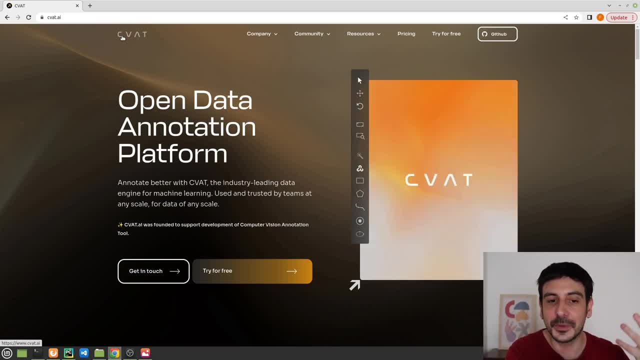 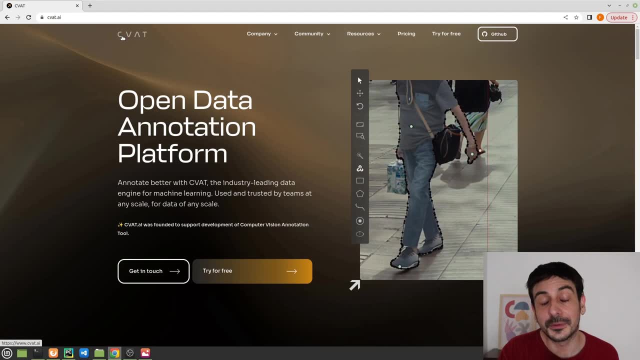 and their disadvantages, and for some situations you prefer to use one of them, and for situations it's better to use another, and for other situations it's better to use another one. CBAT has many advantages and it also has a few disadvantages. I'm not saying it's perfect. 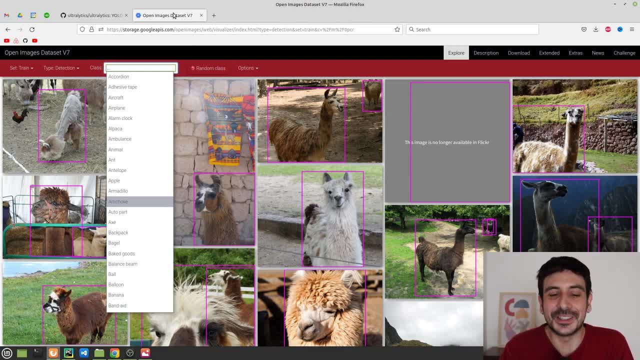 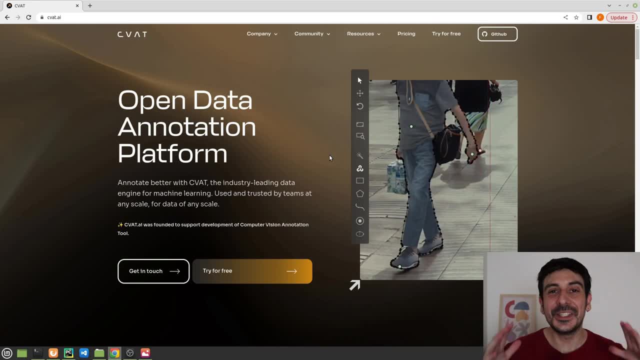 detector, and you have all those different ways to do it and all these different categories and all these different options. So now let's move on to the next step. And now let's continue with the data annotation. You have collected a lot of images, as I have over 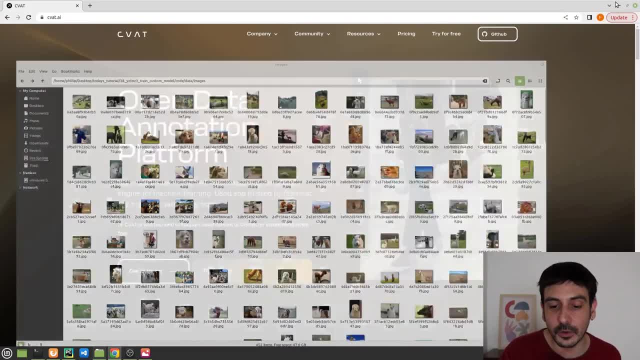 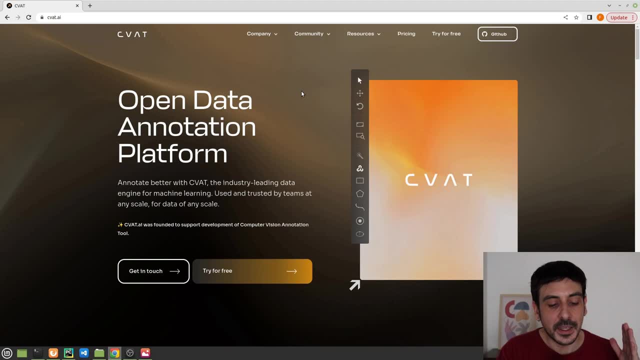 here You have a lot of images which you have collected yourself, or maybe you have downloaded this data from a publicly available dataset and now it's the time to annotate this dataset. Maybe you were lucky enough when you were creating the dataset, and maybe this dataset 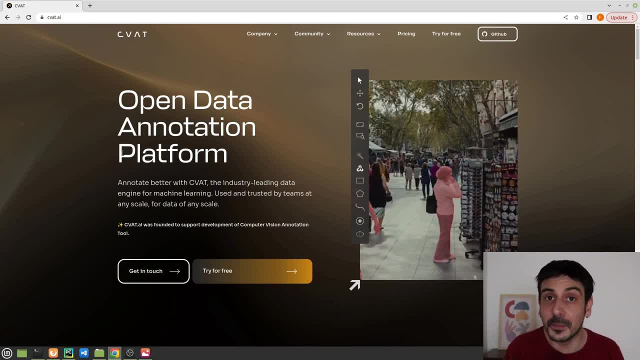 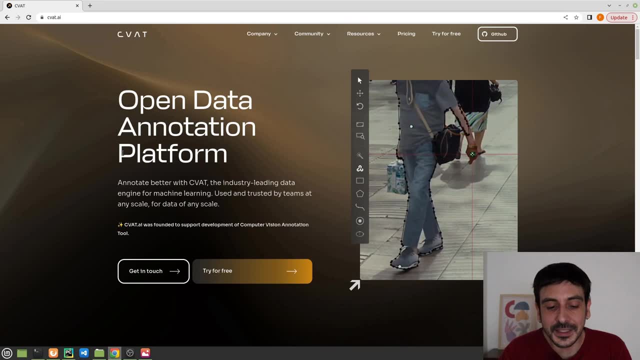 you are using is already annotated. maybe you already have all the bounding boxes from all your objects, from all your categories. maybe that's the case, So you don't really need to annotate your data. but in any other case, for example, if you were using a custom dataset- 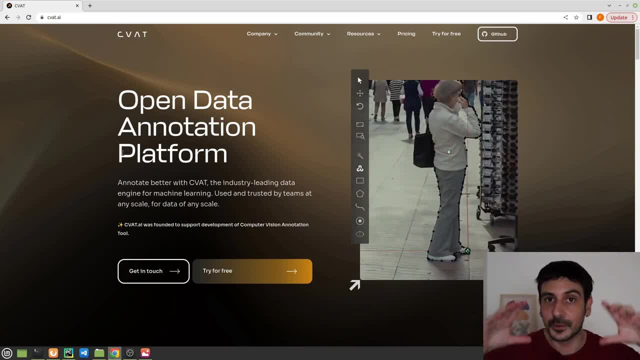 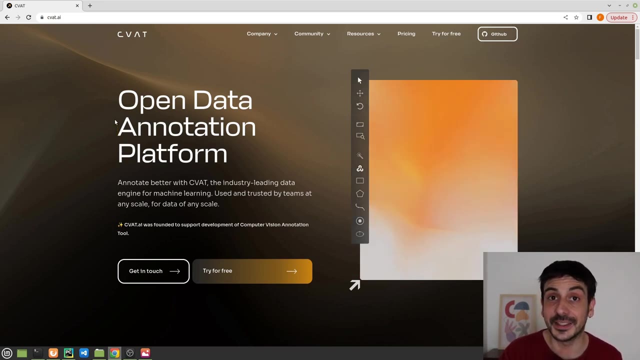 a dataset you have collected yourself with your own cell phone, your camera and so on, something you have collected. In that case, you definitely need to annotate your data. So, in order to make this process more comprehensive and in order to show you like the entire process, let me show you as well how to annotate data. 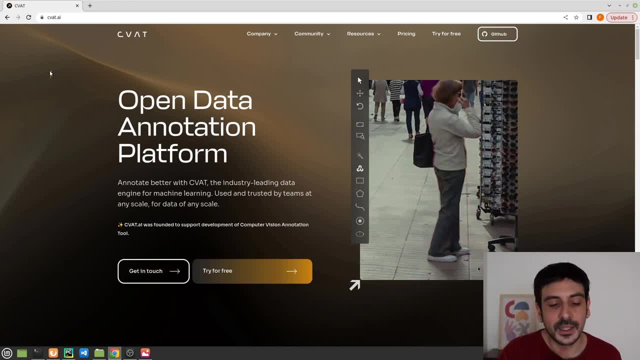 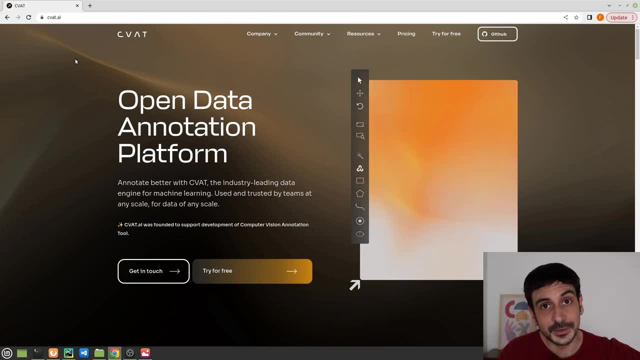 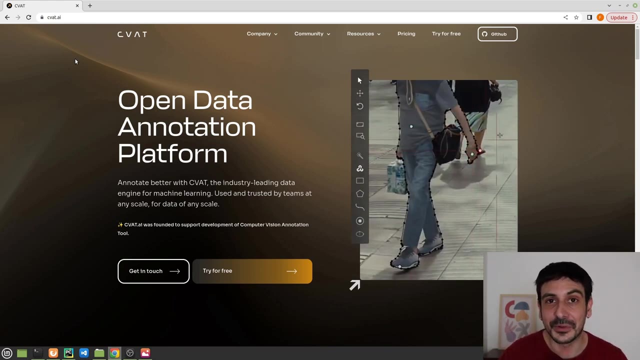 So we are going to use this tool, which is C-B-A-T. This is a labeling tool. I have used it many, many times in many projects. I would say it's one of my favorite tools. I have used pretty much absolutely all the object detection, computer vision related annotation tools. I've 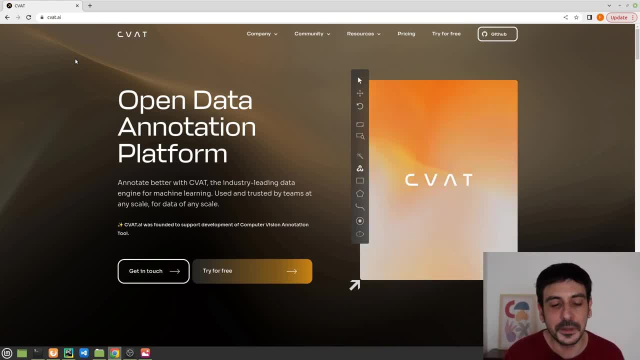 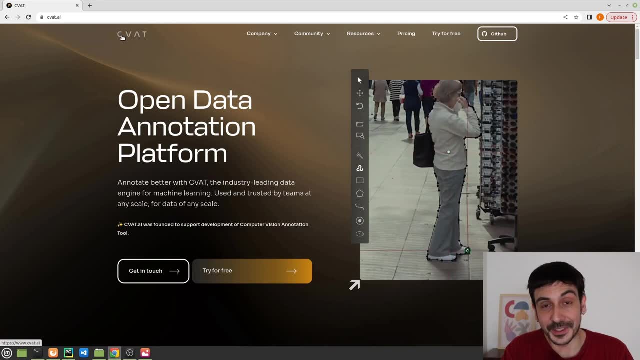 used. maybe I haven't used them all, but I have used many, many, many of them and if you are familiar with annotation tools, you would know that there are many, many of them and none of them is perfect, I would say. all of the different annotation tools have their advantages and their 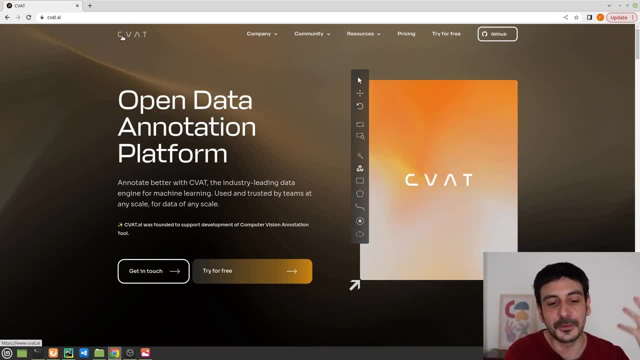 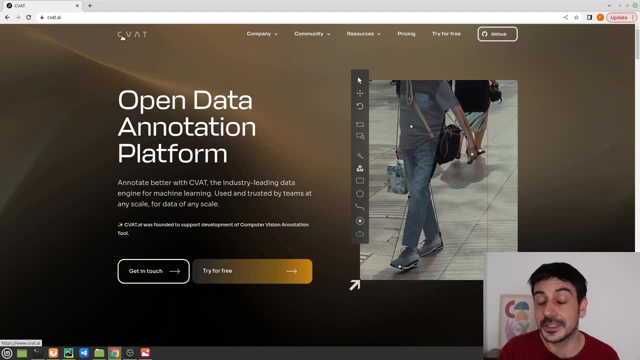 disadvantages, and for some situations you prefer to use one of them, and for other situations it's better to use another one. C-B-A-T has many advantages and it also has a few disadvantages. I'm not saying it's perfect, but nevertheless this is a tool I have used in many, many, many 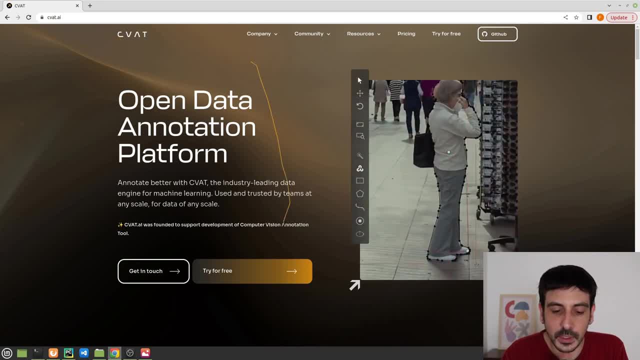 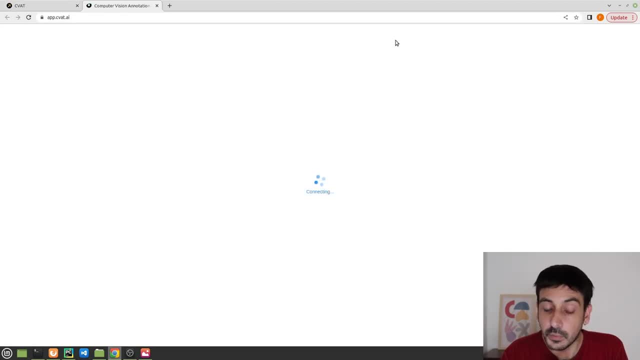 projects and I really, really like it. So let me show you how to use it. You have to go to cbatai and then you select: try for free. There are different pricing options, but if you are going to work on your own or in a very small team, you can definitely use the free version. 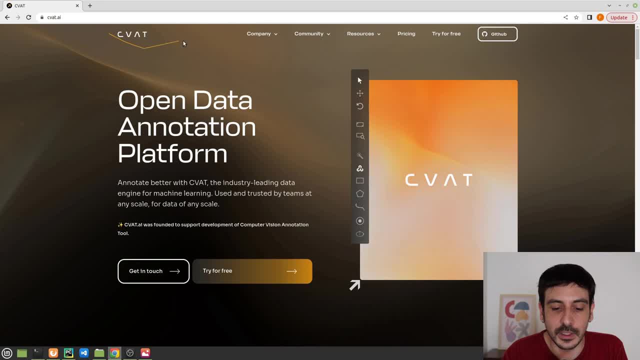 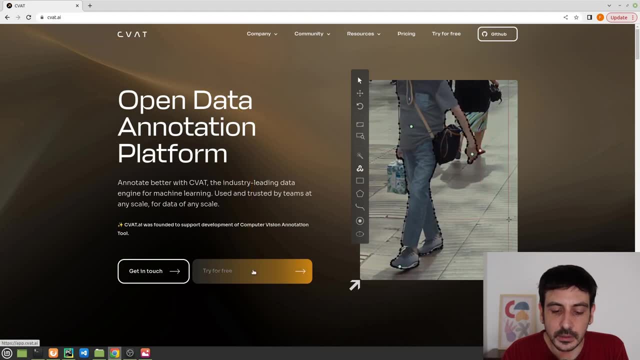 but nevertheless, this is a tool I have used in many projects and I really, really like it. so let me show you how to use it. you have to go to cbatai and then you select. try for free. there are different pricing options, but if you are going to work on your own or in a very small team, 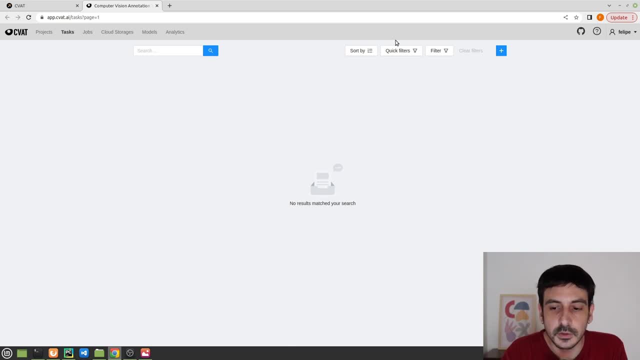 in a very small team. you can definitely use the free version. so I have already logged in. this is already logged into my account. but if you don't have an account, then you will have to create a new one. and yeah, so you you're going to see like a sign up page and you can just create a new account. 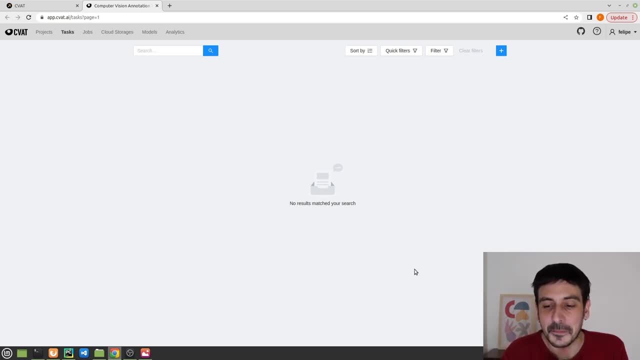 and then you can just log in into that account. so once you are logged into this annotation tool, you need to go to projects and then create a new one. I'm going to create a project which is called alpaca detector, because this is a project I am going to. 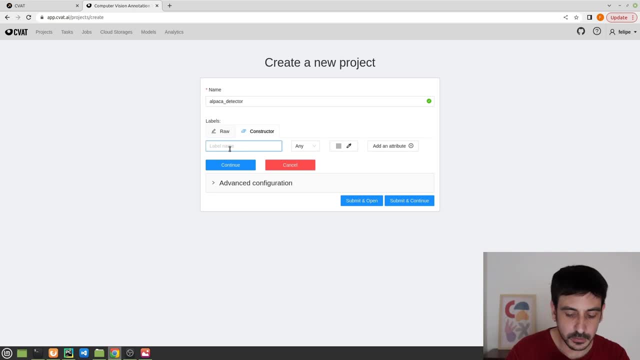 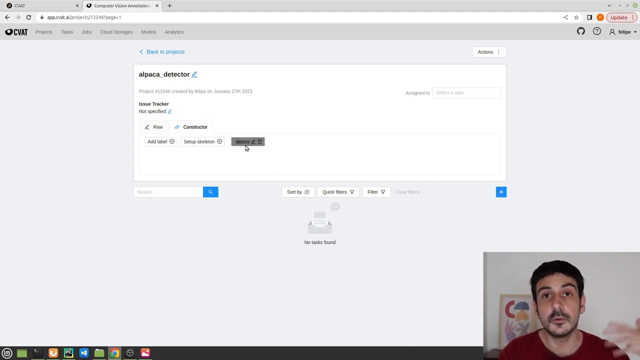 you be working in and I'm going to add a label which, in my case, is going to be only one label, which is alpaca, and then that's pretty much all: submit and open. I have created the project, it has one label, which is alpaca. remember, if your project has many, many different labels, 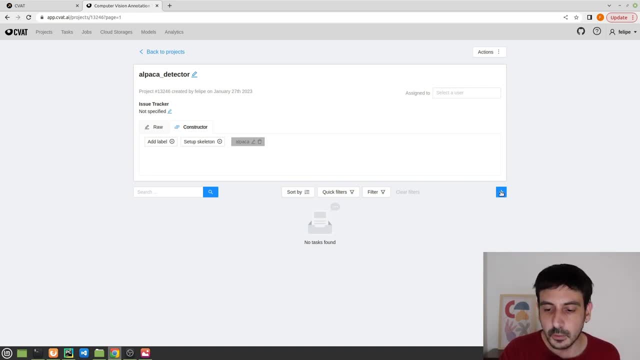 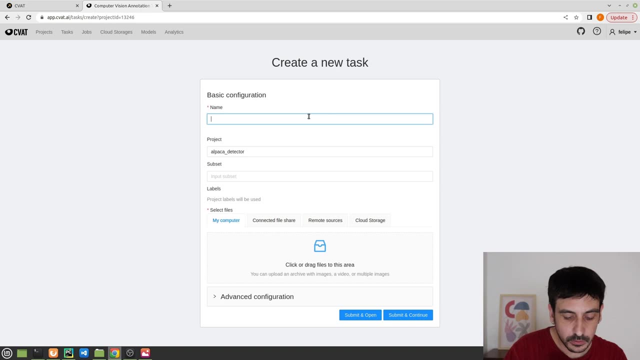 add all the labels you need, and then I will go here, which is create a new task. I am going to create a new annotation task and I'm going to call this task something like alpaca detector- annotation task 001. this is from the project alpaca detector and this will take all the labels from that. 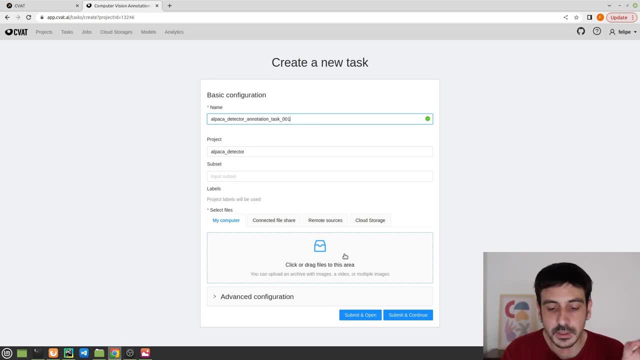 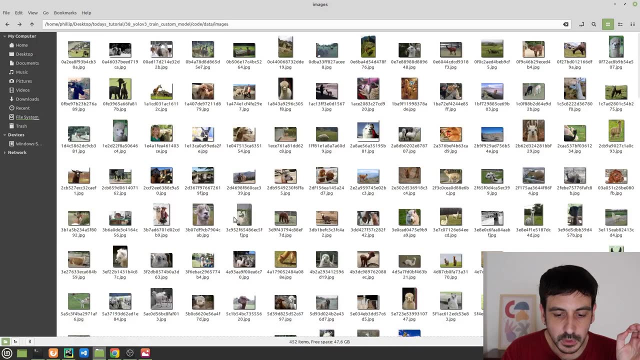 project. now you need to upload all the images you are going to annotate. so in my case, I'm obviously not going to annotate all the images, because you can see these are too many images and it doesn't make any sense to annotate all these images in this. 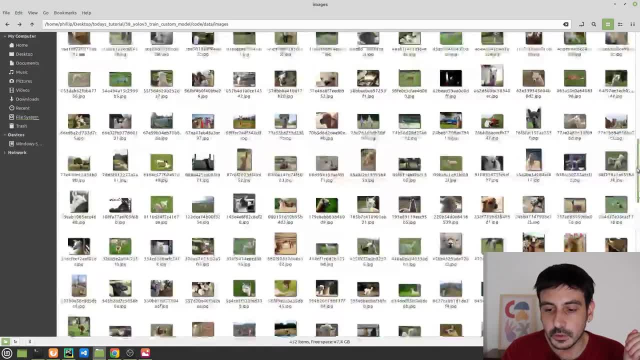 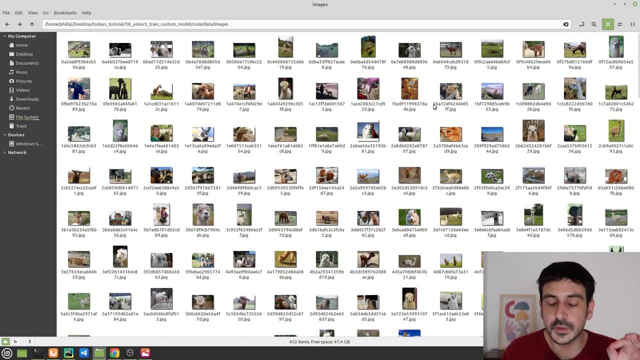 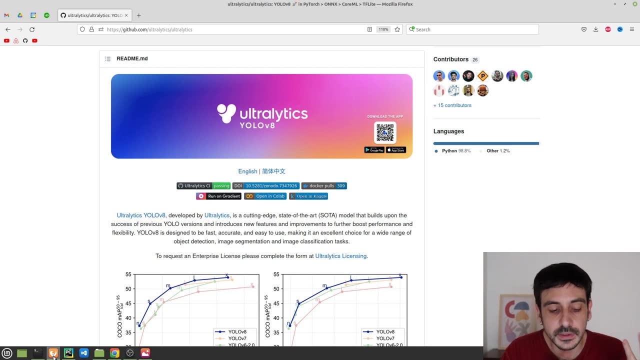 video. these are 452 images, so i'm not going to annotate them all, but i'm going to select a few in order to show you how exactly this annotation tool works and how exactly you can use it in your project. also, in my case, as i have already, as i have downloaded these images from a publicly 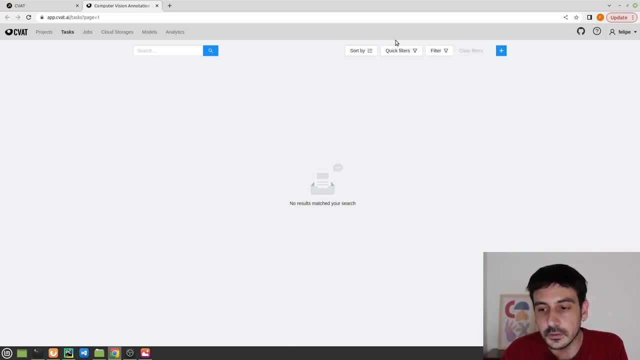 So I have already logged in. This is already logged into my account. but if you don't have an account, then you will have to create a new one. and yeah, so you're going to see sign up page and you can just create a new account and then you can just log in into that. 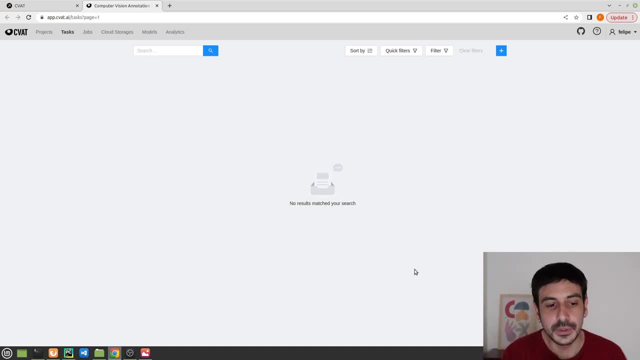 account. So once you are logged into this annotation tool, you need to go to projects and then create a new one. I'm going to create a project which is called alpaca detector, because this is a project I am going to be working in. 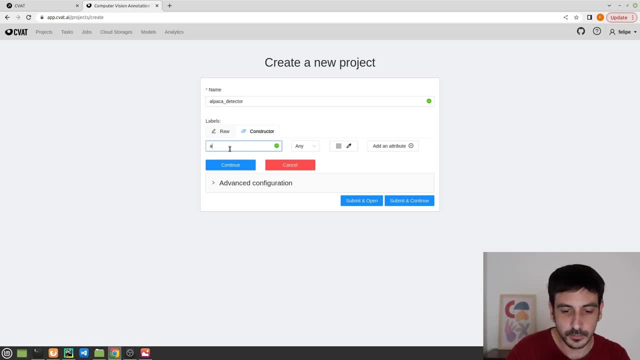 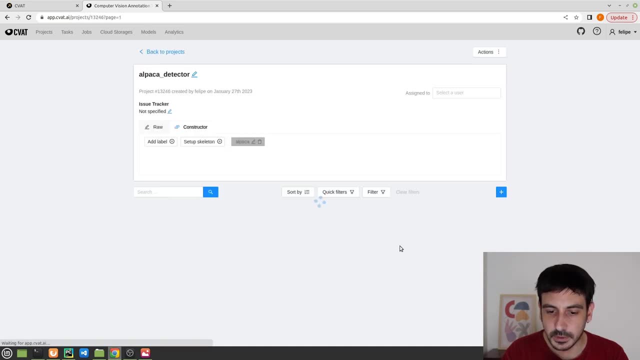 and I'm going to add a label which, in my case, is going to be only one label, which is alpaca, And then that's pretty much all: Submit and open. I have created the project. It has one label which is alpaca. Remember, if your project has many, many different labels, add all the labels. 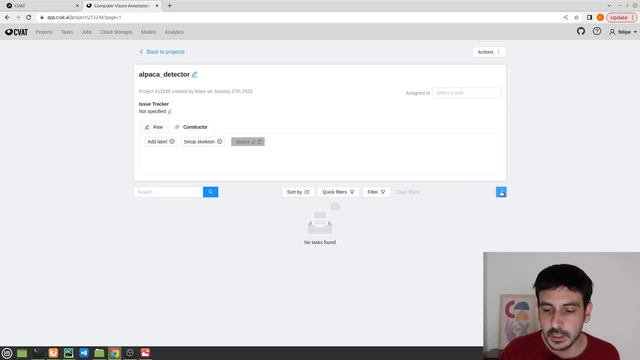 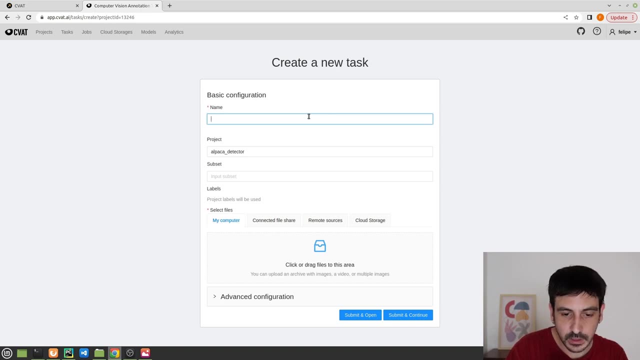 you need, and then I will go here, which is create a new task. I am going to create a new annotation task and I'm going to call this task something like alpaca detector. annotation task zero zero one. This is from the project alpaca detector and this will take all the labels from that project. 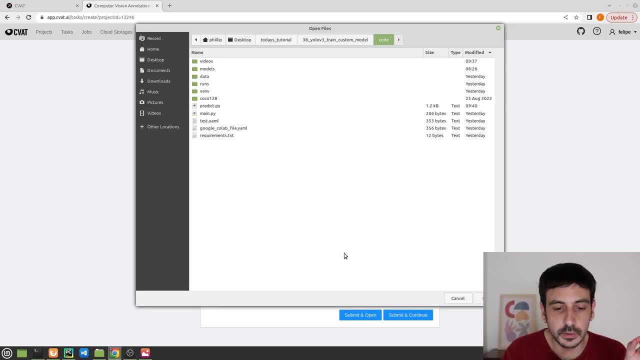 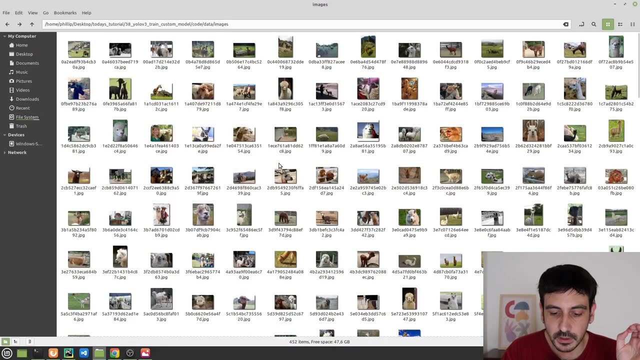 Now you need to upload all the images you are going to annotate. So in my case, I'm obviously not going to annotate all the images, because you can see these are too many images and it doesn't make any sense to annotate all these images in this video. 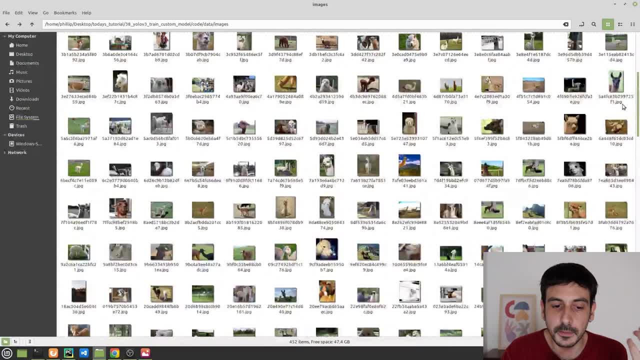 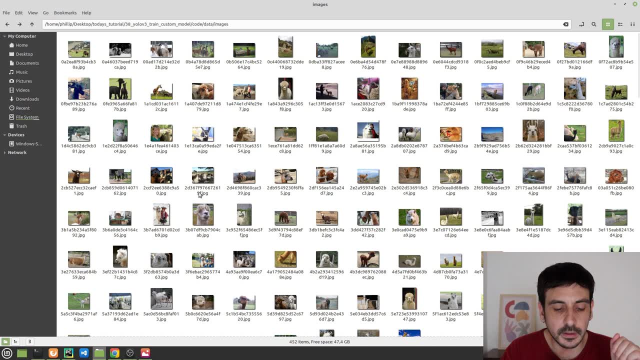 These are 452 images, so I'm not going to annotate them all, but I'm going to select a few in order to show you how to annotate all these images in the project. I'm going to say that here. I'm going to how exactly this annotation tool works and how exactly you can use it in your project, also in: 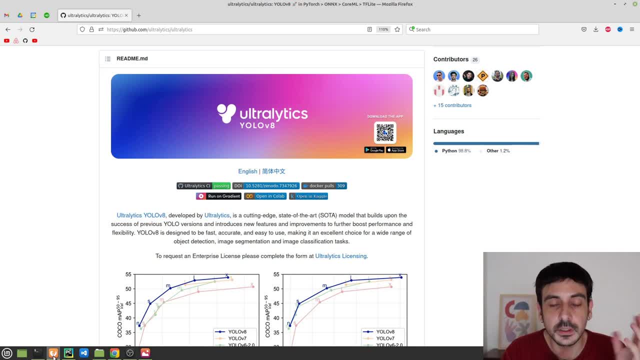 my case, as I have already, as I have downloaded these images from a publicly available data set, from the open images that I said, version 7- I already have the annotations, I already have all the rounding boxes, so in my case I don't really need to annotate this data because I already have. 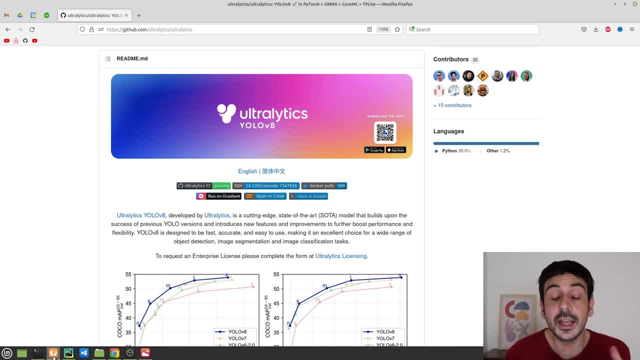 available dataset from the open images dataset version 7. i already have the annotations. i already have all the bounding boxes. so in my case i don't really need to annotate this data because i already have the annotations. but i'm going to pretend i don't, so i can just label a few images and i can. 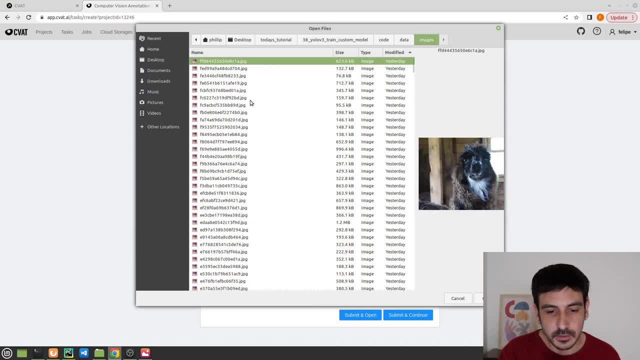 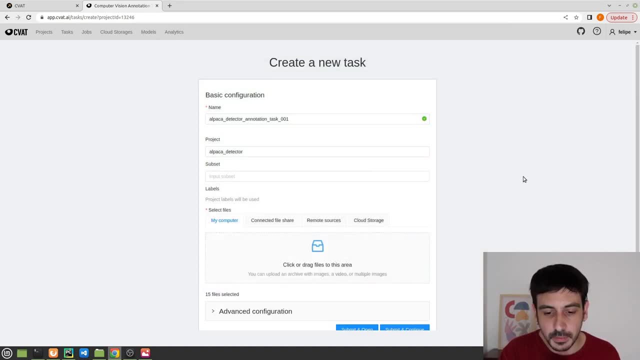 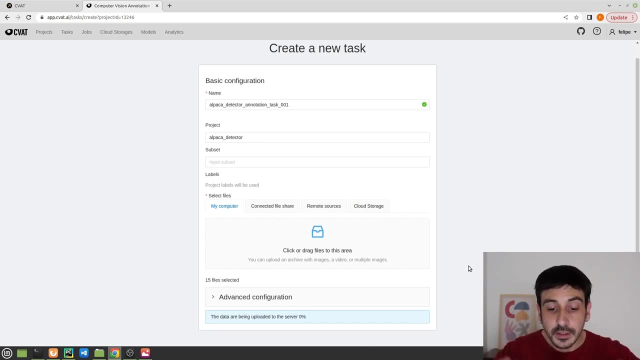 show you how it works. so now i go back here and i'm just going to select something like this many images, right? yeah, i'm just going to select this many images, i'm going to open these images and then i'm going to click on submit and open, right? so this is going to create this task and, at the same time, it's going to 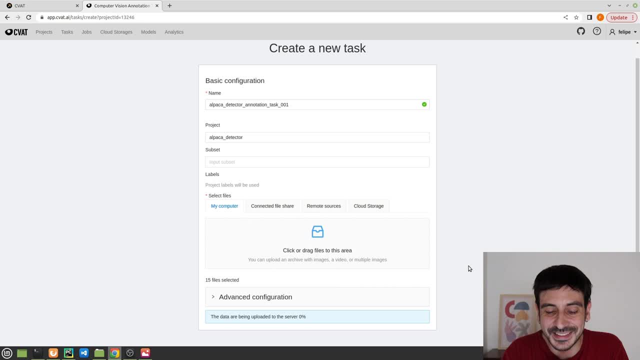 open this task so we can start working on our annotation process. okay, so this is the task i have just created. i'm going to click here in shelf number and this and the job number, and this will open all the images, and now i'm going to start annotating all these images. so we are working on. 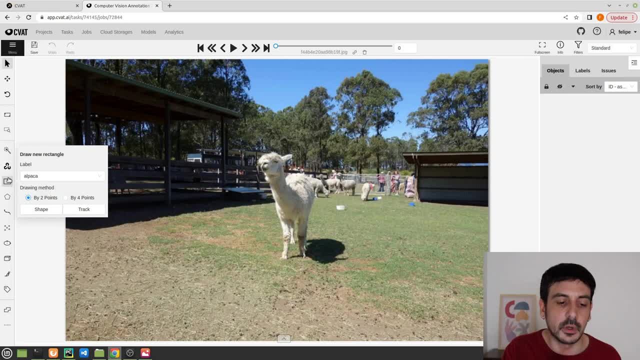 an object detection problem. so we are going to annotate bounding boxes. we need to go here and, for example, if we will be detecting many different categories, we will select what's the category we are going to label now and and that's it. in my case, i'm going to label always the same category. 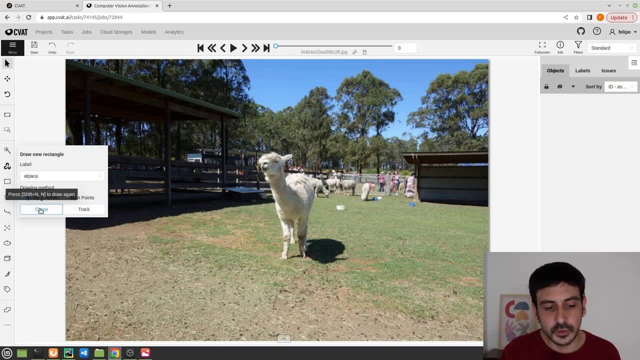 which is alpaca. so i don't really need to do anything here. so i'm going to select shape and let me show you how i do it. i'm going to click in the upper left corner and then in the bottom right corner. so the idea is to enclose the object and only the object. right. the idea is to draw a bounding. 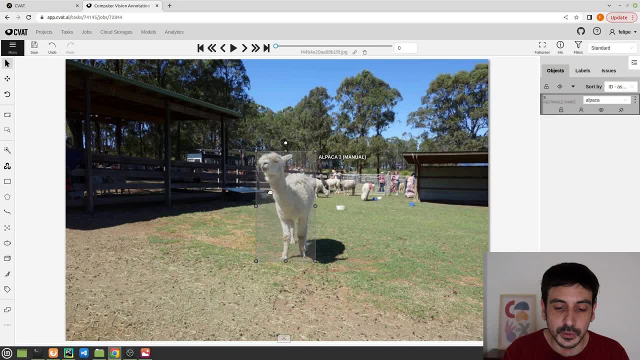 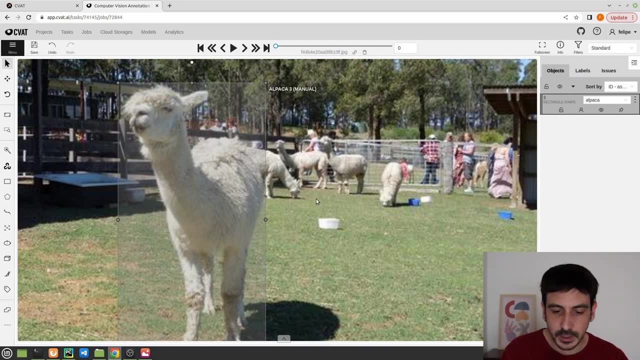 object and anywhere else. right, you only want to enclose this object and you can see that we have our animals in the back right. we have other alpacas, so i'm just going to label them too, and there is a shortcut which is pressing the letter n and you can just create a new bounding box. so 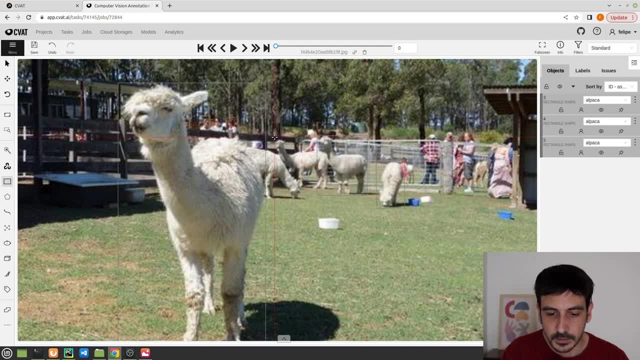 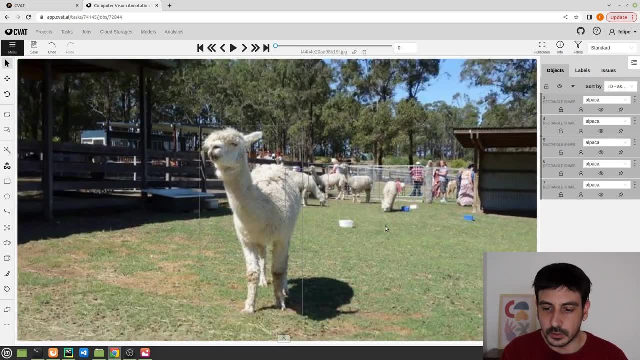 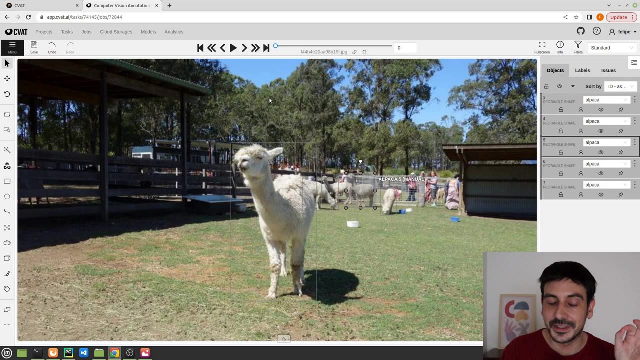 that's another one, this is another one, this is another alpaca, and this is the last one. okay, that's pretty much all. so once you're ready, you can just press ctrl s. that's going to save the annotations. i recommend you to press ctrl s as often as possible, because it's always a good practice. so now everything is saved, i can. 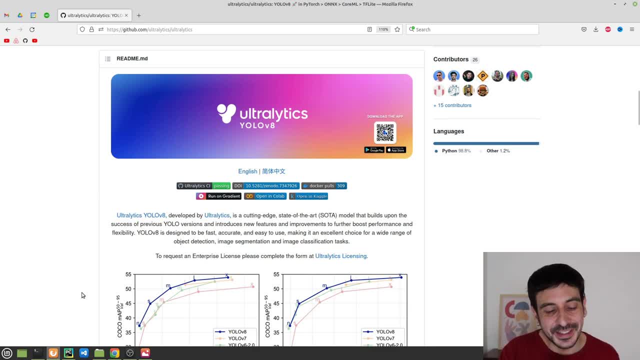 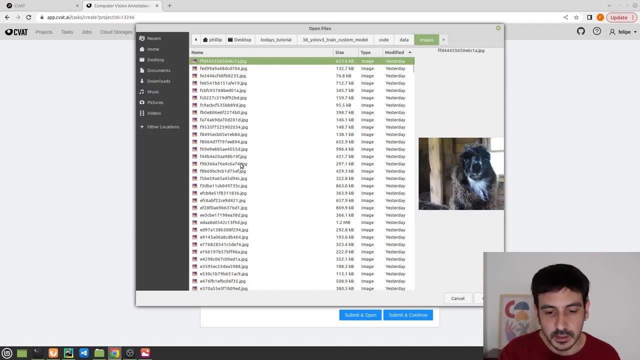 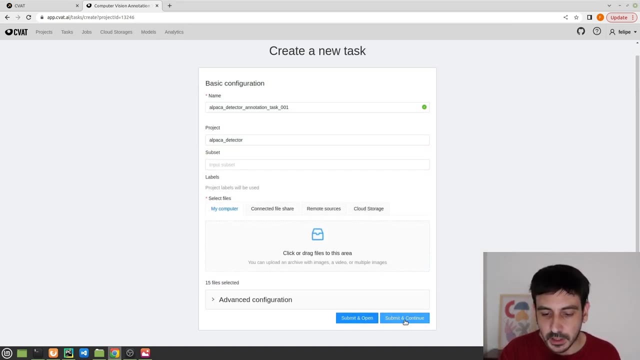 the annotations, but I'm going to pretend I don't, so I can just label a few images and I can show you how it works. and so now I go back here and I'm just going to select something like this many images. right, yeah, I'm just going to select this many images, I'm going to open these images and 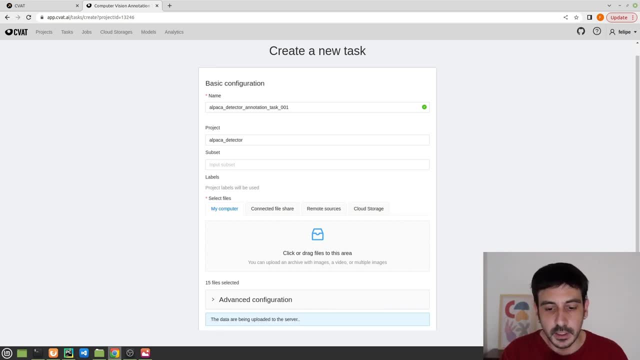 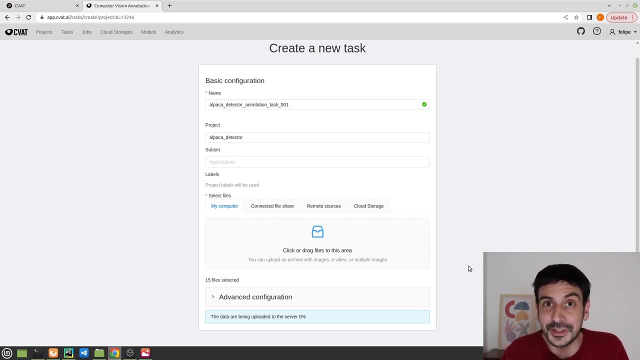 then I'm going to click on submit and open. right, so this is going to create this task and, at the same time, it's going to open this task so we can start working on our annotation process. okay, so this is the task I have just created. I'm going to click here in job number and this and the job. 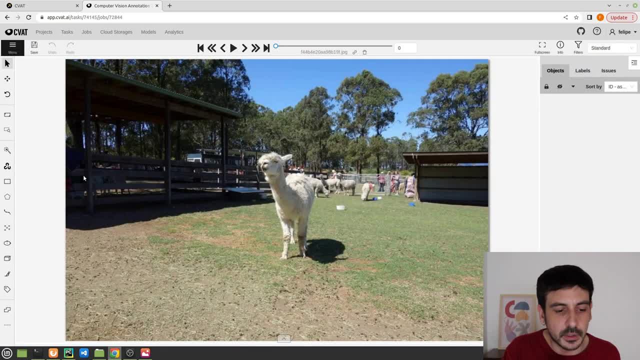 number and this will open all the images. and now I'm going to start annotating all these images. so we are working on an object detection problem. so we are going to annotate bounding boxes. we need to go here and, for example, if we will be detecting many different categories, we will select what's. 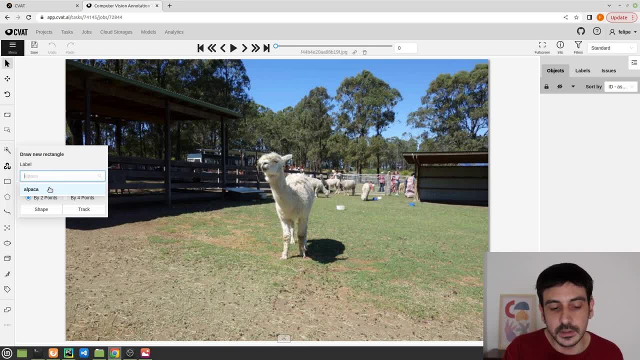 the category we are going to label now, and and that's it. in my case, I'm going to label always the same category, which is alpaca, so I don't really need to do anything here. so I'm going to select shape and let me show you how I do it. 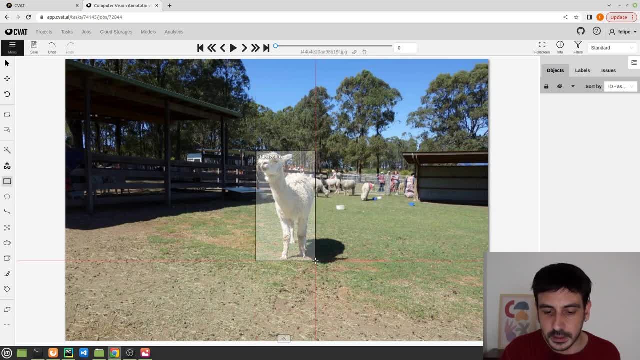 how I do it. I'm going to click in the upper left corner and then in the bottom right corner. so the idea is to enclose the object and only the object, right? the idea is to draw a bonding box around the object and anywhere else. right, you only want to enclose this object and you can. 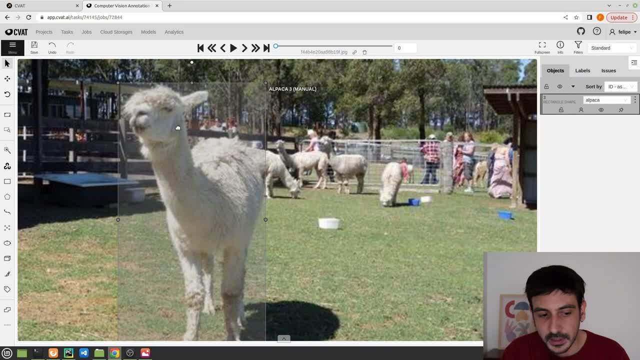 see that we have our animals in the back right. we have other alpacas, so I'm just going to label them too, and there is a shortcut, which is pressing the letter n and you can just create a new boundary box. so that's another one, this is another one, this is another alpaca and this is the last one. 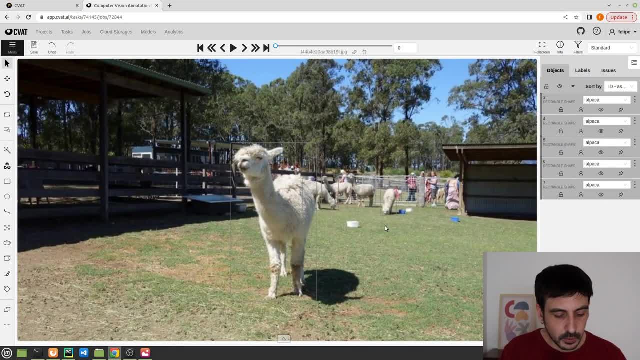 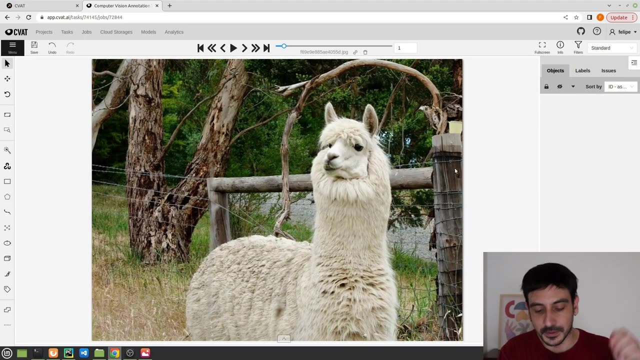 okay, that's pretty much all. so once you're ready, you can just press ctrl s. that's going to save the annotations. I recommend you to press ctrl s as often as possible, because it's always a good practice. so now everything is saved, I can just continue to the next image. now I'm going to 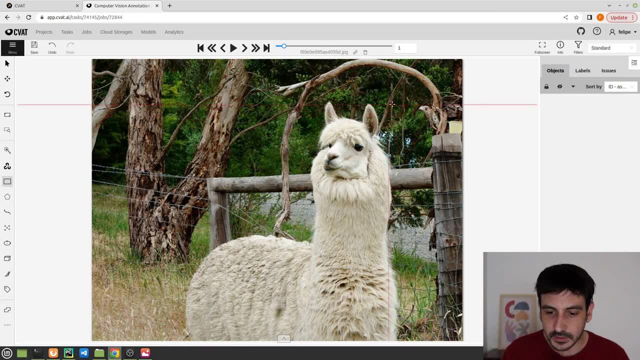 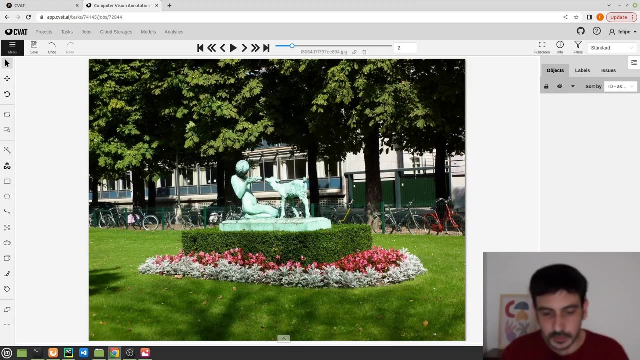 annotate this alpaca and I'm going to do exactly the same process. I can start here. obviously, you can just start in whatever corner you want, and I'm going to do something like this. okay, this image is completely annotated. I'm going to continue to the next image. in this case, I'm going to annotate this alpaca too. 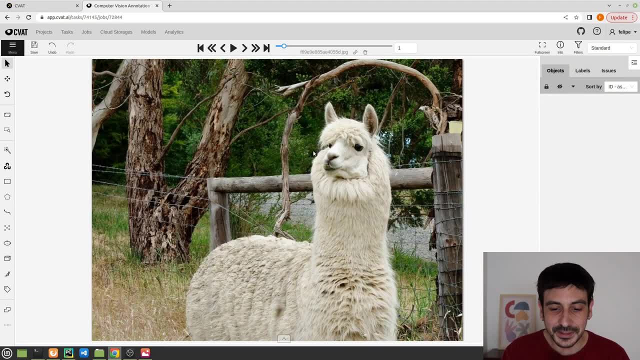 just continue to the next image. now i'm going to annotate this alpaca and i'm going to do exactly the same process. i can start here. obviously, you can just start in whatever corner you want, and i'm going to do something like this. okay, this image is completely annotated. i'm going to continue. 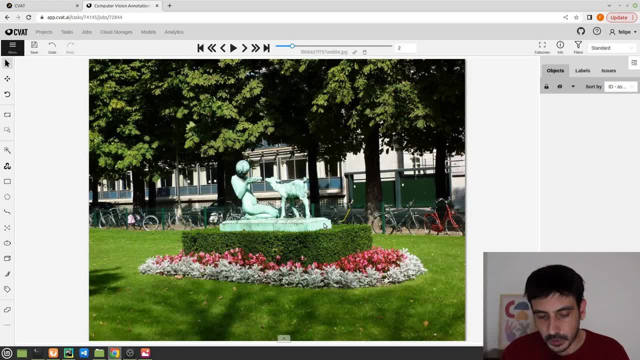 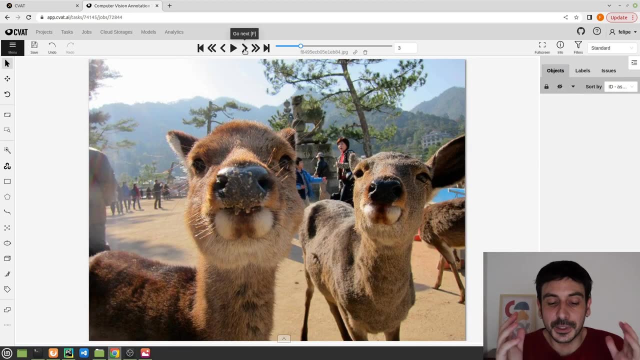 to the next image. in this case, i'm going to annotate this alpaca too. this is not a real alpaca, but i want my object detector to be able to detect these type of objects too, so i'm going to annotate it as well. this is going to be a very good exercise. exercise, because, if you want to work as a machine learning, 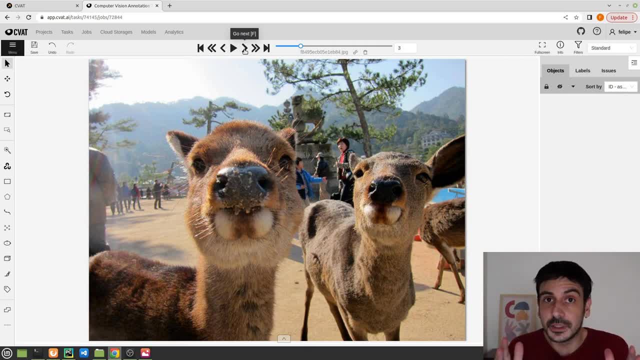 engineer or as a computer vision engineer, annotating data is something you have to do very often. actually, training machine learning models is something you have to do very often. so usually the data annotation is done by other people. right, it's done by annotators. it's done by. 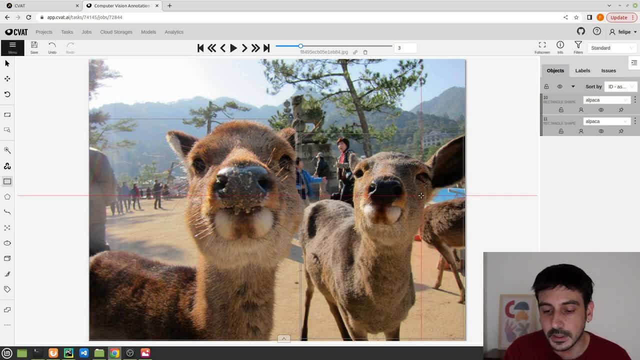 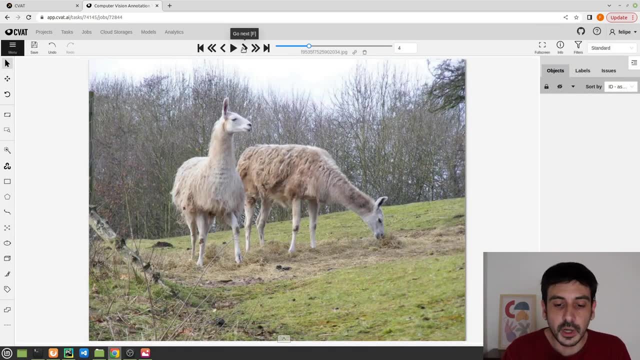 i don't know it's. there are different services you can hire in order to annotate data, but in whatever case, whatever service you use, it's always a very good practice to annotate some of the images yourself, right? because if you annotate some of the images yourself, you are going to be more familiar with the data and you're also going to be more familiar. 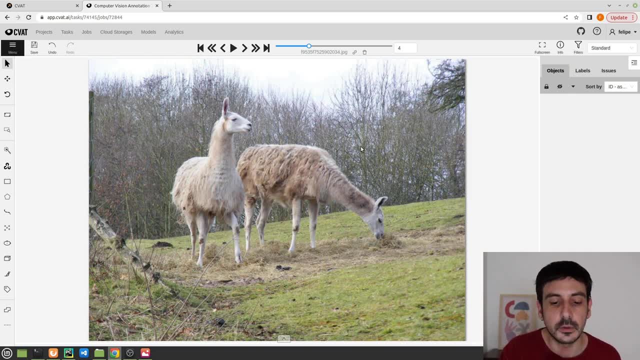 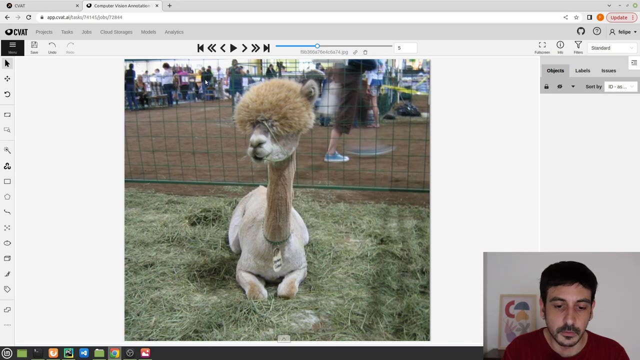 instruct the annotators on how to annotate this particular data, for example. in this case it's not really challenging. we just have to annotate these two objects. but let me show you. there will be other cases, because there will be always situations which are a little confusing. in this case it's not. 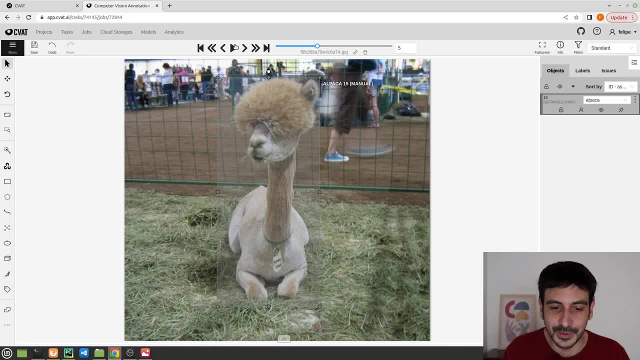 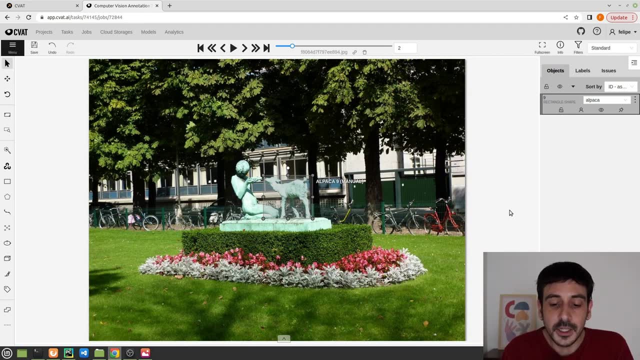 confusing either. I have just to. I have to label that object. but for example, a few images ago, when we were annotating this image, if an annotator is working on this image, it's. that person is going to ask you: what do I do here, should I? 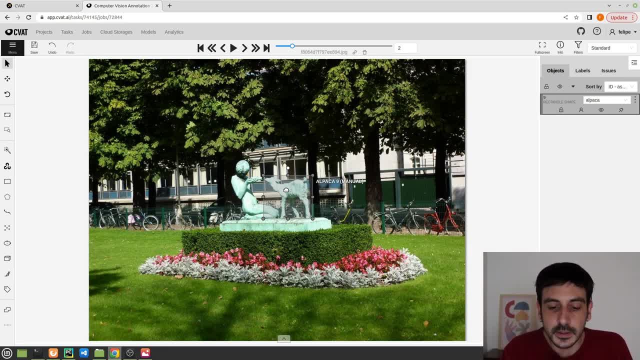 annotate this image or not? right, if an annotator is working on this image and the instructions you provide, they are not clear enough. the this person is going to ask you: hey, what do I do here? should I annotate this image or not? is this an alpaca or not? so, 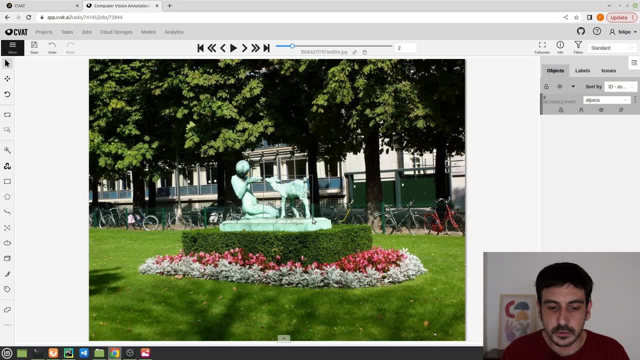 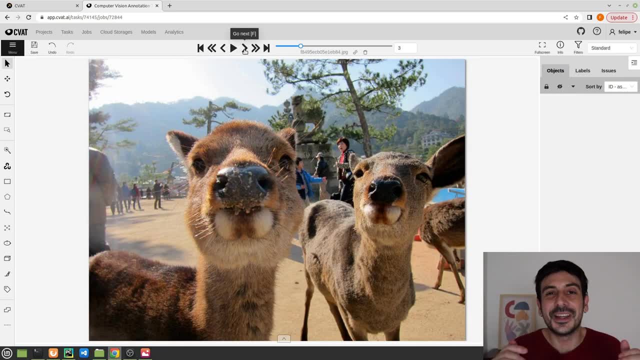 this is not a real alpaca, but I want my object detector to be able to detect this type of objects too, so I'm going to annotate it as well. this is going to be a very good exercise. exercise because if you want to work as a machine learning engineer or as a computer vision engineer, 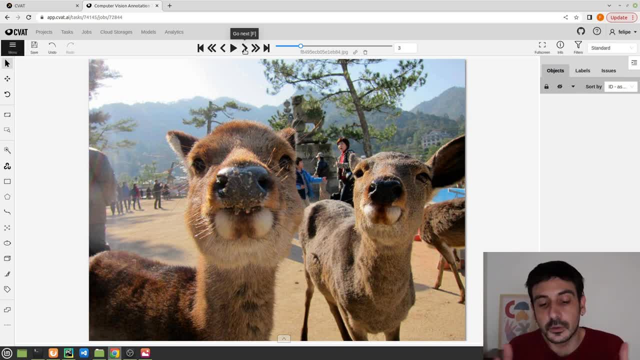 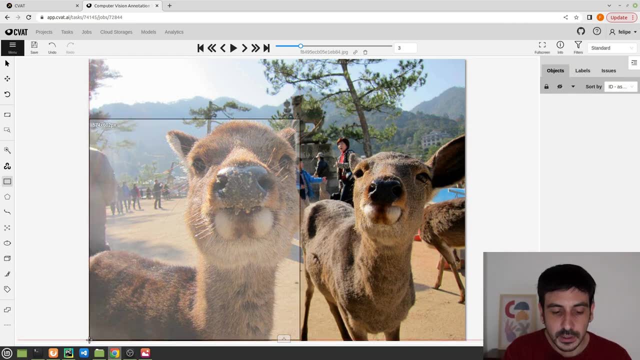 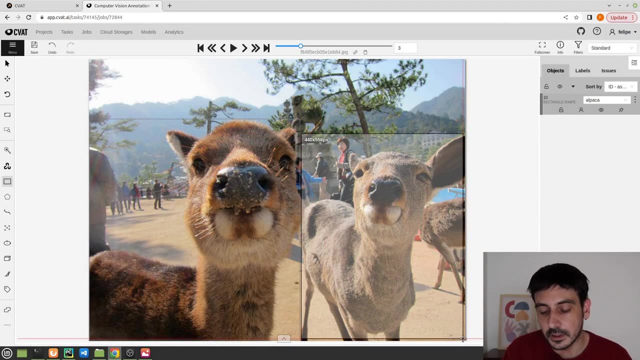 annotating data is something you have to do very often. actually, training machine learning models is something you have to do very often. so usually the data annotation is done by other people. right, it's done by annotators, it's done by- uh, I don't know it's. there are different services you can. 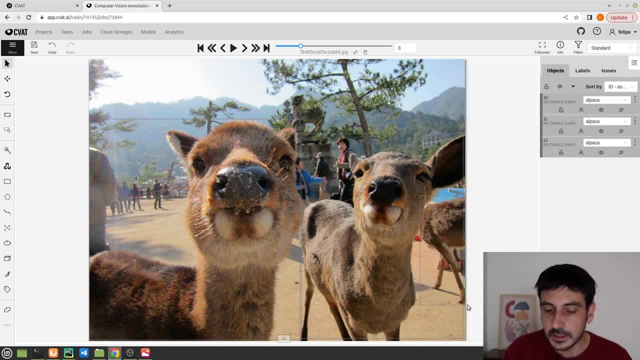 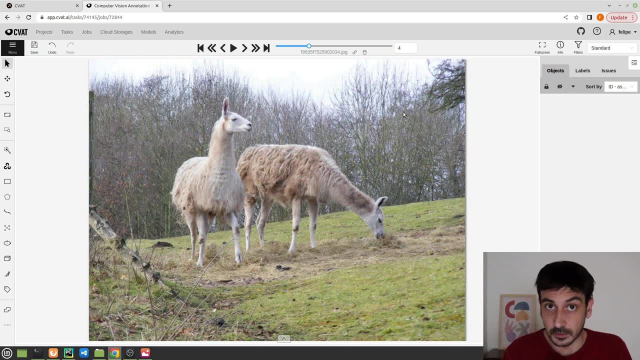 hire in order to annotate data. but in whatever case, whatever service you use, it's always a very good practice to annotate some of the images yourself, right? because if you annotate some of the images yourself, you are going to be more familiar with the data and you're 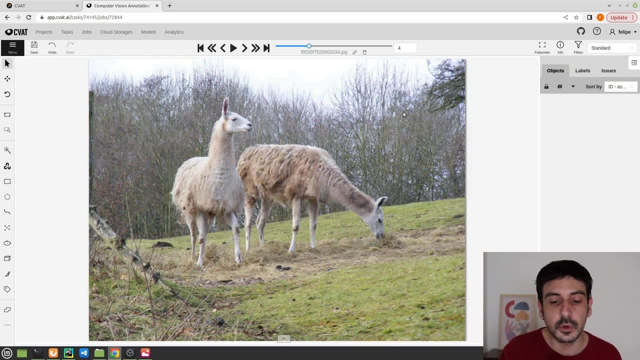 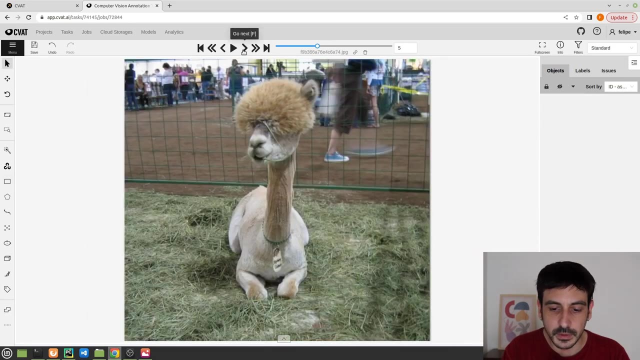 also going to be more familiar on how to instruct the annotators on how to annotate these particular data, for example. in this case it's not really challenging, we just have to annotate these two objects, but let me show you. uh, there will be other cases, because there will be always situations. 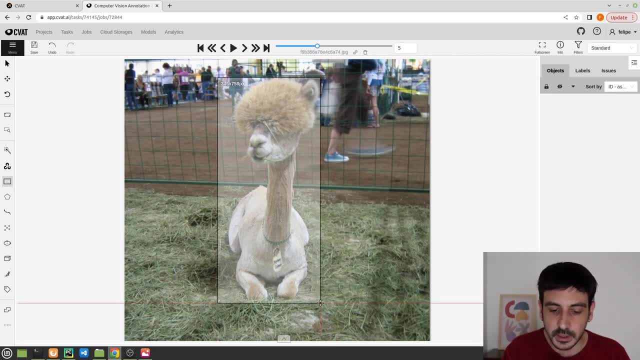 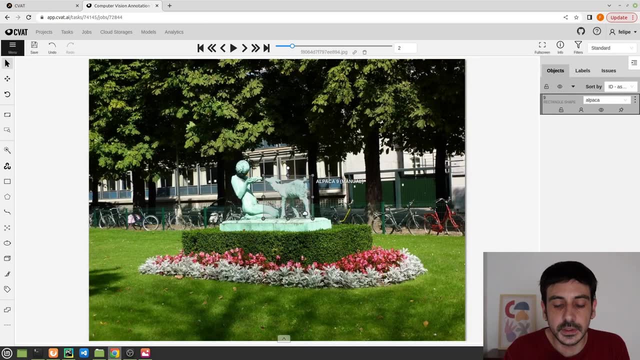 which are a little confusing. in this case, it's not confusing either. I have just to. I have to label that object. but for example, a few images ago, when we were annotating this image, if an annotator is working on this image, it's that person is going to ask you: what do I do here? should I annotate this? 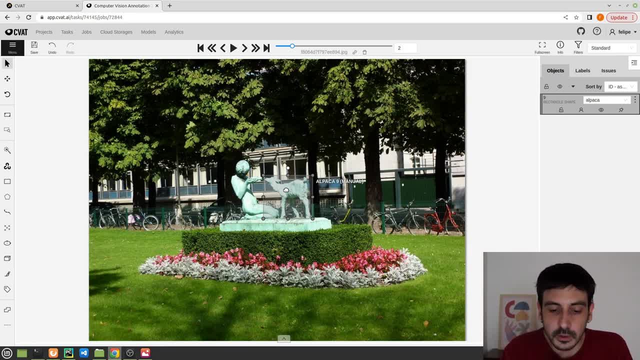 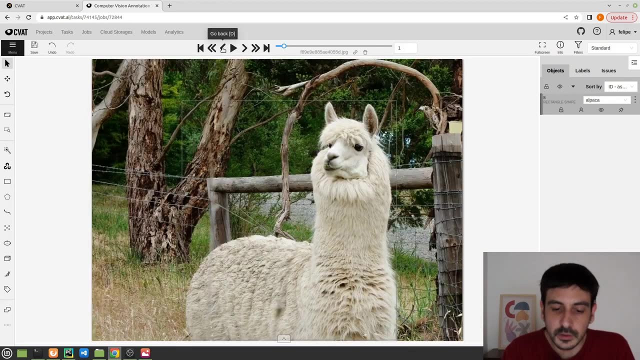 image or not? right, if an annotator is working on this image and the instructions you provide they are not clear enough. the this person is going to ask you: hey, what do I do here? should I annotate this image or not? is this an alpaca or not? so, for example, data situation and our situation will be what happened here, which we 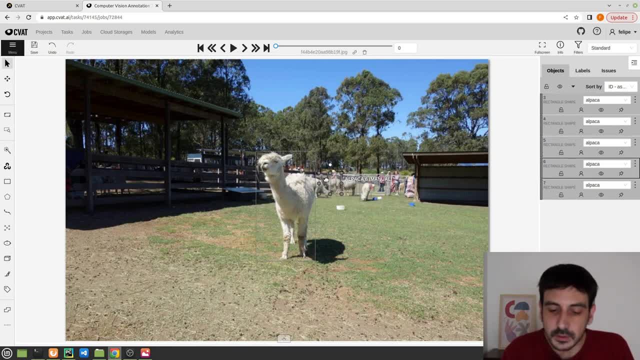 have many different alpacas in the background, and some of them, for example this one, is a little occluded, so there could be an annotator, someone who asks you: hey, do you want me to annotate absolutely every single alpaca, or maybe I can just draw a huge bounding box here in the background? 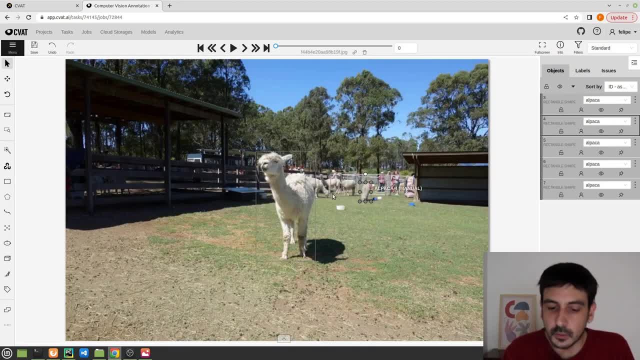 example, data situation and our situation will be what happened here, which we have many different alpacas in the background and some of them, for example this one, is a little occluded, so there could be an annotator, someone who asks you: hey, do you want me to annotate absolutely? 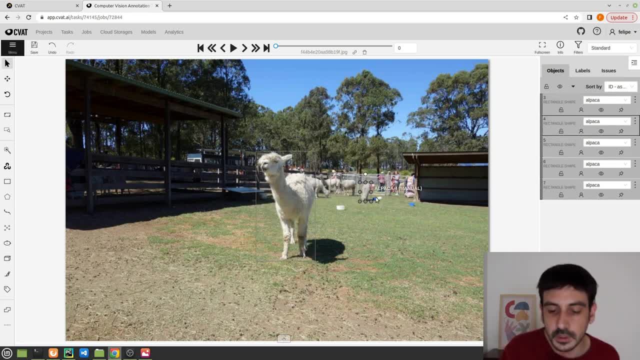 every single alpaca. or maybe i can just draw a huge bounding box here in the background and just say: everything in the background is an alpaca, something like that. when an annotator is working on the images, they are going to have many, many different questions regarding how to. 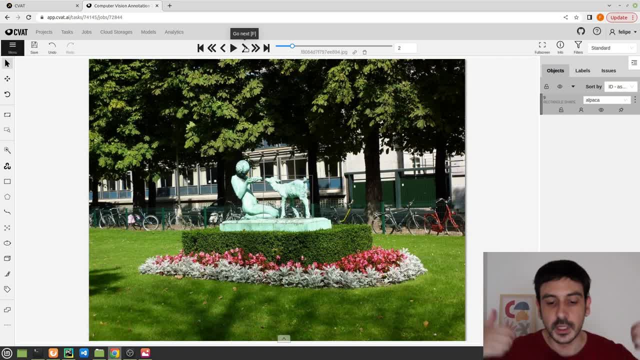 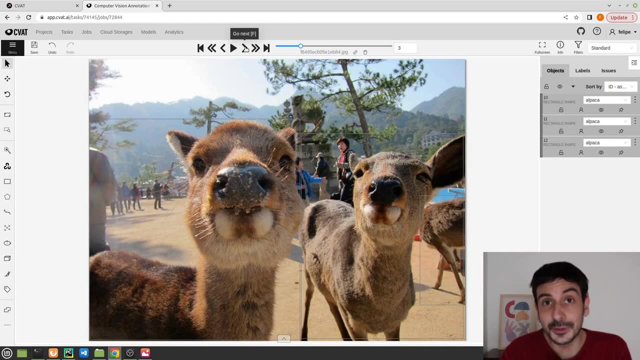 annotate the data, and they are all perfect questions and very good questions, because this is exactly what's about. i mean, when you are annotating data, you are defining exactly what are the objects you are going to detect, right? so what i'm going is that if you annotate some of the 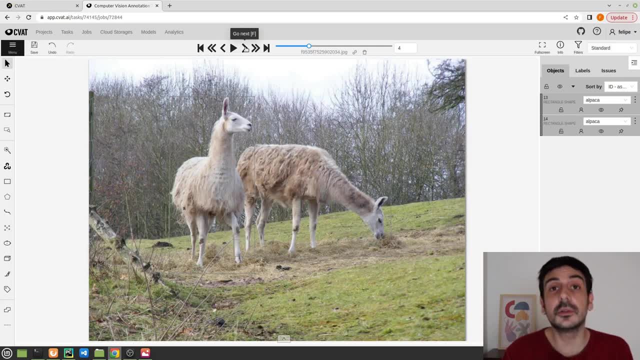 images yourself, you are going to be more familiar on what are all the different situations, on what exactly is going on in the immediate situation. it's going to be the same thing for each video on with your data, so you are more clear in exactly what are the objects you want. 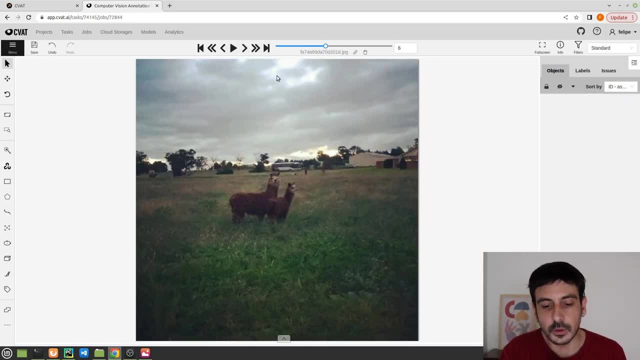 to detect right. so let's continue. this is only to show a few examples. this is another situation. in my case, I want to say that both of them are alpacas, so I'm just going to say something like this, but there could be another person who. 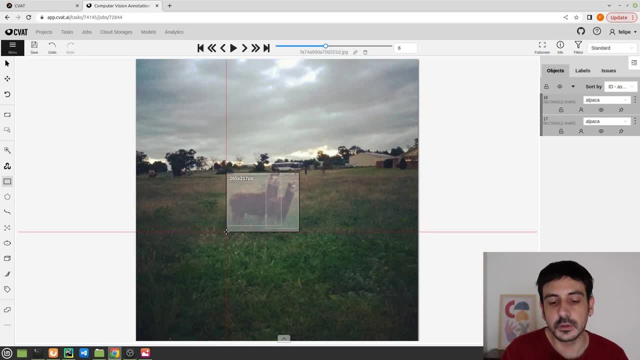 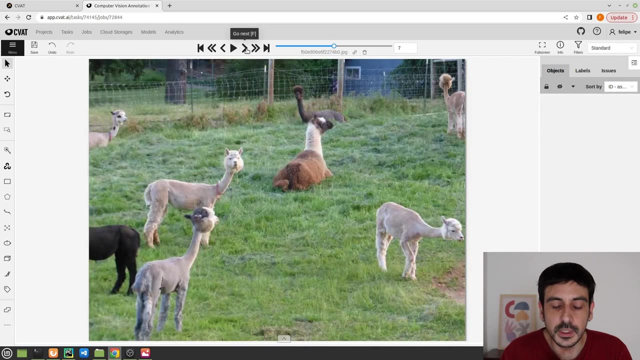 says: no, this is only one annotation. is something like this: right, I'm just going to draw one bounding box enclosing both of them, something like that, and it will be a good criteria. I mean, it will be a criteria, which I guess it would be fine. but whatever your criteria would be, you need one, right? you need a criteria. so 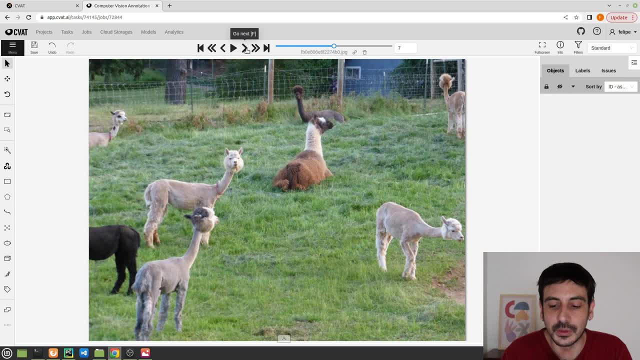 while you are annotating some of the images, is that you are going to further understand what exactly is an alpaca, what exactly is the object you want to consider as alpaca? so I'm just going to continue. this is another case which may not be clear, but I'm just going to continue. 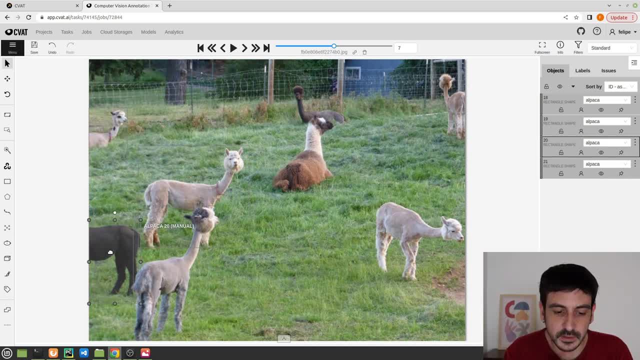 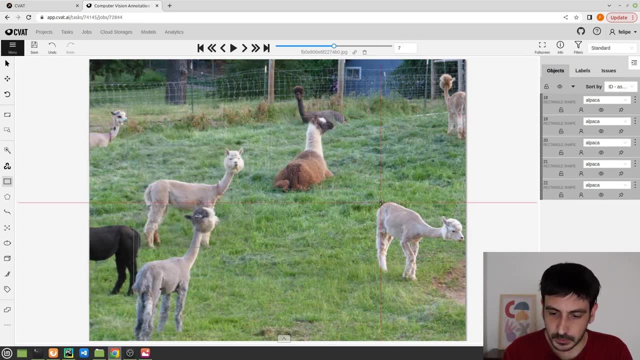 to say this is an alpaca, this black one, which we can only see this part and we don't really see the head. but I'm going to see it. I'm going to say it's an alpaca anyway. this one too, this one two, this one, two also. this is something that 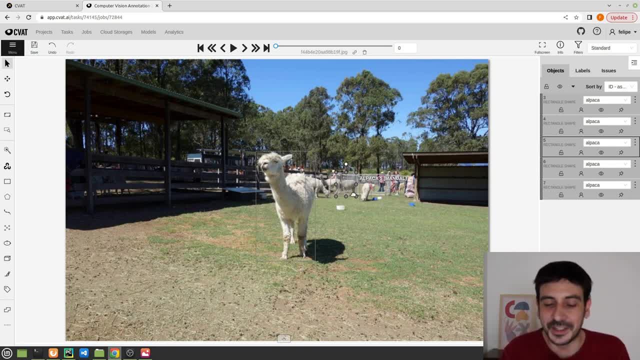 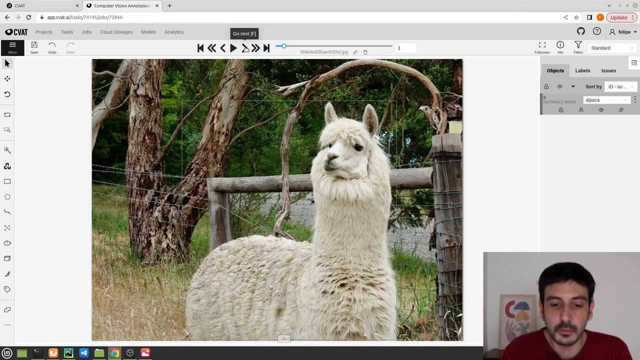 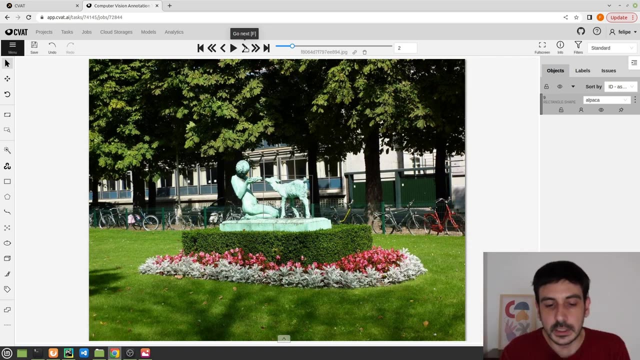 and just say anything. in the background is an alpaca. it's something that when an annotator is working on the images, they are going to have many, many different questions regarding how to annotate the data, and they are all perfect questions and very good questions, because this is exactly what's. 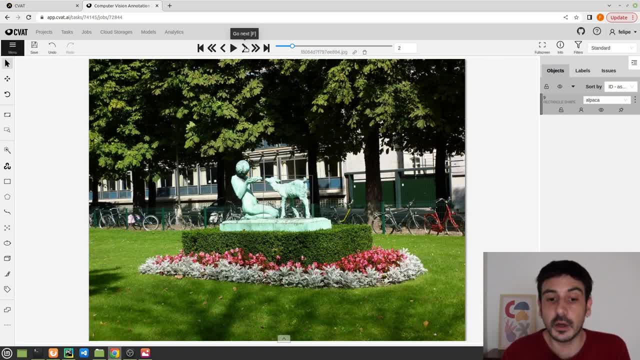 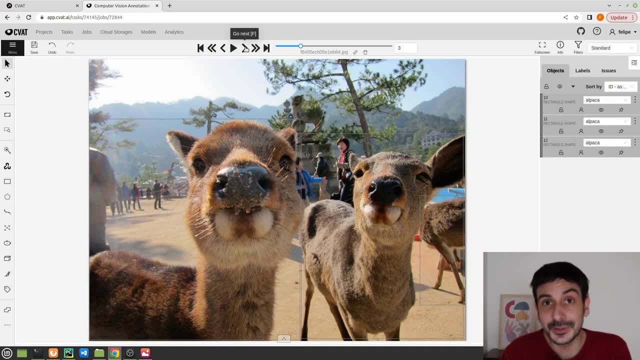 about. I mean, when you are annotating data, you are defining exactly what are the objects you are going to detect, right? so, um, what I'm going is that if you annotate some of the images yourself, you are going to be more familiar on what are all the different situations, on what 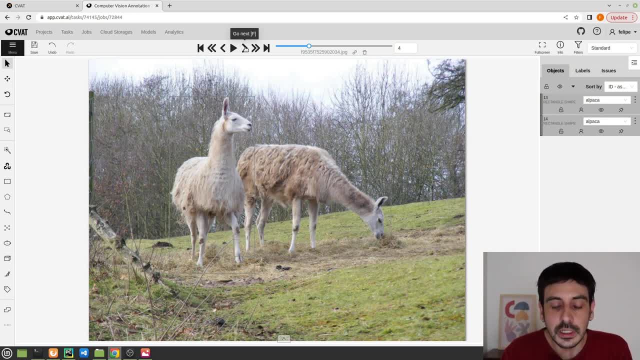 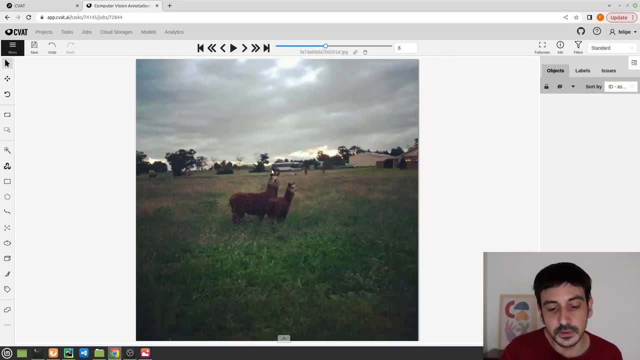 exactly is going on with your data, so you are more clear in exactly what are the objects you want to detect, right? so let's continue. this is only to show a few examples. this is another situation. in my case, I want to say that both of them are alpacas, so I'm just going to say something like: 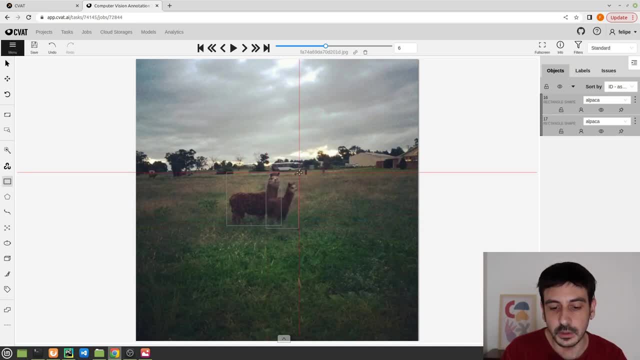 this, but there could be another person who says: no, this is only one, annotation is something, it is one bounding box enclosing both of them, something like that, and it will be a good criteria. I mean, it will be a criteria which I guess it will be fine, but uh, whatever your criteria would be, you 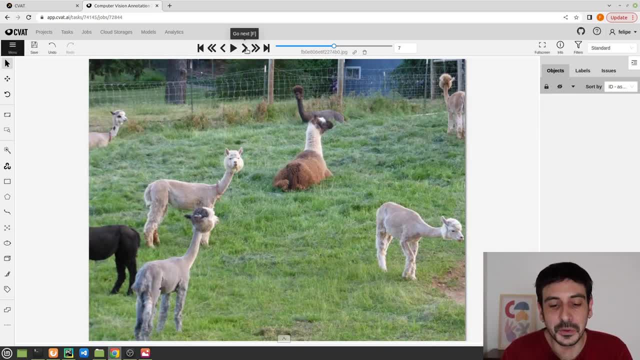 need one right, you need a criteria. so while you are annotating some of the images, is that you are going to um further understand what exactly is an alpaca, what exactly is the object you want to consider as alpaca? so I'm just going to continue. 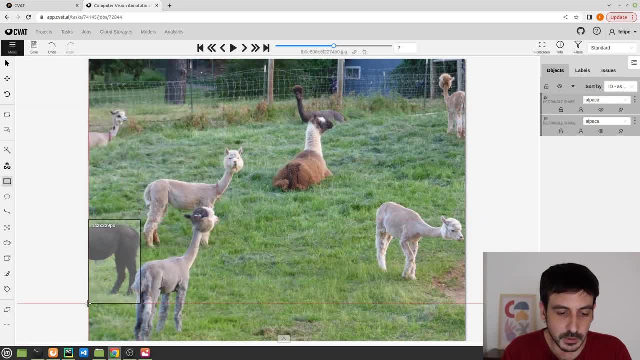 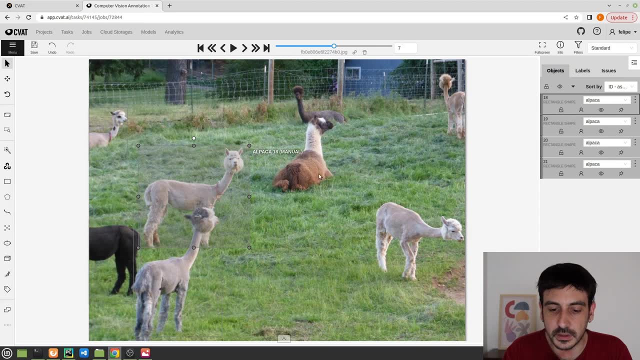 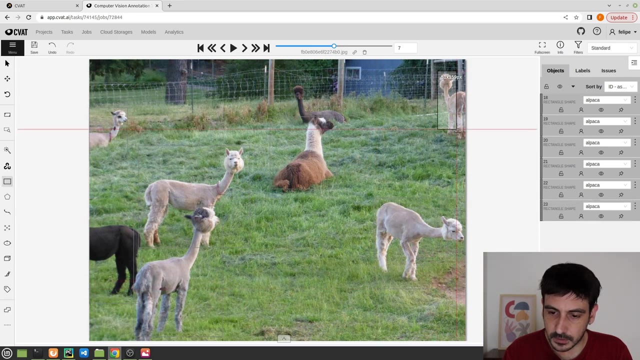 this is another case which may not be clear, but I'm just going to say: this is an alpaca, this black one which we can only see this part and we don't really see the head. but I'm going to see, I'm going to say it's an alpaca anyway, this one too, this one too, this one too also. this is something that 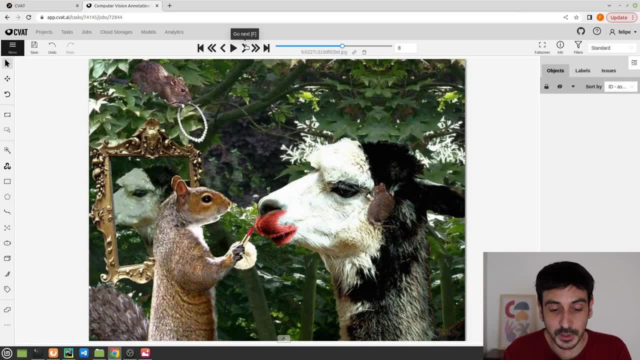 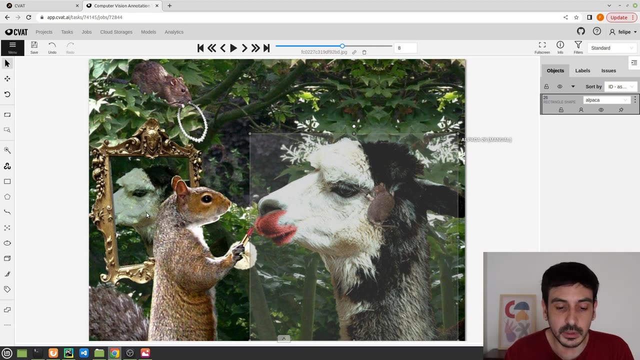 always happens to me when I am working, when I am annotating images, that I am more aware of all the diversity of all these images. for example, this is a perfect, perfect, perfect example, because we have an alpaca which is being reflected on a mirror and it's all. it's only like a very small section of the alpaca. 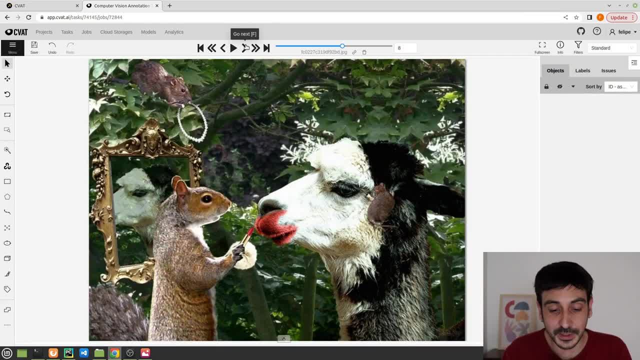 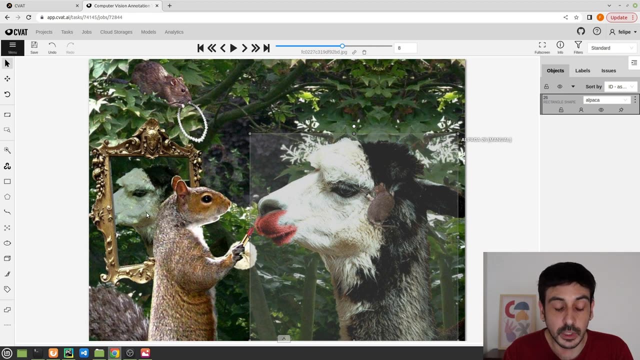 always happens to me when I am working, when I am annotating images, that I am more aware of all the diversity of all these images. for example, these are perfect, perfect, perfect example, because we have an alpaca which is being reflected on a mirror and it's all. it's only like a very small. 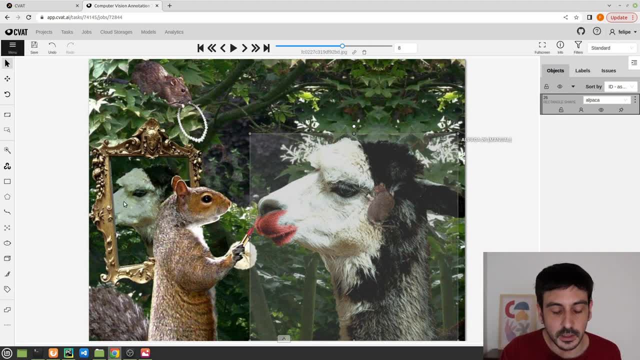 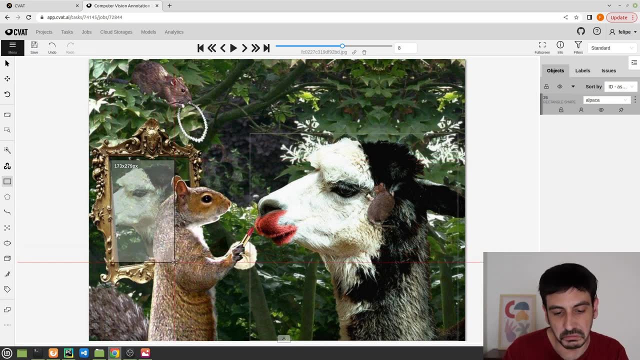 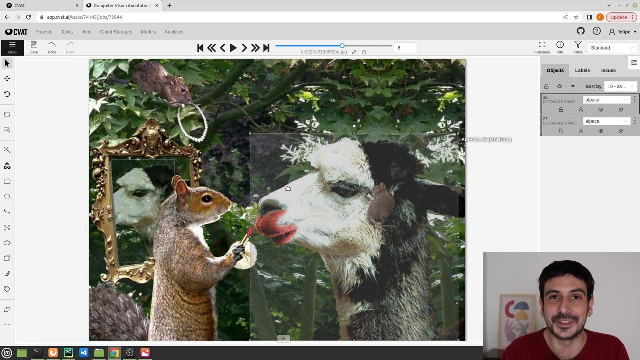 section of the alpaca. it's only like a very small piece of the alpaca's face. so what do we do here? i am going to annotate this one too, because, yeah, that's my criteria, but another person could say, no, this is not the object i want to detect. this is only the object i want to detect, and maybe another. 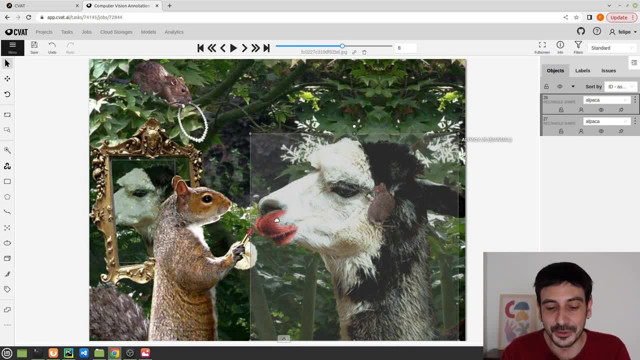 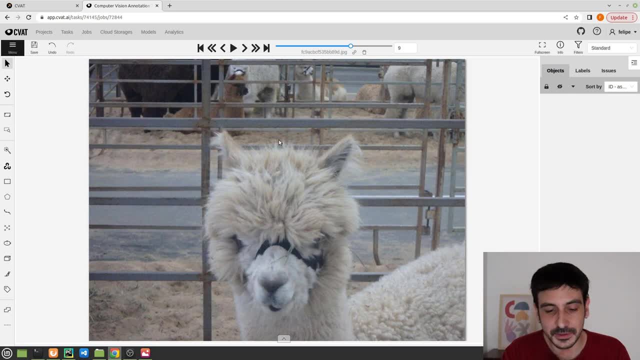 person would say: no, this is not an alpaca. alpacas don't really apply makeup on them. this is not real, so i'm not going to annotate this image. you get the idea right. there could be many different situations and the only way you get familiar with all the different type of situations is if you 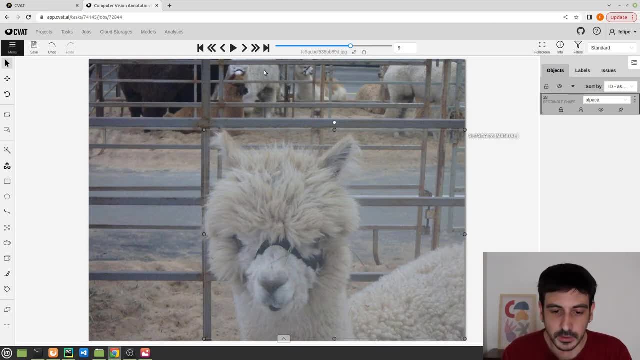 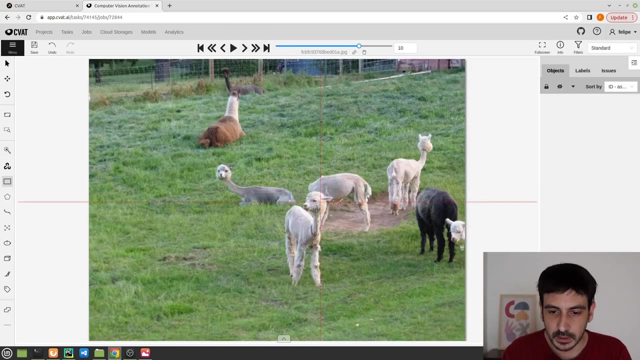 annotate some images yourself. so now let's continue. in my case, i'm going to, i'm going to do something. this because, yeah, i will say, the most important object is this one, and the other ones are like, yeah, it's not really that important if we detect them or not. okay, so let's continue. this is very 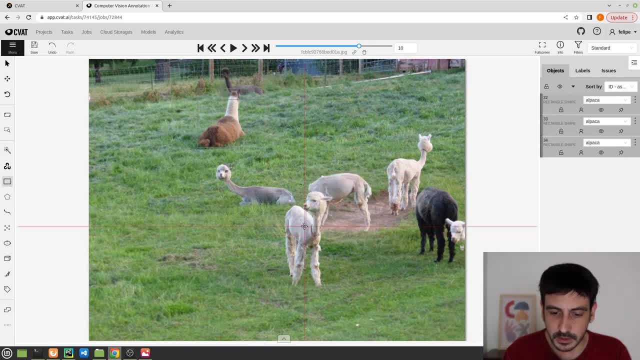 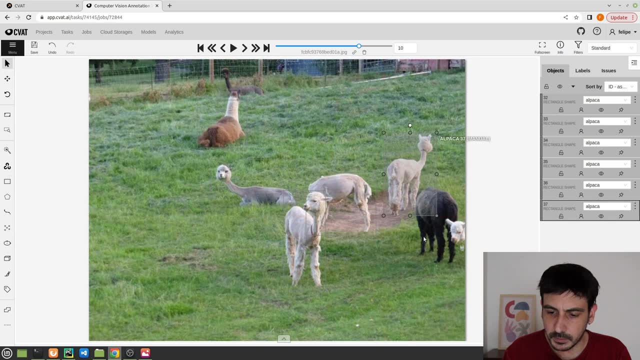 similar to another image. i don't know how many i have selected, but i think it's. we have only a few left. i don't know if this type of animals. they are like natural. i'm very surprised about this. like the head right, it's like it has a lot of hair over here and then it's completely hairless. 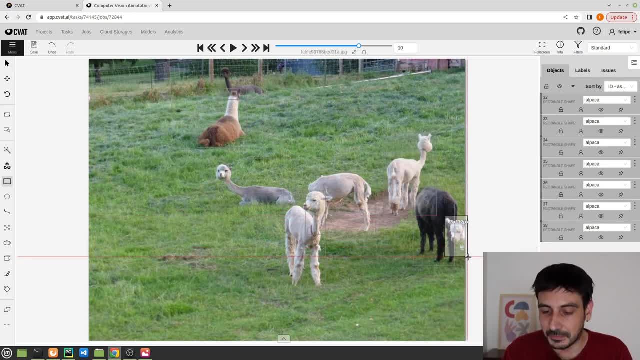 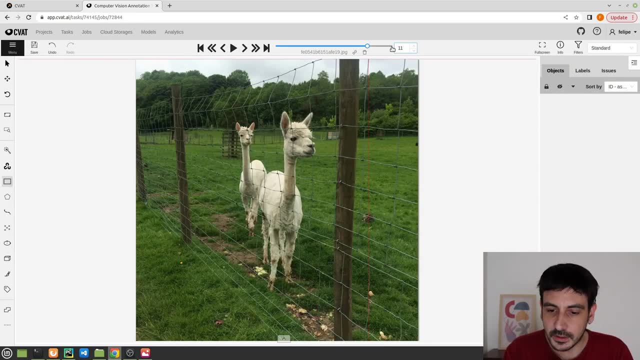 the entire body. i mean, i don't know, i'm surprised. maybe they are made like that, or maybe it's like a natural alpaca. who cares, who cares? let's continue. so we have, let's see how many. we have only a few left, so let's continue. uh, let's see. 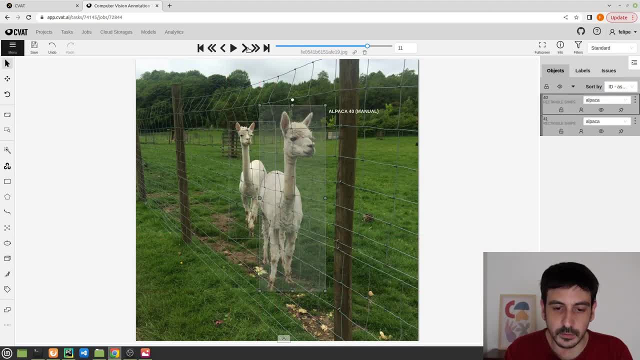 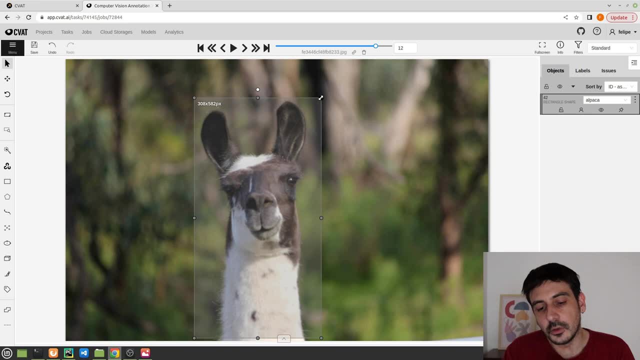 if we find any other strange situation which we have to define if that's an alpaca or not. so i can show you an additional example. also, when you are annotating, you could define your bounding box in many, many different ways. for example, in this case we could define it like this: 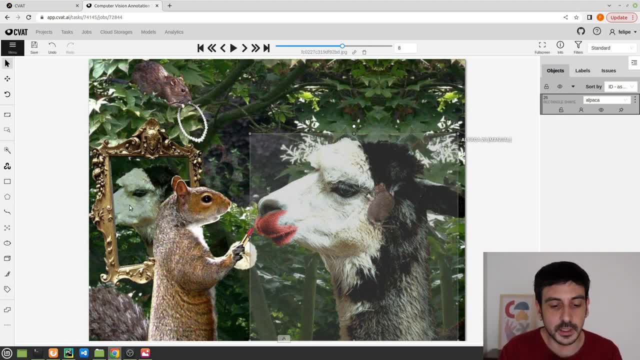 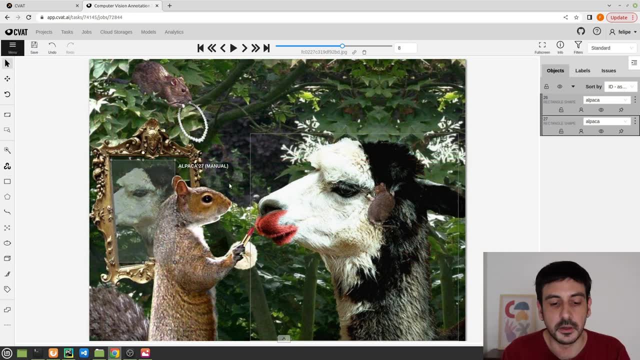 it's only like the, a very small, uh piece of the alpaca's face. so what do we do here? I am going to annotate this one too, because, yeah, that's my criteria, but another person could say, no, this is not the object I want to detect. this is only the object I want to detect, and maybe another person. 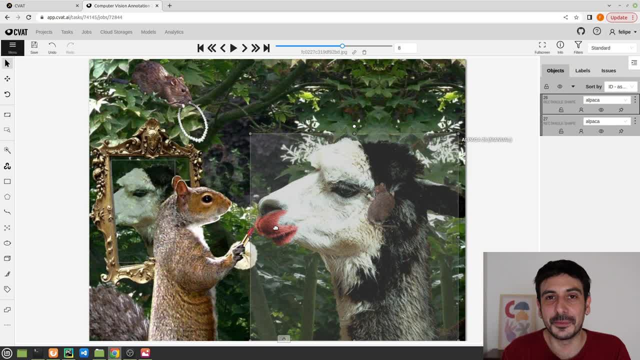 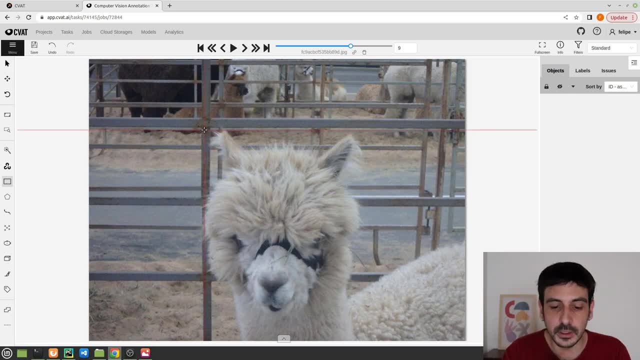 could say: no, this is not an alpaca. alpacas don't really apply makeup on them. this is not real, so I'm not going to annotate this image. you get the idea right. there could be many different situations and the only way you get familiar with all the different type of situations is if you annotate. 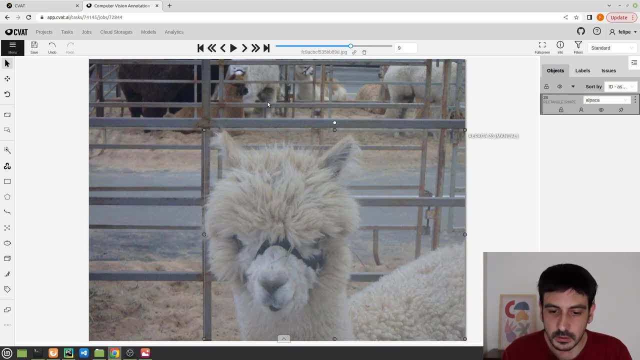 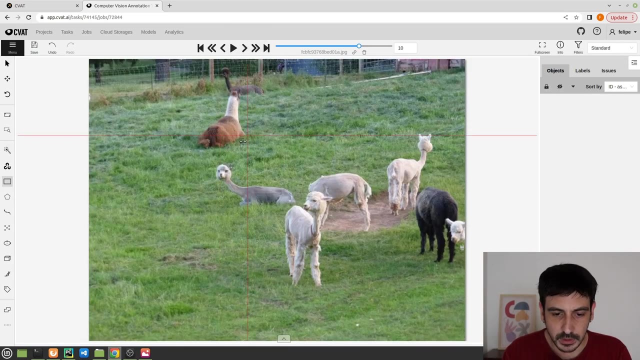 some images yourself. so now let's continue. in my case, I'm going to, I'm going to do something like this because, yeah, I will say, the most important object is this one, and the other ones are like, yeah, maybe that important if we detect them, or not? okay, so let's continue. this is very similar to 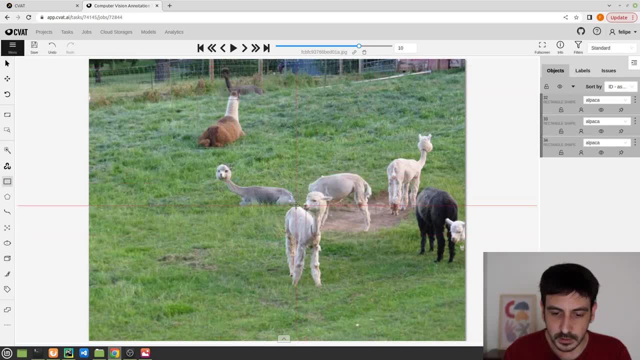 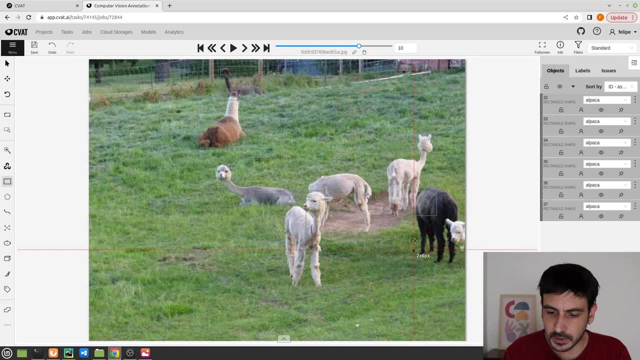 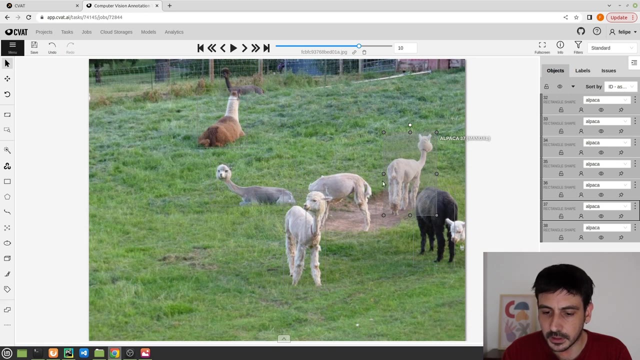 another image. I don't know how many I have selected, but I think it's. we have only a few left. I don't know if this type of animals. they are like natural. I'm very surprised about this. like the head right, it's like it has a lot of hair over here and then it's completely hairless the entire. 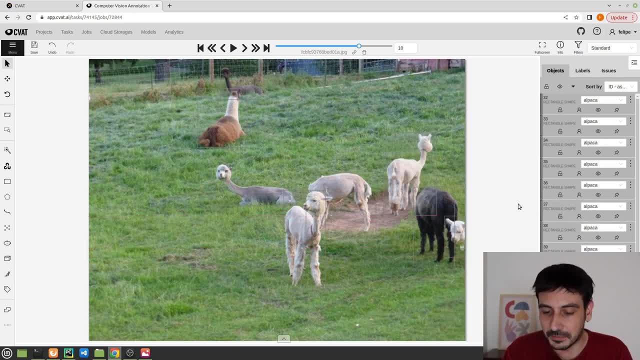 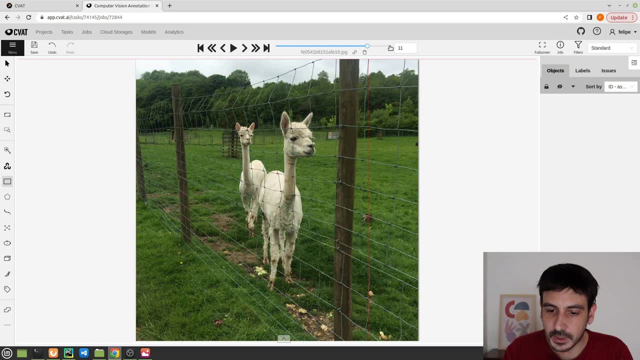 body. I mean, I don't know, I'm surprised. maybe they are made like that, or maybe it's like a natural alpaca. who cares? who cares? let's continue. so we have, let's see how many. we have only a few left, so let's continue. uh, let's see if we 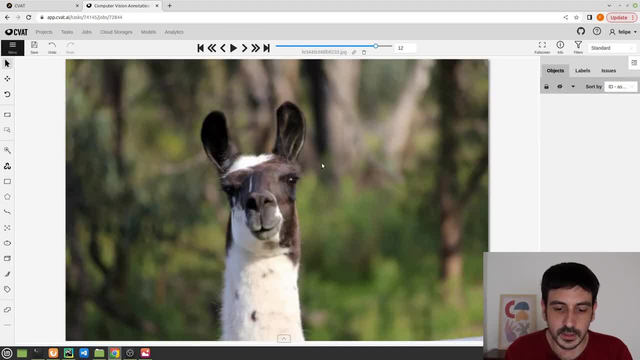 find any other strange situation which we have to define if that's an alpaca or not. so I can show you an additional example. also, when you are annotating, you could define your bounding box in many, many different ways. for example, in this case we could define it like this: 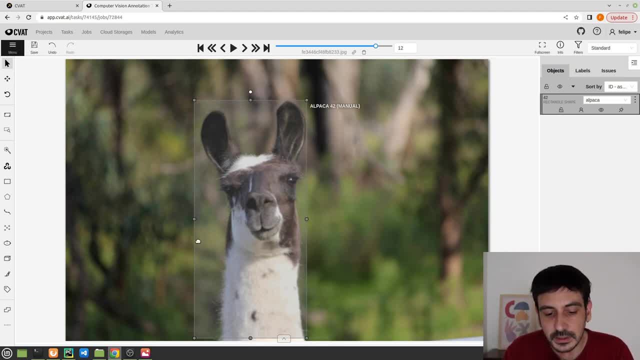 we could define it like this. I mean, we could define it super, super fit to the object, something like this: super, super fit, and we could enclose exactly the object, or we could be a little more relaxed, right, for example, something like this will be okay too. and if we want to do it like this, 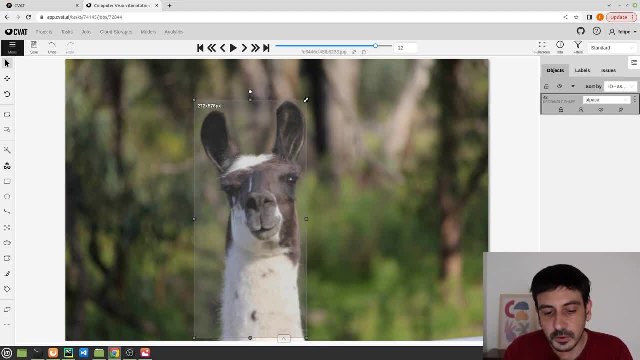 we could define it like this. i mean, we could define it super, super fit to the object, something like this: super, super fit, and we could enclose exactly the object, or we could be a little more relaxed, right, for example, something like this will be okay too. and if we want to do, 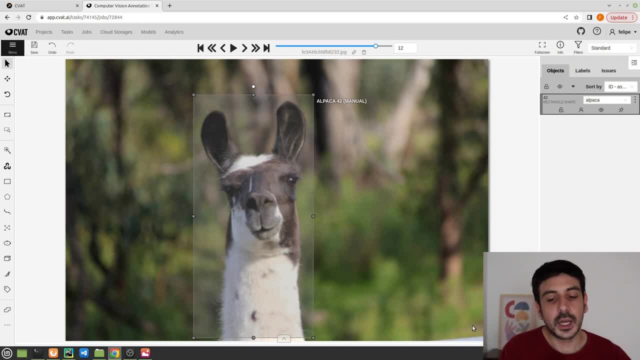 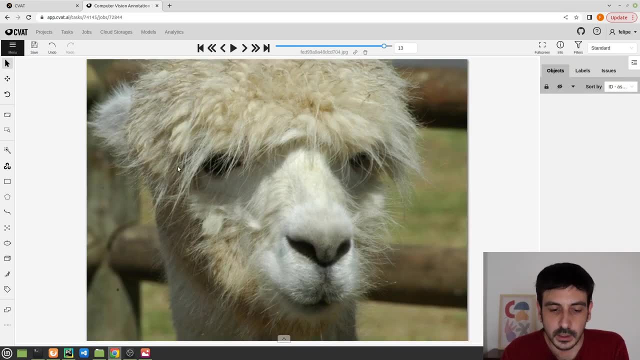 it like this. it will be okay too right, you don't have to be super, super, super, super accurate. you will be like a little more relaxed and it's going to work anyway. now, on this side of the image that i created, this is not the chamaued at the. however, at it is cool. i will do another video and if it doesn't fit, let me know what is going to happen next time. 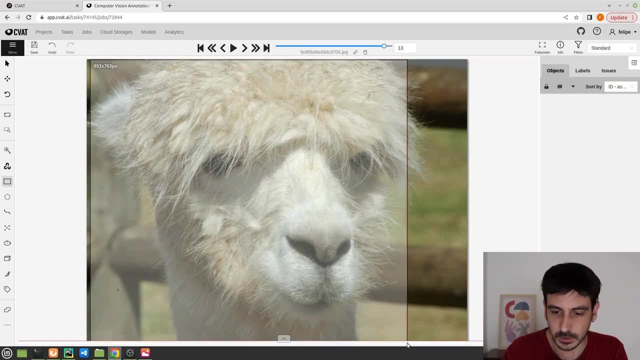 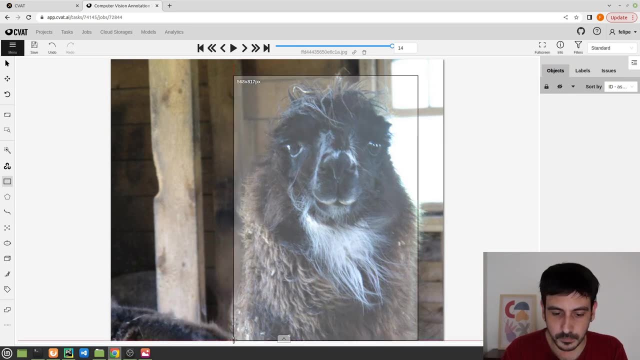 last one, and that's pretty much all. and this is the last one. okay, I'm going to do something like this. I'm going to do like this: I think this is also alpaca, but anyway, I'm just going to annotate this part, so that's pretty much all I'm going. 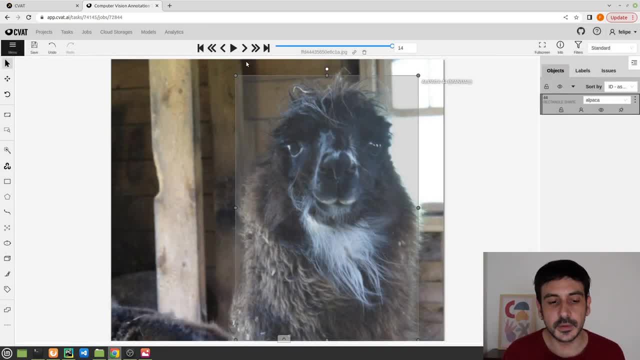 to save, and those are the few images I have selected in order to show you how to use this annotation tool. so that's pretty much all for the data annotation, and remember this is also a very important step. this is a very important task in this process because if we want to train an object detector, we need data. 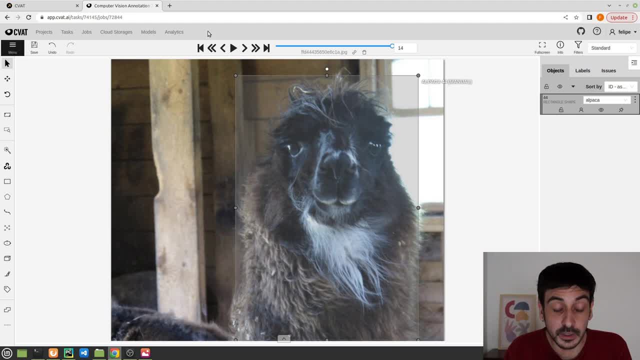 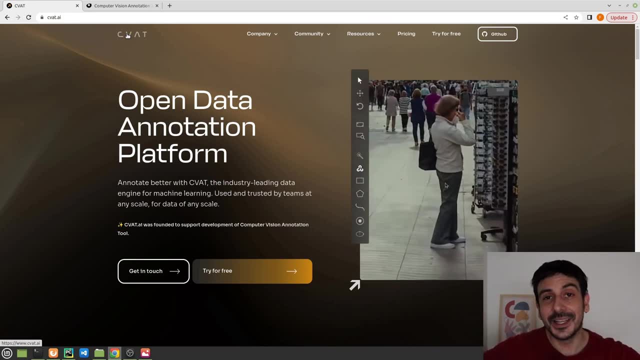 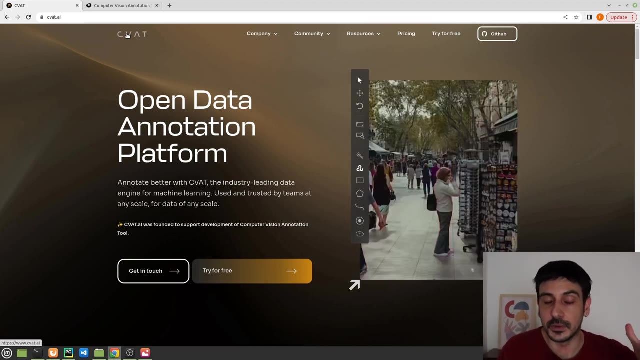 and we need annotated data. so this is a very important, very important part in this process. remember this tool, CBIT. this is only one of the many, many, many available image annotation tools. you can definitely use another one if you want. it's perfectly fine. it's not like you have to use this one at all. you can. 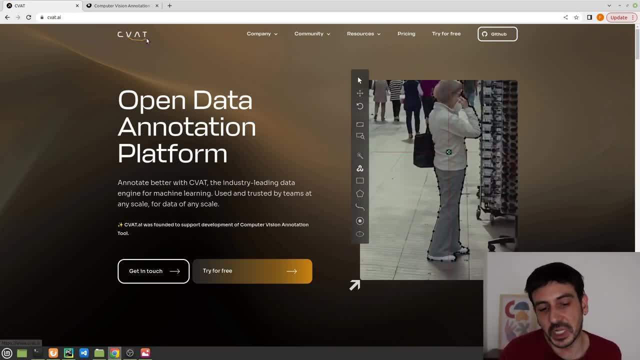 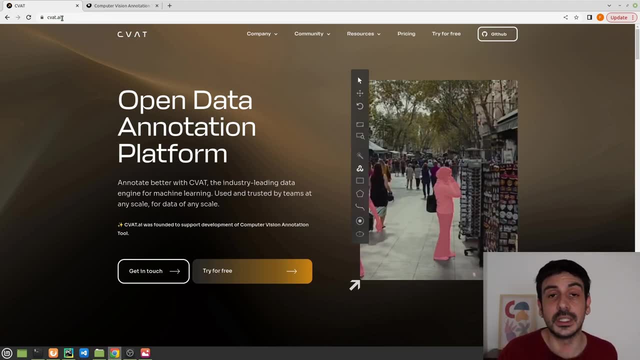 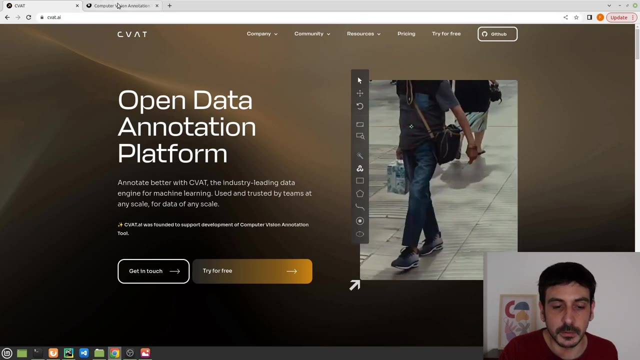 use whatever annotation tool you want, but this is a tool. I think it's very easy to use. I like the fact it's very easy to use. it's also a web application, so you don't really need to download anything to your computer. you can just go ahead and use it from the web. that's also one of its advantages. so, yeah, so. 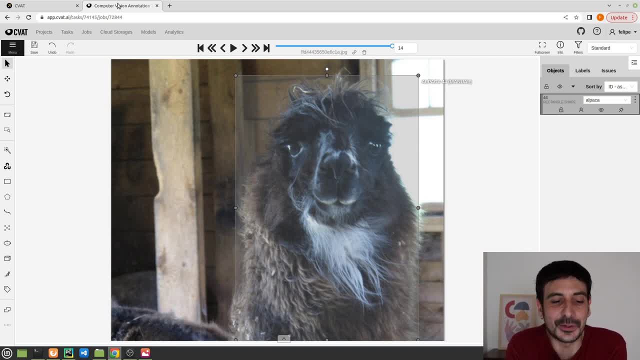 this is the tool I show you in this video how to use in order to train this object detector. is going to be all for this step, and now let's continue with the next part in this process. and now that we have collected and annotated all of our data, now it comes the time to format this. 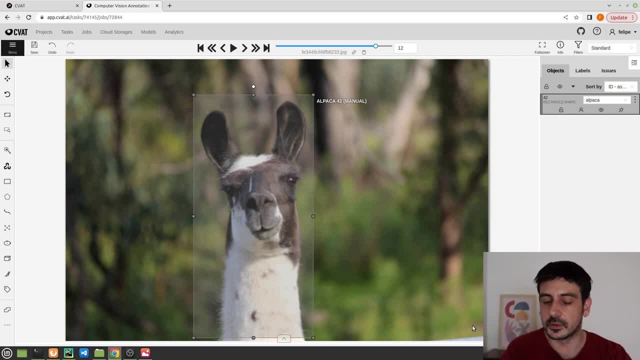 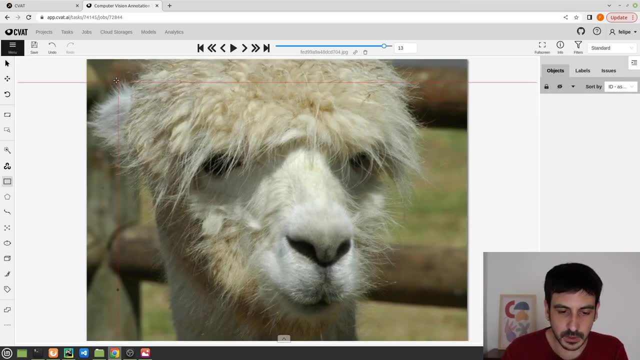 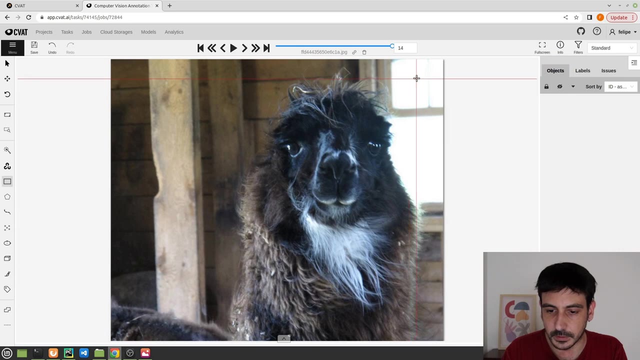 it will be okay too, right, you don't have to be super, super, super, super accurate. you could be like a little more relaxed, and it's going to work anyway. and now in this last one, um, that's pretty much all, and this is the last one, okay. 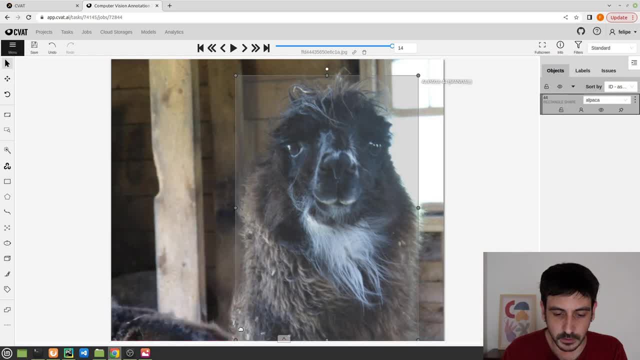 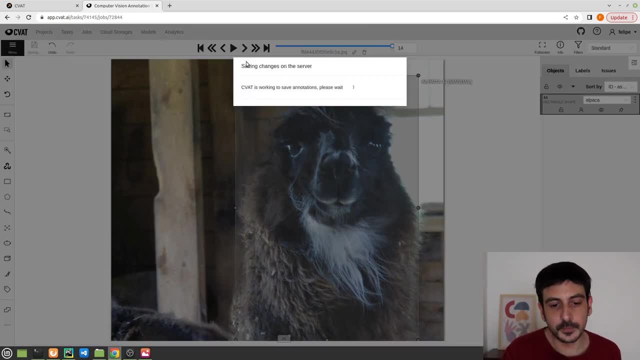 I'm going to do something like this. I'm going to do it like this. I think this is also alpaca, but anyway, I'm just going to annotate this part. so that's pretty much all I'm going to save, and those are the few images I have selected in order to show you how to use this annotation tool. so 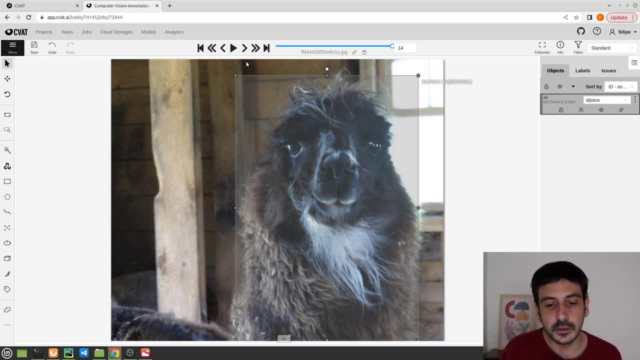 that's pretty much all for the data annotation and remember this is also a very important step. this is a very important task in this process because if we want to train an object detector, we need data and we need annotated data. so this is a very, very important part in this process. remember this tool: cbit. 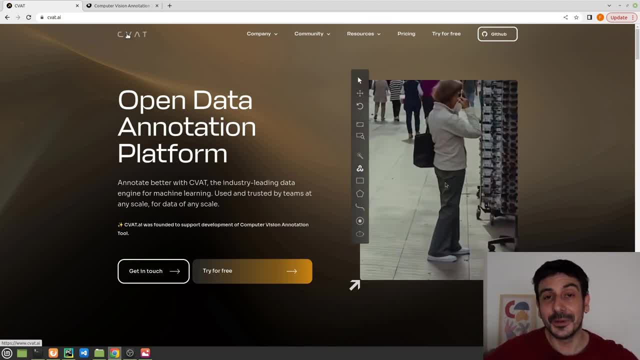 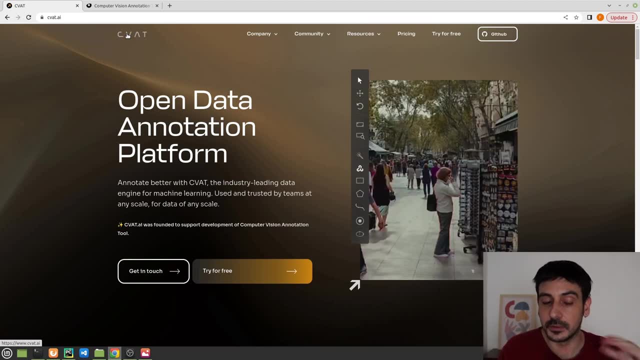 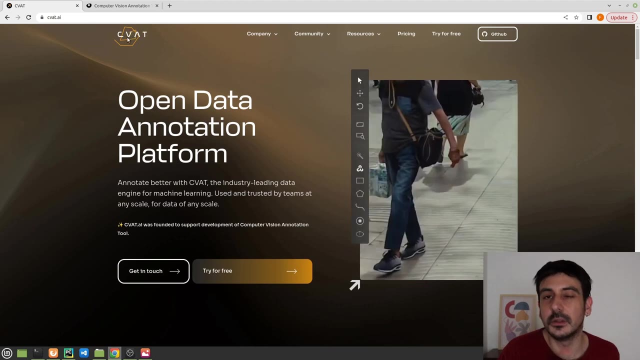 this is only one of the many, many, many available image annotation tools. you can definitely use another one if you want. it's perfectly fine. it's not like you have to use this one at all. you can use whatever annotation tool you want, but this is a tool. i think it's very easy to use. i like the. 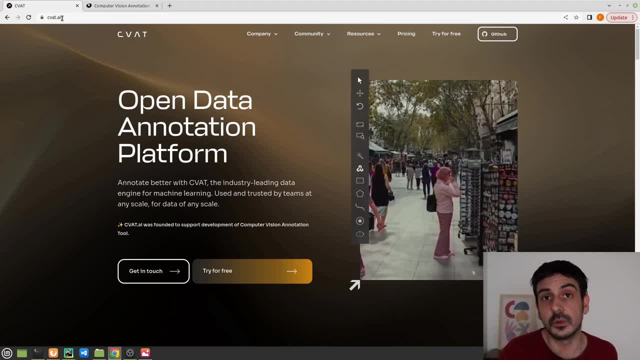 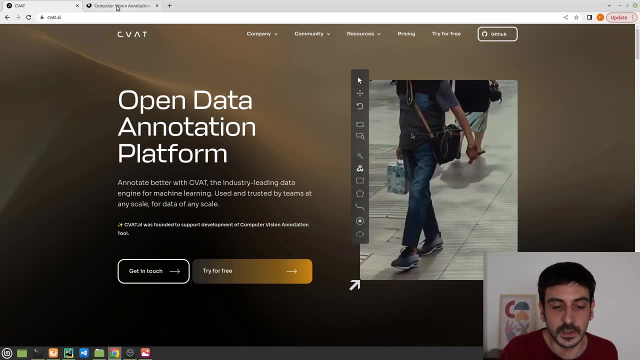 fact, it's very easy to use. it's also a web application, so you don't really need to download anything to your computer. you can just go ahead and use it from the web. that's also one of one of its advantages, so, yeah, so this is the tool i show you in this video how to use in order to 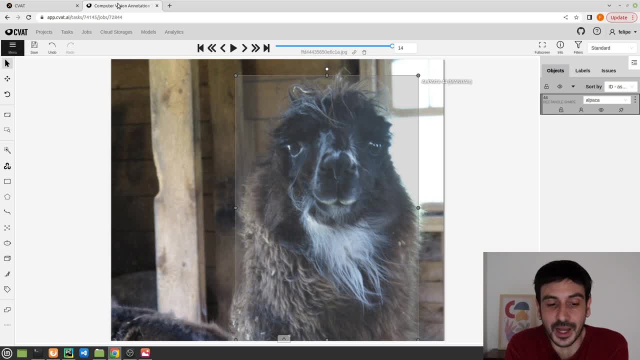 train this object detector. so this is going to be all for this step, and now let's continue with the next part in this process. and now that we have collected and annotated all of our data, now it comes the time to format this data, to structure this data into the format we need in order to 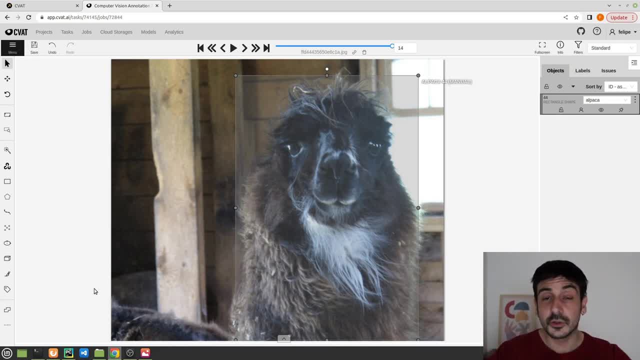 train an object detector using euro v8. when you're working in machine learning and you're training a machine learning model, every single algorithm you work with. it's going to have its own requirements on how to input the data. that's going to happen with absolutely every single. 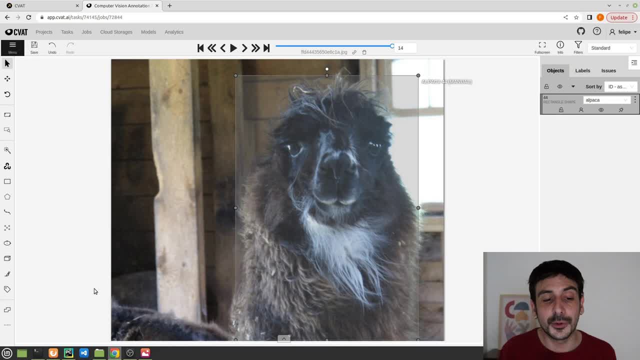 data, to structure this data into the format we need in order to train an object detector using your ob8. when you're working in machine learning and you're training a machine learning model, every single algorithm you work with it's going to have its own requirements on how to input the 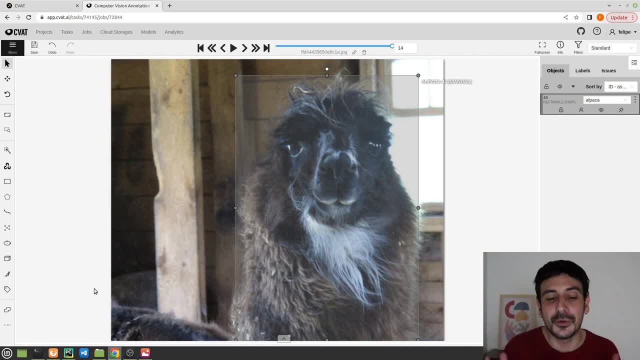 data. that's going to happen with absolutely every single algorithm you will work with. it's going to happen with yolo, with all the different yolo versions, and it's going to happen with absolutely every single argument you are working with. so, specifically, yolo dialog8. 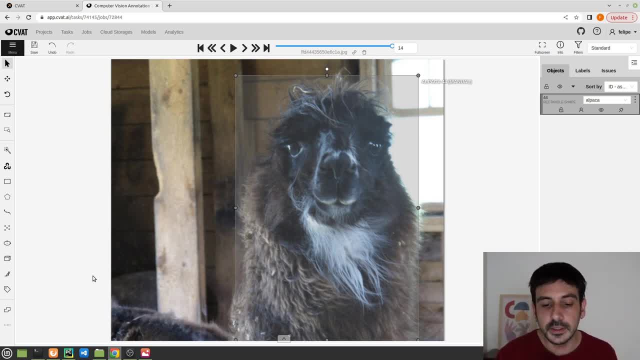 needs the data in a very specific format. so i created this step in this process so we can just take all the data we have generated, all the images and all the annotations, and we can convert all the data from the Joanna V8 algorithm to an ob8 and then we have generated it all right now. 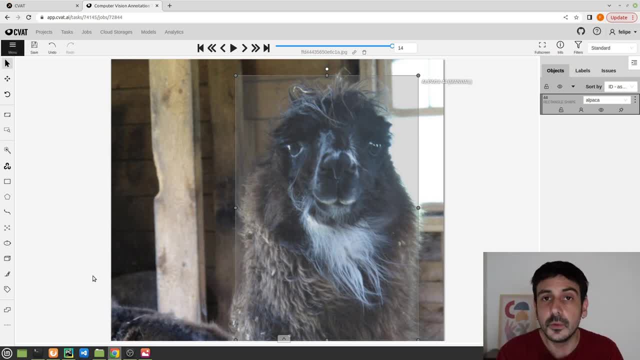 as a return factor, and we can just leave this bare Demon Pixels data so we can also edit the stability these images into the format we need in order to input this data into yellow v8. so let me show you exactly how we are going to do that. if you have annotated the data using cbat, you have to go to: 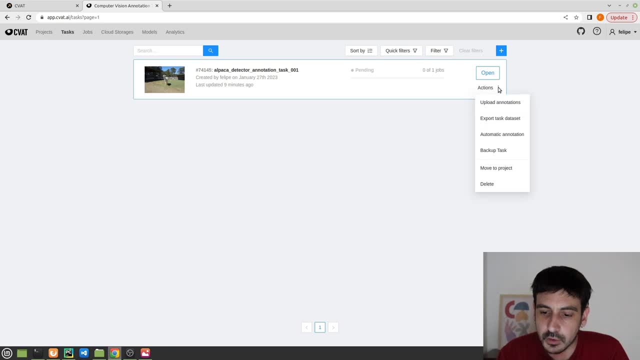 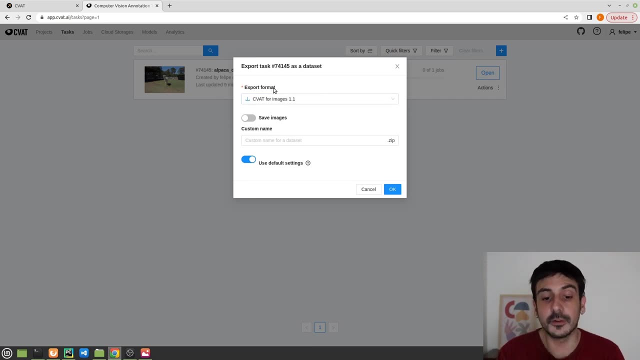 tasks and then you have to select this option and it's export task data set. it's going to ask you the export format so you can export this data into many different formats, and you're going to choose. you're going to scroll all the way down and you're going to choose yolo 1.1. right, then you can also. 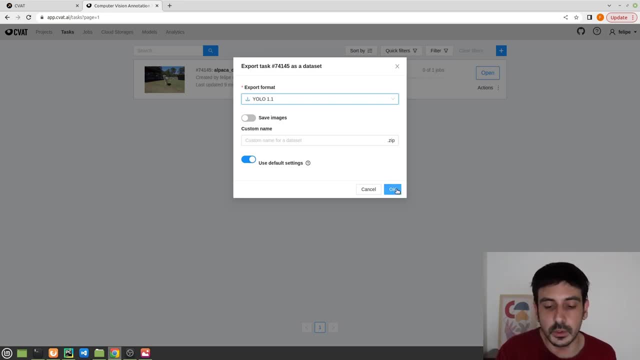 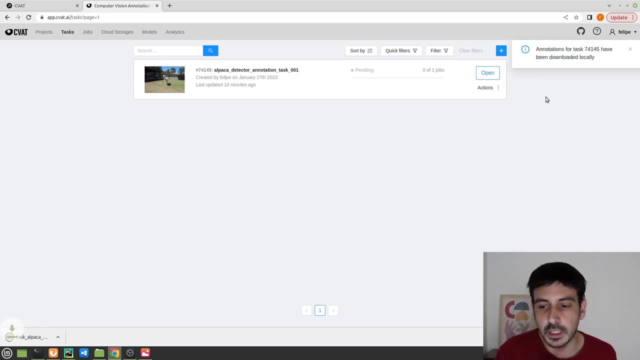 save the images, but in this case, not really needed. we don't really need the images. we already have the images and you're just going to click. ok, now, if you wait a few seconds or a few minutes, if you have a very large data set, you are going to download a file like this. and if i open this, 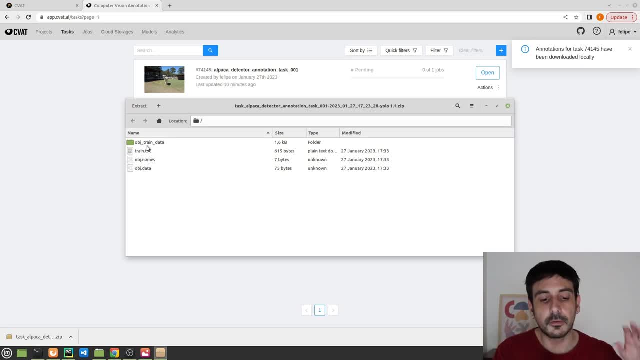 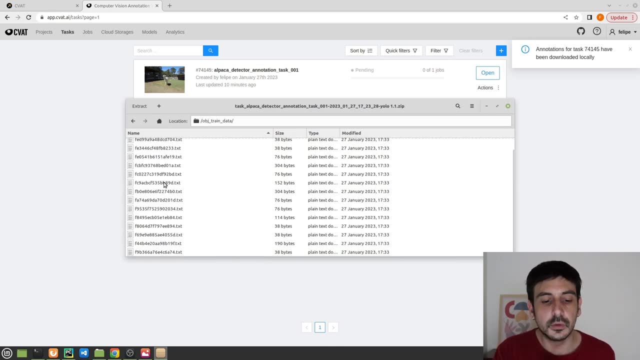 file. you're going to see all these different files. right, you can see we have four different files, or actually three files and a directory. and if i open the directory, this is what you are going to see, which is many, many different file names. and if i go back to the 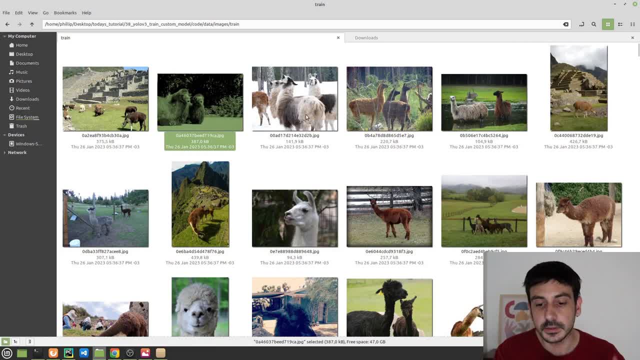 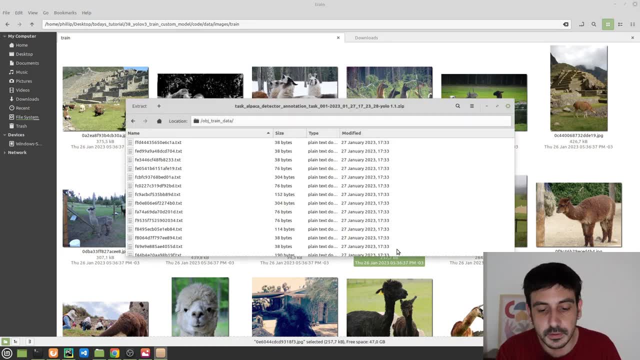 images directory. you will see that all these images, file names, they all look pretty much the same. right, you can see that the, the file name, the, the structure for this file name, looks pretty much the same as the one with as the ones we have just downloaded from cbat. so basically, the way it works. 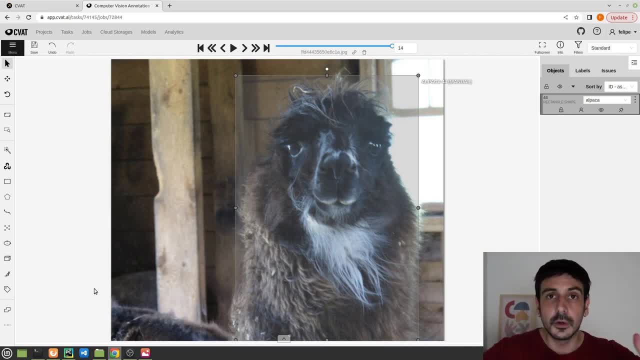 algorithm you will work with. it's going to happen with yolo, with all the different yolo versions, and it's going to happen with absolutely every single algorithm you are working with. so, specifically, yolo, yolo v8 needs the data in a very specific format, so i created this step in this process. 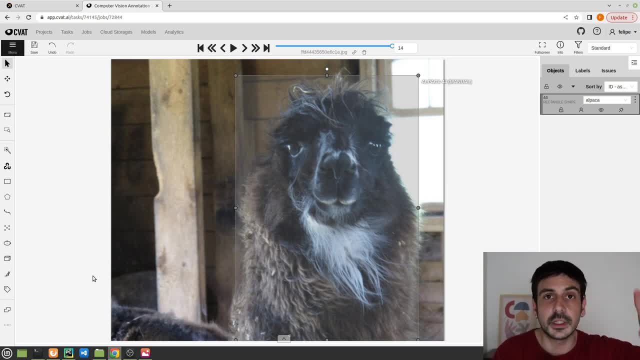 so we can just take all the data we have generated, all the images and all the annotations, and we can convert all these images into the format we need in order to input this data in to yellow v8. so let me show you exactly how we are going to do that. if you have annotated the data, 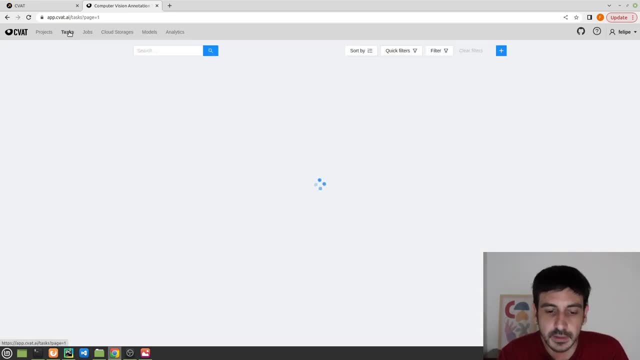 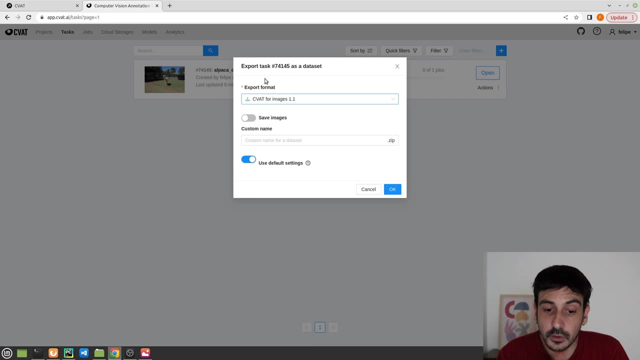 using a cbat. you have to go to tasks and then you have to select this option and it's export task data set. it's going to ask you the export format so you can export this data into many different formats, and you're going to choose. you're going to scroll all the way down and 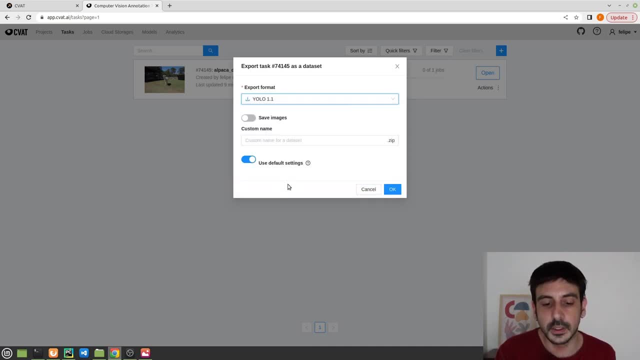 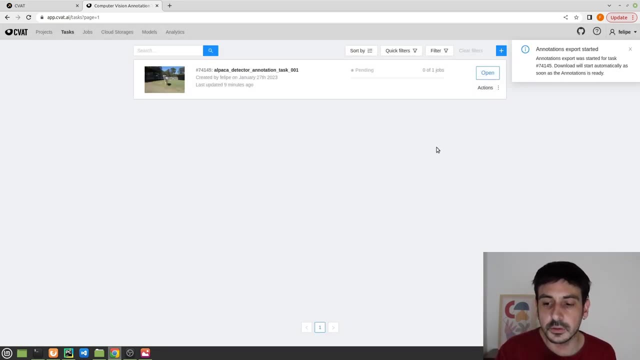 you're going to choose yolo 1.1. right, then you can also save the images. but in this case not really needed, we don't really need the images. we already have the images and you're just going to click. ok now, if you wait a few, 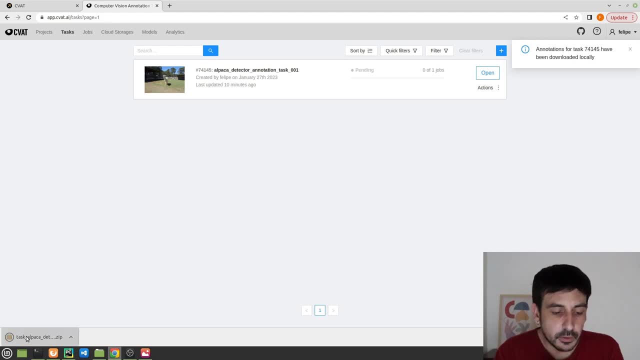 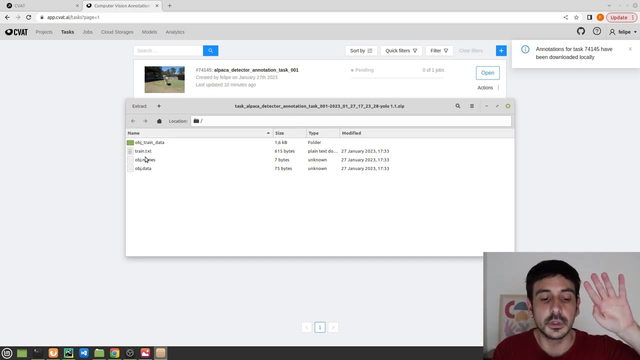 seconds or a few minutes. if you have a very large data set, you are going to download a file like this and if i open this file, you're going to see all these different files. right, you can see we have four different files, or actually three files and a directory, and if i open the directory, this: 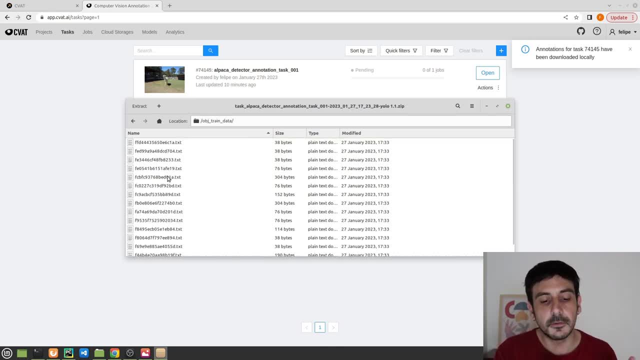 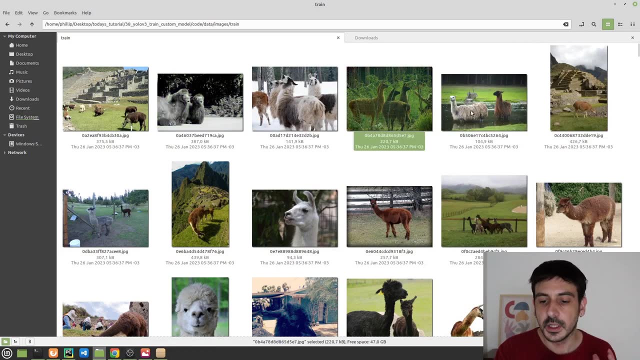 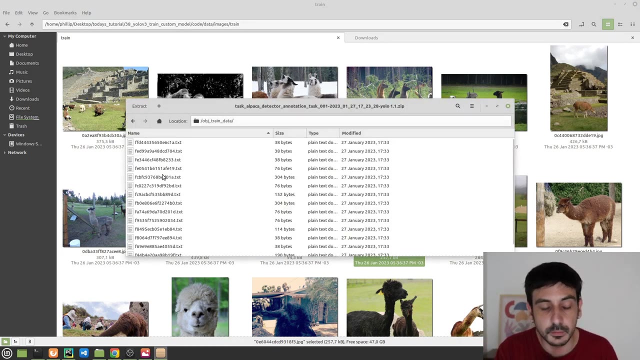 is what you are going to see, which is many, many different finelanes. And if I go back to the images directory, you will see that all these images, file names, They all look pretty much the same. right, You can see that the the file name did. the structure for this file name looks pretty much the same as the one with as the. 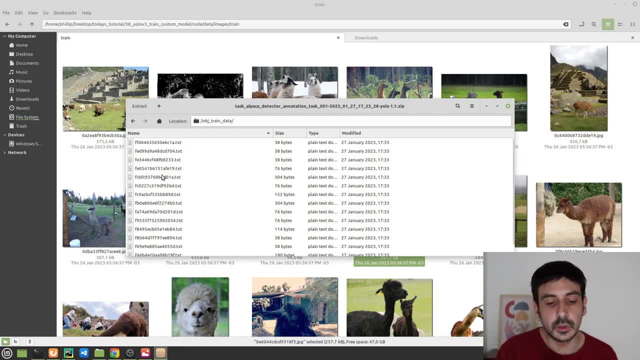 Ones we have just downloaded from CBAT. So basically the way works is that when you are downloading this data into this format, into the yellow format, Every single annotation file is going to be downloaded With the same name as the image you have Annotated, but with a different extension. So if you have an image which was called 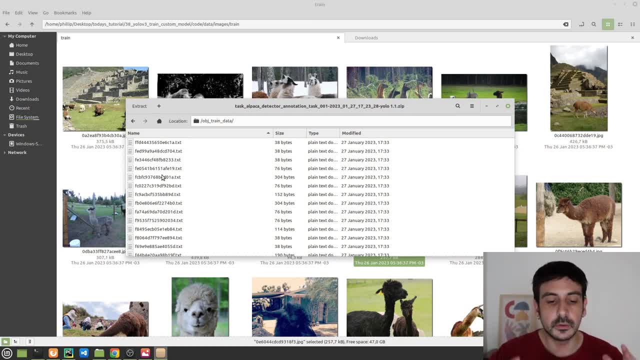 is that when you are downloading this data into this format, into the yolo format, every single annotation file is going to be downloaded with the same name as the image you have annotated, but with a different extension. so if you have an image which was called something dot jpg, then the annotation file for that specific image will be something dot txt, right? 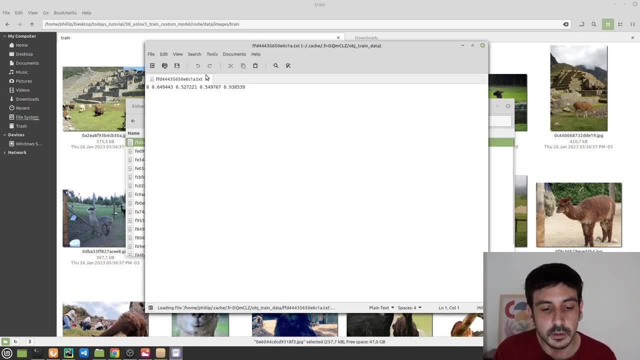 so that's the way it works, and if i open this image, you are going to see something like this. you're going to see, in this case, only one row, but let me show you another one which contains more than one annotation- i remember there were many- for example, this one which contains two different rows and each one of 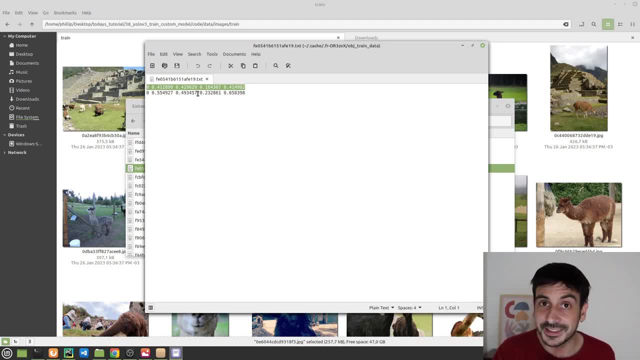 these rows is a different object. in my case, as i only have alpacas in this data set, each one of these rows is a different alpaca, and this is how you can make sense of this information. the first character is the class- the class you are detecting. 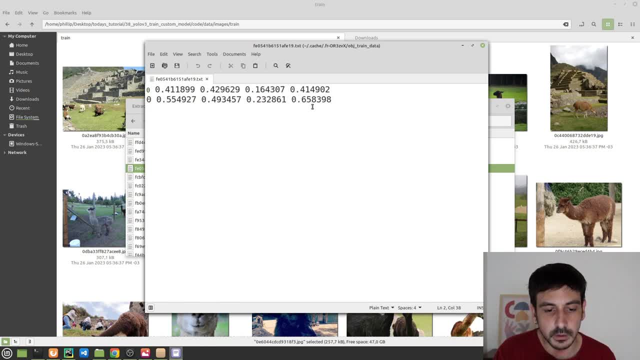 i wanted to enlarge the entire file and i don't know what i'm doing there, okay, okay, the first number is the class you are detecting. in my case, i only have one, so it's only a 0 because it's my only class- and then these four numbers which define the bounding box. 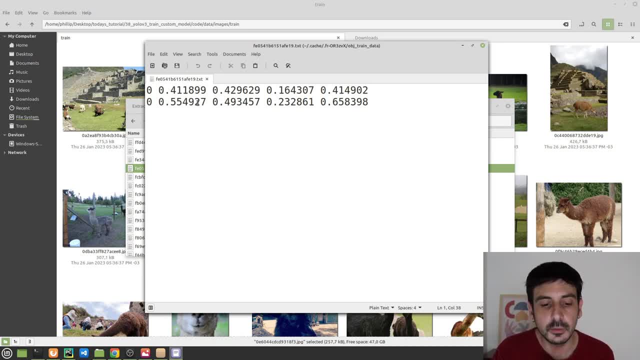 right. this is encoded in the yolo format, which means that the first two numbers are the position of the center or of the bounding box. then you have a number here like this: you see that first two, which methods that mirror the first numbers, and this is who are the last sub-classes. they are, and i used them for some reasons and the other was more for guesswork. in second, because in the 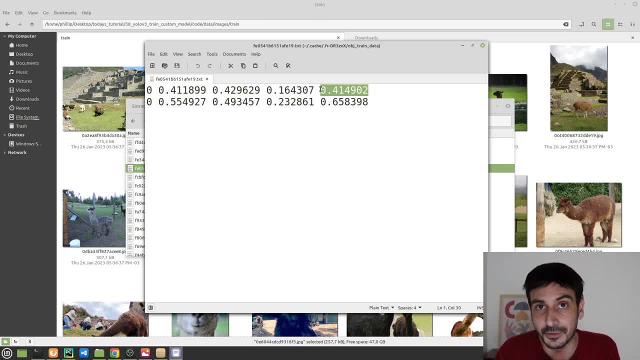 have the width of your bounding box and then the height of your bounding box. this you will notice. these are all float numbers and this basically means that it's relative to the entire size of the image. so these are the annotations we have downloaded, and this is in the exact same format. 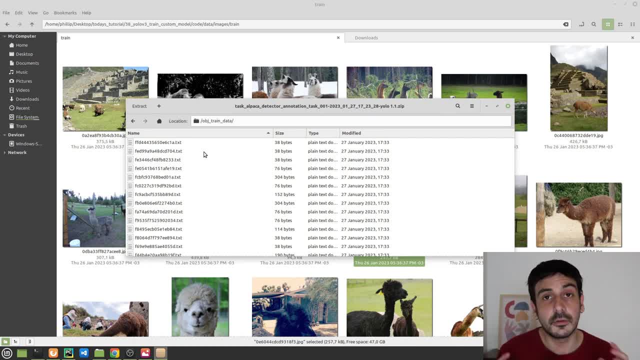 Something dot JPG, then the annotation file for that specific image will be something dot TXT, right, So that's the way it works, And if I open this image, you are going to see something like this: You're going to see, in this case, only one row. 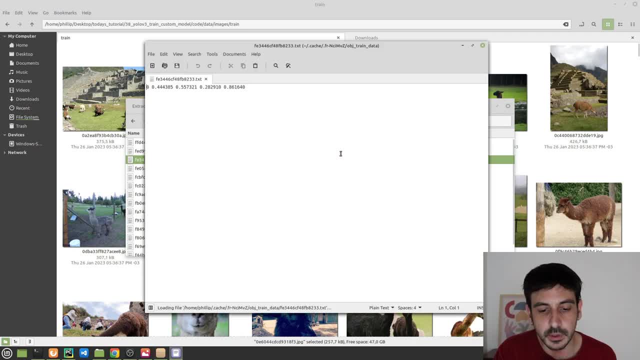 But let me show you another one which contains more Than one annotation- I remember there were many- for example, this one which contains two different rows and each one of these rows is a different object. In my case, as I only have alpacas in this data set, each one of these rows is a different alpaca. 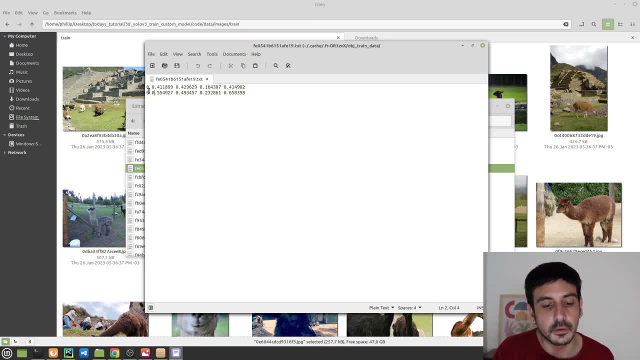 And this is how you can make sense of this information. The first Character is the class- the class you are detecting. I Wanted to enlarge the entire file and I don't know what I'm doing there. Okay, Okay, Okay. the first number is the class you are detecting. in my case, 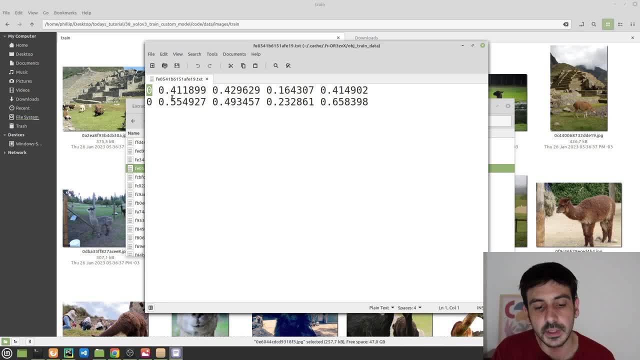 I only have one, so it's only a zero because it's my only class. and then these four numbers which Define the bounding box right. This is encoded in the YOLO format, Which means that the first two numbers are the position of the center or of the bounding box. 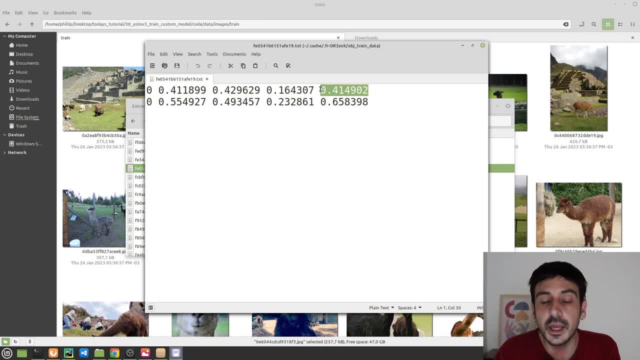 Then you have the width of your bounding box and then the height of your bounding box. This, you will notice, these are all float numbers and this basically means that it's relative to the entire size of the image. So these are the annotations we have downloaded, and this is in the exact same format. 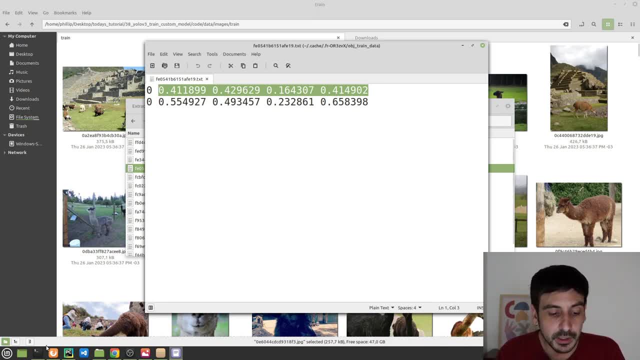 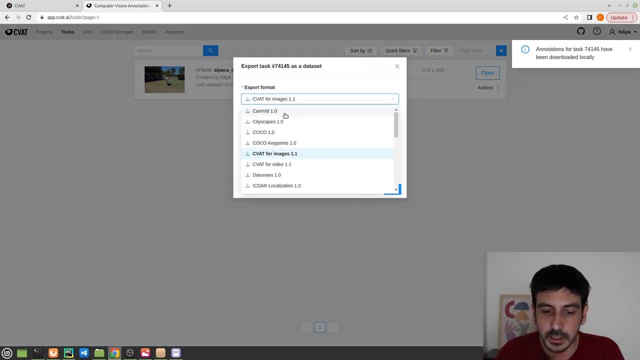 We need in order to train the subject detector. So remember, when I was downloading this, These annotations- we know these- there were many, many, many different options. all of these different options are different formats in which we could save the annotations, and This is very important, because you definitely need to download YOLO, because we are going to work with YOLO and everything. 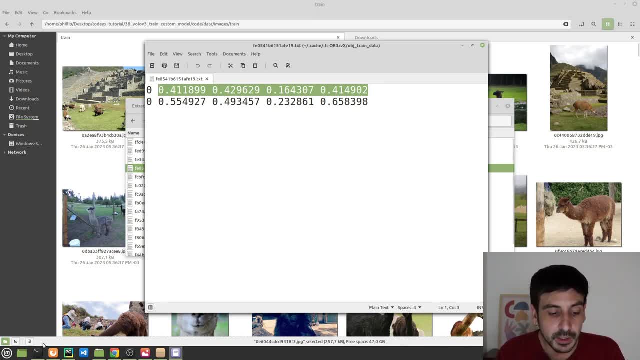 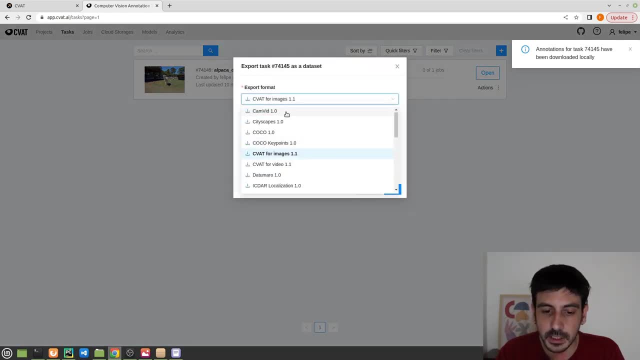 we need in order to train this object detector. so remember, when i was downloading this- uh, these annotations, we noticed there were many, many, many different options. all of these different options are different formats in which we could save the annotations, and this is very important, because you definitely need to download yolo, because we are going to work with yolo, and 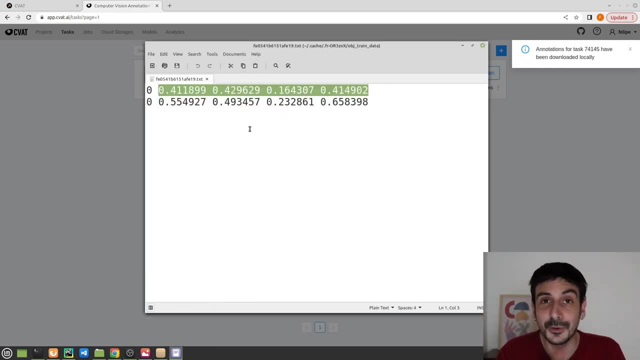 everything is pretty much ready as we need it in order to input into yolo v8, right? if you select yolo, that's exactly the same format you need in order to continue with the next steps, and if you have a specific format, you can do that as well. 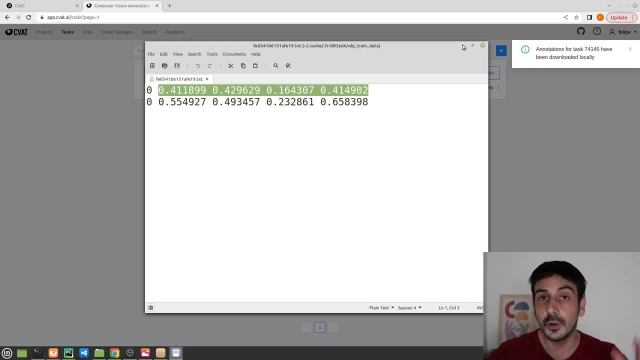 if you have your data into a different format. maybe if you have already collected and annotated your data and you have your data in whatever other format, please remember, you will need to convert these images, or actually to convert these annotations into the yolo format. now, this is one of the things. 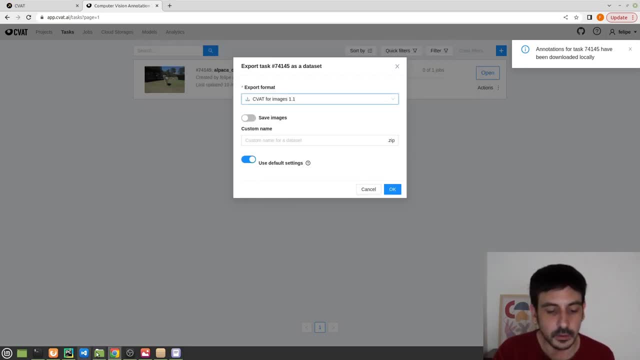 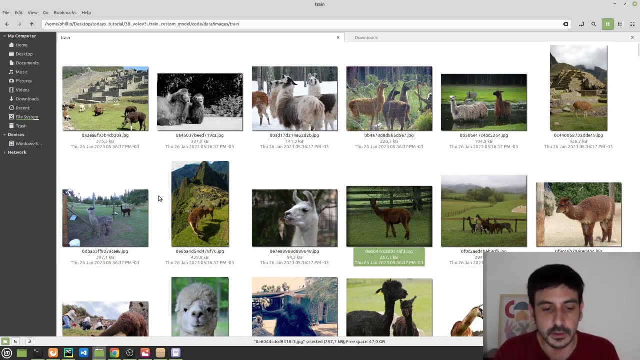 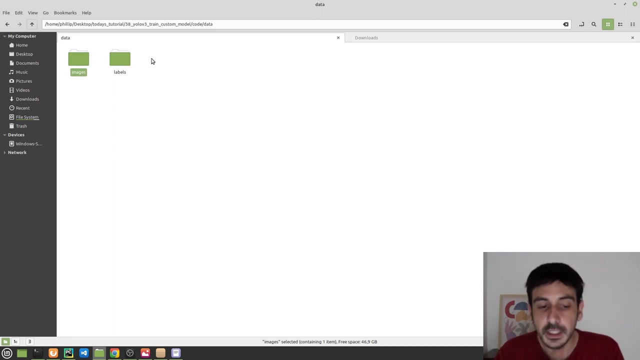 we need for the data. this is one of the things we need in order to. we need to format, in order to structure the data in a way. we can use this object detector with yolo v8, but another thing we should do is to create very specific directories containing this data right. 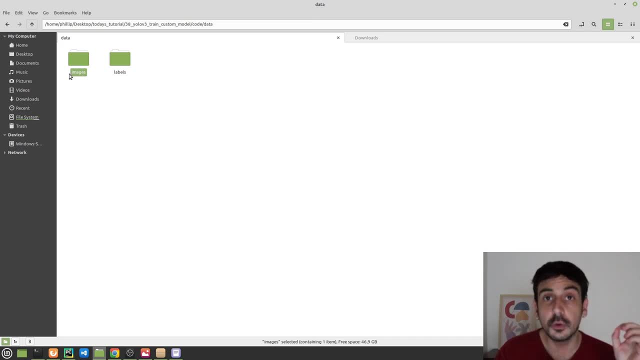 we are going to need two directories. one of them should be called images and the other one should be called labels. you definitely need to input these names. you cannot choose whatever name you want. you need to choose these two names, right? the images should be located in in a directory called images and the labels should be located in a directory called labels. 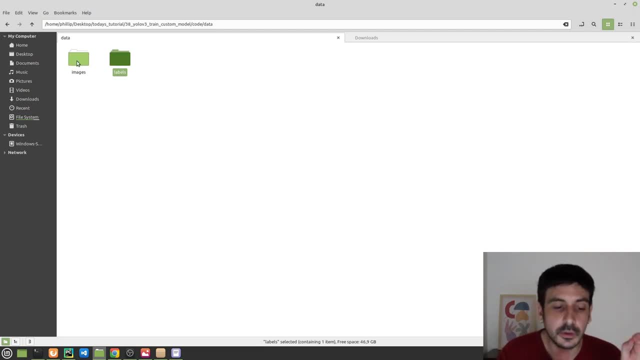 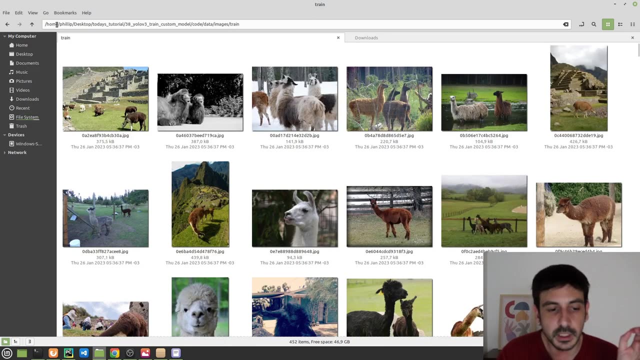 that's the way yolo v8 works, so you need to create these two directories within your images directory is where we are going to have your images. if i click here, you can see that these are all my images. they are all within the images directory. they are all within the train directory. 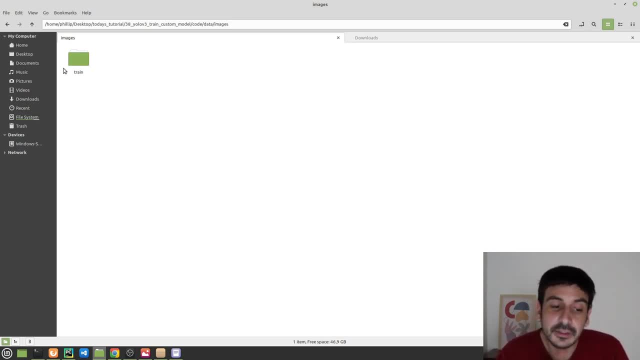 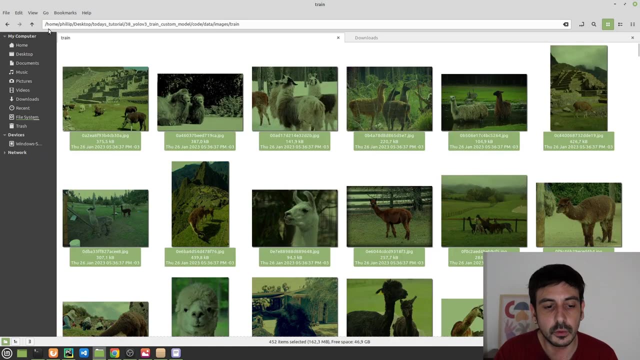 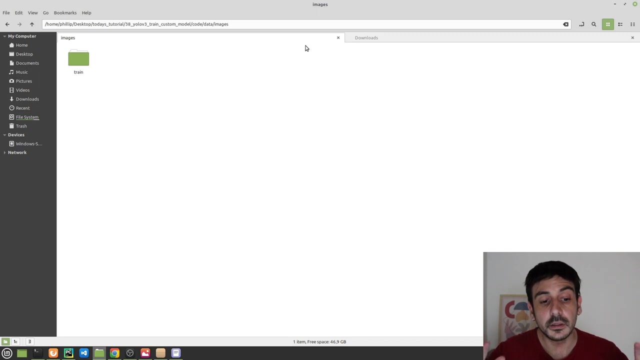 which is within the images directory. this director is not absolutely needed, right? you could perfectly take all your images, all these images, and you could just paste all your images here, right in the images directory, and everything will be just fine. but if you want, you could do something exactly as. 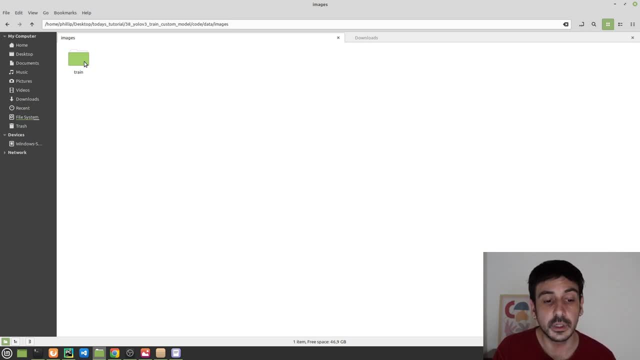 i did over here and you could have an additional directory which is in between images and your data and your images, and you can call this whatever way you want. this is a very good strategy in case you want to have, for example, a train directory containing all the training images and then 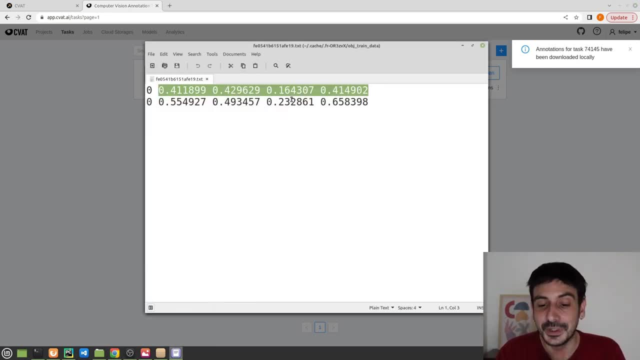 It's pretty much ready, as we need it in order to input into YOLO V8, right? If you select YOLO, That's exactly the same format you need in order to continue with the next steps, And if you have your data into a different format. 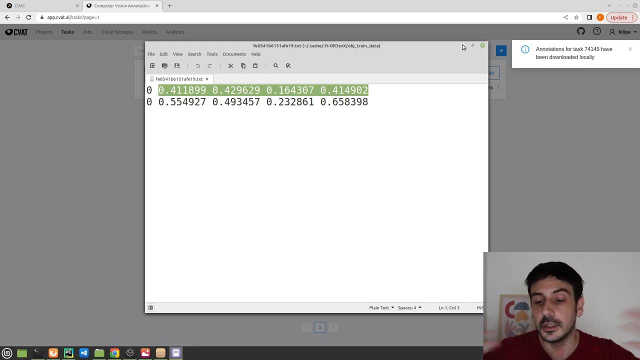 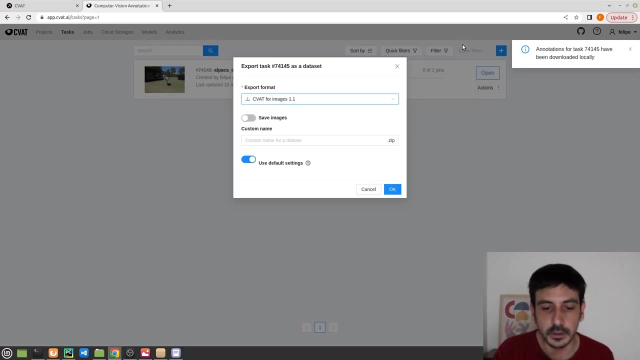 Maybe, if you have already collected and annotated your data and you have your data in whatever other format, Please remember, you will need to convert this image, Or actually to convert these annotations, into the YOLO format. Now, this is one of the things you we need For the data. This is one of the things we need in order to. we need to format in order to. 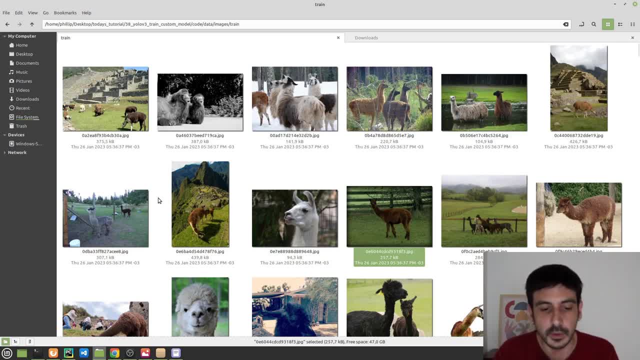 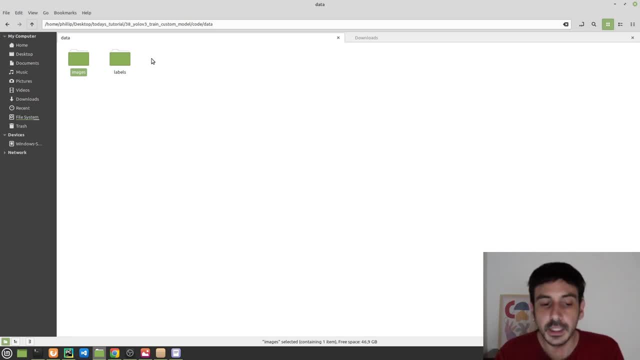 Structure the data in a way. we can use this object detector with YOLO V8, But another thing we should do is to create very specific directories Containing this data. right, We are going to need two directories. One of them should be called Images and the other one should be called labels. 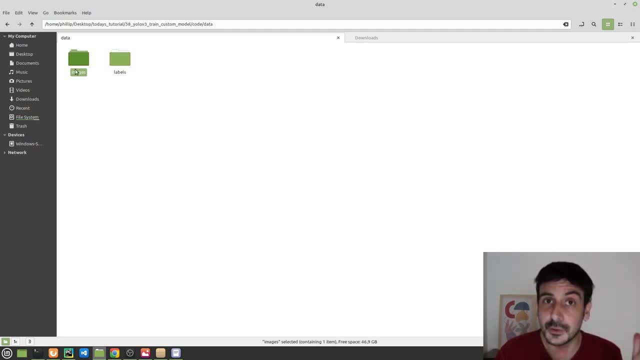 You definitely need to input these names. You cannot choose whatever name you want. You need to choose these two names, right? The images should be located in a directory called images and the labels should be located in a directory called Labels. that's the way YOLO V8 works, So you need to create these two directories within your images directory. is where we are going to. 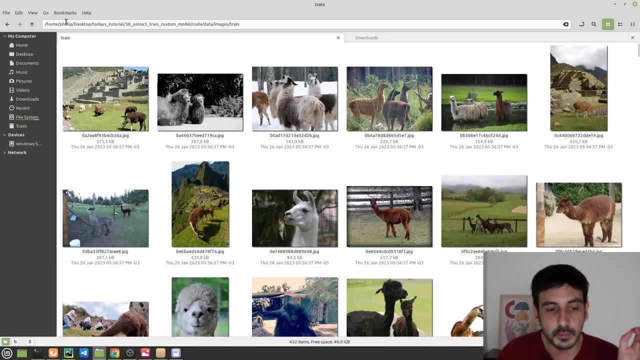 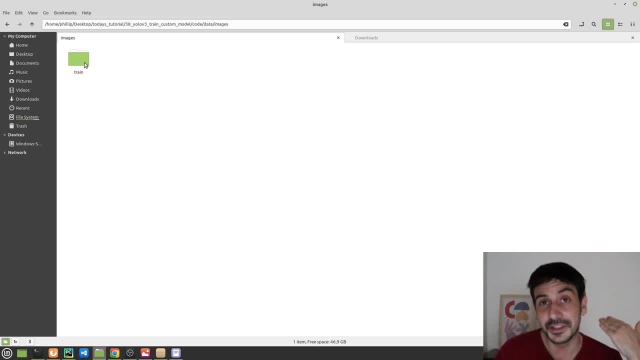 have your images. If I click here, you can see that these are all my images. they are all within the images directory. they are all within the train directory, which is within the images directory. this directory is not absolutely needed, right? you could perfectly take all your images, all these images, and you could just paste all your images here, right in the images directory. 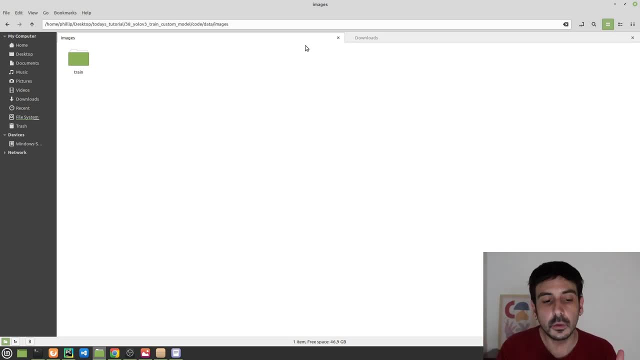 and everything will be just fine. but if you want, you could do something exactly as i did over here and you could have an additional directory which is in between images and your data and your images and you can call this whatever way you want. this is a very good strategy in case you want to have. 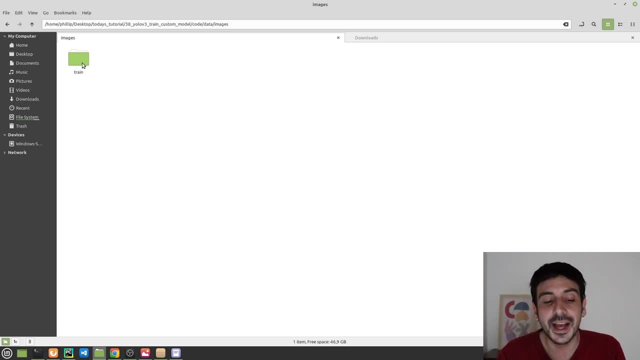 for example, a train directory containing all the training images, and then another directory which could be called validation, for example, and this is where you are going to have many images- in order to validate your process, your training process, your algorithm. and you could do the same with an additional directory which could be called test, for example. 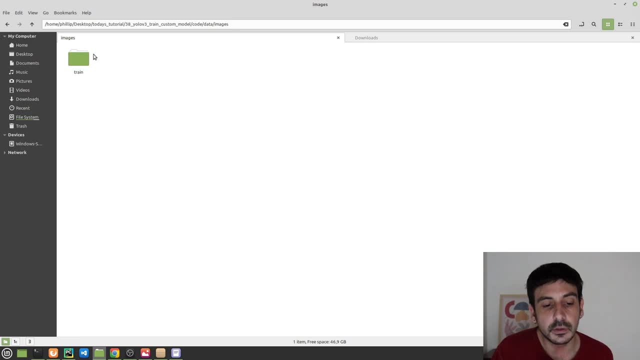 or you can just use these directories in order to um, to label the data right, to create different versions of your data, which is another thing which is very commonly done. so you could create many directories for many different purposes, and that will be perfectly fine, but you could also just: 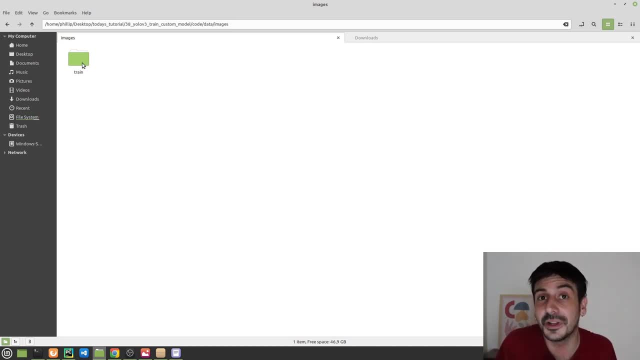 another directory, which could be called validation, for example, and this is where you're going to have many images- in order to validate your process, your training process, your algorithm. and you could do the same with an additional directory which could be called test, for example, or you can just use these directories in order to to label the data right, to create different versions. 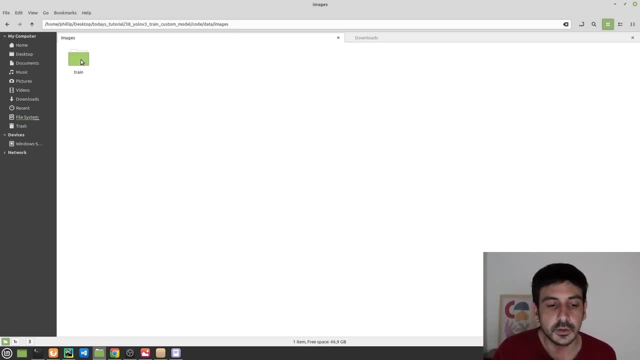 of your data, which is another thing which is very commonly done. so you could create many directories for many different purposes and that would be perfectly fine. but you could also show all the images here, and that's also perfectly fine, and you can see that for the labels directory i. 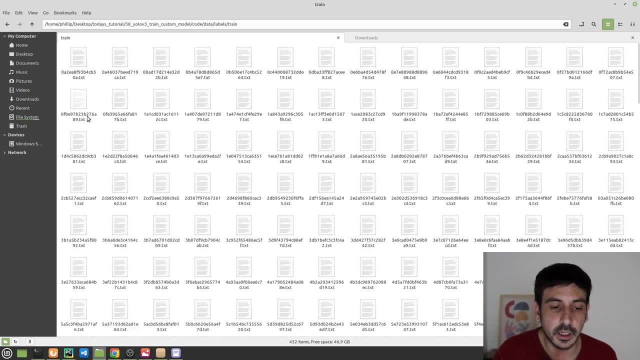 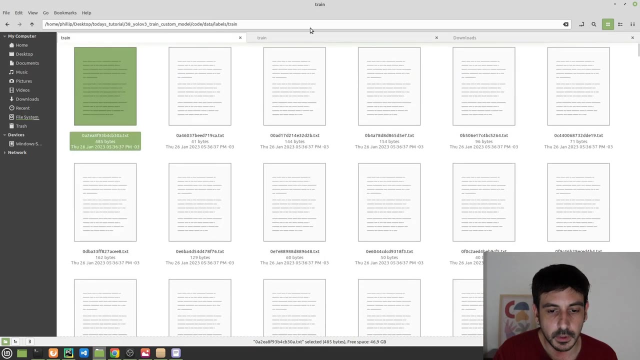 did exactly the same. we have a directory which is called train, and within this directory it's that we have all these different files and for each one of these files, let me show you like this it's going to be much better. for each one of these files, for each one of these txt files we will have. 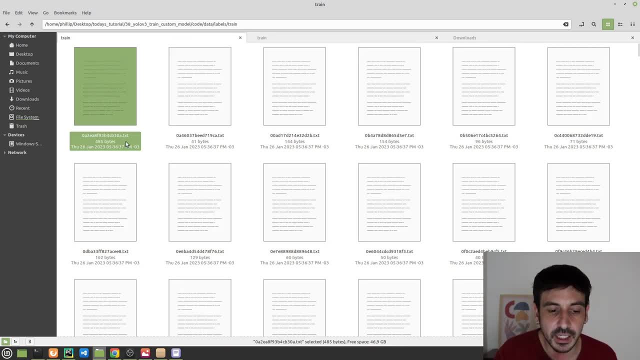 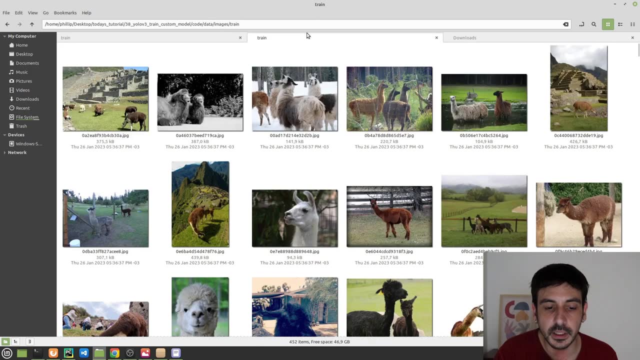 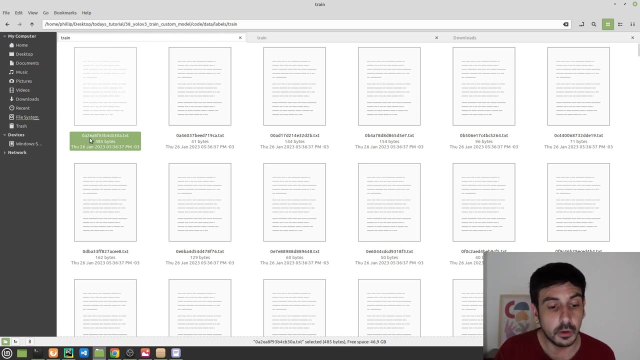 an image in the images directory which is called exactly the same. exactly the same file name, but a different extension, right? so in this case, this one is called dot txt and this one is called dot gpg, but you can see that it's exactly exactly the same file name. for example, the first image is called: 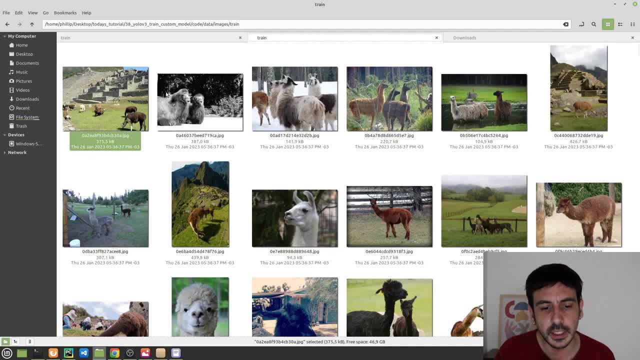 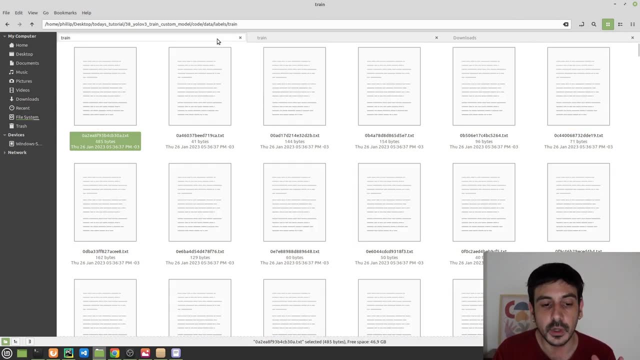 o a, 2, e, a, 8, f and so on, and that's exactly the same name as for the first image in the images directory, which is called o a, 2, e, a, 8 and so on. so basically, for absolutely every image in your images directory you need to have 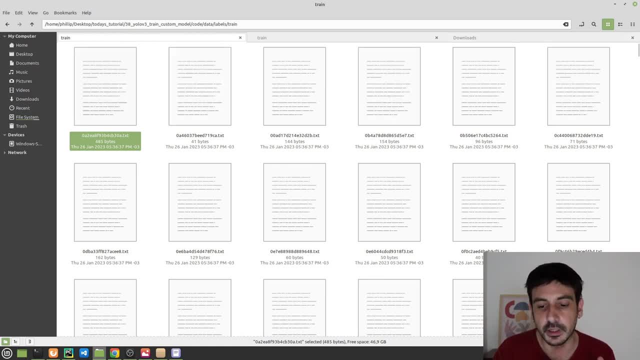 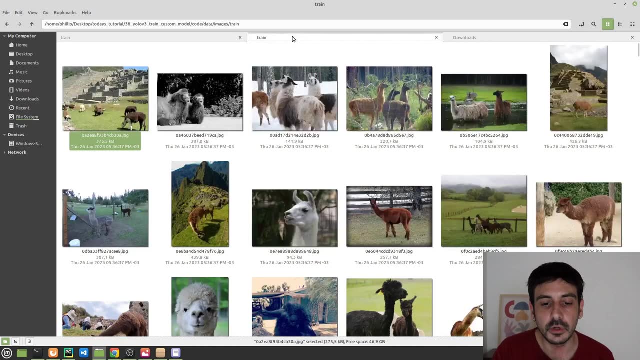 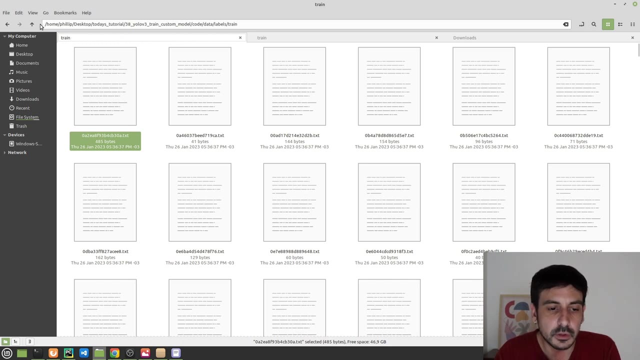 an annotations file and a file in the labels directory which is called exactly the same. exactly the same but with a different extension. if your images are dot gpg, your annotations files are dot txt. so that's another thing which also defines the structure you'll need for your data, and that's pretty much all. so remember you need. 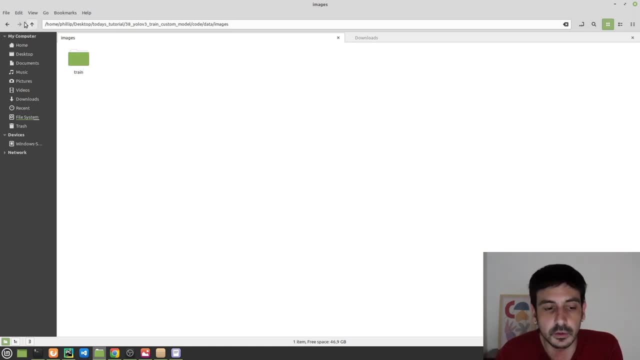 paste all the images here and that's also perfectly fine, and you can see that for the labels directory i did exactly the same. we have a directory which is in between the images directory and instead of building the files in the path directory which is in between the images directory, we have 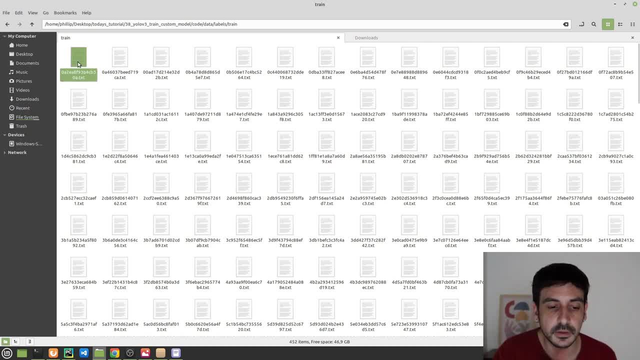 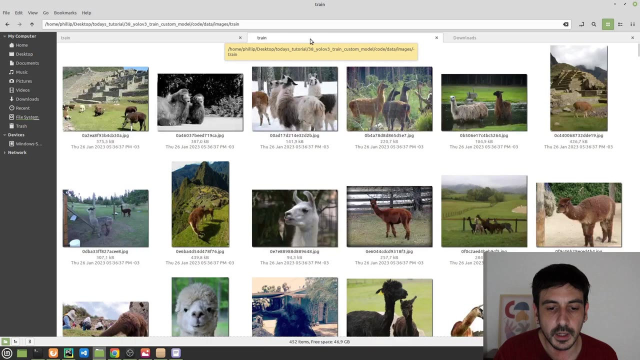 one, this, which is actually called train- and within these directories that we have all these different files, and for each one of these files, let me show you like this: it's going to be much better. for each one of these files, for each one of these txt files. 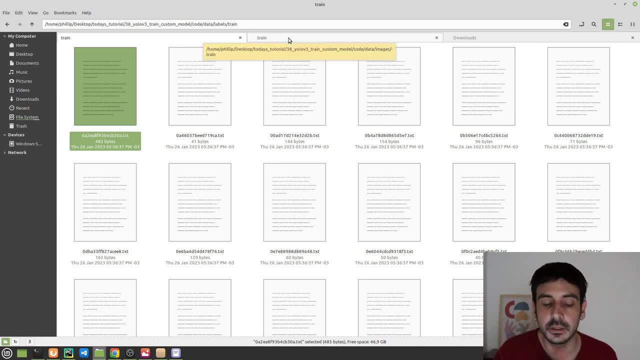 we will have an image in the images directory which is called exactly the same, exactly the same case. this one is called dot txt and this one is called dot gpg, but you can see that it's exactly exactly the same file name. for example, the first image is called oa2ea8f, and so on, and that's. 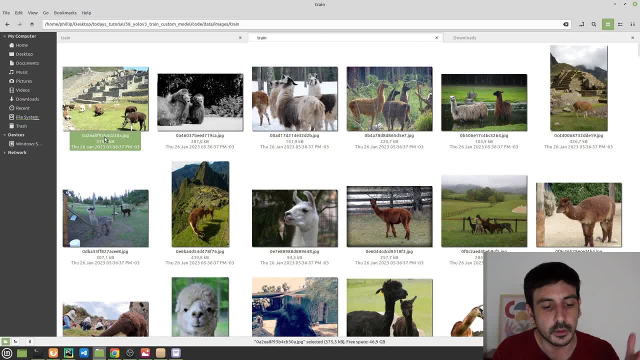 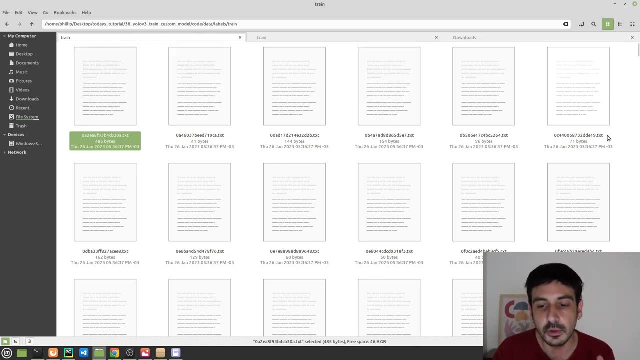 exactly the same name as for the first image in the images directory, which is called oa2ea8 and so on. so basically, for absolutely every image in your images directory, you need to have an annotations file and a file in the labels directory which is called exactly the same. 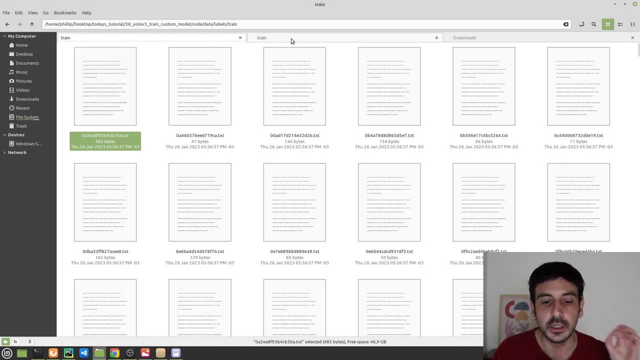 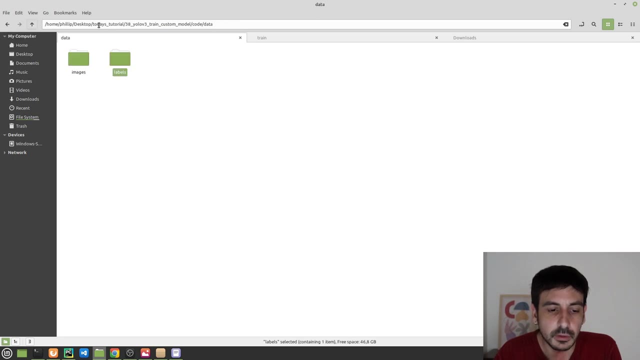 exactly the same, but with a different extension. if your images are dot gpg, your annotations files are dot txt. so that's another thing which also defines the structure you need for your data, and that's pretty much all. so remember you need to have two directories. one of them is called 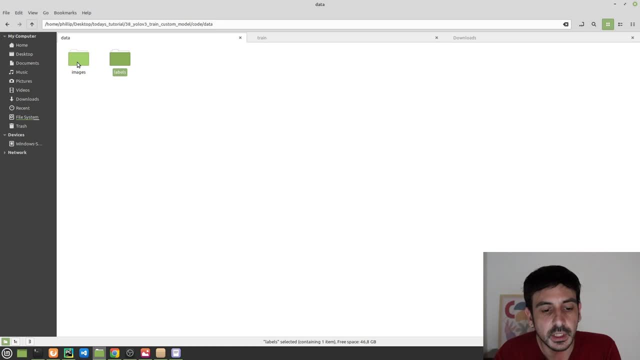 to read thechas and this form is rather difficult for me, but if you're more experienced or you know, have two directories. one of them is called images, the other one is called labels. within the images directory is where you're going to have all your images and within your labels directories where 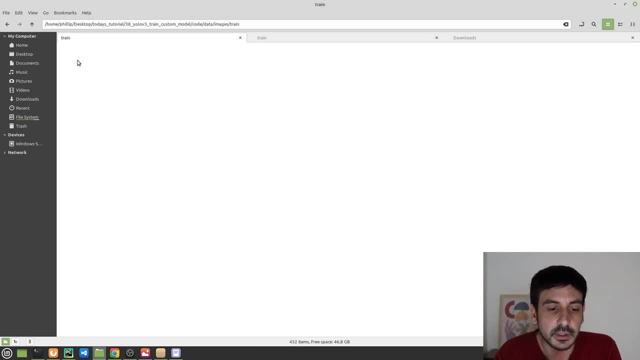 images, the other one is called labels, within the images directory is worked out, the other one is called labels, and so on, and so forth, and so on, and so on, and so on. you're going to have all your images and within your labels, directories where you will have all. 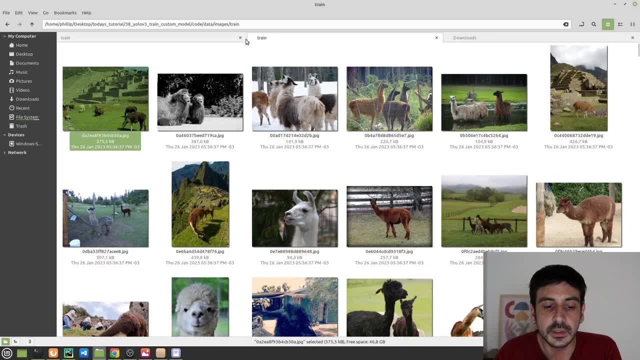 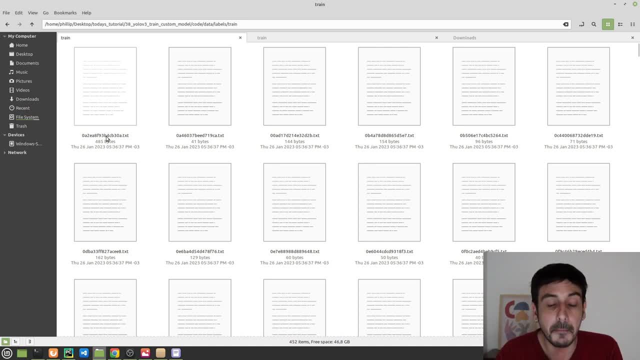 your annotations or your labels, and for absolutely every single image in your images directory, you will need to have a file in the labels directory which is called exactly the same but with a different extension. if the, if your images are jpg, your annotations file should be txt and 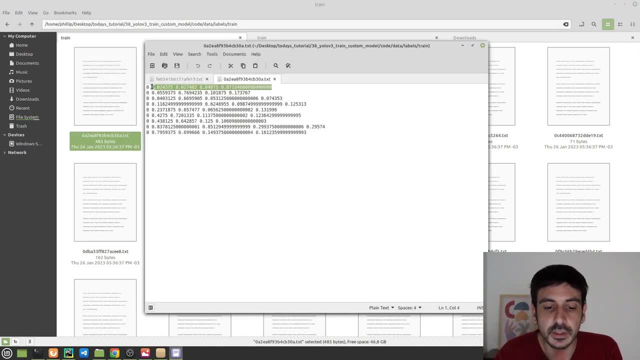 the labels should be expressed in the yellow format, which is as many rows as objects in that image, and every single one of these rows should have the same structure. you are going to have five terms. the first one of them is the class id. in my case, i only have one class id. i'm only 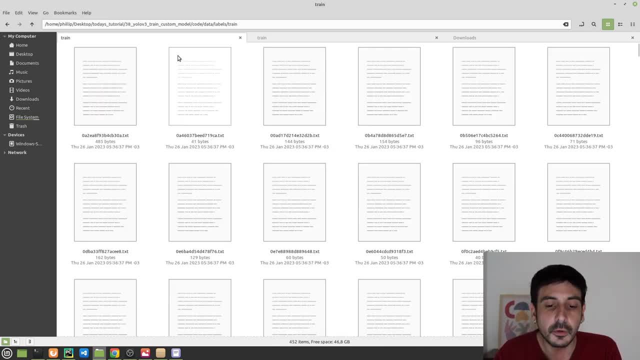 you will have all your annotations, or your labels, and for absolutely every single image in your images directory, you will need to have a file in the labels directory which is called exactly the same but with a different extension. if the if your images are dot jpg, your annotations file should be: 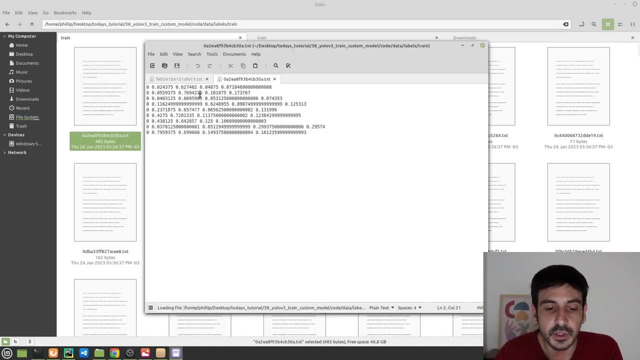 dot txt and the labels should be expressed in the yellow format, which is as many rows as objects in that image, and every single one of these rows should have the same structure. you are going to have five terms. the first one of them is the class id. in my case, i only have one class id. i'm only 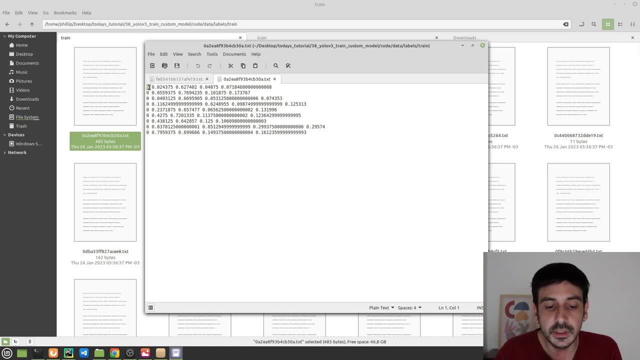 detecting alpacas. so in my case this number will always be zero. but if you're detecting more than one class, then you will have different numbers. then you're going to have in your database the number of objects that you have, which is the same structure, and in this case i'm only detecting one. 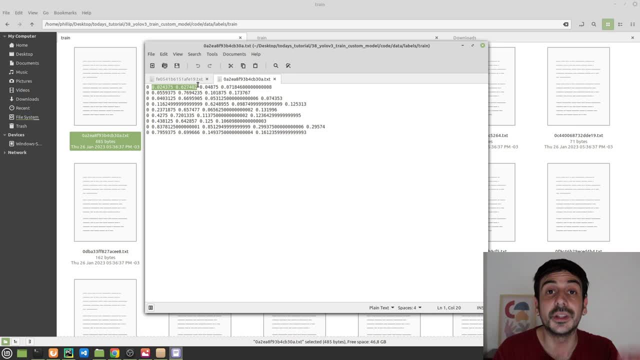 you have the position, the x and y position of the center of the bounding box, and then you will have the width, and then you will have the height, and everything will be expressed in relative coordinates. so, basically, this is the. this is a structure you need for your data and this is what this step is. 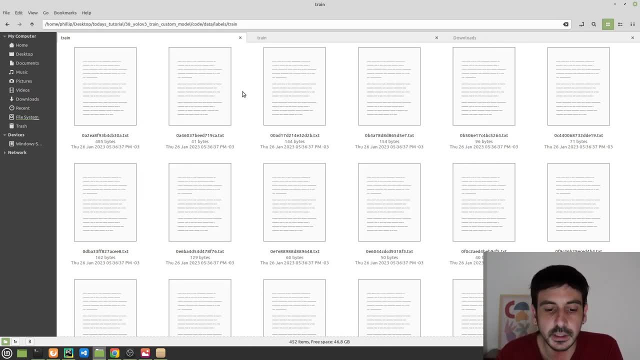 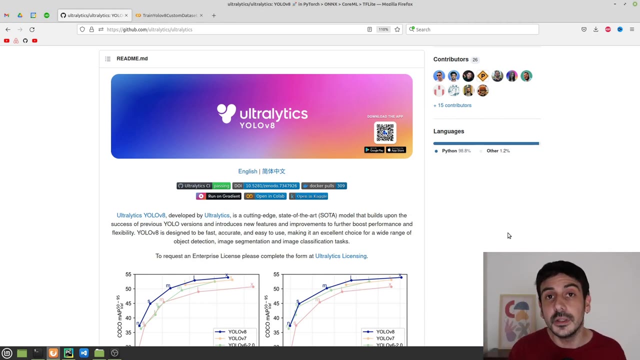 about. so that's pretty much all about converting data or about formatting the data, and now let's move on to the training. now is where we are going to take all this data and we are going to train our object detector using YOLOv8. so, now that we have taken the data into the format we need in 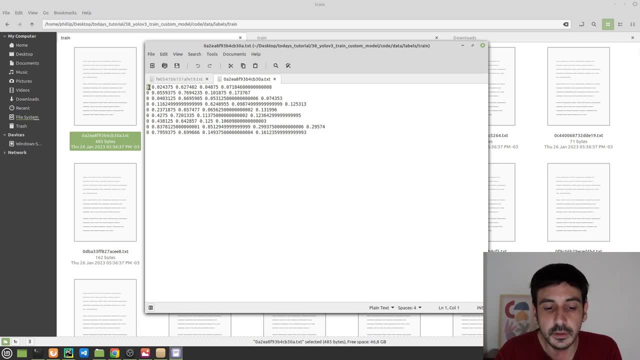 detecting alpacas. so in my case this number will always be zero. but if you're detecting more than one class, then you will have different numbers. then you have the positions, the x and y position of the center of the bounding box, and then you will have the width, and then you 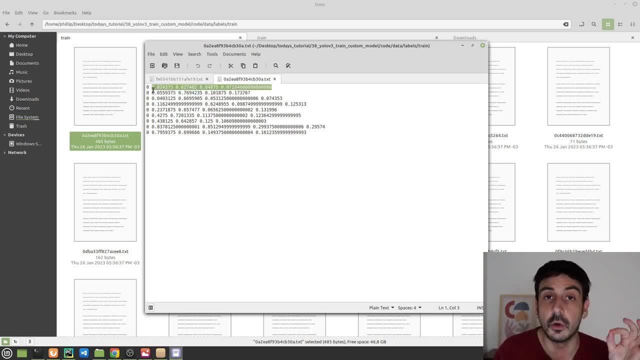 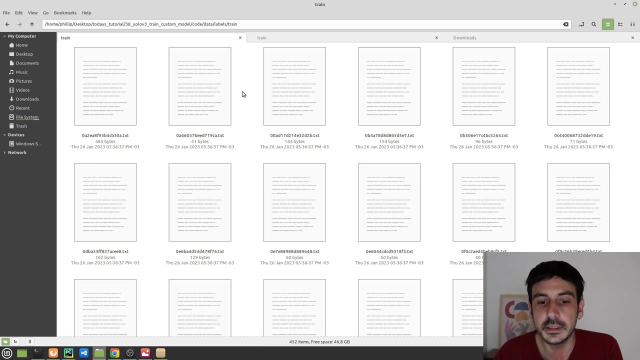 will have the height and everything will be expressed in relative coordinates. so, basically, this is the. this is a structure you need for your data, and this is what this step is about. so that's pretty much all about converting data, or about formatting the data, and now let's move on to the. 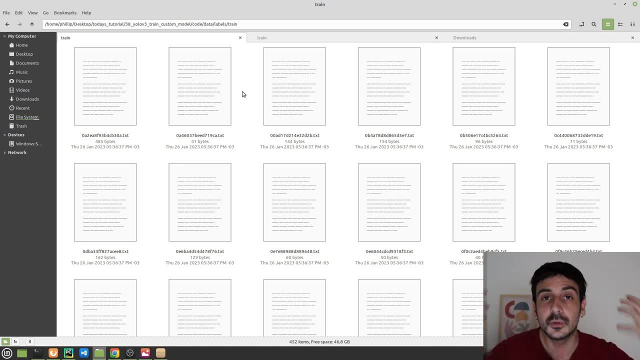 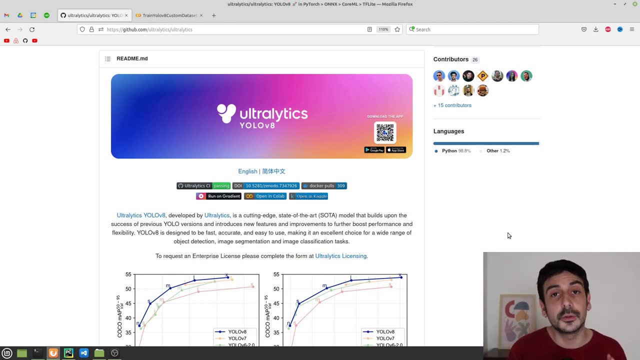 training now is where we are going to take all this data and we are going to train our object detector using YoloV8. so, now that we have taken the data into the format we need in order to train YoloV8, now comes the time for the training. now it comes the time where we are going to take this. 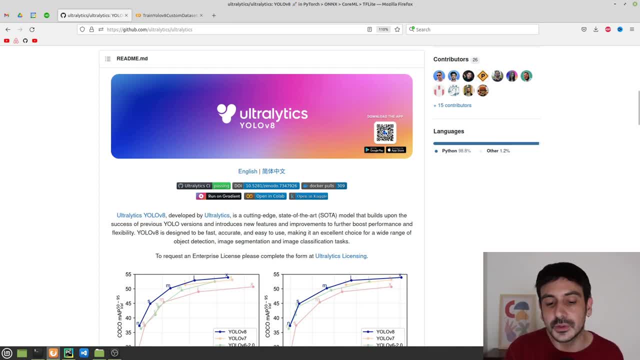 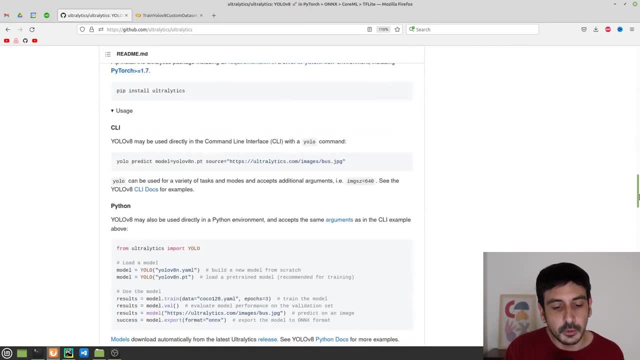 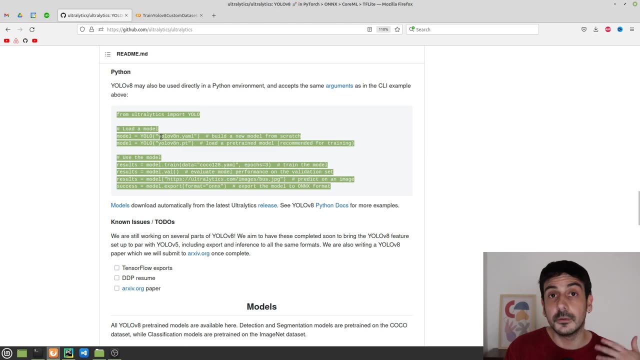 custom data set and we are going to train an object detector using YoloV8. so this is YoloV8 official repository, and the one of the things i like the most about YoloV8 is that in In order to train an object detector, we can do it either with Python, with a very few, only a few Python instructions. 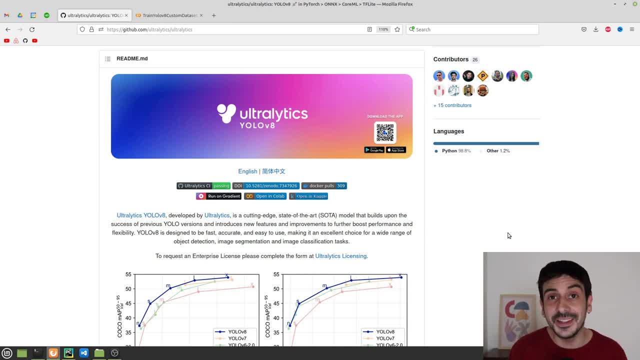 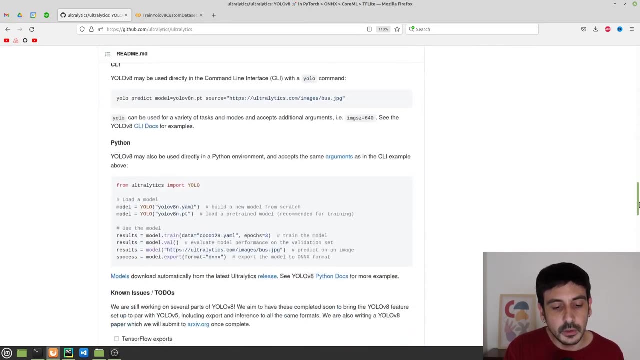 order to train YOLOv8. now comes the time for the training. now it comes the time where we are going to take this custom data set and we are going to train an object detector using YOLOv8. so this is YOLOv8 official repository, and the one of the things i like the most about YOLOv8 is that it. 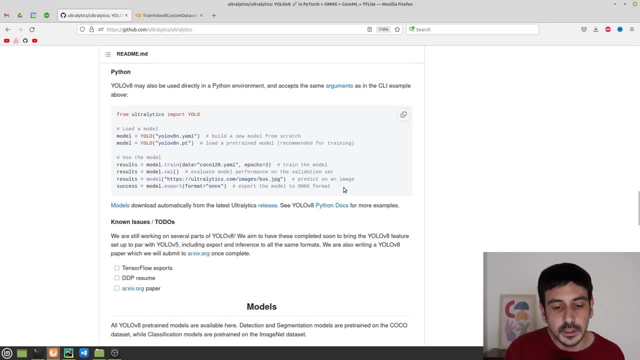 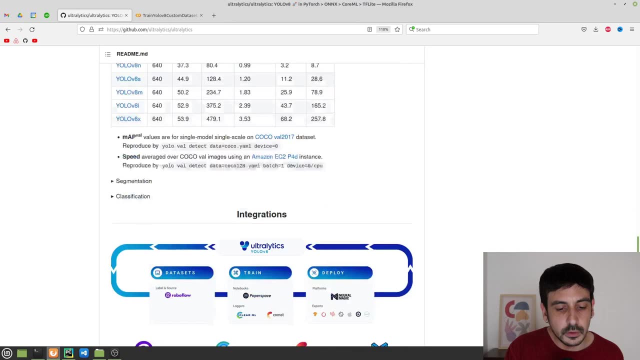 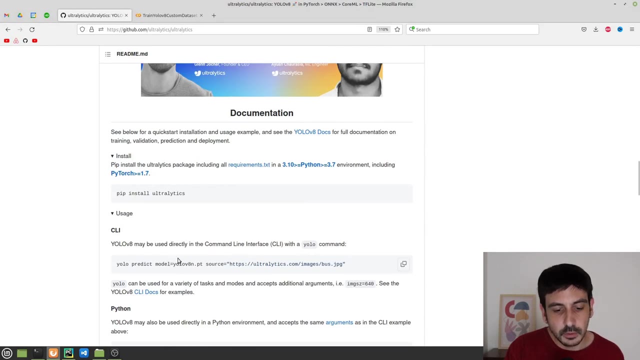 is that, in order to train an object detector, we can do it either with python with a very few, only a few python instructions, or we can also use a command line utility. let me see if i find it over here. we can also execute a command like this in our terminal, something that looks like this and: 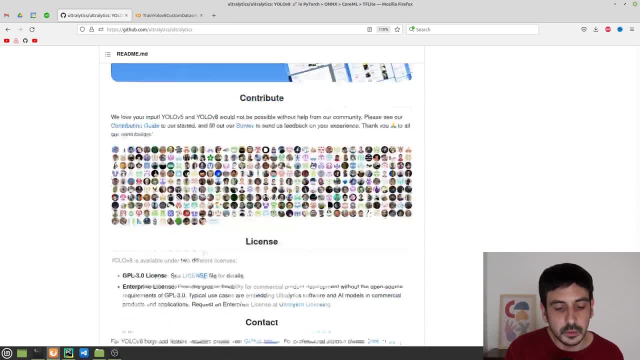 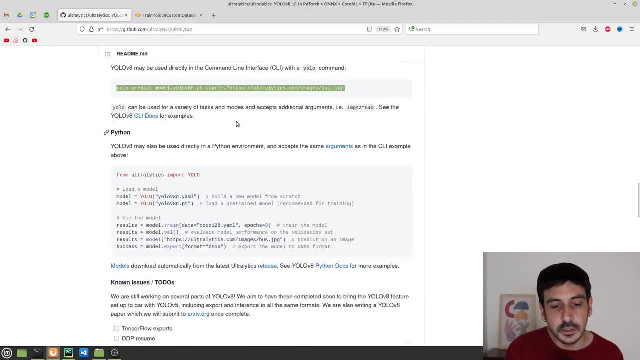 Or we can also use a command line utility. Let me see if I find it over here. We can also execute a command like this in our terminal, something that looks like this, And that's pretty much all we need to do in order to train this object detector. 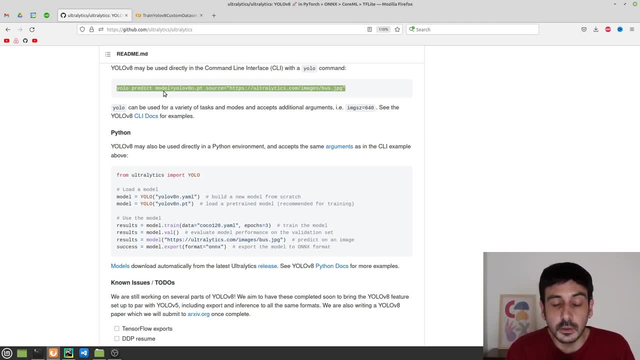 That's something I really, really liked. that's something I'm definitely going to use in our projects from now on, Because I think it's a very, very convenient and a very easy way to train an object detector or a machine learning model. So this is the first thing we should notice about YOLOv8. 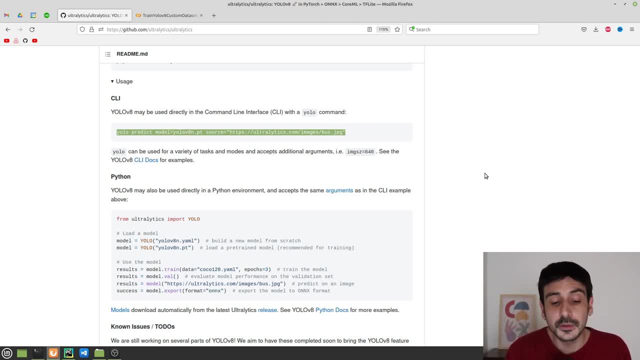 There are two different ways in which we can train an object detector. We can either do it in Python, as we usually do, or we can run a command in our terminal. I'm going to show you both ways, so you're familiar with both ways, And also I mentioned that I am going to show you the entire process on a local environment in a Python project. 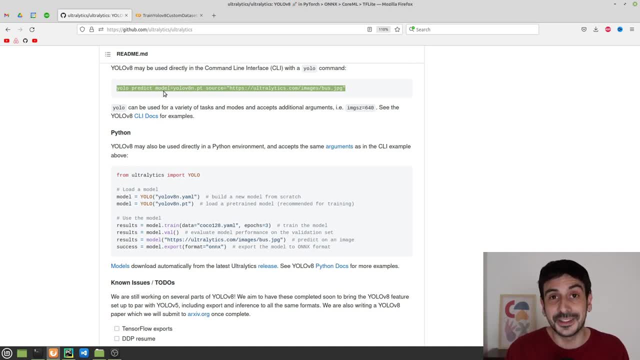 that's pretty much all we need to do in order to train this object detector. that's something i really really liked. that's something i really really liked and i'm going to show you how to. i'm definitely going to use in our projects from now on, because i think it's a very, very convenient. 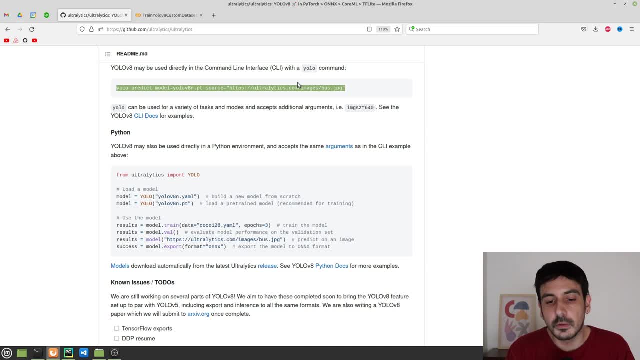 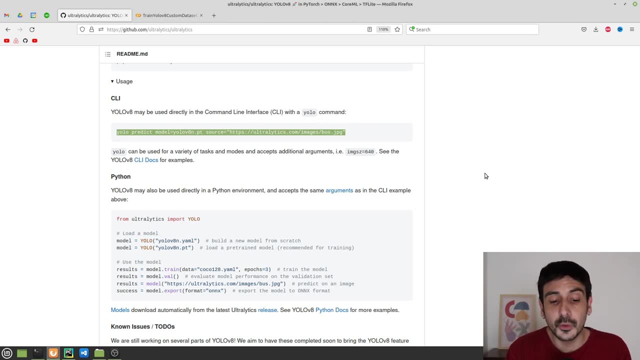 and a very easy way to train an object detector or a machine learning model. so this is the first thing we should notice about YOLOv8. there are two different ways in which we can train an object detector. we can either do it in python, as we usually do, or we can run a command in our terminal. 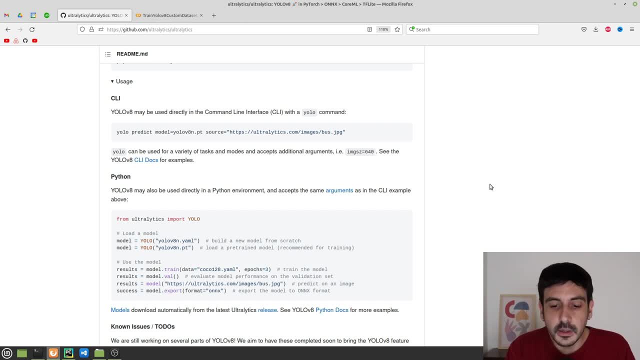 i'm going to show you both ways, so you're familiar with both ways. and also i mentioned that i am going to show you the entire process of training an object detector and i'm going to show you how to do the entire process on a local environment in a python project. and i'm also going to show you this: 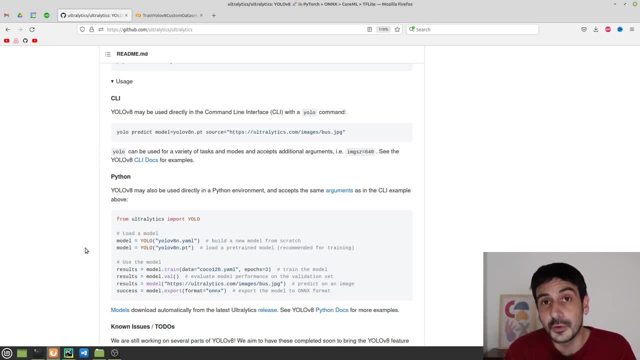 process in a google collab. so i know there are people who prefer to work in a local environment- i am one of those people- and i know that there are other people who prefer to work on a google collab. so, depending on which, in which group are you, i am going to show you both ways to do it so you can. 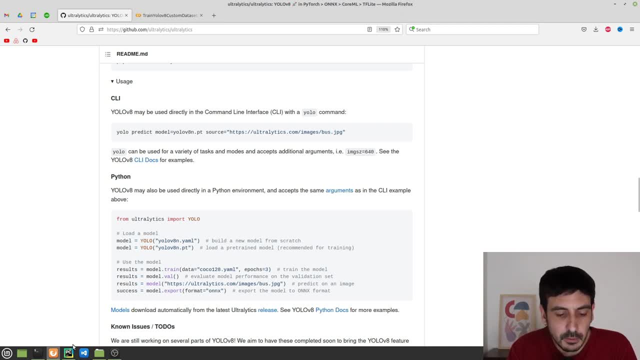 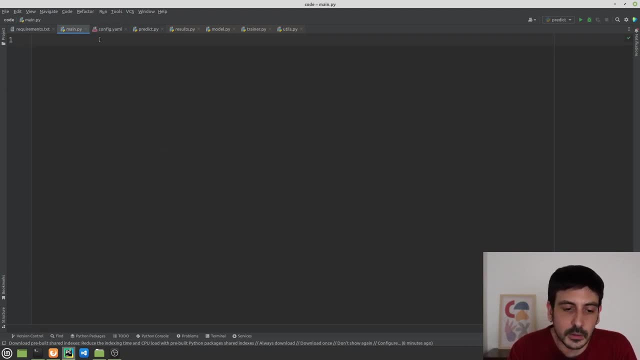 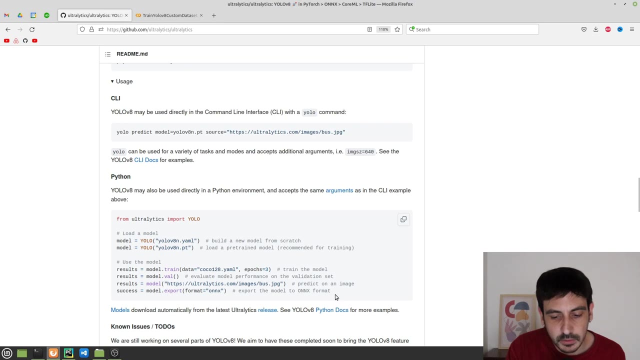 just choose the one you like the most. so let's start with it. and now let's go to pycharm. this is the project i created for this training, and this is the file we are going to edit in order to train this object detector. so the first thing i'm going to do is to just copy a few lines. i'm just 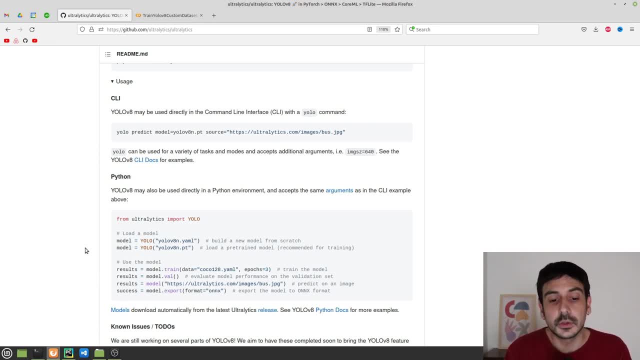 And I'm also going to show you this process in a Google Collab. So I know there are people who prefer to work in a local environment. I am one of those people and I know that there are other people who prefer to work on a Google Collab. 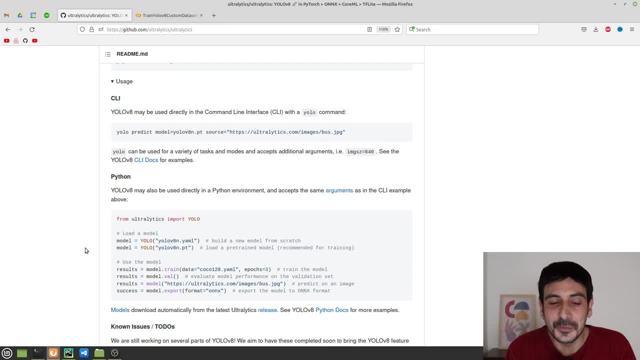 So, depending on which, in which group are you, I am going to show you both ways to do it, so you can just choose the one you like the most. So let's go. Let's start with it, and now let's go to PyCharm. This is a PyCharm project I created for this training. 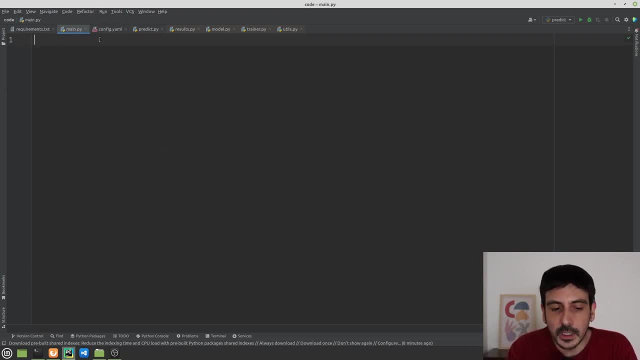 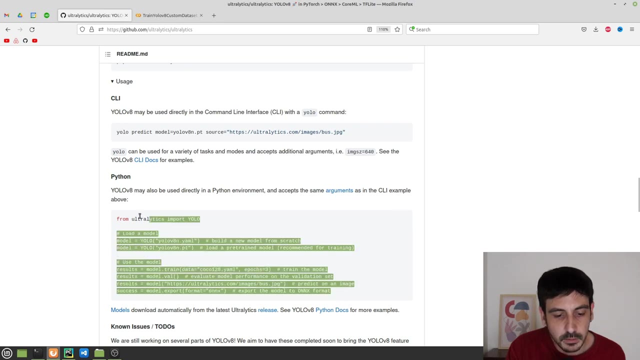 And this is the file we are going to edit in order to train this object detector. So the first thing I'm going to do is to just copy a few lines. I'm just going to copy everything and I'm going to remove everything we don't need. 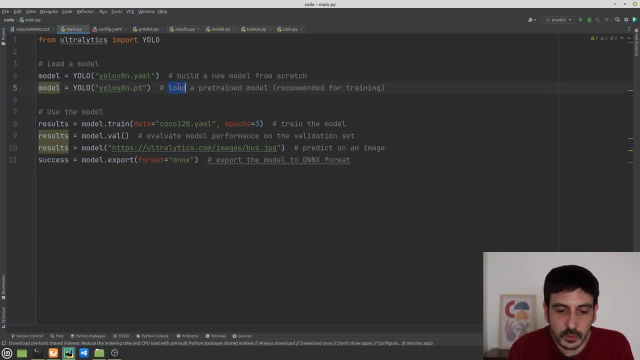 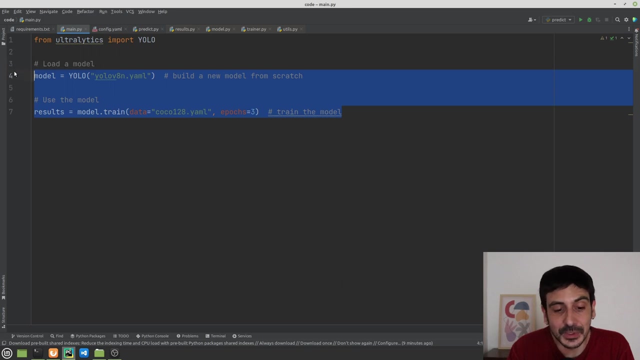 Copy and paste. So we want to build a new model from scratch, So we are going to keep this sentence And then we are going to train a model. So we are just going to Remove everything but the first sentence And that's all Right. These are the two lines we need in order to train an object detector using YOLOv8. 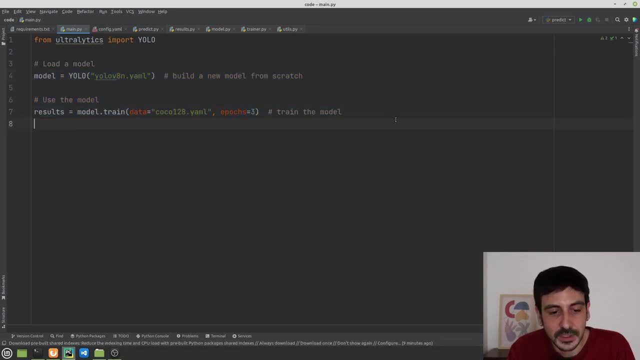 Now we are going to do some adjustments. Obviously, the first thing we need to do is to import Ultralytics, Which is a library we need to use in order to train a YOLOv8 model, And this is a Python library we need to install, as we usually do. 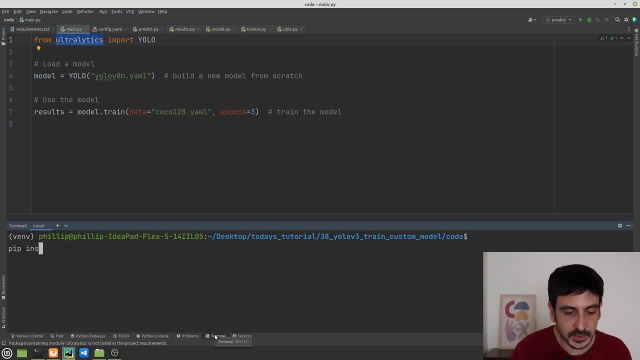 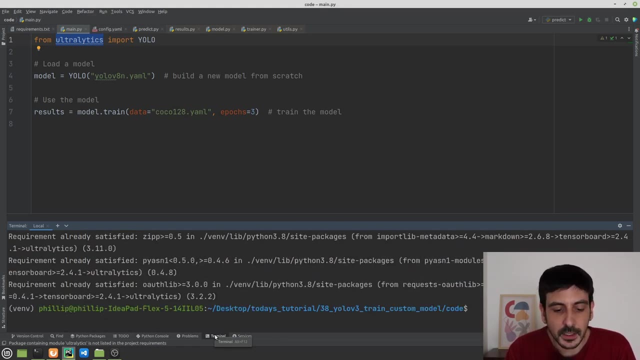 We go to our terminal And we do something like pp, install and the library name. In my case, nothing is going to happen because I have already installed this library. But please remember to install it And also please mind that when you are installing this library, This library has many, many, many dependencies. 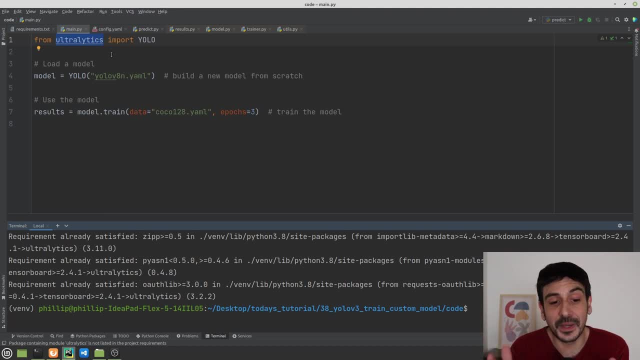 So you are going to install many, many, many, many different Python packages, So it's going to take a lot of space. So definitely, please be ready for that, Because you need a lot of available space in order to install this library And it's also going to take some time. 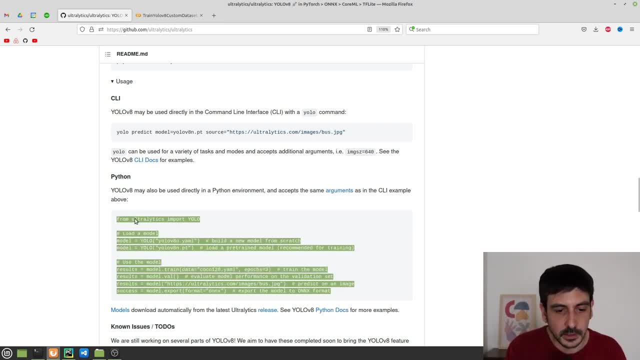 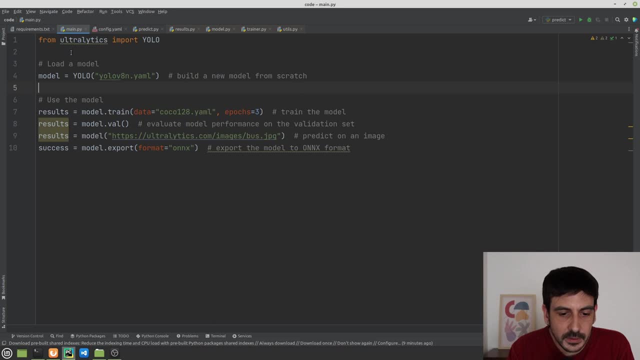 going to copy everything and i'm going to remove everything. we don't need copy and paste. so we want to build a new model from scratch, so we are going to keep the this sentence and then we are going to train a model. so we are just going to remove everything but the first sentence, and that's all. 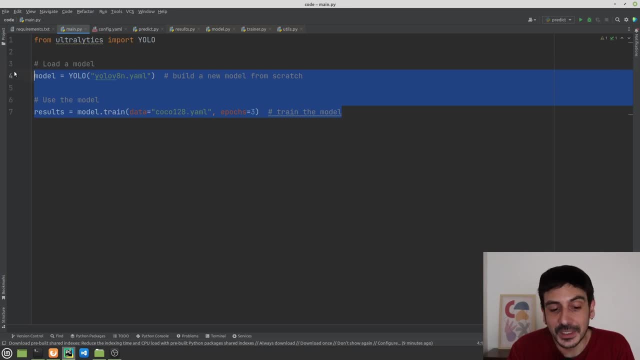 right, these are the two lines we need in order to train an option detector using yellow v8. now we are going to do some adjustments, the obviously the first thing we we need to do is to import ultralytics, which is a library we need to use in order to import yellow, in order to train a yellow. 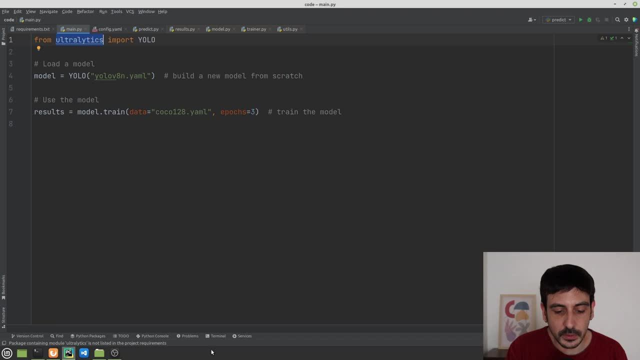 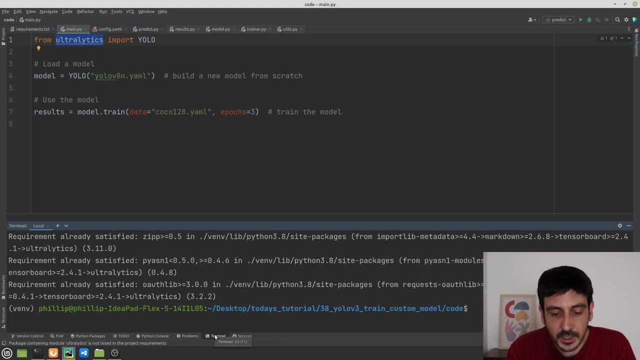 v8 model and this is a python library we need to install. as we usually do. we go to our terminal and we will call um into the game. in my case, nothing's going to happen because i have already installed this library. but please remember to install it and also please mind that when you are installing. 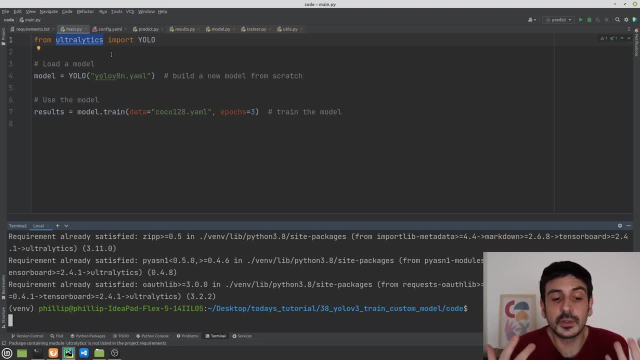 this library. this library has many, many, many dependencies, so you are going to install many, many, many, many different python packages, so it's going to take a lot of space. so definitely, please be ready for that, because you need a lot of available space in order to install this library. 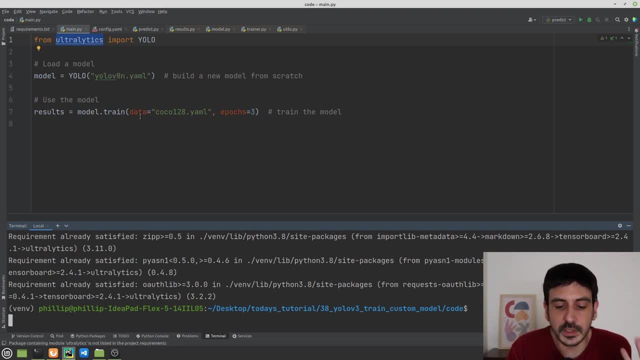 and it's also going to take some time because you are in one of the relatively small functions of the network, so you can do it and it's not gonna take a lot of time in terms of coding just to understand how to do it, because, as you're gonna do it so that the program doesn't need to have many devices, 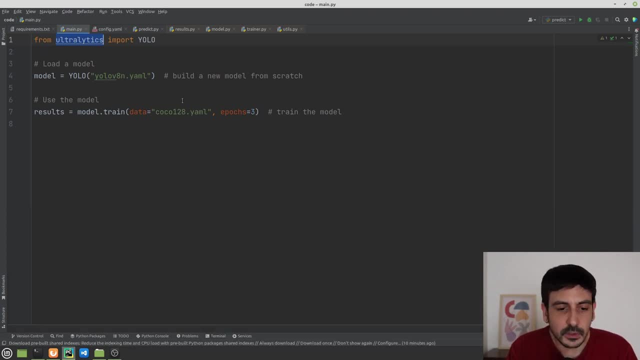 the program has many, so that's how i'm going to see what we are going to do in order to do this, and one way: installing many, many, many different packages. but anyway, let's continue. please remember to install this library. and these are the two sentences we need in order to run this training from a python. 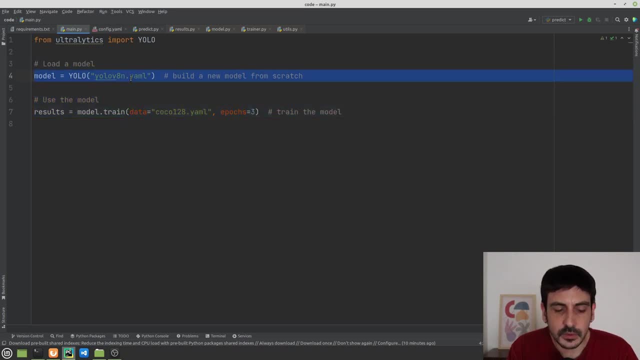 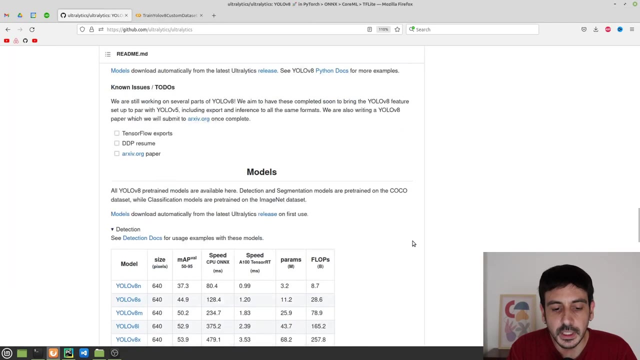 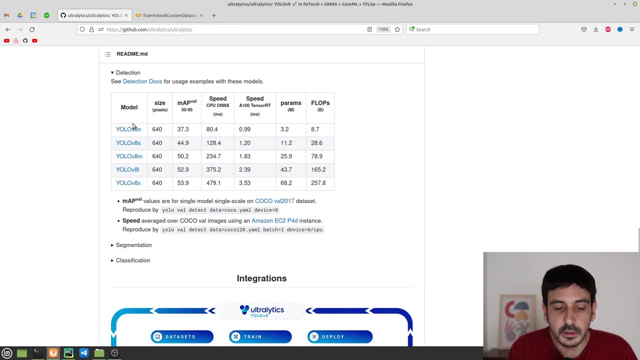 from a python script, so this sentence, we're just going to leave it as it is. this is where we are loading the specific yolo v8 architecture. the specific yellow v8 are a model we are going to use. you can see that we can choose from any of all of these different models. these are different. 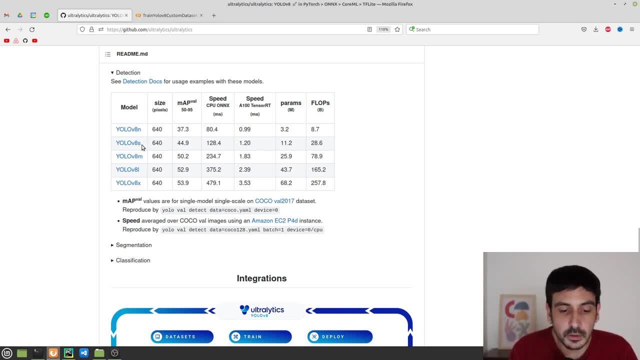 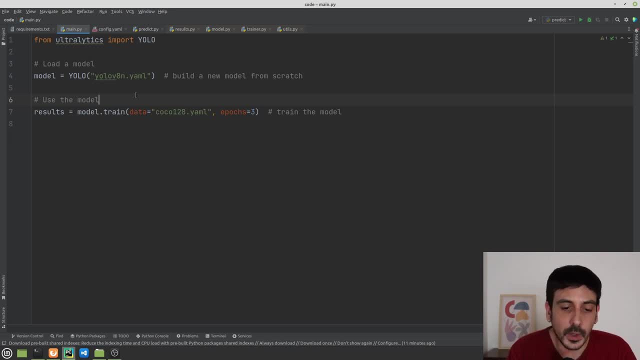 versions or these are different sizes for yellow v8. you can see we have nano, small, medium, large or extra large. we are using the nano version, which is the smallest one or is the lightest one, and this one we are going to use the yellow v8 nano, the yellow v8 n. then about the training, about 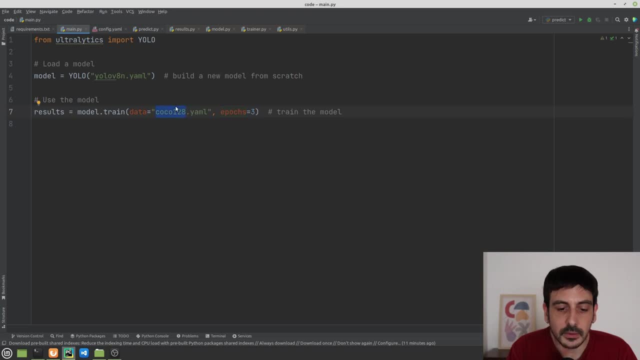 this whole sentence. we need to edit this file right. we need a yaml file which is going to contain all the configuration for our training. so i have created this file and i have now this file: configyaml. i'm not sure if this is the most appropriate name, but anyway, this is the name. 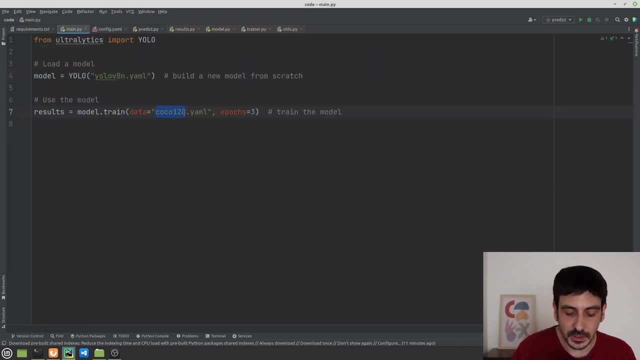 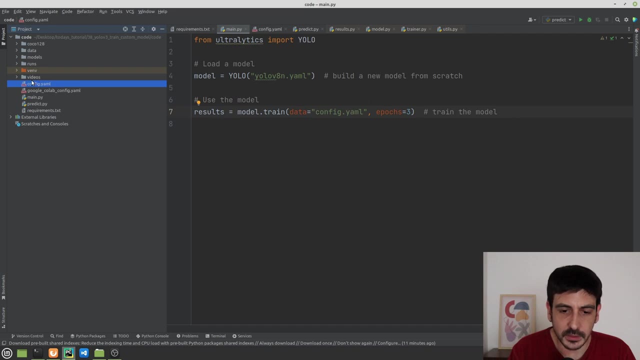 i have chosen for this file. so what i'm going to do is just edit this parameter and i'm going to input configyaml. this is where the config jam is located. this is where the mainpi is located. they are in the same directory. so if i do this, it's going to work just fine. and then let me show. 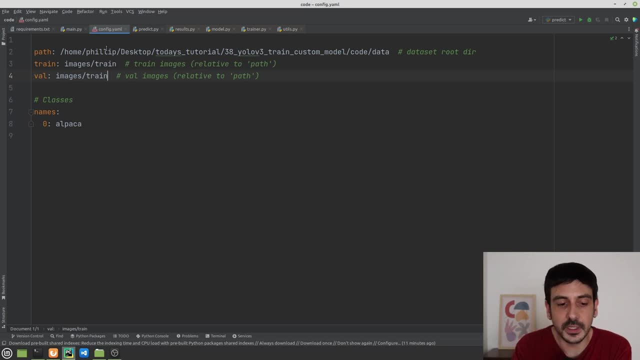 you the configuration file. so i have a very simple configuration file. we only have a few keys, which are path, train, ball and then names. right, let's start with the names. let's start with this. this is where you are going to set all your different classes, right, you are training an. 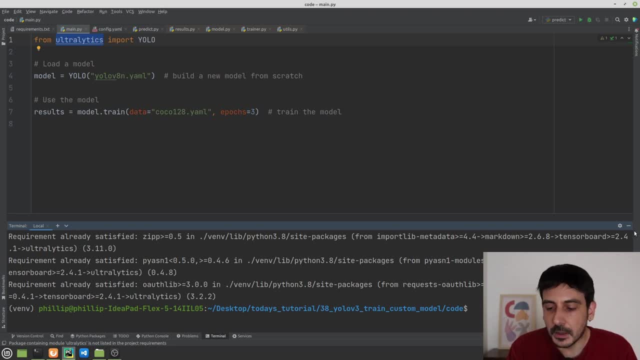 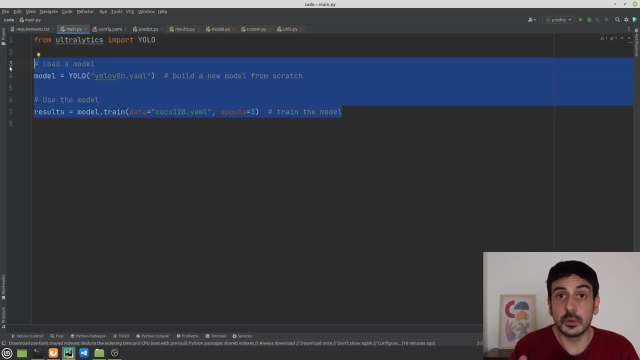 Because you are installing many, many, many different packages. But anyway, let's continue. Please remember to install this library. And these are the two sentences we need in order to run this training from a Python script. So this sentence, we are just going to leave it as it is. 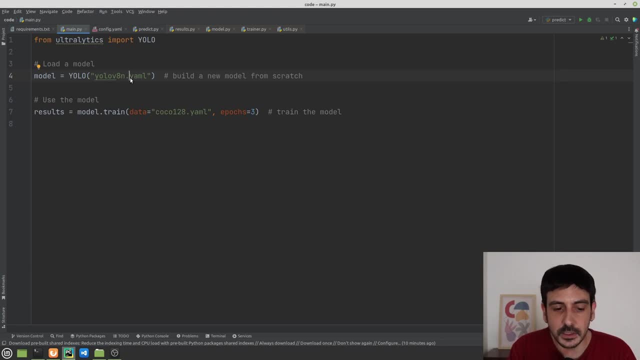 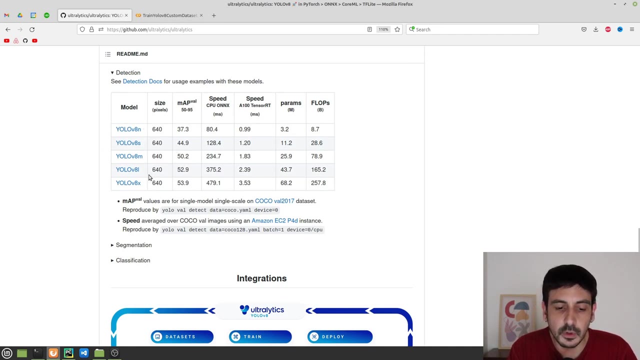 This is where we are loading the specific YOLOv8 architecture, The specific YOLOv8 model, The YOLOv8 model we are going to use. You can see that we can choose from any of all of these different models. These are different versions or these are different sizes for YOLOv8. 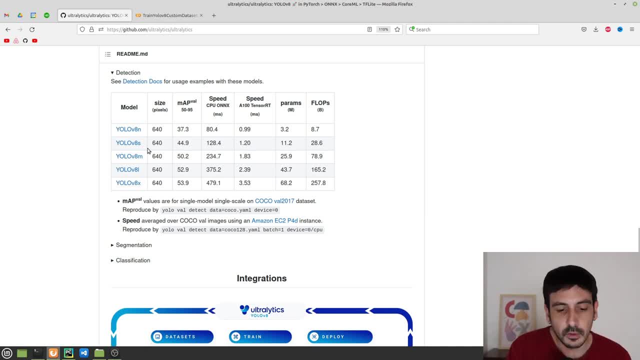 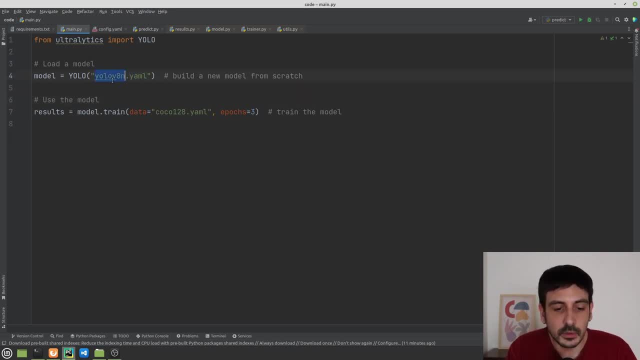 You can see, we have nano, small, medium, large or extra large. We are using the nano version which is the smallest one or is the lightest one, And this one we are going to use, the YOLOv8 nano, the YOLOv8n. 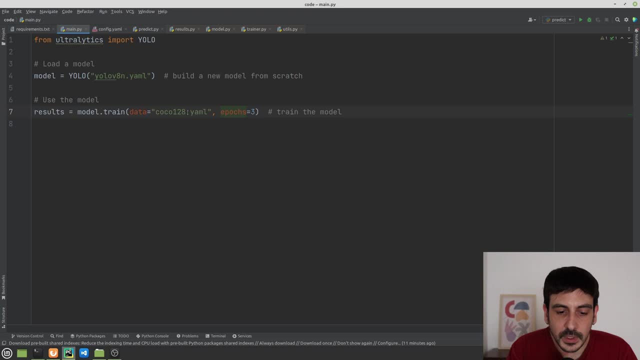 Then about the training, about this whole sentence. We need to edit this file right. We need a YAML file which is going to contain all the configuration for our training. So I have created this file and I have named this file configyaml. I'm not sure if this is the most appropriate name. 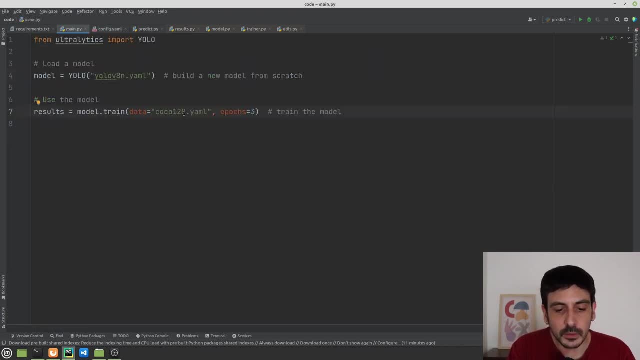 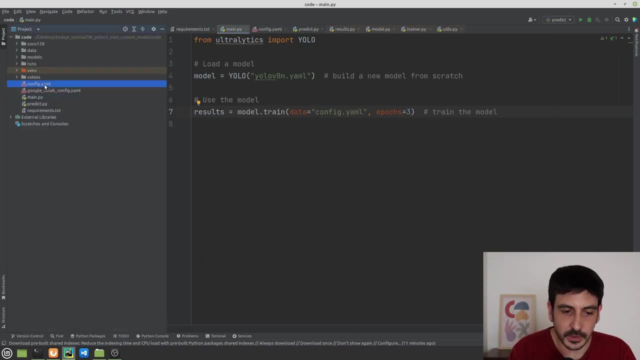 But anyway, this is the name I have chosen for this file. So what I'm going to do is just edit this parameter And I'm going to input configyaml. This is where the configyaml is located. This is where the mainpi is located. They are in the same directory. 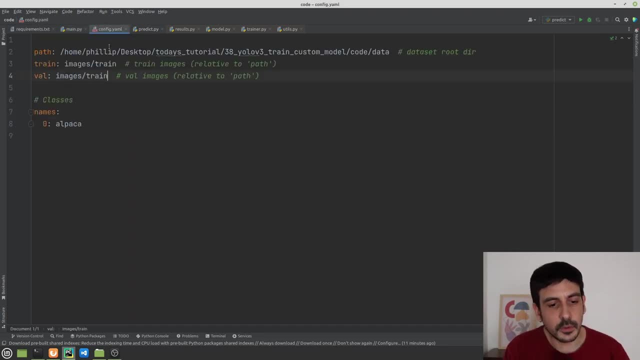 So if I do this, it's going to work just fine. And then let me show you the structure for this configyaml. You can see that this is a very, very, very simple configuration file. We only have a few keys, which are path, train, val and then names, right? 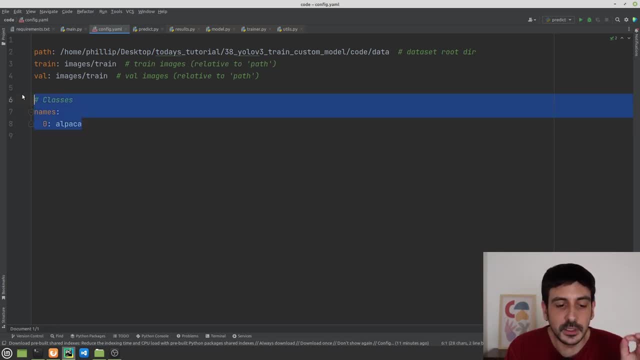 Let's start with the names. let's start with this: This is where you are going to set all your different classes right. You are training an object detector. You are detecting many different categories, Many different classes, And this is where you are going to input. 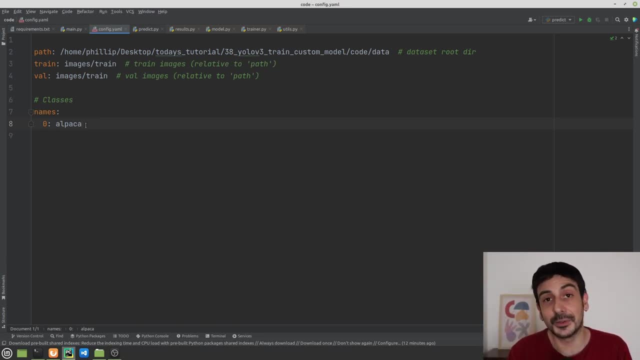 This is where you are going to type all of those different classes. In my case, I'm just detecting alpacas. That's the only class I am detecting, So I only have one class. It's the number 0 and it's called alpaca. But if you are detecting additional objects, 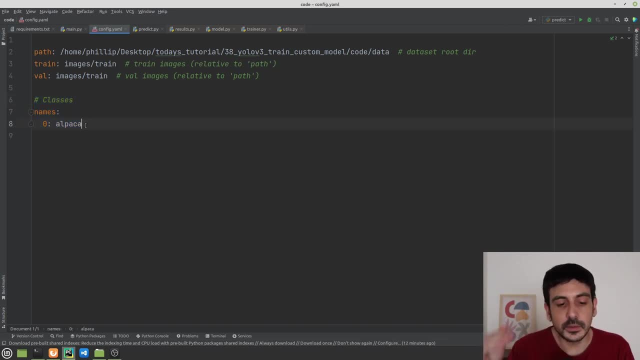 object detector. you are detecting many different categories, many different classes, and this is where you are going to input is where you're going to type all of those different classes. in my case, i am detecting alpacas. that's the only class i am detecting, so i only have one class is the number. 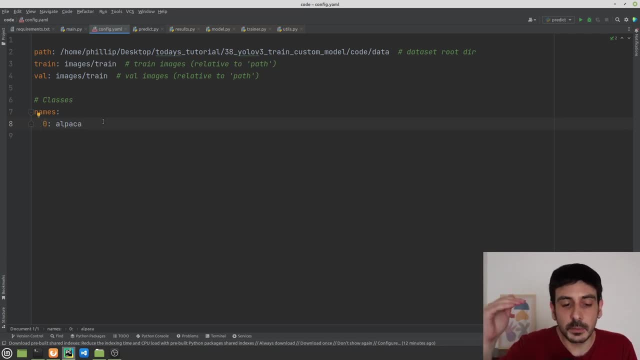 zero and it's called alpaca. but if you're detecting additional objects, please remember to include all the list of all the objects you are detecting. then, about these three parameters, these three arguments, the path is the absolute path to your directory containing images and annotations, and please remember to include the absolute path. 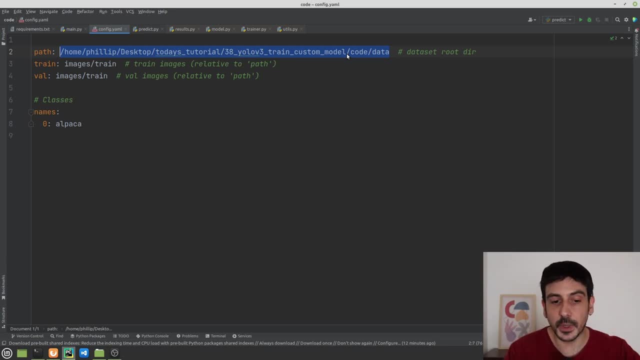 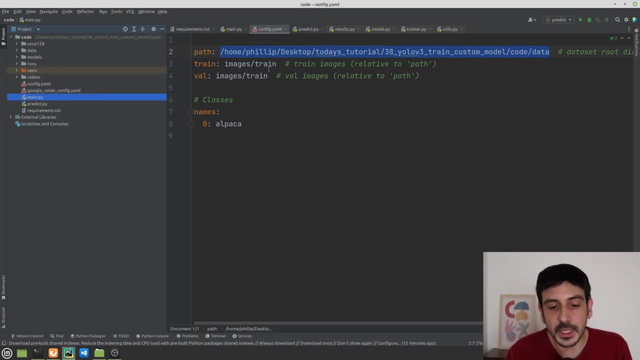 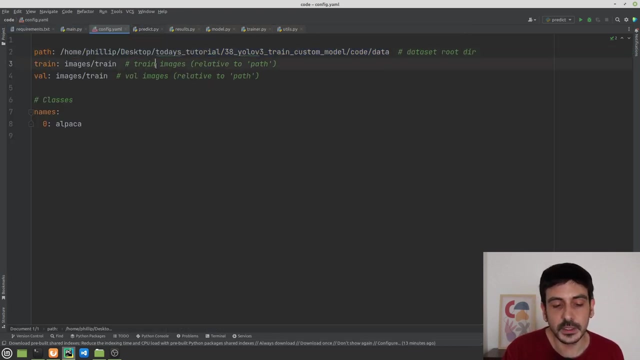 ran some issues when i was trying to specify a relative path, relative from this directory, from my current directory where this project is created, to the directory where my data is located. when i was using a relative path, i had some issues and then i i noticed that there were other people. 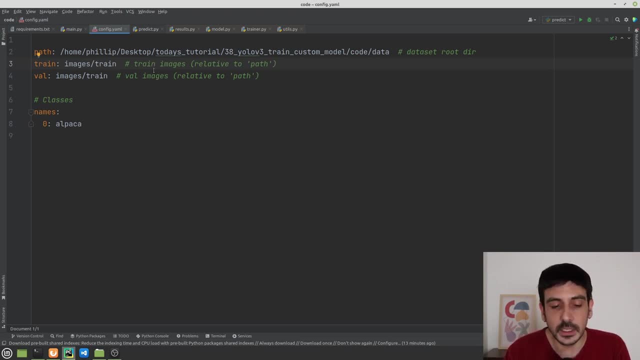 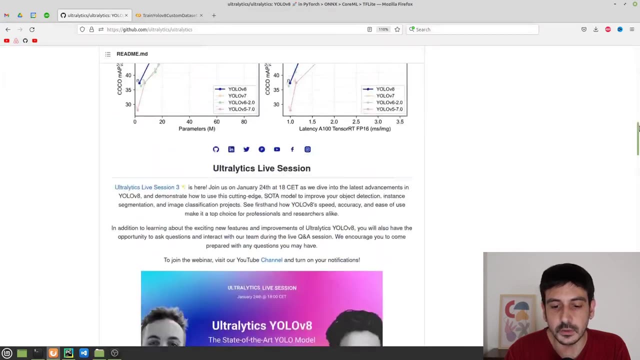 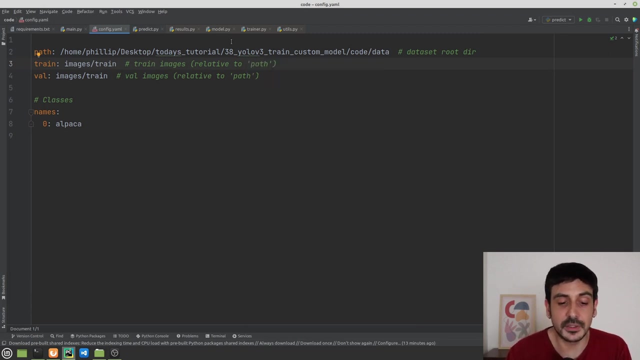 having issues as well. i noticed that in the github repository from yolo v8. i noticed this in the in the issues section. there were other people having issues when they were specifying a relative path. so the way i fix it and it's a very good way to fix it. it's a very easy way to fix it, it's just. 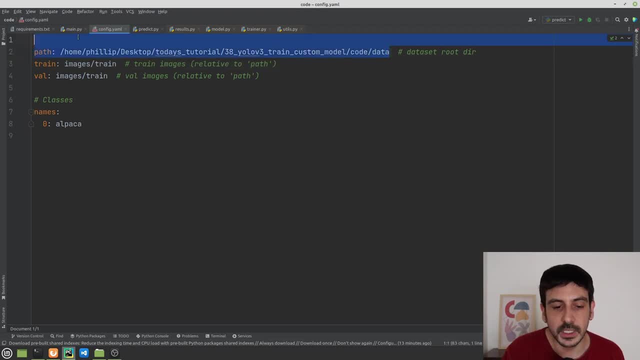 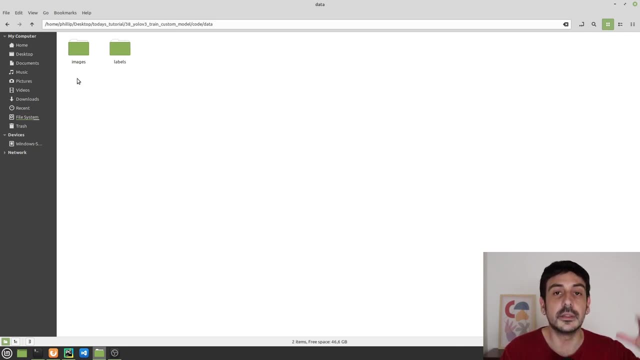 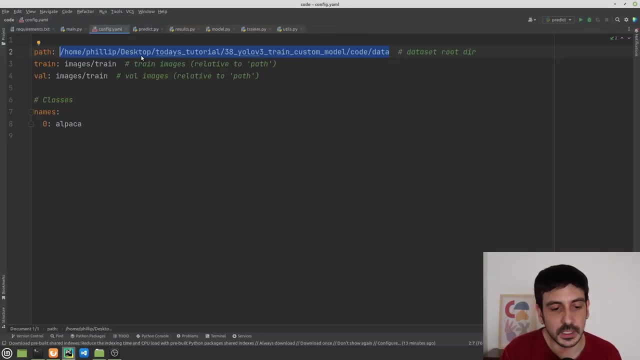 specifying an absolute path. remember, this should be an absolute path. so this is the path to this directory, to the directory containing the images and the labels directories. so this is this is the path you need to specify here, and then you have to specify the territories path from this location to where your images are located, like the specific. 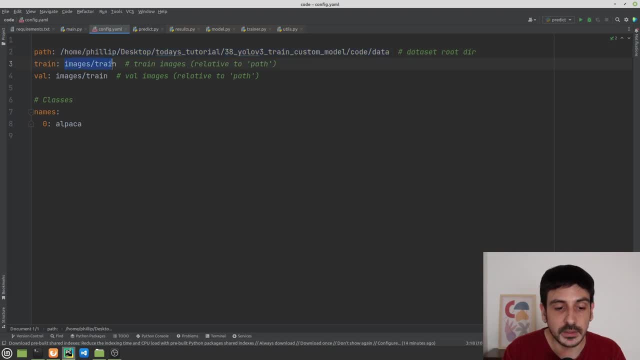 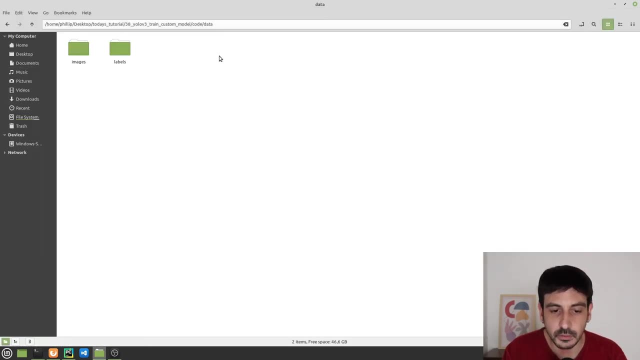 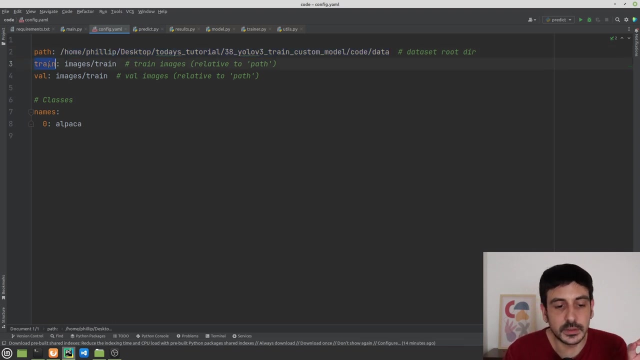 images are located right. in my case they are in images dot slash train relative to this path. if I show you this location, which is my root directory, then if I go to images train, this is where my images are located, right. so that's exactly what I need to specify and and then you can see that this is the train data. this is. 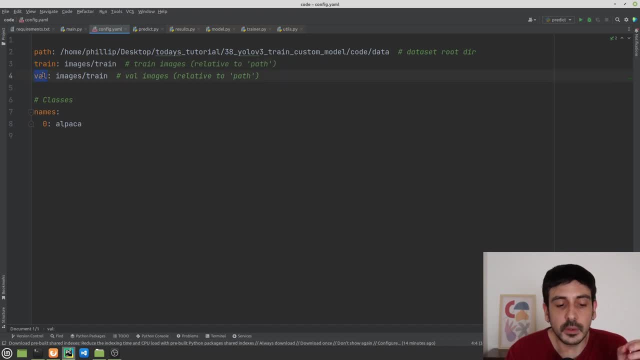 the data the algorithm is going to use as training data, and then we have another keyword, which is Val right, the validation that I said. in this case, we are going to specify the same data as we use for training, and the reason I'm doing this is because we want to keep things simple in this tutorial. I'm just 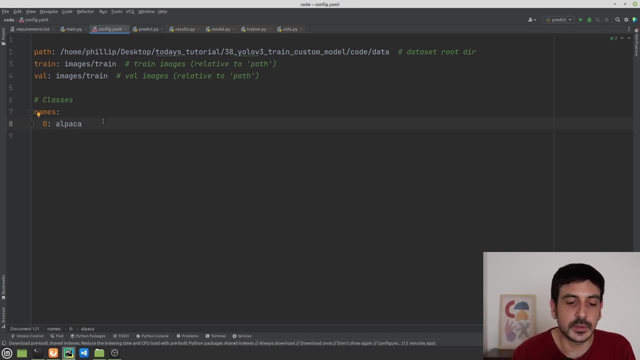 Please remember to include all the list of all the objects you are detecting. Then, about these three parameters, These three arguments, The path is the absolute path to your directory containing images and annotations. And please remember to include the absolute path. I ran some issues when I was trying to specify a relative path. 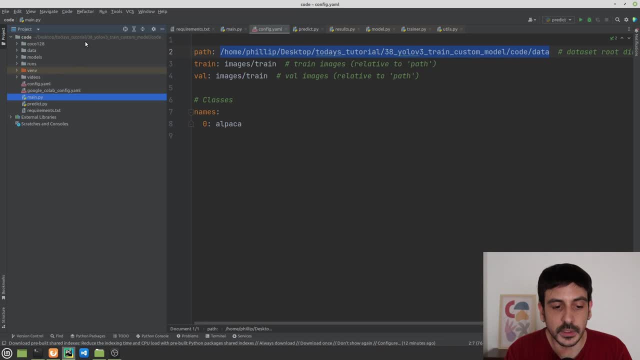 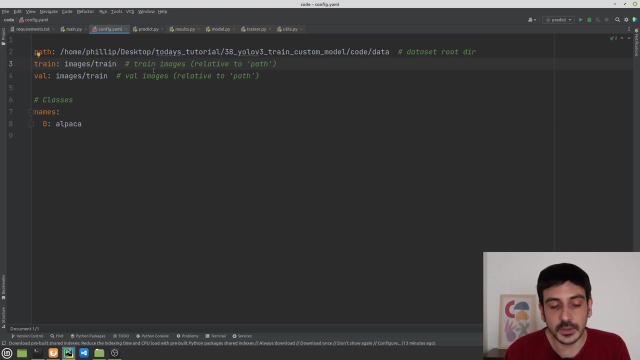 Relative from this directory, From my current directory where this project is created, To the directory where my data is located. When I was using a relative path, I had some issues And then I noticed that there were other people Having issues as well. I noticed that in the GitHub repository from YOLOv8. 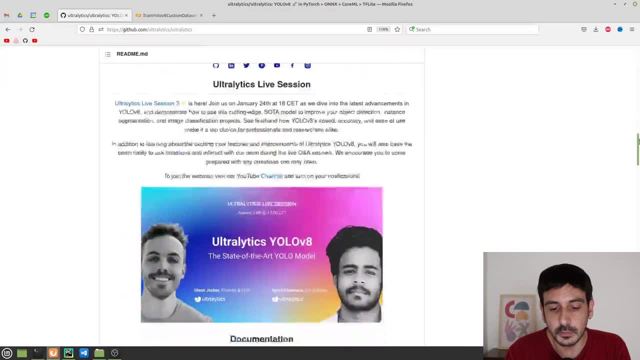 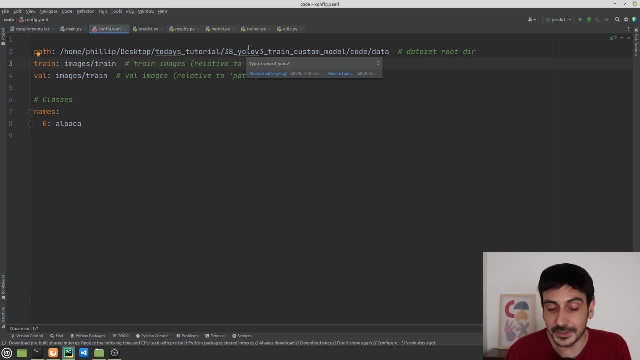 I noticed this in the issues section. There were other people having issues When they were specifying a relative path. So the way I fix it- And it's a very good way to fix it- It's a very easy way to fix it- It's just specifying an absolute path. 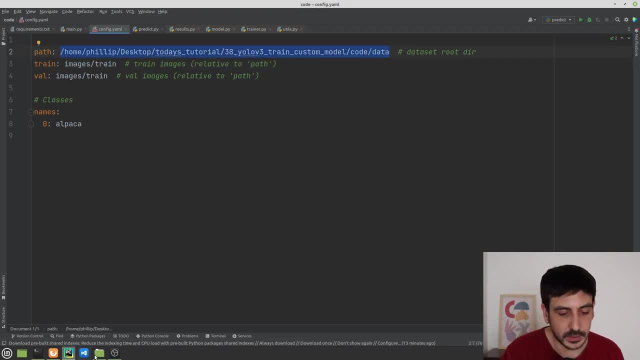 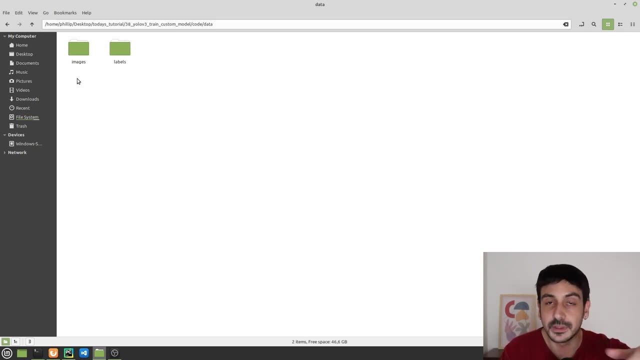 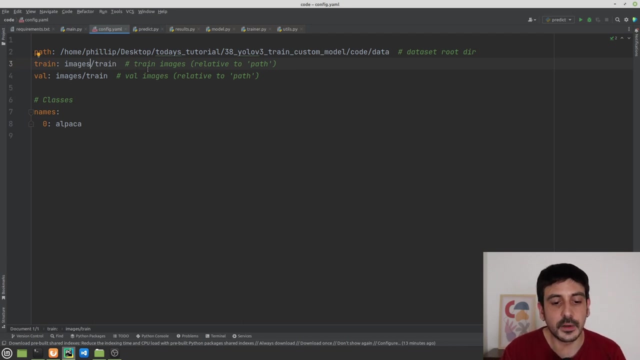 Remember, this should be an absolute path. So this is the path to this directory, To the directory containing the images And the labels directories. So this is the path you need to specify here, And then you have to specify the relative path From this location To where your images are located. 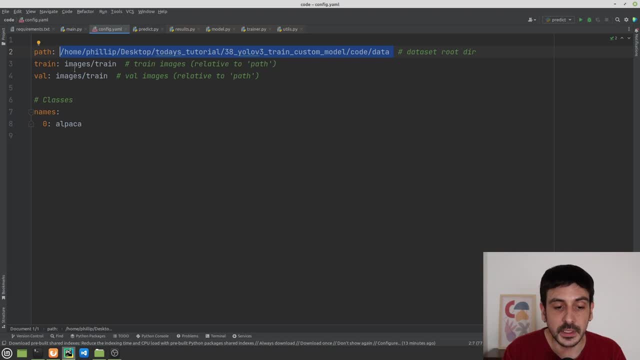 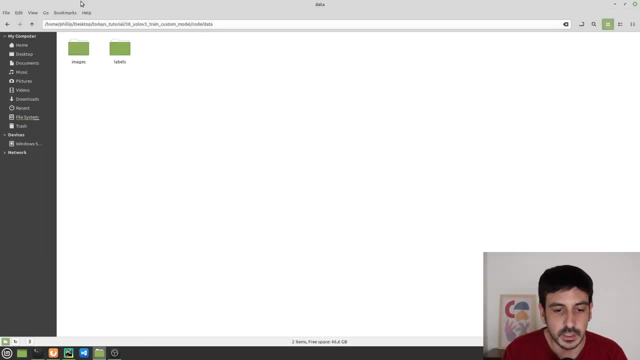 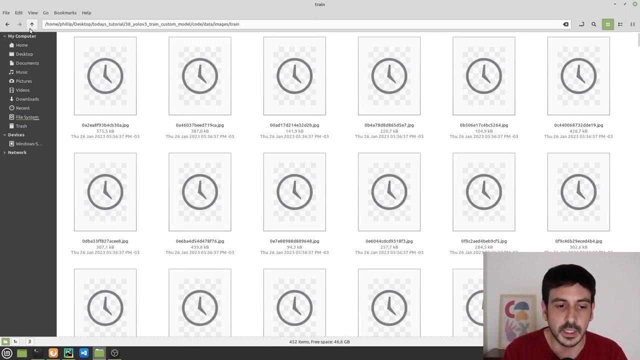 Like, the specific images are located right. In my case, they are in imagesslash train Relative to this path. If I show you this location, Which is my root directory, Then if I go to images train, This is where my images are located, right? 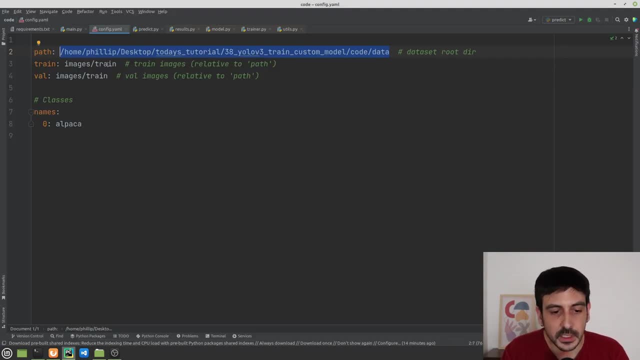 So that's exactly what I need to specify, And then you can see that This is the train data, This is the data the algorithm is going to use As training data. And then we have another keyword, which is Val right, The validation that I set In this case, we are going to specify: 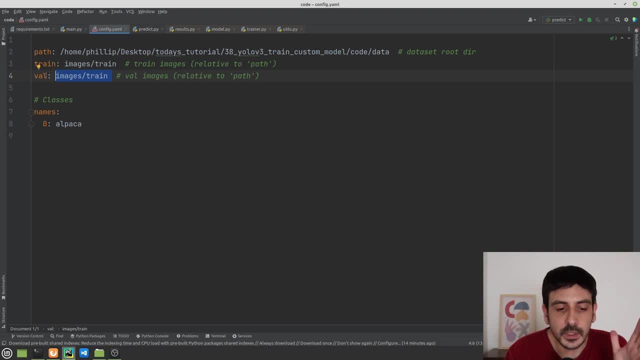 The same data as we used for training, And the reason I'm doing this is because We want to keep things simple. In this tutorial, I'm just going to show you the entire process Of how to train an object detector Using YOLOv8 on a custom dataset. 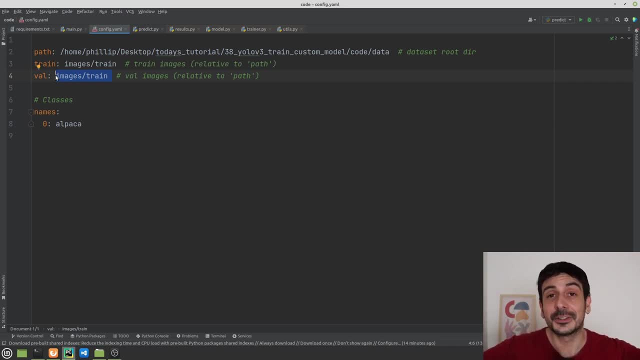 going to show you the entire process of how to train an object detector using YoloVision V8 on a custom data set. I want to keep things simple, so I'm just going to use the same data. so that's pretty much all for this configuration file. now going. 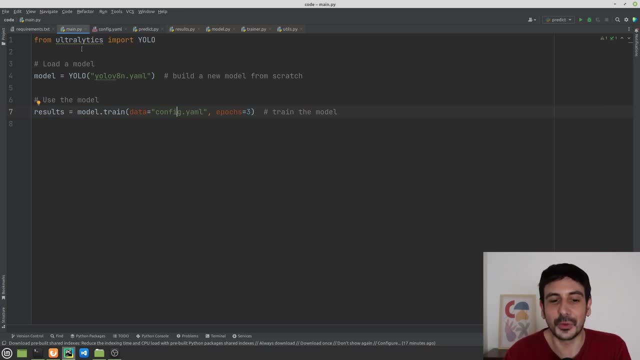 back to main. that's pretty much all we need in order to train an object detector using YoloVision V8 from python. that's how simple it is. so now I'm going to execute this file, I'm going to change the number of epochs. I'm going to do 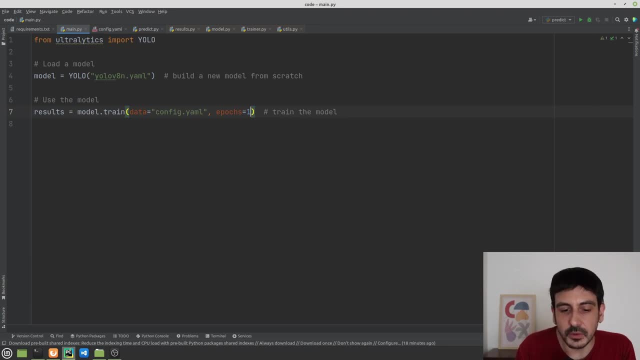 this for only one epoch, because the only thing I'm going to show you for now is how this runs. I'm going to show you the entire process and once we notice how everything is working, once we notice everything is up and running, everything is working fine. we can just continue, but let's just do this process, let's just do. 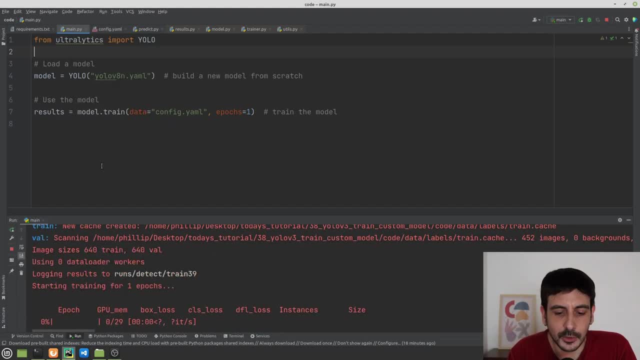 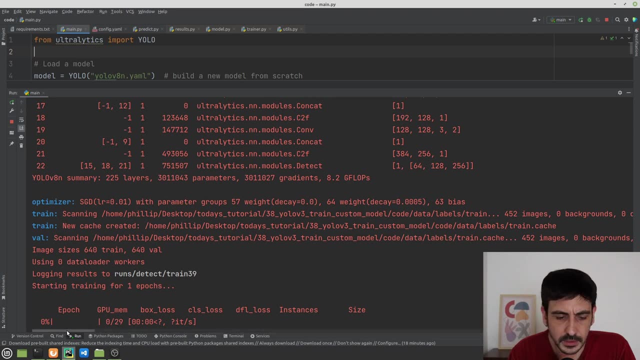 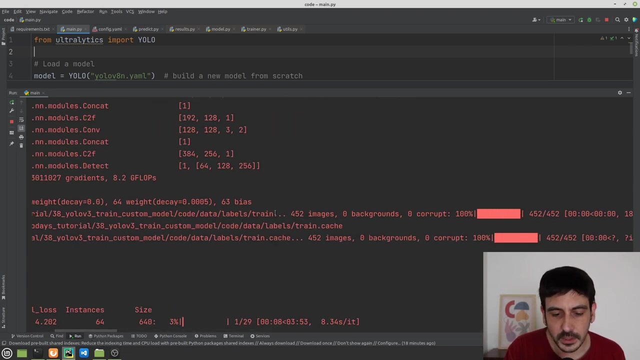 this training for only one epoch, so we can continue. you can see that now it's loading the data. it has already loaded data. you can make use of all the different information, of all these different debugging information we can see here. you can see, now we were loading 452 images and we were able to. 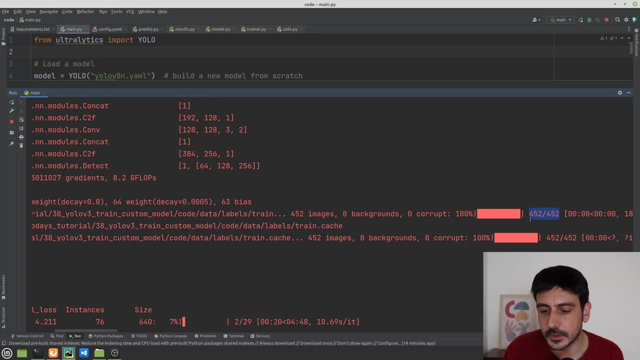 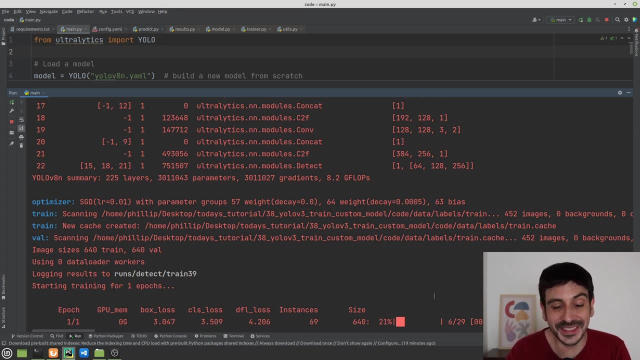 load all the images right- 452 from 452- and if I scroll down, you can see that we have additional information, additional values which are related to the training process. this is how the training process is going right: we are training this object detector and this additional information which we are given through. 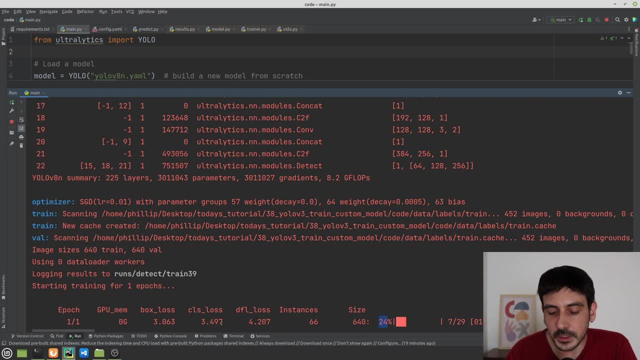 this process have to do is only waiting. we have to wait until this process is completed. so I am going to stop this video now and I'm going to fast forward this video until the end of this training and let's see what happens. okay, so the training is. 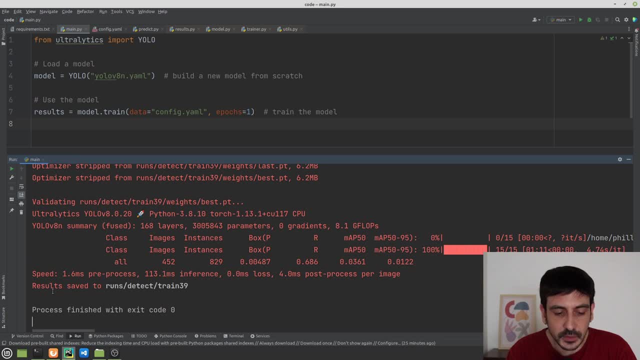 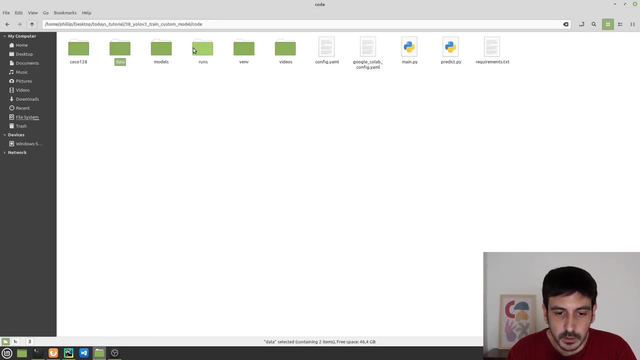 now completed and you can see that we have an output which says results saved to runs detect, train 39. so if I go to that directory- runs detect and train 39- you can see that we have many, many different files and these are files which are related to how the training process was done, right, for example, if I 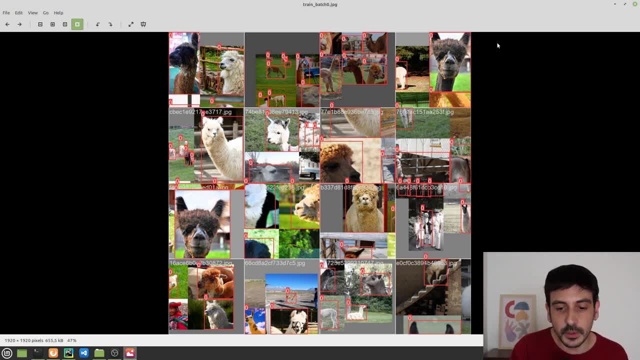 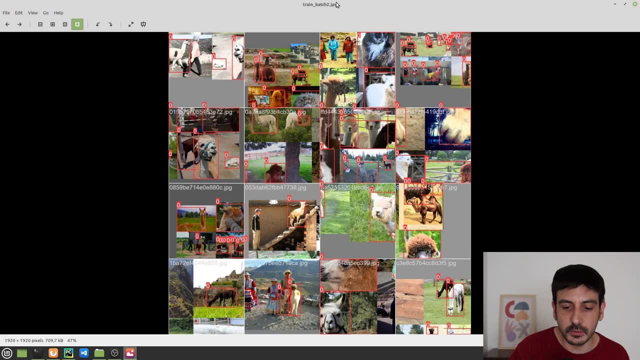 show you these images. these are a few batches of images which were used in order to train this algorithm. you can see a name is train batch 0 and train batch 1, anything we have a train batch 2, so we have a lot of different images of 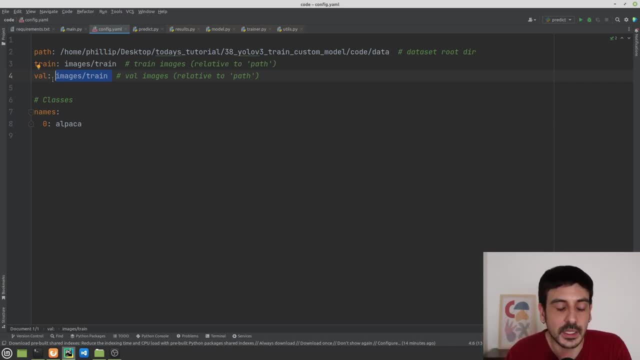 I want to keep things simple, So I'm just going to use the same data. So that's pretty much all for this configuration file. Now, going back to main, That's pretty much all we need in order to train An object detector using YOLOv8. 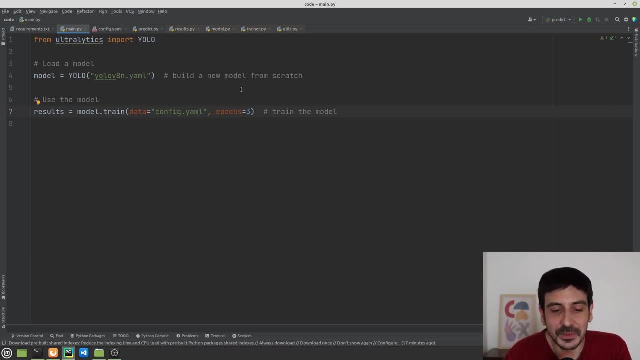 From Python. That's how simple it is. So now I'm going to execute this file. I'm going to change the number of epochs. I'm going to do this for only one epoch, Because the only thing I'm going to show you for now Is how this runs. 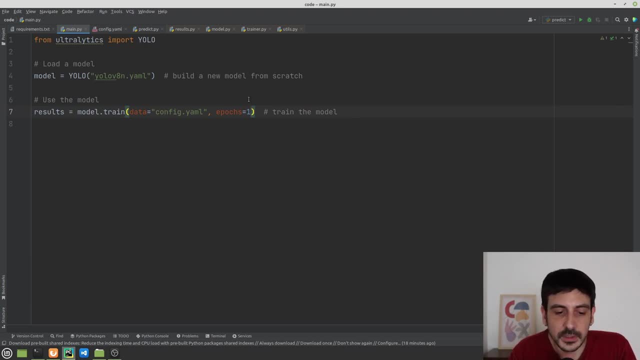 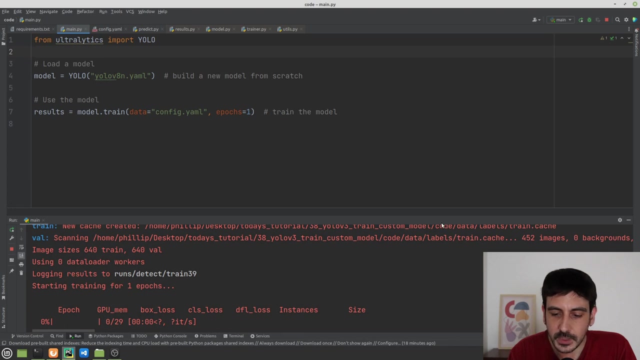 I'm going to show you the entire process, And once we notice how everything is working, Once we notice everything is up and running, Everything is working fine, We can just continue. But let's just do this process, Let's just do this training for only one epoch, So we can continue. 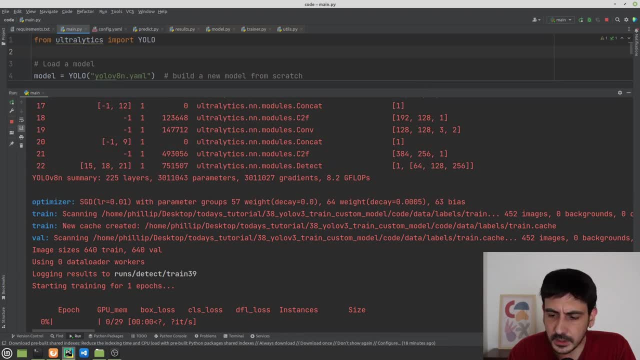 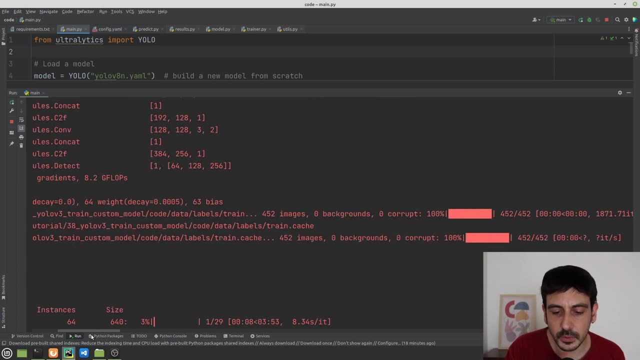 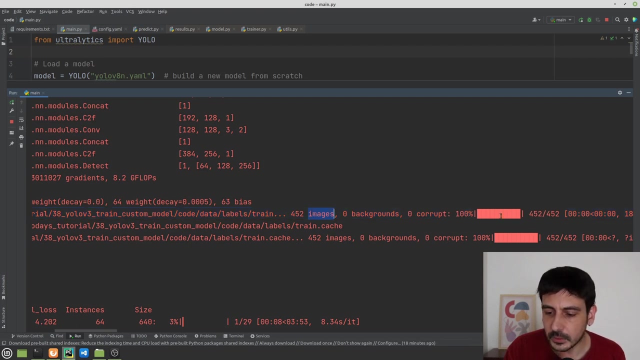 You can see that now it's Loading the data. It has already loaded the data. You can make use of all the different information, Of all this different debugging information We can see here. You can see now we were loading 452 images And we were able to load all the images. 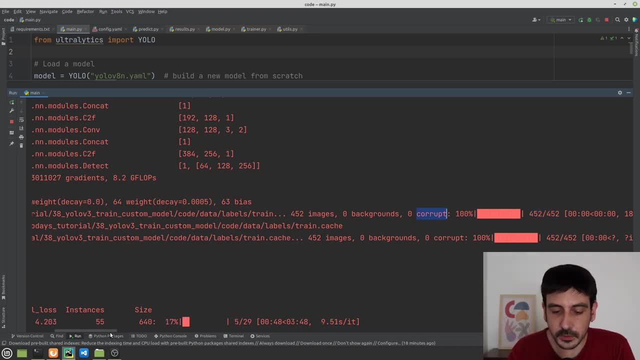 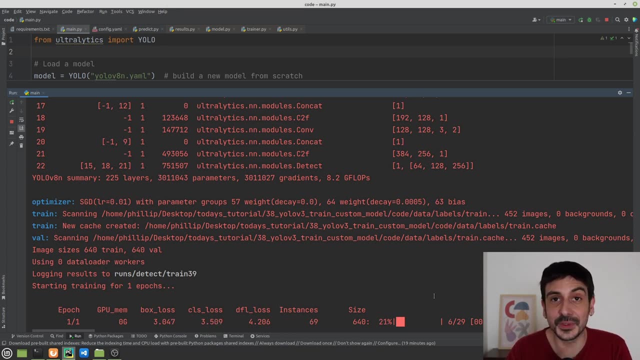 Right, 452 from 452, And if I scroll down, you can see that we have Additional information, additional values Which are related to the training process. This is how the training process is going, Right: we are training this object detector And this additional information Which we are given through this process. 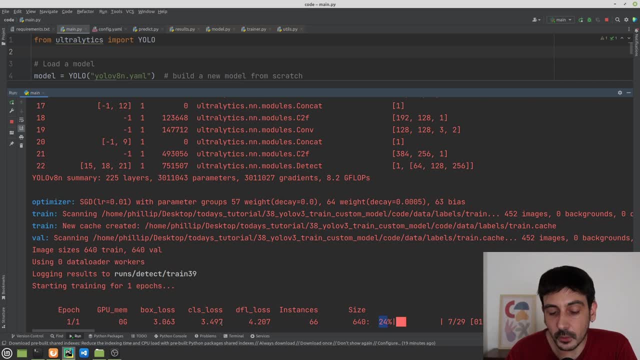 So, for now, the only thing we have to do Is only waiting. We have to wait until this process is completed. So I'm going to stop this video now And I'm going to fast forward this video Until the end of this training. And let's see what happens. 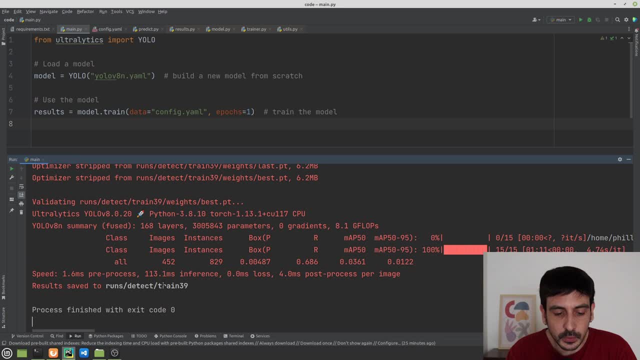 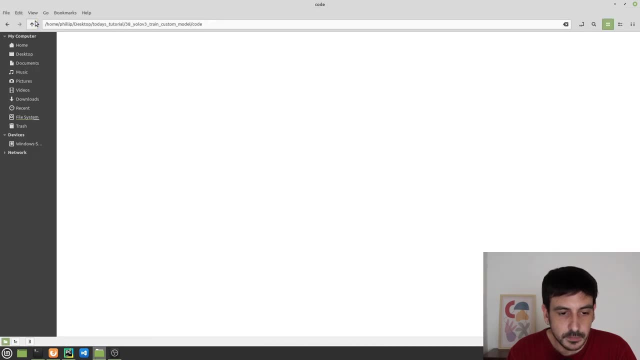 Ok, so the training is now completed And you can see that we have an output Which says results saved to runs, detector And train 39. So if I go to that directory- Runs, detect and train 39- You can see that we have many, many different files. 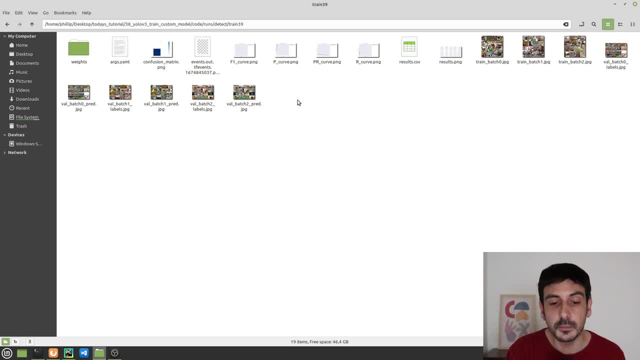 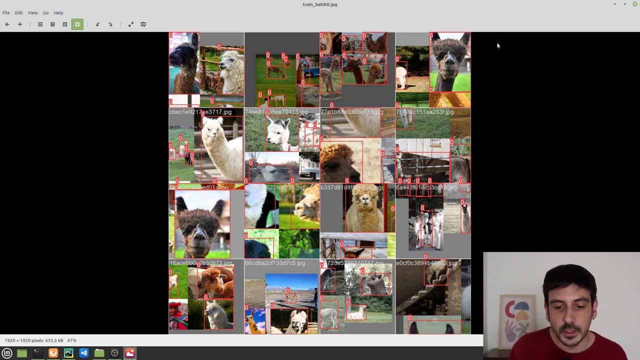 And these are files which are related to How the training process was done. Right, for example. if I show you these images, These are a few batches of images Which were used in order to train this algorithm. You can see the name is train batch 0 And train batch 1. 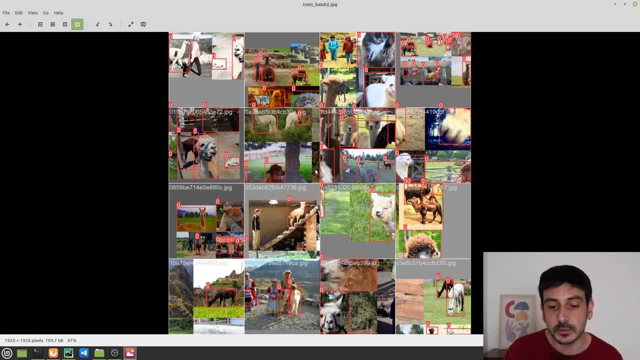 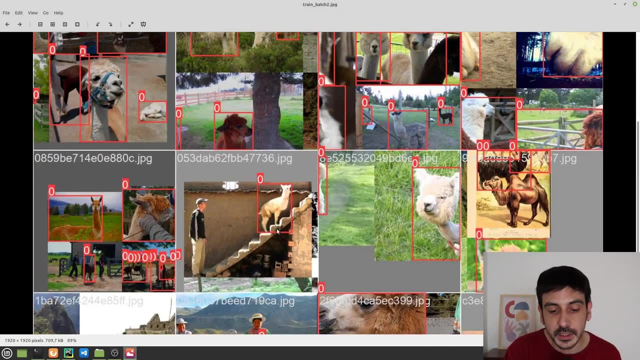 And I think we have a train batch 2. So we have a lot of different images Of a lot of different alpacas, Of different images we used for training, And they were all put together, They were all concatenated Into these huge images So we can see exactly the images. 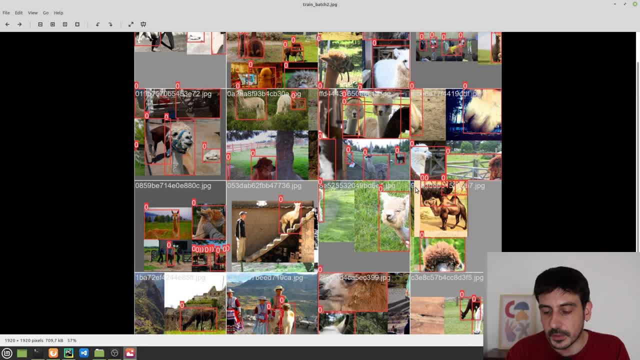 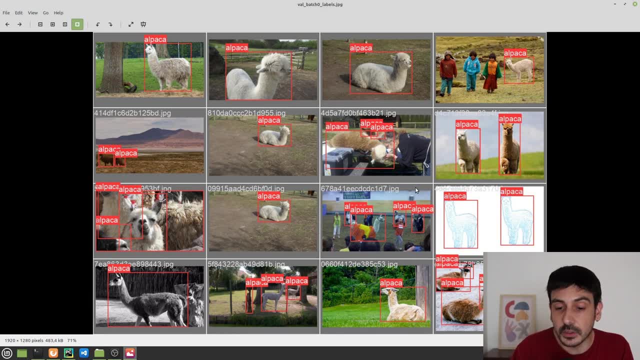 Which were used for training And the annotation on top of them Right, the bounding boxes on top of them. And we also have similar images, But for the validation data set Right. remember in this case We are using the same data as validation As we use for training. 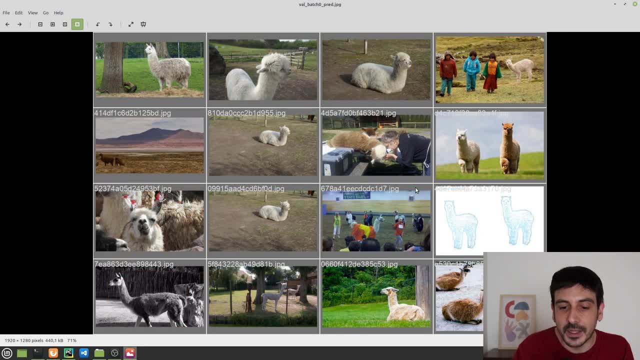 So it's exactly the same data. It's not different data, But these were the labels in the validation data set, Which is the training data set, And these were the prediction on these same images. Right, you can see that we are not detecting anything. We don't have absolutely any prediction. 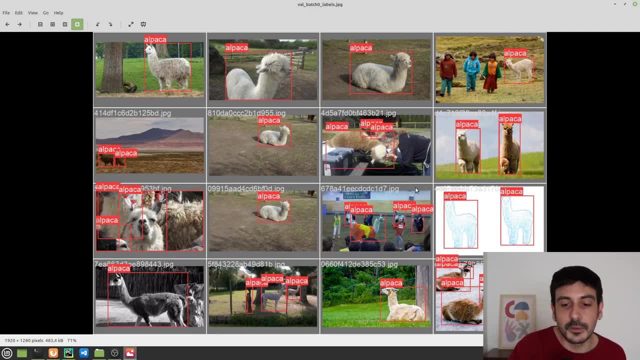 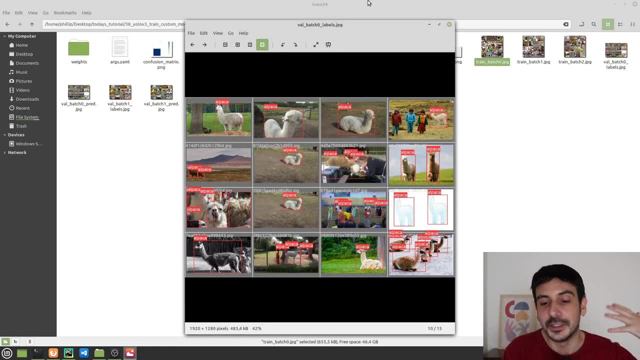 We don't have absolutely any bounding boxes. This is because we are doing a very shallow training. We are doing a very dummy training. We are training this algorithm only for one epoch. This was only an example. To show you the output, How it looks like, To show you the entire process. 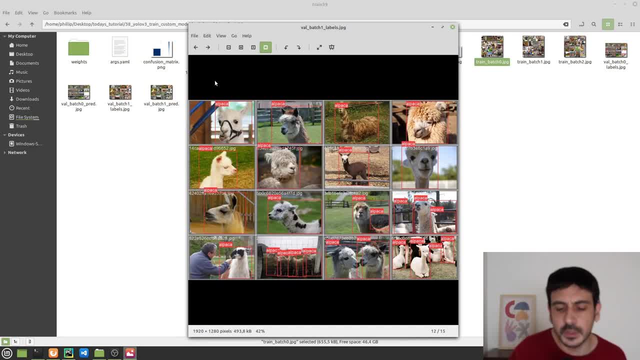 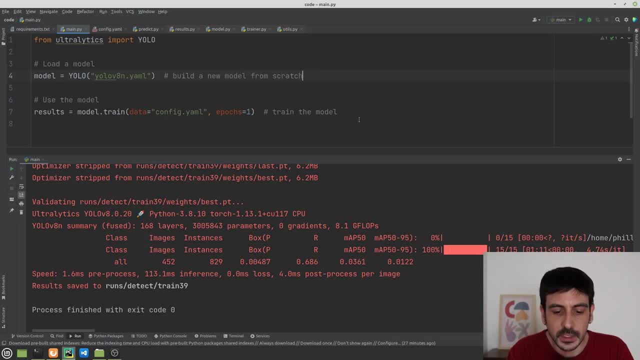 But this is not a real training. But nevertheless, This is some. These are some files. I'm going to show you better When we are in the next step. For now, let me show you how the training is done From the command line, From the terminal, using the command. 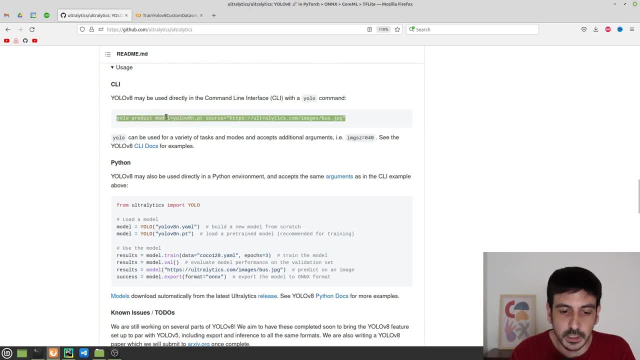 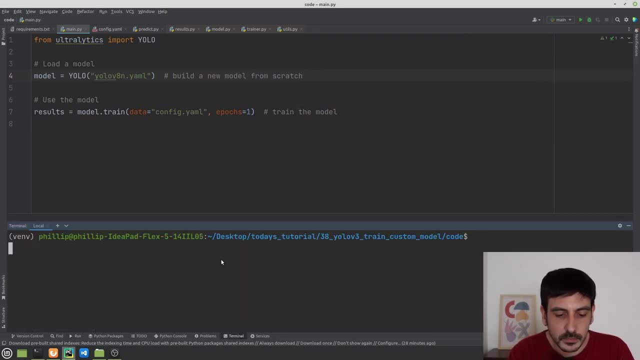 I show you over here Using a command like this, And also let me show you how this training is done On a Google Collab. So, going to the terminal, If we type something like this, YOLO, detect train data. I have to specify the configuration file, Which is configyaml. 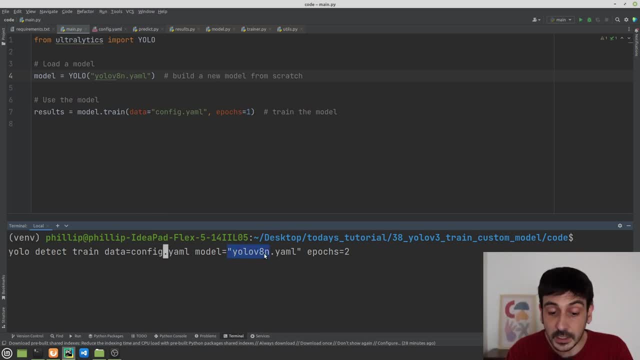 And then modelyolob8nyaml, And then the number of epochs. This is exactly the same as we did here. Exactly the same. It's going to produce exactly the same output. I'm just going to change the number of epochs for once, So we make it exactly the same. 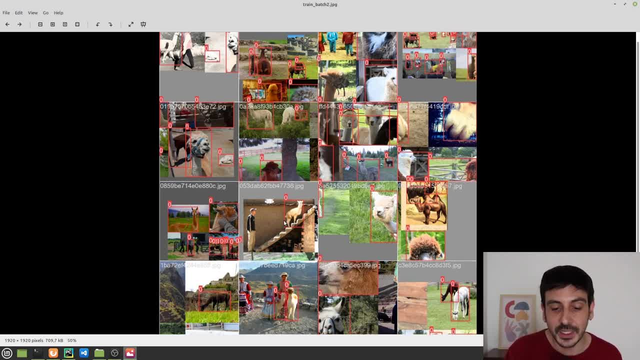 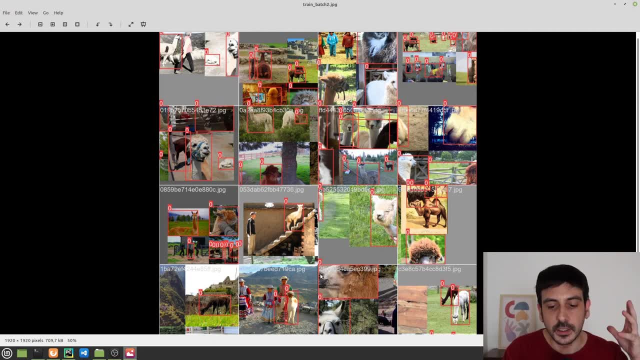 a lot of different alpacas, of different images we use for training and they were all put together. they were all concatenated into these huge images so we can see exactly the images which were used for training and the annotation on top of them. right, the bounding boxes on top of. 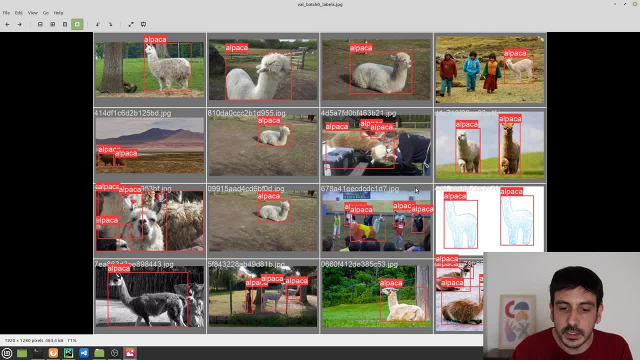 them and we also have similar images. but for the validation data set right, remember, in this case we are using the same data as validation as we use for training, so it's exactly the same data. it's not different data. but these were the labels in the validation that I said, which is the training that I said. 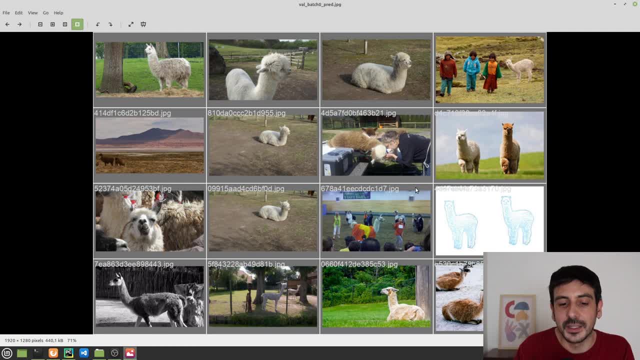 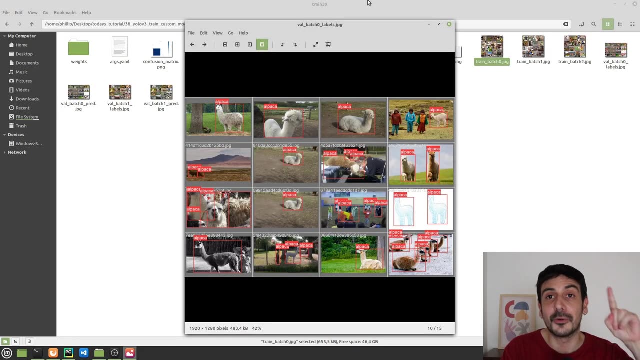 and these were the prediction on these same images. right, you can see that we are not detecting anything. we don't have absolutely any prediction, we don't have absolutely any bounding box. this is because we are doing a very shallow training. we are doing a very dummy training. we are training this algorithm. 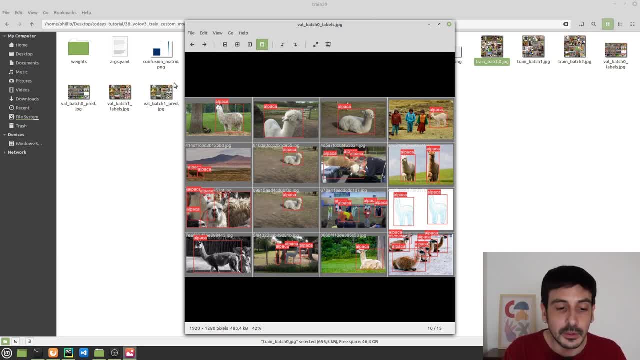 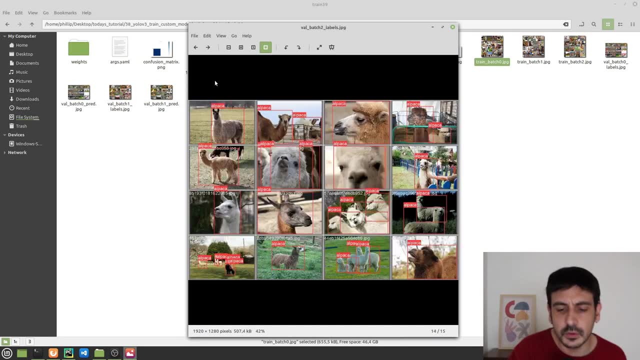 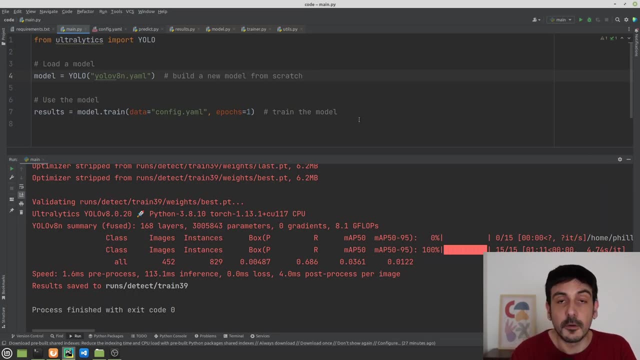 only for one Epoch. this was only an example to show you the output, how it looks like, to show you the entire process, but it is not a real training, but nevertheless, this is some. these are some files I'm going to show you, uh, when we are in the next step. for now, let me show you how the training is done. 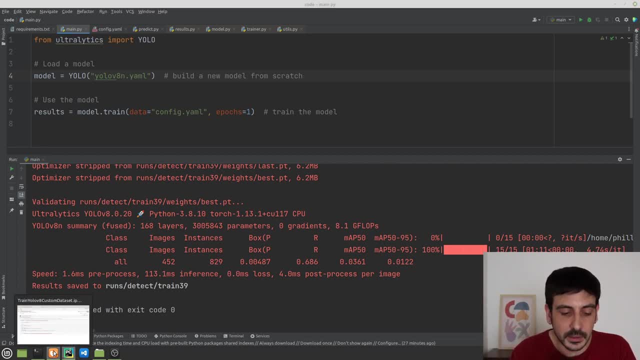 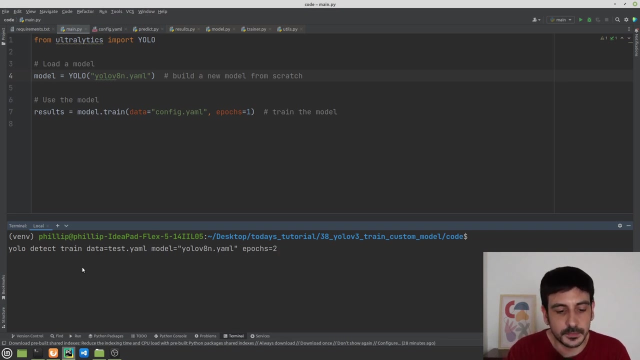 from the command line, from the terminal, using the command. I show you uh over here using a command like this, and also let me show you how this training is done on a Google collab. so, going to the terminal, if we type something like this, YOLO detect. 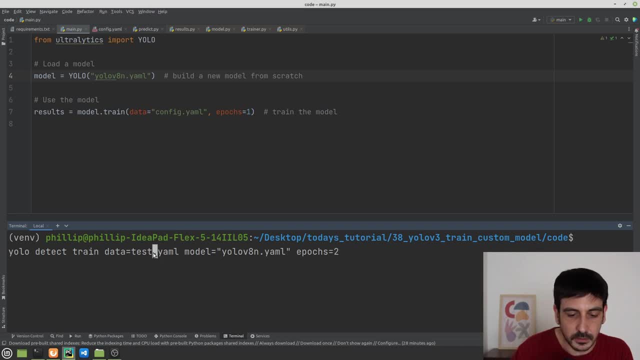 train data. I have to specify the configuration file, which is configyaml, and then modelyolov8nyaml, and then the number of Epochs. this, it's exactly the same as we did here. exactly the same. it's going to produce exactly the same output. I'm 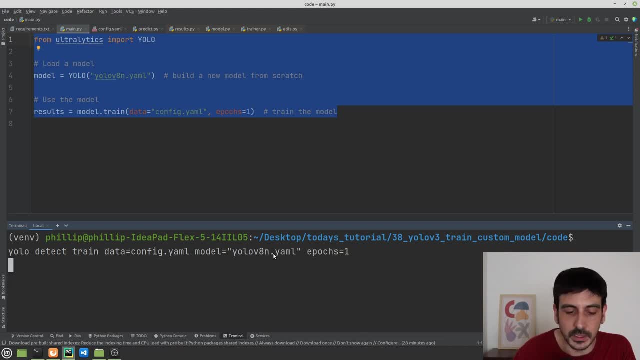 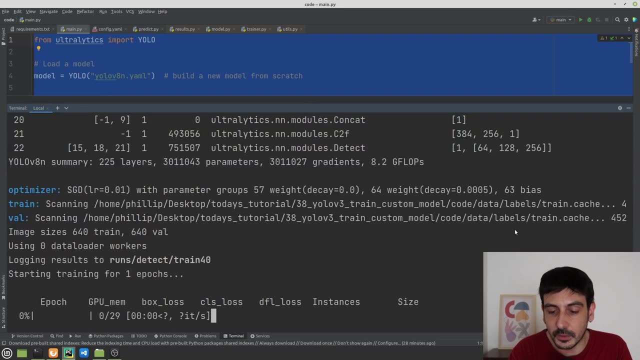 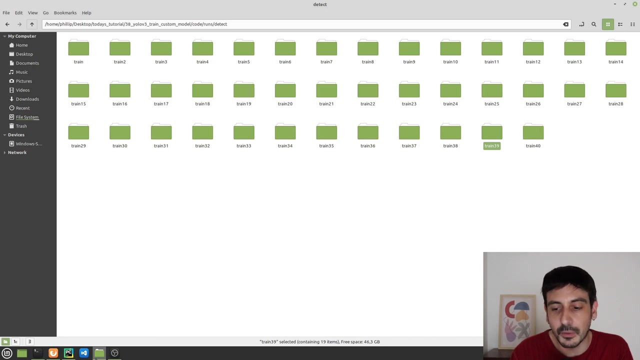 just going to change the number of Epochs for one, so we make it exactly the same and let's see what happens. you can see that it we have exactly the same output, we have load all the images and now we are starting a new training process and after this training process we are going to have a new run. 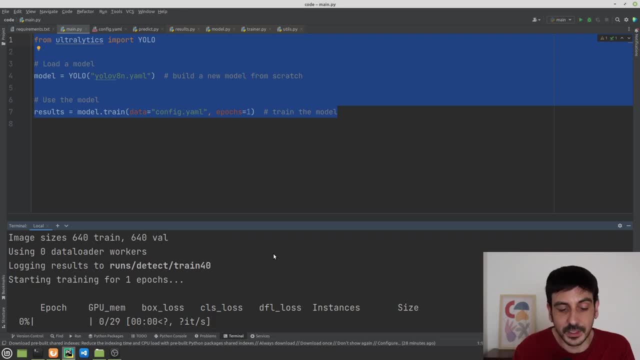 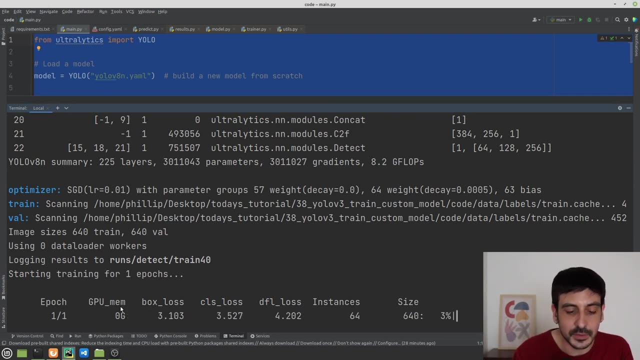 And let's see what happens. You can see that we have exactly the same output. We have loaded all the images And now we are starting a new training process, And after this training process, We are going to have a new run Which we have already created, a new directory. 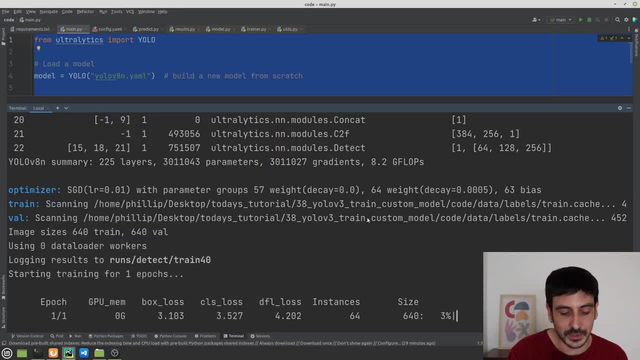 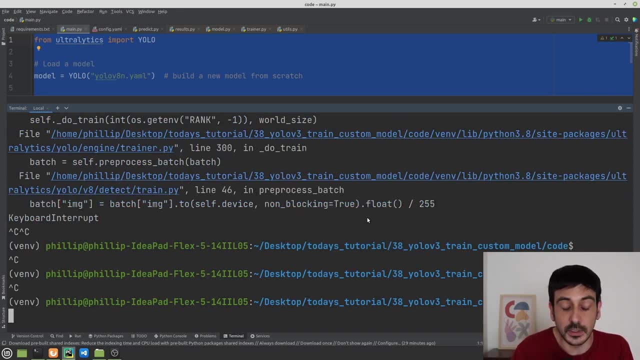 Which is train40, And this is where we are going to save All the information related to this training process. So I'm not going to do it, Because it's going to be exactly the same As the one we did before, But this is exactly how you should use. 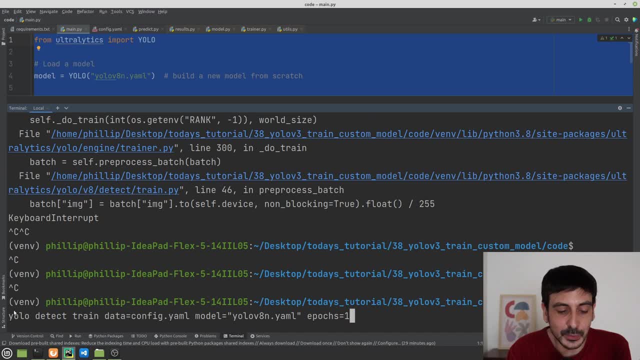 The command line Or how you can use this utility In order to do this training from the terminal. You can see how simple it is. It's amazing how simple it is, It's just amazing. And now let me show you how Everything is done from a Google Colab. 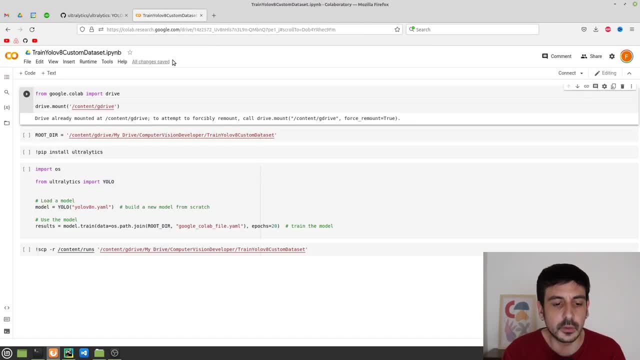 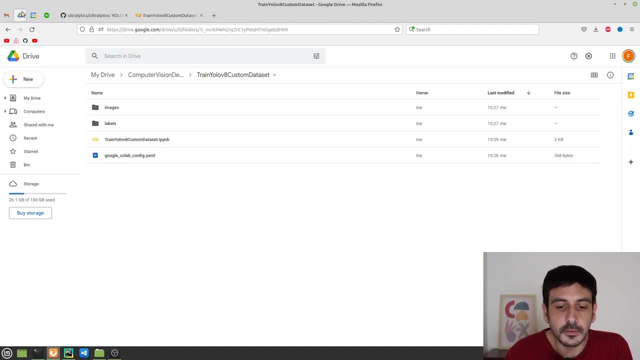 So now let's go back to the browser So I can show you this notebook I created In order to train YOLOv8 from a Google Colab. If you are not familiar with Google Colab, The way you can create a new notebook Is going to Google Drive. 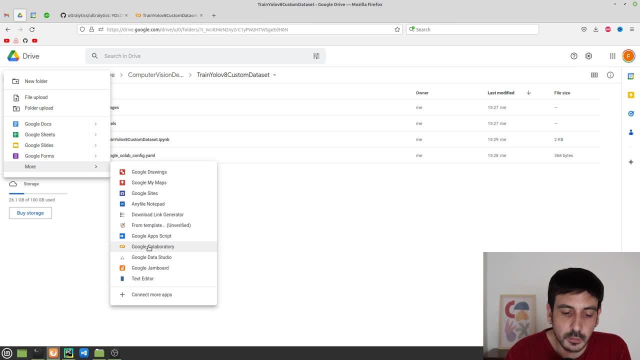 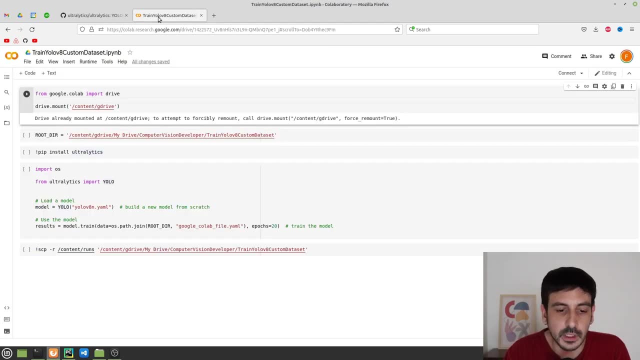 You can click New More And you select the option Google Collaboratory. This is going to create a new Google Colab notebook And you can just use that notebook to train This object detector. Now let me show you this notebook And you can see that it contains only: 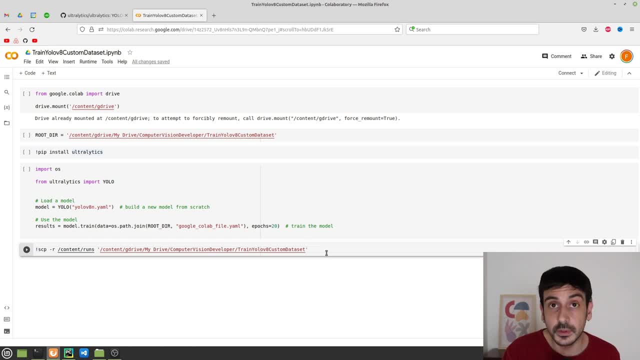 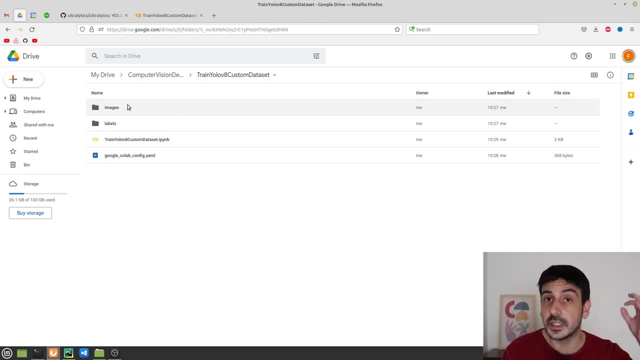 1,, 2,, 3,, 4, 5 cells. This is how simple this will be. The first thing you need to do Is to upload the data you are going to use In order to train this detector. It's going to be exactly the same data. 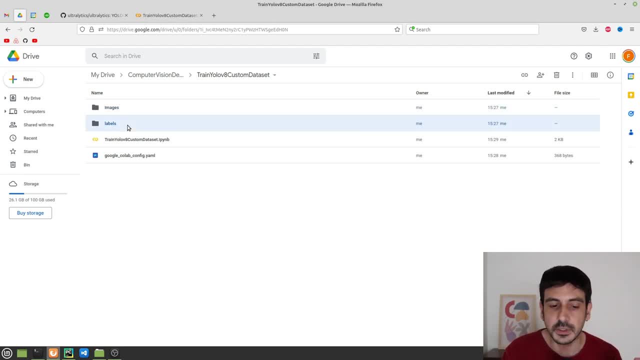 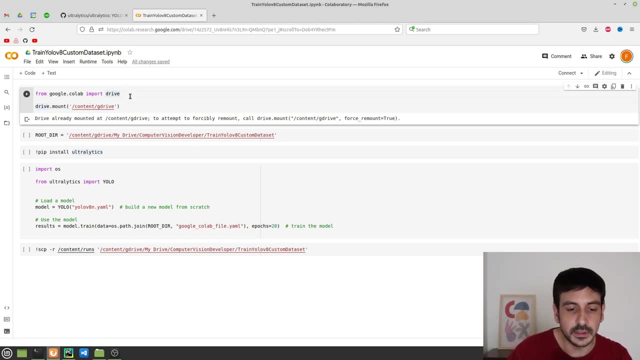 As we used before. So these are exactly the same directories- The images directory and the labels directory We used before- And then the first thing we need to do Is to execute this cell, Which mounts Google Drive Into this instance Of Google Colab. So the only thing I'm doing. 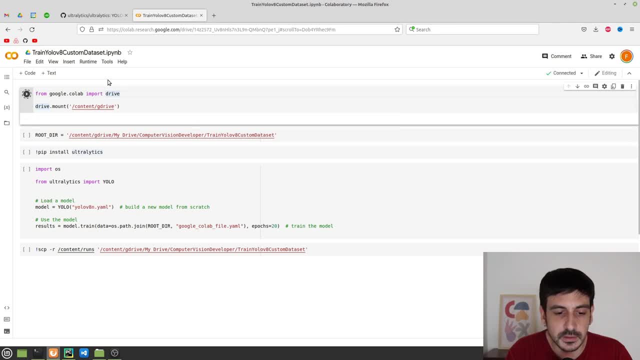 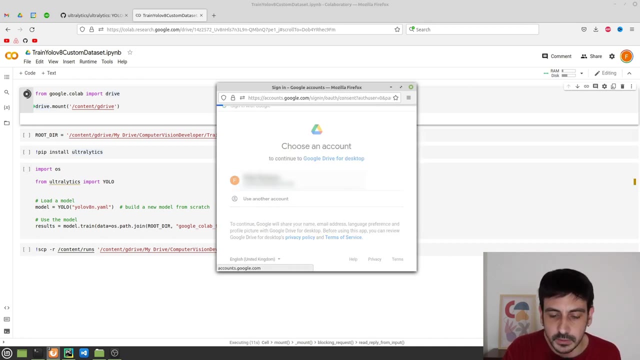 Is just press. I just pressed enter into this cell, And this may take some time, But it's basically. The only thing it does is to connect To Google Drive, So we can just access the data We have in Google Drive. So I'm going to select my account. 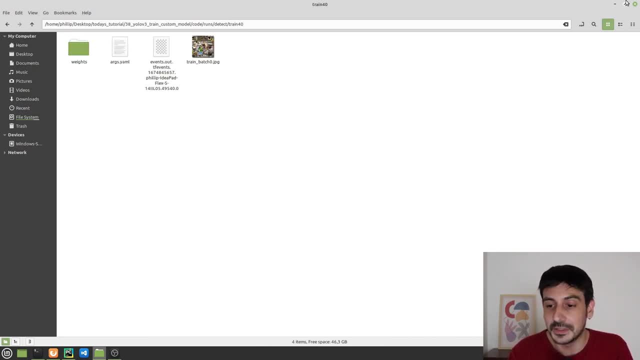 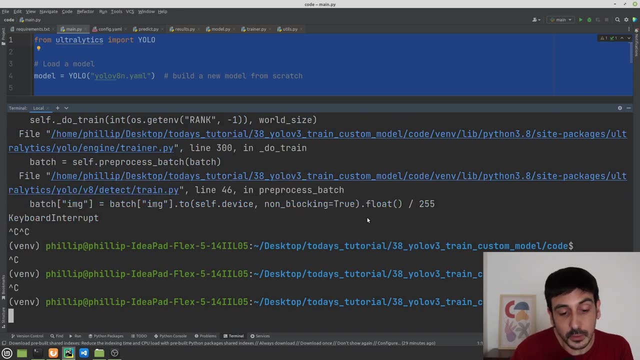 which we have already created, the new directory which is train 40, and this is where we are going to save all the information related to this training process. so I'm not going to do it, because it's going to be exactly the same as the one we did before, but this is exactly how you. 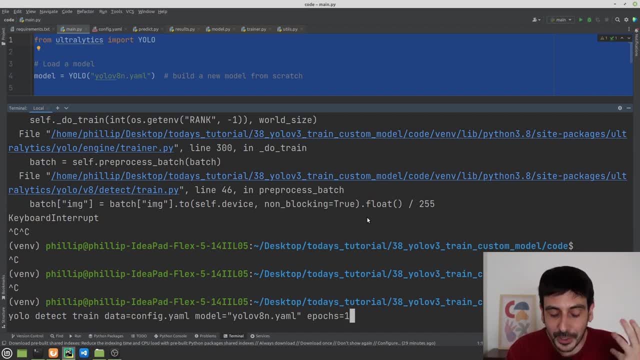 should use the command line. your how you can use this utility in order to, uh, do this training from the terminal. you can see how simple it is. it's amazing how simple it is. it's just amazing. and now let me show you how everything is done from a Google collab. so now let's go back to the browser. 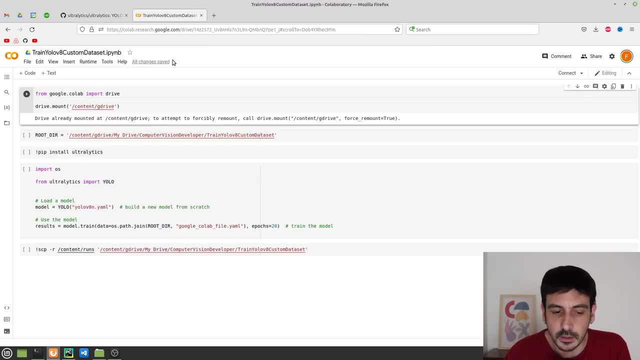 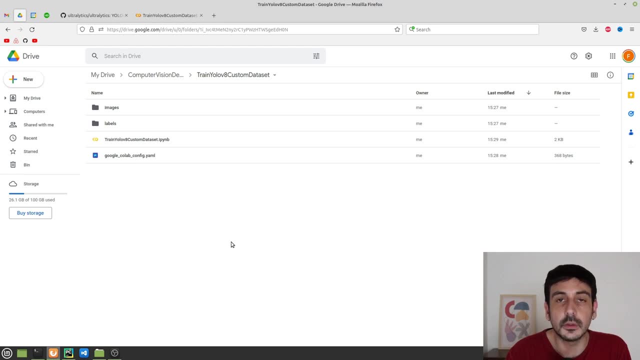 so I can show you this notebook I created in order to train a yellow V8 from a Google collab. if you're not familiar with Google collab, the way you can create a new notebook is going to go Google drive. you can click new more and you select the option Google collaboratory. 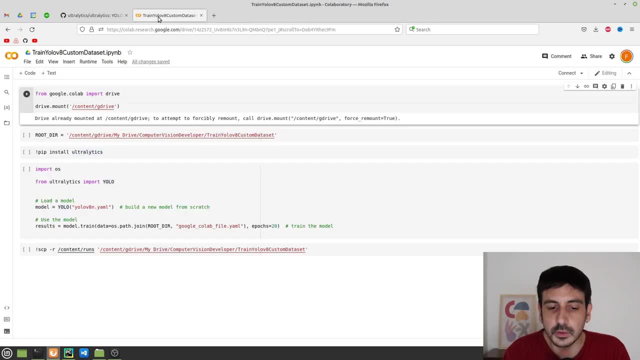 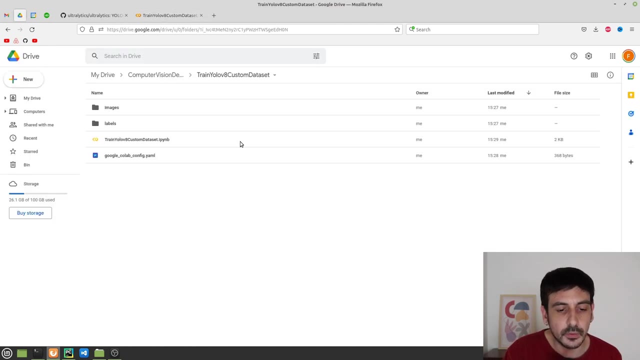 this is going to create a new Google collab notebook, and you can just use that notebook to train this object detector. now let me show you this notebook and you can see that it contains only one, two, three, four, five cells. this is how simple this will be. the first thing you need to do is to upload. 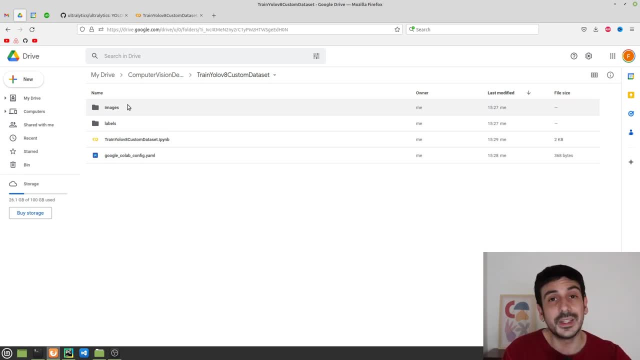 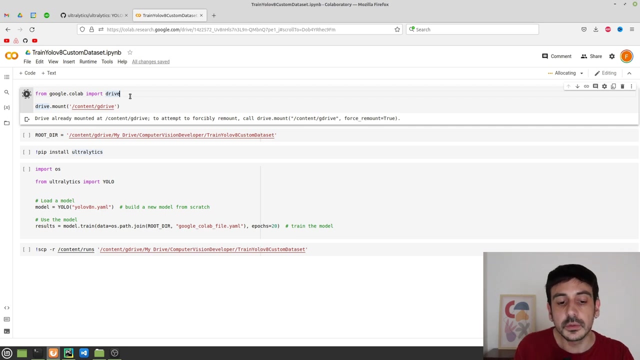 the data you are going to use in order to train this detector. it's going to be exactly the same data as we used before, so these are exactly the same directories- the images directory and the labels directory- we used before. and then the first thing we need, we need to do, is to execute this cell, which mounts Google Drive. 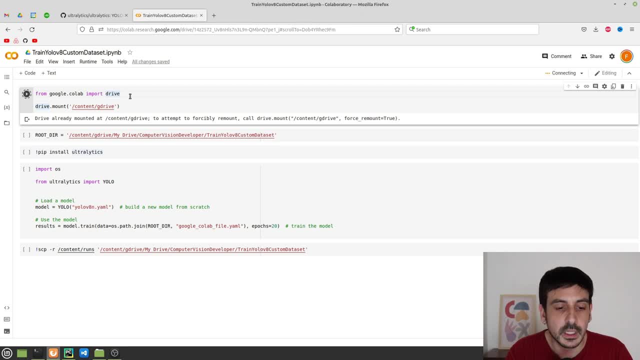 into this instance of Google, of Google collab. so the only thing I'm doing is just press. I just pressed enter into this cell, and this may take some time, but it's basically. the only thing it does is to connect to Google Drive, so we can just access the data we have in Google Drive. so I'm 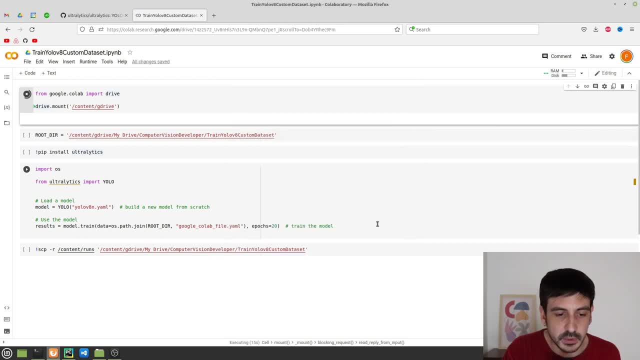 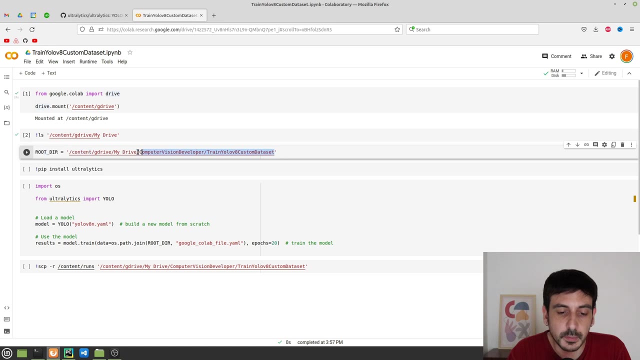 going to save my account and then allow and that's pretty much all. then it all comes to where you have the data in your Google Drive, right in the specific directory where you have uploaded the data. in my case, my data is located in this part, right, this is my home in Google Drive. 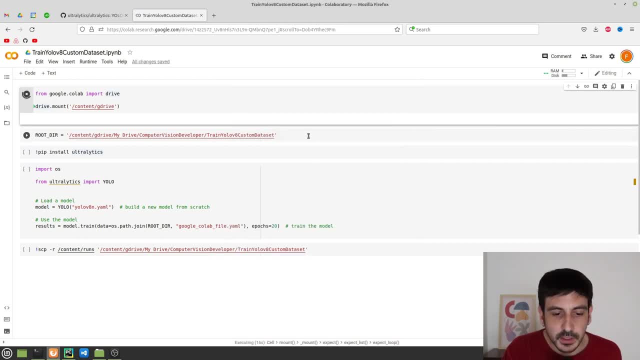 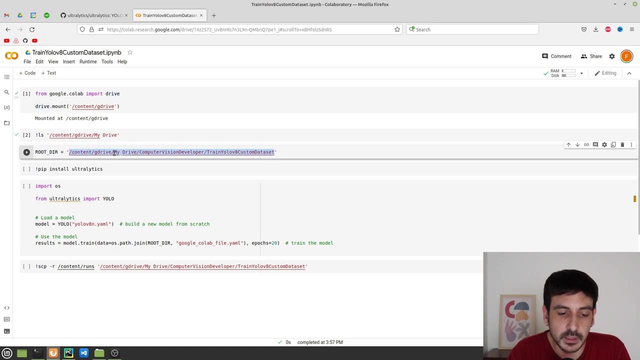 And then allow And that's pretty much all. Then it all comes to Where you have the data In your Google Drive, In the specific directory where you have Uploaded the data. In my case, my data is located In this path: This is my home In Google Drive, And then this is the relative path. 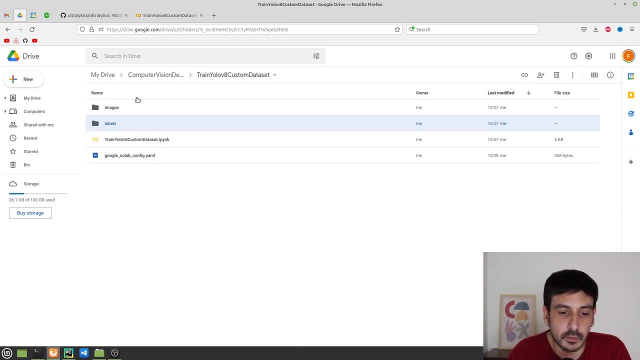 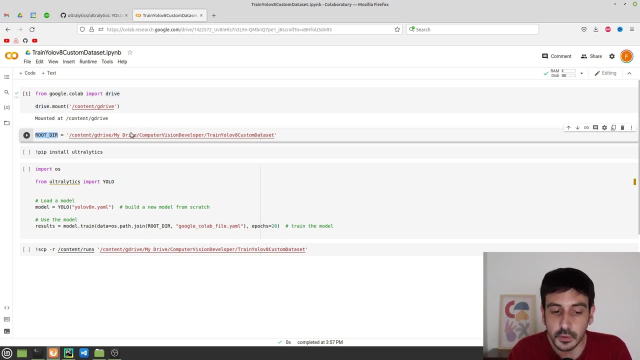 To the location Of where I have the data And where I have all the files related to this project. So remember to specify this root directory As the directory where you have Uploaded your data, And that's pretty much all. Then I'm just going to execute this Cell so I save this variable. 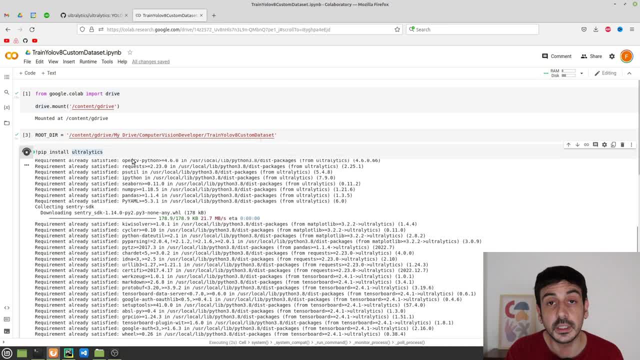 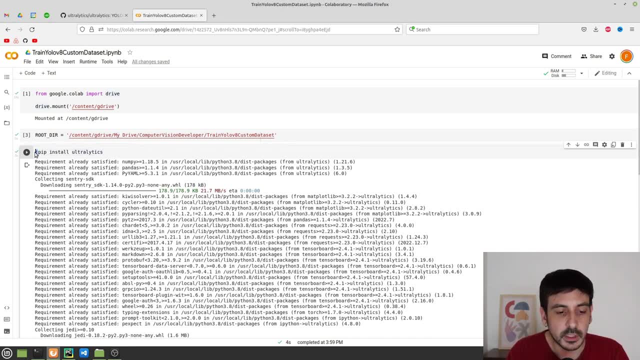 I'm going to execute this other cell, Which is pip install ultralytics. The same command I run from the Terminal in my local environment. Now I'm going to run it in Google Colab. Remember, you have to start this command By the exclamation point, Which means you are running. 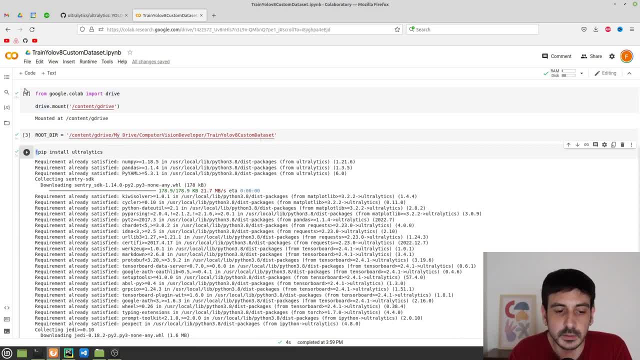 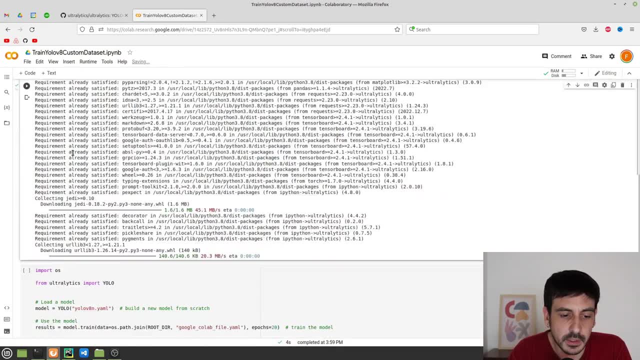 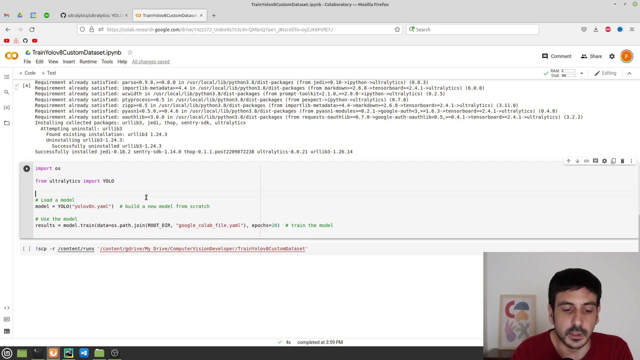 A command in the terminal Where this process is being Executed or where this notebook Is being launched. So remember to include the exclamation point. Everything seems to be Ok, everything seems to be ready, And now we can continue to the next Cell, which is this one. 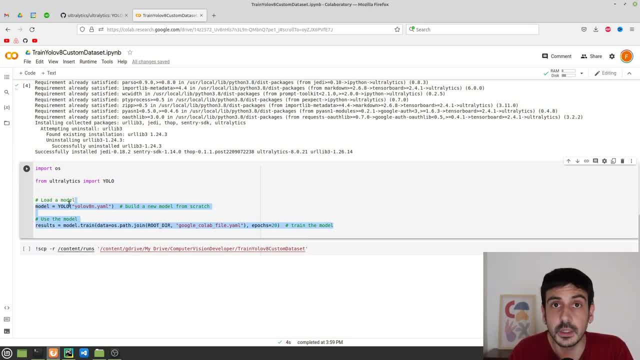 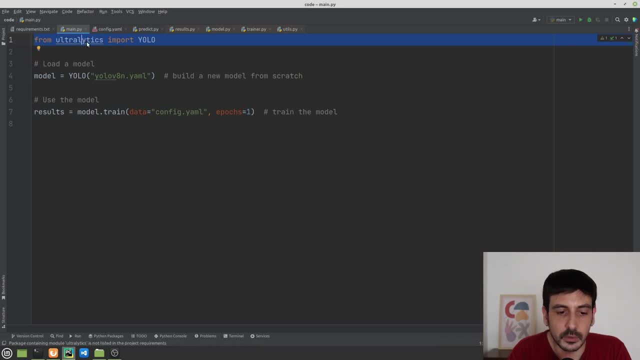 You can see that we have done Exactly the same structure, We have input, exactly the same lines As in our local environment. If I show you this again, You can see we have imported ultralytics, Then we have defined this yellow object And then we have called modeltrain. 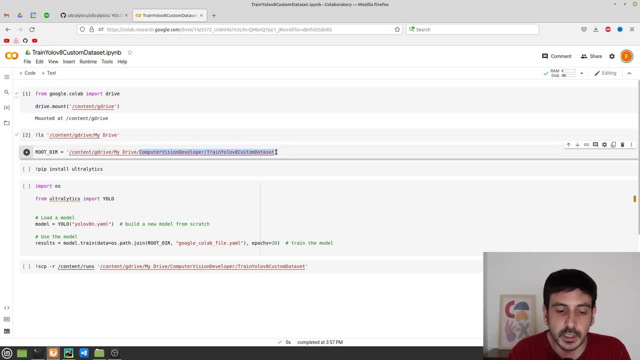 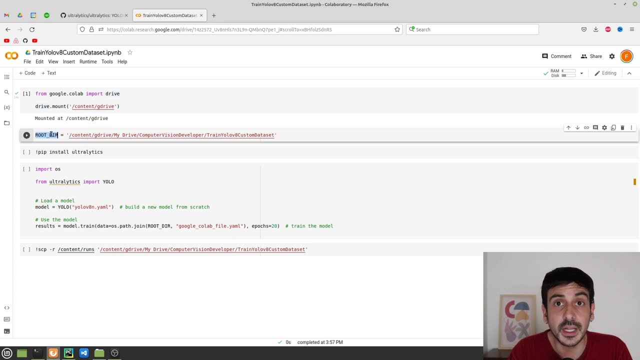 and then this is the relative part to the location of where I have the data and where I have all the files related to this project. so remember to specify this root directory as the directory where you have uploaded your data. and that's pretty much all, and then I'm just going to 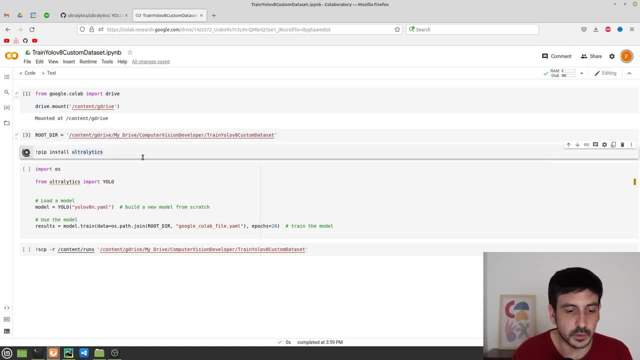 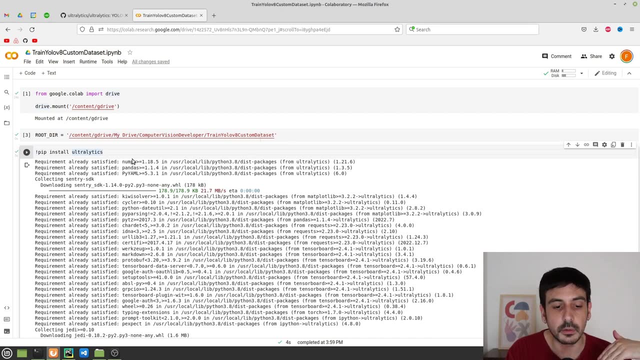 execute this cell. so I save this variable. I'm going to execute this source cell, which is pip: install ultralytics. the same command I run from the terminal in my local environment. now I'm going to run it in Google collab. remember you have to store this command by the exclamation point which: 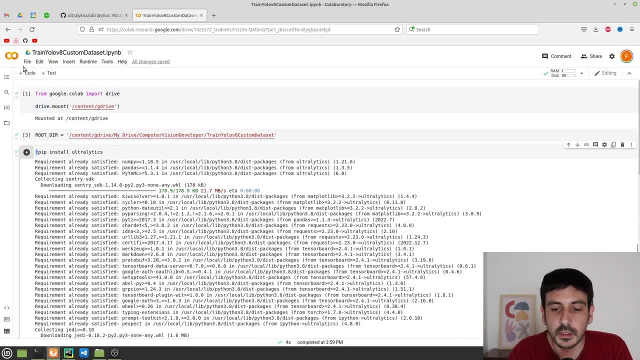 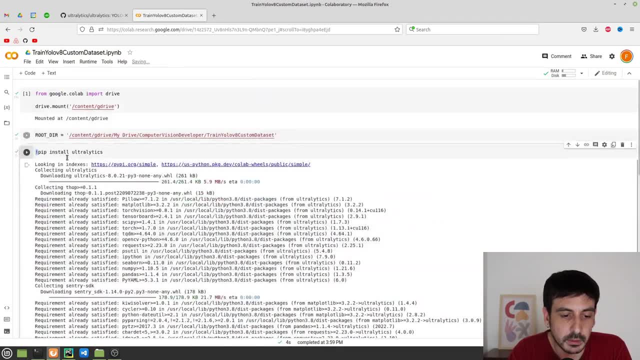 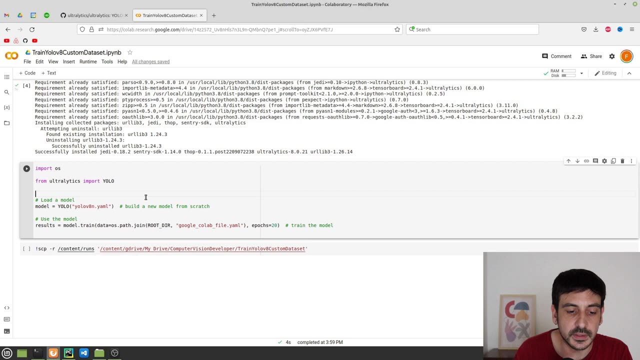 means you are running a command in the terminal where this process is being executed or where this notebook is being launched. so remember to include the exclamation point. everything seems to be okay, everything seems to be ready, and now we can continue to the next cell, which is this one. you can see that we have 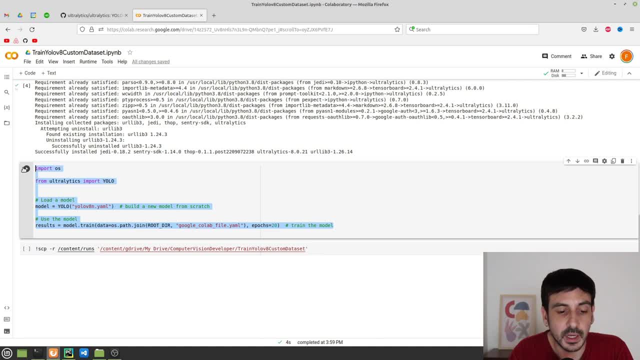 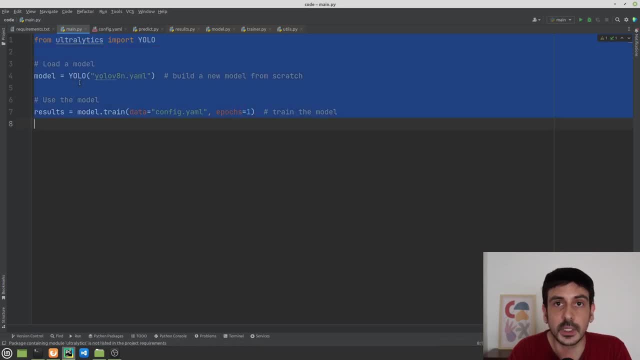 done. exactly the same structure. we have input, exactly the same lines as you know in our local environment. if I show you this again, you can see we have imported ultralytics, then we have defined this yellow object and then we have called modeltrain, and this is exactly the same as we are. 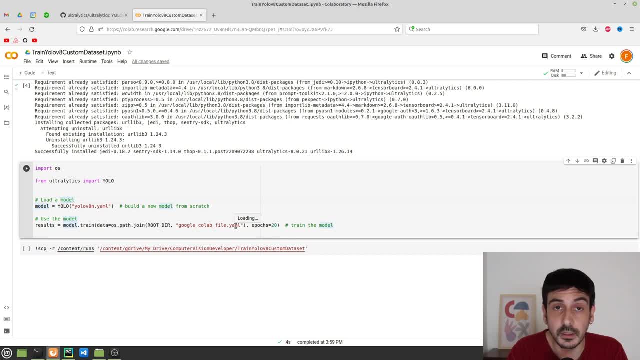 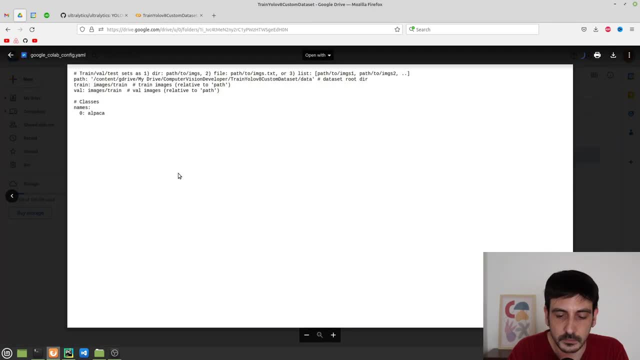 doing here. obviously, we are going to need another yaml file. we are going to need a yaml file in our Google Drive and this is the file I have specified, which has the. it's like exactly the same configuration as in the um, as in the, in the yaml file I show you in my local environment. it's exactly the same idea. 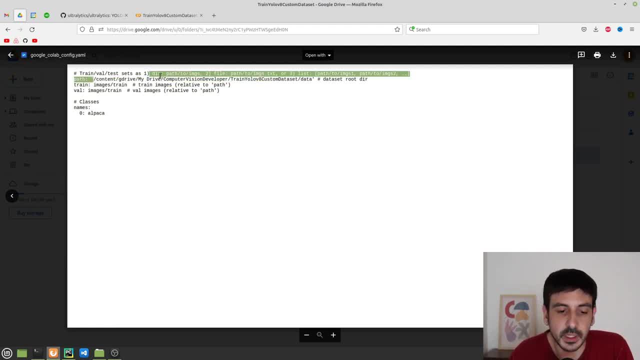 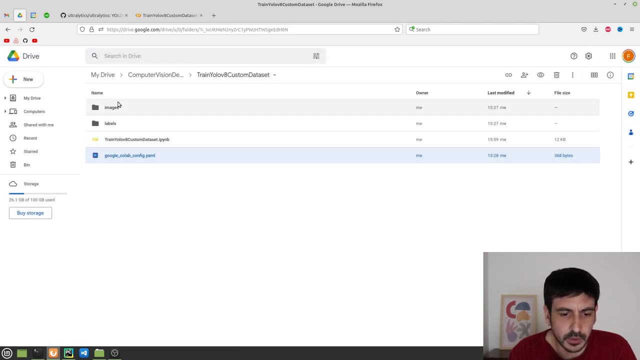 so this is exactly what you should do now: you should specify a, an absolute path to your Google Drive directory. that's the only difference. so that's the only difference, and I see I have a very small mistake, because I see I have data here and here. I have just uploaded images and labels in. 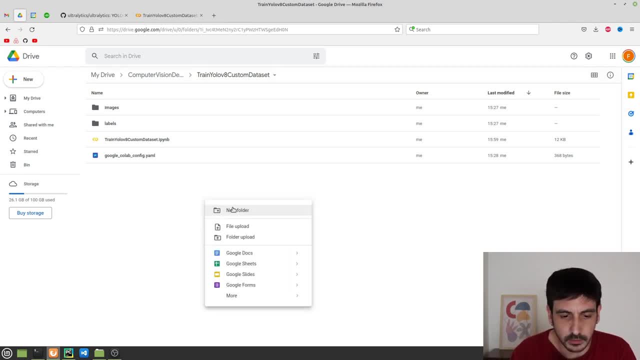 the directory, but they are not within another directory which is called data. so let me do something. I'm going to create a new directory which is called data- images, labels. I'm just going to put everything here right, so everything is consistent. so now everything is okay: images, then train and then. 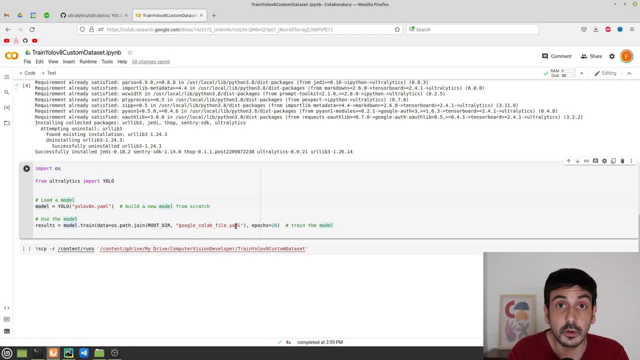 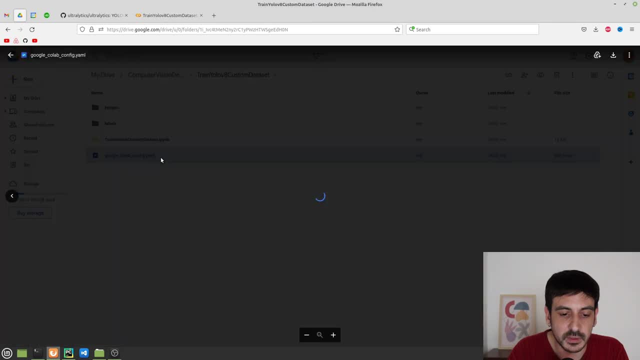 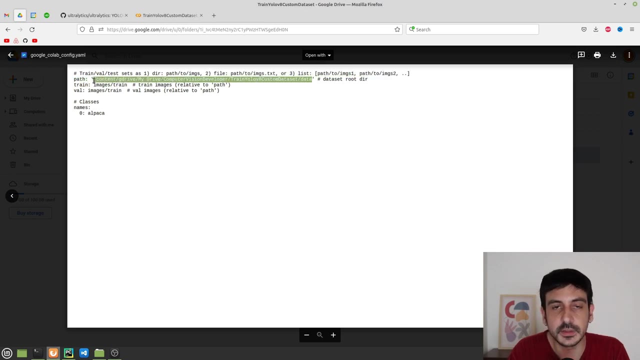 And this is exactly the same As we are doing here. Obviously, we are going to need another YAML file. We are going to need a YAML file In our Google Drive, And this is the file I have specified, Which Has the. It's like exactly the same Configuration as in: 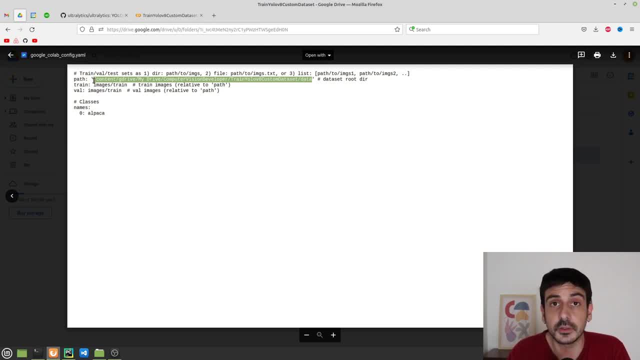 The In the YAML file I showed you In my local environment. It's exactly the same idea, So this is exactly what you should do Now. you should specify an absolute path To your Google Drive directory. That's the only difference, And I see I have a very small mistake. 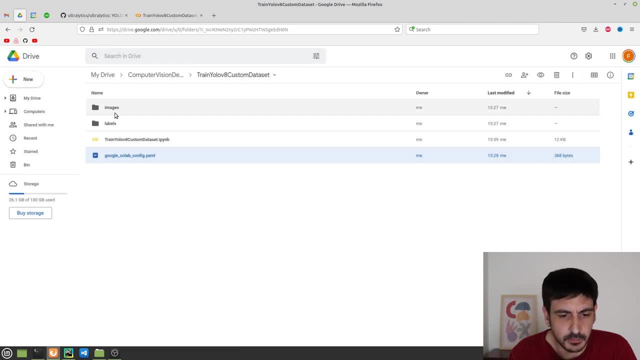 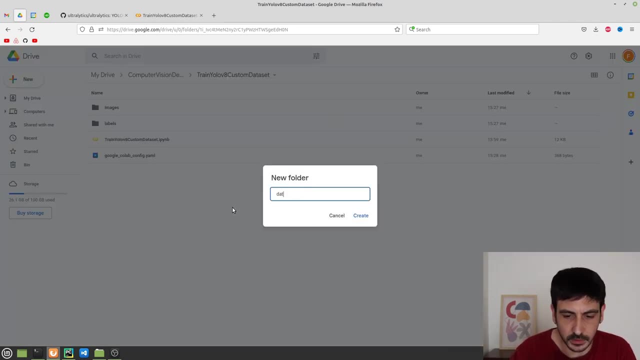 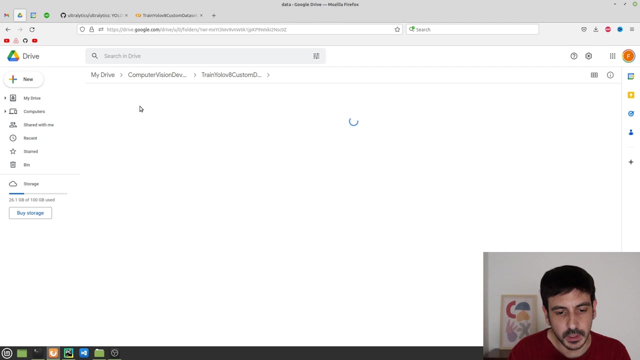 Because I see I have data Here, So I'm going to Just upload the images and labels In the directory, But they are not within another directory, Which is called data. So let me do something. I'm going to create a new directory Which is called data- images, labels. 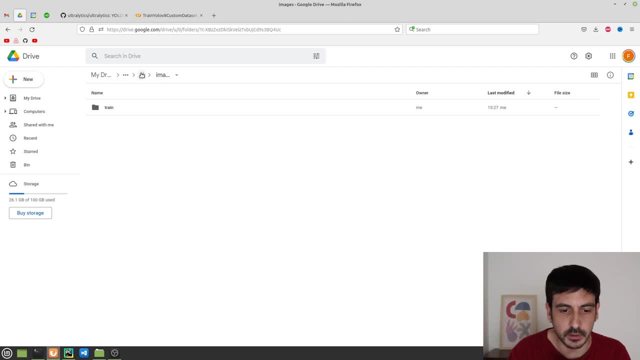 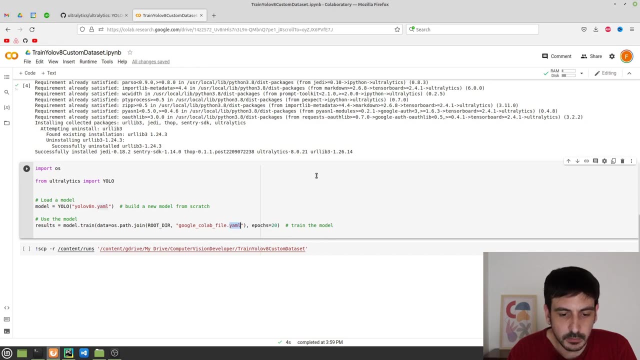 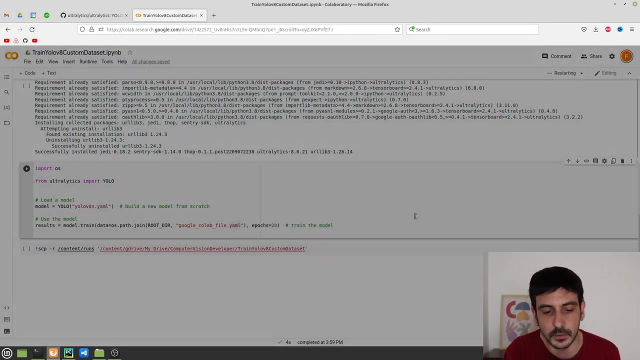 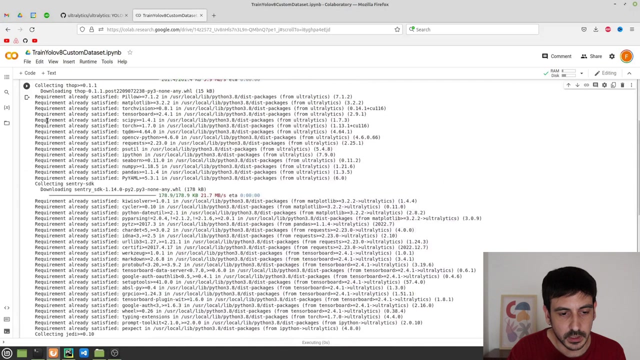 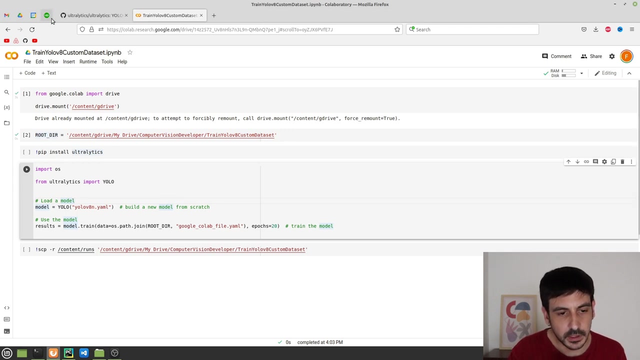 I'm just going to put everything here Right, so everything is consistent. So now everything is ok: Images, then train, And then the images are within this directory, So everything is ok, And then, after that, I'm going to Extract it And then I'm going to 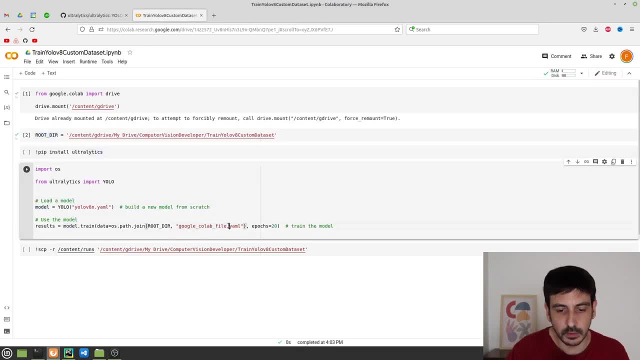 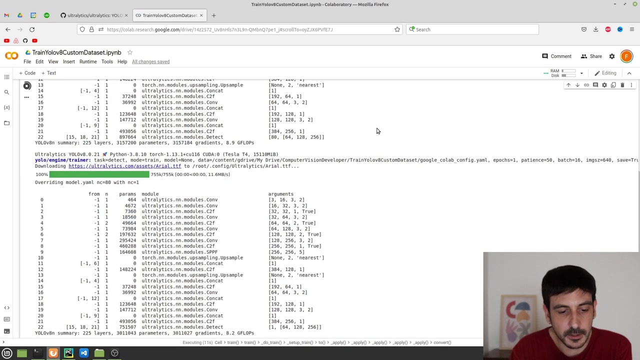 I'm going to, If I have a Site, Or i'm just going to run it for one epoch. so everything is exactly the same as we did in our local environment. and now let's see what happens. so you can see that we are doing exactly the same process. everything looks pretty much the same as it did before. we are loading the data. we 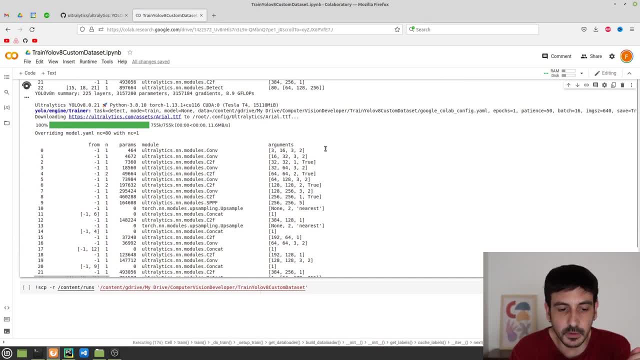 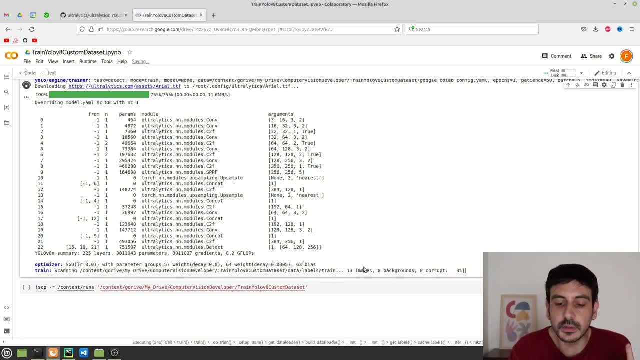 are just loading the, the modules, everything. it's going fine and this is going to be pretty much the same process as before. you can see that now we are it. it takes some additional time to load the data because now you have, you are running this environment, you're running this, uh, node boot. 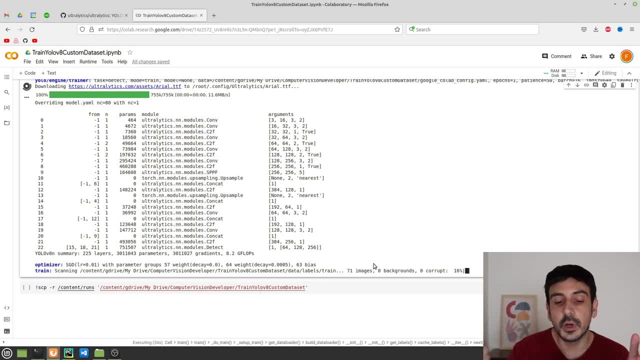 in a given environment and you're taking the data from your google drive, so it takes some time. it's it's a slower process, but it's definitely the same idea, so the only thing we need to do now is just to wait until all this process to be completed, and that's pretty much all. 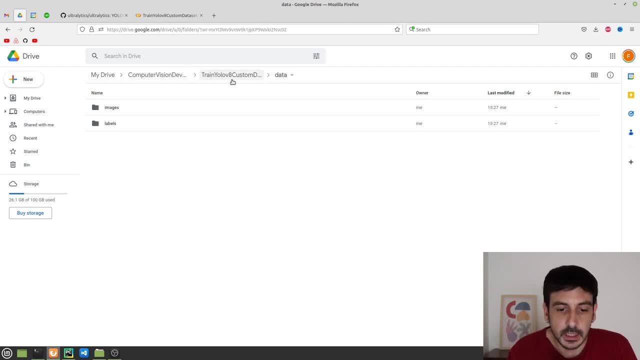 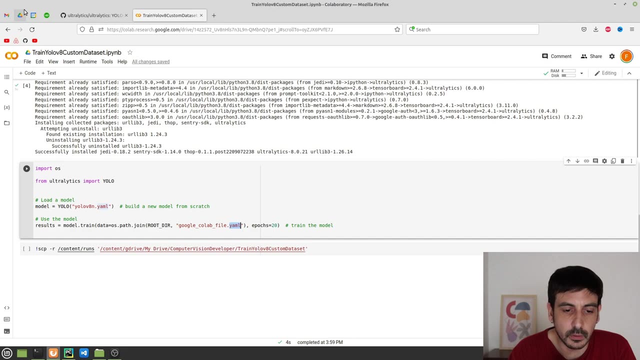 the images are within this directory, so everything is okay. now let's go back to the Google collab. every time you make an edit, or every every time you do something in Google Drive, it's always a good idea to restart your runtime. so that's what I'm going to do. I'm going to execute the commands. 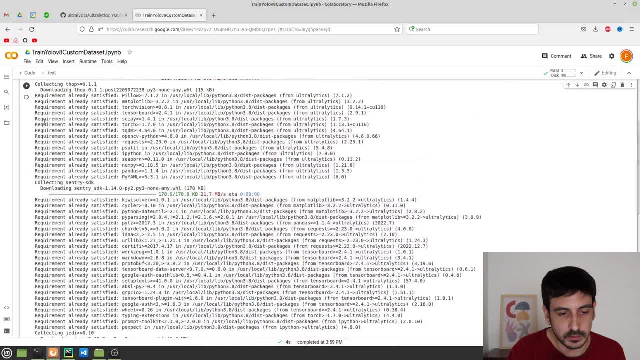 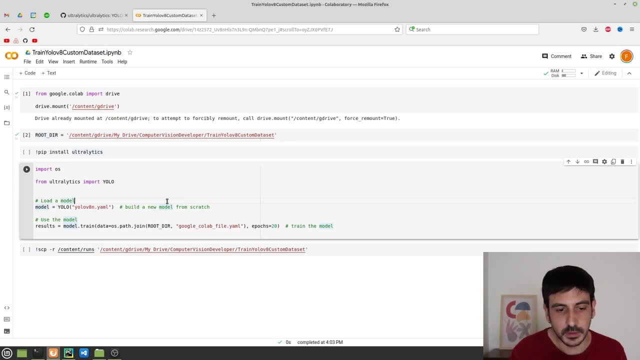 again. I don't really need to pip install this library again, because it's already installed into this environment, and then I'm going to execute this file. I think I have to do an additional edit, which is this file: now it's called googlecomfig and that's pretty much all I'm just going to run. 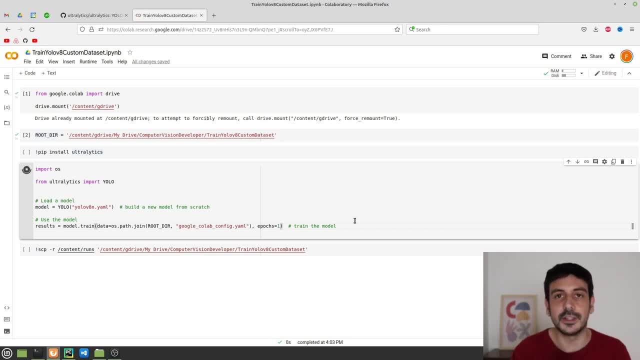 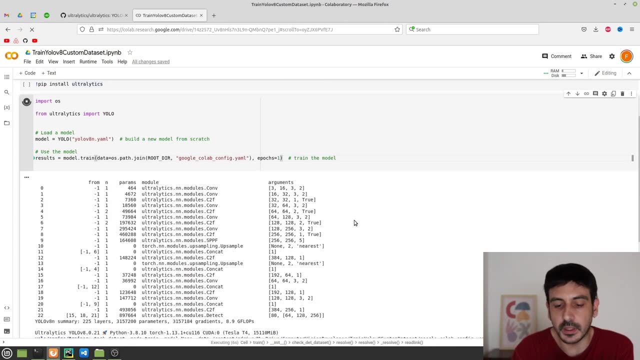 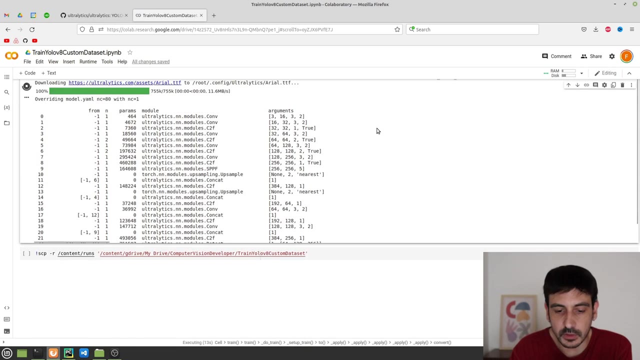 it for one Epoch. so everything is exactly the same as we did in our local environment. and now let's see what happens. so you can see that we are doing exactly the same process. everything looks pretty much the same as it did before. we are loading the data, we are just loading the, the modules, everything it's going fine, and this: 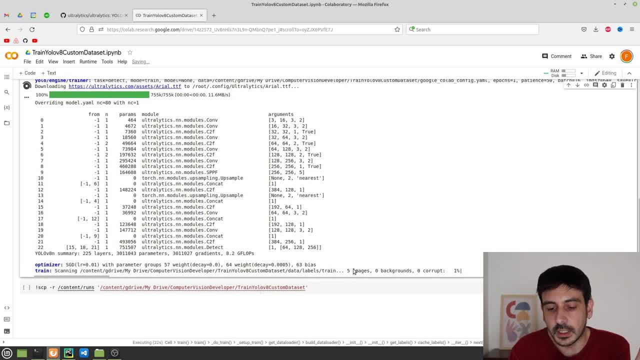 is going to be pretty much the same process as before. you can see that now we are it. it takes some additional time to load the data because now you have, you are running this environment, you're running this notebook in a given environment and you're taking the data from. 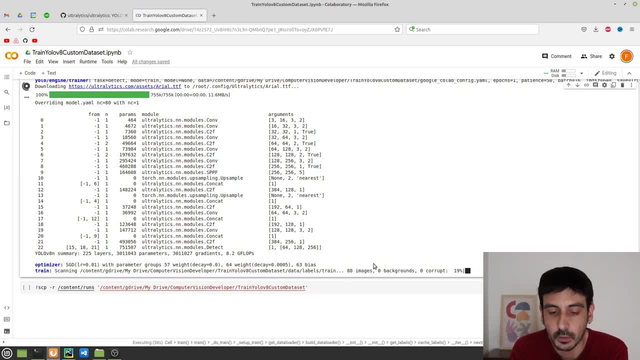 your Google Drive, so it takes some time. it's it's a slower process, but it's definitely the same idea. so the only thing we need to do now is just to wait until all this uh process to be completed, and that's pretty much all. I think it doesn't really make. 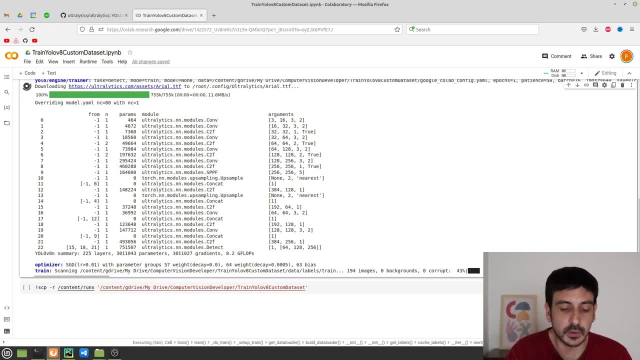 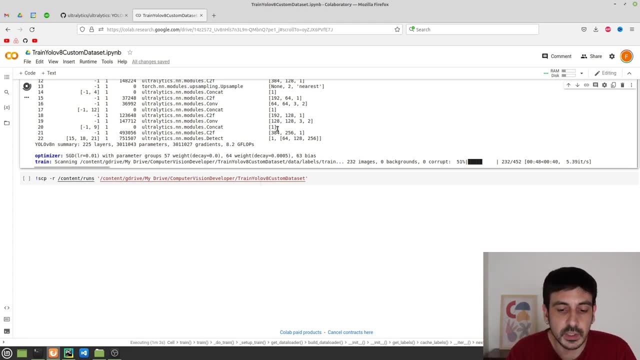 any sense to wait, because it's like it's going to be exactly the same process as we did from our local environment. at the end of this execution, we are going to have all the results in a given directory, which is the directory of the notepad which is running this process. so at the end of 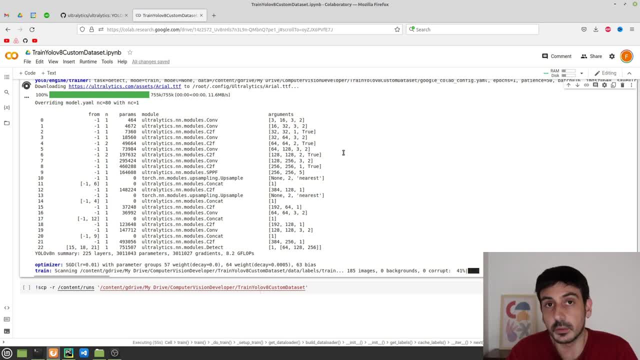 and that's it, guys. thank you so much for watching and i'll see you in the next video, bye-bye. think it doesn't really make any sense to wait, because it's like it's going to be exactly the same process as we did from our local environment at the end of 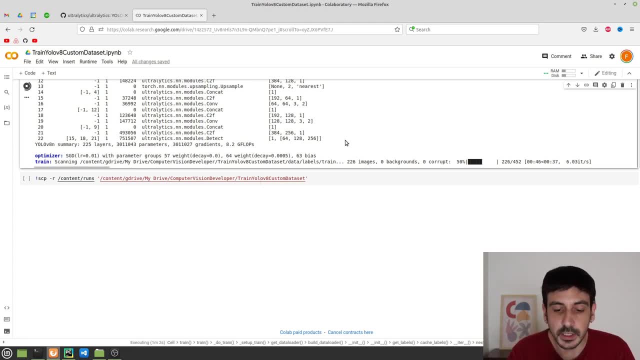 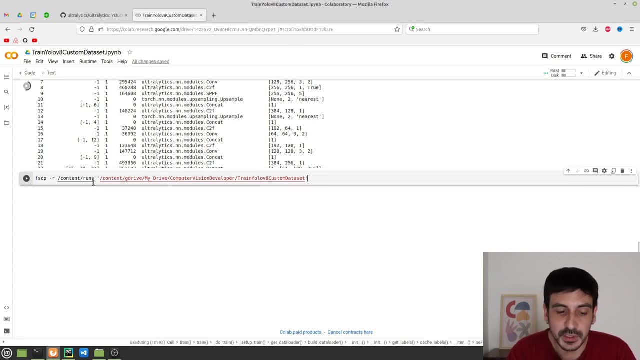 this execution, we are going to have all the results in a given directory, which is the directory of the notepad which is running this process. so, at the end of this process, please remember to execute this command, which is going to take all the files you have defined in this runs directory, which contains all the runs. 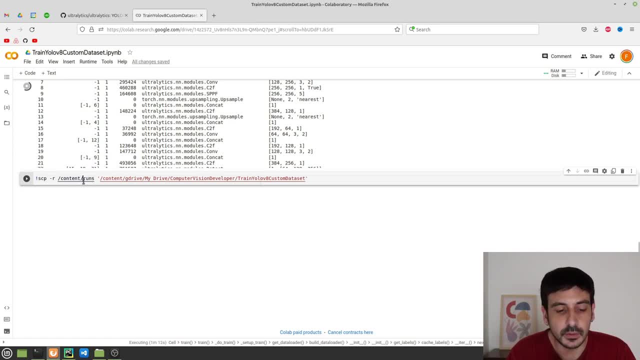 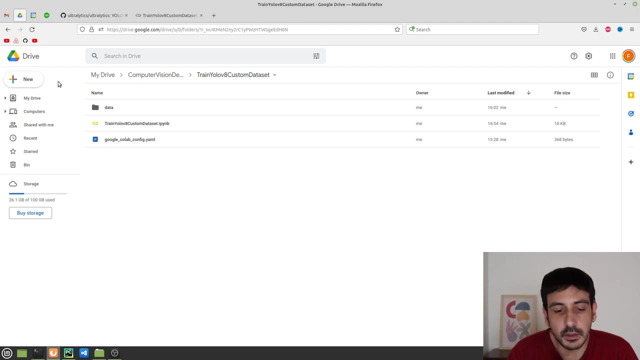 this process. please remember to execute this command, which is going to take all the files you have defined in this runs directory, which contains all the runs you have made, all the results you have produced, and it's going to take all this, all this directory, into the directory you have chosen for your files and your data and your rule: collab. 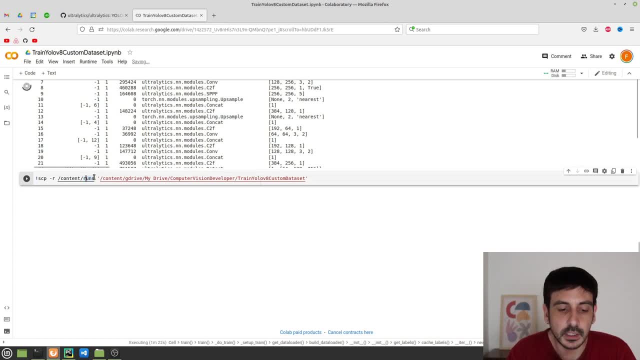 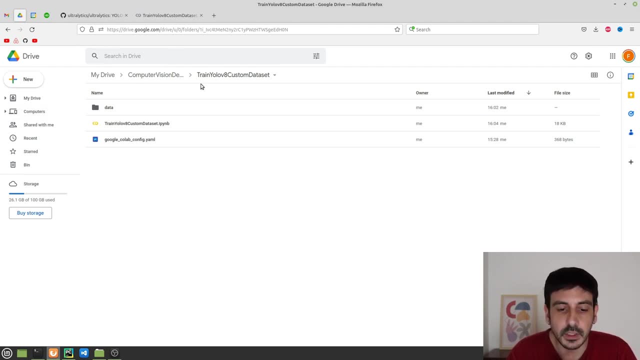 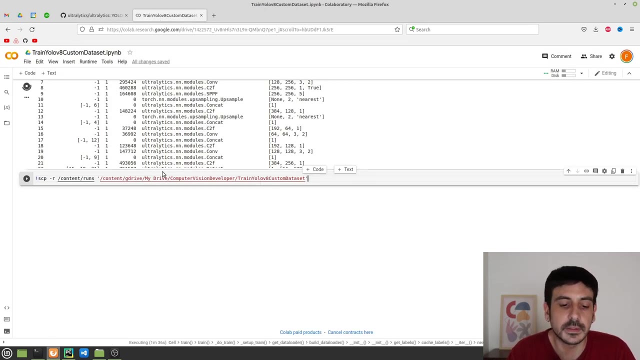 you have made, all the results you have produced, and it's going to take all these, all these directory, into the directory you have chosen for your files and your data and your rule call up and so on. please remember to this because otherwise you would not be able to access this data and is the data which 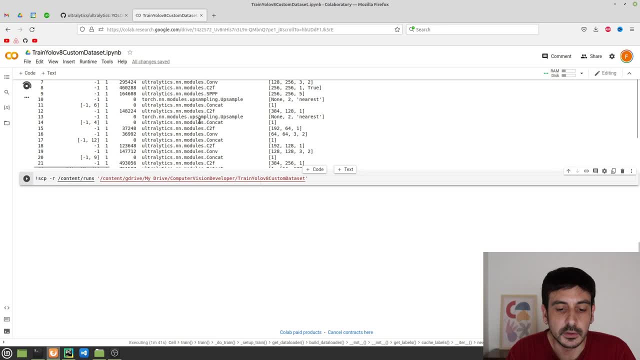 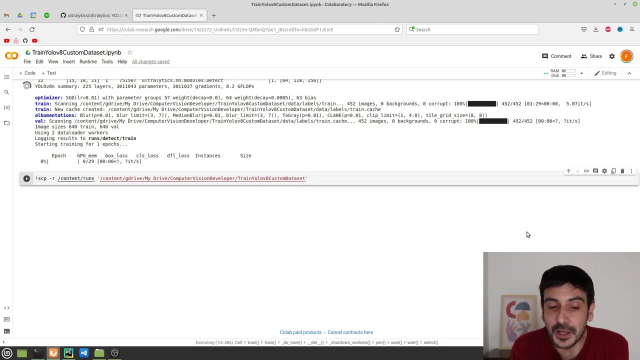 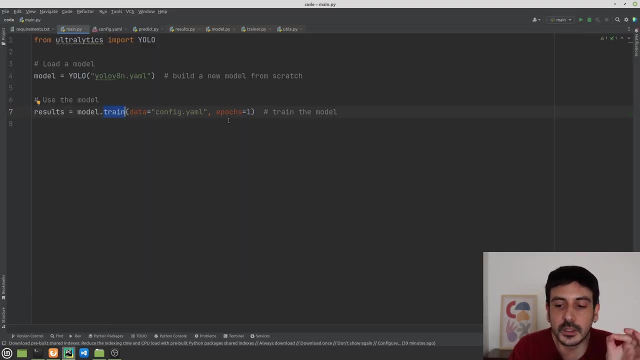 contains all the results and everything you have just trained. so this is how you can train a yellow v8- and, obviously, detector using yellow v8 in a Google Drive colab, and you can see that the process is very straightforward and it's pretty much exactly the same process, exactly the same idea as we did in our local environment, and that's it. 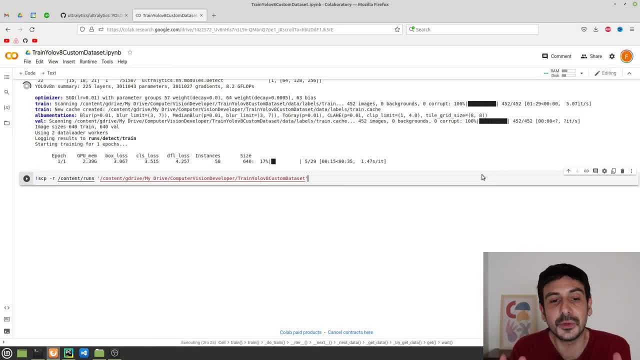 so that's how easy it is to train an object detector using yolo v8 once you have done everything we did with the data right. once you have collected the data, you have annotated the data, you have taken everything into the format yolo v8 needs in order to train an object detector. 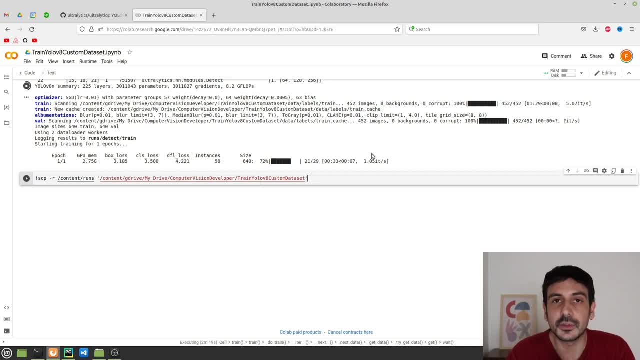 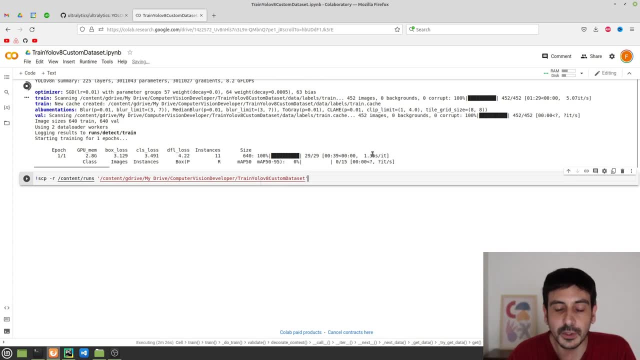 once everything is completed, then running this process, running this training, is super straightforward. so that's going to be all about this training process, and now let's continue with the testing. now let's see how these models we have trained, how they performed right. let's move to the next step, and this is the last step in this process. this is where we are going to take the 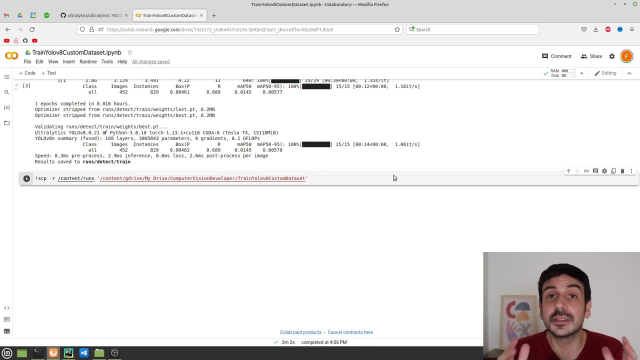 model we produced in the training step and we're going to test how it performs. this is the last step. this is the last step in this process. this is the last step in the tutorial step, like you obviously step in this process. this is how we are going to complete this training of an object detector using 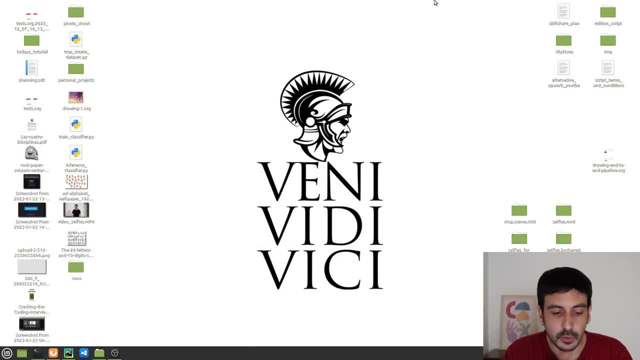 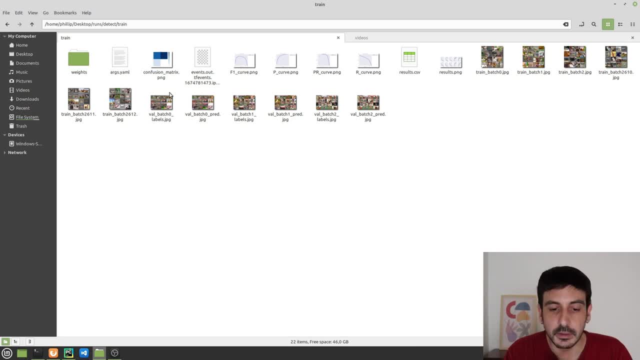 YOLOv8. so, once we have trained a model, we go to the, to this directory- remember, to the directory i showed you before regarding the directory where all the information was saved, where all the information regarding this training process was saved, and obviously i i'm not going to show you. 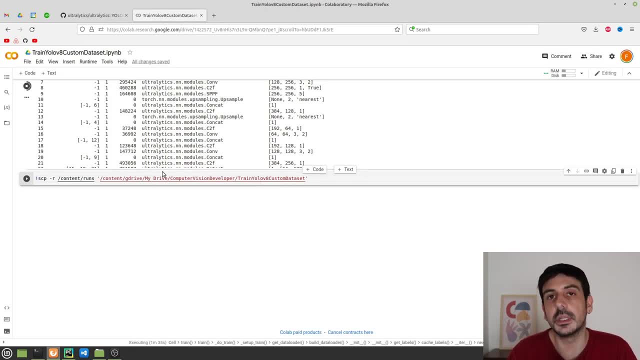 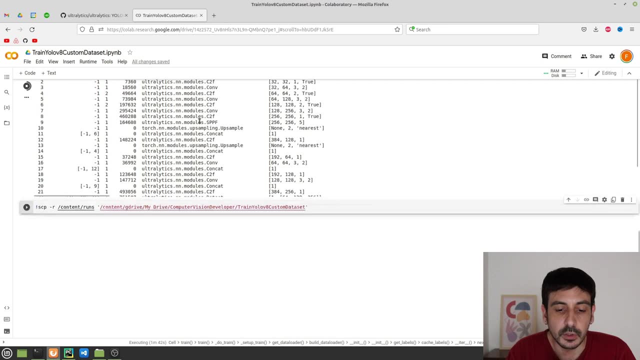 and so on. please remember to do this because otherwise you would not be able to access this data, and this is the data which contains all the results and everything you have just trained. so this is how you can train a yellow v8, an object detector, using yellow v8 in a Google. 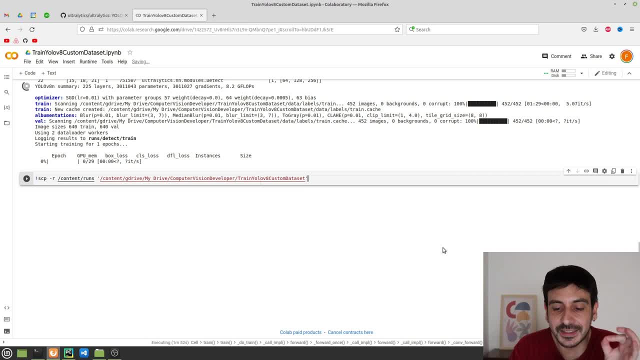 collab and you can see that the process is very straightforward and it's pretty much exactly the same process, exactly the same idea as we did in our local environment, and that's it. so that's how easy it is to train an object detector using yellow v8 once you have done everything we did. 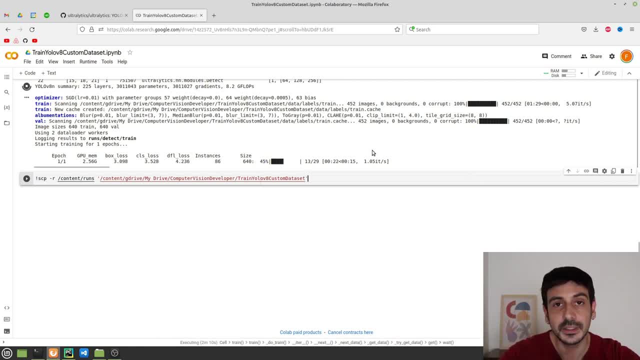 with the data right, once you have collected the data, you have annotated the data, you have written everything into the format yellow v8 needs in order to train an object detector. once everything is completed, then running this process, running this training, is super straightforward. so that's going to be all about this training process, and now let's continue with the testing. now let's. 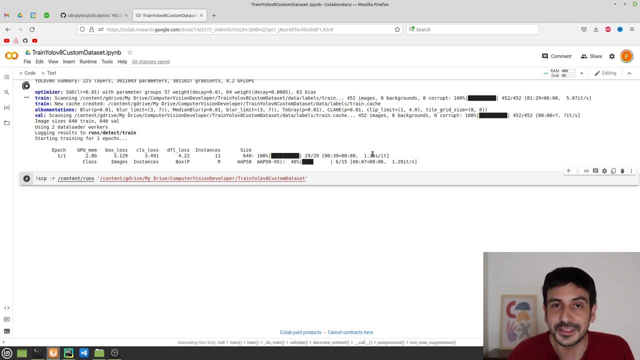 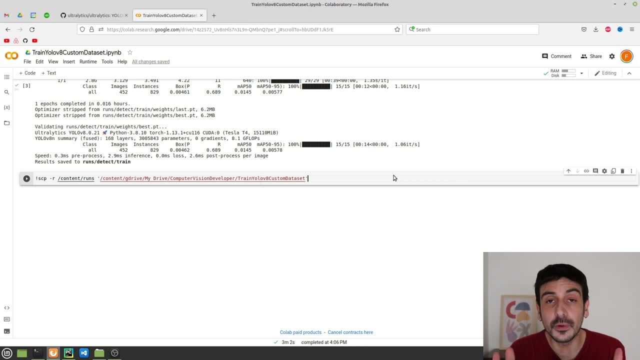 see how these models we have trained, how they performed right. let's move to the next step, and this is the last step in this process. this is where we are going to take the model we produced in the training step and we're going to test how it performs. this is the last step in this process. 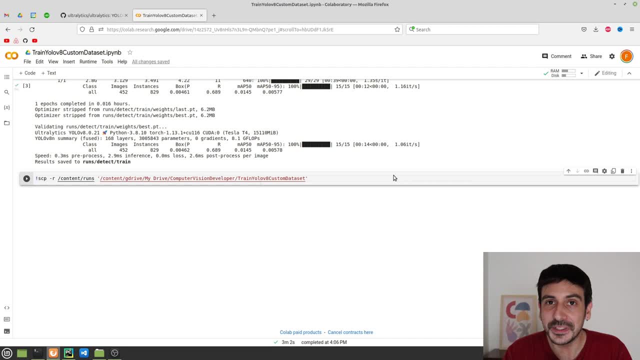 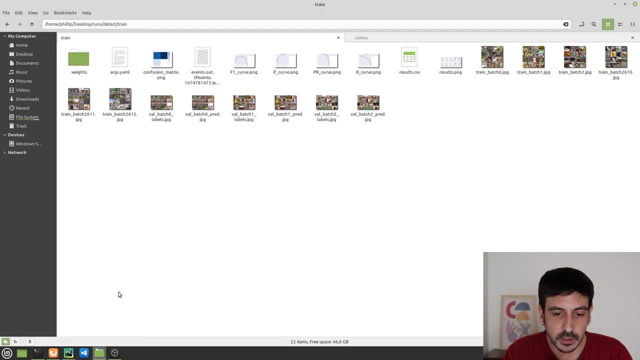 this is how we are going to complete this training of an object detector using yellow v8. so, once we have trained a model, we go to the, to this directory- remember- to the directory I showed you before regarding the directory where all the information was saved, where all the information 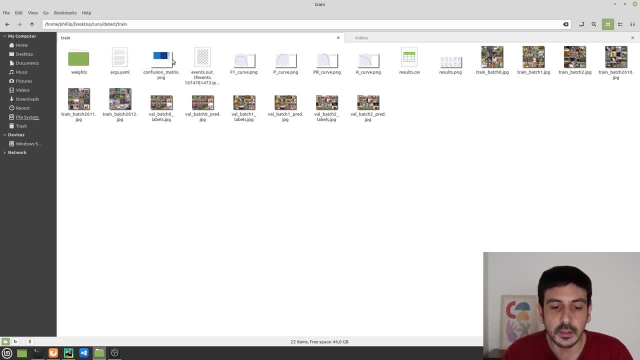 regarding this training process was saved and obviously I I'm not going to show you the training we just did, because it was like a very shallow training, like a very dummy training, but instead I'm going to show you the results from another training I did when I was preparing this. 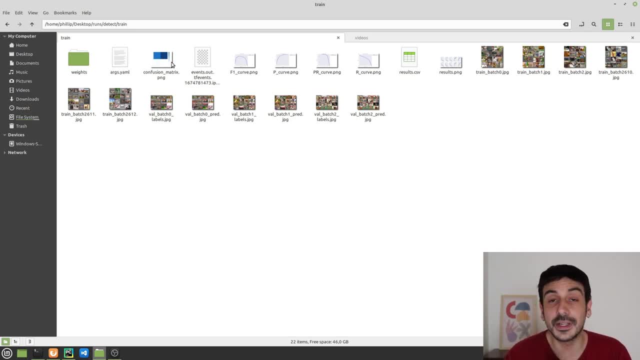 the training we just did, because it was like a very shallow training, like a very dummy training. but instead i'm going to show you the results from another training i did when i was preparing this video, where i conducted exactly the same process, but the training process was done for. 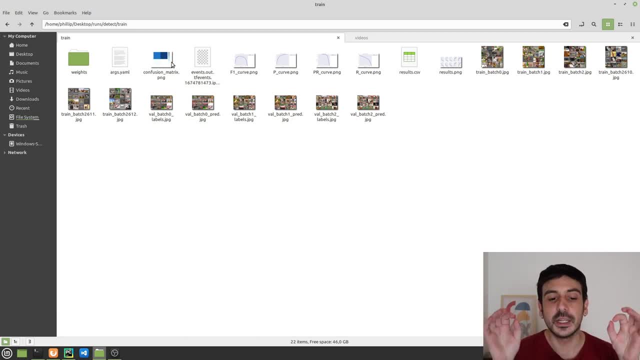 video where I conducted exactly the same process, but the training process was done for 100 Epochs, so it was like a more deeper training, right? so let me show you all the files we have produced so you know what are all the different tools you have in order to test the performance of the model. 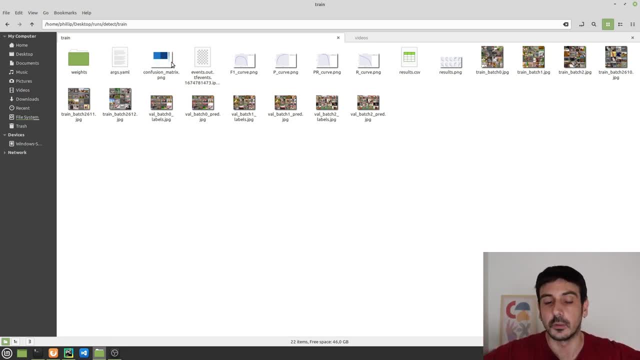 100 epochs, so it was like a more deeper training, right? so let me show you all the files we have produced so you know what are all the different tools you have in order to test the performance of the model you have trained. so basically, you have a confusion matrix which is going to give 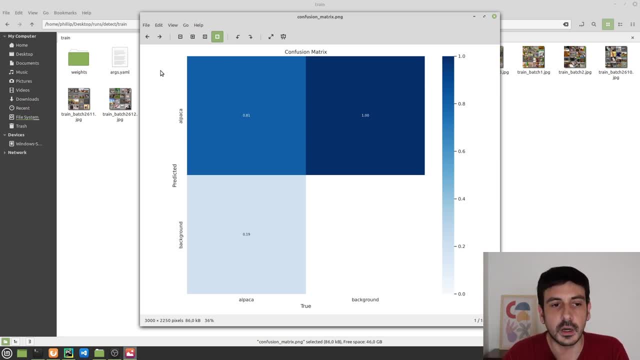 you a lot of information regarding how the different classes are predicted, or how all the different classes are confused, right? if you are familiar with how a confusion matrix looks like, or it should look like, then you will know how to read this information. basically, this is going to give you information regarding how all 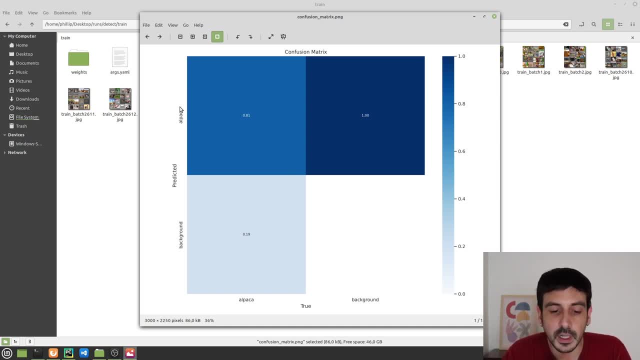 the different classes were confused. in my case, I only have one class, which is alpaca, but you can see that this generates another category which is like a default category, which is background, and we have some information here. it doesn't really say much. it says how these classes are confused, but given 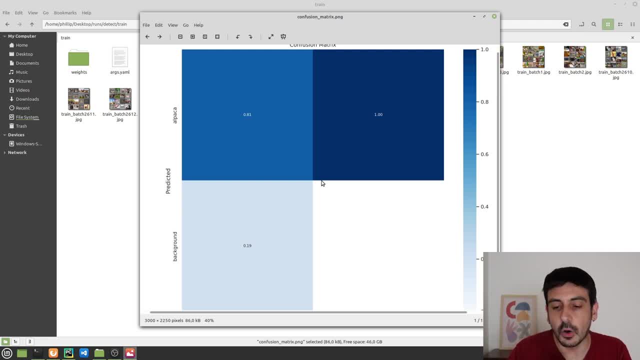 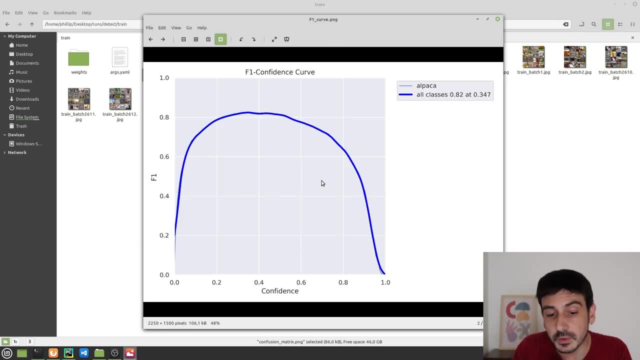 that this is an option detector. I think the most valuable information it's in other metrics, in other outputs. so we are not really going to mind this confusion matrix. then you have some plots, some curves. for example, this is the f1 confidence curve. we are not going to mind this plot either. remember, we are just starting to train up an. 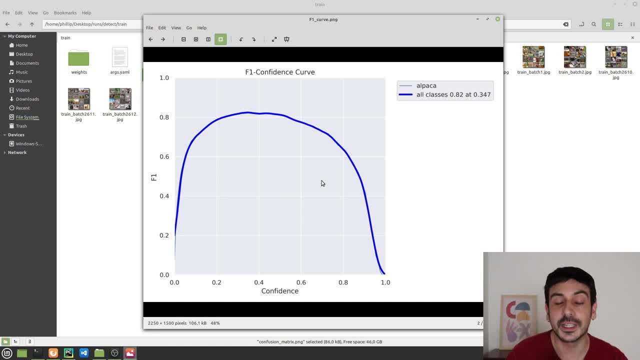 object detector using YOLOv8. the idea for this tutorial is to make it like a very introductory training, a very introductory process, so we are not going to mind in all these different plots we have over here, because it involves a lot of knowledge and a lot of expertise to extract all the information from these. 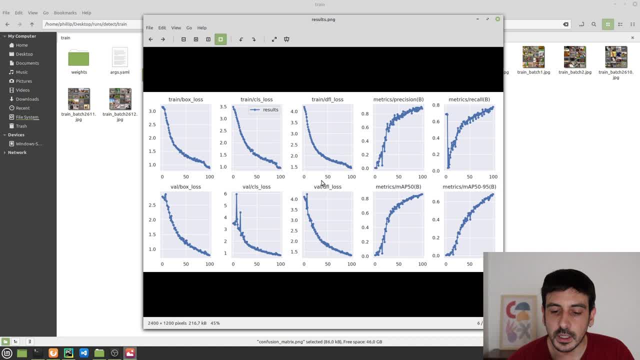 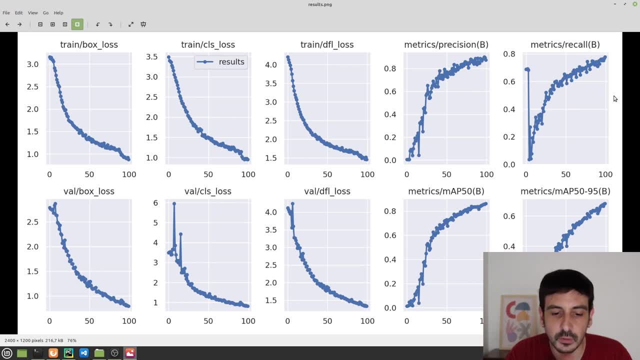 plots, and it's not really the idea for this tutorial. let's do things together. Let's do things together differently. let's focus on this plot, which is also available in the results, which were saved into this directory, and you can see that we have many, many, many. 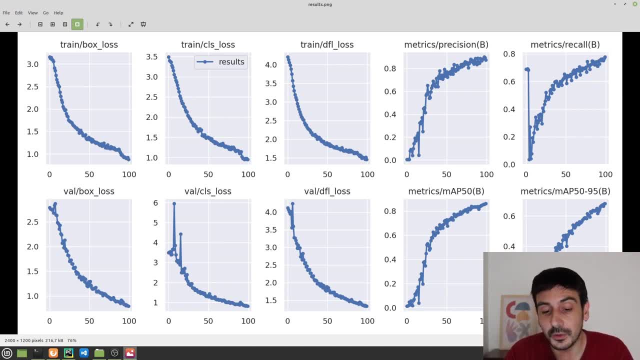 different plots. you can definitely go crazy analyzing all the information you have here, because you have one, two, three, four, five, ten different plots. you could knock yourself out analyzing and just extracting all the information from all these different plots. but again, the idea is to make it a very introductory. 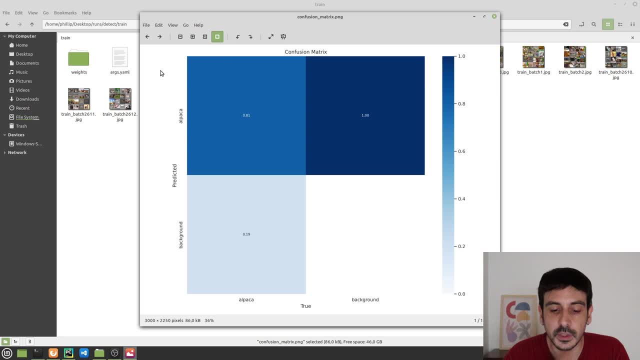 you have trained. so, basically, you have a confusion Matrix which is going to give you a lot of information regarding how the different classes are predicted, or how all the different classes are confused. right, if you are familiar with how a confusion Matrix looks like or it should look like, then you will know how. 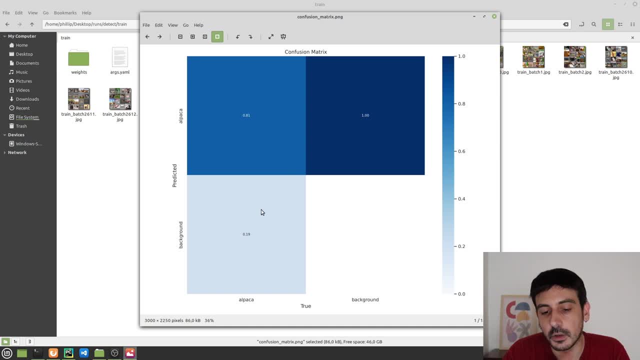 to read this information. basically, this is going to give you information regarding how all the different classes were confused. in my case, I only have one class, which is alpaca, but you can see that this generates another category which is like a default category, which is background, and we have some information here. it doesn't really say much. it says how these classes 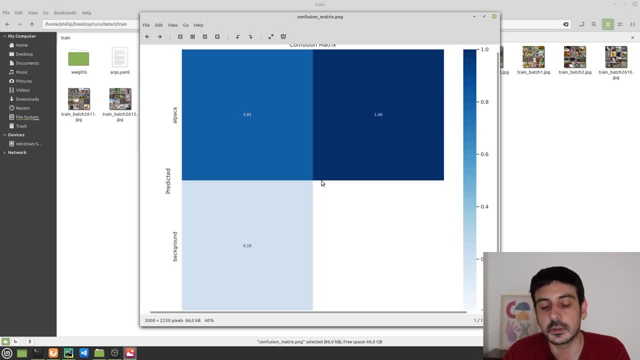 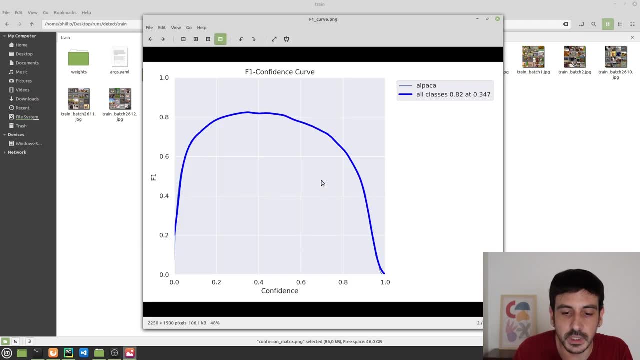 are confused. but, um, given that this is an option detector, I think the most valuable information it's in other metrics, in other outputs. so we are not really going to mind this confusion Matrix. then you have some plots, some curves. for example, this is the f1 confidence curve. we are not going to 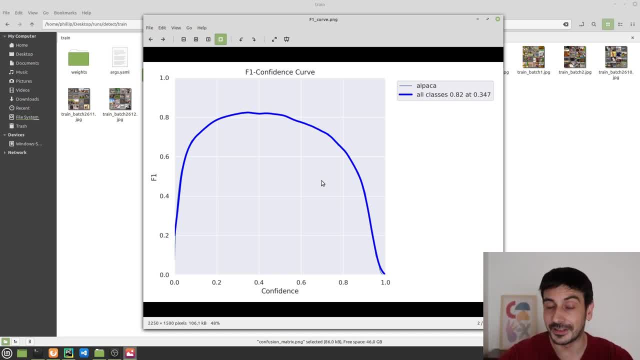 mind this plot either. remember, we are just starting to train an object detector using yellow v8. the idea for this story is to make it like a very introductory training, a very introductory process. so we are not going to mind in all these different plots we have over here, because 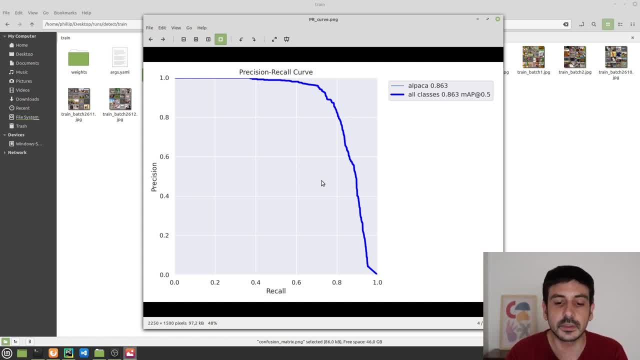 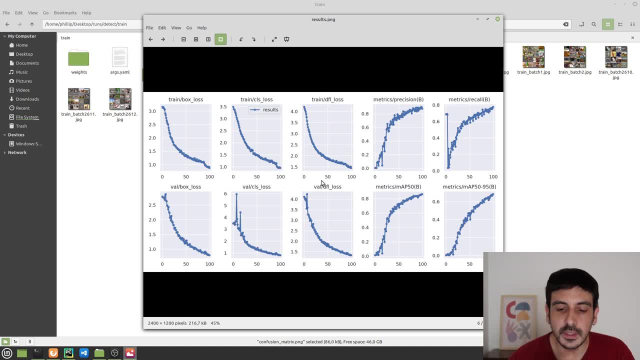 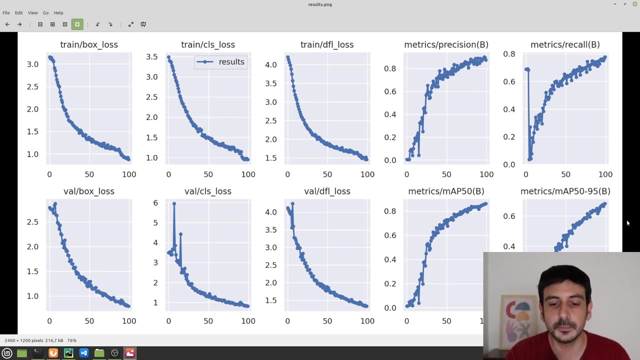 it involves a lot of knowledge and a lot of expertise to extract all the information from these plots, and it's not really the idea for this tutorial. let's do things differently. focus on this plot, which is also available in the results which were saved into this directory, and you can see that we have many, many, many different. 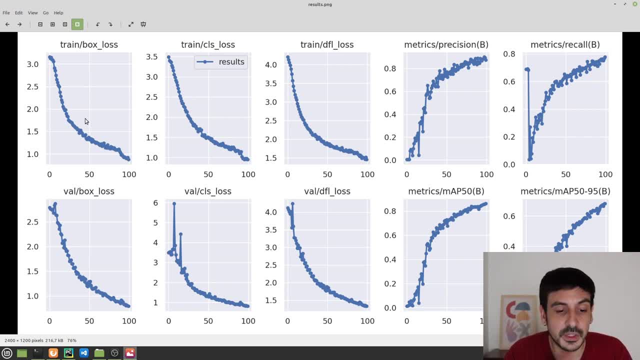 plots. you can definitely go crazy analyzing all the information you have here, because you have one, two, three, four, five, ten different plots. you could knock yourself out analyzing and just extracting all the information from all these different plots. but again, the idea is to make it a very introductory video. 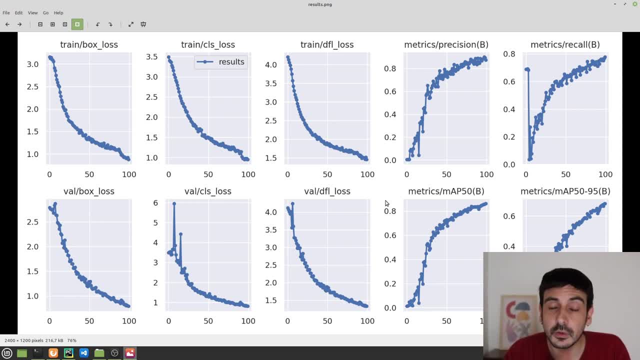 and a very introductory tutorial. so long story short. I'm just going to give you one tip of something, the one thing you should focus on these plots for now, if you're going to take something from this video, from this: how to test the performance of a model you have just trained using YOLOv8 to train an. 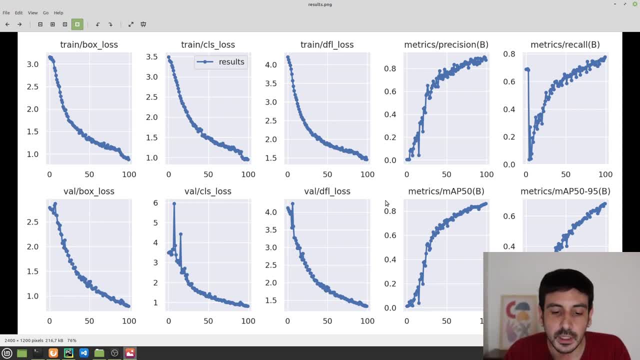 video and a very introductory tutorial. so long story short. I'm just going to give you one tip of something, the one thing you should focus on these plots for now, if you're going to take something from this video, from this: how to test the performance of a model you have just trained using YOLOv8 to train. 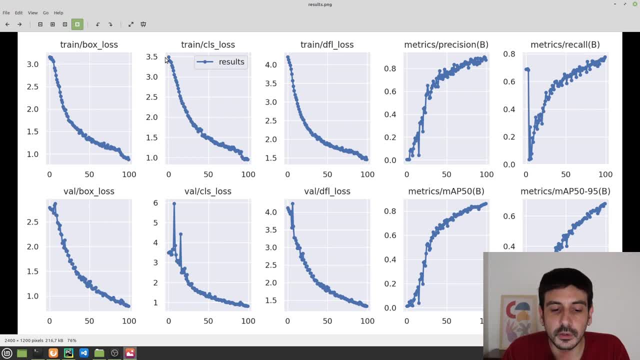 an object detector is this: make sure your loss is going down right. you have many plots. some of them are related to the loss function, so some of them are function. which are this one, this one and this one? this is for the training set and these are related for the validation set. make sure all of your losses are going down right. this is like a 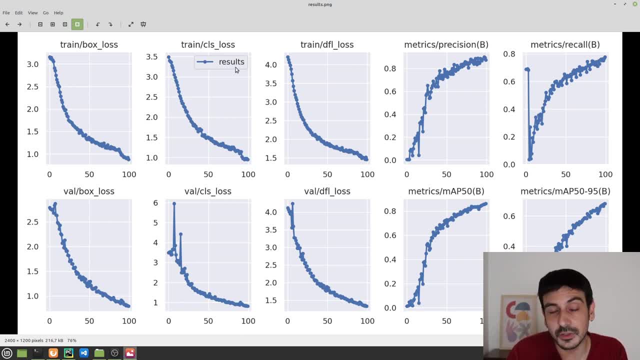 very, i would say a very simple way to analyze these functions or to analyze these plots, but that's i would say that that's more powerful, that it will appear. make sure all your losses are going down because, given the loss function, we could have many different situations. we could. 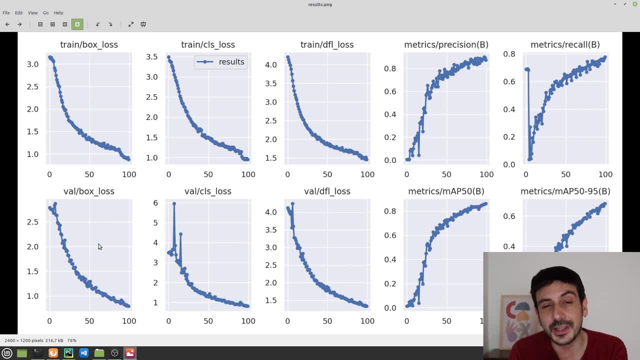 have a loss function which is going down, which i will say it's a very good situation. we could have a loss function which started to go down and then just it looks something like a flat line, and if we are in something that looks like a flat line, it means that our training process has stuck, so it 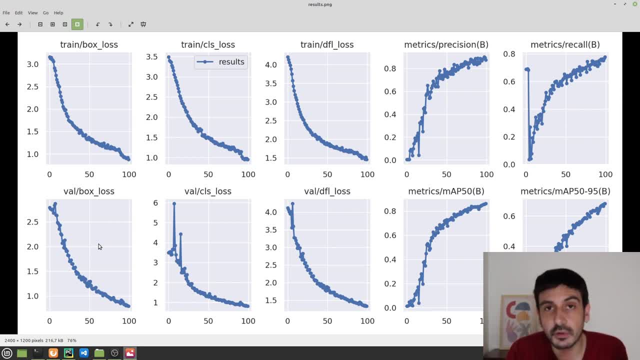 could be a good thing, because maybe the, the algorithm, the machine learning model already learned everything it had to learn about this data, so maybe a flat line is not really a bad thing. maybe, i don't know, you will have to analyze other stuff. or if you look at your loss function, you could also have a situation where your loss 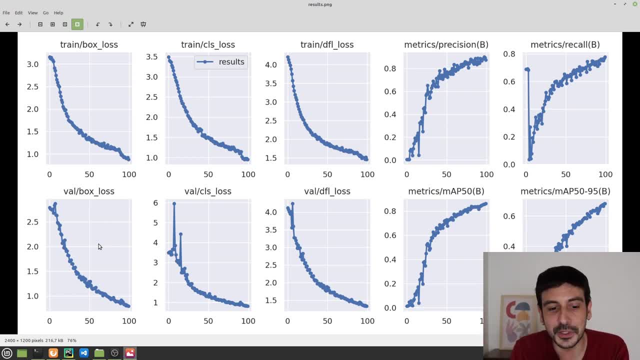 function is going up right. that's the other situation, and if you, my friend, have a loss function which is going up, then you have a huge problem. then something is obviously not right with your training and that's why i'm saying that analyzing your loss function is not a good thing. 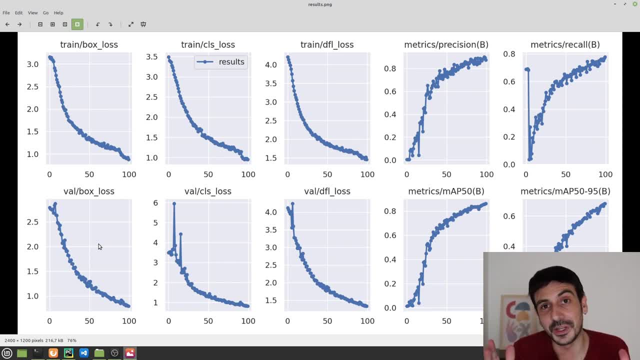 because if you have a loss function, what happens with your loss is going to give you a lot of information. ideally it should go down. if it's going down, then everything is going well. most likely. if it's something like a flat line, well, it could be a good thing or a bad thing, i don't know. 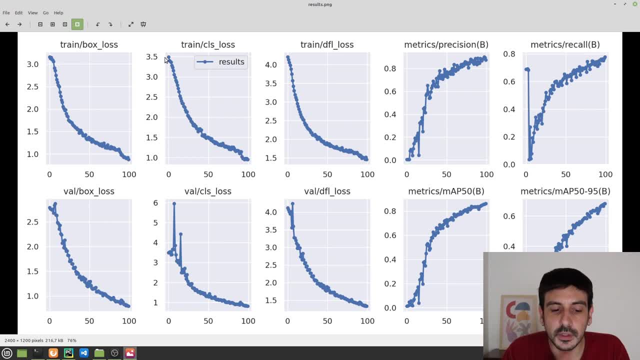 object detector is this: make sure your loss is going down right. you have a many plots. some of them are related to the loss function, which I'm going to show you in this video, and I'm going to show you how to make sure this one, this one and this one, this is for the training set and these 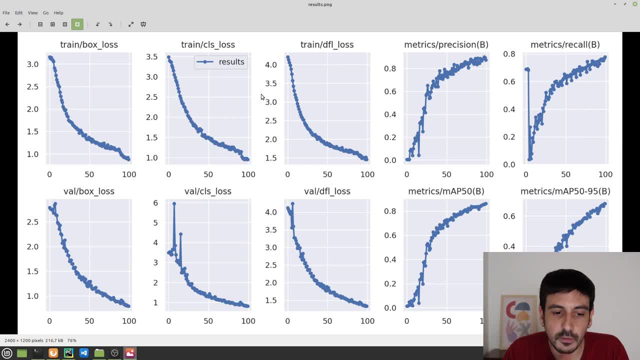 are related for the validation set. make sure all of your losses are going down. right, this is like a very- I would say a very- simple way to analyze these functions or to analyze these plots, but that's. I will say that that's more powerful that it will appear. make sure all your losses are going down, because 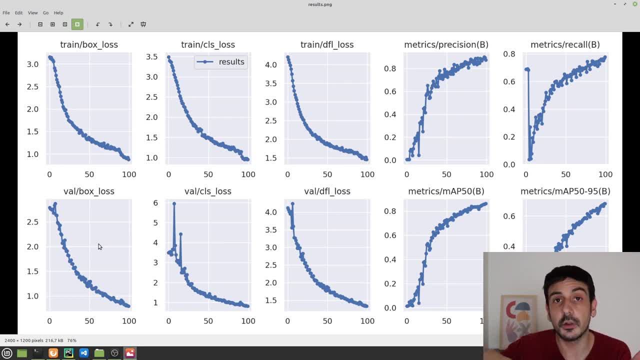 given the loss function, we can see that it's going down and it's going down. and for finding the loss function, we could have many different situations. we could have a loss function which is going down, which I will say it's a very good situation. we could have a loss function which is short to go down and then just 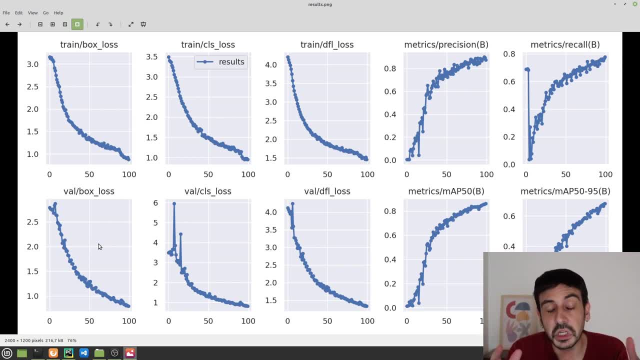 it looks something like a flatline, and if we are in something that looks like a flatline, it means that or training process has stuck. so it could be a good thing because maybe the algorithm, the machine-learning model, already learned. a flat line is not really a bad thing. maybe- i don't know, you will have to analyze other stuff. 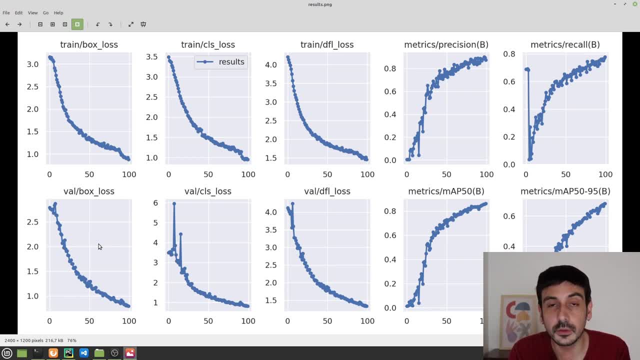 or if you look at your loss function, you could also have a situation where your loss function is going up. right, that's the other situation. and if you, my friend, have a loss function which is going up, then you have a huge problem, then something is obviously not right with your. 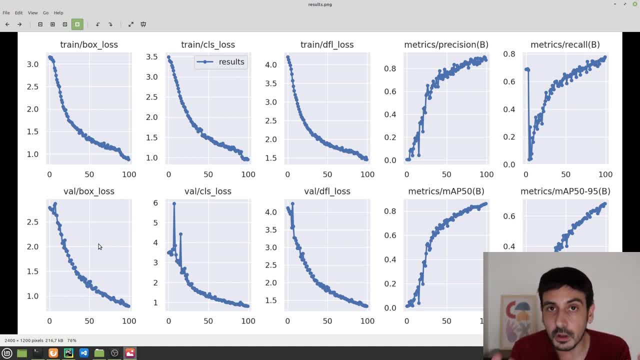 training, and that's why i'm saying that analyzing your loss function- what happens with your loss- is going to give you a lot of information. ideally it should go down. if it's going down, then everything is going well, most likely. if it's something like a flat line, well, it could be a good. 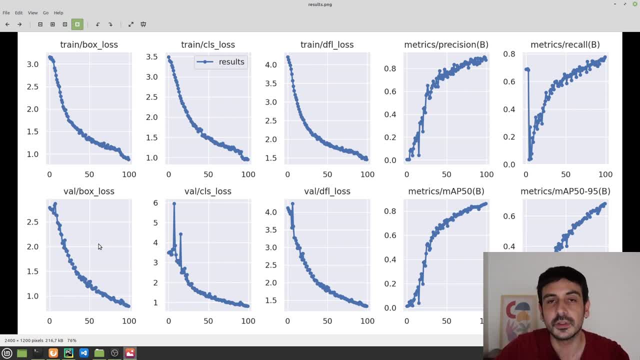 thing or a bad thing? i don't know. we could be in different situations, but if it's going up, you have done something super, super wrong. i don't know what's going on in your code. i don't know what's going on- you, your training process, but something is obviously wrong. right, so that's like a very simple and a. 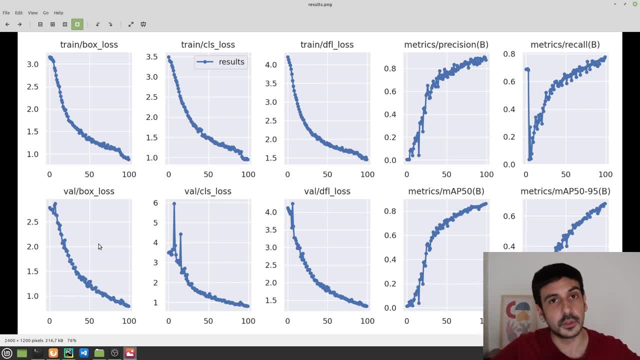 we could be in different situations, but if it's going up, you have done something super, super wrong. i don't know what's going on in your code, i don't know what's going on in your training process, but something is obviously wrong, right? so that's like a very simple and a very naive way to analyze all this information. but 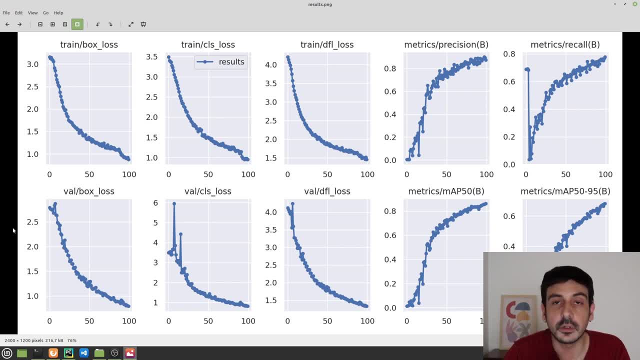 trust me, that's going to give you a lot, a lot of information in order to start working on this, testing the performance of this model. but i would say that, looking at the plots, analyzing all this information and so on, i would say that's more about research, but that's what people who do research like to do. 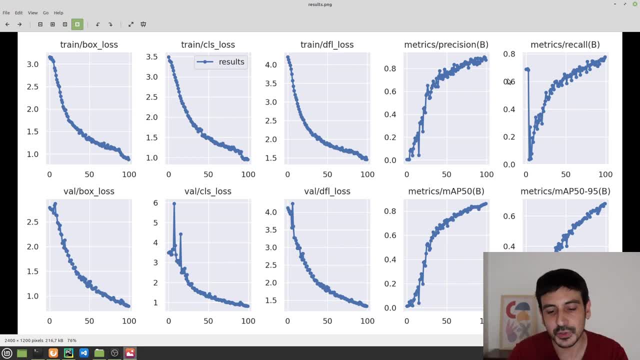 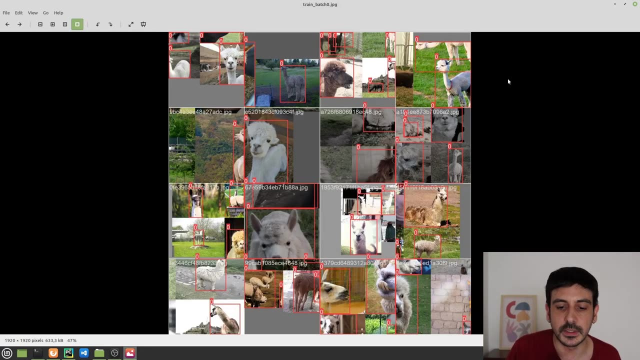 and i'm more like a freelancer. i don't really do like research, so i'm going to show you another way to analyze this performance or this, the mode we have just trained, which from my perspective, it's a more. it makes more sense to analyze it like this: 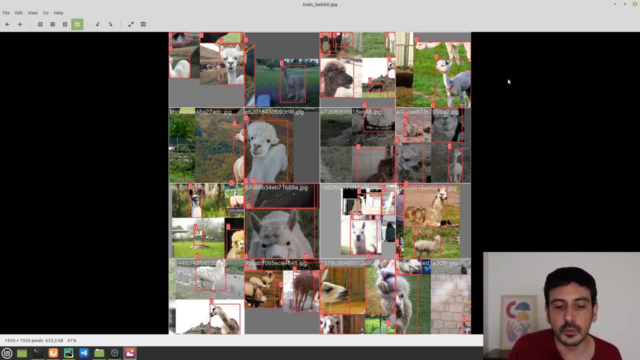 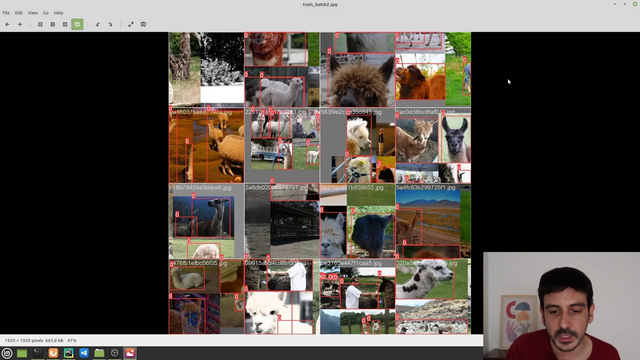 and it involves to see how it performs with real data, right, how it performs with data you have used in order to make your inferences and to see what happened. so the first step in this more practical, more visual evaluation of this model, of how this model performs, is looking at these images. 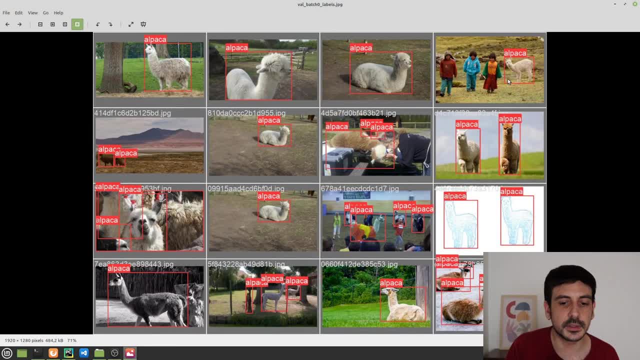 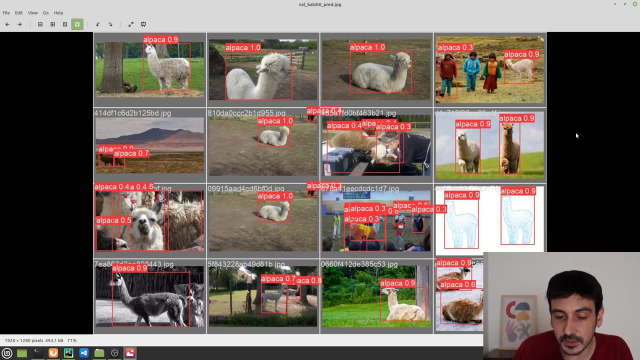 and remember that before, when we looked at these images, we had this one, which was regarding the labels in the validation set, and then this other one, which were the predictions, were completely empty. now you can see that the the predictions we have produced, they are not completely empty and we are detecting the position of our alpacas super-summing-up. 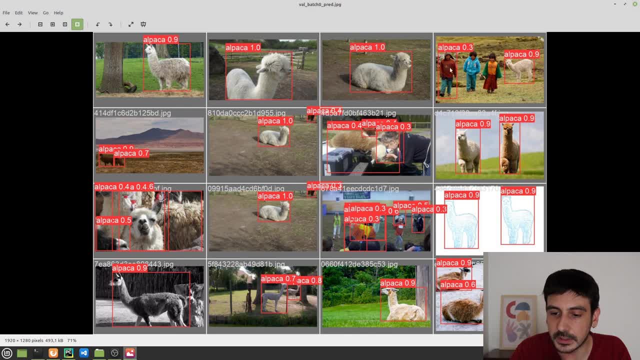 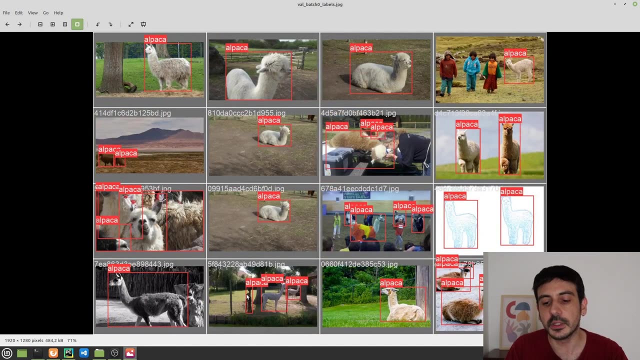 super accurately. we have some mistakes actually. for example, here we are detecting a person as an alpaca. here we are detecting also a person as an alpaca and we have some misdetections. for example, this should be an alpaca and it's not being detected. so we have some misdetections. 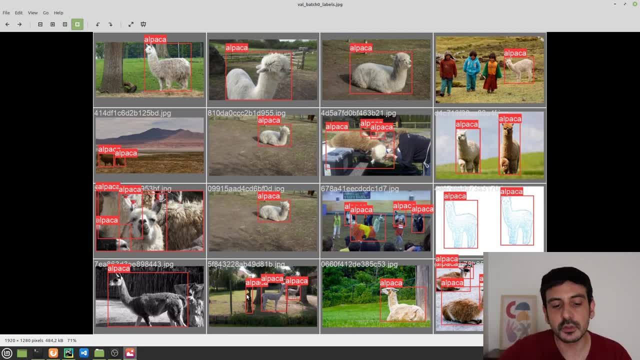 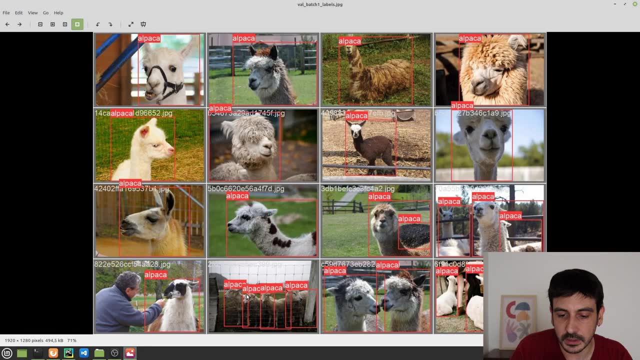 but you can see that the the results are pretty much okay. right, everything looks pretty much okay. the same about here. if we go here, we are detecting pretty much everything. we have a misdetection here. we have an error over here because we are detecting an alpaca where there's 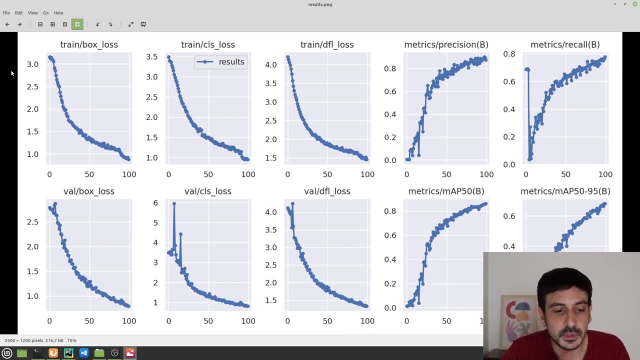 very naive way to analyze all this information, but, trust me, that's going to give you a lot, a lot of information in order to start working on this, testing the performance of this model. but i will say that, looking at the plots, analyzing all this information and so on. 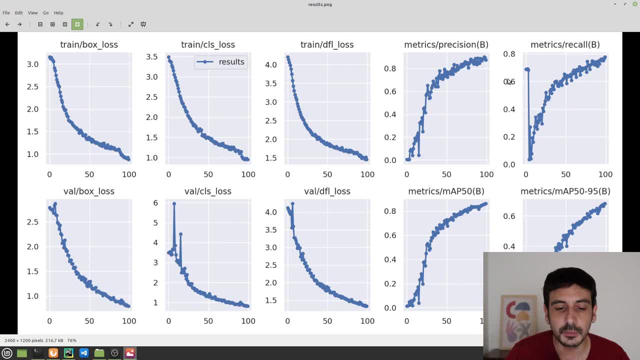 i will say that's more about research, but that's what people who do research like to do, and i'm more like a freelancer. i don't really do like research. so i'm going to show you another way to analyze this performance, or this, the model we have just trained, which, from my perspective, 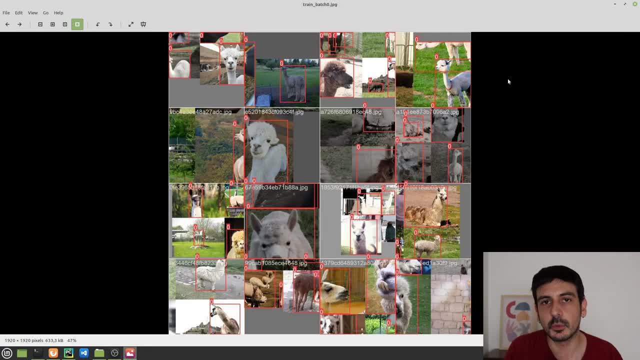 it's a more. it makes more sense to analyze it like this, and it involves to see how it performs with real data, right, how it performs with data you have used in order to make your inferences and to see what happened. so the first step in this more practical, more visual evaluation of this model, of how this 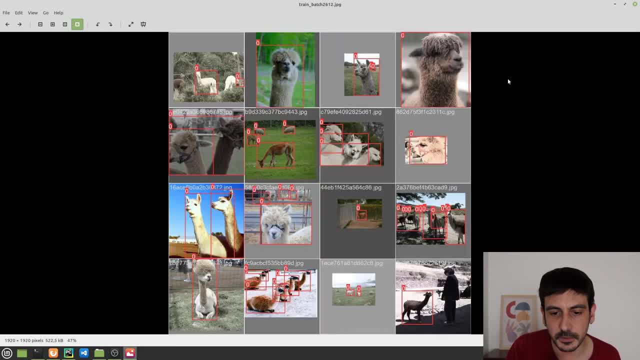 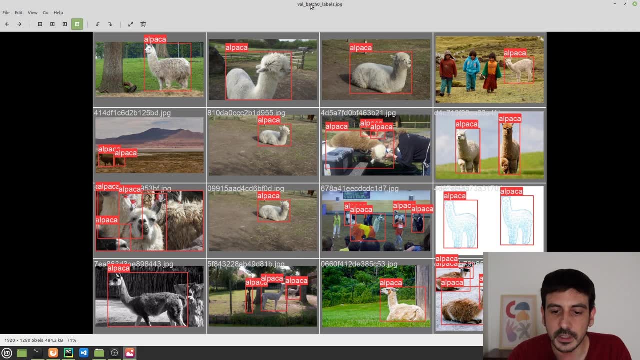 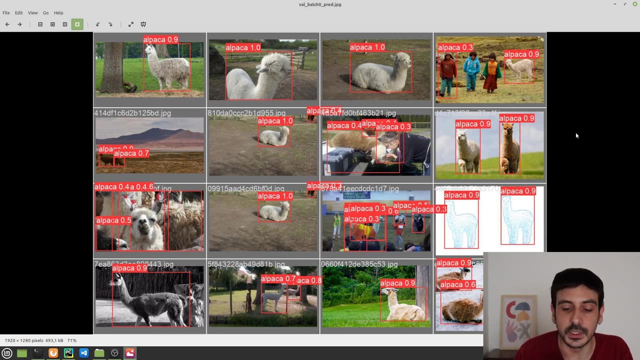 model performs is looking at these images and remember that before, when we looked at these images, we had this one which was regarding the labels in the validation set, and then this other one which were the predictions, were completely empty. now you can see that the the predictions we have produced- they are not completely empty and we 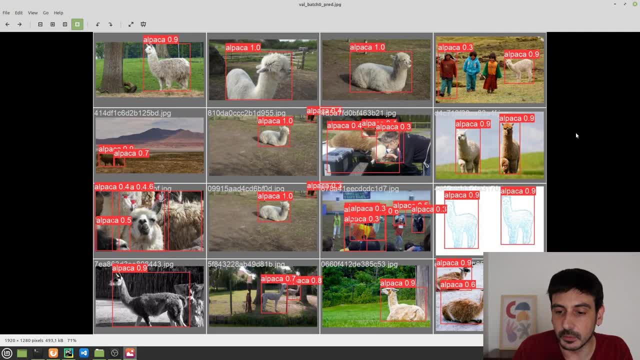 are detecting the position of our alpacas super, super accurately. we have some mistakes actually. for example, here we are detecting a person as an alpaca, here we are detecting also a person as an alpaca and we have some misdetections. for example, this should be an alpaca and it's not being. 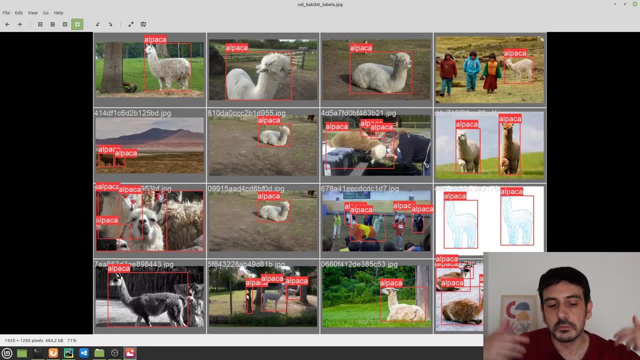 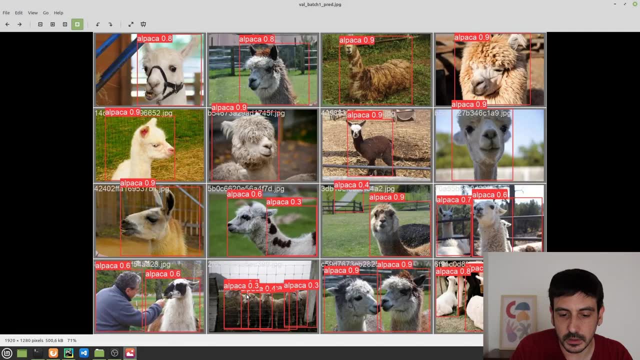 detected. so we have some misdetections, but you can see that the the results are pretty much okay, right, everything looks pretty much okay. the same about here. if we go here, we are detecting pretty much everything. we have a misdetection here. we have an error over here. 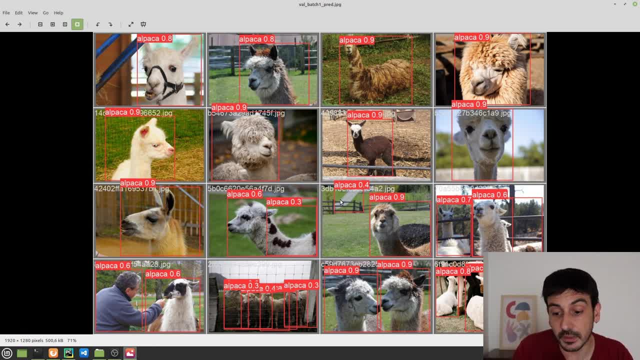 because we are detecting an alpaca where there's actually nothing. so things are not perfect, but everything seems to be pretty much okay. that's the first way in which we are going to analyze the performance of this model, which is a lot, because it's like a very visual way to see how it performs. 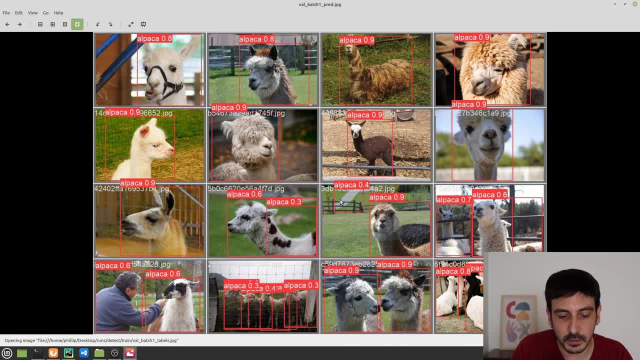 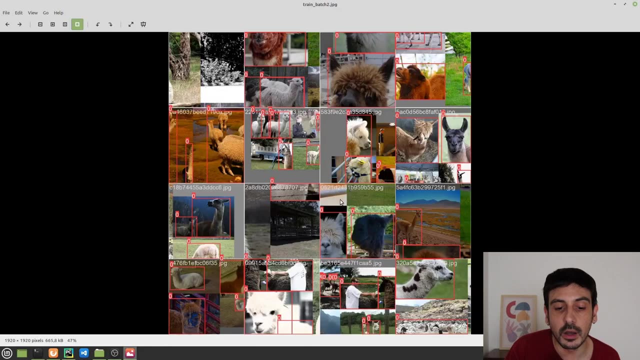 actually nothing, so things are not perfect, but everything seems to be pretty much okay. that's the first way in which we are going to analyze the performance of this model, which is a lot, because it's like a very visual way to see how it performs. we are not looking at plots, we are not looking at 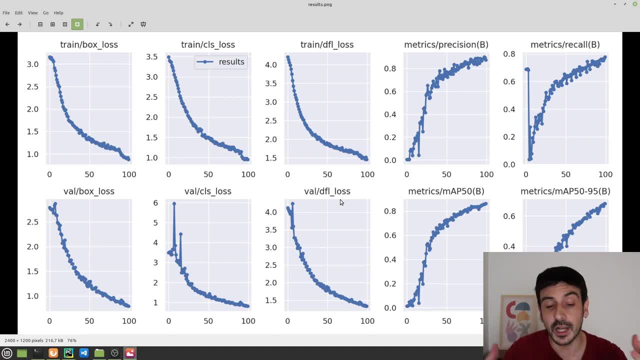 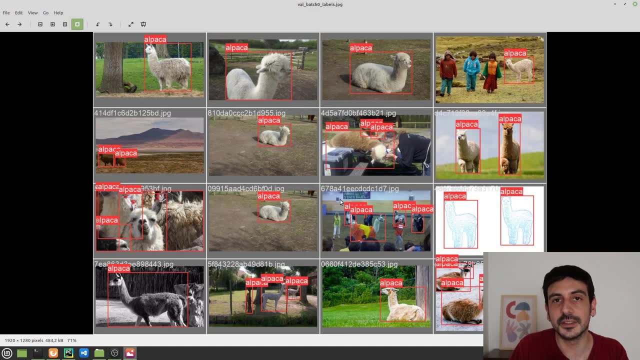 metrics right. we are looking at real examples and to see how this model performs on real data. maybe i am biased to analyze things like this, because i'm a freelancer and the way it usually works when you are a freelancer is that if you are building this model to deliver this project. 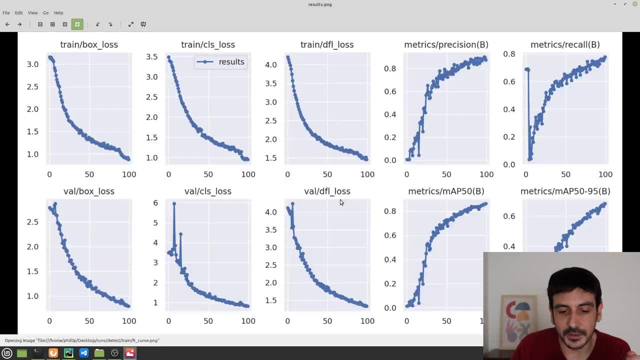 for a client and you tell your client: oh yeah, the model was perfect. take a look at all these plots, take a look at all these metrics. everything was just amazing. and then your client tests the model and it doesn't work. the client will not care about all the pretty plots, and so on, and so on. 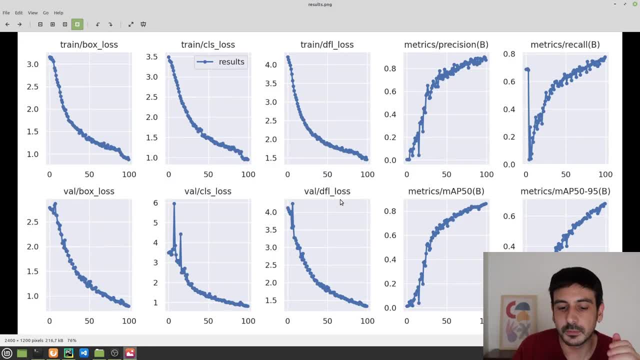 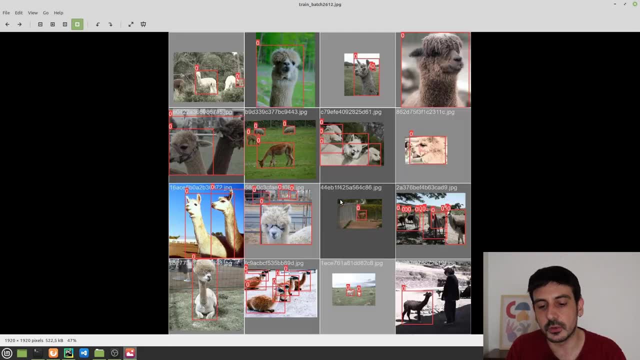 right. so that's why i don't really mind a lot about these plots. maybe i am biased because i am a freelancer and that's how freelancing works, um, but i prefer to do like a more visual evaluation. so that's the first step we will do and we can notice already we are having a better performance. 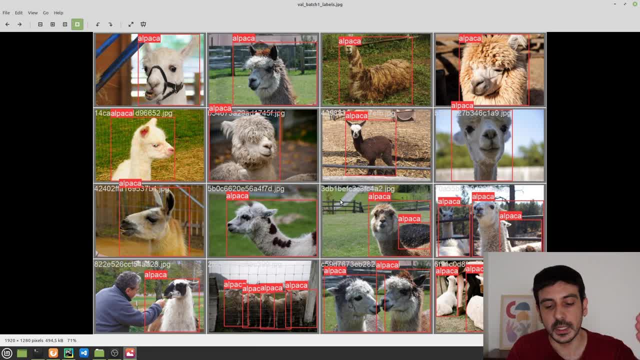 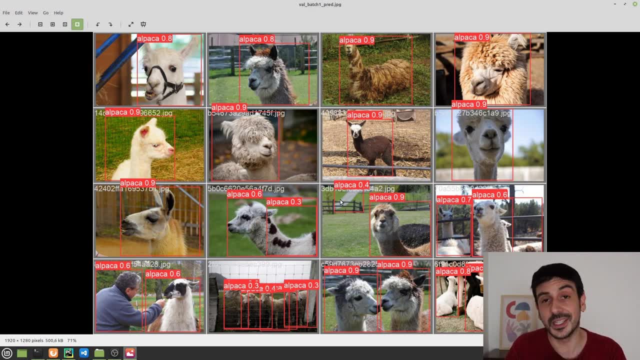 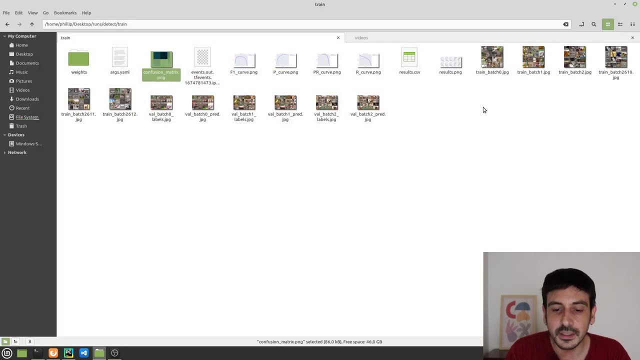 we are having an okay performance, but this data we are currently looking at right now- remember the validation data. it was pretty much the same data we use as training, so this doesn't really say much. i'm going to show you how it performs on data which the algorithm 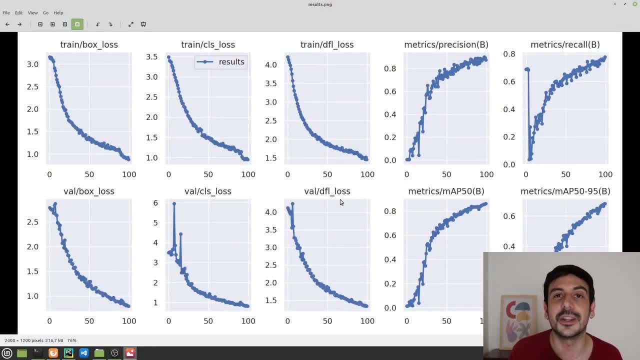 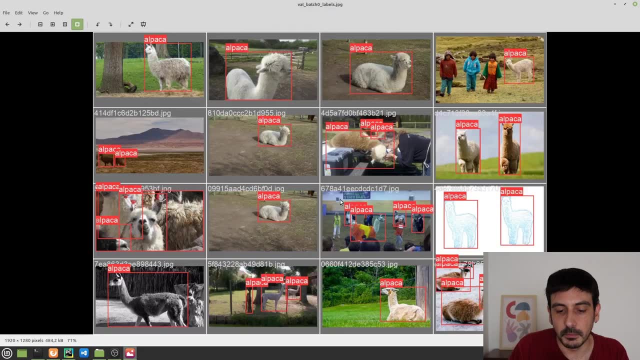 we are not looking at plots. we are not looking at metrics, right, we are looking at real examples and to see how this model performs on real data. maybe i am biased to analyze things like this, because i'm a freelancer and the way it usually works when you are a freelancer is that 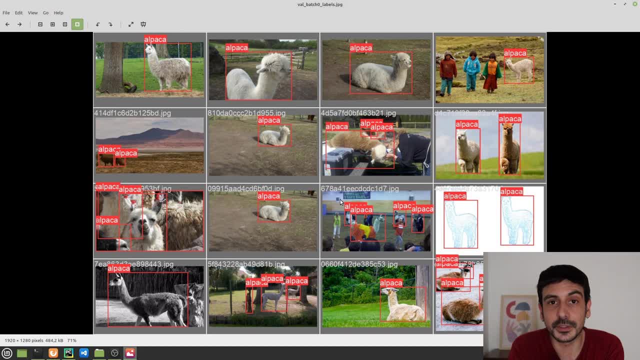 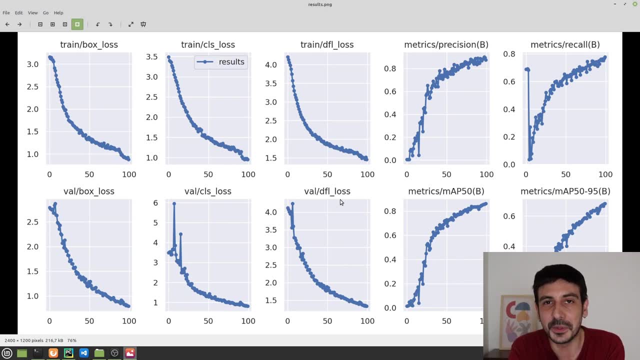 if you are building this model to deliver this project for a client and you tell your client: oh yeah, the model was perfect, take a look at all these plots, take a look at all these metrics, everything was just amazing. and then your client tests the model and it doesn't work. 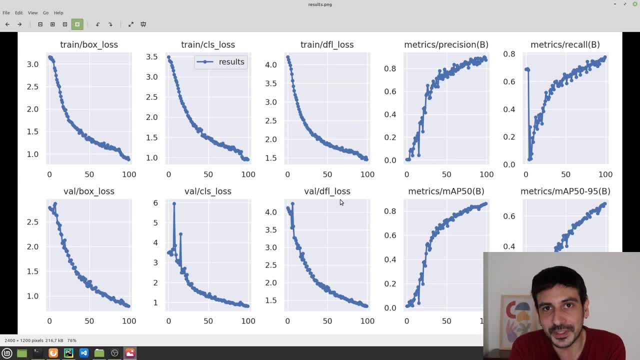 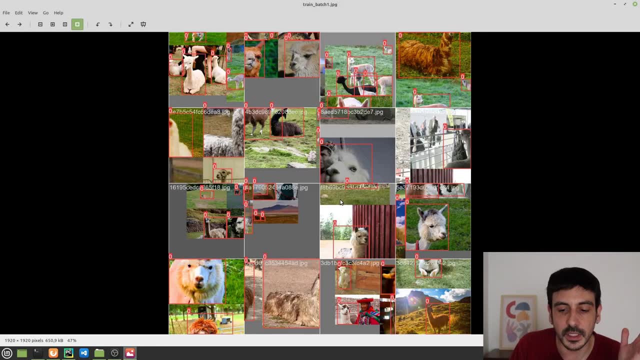 the client will not care about all the pretty plots and so on, right, so that's why i don't really mind a lot about these plots. maybe i am biased because i am a freelancer and that's how freelancing works, but i prefer to do like a more visual evaluation. so that's the first step we will. 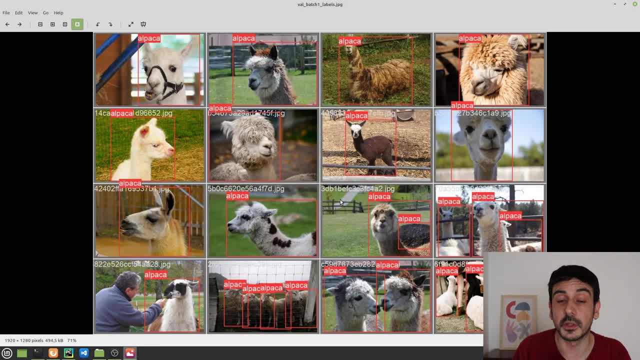 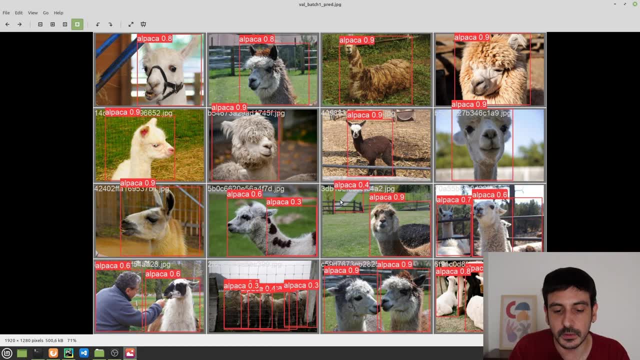 do and we can notice already we are having a better performance, we are having an okay performance. but this data we are currently looking at right now, remember the validation data. it was pretty much the same data we use as training, so this doesn't really say much. i'm going to show you. 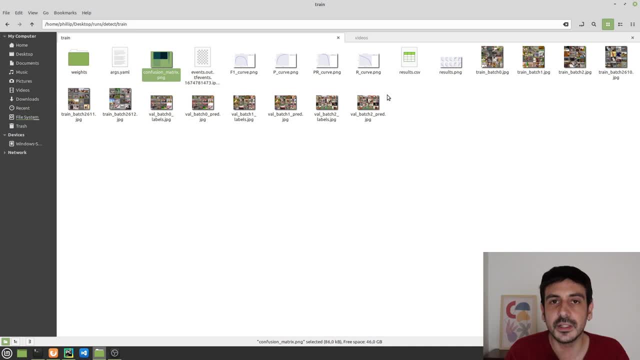 how it performs on data which the algorithm have never seen, with completely and absolutely unseen data, and this is a very good practice if you want to test the performance of a model. so i have prepared a few videos, so let me show you these videos. they are basically that. remember, this is. 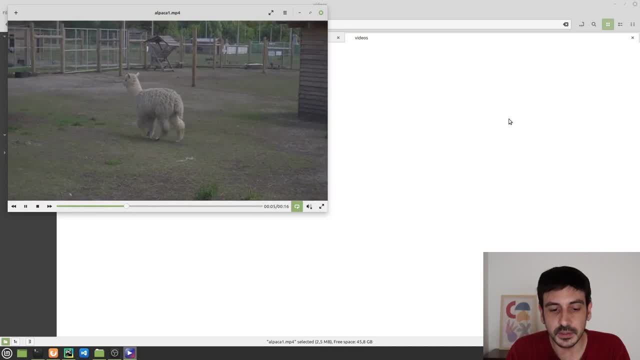 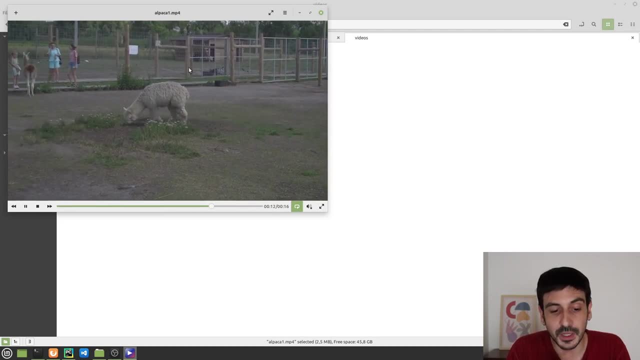 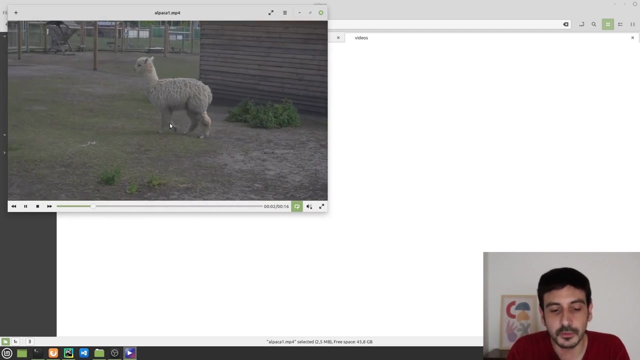 completely unseen data and this is the first video. you can see that this is an alpaca which is just being an alpaca, which is just walking around. it's doing its alpaca stuff, it's having an alpaca everyday life. it's just being an alpaca, right. it's walking around from. 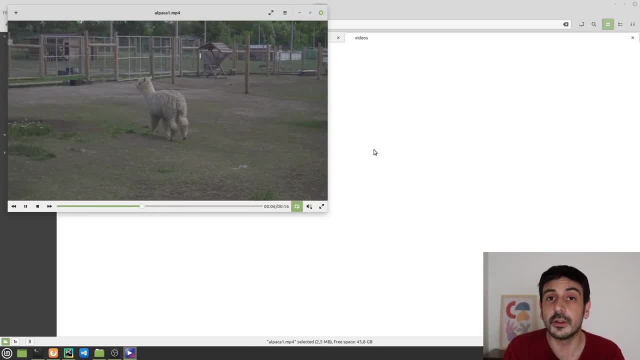 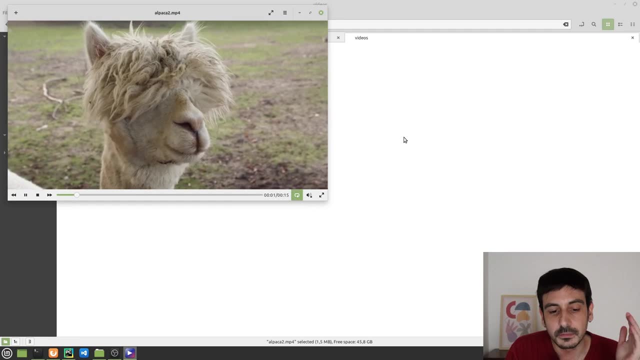 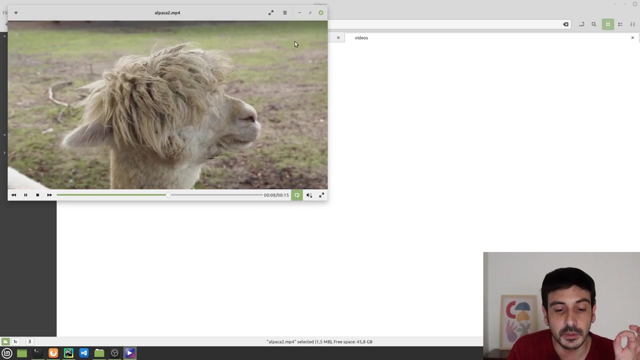 one place to the other doing a doing nothing. now it's doing its alpaca stuff, which is a lot. this is one of the videos i have prepared. this is another video which is also alpaca, doing alpaca related stuff. so this is another video we are going to see. remember this. 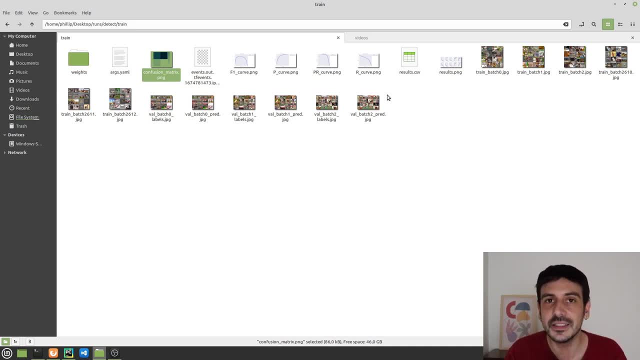 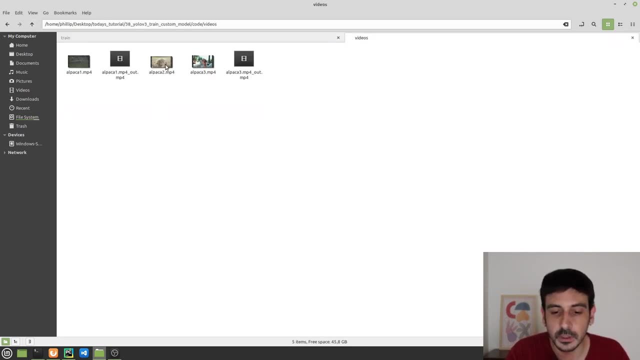 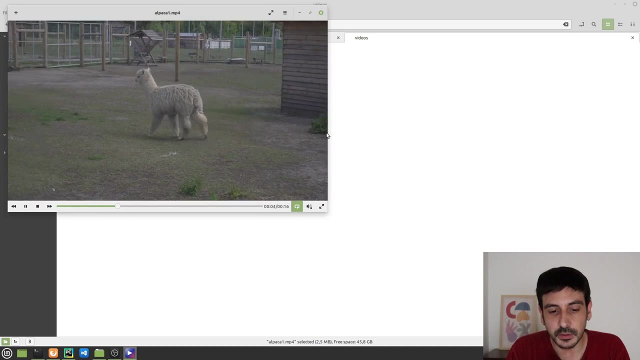 have never seen, with completely and absolutely unseen data, and this is a very good practice if you want to test the performance of a model. so i have prepared a few videos, so let me show you these videos. they are basically, remember, this is completely unseen data and this is the first video. 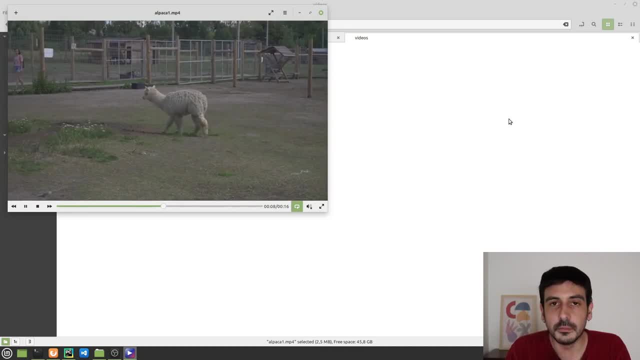 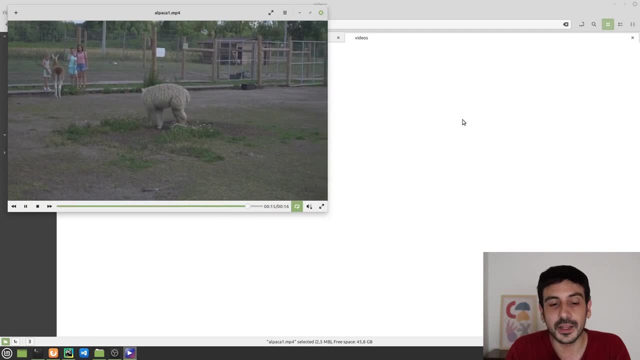 you can see that this is an alpaca which is just being an alpaca, which is just walking around, it's doing its alpaca stuff, it's having an alpaca everyday life. it's just being an alpaca, right it's. 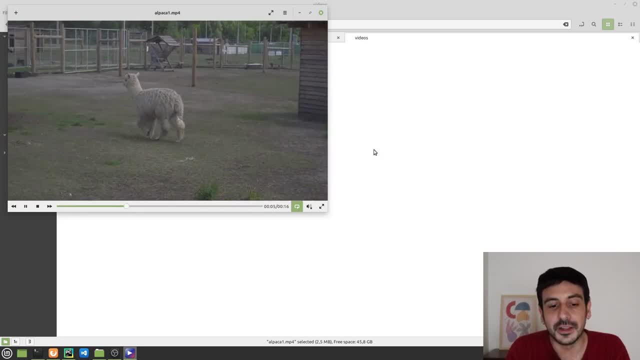 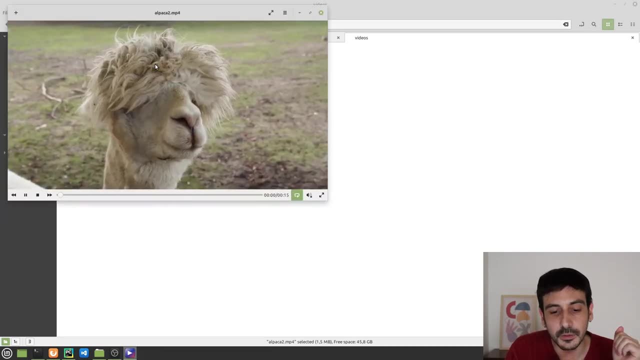 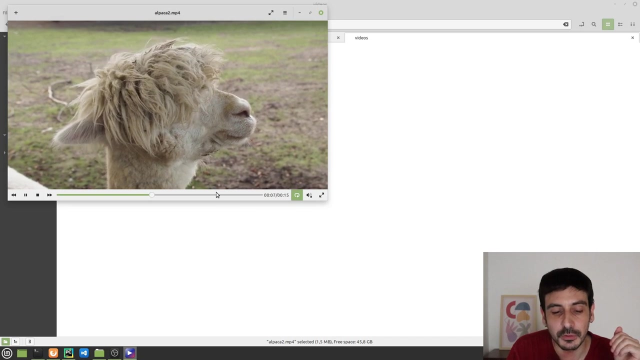 walking around from one place to the other, doing, uh, doing nothing. no, it's doing its alpaca stuff, which is a lot. this is one of the videos i have prepared. this is another video, which is also an alpaca, doing alpaca related stuff. um, so this is another video we are going to see. 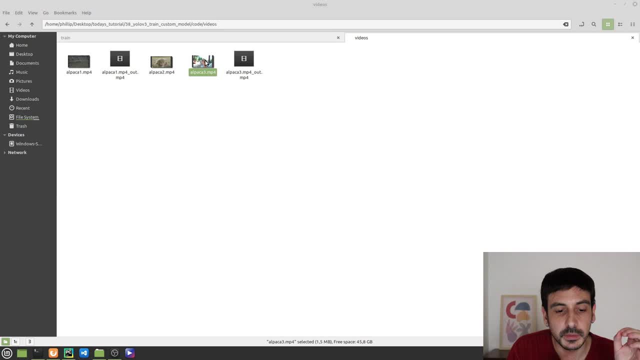 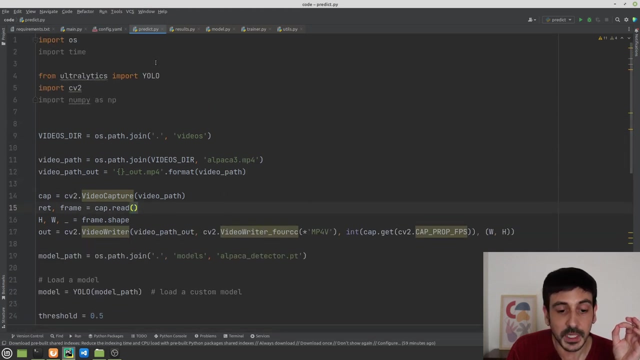 remember this is completely unseen data and i also have another video on the alpaca stuff over here, so i'm going to show you how this model perform on these three videos. i have made a script in python which loads these videos and just calls the predict uh metal from yellow, from yellow v8. we. 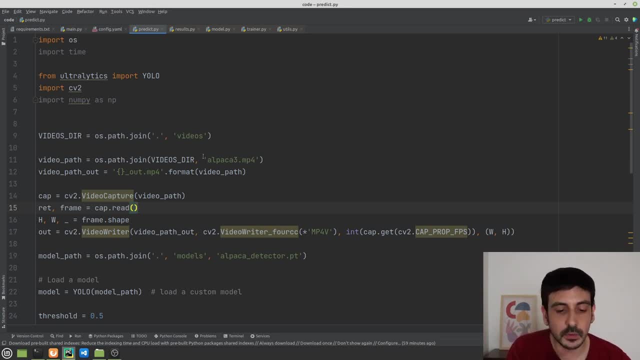 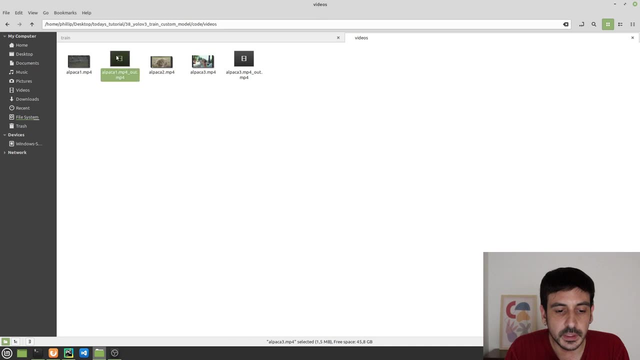 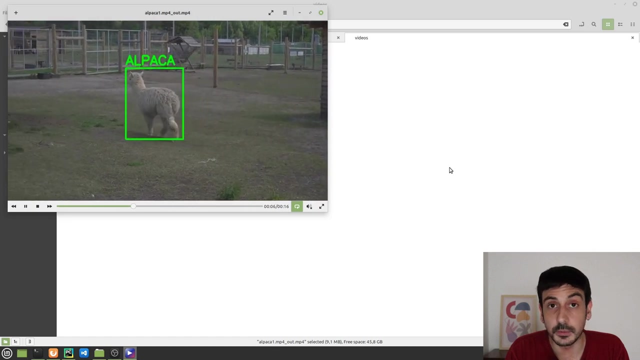 are loading the model we have trained and we are applying all the predictions to this model and we are seeing how it performs on these videos. so this is the first video i show you and these are the are getting. you can see we are getting an absolutely perfect detection. remember, this is 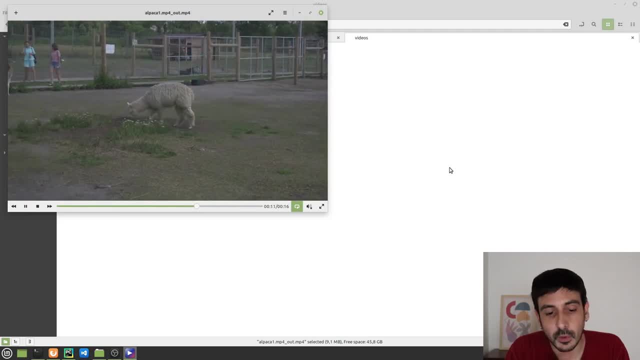 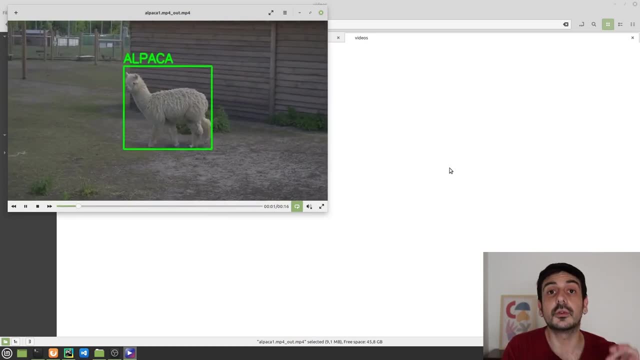 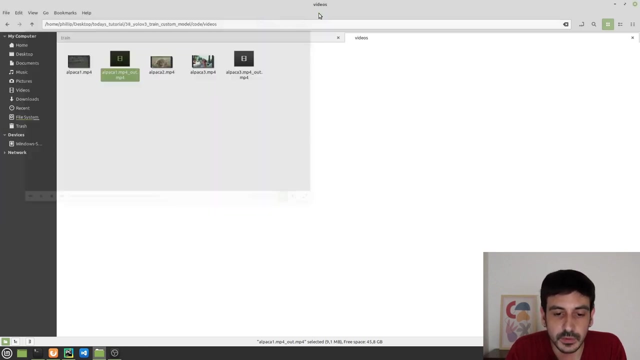 completely unseen data and we are getting- i'm not going to say a 100 perfect detection, because we are not, but i would say it's pretty good. i would say it's pretty, pretty good in order to start working on this training process. yeah, i would say it's pretty good. so this is one of the examples. 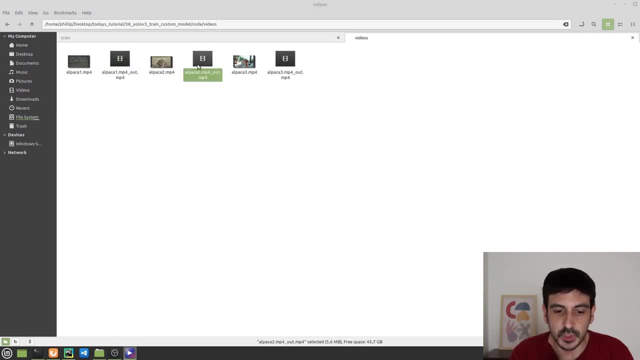 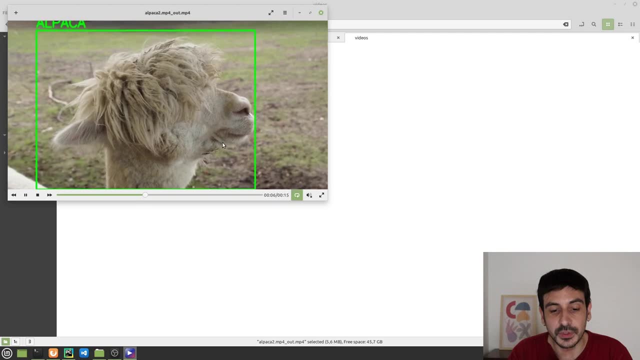 then let me show you another example, which is this one and this is the other video i show you, and you can see that we are also detecting exactly the position of the alpaca. in some cases the text is going outside of the frame because we don't really have space, but 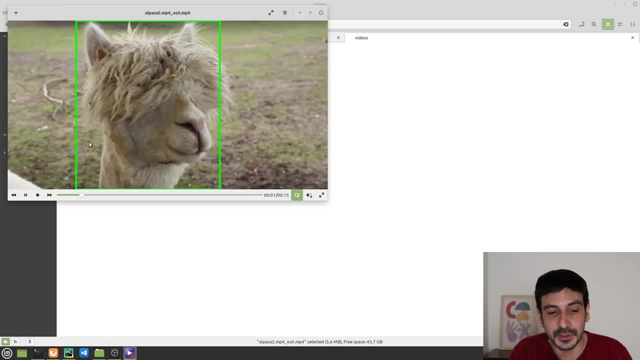 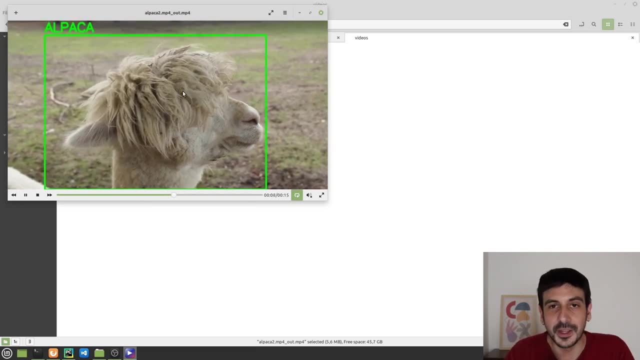 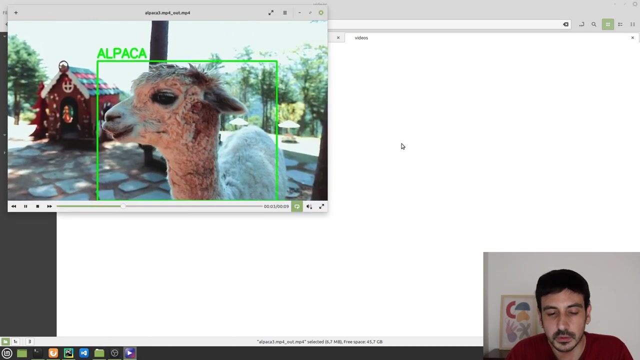 everything seems to be okay in this video too. so we are detecting exactly the position of this alpaca, the bonding box in some cases not really fit to the alpaca face, but yeah, but everything seems to be working fine. and then the other video i show you. you can see, in this case, the detection. 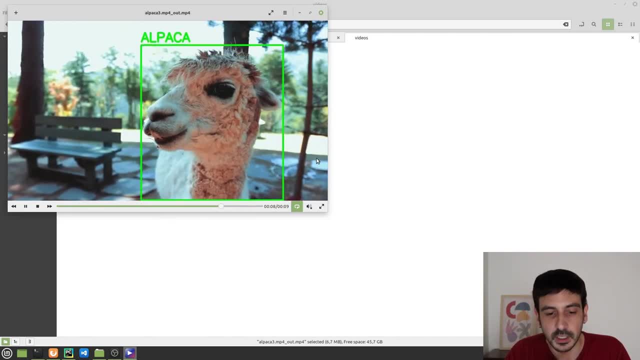 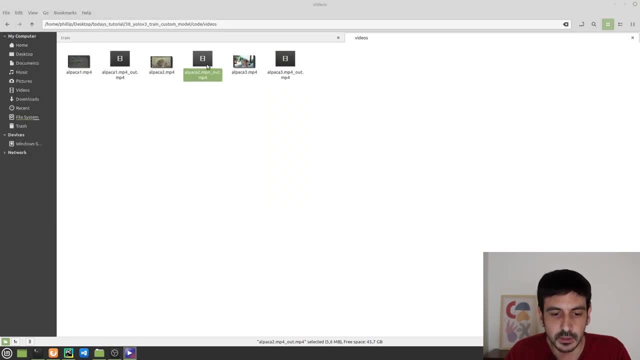 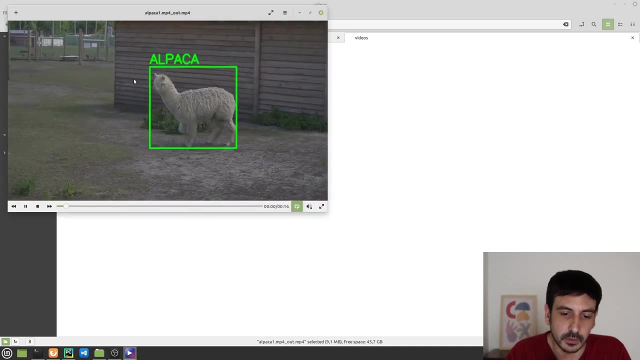 is broken. we have many miss detections, but now everything is much better and, yeah, in this case it's working better too. it's working well. i would say, in these three examples, this one, it's the one that's performing better, and then the other one i really like how it performed too in this case. 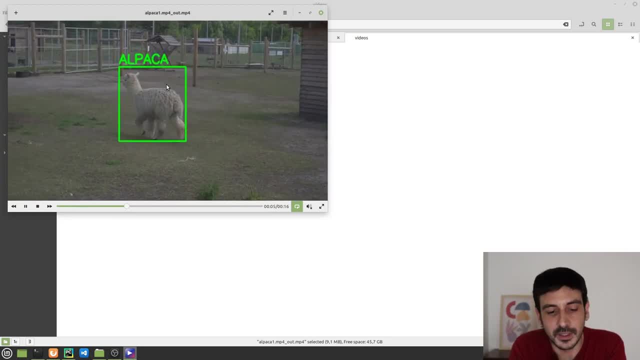 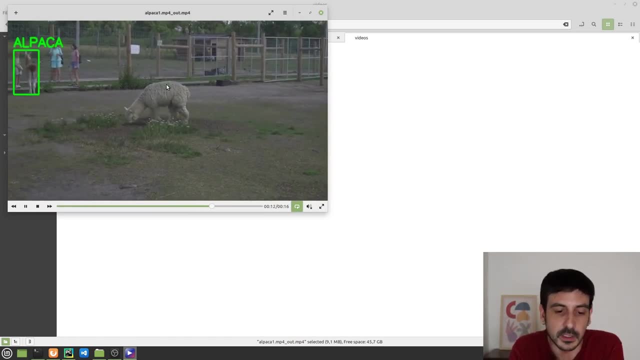 where the alpaca was like starting its alpaca journey. um, and yeah, we, we had like a very good detection and a very stable detection. then it like breaks a little but nevertheless i would say it's okay. it's also detecting this alpaca over here. 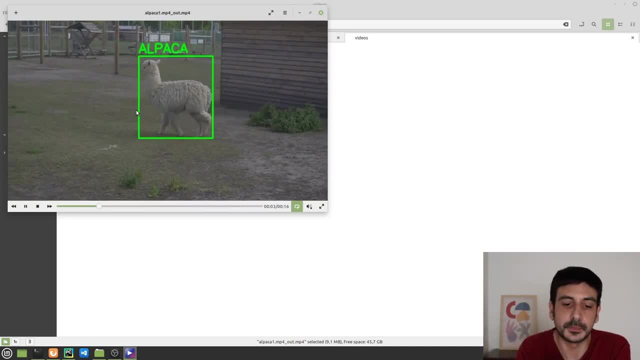 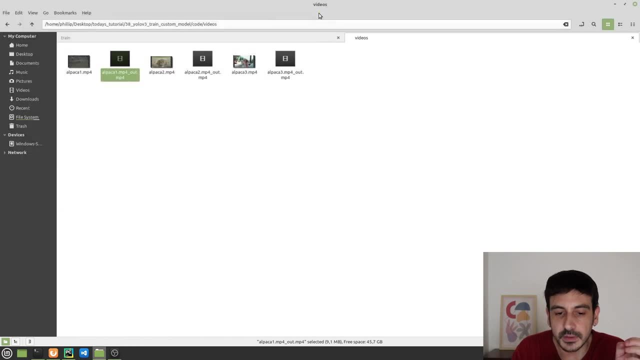 so i would say it's working pretty much okay. so this is pretty much how we are going to the testing in this phase. remember that if you want to test the performance of the model you have just trained using yolo v8, you will have a lot. 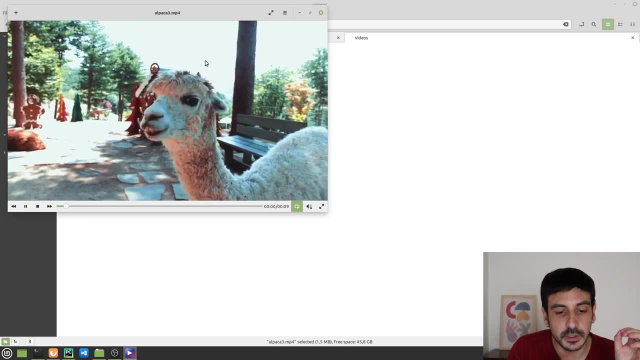 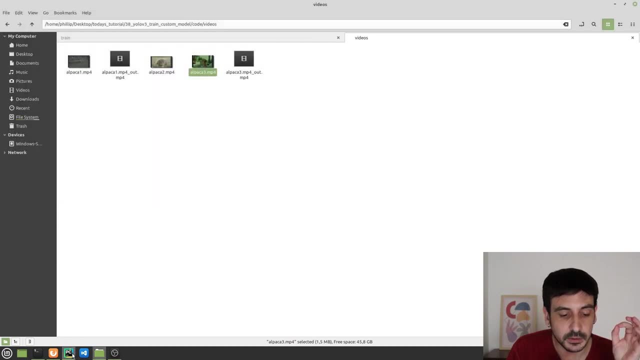 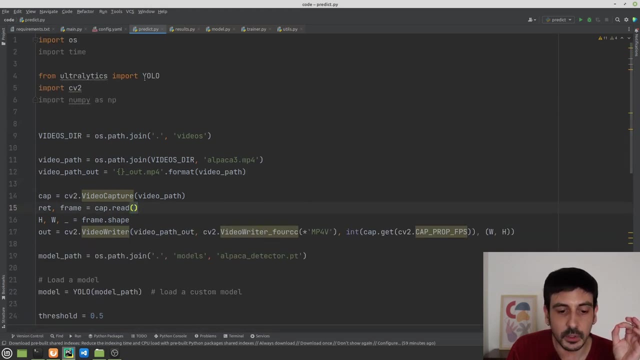 completely unseen data, and i also have another video over here. so i'm going to show you how this model perform on these three videos. i have made a script in python which loads these videos and just calls the predict method from yellow 8. from yellow 8. we are loading the model we have trained. 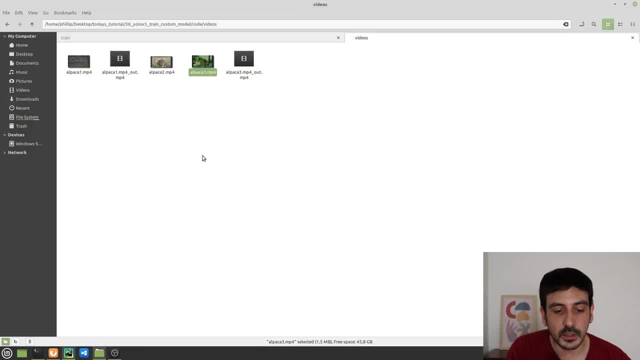 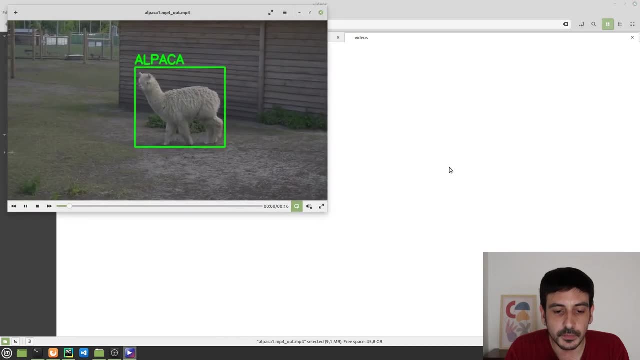 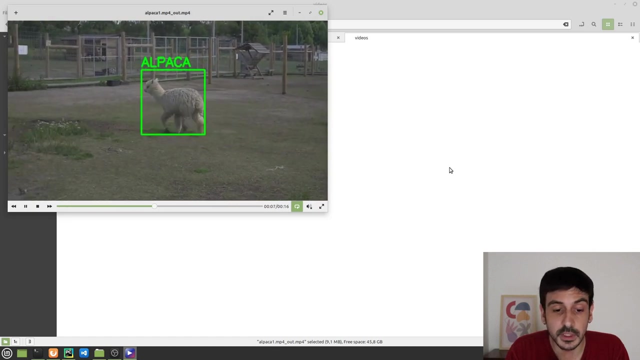 and we are applying all the predictions to this model and we are seeing how it performs on these videos. so this is the first video i show you and these are the detections we are getting. you can see, we are getting an absolutely perfect detection. remember, this is completely unseen data and we are 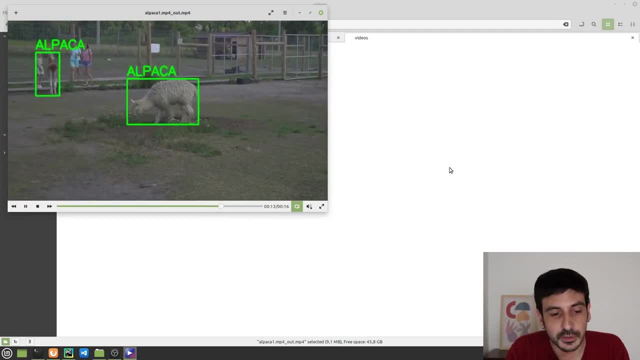 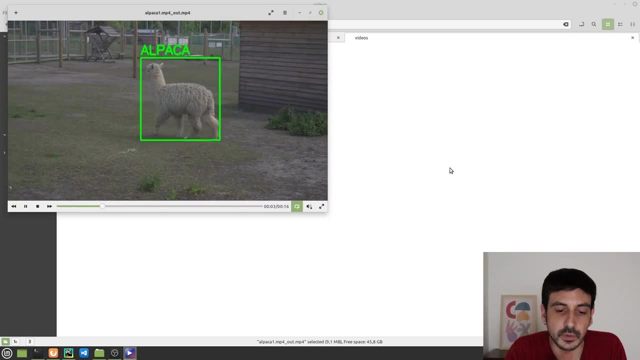 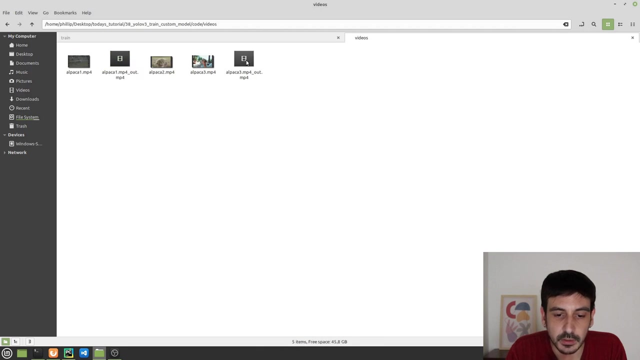 getting. i'm not going to say 100 perfect detection, because we are not, but i would say it's pretty good. i would say it's pretty, pretty good in order to start working on this training process. yeah, i would say it's pretty good. so this is one of the examples. then let me show you. 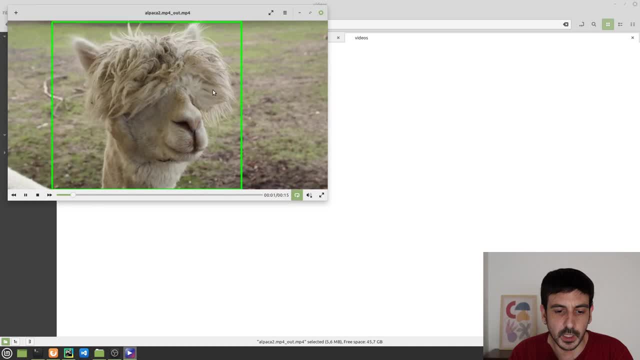 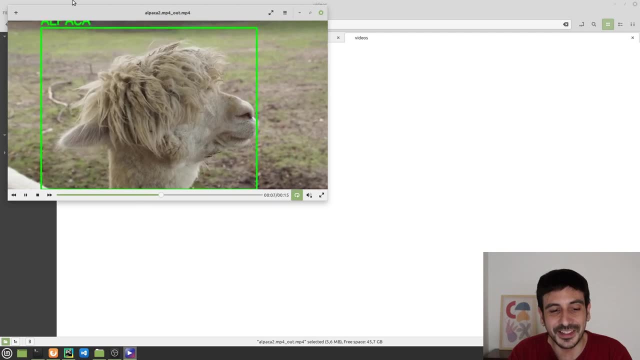 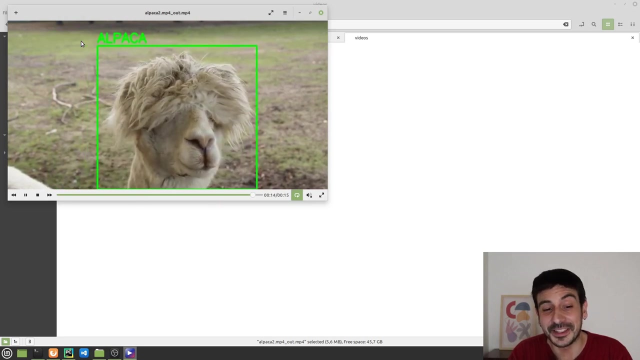 another example, which is this one- and this is the other video i show you- and you can see that we are also detecting exactly the position of the alpaca. in some cases the text is going outside of the frame because we don't really have space, but everything seems to be okay in this video too. 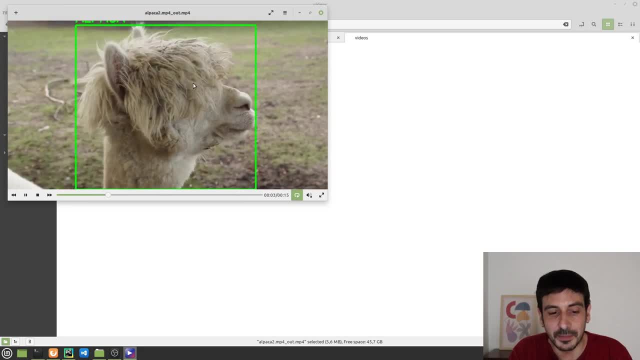 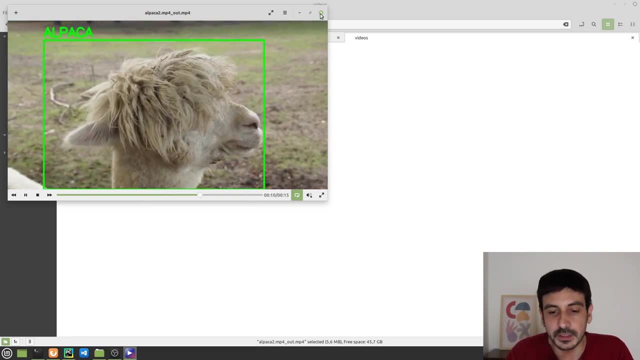 so we are detecting exactly the position of this alpaca, the box in some cases not really fit to the alpaca face, but yeah, but everything seems to be working fine. and then the other video i show you. you can see, in this case the detection is a little broken. 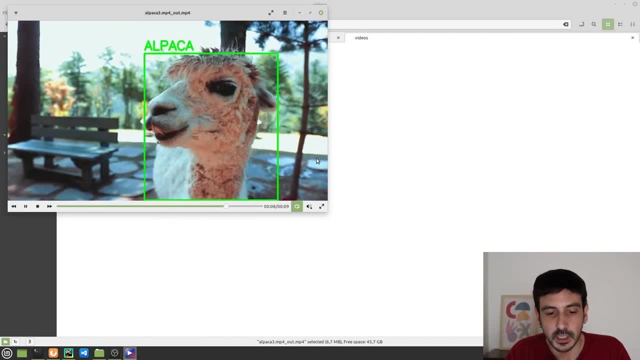 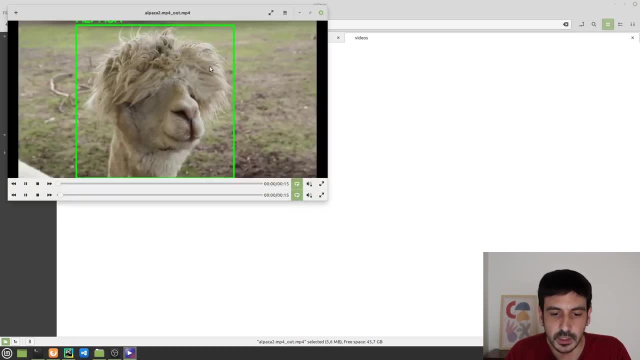 we have many missed detections, but now everything is much better and, yeah, in this case it's working better too. it's working well. i would say, in these three examples, this one it's the one that's performing better, and then the other one i really like how it performed. 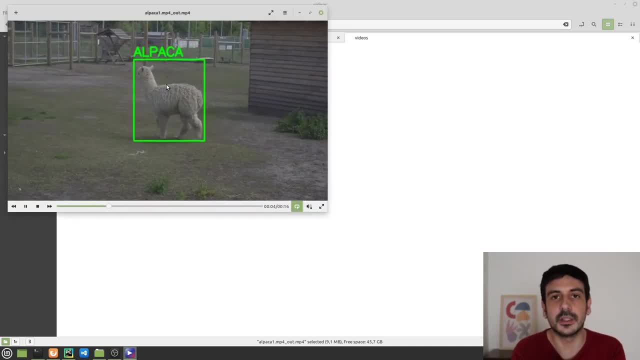 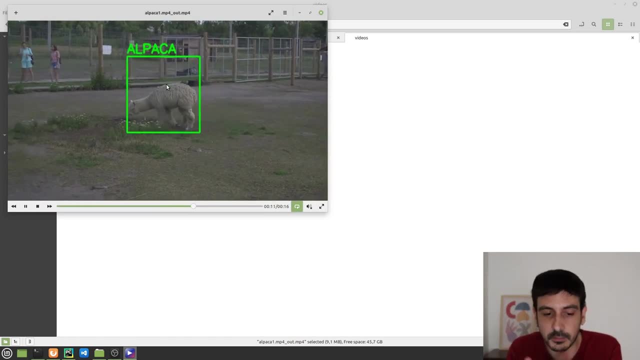 too. in this case, where the alpaca was like starting its alpaca journey, um, and yeah, we, we had like a very good detection and a very stable detection. then it like breaks a little but nevertheless i would say it's okay, it's also detecting this alpaca over here. 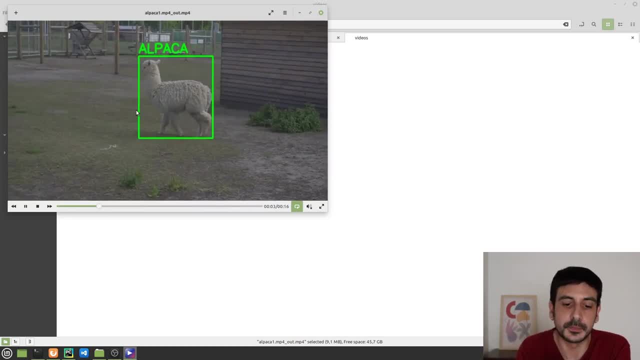 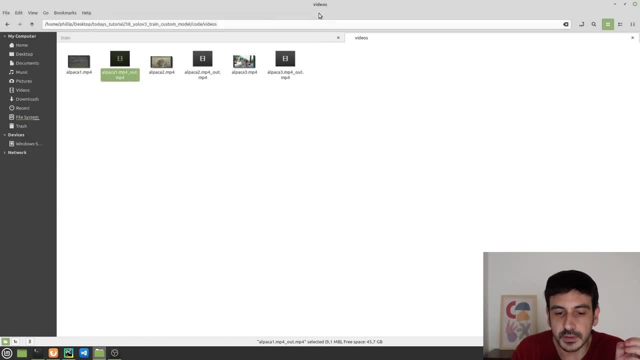 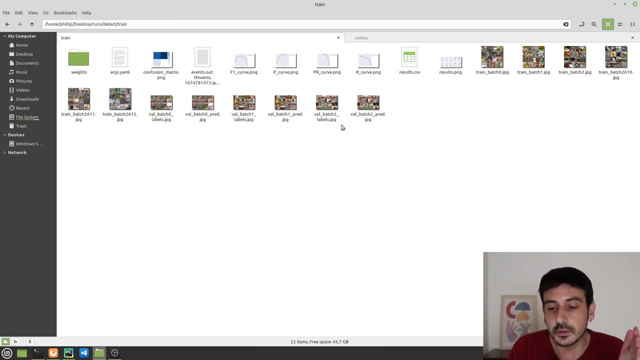 so i would say it's working pretty much okay. so this is pretty much how we are going to do the testing in this phase. remember that if you want to test the performance of the model you have just trained using yellow, you will have a lot of information in this directory, which is created when you are. 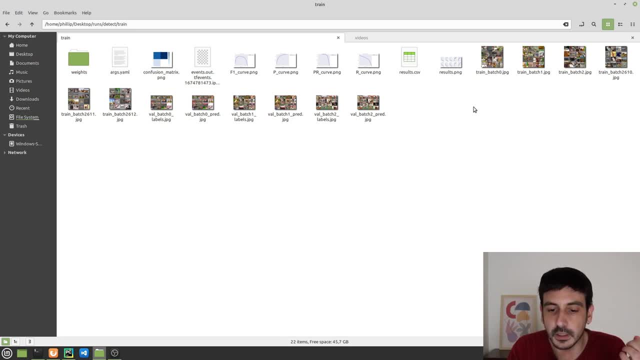 training the model. at the end of your training process you will have all of these files and you will have a lot of information to knock yourself out, to go crazy analyzing all these different plots and so on, or you can just keep it simple and just take a look at what happened. 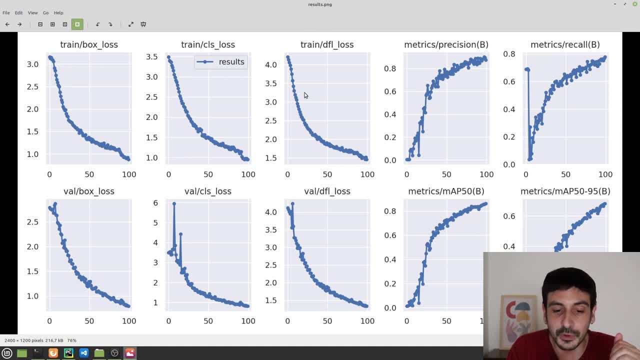 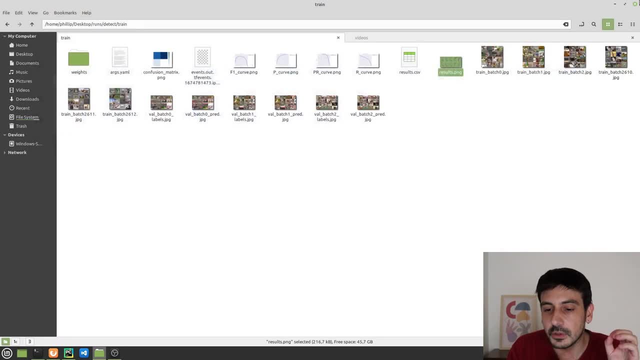 with the training laws and the laws and the validation laws and so on. all the loss functions make sure they are going down. that's the very least thing you need to make sure of, and then you can just see how it performs with a few images or with a few videos. 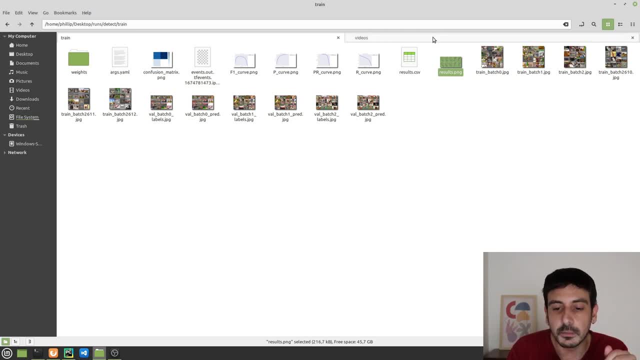 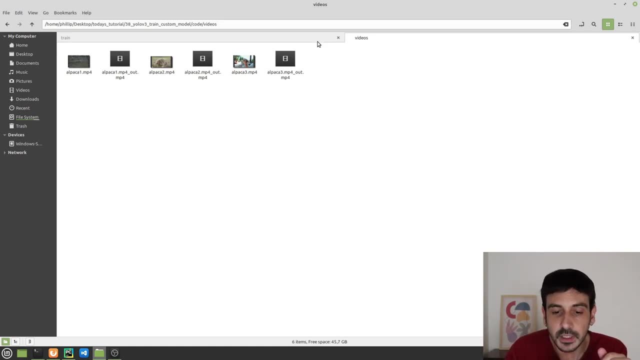 take a look how it performs with unseen data and you can make decisions from there. maybe you can just use the model as it is or you can just decide to train it again. in this case, if i analyze all this information, i see the train. the loss functions are going down and 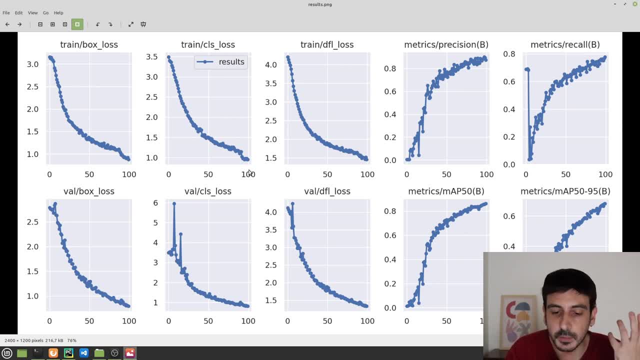 not only they are going down, but i noticed that there's a lot of space to um, to improve these training, to improve the performance, because we haven't reached that moment where everything just appears to be stuck right like that, a flat line. we are very far away from there, so that's something i 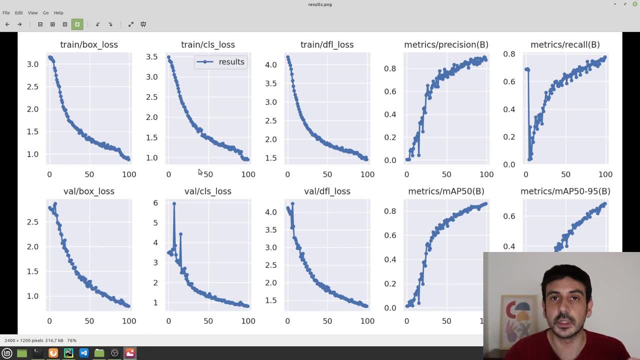 will do. i will do an even deeper training, so we can just continue learning about this process. also, i will change the validation data for something that's completely different for the from the training data, so we have more, more information. and that's pretty much what i will do in order to 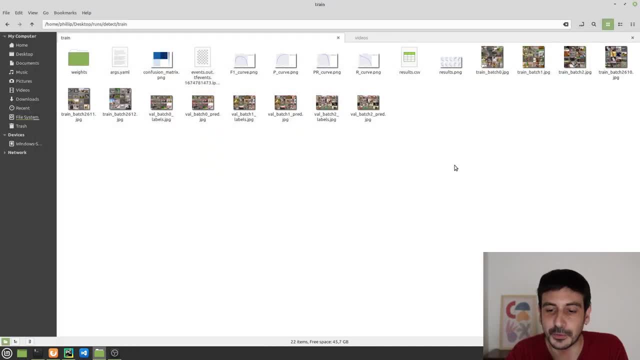 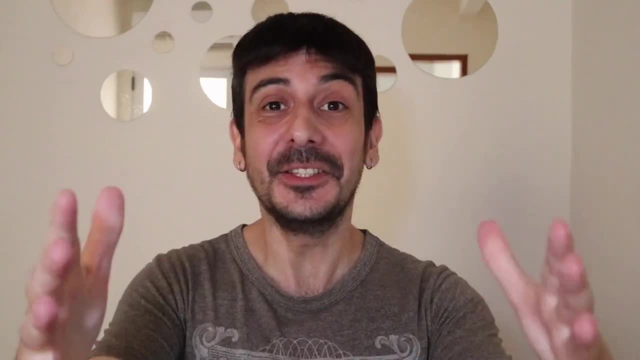 be able to animate better, a better way, if you enjoy trying to do integrate and you know, to make a better model and a more powerful model. hey, my name is felipe and welcome to my channel. in this video, i'm going to show you how to make. 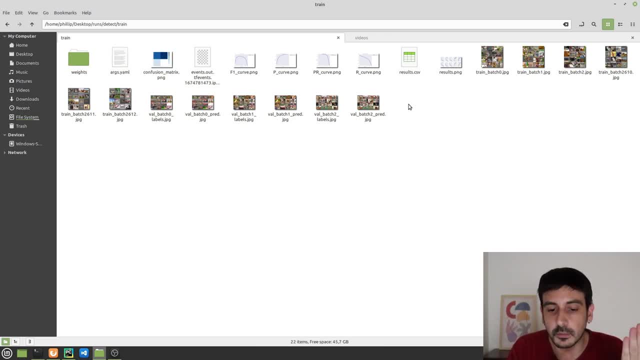 of information in this directory which is created when you are training the model. at the end of your training process, you will have all of these files and you will have a lot of information to knock yourself out, to go crazy, analyzing all these different plots and so on, or you can just keep. 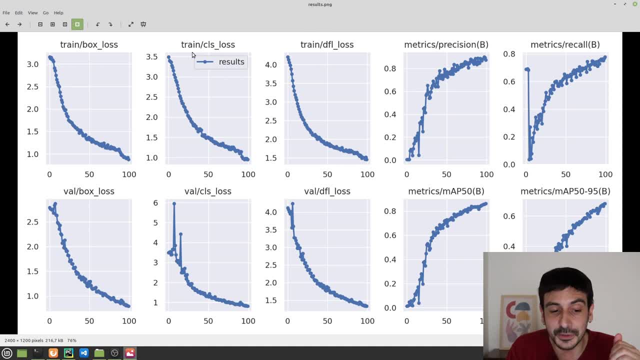 it simple and just take a look at what happened with the training laws and the loss and the validation laws and so on. all the loss functions. make sure they are going down. that's the very least thing you need to make sure of, and then you can just see how it performs with a few images or with 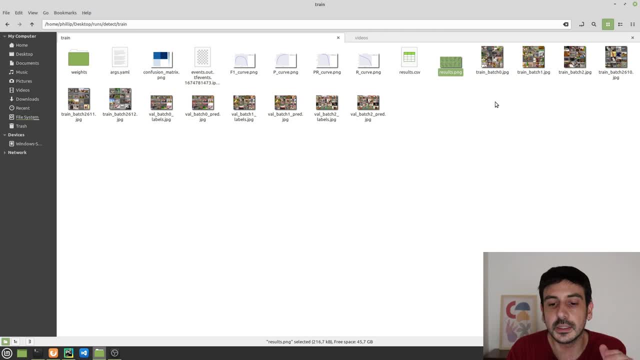 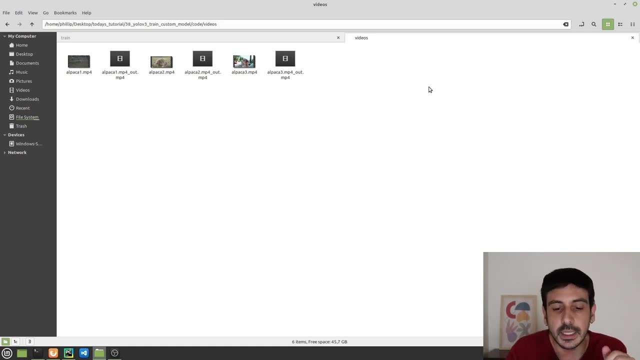 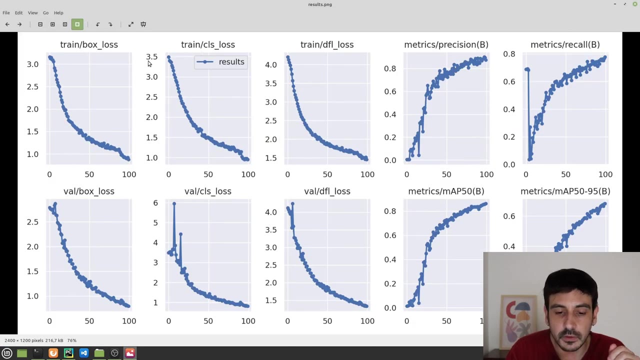 just few videos. uh, take a look how it performs with unseen data and you can make decisions from there. maybe you can just use a as it is or you can just decide to train it again. in this case, if i analyze all this information, i see the train, the loss functions are going down, and not only they are going down, but i notice that. 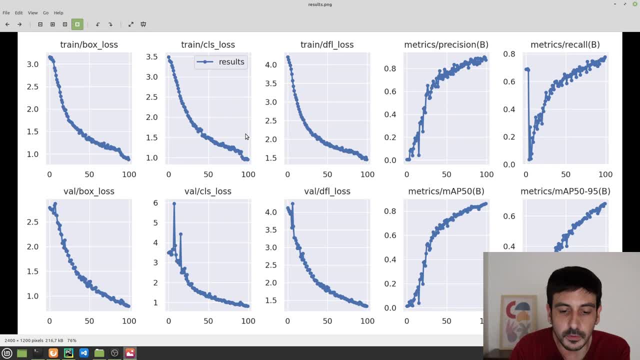 there's a lot of space to to improve this training, to improve the performance, because we haven't reached that moment where everything just appears to be stuck right like that flat line. we are very far away from there, so that's something i will do. i will do an even deeper. 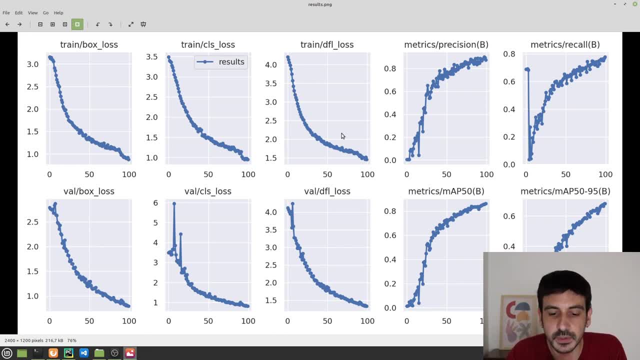 training, so we can just continue learning about this process. also, i will change the validation data for something that's completely different for the from the training data, so we have more, more information. um, and that's pretty much what i will do in order to iterate, in order to make a better. 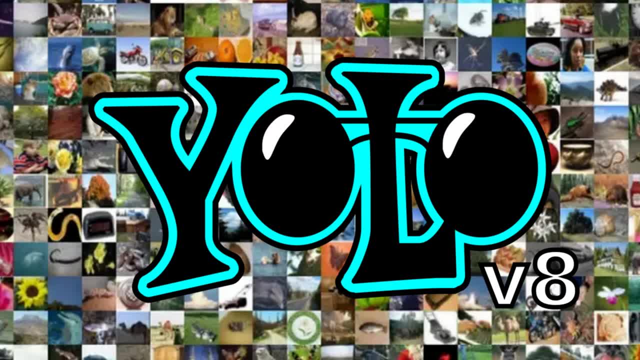 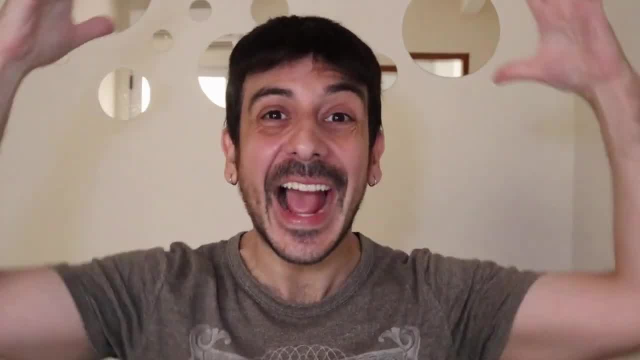 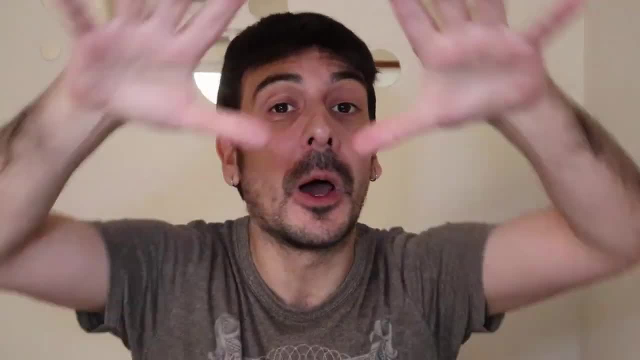 model and a more powerful model. hey, my name is Felipe and welcome to my channel. in this video, i'm going to show you how to make an image classifier using yolo v8 on your own custom data. i'm going to show you every single step of this process, from how to organize the data so it complies with yolo v8, how to do the. 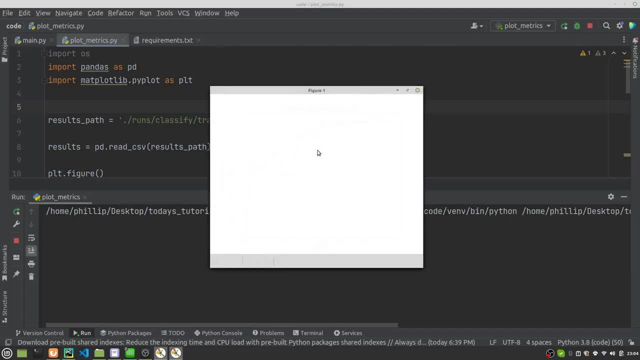 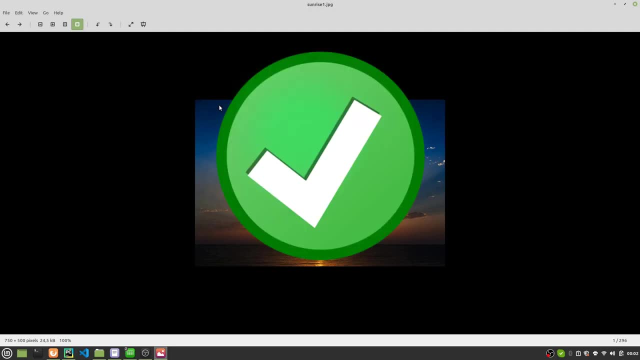 training in your local computer and also from a google collab, how to validate the performance of the model you train and, finally, how to take the image classifier in order to make new predictions. i'm going to show you the entire process. this is going to be an 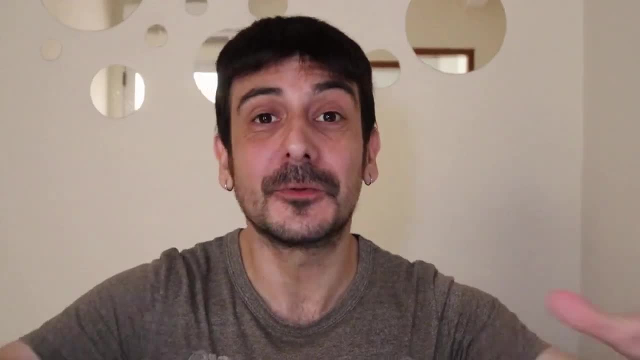 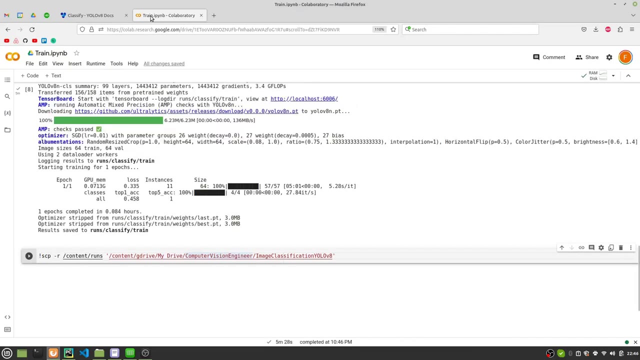 an image classifier using yolov8 on your own custom data. i'm going to show you every single step of this process, from how to organize the data so it complies with the yellow v8, how to do the training in your local computer, and also from a google collab. 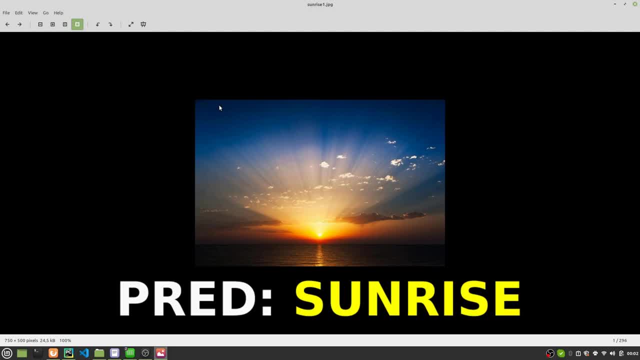 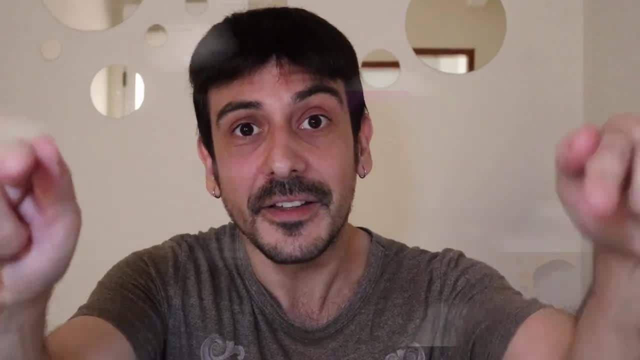 finally, how to take the image classifier in order to make new predictions. i'm going to show you the entire process. this is going to be an amazing tutorial, and now let's get started. so, on today's tutorial, i'm going to show you how to train an image classifier using yellow v8 on your own. 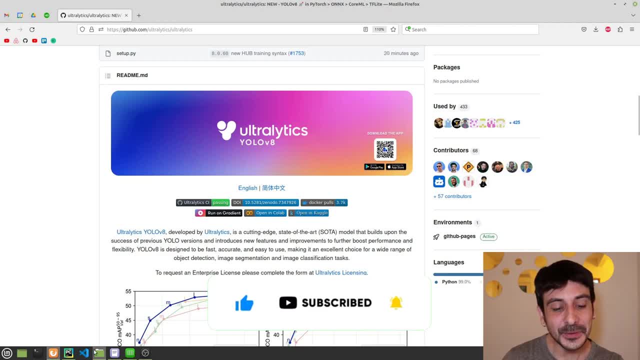 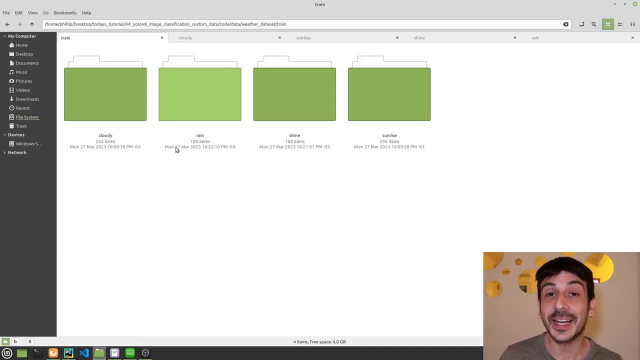 custom data set. so let's get started, and the first thing i'm going to do is to show you the data i am going to use in this tutorial, which is a weather related data set. let me show you the different categories we have and let me show you all the different images how they look like. 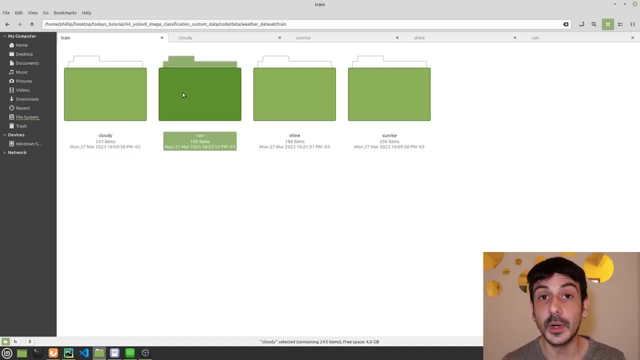 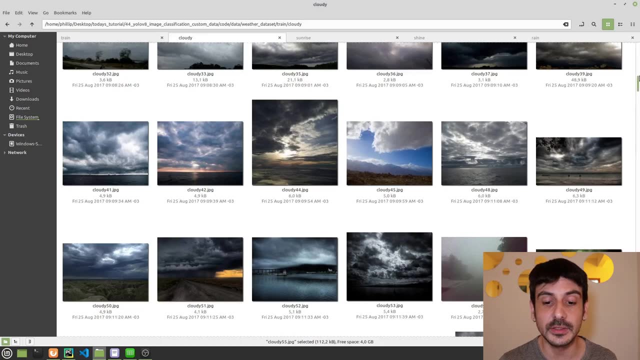 we have four different categories, and they are: cloudy, rain, shine and sunrise. now let me show you each one of these categories. for example, the cloudy category. this is how the images look like. you can see that in each one of these images, we have a sky which is completely cloudy, right? 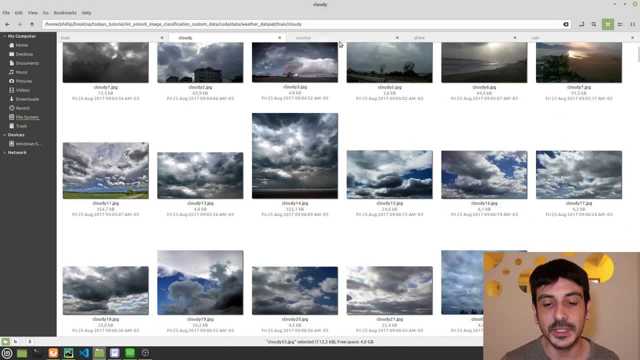 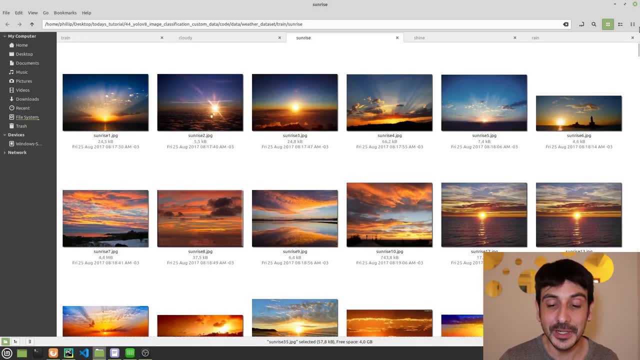 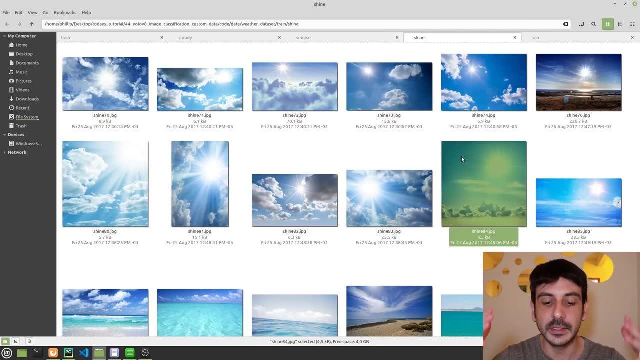 we have many different clouds for each one of these images. now, the sunrise category: it's basically many different pictures of sunrises, so this is how this category look like. and now for the shine category, we have a sky which is completely, completely clear and with a super, super bright sun. right, you have the sun in each one of 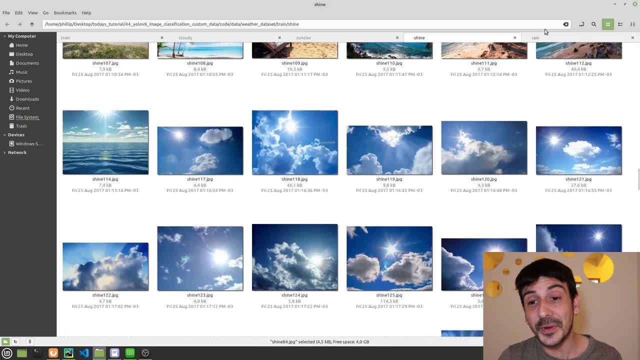 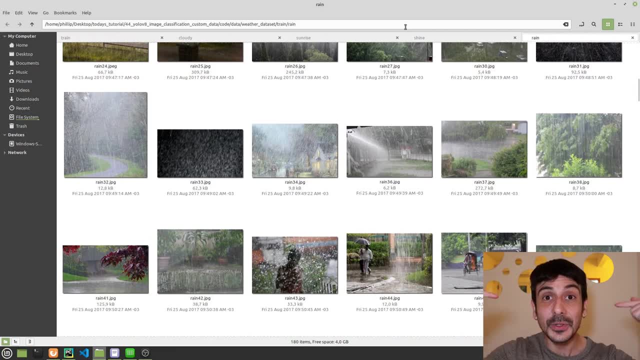 these images and it's super, super, super bright and this is a rainy category and you can see these are many different pictures of super rainy days. so this is basically the data set i am going to use in this tutorial, but obviously you can apply absolutely everything i'm going to show. 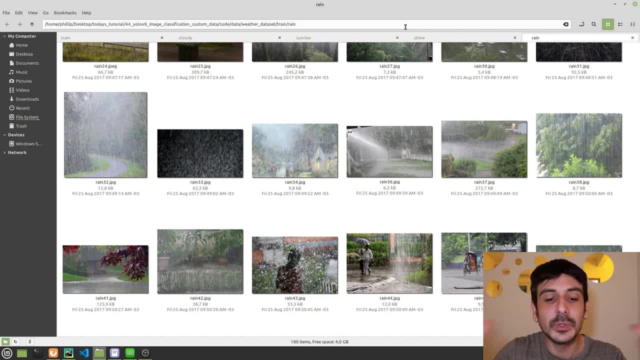 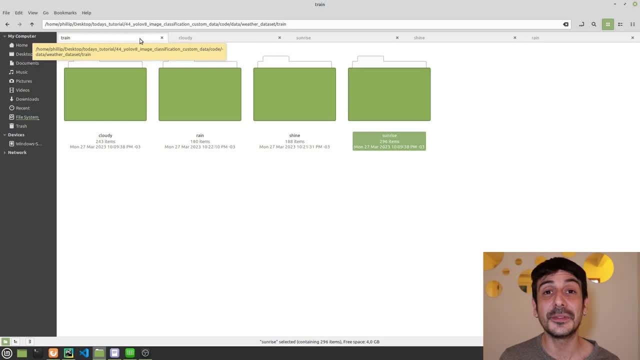 you today to absolutely any type of data set you are going to use in this tutorial. so that's it, bye, bye. going to be able to build any type of image classifier with everything i'm going to say in this tutorial. now let me show you the structure you need for your data, because if you're going to 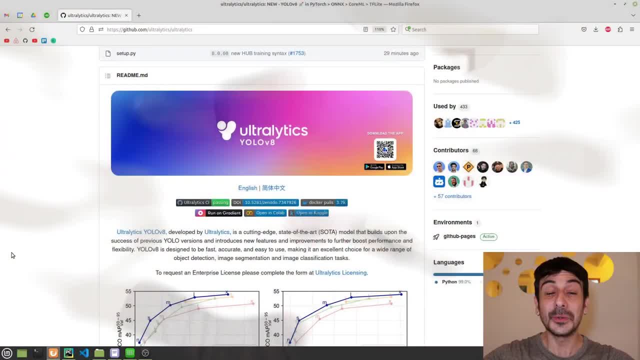 a amazing tutorial, and now let's get started. so, on today's tutorial, I'm going to show you how to train an image classifier using yellow V8 on your own custom data set. so let's get started, and the first thing I'm going to do is to show you the data I am going to use in this tutorial, which 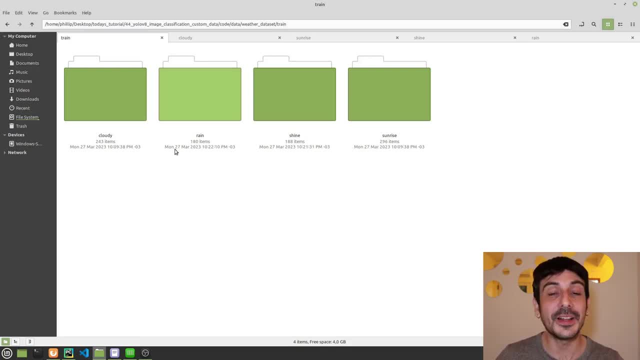 is a weather related data set. let me show you the different categories we have and let me show you all the different images, how they look like. we have four different categories, and they are cloudy, rain, shine and sunrise. now let me show you each one of these categories, for example, the cloudy. 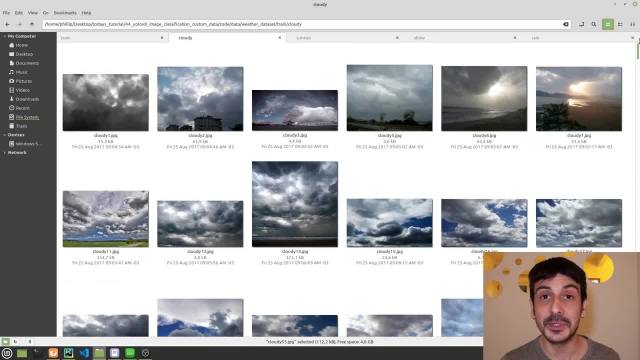 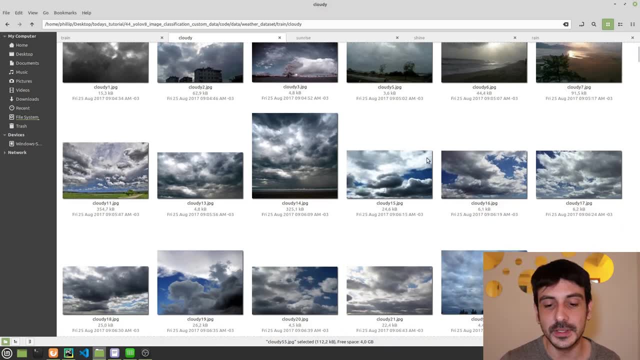 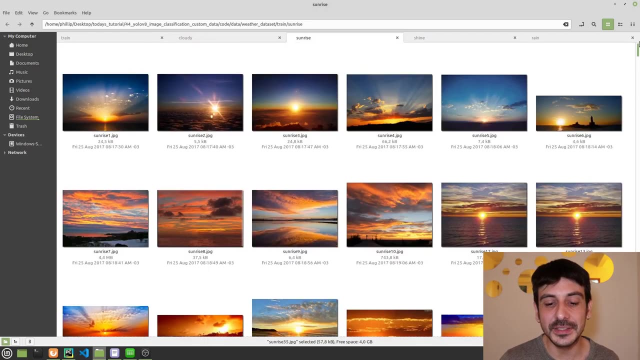 category. this is how the images look like. you can see that in each one of these images, we have a sky which is completely cloudy. right, we have many different clouds for each one of these images. now, the sunrise category: it's basically many different pictures of sunrises, so this is how. 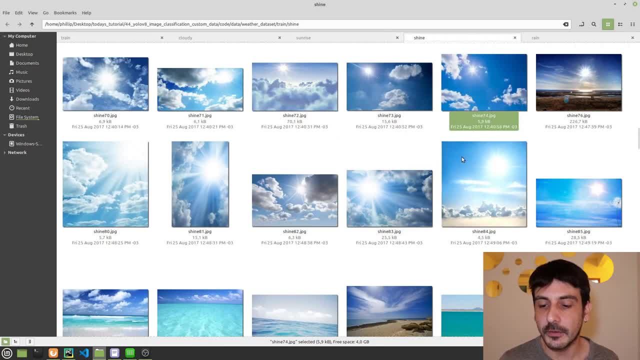 this category look like. and now for the shine category, we have a sky which is completely, completely clear and with a super, super bright sun. right, you have the sun in each one of these images and it's super, super, super bright. and this is a rainy category and you can see these are many different pictures. 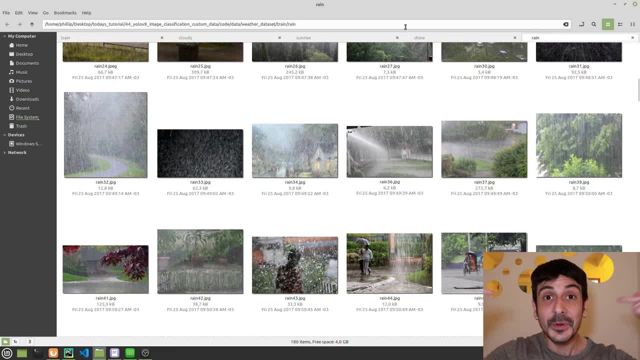 of super rainy days. so this is basically the data set I am going to use in this tutorial, but obviously you can apply absolutely everything I'm going to show you today to absolutely any type of data set. you are going to be able to build any type of image classifier with everything I'm. 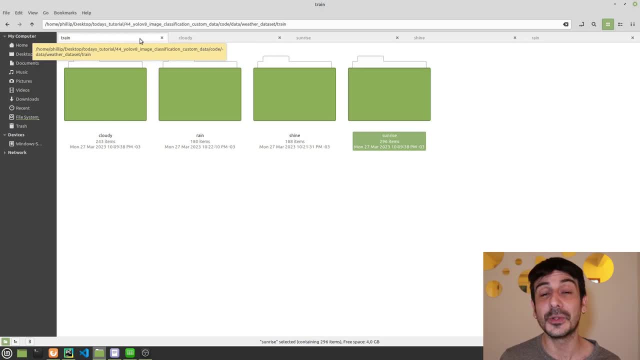 going to say in this tutorial. now let me show you the structure that you need for your data, because if you're going to train an image classifier or if you're going to use yellow V8, yes, the data is super, super important, but you also need to structure, to give. 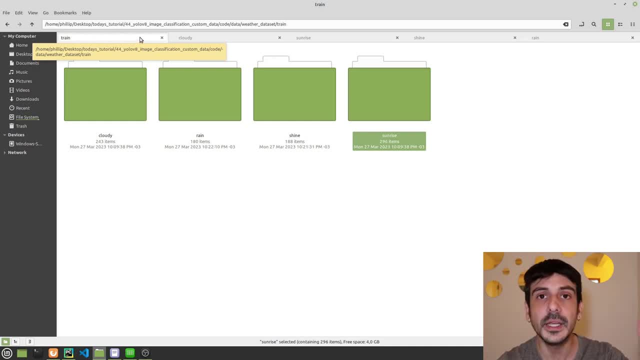 like a format to all of your data so it complies with the way yellow V8 expects your data to be right, or yellow V8 requires your data to be in a given format, in a given structure. so I'm going to show you exactly how to structure your file system so everything looks the way it should. to train an. 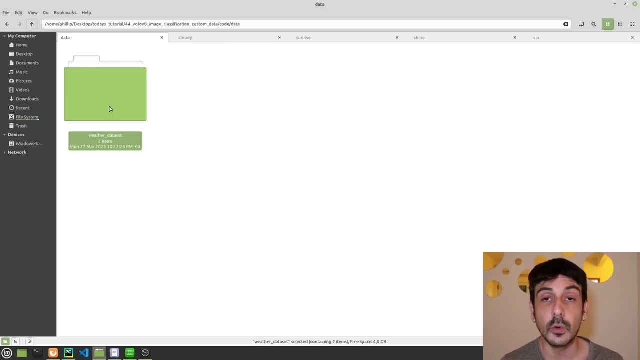 image classifier using yellow V8. so if I show you, I have a directory which is called weather data set, this is going to be the root directory. you can call this directory whatever you want, but you need a directory which is going to be your roots directory and inside this directory you can see. 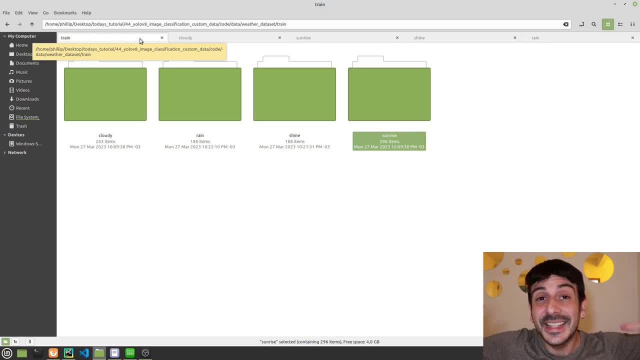 train an image classifier, or if you're going to use yellow v8. yes, the data is super, super important, but you also need to structure, to give like a format to all of your data so it complies with the way yellow v8 expects your data to be right, or yellow v8 requires your data to be in a given 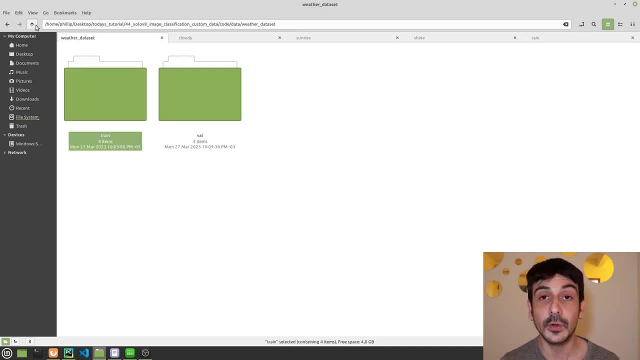 format in a given structure. so i'm going to show you exactly how to structure your file system so everything looks the way it should. to train an image classifier using yellow v8. so if i show you, i have a directory which is called weather data set. this is going to be the root directory. you. 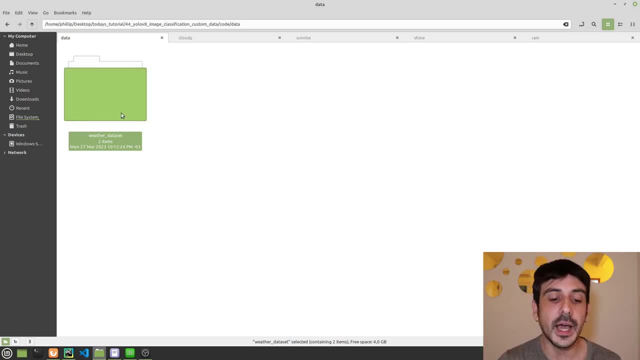 can call this directory whatever you want, but you need a directory which is going to be your root directory, and inside this directory you can see we have two different folders. one of them is called train and the other one is called back, and this is exactly where you're going to have your training data set and your validation data. 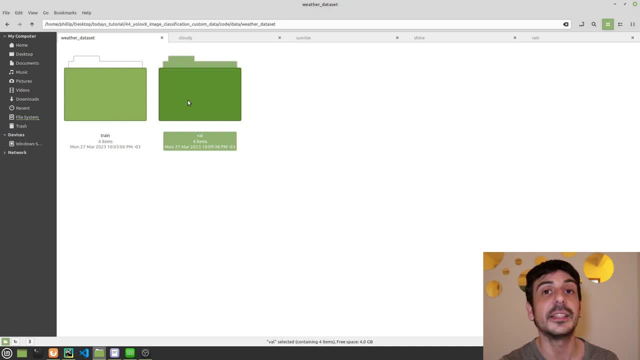 set right. it's very important you name these directories exactly like this. one of them should be called train and the other one val. now, if i show you within the train directory, this is where we are going to have our four directories containing all the different images for all of. 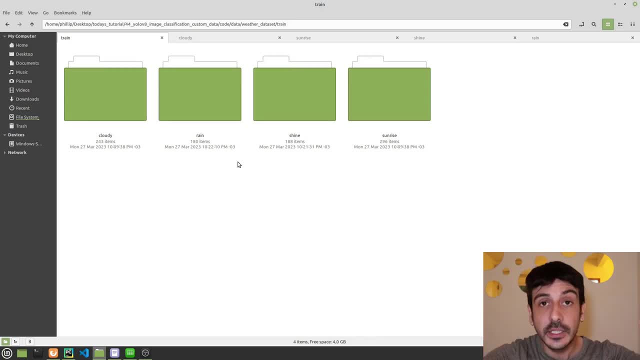 our categories. basically, you need to have as many directories as categories you want to classify with your model. so in my case, i want to classify an image into four directories. so i'm going to classify an image into four directories and i'm going to classify entire images into four different categories, and this is why i have four different directories. 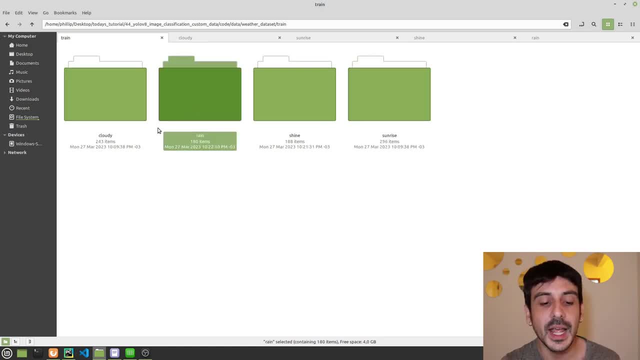 four different models. each one of these directories is named as the category i want to classify my images in right one. one of them is clock, it's called cloudy, the other one is called rain, then shine and then sunrise, and these are the categories i want to classify all my images. 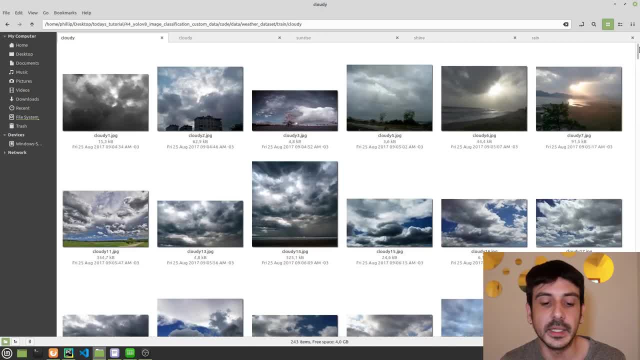 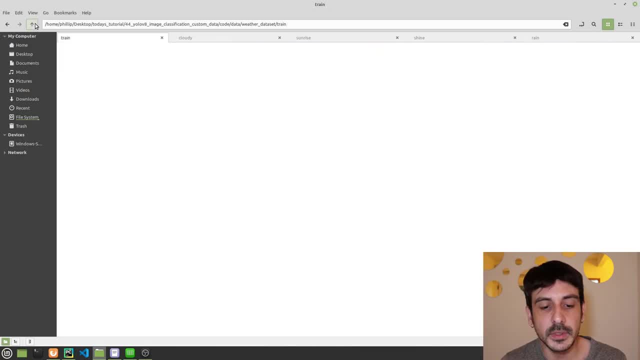 and then within this, these directories, these folders, is where i have all my data within, cloudy is where i have all my data related to the cloudy category, and so on. right the same happens for the rain and the shine and the sunrise category. so this basically the structure you need for your data, the structure you need for your file system in. 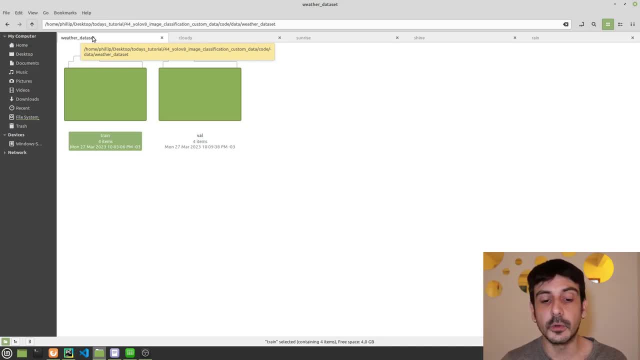 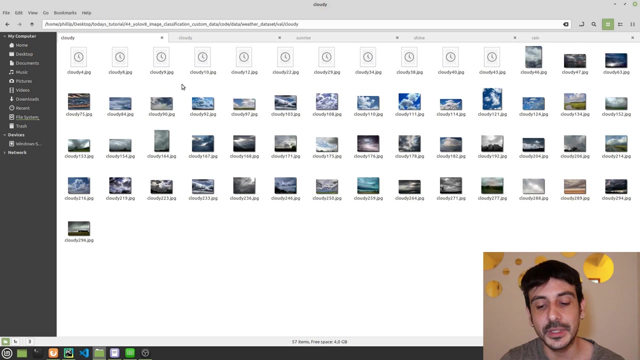 order to comply with what YOLOv8 is expecting for your data. and then, if I go to the ball folder, you can see I have exactly the same structure. I have four different directories and they are named under the categories. I want to classify all my images and then, if I open these directories, 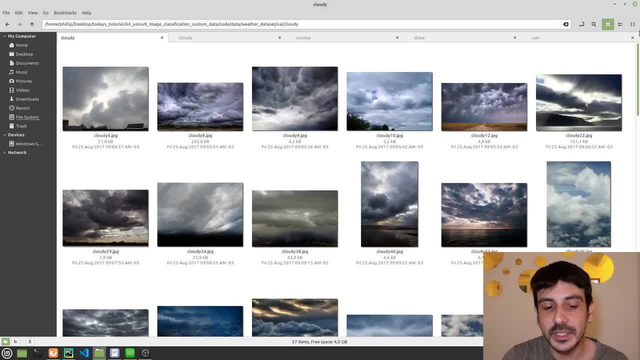 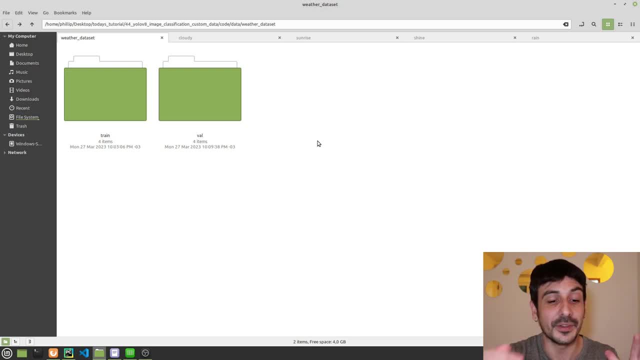 is exactly the same. you can see that I only have different images for that specific category. now, this is very important because from now on, everything is going to be super, super straightforward if you have created this structure for your file system, if your data is exactly in the structure. 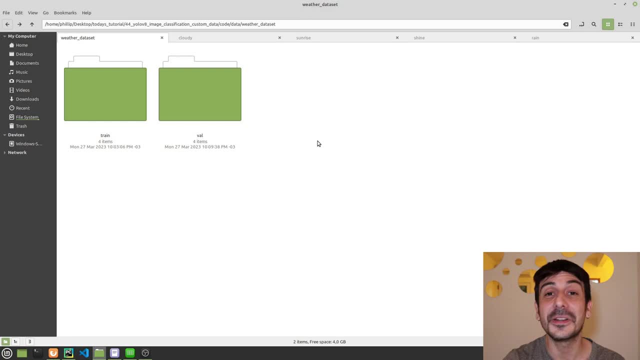 I show you. then it's going to be super simple to train an image classifier using YOLOv8. so this is very, very, very important. now I'm going to show you three different ways in which you can train an image classifier using YOLOv8. 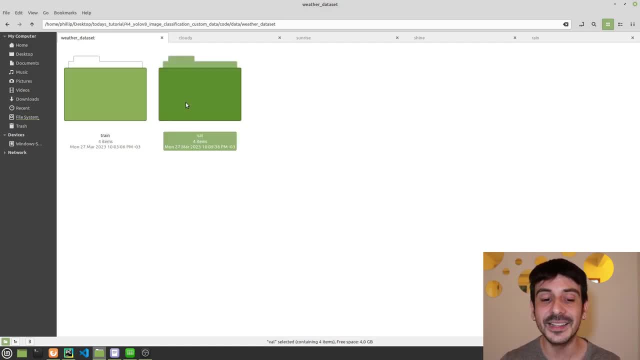 we have two different folders. one of them is called train and the other one is called Val, and this is exactly where you're going to have your training data set and your validation data set right. it's very important you name these directories exactly like this one of them should: 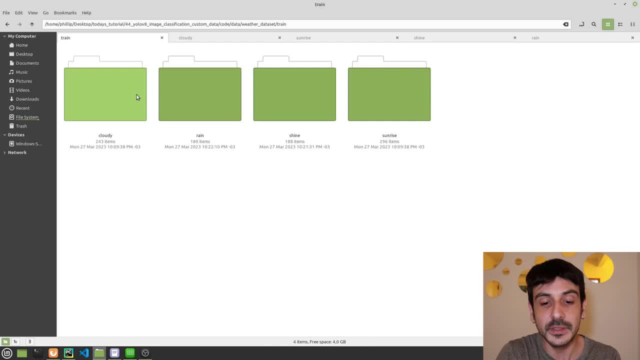 be called train and the other one Val. now, if I show you within the train directory, this is where we are going to have all four directories containing all the different images for all of our categories. basically, you need to have as many directories as categories you want to classify with your model. so 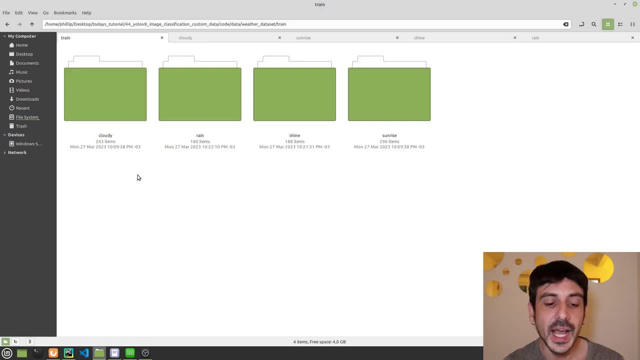 in my case, I want to classify an image into four different categories, and this is why I have four different directories, four different models. each one of these directories is named as the category I want to classify my images in right. one of them is called- it's called cloudy. the other one is called rain. 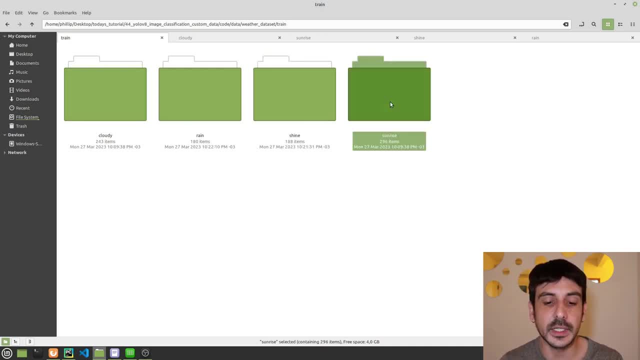 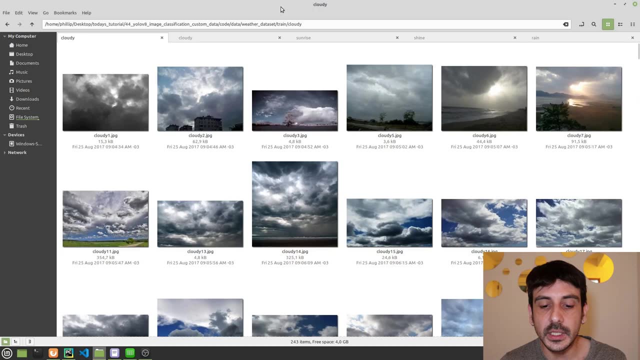 then shine and then sunrise, and these are the categories I want to classify all my images. and then, within these, these directories, these folders, is where I have all my data within cloudy is where I have all my data related to the cloudy category, and so on. right, the same happens for the rain and 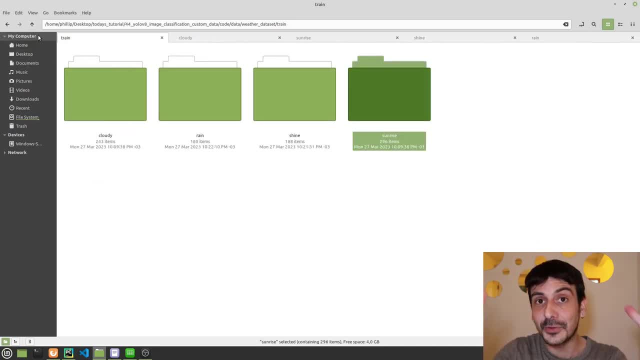 the shine and the sunrise category. so this is basically the structure you need for your data file system in order to comply with what yellow V8 is expecting for your data. and then, if I go to the Val folder, you can see I have exactly the same structure. I have four different directories and 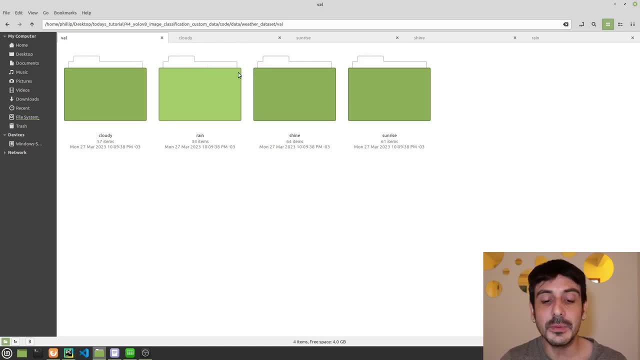 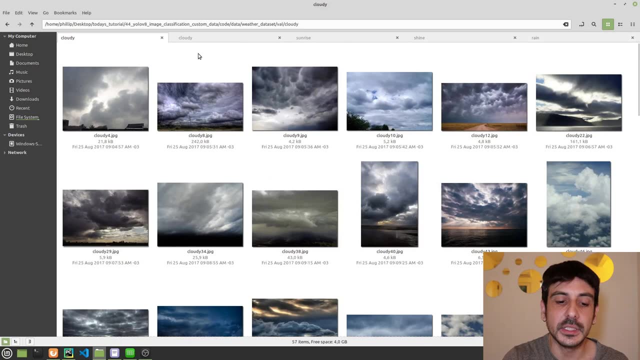 they are named under the categories. I want to classify all my images and then, if I open these directories is exactly the same. you can see that I only have different images for that specific category. now this is very important because from now on, everything is going to be super, super. 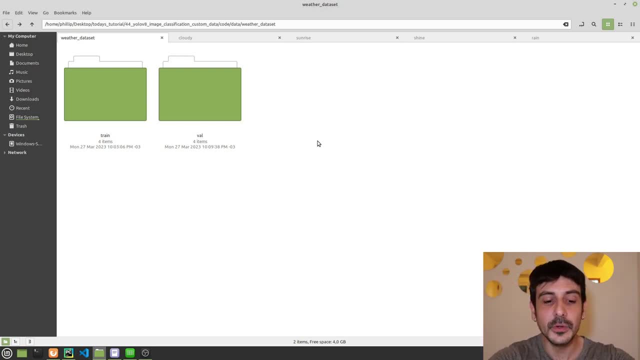 if you have created this structure for your file system, if your data is exactly in the structure I show you, then it's going to be super simple to train. an image classifier is in yellow V8, so this is very, very, very important. now I'm going to show you three different ways in which you can train an. 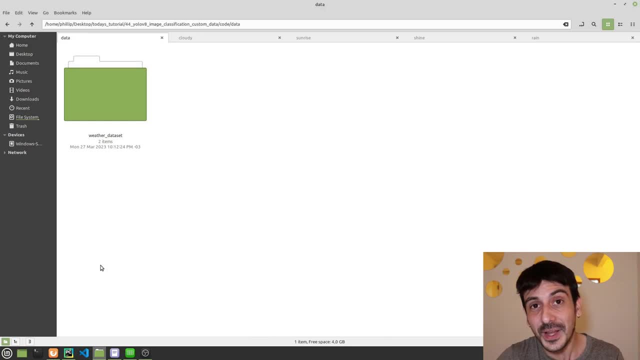 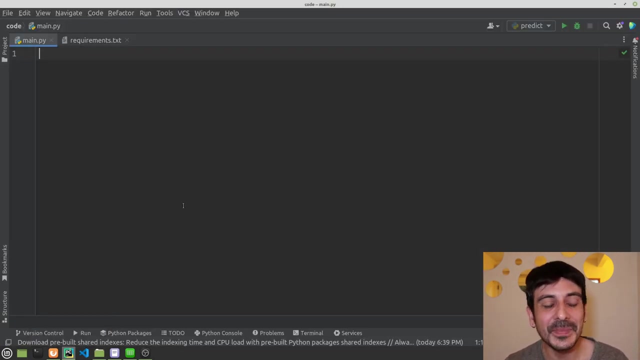 image classifier using yellow V8. so let's start with the first way, which is using a python script. we are going to make a very, very simple script in python in order to train this model and let me show you how to do it. so let's go to pycharm. this is a python project I created for today's tutorial and 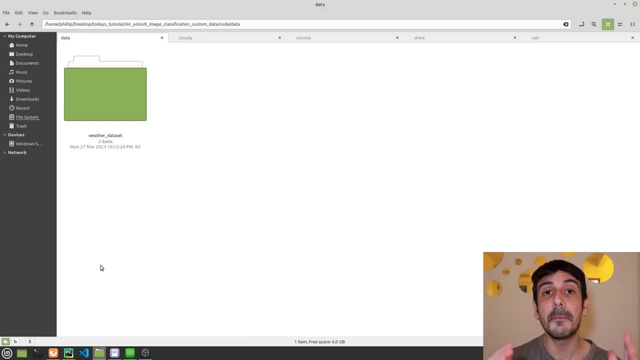 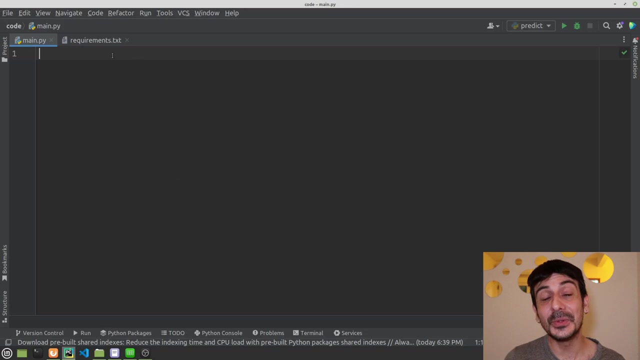 so let's start with the first way, which is using a Python script. we are going to make a very, very simple script in Python in order to train this model, and let me show you how to do it. so let's go to PyCharm. this is a PyCharm project I created for today's tutorial, and the first thing you should 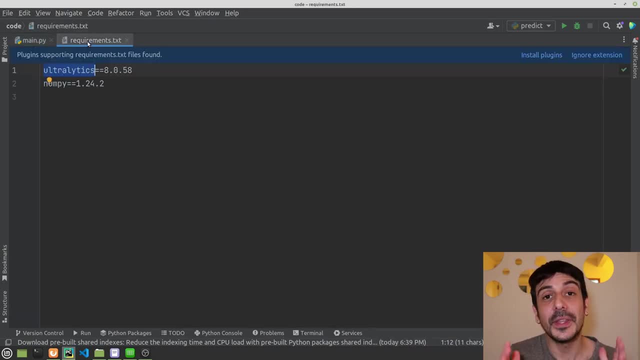 do, if you want to work with YOLOv8, is to install a couple of dependencies, a couple of Python packages. these are two packages we are going to use in this tutorial. one of them is Ultralytics. it's very, very, very, very super important, because this is exactly the library you need in order to 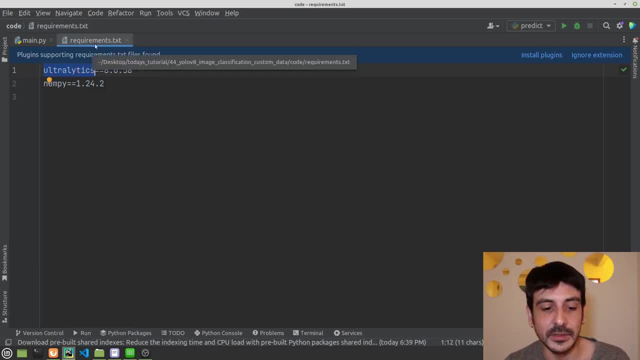 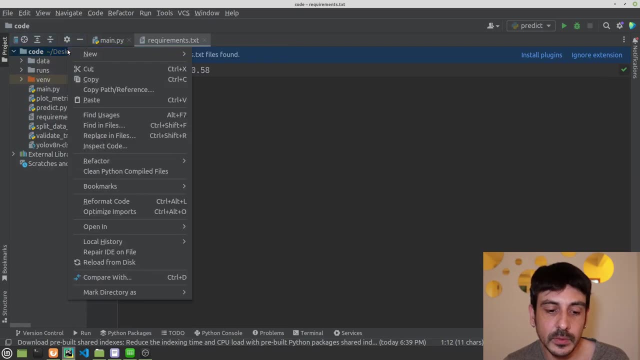 import YOLO in order to train this model using YOLOv8, so you definitely need these two packages now in order to install these packages. this is how we are going to do it. I'm going to show you a way to install these packages which is going to work with whatever your OS, right? if you are a. 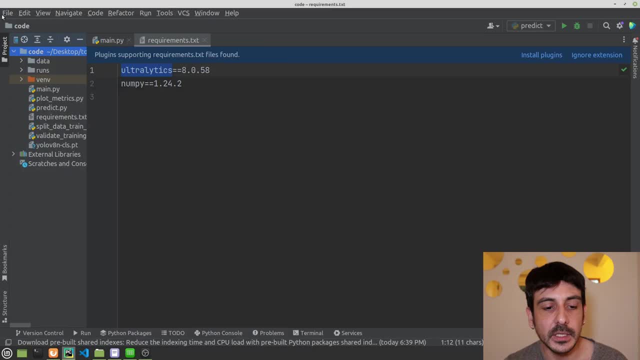 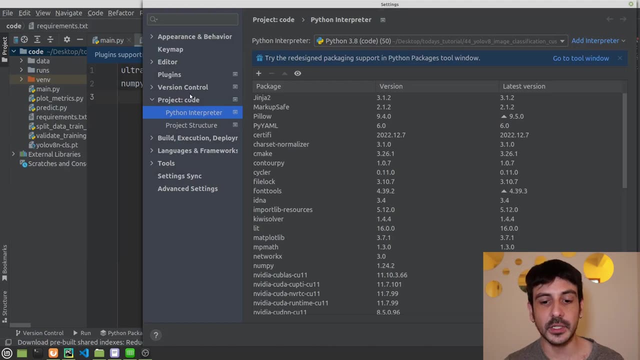 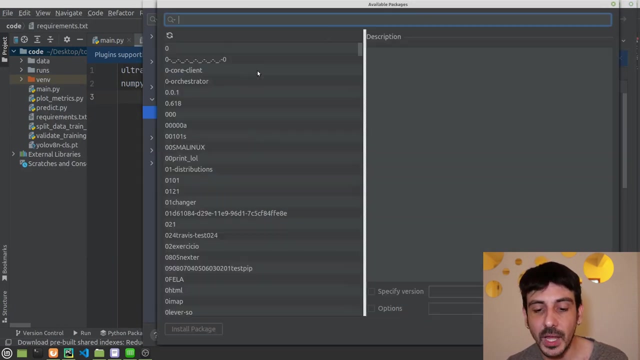 Linux user, or if you are a Windows user, or if you use Mac, it doesn't matter, it's going to work anyway. so you need to go to file, then settings. then you have to select Python interpreter. right, this is the Python interpreter you are going to use. you can see that I'm using Python 3.8, and then you need to click on plus, and this is where 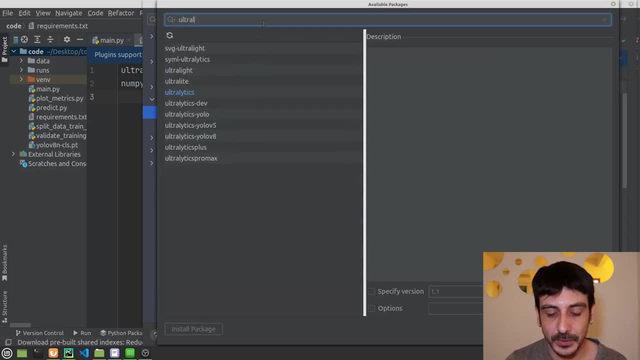 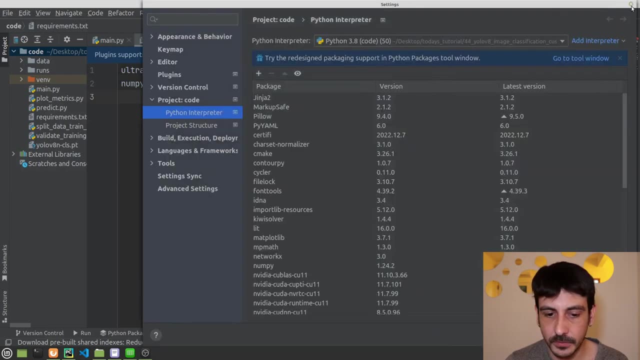 you're going to find. you're going to search for the packages you want to install. in my case, I'm going to search for Ultralytics and the version I'm going to use. let me copy the version first. it's this one, so I'm just going to file setting, then Ultralytics again. 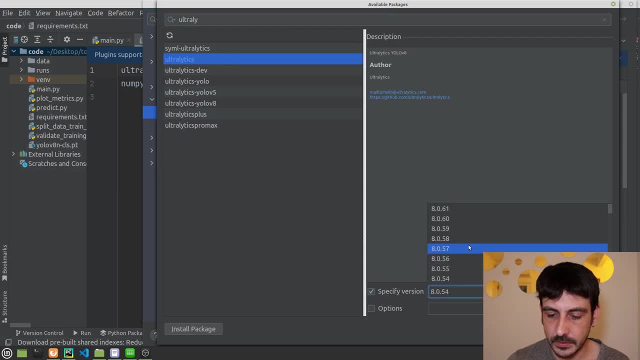 and then the version is this one, okay, and then I click on install package. in my case, I have already installed this dependency, so nothing is going to happen on my computer. but please remember to do it on your computer, because otherwise you will not be able to use or you're not going to be able to do anything of what we are going to be doing today. now let's. 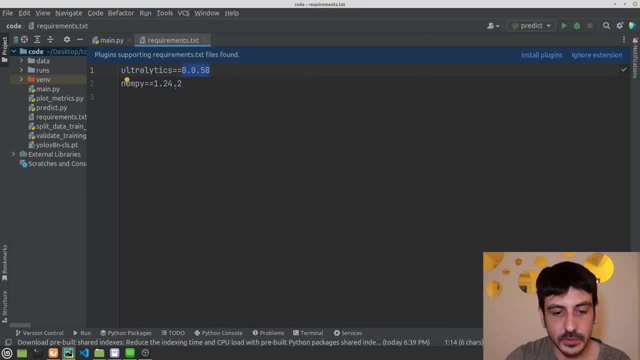 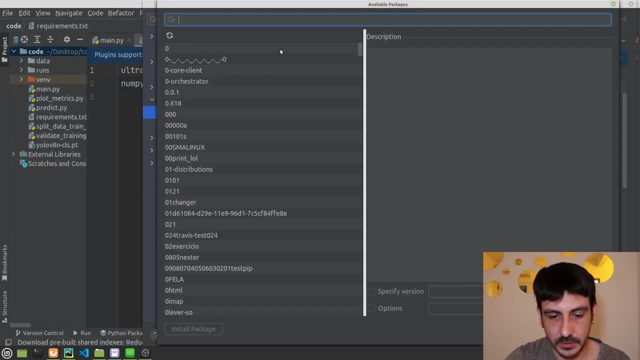 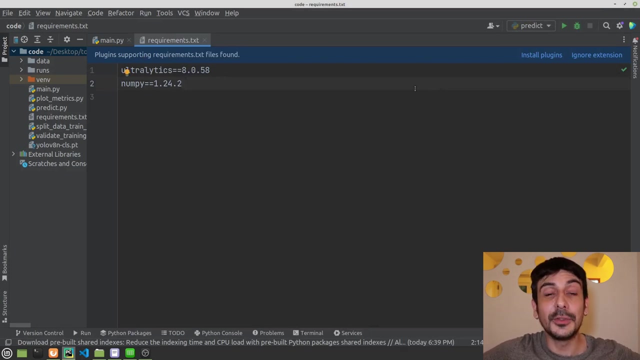 see numpy. what's exactly the version we are going to use? we're going to use 1.24.2, so file settings plus numpy 1.24.2. so everything is okay. now install package. this is like everything is okay. numpy has been installed successfully, so now we are ready to continue once we you have installed. 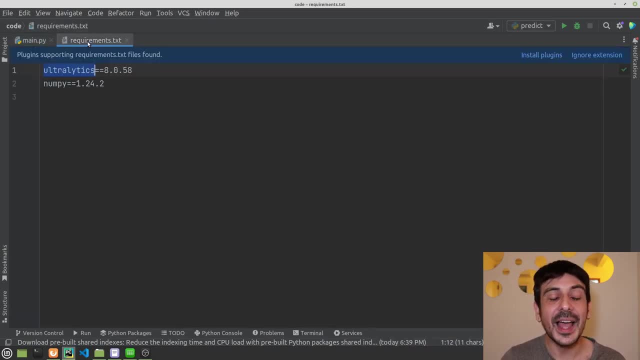 the first thing you should do if you want to work with yellow V8 is to install a couple of dependencies, a couple of python packages. these are two packages we are going to use in this tutorial. one of them is ultralytics and the other one is numpy. ultralytics is very, very, very, very super important. 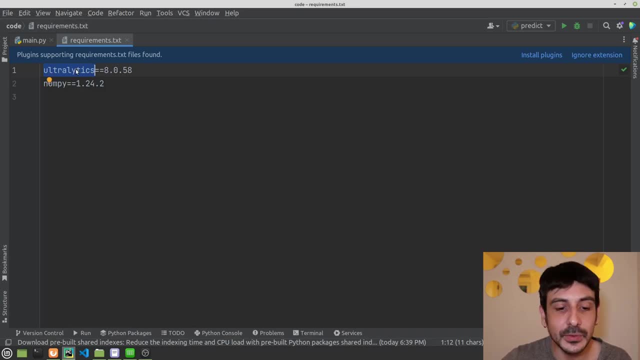 because this is exactly the library you need in order to import YOLO, in order to train this model using yellow V8. so you definitely need these two packages now in order to install these packages. this is how we are going to do it. I'm going to show. 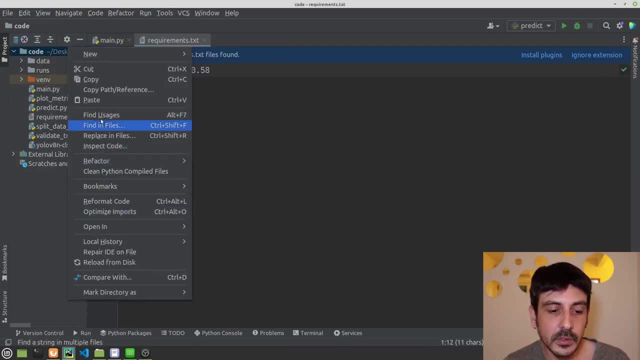 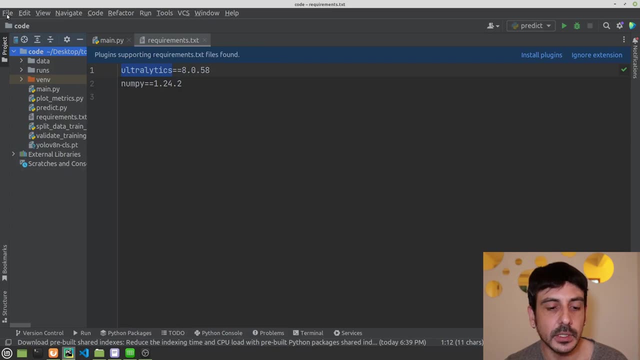 you a way to install these packages which is going to work with whatever your OS, right? if you are a Linux user, or if you are a Windows user, or if you use Mac, it doesn't matter, it's going to work anyway. so you need to go to file, then settings, and then you have to select python. 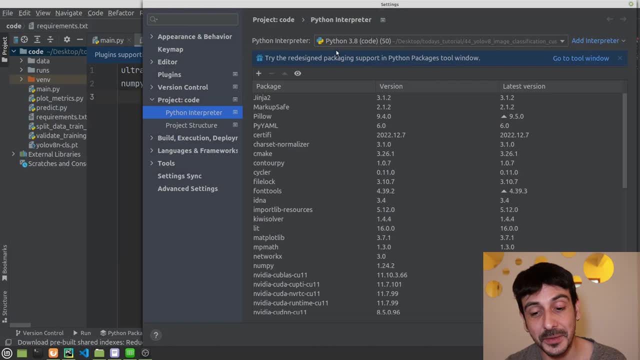 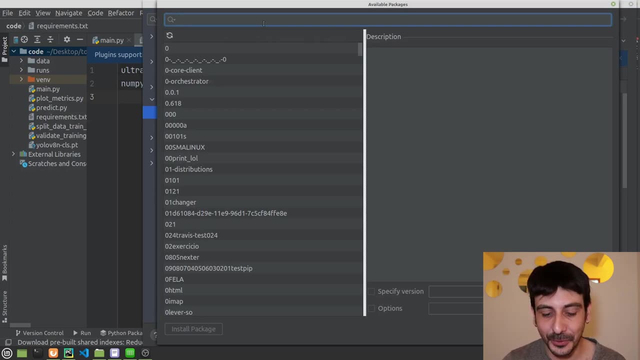 interpreter. right, this is the python interpreter we are going to use. you can see that I'm using python 3.8 and then you need to click on plus and this is where you're going to find. you're going to search for the packages you want to install. in my case, I'm going to search. 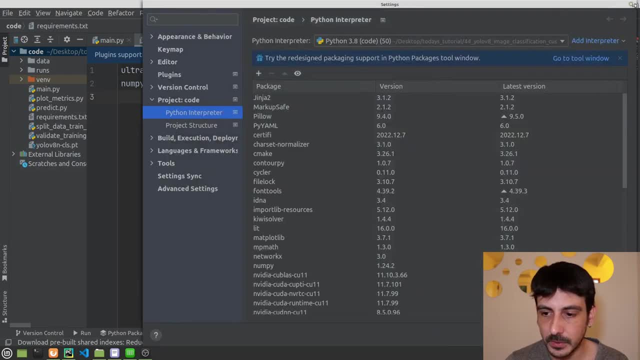 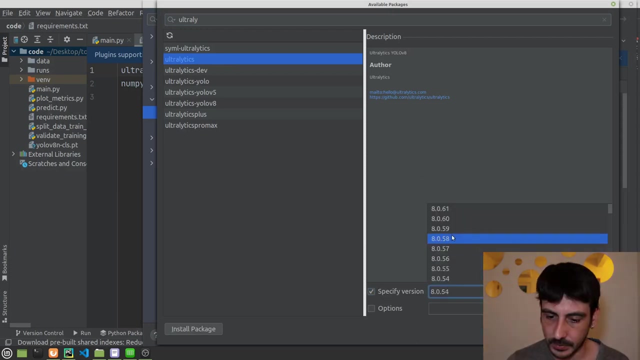 for ultralytics and the version I'm going to use. let me copy the version. first it's this one, so I'm just going to file setting, then ultralytics again, and then the version is this one, okay, and then I click on install package. in my case, I have already installed this dependency, so nothing is going to. 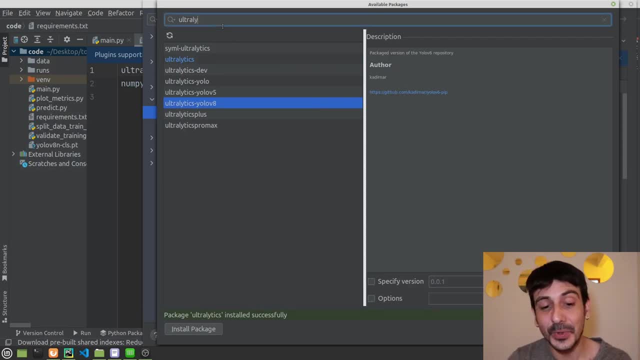 happen on my computer, but please remember to do it on your computer because otherwise you will not be able to use, or you're not going to be able to do, anything of what we are going to be doing today. now let's see numpy. what's exactly the version we are going to use? we're going to use 1.24.2. 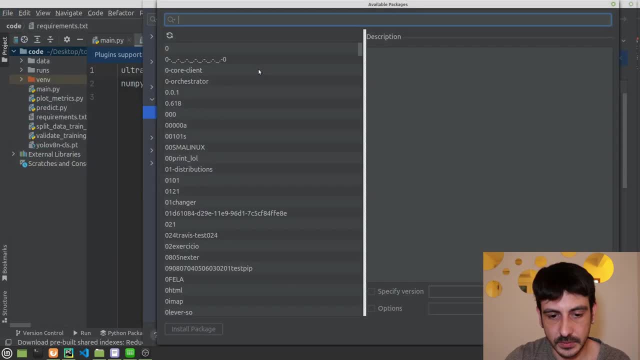 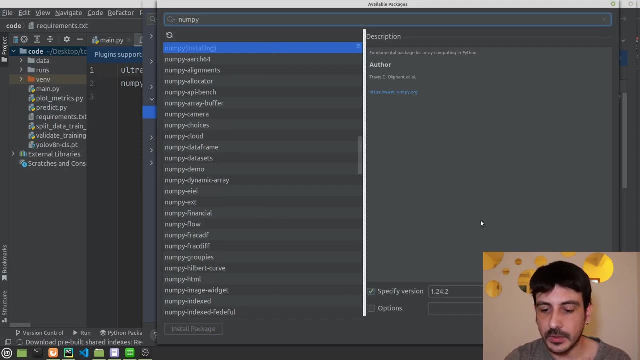 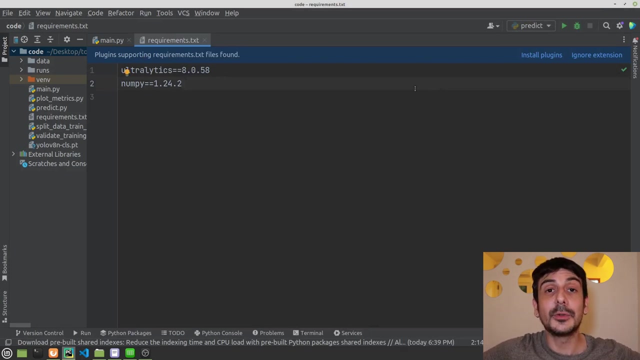 so file settings plus numpy 1.24.2. so everything is okay. now install package. this is like everything is okay. numpy has been installed successfully, so now we are ready to continue. once we you have installed these two dependencies, these two packages, now you're ready to continue. 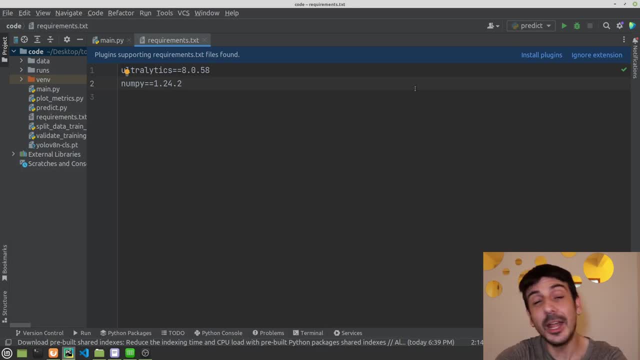 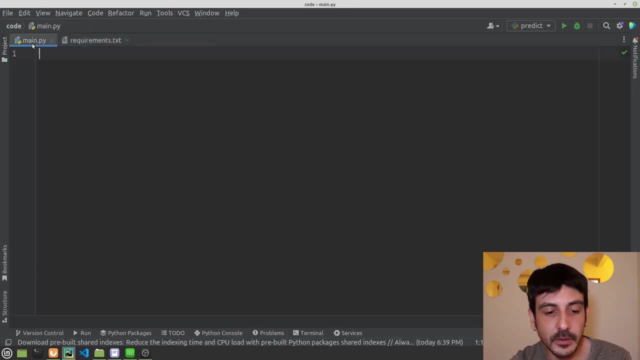 these two dependencies, these two packages. now you're ready to continue, and now you're ready to install your own image classifier using YOLOviate. so let's go to main. this is the file we are going to use in order to code everything we need in order to train this classifier. and let me show you. 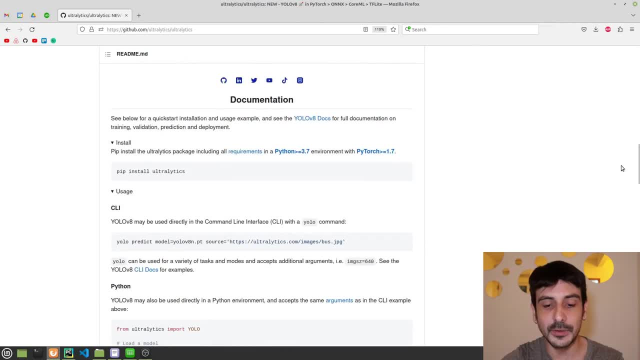 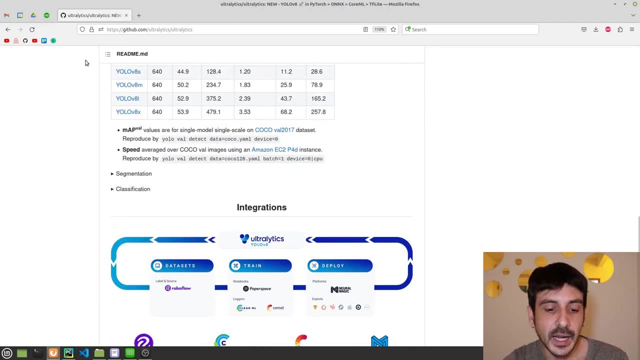 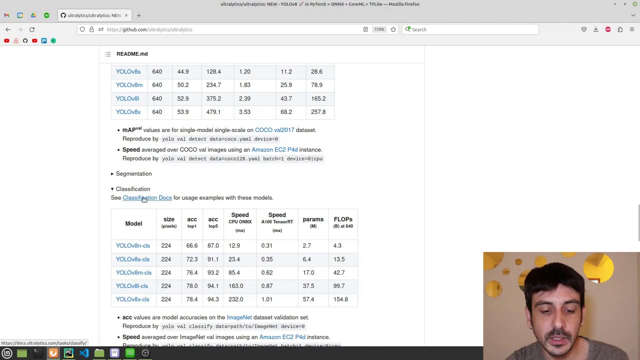 the exactly what's the code you need to type in order to do this training? I'm going to over here to the GitHub repository of Yoloviate and I'm going to select the classification section. right, I'm going for the classification and then here I'm going to click on classification. 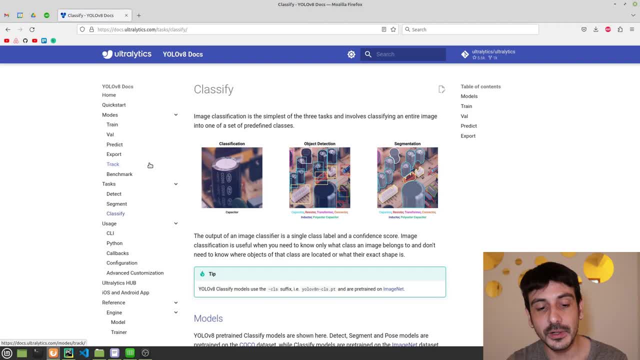 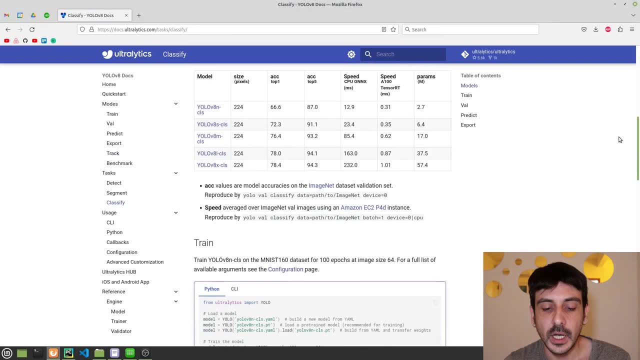 docs. this is going to open a new file, a new url, a new website, a new page. this is exactly the all the information we need in order to train this image classifier. i'm just going to scroll down and i'm going to the train section and this is what we're going. 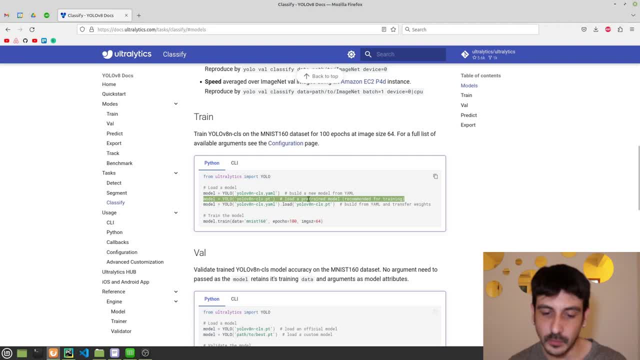 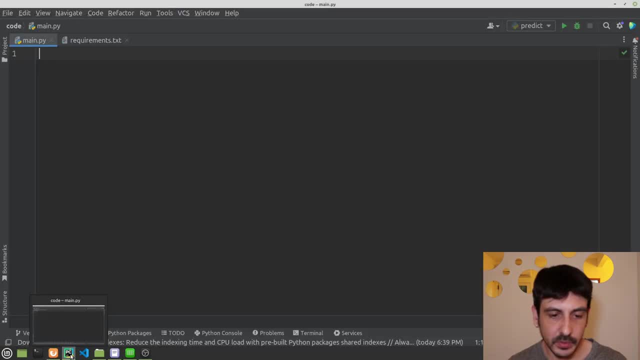 to do? i'm going to copy and paste this line, which is the one in the middle, the one that says: load a pre-trained model recommended for training. i'm just going to copy and then i'm going back to pycharm and i'm just going to paste it. obviously we need to import yolo, otherwise this: 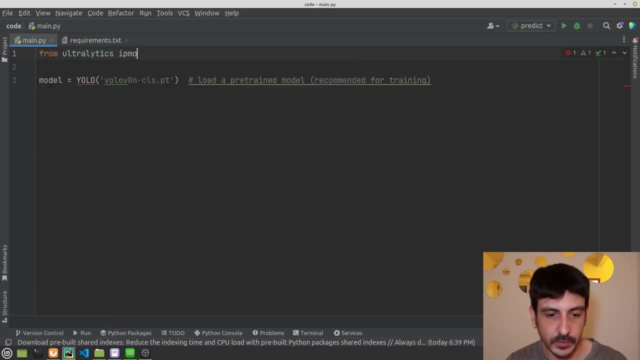 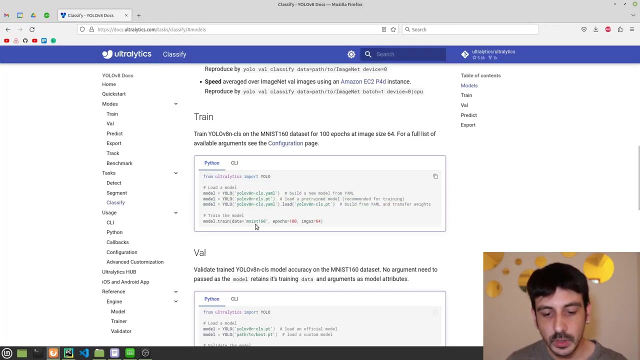 is not going to work. so i'm going to say, from ultralytics import yolo, and that's pretty much all you can see. now we are creating our model, or we are creating the object we are going to use as our model, and then i'm just going to copy and paste this last line, which is: 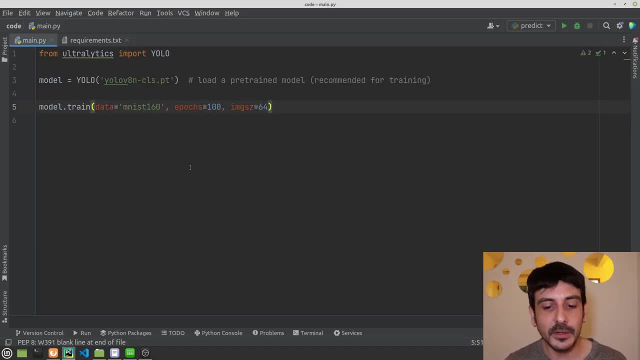 model dot train. i'm going to paste it here and then i'm going to make a few edits. i'm going to leave like this value and i'm going to leave the image size in 64, but then, for the nice reason, i'm going to leave the color. and now let's keep going. i'm going to put it on. the tree. so, as i said before, i'm going to just fill it in there and then i'm just going toppings it up, your css things that you need to do that as well, and if the 3 stores you can find the drei, we're also going to put them. 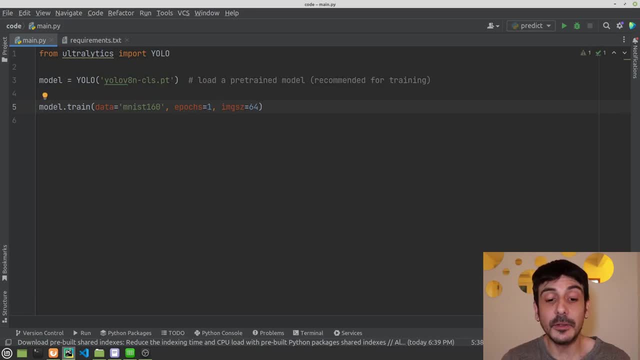 number of a box. I'm going to set it in one right, because the first thing we're going to do is we're going to do a very, very dummy training in order to make sure everything works as expected, in order to make sure everything works properly, and once we are completely and 100 sure everything is okay, we 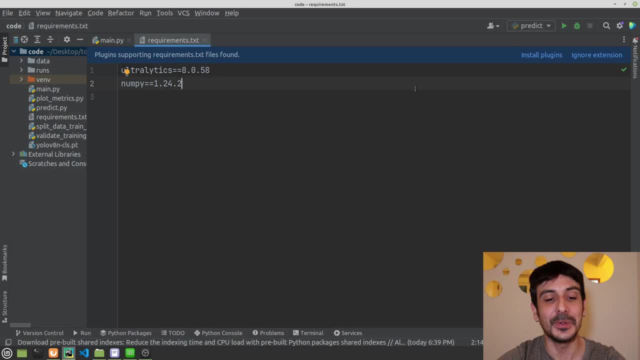 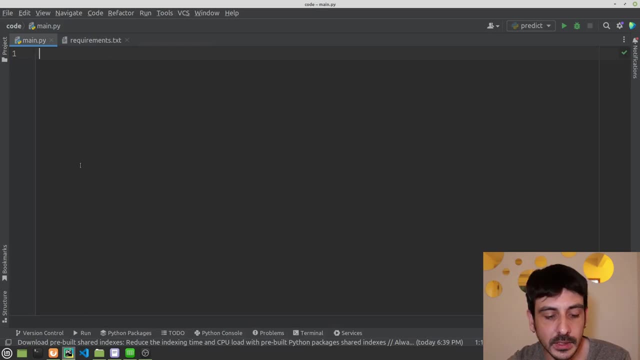 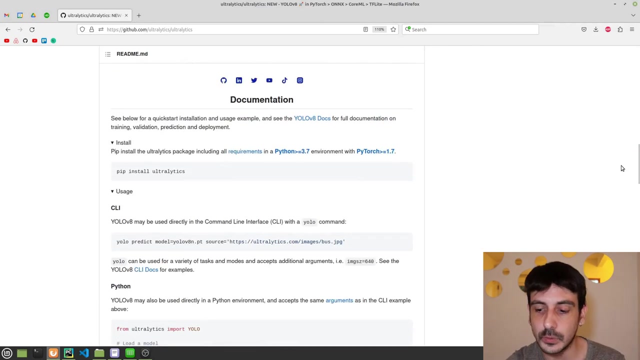 and now you're ready to install your own image classifier using yolovi8. so let's go to main. this is the file we are going to use in order to code everything we need in order to train this classifier, and let me show you the exactly what's the code you need to type in order to do this. 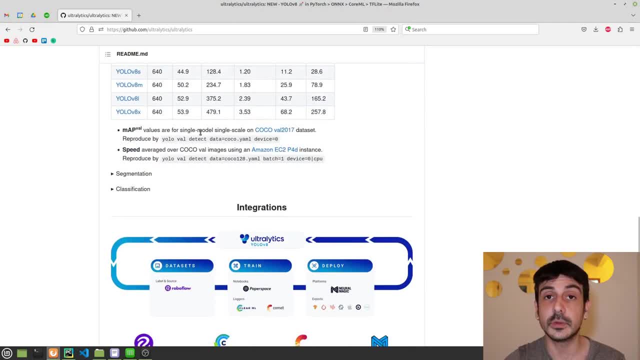 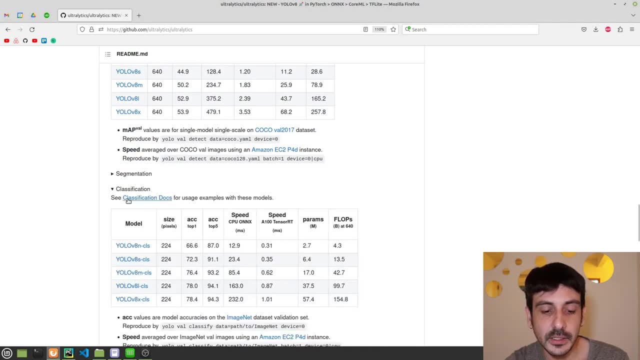 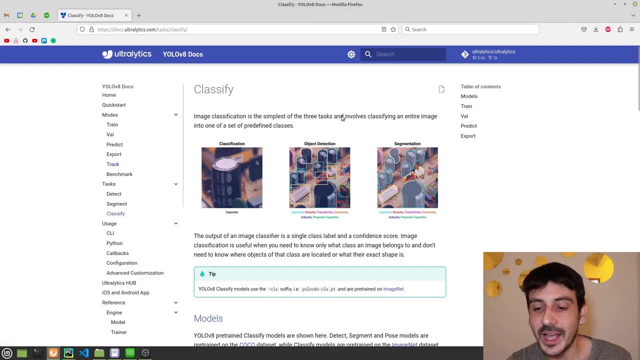 I'm going to over here to the github repository of yolovi8 and I'm going to select the classification section. right, I'm going for the classification and then here I'm going to click on classification ducks. this is going to open a new file, a new URL, a new website, a new page, and this is exactly the. 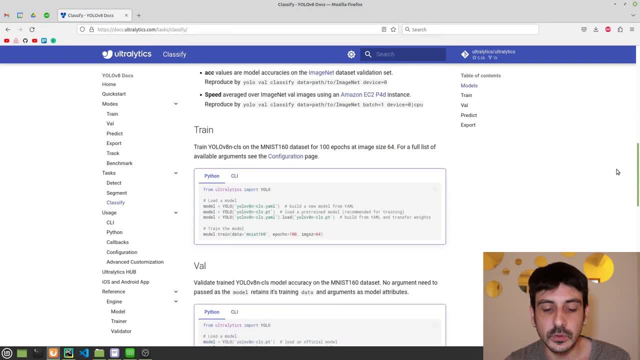 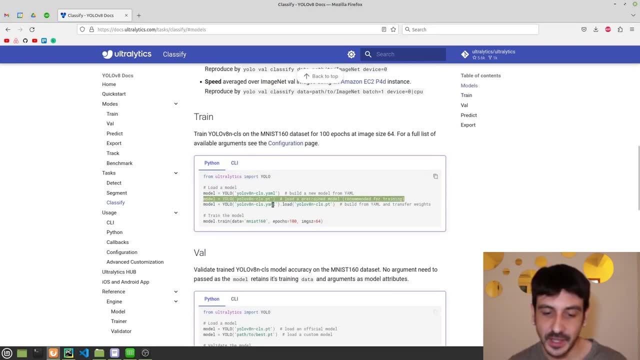 old information we need in order to train this image classifier. I'm just going to scroll down and I'm going to the train section and this is what we're going to do. I'm going to copy and paste this line, which is the one in the middle, the one that says load a pre-trained 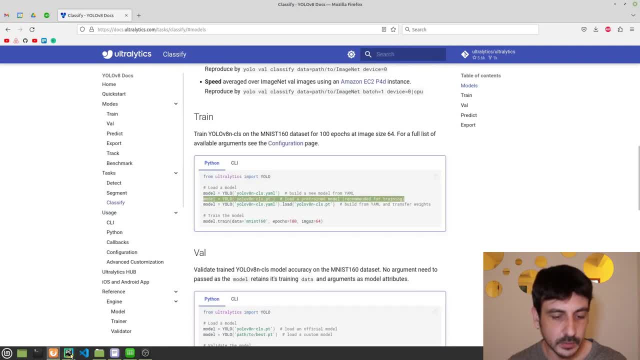 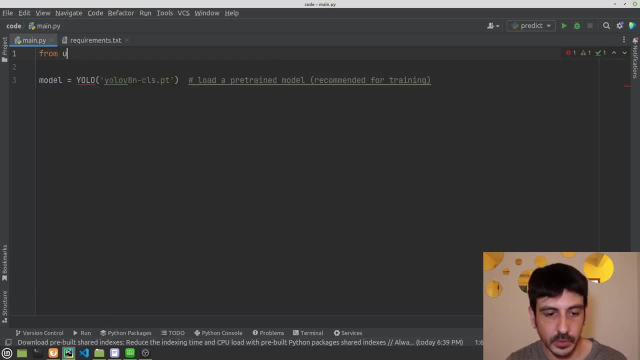 model recommended for training. I'm just going to copy, and then I'm going back to pie charm and I'm just going to paste it. obviously we need to import yolo, otherwise this is not going to work. so I'm going to say: from ultralytics, import yolo. and that's pretty much all you can see now. 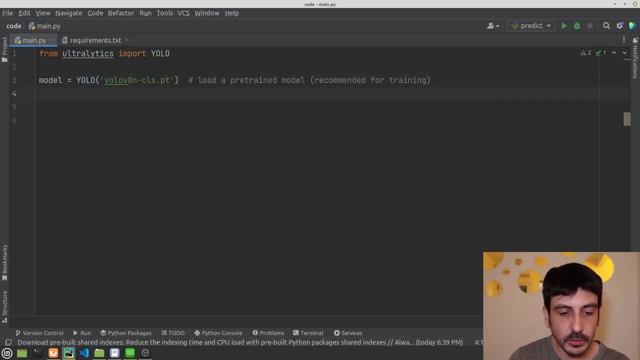 we are creating our model or we are creating the object we are going to use as our model, and then I'm just going to copy and paste this last line, which is modeltrain. I'm going to paste it here, and then I'm going to make a few edits. I'm going to leave like this value. I'm going to 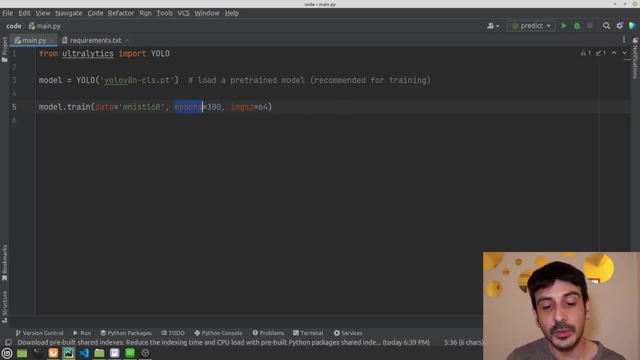 leave the image size in 64, but then, for the number of a box, I'm going to set it in one right, because the first thing we're going to do is we're going to do a very, very dummy training in order to make sure everything works as expected, in order to make sure everything works properly. and once we are, 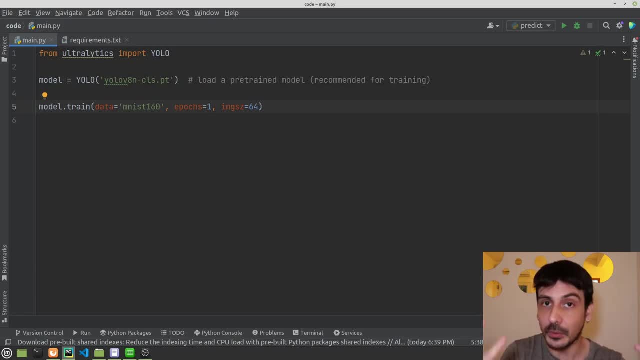 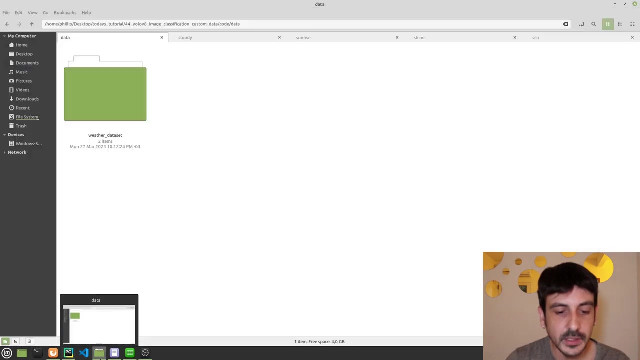 going to move forward with a more deeper training and with a more real training right, but for now, let's just do the training for one Epoch and let's see how it goes then for data, this is where you're going to specify the absolute path to the data you are going to train this model with right in. 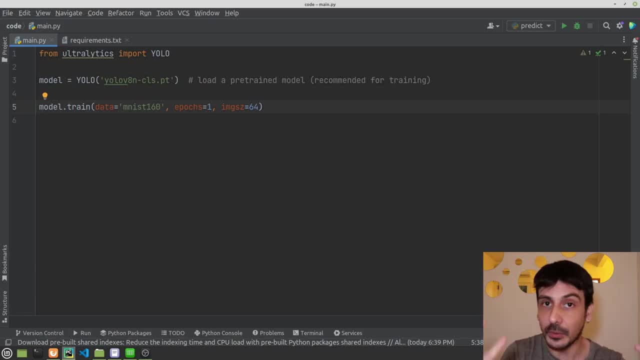 are going to move forward with a more deeper training and with a more real training, right, but for now, let's just do the training for one Epoch and let's see how it goes then for data, these were where you're going to specify the absolute path to the data you are going to train. 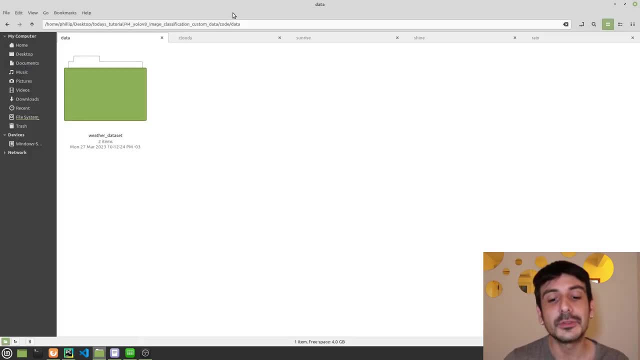 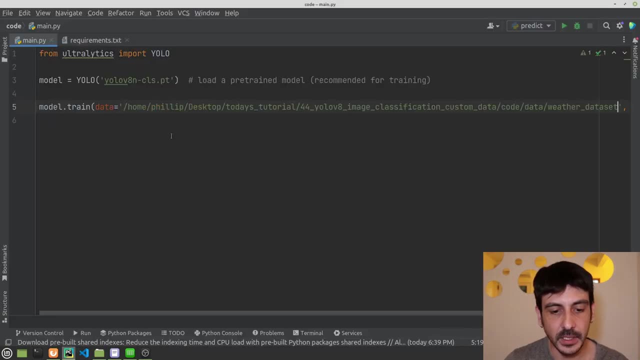 this model with right, in my case, it's going to be this weather data set. so I'm just going to copy and paste the absolute path of this data set, which is this: I'm going to copy this path and I'm going to paste it here. right, this is data I am going to use. remember that you need to specify the absolute. 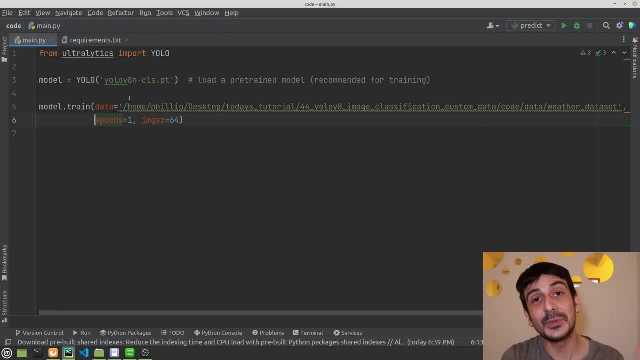 path to the root directory of your data. and remember you need to structure your data into the exact format that you already mentioned, right? otherwise this is not going to work, and that's everything we need in order to train this image classifier, so the only thing I'm going to do is 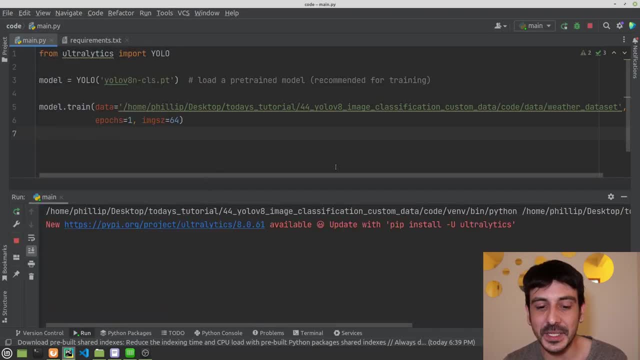 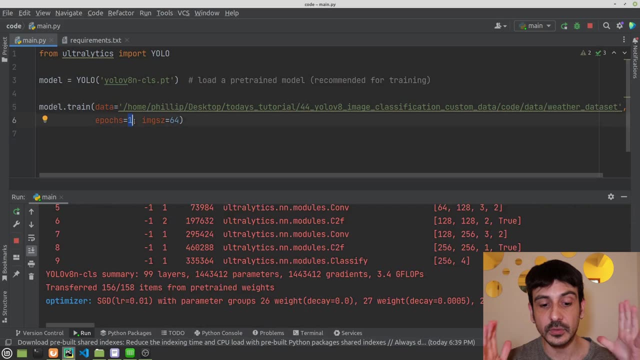 to press play. I'm going to run this script, so let's see what happens. remember we are running this training. we are doing this process for only one Epoch, because we need to make sure everything works properly, and once everything is working properly, we are just going to edit this value. 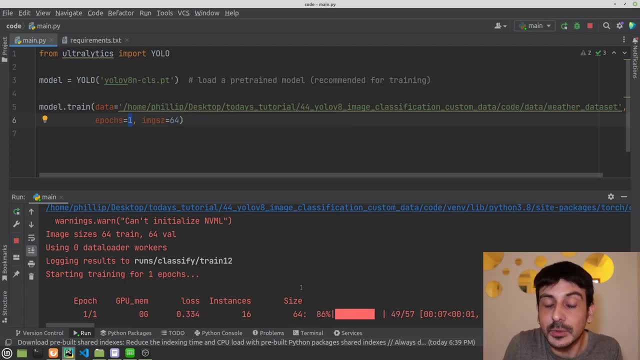 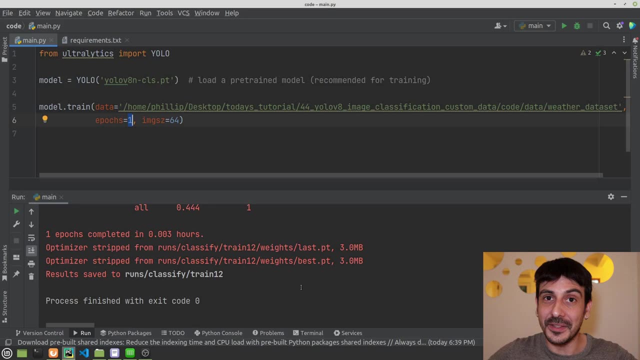 and we're going to make this training for more Epochs. but you can see everything seems to be working properly. so everything seems to be okay and everything seems to be completed and everything seems to be ready. so that's it, and you can see that the results have been saved here in bronze classified. 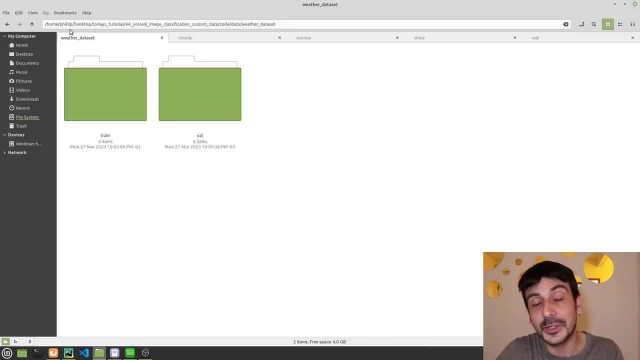 train 12.. so let me show you exactly where this directory, where this location is in my file system. if I go to the project- the Python project I created- into my file system, this is exactly the project I created. this is the file we are currently working in the banepi file. 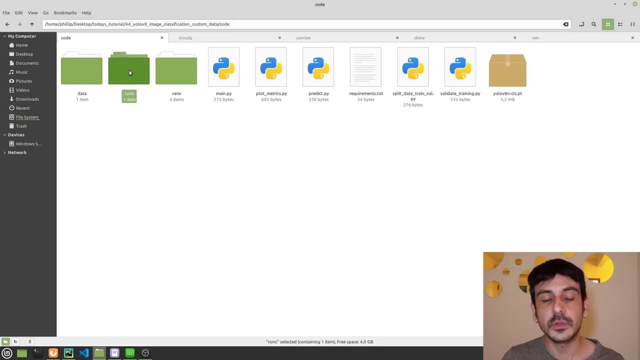 and this is where my data is located, and this is where the runs directory, the runs folder, will be located. this is where we it will be created. you can see that within runs, we have another directory, which is called classify, and here is where you will have many, many, many folders for each one of. 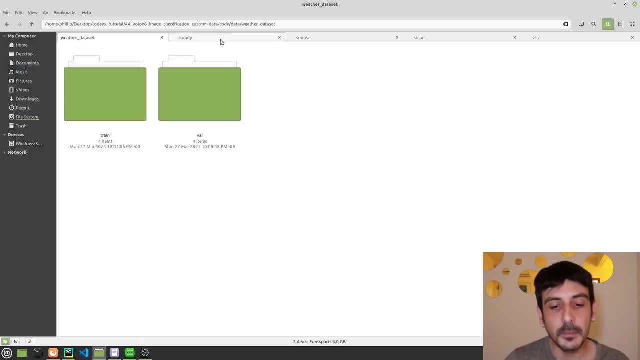 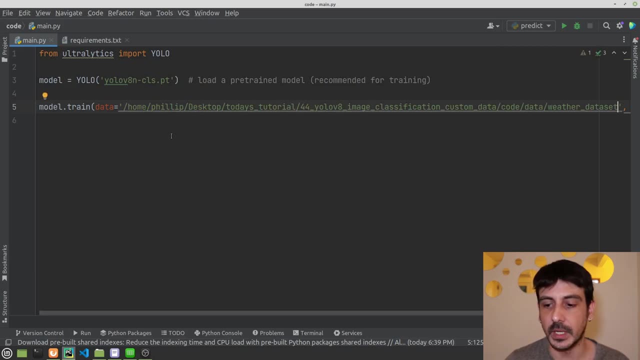 my case, it's going to be this weather data set, so I'm just going to copy and paste the absolute path of this data set, which is this: I'm going to copy this path and I'm going to paste it here. right, this is data I am going to use. remember that you need to specify the absolute path to the root. 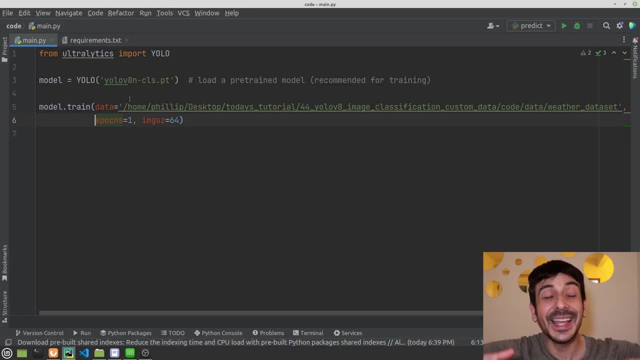 directory of your data, and remember you need to structure your data into the exact format that you already mentioned, right? otherwise this is not going to work, and that's everything we need in order to train this image classifier. so the only thing I'm going to do is to press play. 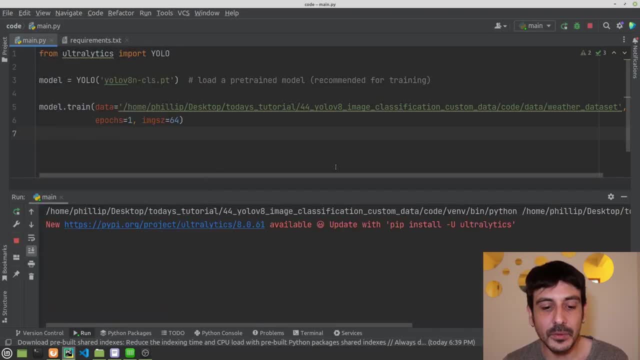 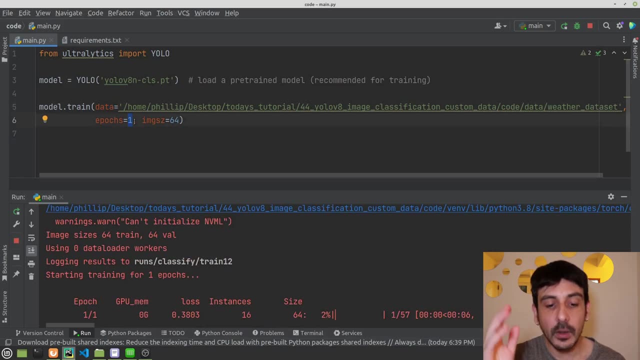 I'm going to run this script, so let's see what happens. remember, we are running this training. we are doing this process for only one Epoch because we need to make sure everything works properly, and once everything is working properly, we're just going to edit this volume. we're going 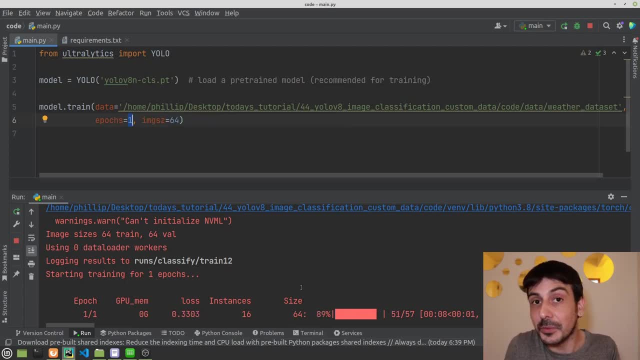 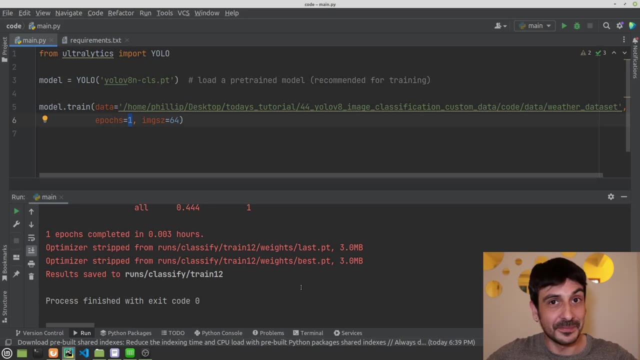 to make this training for more Epochs, but you can see everything seems to be working properly. so everything seems to be okay and everything seems to be completed and everything seems to be ready. so that's it, and you can see that the results have been saved here in bronze classified train 12. so 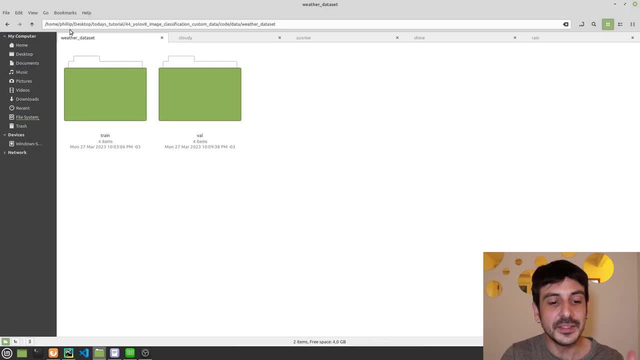 let me show you exactly where this directory, where this location, is in my file system. if I go to the project- the Python project- I created- into my file system, this is exactly the project I created. this is the file we are currently working in, the banepi file, and this is where my data is located. 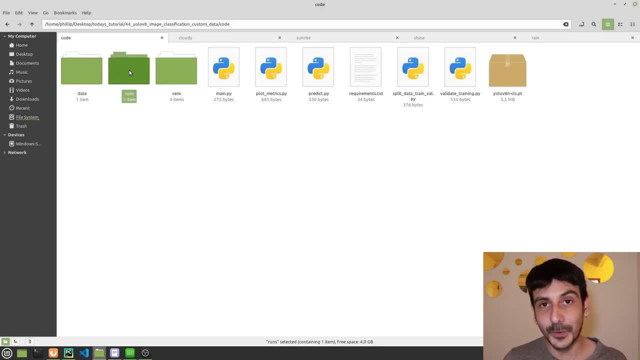 and this is where the runs directory, the runs folder, will be located. this is where we it will be created. you can see that within runs, we have another directory which is called classify, and here is where you will have many, many, many folders for each one of your training processes. 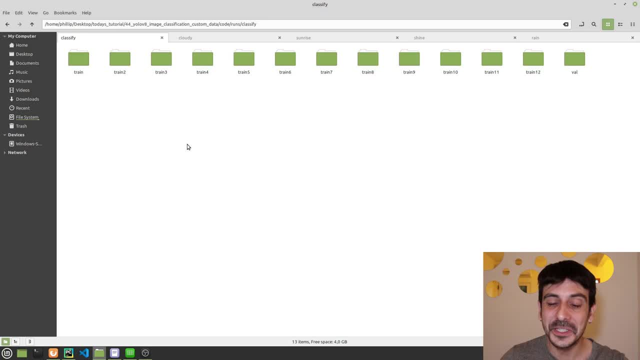 and you can see that, in my case, I have trained this classifier many, many, many different times while I was preparing this video. so there are many directories for me, but this is exactly the one which was just created: the train 12, right train 12.. this is exactly the directory which was just 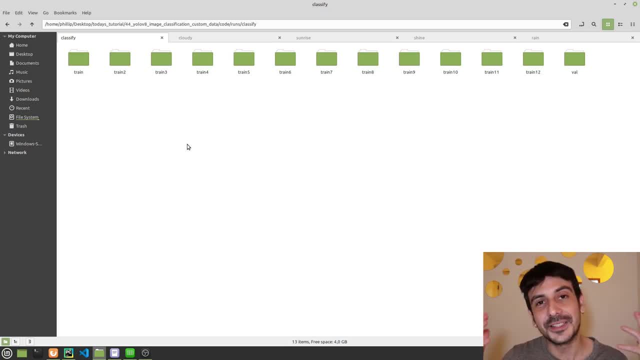 your training processes, and you can see that, in my case, I have trained this classifier many, many, many different times while I was preparing this video. so there are many directories for me, but this is exactly the one which was just created. the train 12, right, train 12. this is exactly the directory which was just 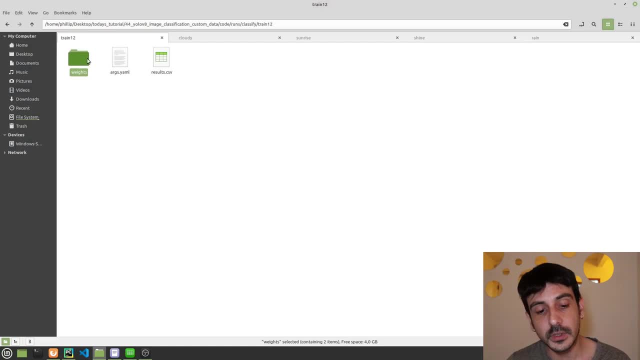 created and if i open this directory, you can see we have a another directory and then we have two files. i'm going to explain what exactly all these different files and all these different folders are and exactly what's the information we have in all these files, but i'm going to do it later. 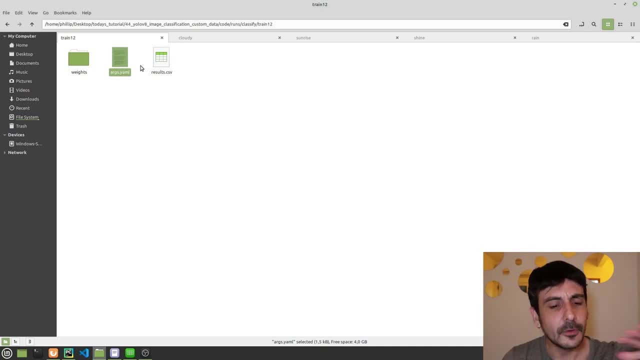 on this tutorial when we are validating this training process. right for now, just remember: all the results will be saved here, will be sell. it will be saved within this folder, within the runs folder, and then within classify, and then a new directory, a new folder will be created for the. 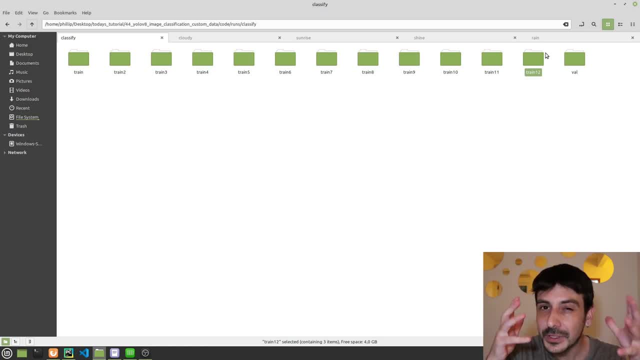 training process you have just executed right. this is something you need to remember for now. but later on this tutorial i'm going to show you exactly how you can validate the training using the information that's within this directory. but for now, let's continue. i'm going to show you now. 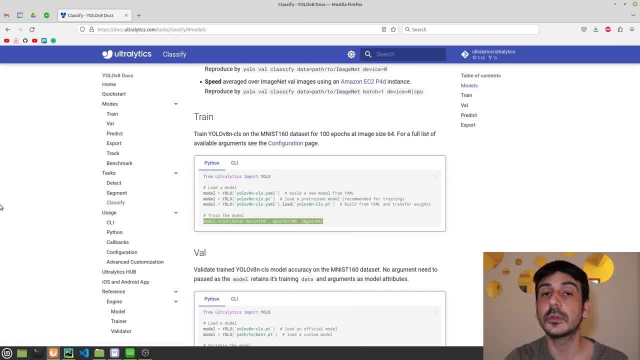 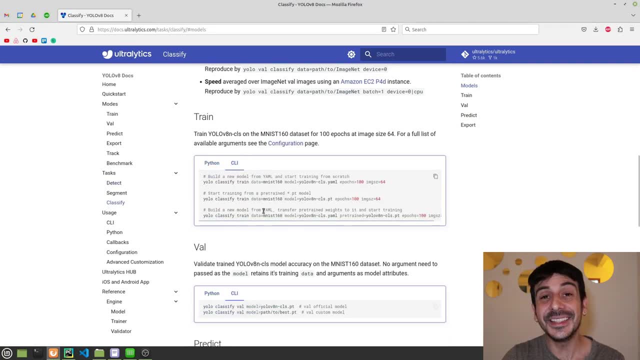 a different one, a different way in which you can train this image classifier using yellow v8. i'm going to, i'm going to show you how to do it using the command line, using this utility, and this is actually like a very, very straightforward way to do this training. let me show you you can. 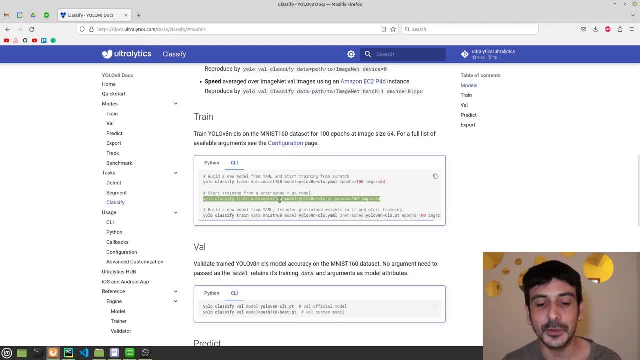 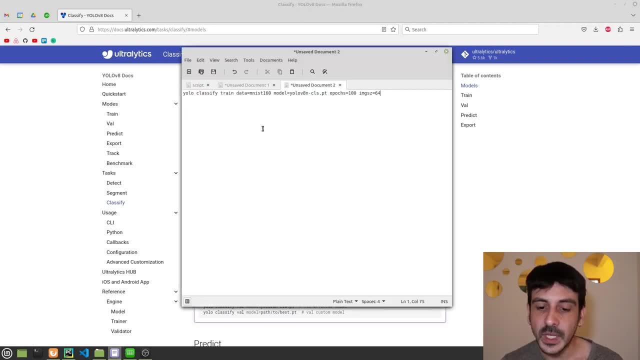 see that we have a three different examples. i'm just going to select this one. i'm going to copy and paste this instruction, this line, and i'm going to show you how to do it. i'm just going to paste it here and you can see that we have many different parameters. right in the first word is: 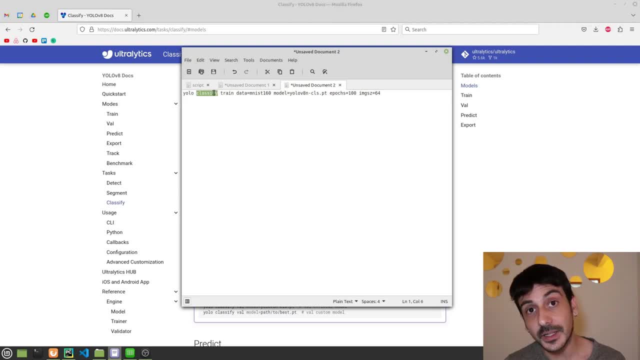 yolo. this is the utility we are going to execute, then classify- this is the task we are going to execute. we are going to train an image classifier and then we are going to train it. so we need we have another keyword, which is train, and then we have these arguments: data model and epochs, and also image size. i'm 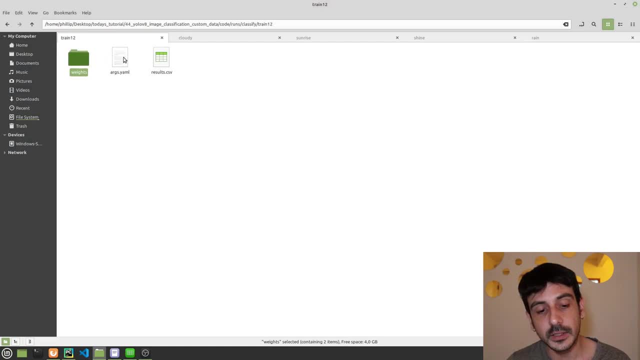 created and if I open this directory, you can see we have a another directory and then we have two files. I'm going to explain what exactly all these different files and all these different folders we have in all these files, but I'm going to do it later on this tutorial when we are validating this. 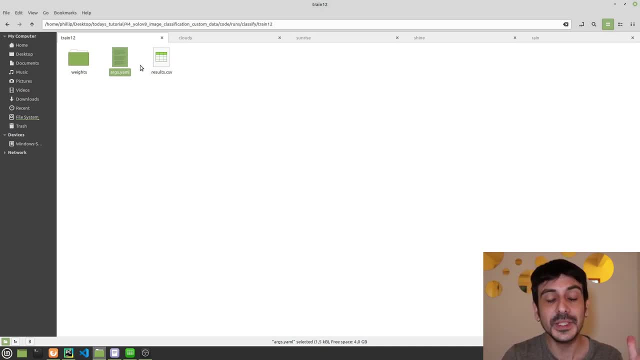 training process. right for now. just remember: all the results will be saved. here will be saved. it will be saved within this folder, within the runs folder, and then within classify and then add new directory. a new folder will be created for the training process. you have just executed right. 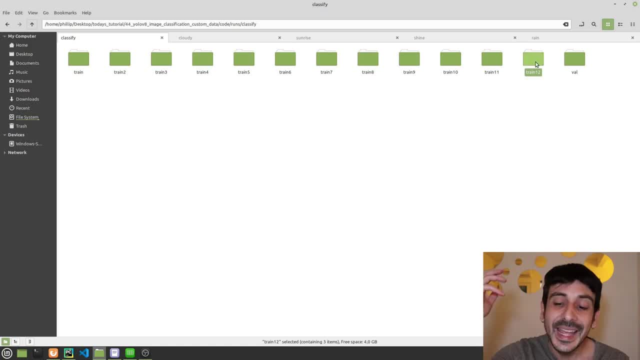 this is something you need to remember for now, but later on this tutorial, I'm going to show you exactly how you can validate the training using the information that's within this directory. but for now, let's continue. I'm going to show you now a different way in which you can train this image classifier using yellow. 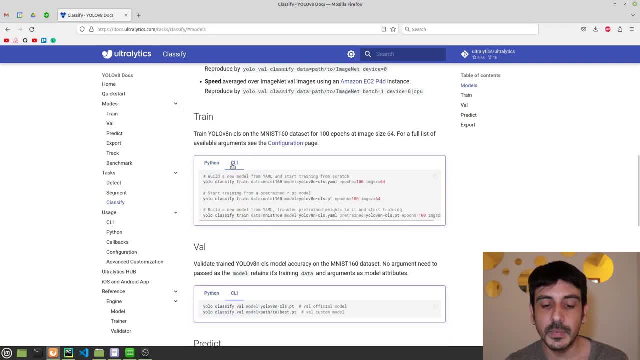 V8 I'm going to, I'm going to show you how to do it using the command line, using this utility, and this is actually like a very, very straightforward way to do this training. let me show you. you can see that we have a three different examples. I'm just going to select this one. I'm going to copy. 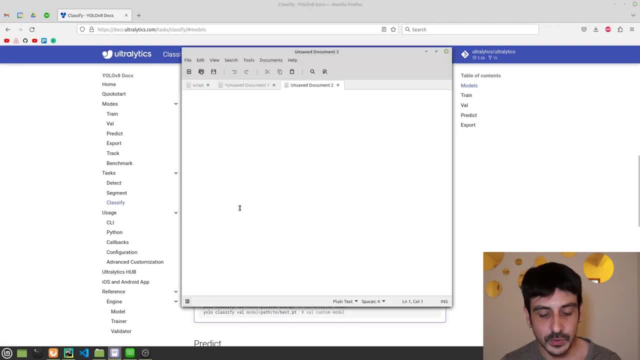 and paste this instruction, this line, and I'm going to show you how I do it. I'm just going to paste it here and you can see that we have many different parameters. right in the first, uh world is Yolo. this is the utility we are going. 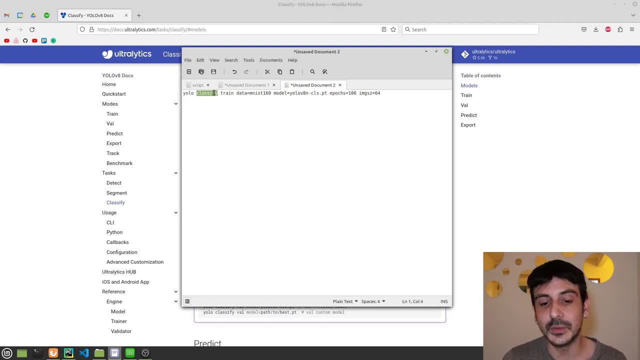 to execute, then classify. this is the task we are going to execute. we are going to train an image classifier and then we are going to train it. so we need we have another keyword, which is train, and then we have these arguments: data model and Epoch, and also image size. I'm going to do exactly the 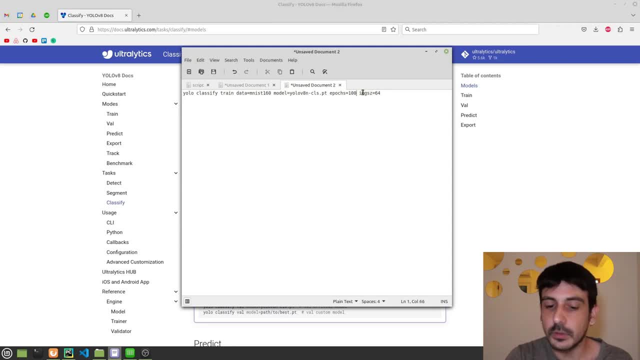 to leave this value in 64, but then i'm going to edit all the other values. so actually i'm going to edit number of epochs, epochs, and i'm also going to edit data for the number of epochs. let's do something similar. i'm just going to do it for one epoch, so we make sure everything runs smoothly. 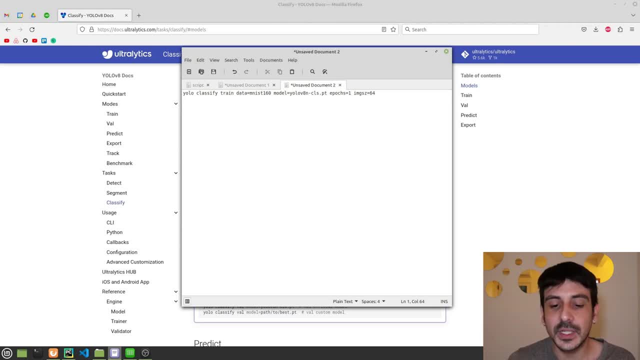 and everything runs properly, and then we can do like a more serious training, a more real training for more epochs. this is exactly the model i'm going to use, so i'm not going to edit this a keyword either. and then i'm going to edit this argument and i'm just going to say this is the. 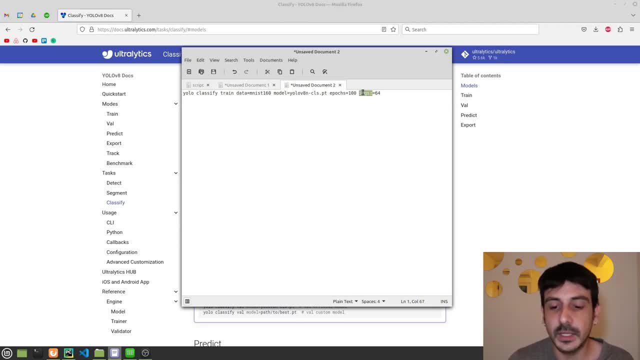 going to do exactly the same with image size. i'm just going to leave this value in 64, but then i'm going to edit all the other values. actually, i'm going to edit number of epochs, epochs, and i'm also going to edit data for the number of epochs. let's do something similar. i'm just going to do it for one epoch. 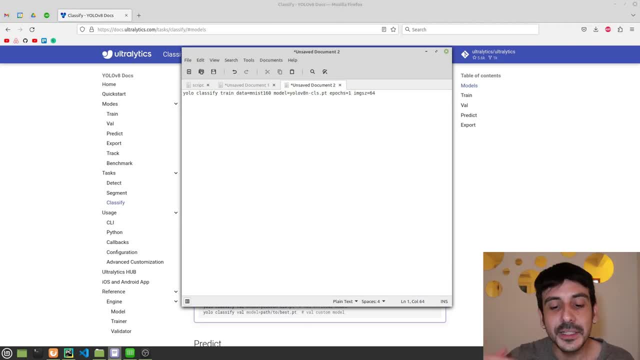 so we make sure everything runs smoothly and everything runs properly, and then we can do like a more serious training, a more real training for more epochs. this is exactly the model i'm going to use, so i'm not going to edit this a keyword either, and then i'm going to edit this argument. 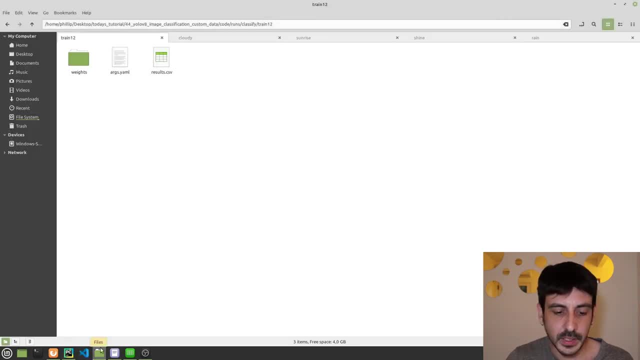 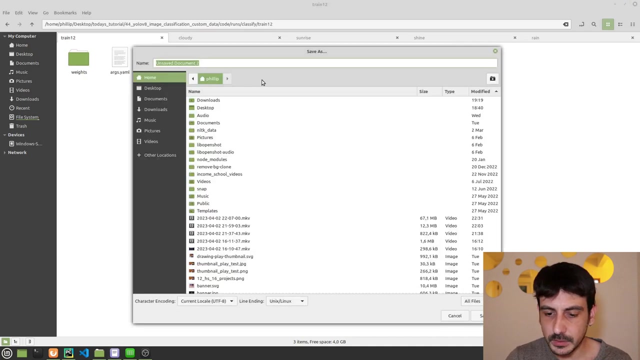 and i'm just going to say this is the absolute path to my data. so this is going to be exactly the same as i have over here, something like this: okay, and that's pretty much all the only thing i need to do now. i'm going to 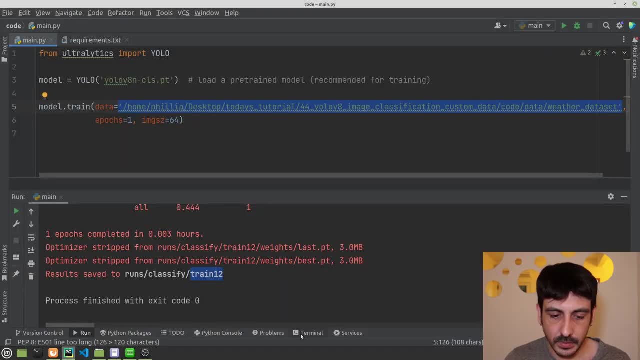 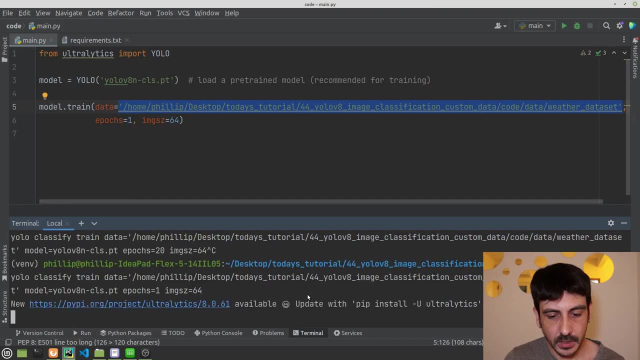 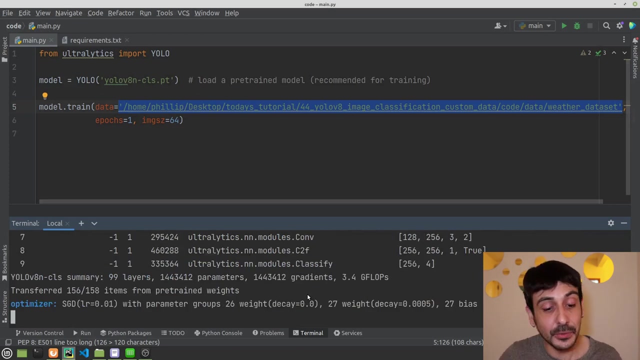 copy and paste this sentence and i'm just going to the terminal and i'm going to do something like this. right, i'm just copying, i have just copy and pasted that sentence and you can see that that's all we need to do in order to train this image classifier, just in the v8. you. 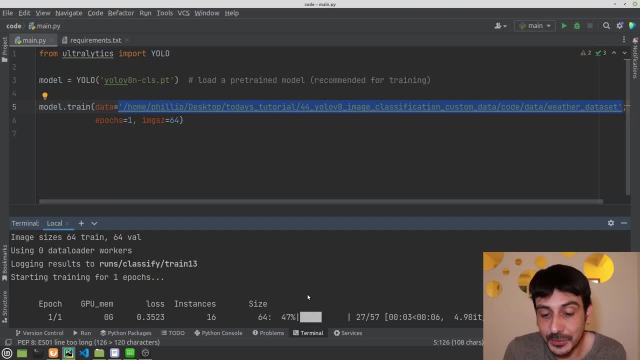 that the model, the training process, has started and everything is running super, super smoothly. so everything is going super, super well. that's all right. that's a very, very quick way and a very straightforward way to do this training. you can see, the training has just- has just been completed. 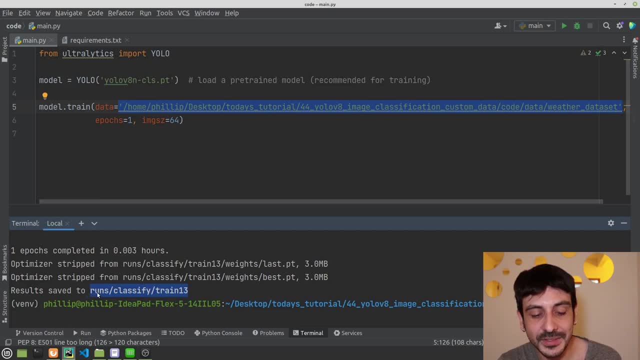 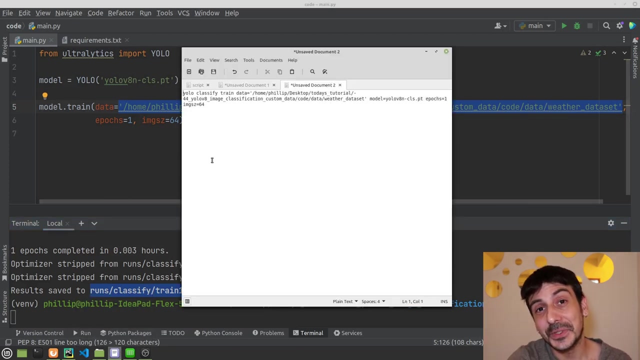 and this is exactly where the results have been saved- to runs classifier train 13.. so everything is completed, everything is ready. you can see how simple, how fast is to train an image classifier just by running this command. now i'm going to show you another way to do this training, which is using 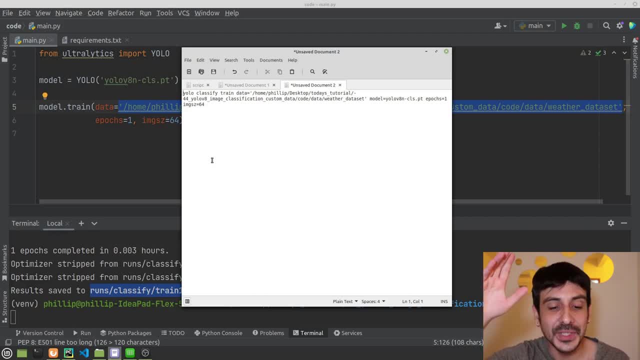 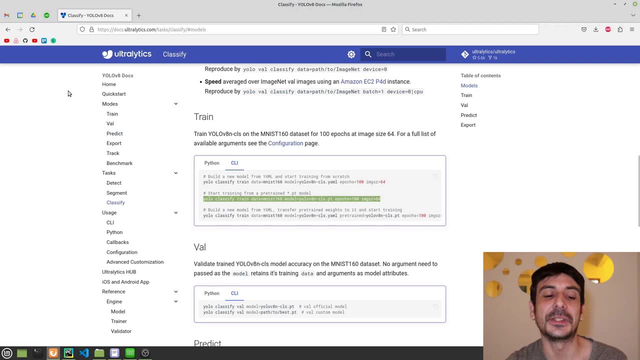 a google collab. we are going to use a jupyter notebook. we are going to use a notebook in a google collab in order to train this model, and this is also like a very good way to do it, so let me show you how to do it. so, basically, you need to go to google drive, you need to go to your google. 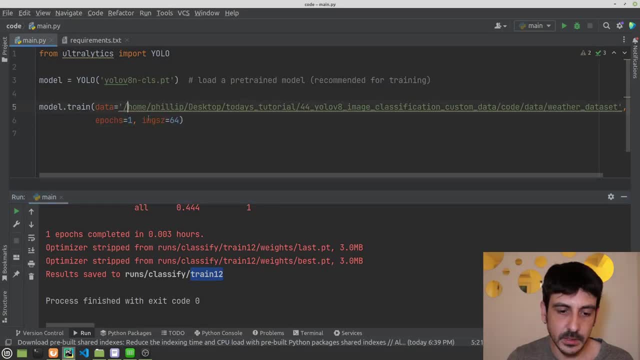 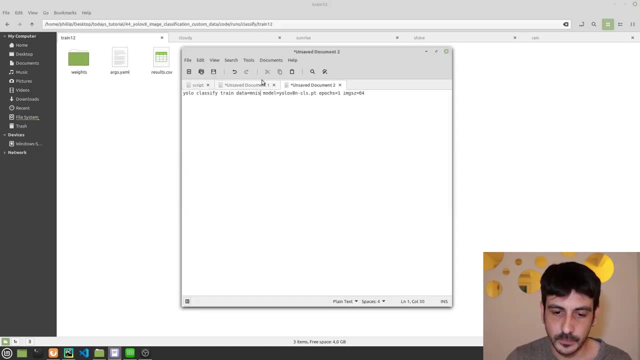 absolute path to my data. so this is going to be exactly the same as i have over here, something like this: okay, and that's pretty much all the only thing i need to do now. i'm going to copy and paste this sentence and i'm just going to a terminal and i'm going to do: 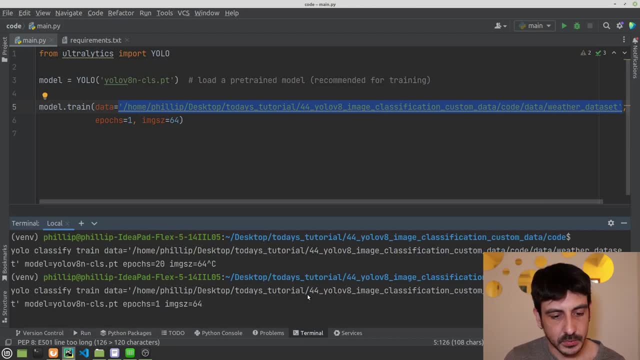 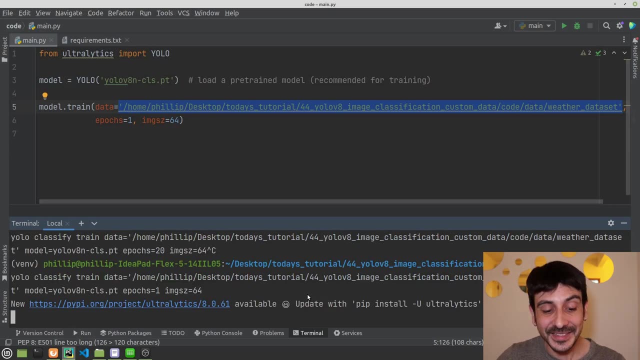 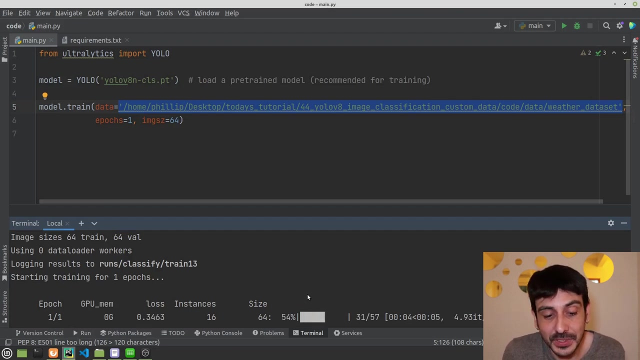 something like this. right, i'm just copying. i have just copy and paste that sentence and you can see that that's all we need to do in order to train this image classifier using w8. you can see that the model, the training process, has started and everything is running super, super smoothly. so 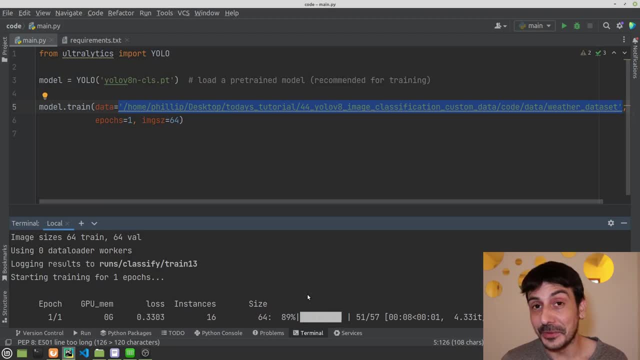 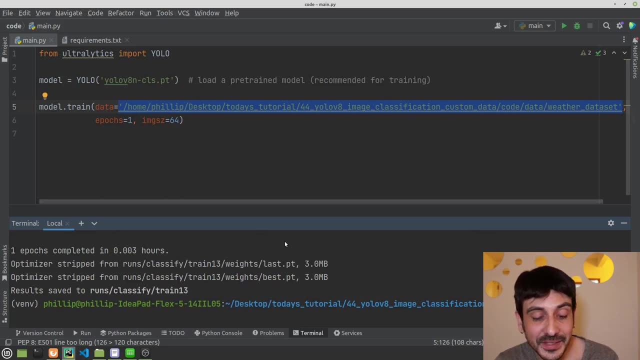 everything is going super, super well. that's all right. that's a very, very quick way and a very straightforward way to do this training. you can see, the training has just, has just been completed, and this is exactly what we're going to do next, where the results have been saved to runs classifier, train 13.. so everything is completed. 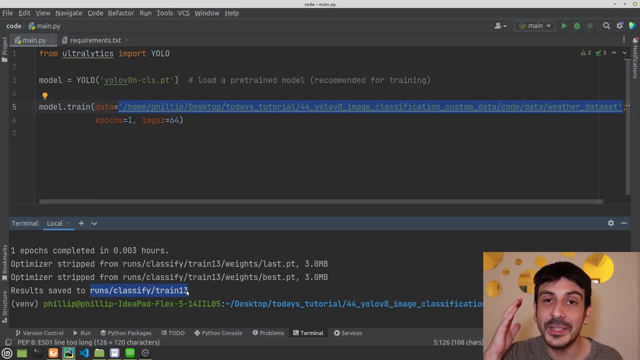 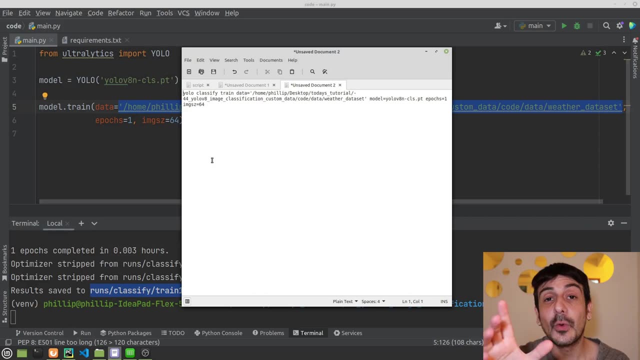 everything is ready. you can see how simple, how fast is to train an image classifier just by running this command. now i'm going to show you another way to this training, which is using a google collab. we are going to use a jupyter notebook. we are going to use a notebook in a google collab, in. 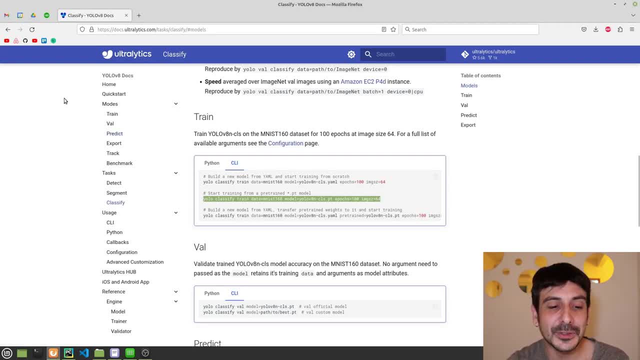 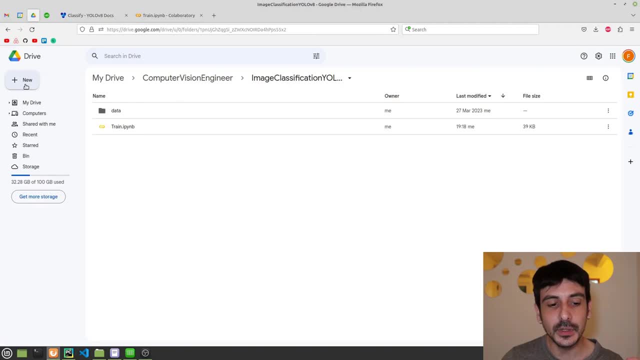 order to train this model, and this is also like a very good way to do it, so let me show you how to do it. so, basically, you need to go to google classifier and then you need to go to google classifier and to google drive. you need to go to your google drive, you need to select new, then more. 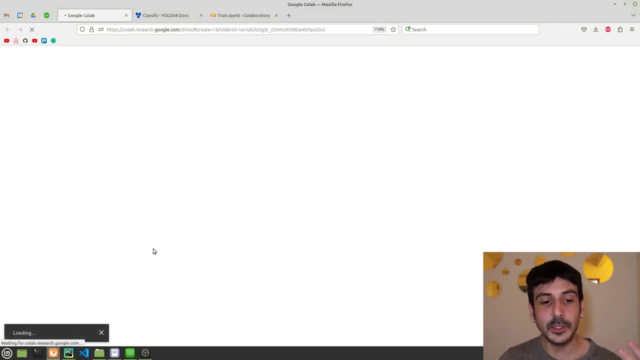 google collaboratory, and this is going to open a new notebook. this is going to open a new notebook in google collab, and this is exactly what you need to do in order to use this notebook to train your v8. now i'm going to show you a notebook i have already created in. 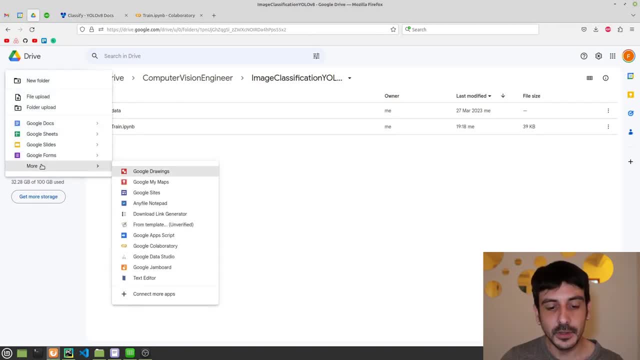 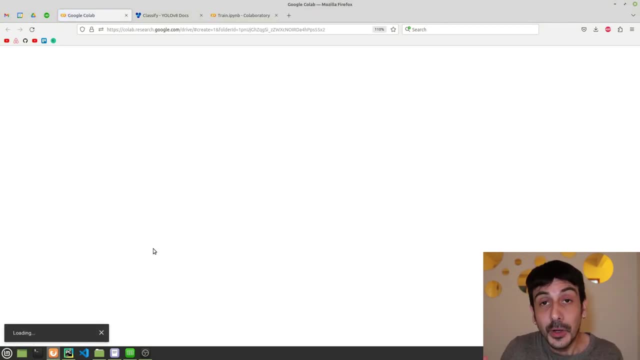 drive you need to select new, then more google collaboratory, and this is going to open a new notebook. this is going to open a new notebook in google collab, and this is exactly what you need to do in order to use this notebook to train your v8. now i'm going to show you a notebook i have already created in. 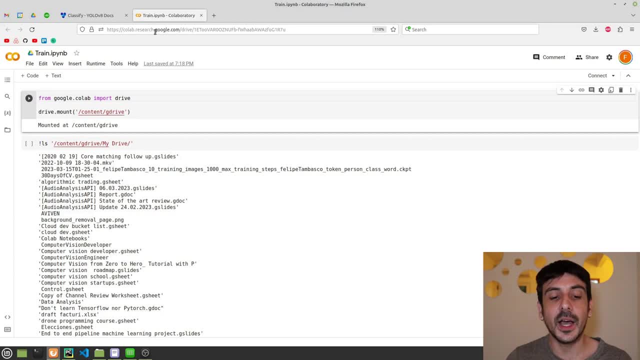 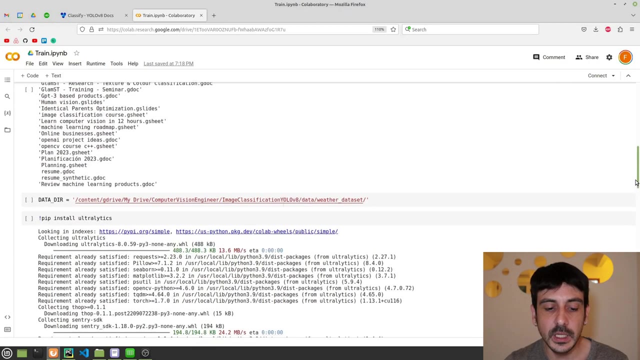 order to train this model, which is this one is called train dot ip, y m b and obviously i'm going to give you exactly this notebook in the github repository of today's video, of today's tutorial, so you can just use this notebook if you want. now i'm going to show you all these different. 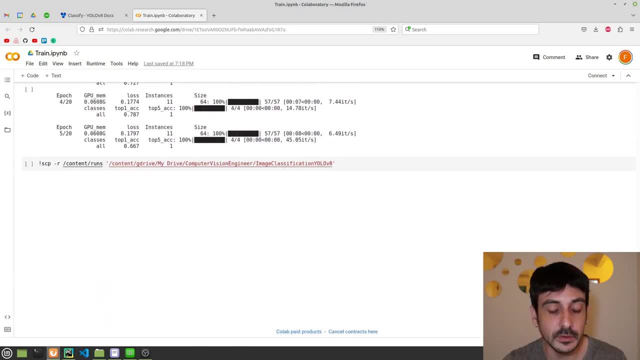 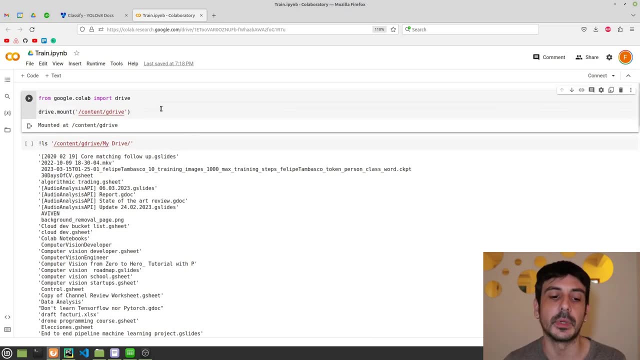 cells, of everything that that's already written on this notebook so you can, so you understand how exactly to use it and how it works and what exactly you are doing at each step. so let's start with the first step, another thing you need to do if you. 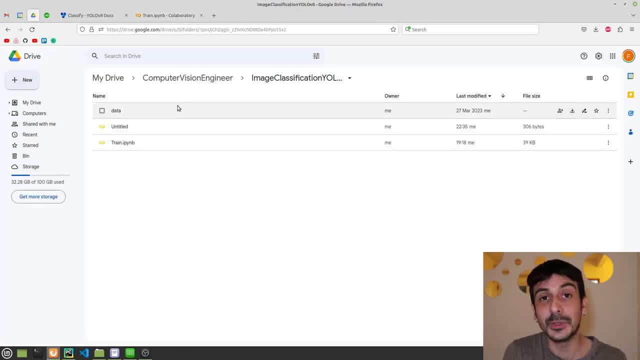 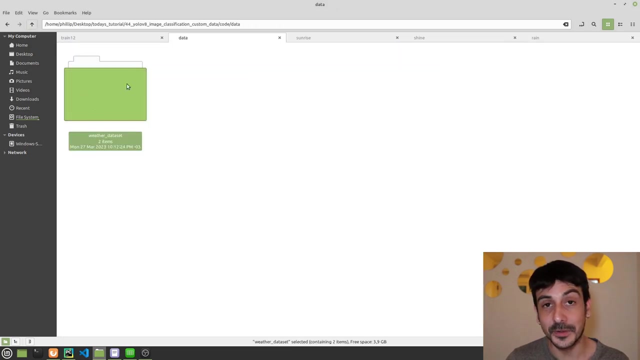 want to train this image classifier is to upload all the data, with all the images and with all your categories, into google drive, obviously. for example, in my case, this is where i have my weather data set. you can see that this directory is exactly the same directory i have over here: weather data set. 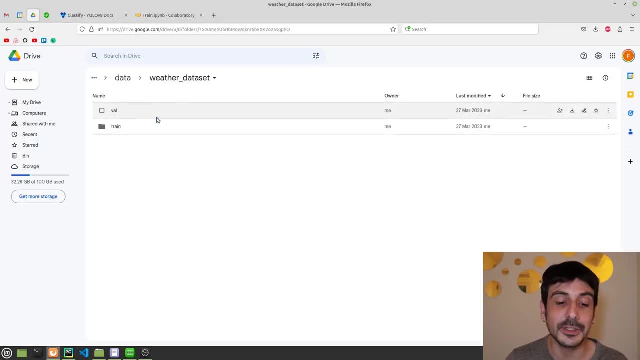 are two directories which are train and ball. if i, if i open this directory, you can see we also have three and balls. so this is exactly exactly the same data as in my local computer. now, this is something very important because remember to do it, because you need the data in your google drive in. 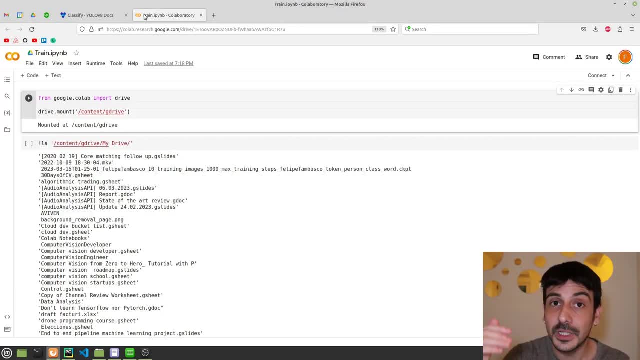 order to train this ball using a google call up. this is a very, very important step. please remember to upload your data into google drive now. once your data is in google drive, then you need to be able to connect your data from the google call app, and in order to do that, you need to execute this. 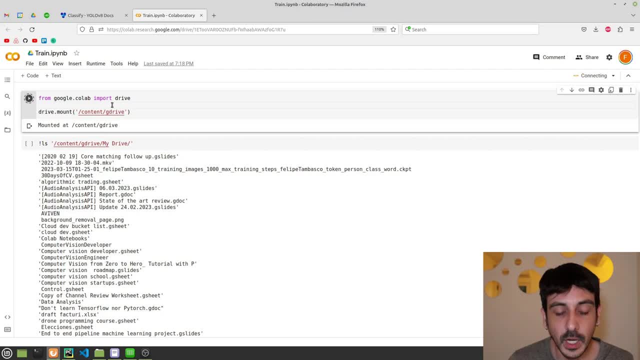 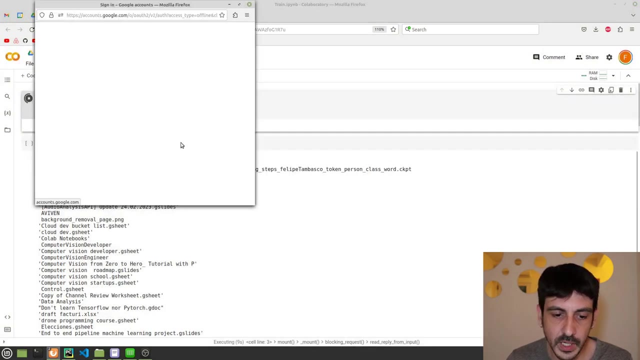 cell. if i click enter, you can see that now you are, i'm going to be asked if i want to connect google call up with google drive and the only thing i need to do is to say i accept. there you can see that it's requesting for my permission. i i say connect to google drive and then i select my 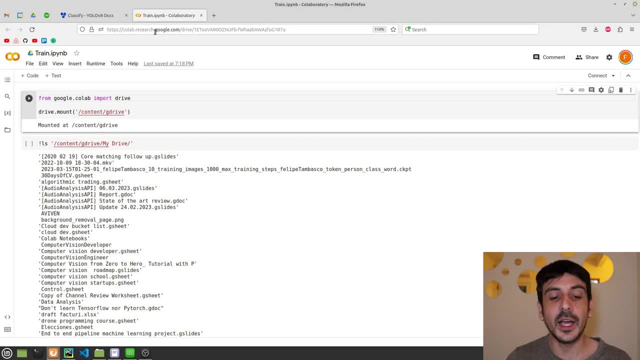 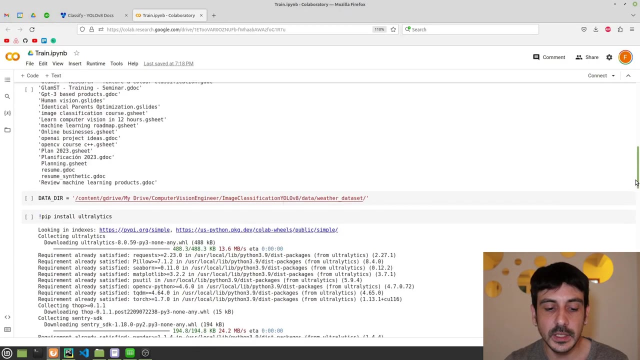 order to train this model, which is this one is called train dot ip, y m b and obviously i'm going to use exactly this notebook in the github repository of today's video, of today's tutorial. so you can just use this notebook if you want. now i'm going to show you all these different. 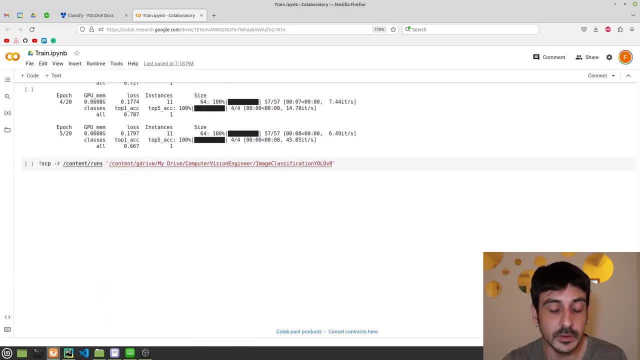 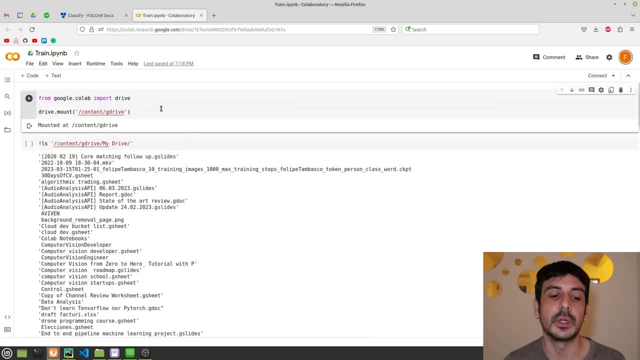 cells, of everything that that's already written on this notebook so you can, so you understand how exactly to use it and how it works and what exactly you are doing at each step. so let's start with the first step, the another thing you need to do if you want to train this image. 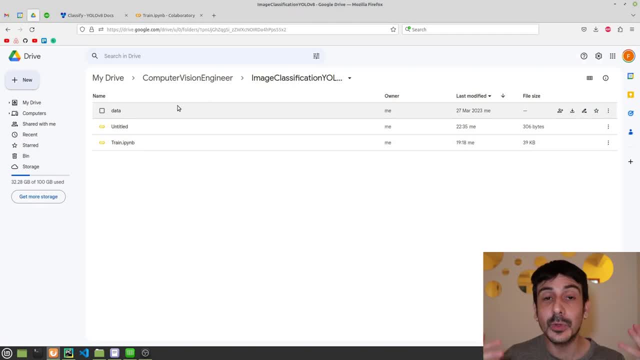 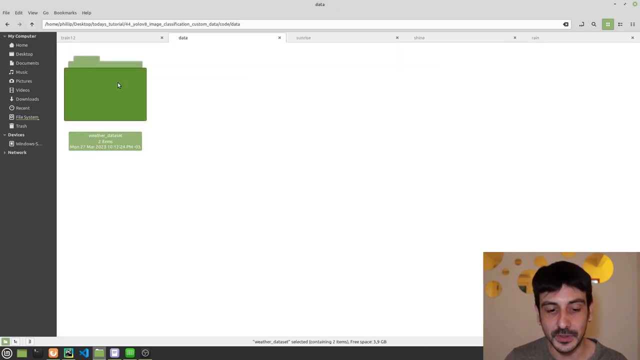 classifier is to upload all the data, with all the images and with all your categories, into google deep, for example. in my case, this is where i have my weather data set. you can see that this directory is exactly the same directory i have over here weather data set within weather data set there. 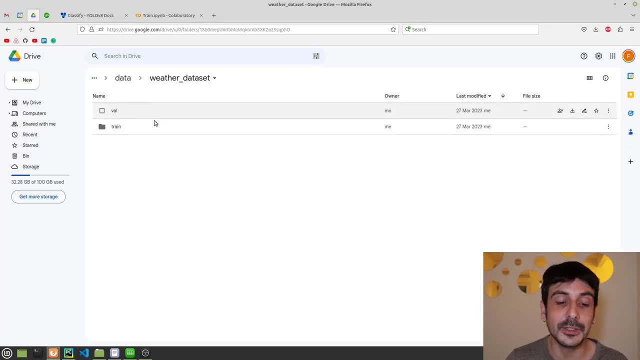 are two directories which are train and ball. if i, if i open this directory, you can see we also have three and balls. so this is exactly exactly the same data as in my local computer. now, this is something very important because remember to do it, because you need the data in your 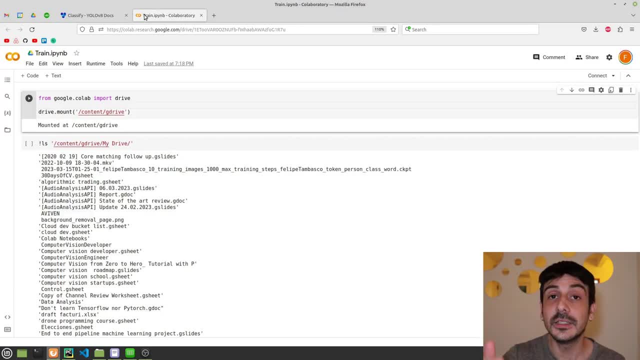 google drive in order to train this ball using a google computer call up. this is a very, very important step. please remember to upload your data into google drive now. once your data is in google drive, then you need to be able to access your data from the google call up, and in order to that, you need to execute this cell. if i click enter, you can see: 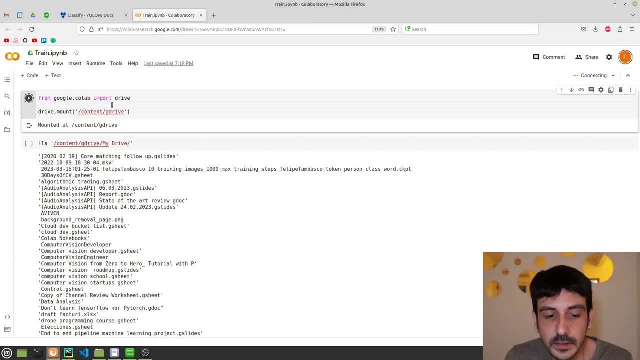 that now you are. i'm going to be asked if i want to connect google, call up with google drive, and the only thing i need to do is to say i accept, and then you can see that it's requesting for my permission. i i say connect to google drive. 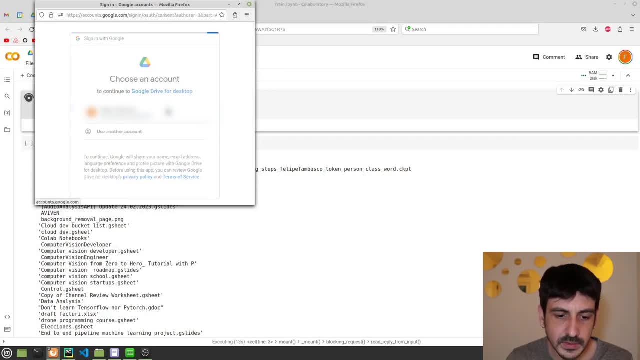 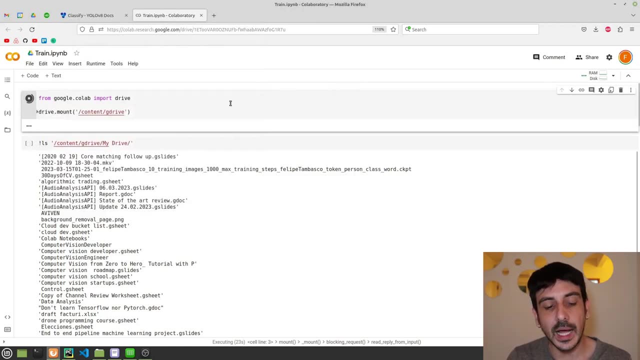 and then i select my account and then basically, is to go scroll down to the bottom of this page and to click allow, and this is going to allow google call up to access all the data you have in your google drive. so this is a very, very, very important step. now, the something that's 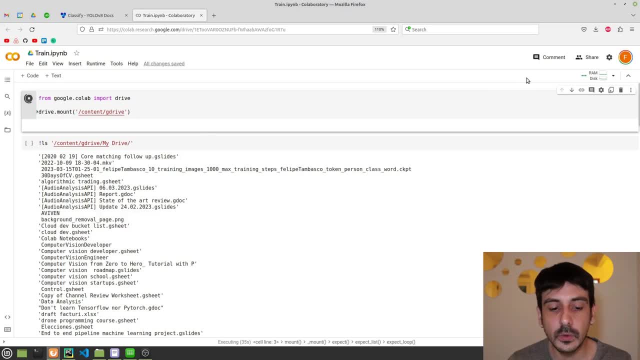 very important is that you need to be able to access your data, so you need to know where your is located in the google drive, right? you need to know exactly what's the path, what's the location of your data in google drive. in my case, let me show you my google drive. you can see that my data 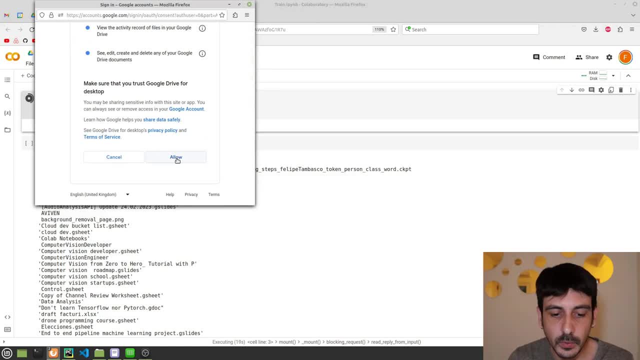 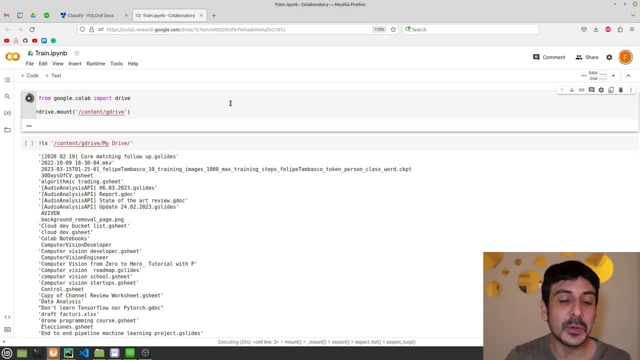 account and then, basically, is to go the bottom of this page and to click allow, and this is going to allow google collab to access all the data you have in your google drive. so this is a very, very, very important step. now, the something that's very important is that you need to be able to access your data, so you 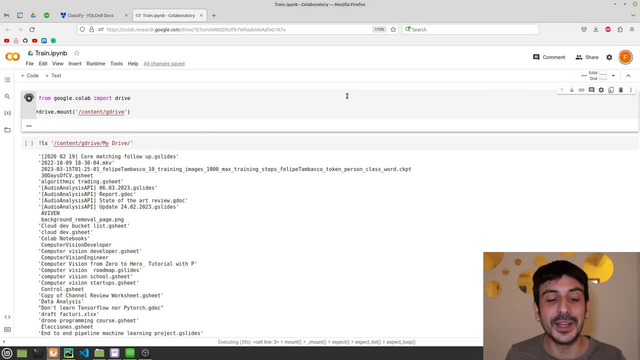 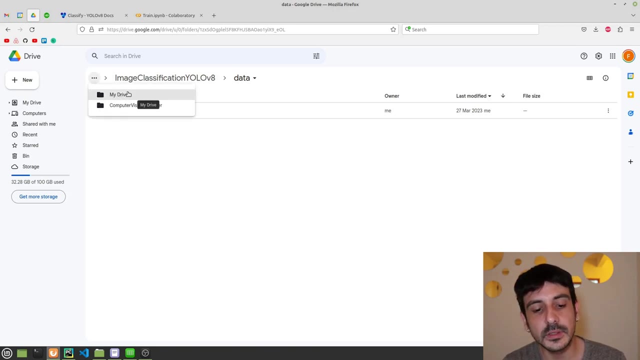 need to know where your data is located in the google drive, right? you need to know exactly what's the path, what's the location of your data in google drive. in my case, let me show you my google drive. you can see that my data is located into a directory. this is my root directory, which is my drive. then i have another. 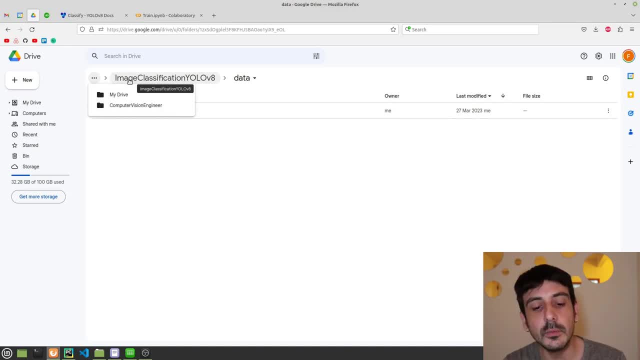 directory which is called computer vision engineer, then another directory which is image classification, euro v8, and then data, and then this is where my weather data set is located. in your case it's going to be different, obviously. it depends on where exactly you have uploaded your data. so 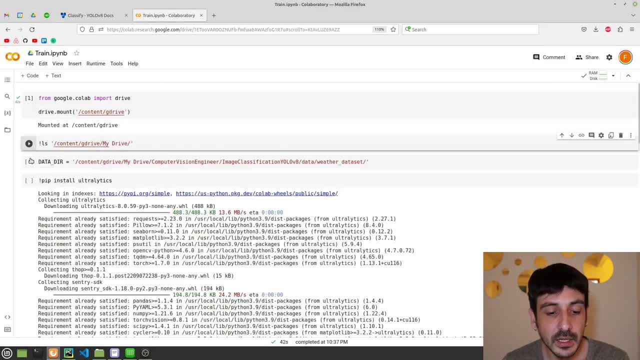 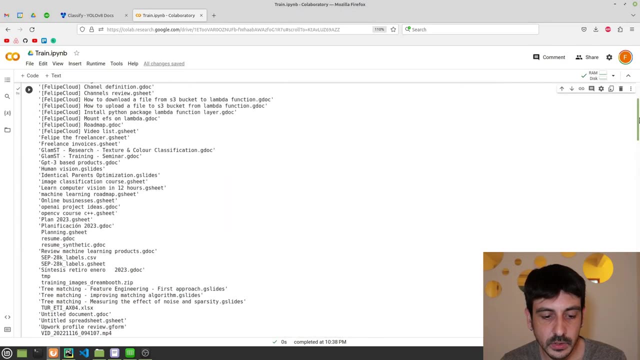 something you may want to do is just to click this ls. you can say something like ls and then you say something like: content: my g drive, my drive, right, you execute this command. and if i execute this command, you're going to see a very, very long list of files, which are basically all the files which 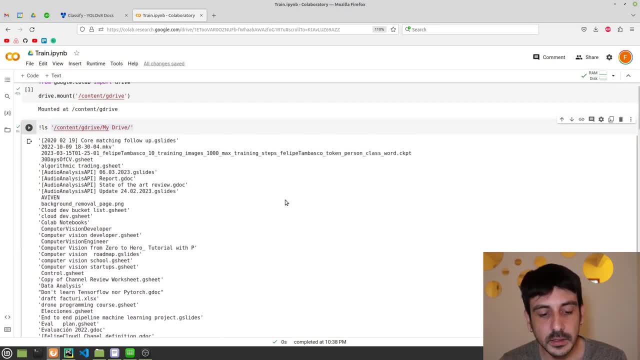 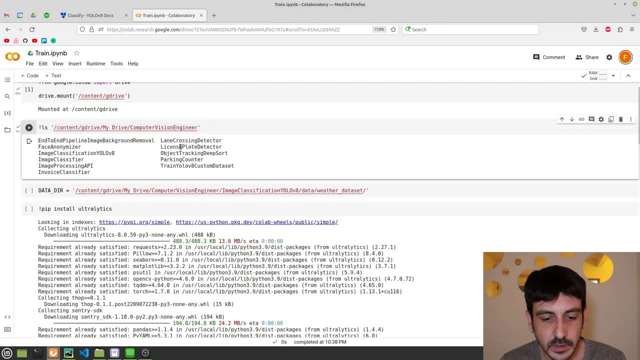 are in my root directory in google drive and, for example, this, where i have the directory which is called computer vision engineer, and if i do ls, you are going to see all these different directories. if i say something like image classification, yellow, v8, then And this is data train dot YIP, YMB, which is exactly this notebook. 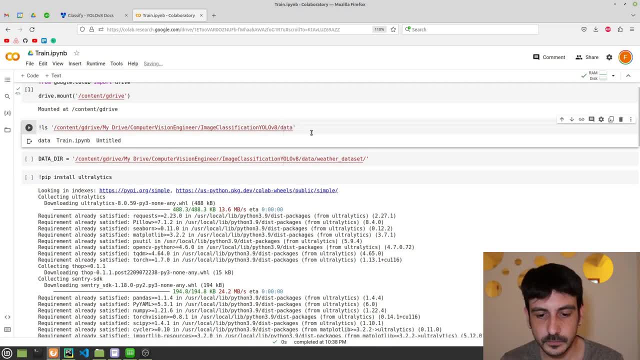 And then, if I say data, this is exactly where the weather data set is located, right? So do something like that, because you definitely need to know what is the path of your data in Google Colab, right? You definitely need to do it in order to continue to the next step. 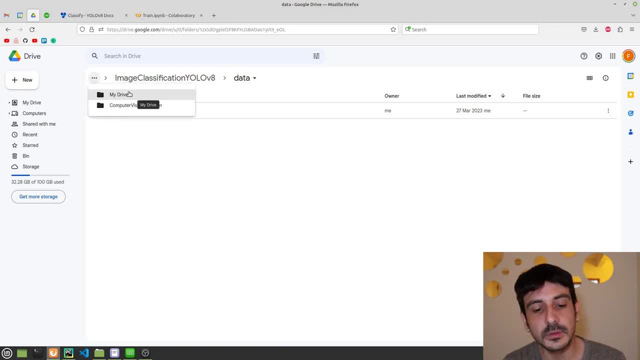 is located into a directory. this is my root directory, which is my drive. then i have another directory which is called computer vision engineer, then another directory which is image classification, euro v8, and then data, and then this is where my weather data set is located. in your case, it's going: 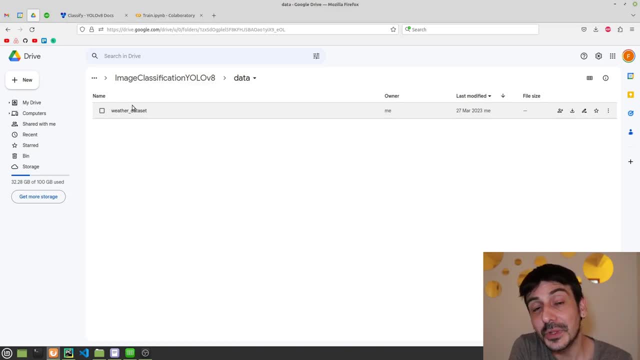 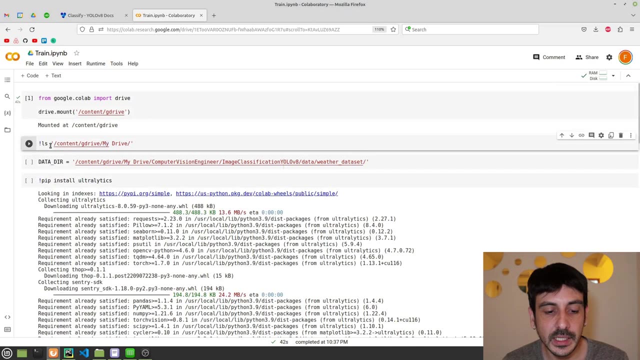 to be different. obviously, it depends on where exactly you have uploaded your data. so something you may want to do is just to click this ls. you can say something like ls and then you say something like content: my g drive, my drive, right, you execute this command. and if i execute this command, you're. 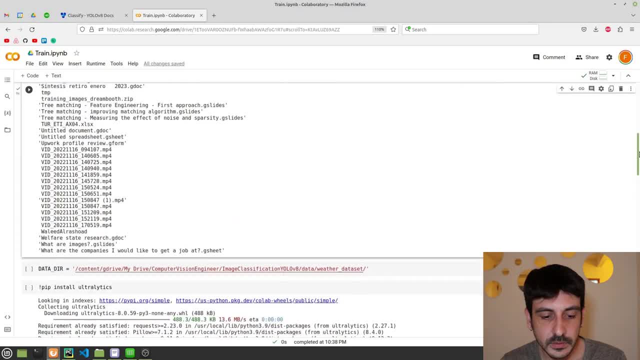 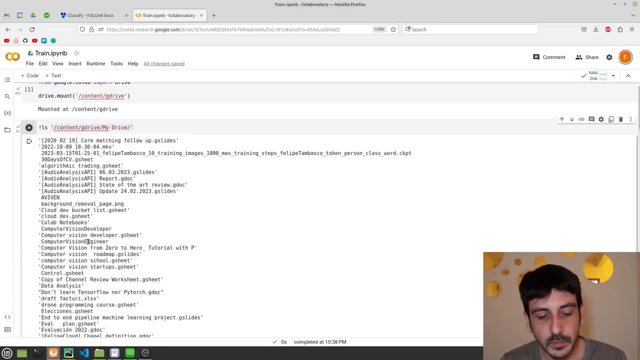 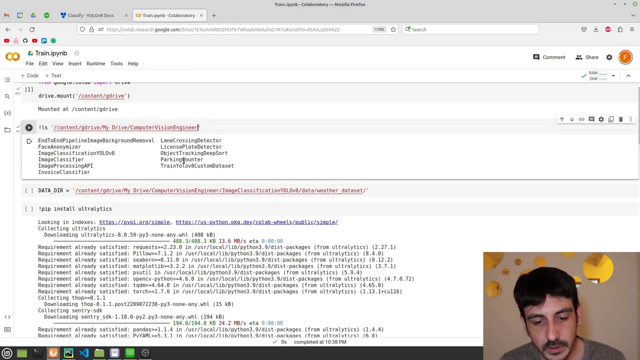 going to see a very, very long list of files, which are basically all the files which are in my root directory in google drive and, for example, this is where i have the directory which is called computer video engineer and if i do ls, you're going to see all these different directories. if i say something like image classification, yellow v8- 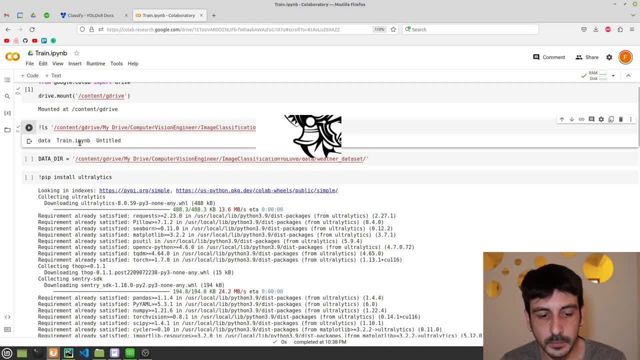 then this is data train dot y, ip y mb, which is exactly this notebook. and then, if i say data, this is exactly where the weather that set is located, right, so do something like that, because you definitely need to know what is the path of your data in google. call up, right? you definitely need to do it in order to continue. 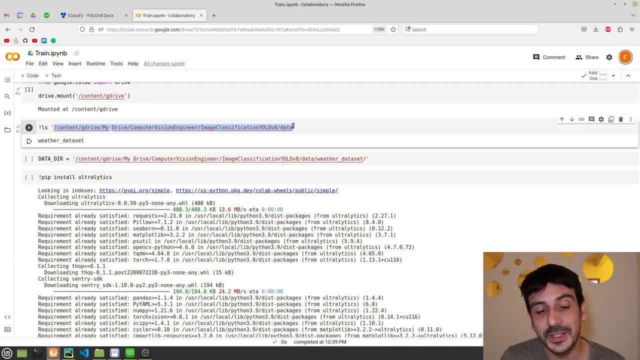 to the next step. this is very important because if you haven't set your data properly, if your data location is not set properly, then yellow v8 will not be able to train your model. this is very, very important. so in my case, this is exactly where the data- the weather data set- is located. right, 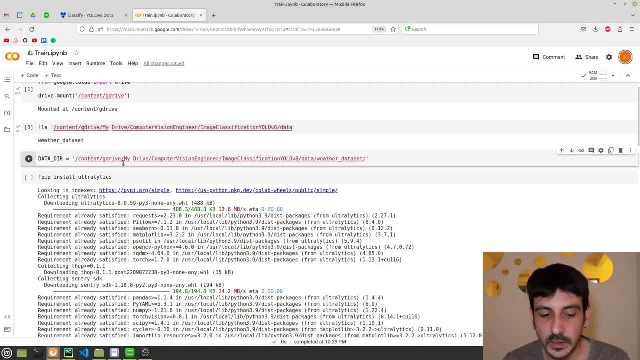 this is the path to the weather data set. so this is the the cell i am going to execute that. this is the value i'm going to save in this value in data directory. in that idea, now i'm going to continue. then we need to pip install ultralytics, which is 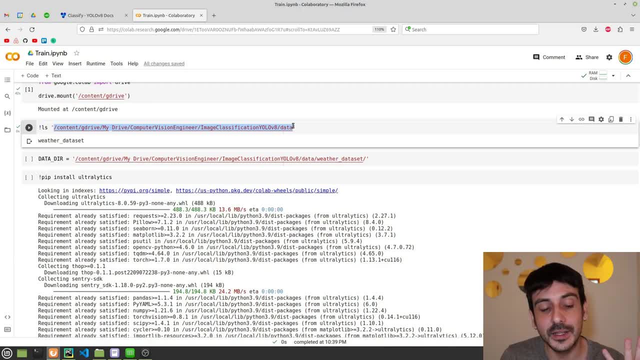 This is very important because if you haven't set your data properly, if your data location is not set properly, then YOLOV8 will not be able to train your model. This is very, very important. So in my case, this is exactly where the data- the weather data set- is located. right, 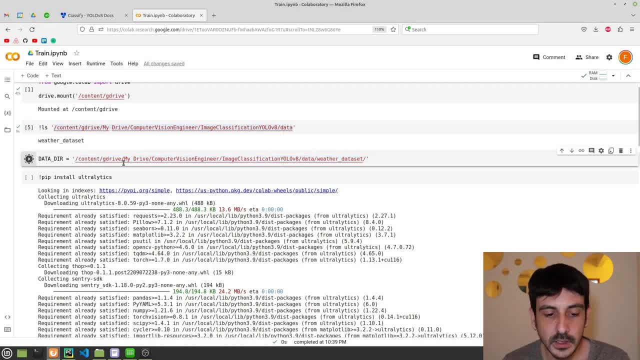 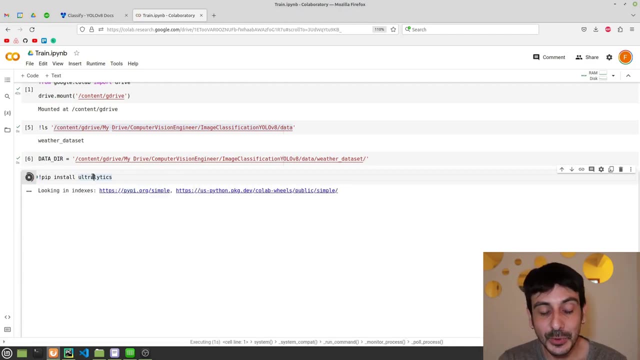 This is the path to the weather data set. So this is the cell I am going to execute that. this is the value I'm going to save in this value in data directory, in data dir. Now I'm going to continue. Then we need to pip install Ultralytics, which is the library we need in order to train this model, in order to use YOLOV8.. 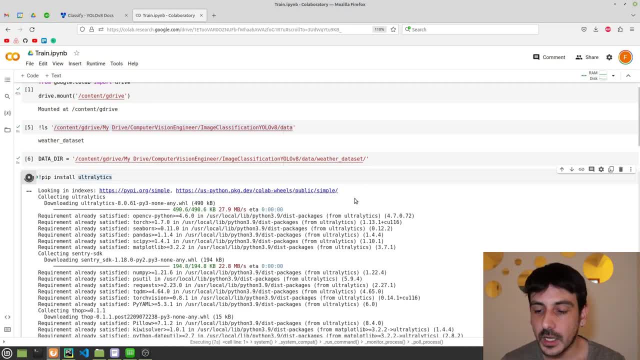 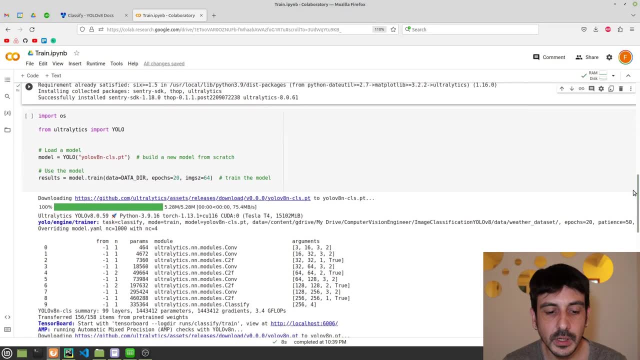 Now, the only thing you need to do is to execute this cell, and everything will run super smoothly. You can see that we have already completed this process. Now I'm going to continue, And the only thing we need to do now is to execute this cell. 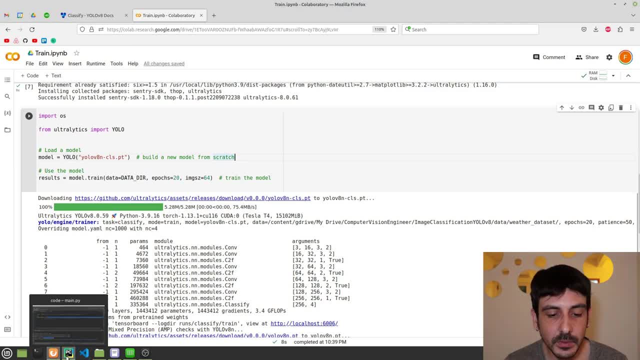 And you can see that the code we have in this cell is very, very similar to the code we have over here right. Basically, we are running Python script from a Google Colab. That's all we're doing. So you can see, we are importing OS and also we are importing the YOLO library. 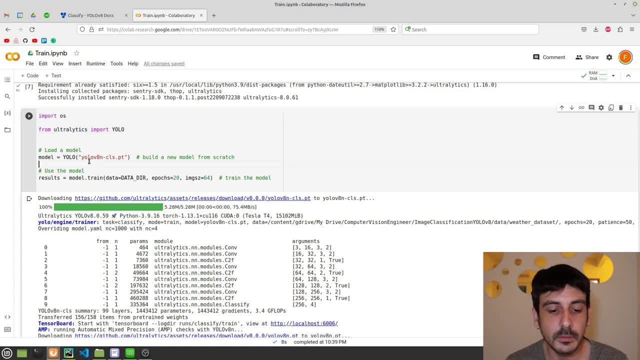 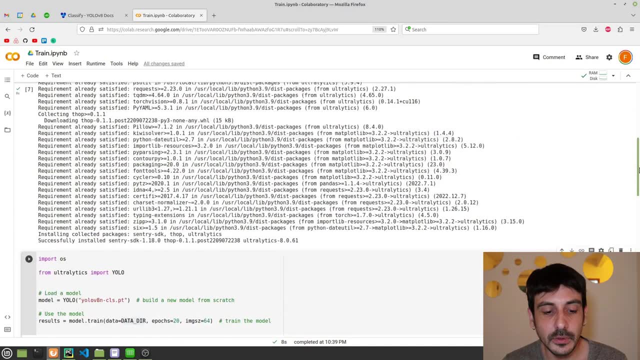 We are importing from Ultralytics, We are importing YOLO, And then we are doing exactly the same as we are doing before, And this is where we are using the data directory, the data dir variable we have defined over here. right, 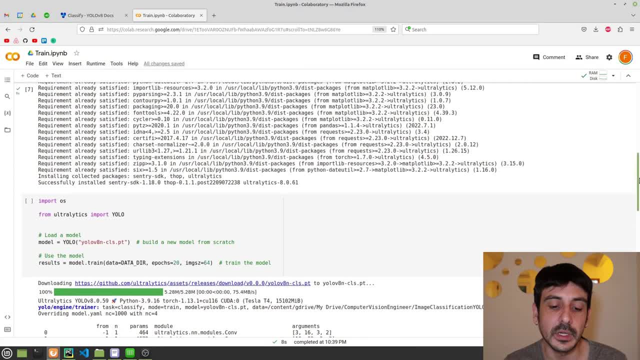 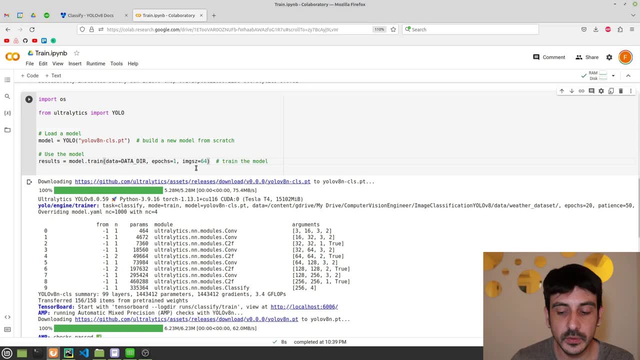 So this is why it's very, very important you set this variable properly. So the only thing I'm going to do, I'm going to do exactly the same as before. I'm just going to do this training for only one epoch. So we make sure everything's okay. 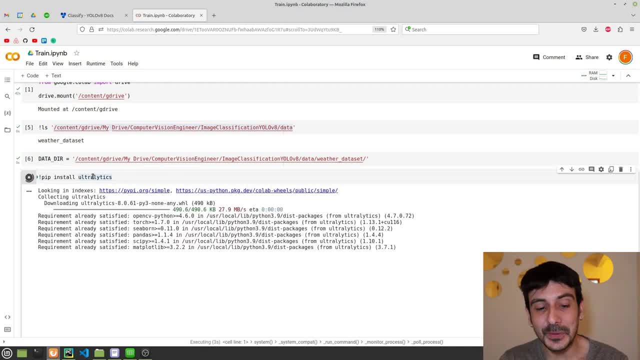 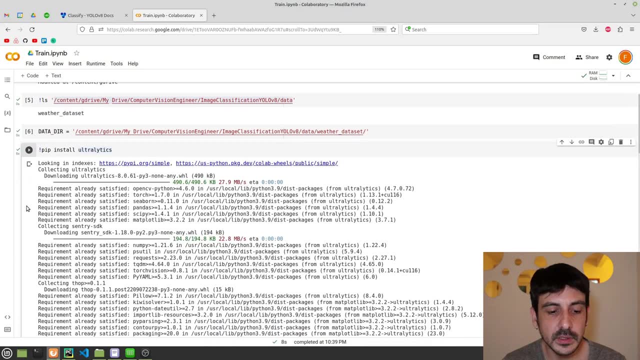 the library we need in order to train this model, in order to use yellow v8. now, the only thing you need to do is to execute this cell and everything will run super smoothly. you can see that we have already completed this process. now i'm going to continue, and the only thing we need to do now 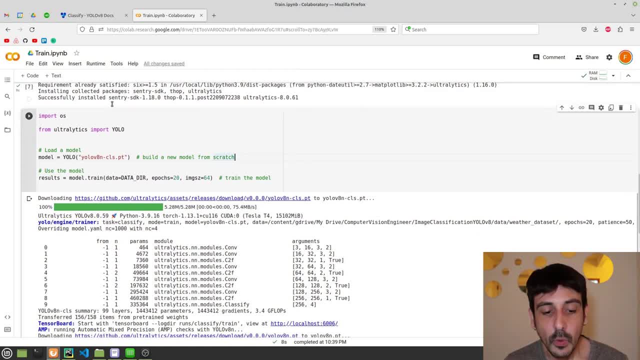 is to execute this cell, and you can see that the code we have in this cell is very, very similar to the code we have over here. right? basically, we are running a python script from a google collab. that's all we're doing. so you can see, we are importing os and also we are importing the yolo library. we are importing from. 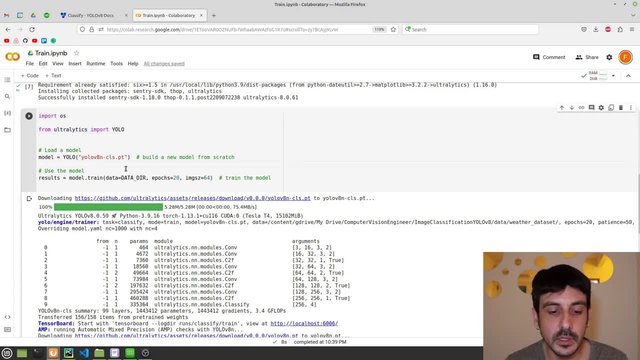 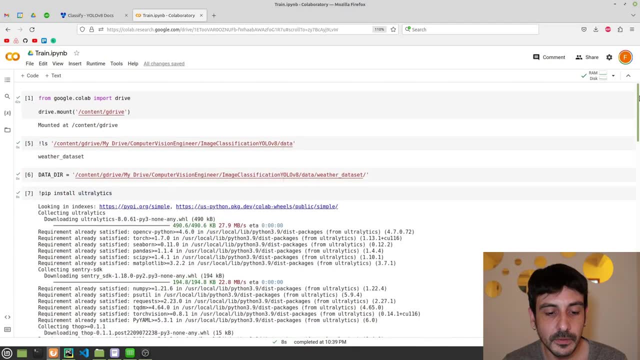 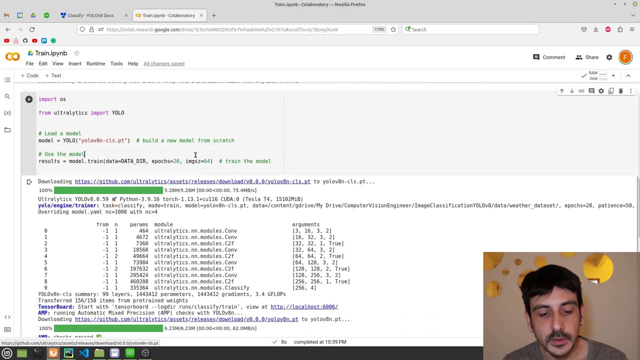 ultra league. we are importing yolo, and then we are doing exactly the same as we are doing before, and this is where we are using the data directory, the data dear variable we have defined over here. right, so this: this is why it's very, very important you set this variable properly. so the only thing i'm 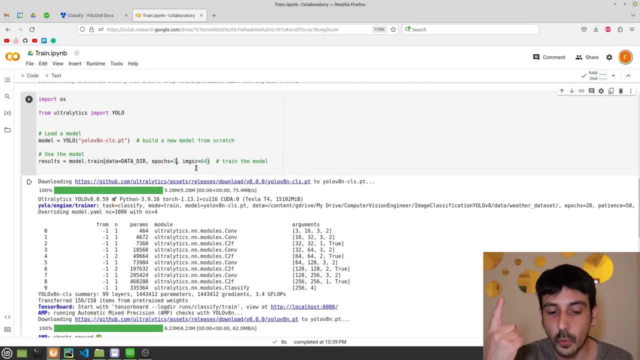 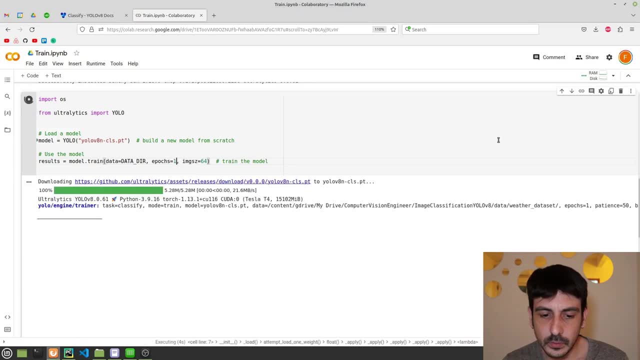 going to do? i'm going to do exactly the same as before. i'm just going to do this training for only one epoch, so we make sure everything's okay. i'm going to press enter- and that should be it- in order to do all this training. the first time you execute this training, it may take a little longer. 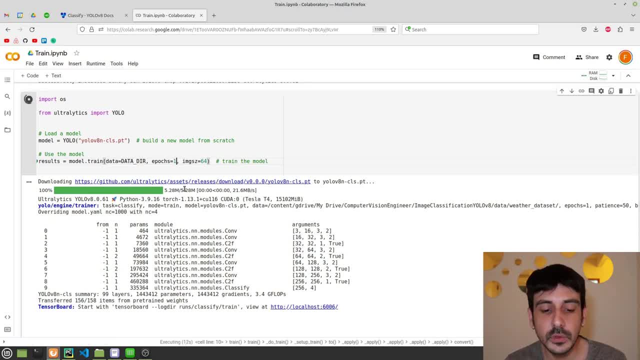 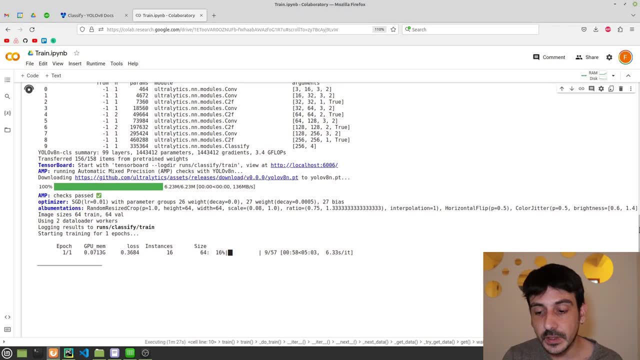 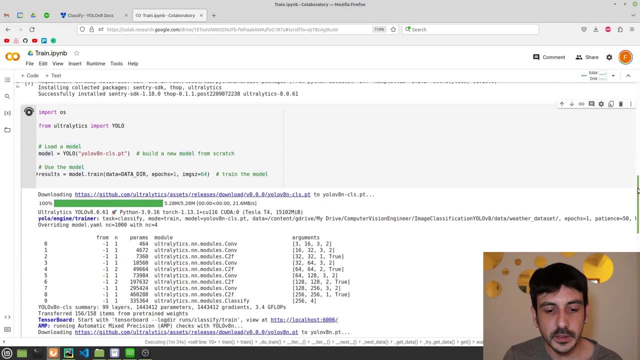 because you are downloading all the weights and you are downloading the modules and everything, but after that, everything should be much, much quicker. okay, so you can see that now the training process is on, it's in progress, everything is going super, super well and from now on, the only thing we need to do is to edit the number of epochs. 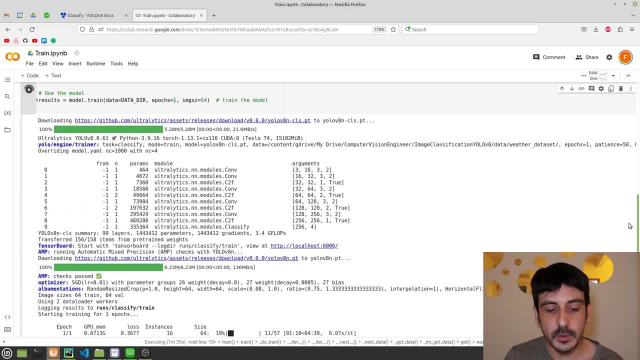 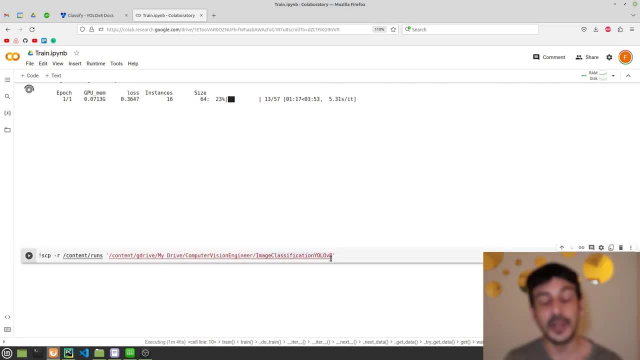 so we do like a more deeper training, but i would say everything is working super, super, super properly. so now let's move to the other cell. so i show you what exactly you need to do once everything is completed. once everything is completed, the only thing you need to do is to run. 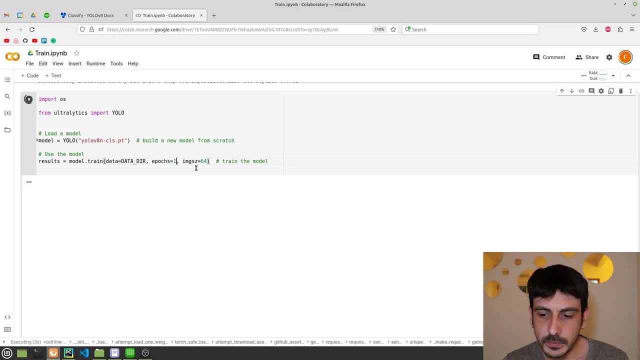 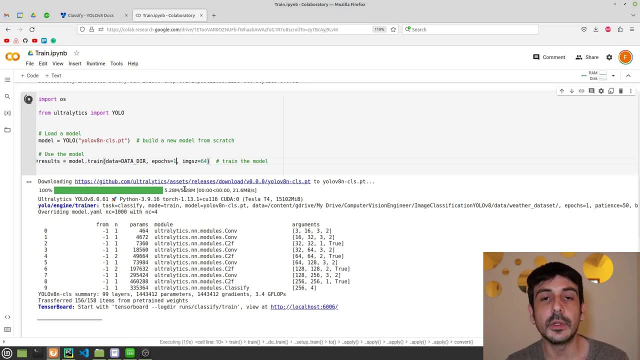 I'm going to press enter- And that should be it- in order to do all this training. The first time you execute this training, it may take a little longer, because you are downloading all the weights and you are downloading the modules and everything, But after that, everything should be much, much quicker. 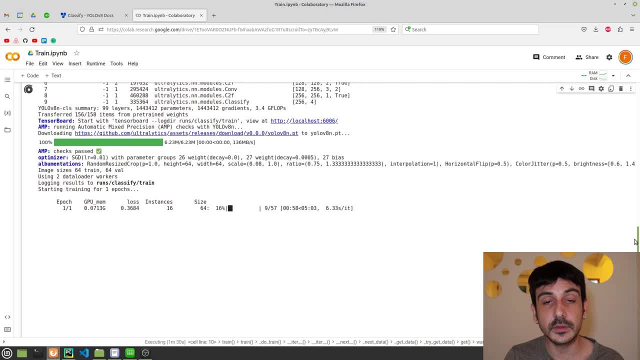 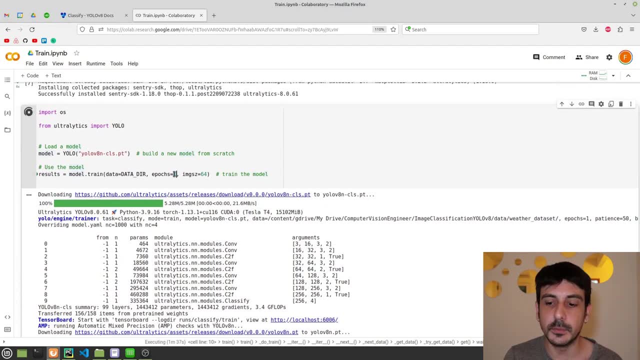 Okay, so you can see that now the training process is in progress. Everything is going super, super well, And from now on, the only thing we need to do is To edit the number of epochs, So we do like a more deeper training. 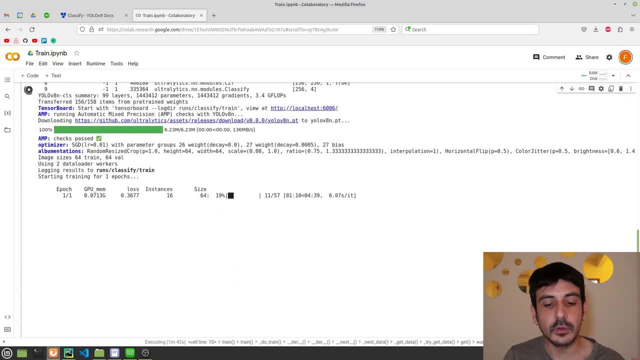 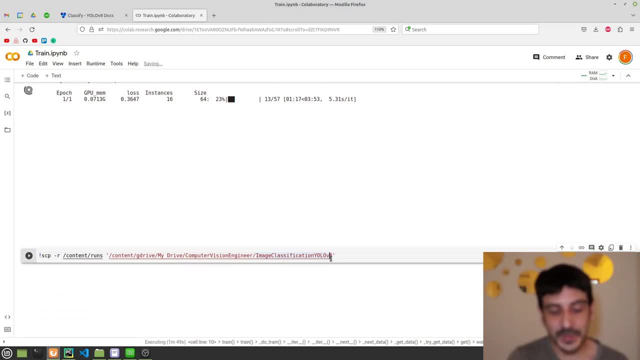 But I will say: everything is working super, super, super properly. So now let's move to the other cell. So I show you what exactly you need to do once everything is completed. Once everything is completed, the only thing you need to do is to run this cell. 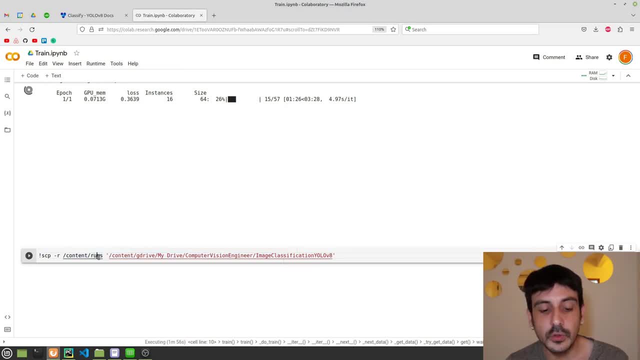 So you are copying. You are going to copy all your results which were saved on this directory. You are going to copy everything on your Google Drive, right? Because, remember, you are working on a Google Collab, you're working on an environment which is your Google Collab environment. 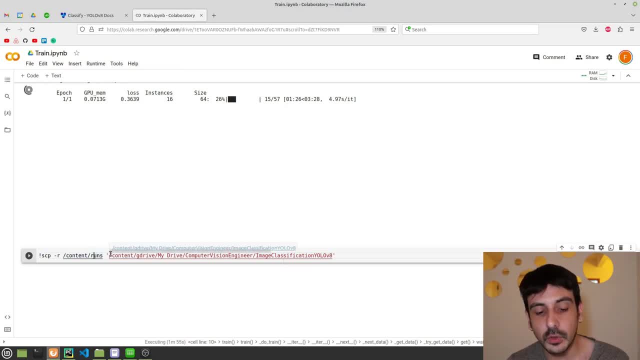 this cell, so you are copying. you are going to run this cell, so you are copying. you are going to copy all your results which were saved on this directory. you're going to copy everything on your google drive, right? because, remember, you are working on a google call up, you're working on an. 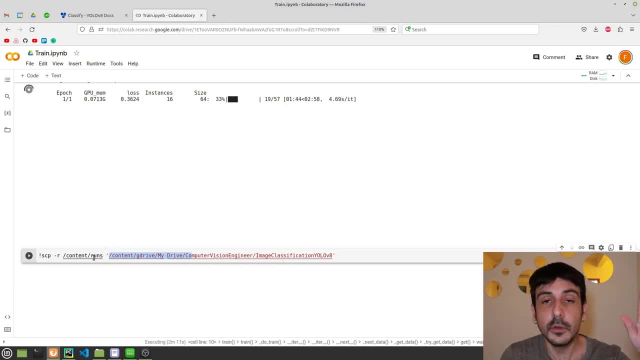 environment, which is your google collab environment. if you don't do something like this, it's going to be super, super hard for you to get the data you have just trained right, to get your results, to get your mode, your weights. it's going to be super, super hard because everything is located in your 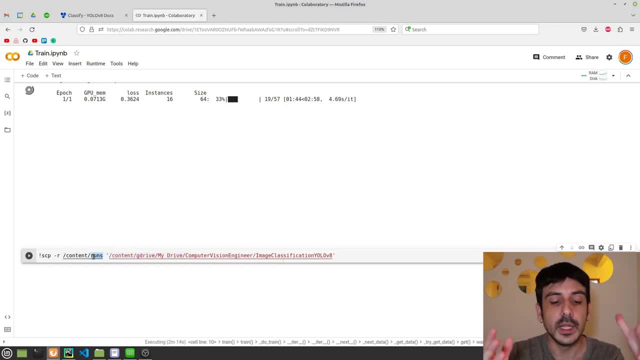 If you don't do something like this, it's going to be super, super hard for you to get the data you have just trained right, To get your results, to get your model, your weights is going to be super, super hard because everything is located in your Google Collab environment. 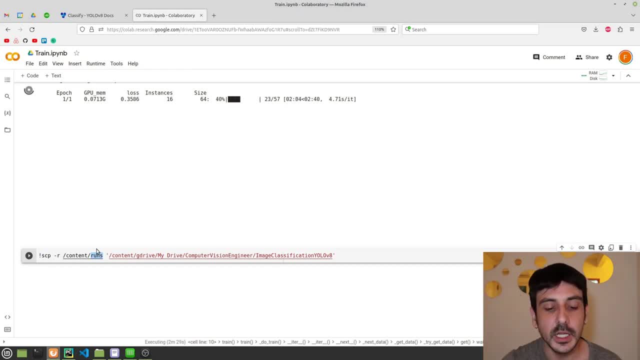 And long story short, it's going to be much, much simpler and much, much better if you just do something like this And you just copy Everything- all the results which were saved in this directory into your Google Drive- is going to be much, much better, because it's going to be much easier to download the weights, to download the results and so on. 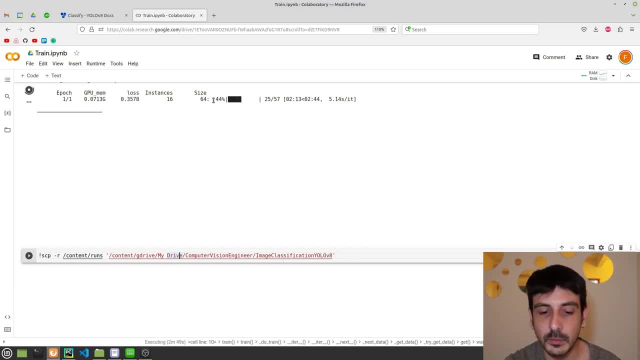 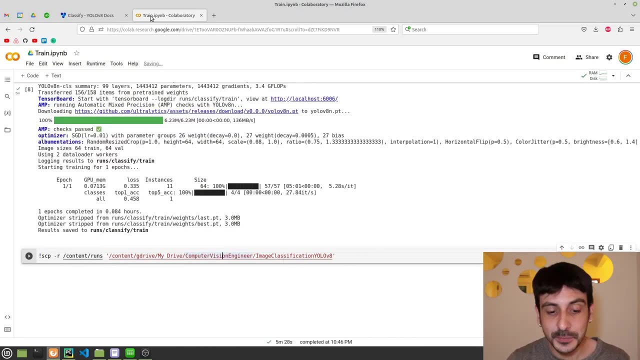 So now I'm just going to wait a couple of minutes so everything is completed over here, and then I can show you how to copy the results into your Google Drive. OK, now the training process has been completed and you can see that the results have been saved into runs. classified train. 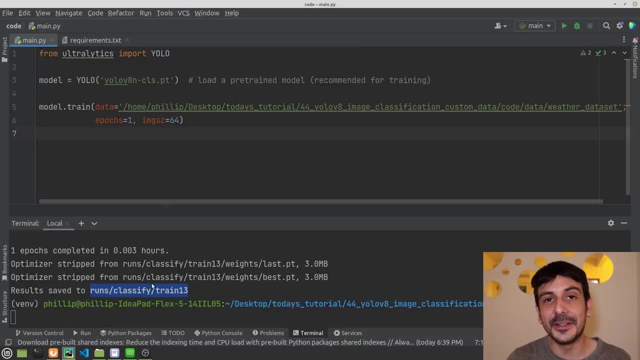 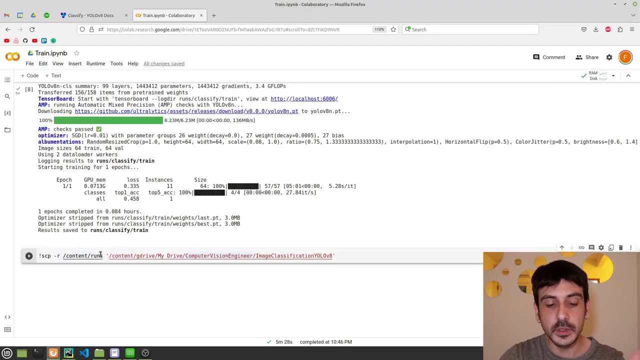 So these have very similar output To the one we just noticed when we were training on our local environment. Now, the only thing we need to do is to copy everything into our Google Drive, So everything is much, much simpler if we want to download these results or to do whatever we want. 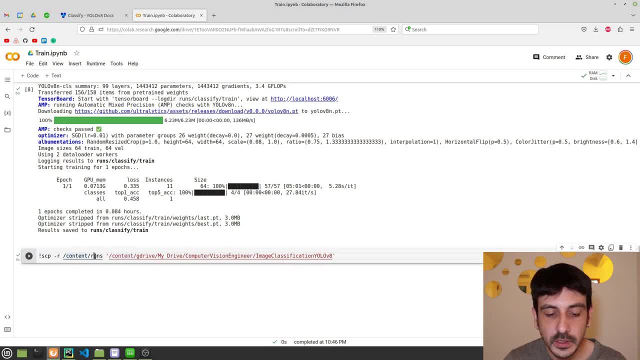 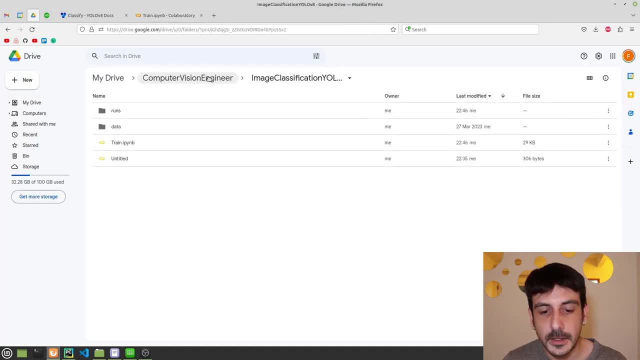 So the only thing I'm going to do is to run this cell and everything will be copied into this directory, which is the same directory where I have my data and where I have my my Google Collab. Right now, you can see that everything has been copied already. 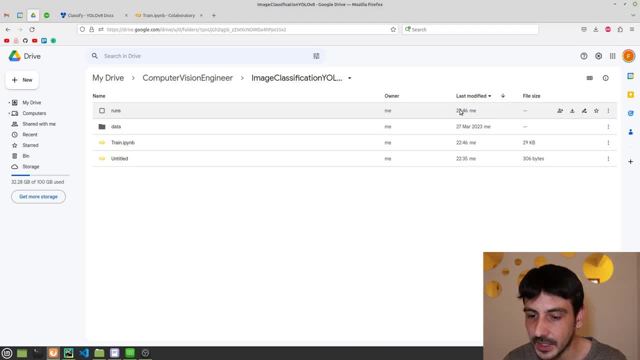 This is direct. I have just copied. This is the time is the current time, So this is the result of the cell I have just executed And if I go to runs- classified train, you can see that these are all the results we have generated. 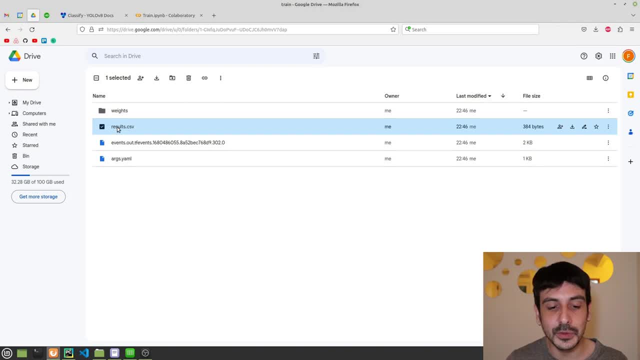 This is the CSV file containing many different results which I'm going to show you in a few minutes, And these are the weights and so on. So, from now on, if we want to get this data, or if we want to analyze this data, the only thing we need to do is to select runs. 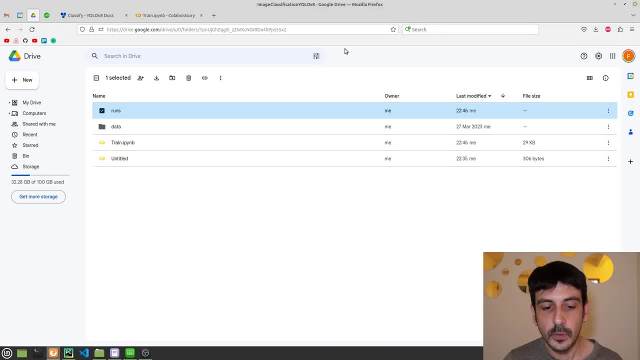 And then we just need to click download and this is going to download all these directory into your local drive. Right, You can see everything is being shipping and once everything is shipped, the directory will be downloaded into my local computer And you can see that this directory has just been downloaded. 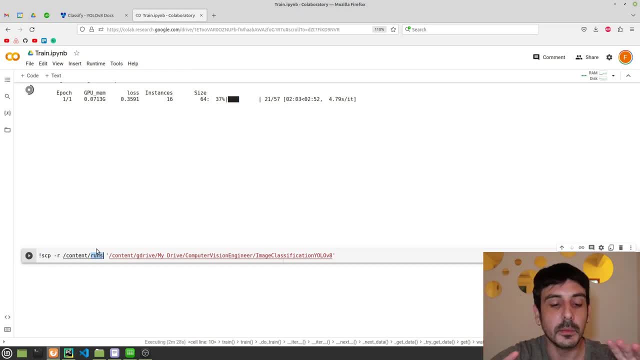 love, environment and long story short is going to be much, much simpler and much, much better if you just do something like this and you just copy everything, all the results which were saved in this directory- into your google drive. it's going to be much, much better because it's going. 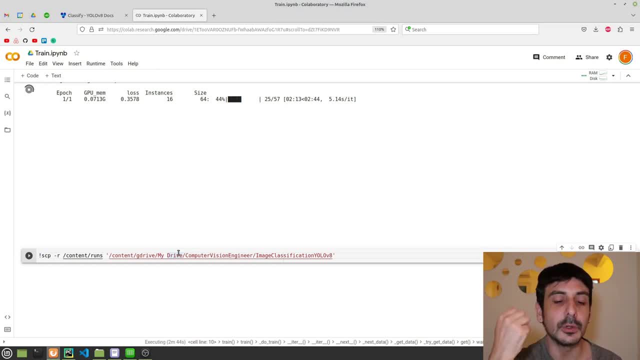 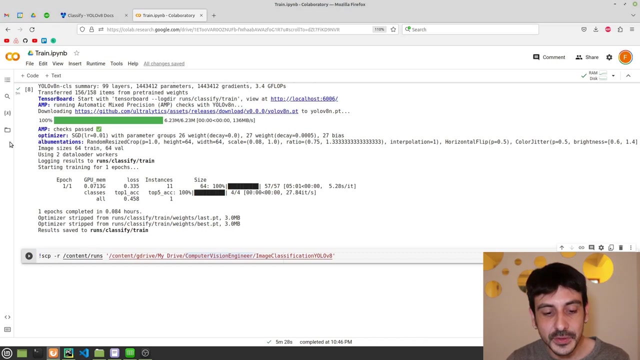 to be much easier to download the weights, to download the results and so on. so now i'm just going to wait a couple of minutes so everything is completed over here, and then i can show you how to copy the results into your google drive. okay, now the training process has been completed and you can see that the results have been saved. 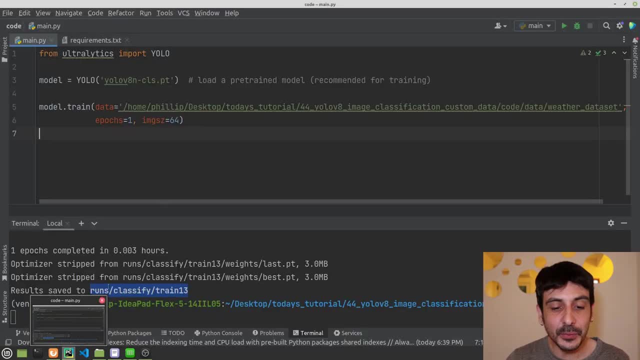 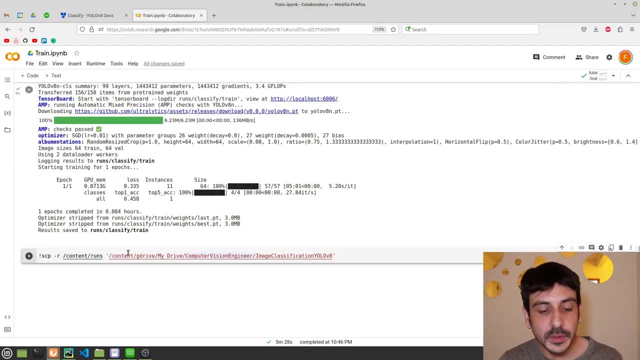 into runs, classify train. so this is a very similar output to the one we just noticed when we were training on our local environment. now, the only thing we need to do is to copy everything into our google drive. so everything is much, much simpler if we want to. 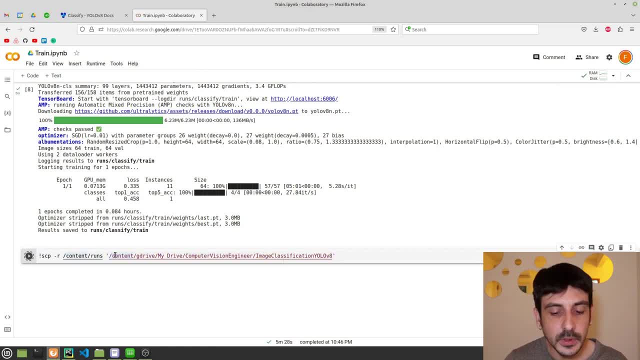 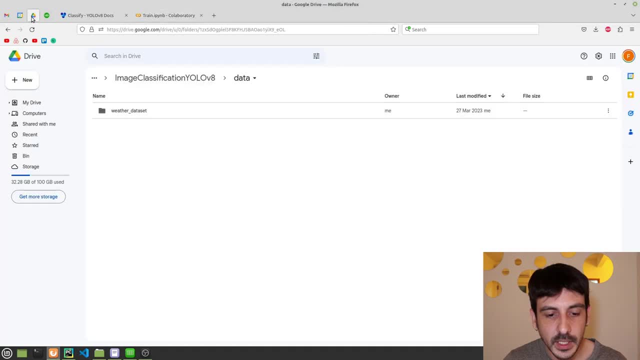 download these results or to do whatever we want. so the only thing i'm going to do is to run this cell and everything will be copied into this directory, which is the same directory where i have my data and where i have my- uh, my- google collab. right now, you can see that everything. 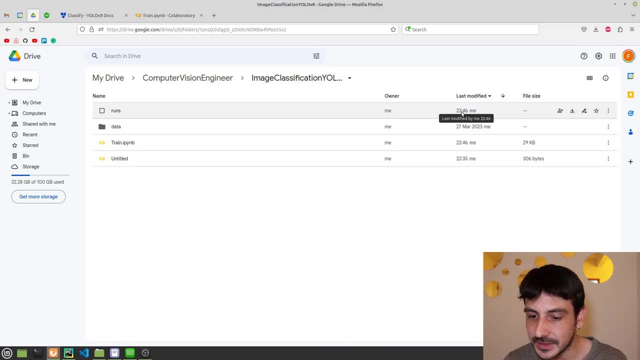 has been copied already. this is the directory i have just copied. this is the time. this is the current time. so this is the result of the cell i have just executed and if i go to runs, classify train, you can see that these are all the results we have generated. this is the csv file containing 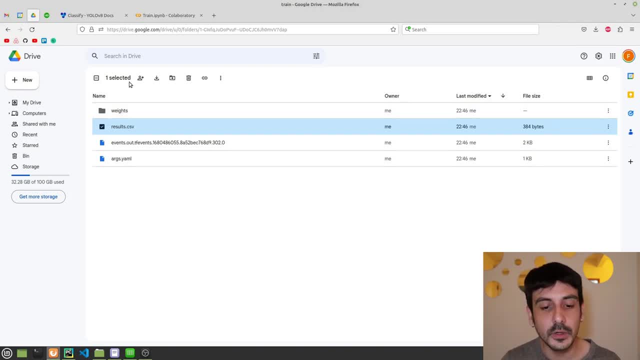 many different results, which i'm going to show you in a few minutes, and these are the weights and so on. so, from now on, if we want to get this data, or if we want to analyze this data, the only thing we need to do is to select runs, and then we just need to click download and this is going to download. 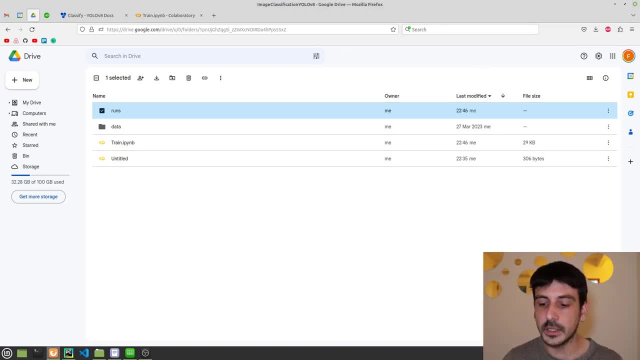 all this directory into your local drive. right, you can see everything is being shipping and once everything is shipped, the uh, this directory will be downloaded into my local computer and you can see that this directory has just been downloaded. so everything is everything is being shipped. working shows: fine. now, this is pretty much all in order to show you three different ways in which. 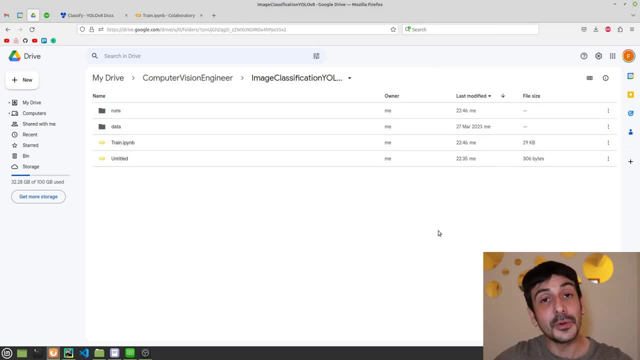 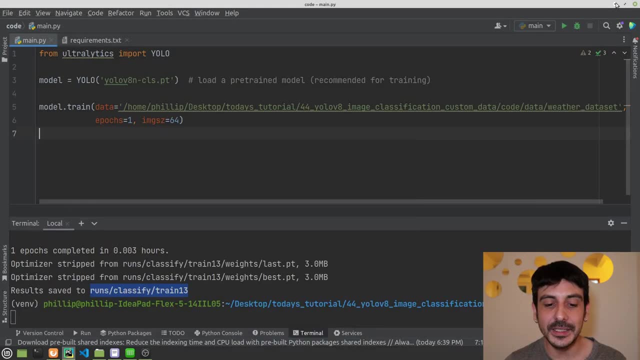 So everything is working just fine. Now, this is pretty much all in order to show you three different ways in which you can train an image classifier using YOLO V8.. And now let's do the The deeper training. right, I'm just going to take this script and I'm going to edit the number of epochs. 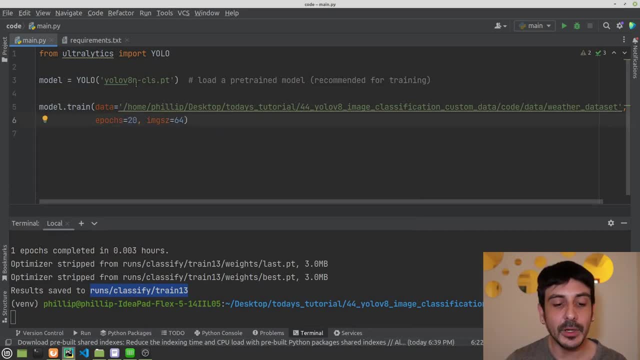 So we do this training for something like 20 epochs. I have already been doing some tests and 20 epochs is just enough for this data set, for the data set I am using in this tutorial, So 20 will be just fine. Now the only thing we need to do is to click on run. 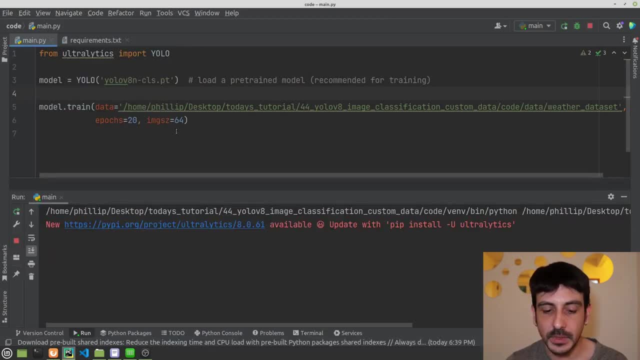 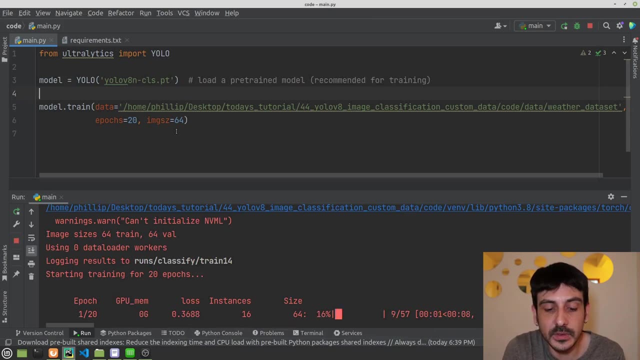 I'm just going to run this script as it is, and everything will be exactly the same as before. Everything will be Exactly the same, right We are. just we just need to wait until this process is completed. We don't need to do anything from now on, but this process will be executed for 20 epochs. 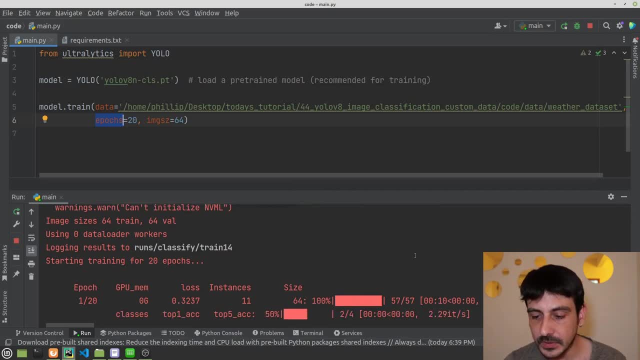 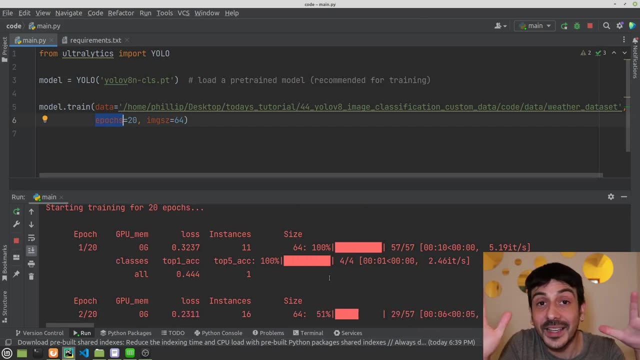 So the only thing I'm going to do is to wait until this process is completed, And once everything is completed, we are going to validate this training process. I'm going to show you how to analyze if all this process was done successfully or not, if you have successfully trained a good image classifier or not. 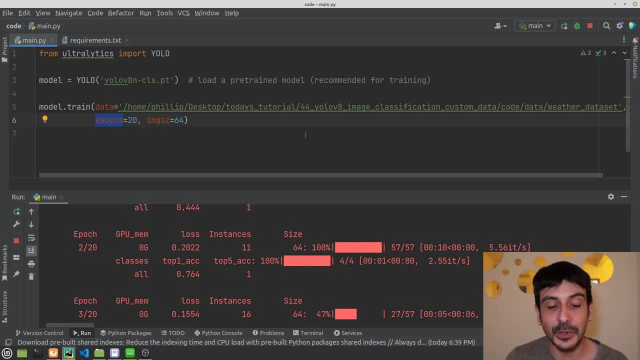 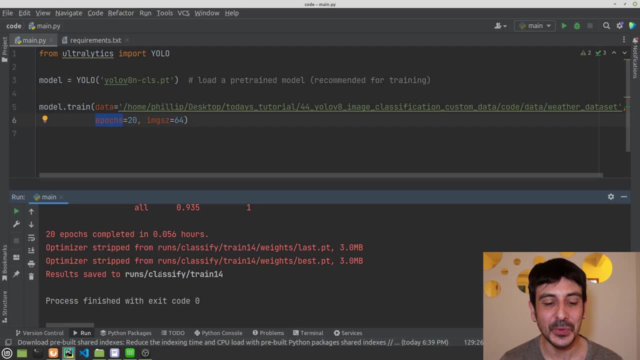 So I'm just going to pause the recording here and I'm going to fast forward until this is completed. OK, so the training process has been completed and now let me show you all the results which were saved here into runs, classify and train 14.. 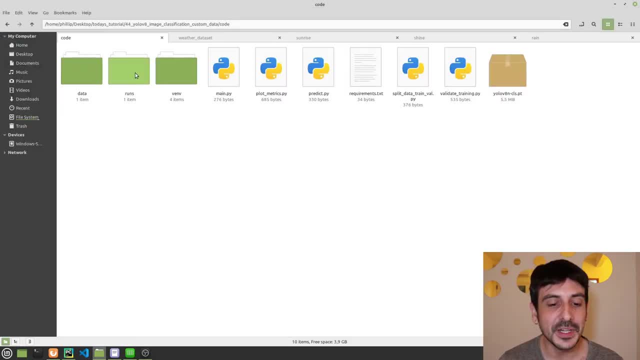 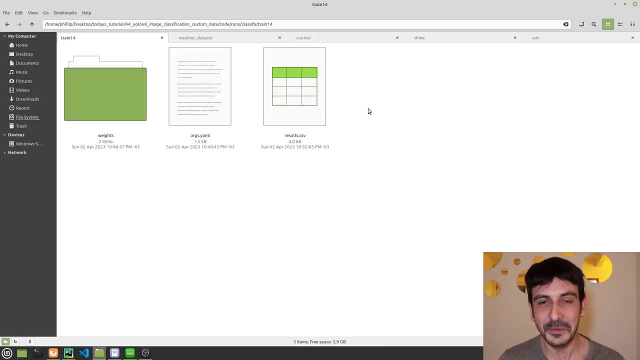 Now let me show you this directory, this folder, in my local computer. If I go to runs, classify and then train 14, this is where all the results have been saved. And this is everything we are going to analyze now. Now we're going to decide. 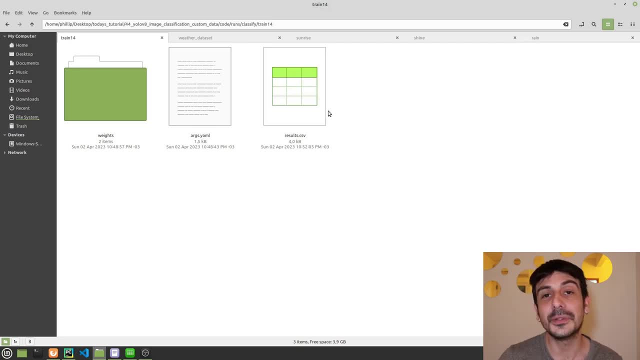 If the model We have trained is a good model or not. we are going to decide if this is a model we can use or not. So you can see that there are two files. are that YAML results, that CSV and another directory called weights? 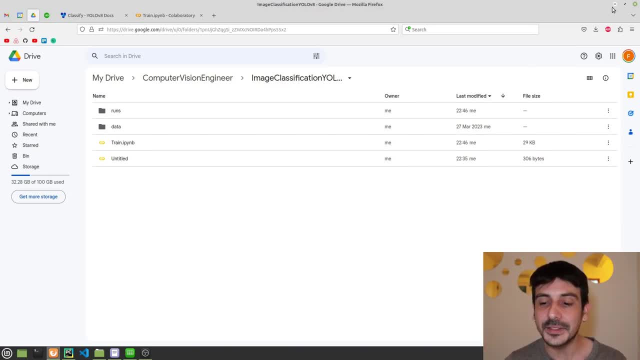 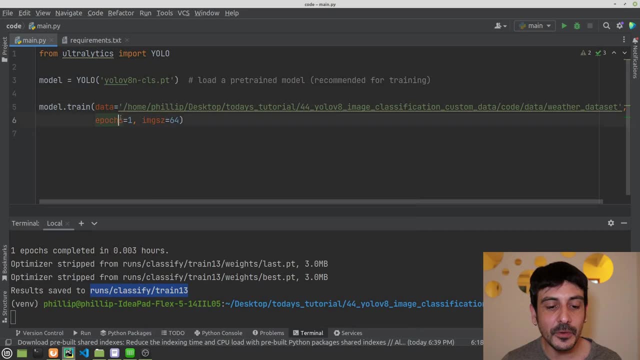 you can train an image classifier using yolo v8. and now let's do the the deeper training, right? i'm just going to take this script and i'm going to edit the number of epochs so we do this training for something like 20 epochs. i have already been doing some tests and 20 epochs is just enough for. 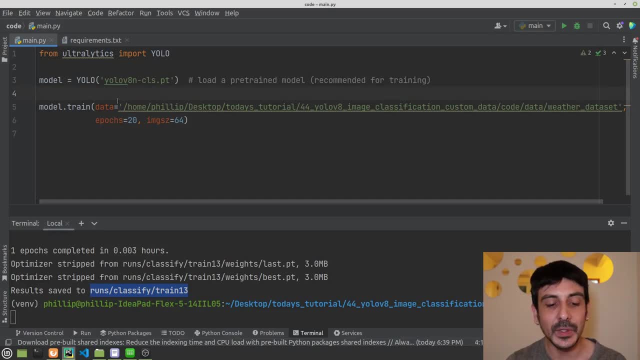 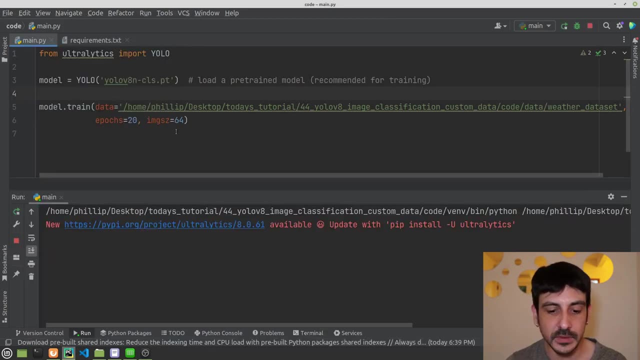 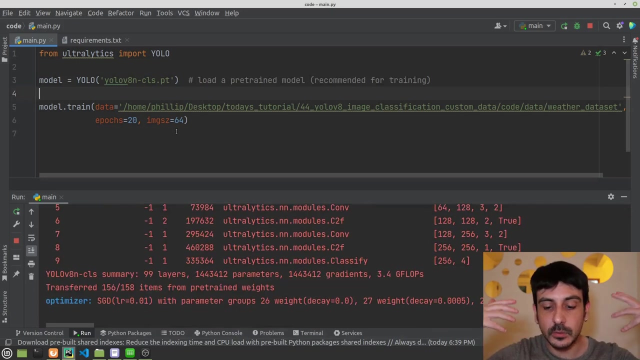 this data set for the data set i am using in this tutorial. so 20 will be just fine. now the only thing we need to do is to click on run. i'm just going to run this script as it is and everything will be exactly the same as before. everything will be exactly the same, right, we are just. we just need. 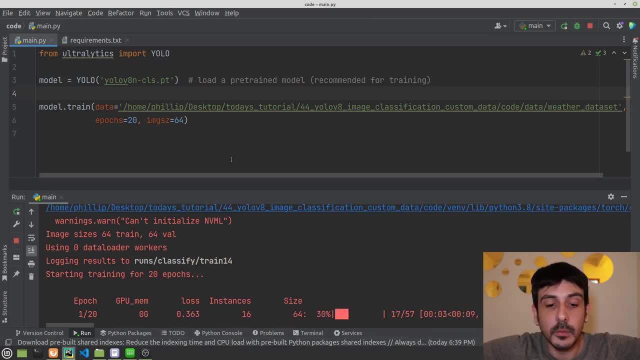 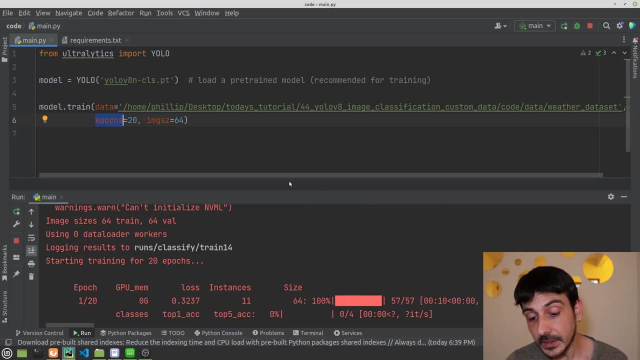 to wait until this process is completed. we don't need to do anything from now on, but this process will be executed for 20 epochs, so the only thing i'm going to do is to wait until this process is completed, and once everything is completed, we are going to validate this training process. i'm going 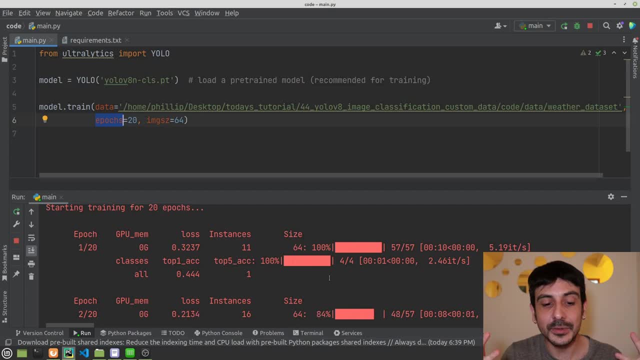 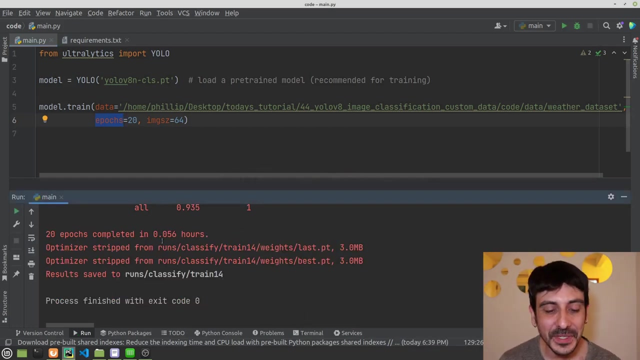 to analyze if all this process was done successfully or not, if you have successfully trained a good image classifier or not. so i'm just going to pause the recording here and i'm going to fast forward until this is completed. okay, so the training process has been completed and now let 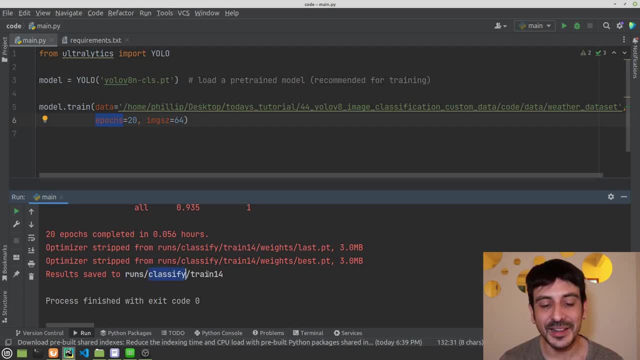 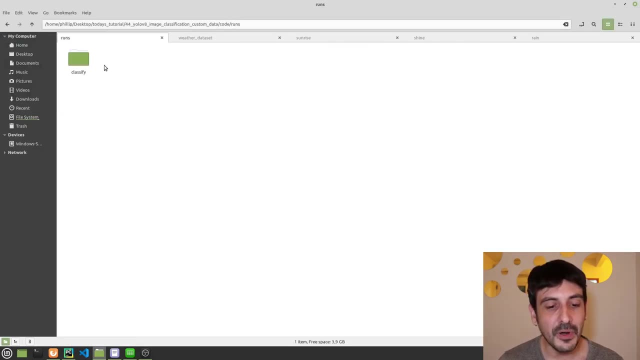 me show you all the results which were saved here into runs, classify and train 14.. now let me show you this directory, this folder in my local computer. if i go to runs, classify and then train 14, this is where all the results have been saved and this is everything we are. 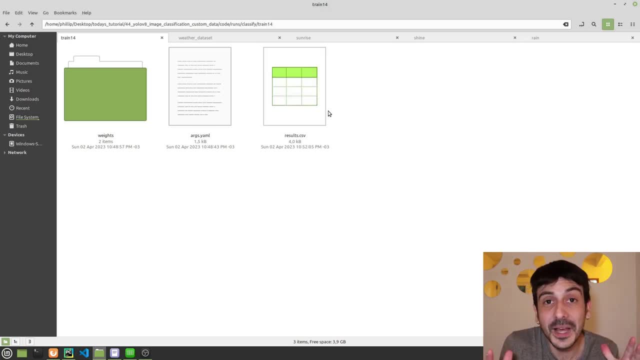 going to analyze now. now we are going to decide if the model we have trained is a good model or not. we are going to decide if this is a model we can use or not. so you can see that there are two files. are that yaml, resultscsv, and another another directory called weights. let's start by. 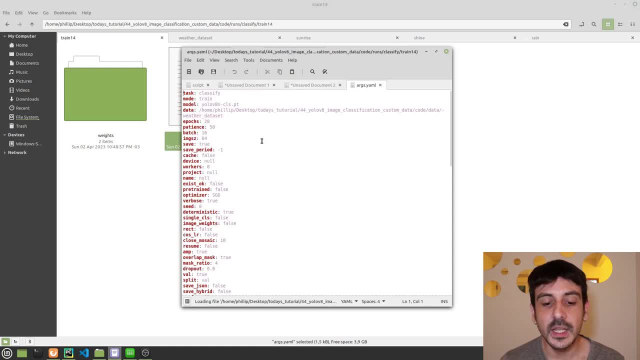 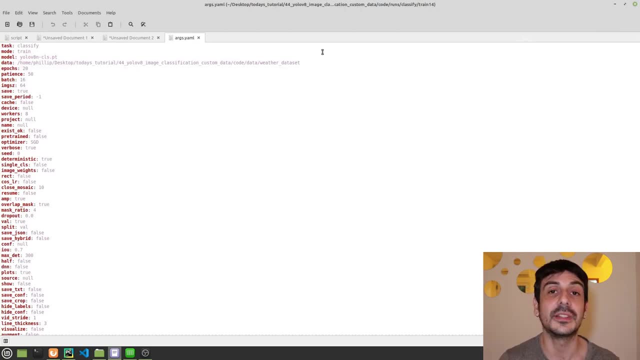 argsyaml. if i open this file, you can see that this is something like a config file, and this is exactly the entire configuration file which we have just used in order to train this model. this is very important because this is a super, super comprehensive list of all the hyper. 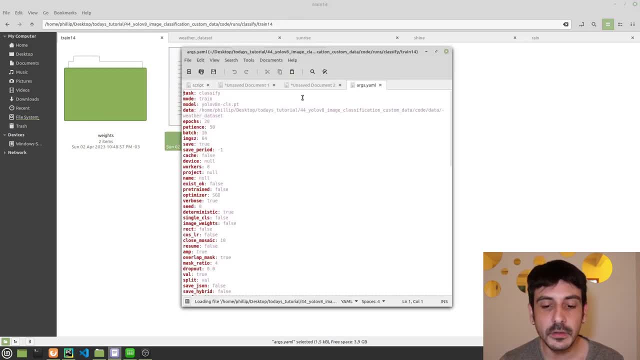 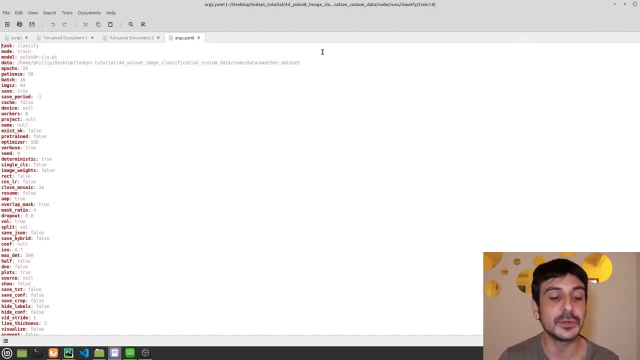 Let's start by arcsyaml. If I open this file, you can see that this is something like a config file, and this is exactly the entire configuration file which we have just used in order to train this model. This is very important because this is a super, super comprehensive. 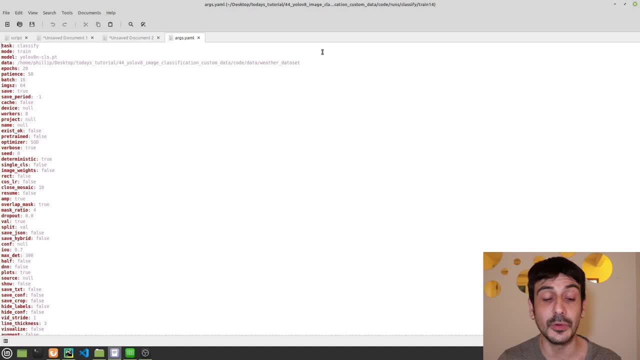 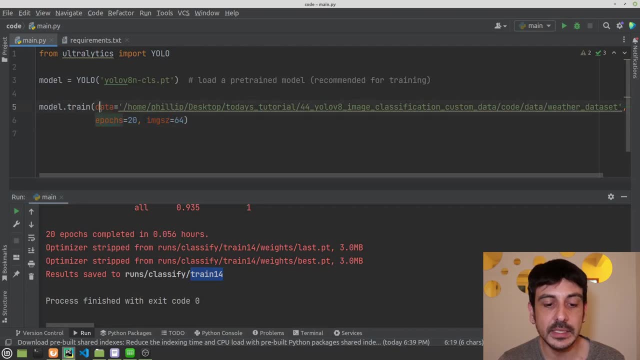 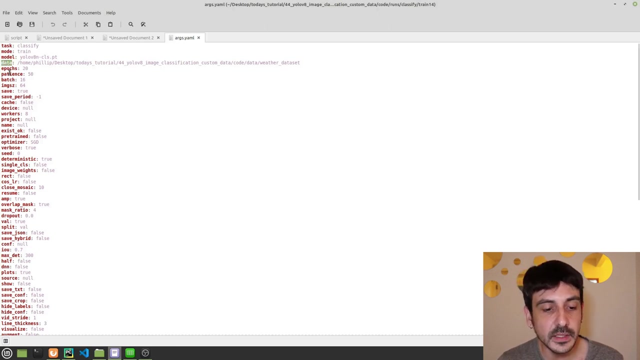 List of all the parameters we have used in order to train this model And, for example, the only parameters we have specified are image size, number of epochs, and then date and the location of the data. we have just used, And you can see that we have a keyword which is data, the epochs, then image size. 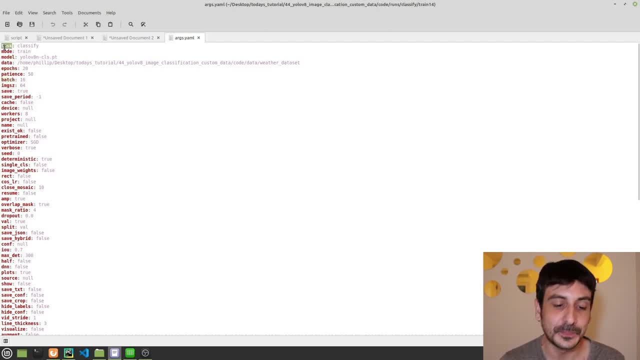 And then we have many, many, many other keywords as well. This is very important because these are absolutely all the keywords we have used. We have used all these default values And we have used all these default values, And we have used all these default values. 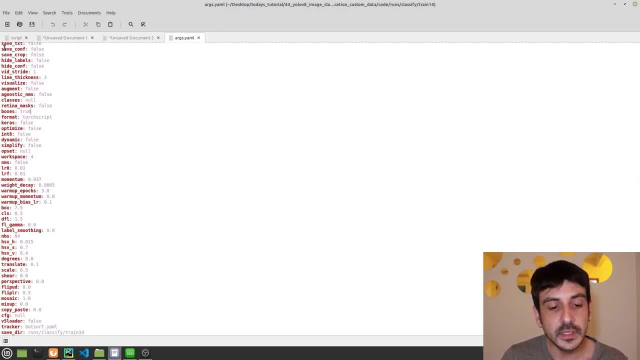 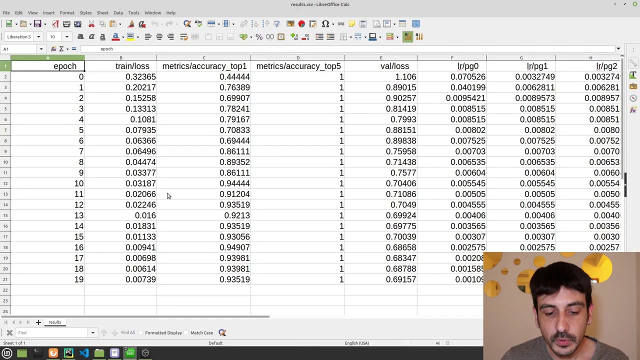 values which were set for all these different keywords, and this is important in case we want to train a new model and we want to make some changes into some of these hyper parameters. now let me show you the other file, which is the resultscsv file. that will say: this is much. 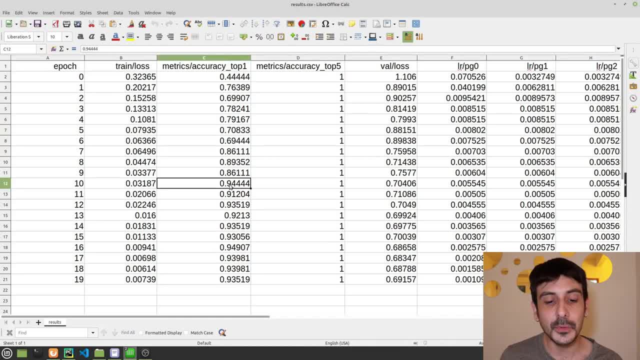 more important. this is like the, the file containing all the information we need in order to decide if this is a good model or not, and you can see that we have many different rows, each row for one of our training Epox. right, we have trained this model for 20 Epox and you can see that we have 20 rows. 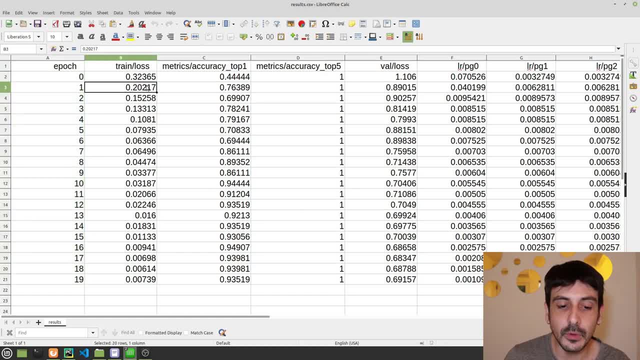 for each one of these Epochs and for each one of these rows, we have all this different information and we are going to focus on these three values: on the training laws, the accuracy, the- this is the accuracy of the validation set- and then also the validation laws- right. these are the three. 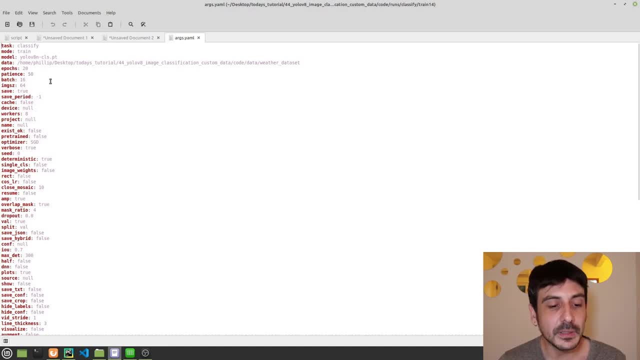 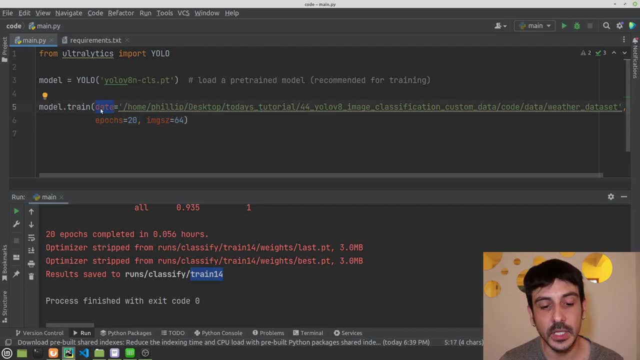 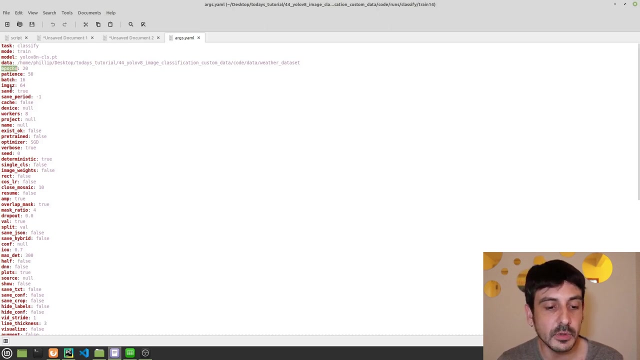 parameters we have used in order to train this model and, for example, the only parameters we have specified are image size, number of epochs and then data, the location of the data. we have just used, and you can see that we have a keyword which is data, then epochs, then image size, and then we have 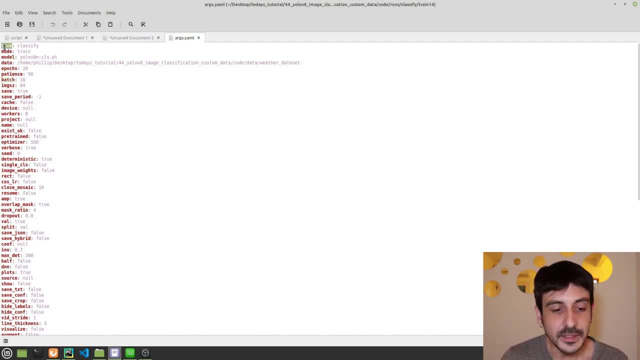 many, many, many other keywords as well. this is very important because these are absolutely all the keywords we have used. we have used all these default values which were set for all these different keywords, and this is important in case we want to train a new model and we want to make 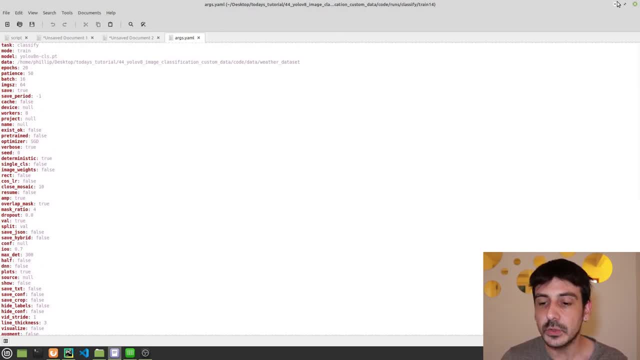 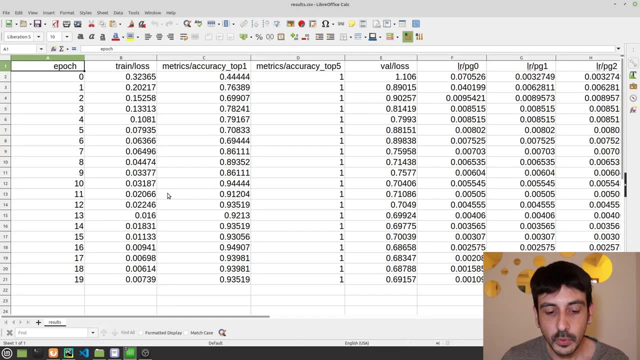 some changes into some of these hyper parameters. now let me show you the other file, which is the resultscsv file. that will say: this is much more important. this is like the, the file containing all the information we need in order to decide if this is a good model or not, and you can see that we 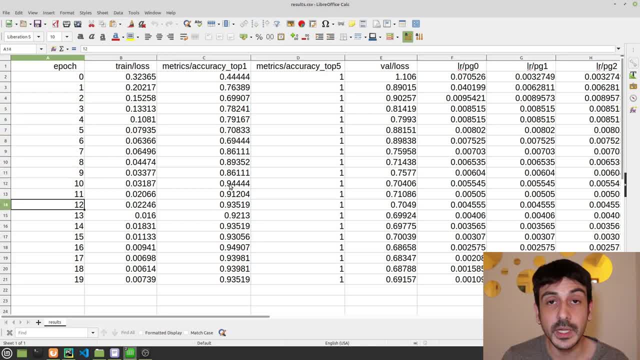 have many different rows, each row for one of four training epochs. right, we have trained this model for 20 epochs and you can see that we have 20 rows for each one of these epochs and for each one of these rows, we have all this different information and we are going to focus on these three values. 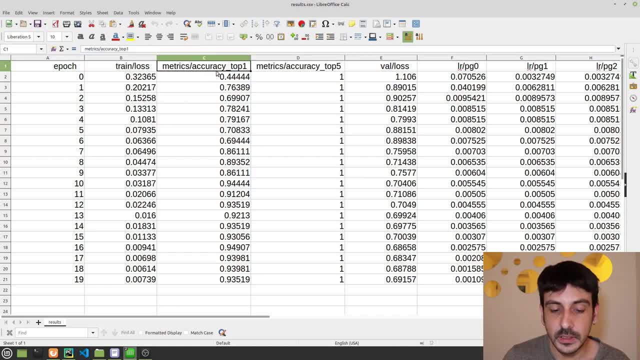 on the training laws, the accuracy, the- this is the accuracy of the validation set- and then the validation loss right. these are the three keywords in which we are going to focus on this tutorial in order to validate this model, and i'm going to give you, like a very, very quick tip, like 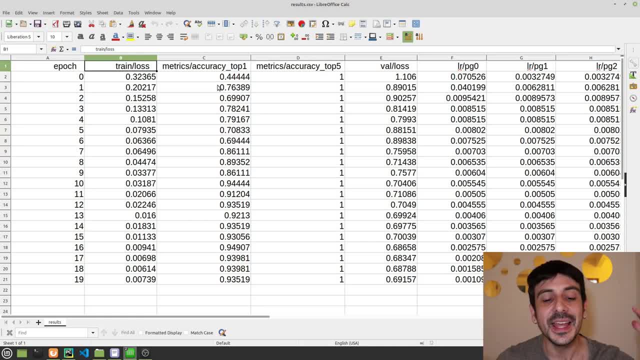 a very quick way in order to analyze this training process, which is make sure the training laws and the validation laws are going down through this training process and also make sure the accuracy goes up. and i know you're thinking: hey, this is a very simple way to analyze this process, oliver. 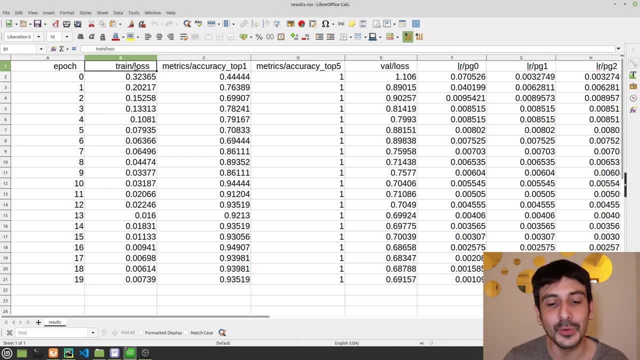 keywords in which we are going to focus on this tutorial in order to validate this model, and I'm going to give you like a very, very quick tip, like a very quick way in order to analyze this training process, which is make sure the training laws and the validation laws are going down through this training process and also 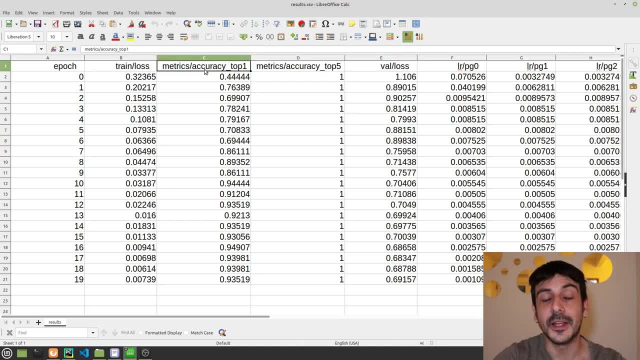 make sure the accuracy goes up, and i know you're thinking, hey, this is a very simple way to analyze this process. olipe, yeah, i agree with you. this is a very simple way, but at the same time, it's very robust. this is like a very simple but, at the same time, very powerful way to decide if you have a 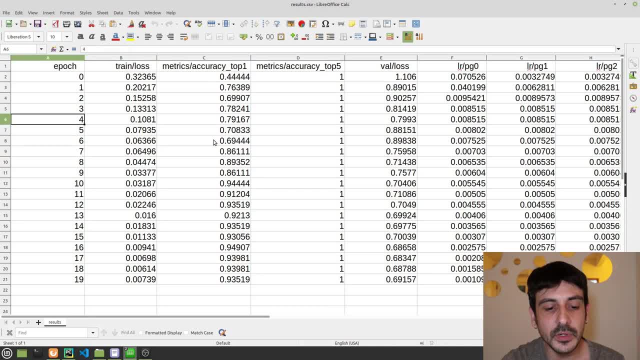 good model or not. now we can analyze all these numbers, but i think it's going to be much, much better and it's going to be much, much prettier if we make a plot with all these numbers. right, because we have epochs in this, in this column, in this coordinate, and we also have all these. 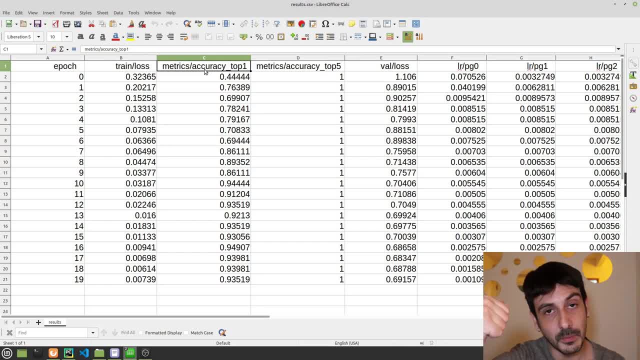 yeah, i agree with you. this is a very simple way, but at the same time, it's very robust. this is like a very simple but, at the same time, very powerful way to decide if you have a good model or not. now we can analyze all these numbers, but i think it's going to be much, much better and it's going 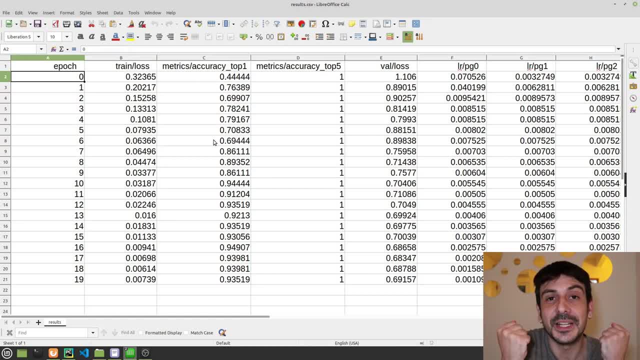 to be much, much prettier if we make a plot with all these numbers. right, because we have epochs in this um, in this column, in this coordinate, and we also have all these different values and we can definitely plot these values across all these different epochs. so let me show you a python file i have created and this is: 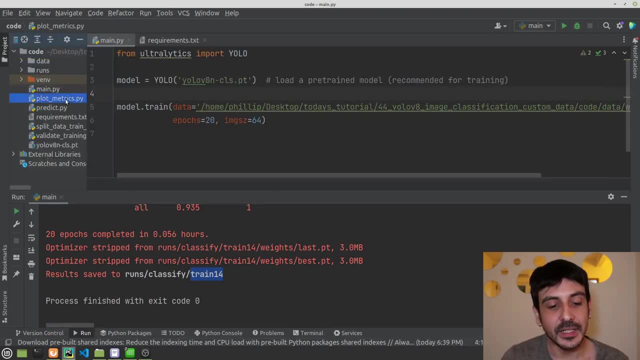 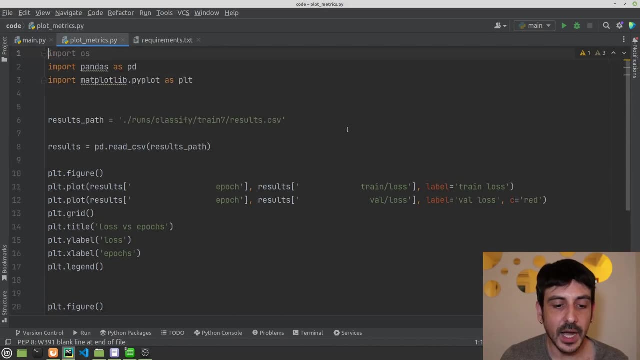 exactly what this python file does. this file is called plot metrics and if i open this file, you can see that it basically we need to set a patch to a resultscsv file. in our case, i'm going to set it to train 14 and you can see that this is wrong. classified train 14 and then resultscsv. 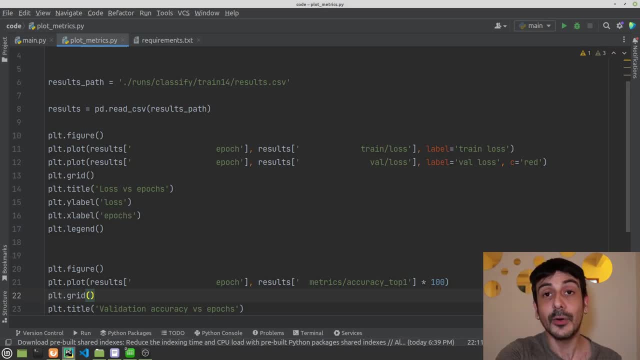 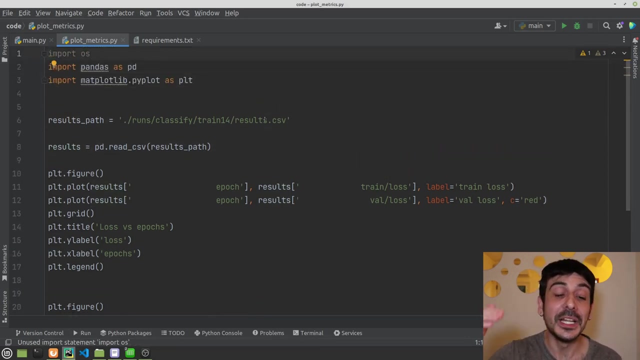 and then this is only like some logic, some very simple logic: to take all the data from this resultscsv file and to do some plots with it. right, that's all we're doing. we're just taking the data and doing some plots, and this file will be available in the github repository of this project, of this tutorial. 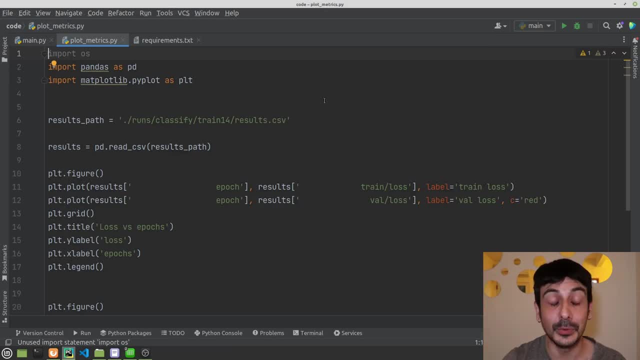 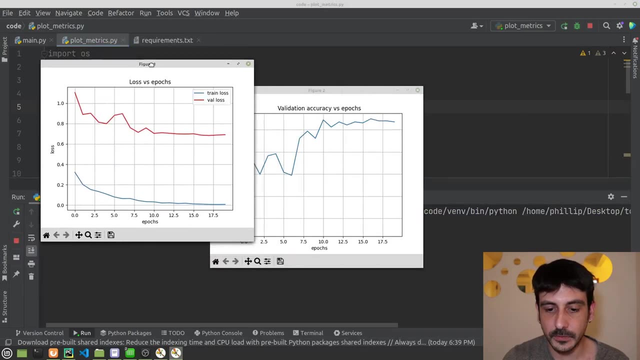 so you can definitely take this file and you can just use it to plot your functions as well. all i'm going to do now is just press play and you can see that if we wait only a few seconds, we get all these two plots right. this is all the information in our csv file, right? 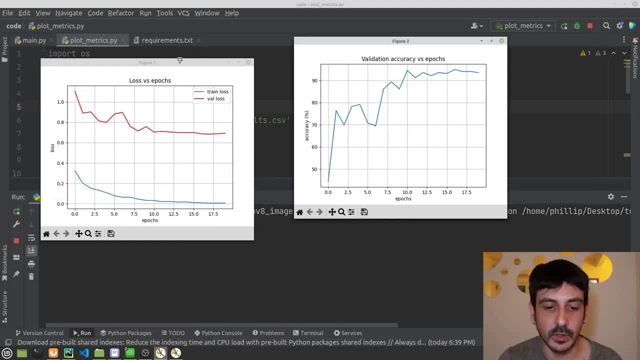 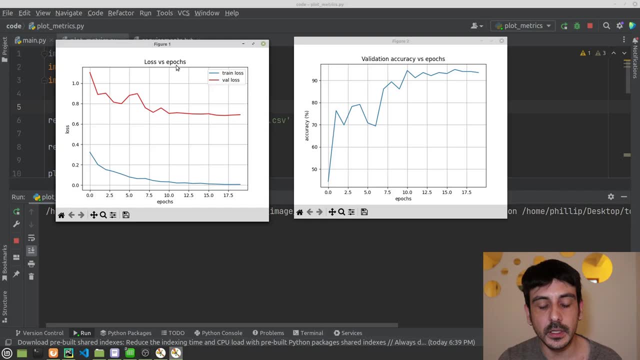 everything i show you over here it's summarized on these two plots. so this is exactly what i mean with make sure your loss is going down. this is your, this is our loss in the training set and in the validation set. in the training set we are plotting the loss in blue and in the validation set is red and you can see that. 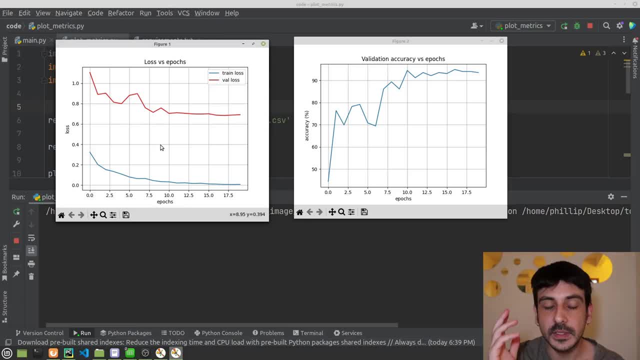 in both cases, the loss is going down right. we. we is exactly what we expect. it's exactly what we want now. this is a very, very simple way to analyze this process, but, trust me, this is also a very powerful way. right, this is something that's very 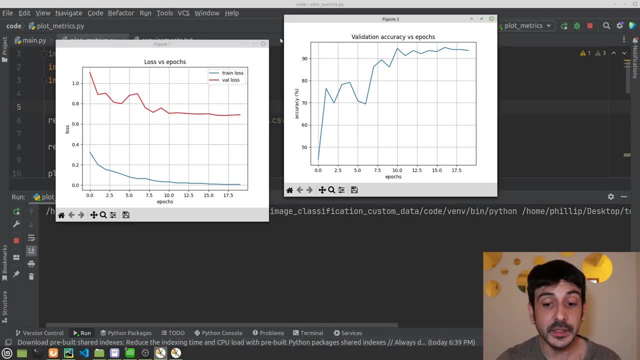 very healthy. something that looks like this is very healthy. and then for this other plot, which is how the validation accuracy evolves through this training process, you can see that the validation accuracy goes up when we increase the number of epochs. right, you can see that, starting from the 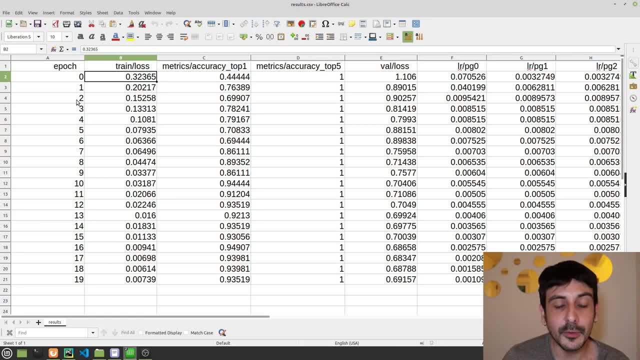 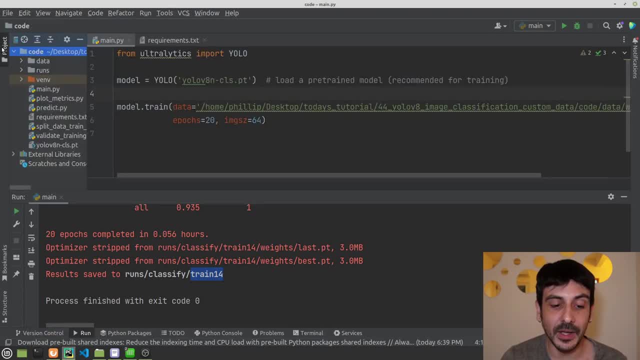 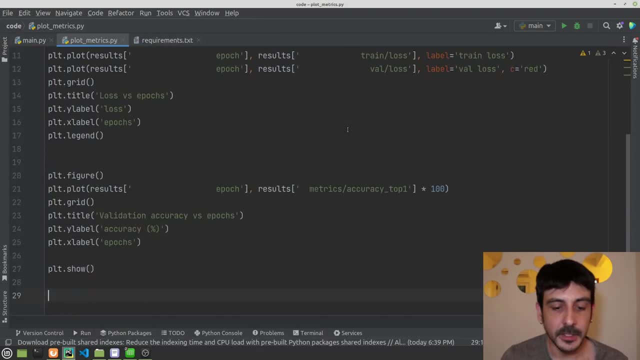 different values and we can definitely plot these values across all these different epochs. so let me show you a python file i have created and this is exactly what this python file does. this file is called plot plot metrics and if i open this file, you can see that it basically we need to set a pad to a resultscsv. 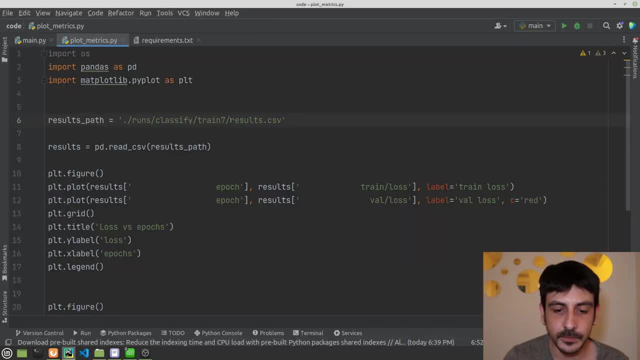 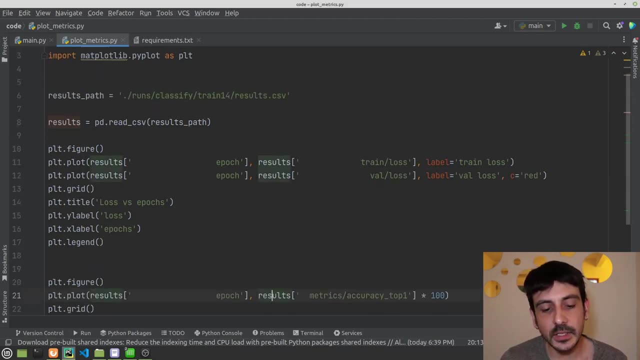 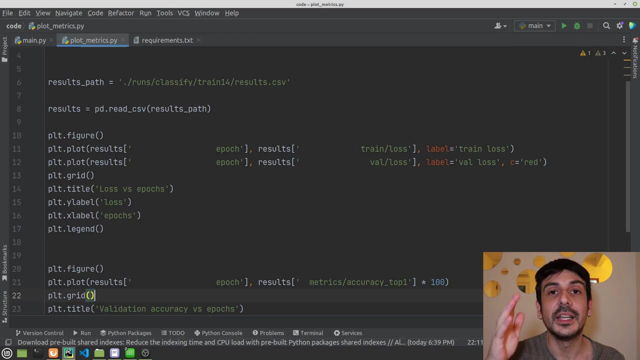 file. in our case, i'm going to set it to train 14, and you can see that this is wrong. classify train 14 and then resultscsv, and then this is only like some logic, some very simple logic: to take all the data from this resultscsv file and to do some plots with it. right, that's all we're doing. we're 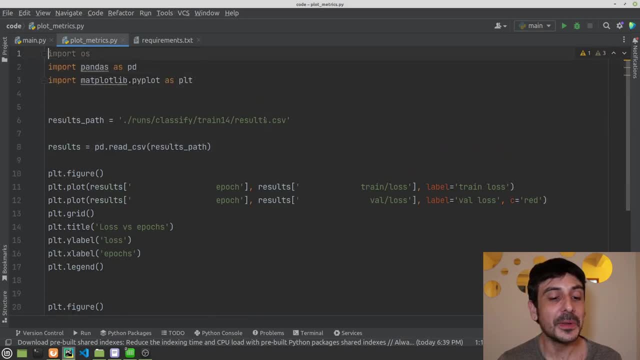 just taking the data and we're going to do some plots with it. right, that's all we're doing. we're doing some plots and this file will be available in the github repository of this project, of this tutorial, so you can definitely take this file and you can just use it to to plot your functions as. 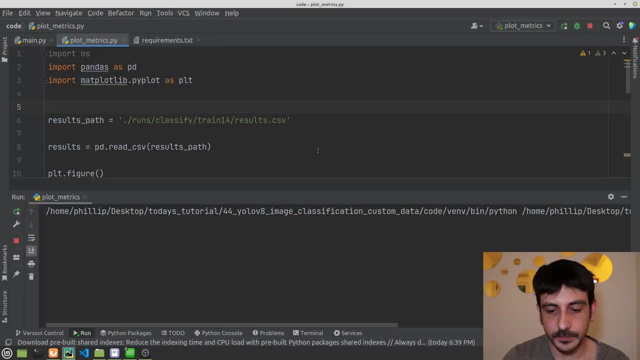 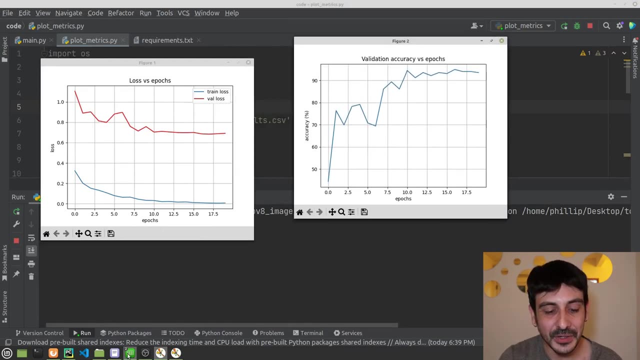 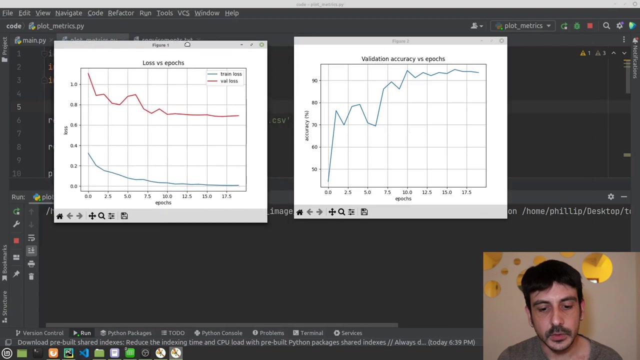 well, all i'm going to do now is just press play and you can see that if we wait only a few seconds, we get all these two plots right and this is all the information in our csv file, right? everything i show you over here, it's summarized on these two plots. so this is exactly what i'm going. to. Я думаю, еслиragen у вас понай veure, вы не сможете зарегистрировать. смотрите, lihatple, Mercy, Look Pain. This is a very, very little, but amazing result. 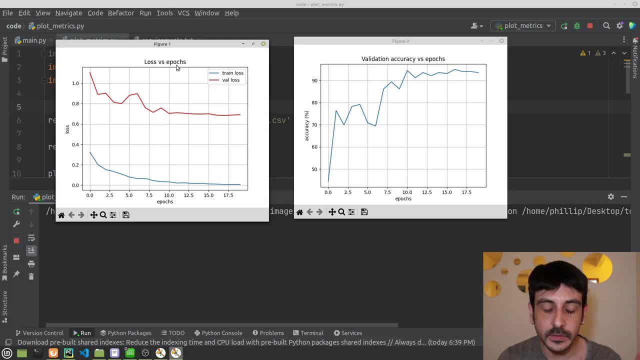 your loss is going down. this is your uh. this is our loss in the training set. this is your uh. this is our loss in the training set and in the validation set. in the training set, we are plotting the loss in blue and in the validation set is red, and you can see that in both cases the loss is going down right, which is exactly what we expect. 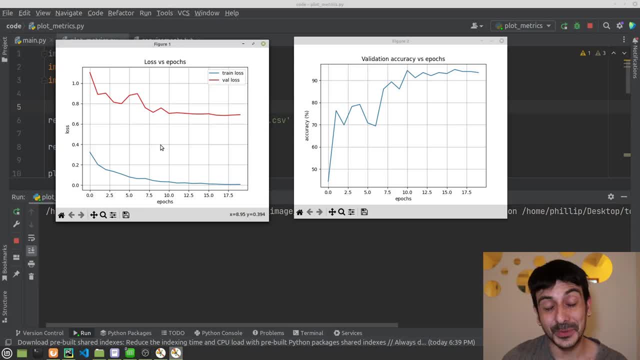 it's exactly what we want now. this is a very, very simple way to analyze this process, but trust me, this is also a very powerful way. right, this is something that's very, very healthy, something that looks like this: it's very healthy. and then for this other plot, which is how the validation 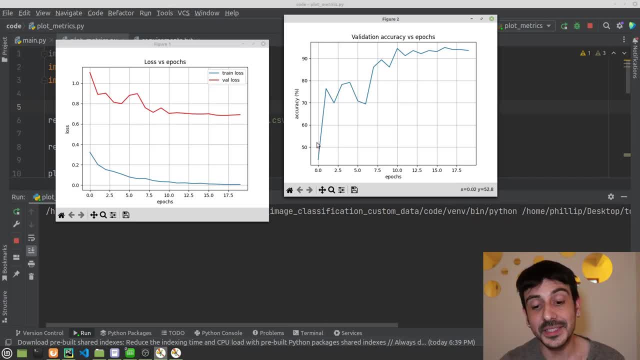 accuracy evolves through this training process. you can see that the validation accuracy goes up when we increase the number of epochs, right, you can see that starting from the 10th epoch or so, everything starts to be like somehow idle. right, we are not really gaining a lot of accuracy from 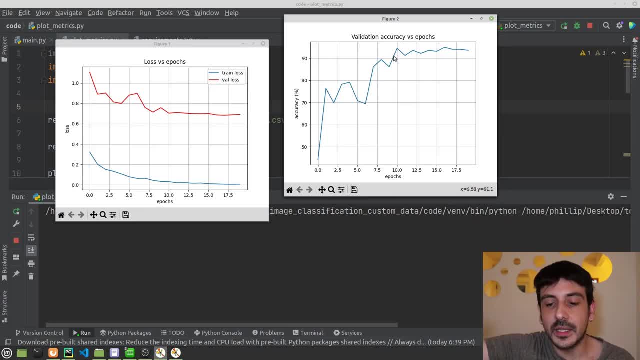 10th epoch or so, everything starts to be like somehow idle. right, we are not really gaining a lot of accuracy from here, but we are not losing accuracy either. right, we are just in something like a plateau, and this is exactly how a forced validation accuracy plot should look like. right, 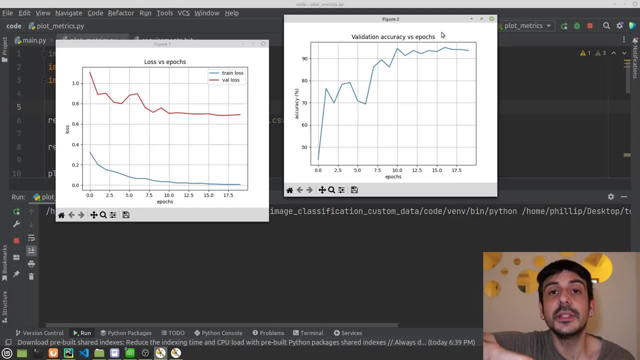 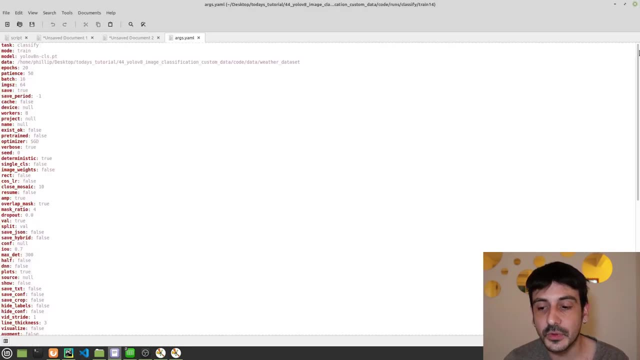 we are starting from a very low value and then we are just increasing our accuracy until we reach a very high value of accuracy. right, this is like a very healthy training process. now, obviously, we could, you know, make this process even better if we just tune, if we just change some of these parameters and if we 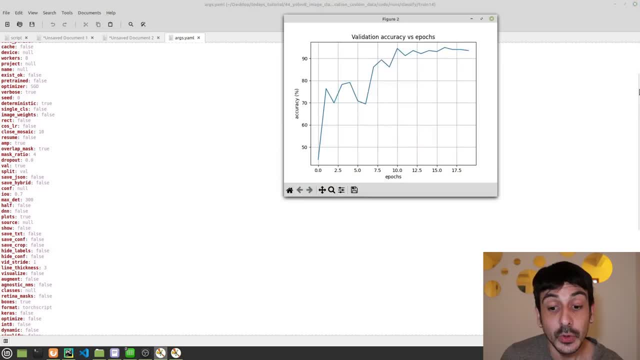 do like a more customized training- i'm sure we are- we will be able to have a better model right because, remember, we are using all the default values. so, as it usually goes, if we make like a more customized training and we have different and we try different parameters and so on, we should. 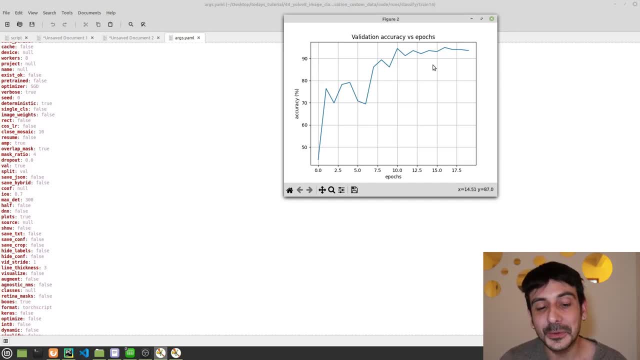 be able to get like a better model. but obviously we are not going to do it in this tutorial because i just want to show you like the end-to-end on how to train this image classifier. but remember you could do it even better than this if you make like a more custom model. so this is pretty much. 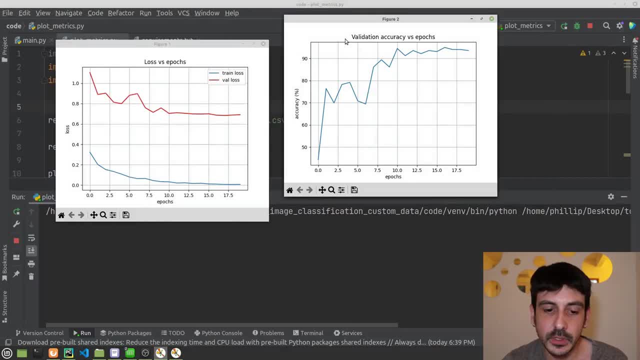 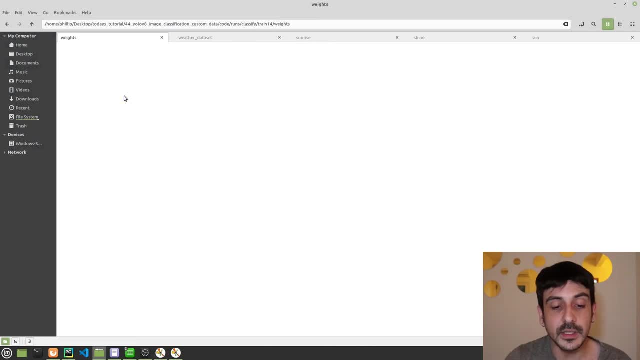 all for analyzing these plots, which are the validation, accuracy and the loss function, in order to validate your training. and then it's like the this directory, which is the weights directory. you can see that this directory is called weights and this is exactly where the models will be saved. 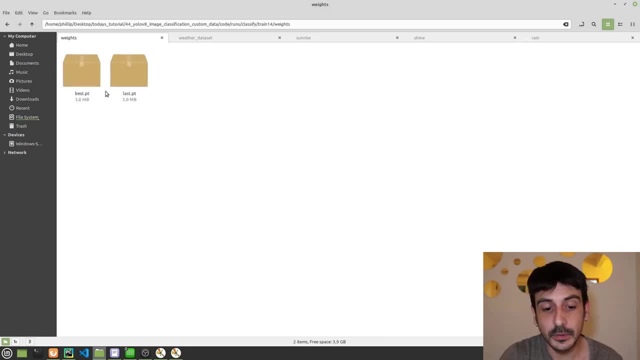 you. this is very important because you have trained a model and now, obviously, you want this model in order to use it in your images, in your data. and this is exactly where you are going to find this model. and you can see that you have two different files. one of them is called lastpt and the other 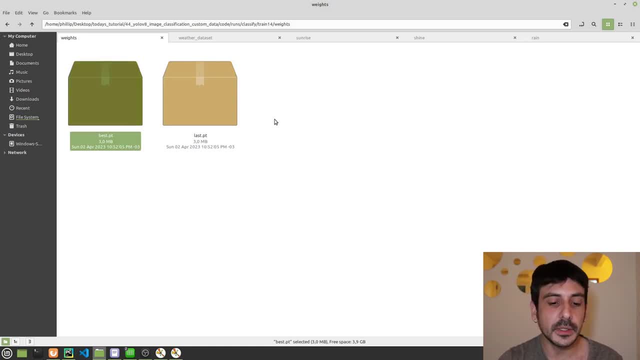 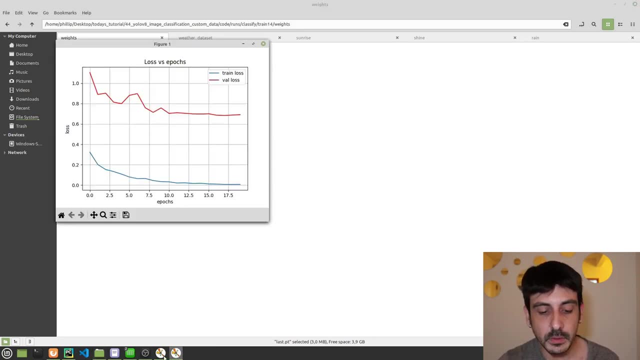 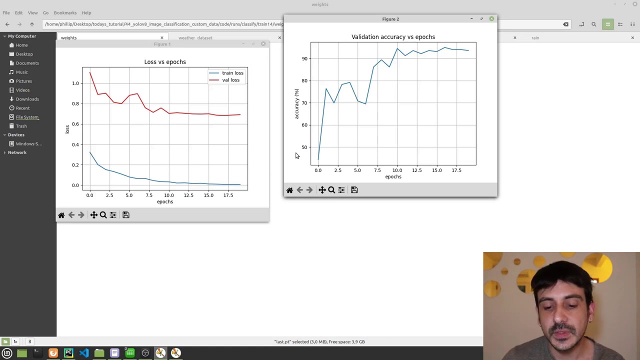 one is called bestpt. now let me explain exactly what these two files are and exactly what they mean. so remember how this training process works right. remember that you have a model. you have a deep learning model which is comprised of many, many, many different weights, and the way it goes is that 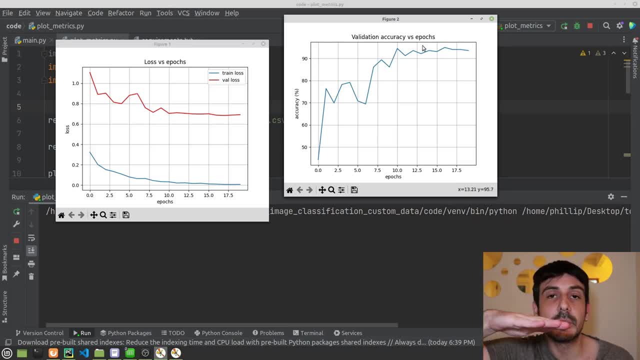 here, but we are not losing accuracy either. right, we are just in something like a plateau, and this is exactly how a trade, a validation accuracy plot, should look like. right, we are starting from a very low value and then we are just increasing our accuracy until we reach a very high value of 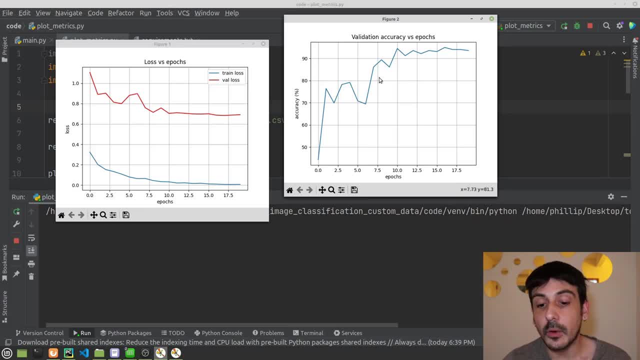 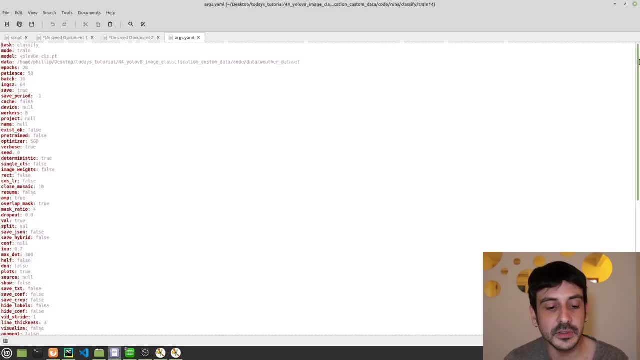 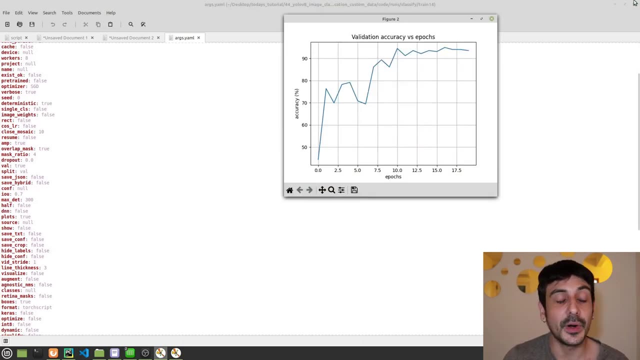 accuracy right. this is like a very healthy training process. now, obviously, we could make this process even better if we just tune, if we just change some of these parameters and if we do like a more customized training- i'm sure we are- we will be able to have a better. 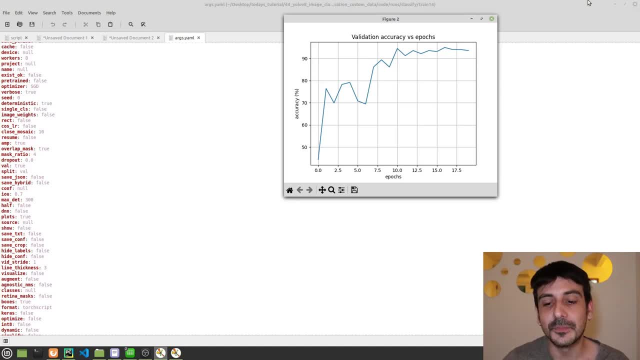 motivation to do this training and i'm sure we will be able to do this training and i'm sure right because, remember, we are using all the full values. so, as it usually goes, if we make like a more customized training and we have different and we try different parameters and so on, we should be 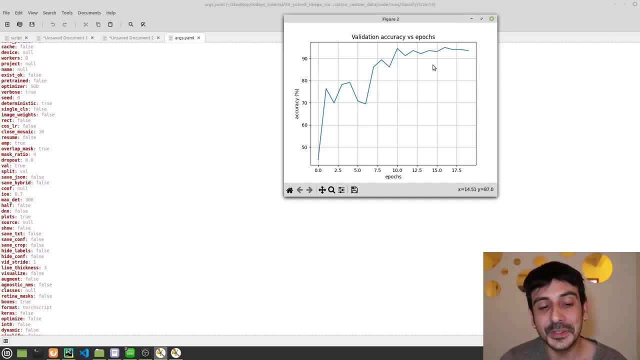 able to get like a better model. but obviously we are not going to do it in this tutorial because i just want to show you, like the end to end, on how to train this image classifier. but remember you could do it even better than this if you make like a more custom model. so this is pretty much. 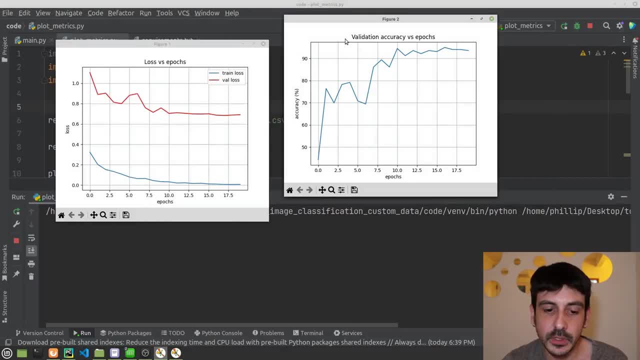 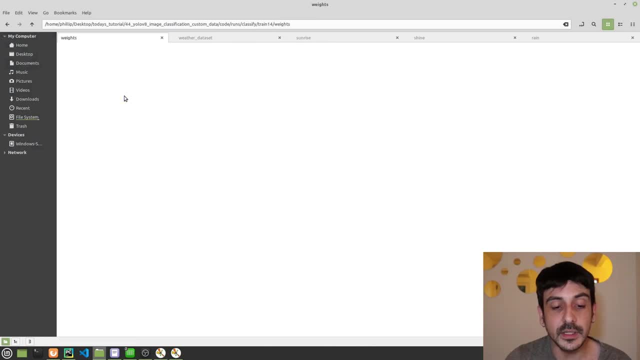 for analyzing this plots, which are the validation, accuracy and the loss function in order to validate your training. and then it's like the this directory, which is the weights directory. you can see that this directory is called weights and this is exactly where the models will be saved. this is very important because 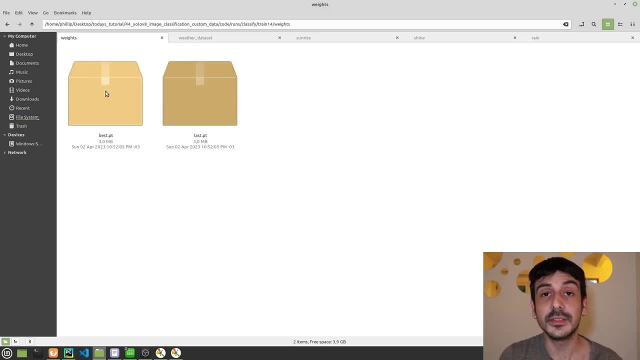 you have trained a model and now, obviously, you want this model in order to use it in your images, in your data, and this is exactly where you're going to find this model and you can see that you have two models. you have two models and you can see that there's two models E, which are essentially 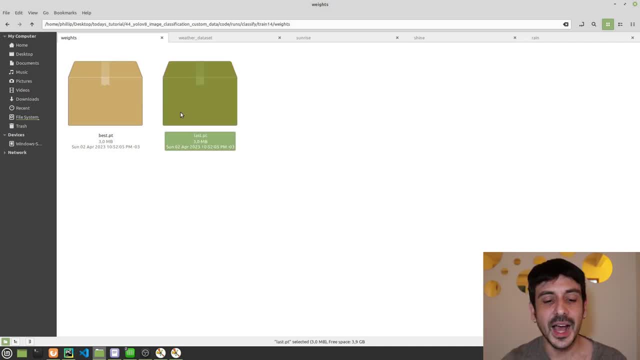 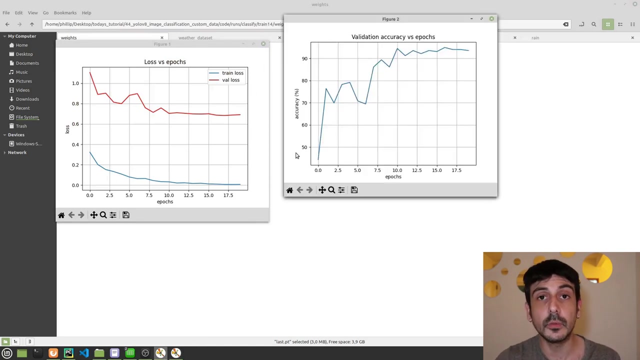 two different files. one of them is called lastpt and the other one is called bestpt. now let me explain exactly what these two files are and exactly what they mean. so remember how this training process works right. remember that you have a model. you have a deep learning model, which 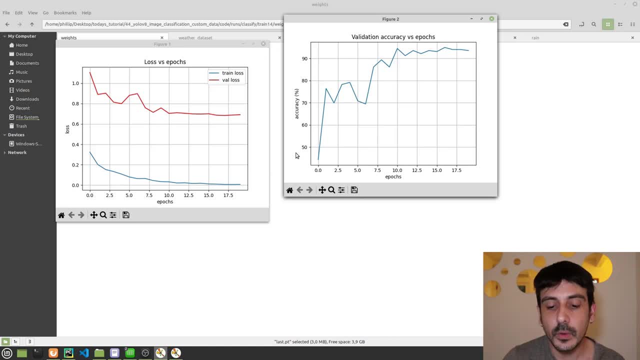 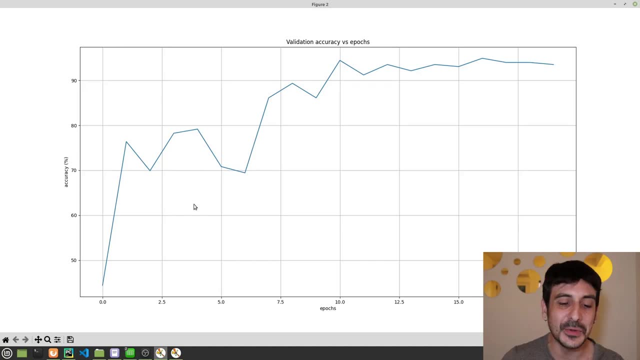 is comprised of many, many, many different weights, and the way it goes is that at the end of every epoch, right at the end of the first epoch, of the second epoch, of the third epoch, and so on, you are updating the weights of your model, you are updating the weights of your architecture of. 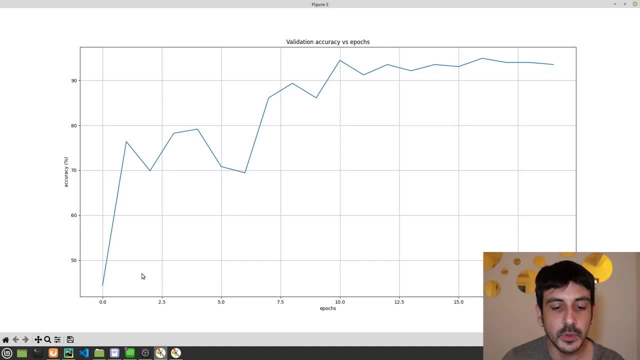 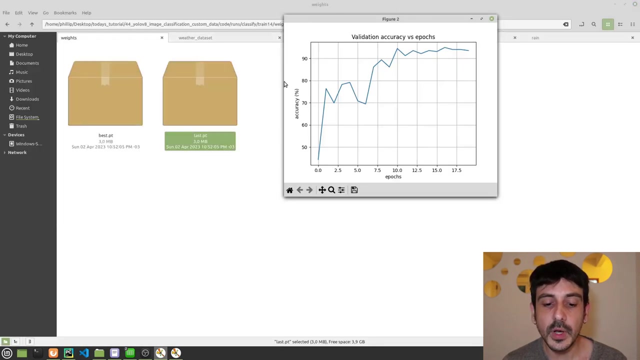 at the end of every epoch, right at the end of the first epoch, of the second epoch, of the third epoch, and so on, you are updating the weights of your model. you are updating the weights of your architecture, of your deep learning model. so the the way it works is that at the end of every epoch, 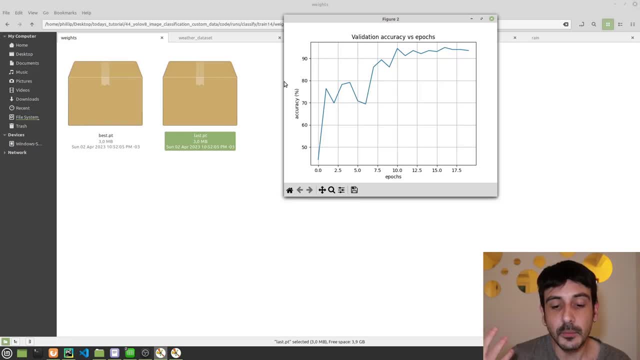 you have a model available which is a model you have trained so far with all the process you have followed so far. so lastpt means that you are taking the model which was the result of the last epoch of your training process, right. remember, at the end of absolutely every single: 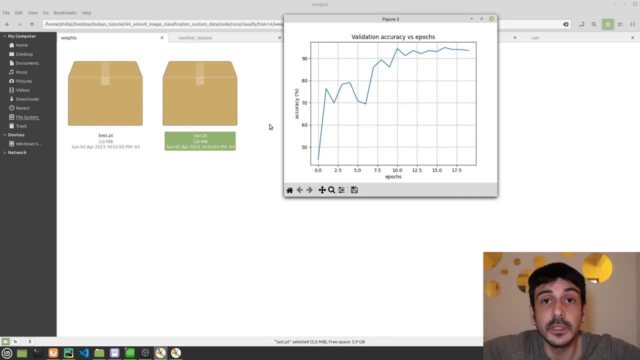 epoch. you have a model available. you have a model which you can definitely use, if you want to, in order to produce your inferences and so on. so lastpt only means that you are taking the last model, the model which was produced at the end of your training process. so lastpt means that you 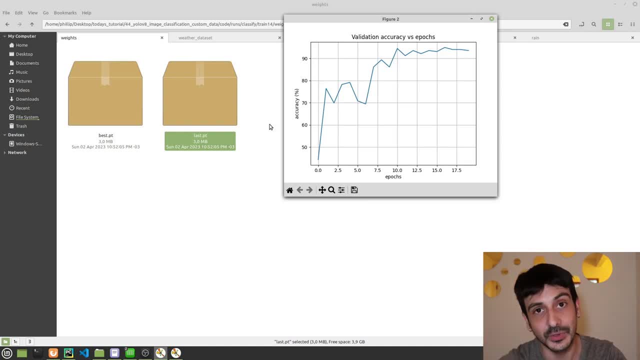 are training process, at the end of the last epoch in your training process, so at the end of the 20th epoch in our training process, we are producing this model, which is lastpt. but you may wonder: hey, felipe, yeah it's, it's great because at the end of our training process- or accuracy is something like- 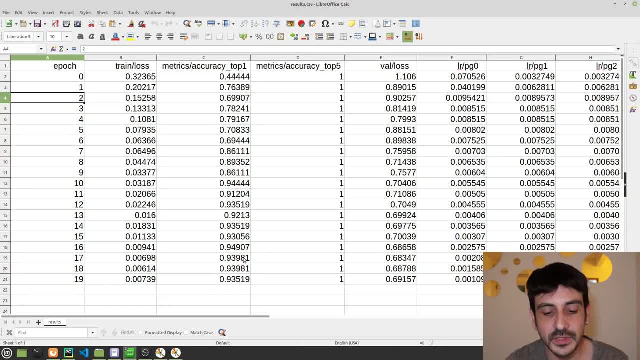 a 93 percent right and 93 percent is it's. it's a very good accuracy. but if we take the accuracy, if we take the model at the end of the 16th epoch, for example, or accuracy it's, it's higher, it's a 94.9- maybe it makes more sense to take that model instead. 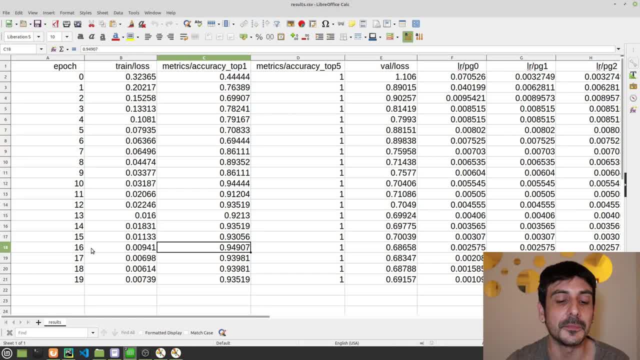 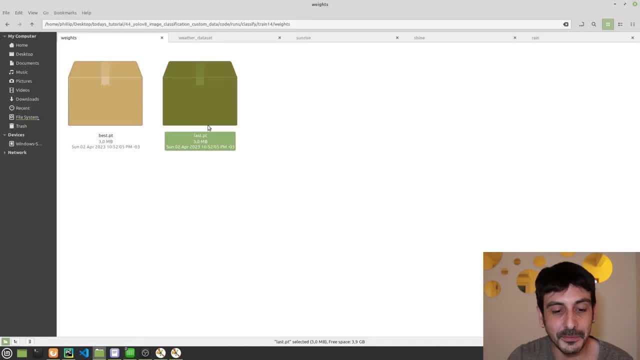 right because we have an even better accuracy. we have an even higher accuracy, and if you ask me something like that, i would say: yeah, you're perfectly right, you're, you're super, super right. that's a very valid argument and that's exactly what the bestpt model is: right, we are saving. 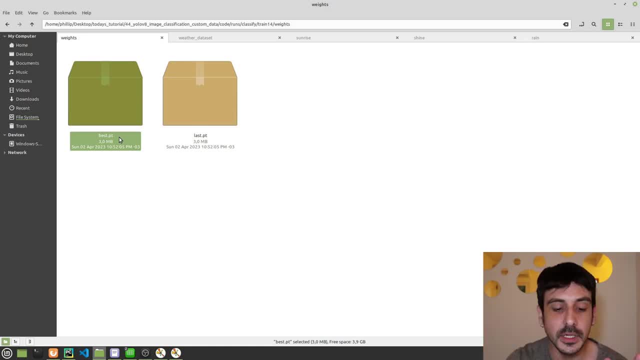 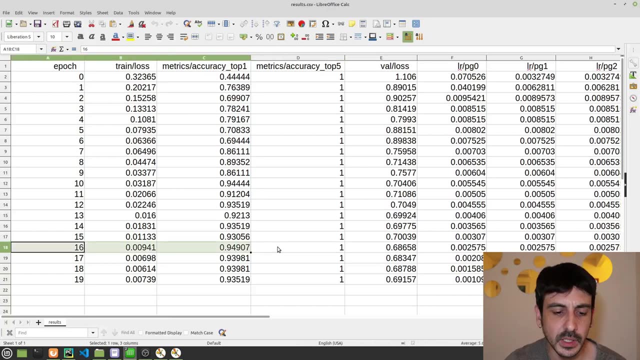 the weights of the best model in our entire training process. so if we look at our data, the best model in our training process is this one. if i'm not mistaken right, it's the model we produced at the end of the 16th epoch and our accuracy, or radiation accuracy, was 94.9. 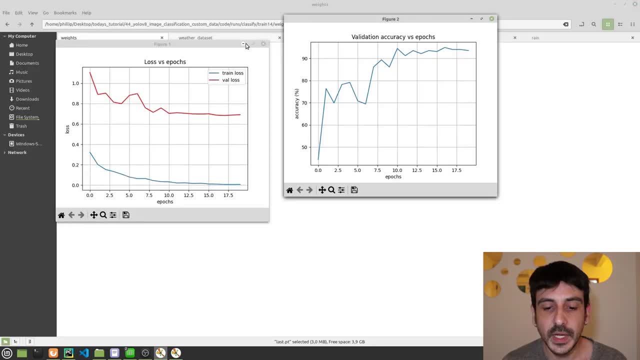 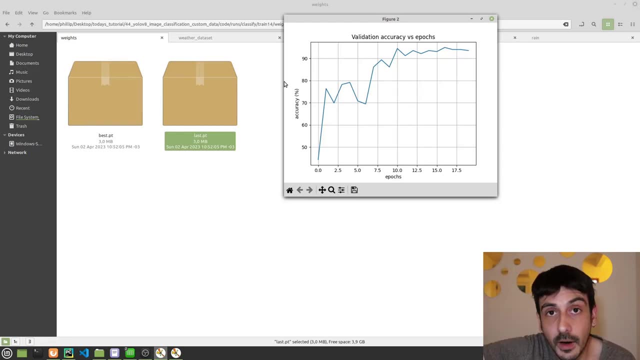 your deep learning model. so the the way it works is that at the end of every epoch you have a model available which is a model you have trained so far with all the process you have followed so far. so lastpt means that you are taking the model which was the result of the last epoch of your 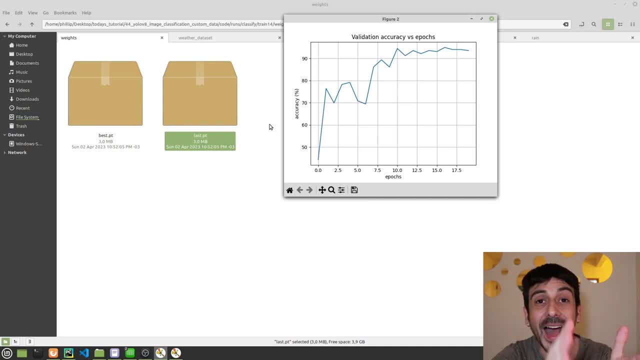 training process. right, remember, at the end of absolutely every single epoch, you have a model available. you have a model which you can definitely use, if you want to, in order to produce your inferences and so on. so lastpt only means that you are taking the last model, the model which was produced at the end of your 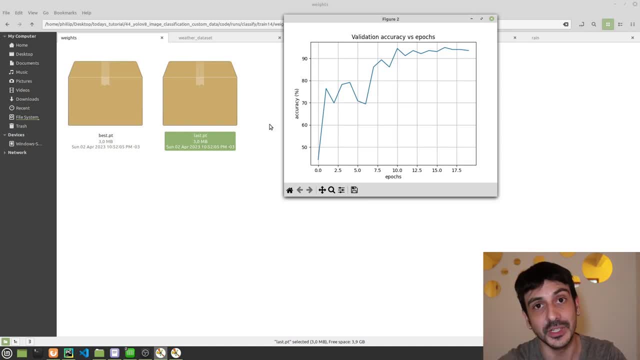 training process. at the end of the last epoch in your training process, so at the end of the 20th epoch in our training process, we are producing this model, which is lastpt. but you may wonder: hey, felipe, yeah it's, it's great because at the end of our training process, 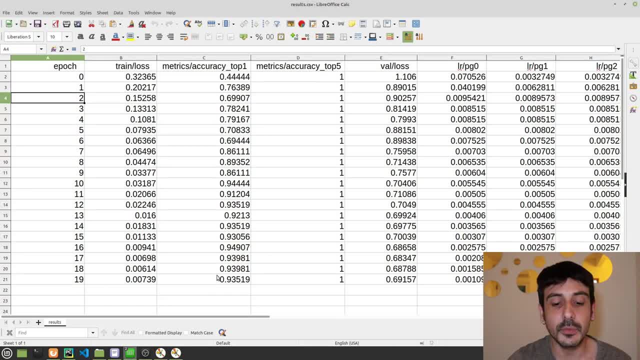 or accuracy is something like a 93 percent. right, and 93, it's, it's, it's a very good accuracy. but if we take the accuracy, if we take the model at the end of the 16th epoch, for example, or accuracy, it's, it's higher, it's a 94.9 percent. maybe it makes more sense to take that model instead, right? 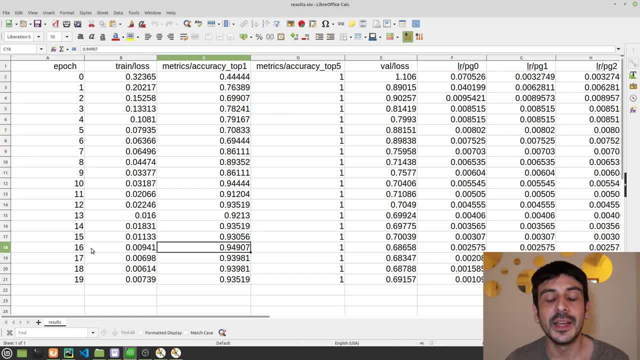 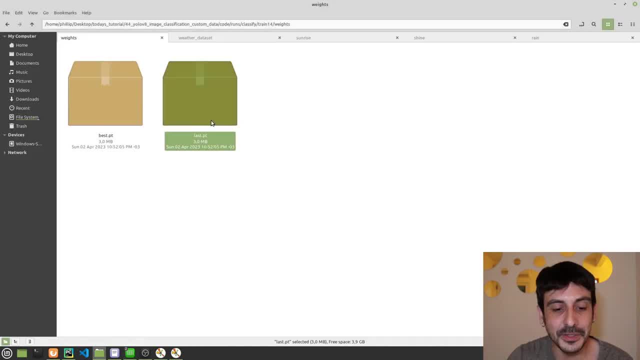 because we have an even better accuracy. we have an even higher accuracy, and if you ask me something like that, i would say: yeah, you're perfectly right, you're, you're super, super right. that's a very valid argument and that's exactly what the bestpt model is. right, we are saving the weights. 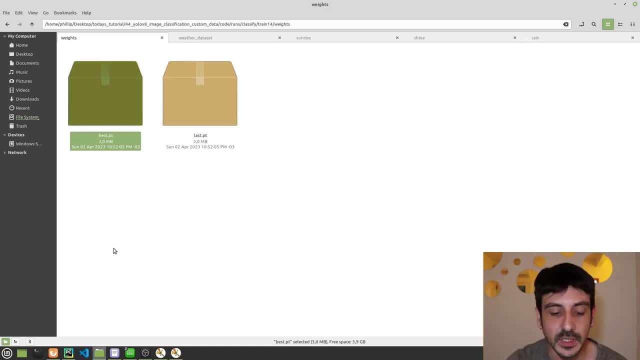 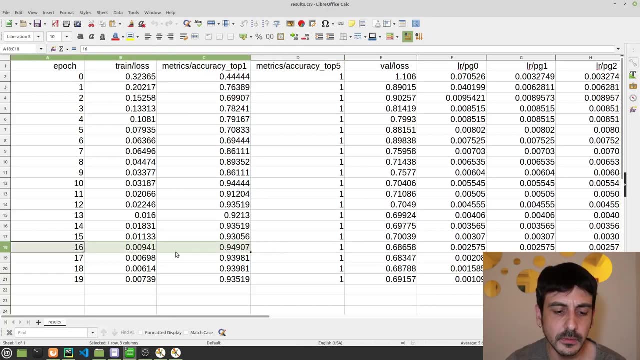 of the best model in our entire training process. so if we look at our data, the best model in our training process is this one. if i'm not mistaken right, it's the model we produced at the end of the 16th epoch, and our accuracy, or radiation accuracy, was the best model in our training. 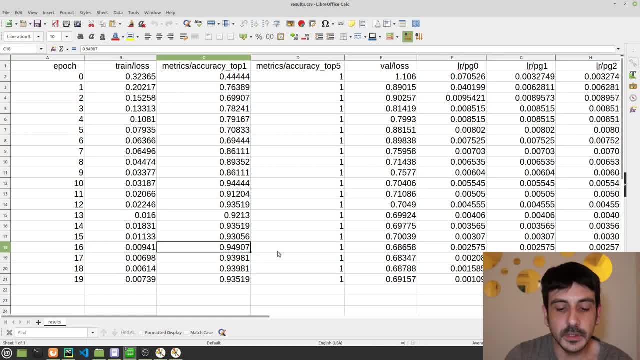 process it was 94.9 percent. so this is definitely higher than the accuracy we got at the end of this training process, which has, which was a 93.5 percent, and if we will take the best model we have produced in the entire process, in the entire training process, then we will definitely need to. 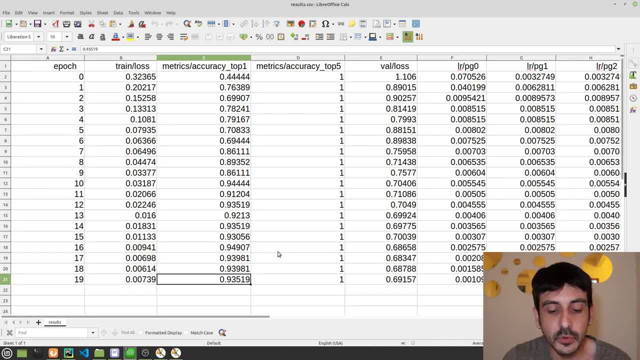 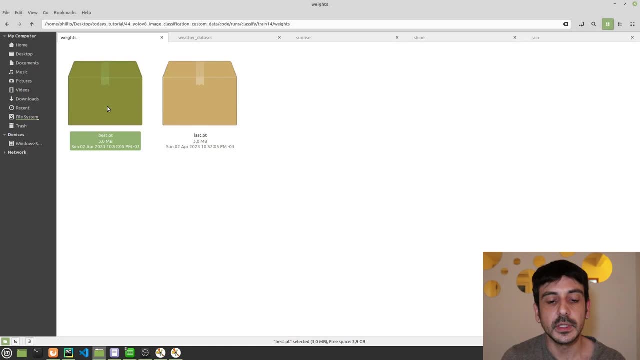 so this is definitely higher than the accuracy we got at the end of this training process, which has, which was 93.5 percent, and if we will take the best model we have produced in the entire process, in the entire training process, then we will definitely need to take this model. so this is exactly what bestpt represents: is the best training. 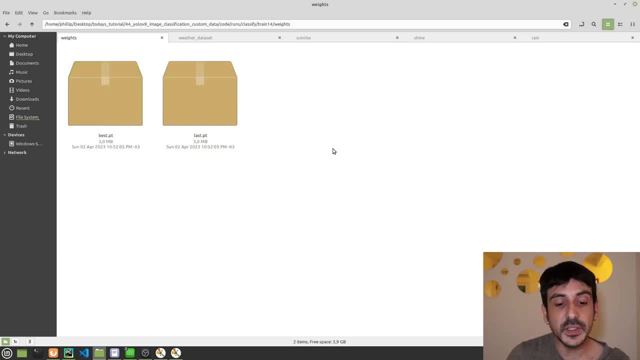 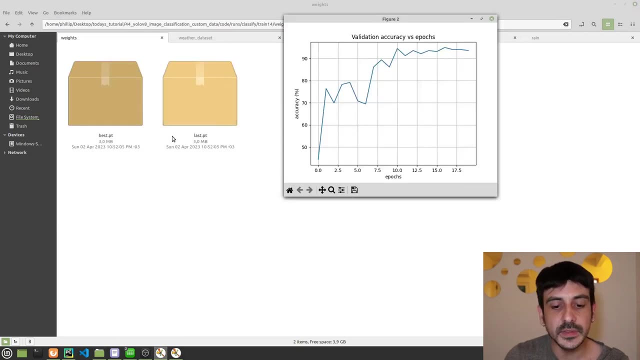 the best model you have trained in your training process. and, if you ask me, what i usually do is taking the model which was produced at the end of this training process. right, what i usually do is taking the lastpt file because i consider that this, this is the model we have produced at the 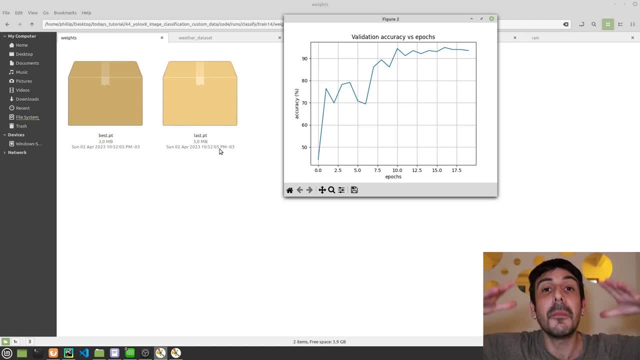 end of the training process. in this model, we are summarizing much more information, right, because we are considering much more data. we are considering much more everything in all this training process, many things are going on, many, many things are going on and, remember, there's a lot of randomness in this training process. so i, me personally, i consider that if 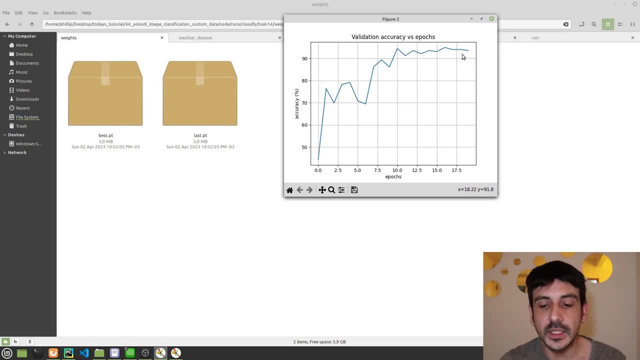 i take the model which was trained at the end of this process is a much better option that if i choose another one. if i choose, like the best model or the model which i got the highest accuracy, but it's not the last model. that's what i usually do. i usually take the last model which was 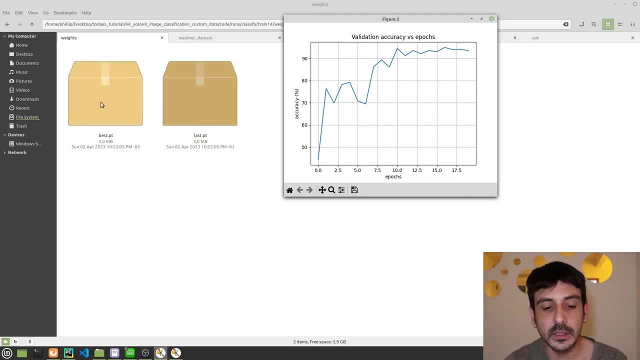 produced at the end of the training process. but if you want to take the best model, if you want to take the bestpt, it also makes sense because you are taking the model which produced the highest accuracy right. so you can do either one of them and i think it's a very, a good option. that's why 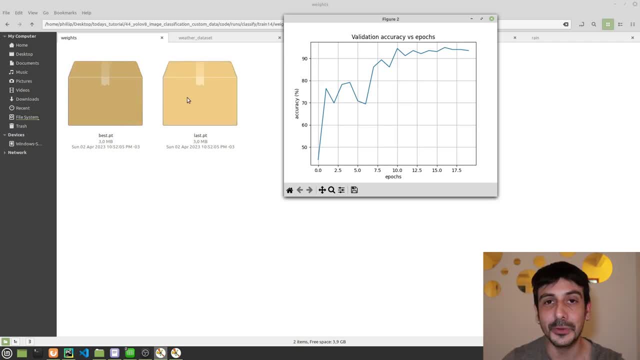 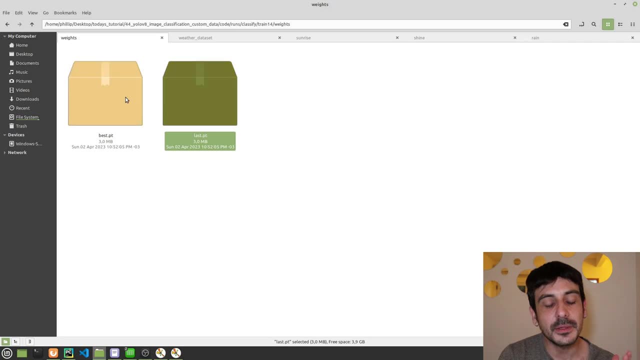 you have these two files because you can use one of them or you can use the other one, and i will say that making like a very, very like the best decision on which mode to use depends on many different variables, depends on many different things, depends on your data, depends on your problem, depends on your use case depends. 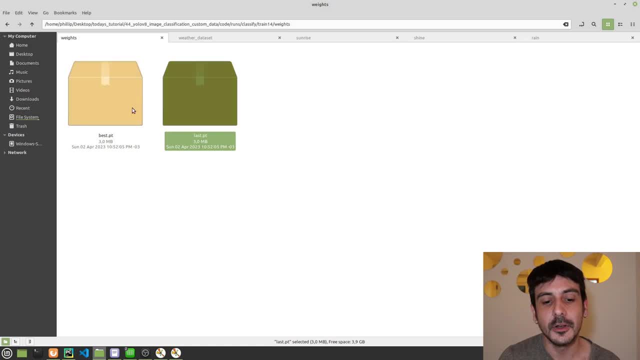 depends on your training process, depends on many, many different things. which is the best option, right? so remember, you have these two models and it's all up to you. it's all up to your specific project and it's all up to your preferences which model you want to use, right, if the best model? 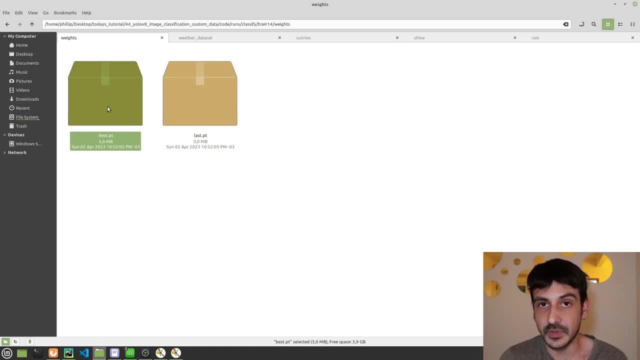 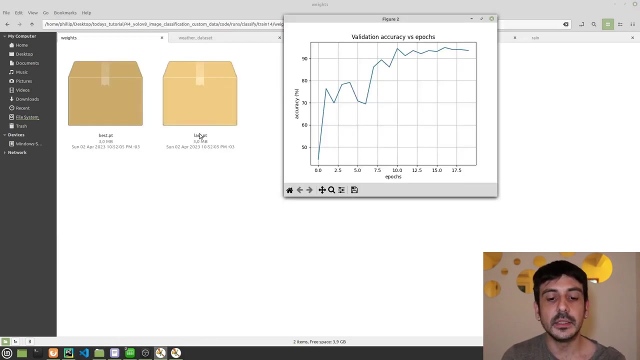 take this model. so this is exactly what bestpt represents: is the best training, the best model you have trained in your training process. so let's take a look at the model which was produced at the end of this training process. right, what i usually do is take the lastpt file, because i consider that this, this is a model we 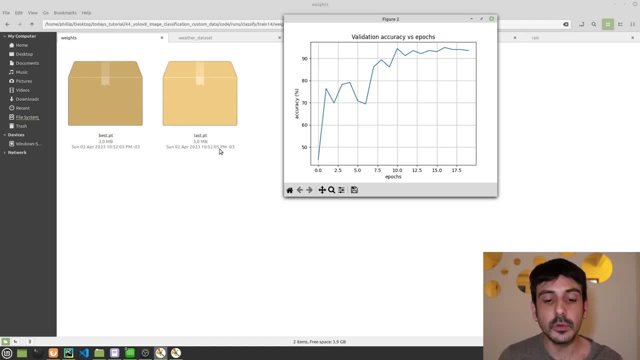 have produced at the end of the training process. in this model, we are summarizing much more information. right, because we are considering much more data. we are considering much more everything in all this training process. many things are going on, many, many things are going on and remember. 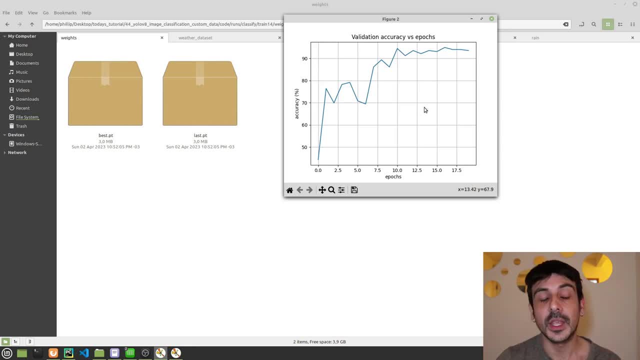 there is a lot of randomness in this training process, so i, me personally, i consider that if i take the model which was trained at the end of this process is a much better option that if i choose a another one, if i choose, like the best model or the model which i got the highest accuracy, but it's not the last. 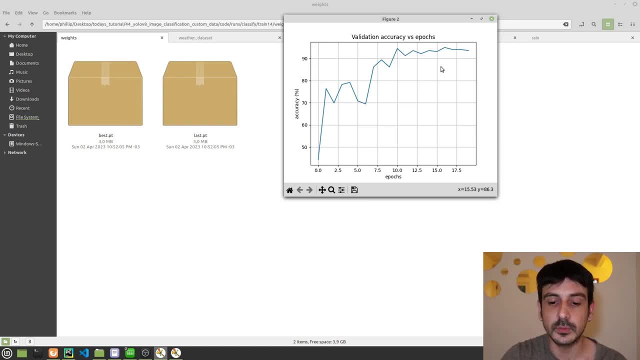 model. that's what i usually do. i usually take the last model which was produced at the end of the training process. but if you want to take the best model, if you want to take the bestpt, it also makes sense because you are taking the model which produced the highest accuracy. 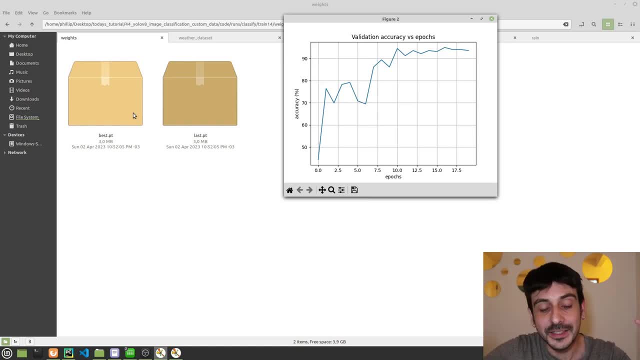 right. so you can do either one of them, and i think it's a very, a good option. that's why you have these two files, because you can use one of them or you can use the other one, and i will say that making like a very, very like the best decision on which mode to use depends on many different variables. 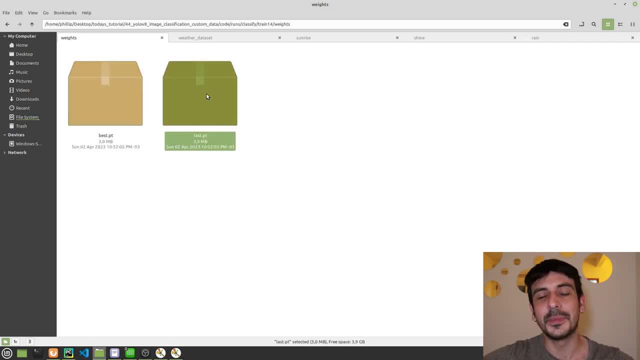 depends on many different things, depends on your data, depends on your problem, depends on your use case depends. depends on your training process, depends on your training process, depends on your process, depends on many, many different things. which is the best option, right? so remember, you have these two models and it's all up to you, it's all up to your specific project and it's all up to. 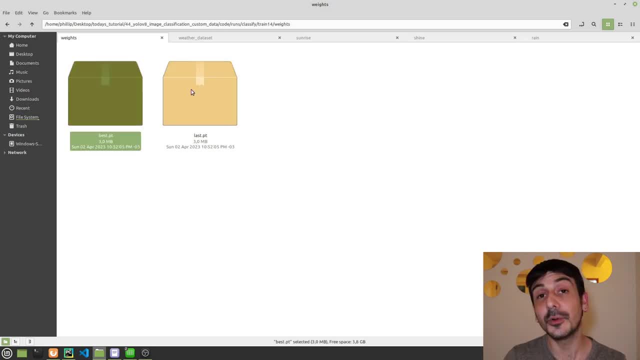 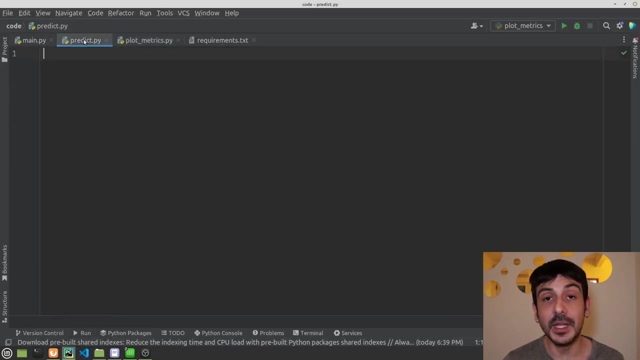 your preferences, which model you want to use, right, if the best model which you have produced through the entire training process, or if you want to use the last model, the model which you have produced at the end of your training process. so now let's go back to pycharm, because now it's time to 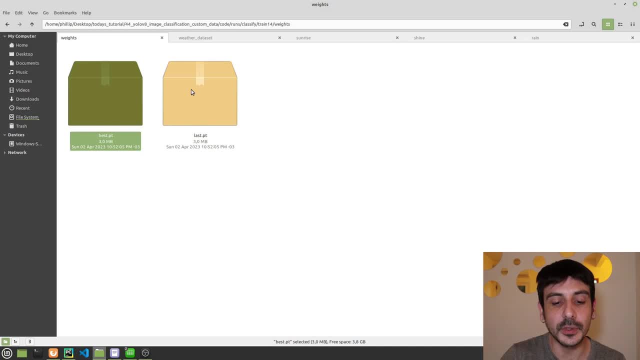 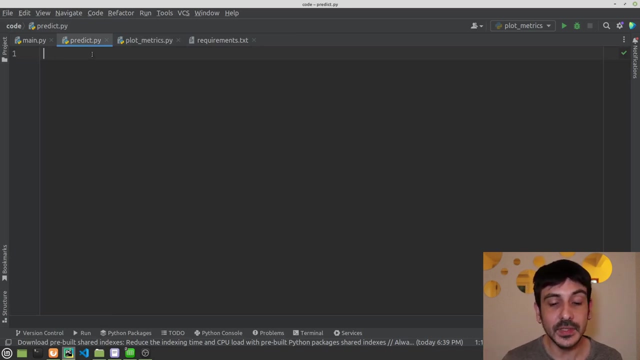 which you have produced through the entire training process or, if you want to use the last model, the model which you have produced at the end of your training process. so now let's go back to PyCharm, because now it's time to make our inferences, now it's time to predict new samples. 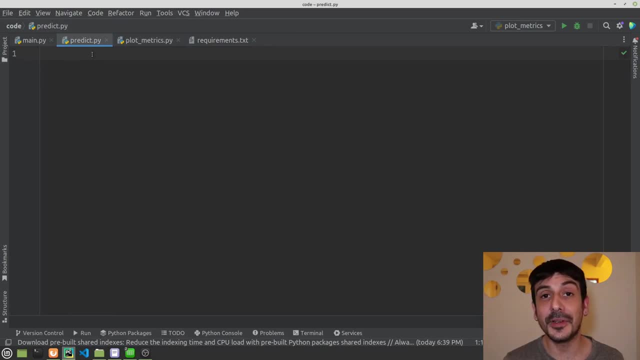 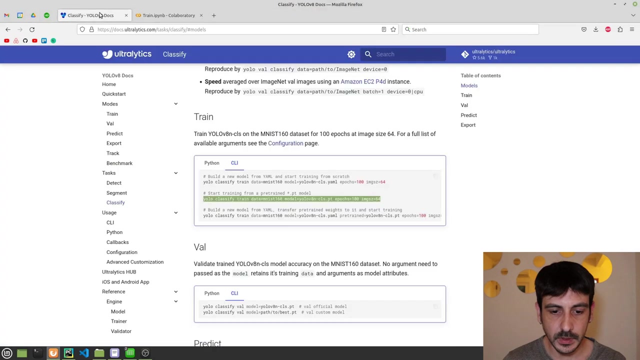 right, we are going to input an image and we're going to use our image classifier in order to predict which category this image belongs to. so let me show you how to do it. i'm going to import from ultralytics, import yolo, and then let's go back to this page, because now we are going to move. 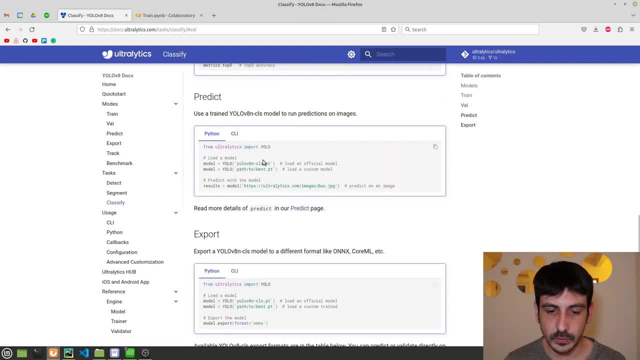 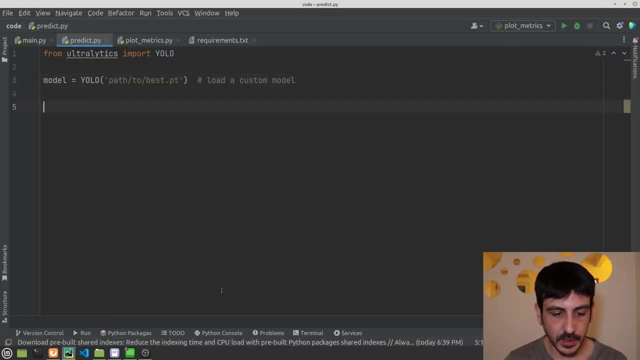 to the predict section, and the only thing i'm going to do is to copy this sentence. i'm going to paste it here, and then i'm going to specify the path, the absolute path, to the model which we have trained. right, we don't really need to make it like the absolute path. 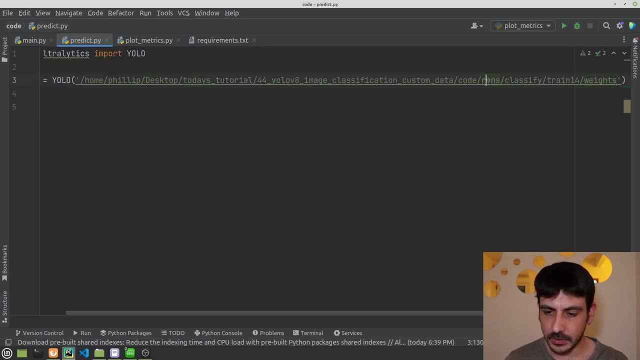 we can use the relative path. so i'm going to do something like this, right, sorry, something like this. so this is the path to the model we have just trained, right? this is the last model which we produce at the end of this training process and this is the model i'm going to use in order. 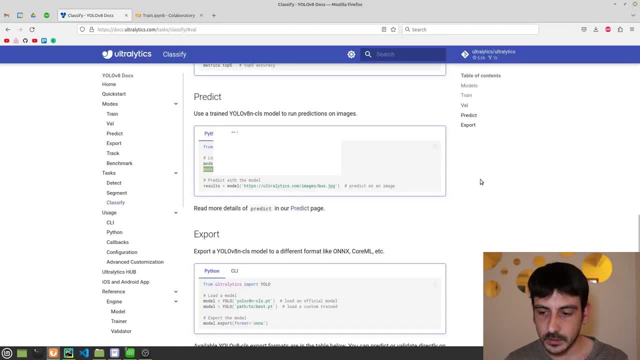 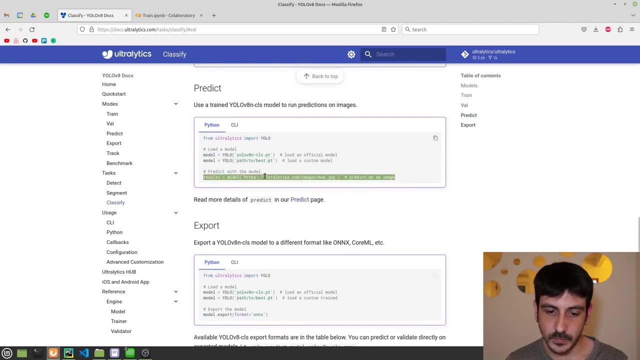 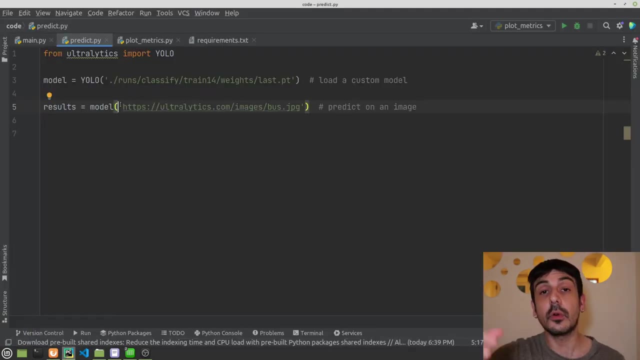 to show you how this works. and now let's copy this additional sentence, which is: results: equal model and the model pad, the image path. right. you can see that you can use an image in your local computer, in your file system, or you can also use something like an url, for example in: 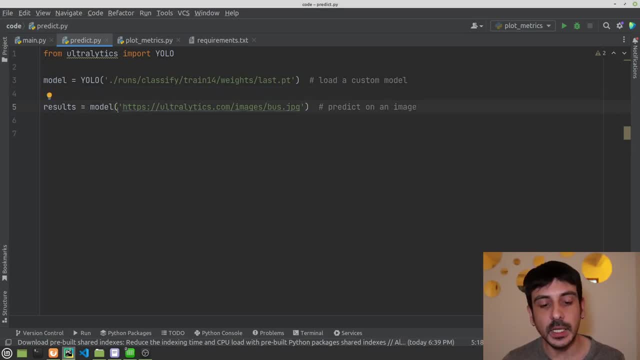 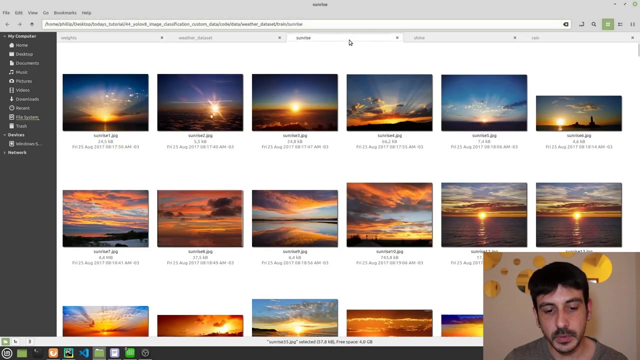 this in this case, in this example which is in the yolo v8 website, you can see that the example is using a new arrow and this is also going to work. so in my case, i'm going to use an image in my local computer. i'm going to use one of the images i used for training, because i only want to show you. 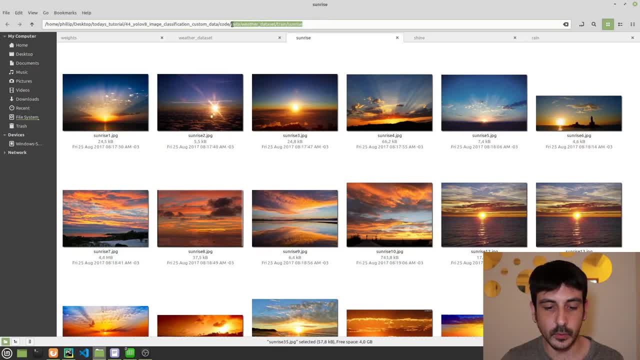 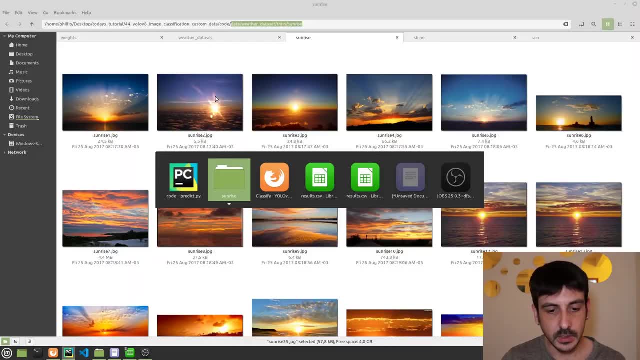 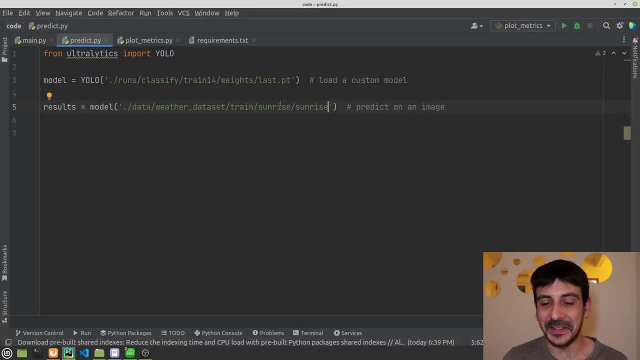 how this works. but obviously you can use whatever data, whatever image you want. so this is the image i am going to use. i'm just going to use, i'm just going to inference this image right, which is the first image in my sunrise category data. so this is going to be something like sunrise1.jpg. 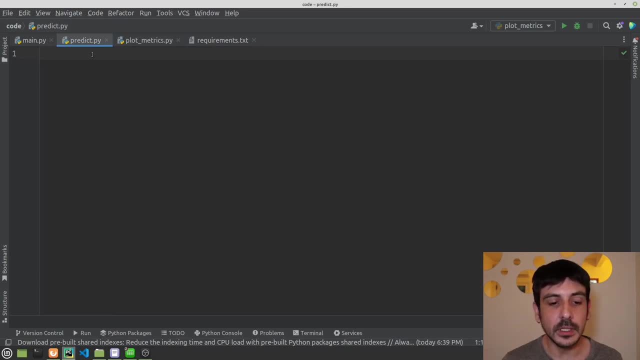 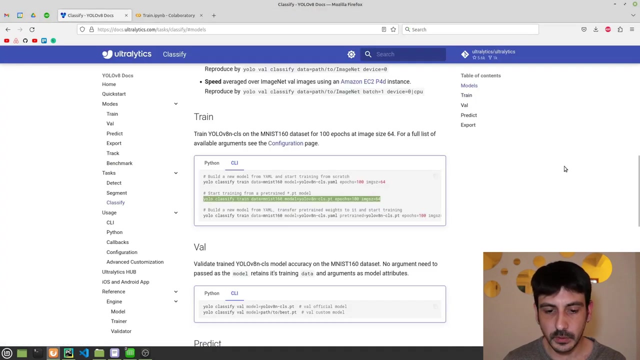 make our inferences. now it's time to predict new samples. right, we are going to input an image and we're going to use our image classifier in order to predict which category this image belongs to. so let me show you how to do it. i'm going to import from ultralytics, import yolo, and then let's go back to this page, because now 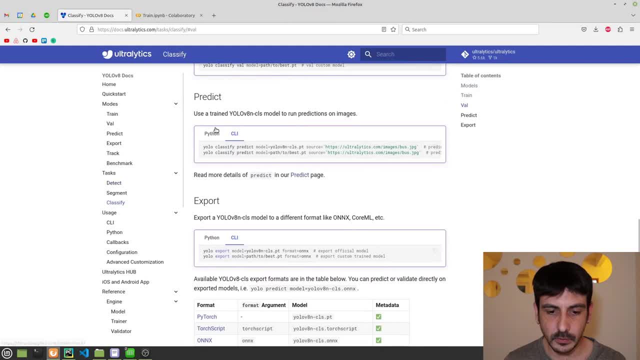 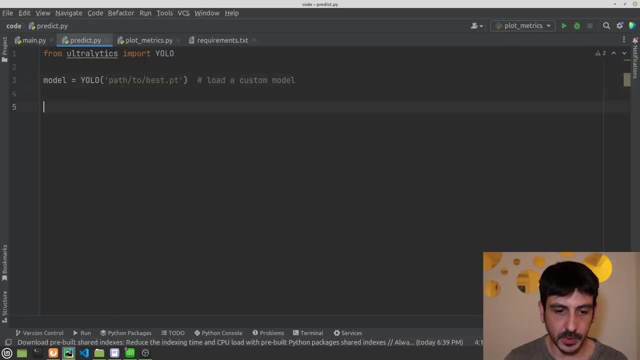 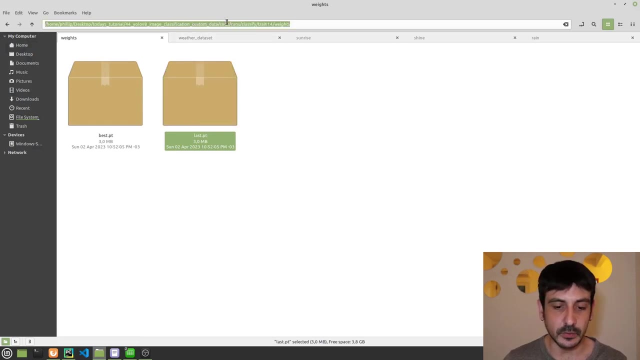 we are going to move to the predict section, and the only thing i'm going to do is to copy this sentence. i'm going to paste it here and then i'm going to specify the path, the absolute path, to the model which we have trained. right, we don't really need to make it like the absolute. 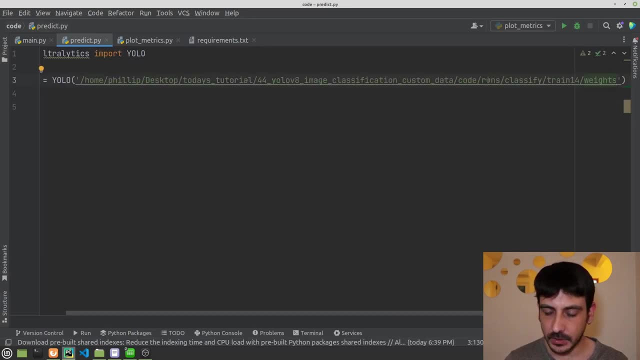 path, we can use the relative part. so i'm going to do something like this, right, sorry, something like this. so this is the path to the model we have just trained, right? this is the last model which we produce at the end of this training process and this is the. 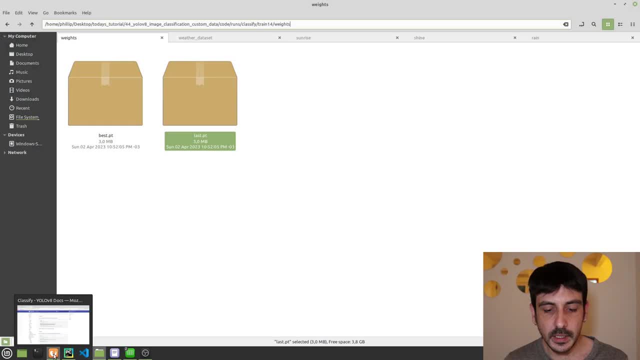 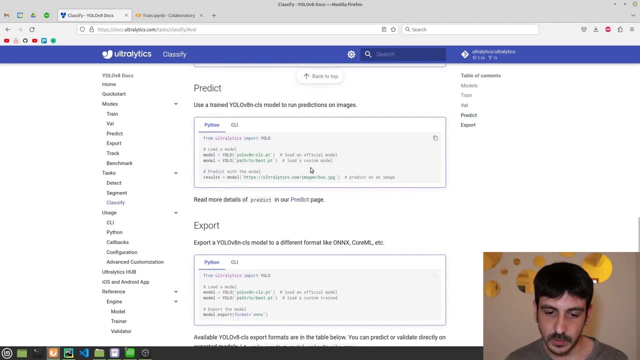 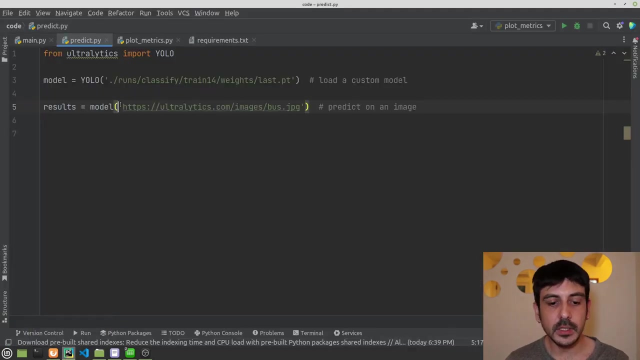 model i'm going to use in order to show you how this works. and now let's copy this additional sentence, which is: results: equal model and the model path, the image path. right, you can see that you can use an image in your local computer, in your file system, or you can also use something. 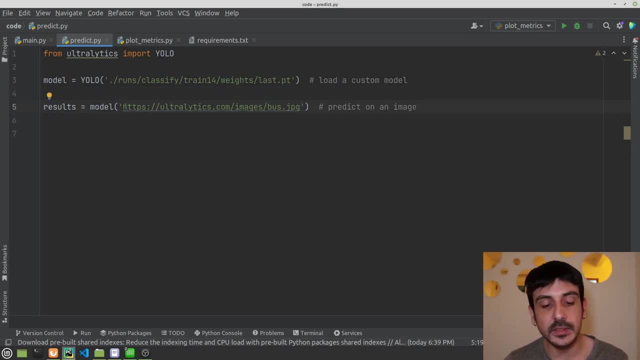 like an url, for example, in this case, i'm going to use an image in my local computer, in my file system. for example, in this, in this case, in this example, which is in the yellow v8 website, you can see that the example is using a neural and this is also going to work, so in my case, i'm going to use an. 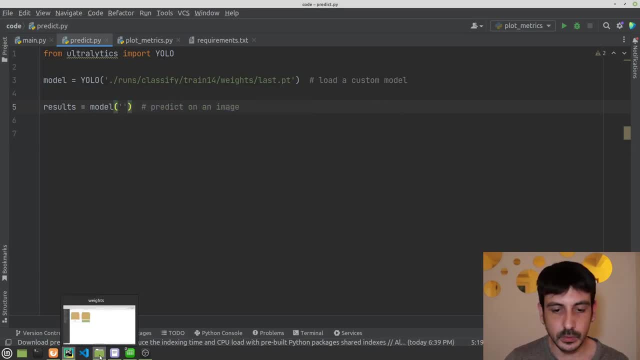 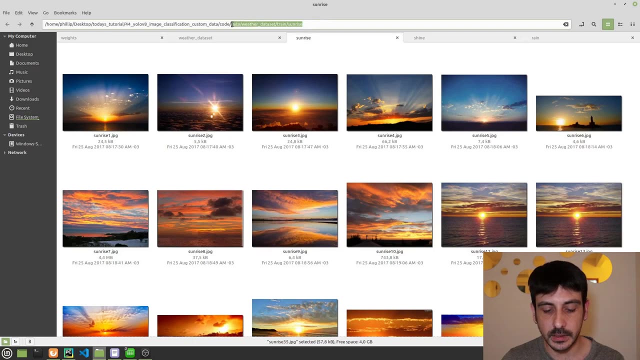 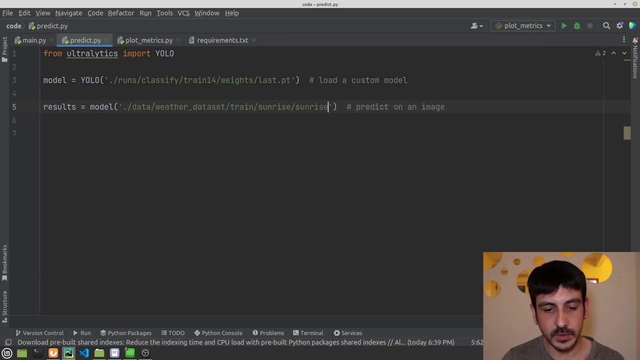 image in my local computer. i'm going to use one of the images i used for training because i only want to show you how this works, but obviously you can use whatever data, whatever image you want. so this is the image i am going to use. i'm just going to use, i'm just going to inference this. 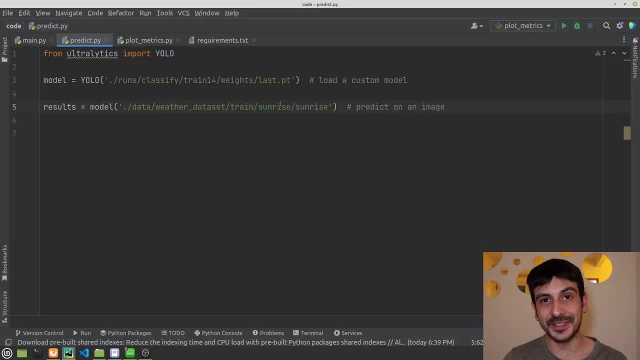 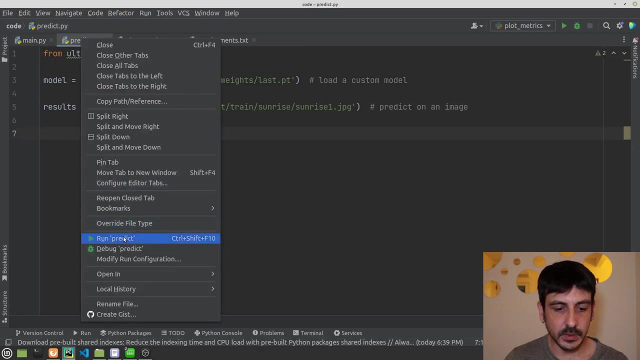 image right, which is the first image in my sunrise category data. so this is going to be something like sunrise1.jpg and this is pretty much all. so these are the results. the first thing i'm going to do is just trying to run this code and let's see what happens. everything should run smoothly. 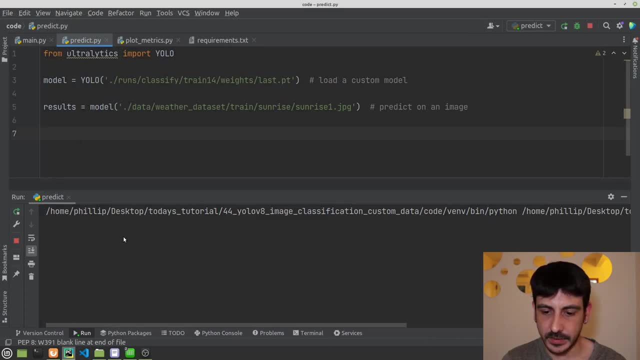 but this is where we are going to see if we have an error or something needed. we may need to wait a couple of seconds and everything seems to be working fine because we didn't get any error. so what I'm going to do now is I'm going to 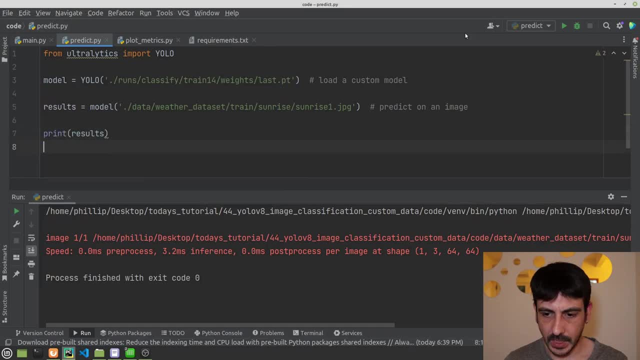 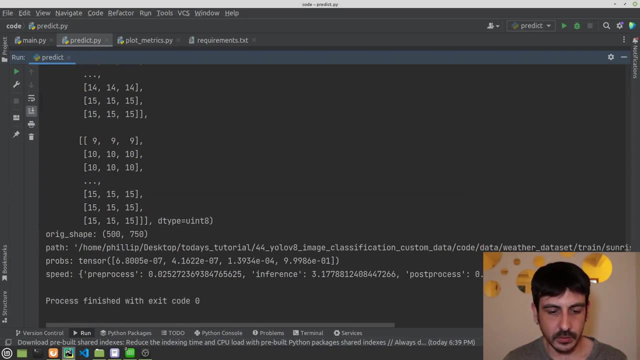 print results because I want to show you a couple of things. so this is the entire information we are getting when we are printing results. right, you can see that this is a lot of information. we have these probabilities, which is the inferences we are making. this is exactly the result of applying our image. 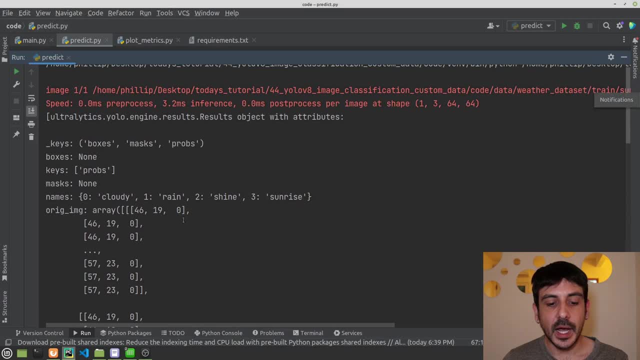 classifier and then we have a lot of information, another object or another result which is very important, is this one, which are the names of the categories we have just train or image classifier on right you can see this is cloudy, rain, shine, sunrise, and also you can see that we have different. 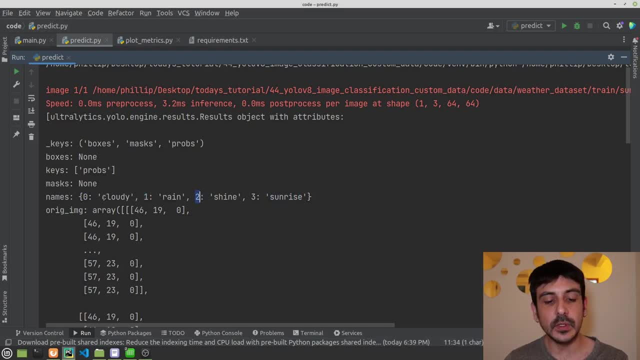 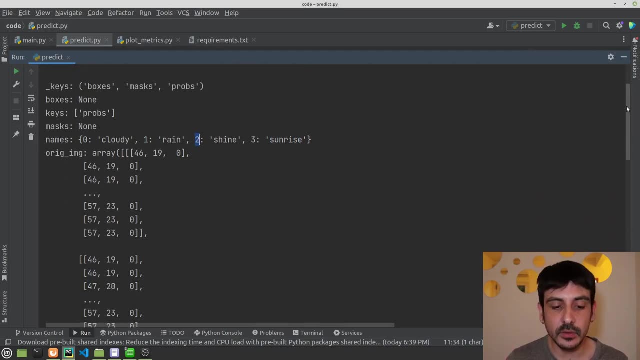 interval use for each one of these categories. so this is something like a dictionary, because we are going to have our result for from applying our image classifier and then, with this result, which is going to be an integer, we are going to call this dictionary. we're going to call this object because we want. 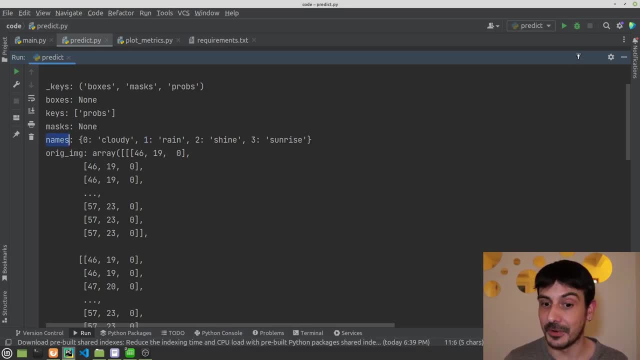 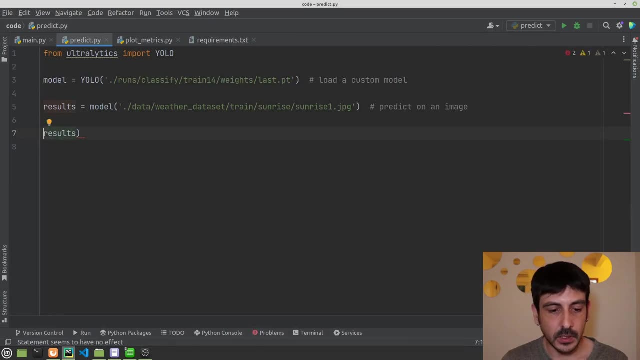 to know exactly what's the name of the category we have just inferenced, right? so this is how we're going to do it. i'm going to call another variable, which is going to be names, something like names, dictionary names, ticked, and this is results zero, because results is a list. in this case, we only 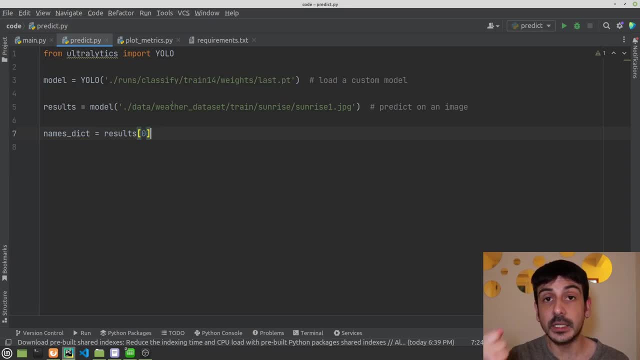 want to access the first element, because we are only predicting an individual image. so this is the, the element we we want, and then we are going to call dot names and that's pretty much all. then i'm going to define another variable, which is props, and this is results: zero dot props. 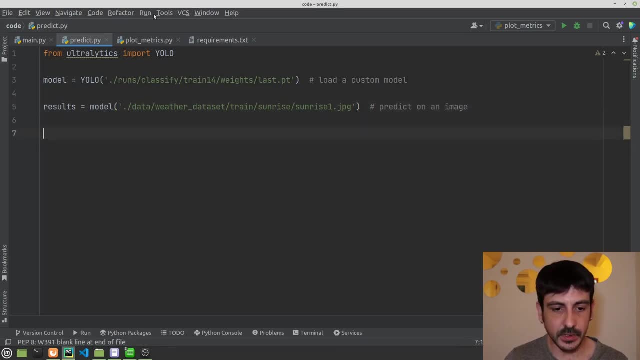 and this is pretty much all. so these are the results. the first thing i'm going to do is just trying to run this code and let's see what happens. everything should run smoothly, but this is where we're going to see. if we have any error or something like that, we may need to wait a couple. 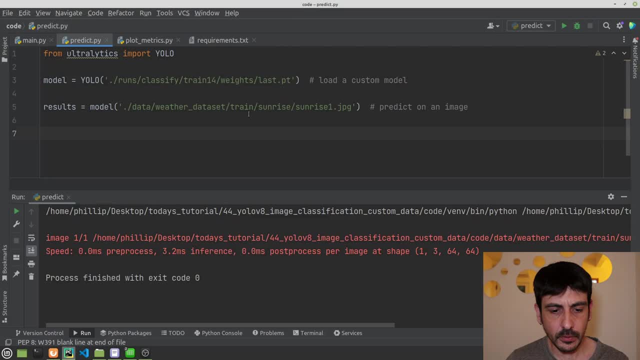 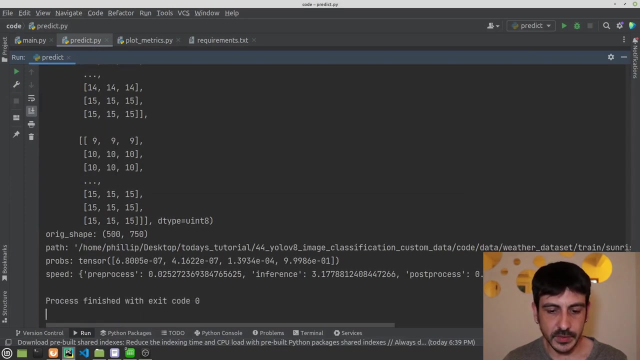 of seconds and everything seems to be working fine because we didn't get any error. so what i'm going to do now is i'm going to print results because i want to show you a couple of things. so this is the entire information we are getting when we are printing results. right, you can see that this is. 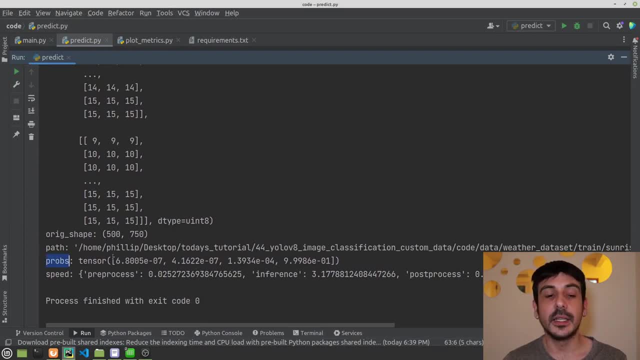 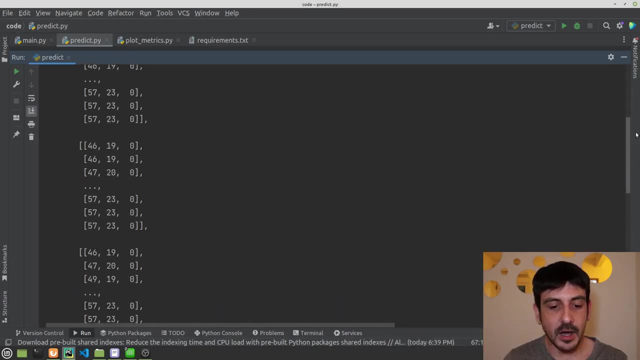 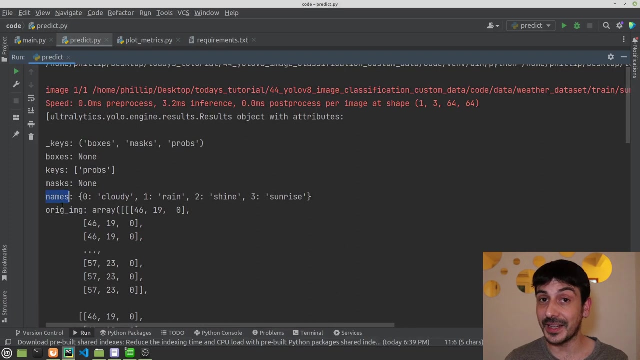 a lot of information. we have these probabilities, which is the inferences we are making. this is exactly the result of applying our image classifier, and then we have a lot of information. another object or another result which is very important is this one: which are the names of the? 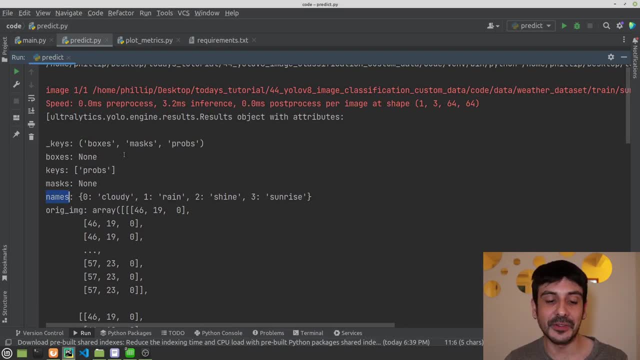 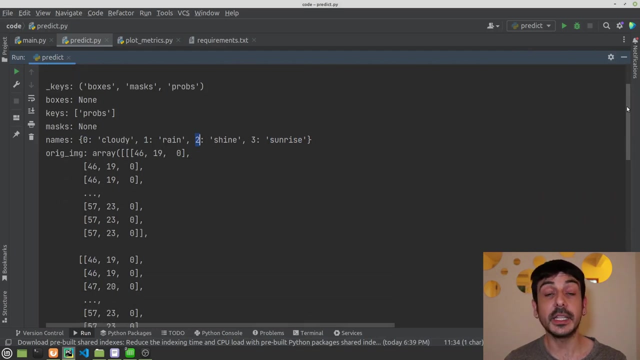 categories we have just trained, or image classifier on right you can see this is cloudy rain, shine, rise. and also you can see that we have different interval values for each one of these categories. so this is something like a dictionary, because we are going to have a result for from applying. 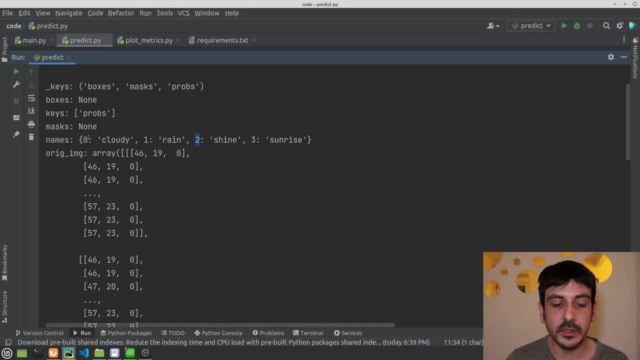 our image classifier and then, with this result, which is going to be an integer, we are going to call this dictionary, we're going to call this object, because we want to know exactly what's the name of the category we have just inferenced. right? so this is how we're going to do it. i'm going to 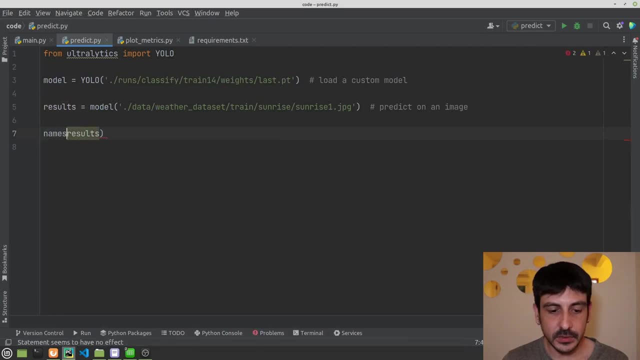 call another variable, which is is going to be names, something like names, dictionary names- ticked, and this is results- zero, because results is a list. in this case, we only want to access the first element, because we are only predicting an individual image. so this is the, the element we we want, and then we 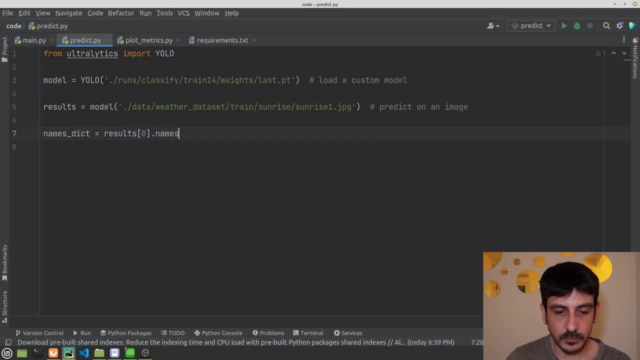 are going to call dot names, and that's pretty much all. then i'm going to define another variable, which is props, and this is results: zero dot props and this is the probability vector of all the different categories we are trying to classify, right? so we are going to have a length four. 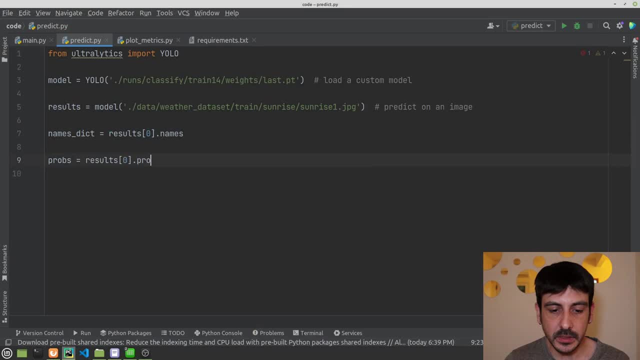 and this is the probability vector of all the different categories we are trying to classify right. so we are going to have a length four array with the probabilities of the different classes we are classifying right. so let me show you how props looks like. i'm going to print props and i'm 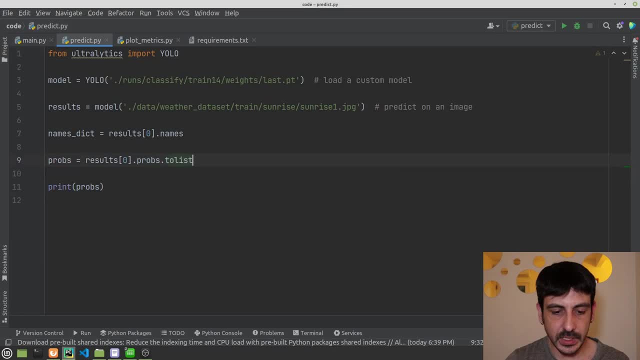 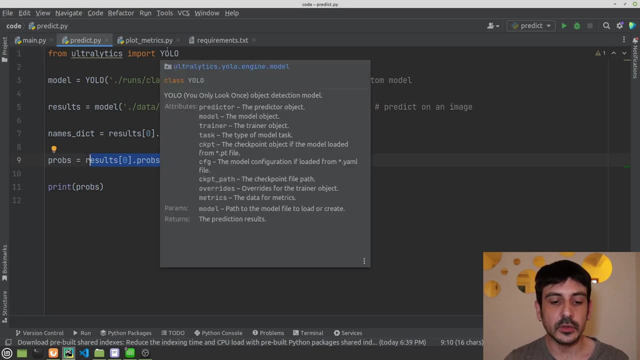 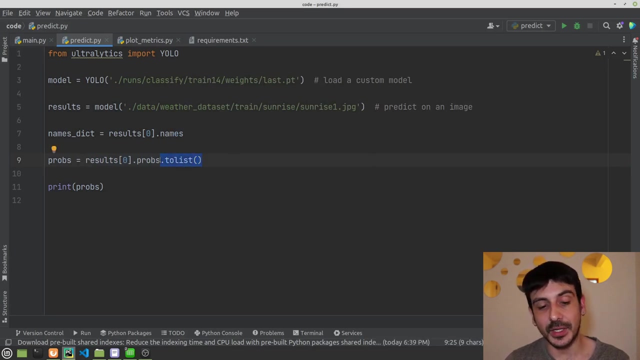 going to do something else. i'm going to say to list. so we make this object into a list, and i'm going to say to list. and i'm going to say to list. and i'm going to say to list, We are using YOLO, which is based on PyTorch. so if we don't do this, if we don't call this method, we will be working with a torch object, right with a tensor. so we don't really want to do that. so that's why I'm doing this toList. 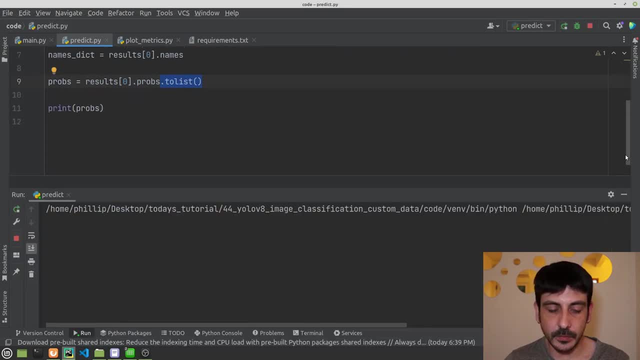 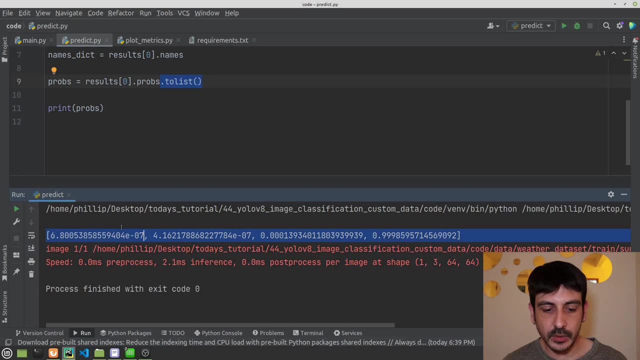 Now I'm going to print props, so I show you how it looks like and I show you how to continue from here. Okay, you can see that this is a result we got from applying, from printing props, and you can see that this is a list with four elements: one, two, three and four- and each one of these elements are the probabilities of this image to be one of these categories, right? 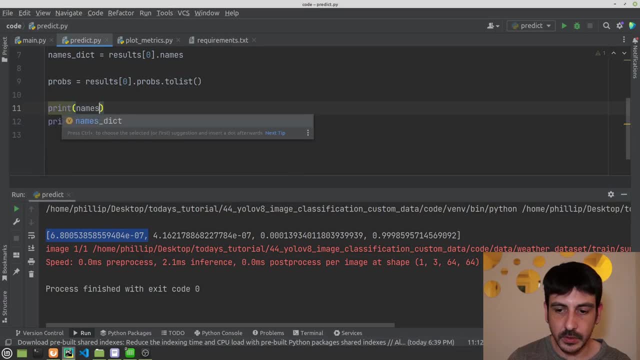 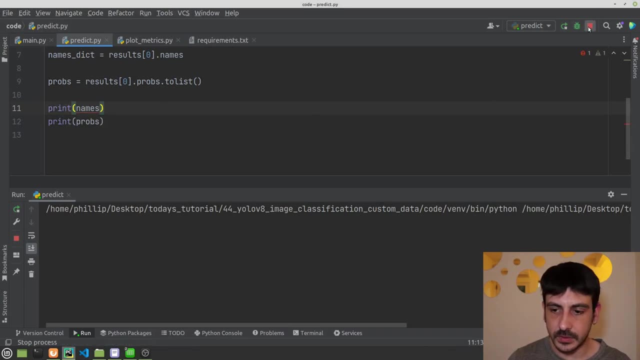 Let's print the names too, so we have all the information in our screen. I want to show you. I want to show you something, so I'm going to print- sorry, this one, This wasn't names, this was names dict. and now let's wait a couple of seconds, because I want to show you not only the probabilities but also the class names, so it's a little more clear what exactly I'm going to show you now. 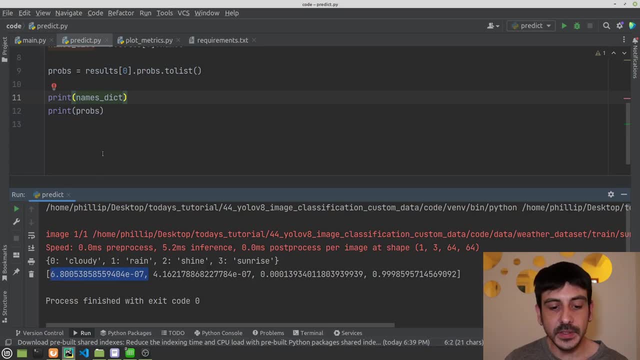 So this means that this number is the probability for this image to be cloudy, right. This other number is the probability for this image to be rain. this other number is the probability to be shine, and then this, This last number, is the probability to be sunrise, and you can see by the values that we are definitely classifying this image as sunrise, right. 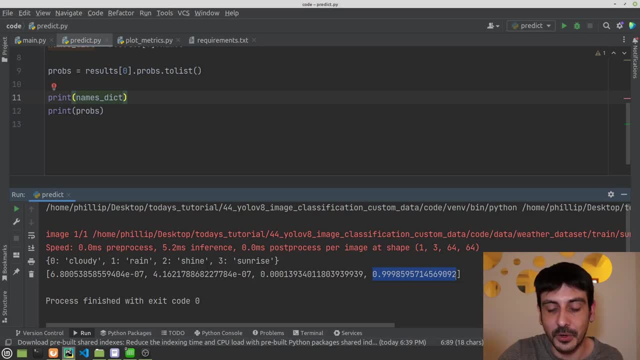 Because this is almost a one. this is almost like a super, super confident and absolutely confident classification. So this is exactly the category we are classifying for this image, and this is how to make sense of this information. So what I'm going to do now is to print names, dict, and then I'm going to call mpargument. 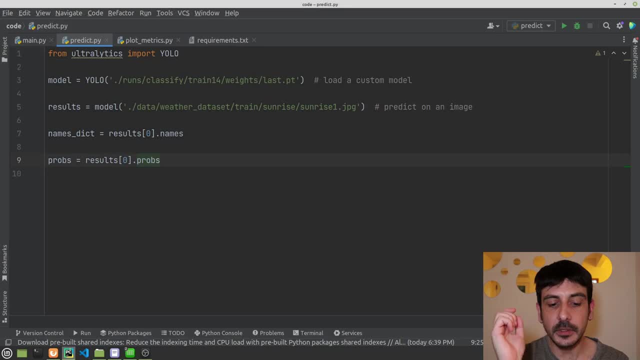 array with the probabilities of the different classes. we are classifying, right. so let me show you how props looks like. i'm going to print props and i'm going to do something else. i'm going to say to list. so we make this object into a list. we are using yolo, which is based on pytorch. 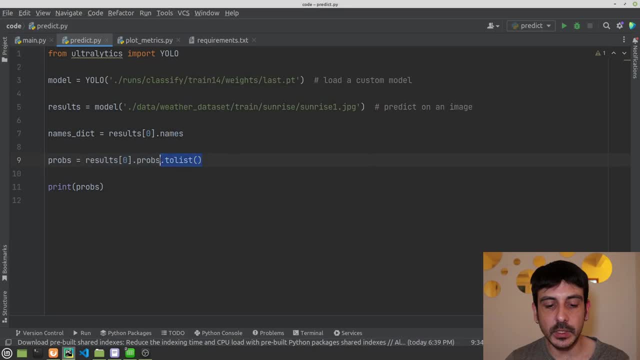 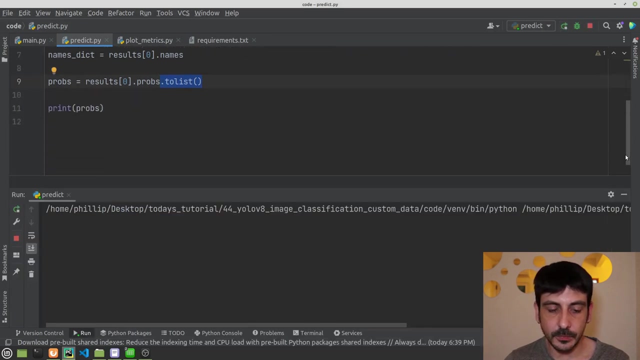 so if we don't do this, if we don't call this method, we will be working with a torch object right with a tensor. so we don't really want to do that. so that's why i'm doing this to list. now i'm going to print props, so i show you how it looks like and i'll show you. 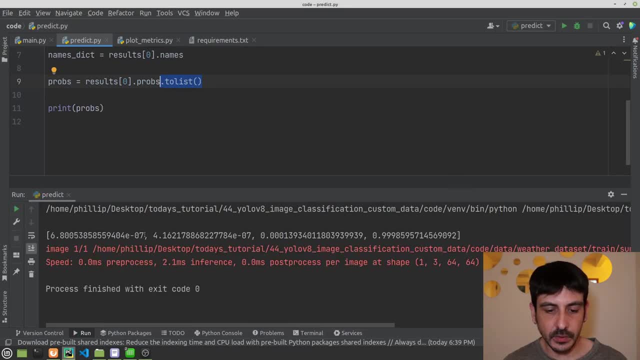 how to continue from here. okay, you can see that this is a result we got from applying, from printing props, and you can see that this is a list with four elements: one, two, three and four- and each one of these elements are the probabilities of this image to be one of these categories. right, let's print the names too, so we have all the information in. 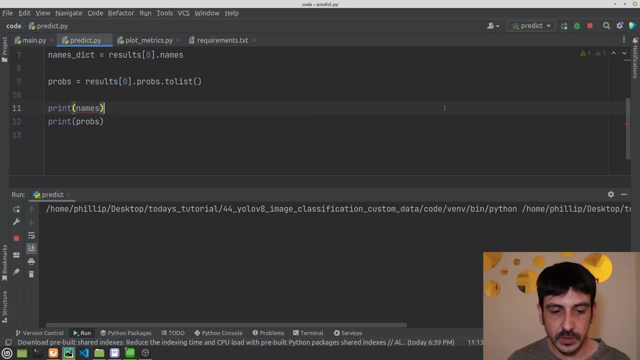 our screen. i want to show you. i want to show you something, so i'm going to print- sorry, this wasn't names, this was names dict. and now- let's wait a couple of seconds- i want to show you not only the probabilities, but also the class names, so it's a little clearer what exactly i'm going to show you now. so this means: 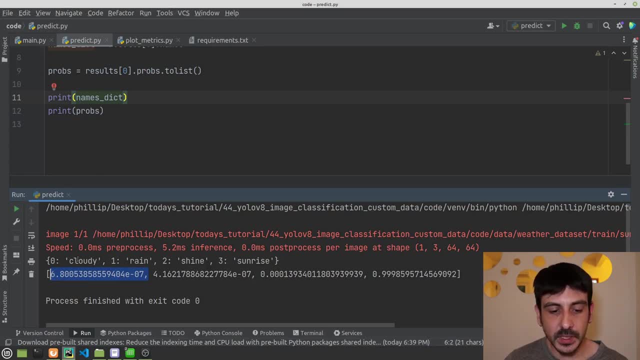 that this number is the probability for this image to be cloudy. right, this other number is the probability for this image to be rain. this other number is the probability to be shine, and then this last number is the probability be sunrise, and you can see by the values that we are definitely classifying this image as sunrise. 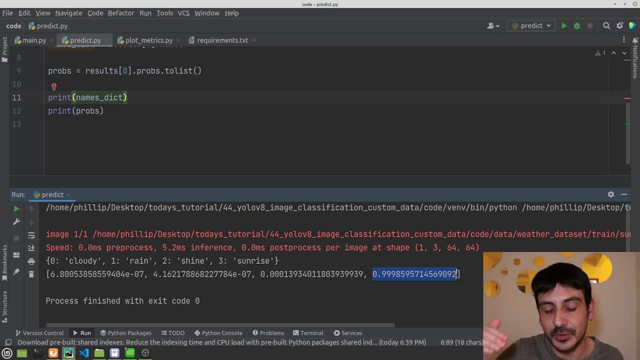 right, because this is almost a one. this is almost like a super, super confident and absolutely confident classification. so this is exactly the category we are classifying for this image, and this is how to make sense of this information. so what i'm going to do now is to print. 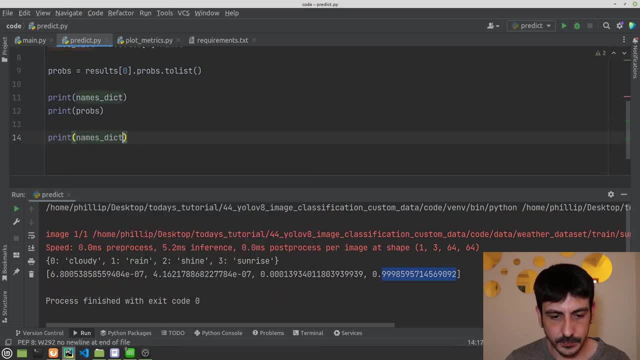 names, dict, and then i'm going to call np, dot, argument argmax, and then i'm going to input the probability list i shall show you, and obviously i need to import numpy as mp, otherwise it's not going to work and basically what we are doing here is that. 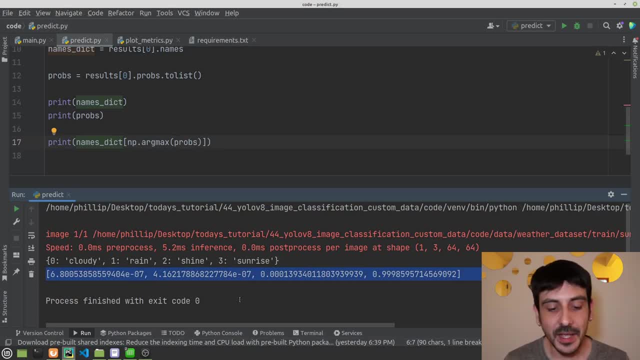 we are looking at this list, the one containing all of our probabilities is we are taking a look at the maximum number, which in this case is this one, and we are taking the index of this maximum number. so, in this case, this is the first element. so this is the index: 0. 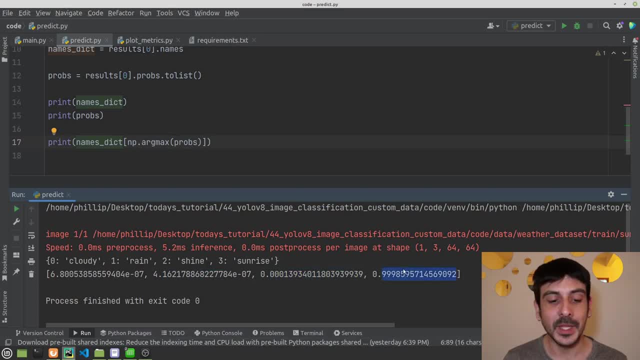 this is 1, this is 2 and this is 3. right, so from this um, from calling np dot argmax props, we are getting 3, and then we are calling the third element of the name: stitch object. so we go here and we see that three. 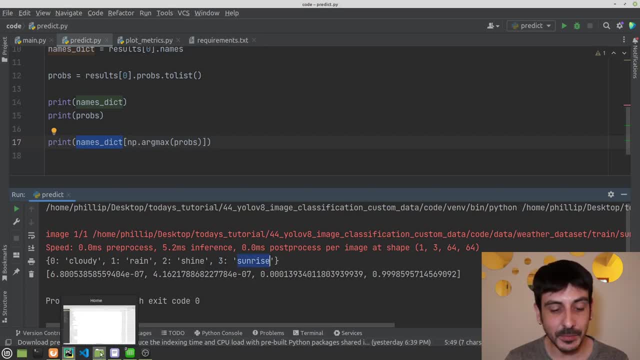 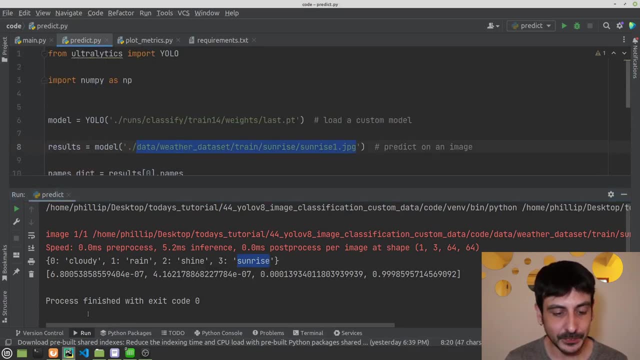 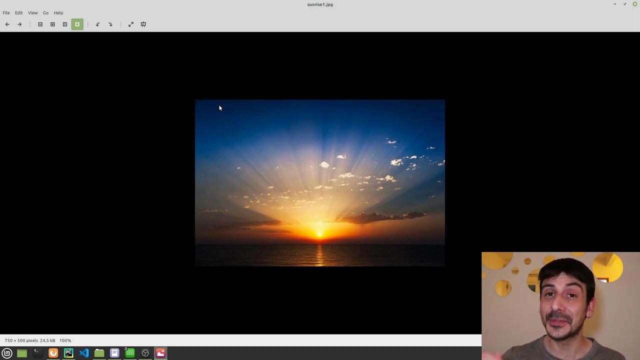 belongs to the sunrise category, and if we look at this image again, we are going to see we are in fact uploading a sunrise. let me show you. so everything seems to be working fine, and this is going to be all for today. this is exactly how you can train an image classifier using yellow. 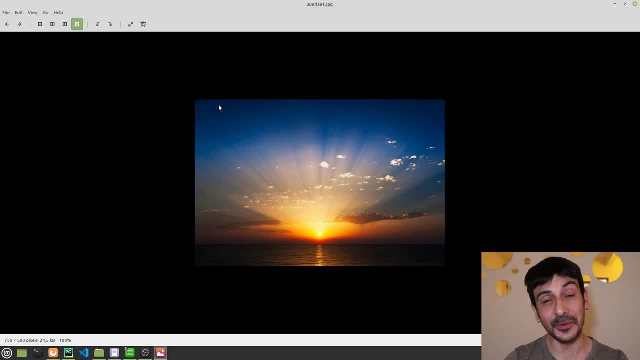 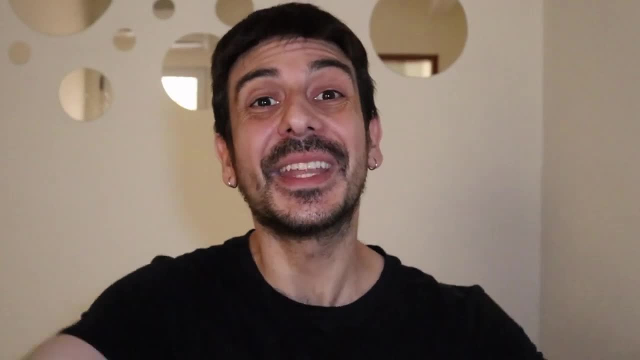 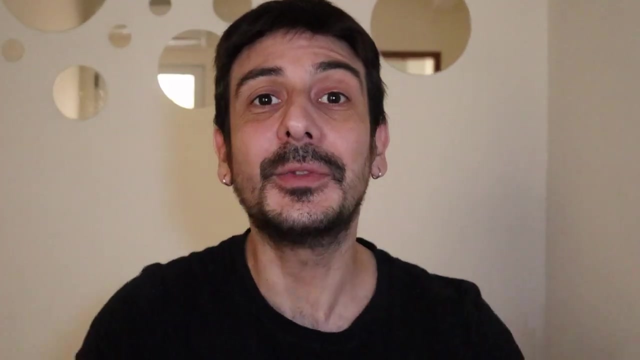 v8 in your own custom data. and this is going to be all for this tutorial. so in my previous videos i show you how to train an image classifier and an object detector using jello v8. now it's the time for semantic segmentation. i'm going to show you the entire process of how to train a semantic segmentation. 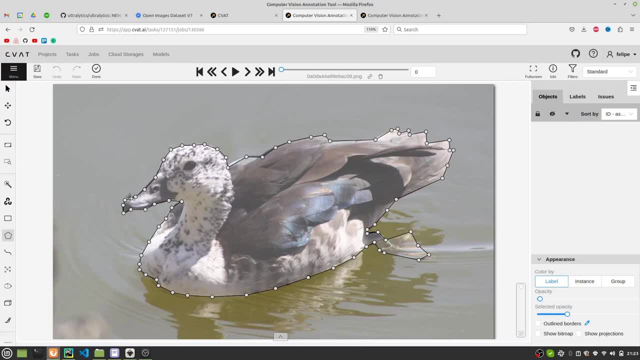 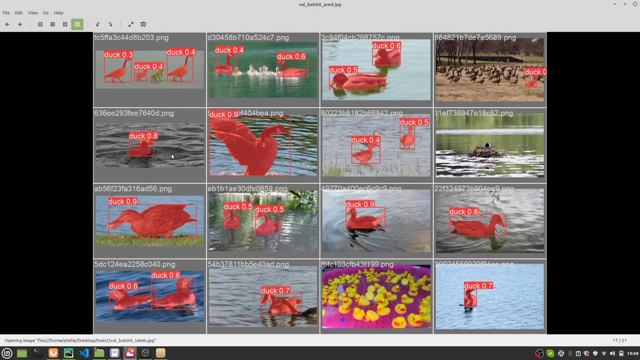 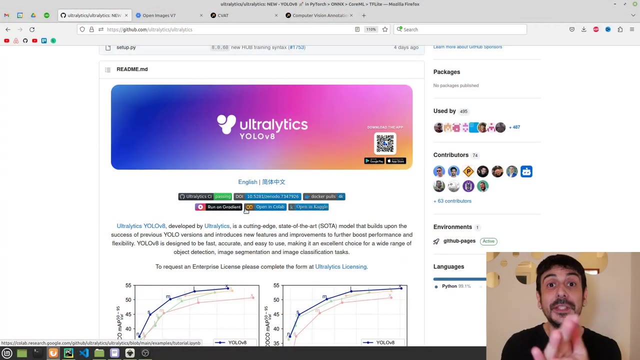 finding uses in yellow v8, from how to annotate the data, how to train the model in your local environment, and also from a google collapse, and finally, a super, super, super comprehensive guide on how to validate the model you trained. my name is felipe, welcome to my channel and now let's get started. so let's start with this tutorial, and everything i'm going to do is i'm going to apply. some data to this망 from jello v8 and i'm going to Verse into thecolab folder. and now let's get started. so let's start with this tutorial and everything i'm going to do is i'm going to preselect some data and you 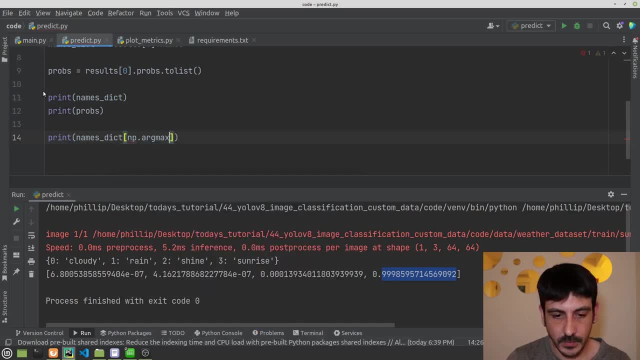 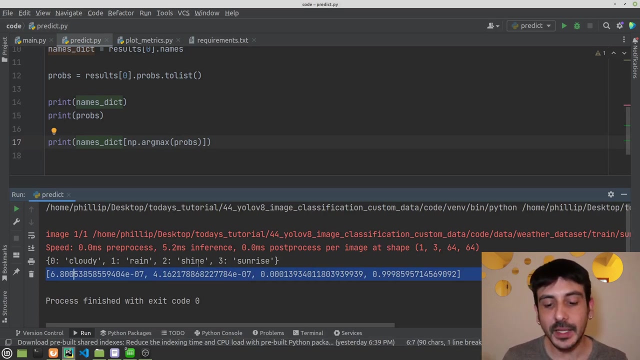 So I'm going to call mpargumentargmax and then I'm going to input the probability list I just showed you, and obviously I need to import nump as mp, otherwise it's not going to work. And basically what we are doing here is that we are looking at this list, the one containing all of our probabilities, we are taking a look at the maximum number, which in this case, is this one. 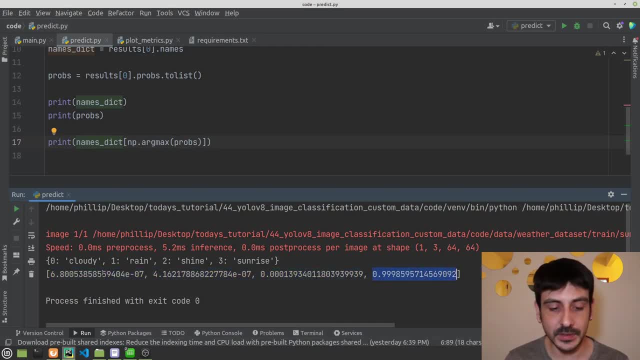 and we are taking the index of this maximum number. so in this case, this is the first element. so this is the index: 0, this is 1,, this is 2, and this is 3, right, So from this, from calling mpargmax props, we are getting 3, and then we are calling the third element of the names, dict object. so we go here and we see that 3 belongs to the sunrise category. 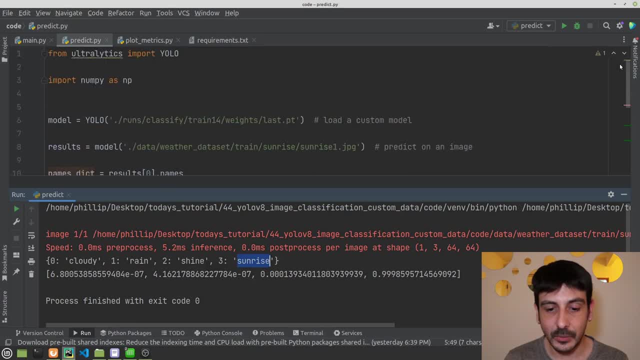 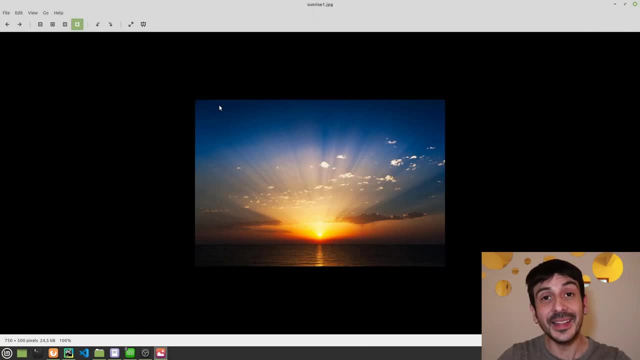 And if we look at this image again, we are going to, As you can see, we are in fact plotting a sunrise. Let me show you. So everything seems to be working fine, and this is going to be all for today. 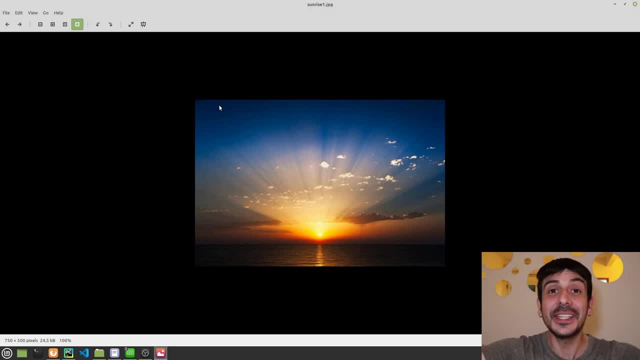 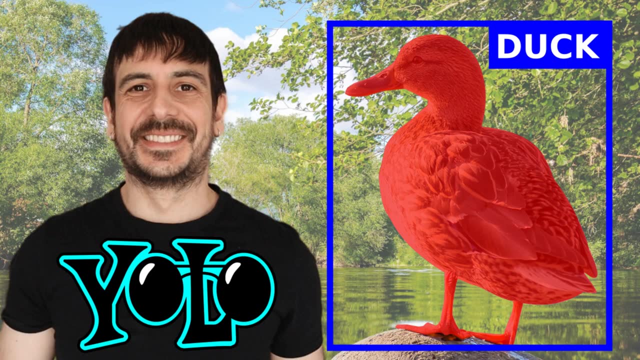 This is exactly how you can train an image classifier using YOLOv8 in your own custom data. and this is going to be all for this tutorial. So in my previous videos, I showed you how to train an image classifier and an object detector using YOLOv8. 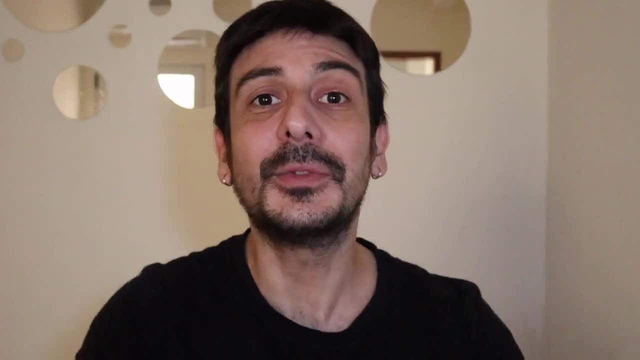 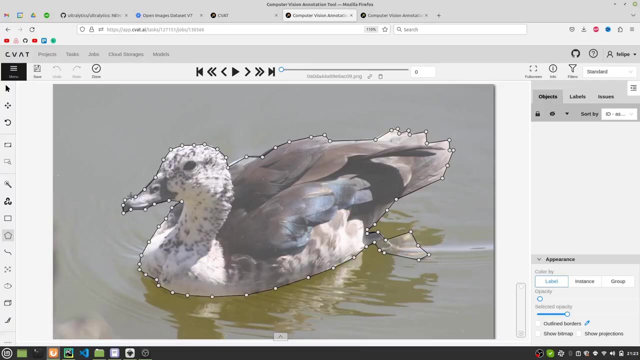 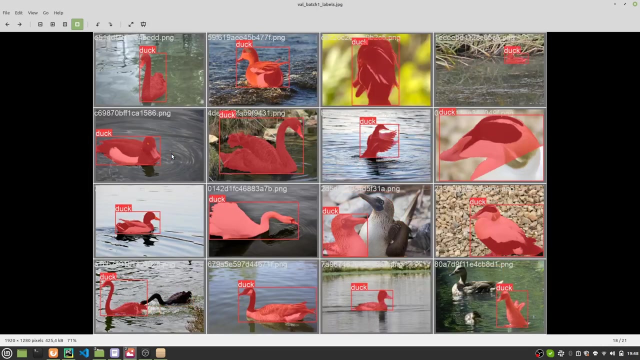 Now is the time for semantic segmentation. I'm going to show you the entire process of how to train a semantic segmentation algorithm using YOLOv8, from how to annotate the data, how to train the model in your local environment, and also from a Google Collab. and finally, a super, super, super comprehensive guide on how to validate the model you trained. 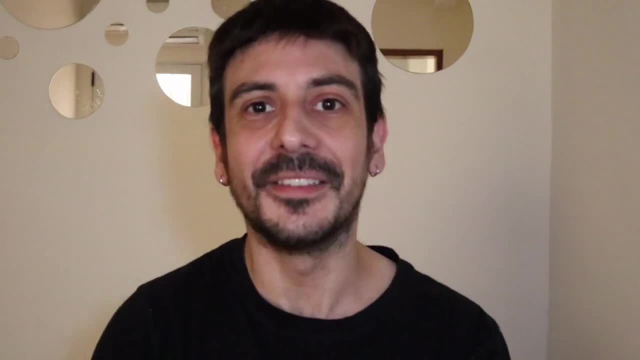 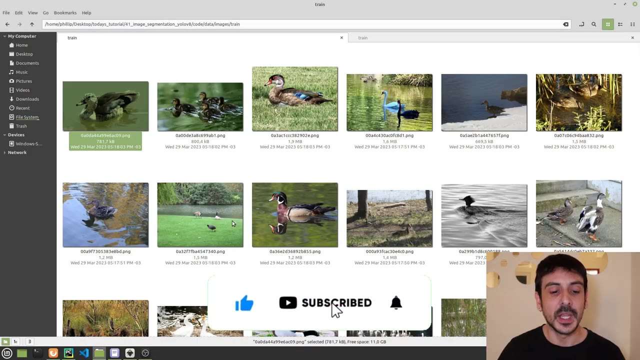 My name is Felipe. welcome to my channel, and now let's get started. So let's start with today's tutorial, and the first thing I'm going to do is to show you the data we are going to be using today. 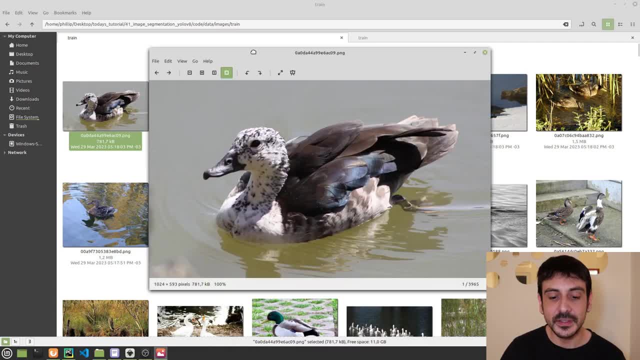 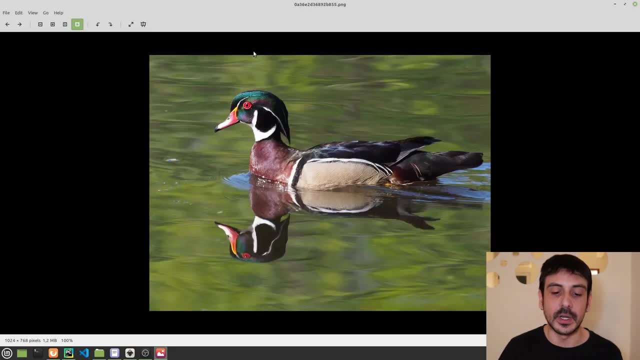 So this is the asset I have prepared for today. So let's go to today's tutorial and you can see that these are images of DAGs. We are going to be using a DAG dataset today, and this is exactly how the images look like. 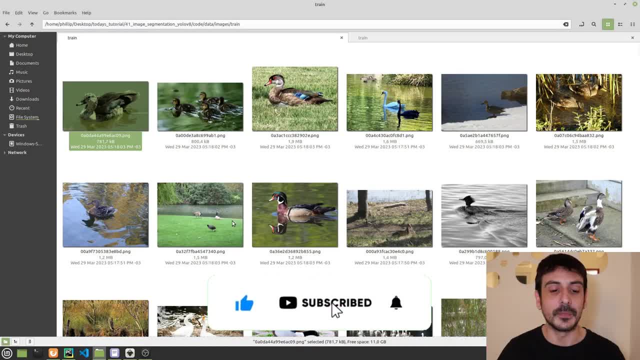 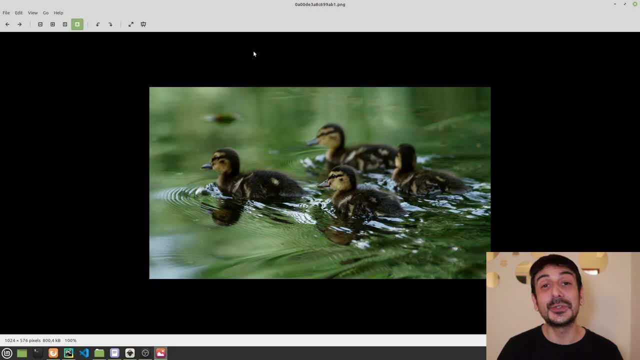 thing i'm going to do is to show you the data we are going to be using today. so this is the asset i have prepared for today's tutorial, and you can see that these are images of ducks. we are going to be using a duck data set today, and this is exactly how the images look like now for each. 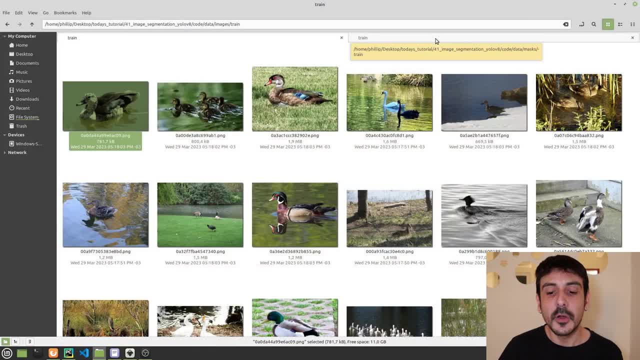 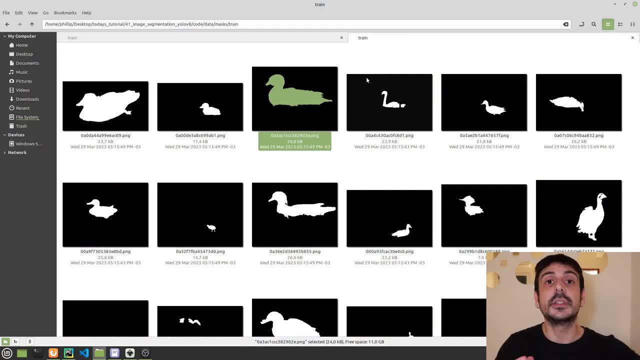 one of our images, for absolutely every single one of our images. we are going to have a binary mask. we are going to have an image, a binary image, where absolutely every single pixel is either white or black, and absolutely every single white pixel. it's the location of our objects. all the white. 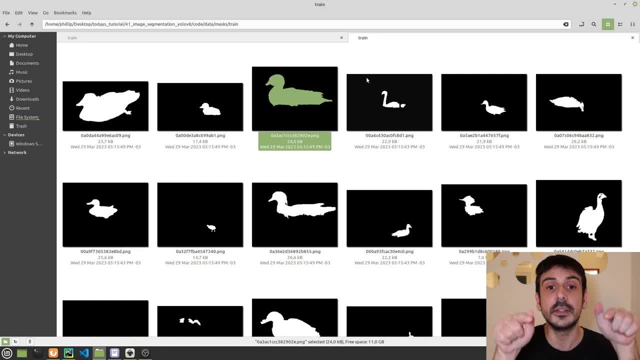 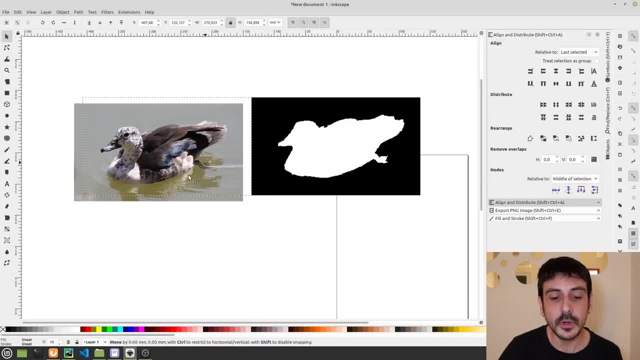 pixels are the location of the objects we are interested in. in this case, the objects are our ducks. so let me show you an example so it's a little more clear what i mean regarding the white pixels are the location of our objects. so these are random image in my data set. this is a random. 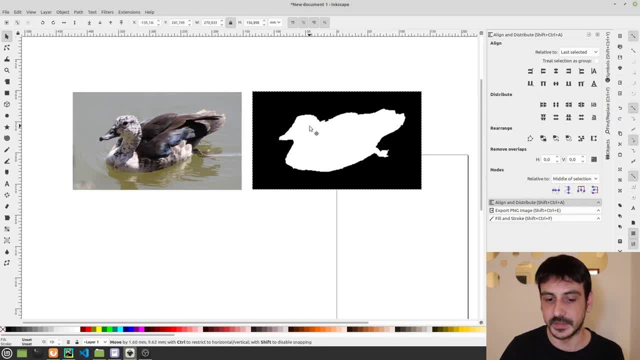 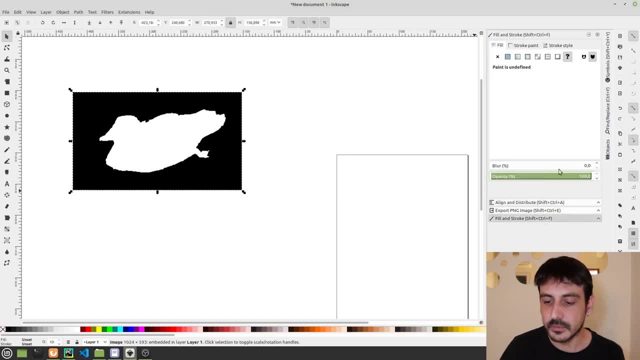 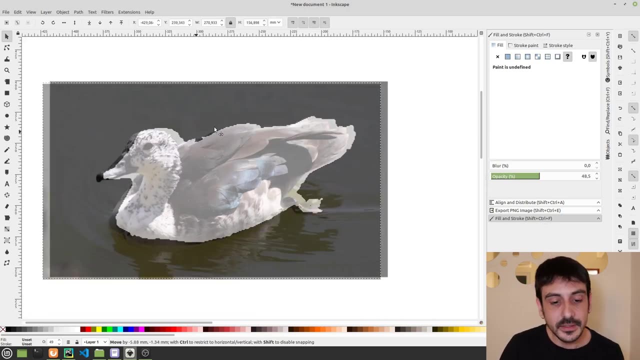 image of a duck and this is exactly its binary mask. so take a look what happens when i align these two images and when i apply something like a transparency, you can see that the binary mask is giving us the exact location of the duck in this image. so this is exactly what it means, that 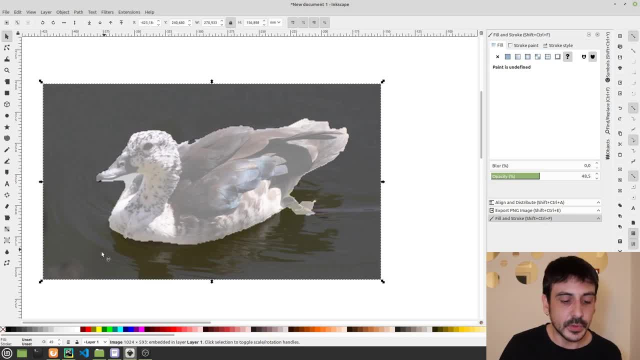 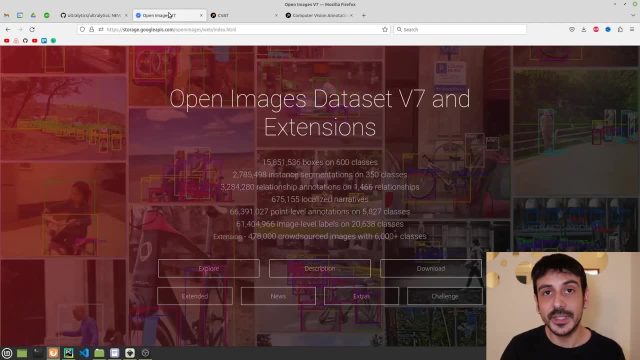 the white pixels are the location of our objects. so this is exactly the data i am going to be using in this tutorial. and now let me show you from where i have downloaded this dataset. this asset, i have found in the open images dataset, version 6.. 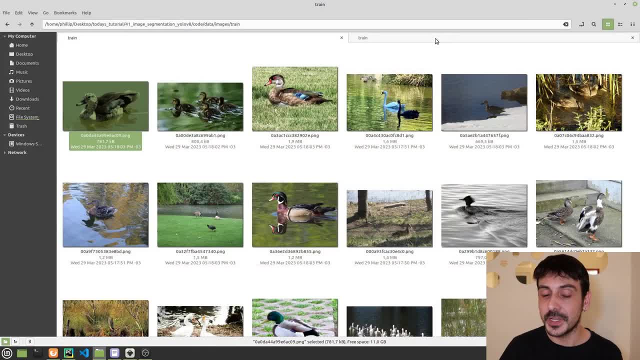 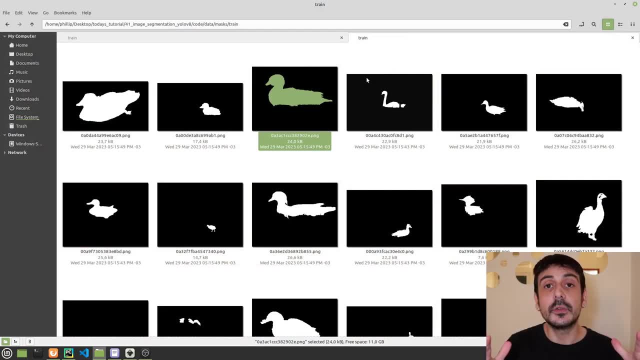 Now, for each one of our images, for absolutely every single one of our images, we are going to have a binary mask. We are going to have an image, a binary image, where absolutely every single pixel is either white or black And absolutely every single white pixel is the location of our objects. 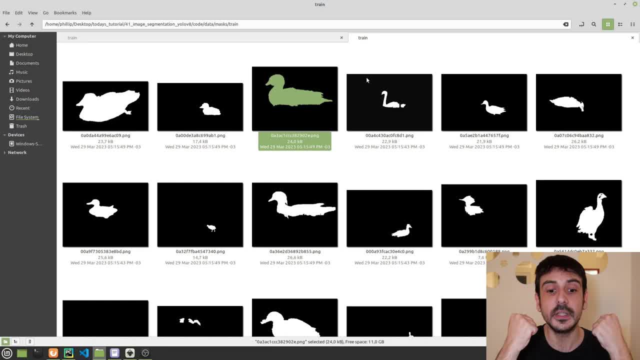 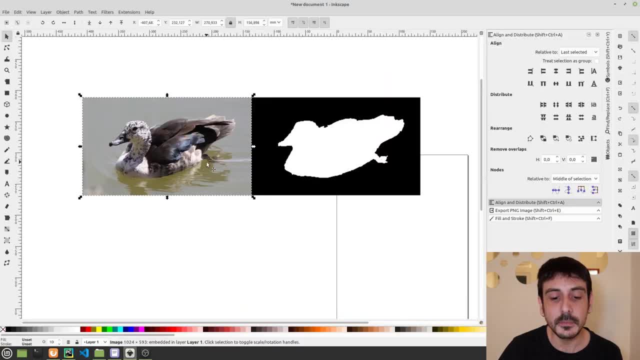 All the white pixels are the location of the objects We are interested in. in this case, the objects are our DAGs. So let me show you an example so it's a little more clear what I mean. regarding the white pixels are the location of our objects. 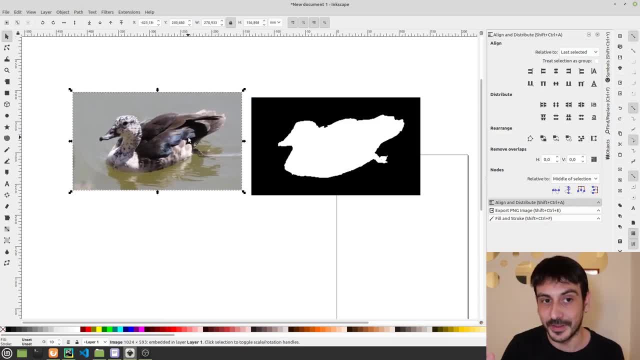 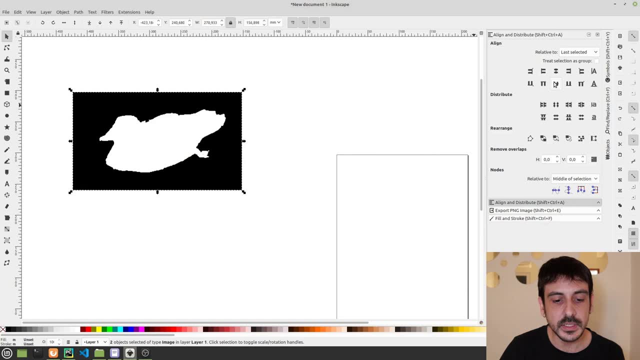 So this is a random image in my dataset. This is a random image of a DAG and this is exactly its binary mask. So take a look what happens when I align these two images and when I apply something like a transparency. 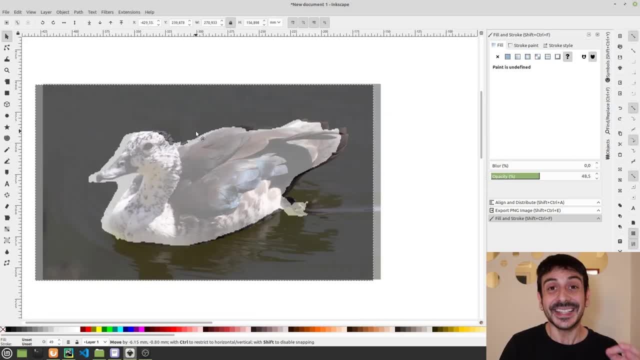 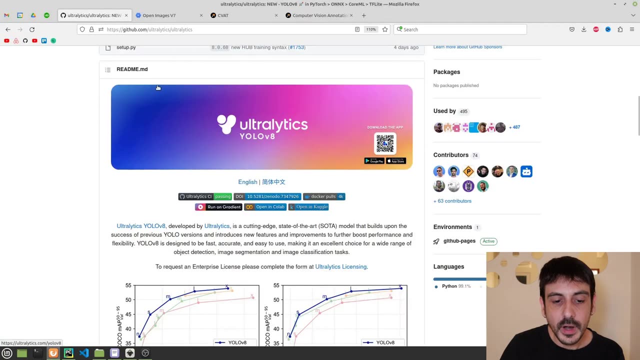 you can see that the binary mask is giving us a binary image. It's giving us the exact location of the DAG in this image. So this is exactly what it means: that the white pixels are the location of our objects. So this is exactly the data I am going to be using in this tutorial, and now let me show you from where I have downloaded this dataset. 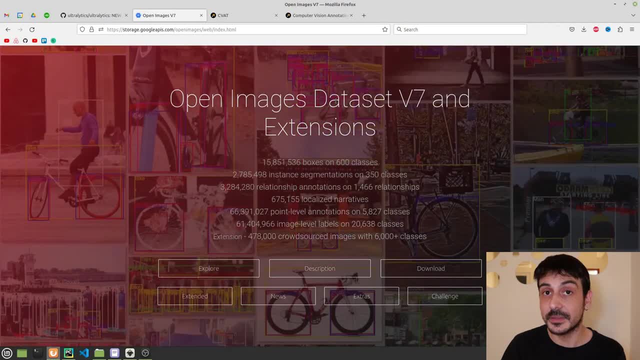 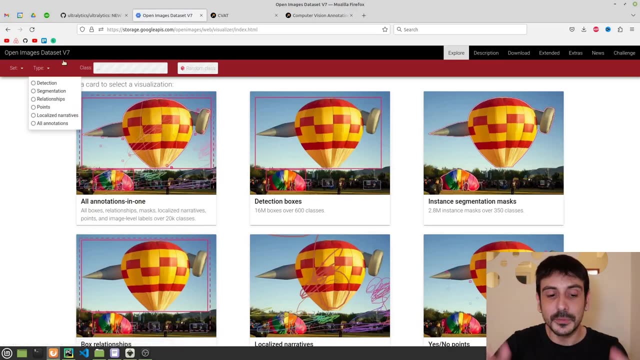 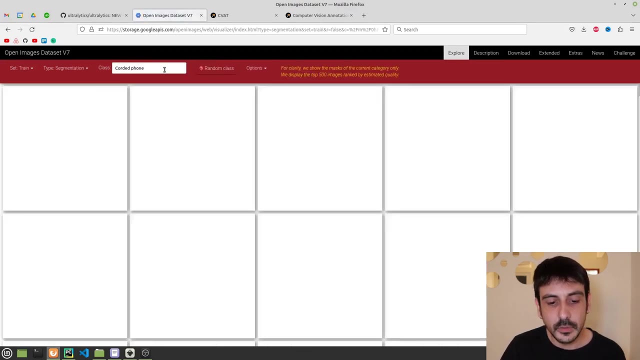 This dataset I have found in the OpenImages dataset version 7.. Let me show you this dataset super, super quickly. This is an amazing dataset you can use for many different computer vision related tasks. For example, if I go to segmentation, you can see that we have many, many, many different categories. 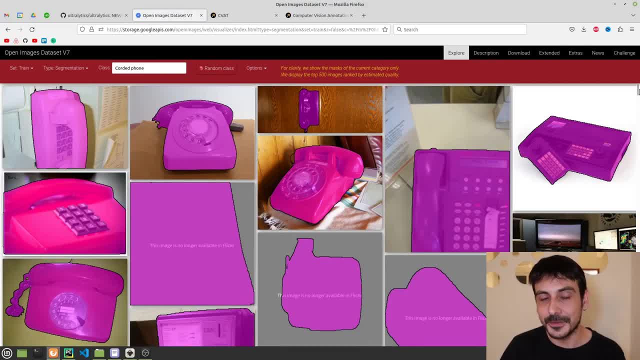 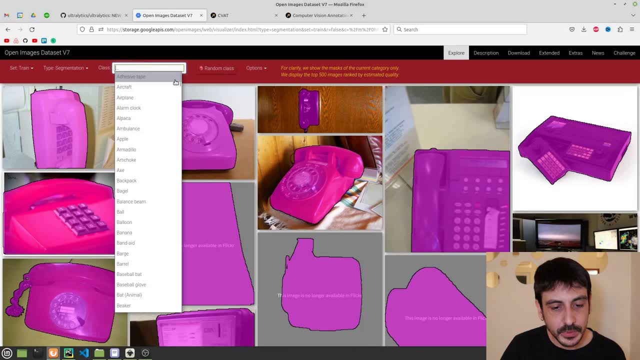 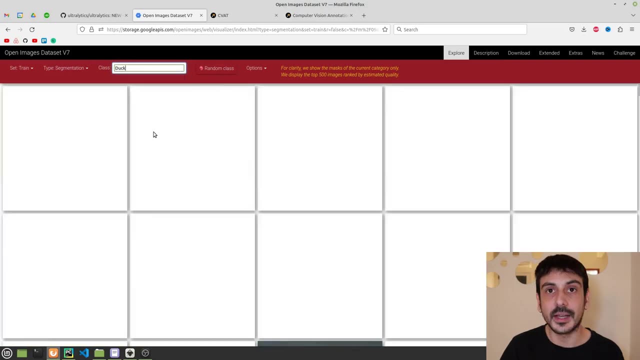 Now we are looking at a random category of fonts. This is, for example, a semantic segmentation dataset of fonts And let me show you. if I go here and I scroll down, you can see that one of the categories is here: DAG. 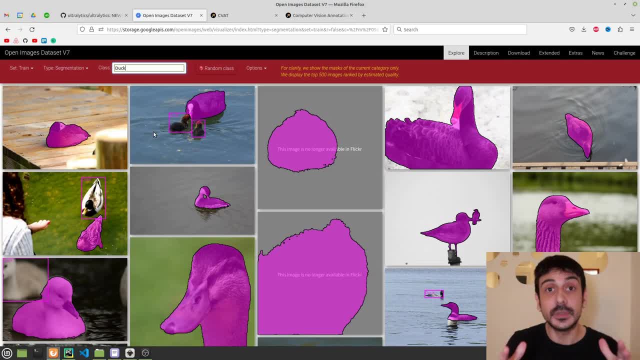 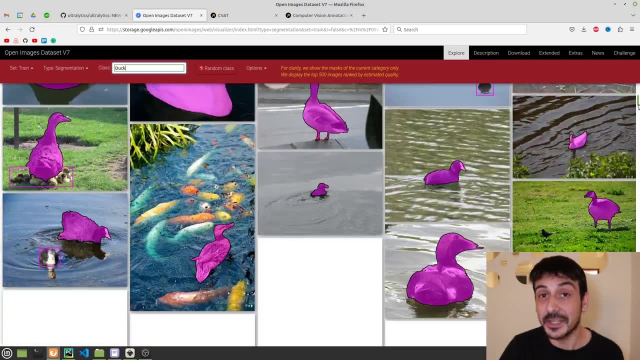 So this is, for example, the exact same data I am going to be using in this tutorial. This is the exact same DAG. This is the exact same DAG data set I am going to be using in order to train a semantic segmentation algorithm using YOLOv8.. 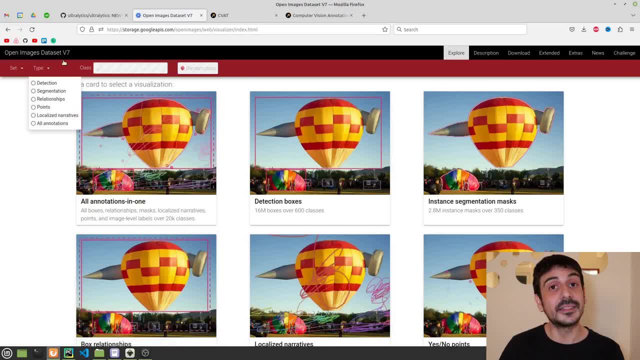 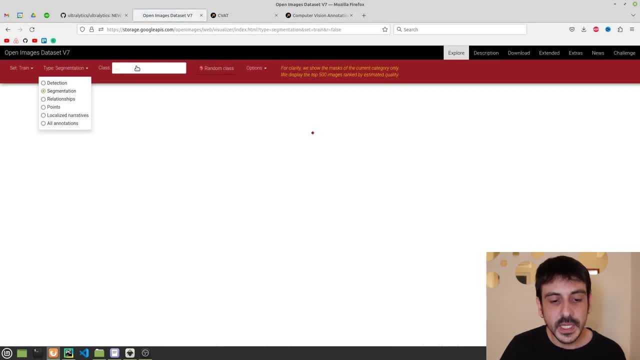 let me show you this data set super, super quickly. this is an amazing data set. you can use for many different computer vision related tasks. for example, if i go to segmentation, you can see that we have many, many, many different categories. now we are looking at a random. 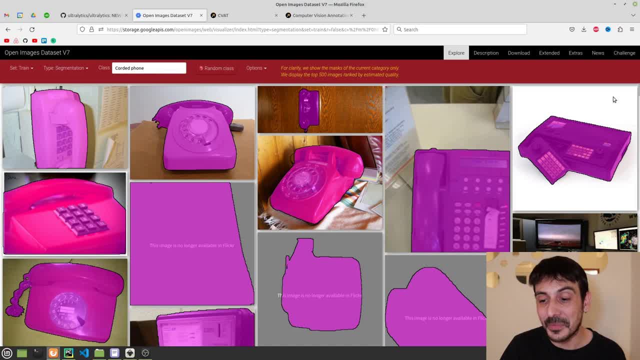 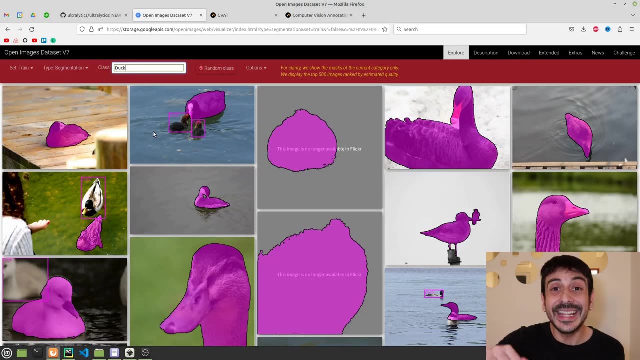 category of phones. this is, for example, a semantic segmentation data set of phones. and let me show you. if i go here and i scroll down, you can see that one of the categories is here duck. so this, for example, the exact same data i am going to be using in this tutorial. this is: 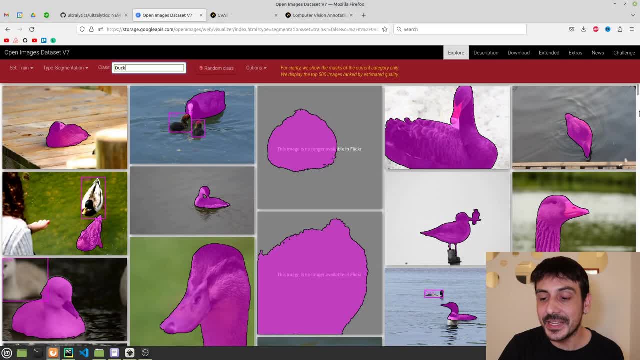 the exact same duck data set i am going to be using in order to train a semantic segmentation algorithm using your lobby 8 and obviously you could download the exact same data i am going to use in this tutorial if you go to open images. that is the version 7. you can just download the. 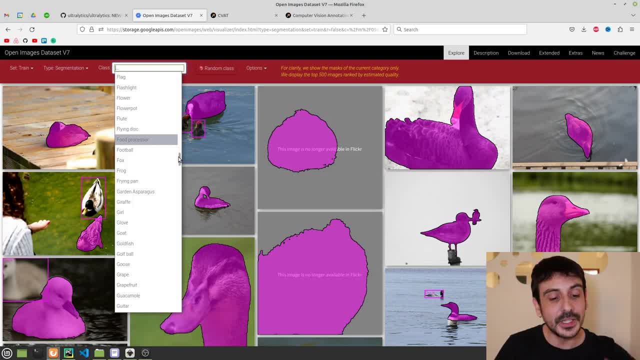 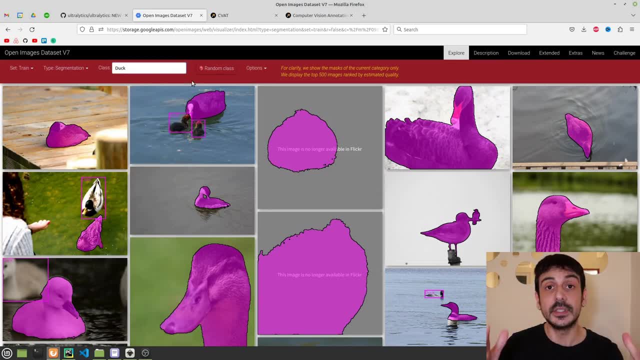 exact same duck that i said i am going to be using today, or you can also download another data set of other categories. so this about the data i am going to use in this project and this about where you can download the exact same data. if you want to, now let me show you a website you can use in order. 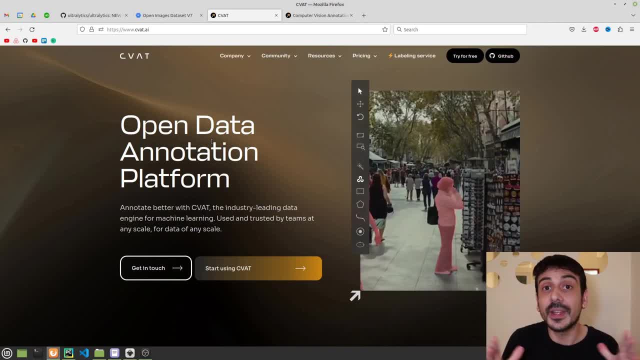 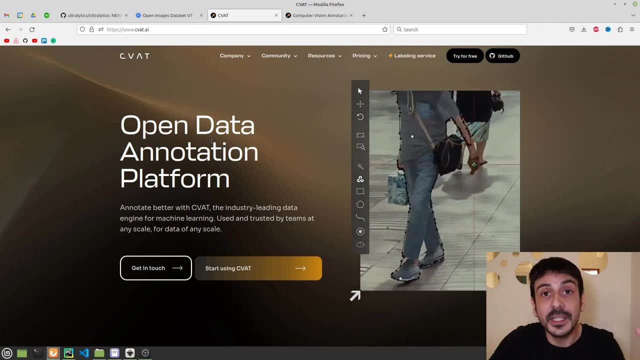 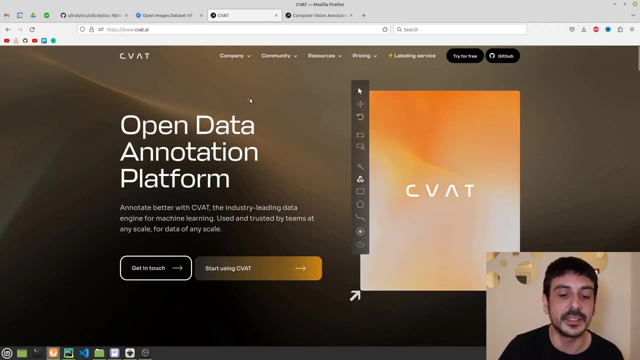 to annotate your data because in my case i have downloaded other set which is already annotated, so i don't have to annotate absolutely any of my images. absolutely all of my images already have its binary masks, right, i already have the masks for absolutely all the images in my data. 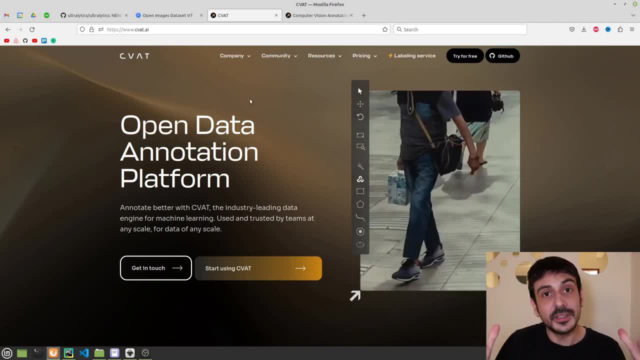 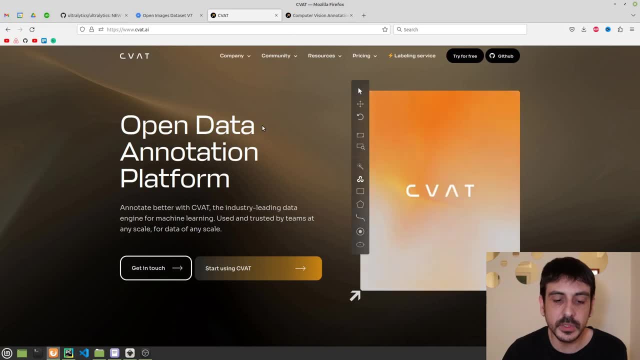 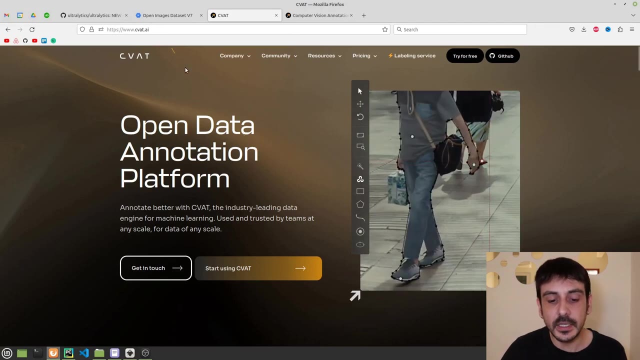 set, but if you're building your data set from scratch, chances are you will need to annotate your images. so let me give you this tool which is going to give you, which is going to be super, super useful in case you need to annotate your data. it's called cbat and you can find it in cbatai. 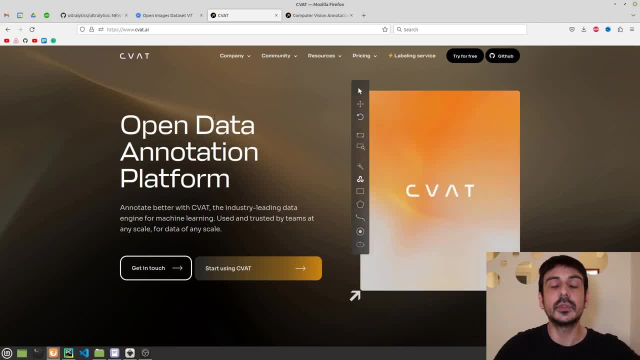 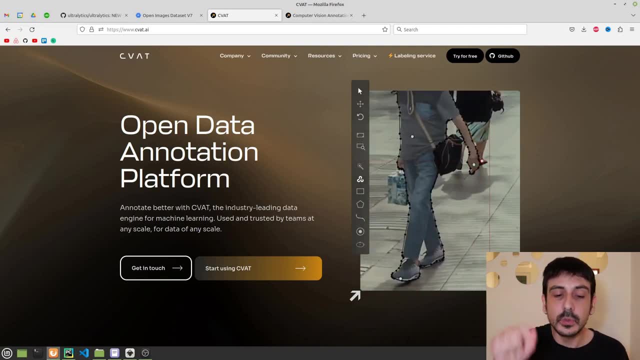 and this is a very, very popular computer vision annotation tool. i have used it- i don't know how many times in my projects and it's very, very popular and it's very useful. so i'm going to show you how to use this tool in order to annotate your images. so the first thing we need to do is to 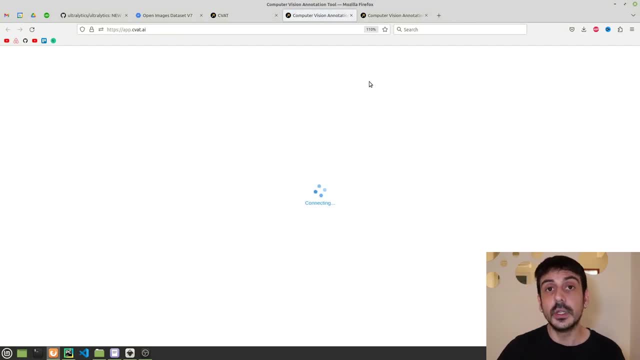 go to start using cbat. this is going to ask you to either register, if you don't have a user already, or to log in. right, i already have a user, so this is logged into my account, and now let me show you how i'm going to do in order to annotate a few images. actually, i'm going to annotate only one. 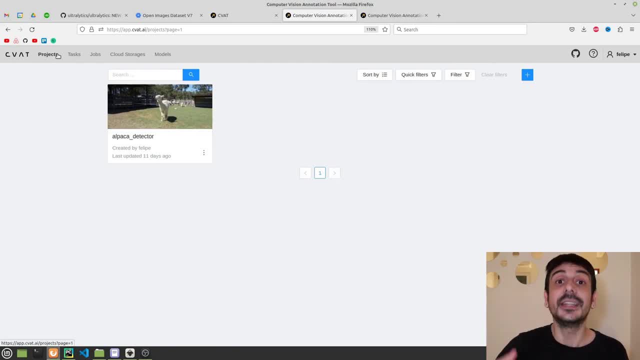 image because i am only going to show you how to use it in order to create a binary mask for your project. but i'm just going to do it with only one image because it's: yeah, you only need to see the process and that's going to be all. so i'm going to projects, i'm going to here to the plus. 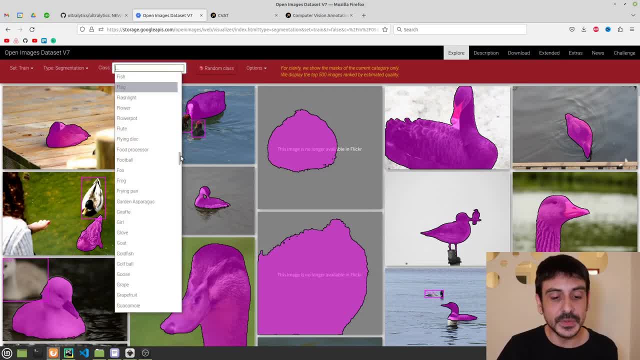 And obviously you could download the exact same data I am going to use in this tutorial. If you go to OpenImages dataset version 7, you can just download the exact same DAG dataset I am going to be using today, Or you can also download another dataset of other categories. 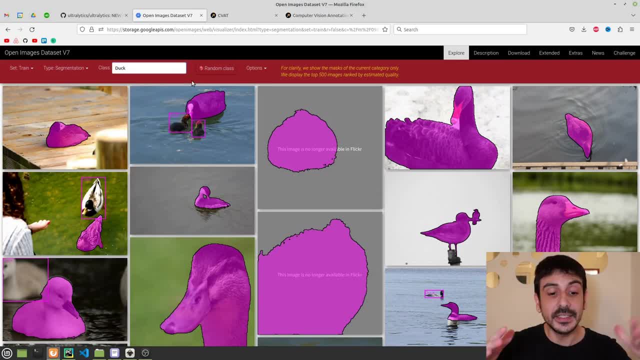 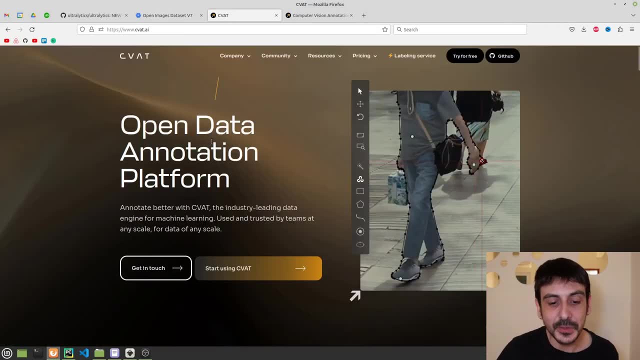 So this is about the data I am going to use in this project, And this is about where you can download the exact same data want to. now let me show you a website you can use in order to annotate your data, because, in my case, 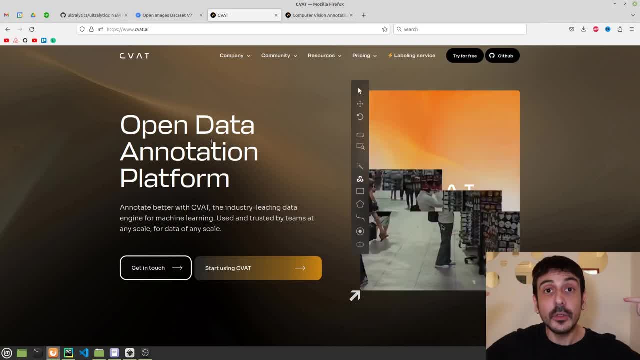 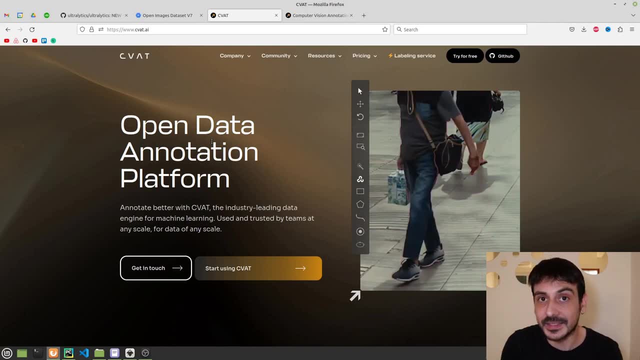 i have downloaded a data set which is already annotated, so i don't have to annotate absolutely any of my images. absolutely all of my images already have its binary masks. right, i already have the masks for absolutely all the images in my data set. but if you're building your data set, 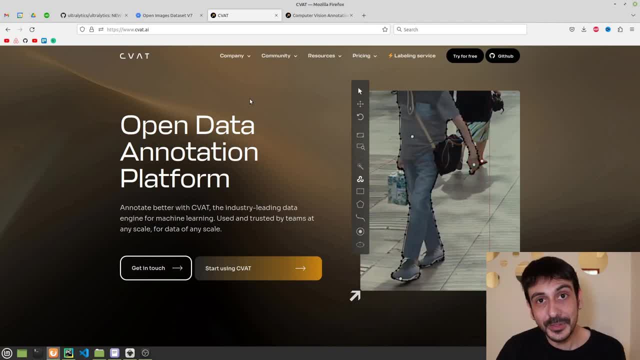 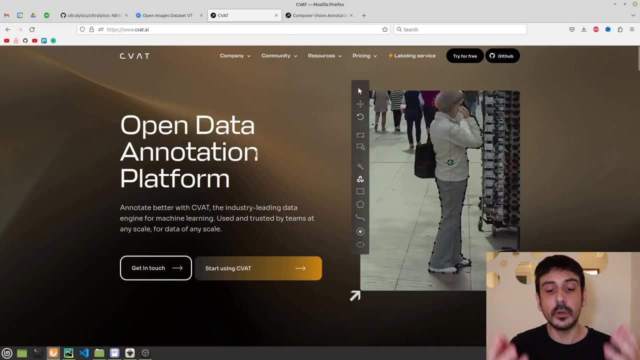 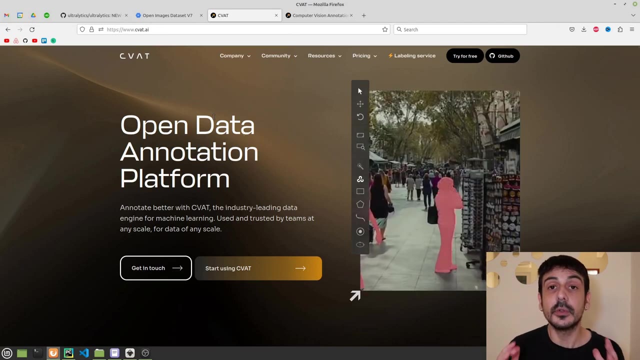 from scratch. chances are you will need to annotate your images. so let me give you this tool which is going to give you, which is going to be super, super useful in case you need to annotate your data. it's called cbat and you can find it in cbatai, and this is a very, very popular computer vision. 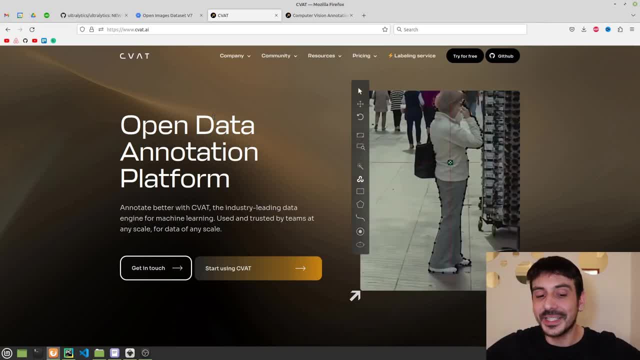 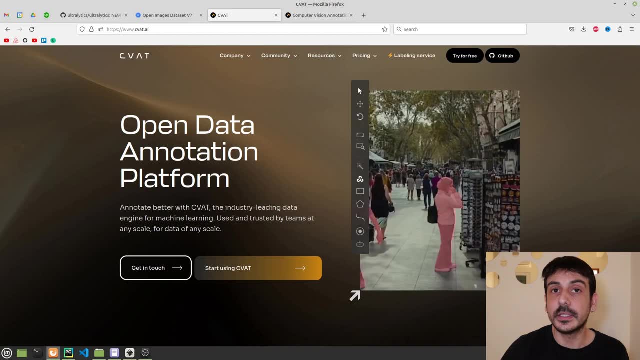 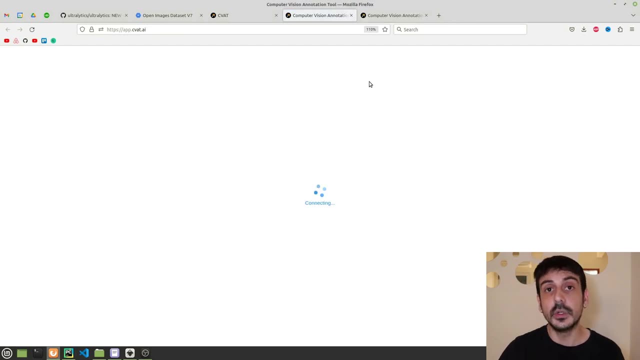 annotation tool. i have used it- i don't know how many times in my projects and it's very, very popular and it's very useful. so i'm going to show you how to use this tool in order to annotate your images. so the first thing we need to do is to go to start using cbat. this is going to ask you to either. 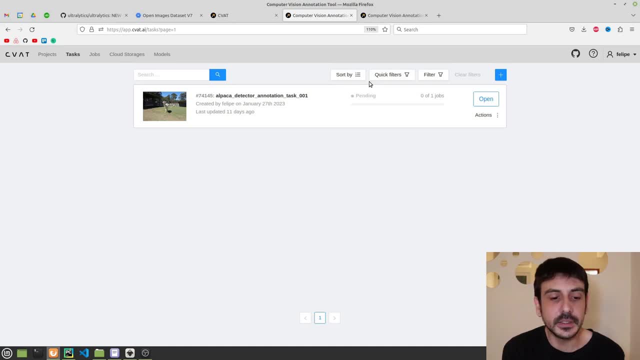 register if you don't have a user already, or to log in. right, i already have an user, so this is logged into my account. and now let me show you how i'm going to do in order to annotate a few images. actually, i'm going to annotate only one image, because i am only going to show you how to use. 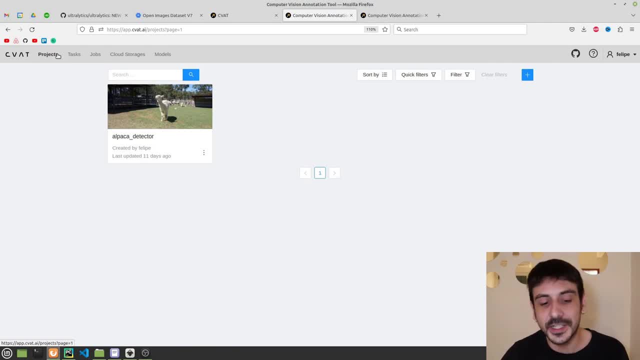 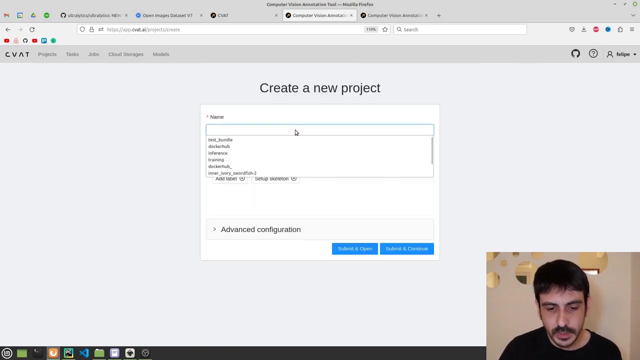 it in order to create a binary mask for your project. but i'm just going to do it with only one. yeah, you only need to see the process and that's going to be all. so i'm going to projects. i'm going to here, to the plus button: create a new project. the name of this project will be duck. 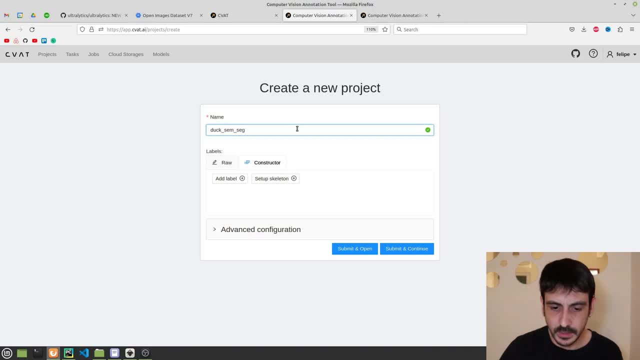 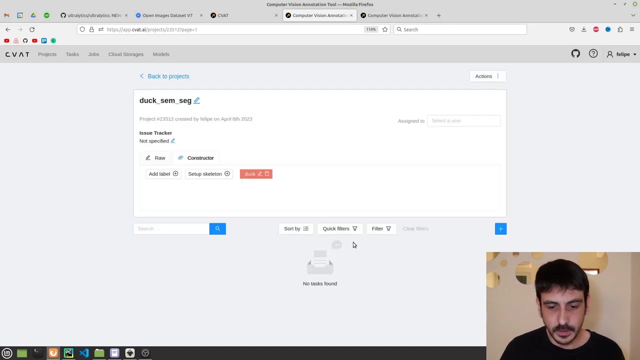 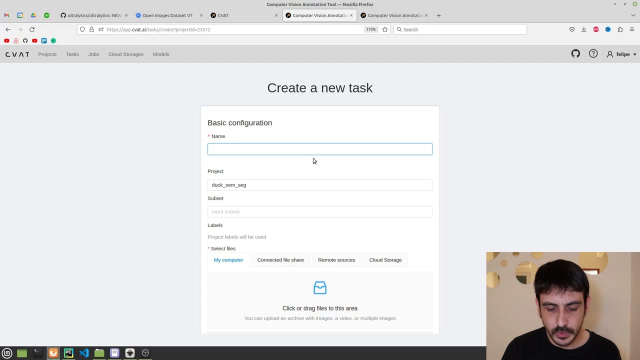 semantic seven sec. this will be the name of my project and it will contain only one label, which is that. so i'm going to press continue and that's pretty much all. submit and open. now i'm going to create a task. this is already. yeah, create new task. the task name will be duck. 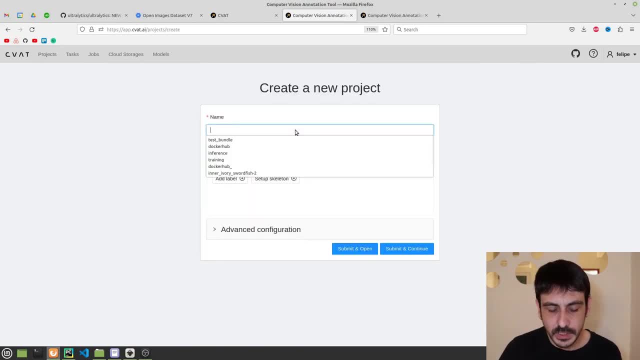 button create a new project. the name of this project will be duck semantic 7 sec. this will be the name of my project and it will contain only one label, which is tag. so i'm going to press continue and that's pretty much all. submit and open. 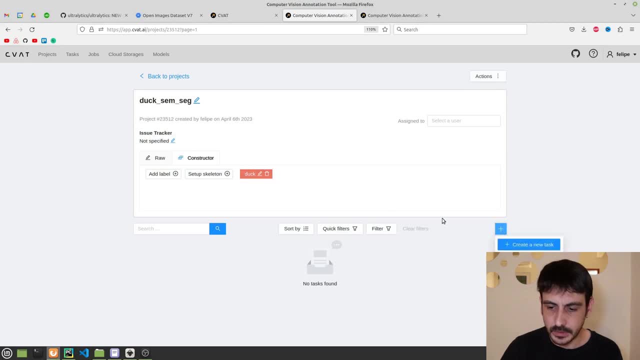 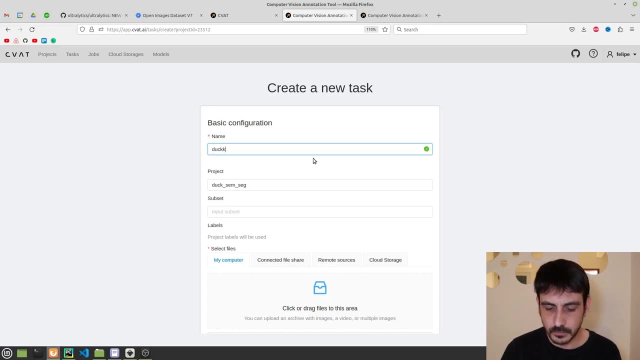 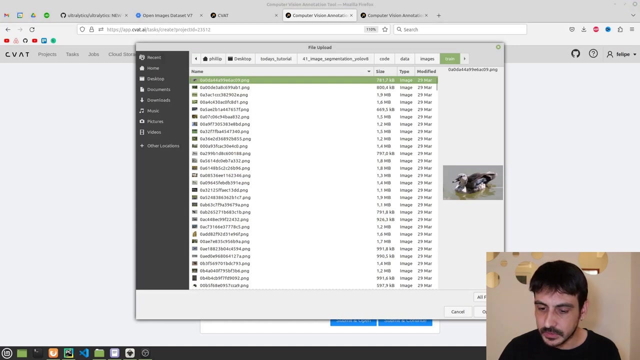 now i'm going to create a task. this is already. yeah, create new task. the task name will be doc. task zero one. it doesn't really matter the name, so i just i should selected a random name. then i'm going to add an image. i'm just going to click on the task and i'm going to add an image. i'm just 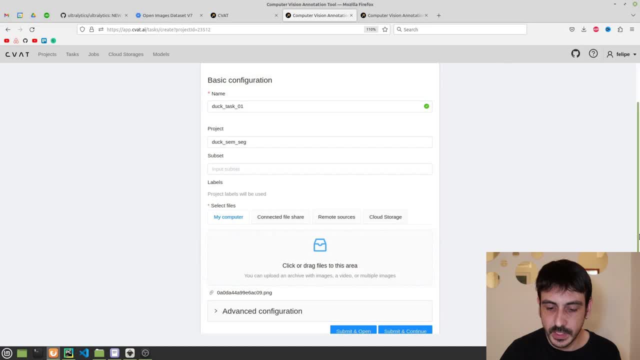 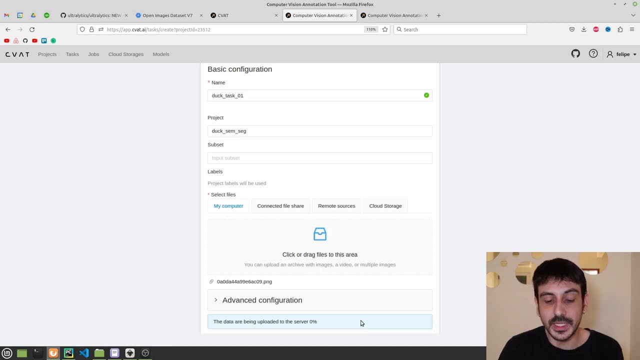 going to select this image. i'm just going to annotate one image- so this is going to be enough- and submit and open, so this is going to take a couple of seconds. this is where you need to select all of your images, all the images you want to annotate, but in my case, i'm only going to select. 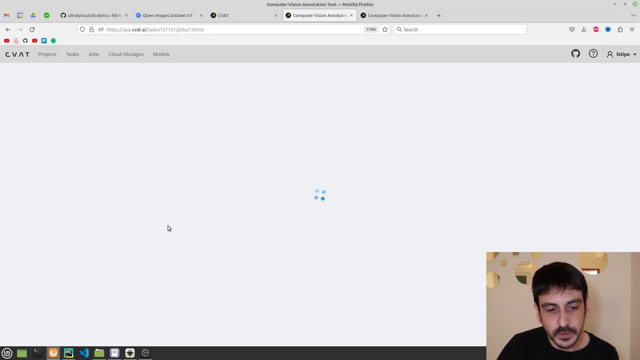 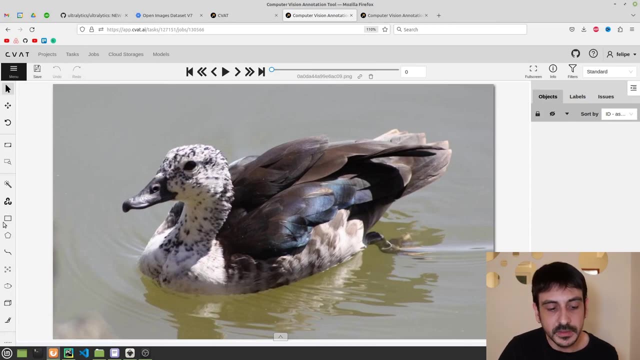 one. so i'm going to press here in job. so this is going to open the annotation job. right now i'm going to show you how you can annotate this image, how you can create a binary mask for this image. you need to go here to draw new polygon, then shape. so i'm going to start over here and this: 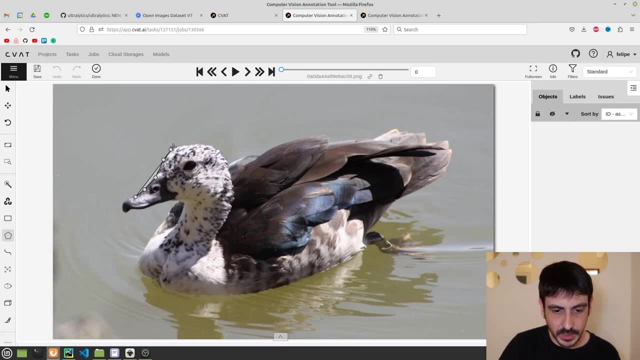 is pretty much all we need to do in order to create the semantic segmentation data set for this image. right, in order to create the binary mask for this image. you can see that i'm just trying to follow the contour of this object and you may notice that the contour i am following. 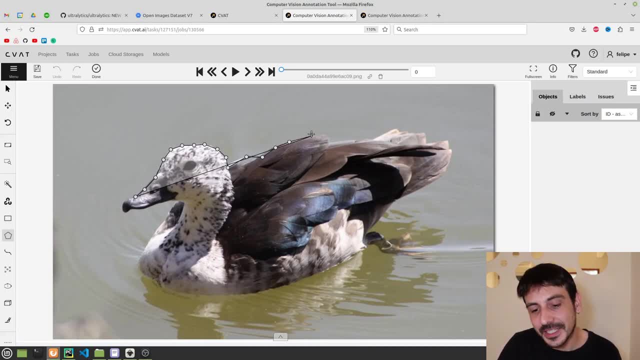 is not perfect. obviously, this is not perfect and it doesn't have to be perfect. if you're creating a data set, if you are creating the mask of a, of an image, if you are creating the mask of an object, then it definitely doesn't need to be pixel wise, perfect, right? you need to make a good mask. 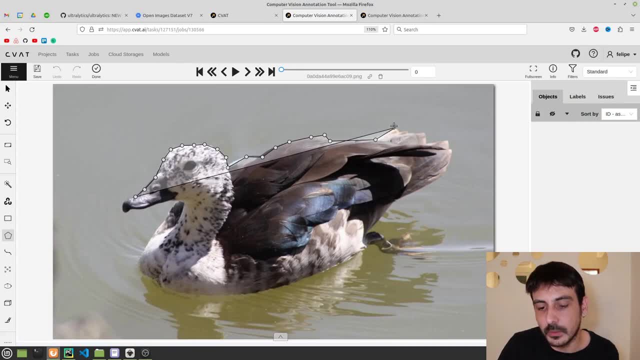 obviously, but something like this, as i am doing right now, will be more than enough. so this is a very time consuming process, you can see, and this is why i have selected only one, because if i do many, many images, it's going to take me a lot of time. 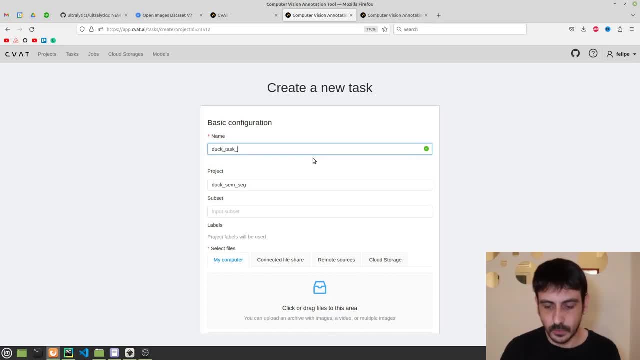 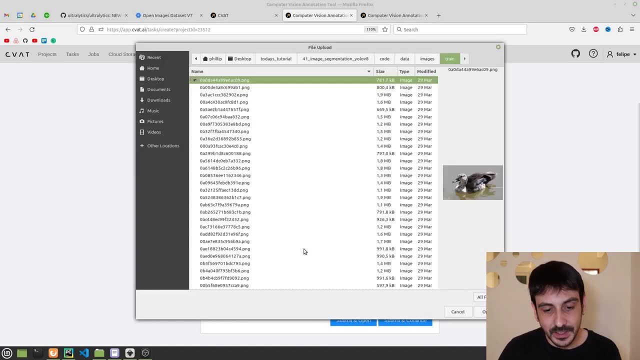 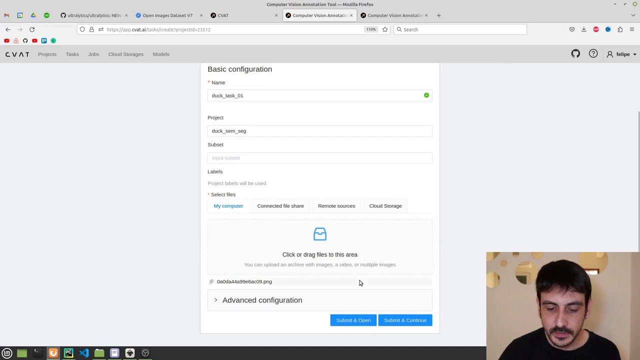 task zero one. it doesn't really matter the name, so i just i just selected a random name. then i'm going to add an image, i'm just going to select this image. i'm just going to annotate one image. so this is going to be enough. submit and open. so this is going to take a couple of seconds. this is where. 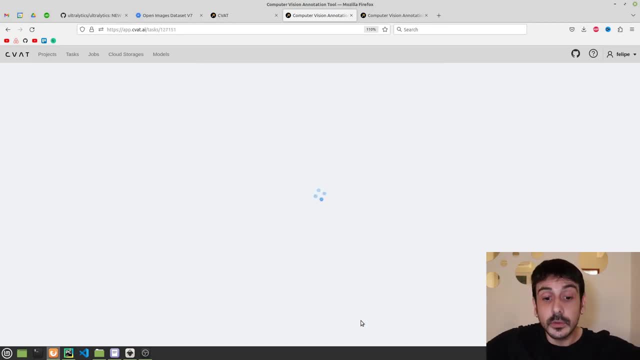 you need to select all of your images, all the images you want to annotate, but in my case i'm only going to select one, so i'm going to press here in job. so this is going to open the annotation job. right now i'm going to show you how you can annotate this image, how you can create a binary. 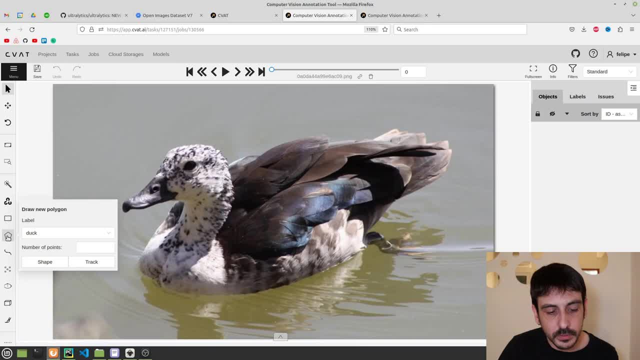 mask for this image. you need to go here to draw new polygon, then shape. so i'm going to start over here, and this is pretty much all we need to do in order to create the semantic segmentation data set for this image. right, in order to create the binary mask for this image. 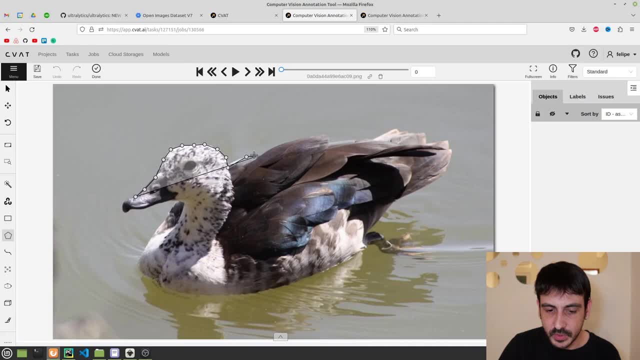 you can see that i'm just trying to follow the contour of this object and you may notice that the contour i am following is not perfect. obviously, this is not perfect and it doesn't have to be perfect. if you're creating a data set, if you are creating the mask of a of an image, if 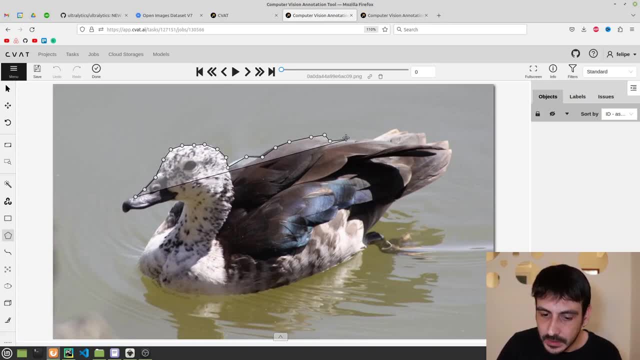 you are creating the mask of an object, then it definitely doesn't need to be pixel wise, perfect, right. you need to make a good mask, obviously, but something like this, as i am doing right now, will be more than enough. so this is a very time consuming process, you can see, and this is why 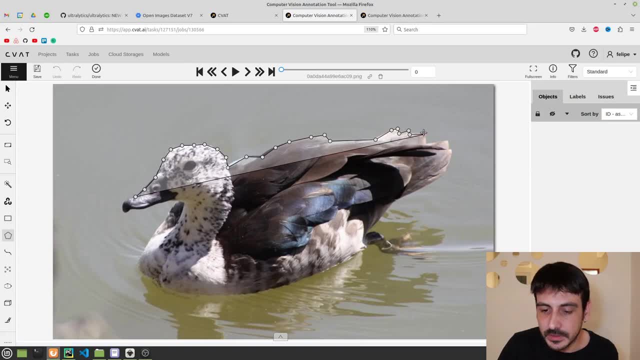 i have selected only one, because if i do many, many images, it's going to take me a lot of time and it doesn't make any sense because it's the idea is only for you to to see how to annotate the images right, so you can see that i'm following. 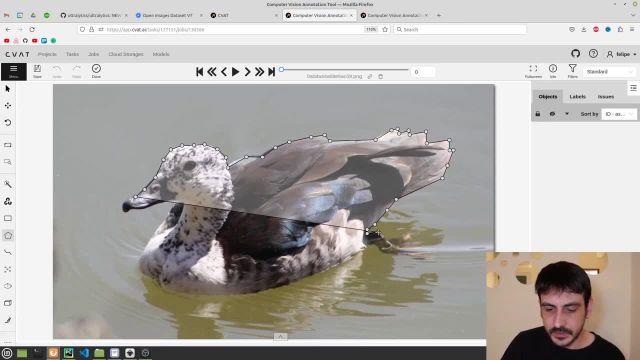 the contour. okay, and this is an interesting part, because we have reached the duck's hand or its leg or something like that, this part of the duck's body, and you can see that this is beneath the water, this is below the water and the. this is where. 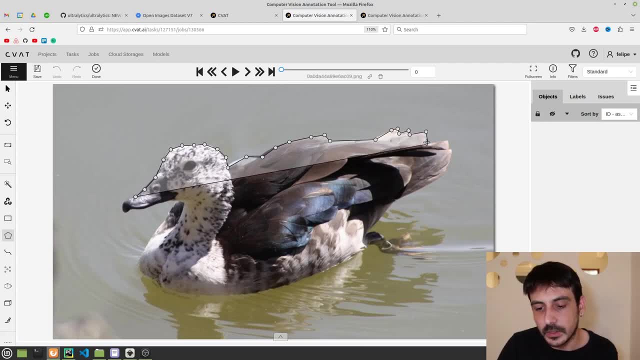 and it doesn't make any sense because it's the idea. it's only for you to to see how to annotate the images right, so you can see that i'm following the contour. okay, and this is an interesting part, because we have reached the duck's hand, or its leg, or 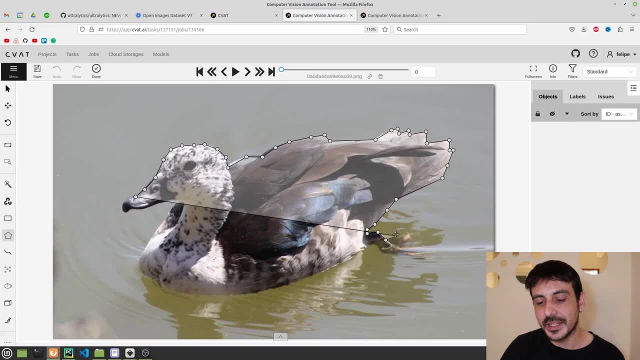 something like that, this part of the duck's body, and you can see that this is beneath the water, this is below the water and the this is where you're going to ask yourself: do you need to annotate this part or not? do you need to annotate this part as if it's part of the duck or not? 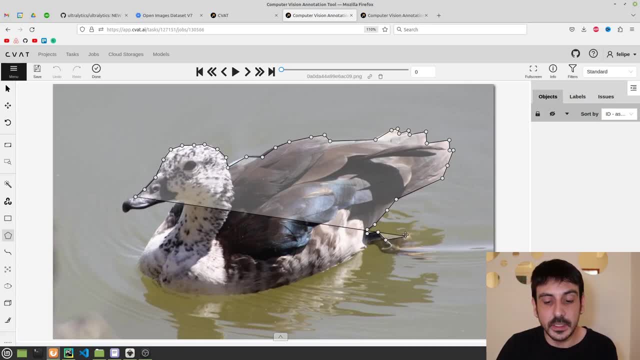 because you you could say, yeah, it's definitely part of this duck, but you are not really seeing a lot of these objects, right, it's like part of the water as well. so this is where you're going to ask yourself if you need to annotate this part or not, and in my case, i'm going to annotate it. but 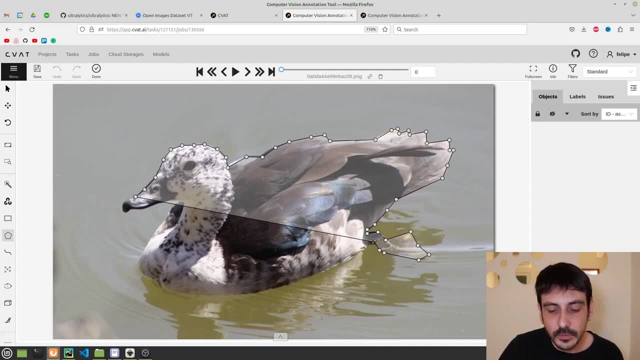 like you can do either way, in all of those sections, in all of those parts where you're not 100 convinced, then that's like a discussion. you could do it, you could not do it, it's up to you. so annotating a few images is always a good practice, because you are going to see. 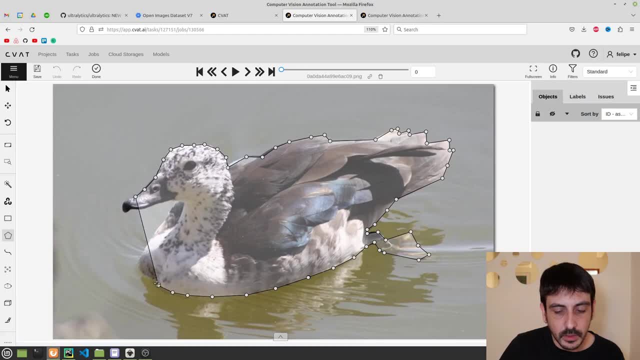 many, many different situations, as i have just seen over here, right where i have just seen, with this part of the duck which now i am super curious. what's the name? if you know what's the name of this part of the duck's body, please let me know in the comments below. i think it's called hand right because it's something like a. 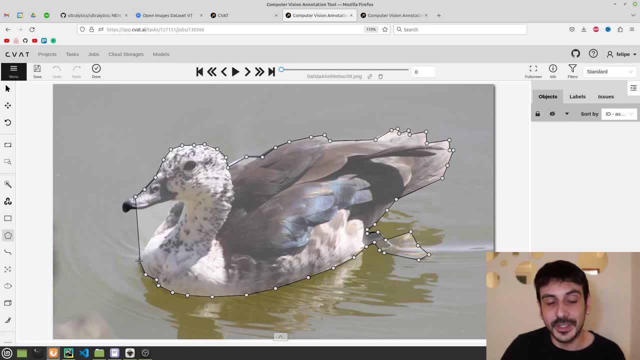 hand they have over there. but let me know if it has another name and you, if you know it, please let me know in the comments below. now let's continue. you can see i'm almost there. i have almost completed the mask of this duck. now i only have to. 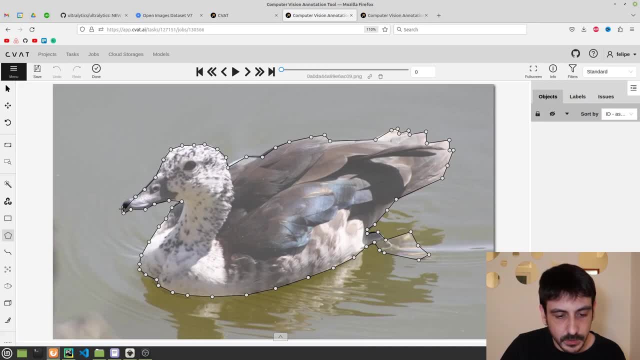 complete this peak, or whatever it's called, it seems. i don't really know much about ducks anatomy- i don't really know how the name of this part either. so anyway, i have already completed it. once i'm completed, i have to press shift n and that's going to be all. so this is the. 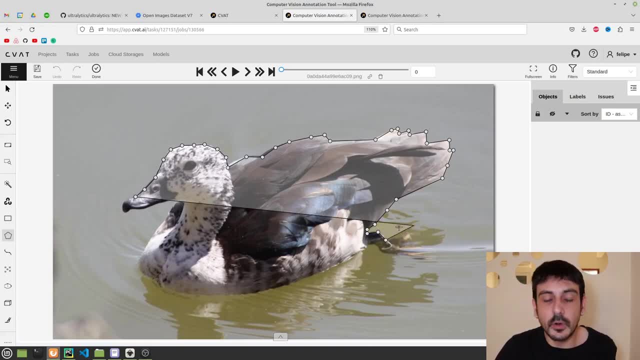 you're going to ask yourself: do you need to annotate this part or not? do you need to annotate this part as if it's part of the duck or not? because you you could say, yeah, it's definitely part of this duck, but you are not really seeing a lot of these objects, right, it's like part of the. 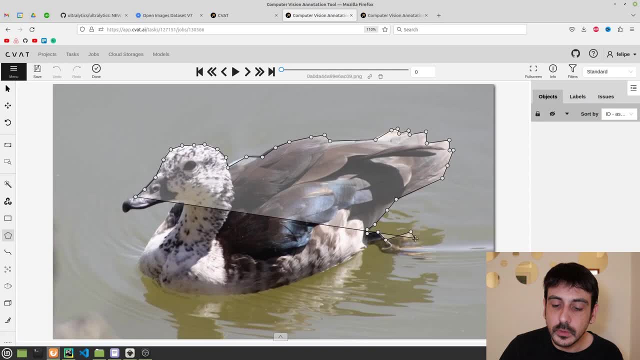 water as well. so this is where you're going to ask yourself if you need to annotate this part or not, and in my case i'm going to annotate it. but it's like you can do either way. in all of those sections, all of those parts where you're not 100 convinced, then that's like a discussion. you could do it. you. 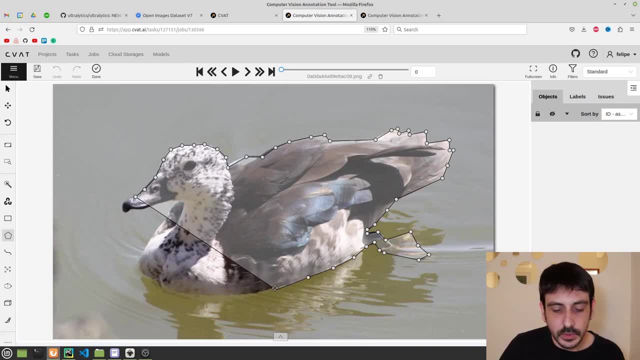 could not do it, it's up to you. so annotating a few images is always a good practice, because you are going to see many, many different situations, as i have just seen over here, right where i have just seen with this part of the duck, which now i am super, super curious. what's the name, if you know? 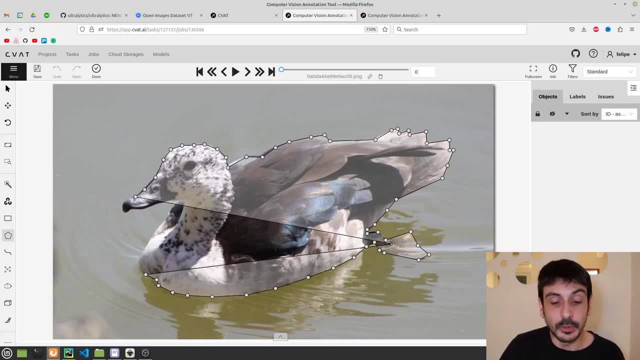 this part of the duck's body. please let me know in the comments below. i think it's called hand right, because it's something like a hand they have over there, but let me know if it has another name and you, if you know it, please let me know in the comments below. now let's continue. you can see i'm. 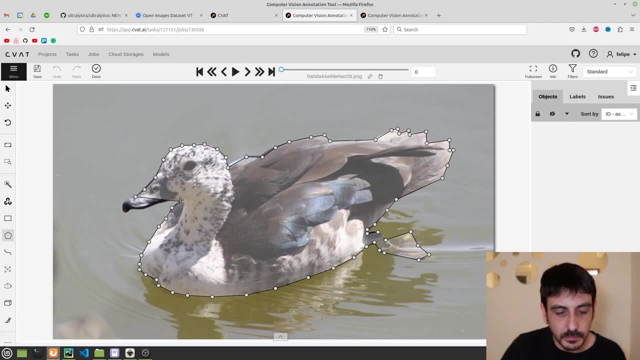 almost there. i have almost completed the mask of this duck. now i only have to complete this peak, or whatever it's called, it seems i don't really know much about ducks anatomy. i don't really know how the name of this part either. so anyway, i have already completed once. 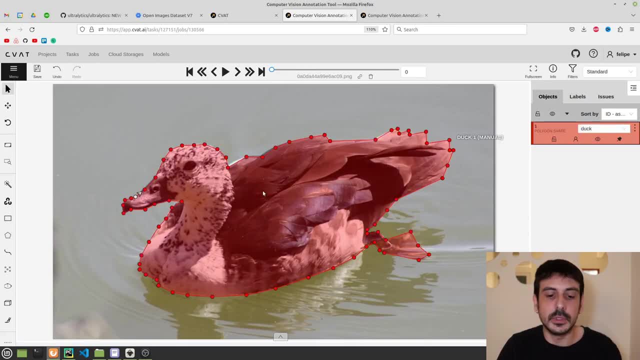 i'm completed, i have to press shift n and that's going to be all. so this is the mask. this is the binary mask i have generated for this object, for this duck, and this is going to be pretty much all what i have to do now is to click save. you can see that this is. this is definitely not a perfect mask. 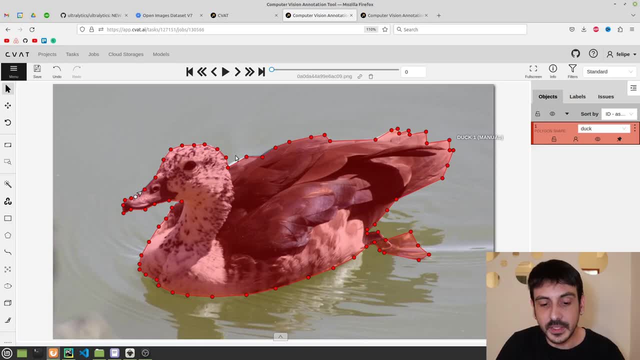 this is not a perfect, like pixel wise, perfect mask, because there are some parts of this duck which are not within the mask, but it doesn't matter. make it as perfect as possible. but if it's not 100 perfect, it's not the end of the world, nothing happens. so i have already saved. 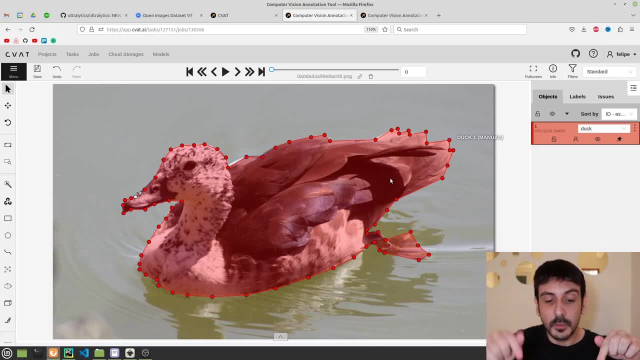 mask. this is the binary mask i have generated for this object, for this duck, and this is going to be pretty much all what i have to do now is to click save. you can see that this is: this is definitely not a perfect mask. this is not a perfect like pixel wise. 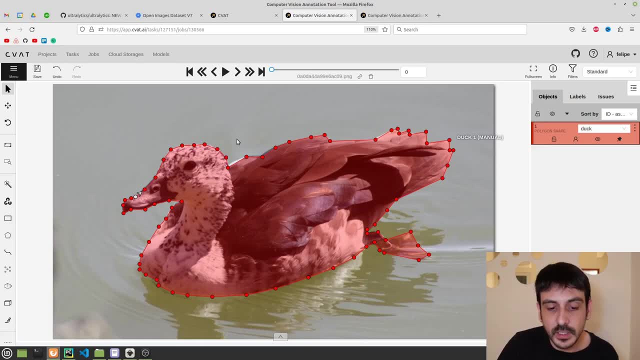 perfect mask, because there are some parts of this duck which are not within the mask, but it doesn't matter. make it as perfect as possible, but if it's not 100 perfect, it's not the end of the world, nothing happens. so i have already saved this image and what i need to do now is to download. 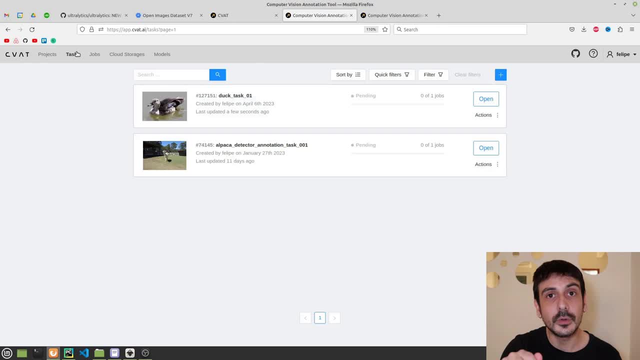 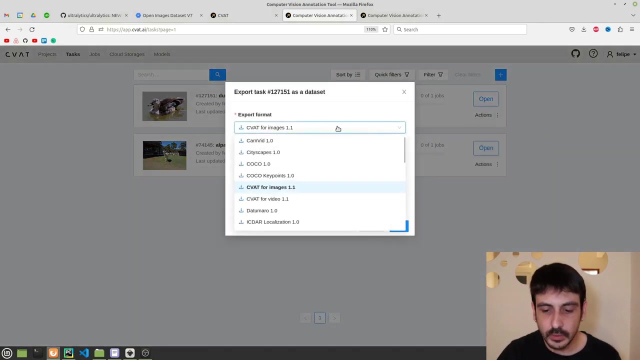 this data so i can show you how to download the data you have just annotated in order to create is the data set. so this is what i'm going to do: i'm going to select this part, this option over here, and i'm going to export task: data set and then i'm going to select. 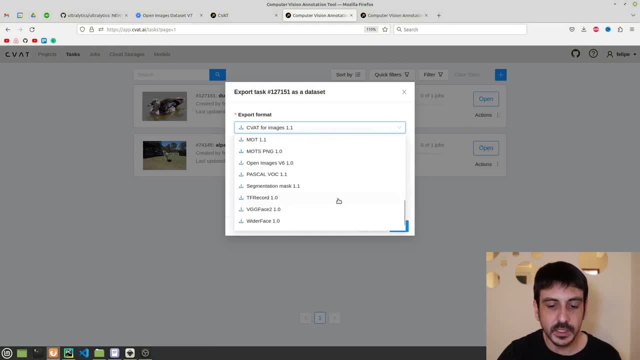 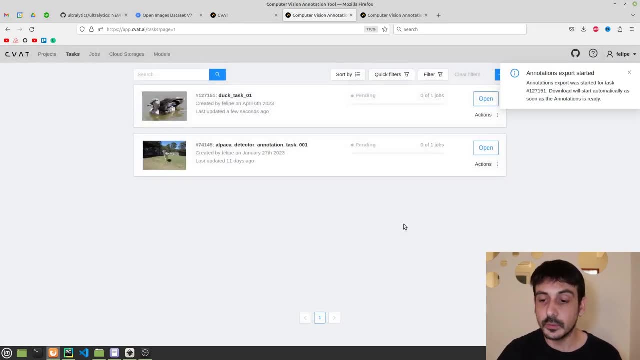 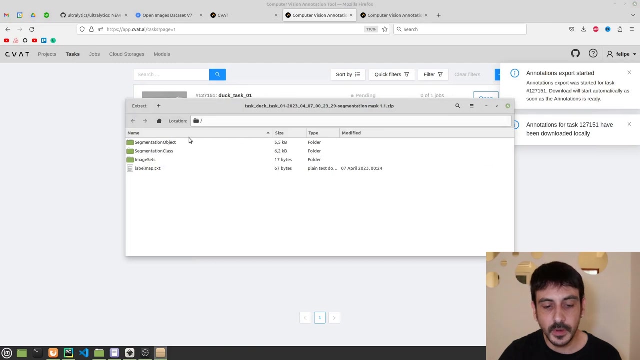 this option, which is segmentation mask 1.1. i'm just going to select that option and i'm going to click okay. so that's going to be all. we only need to wait a couple of minutes and that's pretty much all the data has been downloaded. now i'm going to open this file. enjoy it just one more time, guys. 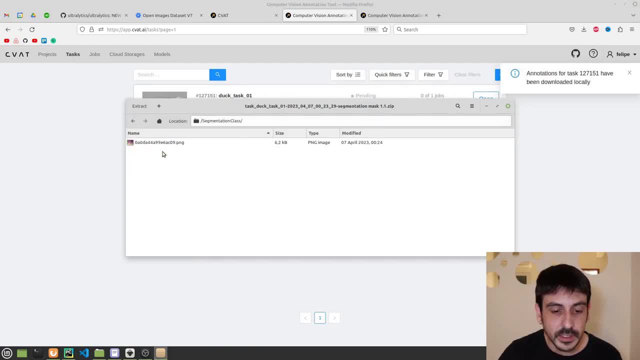 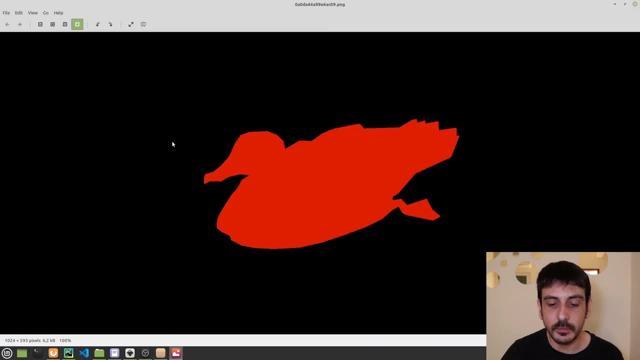 file and basically, the images you are interested in are going to be here, right? you can see in me, in my case, i only have one image, but this is where you're going to have many, many, many images, and please mind the color. you will get all these images in, right? in my case, i have a download this: 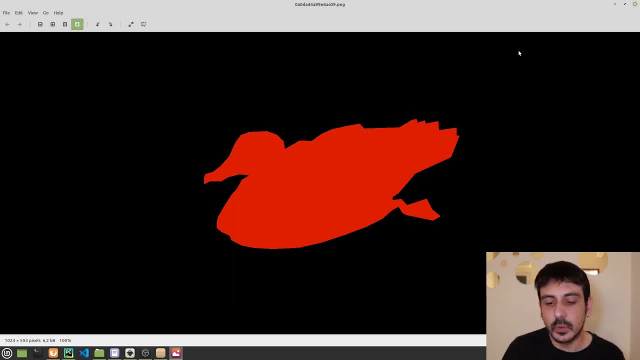 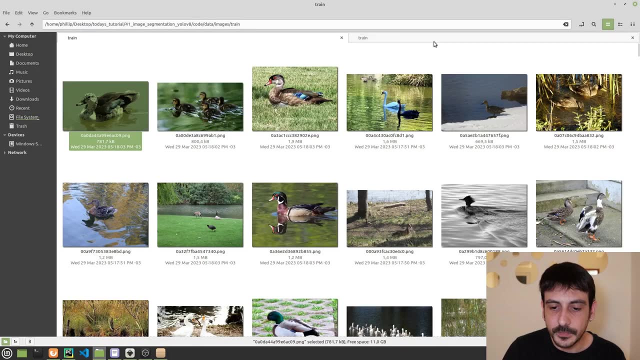 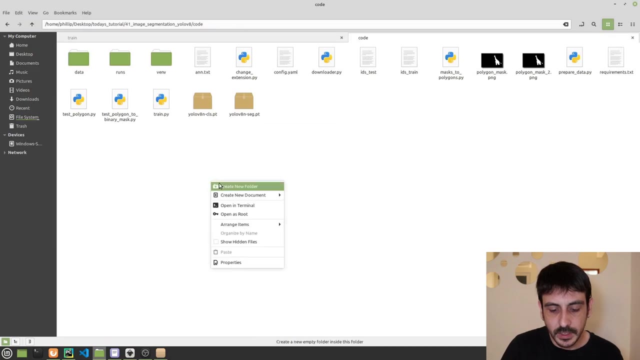 image in red. it doesn't really matter, just mind that you could have something different than white. but once you have all your images, what you need to do is to create a directory. i'm going to show you how i do it. i am going maybe here and i'm going to create a very temporal directory, which 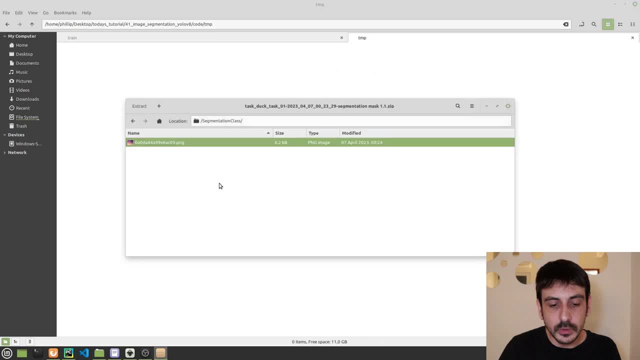 i'm going to call tmp, and this is where i'm going to locate this image. right, and i am going to. i'm going to create two directories: one of them is going to be uh masks and then the other one is going to be called text labels, and you're going to see why in only a minute, and this is where i'm going to locate the. 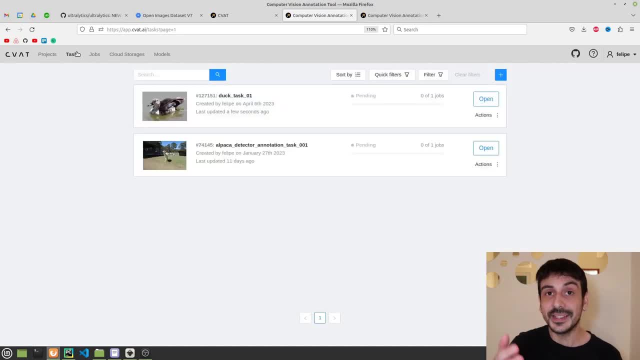 this image, and what i need to do now is to download this data, so i can show you how to download the data you have just annotated in order to create your data set. so this is what i'm going do: i'm going to select this part, this option over here, and i'm going to export task data set. 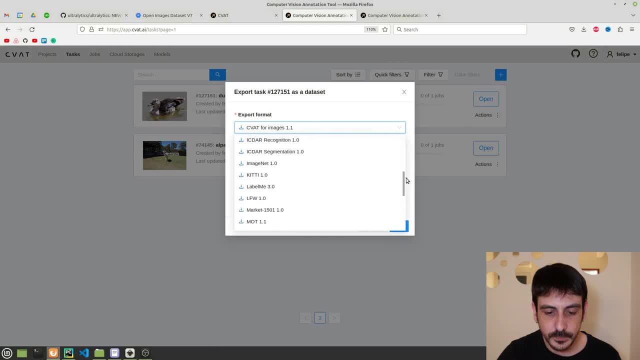 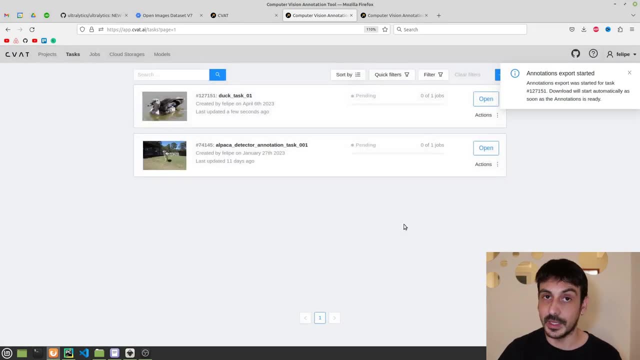 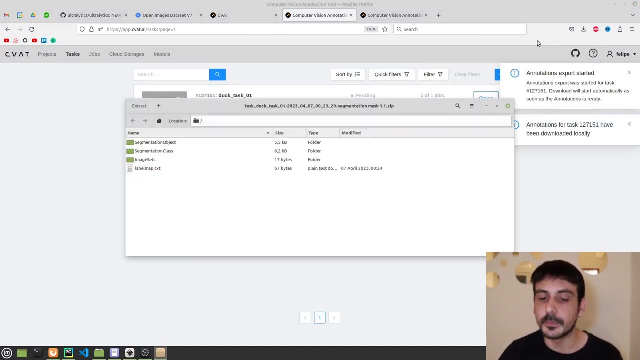 and then i'm going to select this option, which is segmentation mask 1.1. i'm just going to select that option and i'm going to click ok. so that's going to be all. we only need to wait a couple of minutes and that's pretty much all the data has been downloaded. now i'm going to open this. 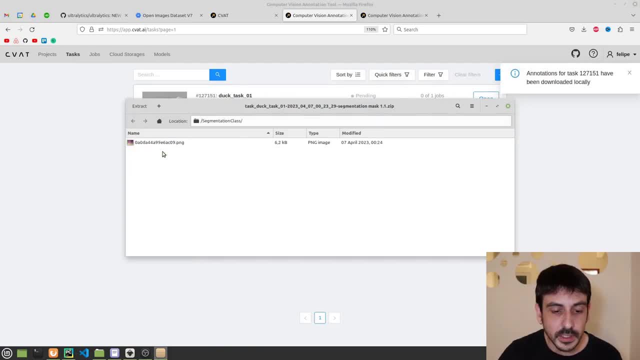 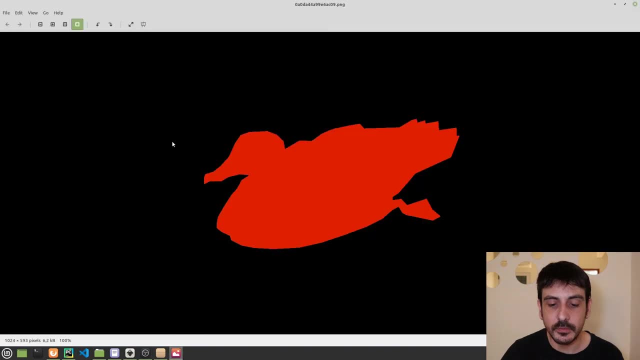 file and basically, the images you are interested in are going to be here, right? you can see in me, in my case, i only have one image, but this is where you're going to have many, many, many images, and please mind the color. you will get all these images in, right? in my case, i have a download this: 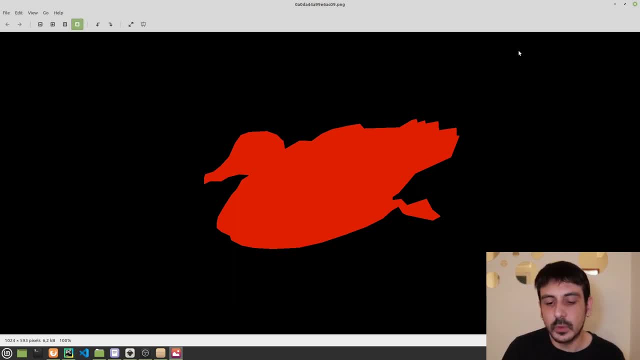 image in red. it doesn't really matter, just mind that you could have something different than white. but once you have all your images, what you need to do is to create a document that's going to be a document that's going to be a document that's going to be a. 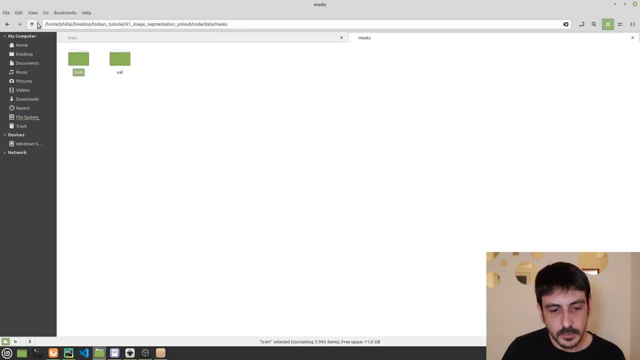 directory. i'm going to show you how i do it. i am going, maybe here and i'm going to create a very temporal directory, which i'm going to call tmp, and this is where i'm going to locate this image, right, and i am going to. i'm going to create two directories. one of them is going to be masks. 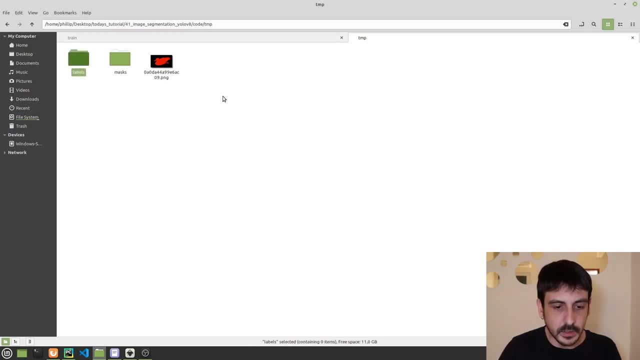 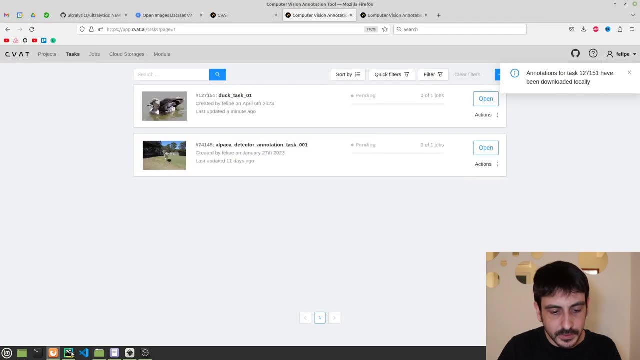 and then the other one is going to be called labels, and you're going to see why in only a minute. and this is where i'm going to locate the mask here. and then i am going to pycharm because i have. And this is where i'm going to locate the mask here. and then i am going to pycharm because i have. 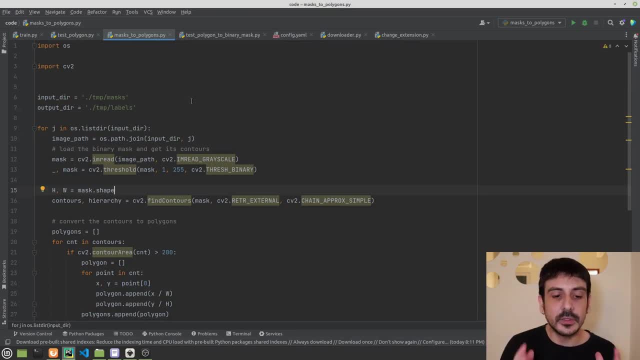 created a script, a python script, which is going to take care of a very, very, very important process. we have created masks which are images, which are binary images, and that's perfect, because that's exactly the information we need in order to train a semantic segmentation iring. but the way 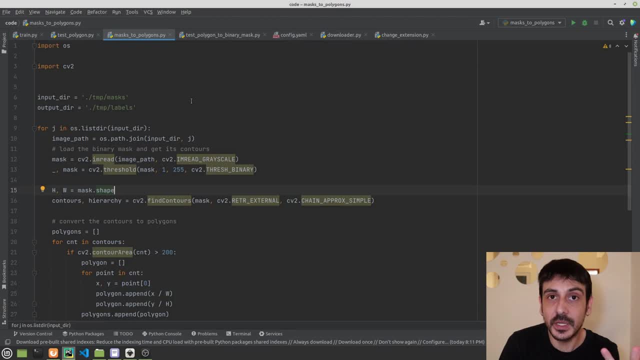 Ullo V8 works is a bit more complicated than i expected, but we can use it to create a very, very we need to convert this image, this binary image, into a different type of file. we are going to keep exactly the same information, but we are going to convert this image into another type of file. 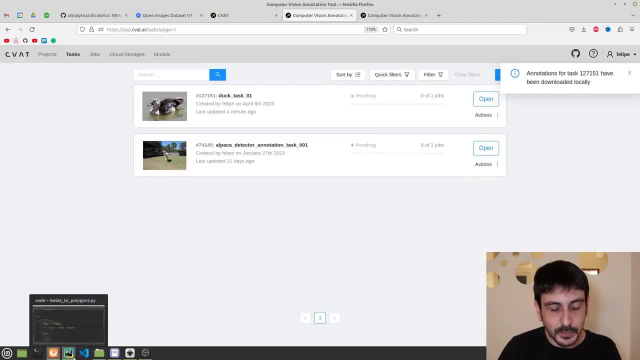 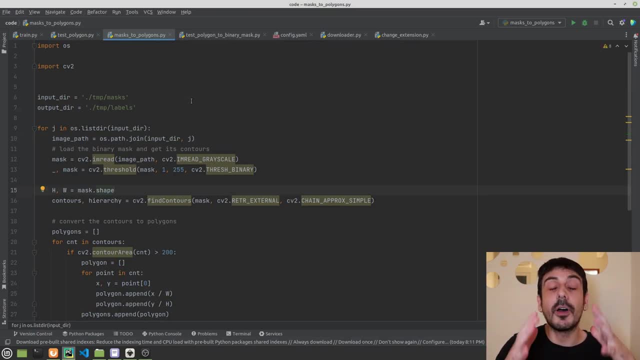 mask here. and then i am going to python, because i have created a script, a python script, which is going to take care of a very, very, very important process. we have created masks which are images, which are binary images, and that's perfect, because that's exactly the information. 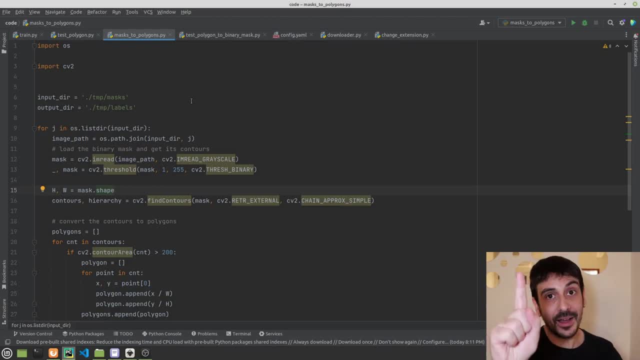 we need in order to train a semantic segmentation algorithm. but but the way yolo v8 works, we need to convert this image, this binary image, into a different type of file. we are going to keep exactly the same information, but we are going to convert this image into another type of file. so let me show you how. this is a python file i have created in. 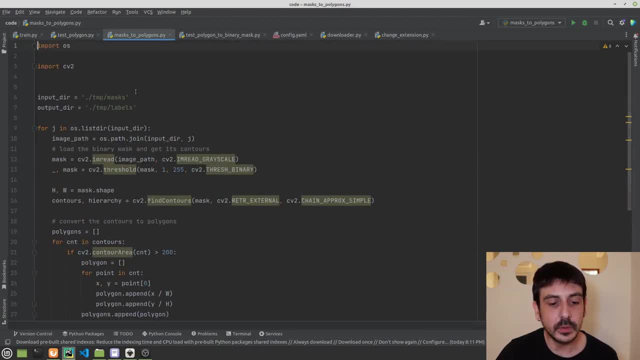 order to take care of this process, and the only thing you need to do is to edit these fields. this is where you're going to put all the masks. this is a directory which is going to contain all the masks you have generated, and this is going to be the output directory. you can see that these two 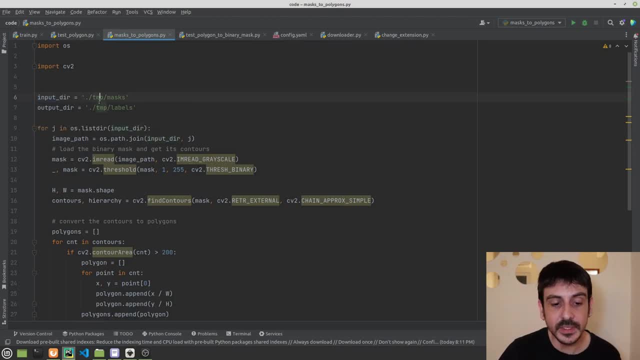 variables are already named properly in my case, because this is a tmp directory i have just created. this is where i have located the mask i have just generated with cpat and this is my output directory. so take a look what happens when i press play. so the script has just been. 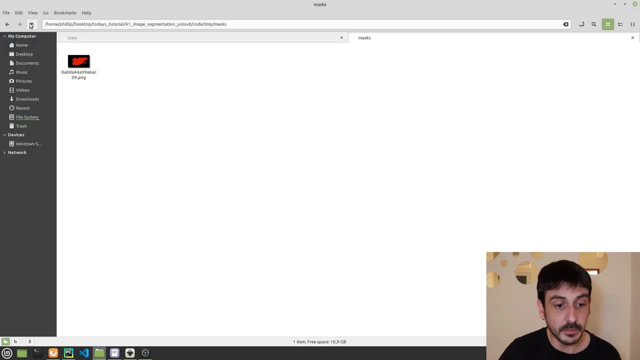 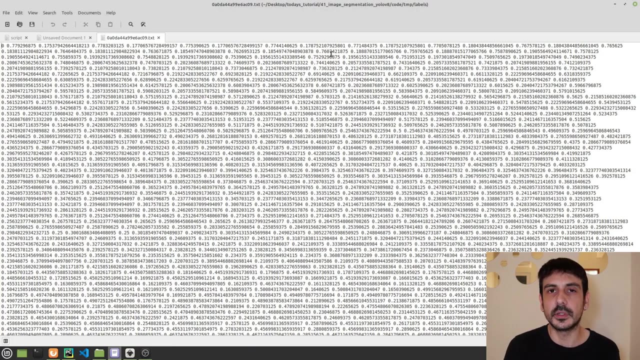 executed, everything is okay. this is the mask i have. i have input and this is the file which was generated from this mask, and this looks super, super, super, absolutely crazy. right, it's a lot of numbers. it's like a very, very crazy thing. without going to the details, let's just say: 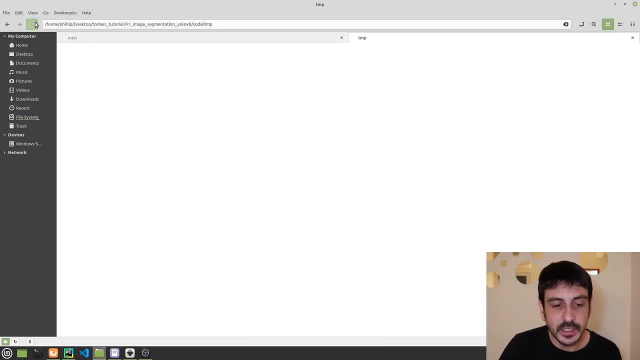 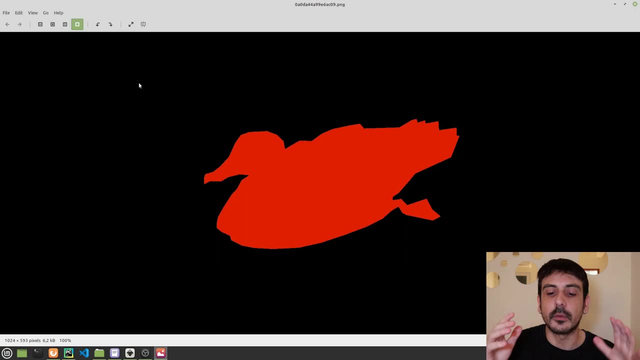 that this is exactly the same information we had here. this is exactly exactly the same information we have here, but in a different format. let's, let's keep that idea right: exactly the same information in a different format, and that's exactly the format. yolo v8. 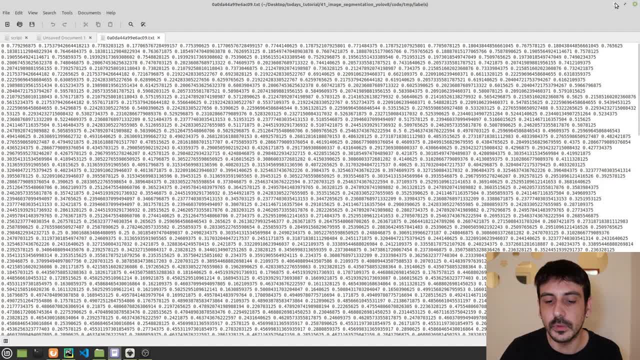 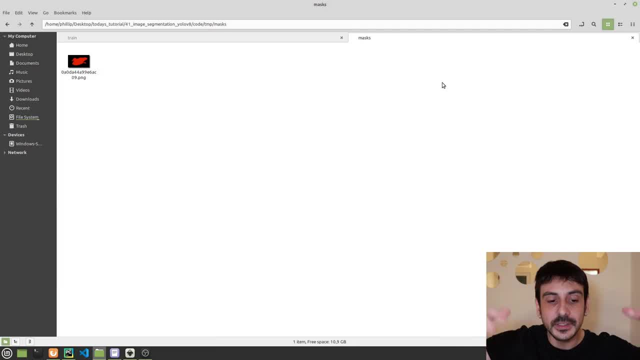 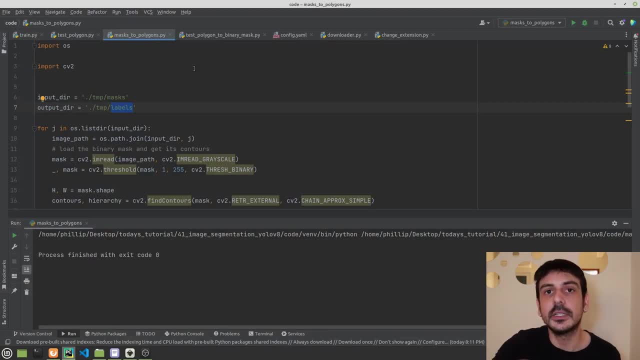 needs in order to train the semantic segmentation model. so this is exactly what you need to do: once you have created all of your masks, you need to download these files into your computer and then please, my please, execute this script so you can convert your images into a different type of files. 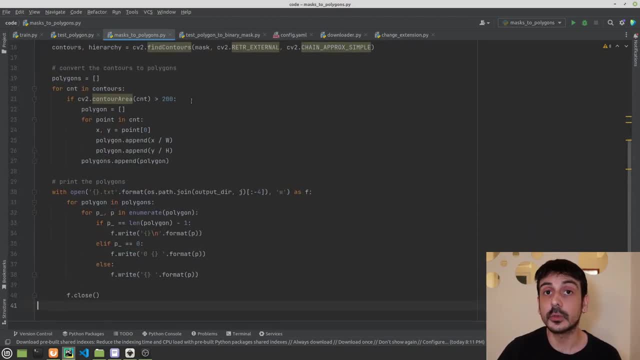 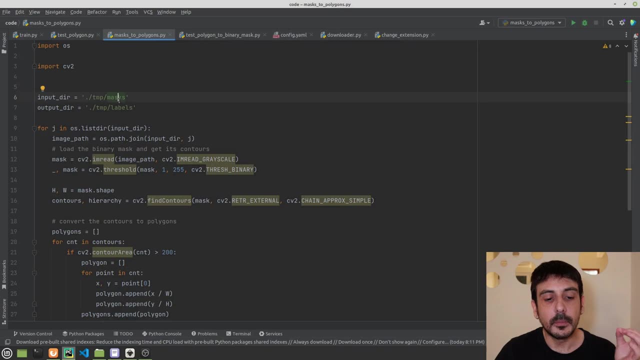 so let me show you how. this is a phyton file i have created in order to take care of this process, and the only thing you need to do is to edit these fields. this is where you're going to put all the masks, this directory which is going to contain all the masks you have generated, and 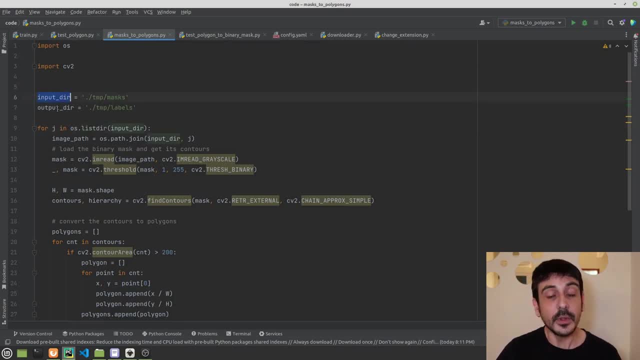 this is going to be the output directory. you can see that these two variables are already named properly in my case, because this is a tmp directory i have just created. this is where i have located the mask i have shared with cpat, and this is my output directory. so take a look what. 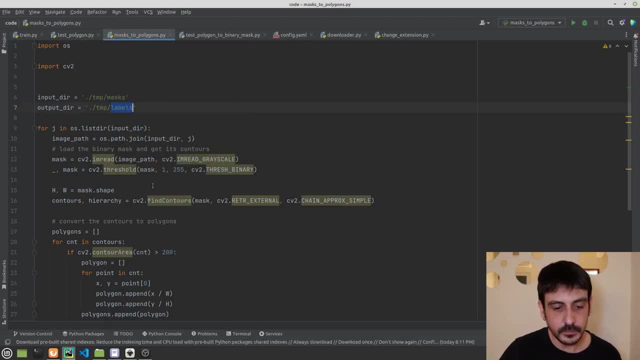 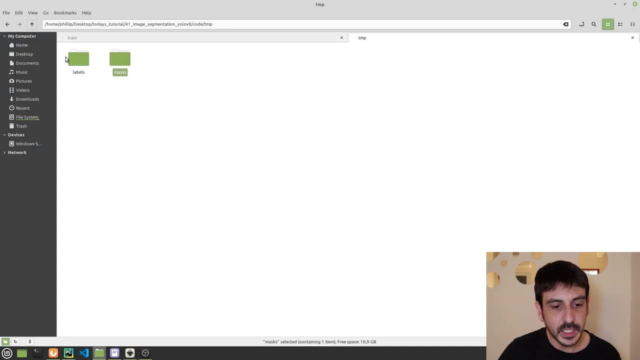 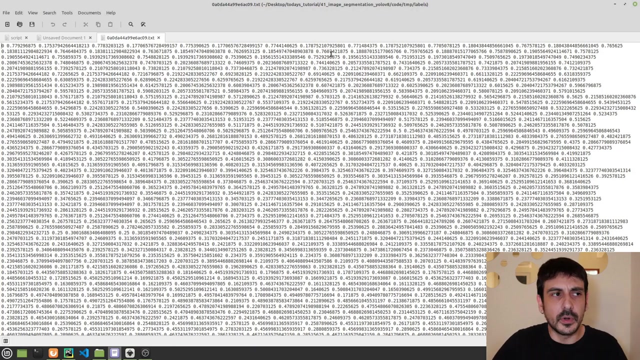 happens when i press play. so the script has just been executed, everything is okay. this is the mask i have, i have input and this is the file which was generated from this mask, and this looks super, super, super, absolutely crazy. right, it's a lot of numbers, it's like a very, very crazy thing. without going to the details, let's just say that this is exactly. 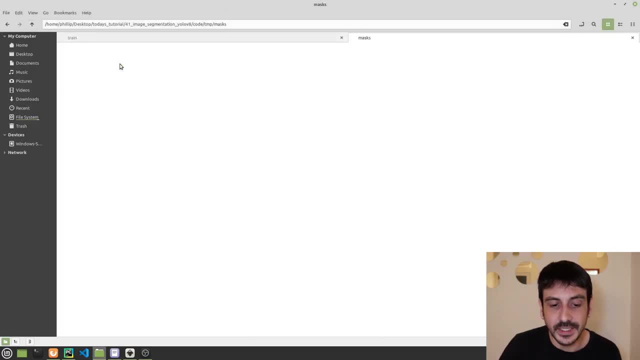 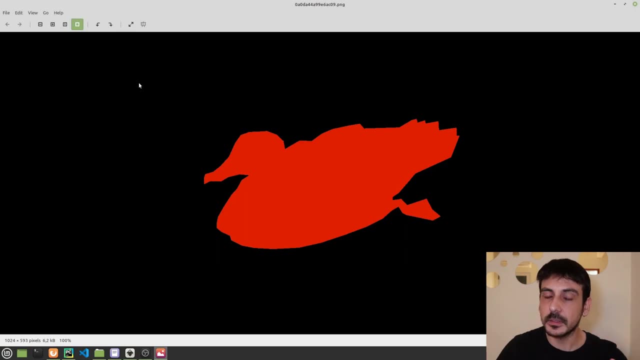 the same information we had here. this is exactly exactly the same information we have here, but in a different format. let's, let's keep that idea right: exactly the same information in a different format, and that's exactly the format yolo v8 needs in order to. 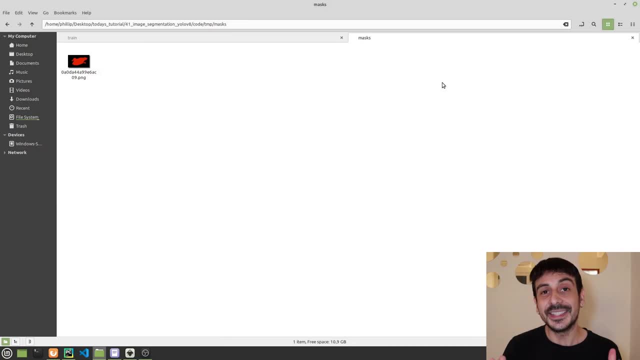 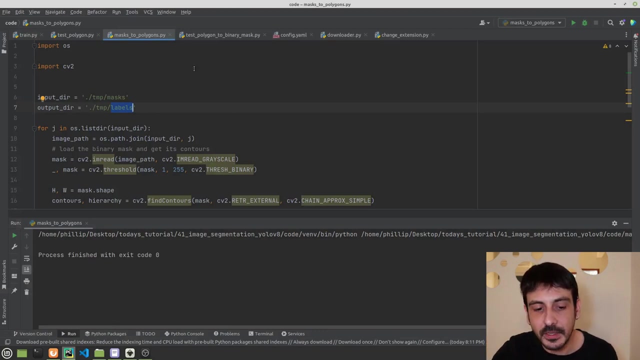 train the semantic segmentation model. so this is exactly what you need to do: once you have created all of your masks, you need to download these files into your computer and then please, my please, execute this script so you can convert your images into a different type of files. and obviously this: 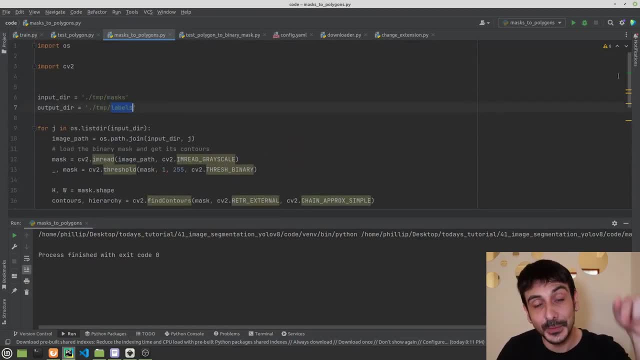 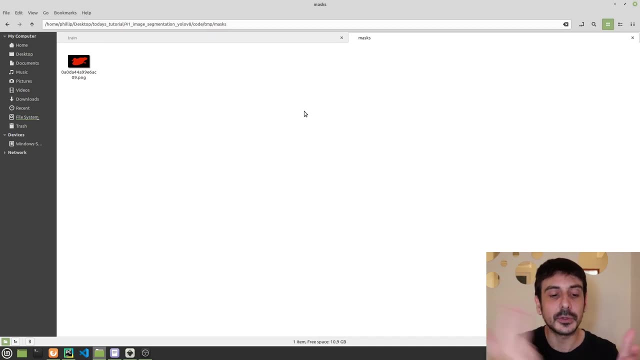 script will be available in the github repository of today's tutorial. so that's pretty much all in order to create your, your annotations, and in order to download the github repository all of these annotations, and in order to format everything the way you should. now let me show you the structure you need to format, the way you need to structure all of your. 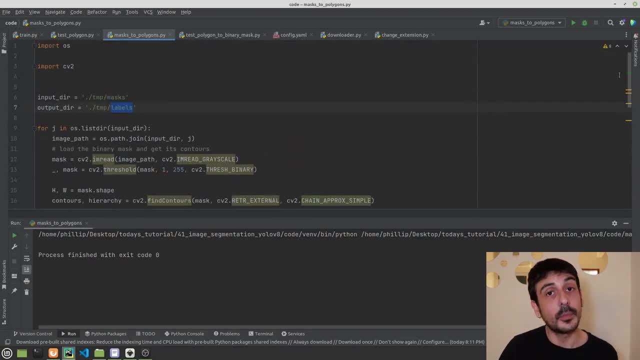 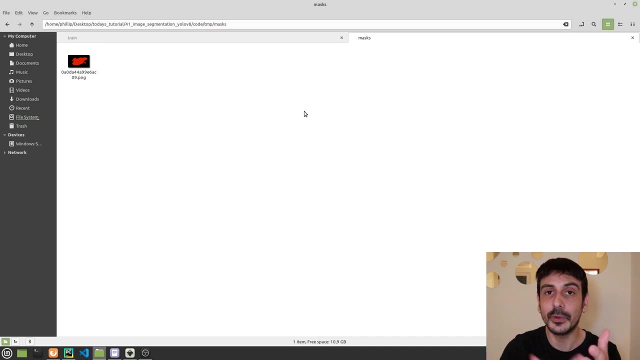 and obviously, this script will be available in the github repository of today's tutorial. so that's pretty much all. in order to create your, your annotations, in order to download these annotations and in order to format everything the way you should. now let me show you the structure you need to format, the way you need to structure. 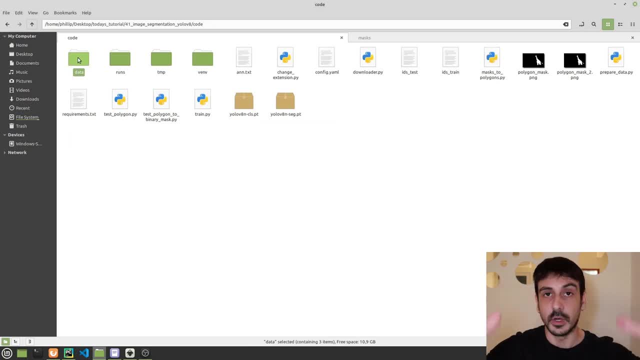 all of your file system so it complies with yolo v8. remember, this is something we have already done in our previous tutorials regarding yolo v8. once you have your data, you need to structure your data, you need to format your data, you need to structure your file system so yolo v8. 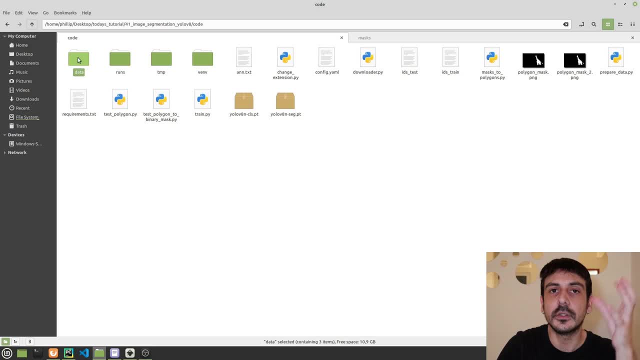 finds absolutely where everything is located right. you're going to locate your images in a given directory. you're going to locate your annotations, your labels, in another directory. so everything is just the way your lobby 8 expects it to be right. so let me show you. i have a directory which is my 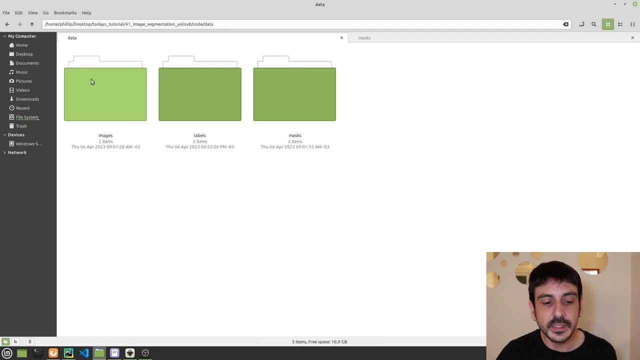 root directory, which is called data within data. i have three directories, but this directory, the masks directory, is not really needed. it's just there because that's the way i i got my, my, my masks, my data. but it's not really needed and in order to show you this, 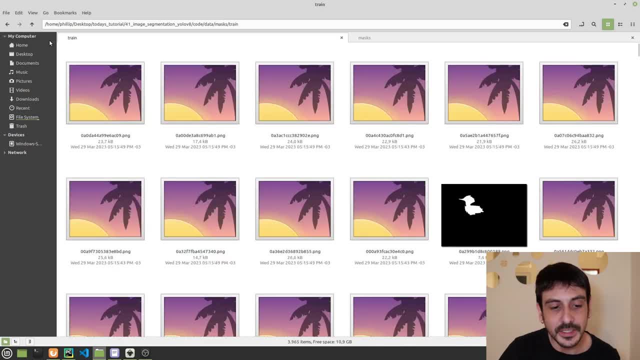 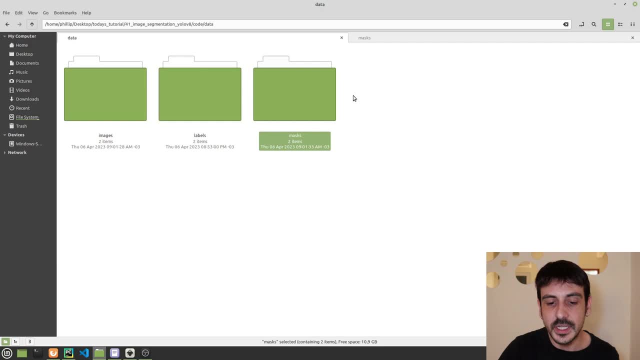 directory, which is the one containing all of my binary masks. in order to be more clear that this is not needed for this part of this process. what i'm going to do is i'm going to delete this directory right now. it's gone. okay, now we only have two directories, and these are exactly. 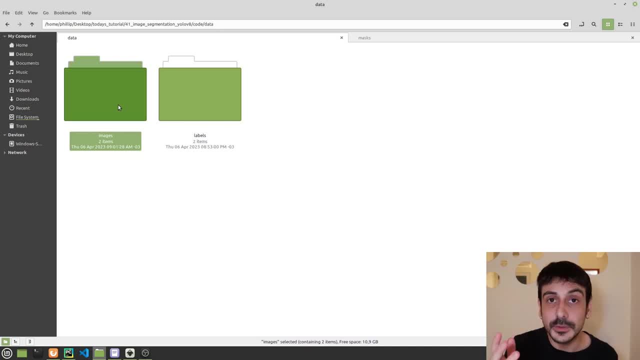 the directories we need in this part of this process where we are creating all the structure, so images. you can see that we have two directories. one of them is called images, the other one it's called labels within images. we have two other directories. one of them is called 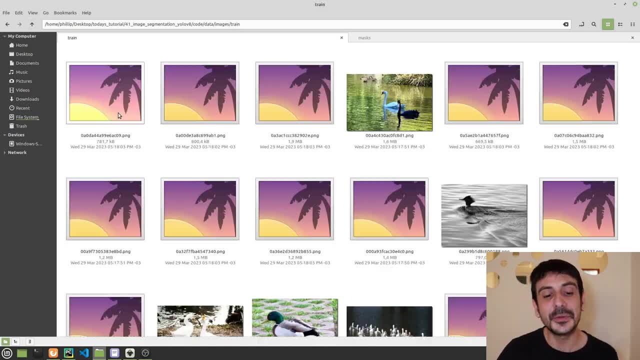 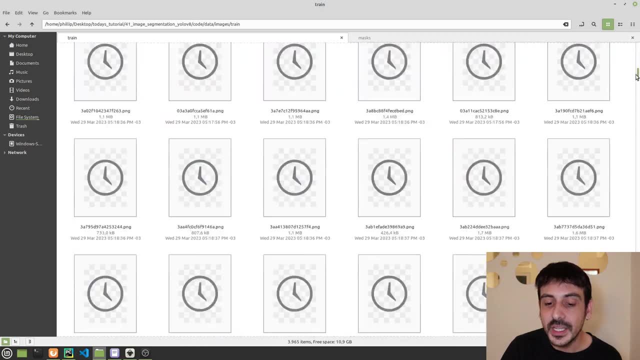 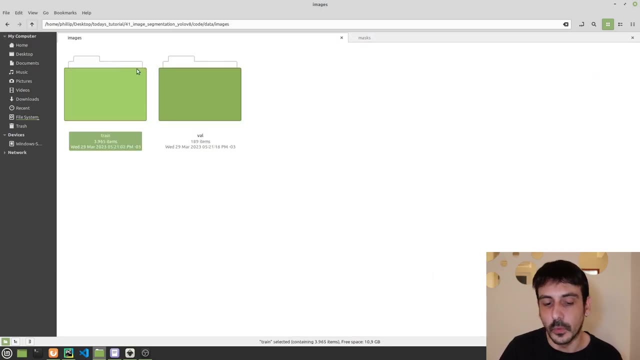 train and there one is called valve and train is directory where we are going to have all of our training data. this is where we are going to have all of our training images. these are all the images yellow v8 is going to use in order to train the module, in order to train the semantic segmentation model. then bell also contains images. 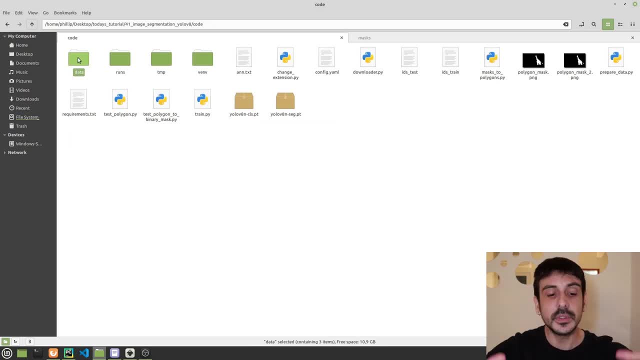 file system so it complies with yolo v8. remember, this is something we have already done in our previous tutorials regarding yolo v8: once you have your data, you need to structure your data, you need to format your data, you need to structure your file system. so yolo v8 finds absolutely where. 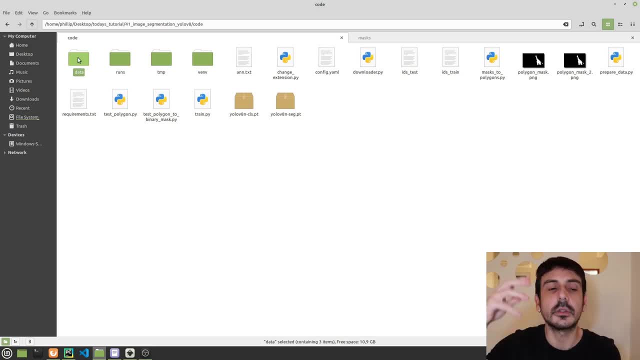 everything is located right. you're going to locate your images in a given directory. you're going to locate your annotations, your labels, in another directory. so everything is just the way your lobby 8 expects it to be right. so let me show you. i have a directory which is my root directory. 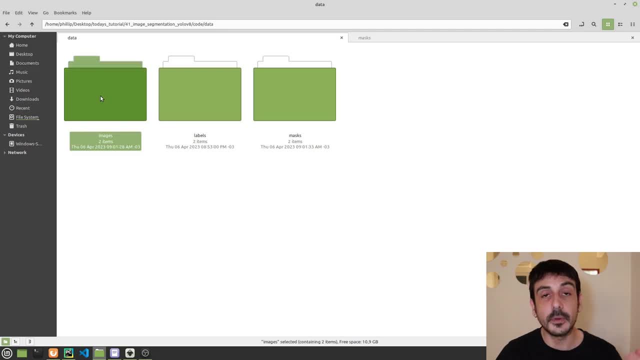 which is called data within data. i have three directories, but this directory, the masks directory, is not really needed. it's just there because that's the way i i got my, my, my masks, my data. but it's not really needed in order to show you this directory, which is the one containing all. 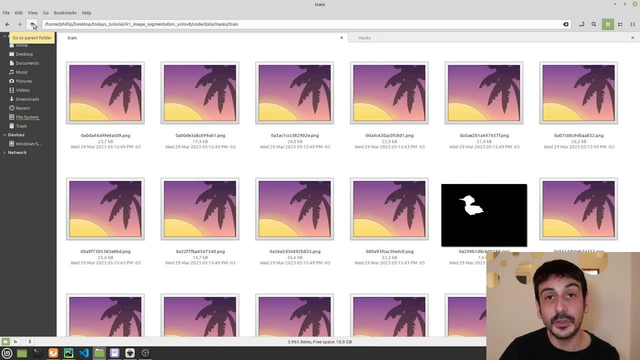 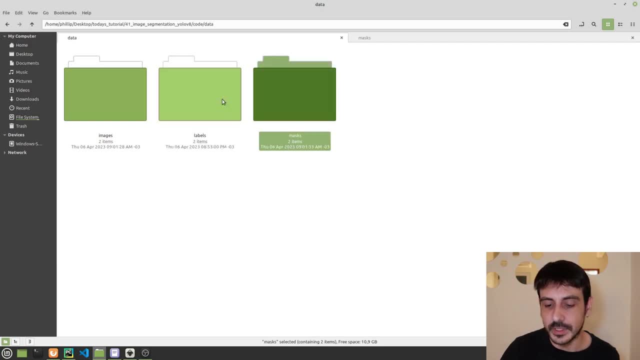 of my binary masks in order to be more clear that this is not needed for this part of this process. what i'm going to do is i'm going to delete this directory right now. it's gone. okay, now we only have two directories, and these are exactly the directories we need. 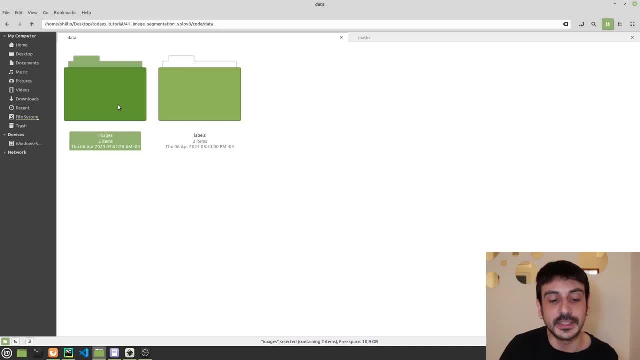 in this part of this process where we are creating all the structure for our data. so images, you can see that we have two directories. one of them is called images, the organ's called labels within images. we have two other directories. one of them is called train and the other one is called ball. 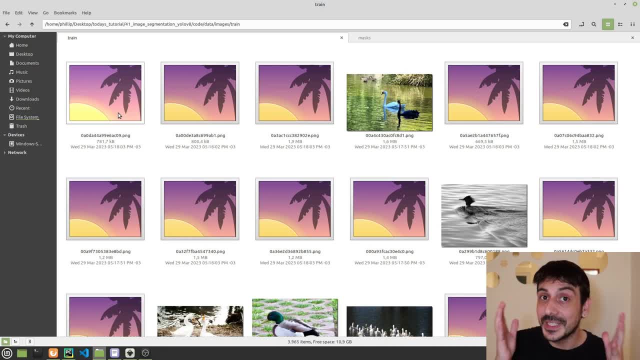 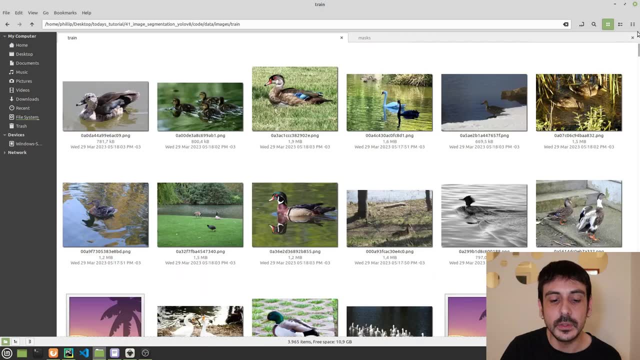 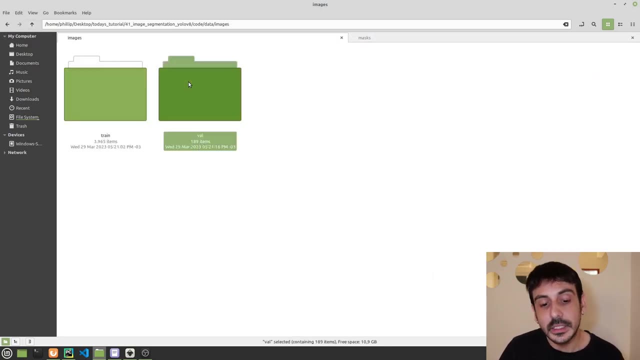 and train is directly where we are going to have all of our training data. this is where we are going to have all of our training images. these are all the images yolo v8 is going to use in order to train the model, in order to train the segmentation model, then valve- it also contains images and these: are the images we are going to use now. if you have a particular capture screen or 6 goron of the machine, we are going to have any images linked and those images are all going to be Labor in the software CKtreeurg or Puttingr2.com. bye, bye. 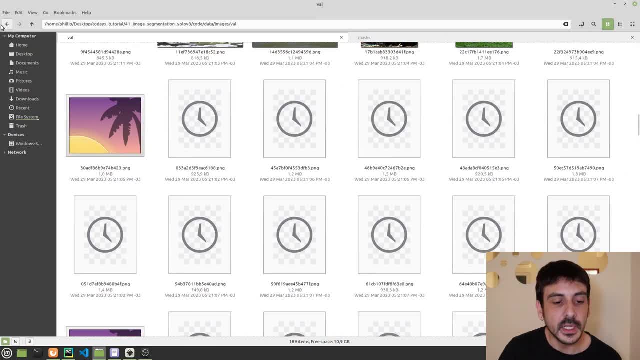 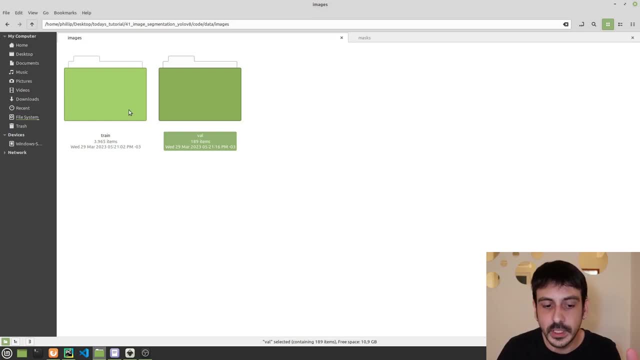 to use in order to validate the model right. so remember, you need to have two directories. one of them should be called train. it's very important the name. it should be called train and everyone should be called val. now, going back, you can see that we have two directories. one of them is images. 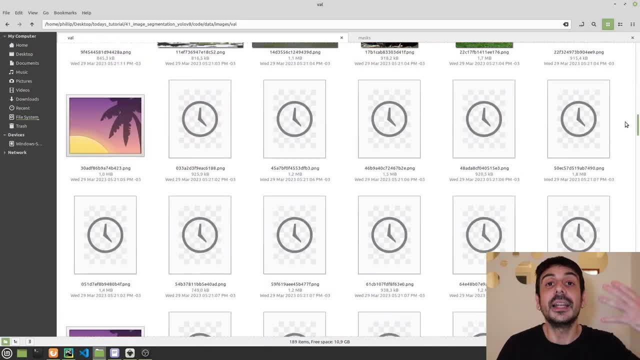 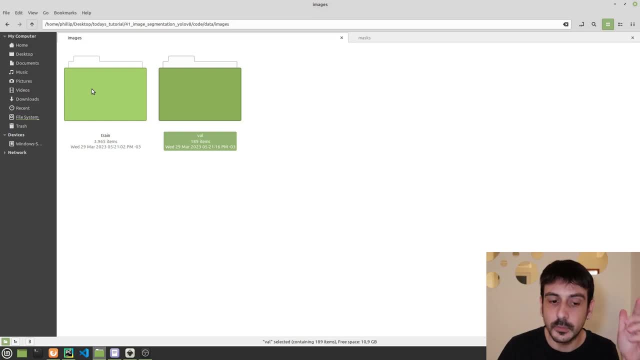 and these are the images we are going to use in order to validate the model right. so remember, you need to have two directories. one of them should be called train. it's very important the name. it should be called train and everyone should be called val. now, going back, you can see that we 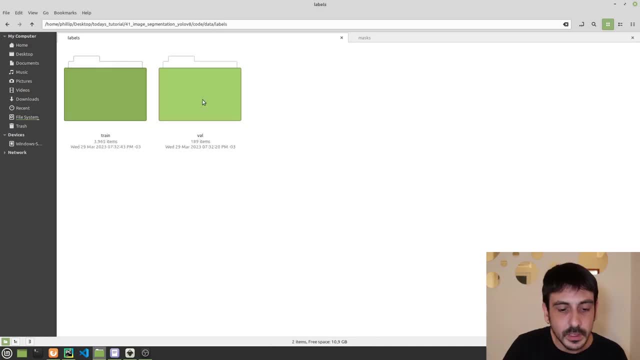 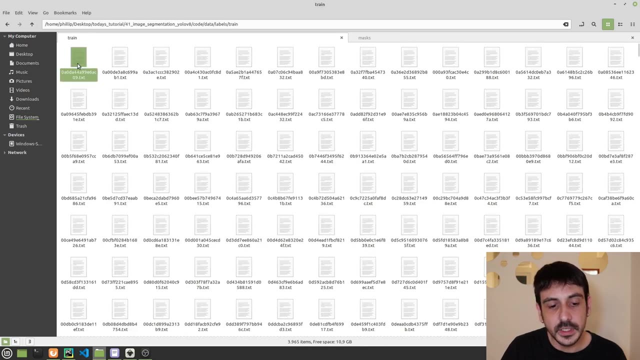 have two directories. one of them is images, the other one is label, and if i go within labels, you can see that there are two other directories also. they are named train and ball and if i open these directories, these are the type of files i have generated with the exact same script i showed you. 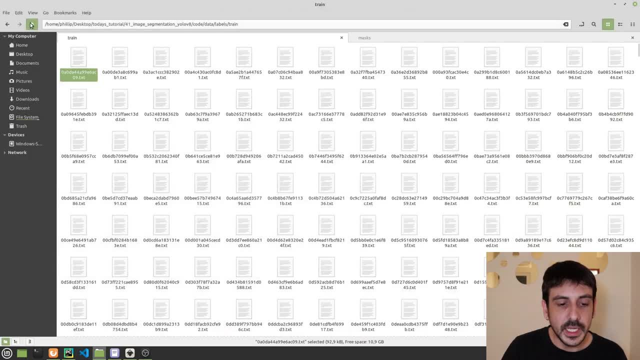 a few minutes ago. so within labels we have two directories: train and ball, and train are all the annotations we have generated from the training data, from the training masks. right, long story short, we have our root directory. within the root directory have two directories. one of them is called images. 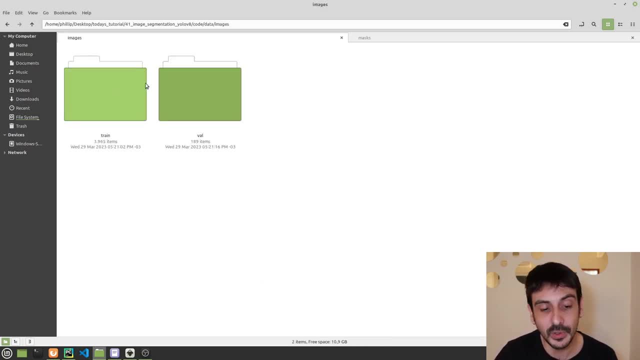 one is called labels within images. we have two directories: train and ball. within train and within ball. it's all of our data, all of our images and within labels. it's exactly the same structure: two directories: train and ball, and within train and within ball. it's where we locate all of our 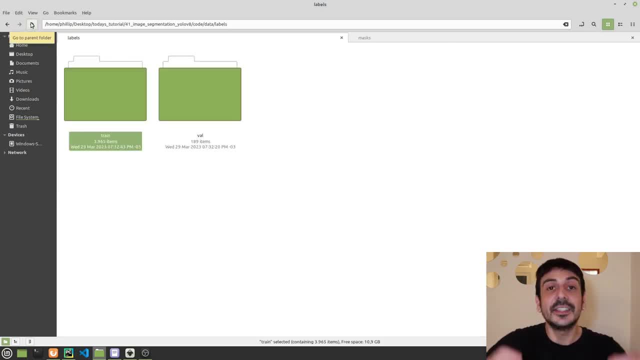 annotations: right, that's exactly the structure you need for your data. please remember to structure your file system like this, otherwise you may have an issue when you are trying to train a semantic segmentation model using yellow v8. so that's pretty much all in order. how to structure the. 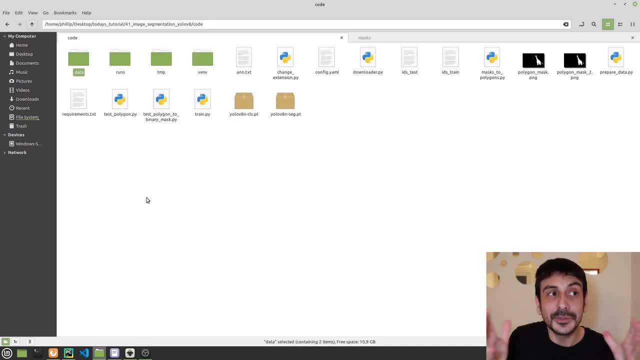 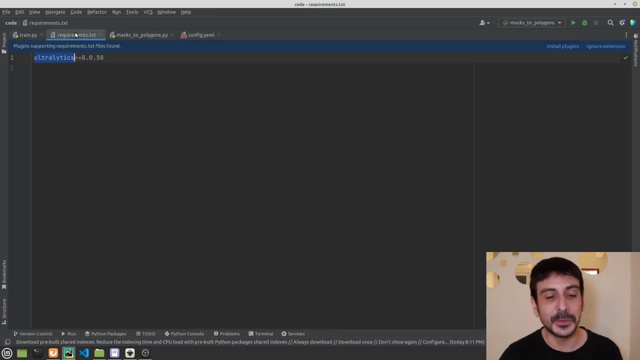 data. and now let's move to the interesting part. let's move to the most fun part, which is training this semantic segmentation model. now let's move to pycharm and i will show you how to train it from your local environment. so let's continue. this is a python project i created for today's tutorial. 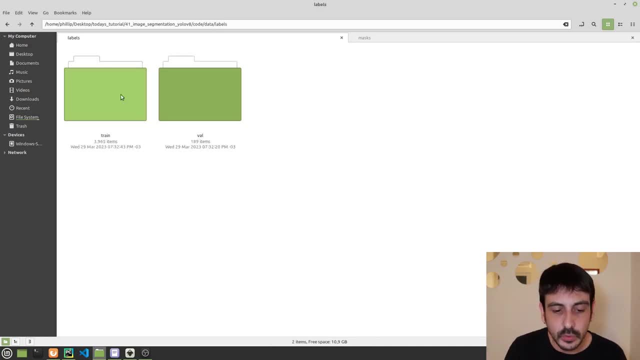 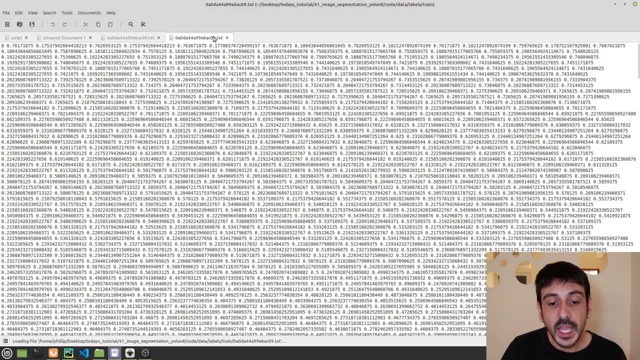 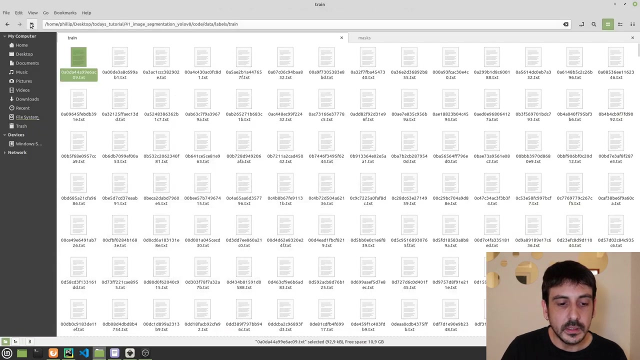 the other one is label and if i go within labels, you can see that there are two other directories also. they are named train and ball and if i open these directories, these are the type of files i have generated with the exact same script i showed you a few minutes ago. so within labels we 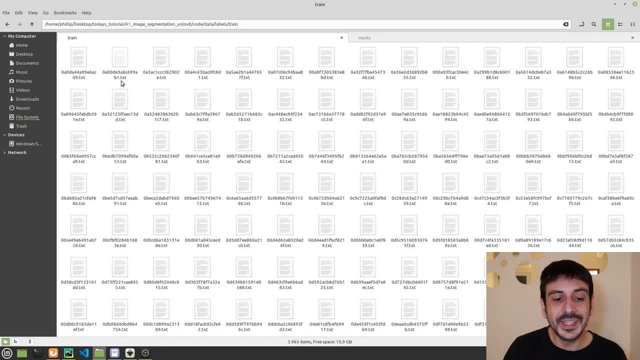 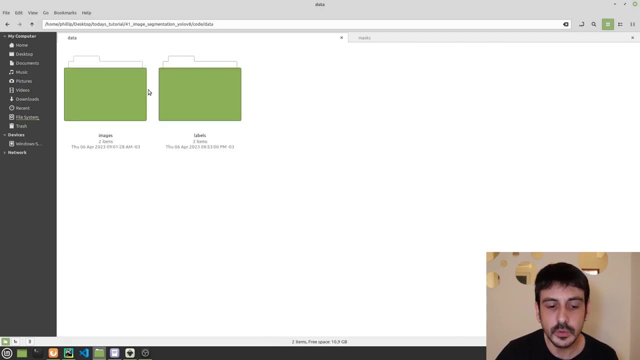 have two directories: train and ball. and train are all the annotations we have generated from the training data, from the training masks. right, a long story short. we have our root directory. within the root directory, we have two directories. one of them is called images, the other one is: 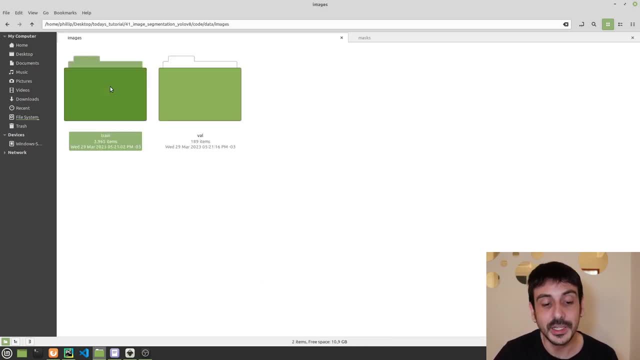 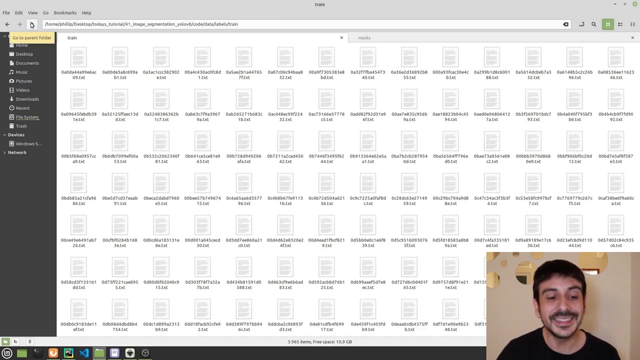 called labels within images. we have two directories: train and ball. within train and within ball. it's all of our data, all of our images and within labels. it's exactly the same structure: two directories: train and ball and within train and within ball. it's where we locate all of our annotations. right, that's exactly the structure. 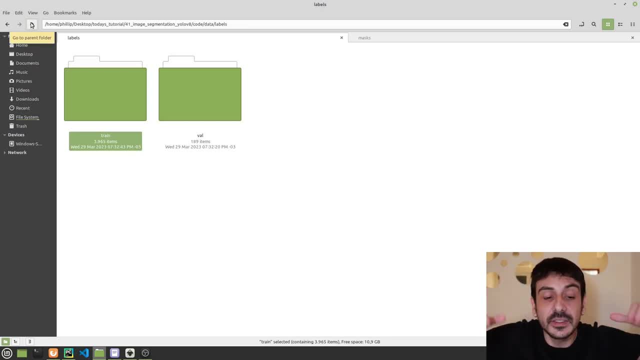 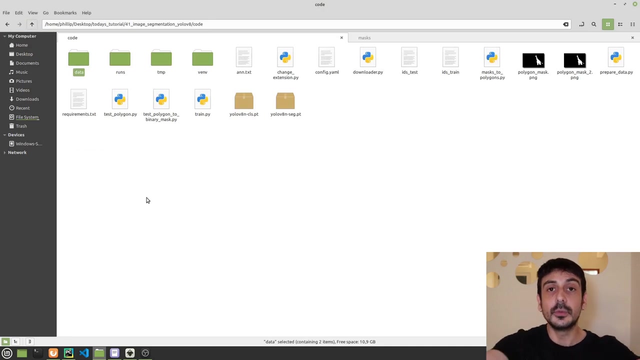 you need for your data. please remember to structure your file system like this, otherwise you may have an issue when you are trying to train a semantic segmentation model using yellow v8. so that's pretty much all in order- how to structure the data, and now let's move to the 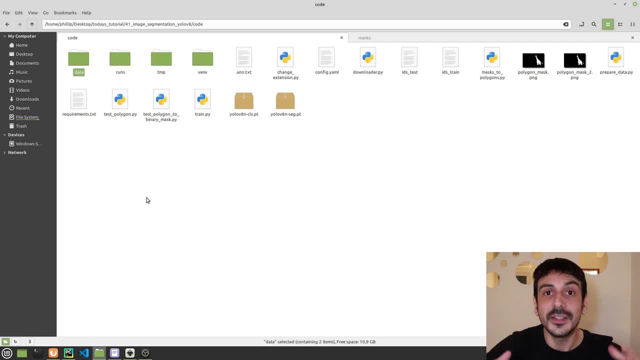 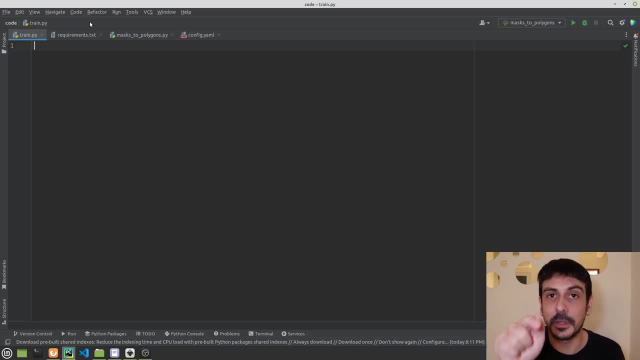 interesting part. let's move to the most fun part, which is training this semantic segmentation model. now let's move to pycharm and i will show you how to train it from your local environment. so let's continue. this is a python project i created for today's tutorial. please remember. 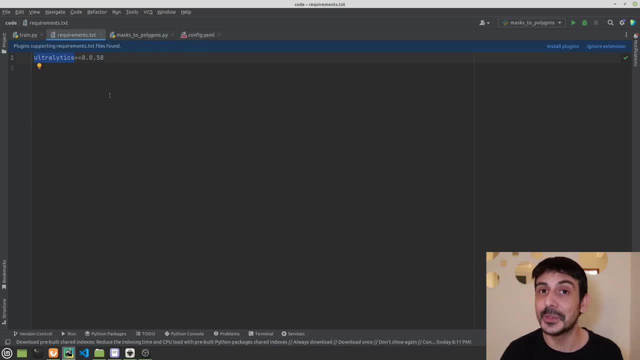 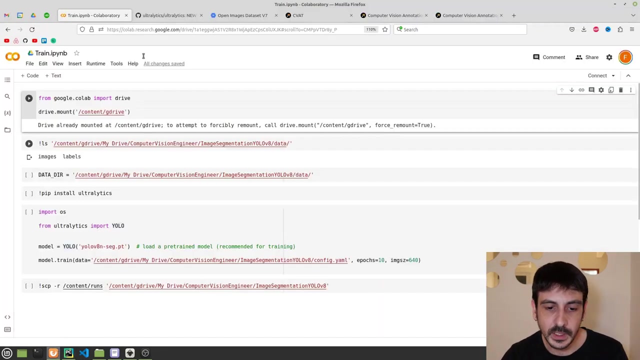 to install these project requirements, otherwise you will not be able to use yellow v8. now let's go to trainpi. this is a python estás script i created, and this is where we are going to do all the coding we need in order to train the semantic segmentation model using yolo v8. and now let's go back to the um yolo v8 official. 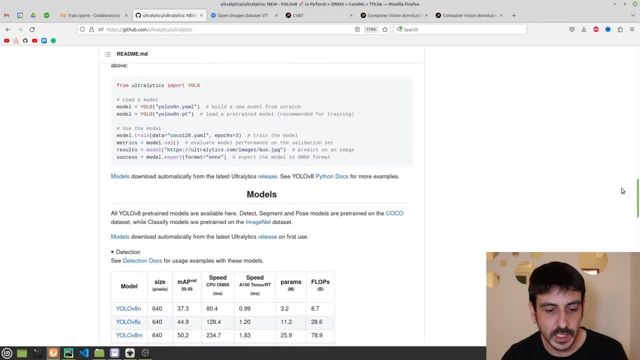 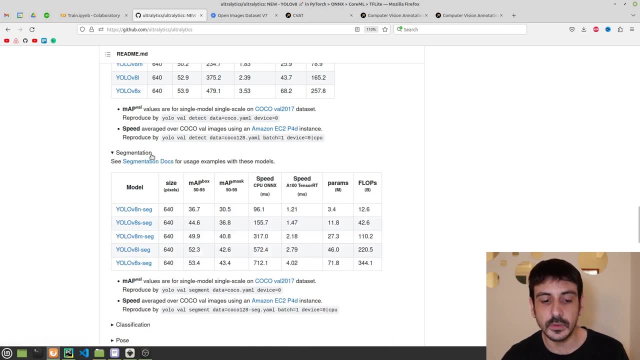 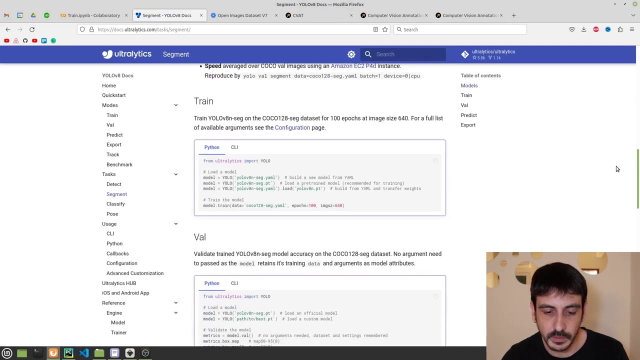 repository, because let's see how exactly we can use this yolo, this model, in order to train the semantic segmentation mode. i'm going to the segmentation section and i'm going to click on segmentation docs. now, this is going to be very, very straightforward. i'm going to train, i'm going. 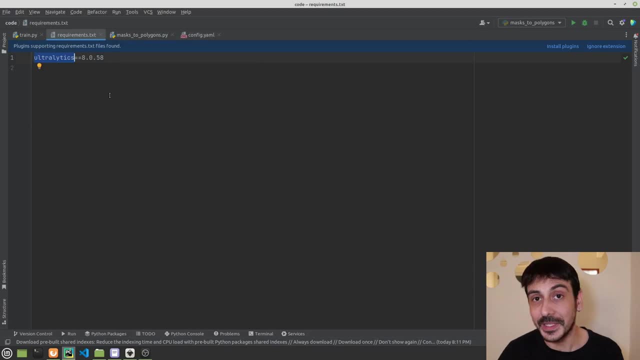 please remember to install these project requirements, otherwise you will not be able to use yellow v8.. now let's go to trainpi. this is a python script i created, and this is where we are going to do all the coding we need in order to train the semantic segmentation model using yellow v8. and now let's. 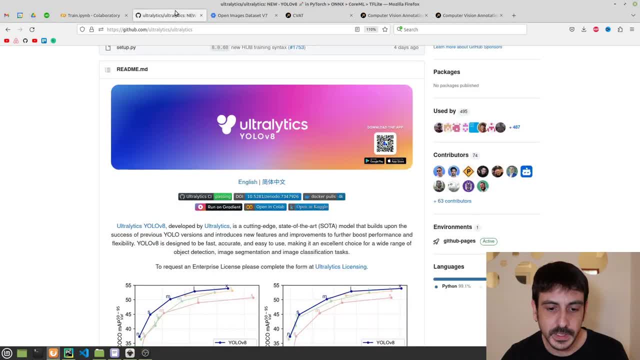 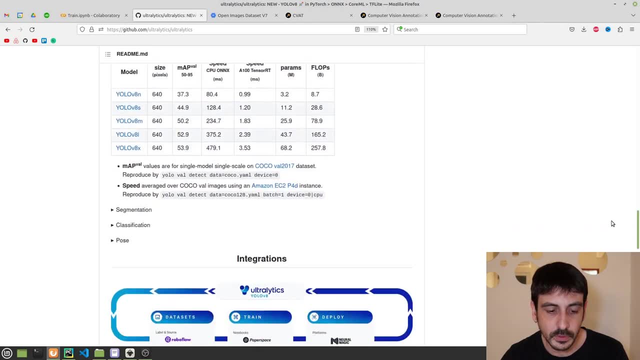 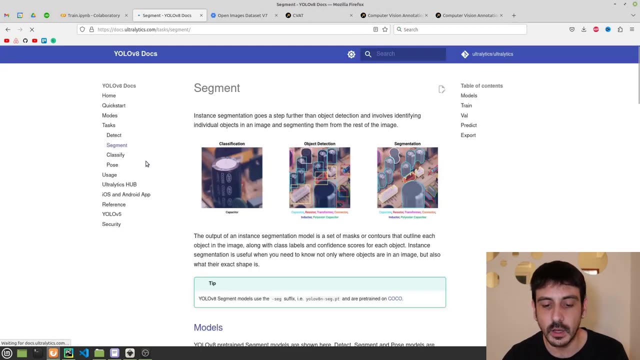 go back to the yellow v8 official repository, because let's see how exactly we can use this yolo, this model. in order to train the semantic segmentation model, i'm going to the segmentation section and i'm going to click on segmentation docs. now, this is going to be very, very straightforward. i'm going to train, i'm going to copy this. 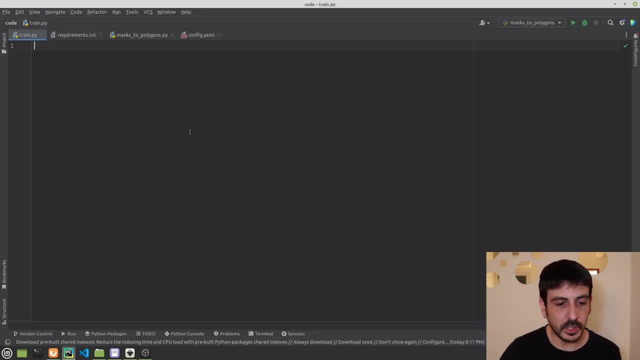 sentence which is a pre-trained model, and i'm going back to pycharm, which is going to copy paste, and then i am going to from ultralytics import yolo. then i'm also going to copy this sentence which is the modeltrain. i'm going to change the number. 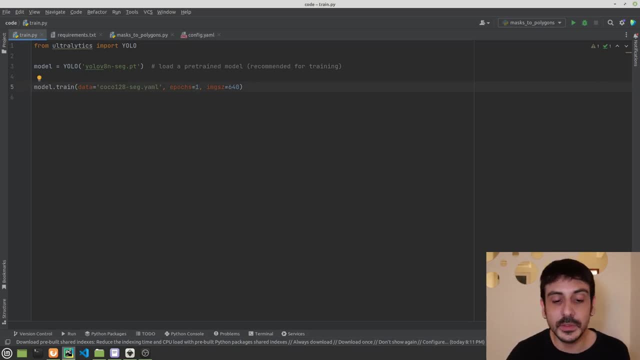 of epochs of uh to something like one, because, remember, it's always very, very healthy if you're, it's always a very good idea to do like a very dummy training, to train the model for only one epoch, to make sure everything is okay, to make sure everything runs smoothly. and then you do like a 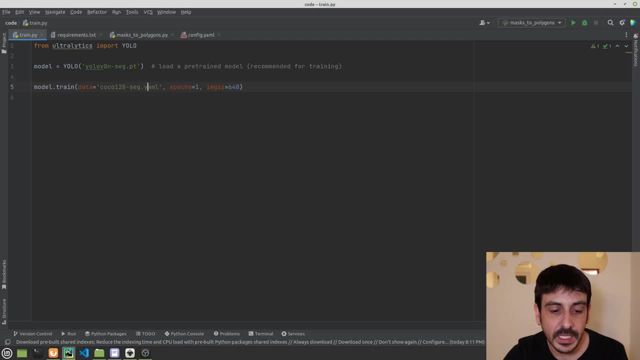 more, more deeper training. so i'm going to change the number of epochs and then i'm also going to change the config file. i'm going to use this config file, which is a config file i have over here, and obviously you will find this config file in the repository of today's video. so long story short. 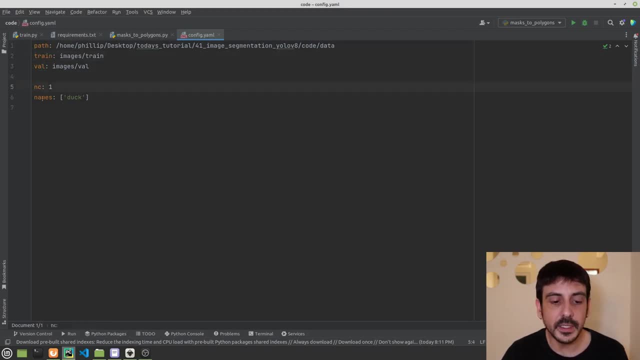 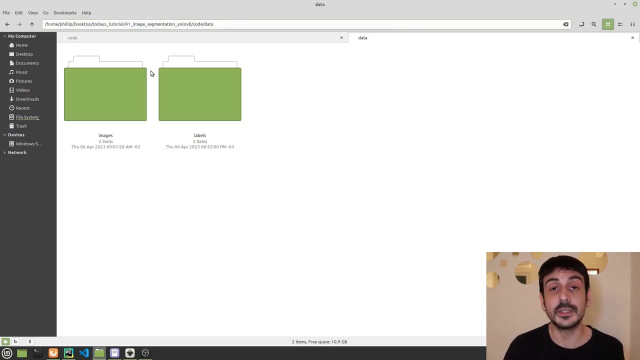 you can see that you have many, many different keywords, but the only one that you need to edit is this one, right? this is the absolute path to your data. in my case, if i copy and paste this path over here, you can see that this is the directory which contains the images and. 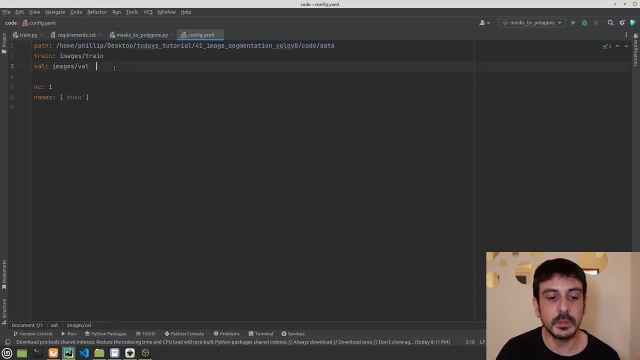 the labels, directories. so long story short, just remember to edit this path to the path to the location of your data, because if you have already structured everything in the web way i mentioned, in the way i show you in this video, then everything else will be just fine. 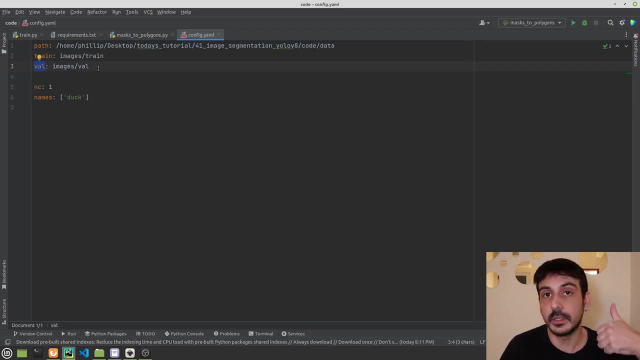 right, the train and the ball keywords are very good as it is. i mean, you can just leave everything as it is, but please remember to edit this field, which is the location of your data. now, going back to trainpi, this is pretty much all we need to do in order to train the semantic segmentation model. 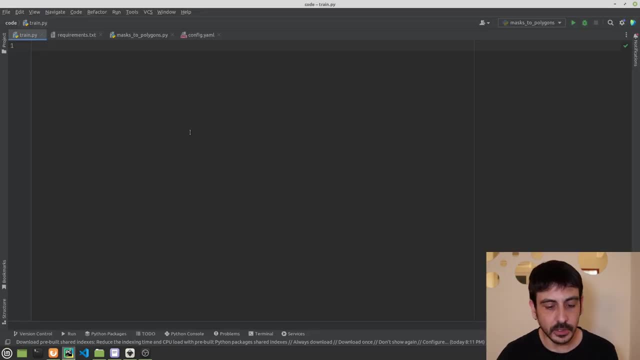 to copy this sentence which is: load a pre-trained model. and i'm going back to pycharm which is going to copy paste, and then i am going to from ultralytics import yolo. then i'm also going to copy this sentence which is the modeltrain: i'm going to change the number of epochs of. 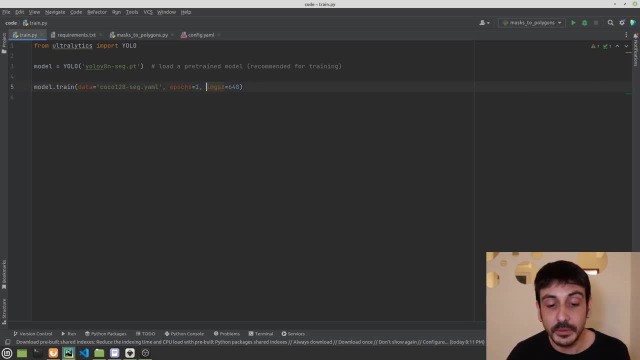 to something like one, because, remember, it's always very, very healthy. it's always a very good idea to do like a very dummy training, to train the model for only one epoch, to make sure everything is okay, to make sure everything runs smoothly. and then you do like a more, more deeper training. so i'm going to change the number of epochs. 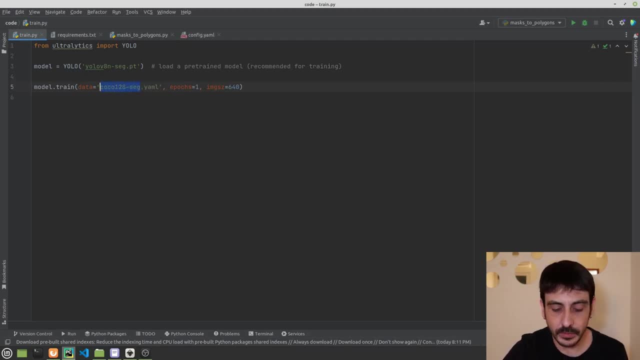 and then i'm also going to change the config file. i'm going to use this config file, which is a config file i have over here, and obviously you will find this config file in the repository of today's video. so, the long story short, you you can see that you have many, many different keywords, but the only one that you need. 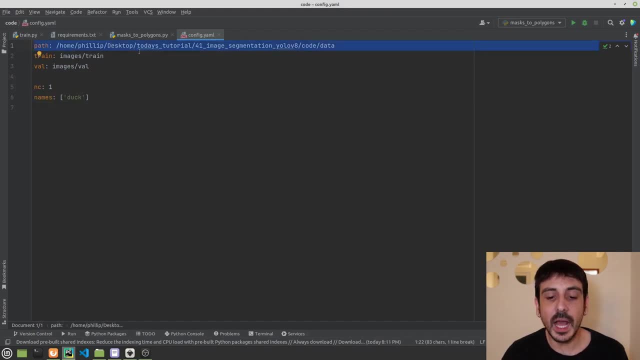 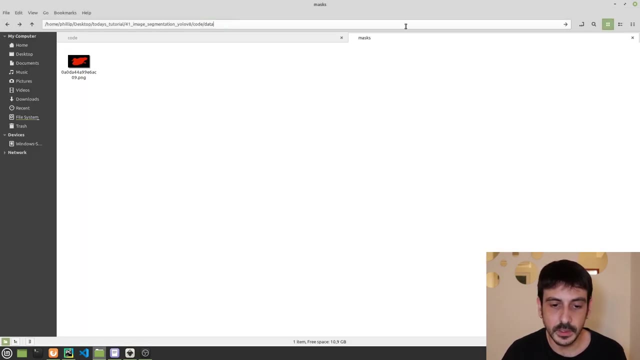 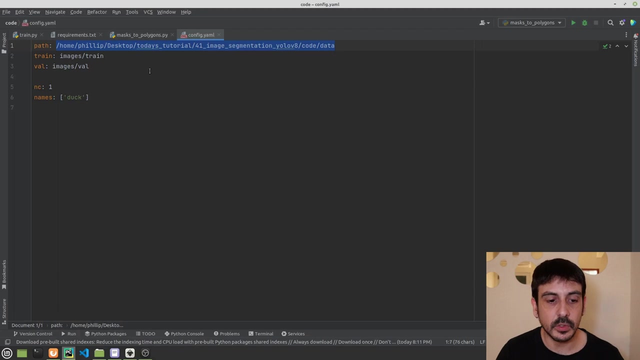 to edit. is this one right? this is the absolute path to your data. in my case, if i copy and paste this path over here, you can see that this is the, the directory which contains the images and the labels directories. so long story short, just remember to edit this path to the path to the. 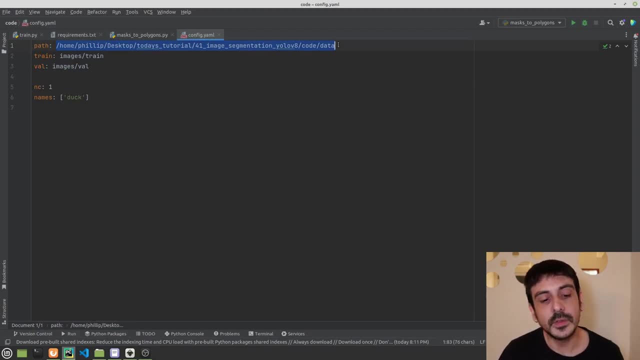 location of your data, because if you want to edit this path to the location of your data, because if you have already structured everything in the way i mentioned, in the way i show you in this video, then everything else will be just fine. right, the train and the ball. keywords are very good as it is. 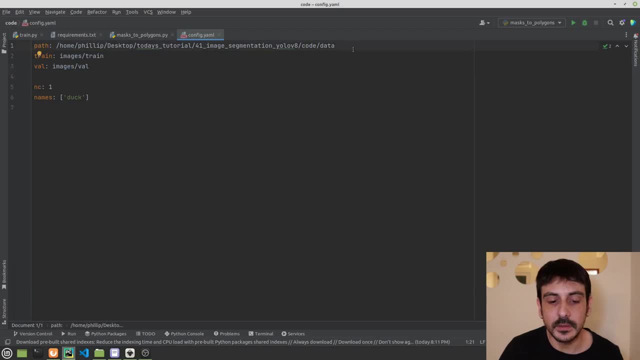 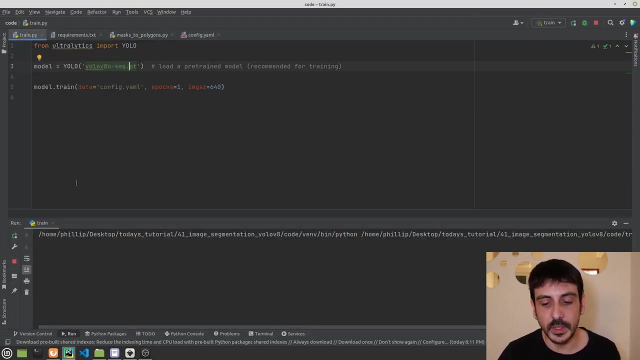 i mean, you can just leave everything as it is, but please remember to edit this field, which is the location of your data. now, going back to trainpi, this is pretty much all we need to do in order to train the semantic segmentation model, so i'm just going to press play and let's see what happens. 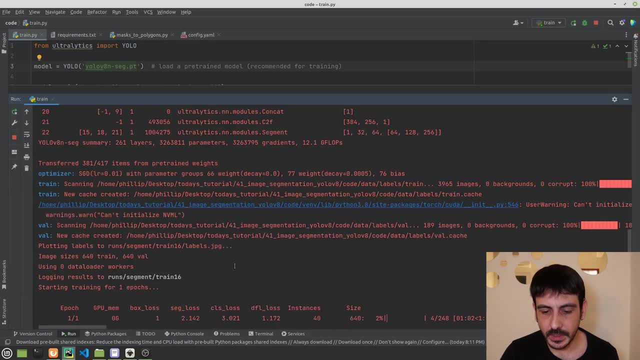 and you can see everything is going well. we are training our model, but everything is taking forever. everything is just going to take forever, even though we are only training this model for only one epoch. everything is going to take a lot of time, so what i'm going to do instead is just 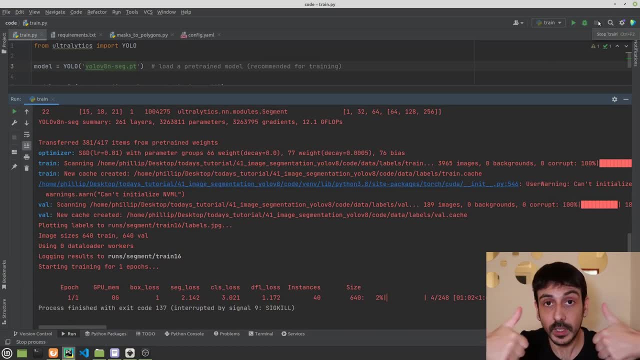 press stop. i'm going to stop this training. everything is going well. i'm not stopping this training because i had an error or something. no, everything is going well. but i am going to repeat the exactly the same process from a jupiter notebook in my google collab. 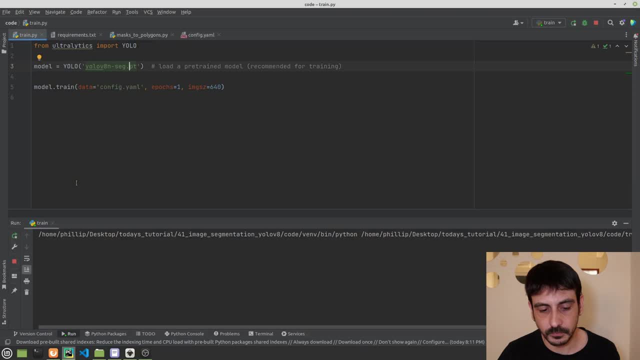 so i'm just going to press play and let's see what happens, and you can see everything is going well. so i'm just going to press play and let's see what happens, and you can see everything is going well. so i'm just going to press play and let's see what happens, and you can see everything is going well. we are training our model, but everything. 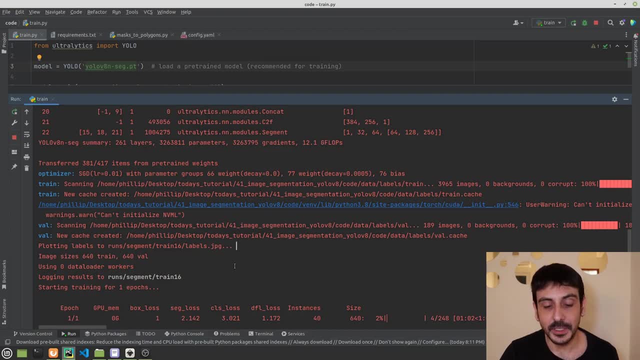 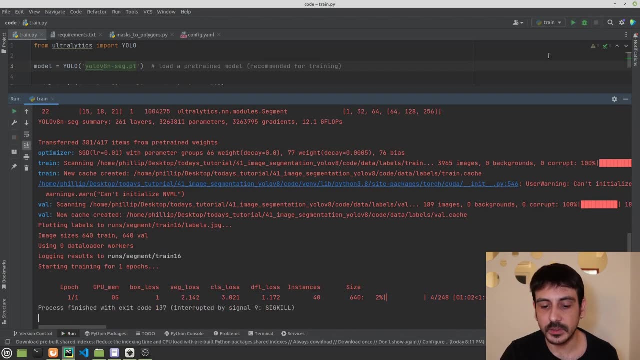 it's taking forever. everything is just going to take forever, even though we are only training this model for only one epoch. everything is going to take a lot of time, so what i'm going to do instead is just press stop. i'm going to stop this training. everything is going well. i'm not stopping. 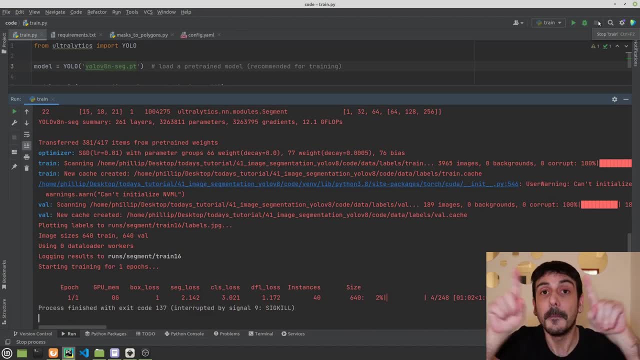 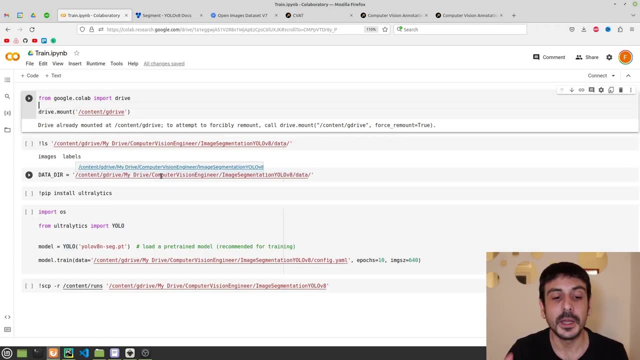 this training because i had an error or something. no, everything is going well. but i am going to repeat the exactly the same process from a jupiter notebook in my google collab, because if i use google collab, i'm going to have access to a free gpu and it's going to make the process much, much, much, much. 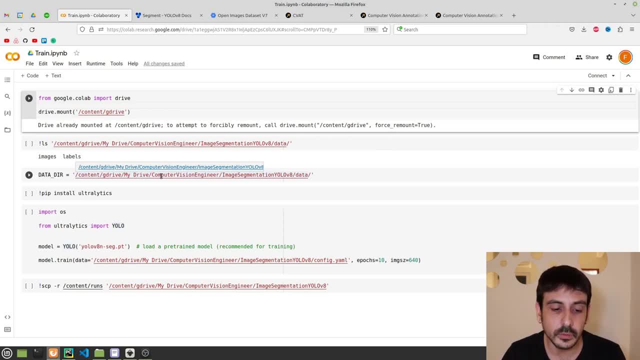 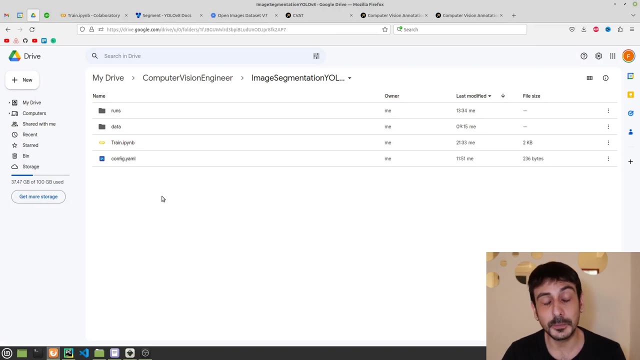 much faster. so i am going to use a google collab in order to train this model, and i recommend you to use a google collab as well, so i'm going to show you how to do it from your google collab environment. please remember to upload your data before doing anything in google collab, please. 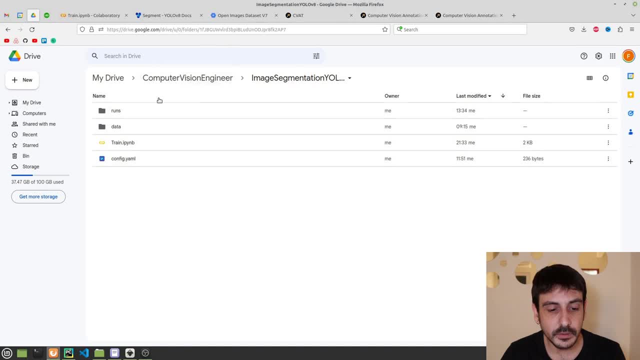 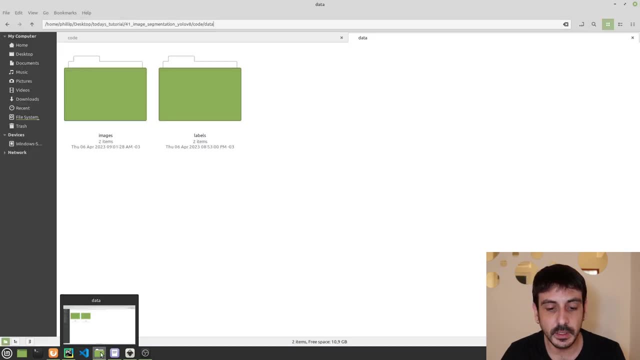 remember to upload your data, otherwise it's not going to work. for example, here you can see i have many directories when one of these directories is data and within data you have labels and images, and these are exactly the same directories they have over here. so i have already uploaded my data into my google drive. please remember to do it. 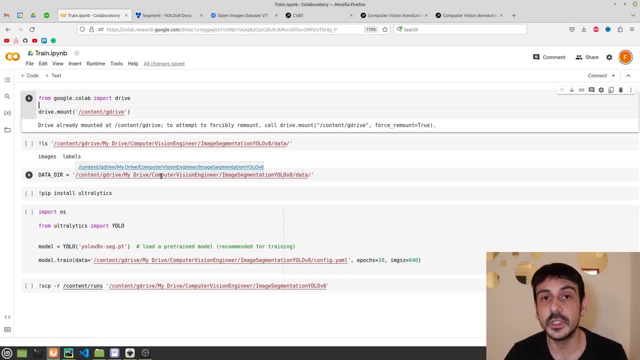 because if i use google collab, i'm going to have access to a free gpu and it's going to make the process much, much, much, much, much faster. so i am going to use a google collab in order to train this model, and i recommend you to use a google collab as well, so i'm going to show you how to do. 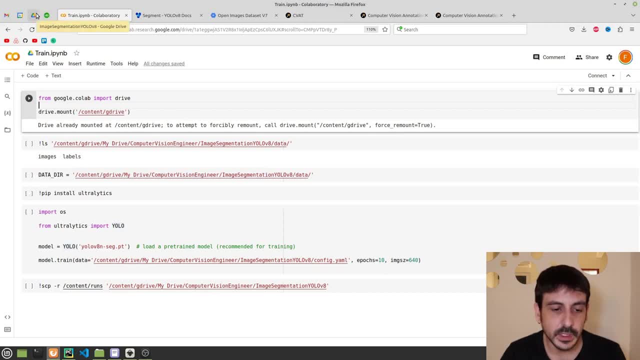 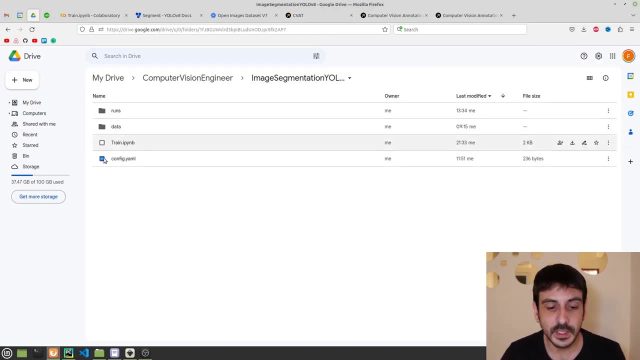 it from your google collab environment. please remember to upload your data before doing anything in google call. please remember to upload your data, otherwise it's not going to work. for example, here: one of these directories is data and within data you have labels and images, and these are exactly. 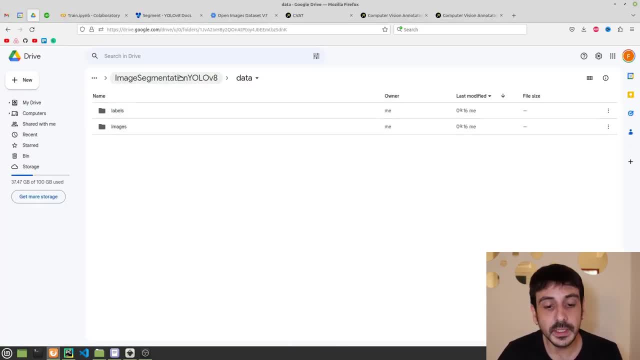 the same directories they have over here, so i have already uploaded my data into my google drive. please remember to do it too, otherwise you will not be able to do everything we're going to do just now. right? so that's one of the things you need to upload, and then also remember to upload. 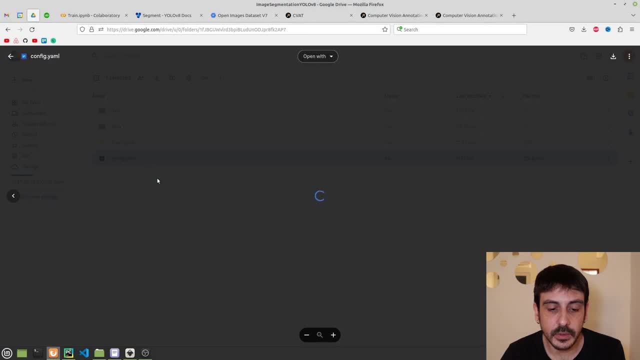 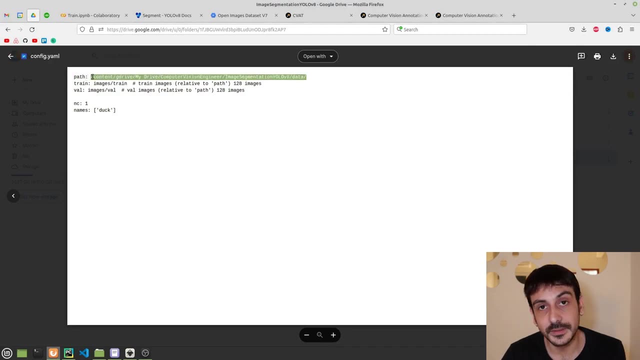 this configyaml file, the same file i show you in my local computer. you also need this file here. the will need to edit is this path, because now you need to specify the path, the location of your data in google drive. so i'm going to show you exactly how to locate your data into your google drive and 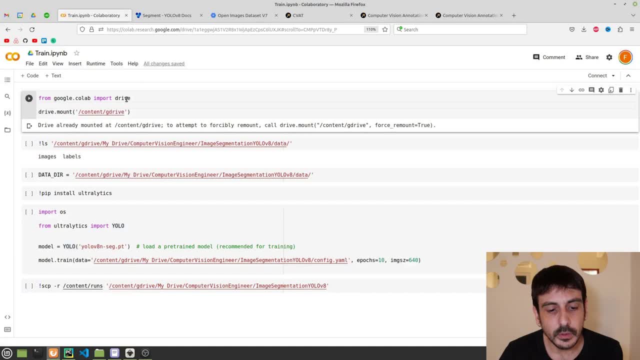 now let's move to the jupiter notebook. obviously, i'm going to give you this notebook. this is going to be in the github repository of today's tutorial, so you can just use this notebook. i'm just going to show you how to execute absolutely every single cell and how everything works right and exactly. 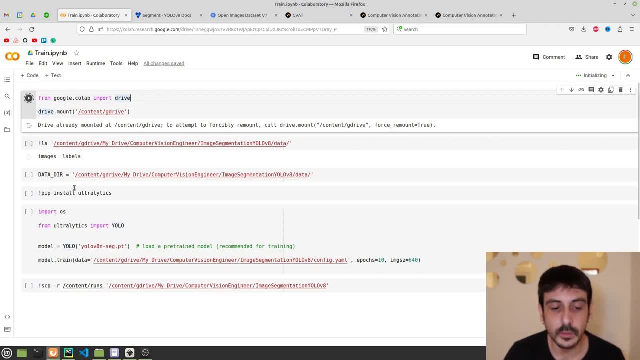 thing, exactly what everything means, right, exactly what are you doing in absolutely every single cell. so the first thing i'm doing is just connecting my google collab environment with google drive because, remember, we need to access data from google drive, so we definitely need to allow google collab to access google drive. so i'm just going to select my account and then i scroll all. 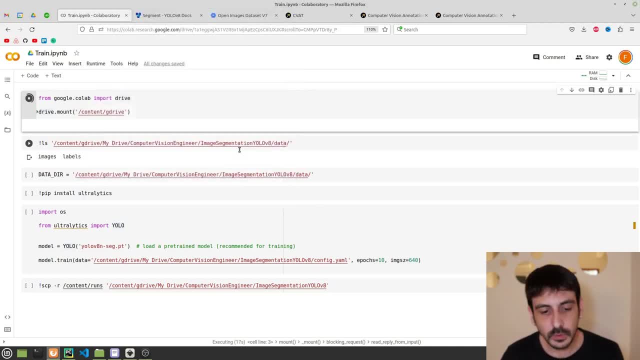 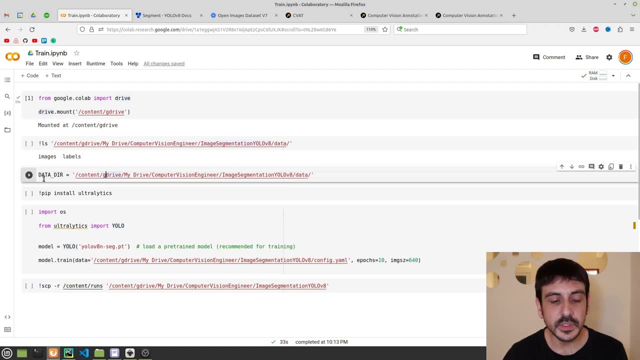 the way down and press allow. that's going to be pretty much all we need to wait a couple of seconds, and now let's continue. what i'm going to do now is to define this variable, which is data dealer, and this is the location of my data in my google drive. now, please mind this path, this. 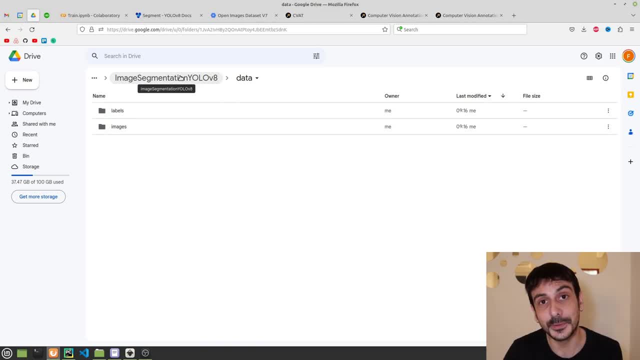 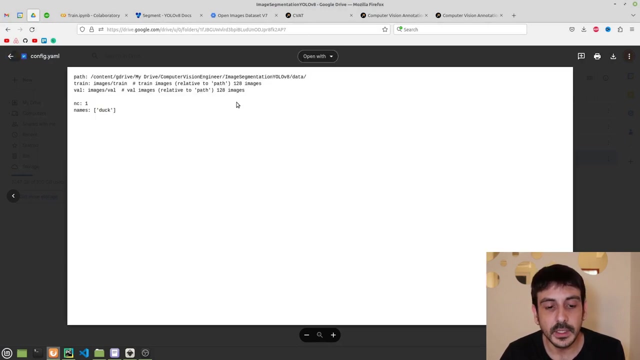 too, otherwise you will not be able to do everything we're going to do just now. right? so that's one of the things you need to upload, and then also remember to upload this configyaml file, the same file i show you in my local computer. you also need this file here, the only thing you 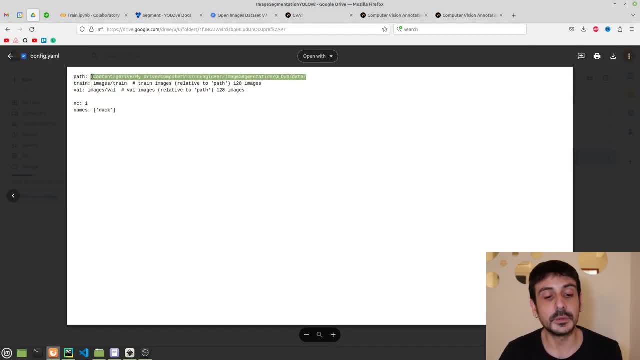 will need to edit is this configyaml file, the same file i show you in my local computer. you also need this file here. the only thing you will need to edit is this path, because now you need to specify the path, the location of your data in google drive. so i'm going. 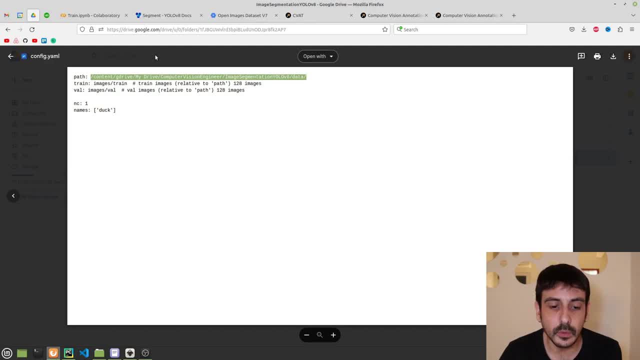 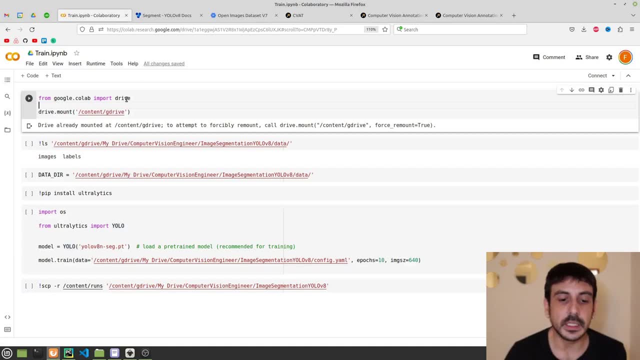 to show you exactly how to locate your data into your google drive. and now let's move to the jupyter notebook. obviously, i'm going to give you this notebook. this is going to be in the github repository of today's tutorial, so you can just use this notebook. i'm just going to show you how to. 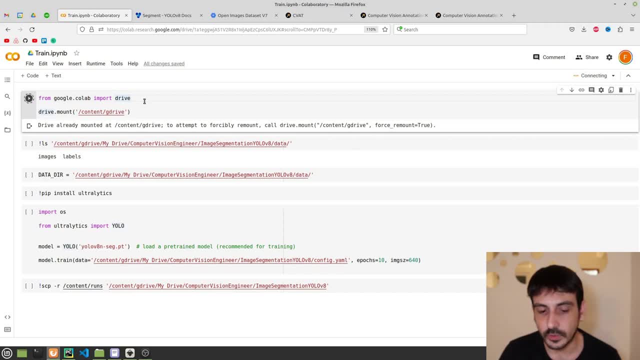 execute absolutely every single cell and how everything works right, and exactly how everything, exactly what everything means right, exactly what are you doing in absolutely every single cell. so the first thing i'm doing is just connecting my google collab environment with google drive because, remember, we need to access data from google drive, so we definitely need to allow. 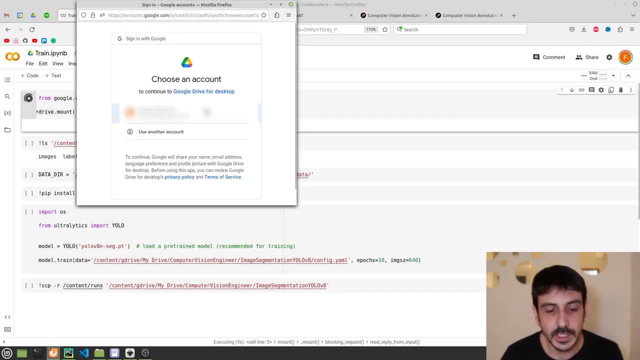 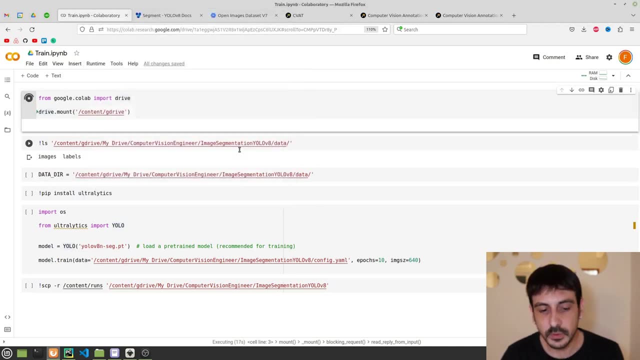 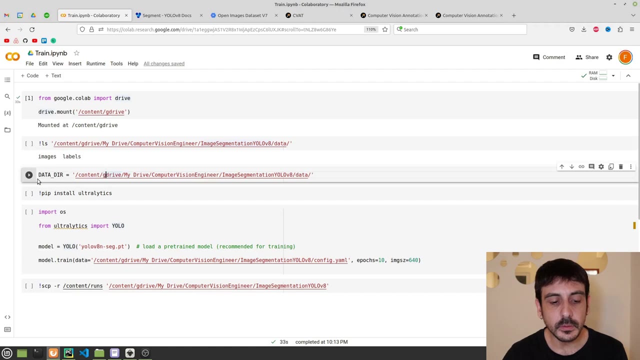 google collab to access google drive. so i'm just going to select my account and then i scroll all the way down and press allow. that's going to be pretty much all we need to wait a couple of seconds, and now let's continue. what i'm going to do now is to define this variable, which is data. 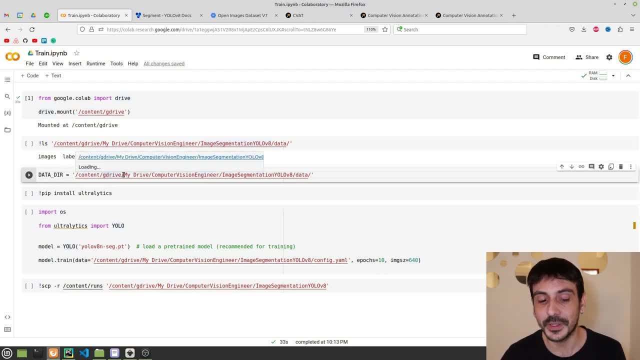 dir, and this is the location of my data in my google drive. now, please mind this path, this location, because please mind the way this is structured, right. please mind. the first word is content, then g drive, then my drive and then is my relative path to my data. 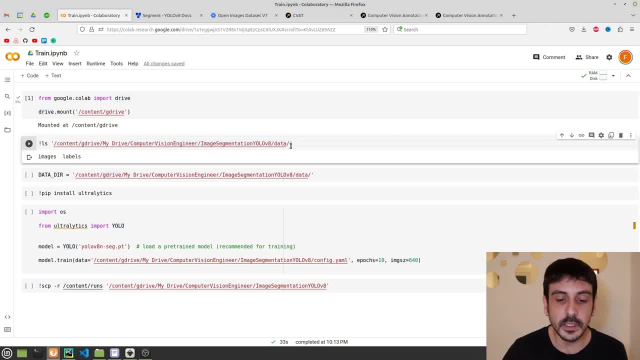 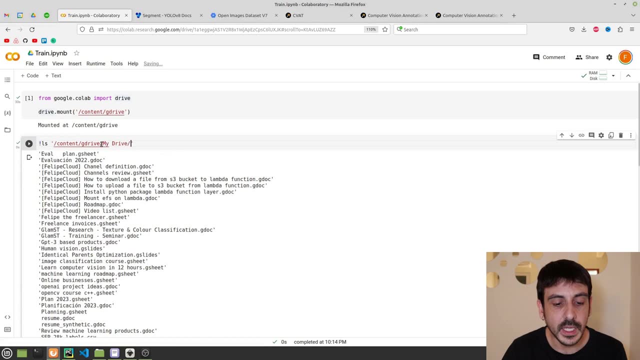 so if you want to know exactly where you have uploaded your data, if you're not completely sure where you have uploaded your data, what you can do is to do an ls, like i'm doing right now, and this is going to give you all the files you have in the root directory of your google drive. 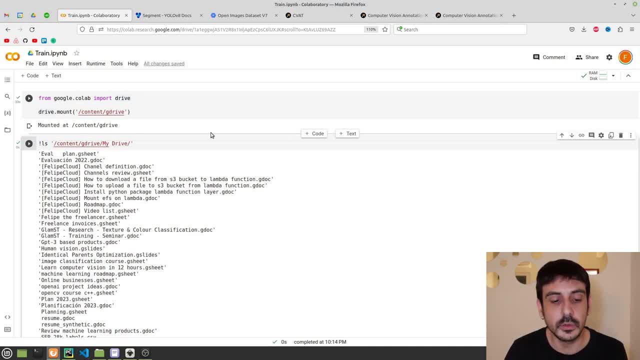 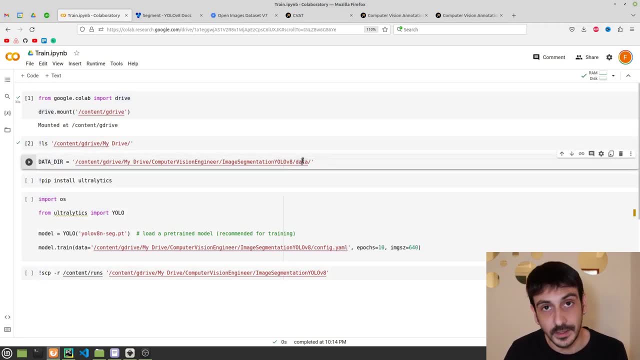 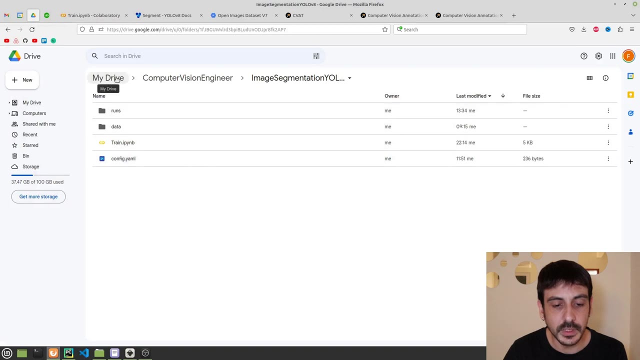 then from there, just navigate until the directory where you have uploaded your data. in my case is my drive- computer vision, engineer, image segmentation- yellow v8- and then data. that's exactly where my data is located in google drive. if i go to this directory, you can see that this is my drive. 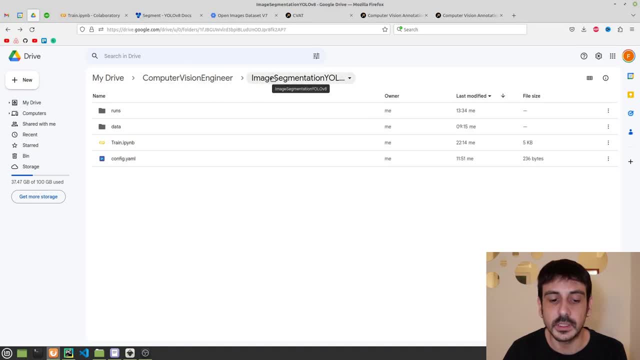 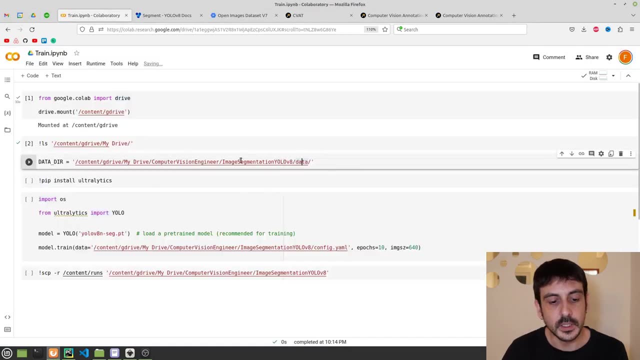 you can see that this is my drive- then computer vision, engineer image segmentation- yellow v8- and then data, and this is exactly what i have over here. so, once you have located your data, the only thing you need to do is to edit this cell and to press enter. so everything is ready. 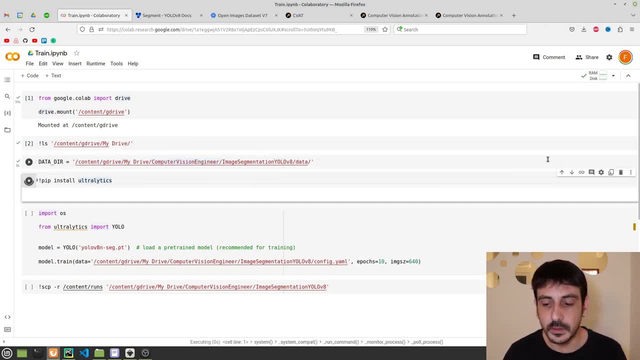 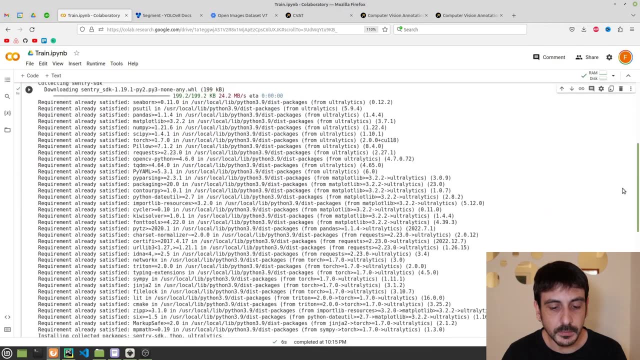 now i'm going to install ultralytics so i can use yellow v8 from the notebook, and this is going to take a few seconds, but this is going to be ready. no time or something you need to do from your google collab is to go to runtime and change. 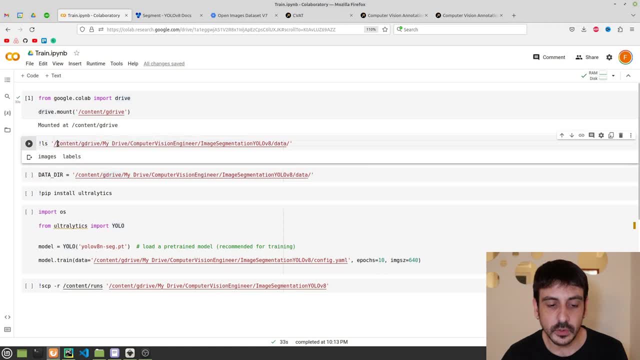 location, because please mind the way this is structured, right, please mind. the first word is content, then g drive, then my drive and then is my relative path to my data. so if you want to know exactly where you have uploaded your data, if you're not completely familiar with the data you 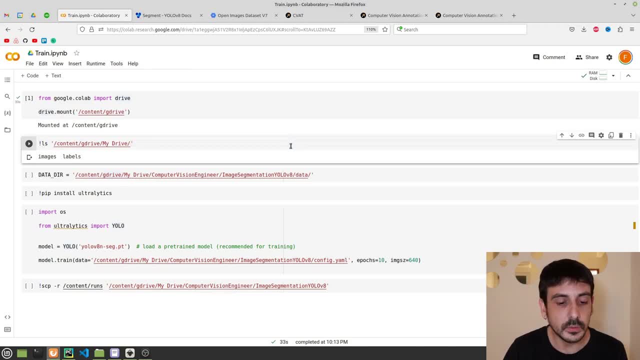 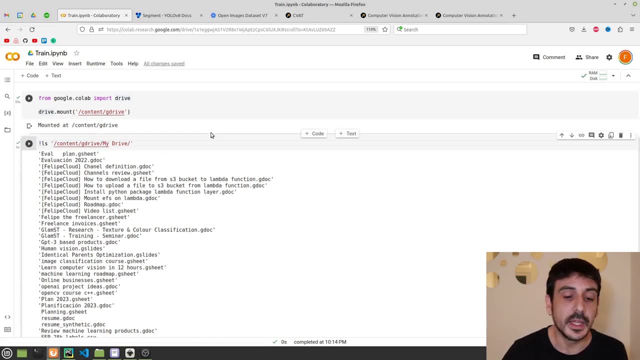 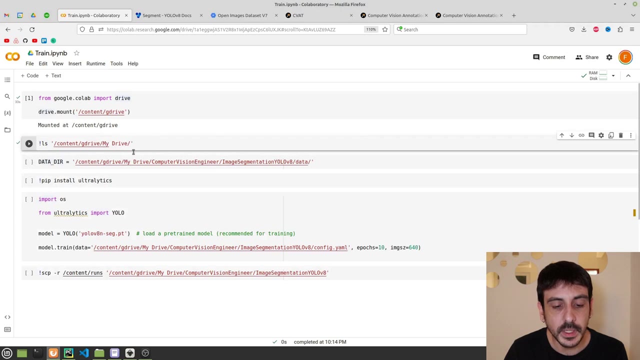 have uploaded your data. what you can do is to do an ls, like i'm doing right now, and it is going to give you all the files you have in the root directory of your google drive. then, from there, just navigate until the directory where you have uploaded your data- in my case is my drive. 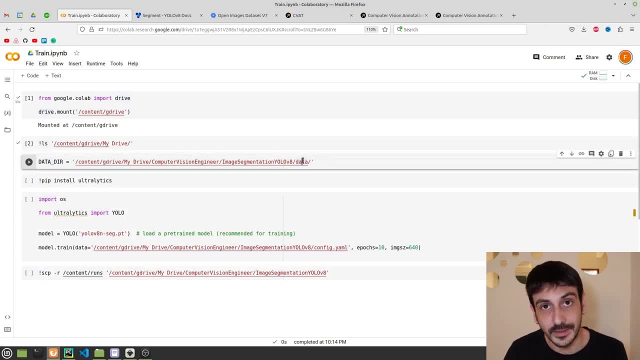 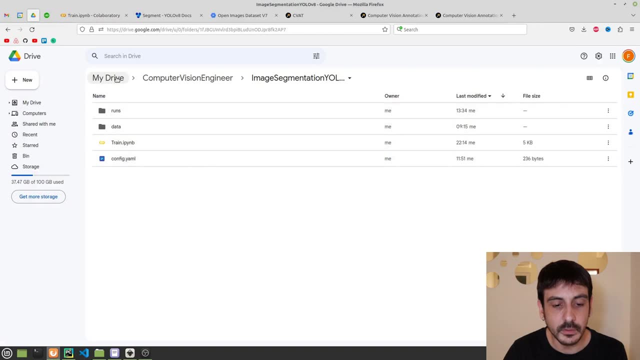 computer vision engineer image segmentation- yellow v8- and then data. that's exactly where my data is located in google drive. if i go to this directory, you can see that this is my drive, then computer vision engineer image segmentation- yellow v8. and then data, and this is exactly what i. 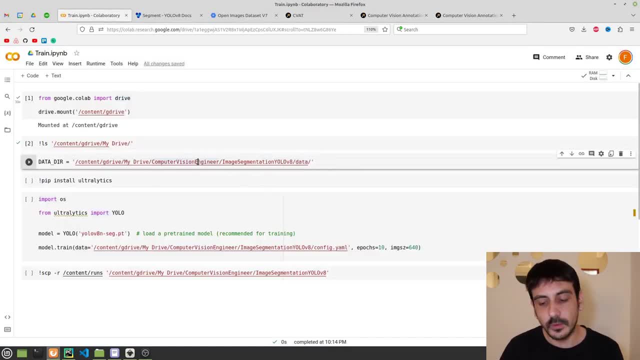 have over here. so once you have located your data, the only thing you need to do is to edit this cell and to press enter, so everything is ready. now i'm going to install ultralytics so i can use ulo v8 from the notebook, and this is going to take a few seconds, but this is going to be. 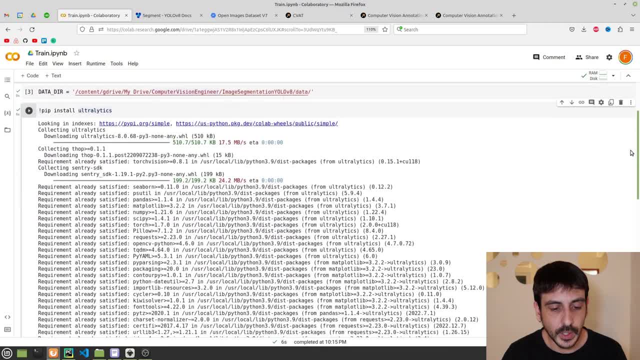 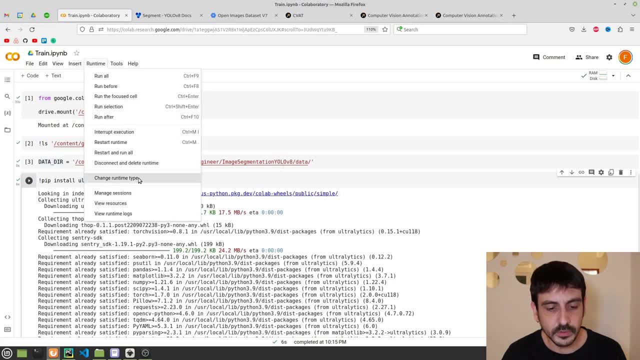 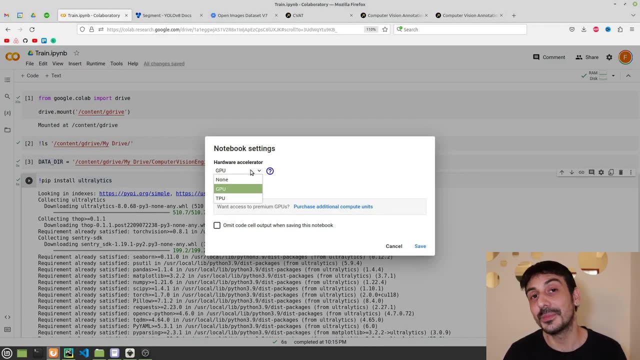 ready in just a few moments, in no time or something you need to do from your google collab is to go to runtime and change runtime type. just make sure it says gpu. just make sure you are using a google collab with gpu, because if you are not using a google collab with gpu, everything is pretty much pointless right. 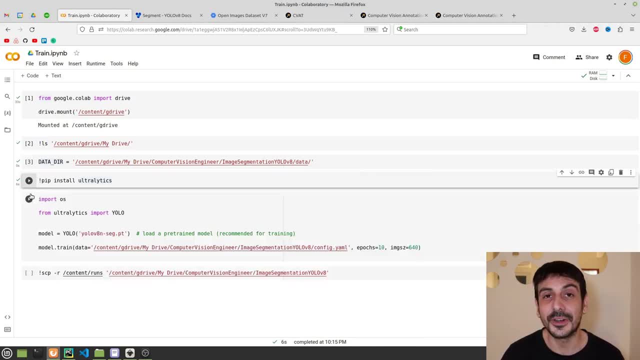 so just remember to to check if you are using a google collab with gpu or not. just do it before you start all this process, because otherwise you will need to to run absolutely everything again. so let's continue. i have already installed the ultralytics and now i am going to run this. 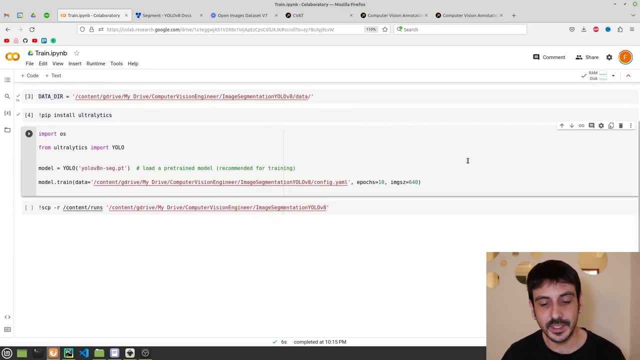 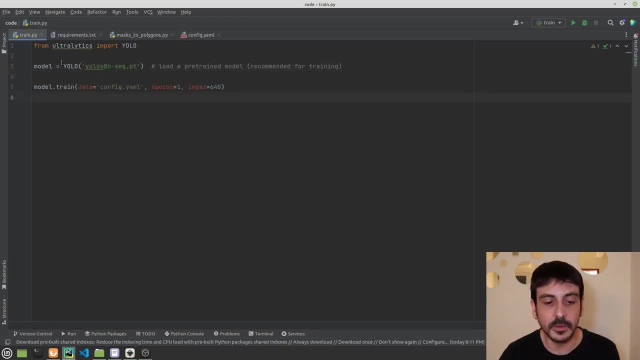 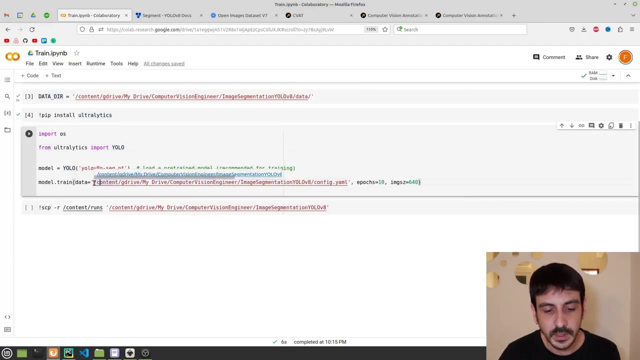 cell and, if you realize, this is exactly, exactly the same type of information, the same code i have over here in my local environment. right, i'm just defining the model and then i am just training this model. so what i need to do now is just press enter and also mind that i have specified. 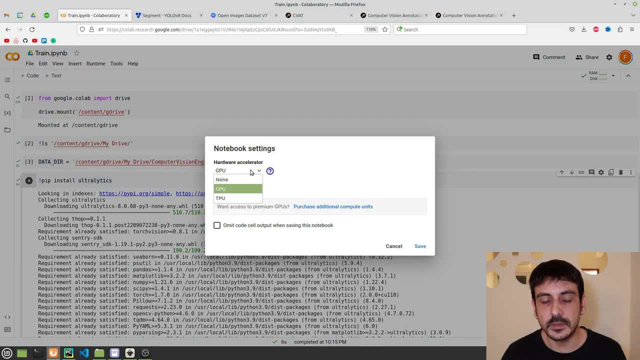 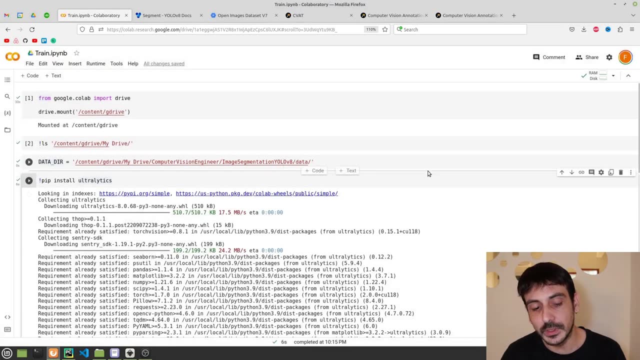 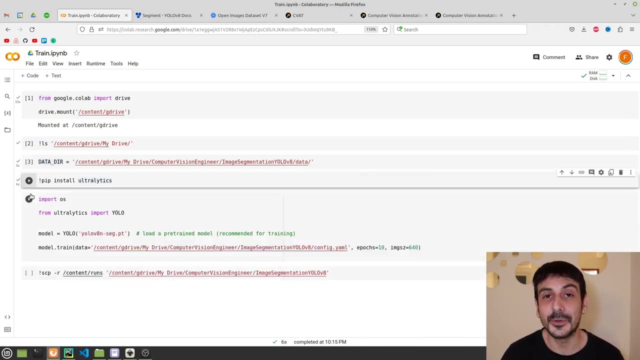 runtime type. just make sure it says gpu. just make sure you are using a google collab with gpu, because if you are not using a google collab with gpu, everything is pretty much pointless, right? so just remember to uh to check if you are using a google collab with gpu or not. just do it before you start. 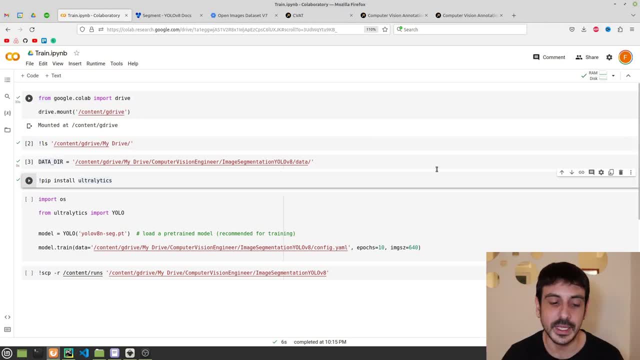 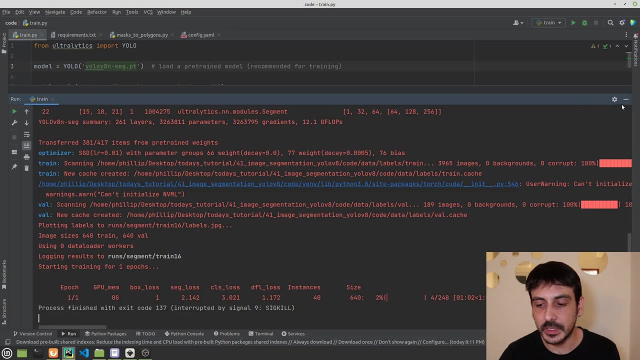 process, because otherwise you will need to to run absolutely everything again. so let's continue. i have already installed the ultralytics and now i am going to run this cell and, if you realize, this is exactly exactly the same type of information, the same code i have over here. 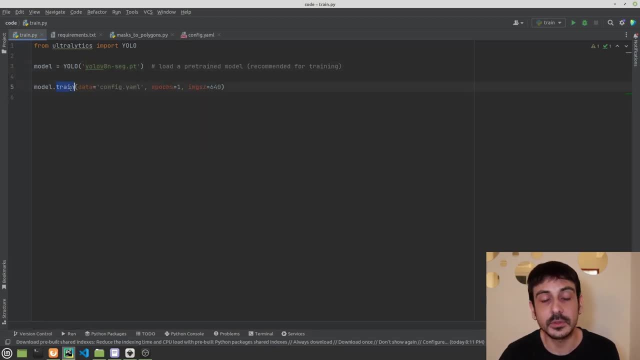 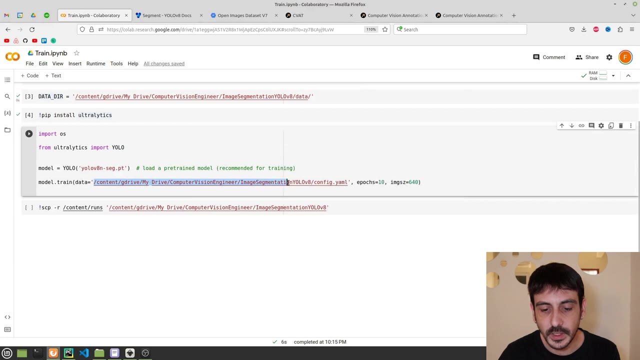 in my local environment. right, i'm just defining the model and then i am just training this model. so what i need to do now is just press enter and also mind that i have specified the config file right, the location of my config file, and now i'm going to run a full training, or actually i'm going 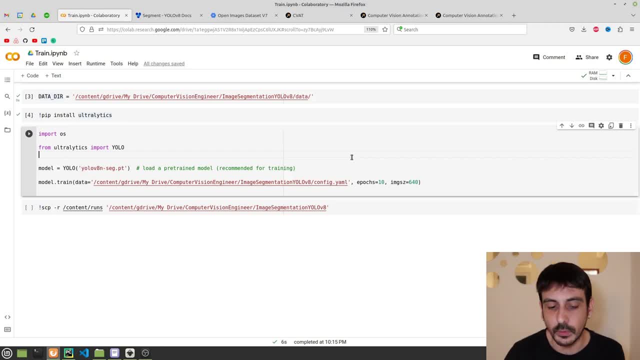 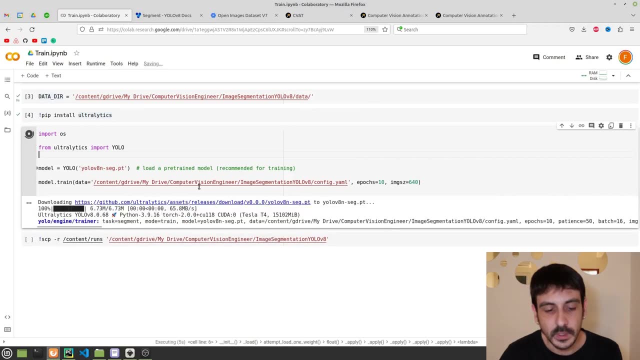 to run a training for 10 epochs. so this is what i'm going to do, and this is also going to take some time. although we are going to use a gpu, this is going to take a few minutes as well. so what i'm going to do now is just i'm going to wait until this is completed and i'm going to 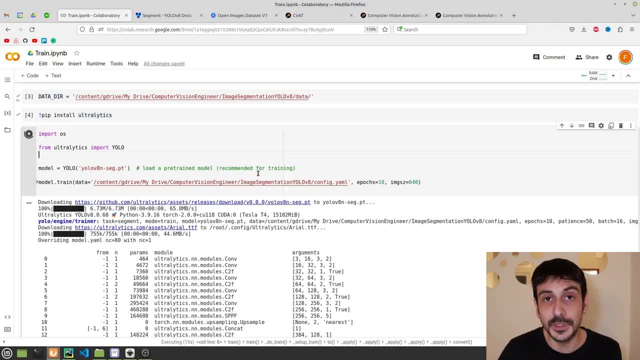 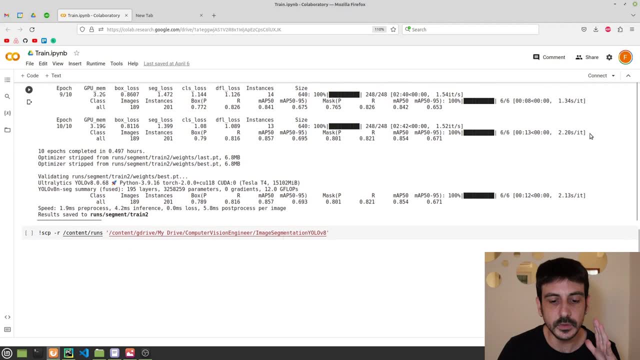 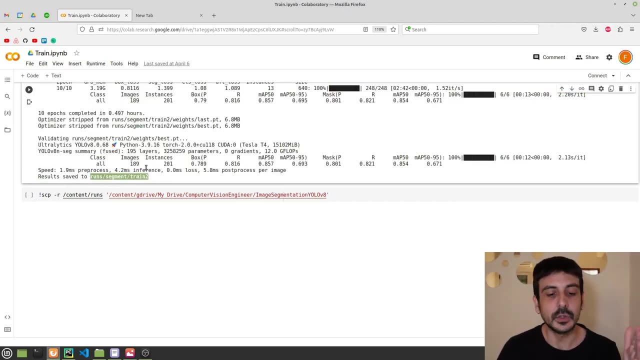 post my recording here, and i'm just going to fast forward this video until this process is completed. okay, so the training process is now completed. we have trained this model and everything is just fine, and you can see the results have been saved here under runs segment and train 2.. so the only thing we need to do now is to get the results. we 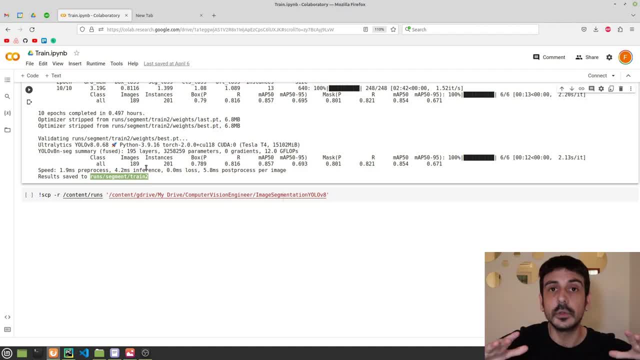 got from this training. we need to get the weights, we need to get all the results, all the different metrics, all the different plots, because what we need to do now is to analyze this training process. we need to validate that everything is just fine, right. so what we are going to do now is to get all 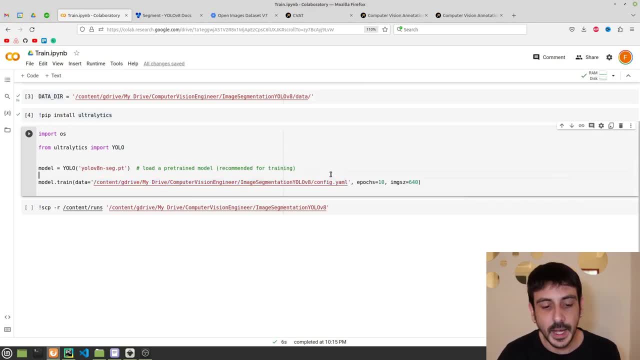 the config file, right, the location of my config file, and now i'm going to run a full training, or actually, i'm going to run a training for 10 epochs. so this is what i'm going to do, and this is also going to take some time. although we are going to use a gpu, this is going to take a few minutes, as 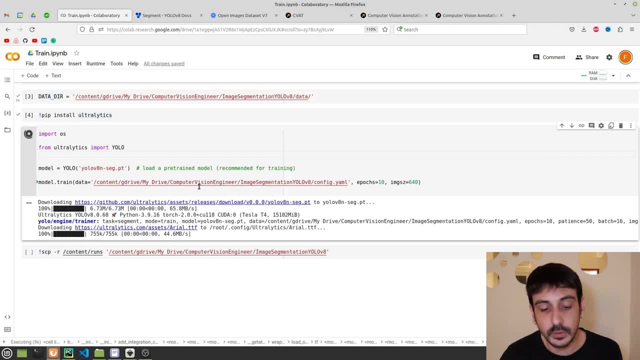 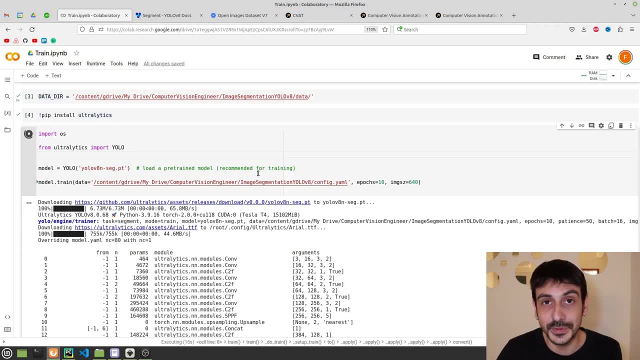 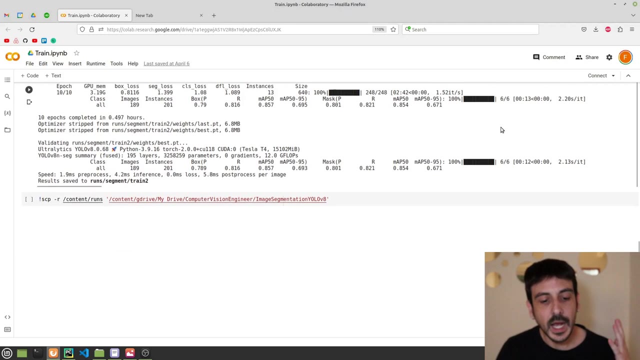 well. so what i'm going to do now is just i'm going to wait until this is completed and i'm going to pause my recording here and i'm just going to fast forward this video until this process is completed. we have trained this mod and everything is just fine and you can see the results have been saved. 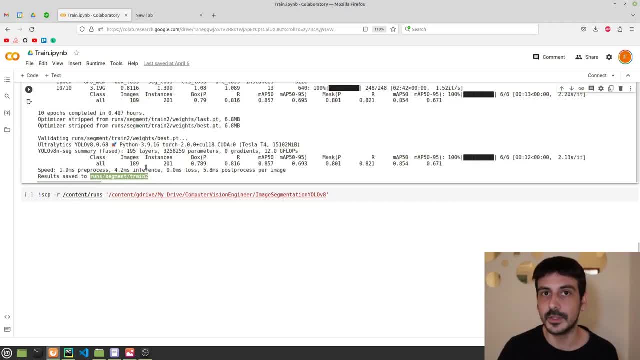 here and the runs segment and train too. so the only thing we need to do now is to get the results we got from this training. we need to get the weights, we need to get all the results, all the different metrics, all the different plots, because what we need to do now is to analyze this training. 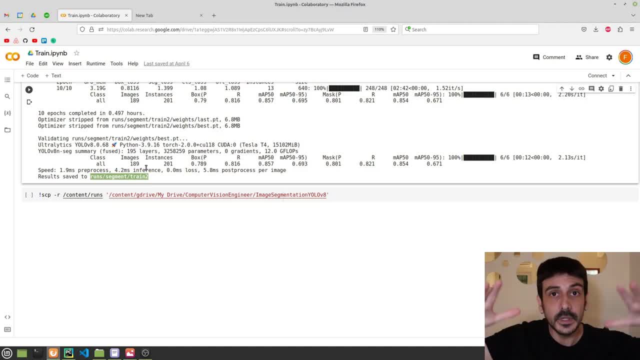 process. we need to validate that everything is just fine right. so what we are going to do now is to get all the results from the training that we have received this information, and the easiest way to do it is just running this command. what we will do when? 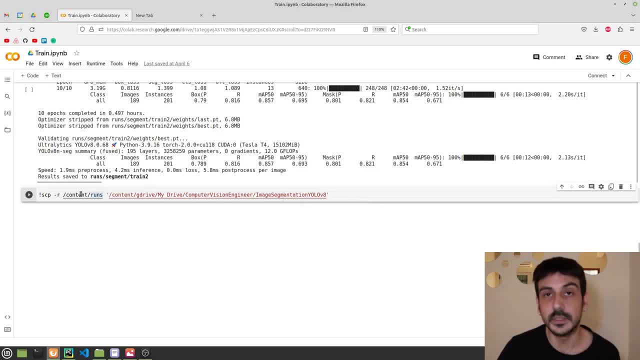 running this command, we are going to copy all the content in this directory, where it's the, where the results have been saved under our google drive. right, remember to edit this url, remember to edit this path, this location, because you want to copy everything into a directory, into your google. 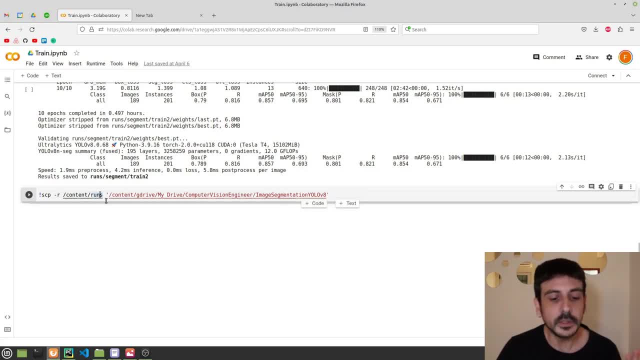 the results, and the easiest way to do it is just running this command. what we will do when running this command? we are going to copy all the content in this directory, where it's the, where the results have been saved under our google drive, right? remember to edit this url. remember to edit this. 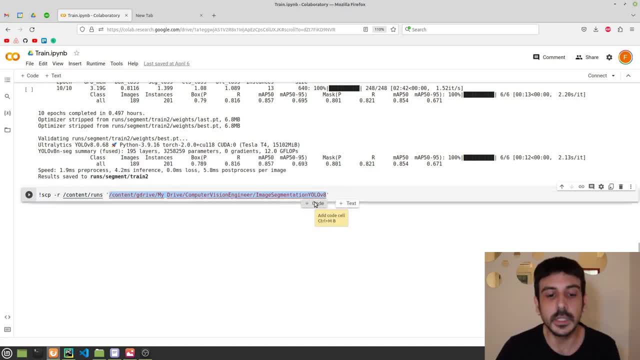 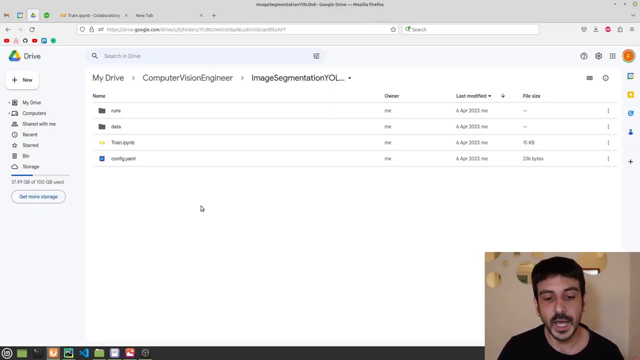 path this location because you want to copy everything into a directory, into your google drive. so just make sure everything is okay, make sure this location makes sense. you can just execute this cell and you're going to copy everything into your google drive. now let me show you my google drive. i have already executed this cell, so everything it's under my 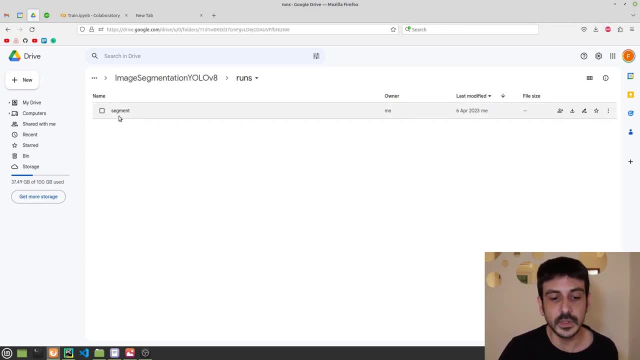 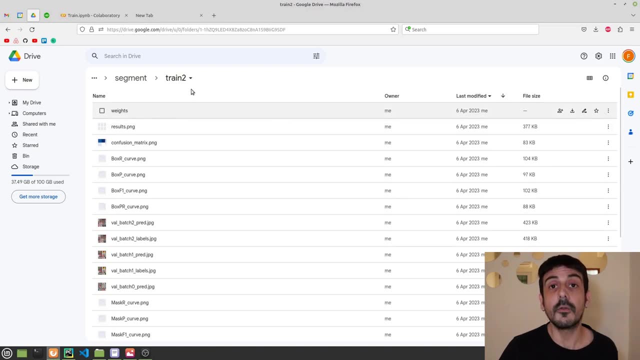 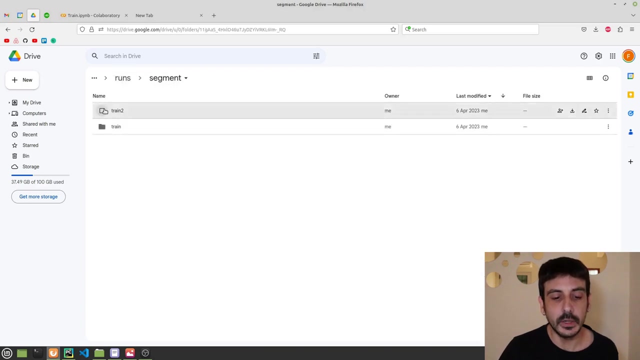 google drive. this runs directory which was created when i run that cell and under this other directory, which which is called segment, we have trained you. so these are all of our results. these are the results we are now going to analyze. so what i'm going to do now is just to download this. 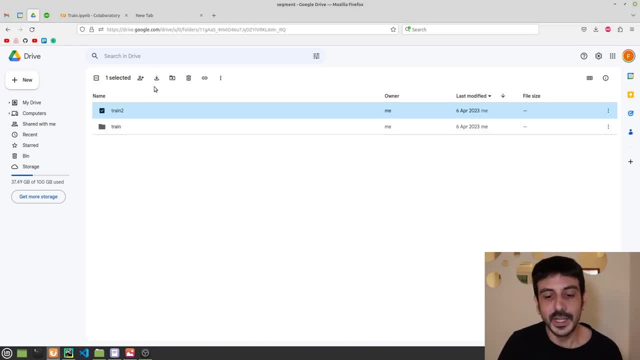 and once we have this directory into our local computer, then we are going to take a look at all the plots, at all the metrics, and i'm going to tell you exactly what i usually do in order to validate this training process. so everything is now downloaded, everything is now completed, and 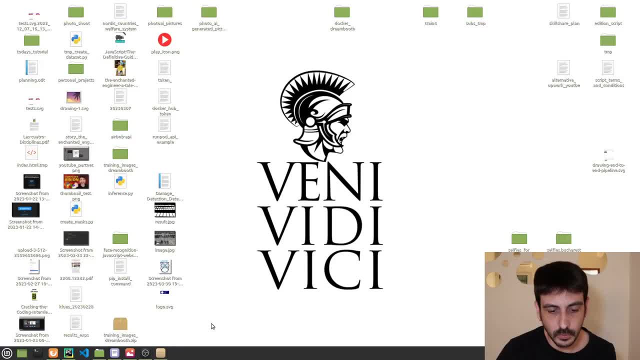 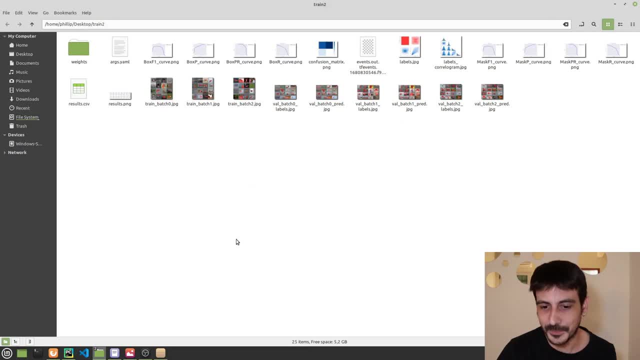 let's take a look at these files. so what i'm going to do is i'm just going to copy everything into my desktop. i need to do some cleaning, by the way. so the these are all the results we got from this training process. you can see that this is 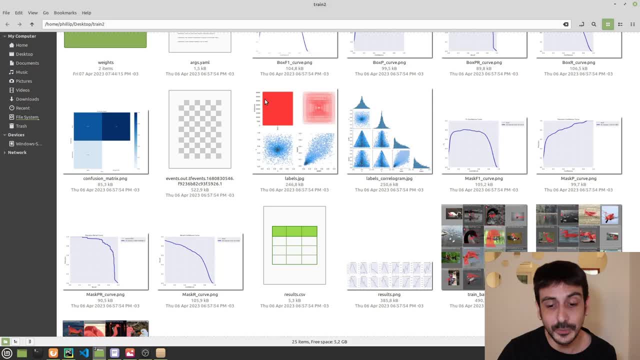 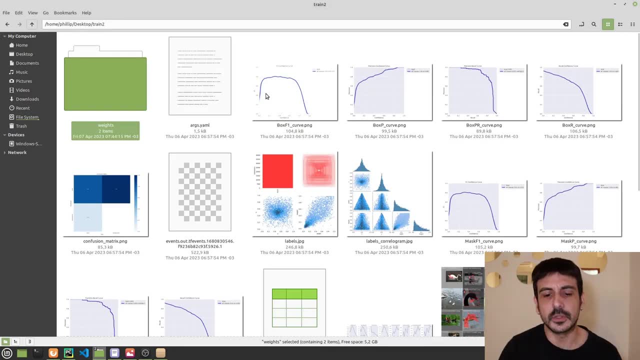 a lot of information. this is definitely a lot of information. right, we have many, many different files. we have many different everything. we have the weights over here. we have a lot of information. so let me tell you, let me give you my recommendation about how to do this evaluation, how. 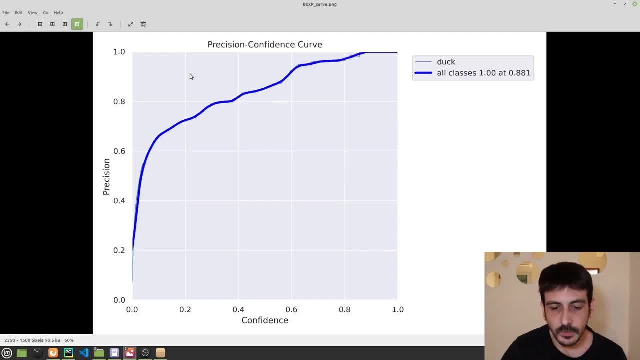 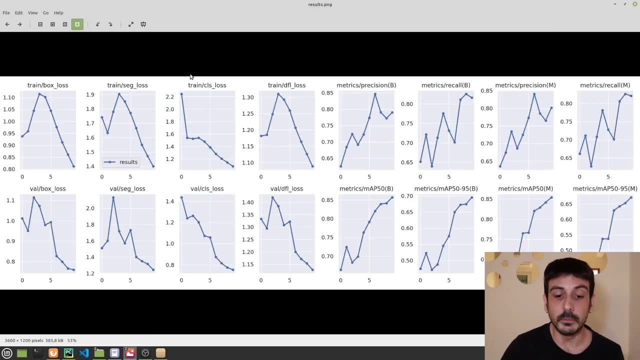 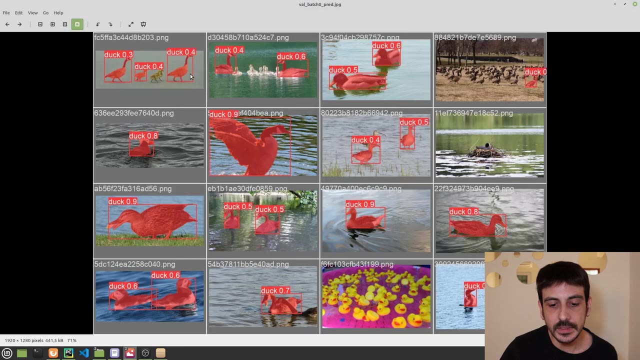 to do this validation from all these plots and from all of these results. i will recommend you to focus on choosing. one of them is this plot, one of the one of them is all of these metrics, and then i'm also going to show you how to take a look at these results, at these predictions from these images. but for now, 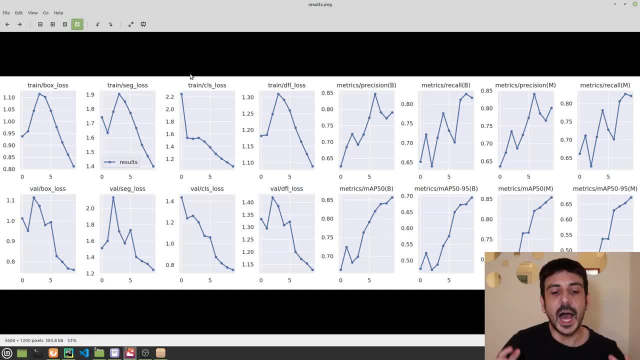 let's start here. you can see that this is a lot of information. these are a lot of metrics and you can definitely knock yourself out analyzing all the information you have here. you can definitely go crazy analyzing all of this information, all of these metrics and all of the 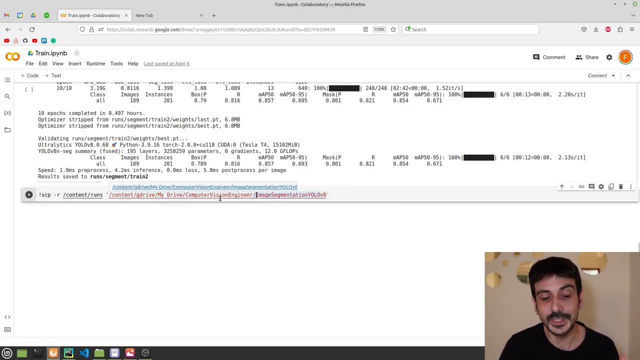 drive. so just make sure everything is okay, make sure this location makes sense and you can just execute this cell and you're going to copy everything into your google drive. now let me show you my google drive. i have already executed this cell, so everything is under my google drive. 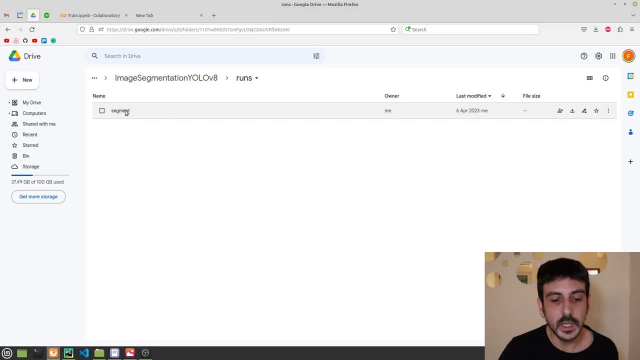 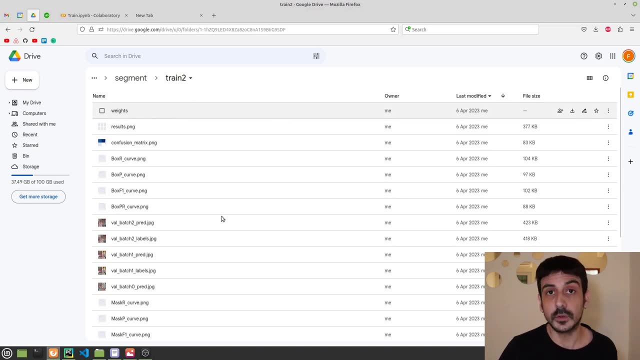 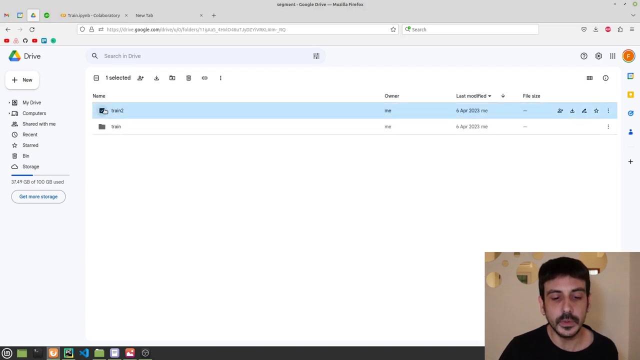 this runs directory which was created when i run that cell and under this other directory, which, which is called segment, we have trained to. so these are all of our results. these are the results we are now you going to analyze. so what i'm going to do now is just to download this directory and once we have, 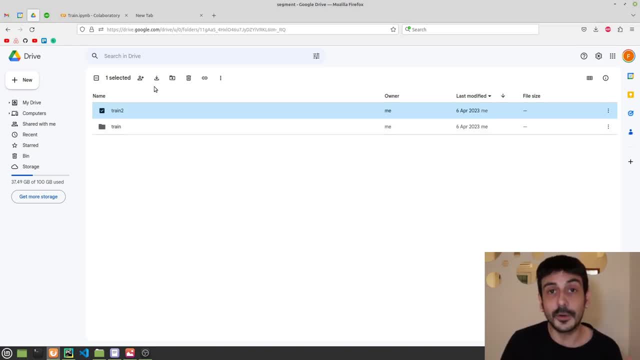 this directory into our local computer, then we are going to take a look at all the plots, at all the metrics, and i'm going to tell you exactly what i usually do in order to validate this training process. so everything is now downloaded, everything is now completed, and let's take a look. 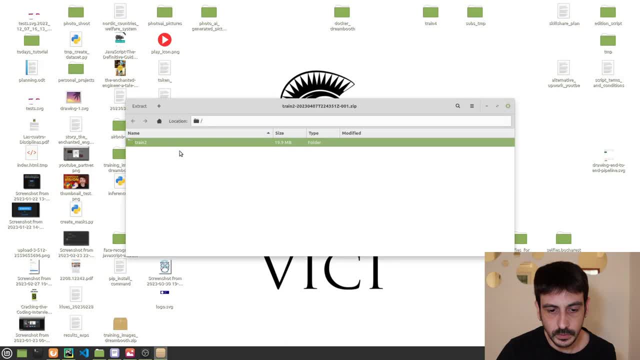 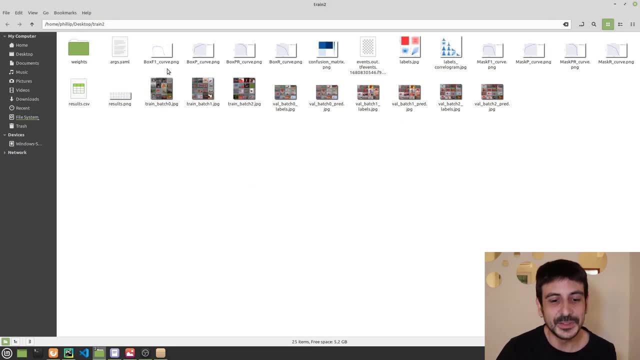 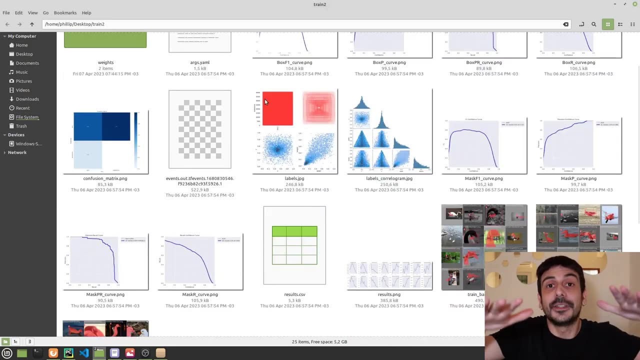 at these files. so what i'm going to do is i'm just going to copy everything into my desktop. i need to do some cleaning, by the way. so these are all the results we got from this training process. you can see that this is a lot of information. this is definitely a lot of. 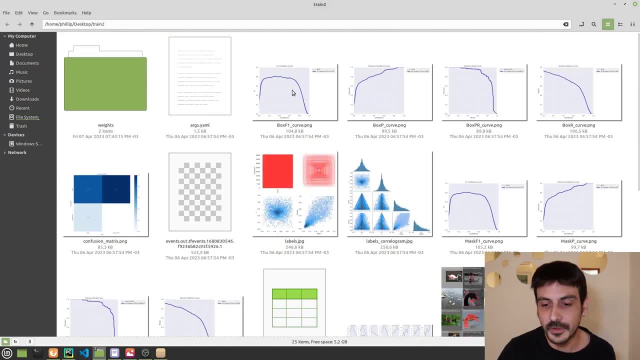 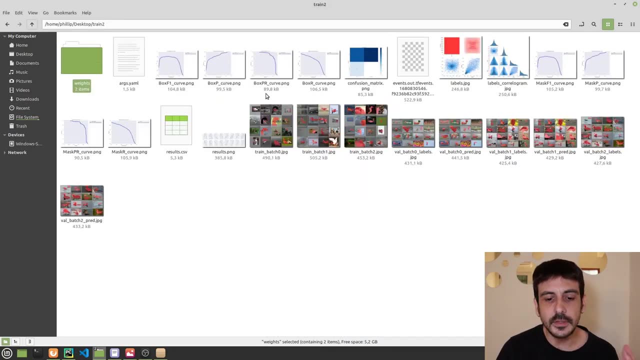 information. right, we have many, many different files. we have many different everything. we have the weights over here. we have a lot of information. so let me tell you, let me give you my recommendation about how to do this evaluation, how to do this validation from what i'm doing is i'm going to put. 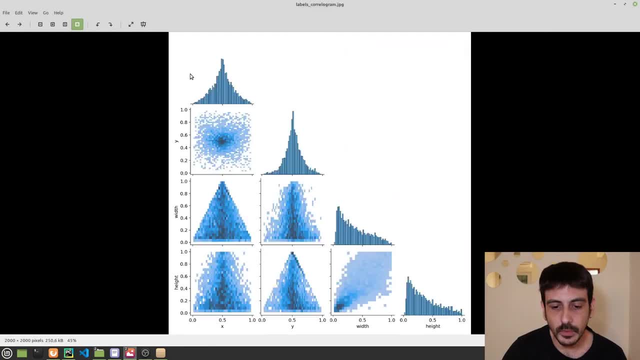 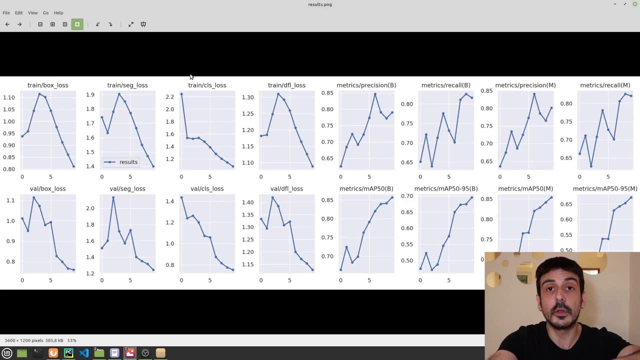 all these plots and from all of these results, I will recommend you to focus on two things. one of them is this plot, one of the one of them is all of these metrics, and then I'm also going to show you how to take a look at these results. 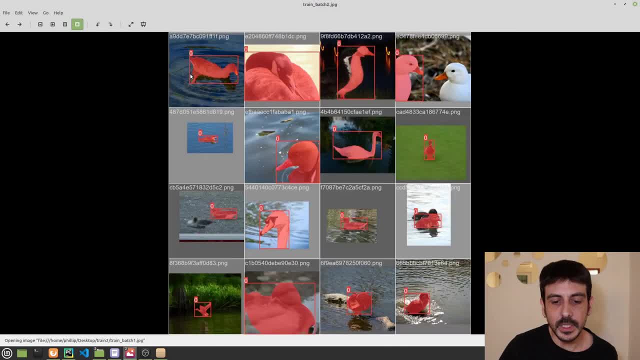 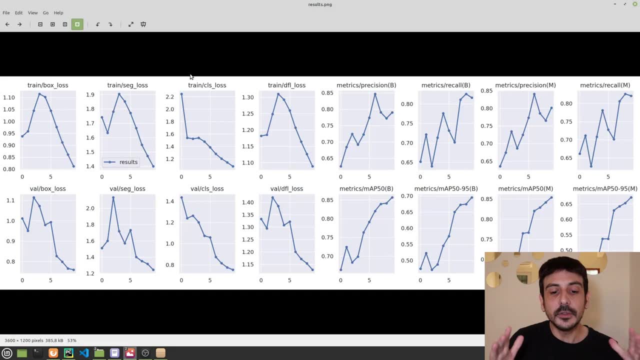 at these predictions from these images. but for now, let's start here. you can see that this is a lot of information. these are a lot of metrics and you can definitely knock yourself out analyzing all the information you have here. you can definitely go crazy analyzing all of this information, all of these plots, but 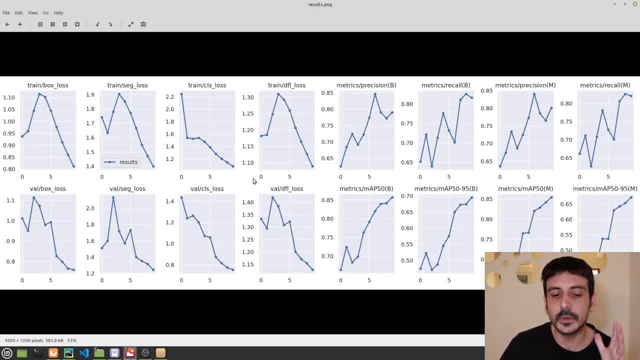 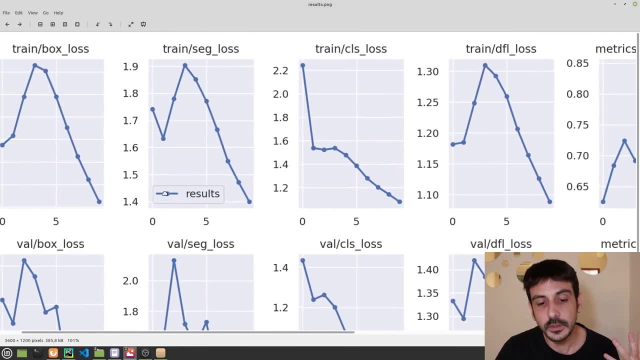 I'm going to show you like a very, very simple and a very straightforward way to do this analysis, to do this validation. this is something that I have already mentioned in my previous videos on YOLOv8 on how to train a model and how to 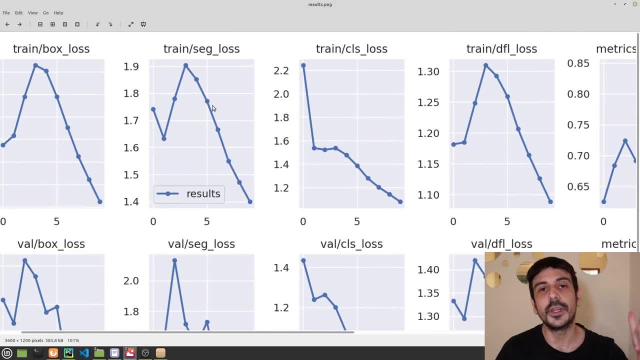 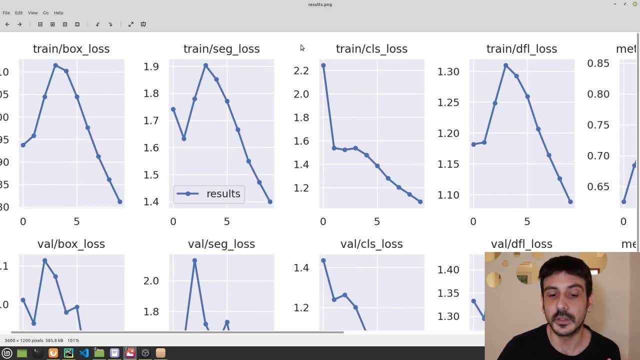 validate this model, which is: take a look what happens with the last function. take a look what happens with your last function. take a look what happens with your last function. take a look what happens with your last plots, with all the plots which are related to the last function, and as this: 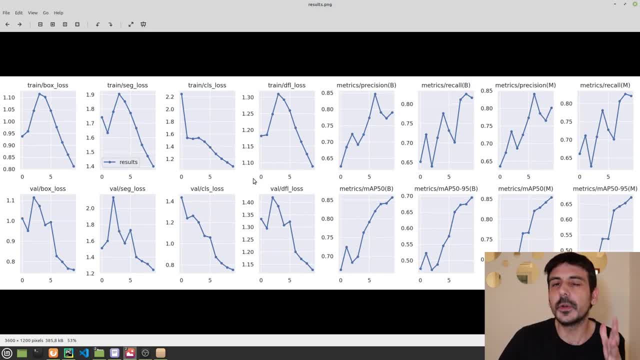 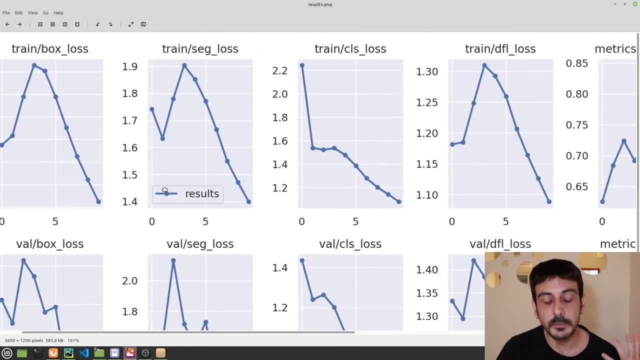 plots, but i'm going to show you like a very, very simple and a very straightforward way to do this analysis, to do this validation. this is something that i have already mentioned in my previous videos on yolo v8, on how to train a model and how to validate this model, which is- take a look what 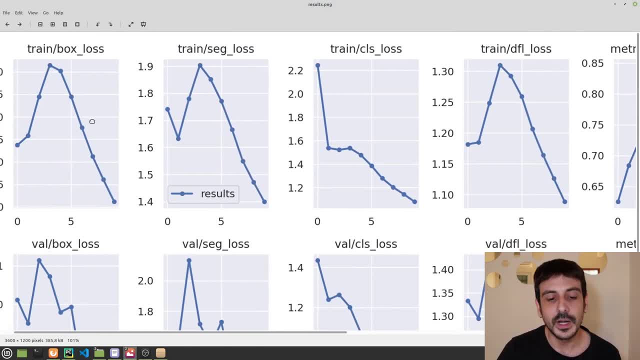 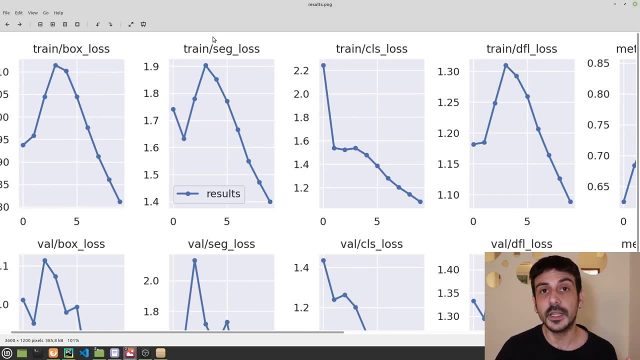 happens with the last function. take a look what happens with your last plots, with all the plots which are related to the last function, and as this is a semantic segmentation type of algorithm, i will tell you. take a look- what happens with this loss, with the segmentation loss. 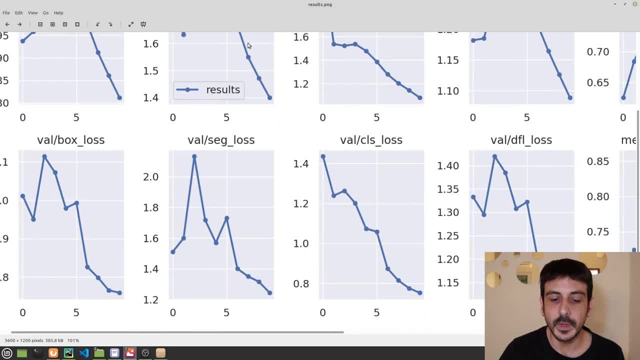 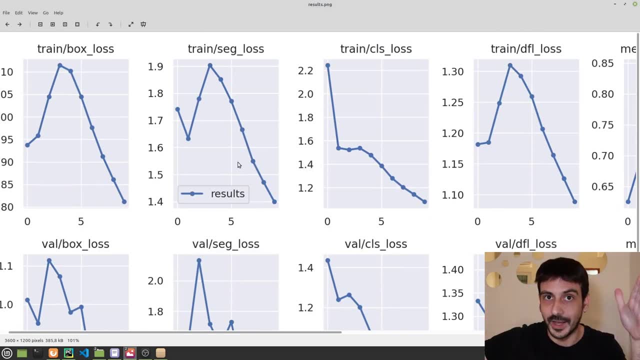 i will say: take a look what happens with the training loss and the validation loss and long story short, just make sure the loss function goes down right. if your loss function is going down, it's likely things are going well. it's not a guarantee. maybe things are not really. 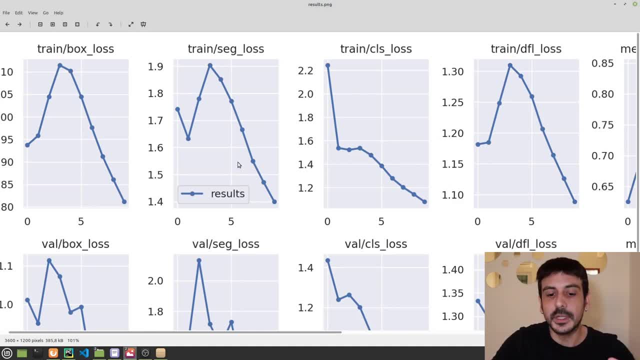 going that well and the model it doesn't really perform that well. it may happen, but i don't know what happens with this loss, with the segmentation loss. i will tell you: take a look what happens with this loss, with the segmentation loss. i will say: take a look what happens with the training loss and the validation loss and long story short, just make sure the loss function goes down right. if your loss function is going down, it's likely things are going well. it's not a guarantee. maybe things are not really going that well and the model it doesn't really perform that well. it may happen, but i 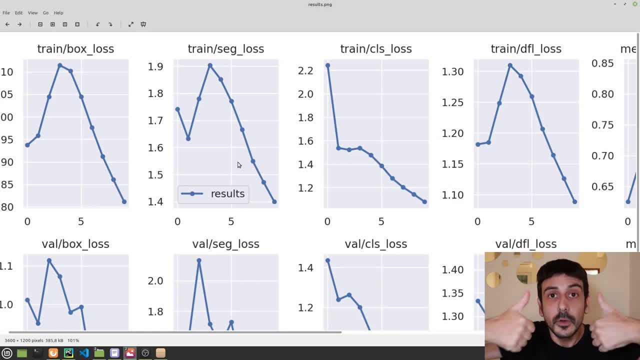 will say that if the loss function is going down, it's a very good sign. if, at the contrary, your lost function is going up, i would say you have a very, very serious problem. i would say there's something which is seriously wrong with your training process, or with your data, or with your 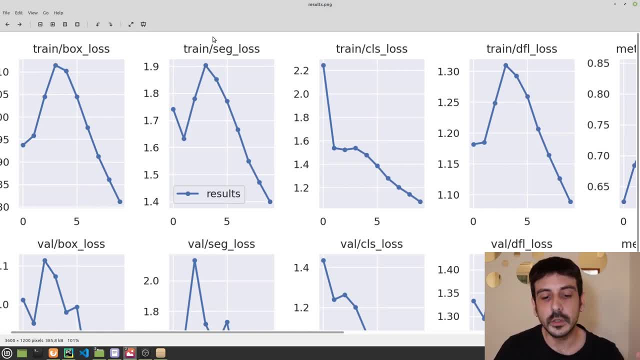 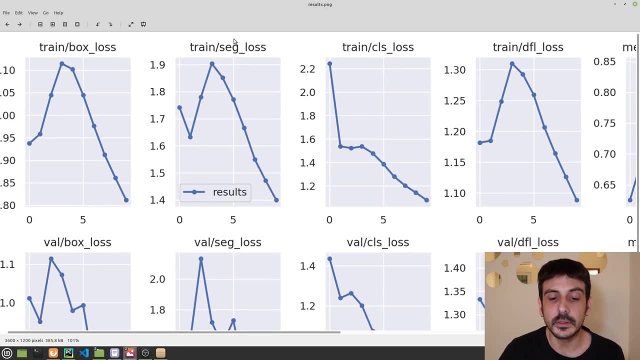 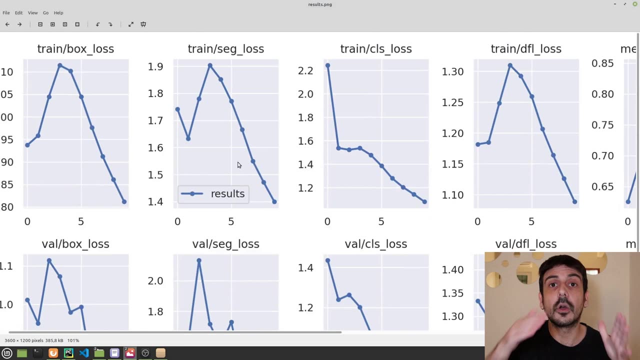 is a semantic segmentation type of algorithm. I will tell you, take a look what happens with this loss, with the segmentation loss. I will say: take a look what happens with the training loss and the validation loss. and long story short. just make sure the loss function goes down right if your loss function is. 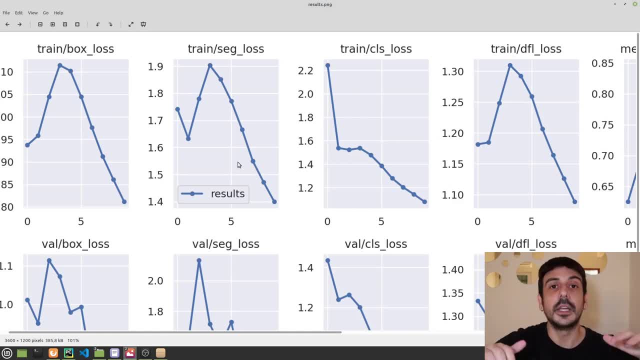 going down. it's likely things are going well. it's not a guarantee. may be things are not really going that well and the model is doesn't really perform that well. it may happen. but I will say that if the loss function is going down, it's a very good sign. 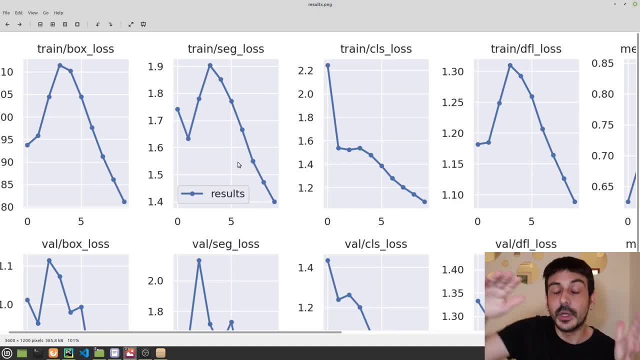 if, at the contrary, your loss function is going up, I will say you have a very, very serious problem. I would say there is something which is seriously wrong with your training process, or with your data, or with your annotations, or with something you have done, something seriously wrong, or 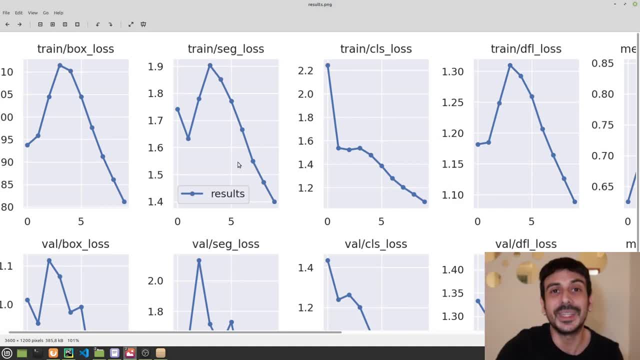 or there's something seriously wrong with your data, but i'm talking about something amazingly wrong, seriously wrong. right, if your loss function is going up. i don't know what's going on, but something is going on. do you see what i mean? so having a loss function which is going down. 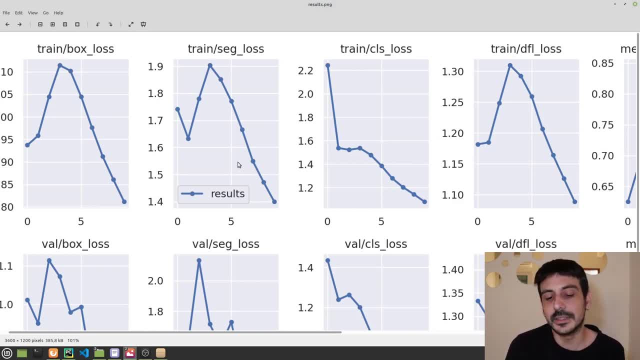 yeah, it's not a guarantee of success. i mean, it's not like it's that a good model for sure. no, you may have a situation where you haven't trained a good model and your loss function is going down anyway, but i would say that it's a very, very good sign. at the very least, your training loss. 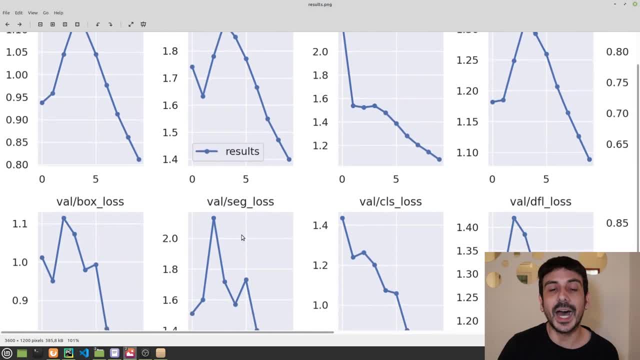 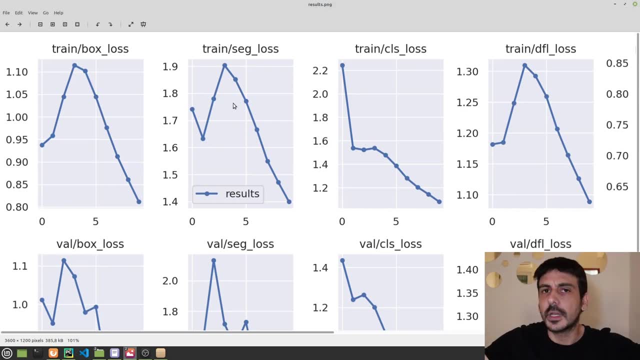 and your validation. loss should go down, and i'm talking about a trend of going down, right? for example, here we have a few epochs in which the loss function is going up. that's okay, that's not a problem. we are looking for a trend. we should have a trend for the loss function to go down. 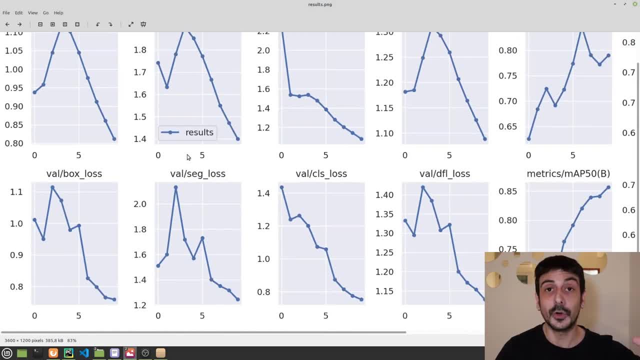 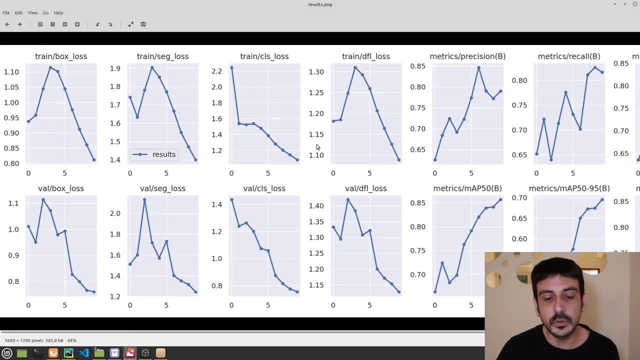 and that's exactly what we have in this situation. so, long story short, that's my recommendation on how to reduce your loss function and how to reduce your loss function and how to reduce your loss function and how to do this value, this validation, how to do this analysis on all the metrics we have. 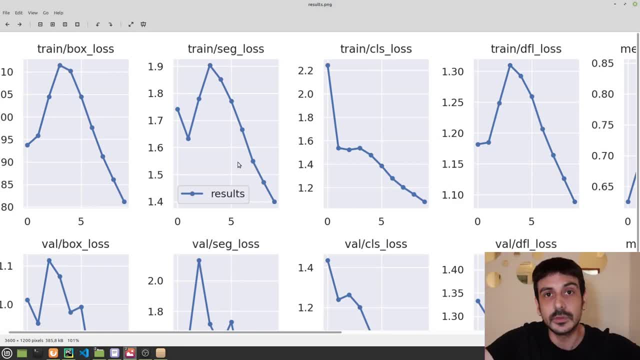 rotations or with something you have done something seriously wrong, or there's something seriously wrong with your data, but i'm talking about something amazingly wrong, seriously wrong. right, if your loss function is going up. i don't know what's going on, but something is going on. do you see what i mean? 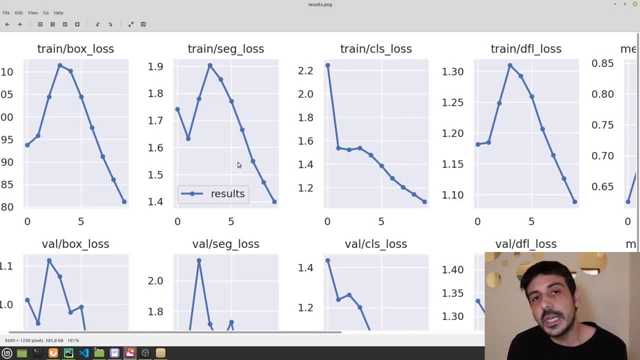 so having a loss function which is going down, yeah, it's not a guarantee of success. i mean, it's not like it's that a good model for sure. no, you may have a situation where you haven't trained a good model and your loss function is going down anyway, but i would say that it's a very, very good sign. 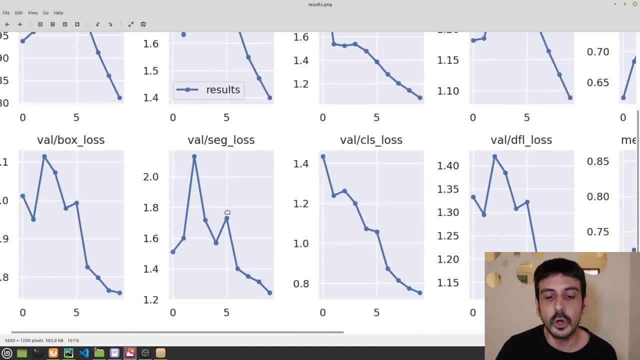 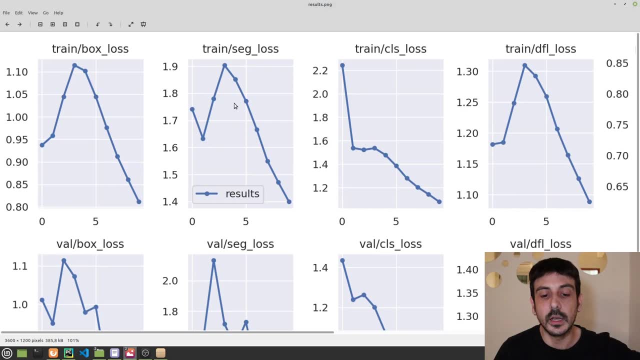 at the very least, your training loss and your validation loss should go down, and i'm talking about a trend of going down, right, for example, here we have a few epochs in which the loss function is going up. that's okay, that's not a problem. we are looking for a trend. 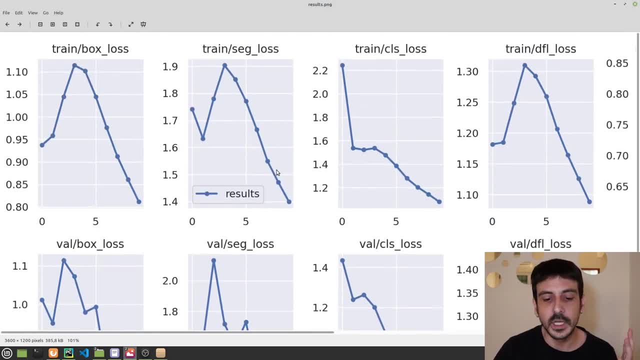 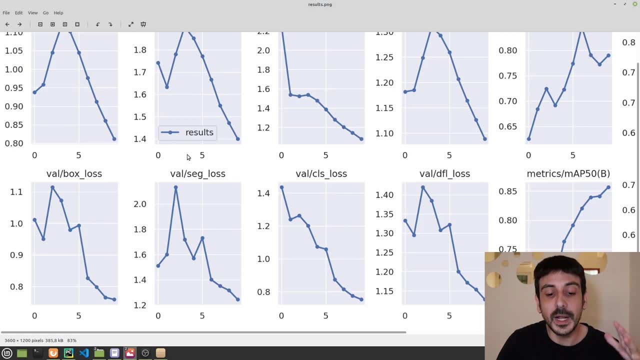 we should have a trend for the loss function to go down, and that's exactly what we have in this situation. so long story short, that's my recommendation on how to do this value, this validation, how to do this analysis on all the metrics we have over here. for now, focus on these. 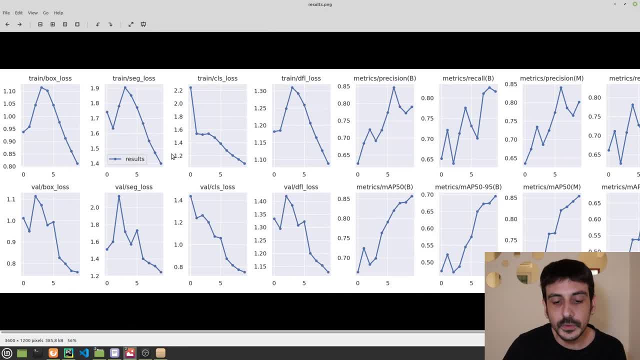 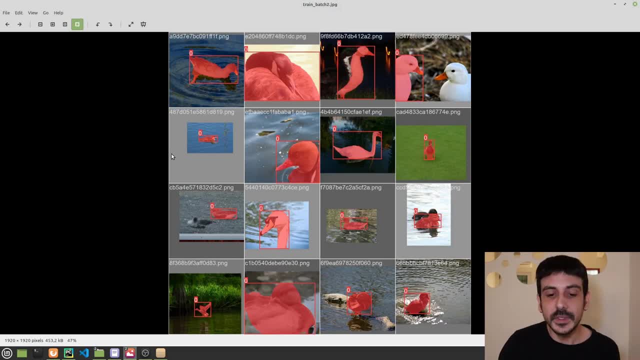 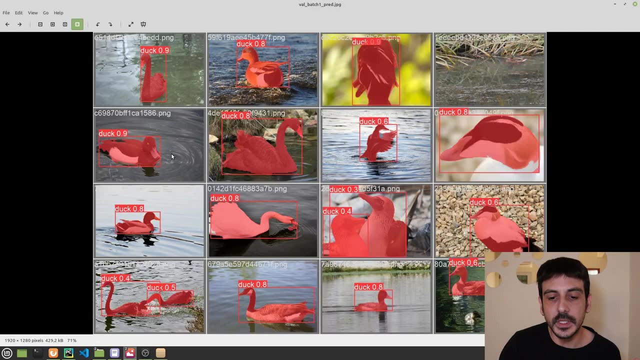 two, and make sure they are going down. and then, in order to continue with this process, with this validation, is that we are going to take a look at what happens with your predictions. how is this ball performing with some data, with some predictions? and for this we are going to take a look. what happens with all of these images? right? 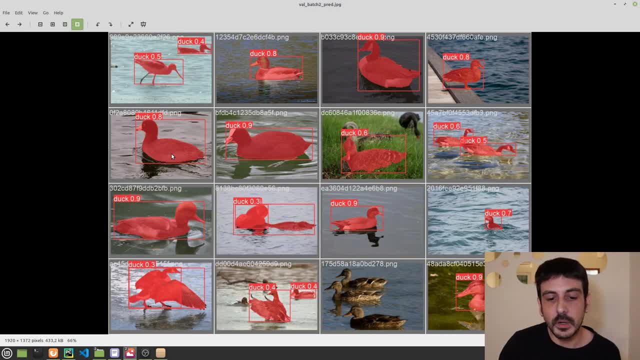 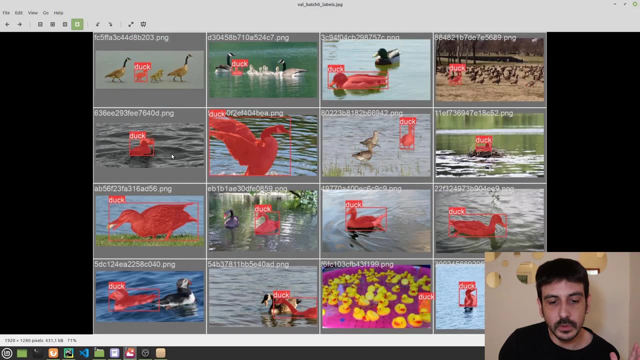 you can see that these are some badges and these are some some of our labels, some of our annotations for all of these images, and then these are some of the predictions for these images. right, we are going to take a look what happens here and, for example, i'm going to show you these results. 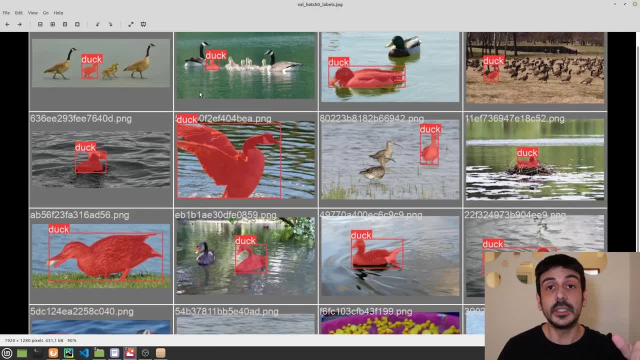 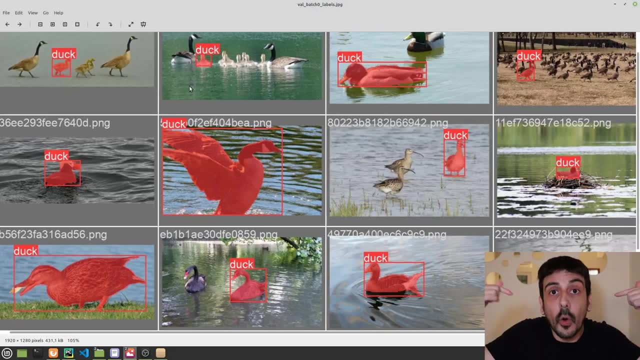 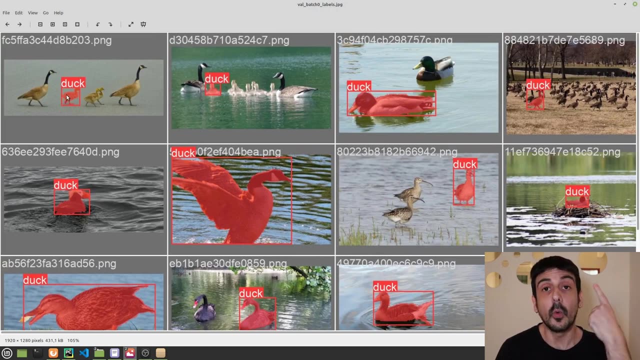 this, this the first image, and you can see that, looking at this image- which, again, these are not all predictions, but this is all data, this is all annotations, these are all labels- you can see that there are many, many, many missing annotations. for example, in this image we are, we only have- 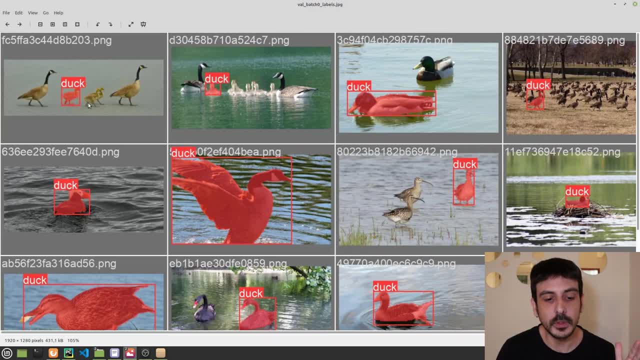 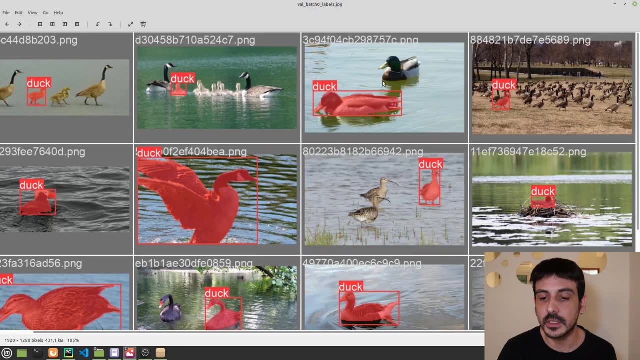 one mask. we only have the mask for one of our ducks. we have one, two, three, four, five ducks, but only one of them is annotated. we have a similar behavior here: only one of the dogs is annotated. here is something similar: only one of them is annotated, and the same happens for absolutely every single. 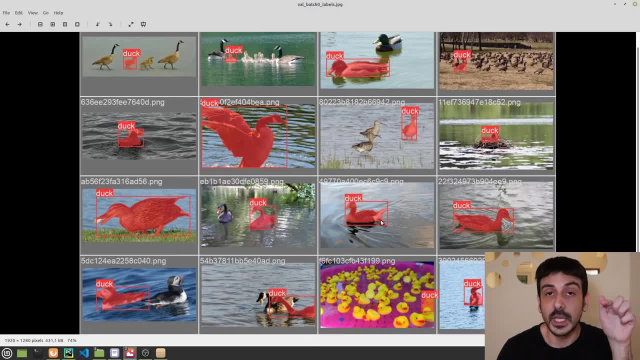 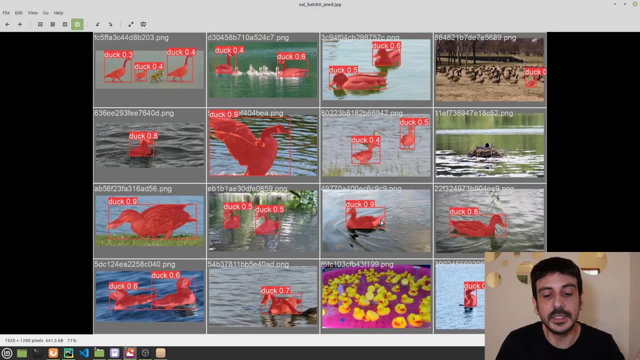 one of this image. so there are a lot of missing annotations in this data we are currently looking at and if i look at the predictions now- these are the same images, but these are all predictions- we can see that nevertheless, we have a lot of missing annotations. the predictions don't really look that bad right, for example, 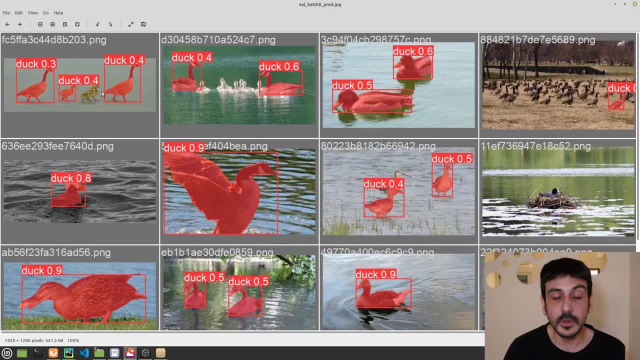 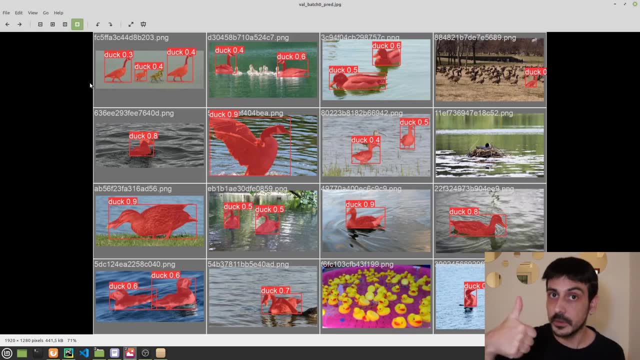 this case we are detecting one, two, three or of the five ducks we, so we have an even better prediction that we have over here. i would say it's not a perfect detection, but i will say it's a very good right. it's like it's not 100 accurate, but it's like very good and i would say it's definitely. 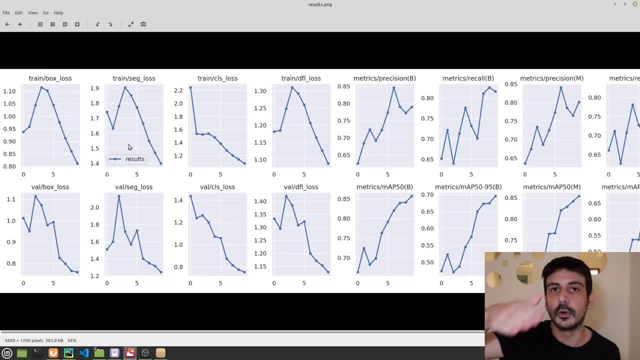 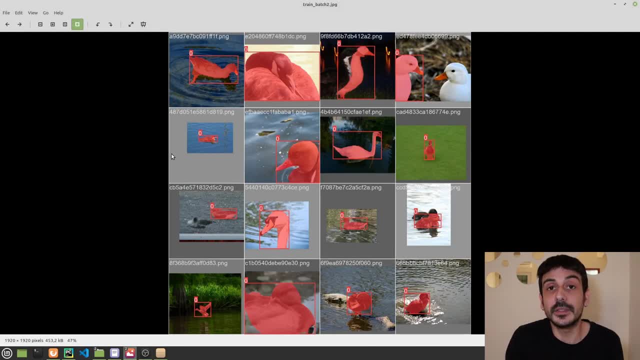 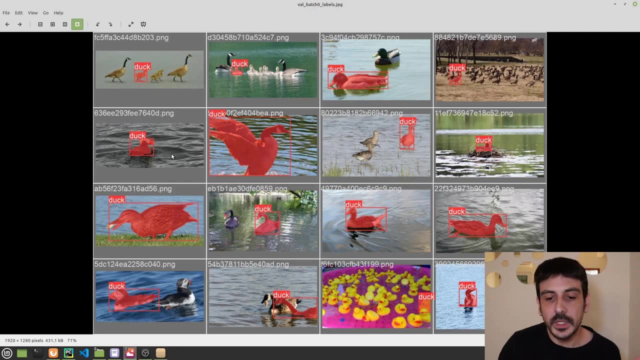 over here for now, focus on these two and make sure they are going down and then, in order to continue with this process, with this validation, is that we are going to take a look at what happens with your predictions. how is this ball performing with some data, with some predictions? and for this we are. 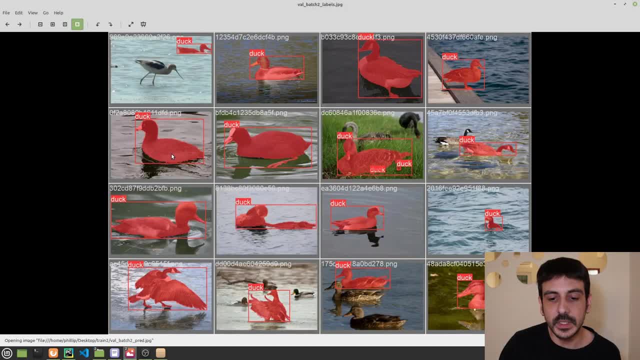 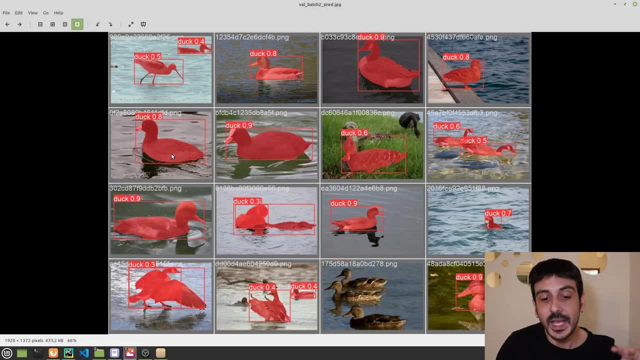 going to take a look what happens with all of these images, right, you can see that these are some badges and these are some some of our labels, some of our annotations for all of these images, and then these are some of the predictions for these images, right? so we are going to take a look what happens here. 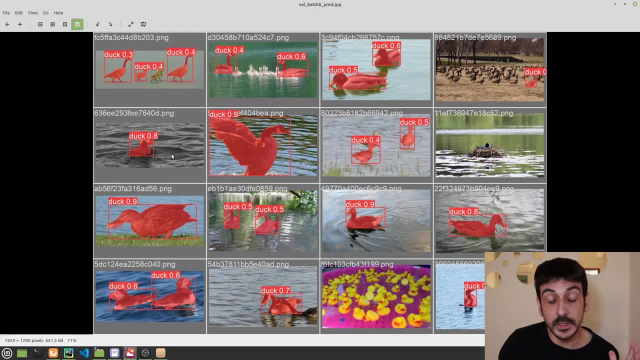 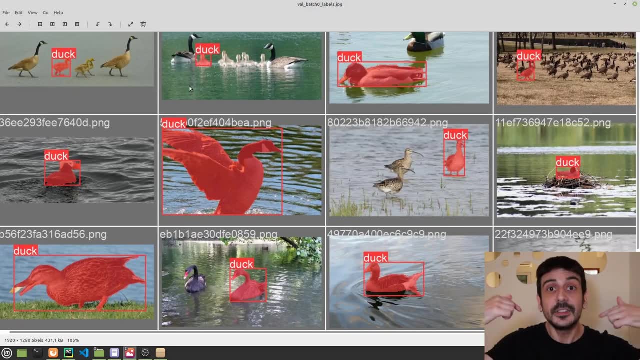 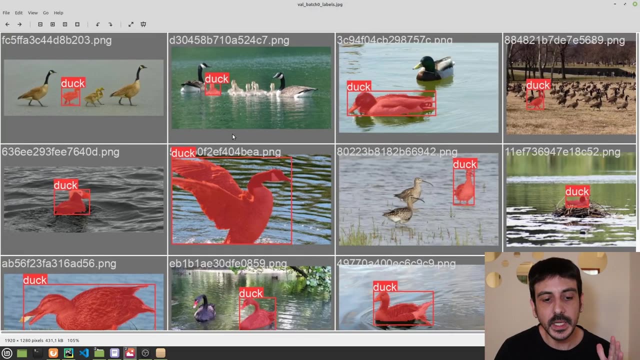 and, for example, i'm going to show you these results, this, this the first image, and you can see that, looking at this image- which, again, these are not all predictions, but this is all data, this is all annotations, these are all labels- you can see that there are many, many, many missing annotations. 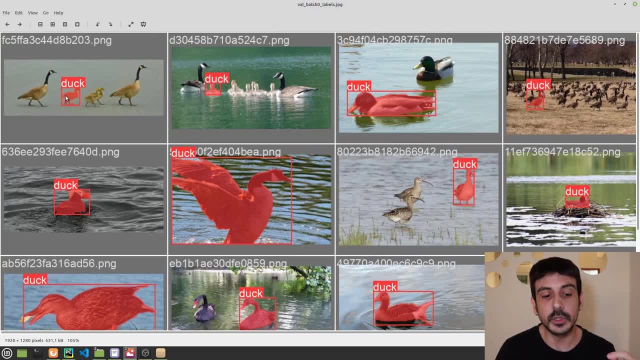 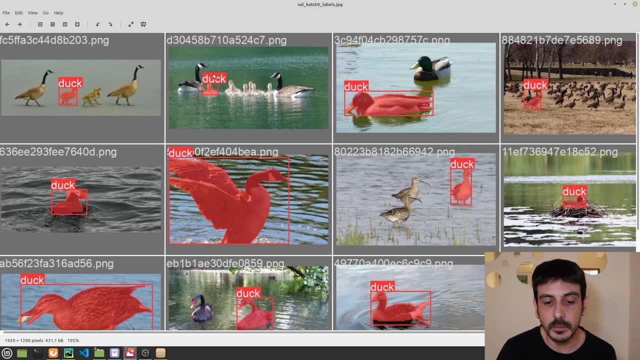 for example, in this image we are, we only have one mask. we only have the mask for one of our dogs. we have one, two, three, four, five ducks, but only one of them is annotated. we have a similar behavior here: only one of the dogs is annotated. here is something similar: only one of them is annotated. 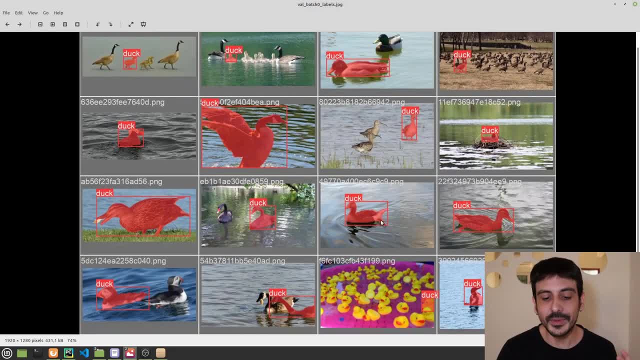 and the same happens for absolutely every single one of this image. so there are a lot of missing annotations in this data we are currently looking at and if i look at the predictions now, these are the same images, but these are all predictions. now, these are the same images, but these are all. 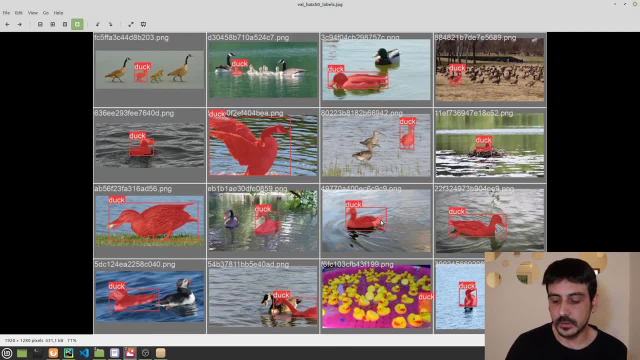 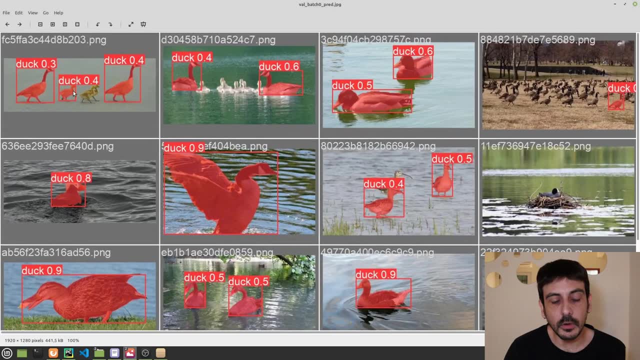 we can see that, nevertheless, we have a lot of missing annotations. the predictions don't really look that bad right. for example, in this case we are detecting one, two, three or of the five dogs we so we have an even better prediction that we have over here. i would say it's not a perfect. 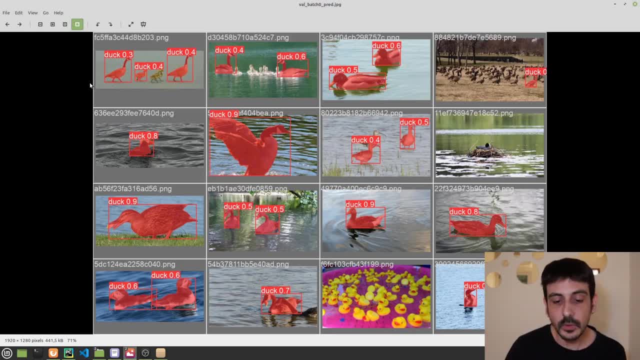 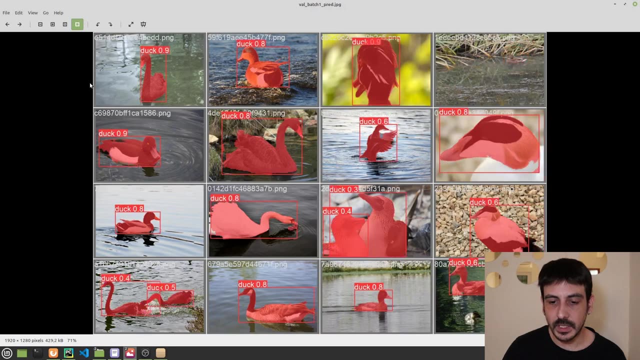 detection, but i would say it's a very good right. it's like it's not 100 accurate, but it's like very good and i would say it's definitely better than the data we use to train this model. so that's what happens with the first image and if i take a look at the other images, i can see a similar behavior. 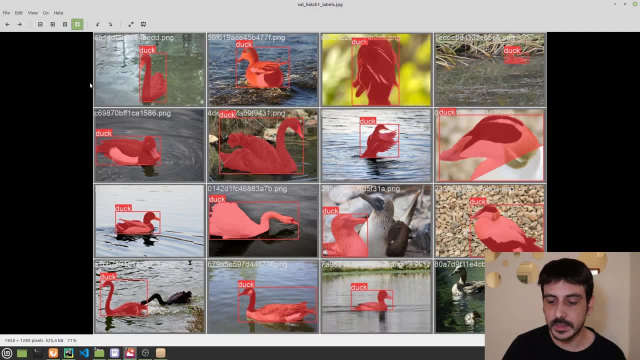 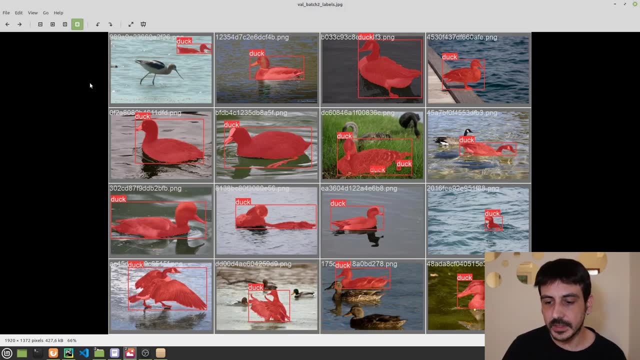 right, these are. these are the, these data we use for training this algorithm, and this is the predictions we got for these images, and so on. right, it seems it's like this, exactly the same behavior, exactly the same situation for this image as well. so my conclusions, by looking at: 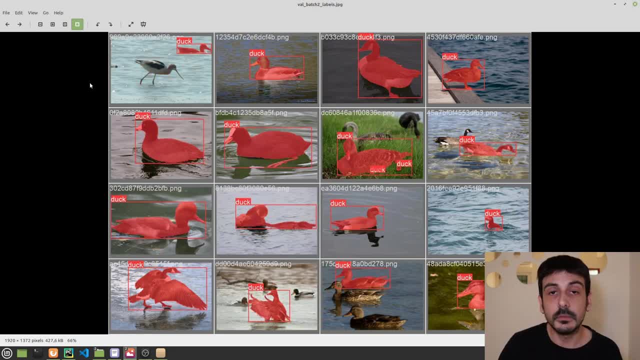 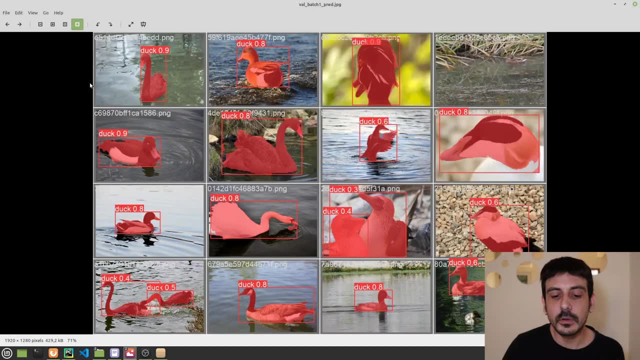 these images by looking at these predictions, is that the model is not perfect, but it's not perfect, but i will say it performs very well, especially considering that the data we are using to train this model seems to be not perfect, seems to have a lot, a lot of missing detections, have a lot of 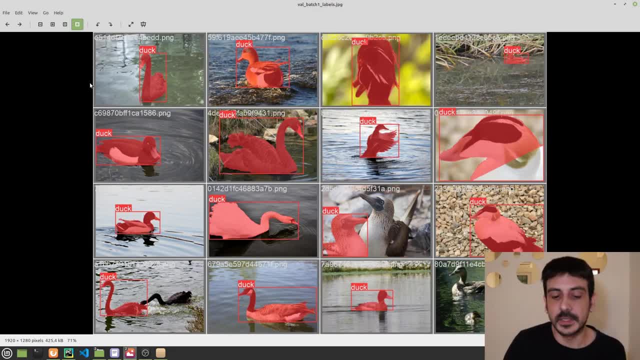 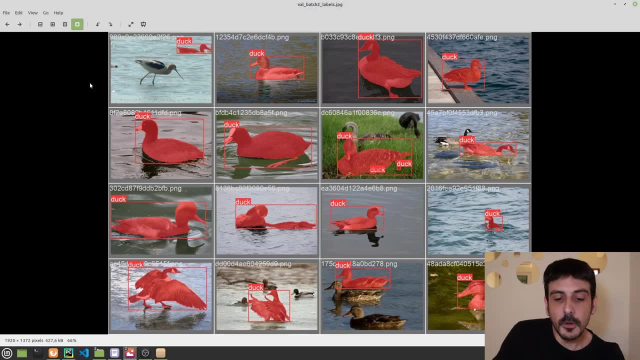 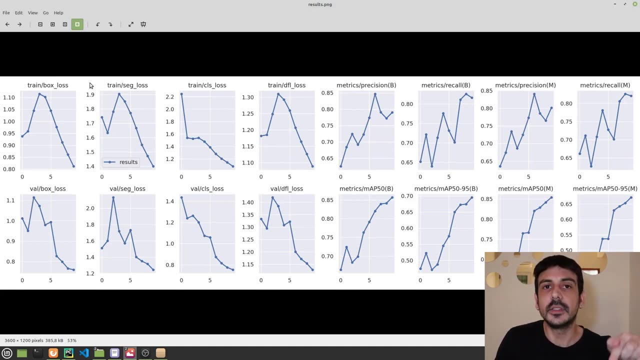 missing um elements, right, a lot of missing objects. so that's our conclusion, that's my conclusion, by looking at these, at these results, and that's another reason for which i don't- i don't recommend you to go crazy analyzing these plots, because when you are analyzing these plots, you 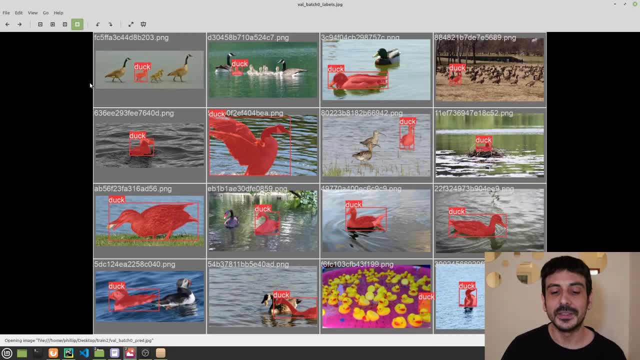 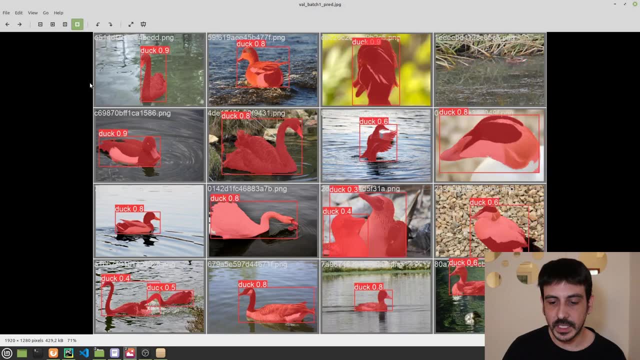 better than the data we use to train this model. so that's what happens with the first image, and if i take a look at the older images, i can see a similar behavior. right, these are. these are the we use for training this algorithm and this is the predictions we got for these images, and so on. 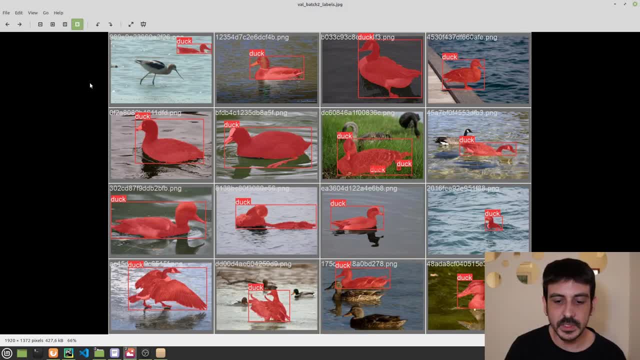 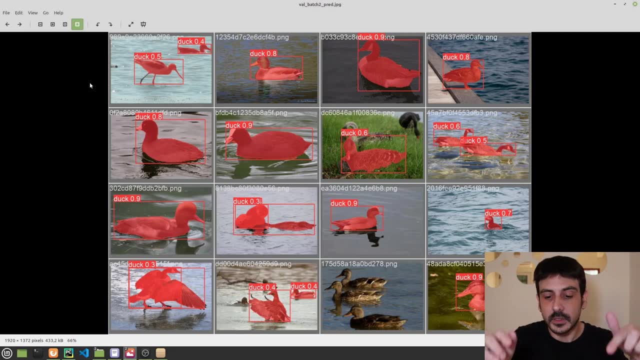 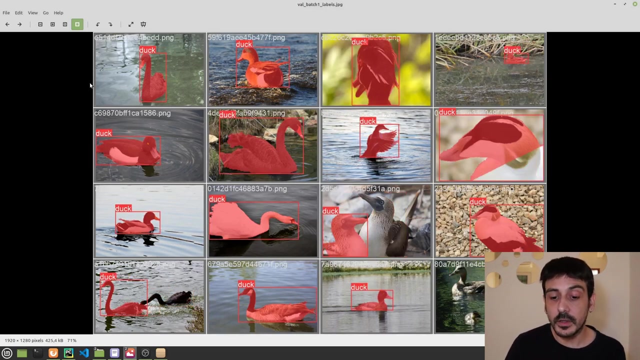 right. it seems it's like this, exactly the same behavior, exactly the same situation- for this image as well. so my conclusions by looking at these images, by looking at these predictions, is that the model is not perfect but, i will say, performs very well, especially considering that the data we are using to train this model seems to be not perfect, seems to have a lot, a lot of. 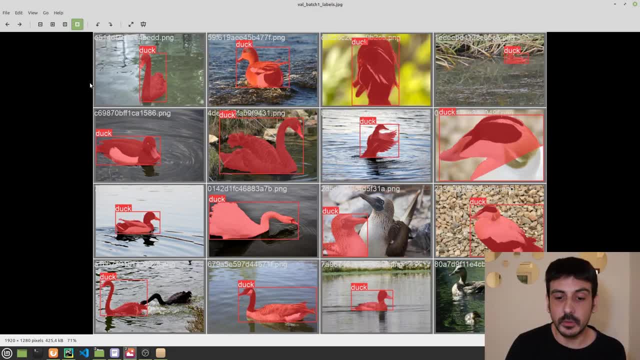 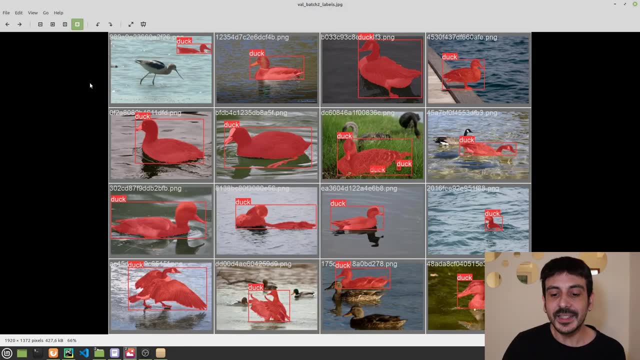 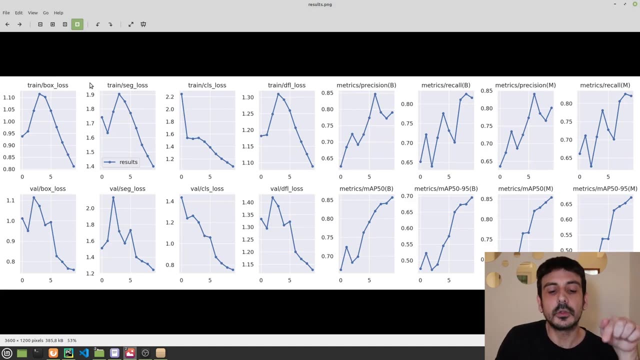 missing detections have a lot of missing elements, right, a lot of missing objects. so that's our conclusion, that's my conclusion by looking at these results, and that's another reason for which i don't- i don't recommend you to go crazy analyzing these plots, because when you are analyzing these, 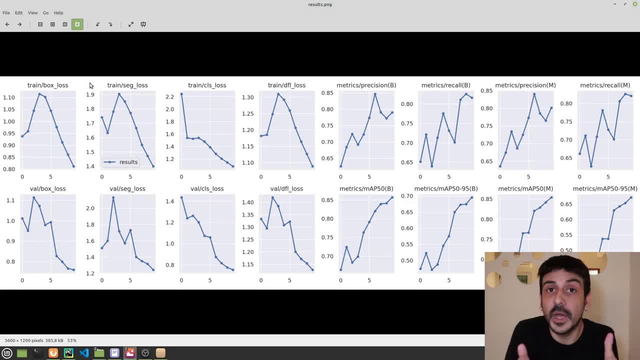 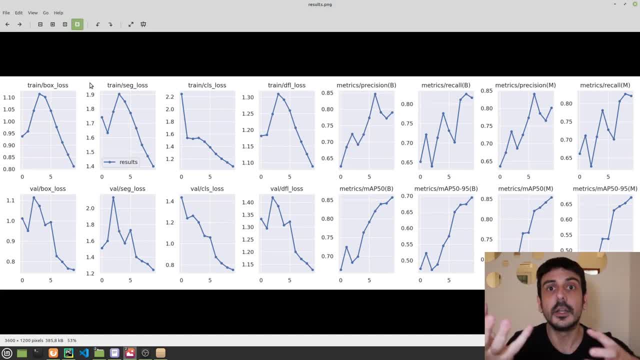 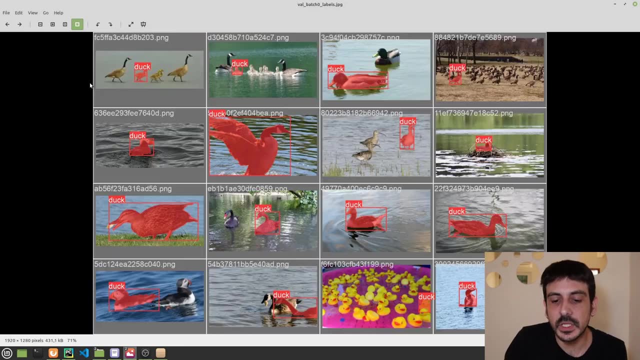 the only thing you're doing is you're comparing your data with your predictions, with the predictions you got with the model, right? so as the only thing you're doing is a comparison between these two things, then the if you have many missing detections or many missing objects, or if you 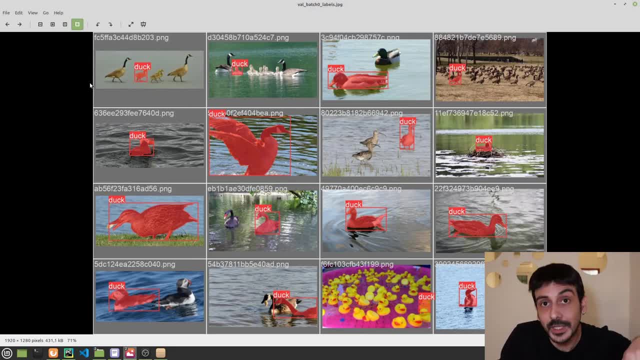 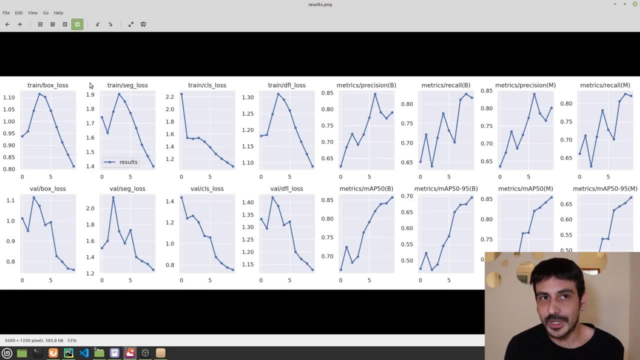 have many different errors in your data, in the data you're using to train the eye green, then this comparison it's a little meaningless, right? it doesn't really make a lot of sense because if you're just comparing one thing against the other, but the thing you are comparing with 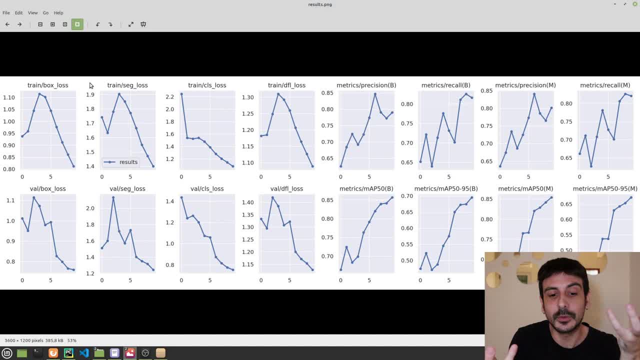 it's. it has a lot of errors, it has a lot of missing objects, and so on. maybe the comparison doesn't make a lot of sense whatsoever, right? that's why i also recommend you to not go crazy when you are analyzing these plots, because they are going to give you a lot. 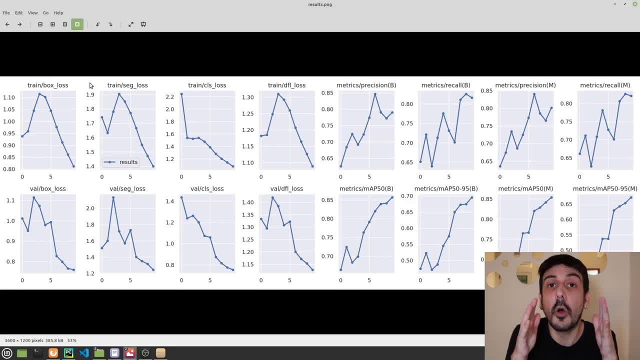 are analyzing these plots. remember, the only thing you are doing is that you are comparing your data- the data you are using in order to train this model- with your predictions. right, the only thing you're doing is you're comparing your data with your predictions, with the predictions you add, with 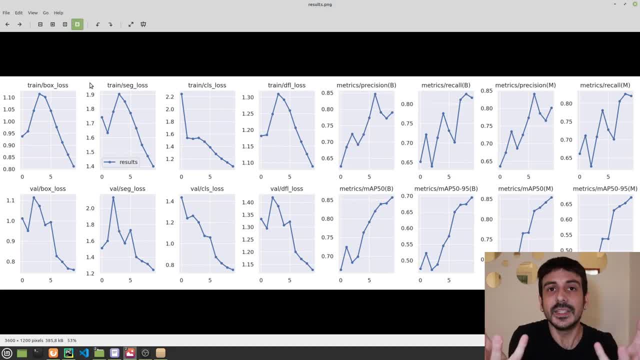 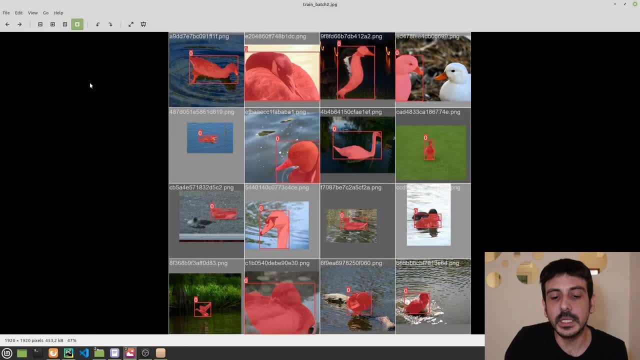 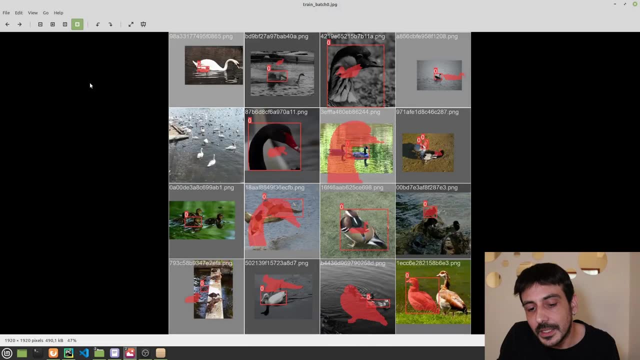 the model, right. so as the only thing you're doing is a comparison between these two things, then the. if you have many missing detections, or many missing objects, or if you have many different errors in your data, in the data you're using to train the eye green, then this comparison. 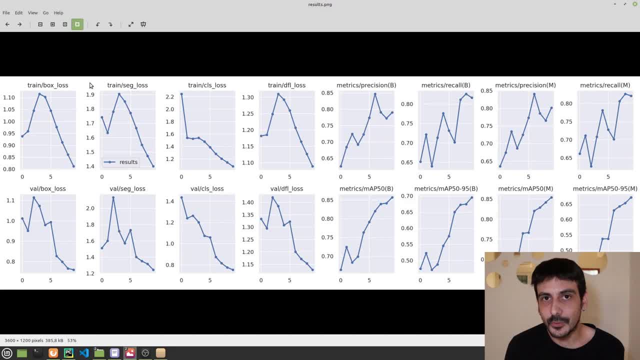 it's a little meaningless, right? it doesn't really make a lot of sense because if you're just comparing one thing against the other, but the thing you are comparing with it's it has a lot of errors, it has a lot of missing objects, and so on, maybe the comparison doesn't make a lot of. 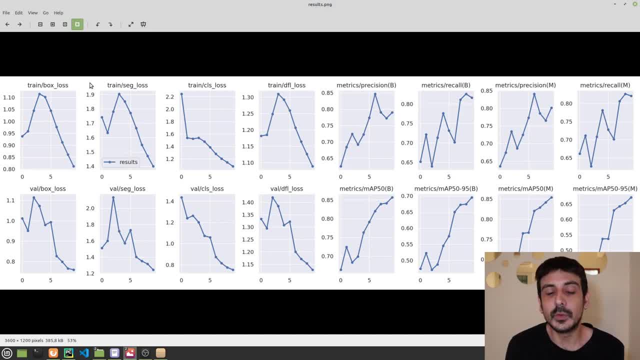 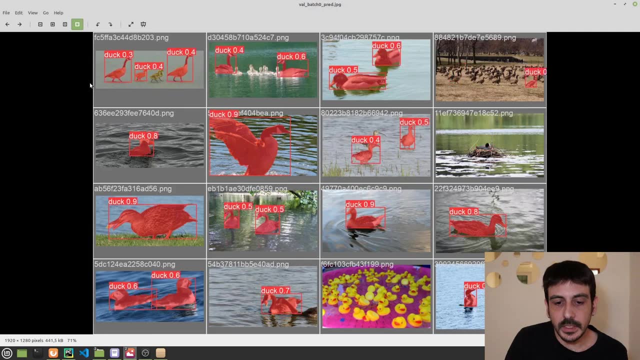 sense whatsoever right. that's why i also recommend you to not go crazy when you are analyzing these plots, because they are going to give you a lot of information, but you are going to have even more information when you are analyzing all of these results, and this is a very, very, very good 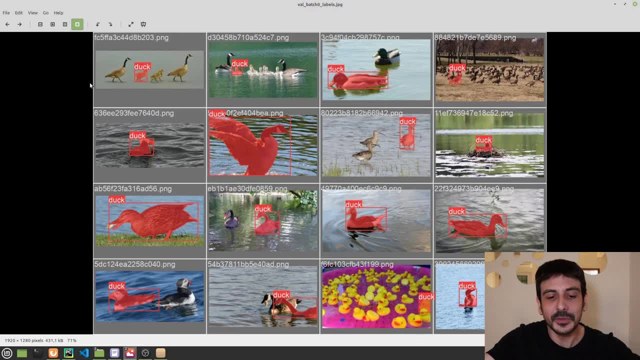 example of what happens in real life when you are training a model in a real project, because remember that building an entire data set, a, a set which is 100 clean and absolutely 100 perfect, is very, very, very expensive. so this is a very good example of what happens in real life. usually the data you're using to train the model, to train the 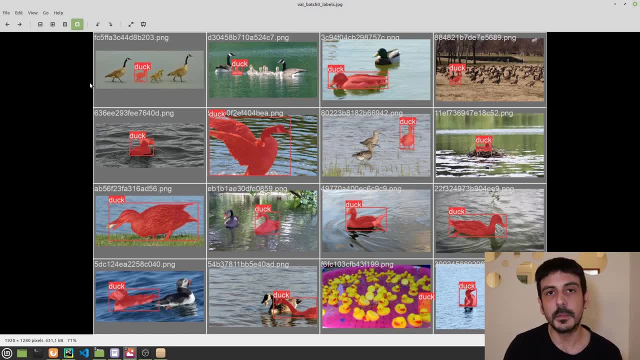 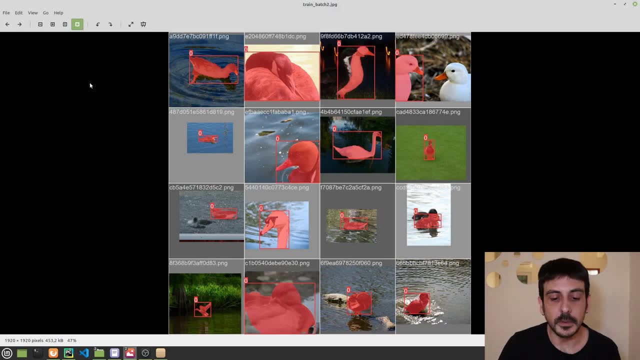 algorithm has a few errors, and sometimes there are many, many, many errors. so this is a very good example of how this validation process looks like with a data which is very similar to the data we have in our data set. so this is a very good example of how this validation process looks. 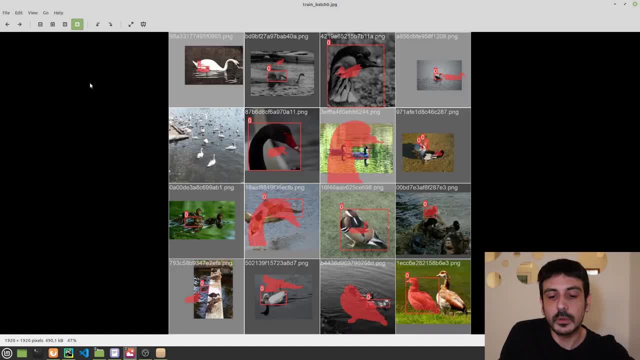 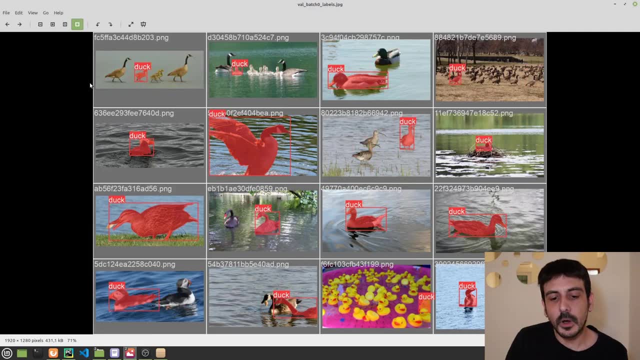 of information, but you are going to have even more information when you are analyzing all of these results. and this is a very, very, very good example of what happens in real life when you are training a model in a real project, because remember that building an entire data set, a data set which is 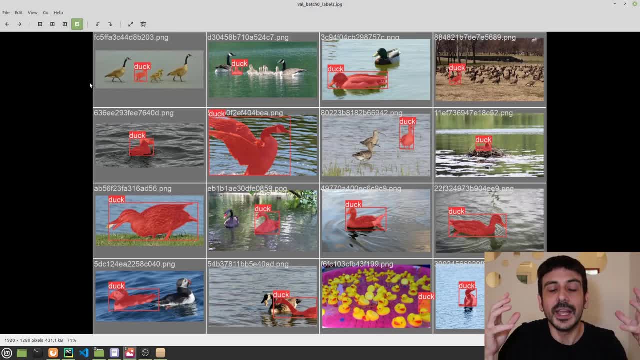 100 clean and absolutely 100 perfect is very, very, very expensive. so this is a very good example of what happens in real life. usually the data you're using to train the model, to train the algorithm, has a few errors, and sometimes there are many, many, many errors. so this is a very good 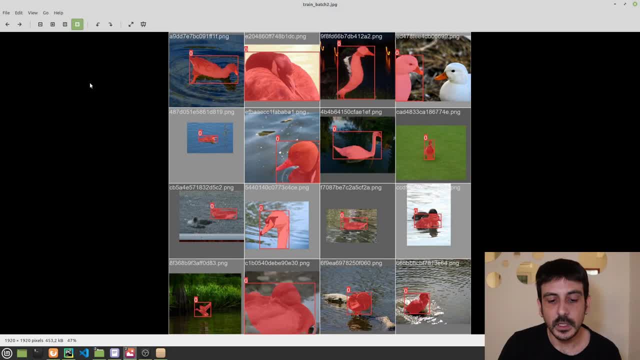 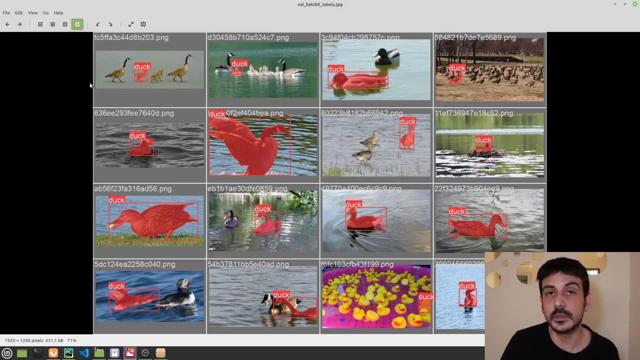 example of how this validation process looks like with a data which is very similar to the data we have in real life, which, in most cases, is not perfect. my conclusion from this evaluation for this validation would be to improve the data. taking a look what's going on with the data and the next step would be to improve. 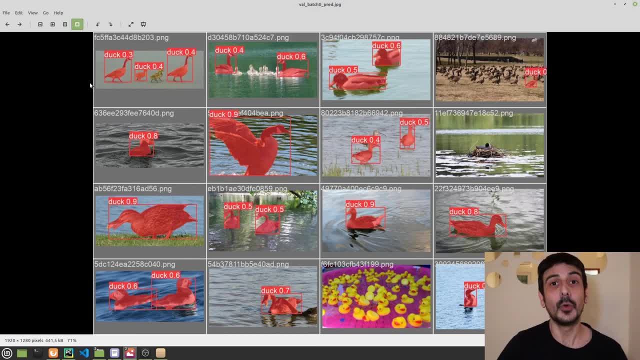 the data and by looking at these results. one of the ways in which i could improve this data is by using the predictions i'm getting instead of the annotations. i used to train this model. you see what i mean. if the annotations in the predictions we are getting are even better than the annotations, 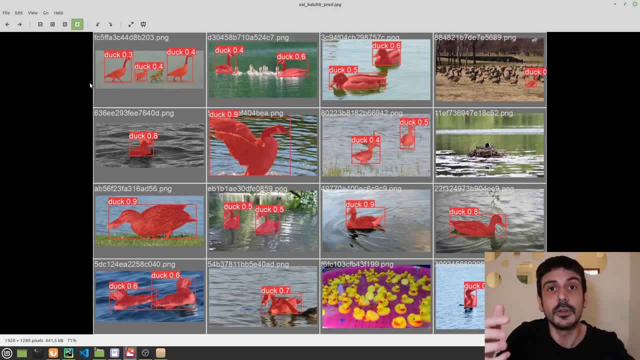 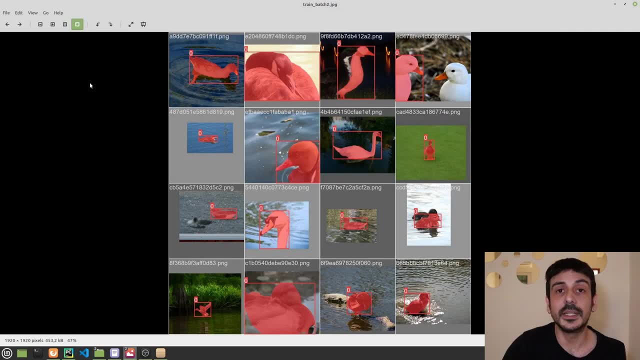 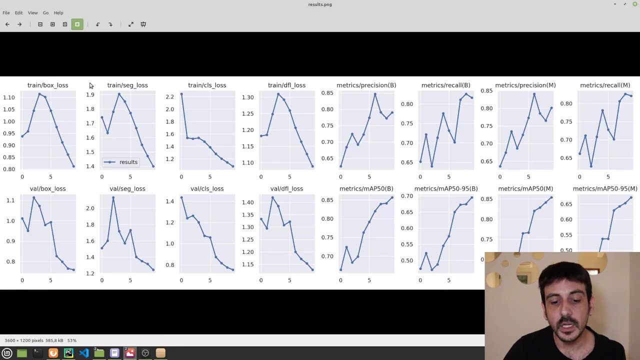 maybe our next step would be to use these predictions in order to train a new model. do you see what i mean? so the by analyzing all of these results, you are going to make decisions on how to move forward, on how to continue, and this is a very good example of how this process look like in a real project. 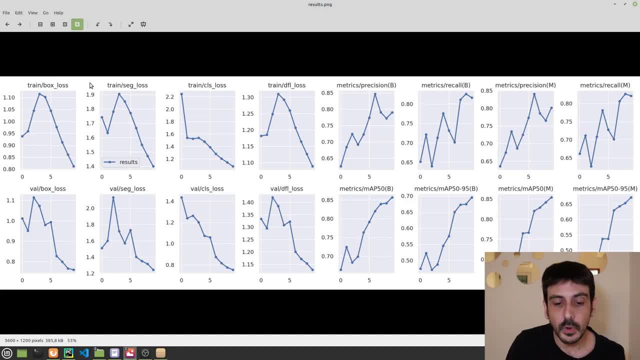 this is pretty much how it works, or how it looks like when you are working in a project. when you are working either in a company or if you are a freelancer and you're delivering a project for a client. this is pretty much what happens, right? there are errors, things happen and you need to. 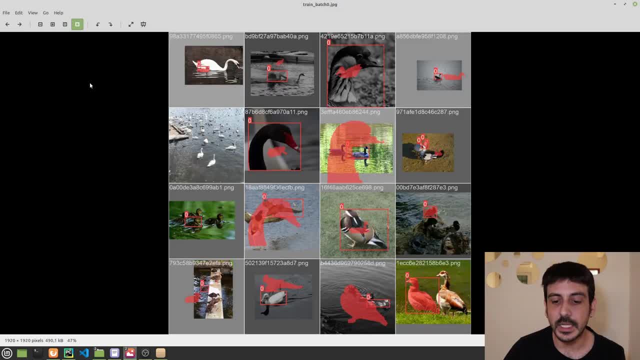 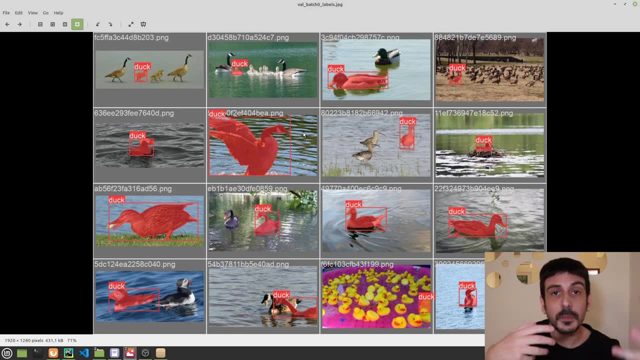 make a decision, given all the information you get with all these analyses. so that's going to be all in order to show you this very simple and very straightforward way in order to validate this training process, in order to make some conclusions regarding what's going on right and regarding to make some decisions, in order how to how to. 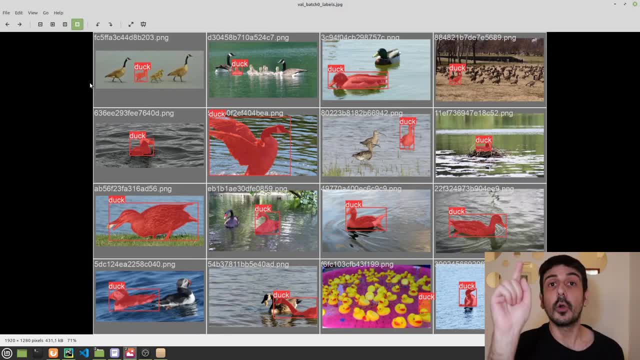 like in real life, which, in most cases, is not perfect. my conclusion from this evaluation for this validation could be improving the data, taking a look what's going on with the data and the next step would be to improve the data and, by looking at these results, one of the ways in which i could. 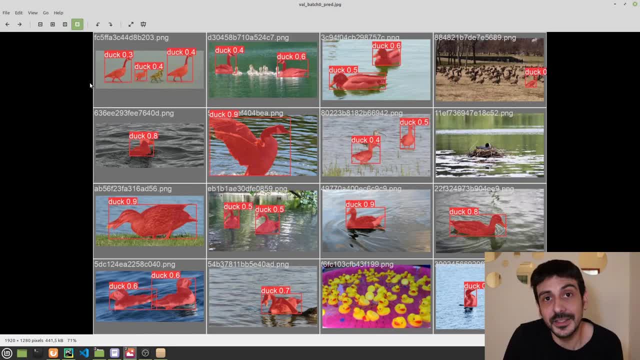 improve this data is by using the predictions i'm getting instead of the annotations i used to train this model. you see what i mean. if the annotations, if the predictions we are getting are even better than the annotations, maybe our next step would be to use these predictions in order to train a new. 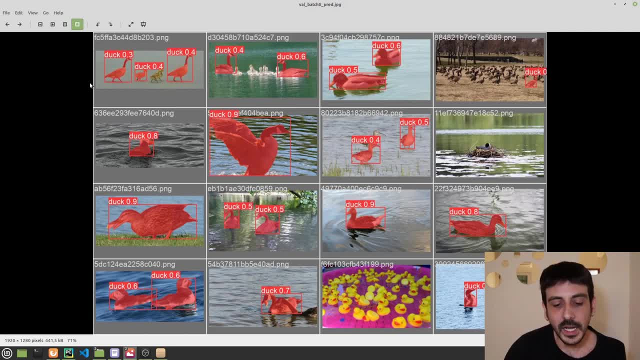 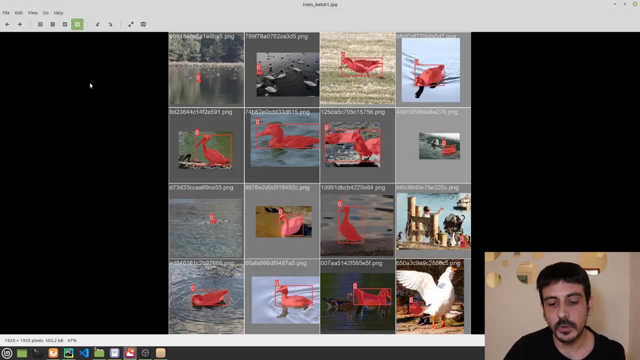 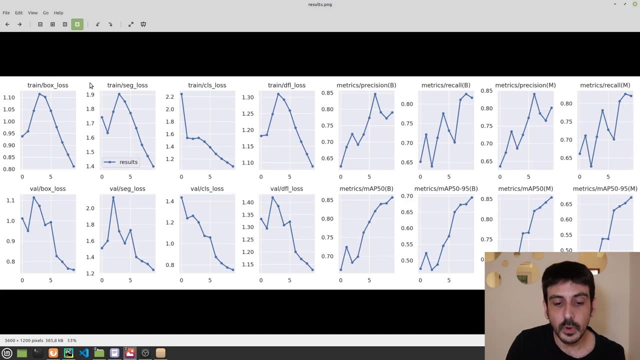 model. do you see what i mean? so the, by analyzing all of these results, you are going to make decisions on how to move forward, on how to continue, and this is a very good example of how this process look like in a real project. this is pretty much how it works, or how it looks like when. 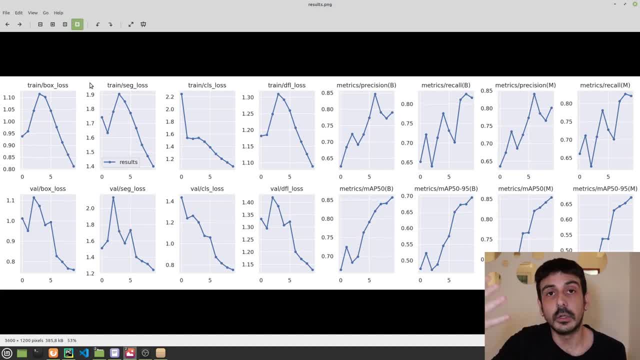 you are working in a project. when you are working either in a company or, if you are a freelancer or a, you're delivering a project for a client. this is pretty much what happens, right? there are errors, things happen, and you need to make a decision, given all the information you get with all these. 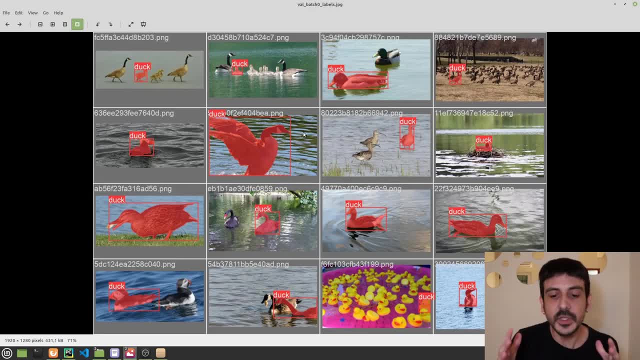 analyses. so that's going to be all. in order to show you this very simple and very straightforward way in order to validate this training process, in order to make some conclusions regarding what's going on right and regarding to make some decisions in order how to how to move forward with. 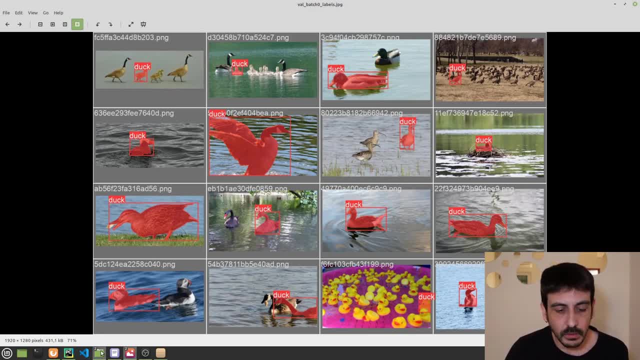 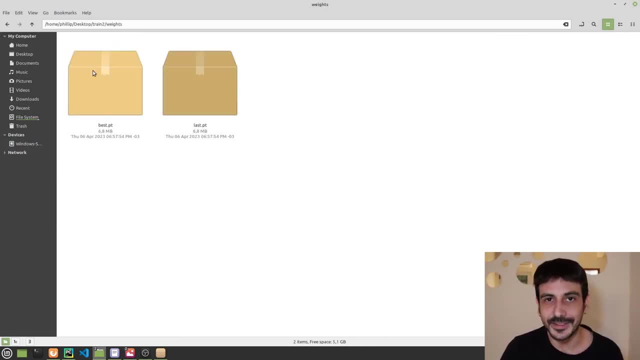 this project or this training process. and now let me show you something else which is within this directory: the weights folder. this is where your weights will be located. right, because if you are training a model, it's because you want to have a model in order to make predictions, in order to 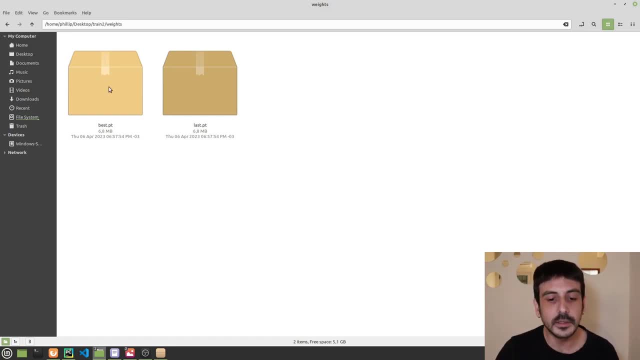 make inferences, and this is where your models will be located. this is where your models will be saved, and this is something i have already mentioned in one of my previous videos regarding yolo v8. remember, you will have two modules. one of them is called lastpt and the other one is bestpt. 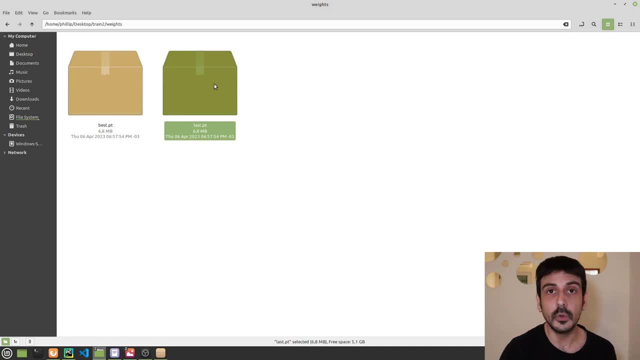 and the way it works is that. remember that when you are training a model, at the end of absolutely every single epoch, you are updating your weights, you are updating your model. so at the end of absolutely every single epoch, you already have a model which is available, which you can use it if you want to. so lastpt means that you are getting the last model, the 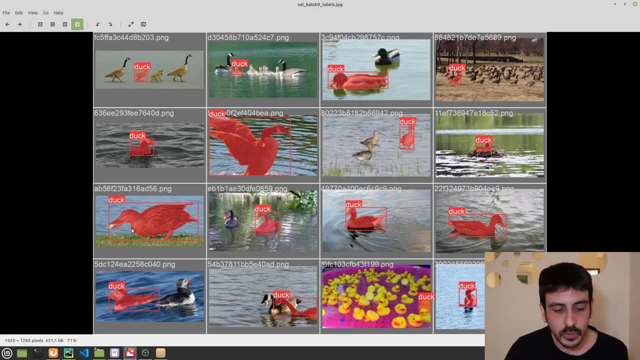 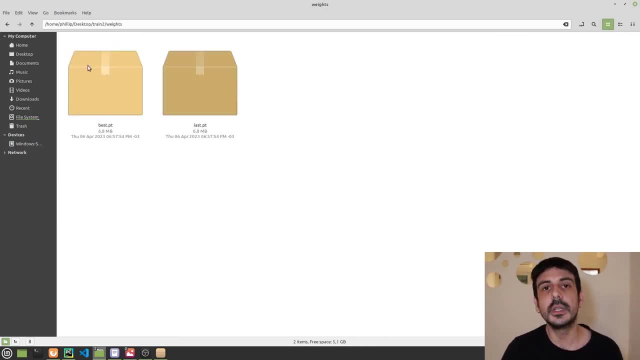 move forward with this project or with this training process. and now let me show you something else which is within this directory: the weights folder. this is where your weights will be located. right, because if you are training a model, it's because you want to train a model and you want to. 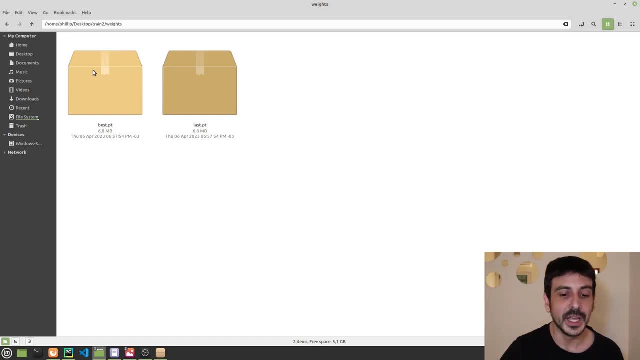 have a model in order to make predictions, in order to make inferences, and this is where your models will be located. this is where your models will be saved and this is something i have already mentioned in one of my previous videos regarding yellow v8. remember, you will have two modules: one: 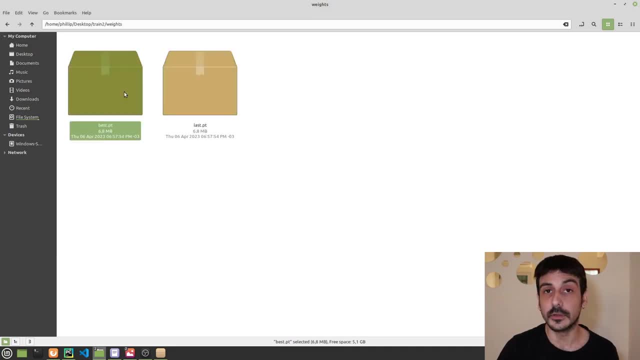 of them is called lastpt and the other one is bestpt, and the way it works is that remember that when you are training a model, at the end of absolutely every single epoch, you are updating your weights, you are updating your model. so at the end of absolutely every single epoch, you already have. 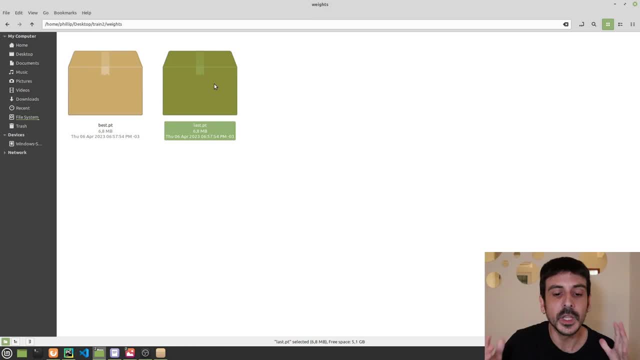 a module which is available, which you can use it if you want to. so lastpt means that you are getting the last model, the model you got at the end of your training process. so in this case i am training a network for 10 epochs, if i remember correctly. so this is the model we got at the end of the 10th. 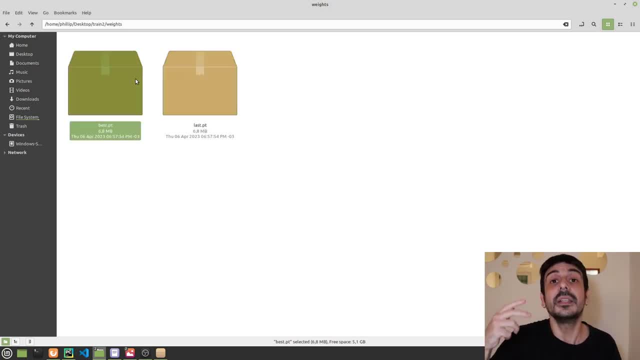 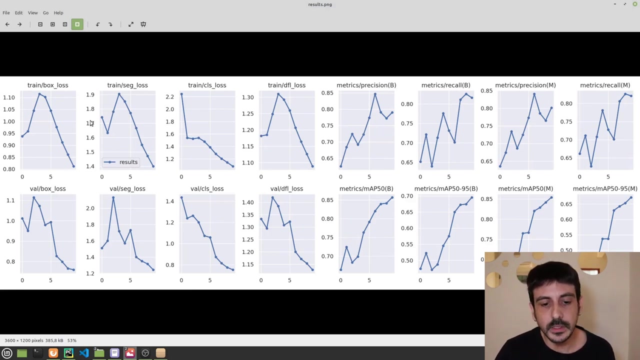 epoch and then bestpt means that you are getting the best model, the best model you train during the entire training process. if i show you the metrics again, let's see the metrics over here. you can see that we have many metrics which are related to the loss function and then other metrics related to the accuracy or how this model is performing. 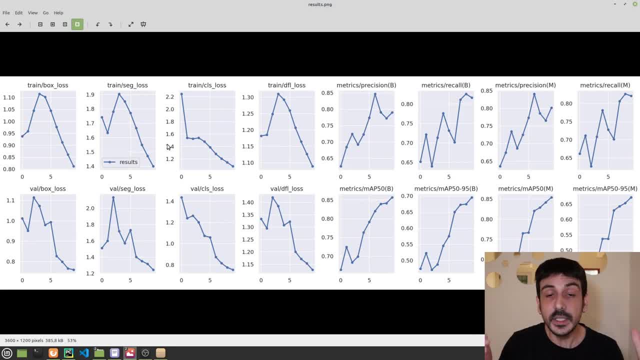 and the way yellow v8 decides what's the best model. in this case, which is a semantic segmentation type of problem, may be related to the loss function. maybe it's taking the model in which you got the minimum loss, or it may be related to some of these plots, some of these 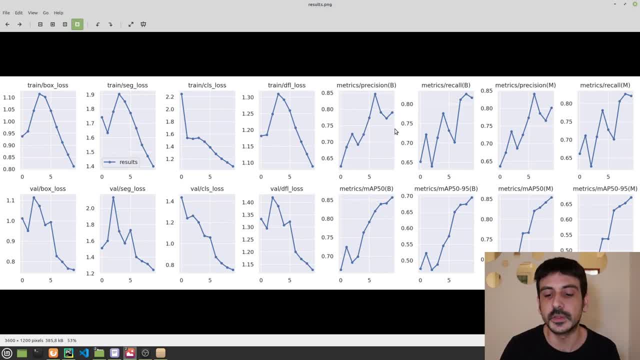 performances which are related to the accuracy, to the performance. maybe it's in the model for which you got the maximum precision, for example, or the maximum recall or something like that. i'm not 100 sure. i should look at the documentation, but the way it usually goes is that lastpt is. 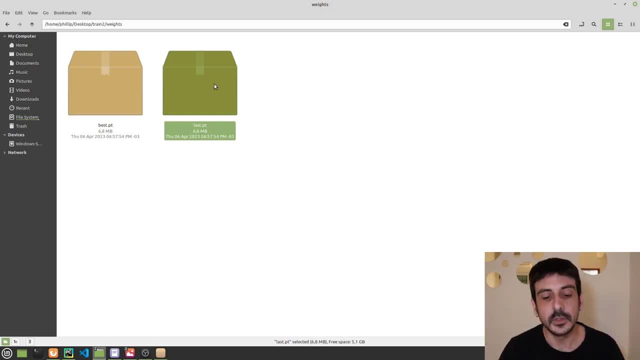 model you got at the end of your training process. so in this case i am training a network for for 10 epochs, if i remember correctly. so this is the model we got at the end of the 10th epoch and then bestpt means that you are getting the best model, the best model you train during the 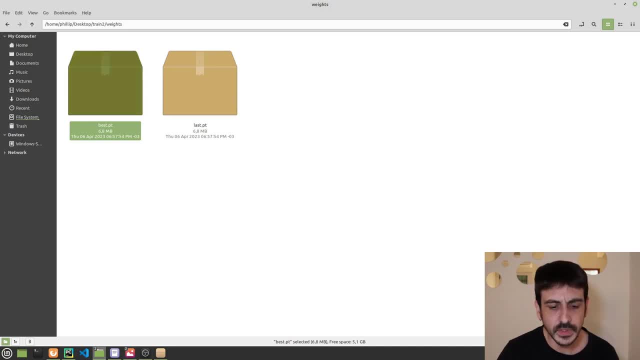 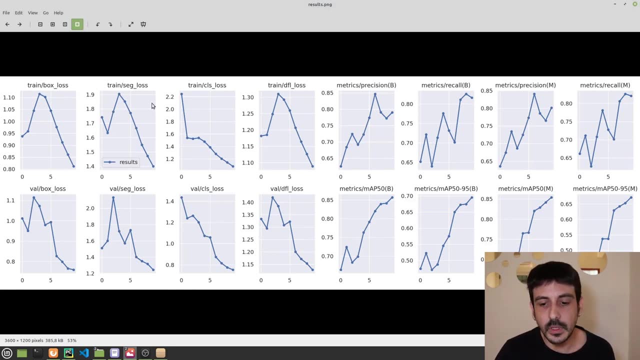 entire training process. if i show you the metrics again, let's see the metrics over here, you can see that we have many metrics which are related to the loss function and then other metrics related to the accuracy or how this model is performing and the way you will be able to design the model. 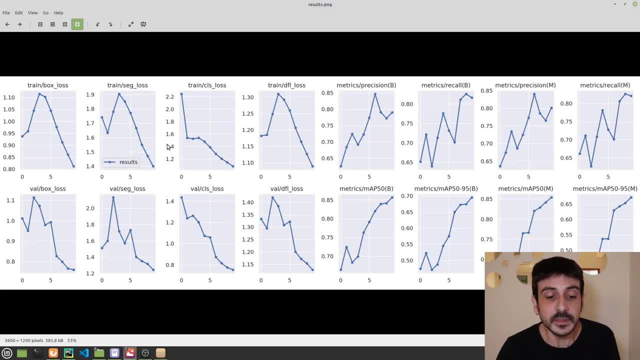 on that particular day. you know what's the best model in this case, which is a semantic segmentation type of problem, maybe related to the loss function, maybe it's taking the model in which you got the minimum loss, or it may be related to some of these plots, some of these performances which are related. 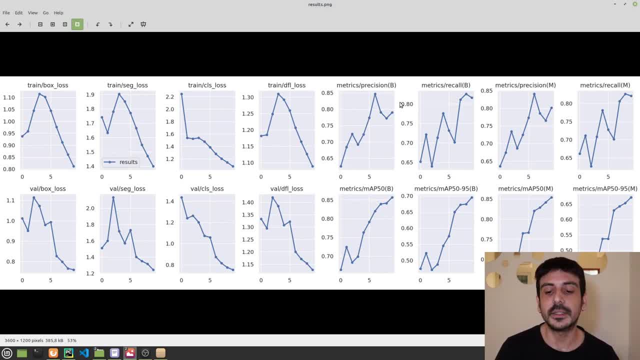 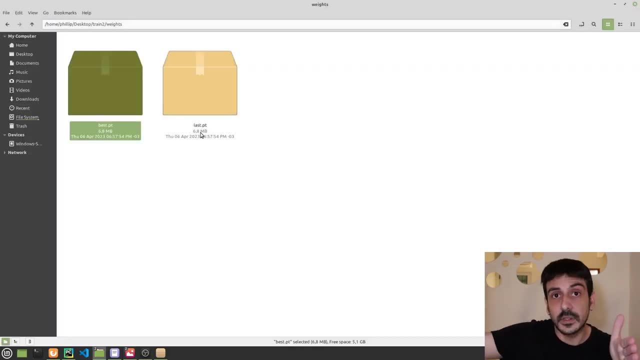 to the accuracy, to the performance. maybe it's getting the model for which you got the maximum precision, for example, or the maximum recall, or something like that. i'm not 100 sure. i should look at the documentation, but the way it usually goes is that lastpt is the last model you train, so it's at the end of 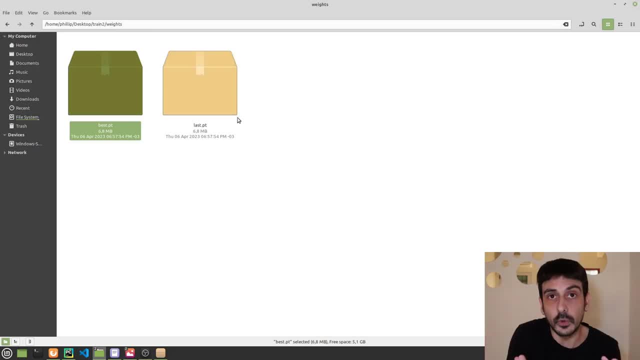 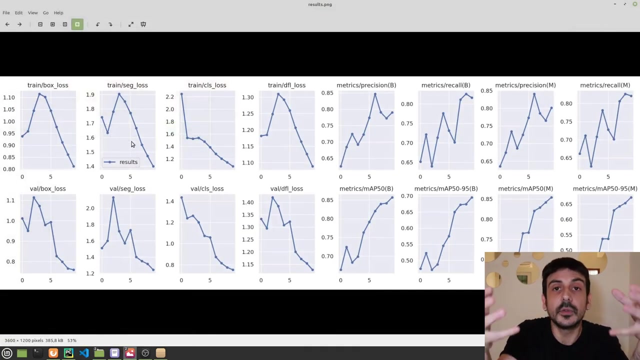 your training process and then bestpt is your best model, and this best model is decided under some criteria. so that's basically how it works, and what i usually do is taking lastpt, because i consider that lastpt is taking is considering way more information, much more information. 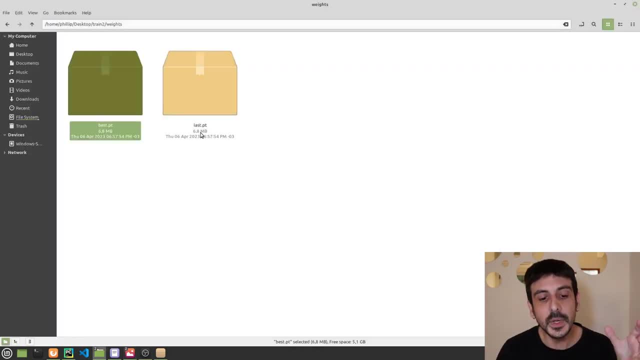 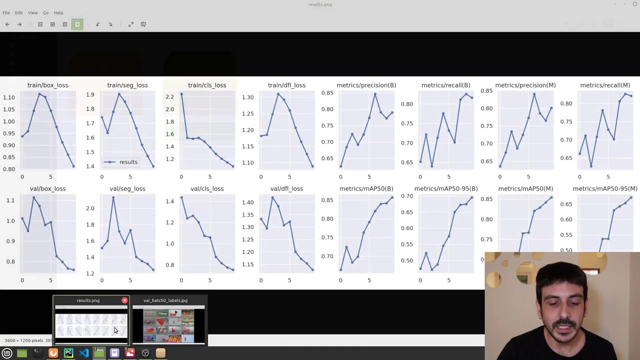 the last model you train, so it's at the end of your training process, and then basept is your best model, and this best model is decided under some criteria. so that's basically how it works, and what i usually do is taking lastpt, because i consider that lastpt is taking is. 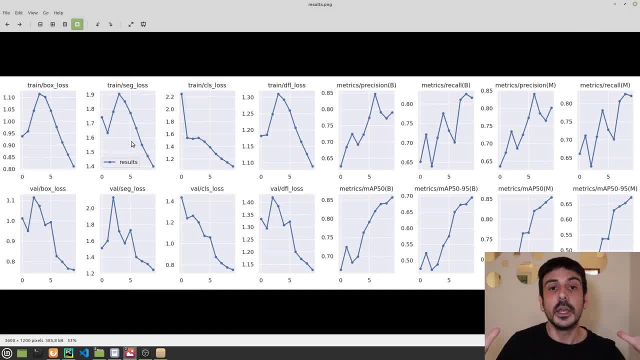 considering way more information, much more information, because we are taking much more data. we are taking much more everything right in all the training process. we are doing many, many different things. so the if you take the last model, you are summarizing way more information. that's the way i see it, so usually i take the last model. 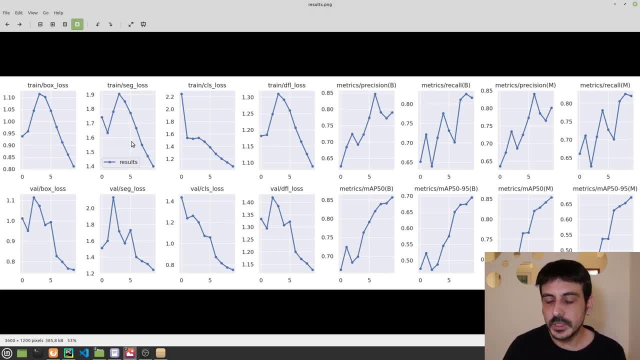 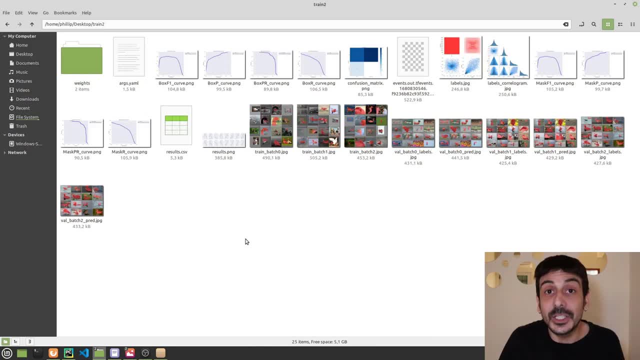 usually i take lastpt, and that's pretty much all, in order to show you this validation, how this validating this model looks like. and now let's move to the prediction. let's see how we can use this model in order to make inferences, in order to make predictions. so let's see how we can do that. 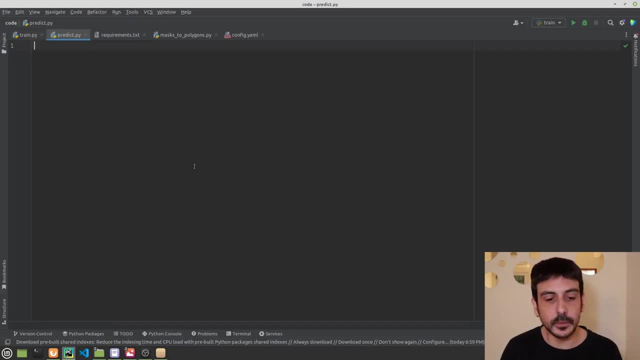 so let's go to pycharm, let's go to the pycharm project of today's video and let's see how we can do this tutorial. and this is a python script i created in order to do these predictions. this python file is called predictpi and this is what we are going to do. i'm going to start importing from: 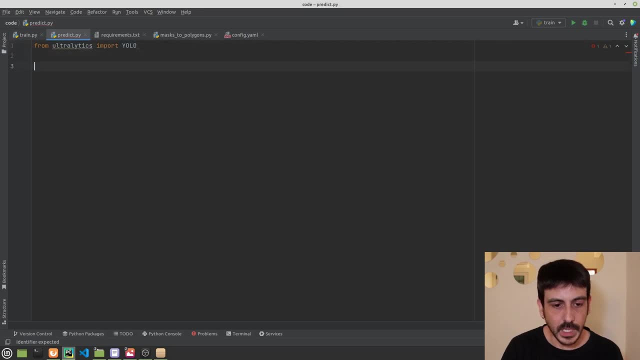 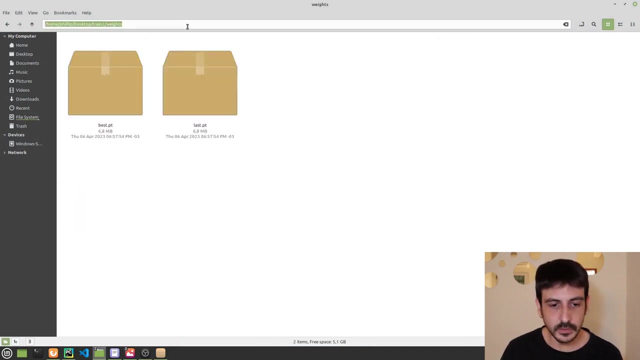 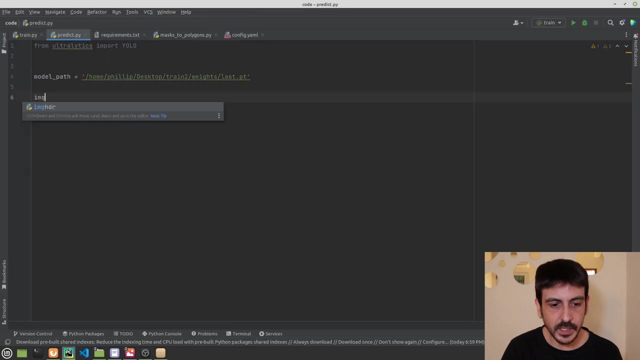 ultralytics, import yolo. and then i am going to define the model path, the model we are going to use, which, in our case, let's use lastpt, from these results, from this directory. so i'm going to specify something like this: lastpt, and then let's define an image path, let's define the image we are going. 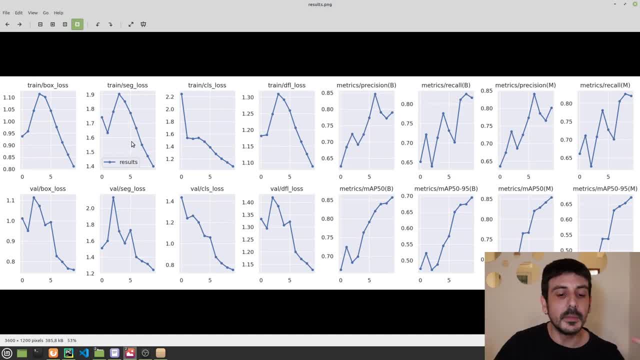 because we are taking much more data. we are taking much more everything right in all the training process. we are doing many, many different things. so the if you take the last model, you are summarizing way more information. that's the way i see it, so usually i take the last model, usually. 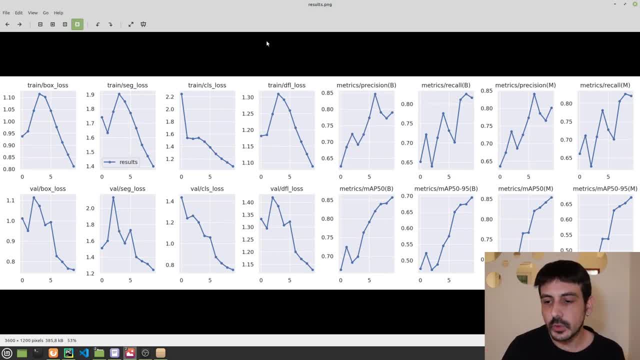 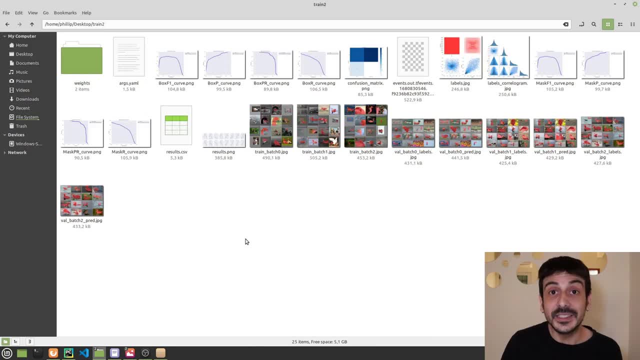 i take lastpt, and that's pretty much all, in order to show you this validation, how this validating this model looks like. and now let's move to the presentation. let's see how we can use this model in order to make inferences, in order to make predictions. 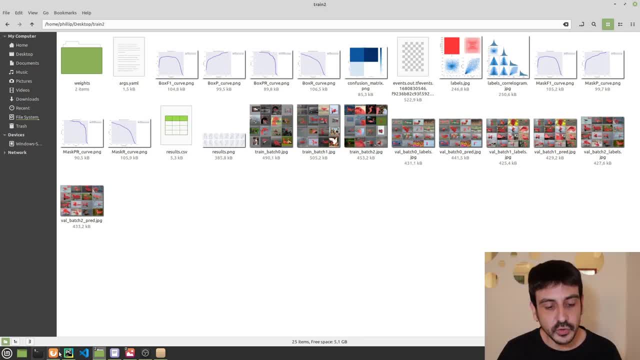 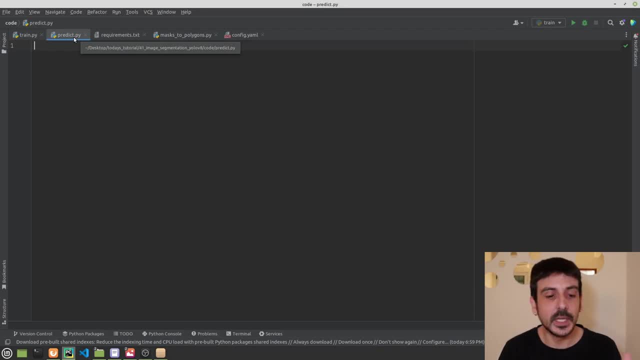 so let's see how we can do that. so let's go to pycharm. let's go to the pycharm project of today's tutorial, and this is a python script i created in order to do these predictions. this python file is called predictpi and this is what we are going to do. i'm going to start importing from ultralytics. 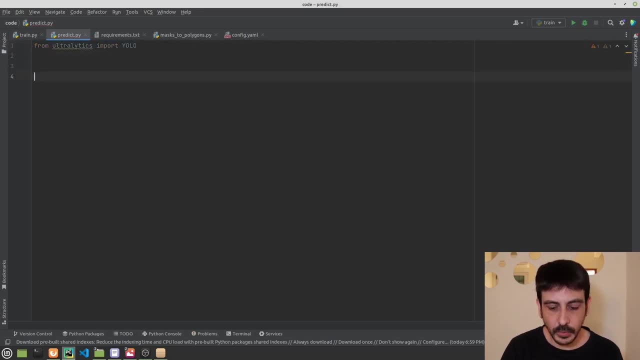 import yolo. and then i am going to define the prediction model path, the model we are going to use, which, in our case, let's use lastpt, from these results, from this directory. so i'm going to specify something like this: lastpt, and then let's define an image path, let's define the image we are going to use in. 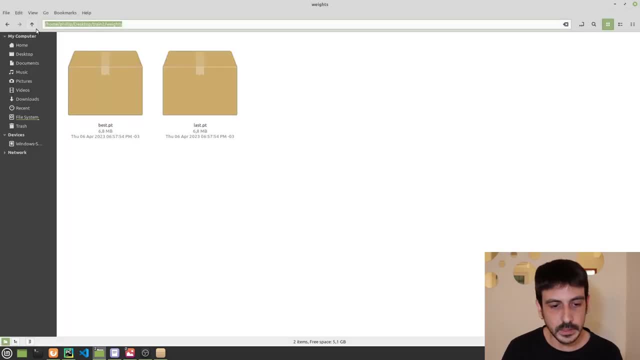 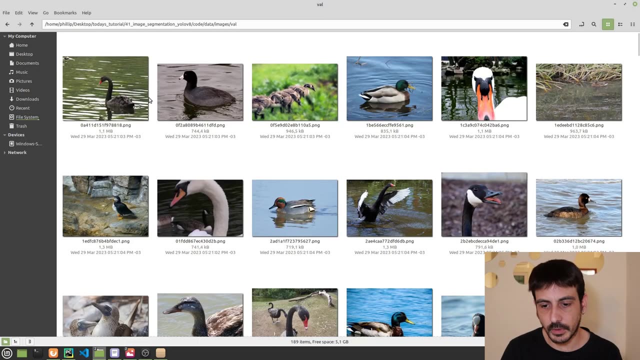 order to get our inferences. so the image will be located. this will be from the, from the validation section, and then we are going to define the image we are going to use in order to get our inferences set. i'm just going to choose a random image, something like this one. so i am going to 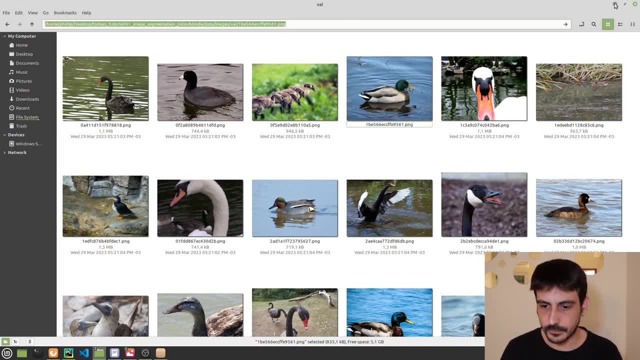 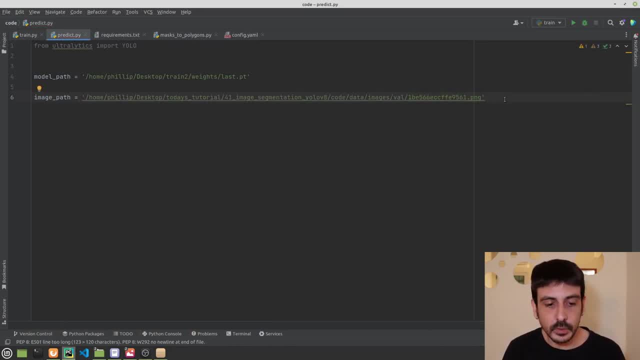 copy paste and i'm just going to paste it here. so this is the image we are going to use in order to test this model, in order to make our predictions. and now i'm going to import cv2 as well, because i'm going to open. i'm going to read this image: 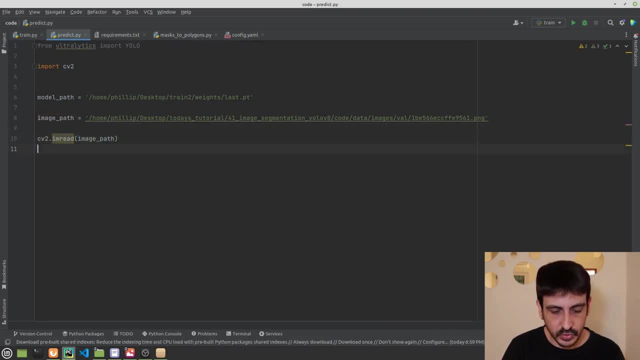 and then i am going to get this image shape. so this will be something like this: this will be image, and then this is image dot shape. okay, and now the only thing we need to do is to get or model by doing something like yolo and then model path. 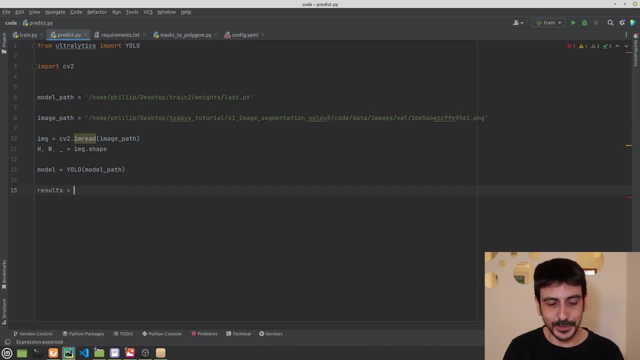 okay, and then we are going to get the results by calling model of our image. right, and this is it. this is all we need to do in order to get all results, in order to get our inferences. but now let's do something else. i am going to iterate for result in results, and now let's. 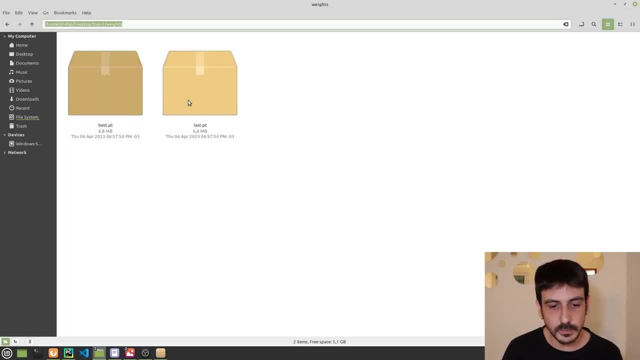 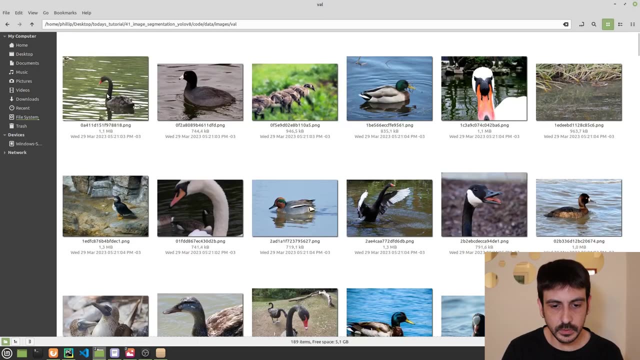 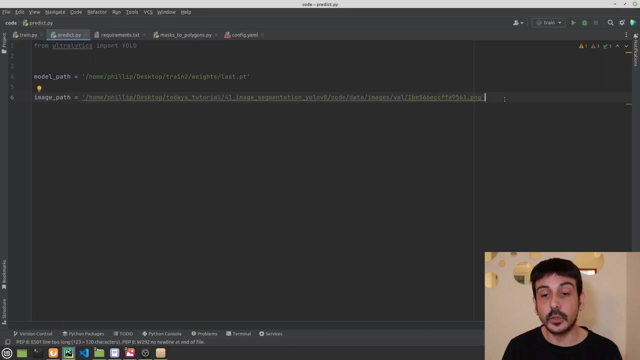 to use in order to get our inferences. so the image will be located. this will be from the, from the validation set. i'm just going to choose a random image, something like this one. so i am going to copy paste and i'm just going to paste it here. so this is the image we are going to use in order to 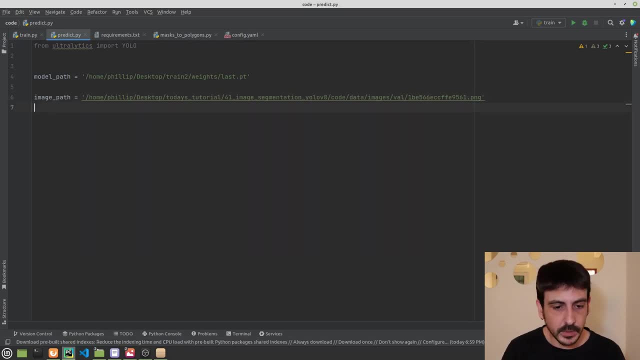 test this mode in order to make our predictions. and now i'm going to import cv2 as well, because i'm going to open, i'm going to read this image and then i am going to get this image shape. so this will be something like this. this will be: 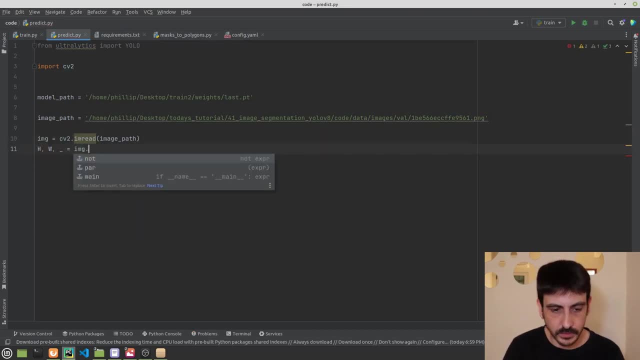 image, and then this is image dot shape: okay, and now the only thing we need to do is to get our model by doing something like yolo and then model path: okay, and then we are going to get the results by calling model of our image. right, and this is it. 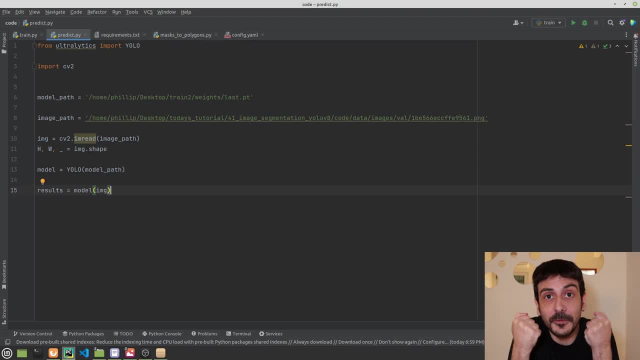 this is all we need to do in order to get all results, in order to get our inferences. but now let's do something else. i am going to iterate for result in results, and now let's take a look at this mask, let's take a look at this prediction. 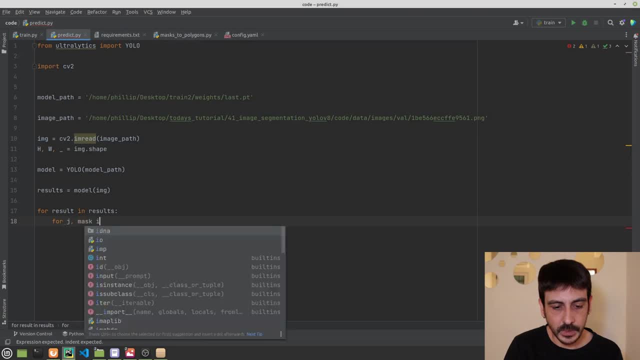 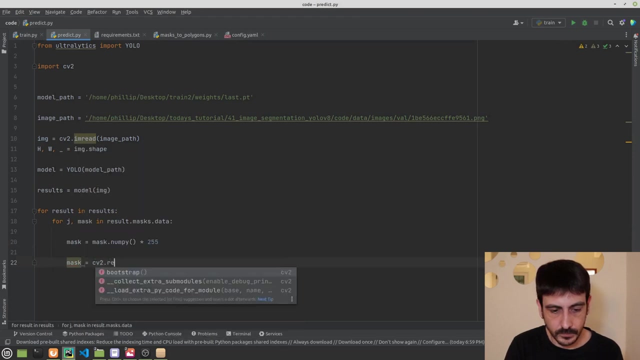 so i'm going to iterate like this for j mask in result dot masks, dot data, and then i am going to say something like mask dot numpy times 255, and this is our mask, and then i am going to resize it to the size of the image. so i'm going to input the mask. 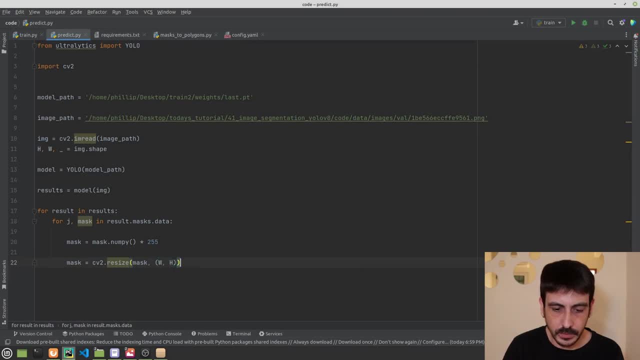 and then this will be. if i'm not mistaken, the order is this: one w and then h. so this is just the way it works. this, this is how we need to do it in order to get the prediction, and then in order to resize this prediction back to the size of the original image. 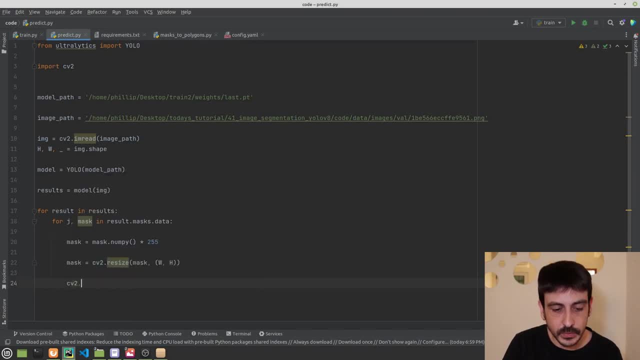 so this is how it goes, and now the only thing we need to do is to call cv2 img. right, and i'm going to save it. i'm going to save it here and the name will be something like that: let's call it output. this is only a test, so we don't really need to go crazy with the name. let's get. 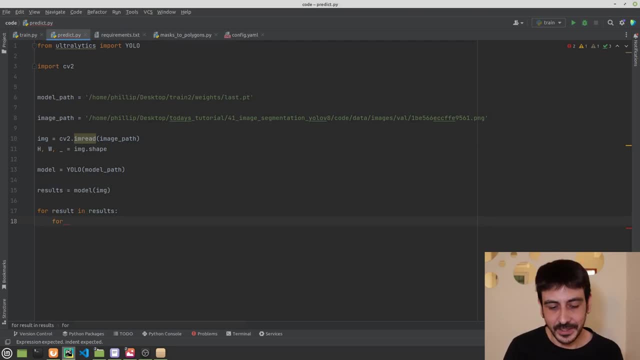 take a look at this mask. let's take a look at this prediction. so i'm going to iterate like this: 4j mask in result: dot masks, dot data. and then i am going to say something like mask dot numpy 255 and this is our mask, and then i am going to resize it. 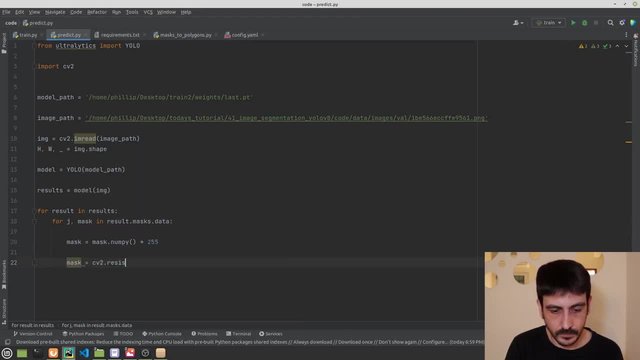 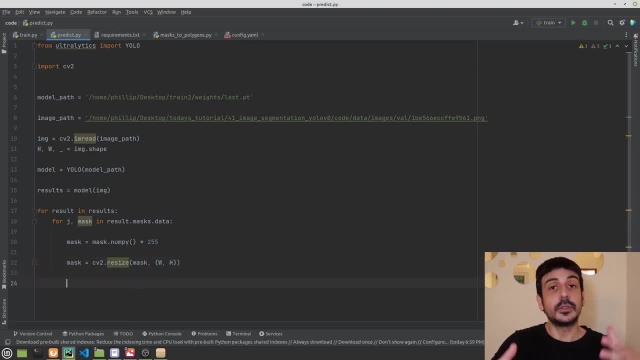 order is this: one w and then h. so this is just the way it works. this, this is how we need to do it in order to get the prediction and then in order to resize this prediction back to the size of the original image. so this is how it goes, and now the only thing we need to do is to call cv2. 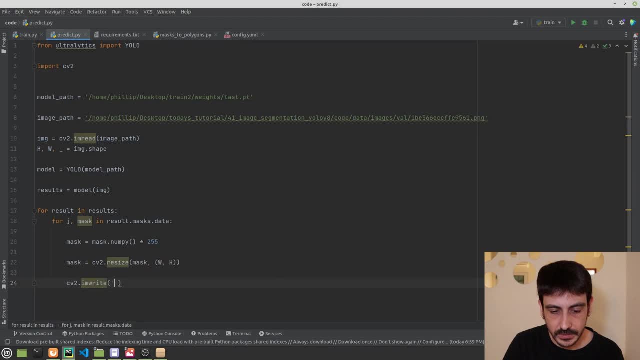 img right, and I'm going to save it. I'm going to save it here and the name will be something like that: let's call it output. this is only a test, so we don't really need to go crazy with the name. let's call it outputpng and this will be our mask, and that's pretty much all that's pretty. 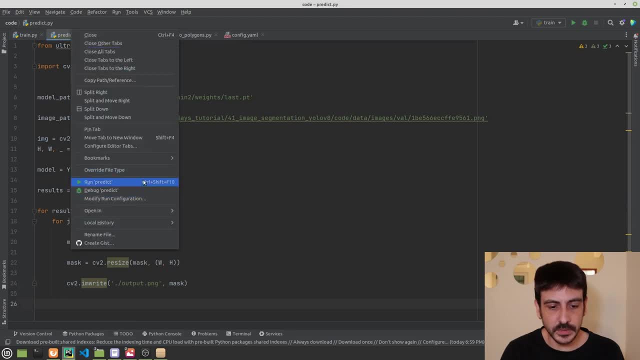 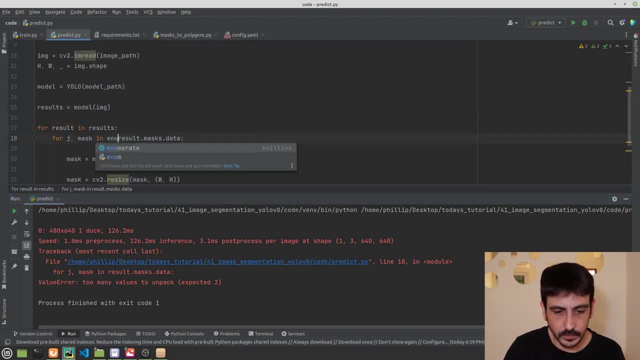 much all. let's see what happens. I'm going to press play, let's see if everything is okay or if we have some error. okay, so I did, I'm going to press play and I'm going to an error and yeah, this is because we need to enumerate. i forgot the enumerate. we are not. 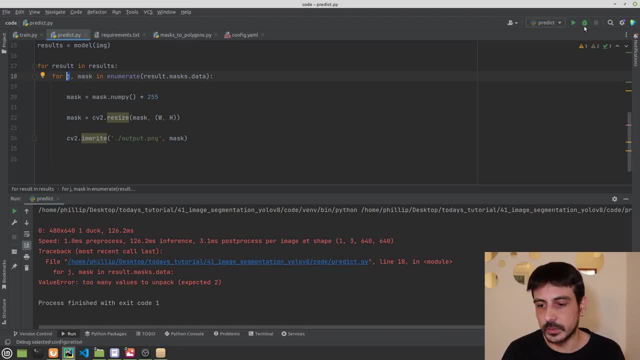 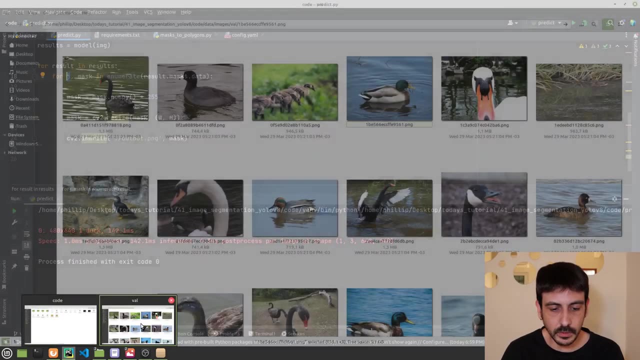 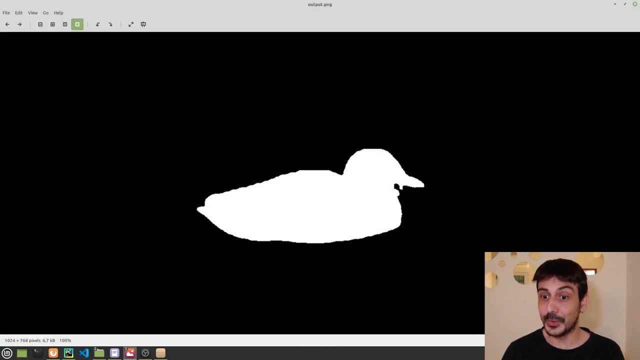 using j actually, so i could just iterate in mask, but let's do it like this. okay, everything run smoothly, everything is okay, we didn't get any error. and now, if i go back to this folder, to this directory, i can see: this is the output. this is the output we got. and now, in order to make 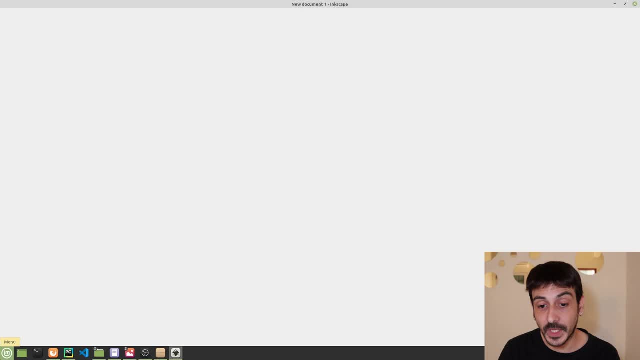 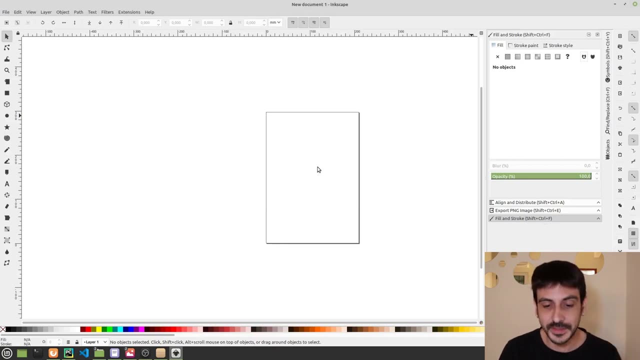 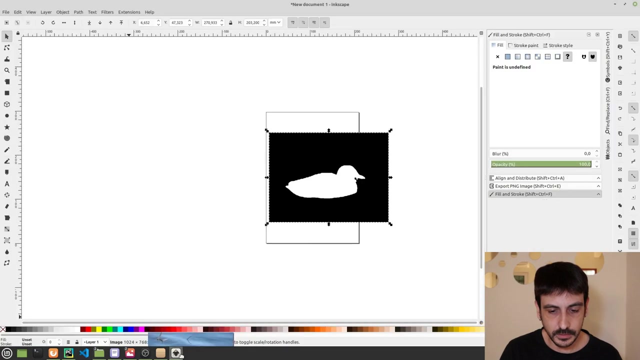 absolutely 100. sure, everything is okay and this is a good mask. this is a good prediction. i'm going to make an overlay. i'm very excited. i don't know if you can tell, but i'm very excited. i'm just going to take this image over here and then i'm going back here and i'm going to take the 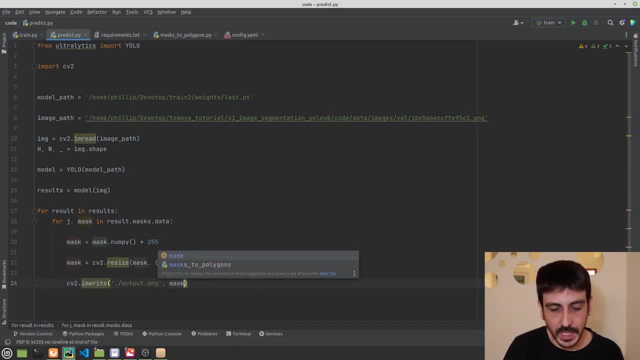 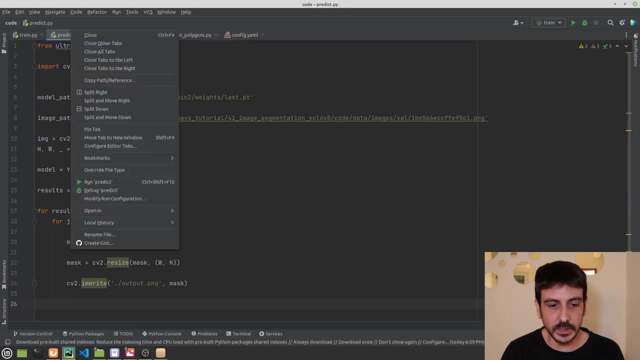 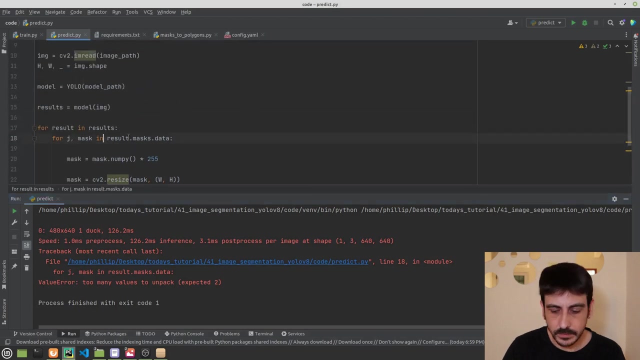 let's call it outputpng and this will be our mask, and that's pretty much all. that's pretty much all. let's see what happens. i'm going to press play. let's see if everything is okay or if we have some error. okay, so i did get an error and, yeah, this is because we need to enumerate. i forgot the enumerate. 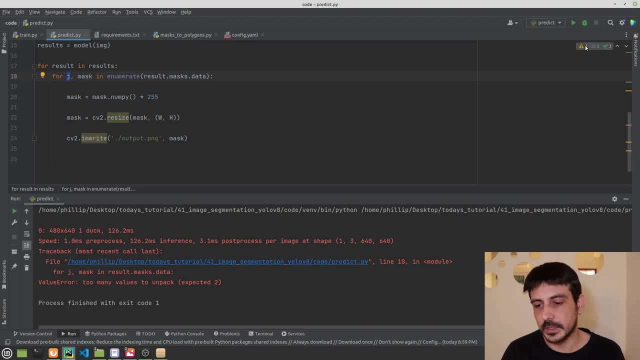 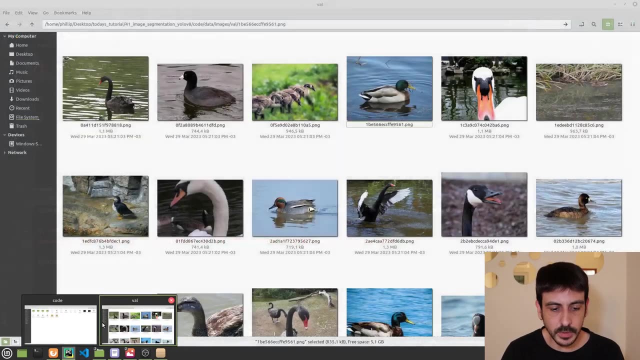 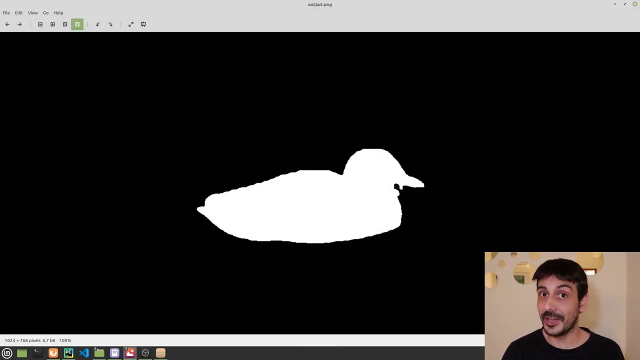 we are not using j actually, so i could just iterate in mask, but let's do it like this. okay, everything run smoothly, everything is okay, we didn't get any error. and now, if i go back to this folder, to this directory, i can see: this is the output. this is the output we got. 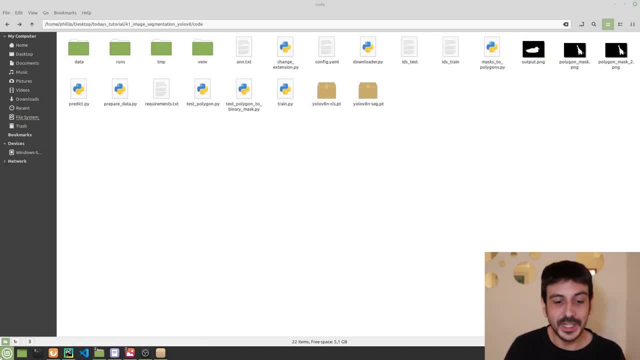 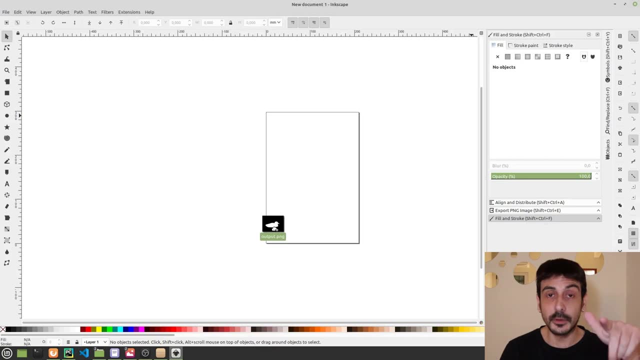 and now, in order to make absolutely a 100: sure, everything is okay and this is a good mask, this is a good prediction. i'm going to make an overlay. i'm very excited. i don't know if you can tell, but i'm very excited. i'm just going to take this image over here and then i'm going back here. 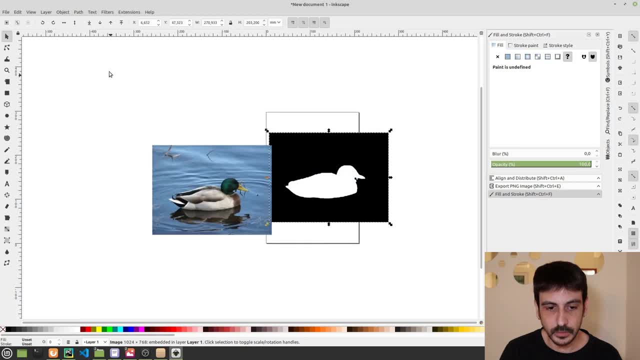 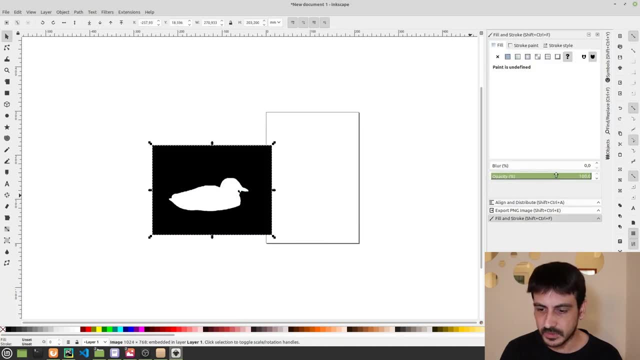 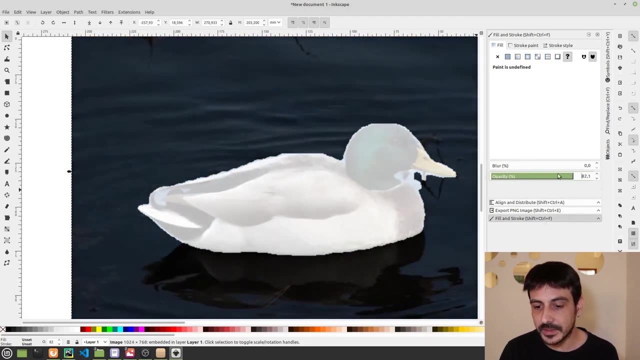 and i'm going to take the original image. i'm going to do an overlay, so this will be raised to top. i'm going to align these two images together and now let's make a transparency and let's see what happens, and you can see that we may not get like a 100 perfect mask, but it's pretty. 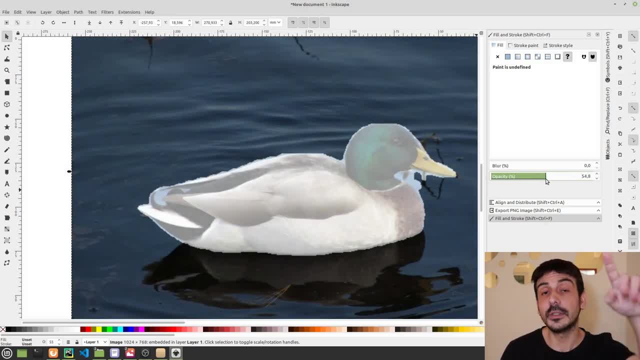 well, it's like a very, very good mask, especially considering the errors we detected in our data. so this is amazing. this is, this is uh, this is a very good detection. this is a very, very good result. so this is going to be all for this tutorial, and this is exactly how you can train. 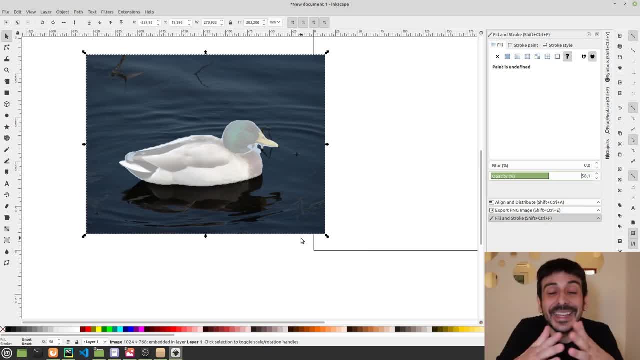 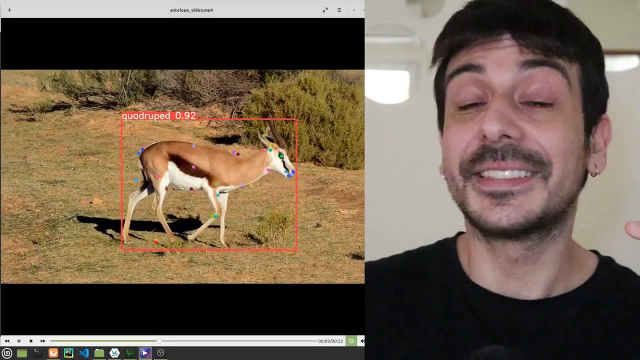 a semantic segmentation model using yolo v8 and is the entire process, from how to annotate the data, how to train the model and how to validate this model, and then how to make some predictions. so this is going to be all for today, so this is exactly what you will be able to. 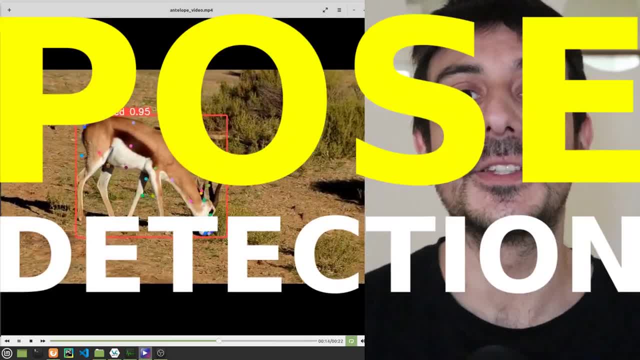 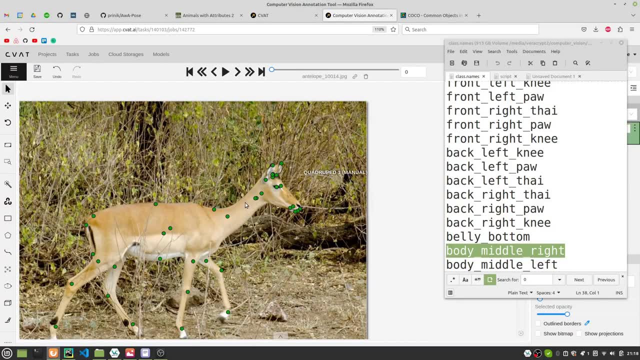 do with today's tutorial. in this video, we're going to work with post detection using yolo v8 and i'm going to show you the entire process, from how to annotate your custom data for free using a computer vision annotation tool, how to prepare your data and your file system for 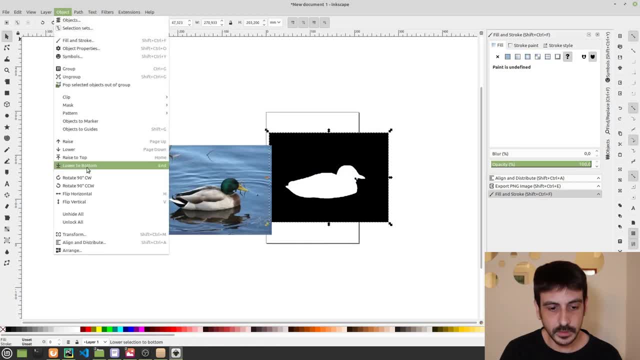 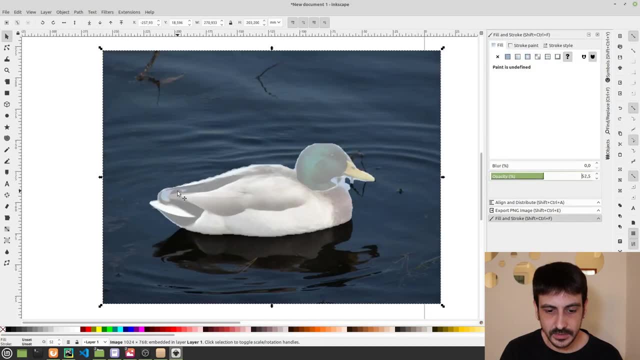 original image. i'm going to do an overlay, so this will be raised to top. i'm going to align these two images together and now let's make a transparency and let's see what happens and you can see that this is the original image and you can see that the image is now going to be. 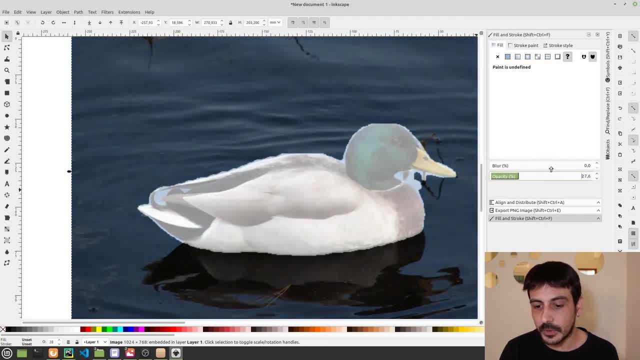 see that we may not get like a 100 perfect mask, but it's pretty well. it's like a very, very good mask, especially considering the errors we detected in our data. so this is amazing. this is, this is, this is a very good detection. this is a very good result. so this is going to be all for this. 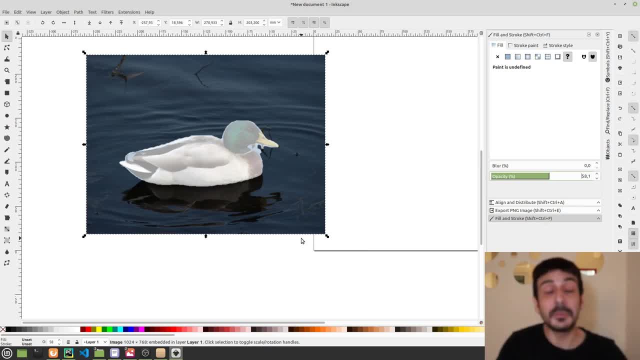 tutorial and this is exactly how you can train a semantic segmentation model using yolo v8, and is the entire process, from how to annotate the data, how to train the model and how to validate this model, and then how to make some predictions. so this is going to be all for today. 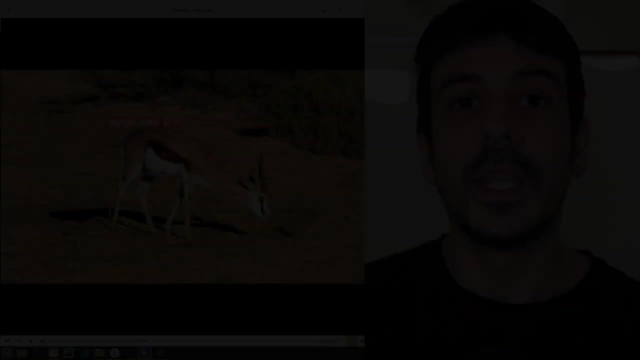 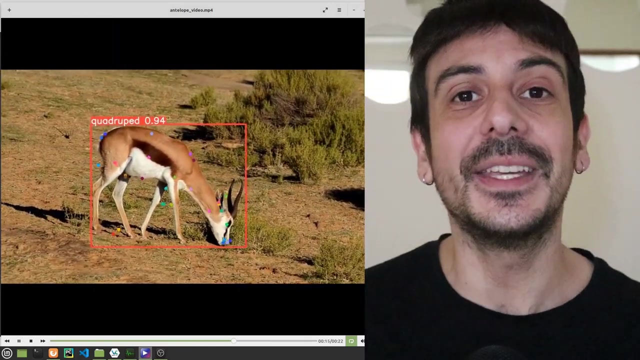 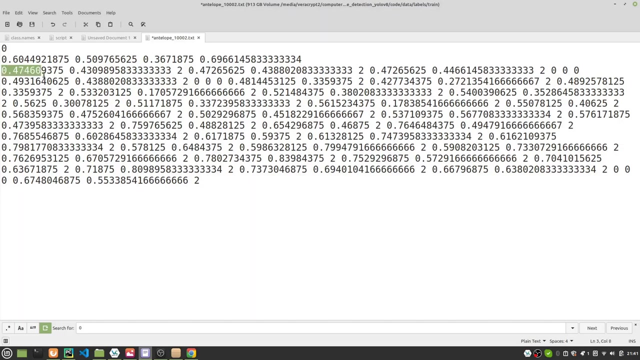 so this is exactly what you will be able to do with today's tutorial. in this video, we're going to work with post detection using yolo v8, and i'm going to show you the entire process, from how to annotate your custom data for free using a computer vision annotation tool, how to prepare your data. 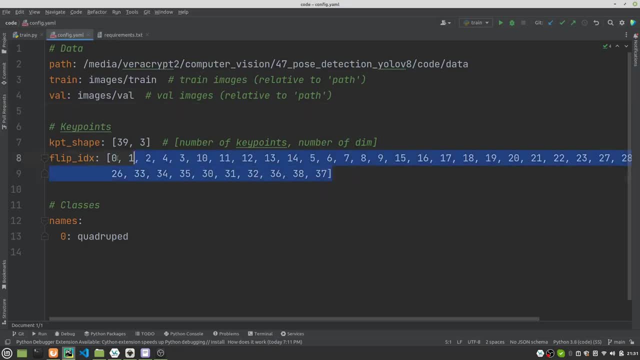 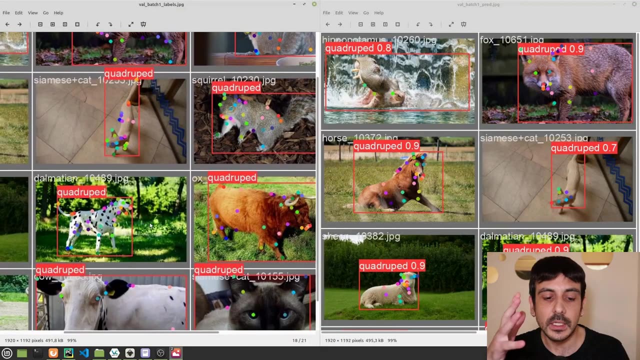 and your files system for training this post detector, how to training in your local computer and also from a google call up, and how to do a super comprehensive evaluation of the model you trained. this is a much more complex problem. in my previous tutorials i show you how to train an image classifier using 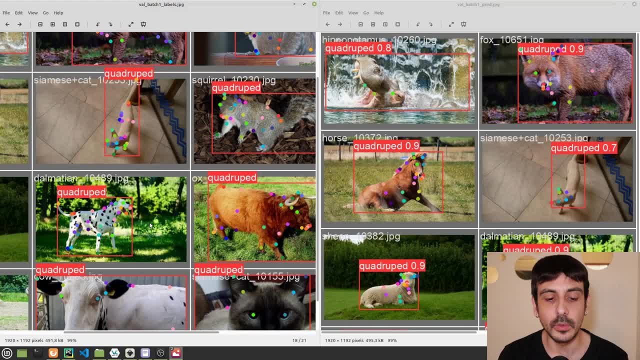 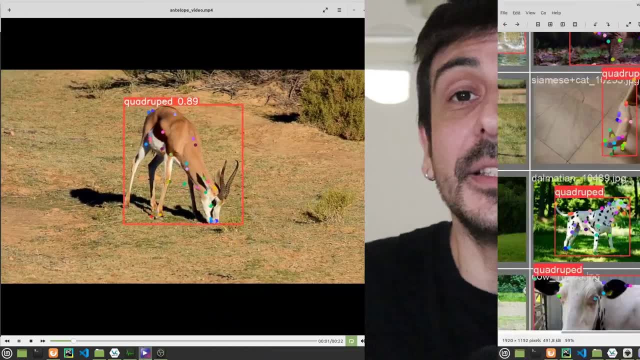 yolo v8, an object detector and an image segmentation model, and i would say that today's model, this key point detector, is much more complex than everything we did before. this is going to be an amazing tutorial. my name is Felipe. welcome to my channel. and now let's get started. and now let me keep on pratique. 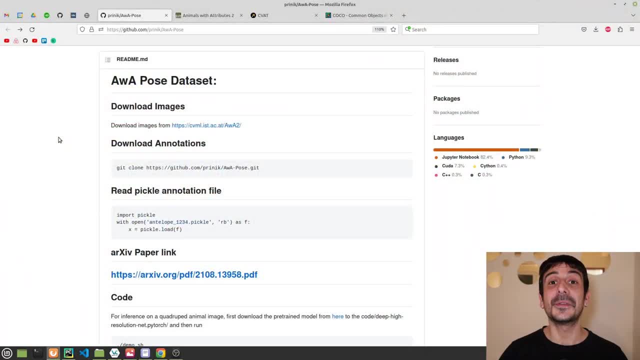 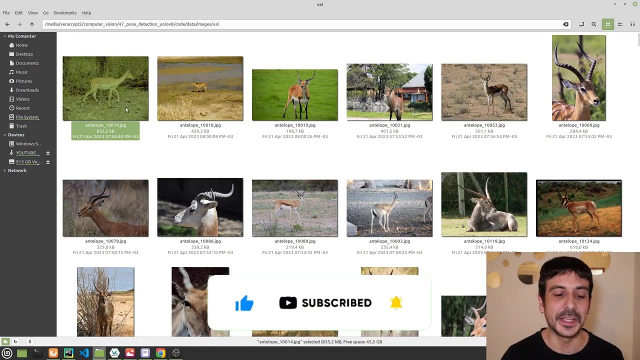 give us one more useful step. and now let me show you the data we are going to use on this tutorial. we are going to use the awa post data set and let me show you exactly how this data looks like. so you can see that these are pictures of many. 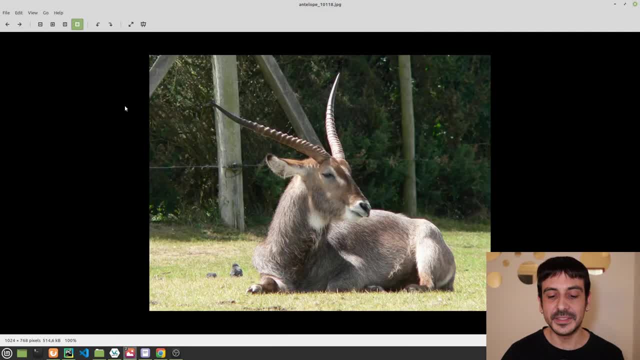 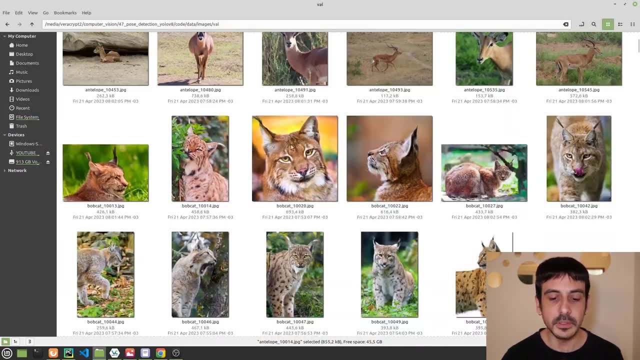 different animals. currently we are looking at antelopes. these are pictures of many different antelopes and if i scroll down in this directory, you are going to see i also have other animals. for example, here this is a bobcat, which is some sort of faidline, some sort of animal. uh, we're even ANTLAPS. 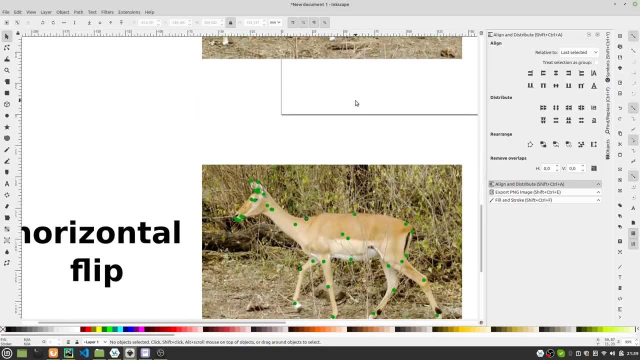 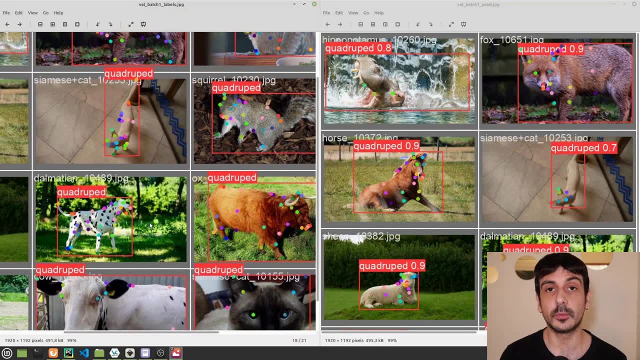 training this post detector, how to training in your local computer and also from a google collab, and how to do a super comprehensive evaluation of the model you trained. this is a much more complex problem. in my previous tutorials i show you how to train an image classifier using yolo v8. 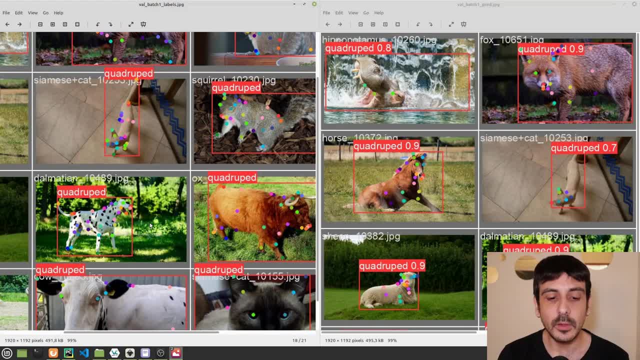 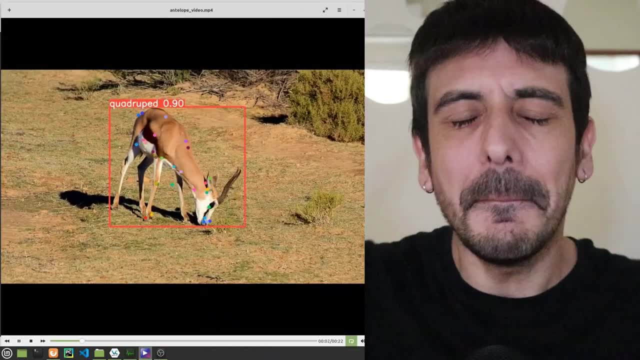 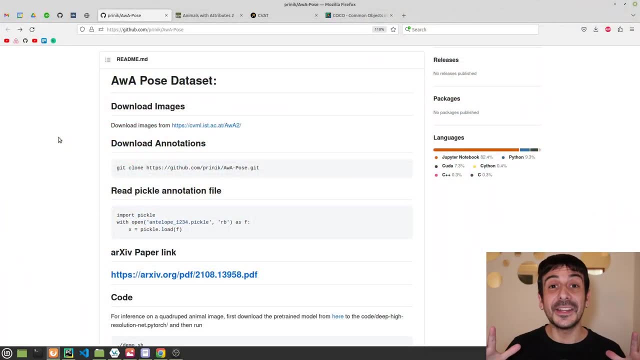 an object detector and an image segmentation model, and i would say that today's model, this key point detector, is much more complex than everything we did before. this is going to be an amazing tutorial. my name is Felipe. welcome to my channel. and now let's get started. and now let me show you the data we are going to use on this tutorial. we're going to use 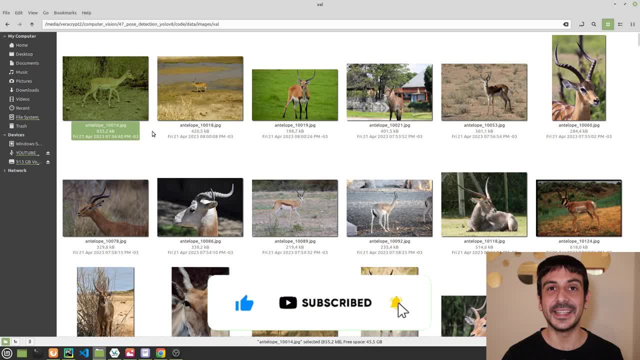 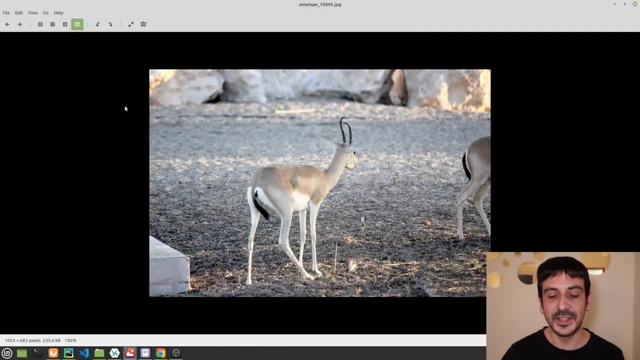 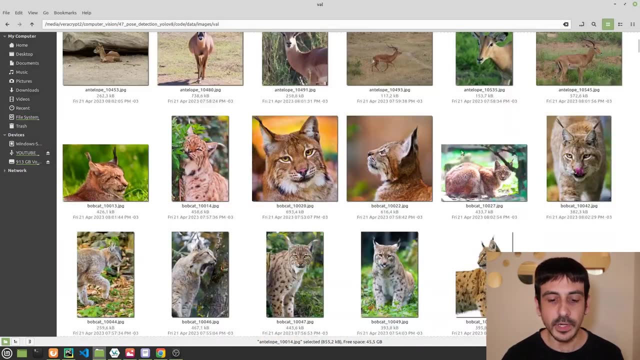 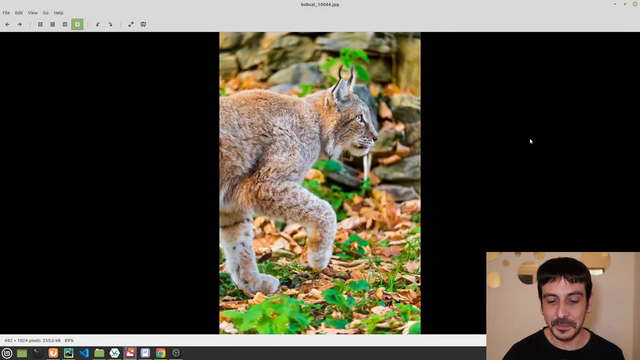 the awa post data set and let me show you exactly how this data looks like, so you can see. these are pictures of many different animals. currently we are looking at antelopes. these are pictures of many different animals in the land filled�os, which is just sort of a. 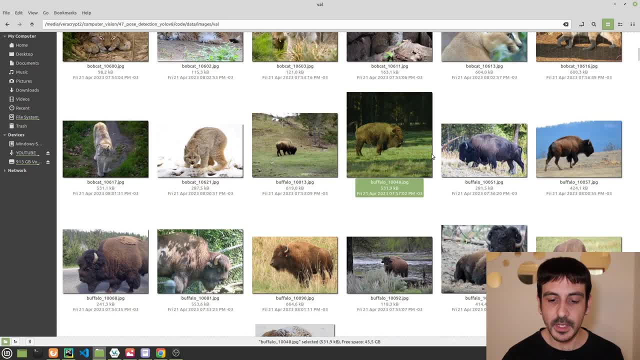 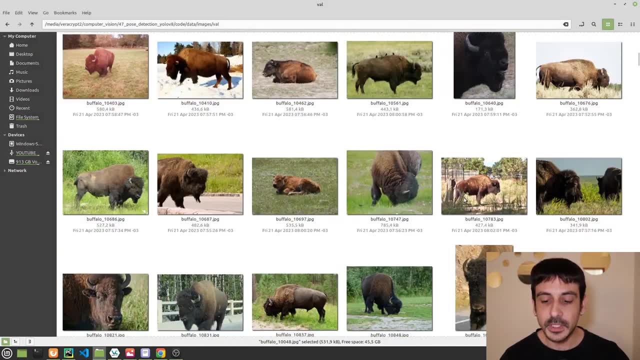 combination of aliens: cole frogs, which is a eigenlijk chihuahua, which means may, Gileh and 알룞, and, as you heard the name of it on the card for the grains distribution app, I'm going to create a new class on all the animals myself, so we will have a class with an animal that is a. 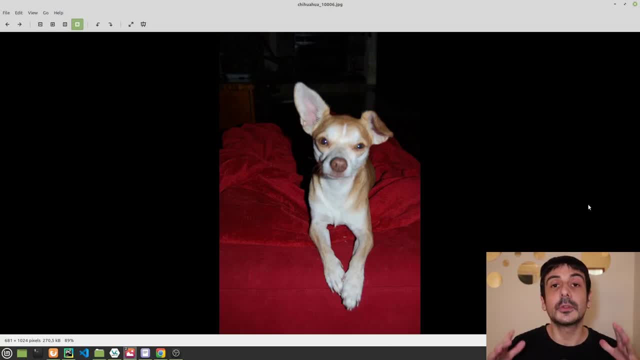 example, here I have a Chihuahua and you get the idea right. we have pictures of many, many, many different animals, and all these animals are quadrupeds because this is a quadruped keypoint detection data set. now let me show you the key points we are going to be detecting for each one. 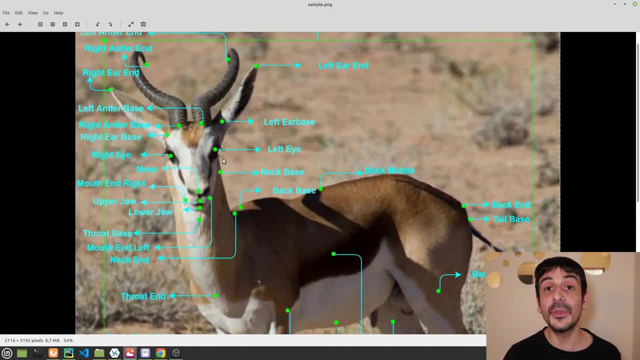 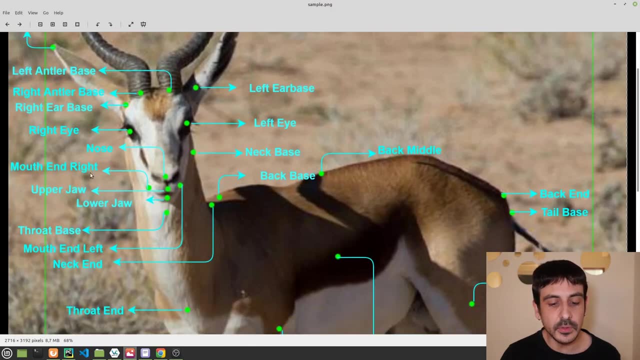 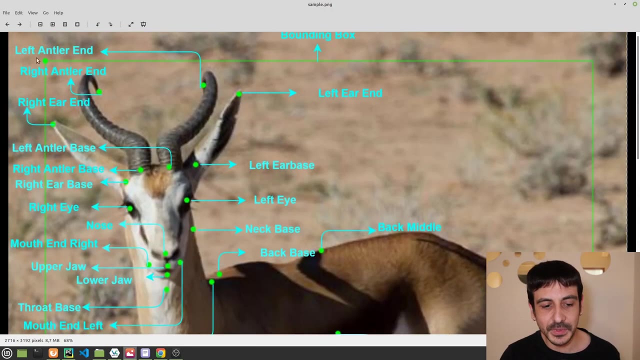 of these animals and you can see that these are many, many different key points. we have 39 key points in total, which is a lot, and we are detecting many different parts, for example, the nose, the eyes, the jaw, the tail, the legs, and also the ears, the horns or whatever they're called, something like. 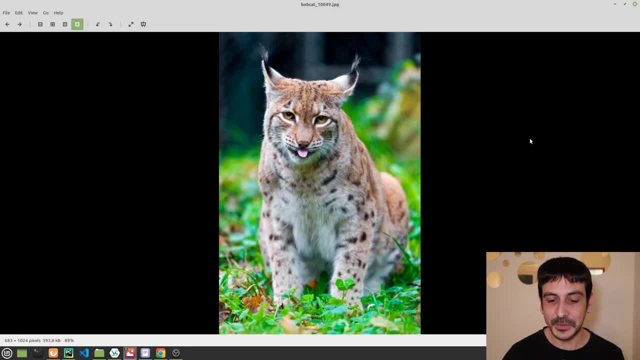 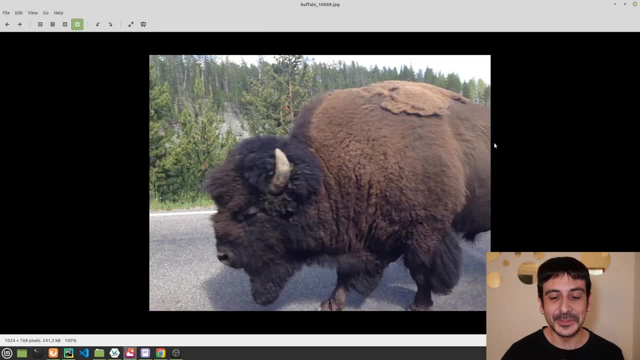 feline, some sort of cat. you can see that these are many different pictures of this animal and if i scroll down a little more, you are going to see i also have buffaloes. so we also have pictures of buffaloes and if i continue scrolling down, you are going to see other pictures of other animals. 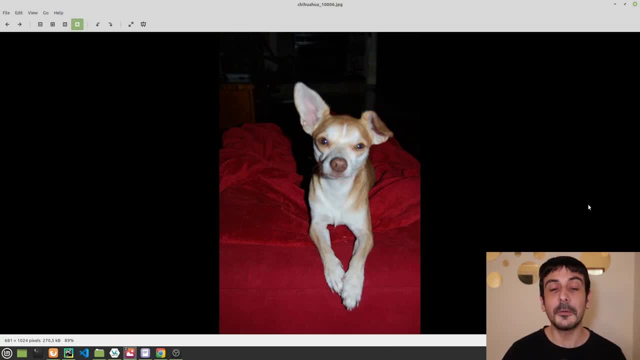 for example, here i have a chihuahua and you get the idea right. we have pictures of many, many, many different animals, and all these animals are quadrupeds because this is a quadruped keypoint detection data set. now let me show you the key points we are going to be detecting for each one. 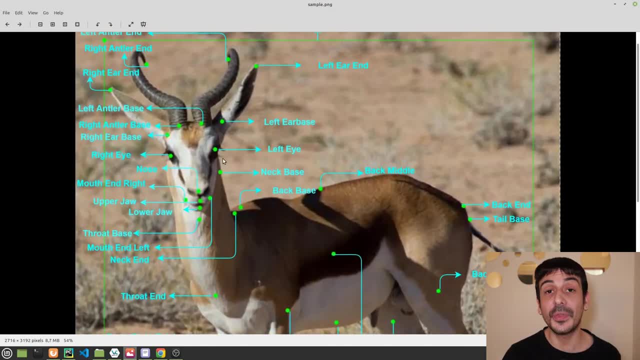 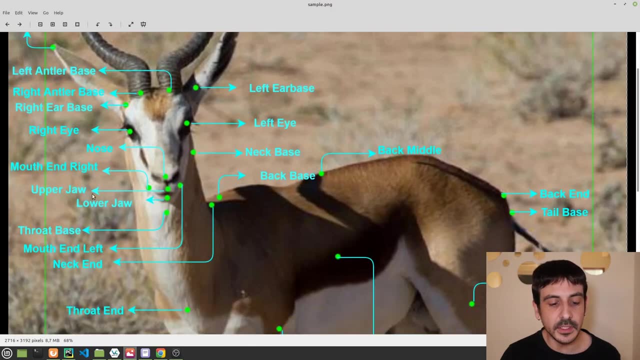 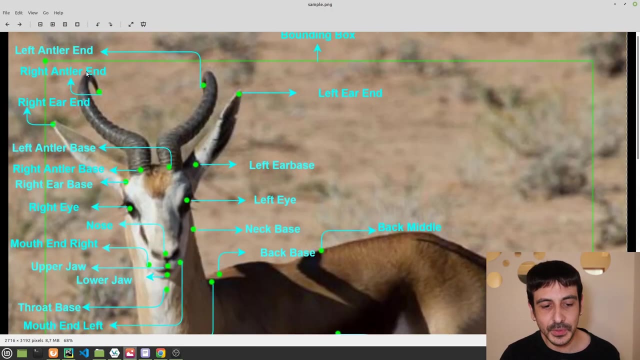 of these animals and you can see that these are many, many different key points. we have 39 key points in total, which is a lot, and we are detecting many different parts, for example, the nose, the eyes, the jaw, the tail, the legs, and also the ears, the horns or whatever they're called, something like. 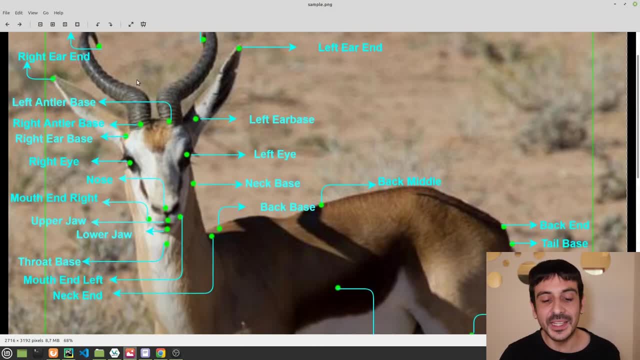 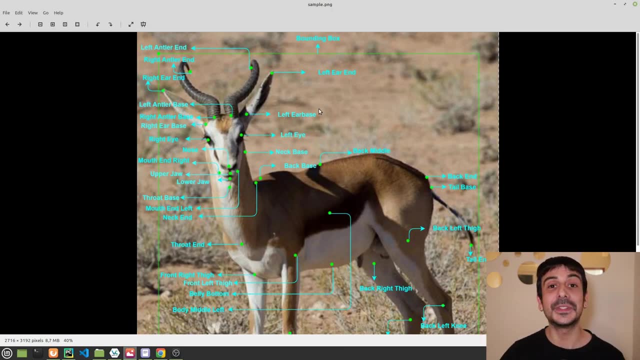 antler, it doesn't matter. we are detecting many, many different parts in these quadrupeds, so this is exactly the data we are going to be using today. i thought it was like a very, very good asset to use in post detection. and now let's continue. so i'm going to show you how to do the entire process of training. 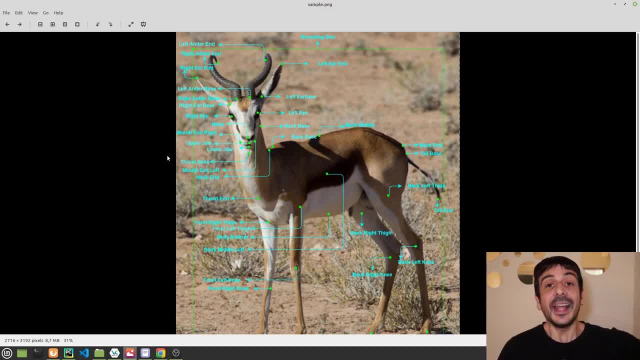 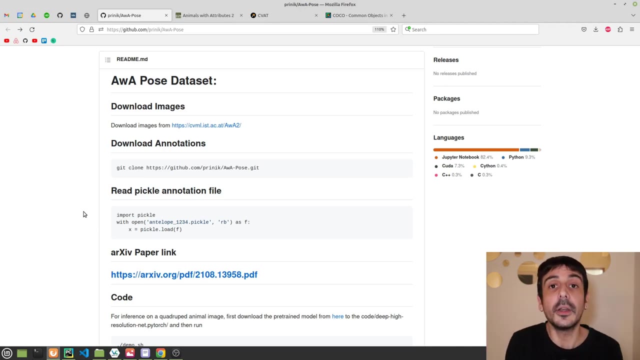 a post detector using yolo v8 on your custom data and in my case, the data i am going to use in this tutorial is already annotated, right? so i already have the annotations for this data. but if you are training this post detector on your custom data, then most likely you will need to annotate the 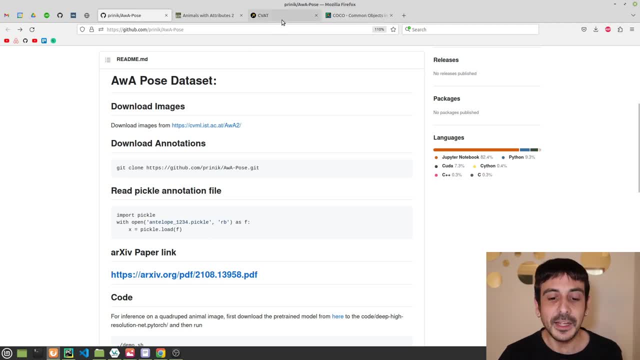 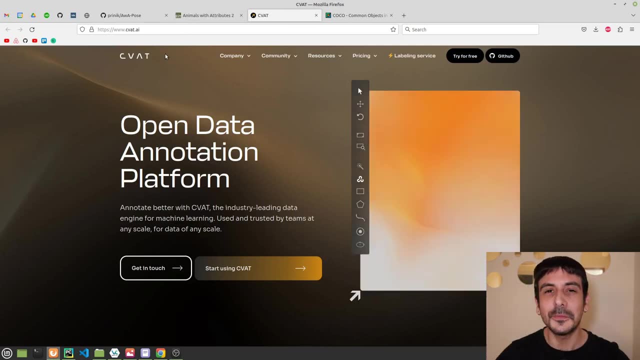 data yourself. so i'm going to show you how to do this and i'm going to show you how to do this in this video. i'm going to show you how you can do that. i'm going to show you how to do the entire annotation process using cvit, which is a very, very popular and a very awesome annotation tool for computer. 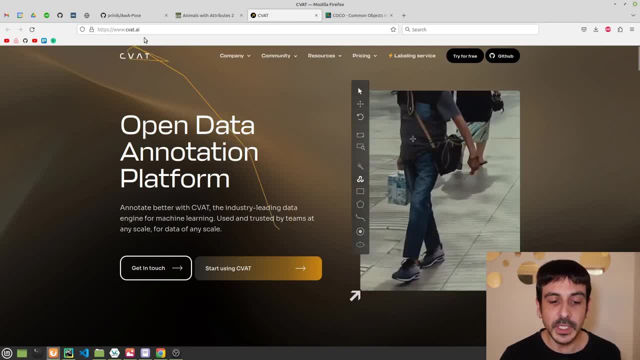 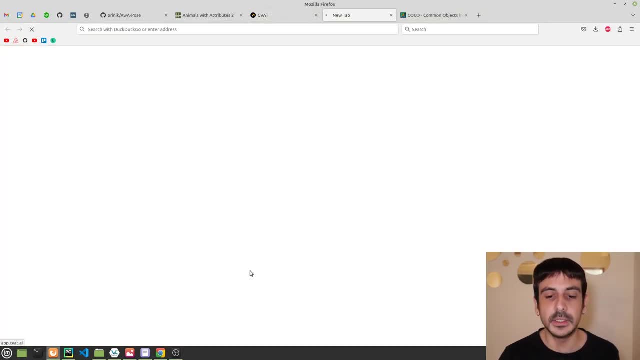 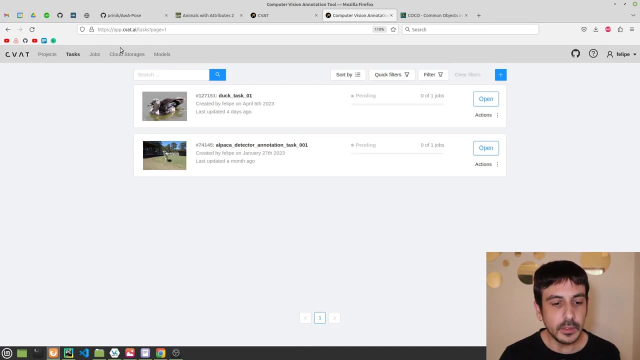 vision and let me show you how to do it. so i'm going to cvitai. this is cvit website and i'm going to click here where it says start using cvit. i'm going to show you how to create a project, how to create a task and how to do all the annotation. now i'm going to projects. 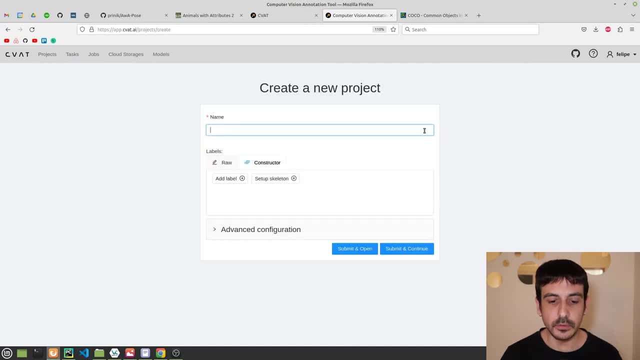 i'm going to click on the plus button, i'm going to click here and create a new project and this is going to be keypoint detection. this is going to be quadruple keypoint detection, which is exactly what we are going to be doing. then add label and i'm going to add quadruple continue. 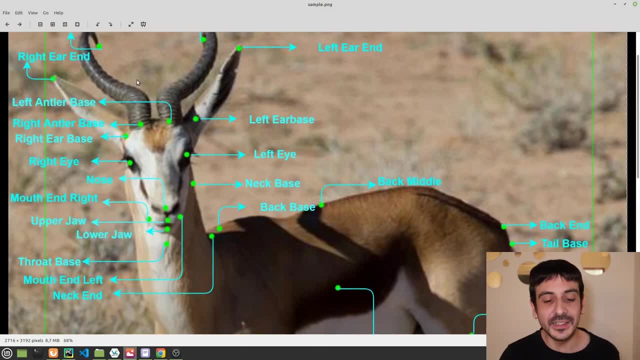 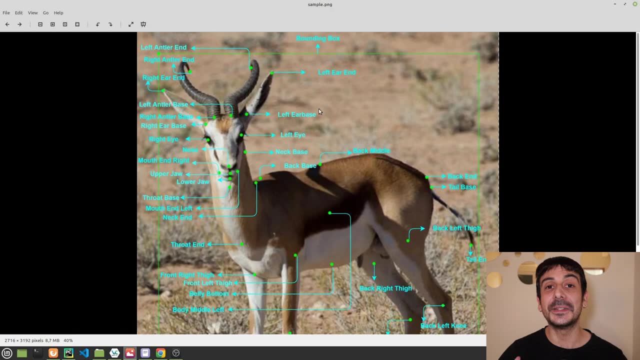 antler, it doesn't matter. we are detecting many, many different parts in these quadrupeds. so this exactly the date that we are going to be using today. I thought it was like a very, very cool asset to use in post detection. and now let's continue. so I'm going to show you how to do. 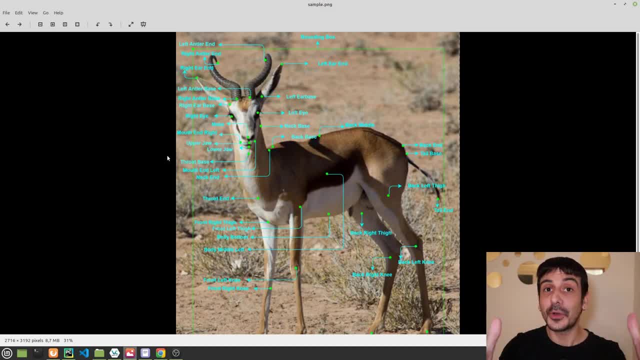 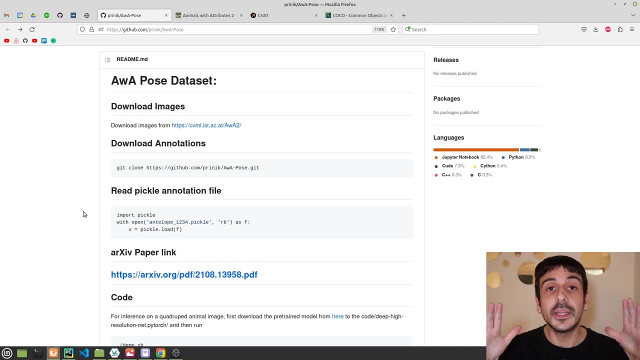 the entire process of training a post detector using YOLOv8 on your custom data and in my case, the data going to use in this tutorial is already annotated, right? so i already have the annotations for this data. but if you are training this post detector on your custom data, then most likely you will need to. 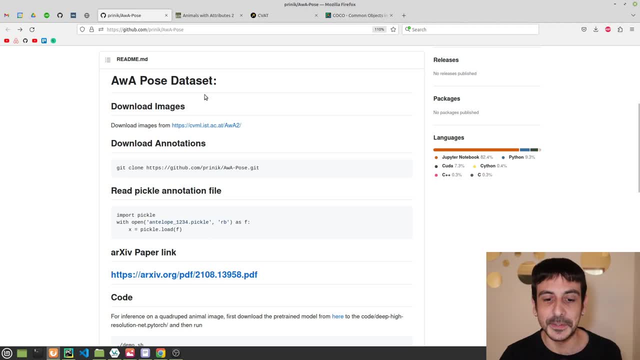 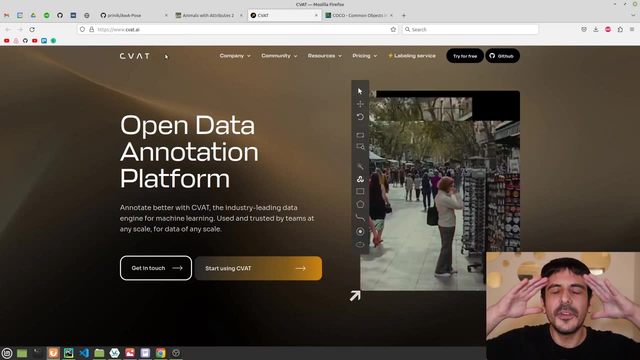 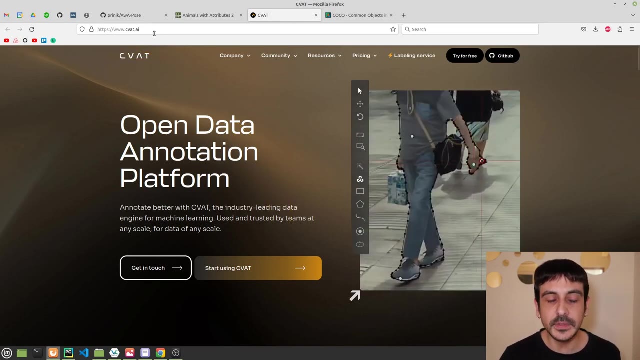 annotate the data yourself. so i'm going to show you how you can do that. i'm going to show you how to do the entire annotation process to using cvit, which is a very, very popular and a very awesome annotation tool for computer vision, and let me show you how to do it. so i'm going to cvitai. 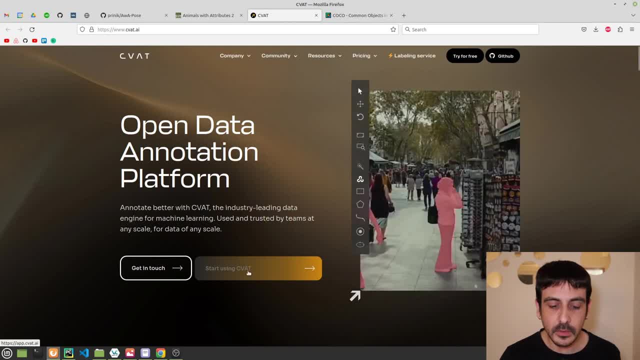 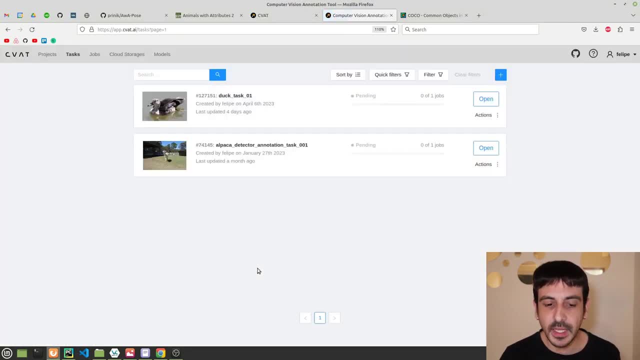 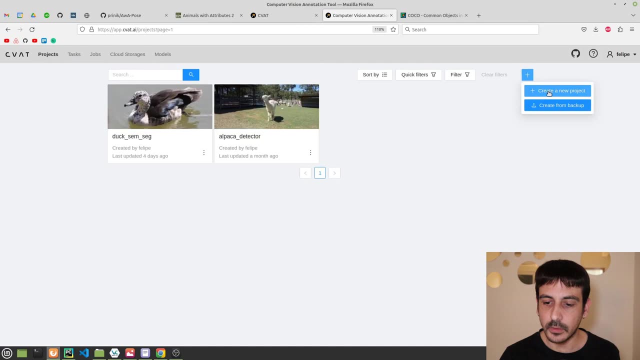 this is cvit website and i'm going to click here where it says start using cvit. i'm going to show you how to create a project, how to create a task and how to all the annotation. now i'm going to projects and i'm going to click the plus button. i'm 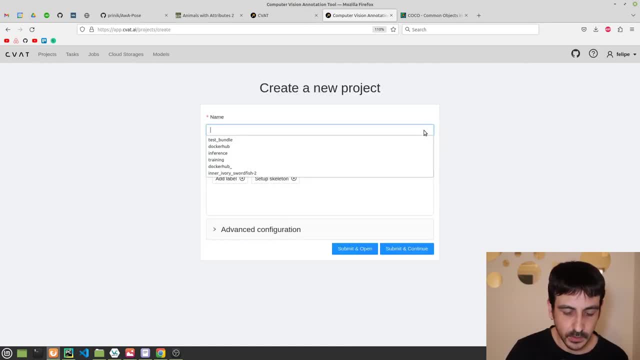 going to click here and create new project, and this is going to be key point detection. this is going to be quadruped key point detection, which is exactly what we are going to be doing. then add label and i'm going to add quadruped continue and that's pretty much all. submit another. 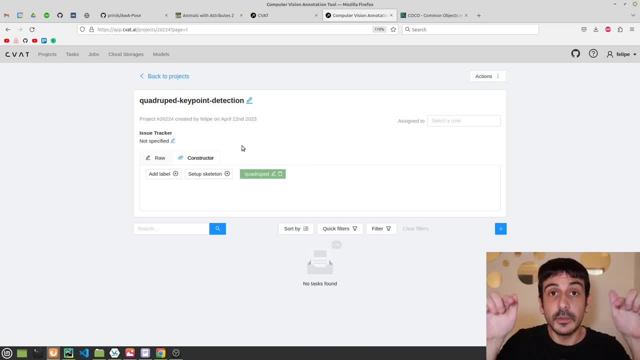 this is where you are going to add absolutely all the labels you have in your custom data. in my case, i only have one label, which is quadruped. now. let's continue. now i'm going to create a task, create new task. the name of this task: 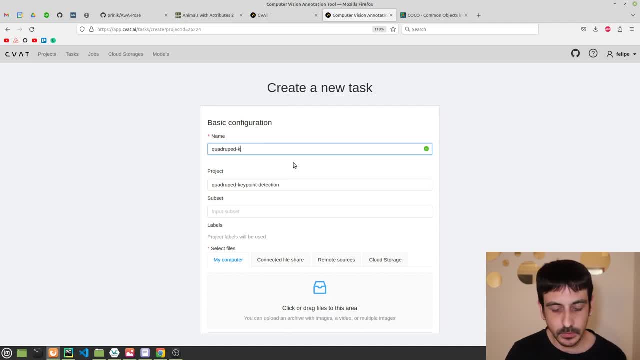 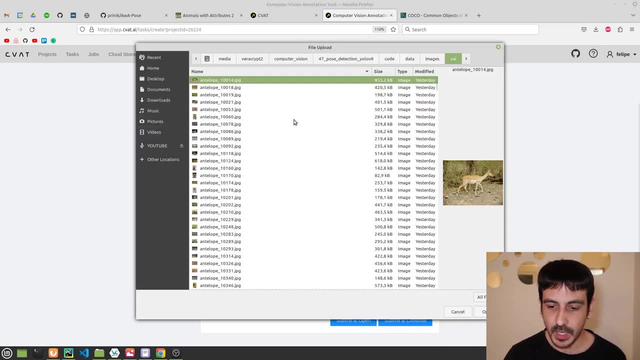 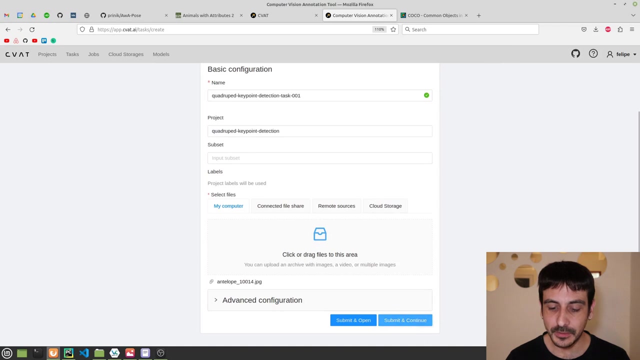 will be something like quadruped keypoint detection, task 001, and i am going to add an image. i'm going to, i'm going to show you how to annotate this data with only one image, so i'm only going to select the first one and then i'm going to. 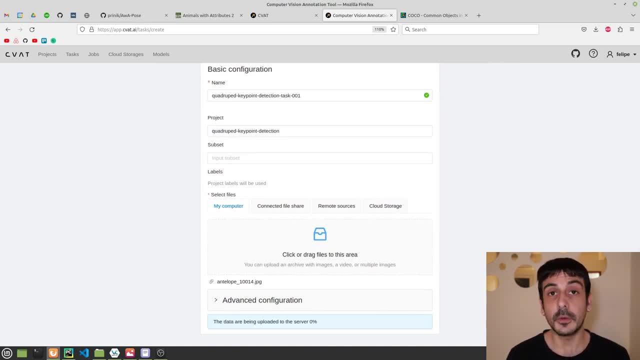 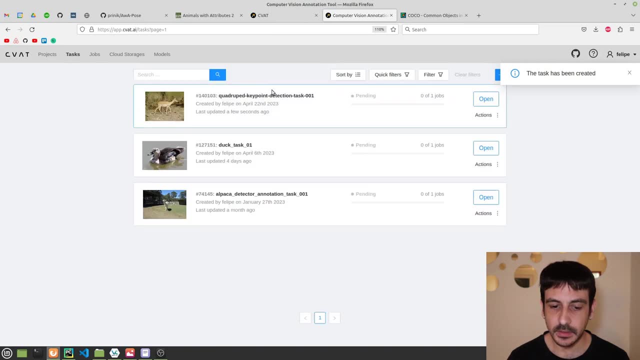 click here in submit and continue. we have to wait a couple of minutes until the data is uploaded into the server, and once everything is completed, we need to go to tasks. this is our, this is the task we have just created, and i'm going to click in open. so this is pretty much. 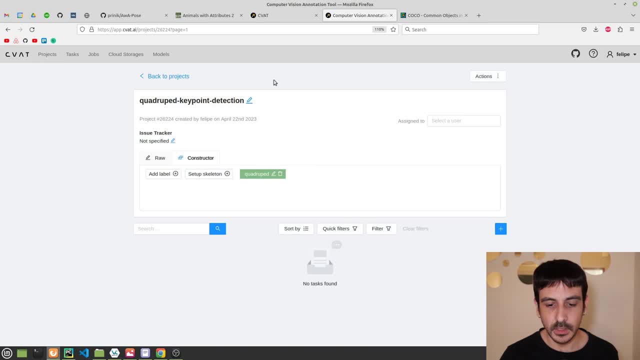 and that's pretty much all. submit another. this is where you are going to add absolutely all the labels you have in your custom data. in my case, i only have one label, which is quadruped. now let's continue. now i'm going to create a task. 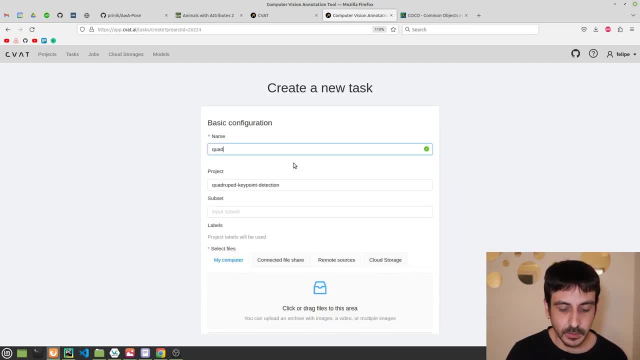 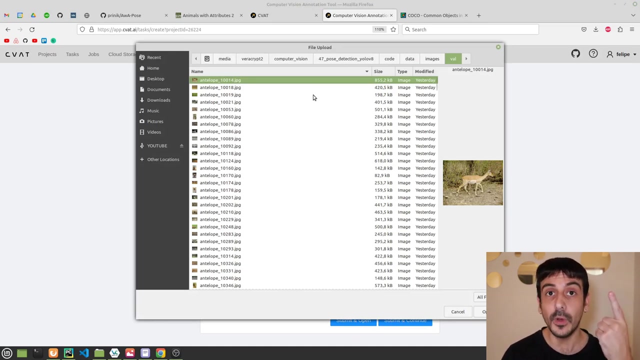 create new task. the name of this task will be something like quadruped keypoint detection, task 001, and i am going to add an image. i'm going to, i'm going to show you how to annotate this data with only one image, so i'm only going to select the first one and then i'm going to. 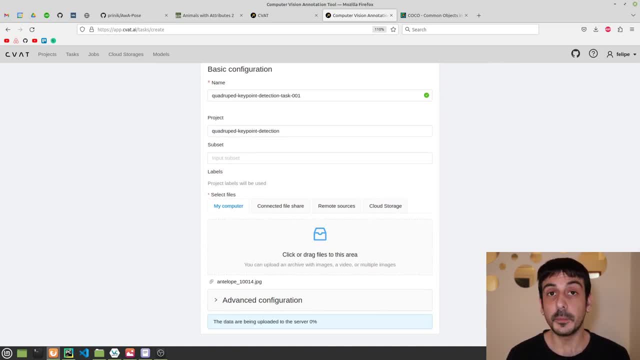 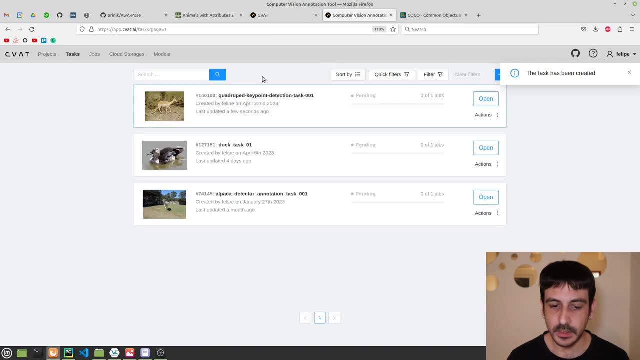 click here and submit and continue. we have to wait a couple of minutes until the data is uploaded into the server and once everything is completed, we need to go to tasks. this is our project and this is the task we have just created, and i'm going to click in open. so this is pretty much. 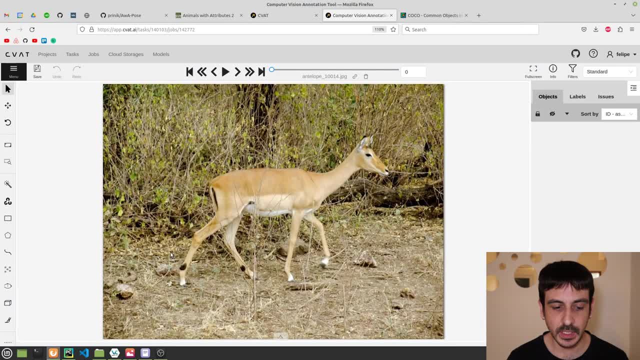 all. now i'm going to click here. this is going to open the task, and now we need to start our annotation process. so you need to click here with where it says draw new points and you need to select the number of point you're going to make. 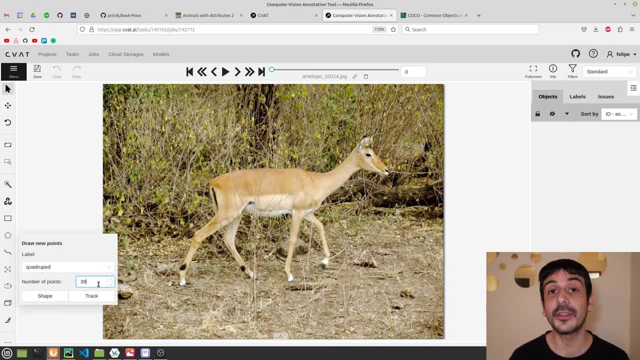 of points you are going to annotate. in my case, i'm going to annotate 39 points, but you need to select as many points as you are going to annotate. so now i'm going to click here in shape and we need to start our annotation process, and something that's very, very, very important is that, once you are 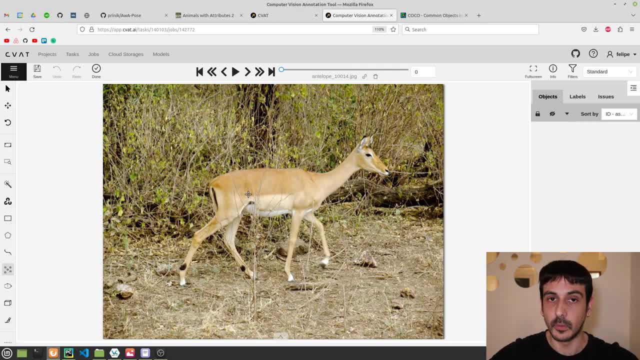 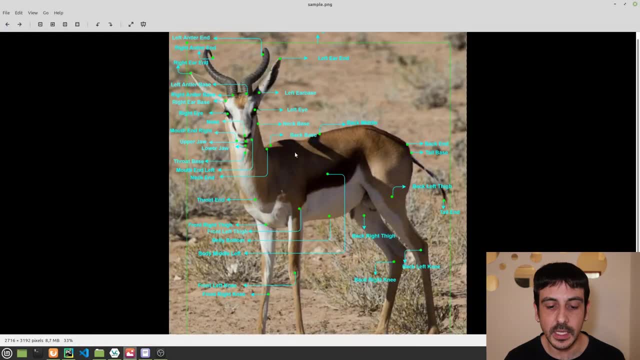 annotating your data, you need to follow a given order. right once you are annotating all of your key points, you need to follow a given order with your key points. if i show you this image again, you can see that we have many, many different key points. we have the location of all the key points. 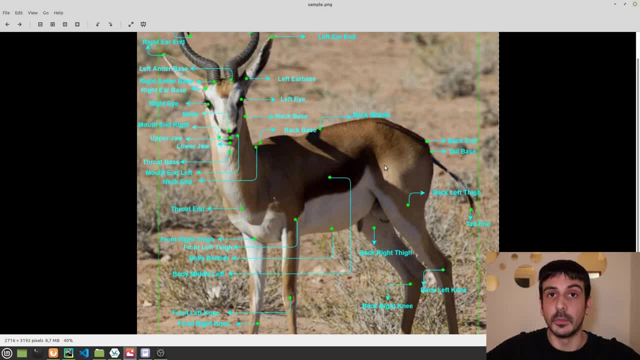 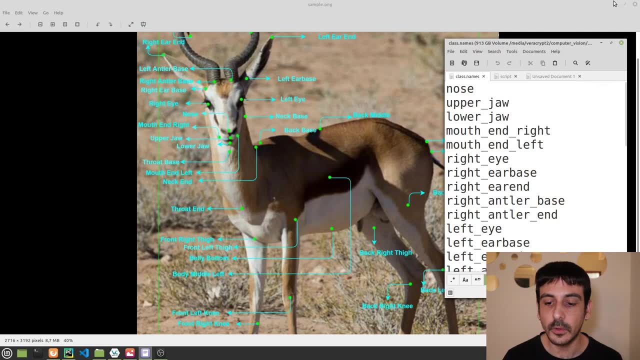 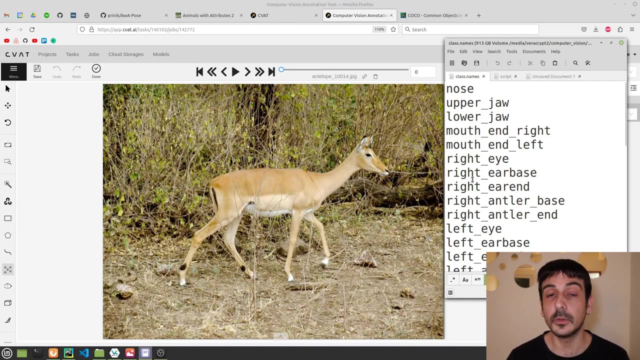 but we don't really have any information regarding the order of these key points. right, this is very, very important because you cannot follow any random order. you need to follow a given order. you need to follow always the same order when you are annotating your data. so this is, for example, the order i am going to follow in this tutorial. you can see that the 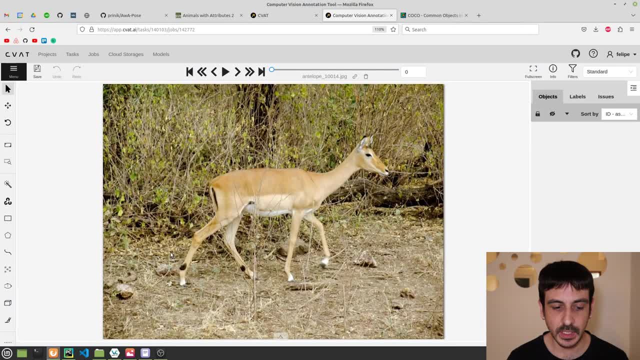 all. now i'm going to click here. this is going to open the task, and now we need to start our annotation process. so you need to click here where it says draw new points and you need to select the number of points you are going to annotate. in my case, i'm going to annotate 39 points, but you need 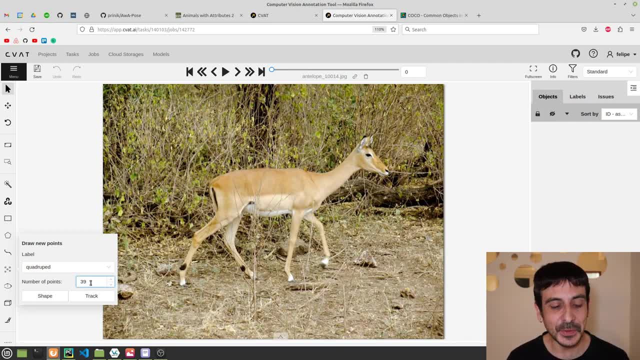 to select as many points as you are going to annotate. so now i'm going to click here in shape in order to start all my data. so we need to start our annotation process, and something that's very, very, very important is that once you are annotating your data, you need to follow a given order, right? 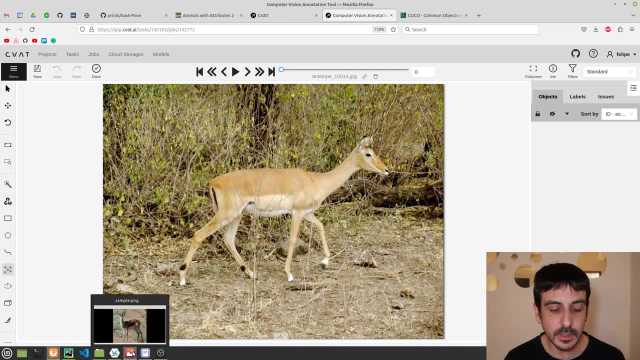 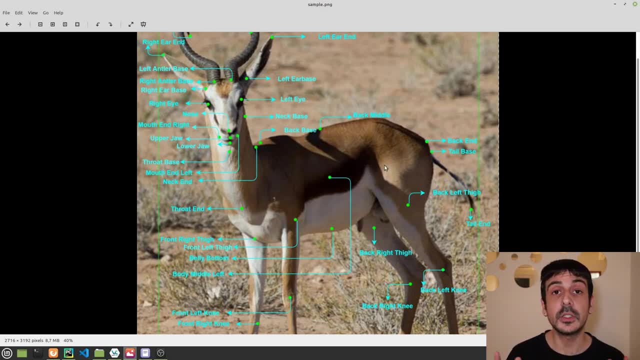 once you are annotating all of your key points, you need to follow a given order with your key points. if i show you this image again, you can see that we have many, many different key points. we have the location of all the key points, but we don't really have any information regarding the order. 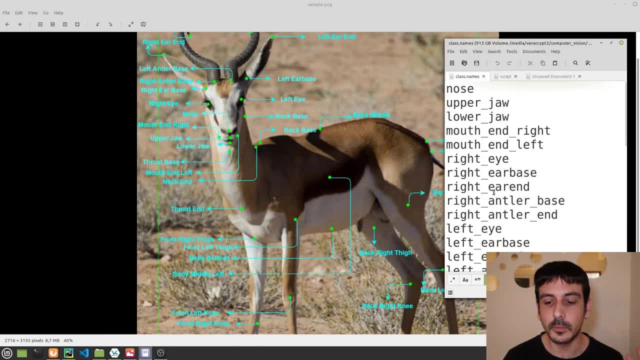 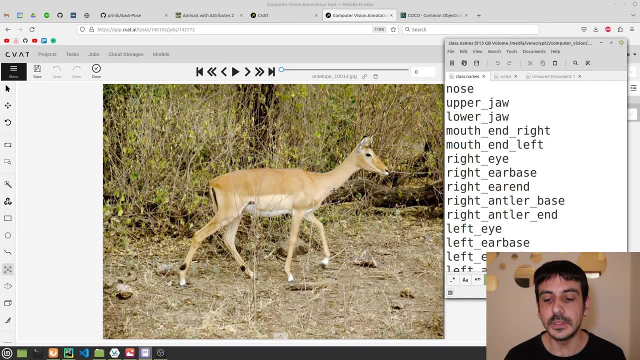 of these key points right? this is very, very important because you cannot order. you need to follow a given order. you need to follow always the same order when you are annotating your data. so this is, for example, the order i am going to follow in this tutorial. you. 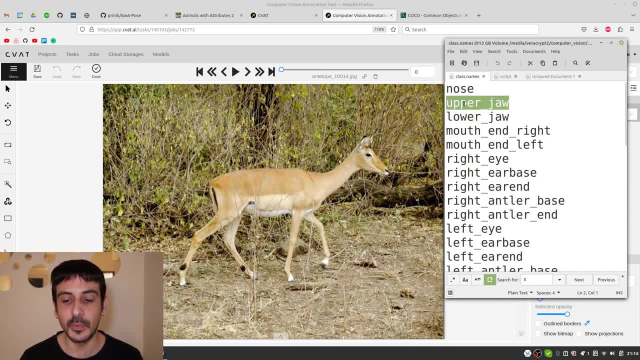 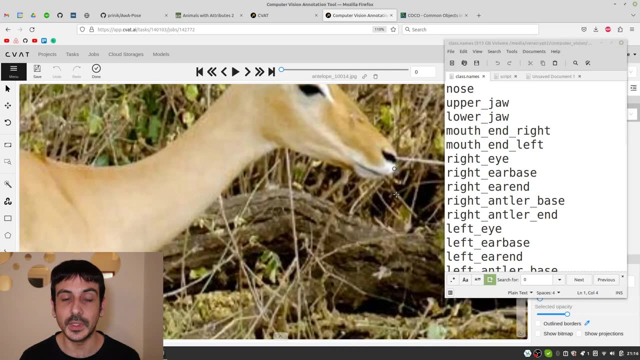 can see that the first key point i'm going to annotate is nose, then upper draw, then lower draw, mount, and right and so on. right, you need to specify a given order for your data. now i'm going to start this annotation process. so the first point is nose, which i'm going to set over here, then the next one. 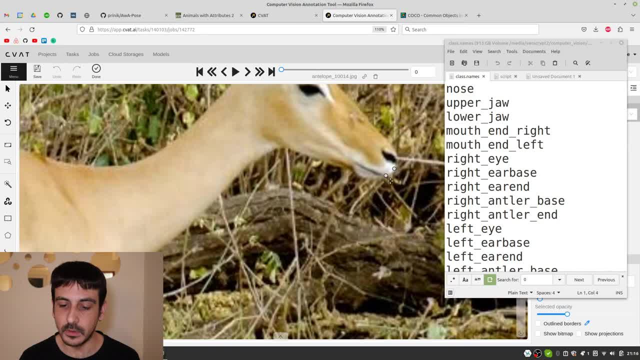 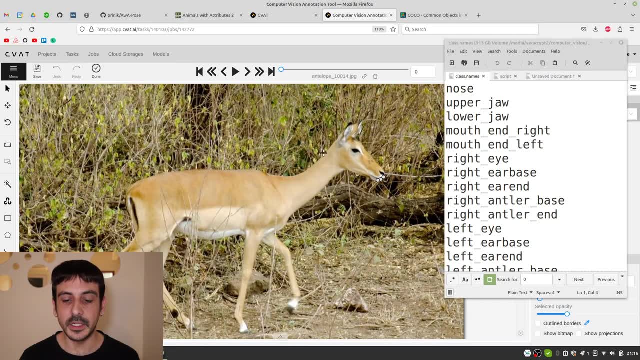 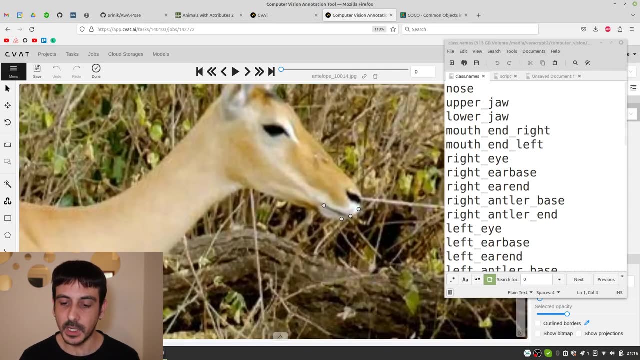 is upper jaw, which is going to be something like this lower jaw here, mount and right, and this is right from the perspective of this animal right. so this is going to be here now, mount and left, and i don't really see the mount and left, but i'm going to say it's around here and i'm going to 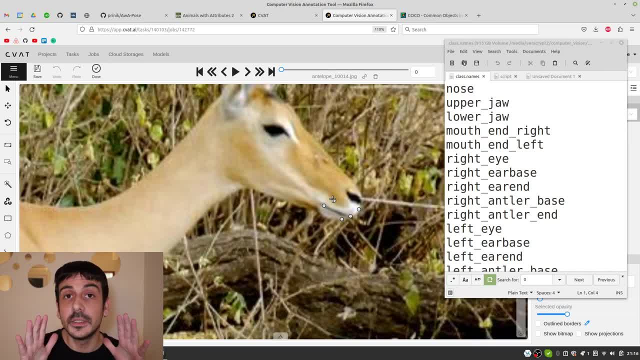 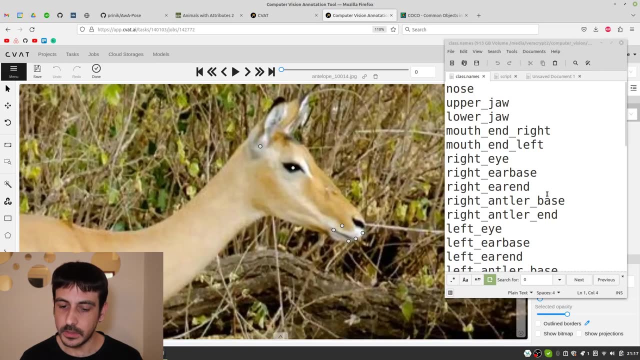 share a few comments later on this tutorial regarding the visibility of our key points. right, but for now, let's just continue. now, the next one is right eye, then right ear base, which is here, and then right ear end, which is over here, and i'm just going to continue with all of this list and i'm going to resume this video. 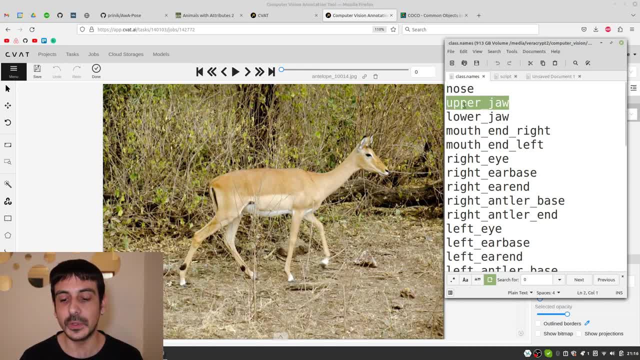 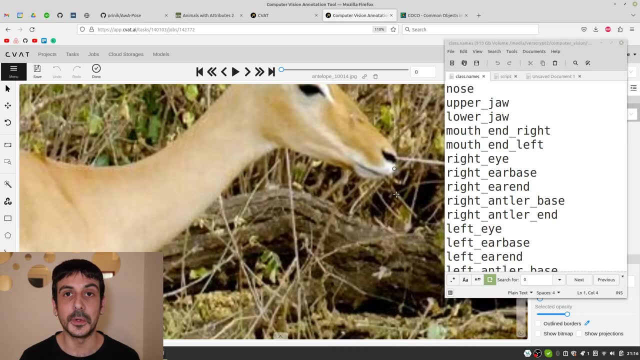 first key point i'm going to annotate is nose, then upper draw, then lower draw, mount and right and so on. right, you need to specify a given order for your data. now i'm going to start this annotation process. so the first point is nose, which i'm going to set over here, then the. 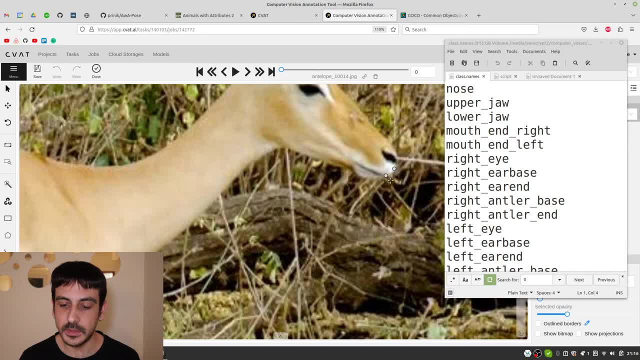 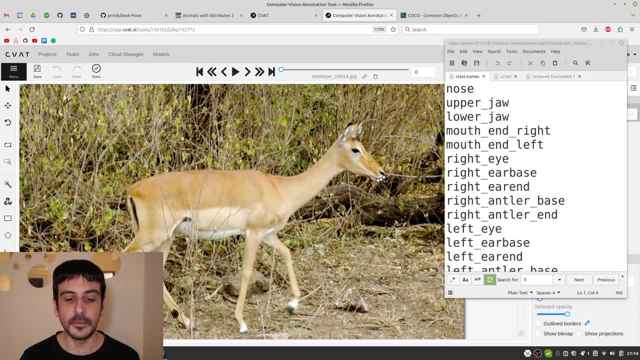 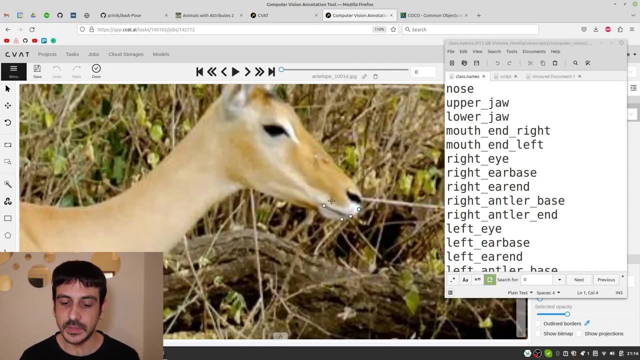 next one is upper jaw, which is going to be something like this lower draw here, mouth and right, and this is the right from the perspective of this animal right. so this is going to be here now: mouth and left, and i don't really see the mouth and left, but i'm going to say it's around. 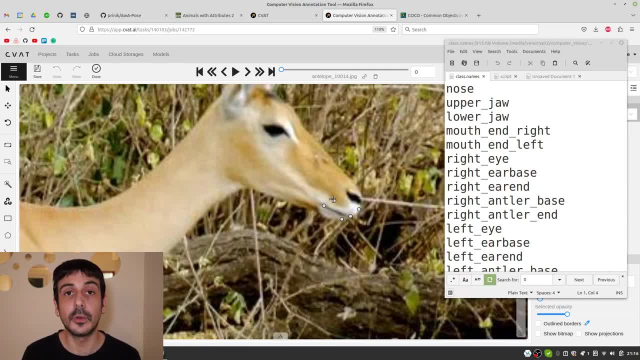 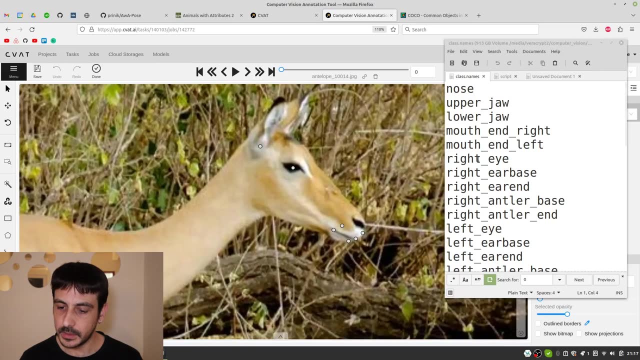 here, and i'm going to share a few comments later on this tutorial regarding the visibility of our key points. right, but for now, let's just continue. now, the next one is right eye, then right ear base, which is here, and then right ear end, which is over here, and i'm just going to 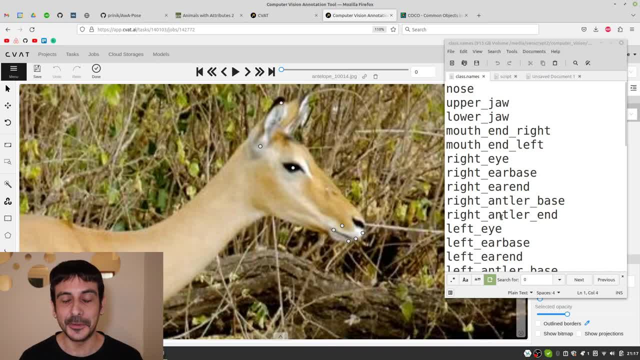 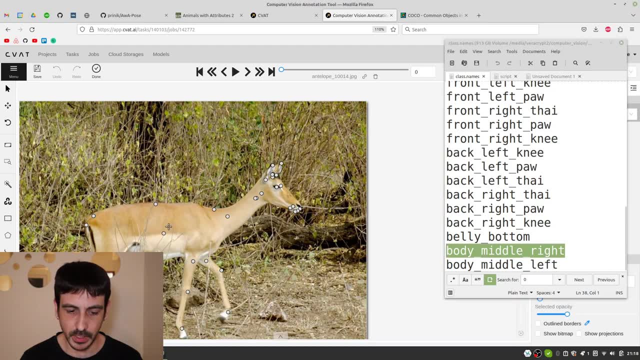 continue, and i'm going to continue, and i'm going to continue, and i'm going to continue with all of this list and i'm going to resume this video when i'm completed. and these are the last two: body middle right, which is around here, and body middle left, which is around here. i don't see. 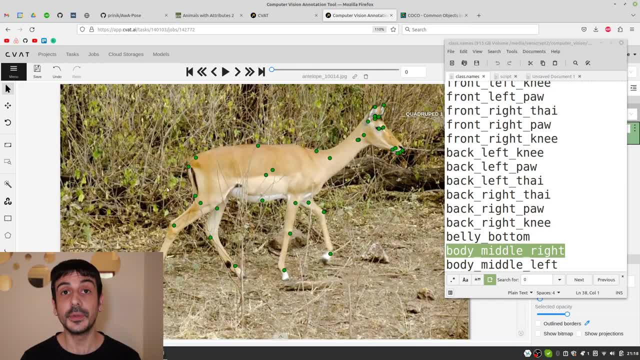 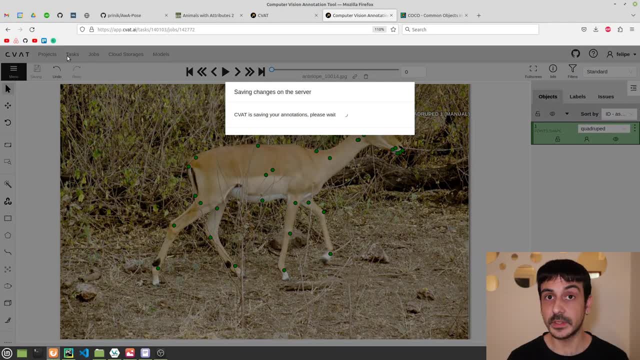 it, but it's around here and you can see that. this is all. these are my 39 key points, and now let me show you how you can export this data, but before before, please remember to click save. otherwise it's always a good practice to click save, and not only you need the key points, but you also need 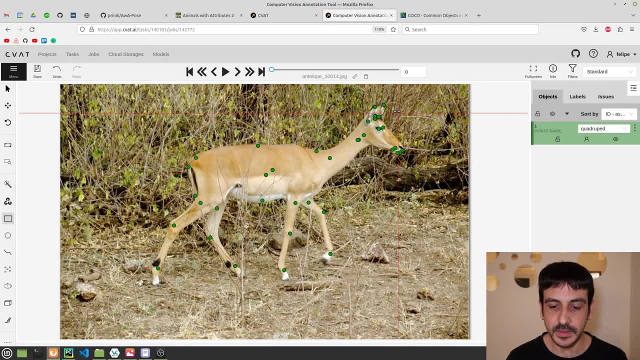 to do the same thing with the other key points, and you can do the same thing with the other key points. you can do the same thing with the other key points and you can do the same thing with the other key points. draw a bonding box around your object. this is very, very, very important, and i'm going to tell you why. 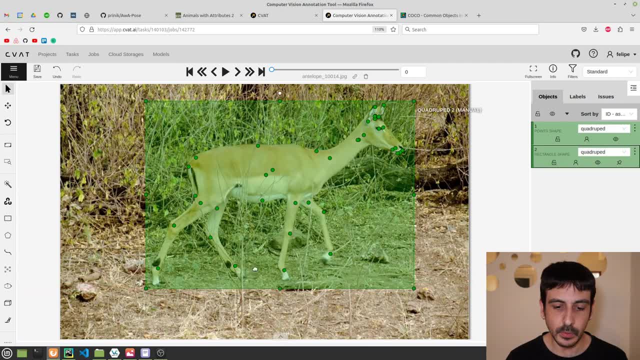 in a few minutes, but for now, remember that not only you need to annotate all of your key points, but you also need to draw a bonding box enclosing your object. so this is how i did it, and now i'm going to click save again. this is the only image i'm going to annotate, but please remember to. 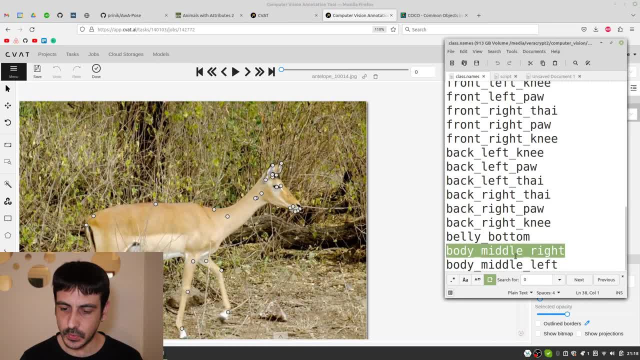 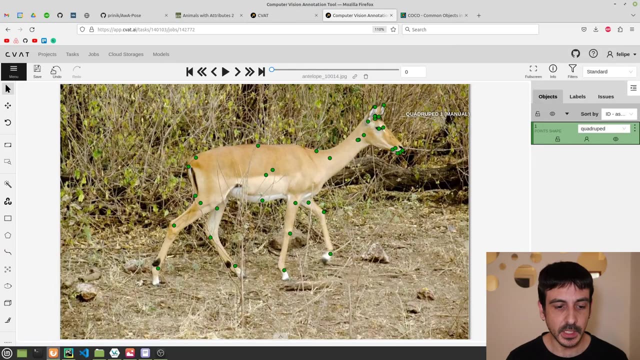 when i'm completed, and these are the last two: body middle right, which is around here, and body middle left, which is around here. i don't see it, but it's around here and you can see that. this is all. these are my 39 key points, and now let me show you how you can export this data. but before, before. 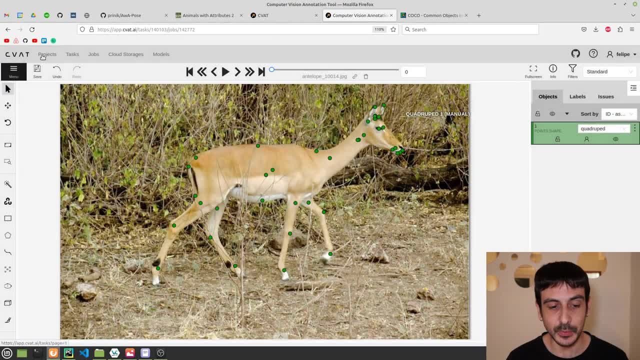 please remember to click save, otherwise it's always a good practice to click save, and not only you need the key points, but you also need to draw a bonding box around your object. this is very, very, very important, and i'm going to tell you why in a few minutes, but for now, remember that. 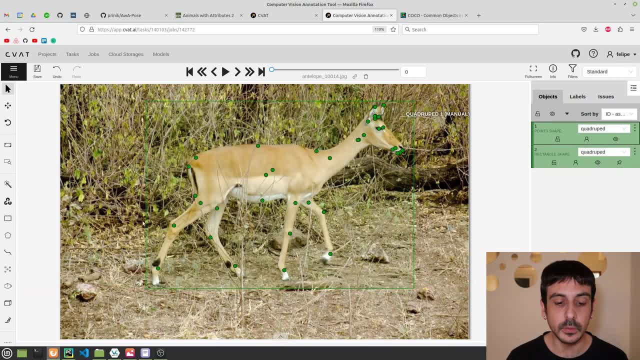 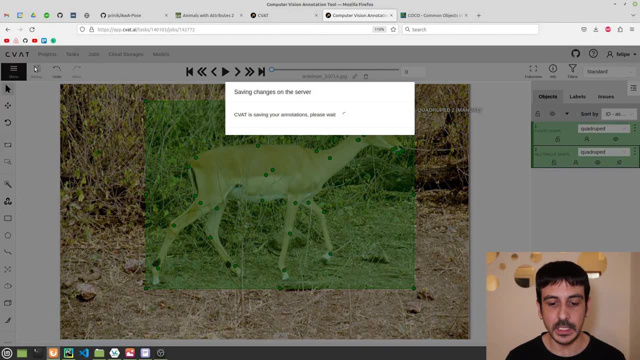 not only you need to annotate all of your key points, but you also need to draw a bonding box enclosing your object. so this is how i did it, and i'm going to click save again. this is the only image i'm going to annotate, but please remember to follow exactly the same process. 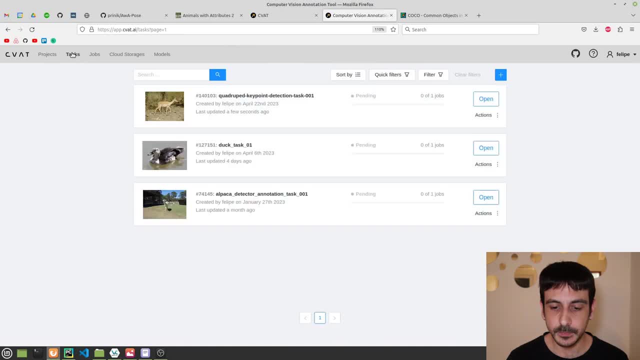 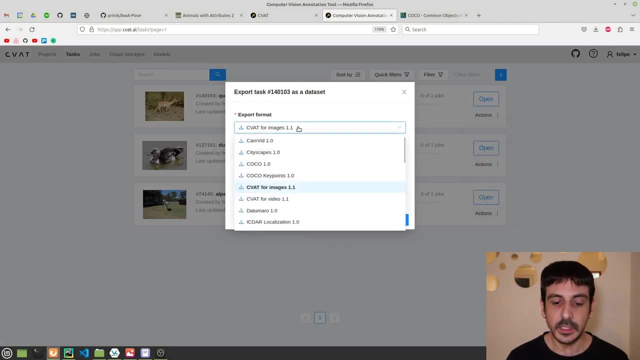 for all of your images. i'm now going to tasks and i'm going to show you how to export this data. you need to click here and export task dataset now. you need to click here and you can see that there are many, many different options in which you can export your data, and one of these options is koko. 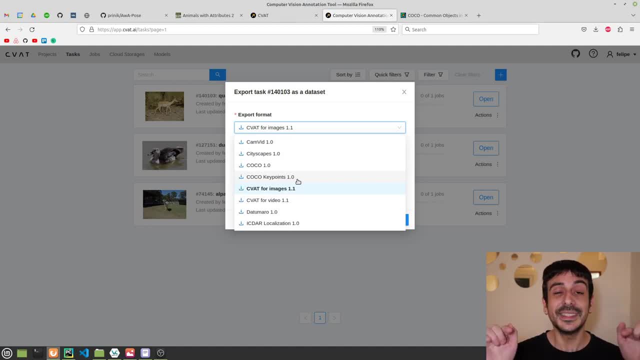 keypoints 1.0, and this is very important because this is the exact format we need for our data. but i have tried to export the data into this format and it's not working. for some reason it's not working, so i'm going to show you how to do it in cvit for images 1.1. 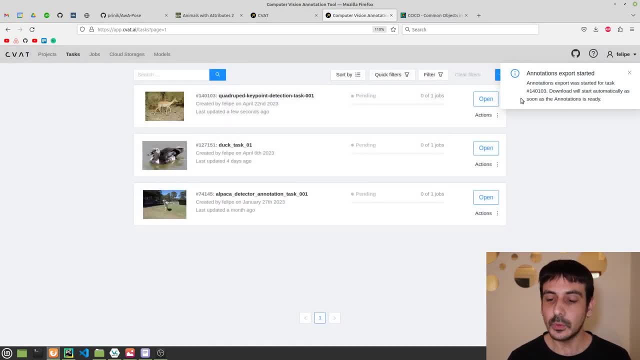 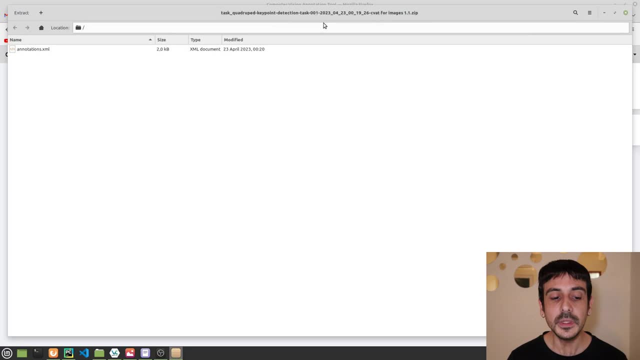 so click here then ok, and then you just have to wait until everything is downloaded. once every thing is fully exported, you are going to see a file, a zip file, and within this file there will be an another file called annotationsxml. now let me open this file so i can show you how it looks like. 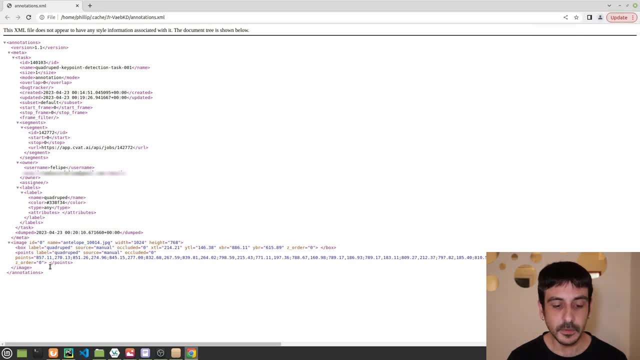 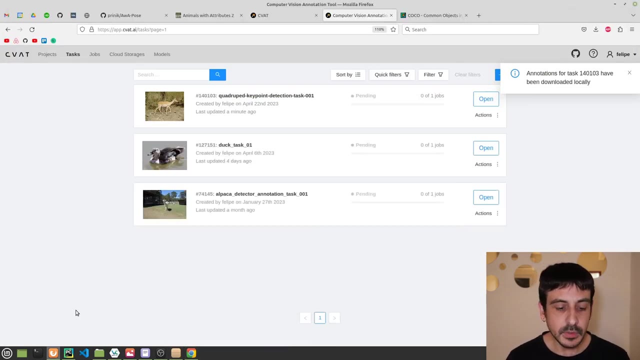 you are going to see something like this and at the bottom of this file, you are going to see all of your annotations and the all the images you have annotated and its annotations, right? so this is exactly the data you are going to generate using cbat. now let me show you how to export your data in cvit. 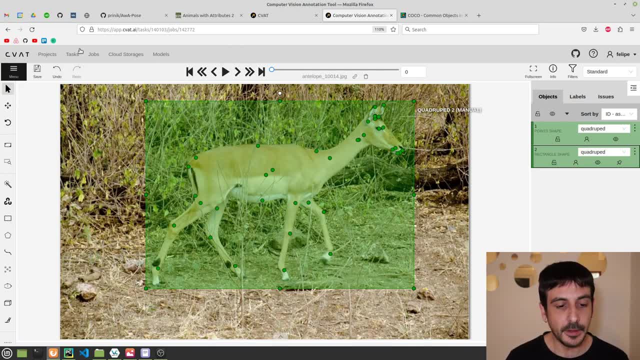 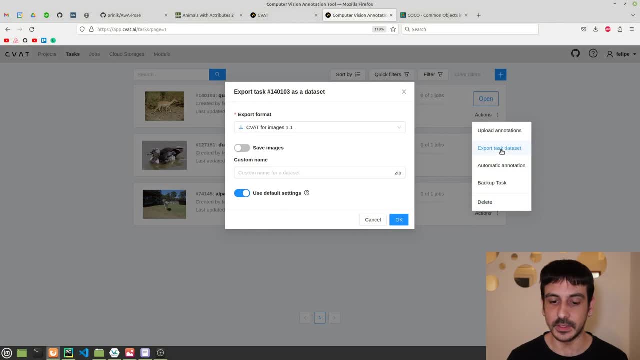 follow exactly the same process for all of your images, and now i'm going to show you how i can do this. now i'm going to tasks and i'm going to show you how to export this data. you need to click here and export task dataset now. you need to click here and you can see that there are many, many. 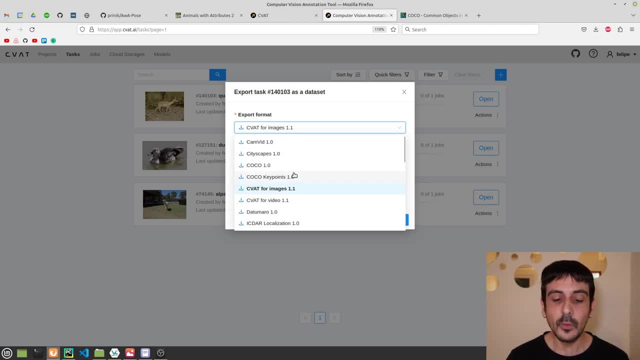 different options in which you can export your data, and one of these options is kogo keypoints 1.0, and this is very important because this is the exact format we need for our data. but i have tried to export the data into this format and it's not working. for some reason it's not working so. 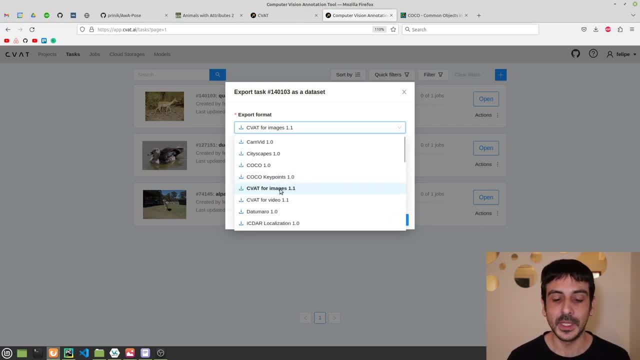 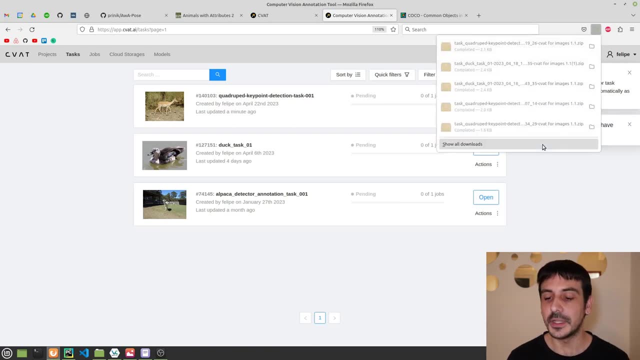 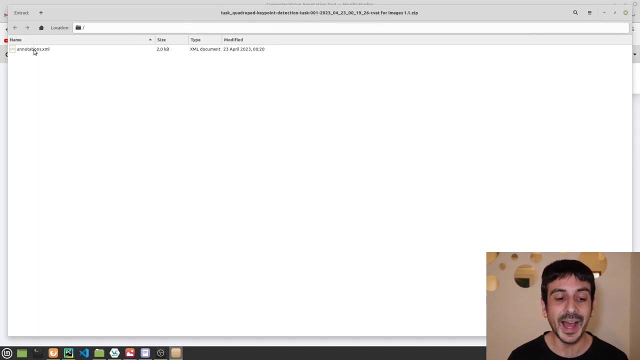 i'm going to show you how to do it in cvit for images 1.1. so click here then. ok, and then you just have to wait until everything is downloaded. once everything is fully exported, you are going to see a file, a zip file, and within this file there will be an another file called annotationsxml. 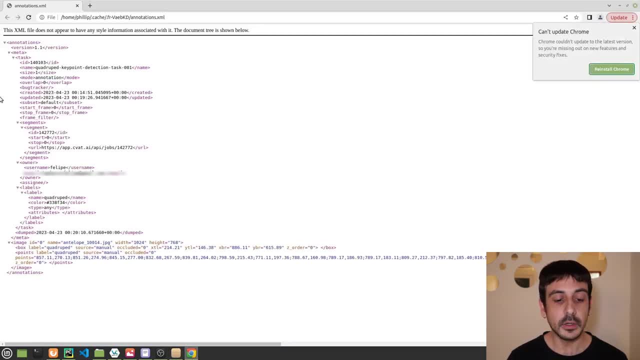 now let me open this file so i can show you how it looks like. you are going to see something like this and at the bottom of this file, you are going to see all of your annotations and the all the images you have annotated and its annotations, right? so this is exactly the data you 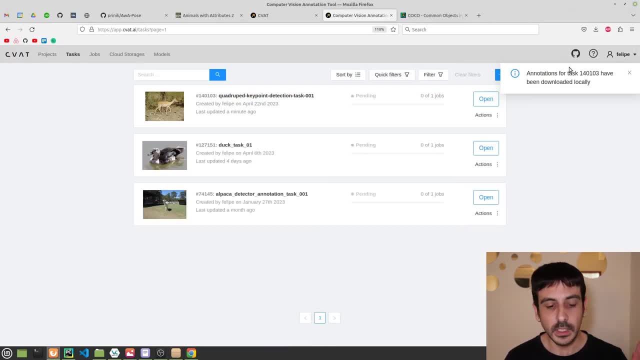 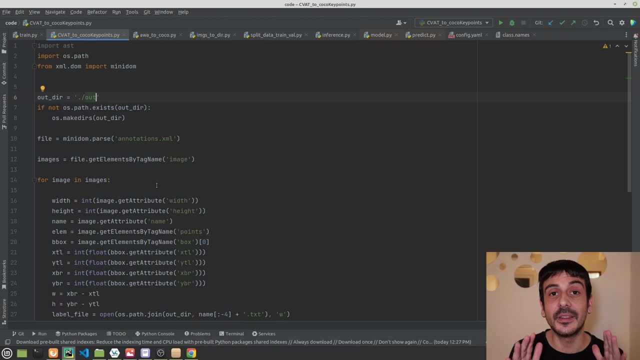 are going to generate using cvit. now let me show you something else. i have created a python project for today's tutorial and let me show you a script i created in this python project. and this script will be super, super, super useful, because now that you have your annotations, now that you have your 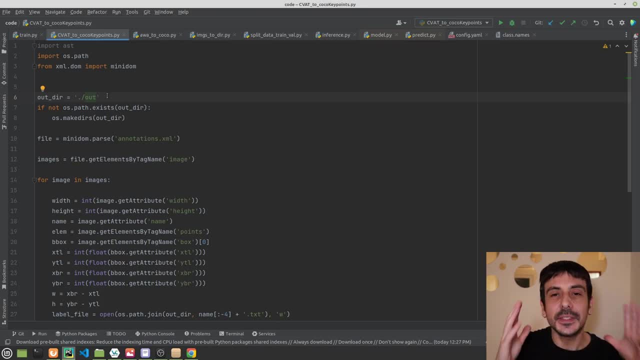 data. you need to convert your annotations into the exact format you need in order to use this post detector using yolo v8. so let me show you basically. you need to specify two variables. one of them is the location of your annotationsxml file, and you also need to specify 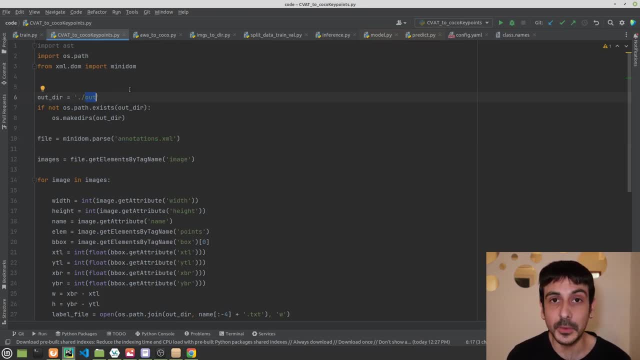 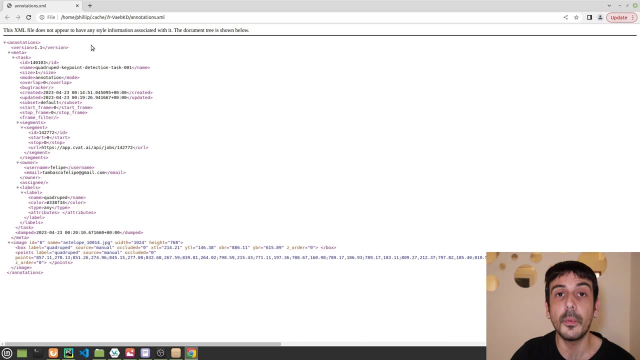 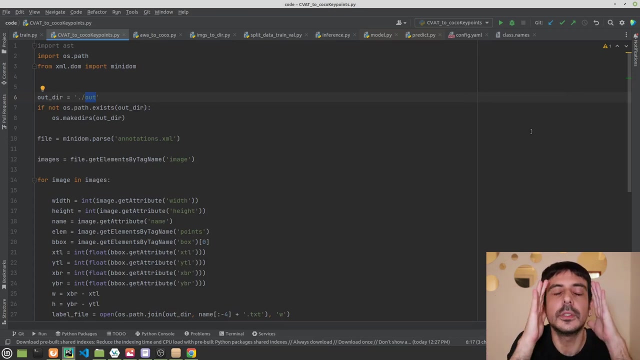 the location of the directory where you want all your data to be saved. right? this script is going to parse through this xml file, is going to parse through this file and it's going to extract all of your annotations into the exact format you need in order to use yellow v8. so remember to specify. 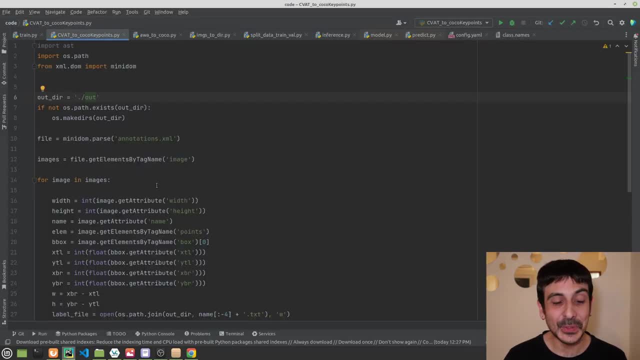 show you something else. i have created a python project for today's tutorial and let me show you a script i created in this python project. and this script will be super, super, super useful, because now that you have your annotations, now that you have your data, you need to convert your annotations. 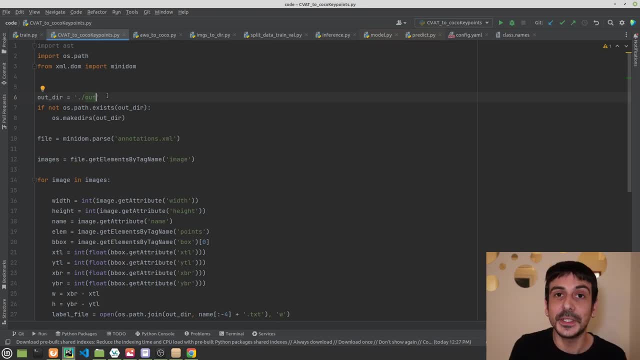 into the exact format you need in order to use this post detector using yolo v8. so let me show you basically. you need to specify two variables. one of them is the location of your annotationsxml, location of your annotationsxml, location of your annotationsxml file, and you also need to specify the location of the directory. 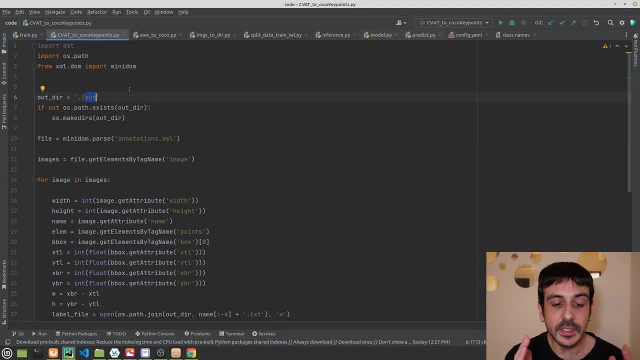 where you want all your data to be saved. right? this script is going to parse through this xml file, is going to parse through this file and it's going to extract all of your annotations and it's going to save all of your annotations into the exact format you need in order to use. 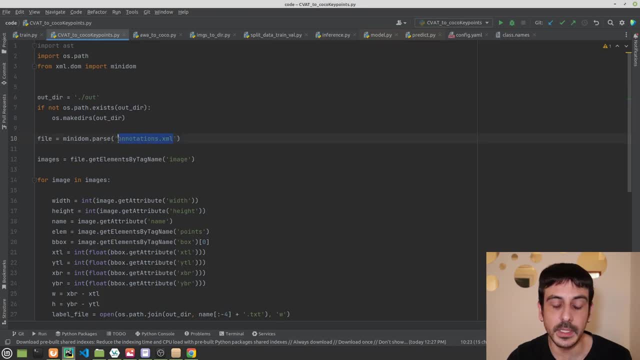 yellow v8. so remember to specify these two paths, these two variables: one of them is the location of your xml file and then where you want all of your newly created annotations to be saved, right where you want this output directory. so once you have set these two variables, the only thing 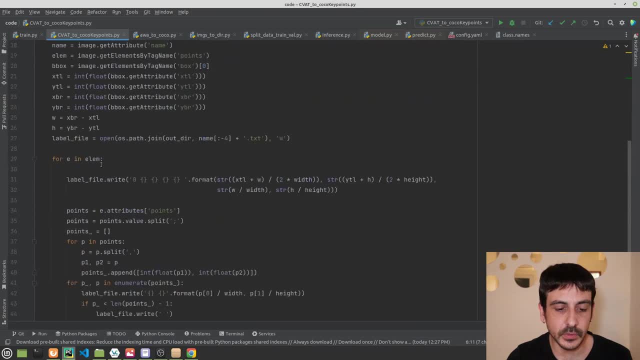 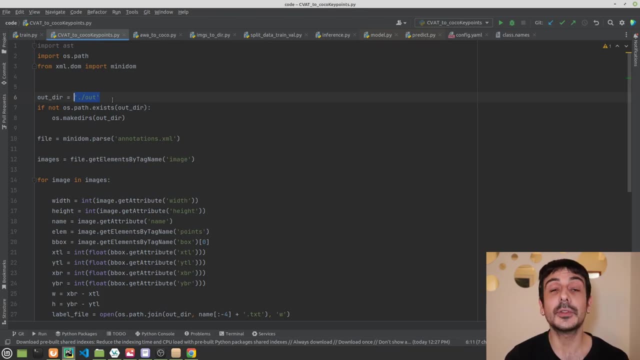 you need to do is to run this script, and everything will run super, super smoothly. and remember, this script will be available in the github repository of today's tutorial, so you can just go ahead and use it. in order to convert all of your data into the format you need to use, yellow v8. and now let's. 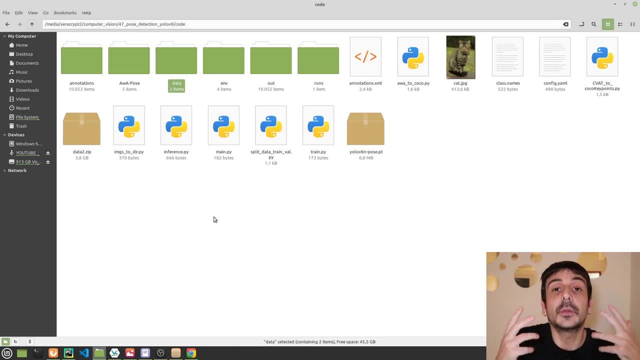 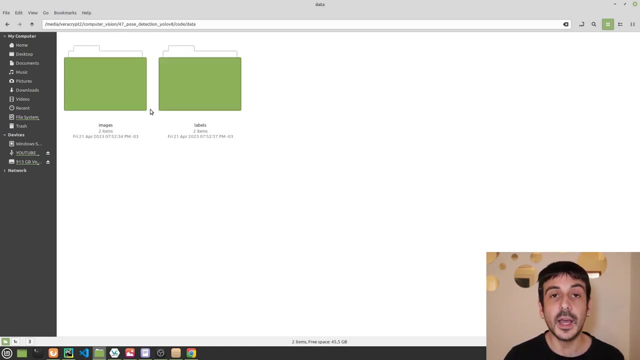 continue. now i'm going to show you how you need to format, how you need to structure all of your data and your file system so it complies with your lobby 8.. so you can see that this is a directory which is called data and this is the root directory where my data is located. you need a directory. 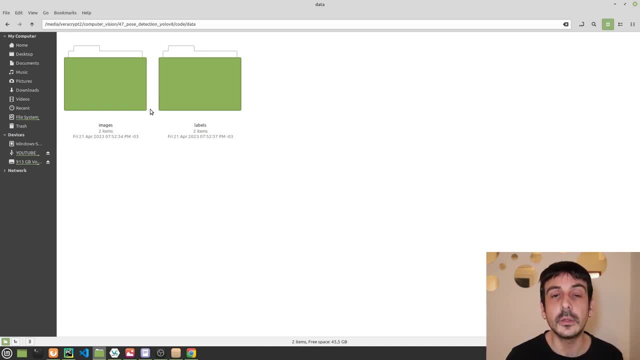 which will be the root directory where your data will be saved, where your data will be located within this root directory. you can see i have two folders. one of them is called images and the other one is called labels. it's very important that you name these two folders. 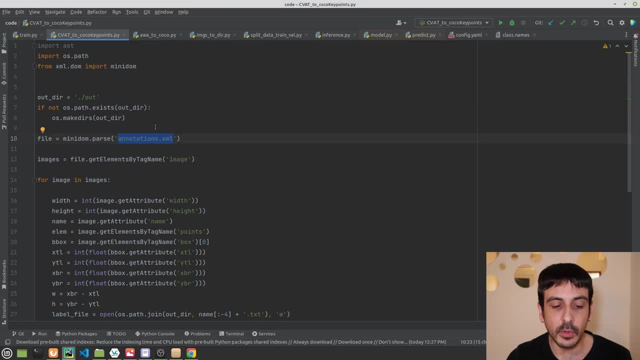 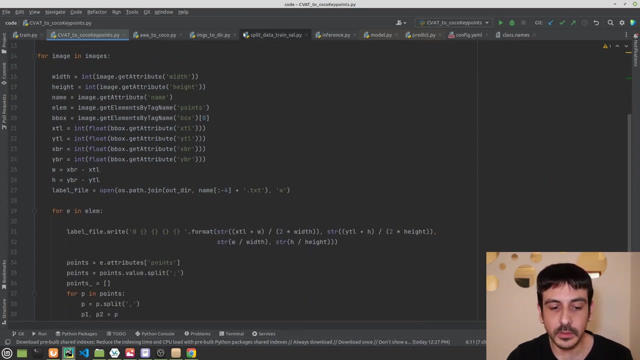 these two paths, these two variables: one of them is the location of your xml file, and then where you want all of your newly created annotations to be saved, right where you want this output directory. so, once you have set these two variables, the only thing you need to do is to run this script. 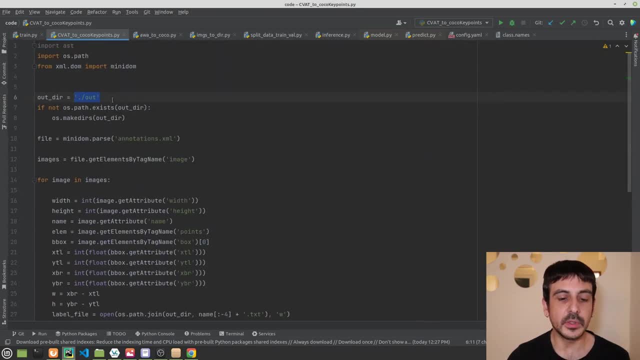 and everything will run super, super smoothly. and remember, this script will be available in the github repository of today's tutorial, so you can just go ahead and use it. in order to convert all of your data into the format you need to use yolo v8. and now let's continue. now i'm going. 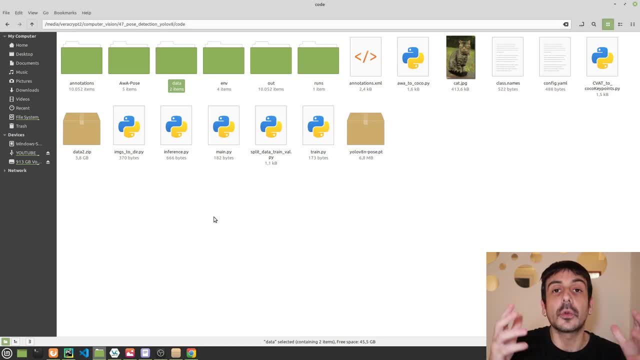 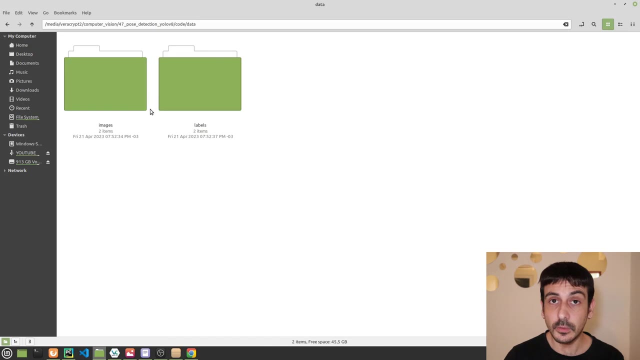 to show you how you need to format, how you need to structure all of your data and your file system so it complies with yolo v8. so you can see that this is a directory which is called data and this is the root directory where my data is located. you need a directory which will be the 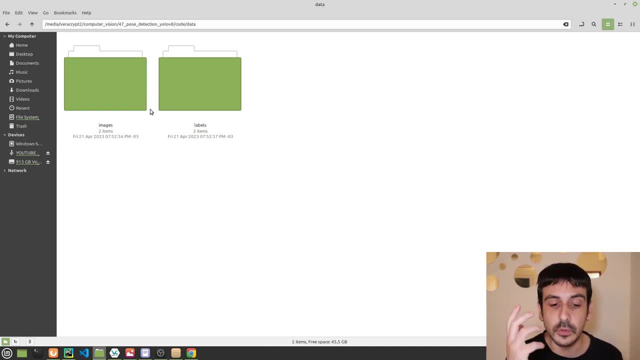 root directory, directory where your data will be saved, where your data will be located within this root directory. you can see i have two folders. one of them is called images and the other one is called labels. it's very important that you name these two folders exactly like this. one of them should be called: 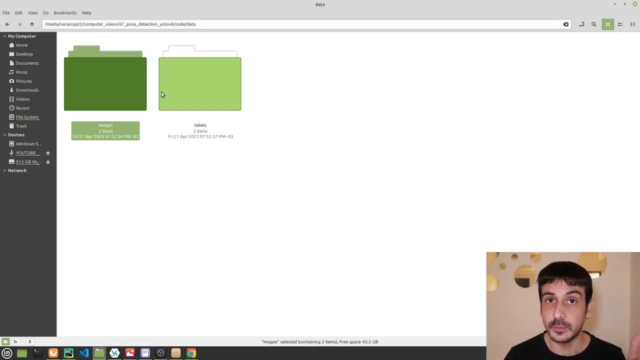 the images, and the other one should be called labels. that's very important. now, if i open one of these folders, you can see i have two other folders. one of them is called train and the other one is called training, and it's very important that you name these directories exactly like this. 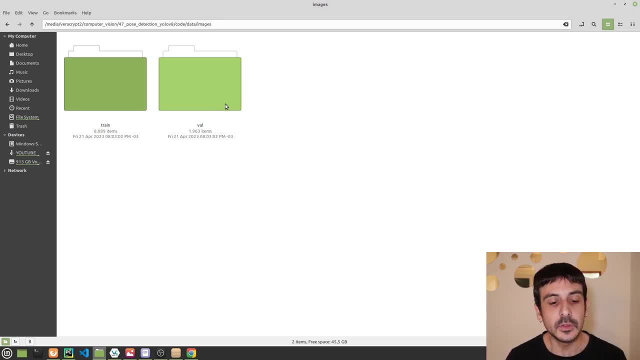 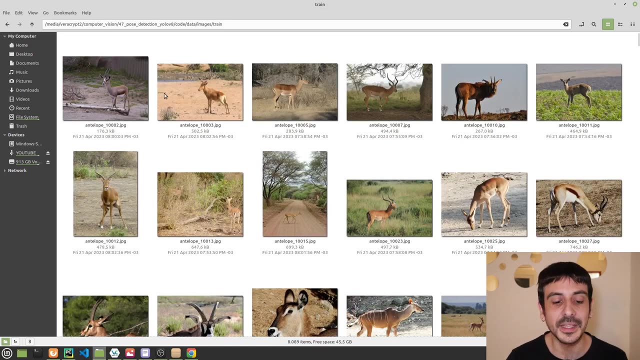 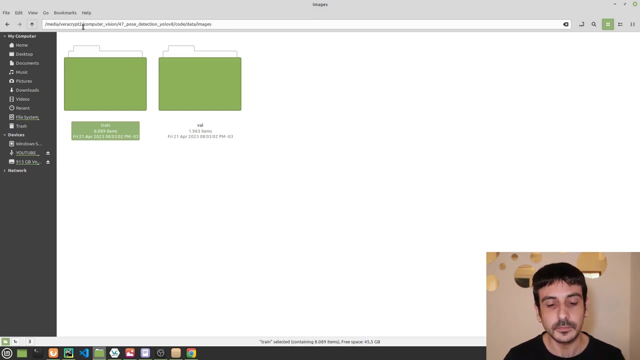 one of them should be called train and the other one should be called valve. so within train is where we will have all of our training data, all of your training images. right, you can see that these are all of our images, which are all the images we are going to use as training data, and within ball it's. 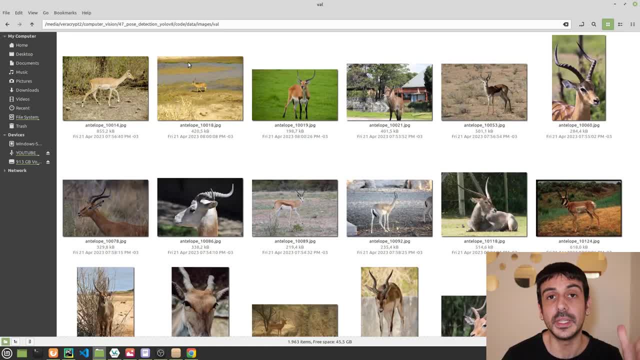 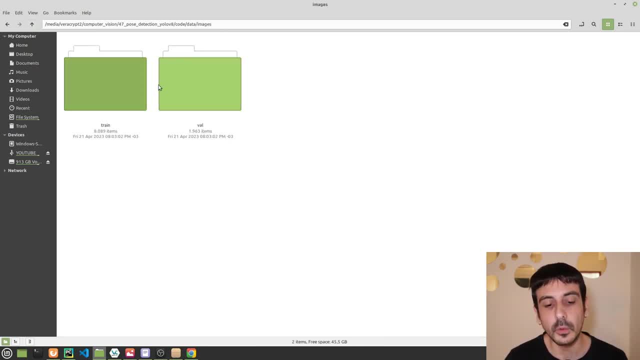 exactly the same. this is all the images we are going to use as a validation data, as a validation or validation set right. so within images, we have two directories. one of them is called train, the other one is called ball, and within each one of these directory is each one of these directories. 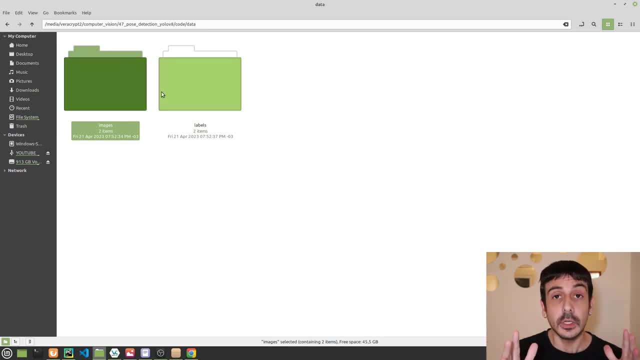 exactly like this: one of them should be called the images and the other one should be called labels. that's very important. now, if i open one of these folders, you can see that i have two other folders. one of them is called train and the other one is called ball, and it's very 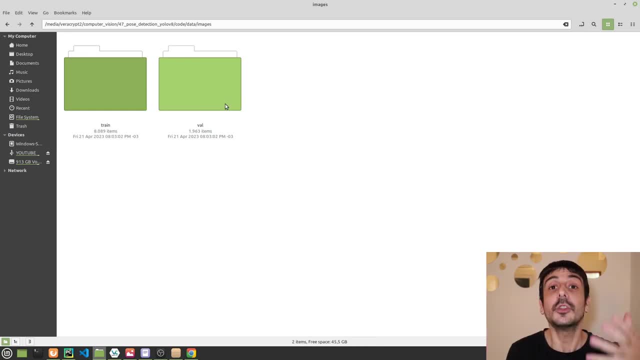 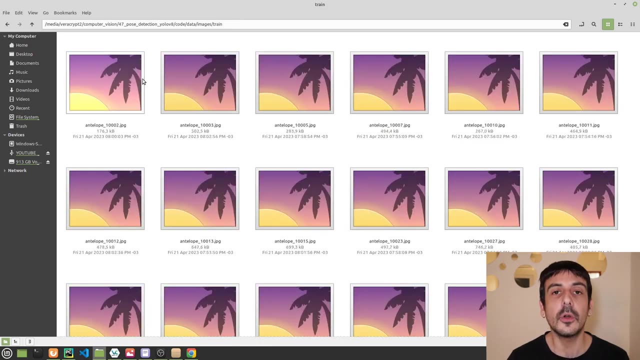 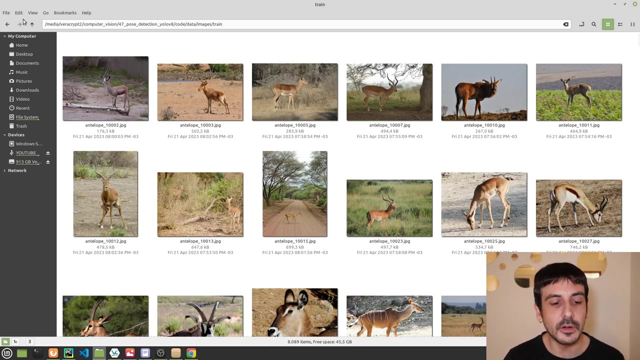 important that you name these directories exactly like this: one of them should be called train and the other one should be called ball is where we will have all of our training data, all of your training images. right, you can see that these are all of our images, which are all the images we are going to use as training data, and 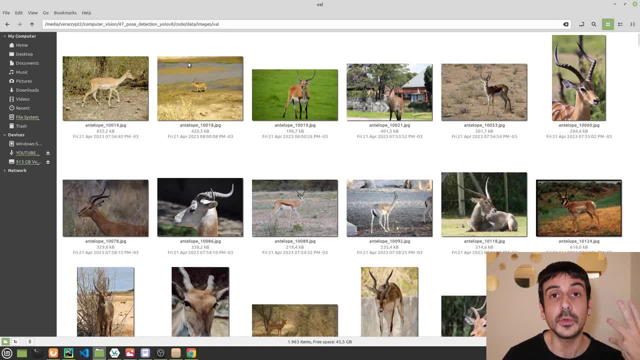 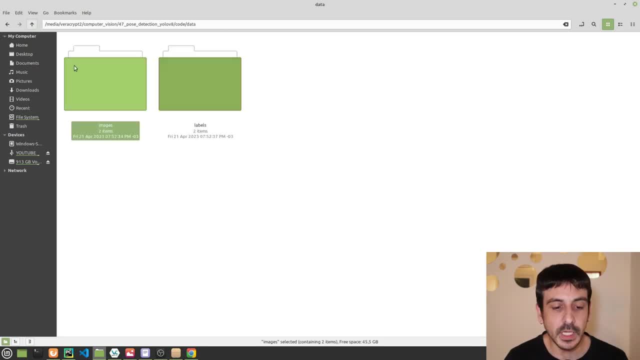 within ball. it's exactly the same. this is all the images we are going to use as a validation data, as our validation set right. so, within images, we have two directories. one of them is called train, the other one is called ball, and within each one of this directory is each one of these directories. 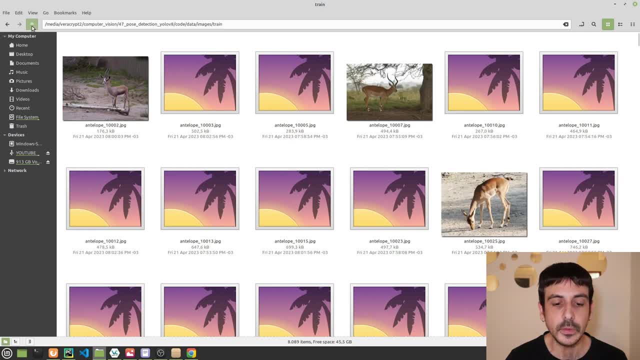 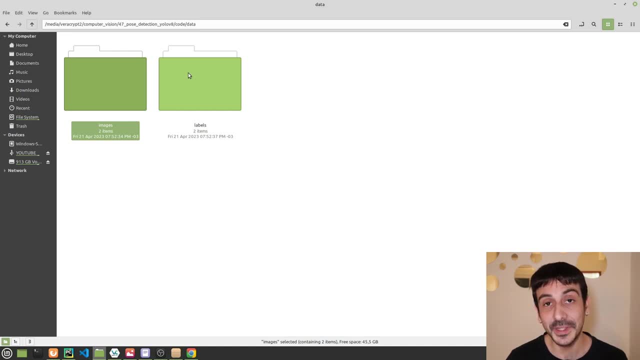 is where we have all of our data, all the data we are going to use in order to train this model, all the images we are going to use in order to train this model. but we also have additional data, which are the labels. now let me show you how this all folder looks like. you can see that within. 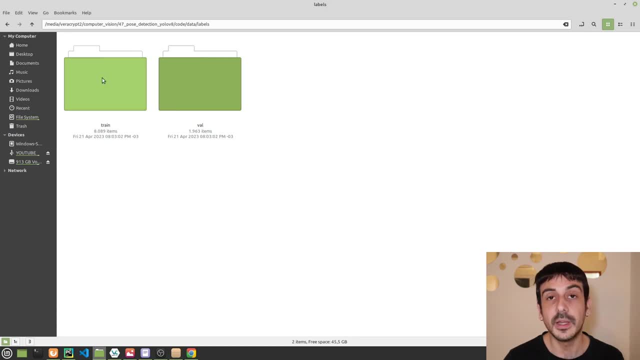 labels. we also have two directories which are also called train and ball, and it's very important that you name these two directories exactly like this: one of them should be called train and the other one should be called ball, and if i open the train directory, you can see that the two directories are. 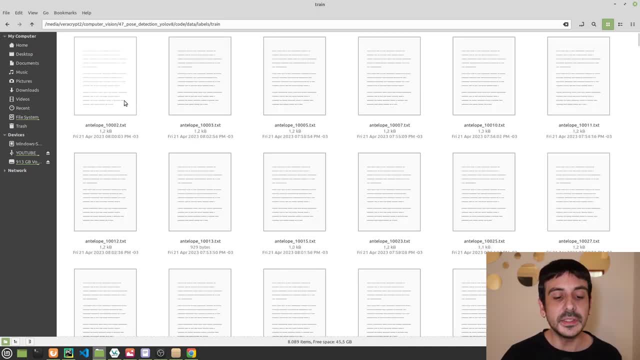 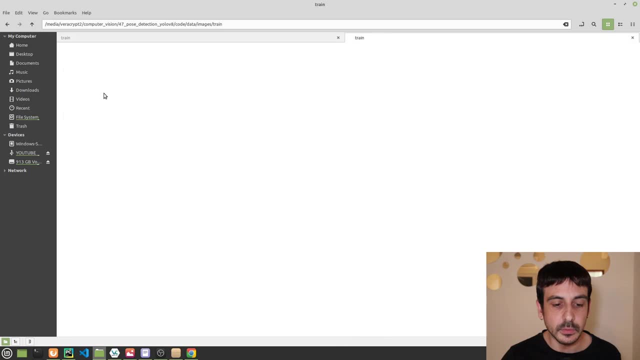 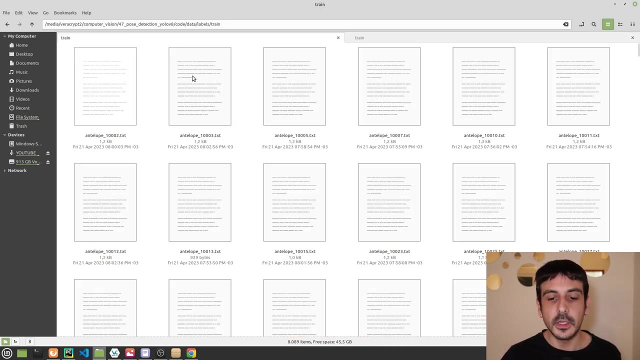 that we have many, many, many txt files and these are basically all of our labels for the training data, for all of our training images. if i go back to images train, you can see that for absolutely every single one of these images we have an annotations file right for absolutely every. 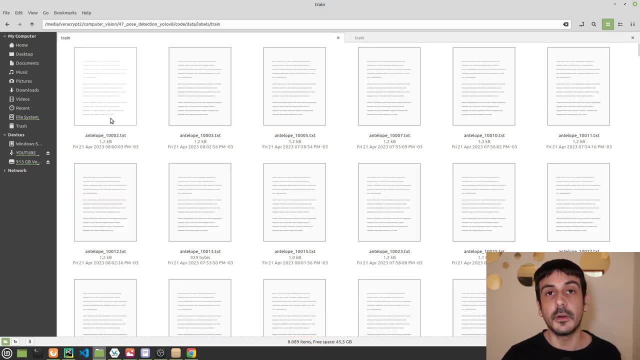 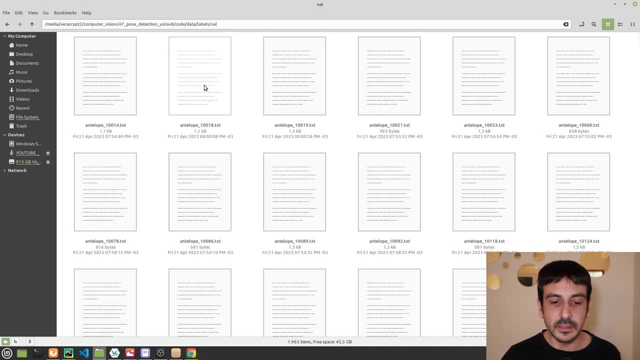 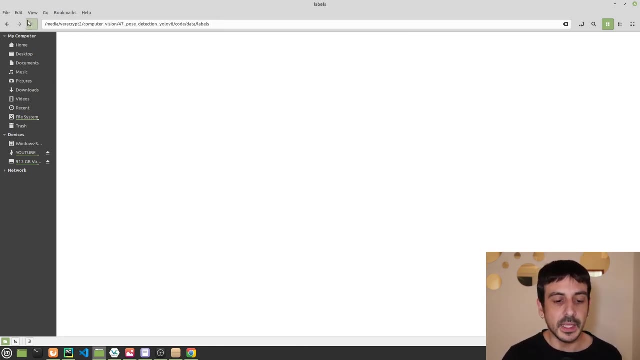 single one of these images. we are going to have a txt file in this folder. and now let me show you: for the order directory, for ball, it's exactly exactly the same, but for the validation data, for the validation images, right? so if i go back again, you can see that we have in the root directory, then images, labels. within images, we have two. 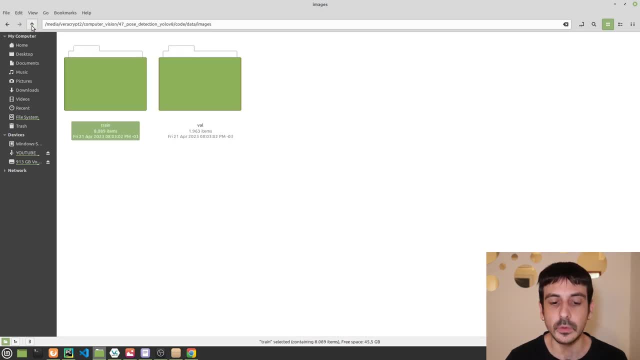 is where we have all of our data, all the data we are going to use in order to train this model, all the images we are going to use in order to train this model. but we also have additional data, which are the labels. now let me show you how this or folder looks like. you can see that within. 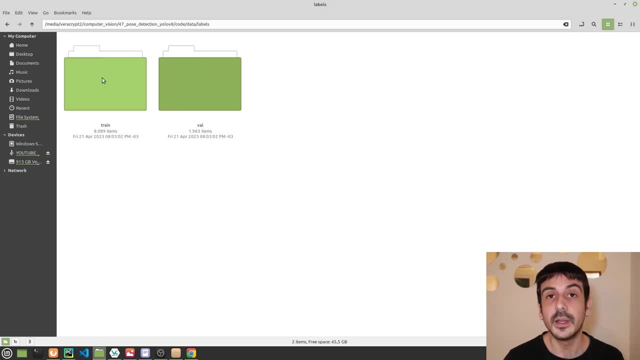 labels. we also have two directories, which are also called train and ball, and it's very important that you name these two directories exactly like this: one of them should be called train and the other one should be called ball, and if i open the train directory, you can see that we have many, many 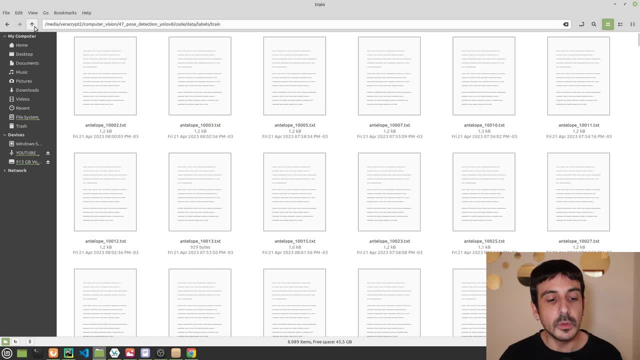 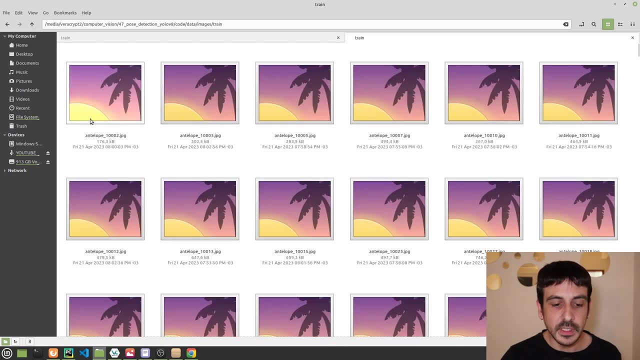 many txt files and these are basically all of our labels for the training data, for all of our training images. if i go back to images train, you can see that for absolutely every single one of these images we have an annotation that is called train and that is called train and that is the. 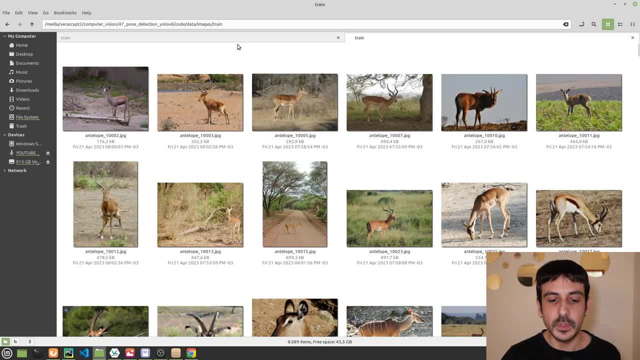 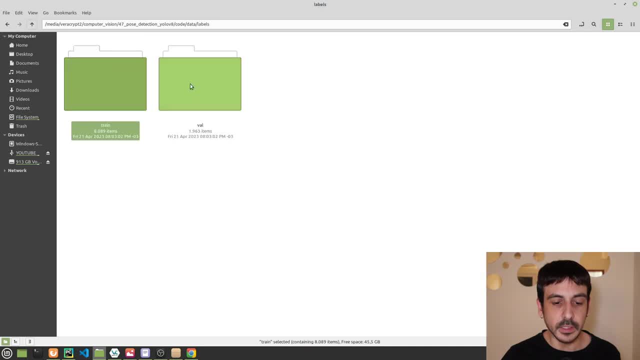 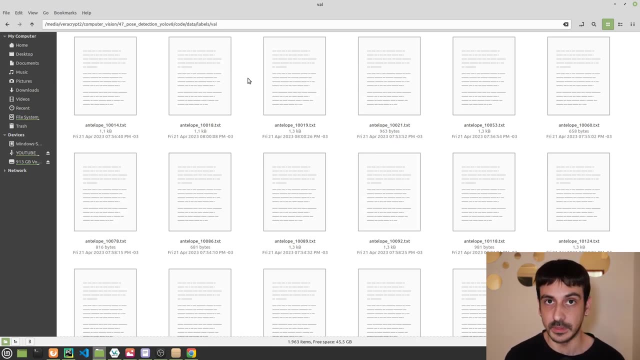 file right, for absolutely every single one of these images. we are going to have a txt file in this folder. and now let me show you. for the other directory, for ball, it's exactly exactly the same, but for the validation data, for the validation images, right? so if i go back again, you can see. 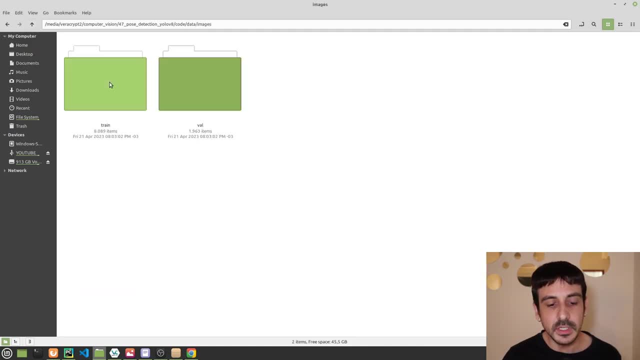 that we have the root directory, then images, labels, within images. we have two directories, train and ball, and within each one of these directories is where we have all of our images. and if we go to labels, we have also two directories, train and ball, and within each one of these directories. 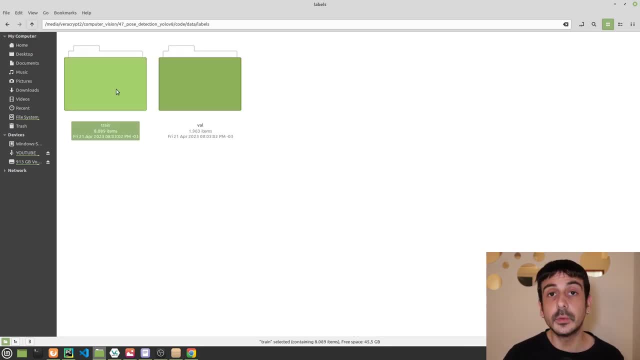 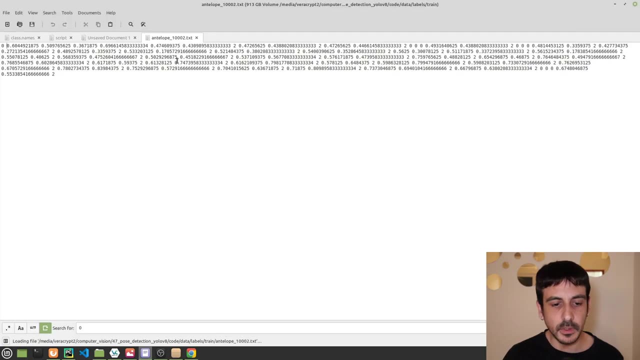 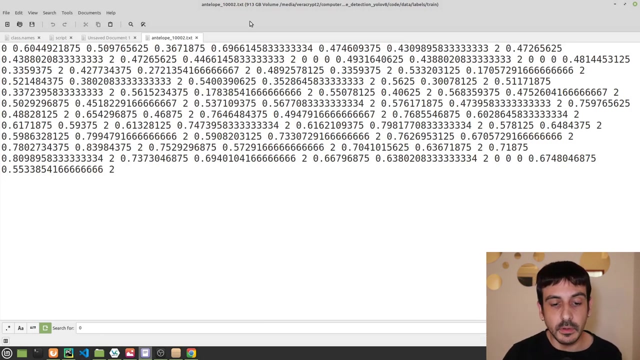 is where we have all of our labels. so this is exactly how you need to structure your file system. and now let me show you one of these annotations files, one of these labels files from the inside. let me show you how they look like. so this is a random annotations file. this is a random txt file. 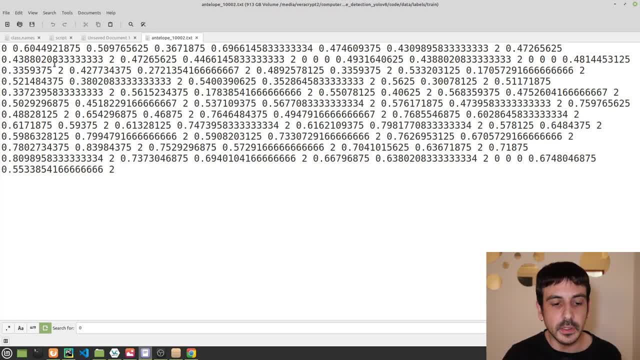 and this is a random txt file. and this is a random txt file. and this is a random txt file- exactly how you need to put all the data inside these files. the annotations are specified in the coco key point format, which is a very popular format for post detection. now let me show you. 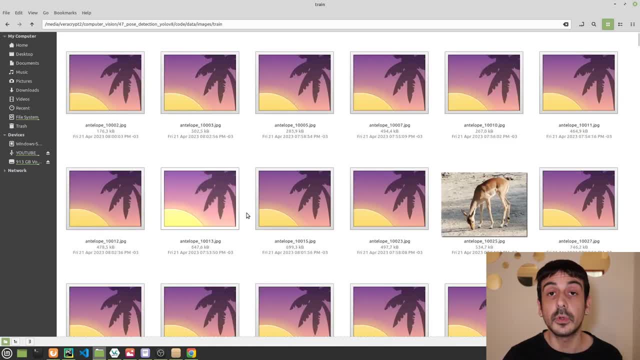 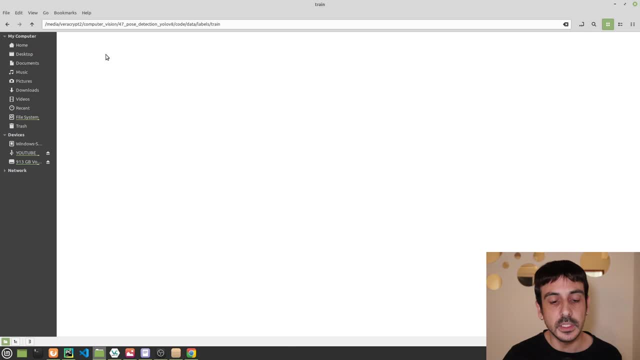 directories- train and ball- and within each one of these directories is where we have all of our images. and if we go to labels, we have also two directories- train and ball- and within each one of these directories is where we have all of our labels. so this is exactly how you need to structure. 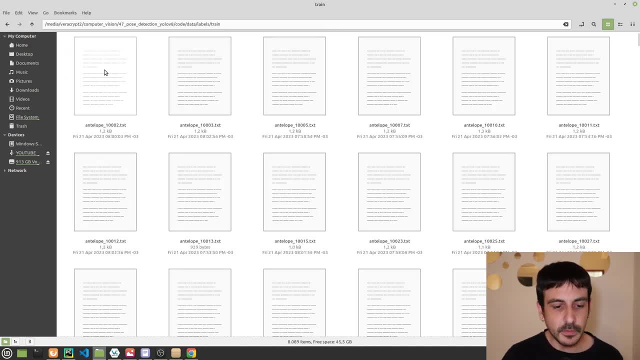 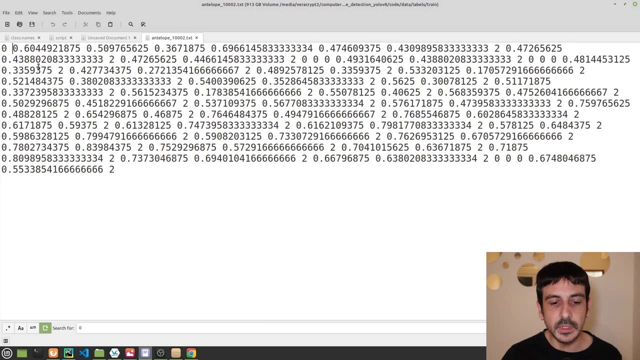 your file system. and now let me show you a little bit more how you create an association with the. show you one of these annotations files, one of these labels files, from the inside. let me show you how they look like. so this is a random annotations file. this is a random txt file. 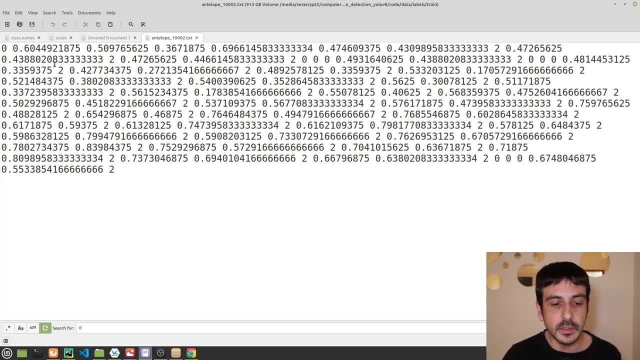 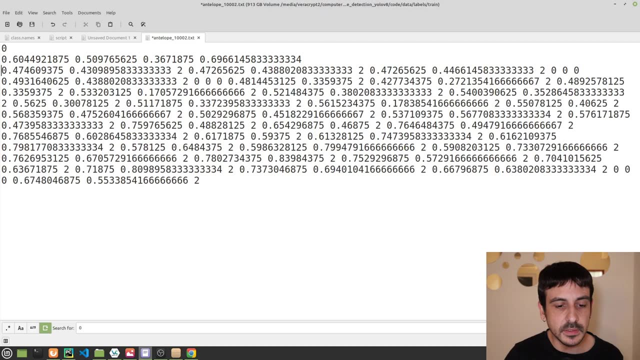 and this is exactly how you need to put all the data inside these files. the annotations are specified in the coco keypoint format, which is a very popular format for post detection. now let me show you something. i'm going to do, something which i'm obviously not going to save the changes. 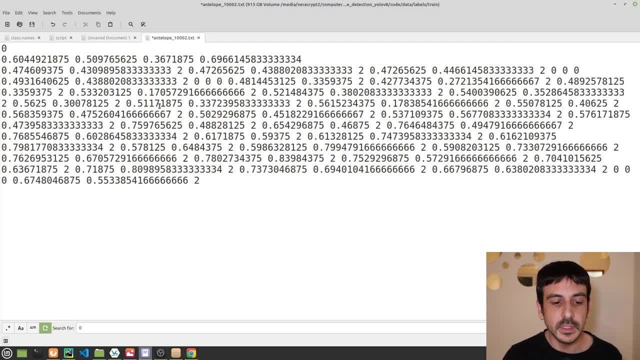 but it's going to be much better. in order to show you how this annotations format works right, how it looks like. so, basically you can see, the first number is a zero and this is our class id. in my case, i'm only, i only have one class, which is quadrupled, so in my case, this number will always. 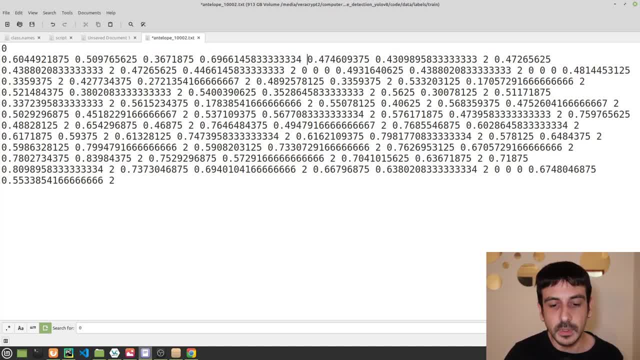 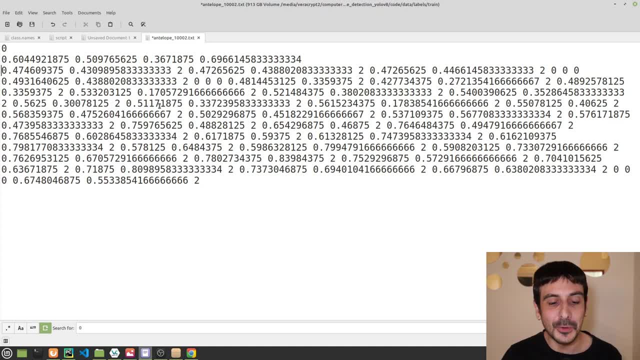 something i'm going to do- something which i'm obviously not going to save the changes, but it's going to be much better- in order to show you how this annotations format works right, how it looks like. so, basically you can see, the first number is a zero and this is our class id. in my case, i'm 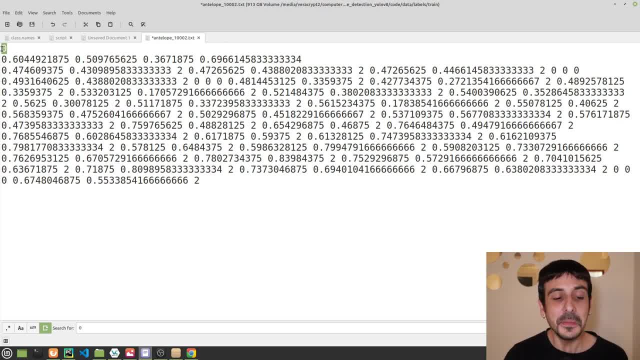 only. i only have one class, which is quadruped, so in my case this number will always be zero. but if you are making this project and you have many, many different classes, please remember that this number should be the class id. so if you have different classes, you will have different numbers. 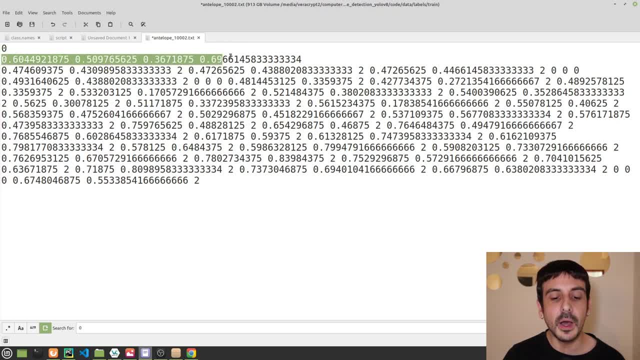 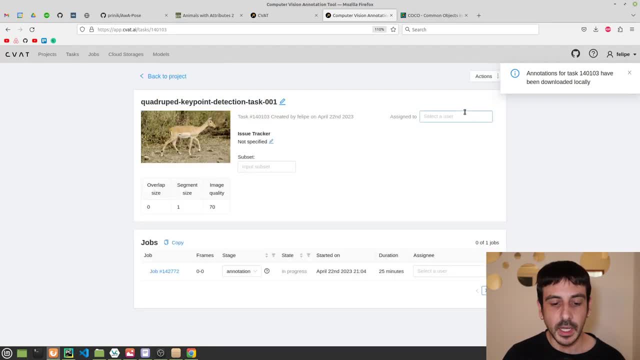 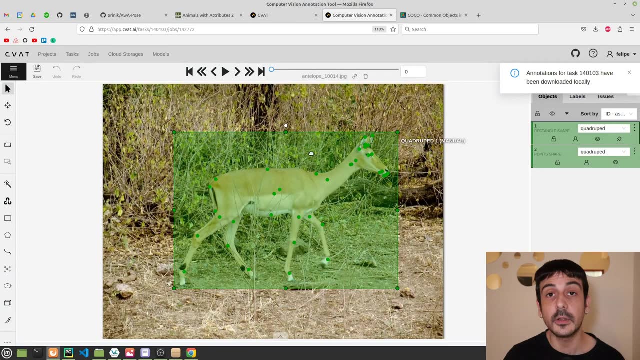 here now. the next four numbers are the bounding box of your object right. remember in cpat when we were annotating this data? i show you that not only we need to annotate the key points, but we also need to annotate the bounding box right, and we annotated the bounding 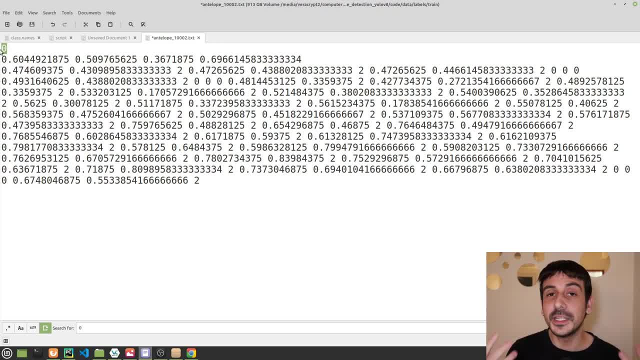 be zero, but if you are making this project and you have many, many different classes, please remember that this number is zero. and if you are making this project and you have many, many different, number should be the class id. so if you have different classes, you will have different. 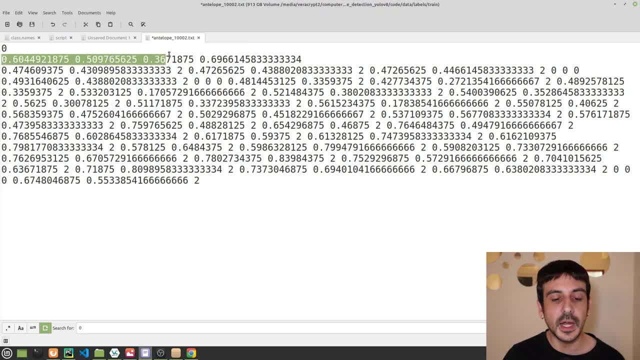 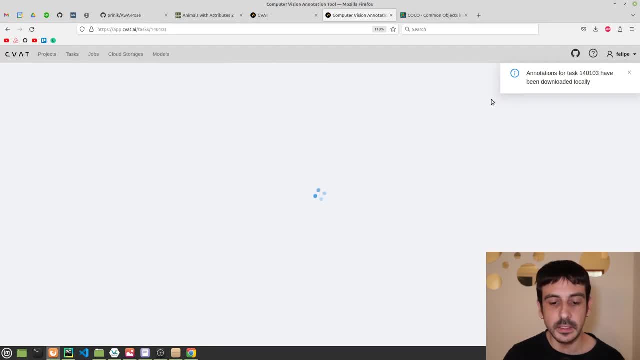 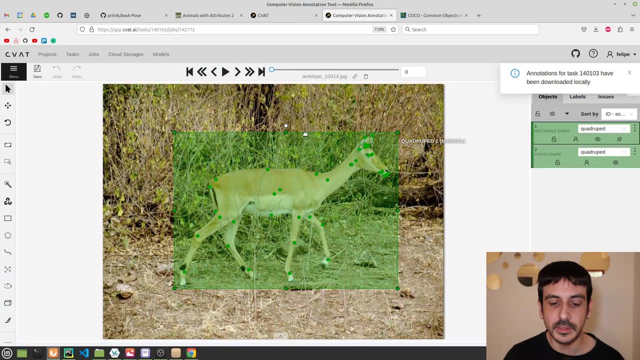 numbers here now. the next four numbers are the bounding box of your object right. remember in cbat when we were annotating this data? i show you that not only we need to annotate the key points, but we also need to annotate the bounding box right, and we annotated the bounding box. so these 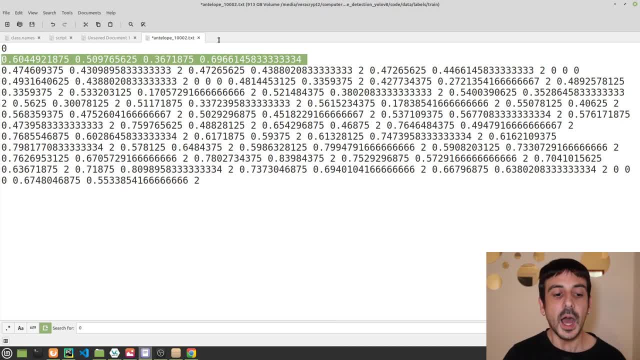 four elements. the four elements that come after the class id are the bounding box right, and this bounding box is specified in the yellow format, which is the x and y position of the center of the bounding box, and then the width and then the height of your bounding box. this is very important. so this number, these two numbers, are the x- y position. 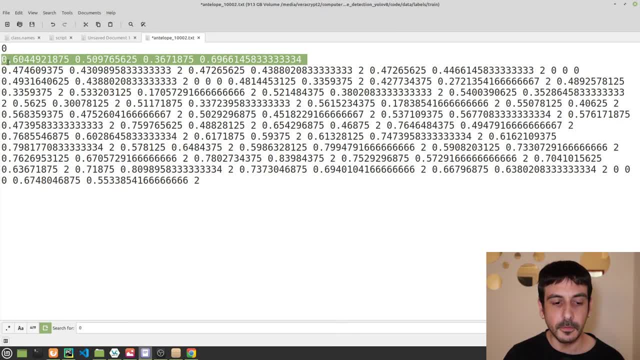 box. so these four elements, the four elements that come after the class id, are the bounding box right, and this bounding box is specified in the yolo format, which is the x and y position of the center of the bounding box and then the width and then the height of your bounding box. this is very important. so this number 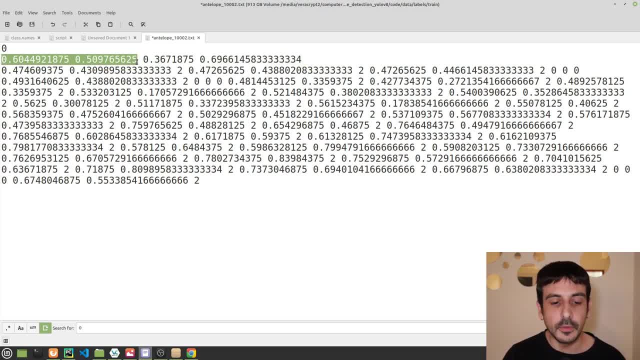 these two numbers are the x, y, position of the center of your bounding box, and then the width and the height and then all of the other numbers. let me show you. you can see that we have these two numbers, which are a float, and then we have the number two, and then we have exactly the same. 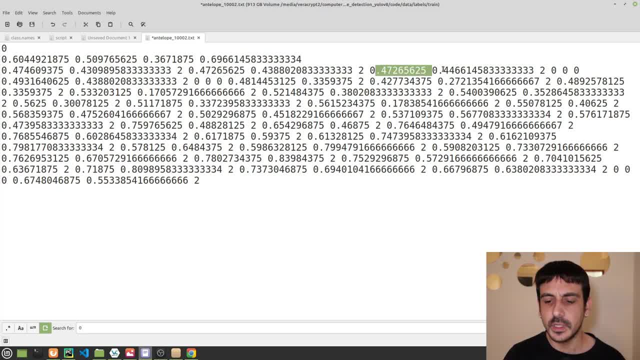 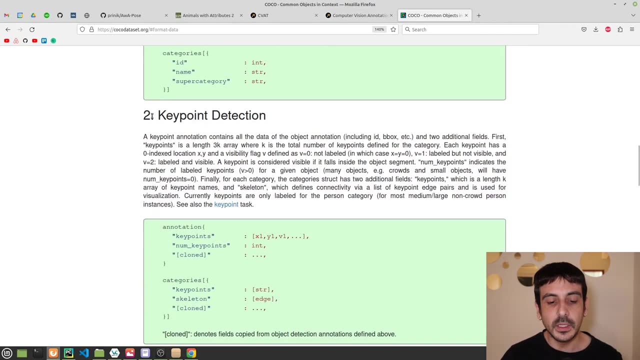 two numbers and another two, then two numbers and another two, then we have three sixes zeros, right? this looks like very, very strange. so now let's go back to my browser, because i want to show you this website, which is cocodata assetorg, and this is where we are going to see exactly how. 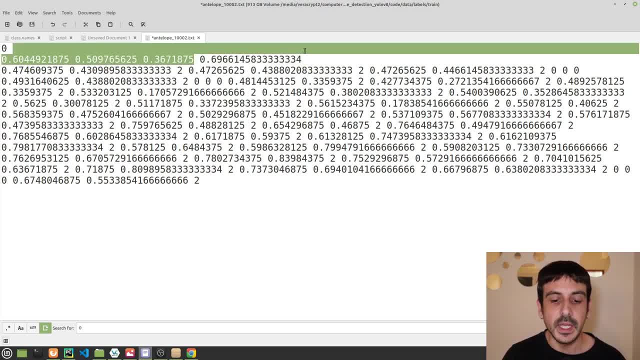 of the center of your bounding box, and then the width and the height, and then all of the other numbers. let me show you. you can see that we have these two numbers, which are the number of the number, which are a float, and then we have the number two, and then we have exactly the same two. 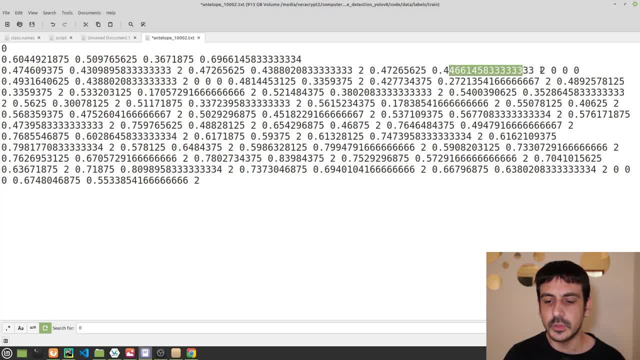 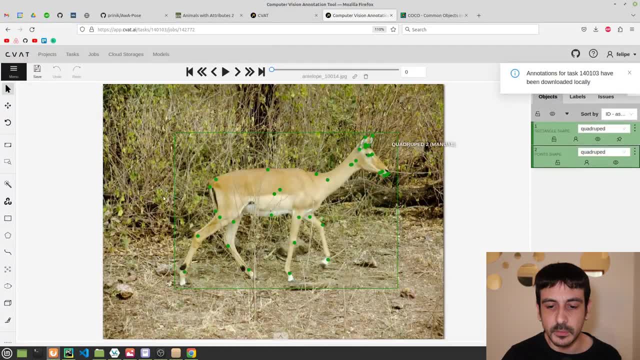 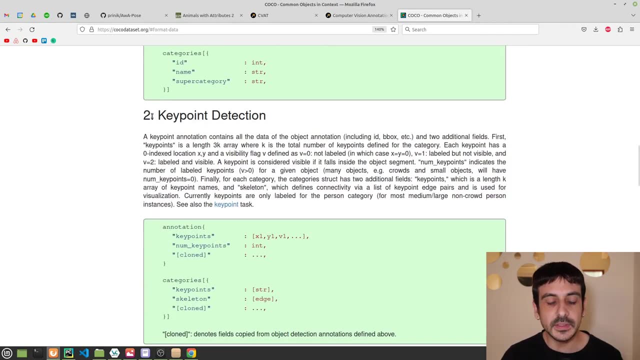 numbers and another two, then two numbers and another two, then we have three zeros, right? this looks like very, very strange. so now let's go back to my browser, because i want to show you this website, which is cocoadassetorg, and this is where we are going to see exactly how this format works. 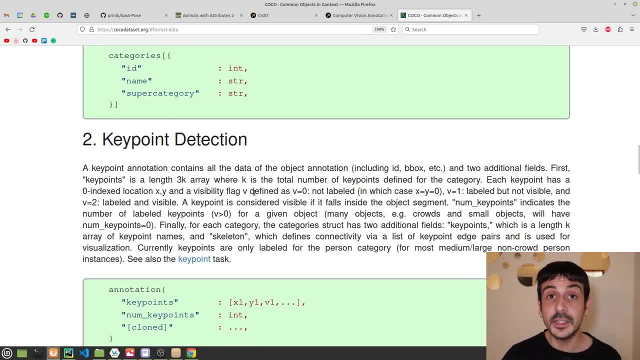 so if i go back to key point detection, you can see that this is our explanation about how this format works, and if i read something which is here, you can see that absolutely every single key point will be specified as x and y and a visibility flag b. so this means that for absolutely every single key point we are going 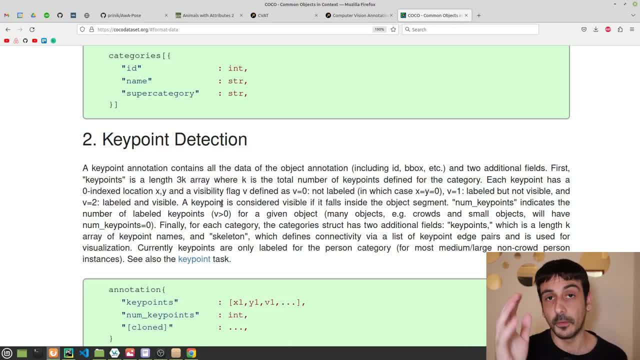 to have three values. we are going to have the x and y position of that given key point and we are also going to have another value, which is b, which is the visibility right. remember we were going to talk about visibility later on this tutorial. this is this is later on this. 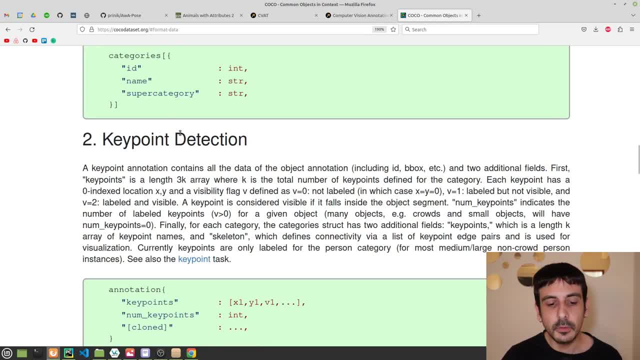 this format works. so if i go back to keypoint detection, you can see that this is our explanation about how this format works, and if i read something which is here, you can see that absolutely every single keypoint will be specified in the x and y position of the bounding box right. 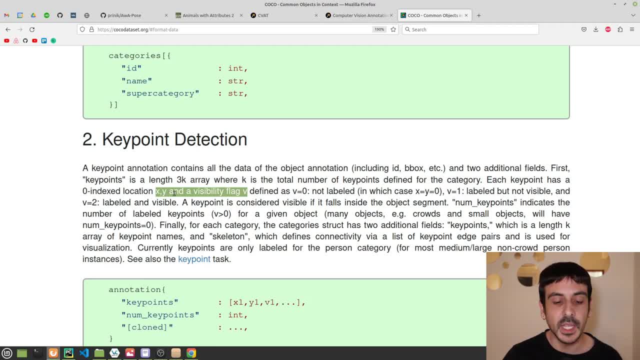 as x and y and a visibility flag, b. so this means that for absolutely every single key point, we are going to have three values. we are going to have the x and y position of that given key point and we are also going to have another value, which is b, which is the visibility right. remember we were 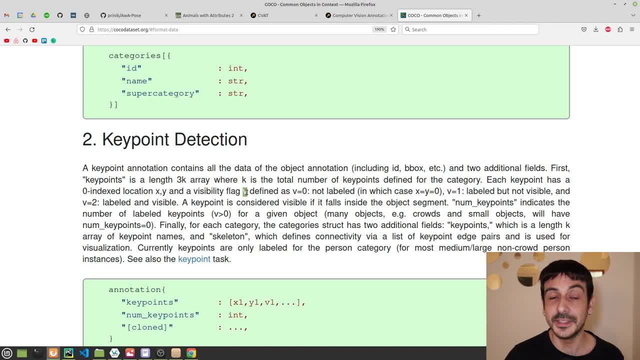 going to talk about visibility later on this tutorial. this is: this is later on this tutorial, so you can see that b has three possible values. b could be zero, and this means that the key point is not labeled, and in this case, x and y is going to be zero. two or b could be one, and this means 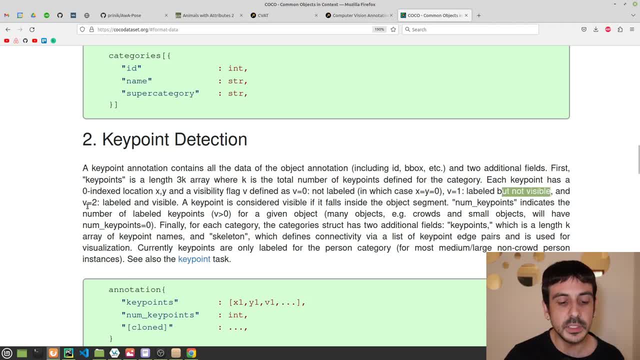 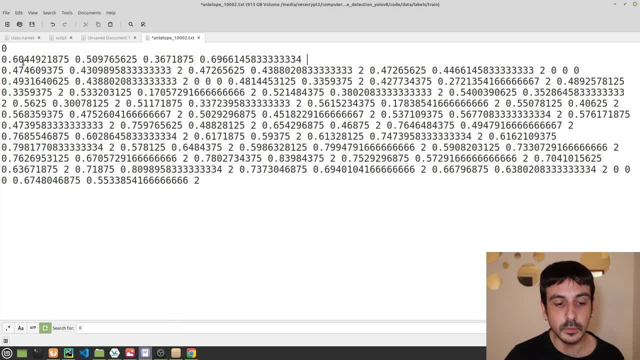 the key point is labeled but it's not visible, or b could be two, and this means the key point is labeled and it's also visible. and if we go back to the, to this file, to the annotations, you can see that if we start over here, we have two numbers. 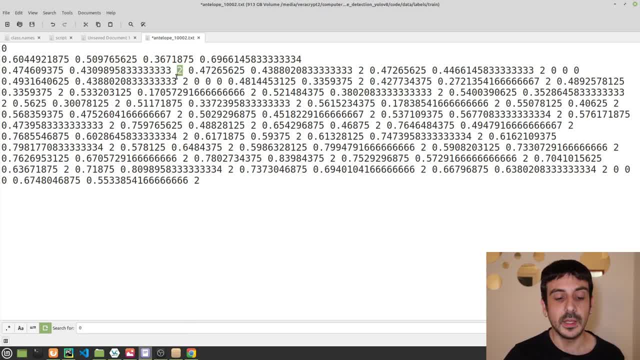 and then we have a two, which means this key point is annotated, is labeled and is also visible. now, if we continue, you can see that we have two numbers. and then we have another two, which means this other key point is also visible. now, if we continue, you can see exactly the same. 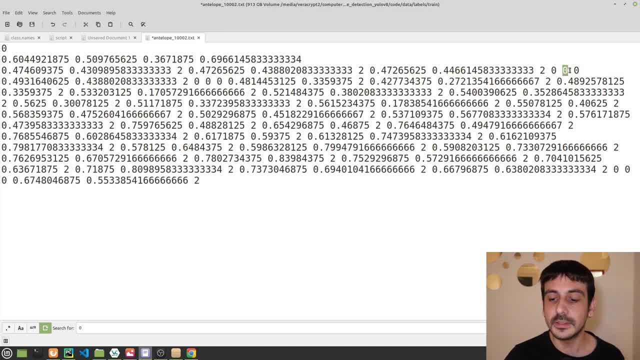 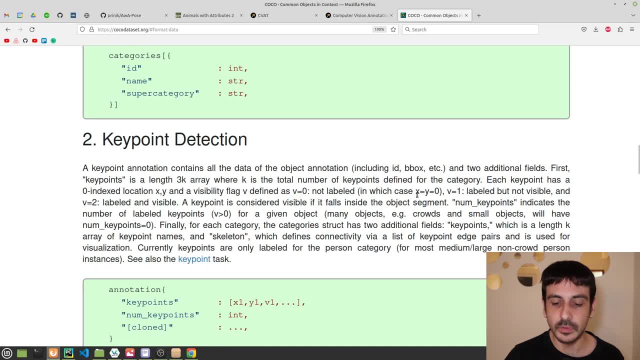 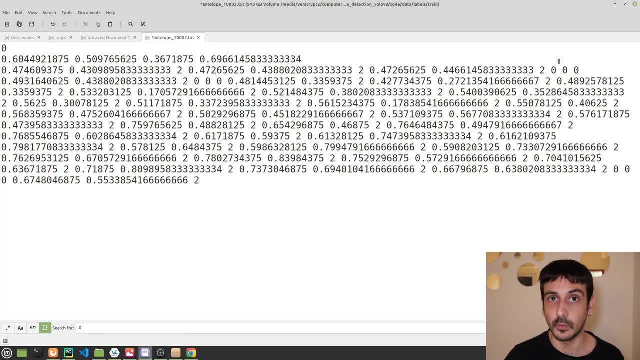 two numbers and then a two, and then, if we continue, you can see that this: we have three zeros and we are in this situation, right, b equals zero, so we also have x and y equals zero, and this means the key point is not labeled for this image, right? so long story short. 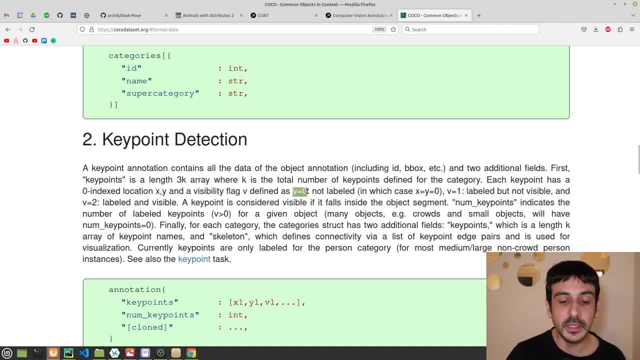 tutorial so you can see that b has three possible values. b could be zero, and this means that the key point is not labeled, and in this case, x and y is going to be zero. two or b could be one, and this means the key point is labeled, but it's not visible. or b could be two, and this means 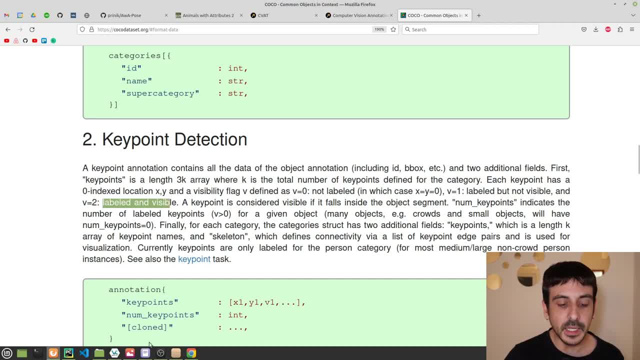 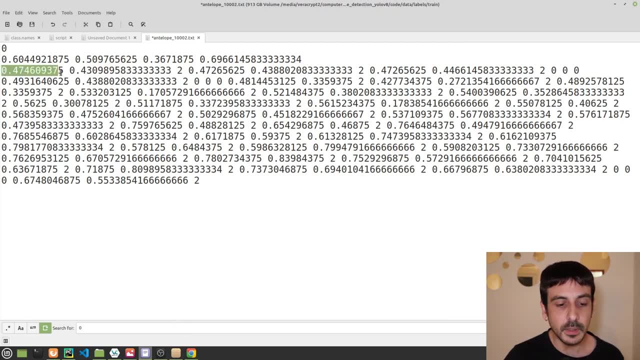 the key point is labeled and it's also visible. and if we go back to the uh, to this file, to the annotations, you can see that if we start over here, we have two numbers and then we have a two, which means this key point is annotated, is labeled and it's also visible. now, if we continue, you can. 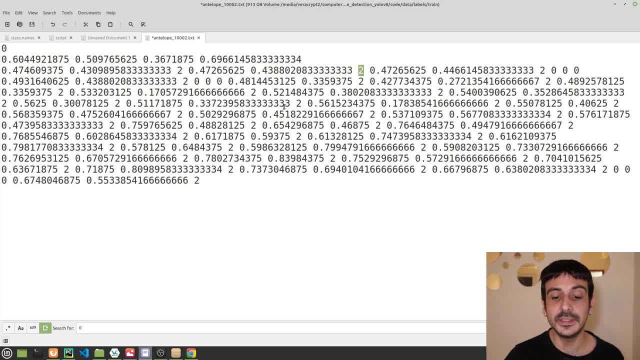 see that we have two numbers and then we have another two, which means this other key point is also visible now: if we continue, you can see exactly the same two numbers and then a two, and then, if we continue, you can see that this: we have three zeros. 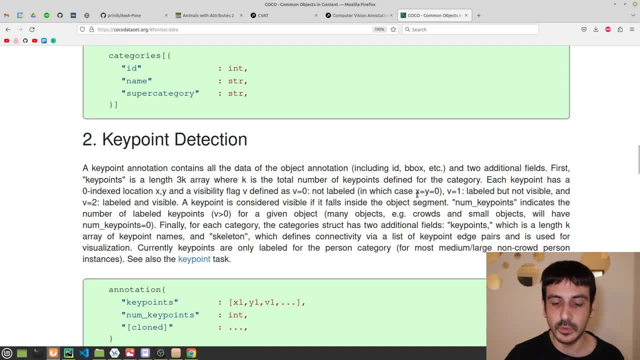 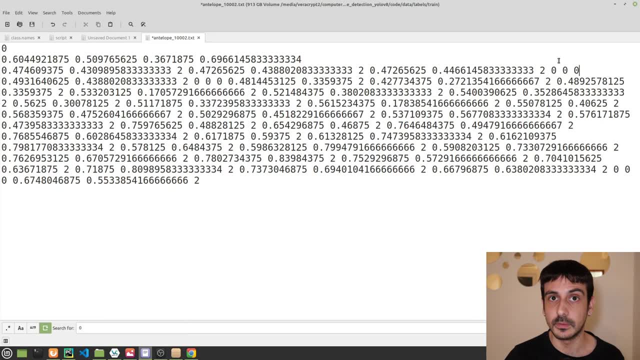 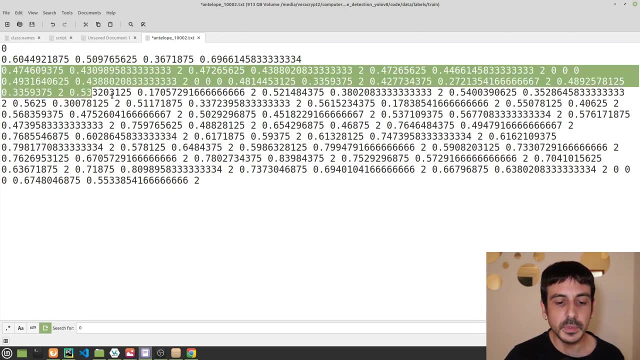 and we are in this situation. right, b equals zero, so we also have x and y equals zero, and this means the key point is not labeled for this image, right? so long story short. after the bounding box, all the other numbers will be the key points and you will have two values for the x and y position, and then 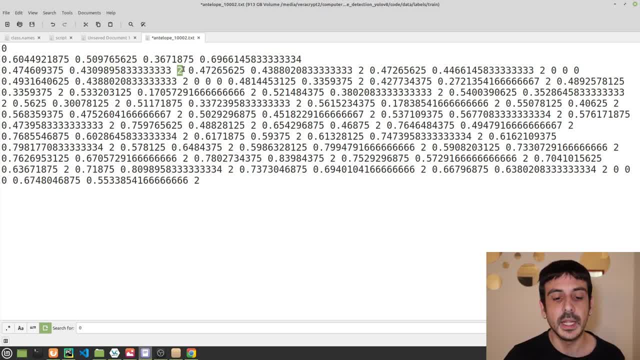 the third value will be the visibility of that even key point. now, this is one of the possible formats in which you could format your data, and this is going to work just fine. but yellow v8 also supports a key point annotation with only two values, which means that if you don't have the 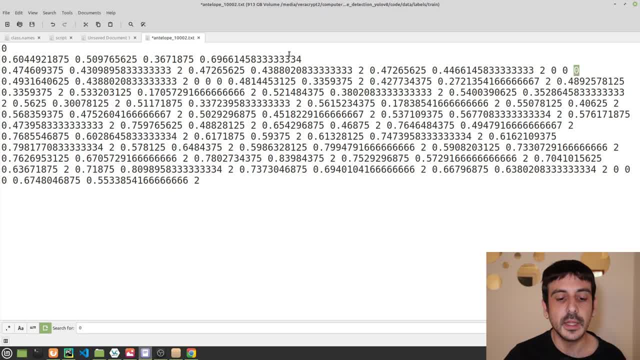 visibility information for all of your key points, then it doesn't matter, because yellow v8 also supports you. input your key points with only the x and y coordinates. so long story short. we have the first number, which is the class ID. then we have four numbers, which are: 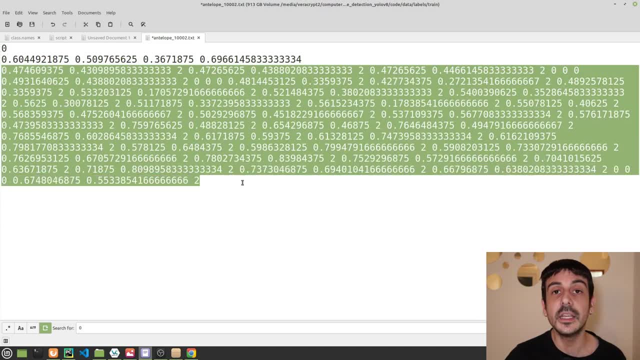 the bounding box and then all of the other numbers are the key points. and you can specify your key points with three coordinates for every key point, which means we we have the x and y and also the visibility for that key point, or you can specify all of your key points with only two coordinates. 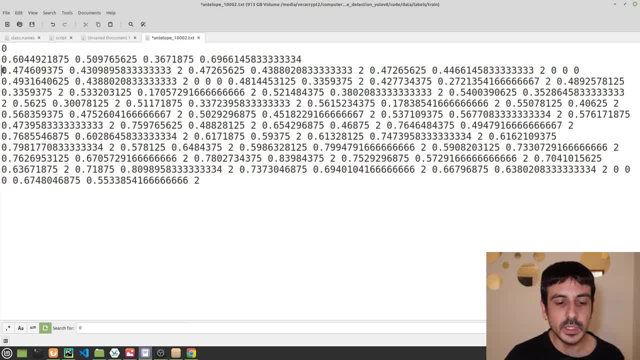 after the bounding box, all the other numbers will be the key points, and you will have two values for the x and y position, and then the third value will be the visibility of that even key point. now, this is one of the possible formats in which you could format your data, and this is going to work just 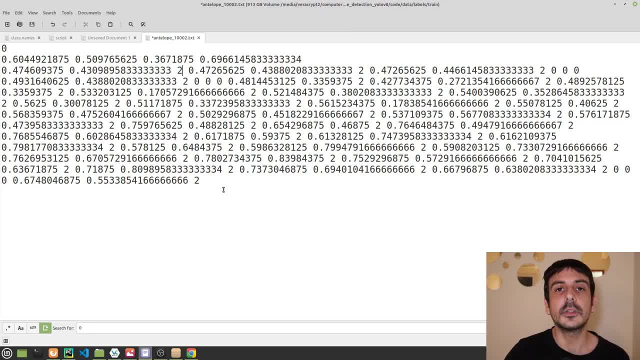 but yolo v8 also supports a key point annotation with only two values, which means that if you don't have the visibility information for all of your key points, then it doesn't matter, because yolo v8 also supports you input your key points with only the x and y coordinates. so long story short. 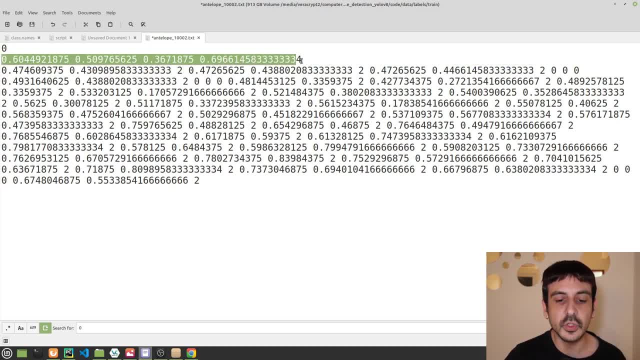 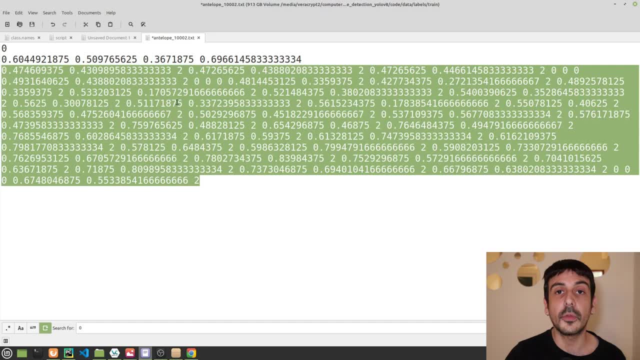 we have the first number, which is the class id, then we have four numbers which are the bounding box, and then all of the other numbers are the key points, and you can specify your key points with three coordinates for every key point, which means we we have the x and y and also the visibility for 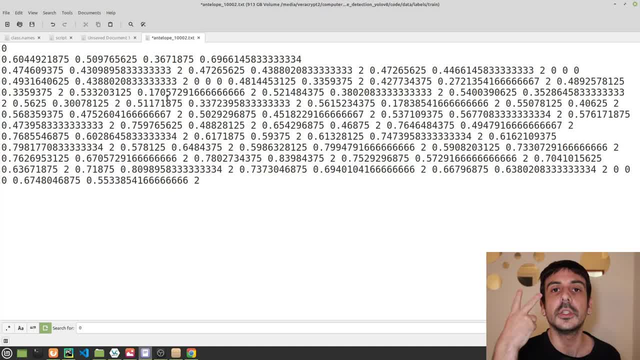 that key point, or you can specify all of your key points with only two coordinates, which means it's the x and the y coordinate of that given key point. so this is the way you need to label your data, this is the way you need to structure all of your annotations, and please remember to do it this way. 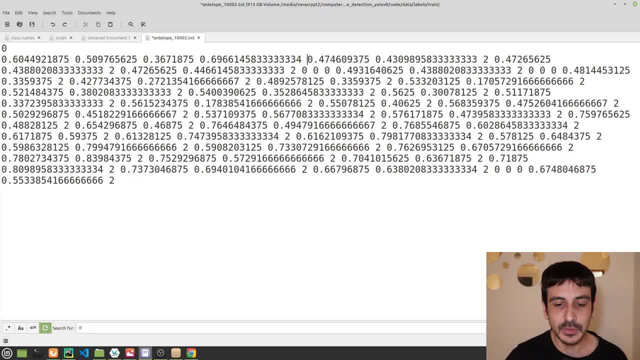 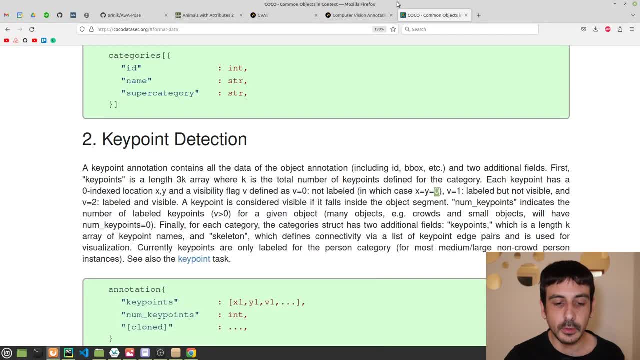 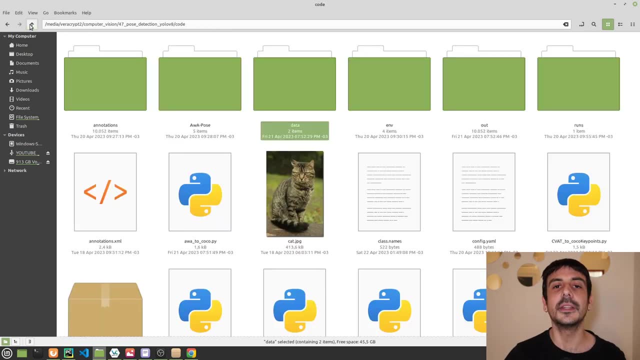 otherwise it's not okay going to work. so now i'm just going to press ctrl c, because obviously i'm not going to save all of your, all of those changes, and that's pretty much all about how to format your data, how to format your file system and how to put your data into the exact format you need in order to train this post. 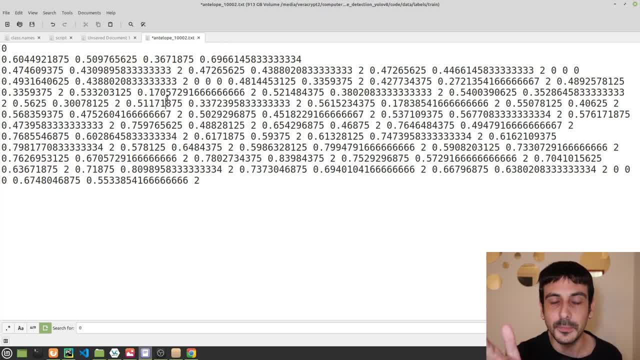 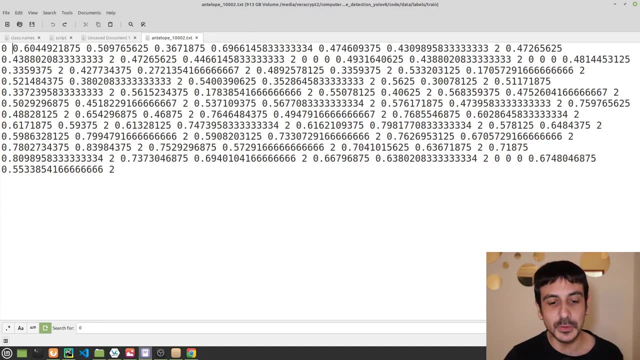 which means it's the x and the y coordinate of that given key point. so this is the way you need to label your data, this is the way you need to structure all of your annotations, and please remember to do it this way, otherwise it's not going to work. so now I'm just going to press ctrl c, because obviously I'm not going to. 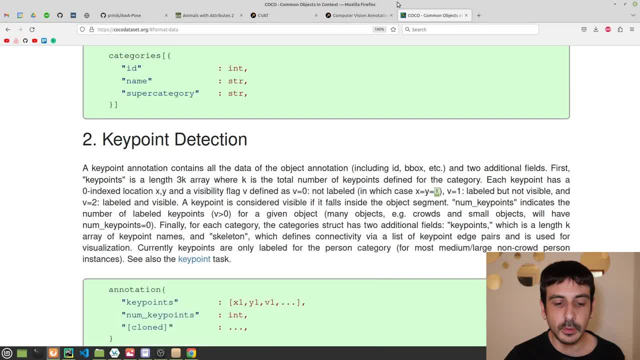 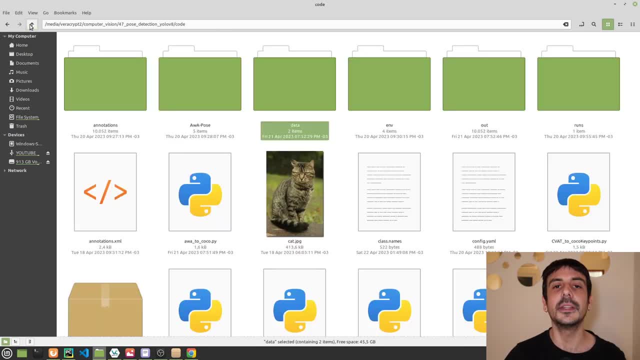 save all of your, all of those changes, and that's pretty much all about how to format your data, how to format your file system and how to put your data into the exact format you need in order to train this post detector using yellow v8. and now let's go back to PyCharm, let's go back to the. 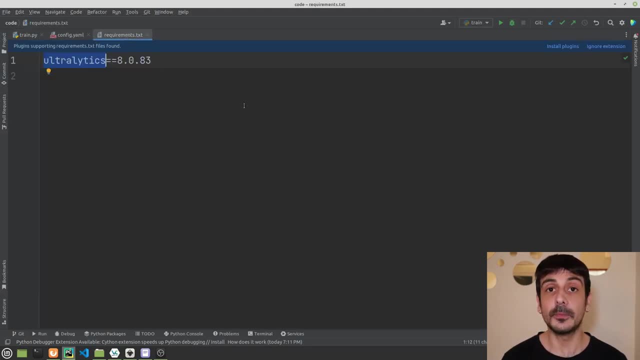 PyCharm project I created for today's tutorial, and the first thing you need to do if you want to train this post detector using yellow v8 is to install the project's requirements, which is basically ultralytics. so please remember to install this package before starting with this training, because otherwise you will not be able. 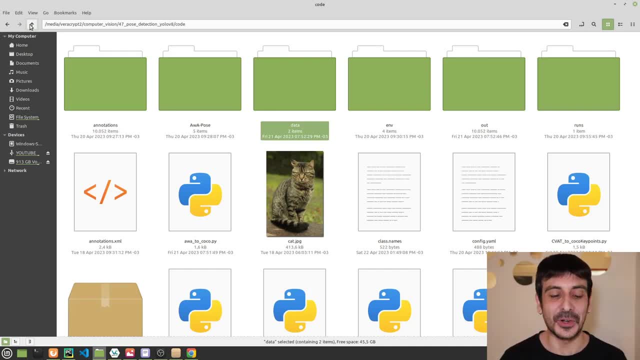 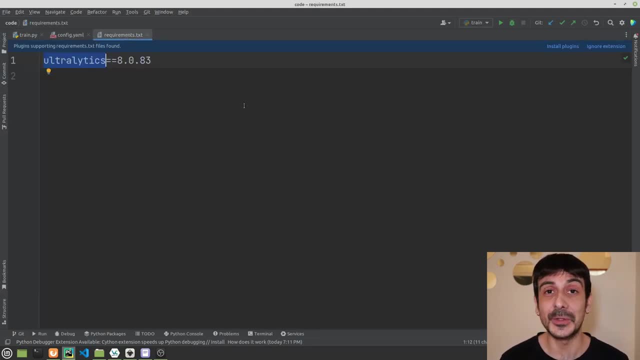 detector using yolo v8. and now let's go back to pycharm. let's go back to the pyjama project i created for today's tutorial, and the first thing you need to do if you want to train this post detector using yolo v8 is to 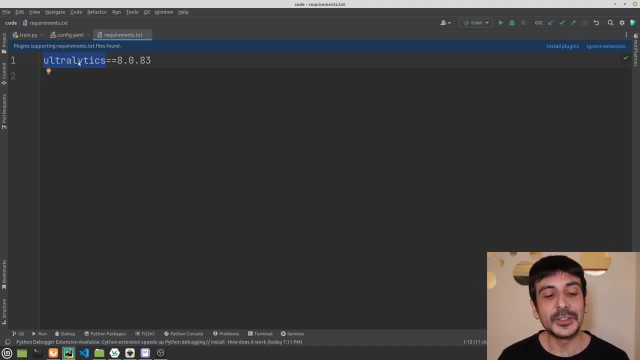 install the projects requirements, which is basically ultralytics. so please remember to install this package before starting with this training, because otherwise you will not be able to train a post detector using yolo v8. so once you have installed ultralytics, let's go back here to 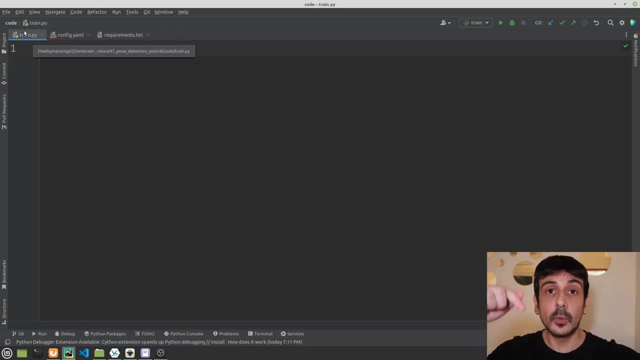 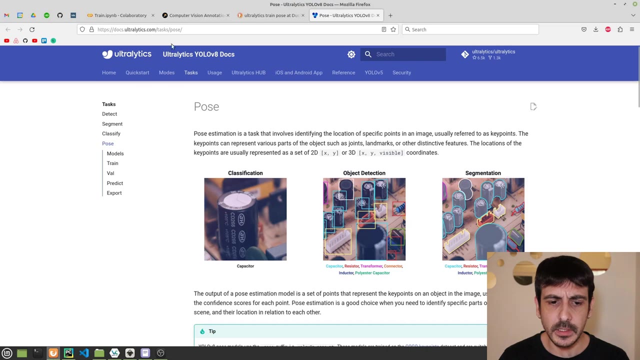 this file i created, which is trainpi. i'm going to show you exactly what you need to code in this file in order to do your training. and in order to do so, let's go back here, which is ultralytics website, and let's go to the training map and the post detector, because now you have to create a post. 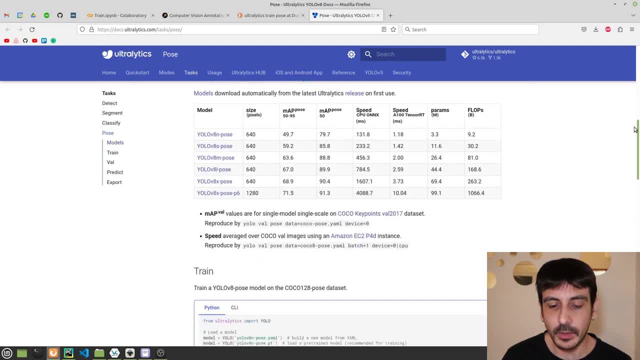 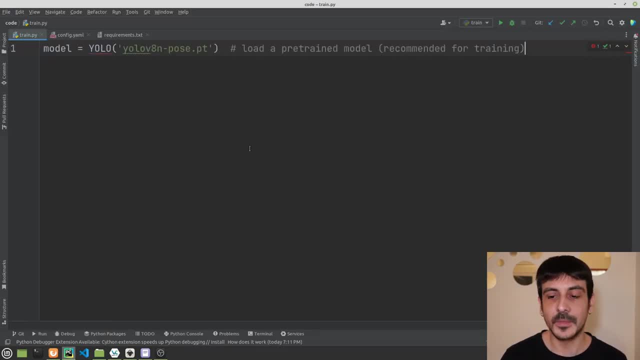 to the pose page and let's scroll down until this section over here, and the only thing i'm going to do is i'm going to copy and paste this line and then i'm going to copy and paste this other line, right? so this is basically all we needed to do in order to train this model, and obviously i need to. 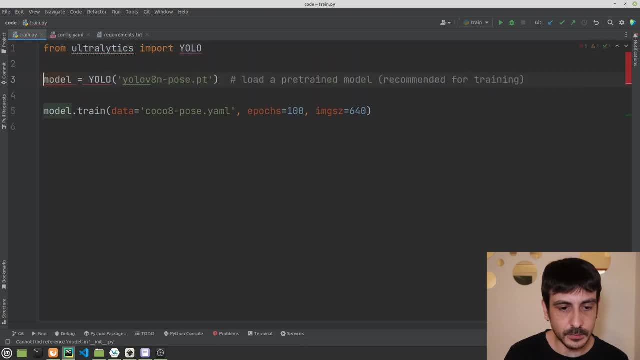 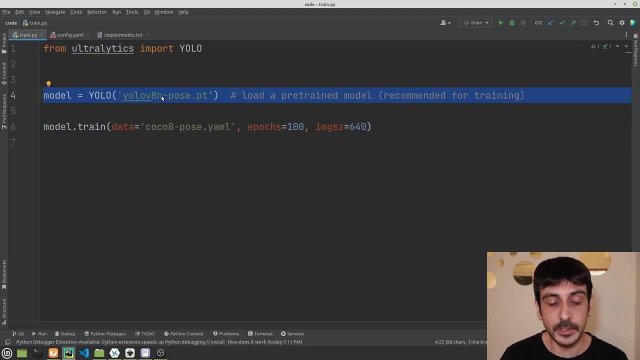 import from multi analytics: import yolo, and that's pretty much all. so this sentence over here, we can just leave it as it is. we can just leave it in this default value. but this one, i am going to make a couple of changes. i'm going to change the number of epochs i'm going to train for only one. 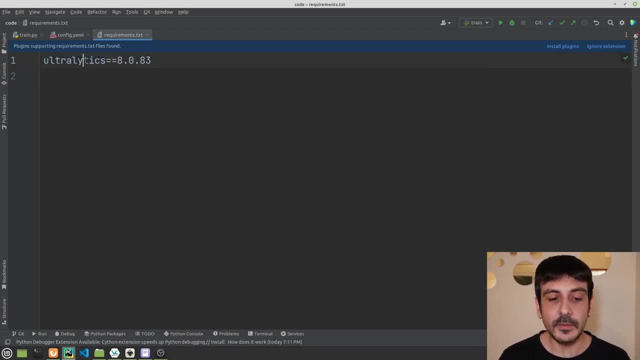 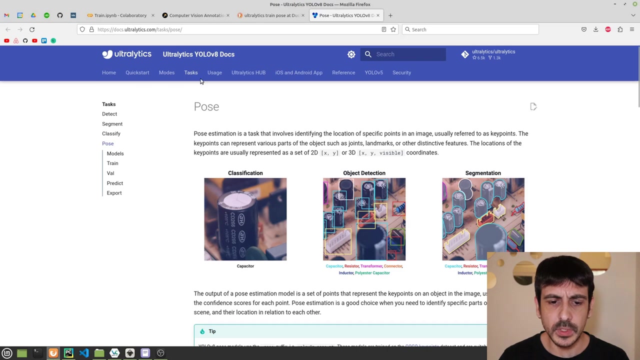 to train a post detector using yellow v8. so, once you have installed ultralytics, let's go back here, to this file I created, which is trainpi. I'm going to show you exactly what you need to code in this file in order to do your training. and in order to do so, let's go back here, which is ultralytics website. 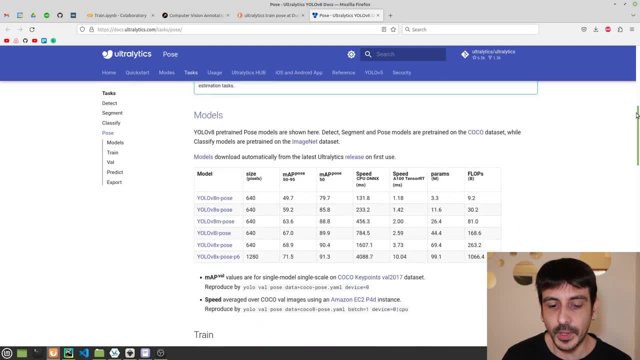 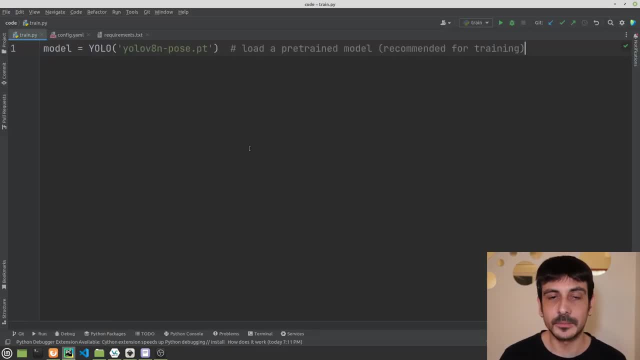 let's go to the pose page and let's scroll down until this section over here, and the only thing I'm going to do is I'm going to copy and paste this line and then I'm going to copy and paste this other line, right? so this is basically all we needed to do in order to train this model, and 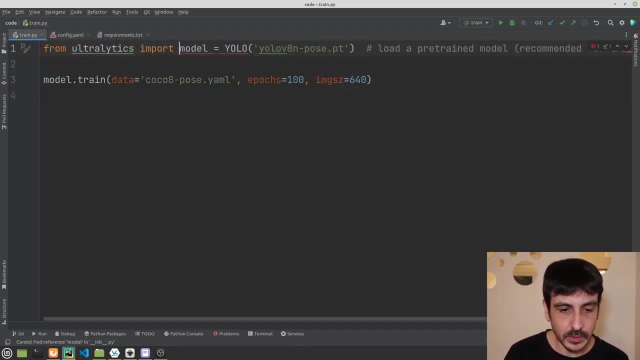 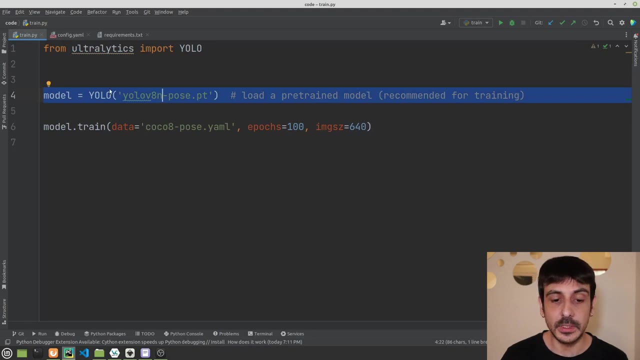 obviously I need to import from Ultralytics, import Yolo, and that's pretty much all. so this sentence over here, we can just leave it as it is. we can in this default value. but this one, i am going to make a couple of changes. i'm going to change the. 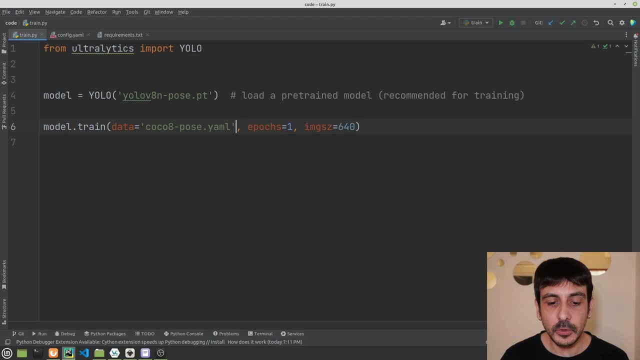 number of epochs. i'm going to train for only one epoch for now, and i'm also going to change change the location of the configuration file. i'm going to use this file, which is configyaml, and now i'm going to show you how this configyaml looks like, so you can see that this is the configuration file. 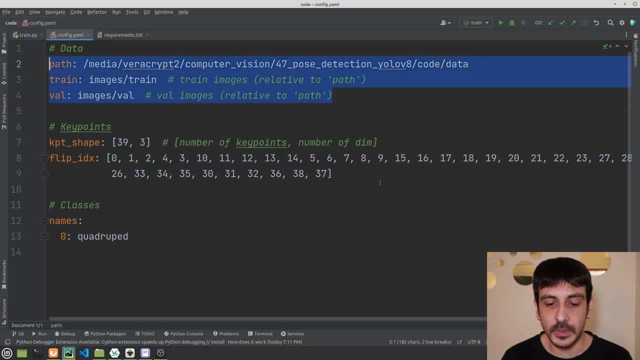 i am going to use in this tutorial. we have three sections, one of them for data, then key points and then classes. and let's go to the data section first. this is where you're going to specify all the locations to your data, to your images and your labels. so basically, you need to specify: 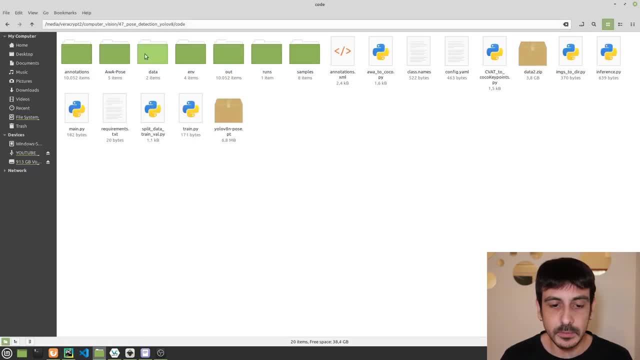 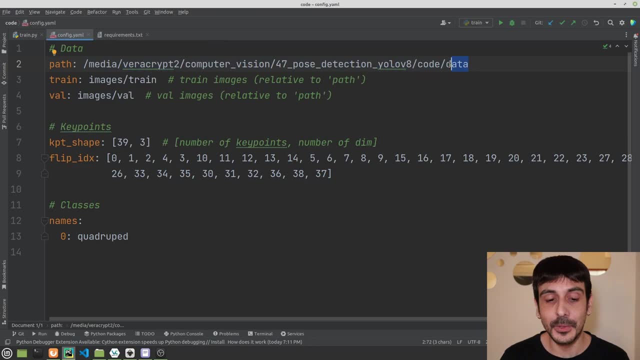 the root directory, the directory containing your data, which in my case is this one. remember the root directory. this is the directory which contains the images and the labels folders, and then you need to specify what's the location of the training images and the validation images. if you have made everything as i show you in this tutorial, as i showed you a few minutes ago, 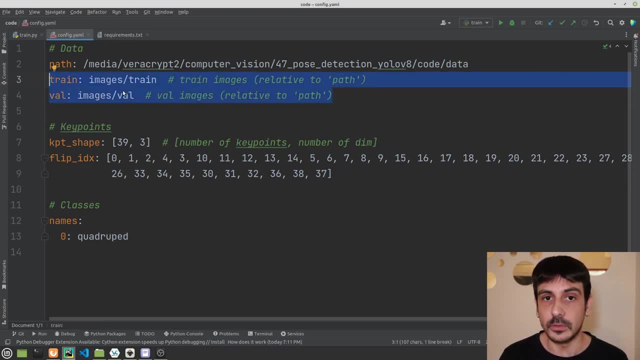 then you can just leave these two lines in these values, right, you can just leave everything as it is and everything will work just fine. the only thing you need to add is the location of your root directory. now let's go to this section over here, which is the key points, and we have two. 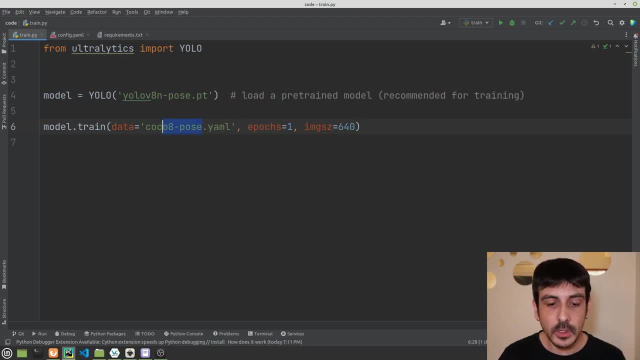 epoch for now, and i'm also going to change change the location of the configuration file. i'm going to use this file, which is configyaml, and now i'm going to show you how this configyaml looks like, so you can see that this is the configuration file i am going to use in this. 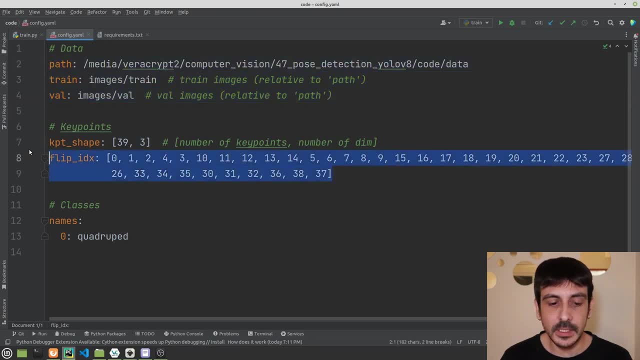 tutorial. we have three sections: one of them for data, then keypoint and then classes. and let's go to the data section first. this is where you're going to specify all the locations to your data, to your images and your labels. so basically, you need to specify the root. 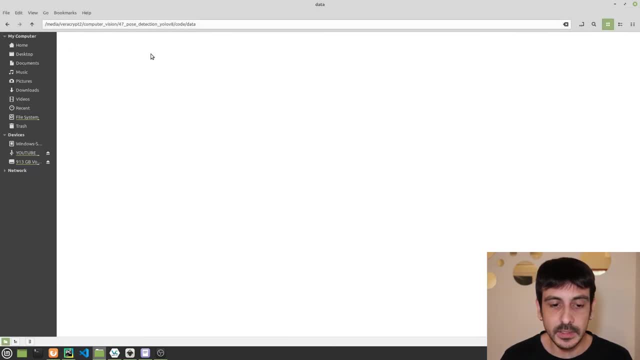 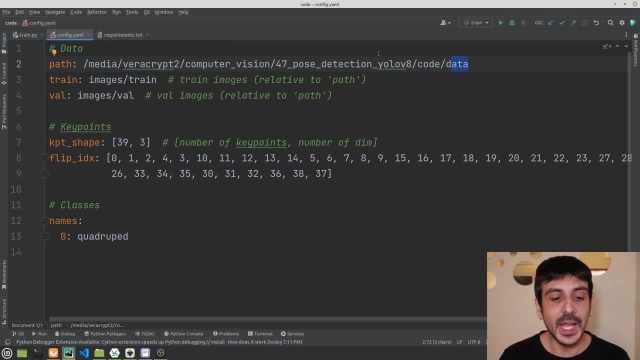 directory, the directory containing your data, which in my case, is this one. remember the root directory. this is the directory which contains the images and the labels folders, and then you need to specify what's the location of the training images and the validation images. if you have made everything as i show you in this tutorial, as i showed you a few minutes ago, 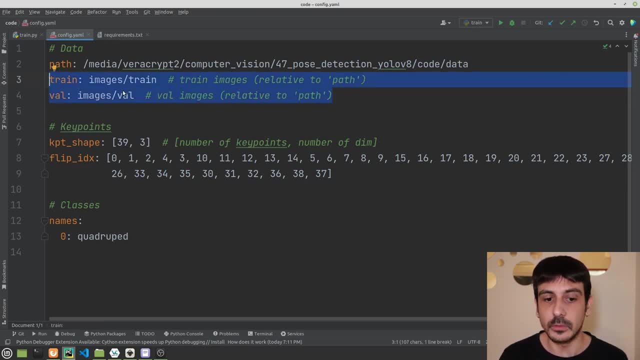 then you can just leave these two lines in these values, right, you can just leave everything as it is and everything will work just fine. the only thing you need to add is the location of your root directory. now let's go to this section over here, which is the keypoints and we have. 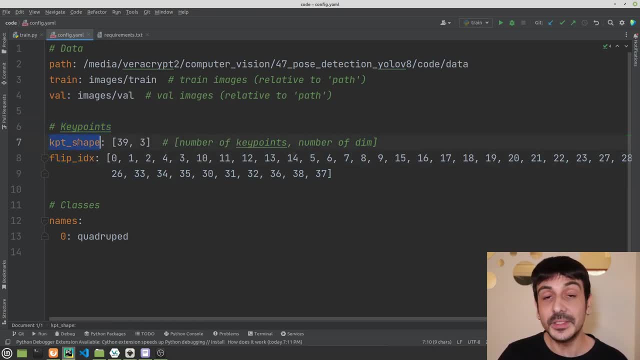 two keywords, which are keypoint shape and flip index, and these two keywords are completely and absolutely new for us. this is something we haven't seen before in any of my previous tutorials about yellow v8, and you can see that in the case of keypoint shape- in my case, it says 393. 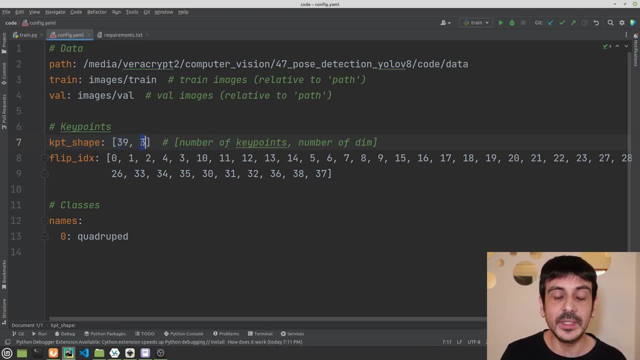 that's because i have 39 keypoints and i'm using the x, y and b format. right, i'm using three values for every single keypoint. so in my case, this that's why i have a three over here. so this is how many keypoints you have in your data and this is what format are you using, if you use you're using 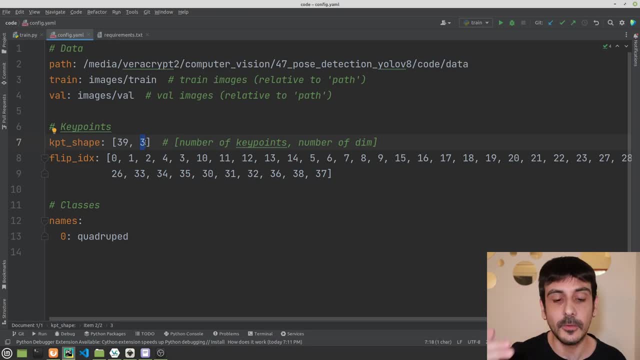 to specify a true, or if you're using the x, y and b format, and in that case you will need to set a three, as i am doing over here. so that's for keypoint shape. and now let me explain what flip index is. and in order to further explain what this keyword means, i made a drawing over here. 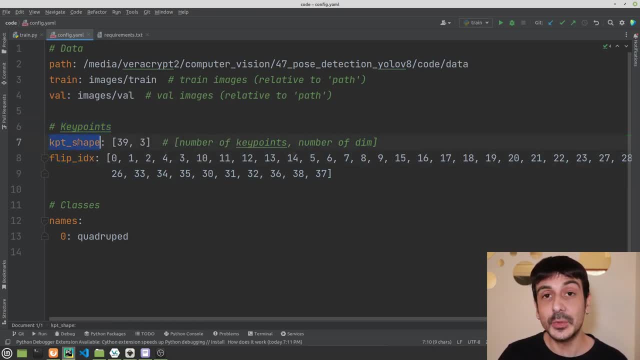 keywords, which are key point shape and flip index, and these two keywords are completely and absolutely new for us. this is something we haven't seen before in any of my previous tutorials about yellow v8, and you can see that in the case of key point shape- in my case, it says 39, 3.. 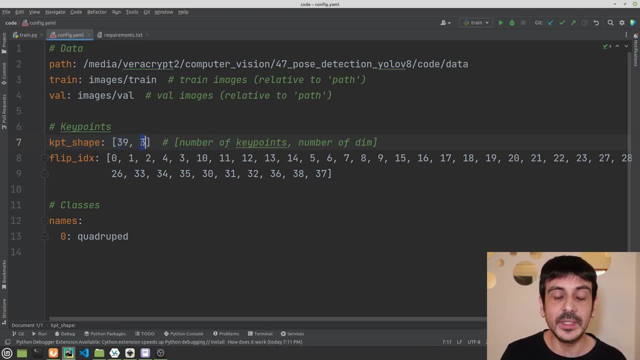 that's because i have 39 key points and i'm using the x, y and b format. right, i'm using three values for every single key point. so in my case, this that's why i have a 3 over here. so this is how many key points you have in your data and this is what format are you using if you use you're using 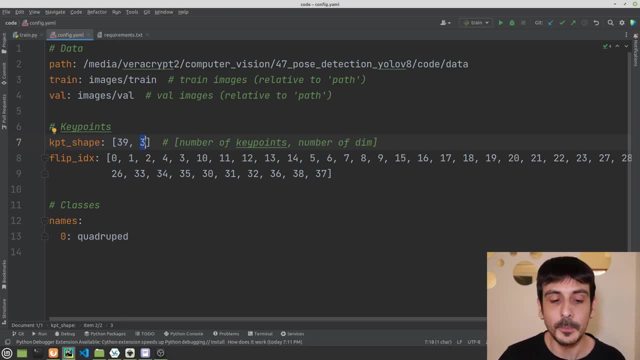 the x- y format. in that case you will need to specify the key point shape and flip index and specify a 2, or if you're using the x, y and b format, and in that case you will need to set a 3, as i am doing over here. so that's for key point shape, and now let me explain what flip index is. 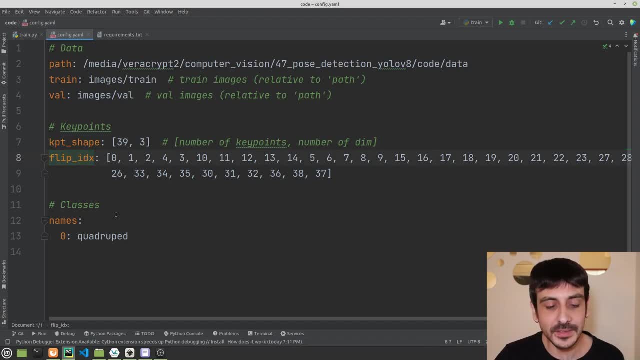 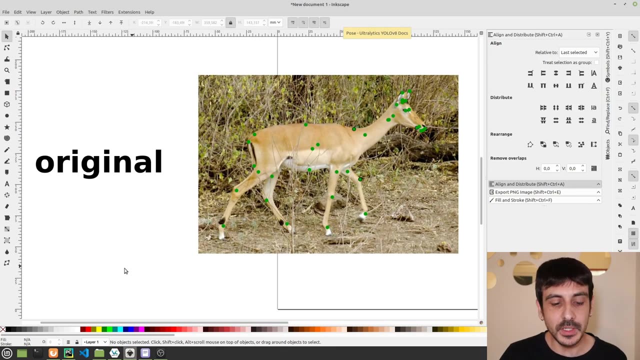 and in order to further explain what this keyword means, i made a drawing over here where i'm going to show you exactly what it means. so you can see that this is a random image in my data set and actually this is the same image i used in order to show you how the annotation process looks like. 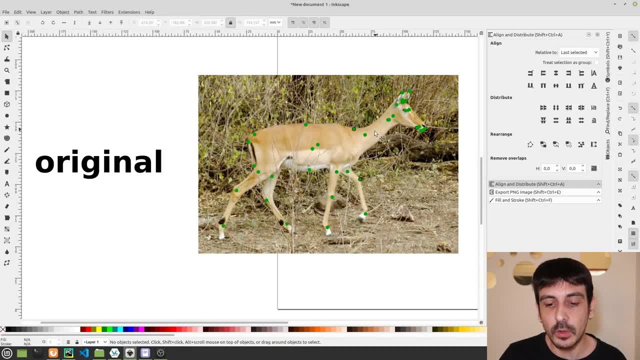 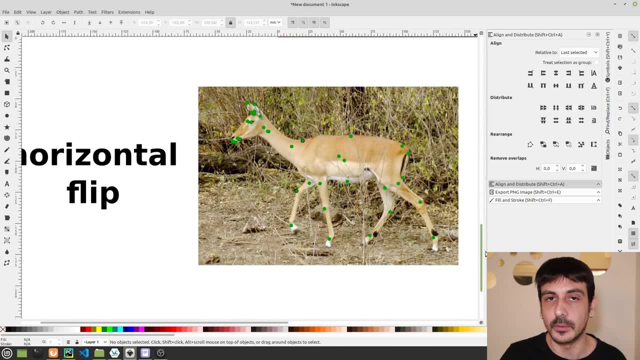 for this data, and you can see, this is a quadruple, with all of its key points drawn on top. right now, let me show you what happens if i flip this image horizontally. right, this is what i get. you can see that this is exactly the same image, but the only thing i did was to flip it horizontally. 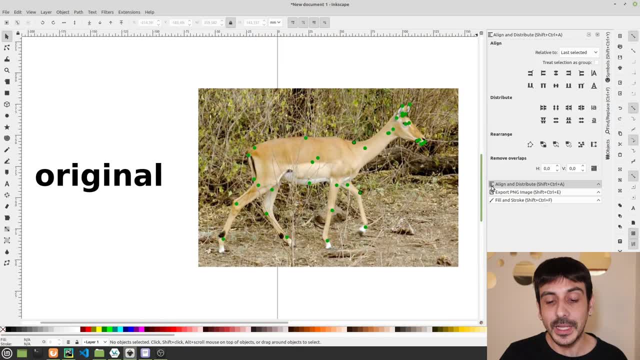 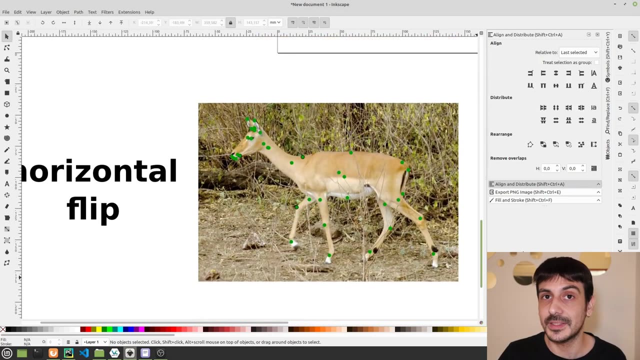 if i flip an image horizontally, the now, everything that used to be one of the sides now is the other side, right. everything that used to be the right side now is the left side side, and the other way around: everything that used to be the left side, now it's the right side. 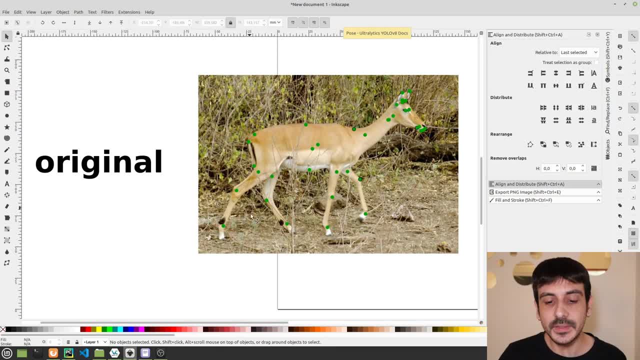 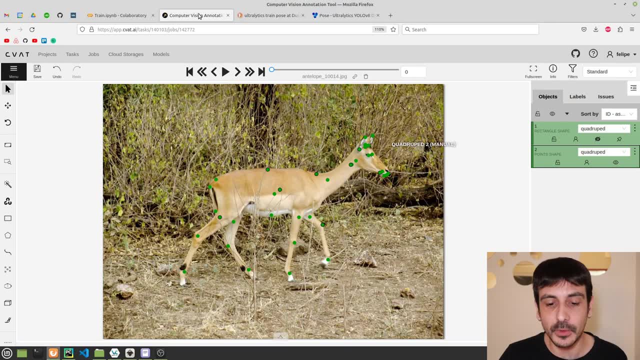 where i'm going to show you exactly what it means. so you can see that this is a random image in my dataset and actually this is the same image i used in order to show you how the annotation process looks like like for this data and you can see, this is a quadruple with all of its keypoints. 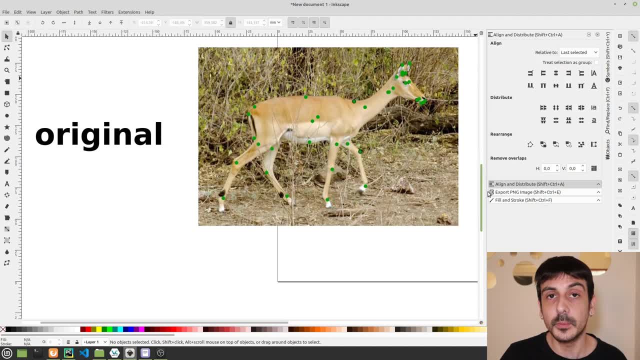 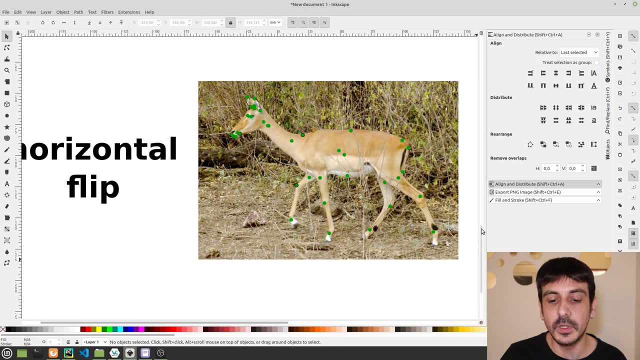 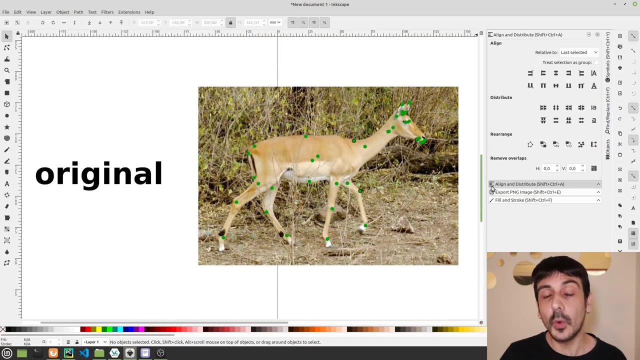 drawn on top. right now, let me show you what happens if i flip this image horizontally. right, this is what i get. you can see that this is exactly the same image, but the only thing i did was to flip it horizontally. if i flip an image horizontally, the now everything that used to be. 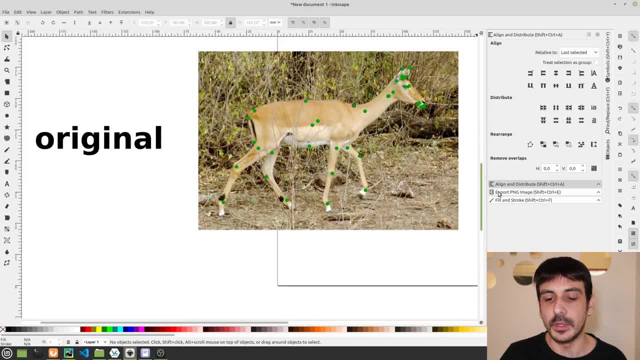 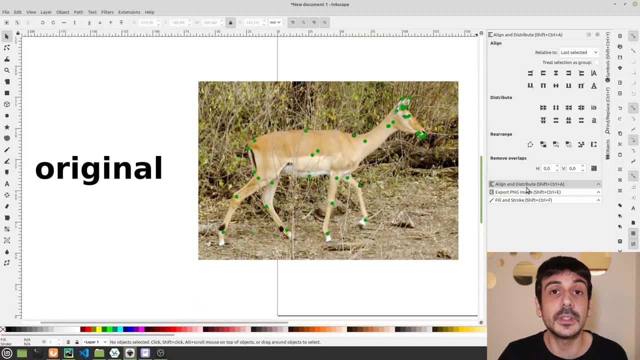 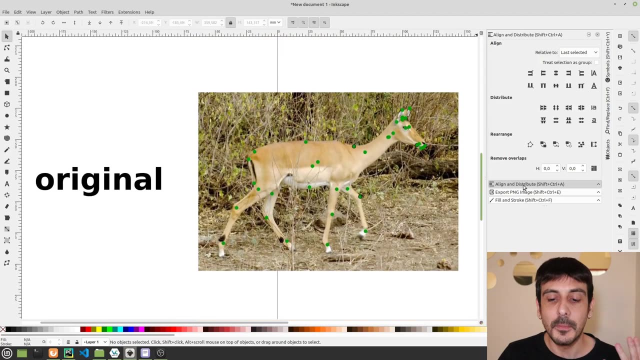 one of the sides now is the other side, right. everything that used to be the right side now is the left side, and the other way around: everything that used to be the left side now it's the right side. that's only what happens when you are flipping an image horizontally. but remember, we have many, many 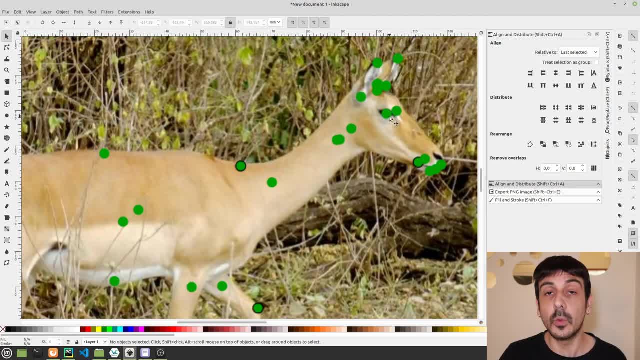 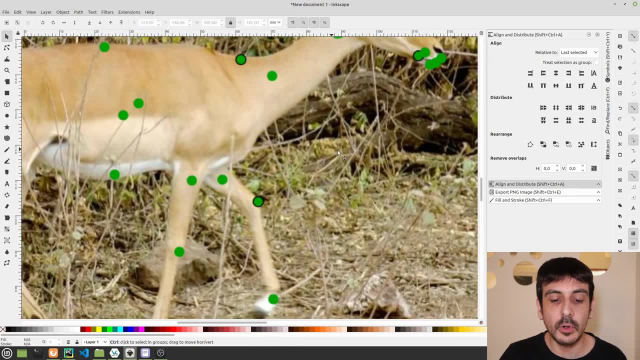 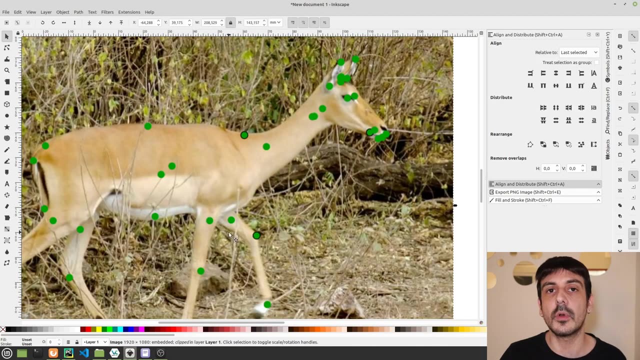 different key points and many of these key points were related to one of the sides. for example, we had a key point for the right eye. we also had key points for the right ear. we had key points for the right legs, and the same situation for the left eye, the left ear and the left legs right. 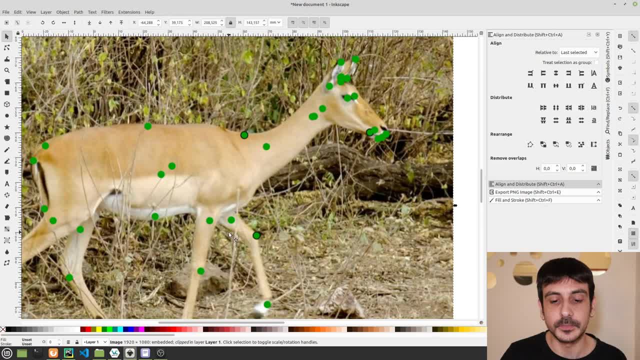 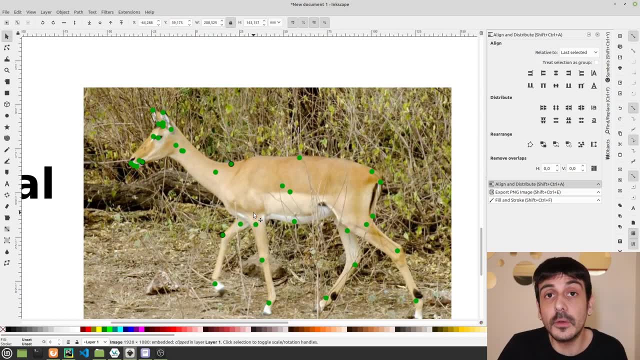 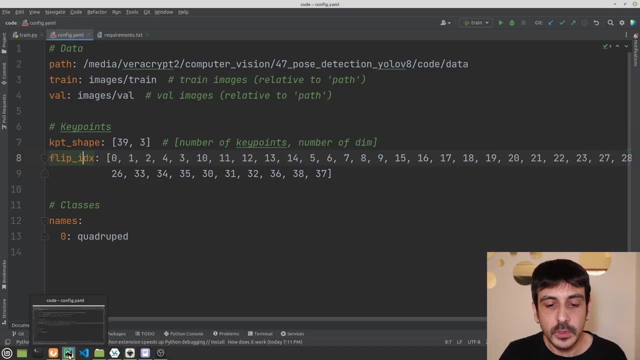 side. so we have all of these key points that are related to one of the sides. if we flip the image horizontally, then we should be doing something with all of these key points which are related to one of the sides, right when we are training a model using yolo v8, when we are 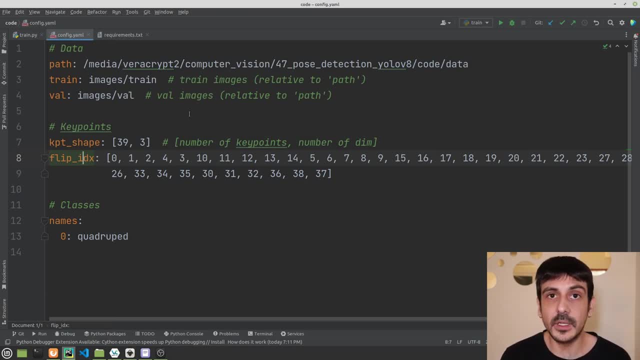 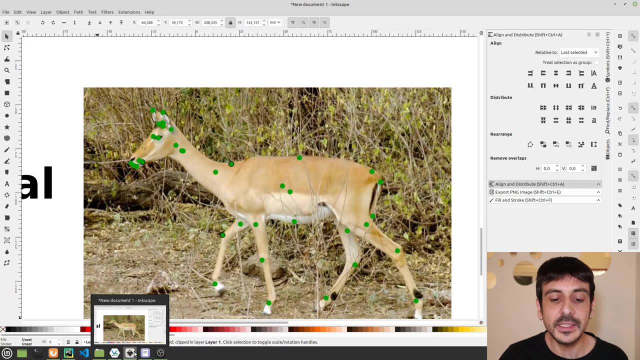 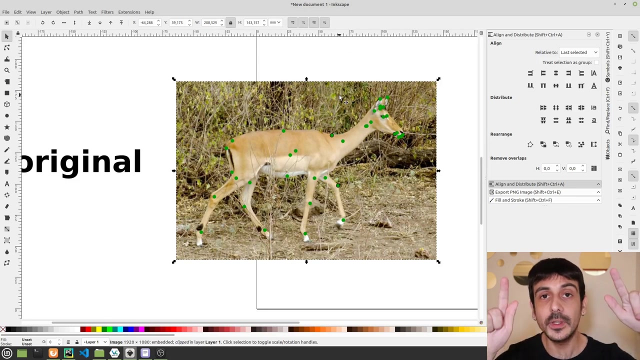 training this type of model. one of the steps, one of the stages in this process, in the training process, is to do something which is called data augmentation, and this data augmentation is called data augmentation means that we are taking the data and we are doing different transformations with this data. one of the transformations we are doing is related to flipping the image. 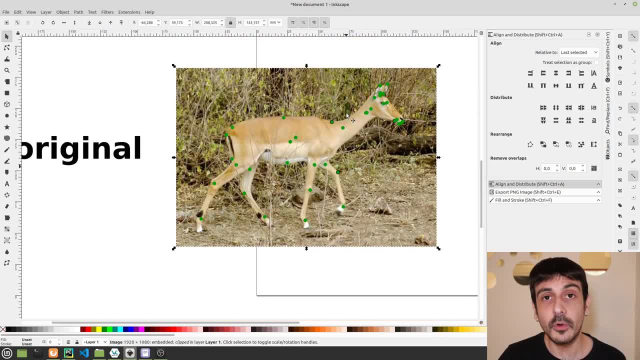 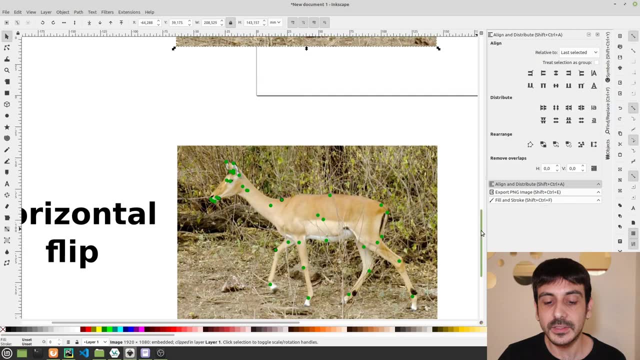 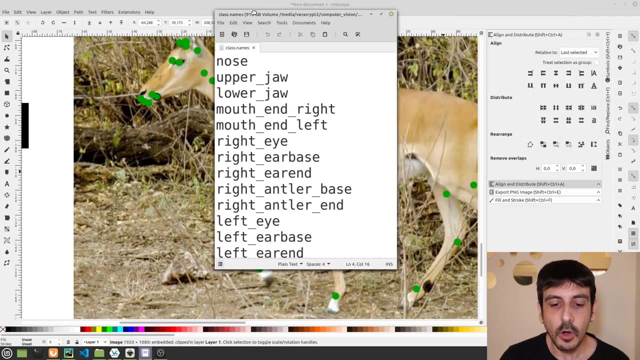 right, so we are going to be flipping some of our images at random and when, every time, we are going to be doing an horizontal flip, we are going to have a situation like this. so now let's go back to the like, to this list, which is the list of all the different key points that are related to this. 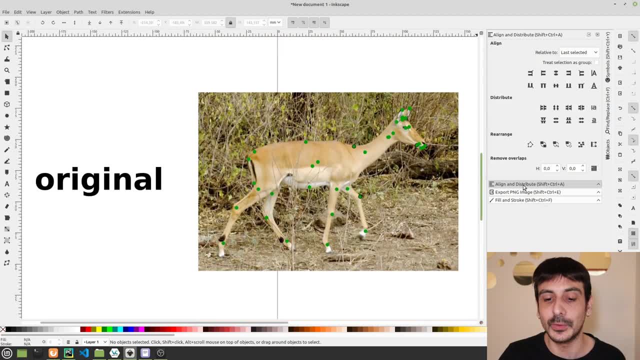 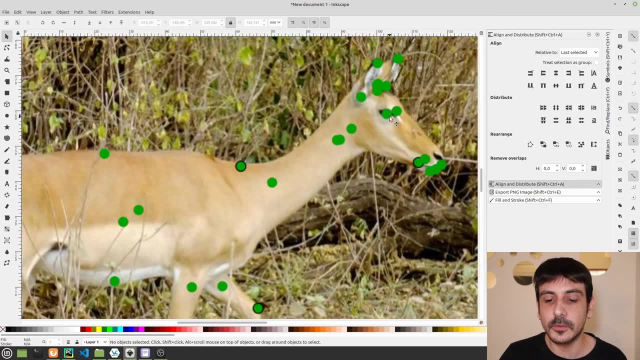 that's only what happens when you are flipping an image horizontally. but remember, we have many, many different key points and many of these key points were related to one of the sides. for example, we had a key point for the right eye. we also had key points for the right ear. we had key 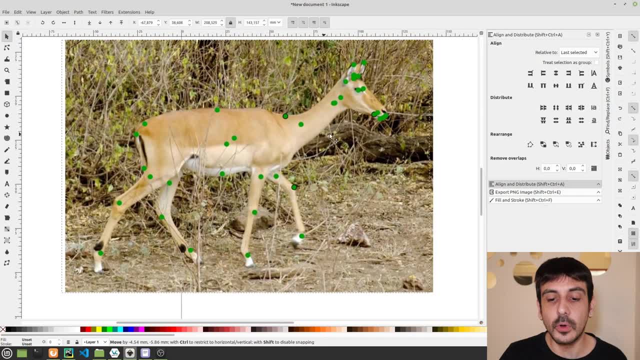 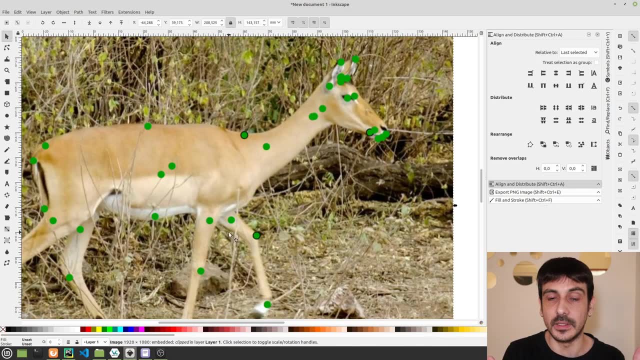 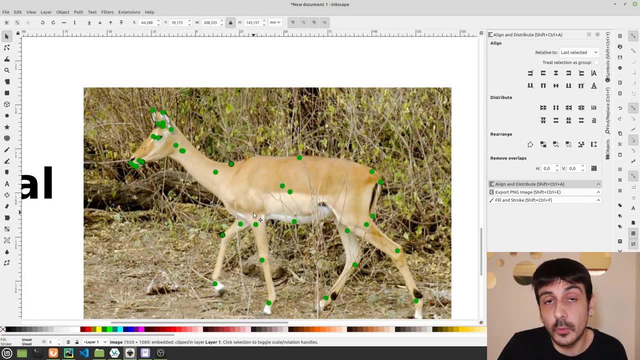 points for the right legs and the same situation for the left eye, the left ear and the left legs. many of our key points are related to one of the sides. if we flip the image horizontally, then we should be doing something with all of these key points which are related to one of the sides. 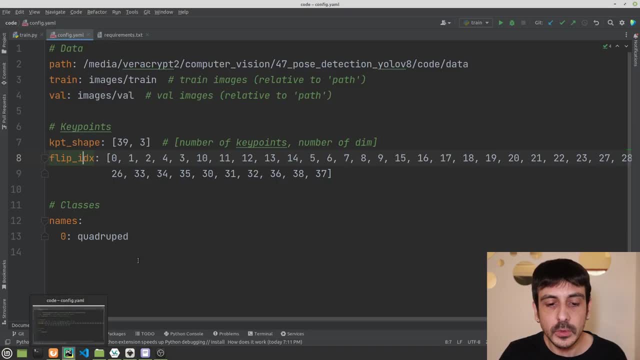 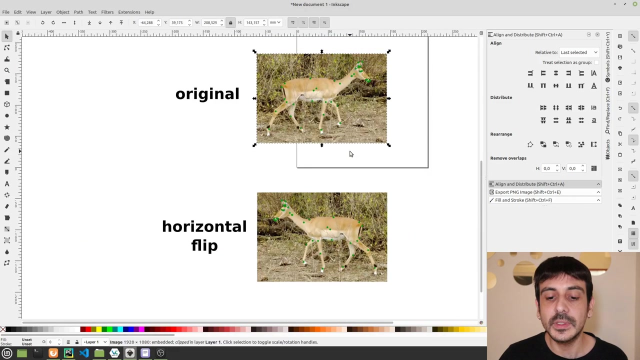 right when we are training a model using yolo v8, when we are training this type of model, one of the steps, one of the stages in this process, in the training process, is to do something which is called data augmentation. and this data augmentation means that we are taking the data and we are doing different transformations with 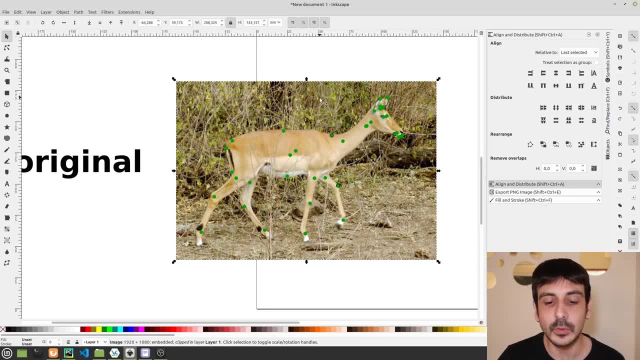 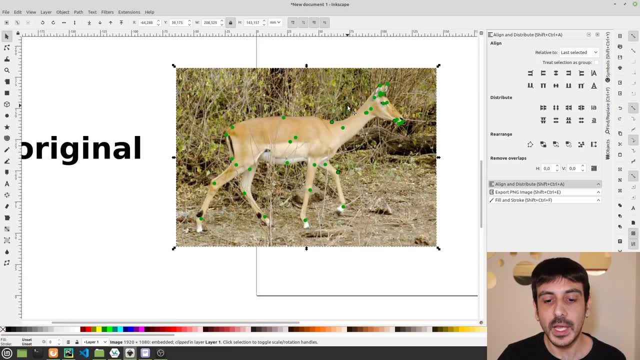 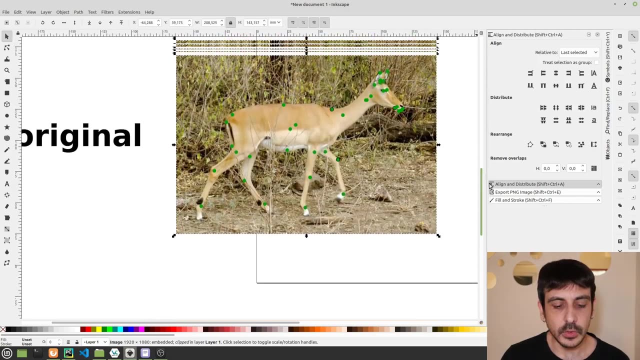 this data. one of the transformations we are doing is related to flipping the image right. so we are going to be flipping some of our images at random and when, every time, we are going to be doing an horizontal flip, we are going to have a situation like this: 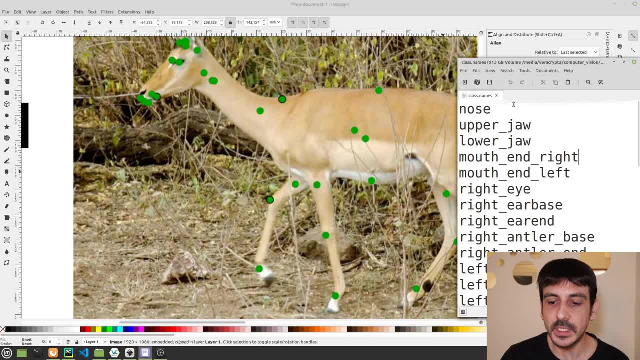 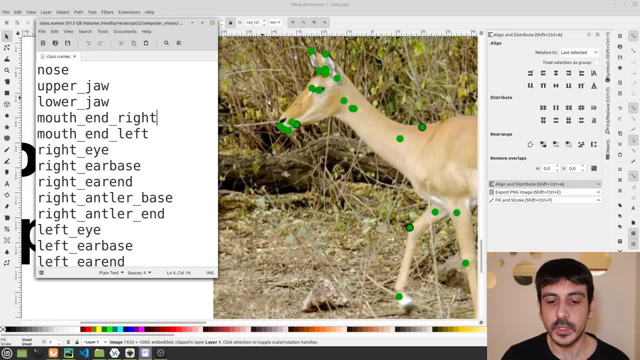 so now let's go back to the like, to this list, which is the list of all the different key points we have in this data set. right, remember i already showed you this list when i was annotating this image, and remember we start with the nose, then the upper draw, then the lower draw, and so on. 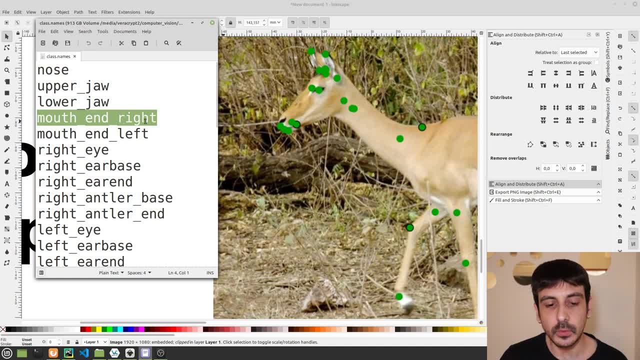 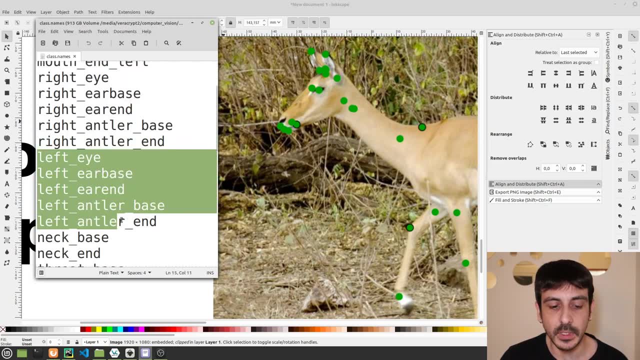 so you can see that some of these key points are related, for example, in this case, to to the right side. this is related to the left side. we have many key points over here which are related to the right side. then we have many key points which are related to the left side. then we have 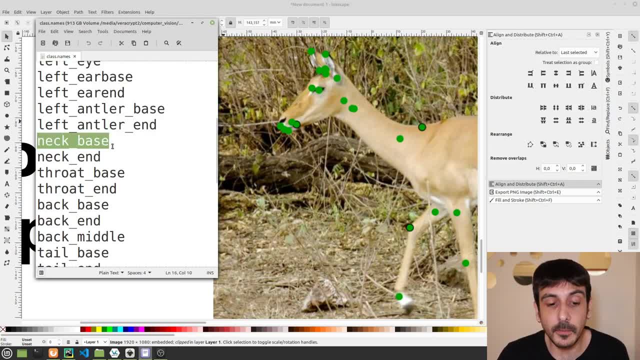 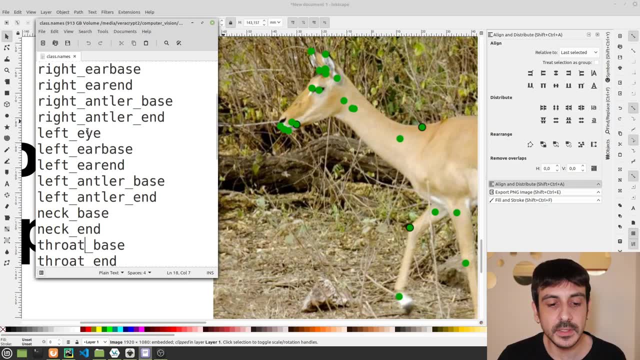 all key points which are not related to any of the sides, for example, neck base, neck end, throat back. these are generic key points and they are not related to any of the sides, and we will need to do something with all the key points which are related to one of the sides for 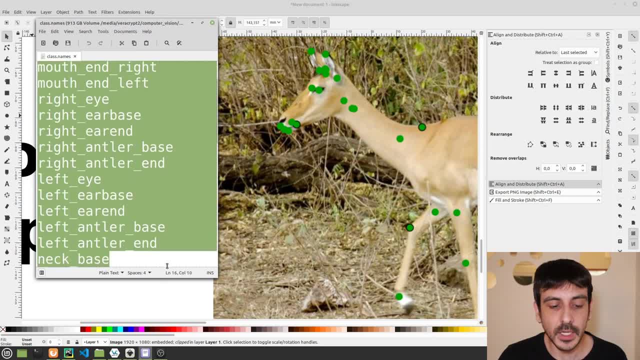 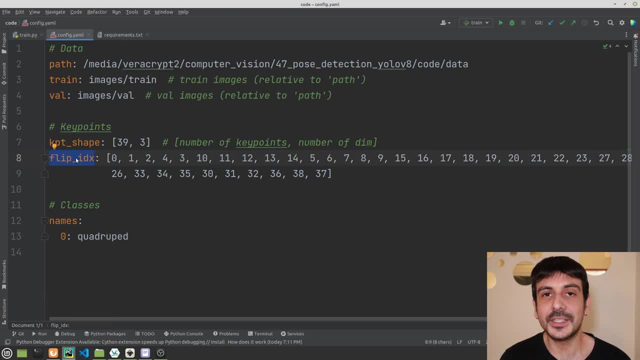 example, these two, then all of these over here and so on. right, you get the idea. that's exactly what we need to do and that's exactly what this flip index keyword does. right, that's exactly the idea, the intuition behind this flip index. so let's go through this list. you can see that the first 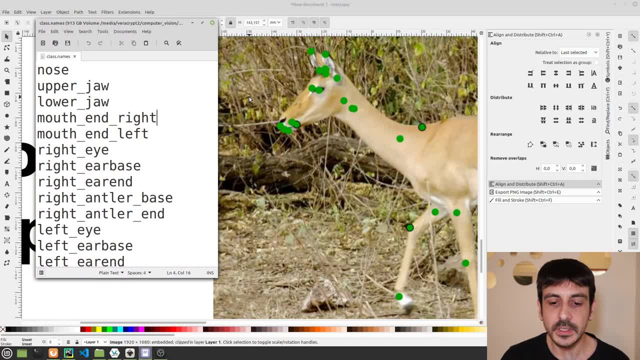 data set right. remember i already showed you this list when i was annotating this image, and remember we start with the nose, then the upper draw, then the lower draw and so on. so you can see that some of these key points are related, for example, in this case to to the 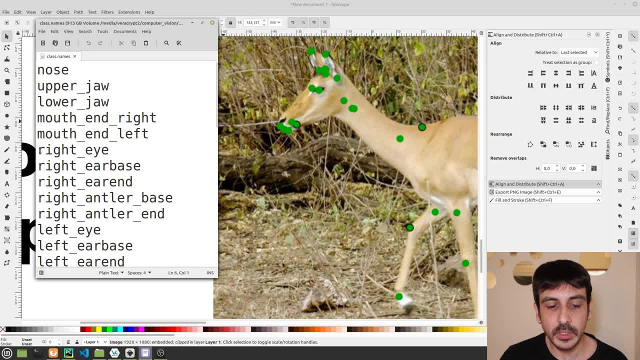 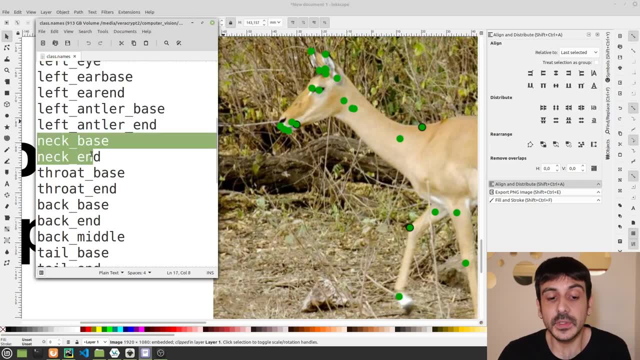 right side. this is related to the left side. we have many key points over here which are related to the right side. then we have many key points which are related to the left side. then we have all key points which are not related to any of the sides, for example, neck base, neck end throat. 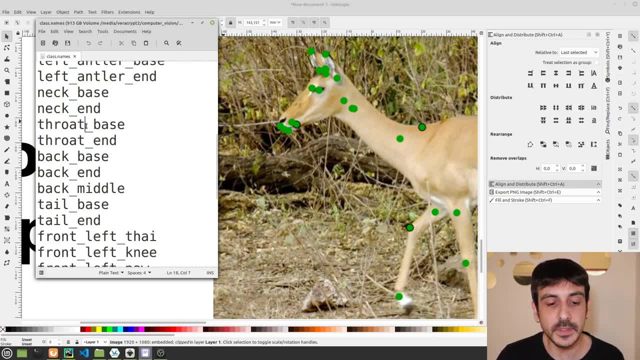 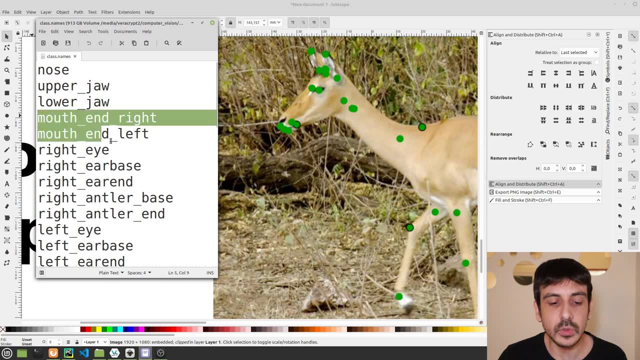 neck. these are generic key points and they are not related to any of the sides, and we will need to do something with all the key points which are related to one of the sides, for example, these two, then all of these over here and so on. right, you get the idea. that's exactly what we need to do. 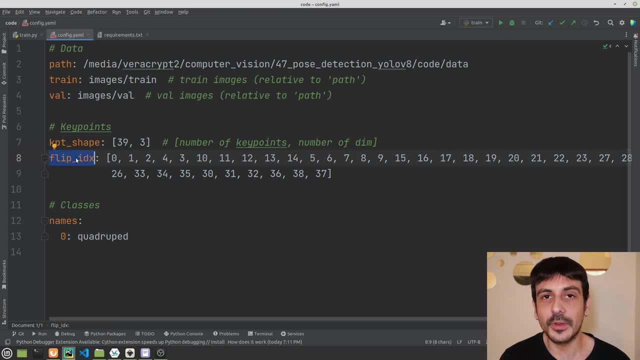 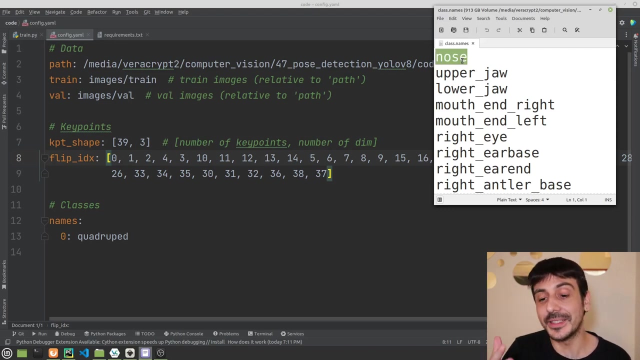 and that's exactly what this flip index keyword does. right, that's exactly the idea, the intuition behind this flip index. so let's go through this list. you can see that the first index element is nose. and if we think about a nose, it's straight in the middle and nothing is going to. 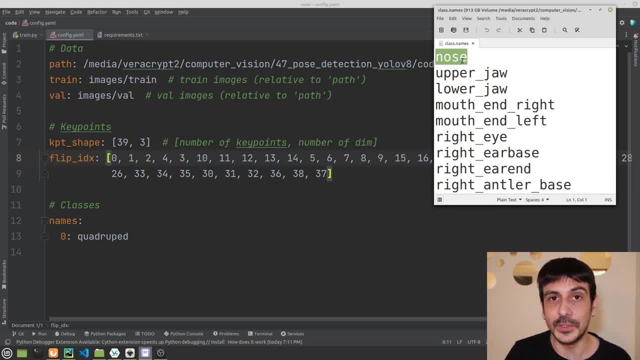 happen when we flip the image right: the nose will continue being the nose, will remain as the nose. and then the next element is the upper draw. exactly the same, nothing will happen with the upper draw will remain being the upper row. after we flip the image horizontally, the same will. 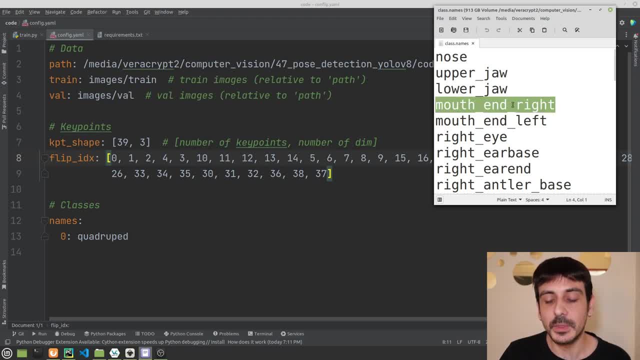 happen with the lower draw. but when we get to this element, this is the mount and right, and we will flip the image horizontally, because the mouse and right, when we flip the image horizontally, will be the mouth and left. and the next element, which is mount and left when we flip the image. 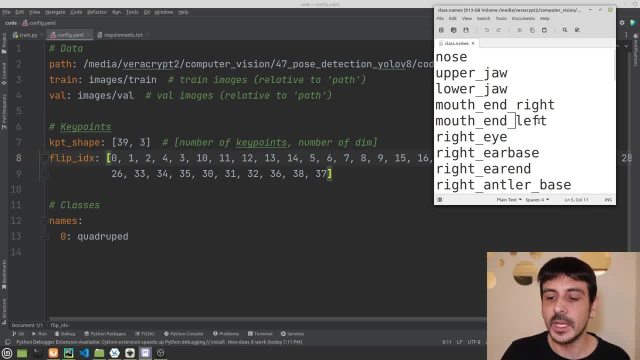 horizontally. now it will be the mount and right. you get the idea. these two values, these two key points, will be flipped when we flip our image right. and now let's take a look at this list we have over here, which is the value for flip index. so we are flipping these two values right, instead of having a three, four, which will be like the. 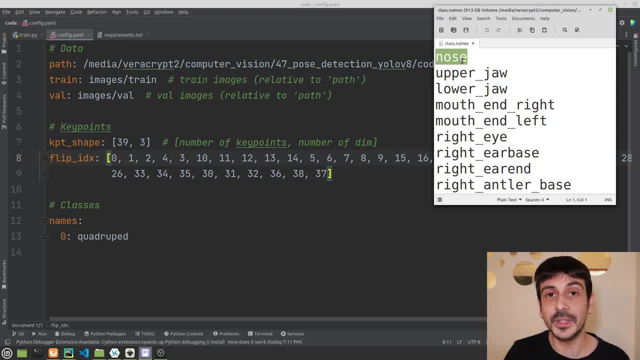 element is nose, and if we think about a nose, it's straight the middle, and nothing is going to happen when we flip the image right. the nose will continue being the nose, will remain as the nose. and then the next element is the upper draw. exactly the same. nothing will happen with the 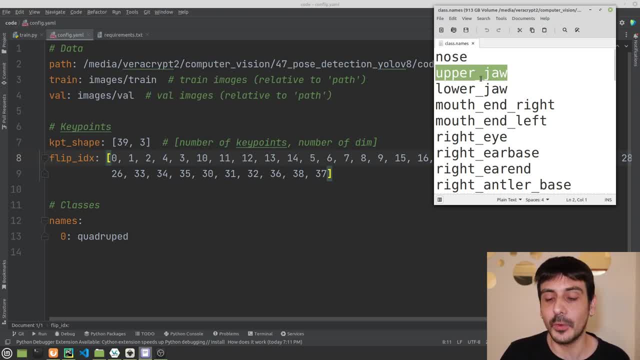 upper draw will remain being the upper row after we flip the image horizontally. the same will happen with the lower draw, but when we get to this element, this is the mount end right, and we will have an issue here here, because the mount end right when we flip the image horizontally. 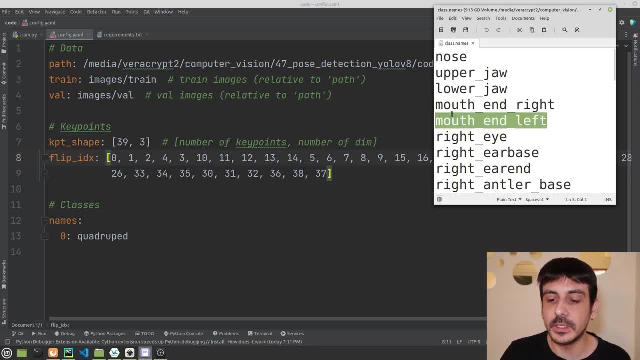 will be the mount end left. And the next element, which is mount end left, when we flip the image horizontally now, it will be the mount end right. You get the idea. These two values, these two key points, will be flipped when we flip our image right. 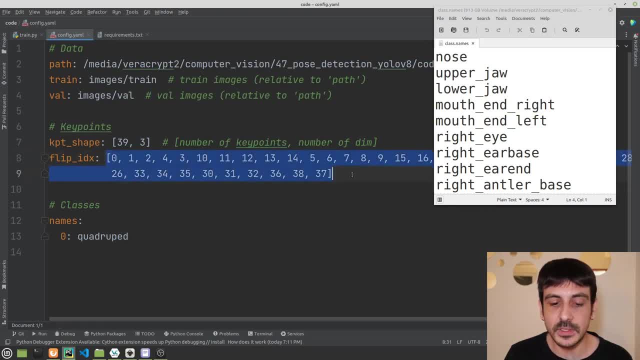 And now let's take a look at this list we have over here, which is the value for flip index, And you can see that the first element is zero, then one, then two, then four, three, right? So we are flipping these two values, right? 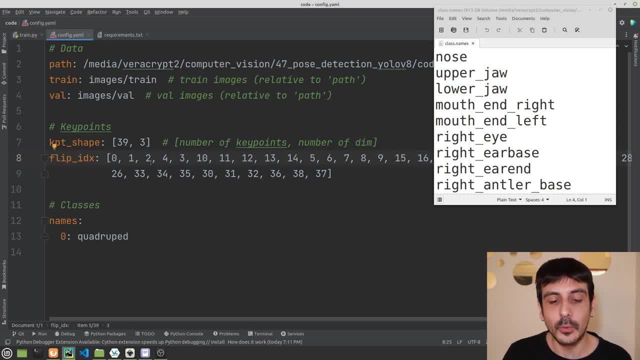 Instead of having a three- four, which will be like the natural order, we have a four- three. we are flipping these two values And these are exactly the indexes of these two key points in the key point order. So, long story short, the only thing we will need to do. 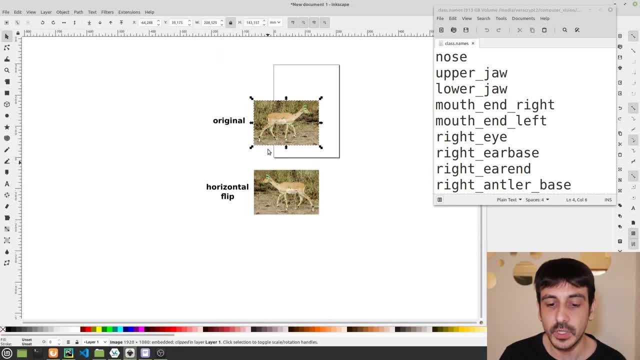 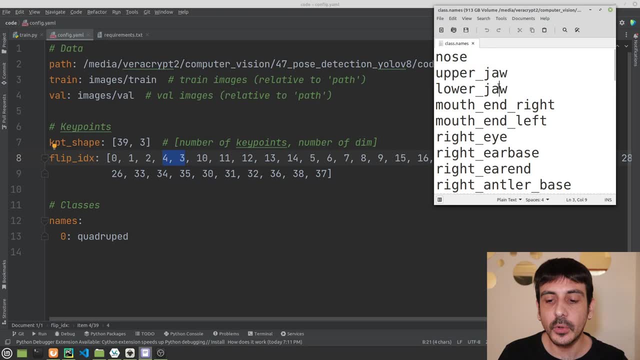 in order to fix this issue we will have when we are flipping our images horizontally. the only thing we will need to do is going through all of our key points, and all of the key points which are related to the right side. we need to flip them in order to make them the left side. 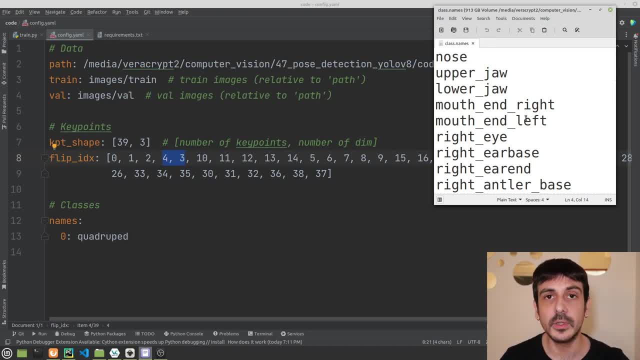 right. We only need to flip the right and the left side. That's the only thing we need to do And that's what we need to specify here in this list. This is how the flipping will be done, So please be super, super careful with this list. And this, remember, is a very important part of this list. So please be super, super careful with this list, And this, remember, is a very important part of this list, And this, remember, is a very important part of this list. 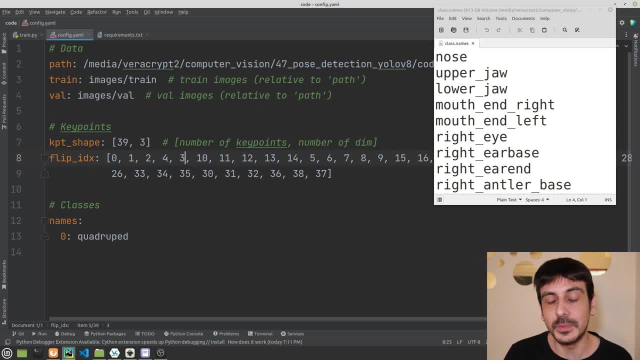 natural order. we have a four three. we are flipping these two values and these are exactly the indexes of these two key points in the key point order. so, long story short, the only thing we will need to do in order to fix this issue we will have when we are flipping these two values is to flip the image. 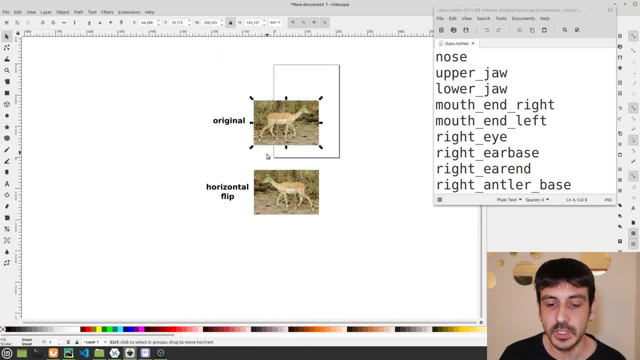 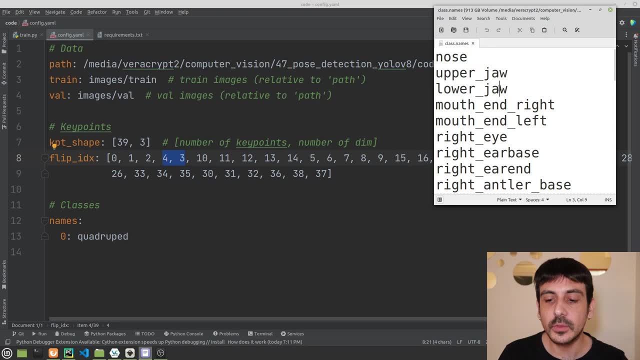 horizontally. so we are flipping these two key points in the key point order. so we are flipping these two values in the key point order and we are flipping the image horizontally. the only thing we will need to do is going through all of our key points and all of the key points. 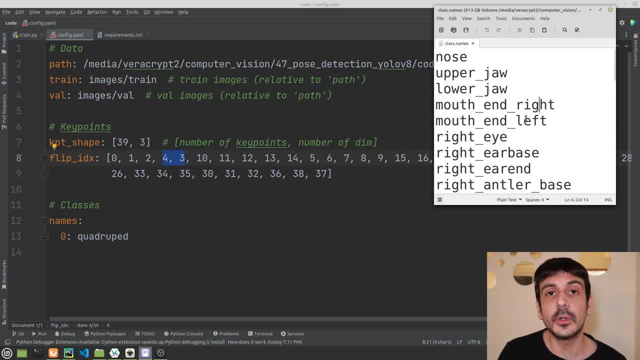 which are related to the right side. we need to flip them in order to make them the left side right. we only need to flip the right and the left side. that's the only thing we need to do and that's what we need to specify here in this list. this is how the flipping 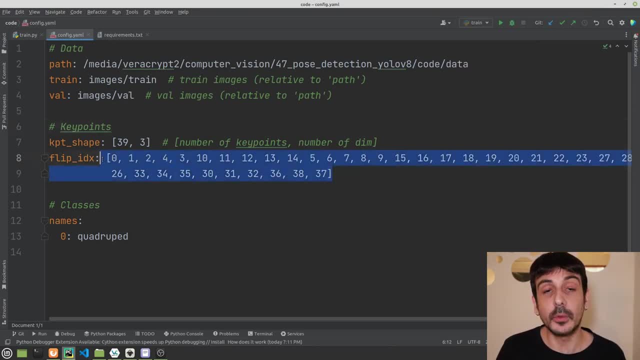 will be done. so please be super, super careful with this list. and this, remember, means how your indexes will be flipped when the image is flipped horizontally. now let's move to this section, and these are all of your names, of all of your objects. in my case, i only have one object, which is 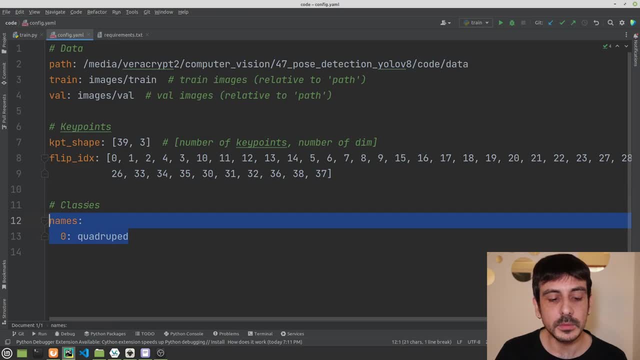 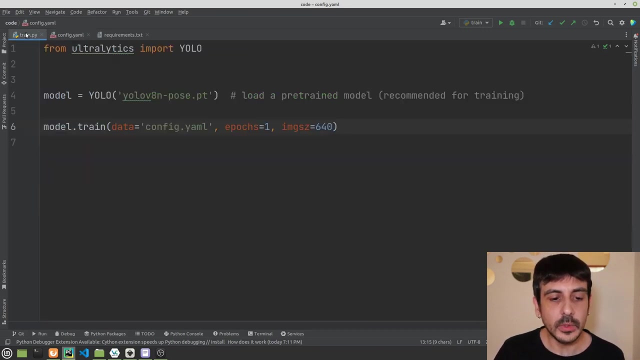 quadruped. so in my case, this is very simple, but please remember to specify all the names and all the class ids for absolutely all of your names. in my case, i only have one class id, which is zero and means quadruped. so that's pretty much all for the configyaml, and now we let's go back to. 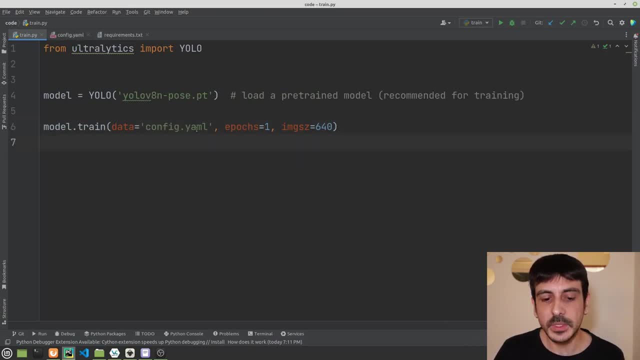 trainpi, and let's continue. so once you have specified this configuration file and you have specified everything we have over here, the only thing you need to do is to execute this script and that's all. that's how easy it is to train this model, but i'm going to stop this training. 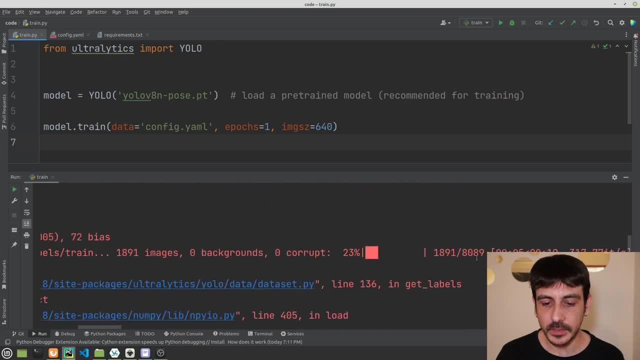 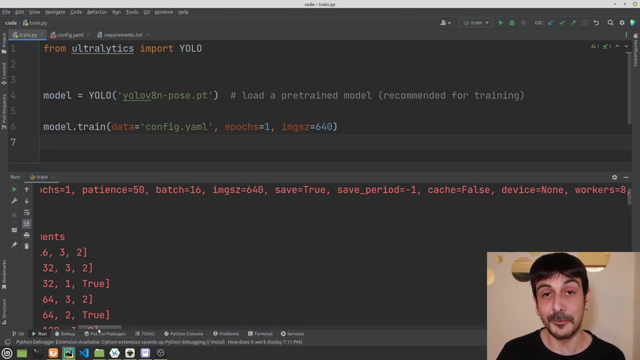 because otherwise it's going to take a lot of time. if i train this model locally, it's going to train. it's going to take a lot of time. i have been doing some tests already and, yeah, it's going to take forever if i do it locally, but this is exactly the process you 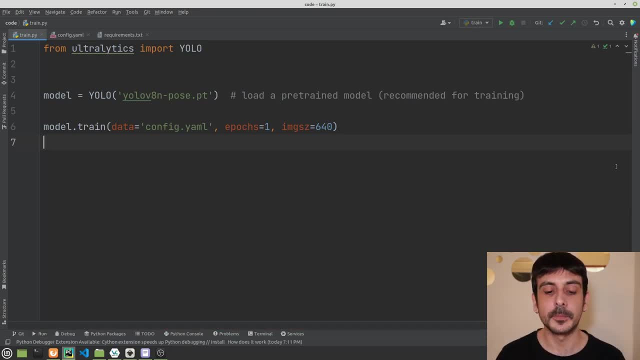 should follow if you want to train this model in your local environment. but i mentioned that i'm also going to show you how to train it in a google collab. so now let's go to my browser and let's see exactly how we can do this training from a google collab. the first thing you will need to do is go. 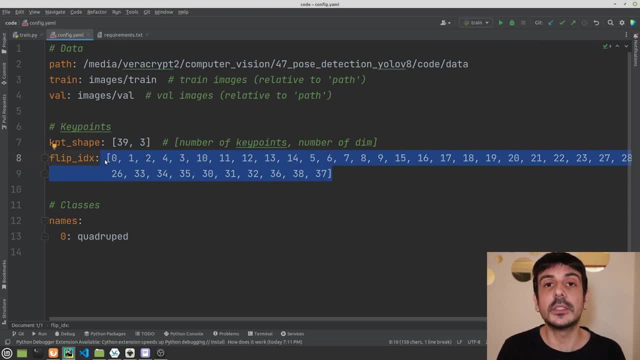 How you'll be flipping your indexes when the image is flipped horizontally. Now let's move to this section, and these are all of your names, of all of your objects. In my case, I only have one object, which is quadruple. 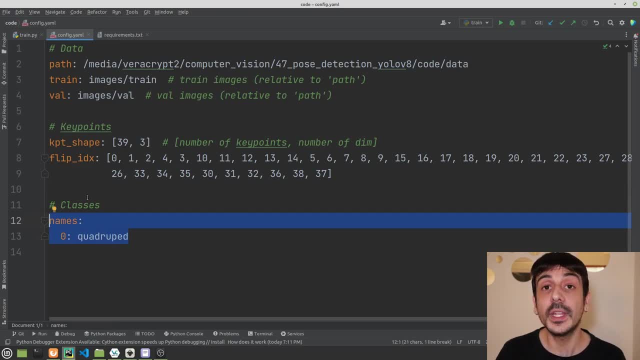 So in my case this is very simple, but please remember to specify all the names and all the class ID for absolutely all of your names. In my case, I only have one class ID, which is zero and means quadruple. So that's pretty much all for the configyaml things. 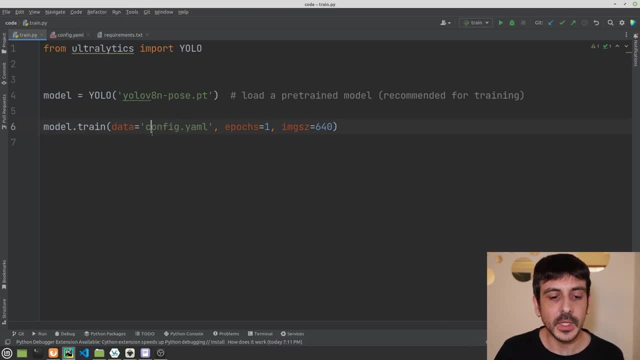 and now we let's go back to trainpi and let's continue. so once you have specified this configuration file and you have specified everything we have over here, the only thing you need to do is to execute this script and that's all. that's how easy it is to train this. 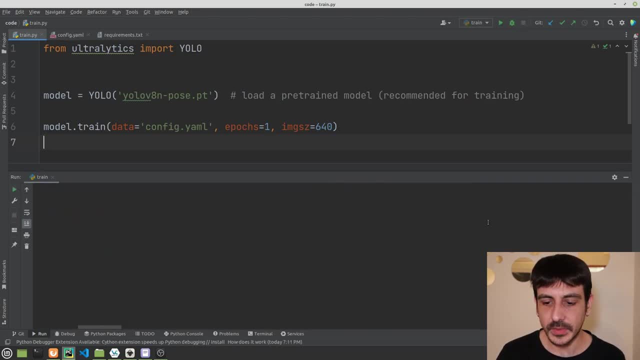 model, but i'm going to stop this training because otherwise it's going to take a lot of time. if i train this model locally, it's going to train. it's going to take a lot of time. i have been doing some tests already and, yeah, it's going to take forever if i do it locally, but this is exactly the process. 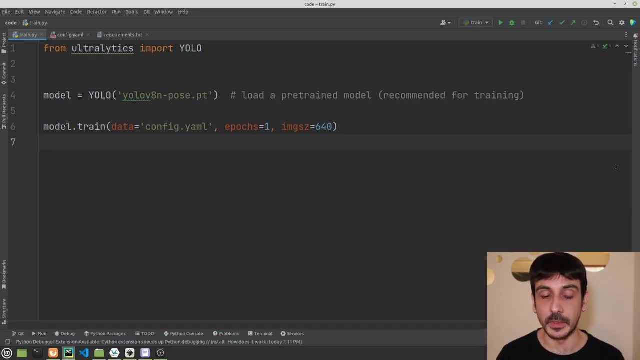 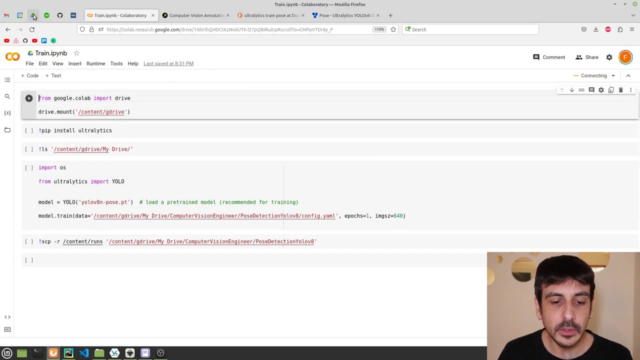 you should follow if you want to train this model in your local environment. but i mentioned that i'm also going to show you how to train it in a google collab. so now let's go to my browser and let's see exactly how we can do this training from a google collab. the first thing you will need to do is 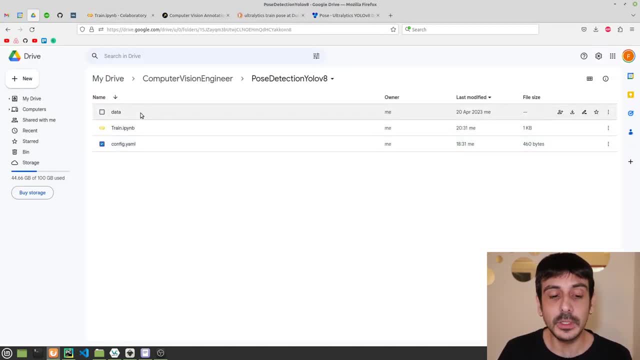 going to your google drive and you will need to upload absolutely all of your data, obviously, because otherwise you will not be able to do it- train this model from your google drive- and also you will need to upload your configyam file and everything will be just exactly the same as the file i showed you in my local computer. 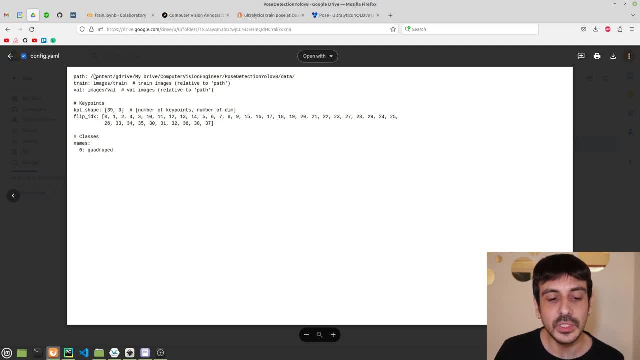 but you will need to edit this field, which is the path right. you can see this path over here. you will need to edit this with the path to your data in google drive. this is very important and otherwise nothing is going to work. so, please remember, you need to edit this path and 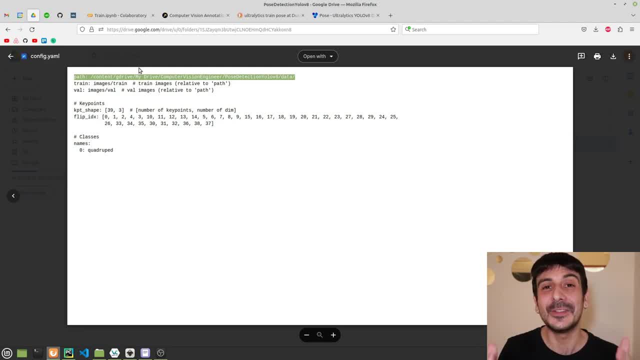 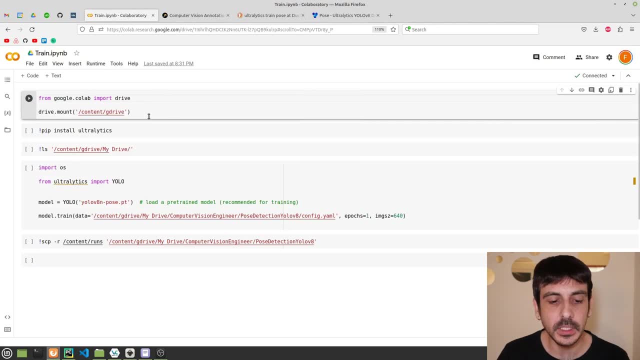 i'm going to show you exactly how to know what's the location of your data in your google drive. now let's go back to this google collab. this is the google call that i created for this tutorial, for this training, and obviously you will be able to find this notebook in the github. 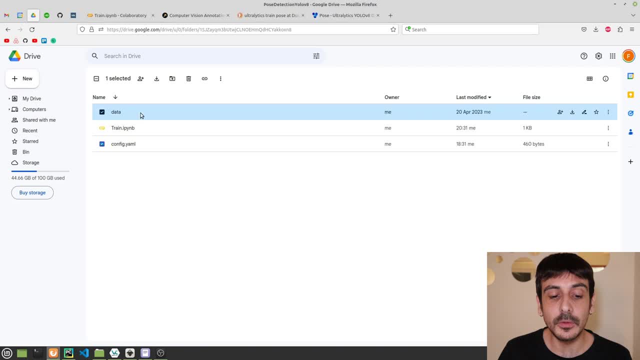 into your google drive and you will need to upload absolutely all of your data, obviously, because otherwise you will not be able to train this model from your Google Drive, and also you will need to upload your configyam file, and everything will be just exactly the same as the. 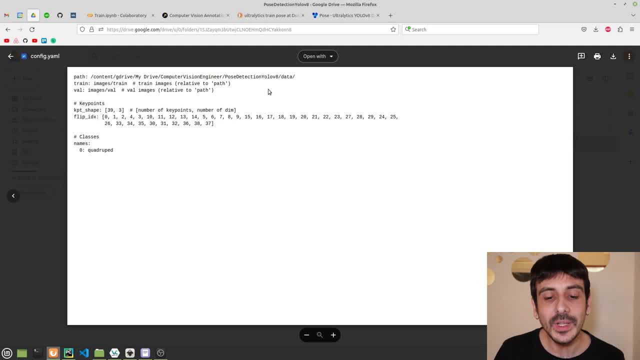 file I show you in my local computer, but you will need to edit this field, which is the path right. you can see this path over here. you will need to edit this with the path to your data in Google Drive. this is very important and otherwise if nothing is going to work. so please remember, you need to edit this. 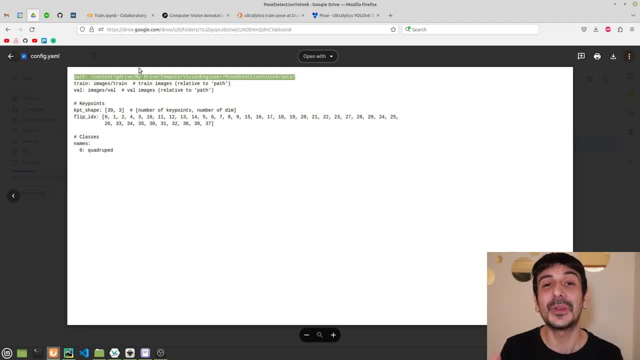 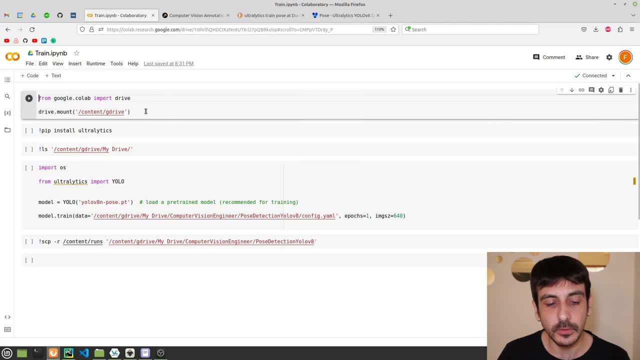 path and I'm going to show you exactly how to know what's the location of your data in your Google Drive. now let's go back to this Google Colab. this is the Google Colab I created for this tutorial, for this training, and obviously you will. 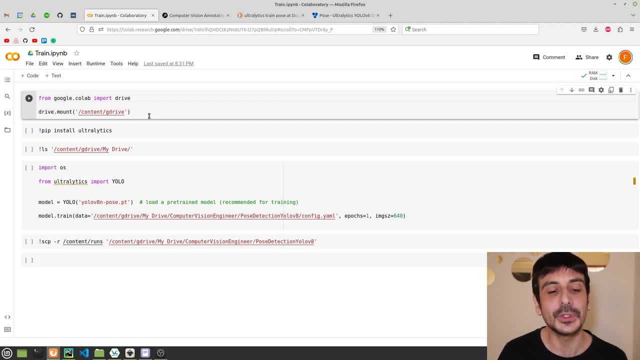 be able to find this notebook in the github repository of today's tutorial. so for now, just follow along. you can see that this: we have only a few cells, and the only thing I'm going to do is to execute these cells one by another, and I'm going to show you how to do that in this tutorial. so for now, 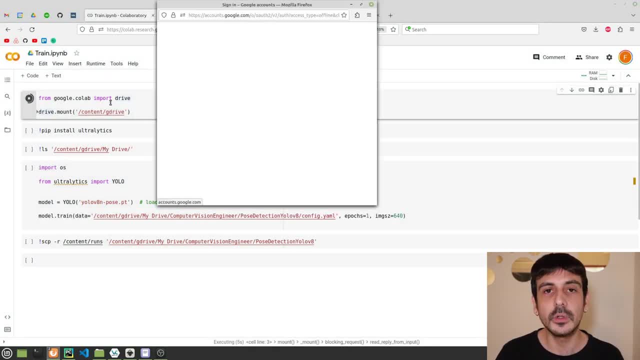 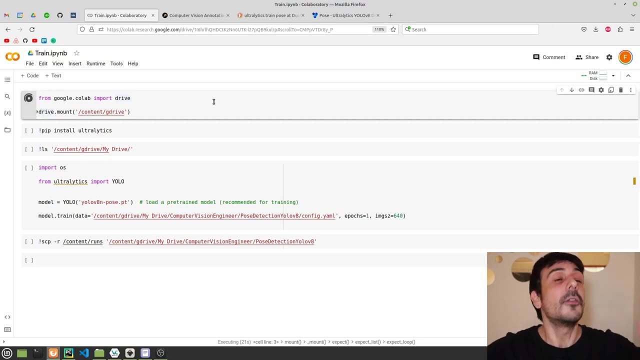 I'm going to start with the first one, which is connecting my Google Colab environment with Google Drive. and now the only thing I have to do is to select my account, then I scroll all the way down and I click allow, and that's basically all we need to do in order to connect or Google Colab with Google Drive. 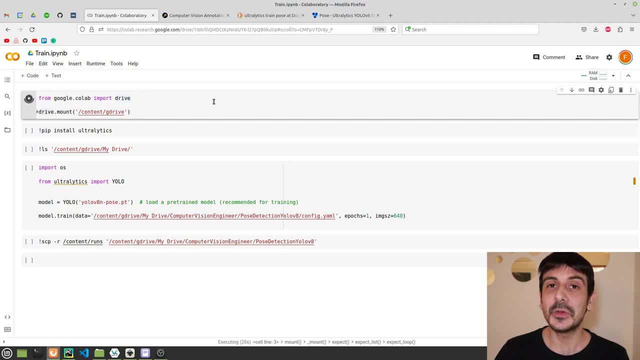 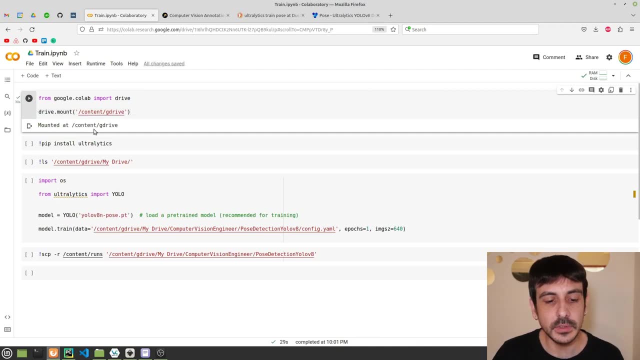 so this way, Google Colab will be able to access the data you have in your Google Drive. we have to wait a few seconds and that's pretty much all. you can see that everything has been mount here in content G Drive, and now the next step is to install ultra or analytics. right, because 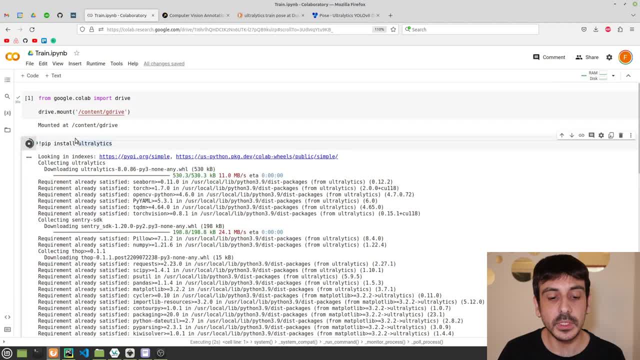 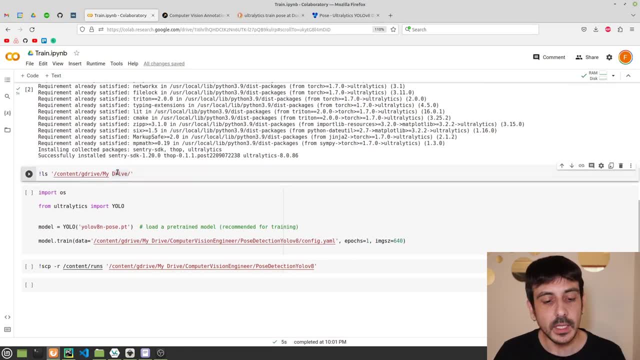 remember we are going to use, or at least with- is the Python package we need to use in order to use yellow 8, and the only thing we need to do is to execute this cell, and everything is now completed. now, in order to continue with the next two cells, you need to know where your data is located in your 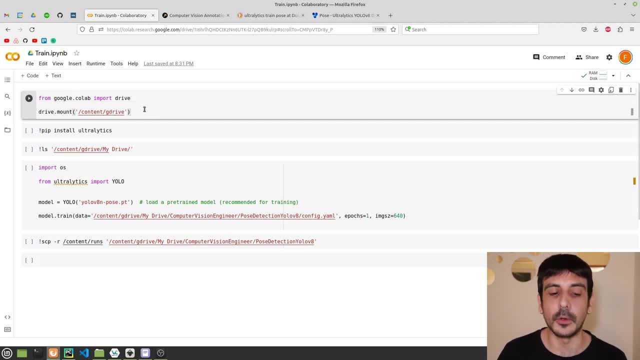 repository of today's tutorial. so for now, just follow along. you can see that this: we have only a few cells, and the only thing i'm going to do is to execute these cells one by one. so i'm going to start with the first one, which is connecting my google collab environment to my google drive, and 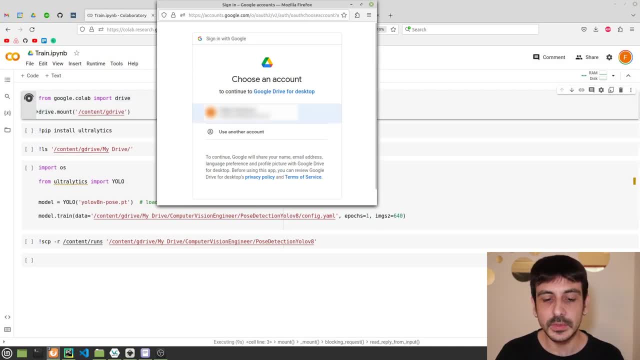 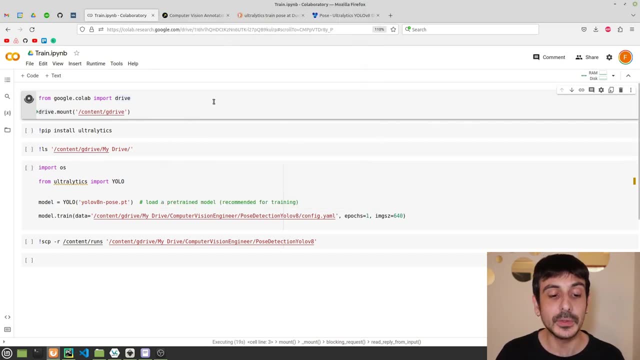 now the only thing i have to do is to select my account, then i scroll all the way down and i click allow, and that's basically all we need to do in order to connect, or google collab with google drive. so this way, google collab will be able to access the data you have in your google drive. 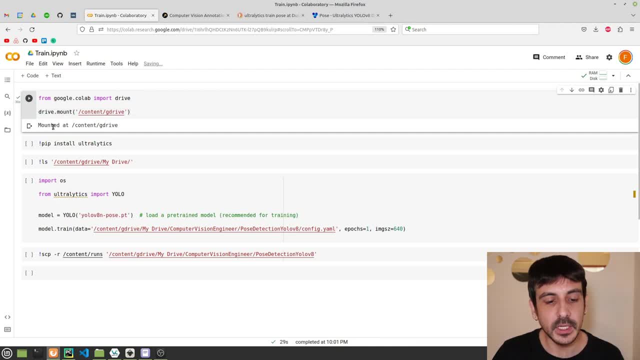 we have to wait a few seconds and that's pretty much all. you can see that everything has been mount here in content g drive and now the next step is to install ultralytics. right, because, remember, we are going to use ultralytics, which is the python package we need to use in order to use 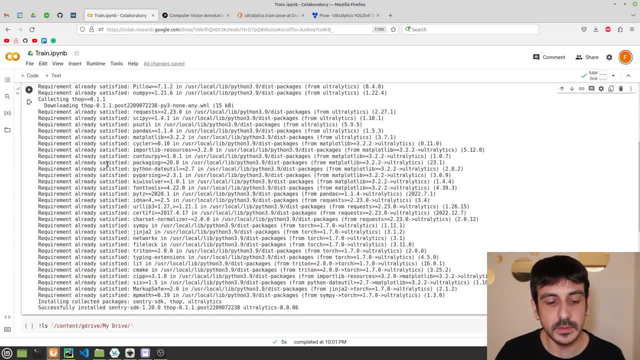 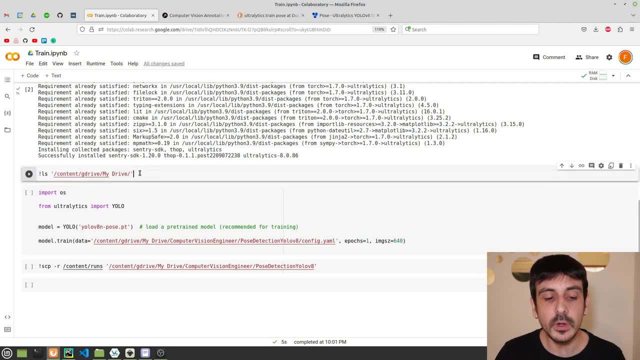 yellow v8, and the only thing we need to do is to execute this cell, and everything is now completed. now, in order to continue with the next two cells, you need to know where your data is located in your google drive. the only thing i'm going to do is to execute this cell, and this is going to list. 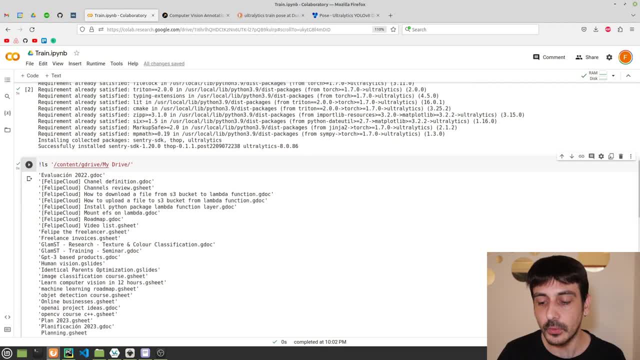 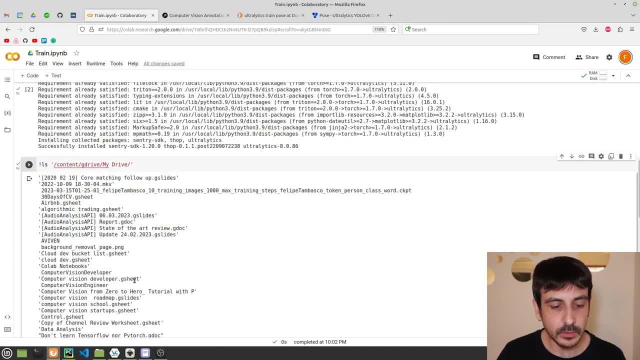 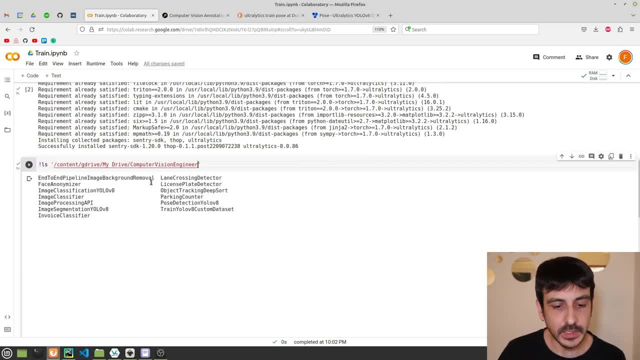 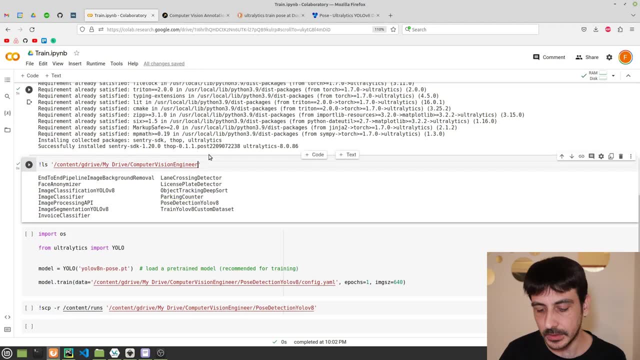 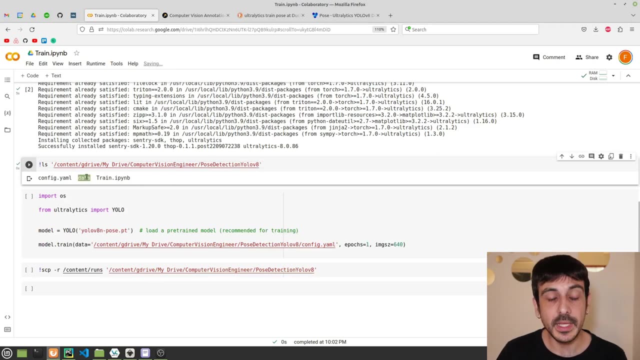 my case, it's located in this folder. if i do ls again, this is the content of this folder, so the only thing i need to do is to locate this directory and then that's it right, this is the content of this directory, which is where my data is located, so the only thing i need to do is 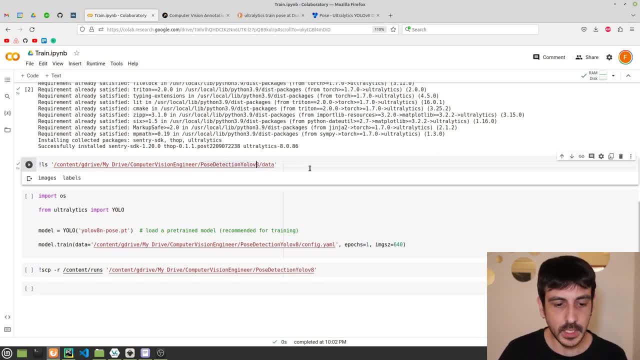 something like this. and that's the. that's the content of my data directory, which contains the two folders, images and labels. now that you know where your data is located in your google drive, now you can just copy and paste this um, this path, in your config file right now that you know exactly where your data. 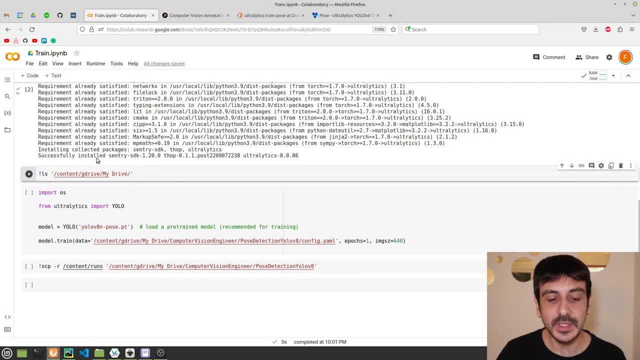 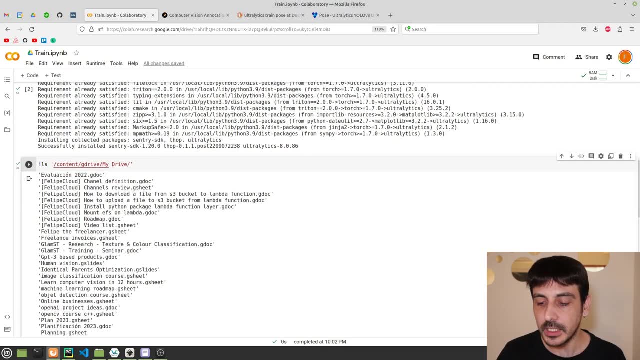 Google Drive. the only thing I'm going to do is to execute this cell and this is going to list absolutely all the files in my local GoogleNaziscom, in my google drive and in my root directory right. you can see that these are many, many, many files. 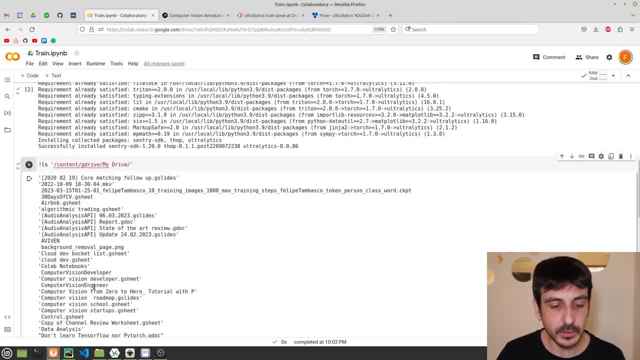 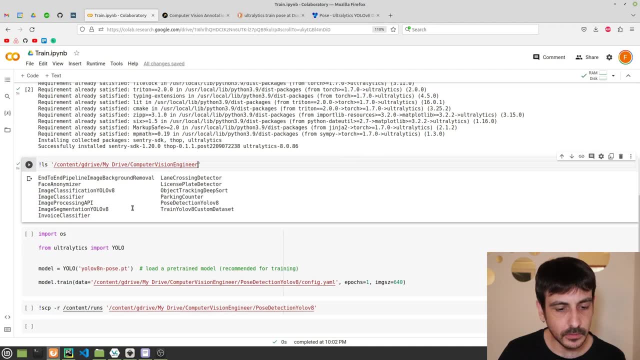 and from here, the only thing i will need to do is to find where my data is located. in my case, it's located in this folder. if i do ls again, this is the content of this folder. so the only thing i need to do is to locate this directory and then that's it right? this is the content of this. 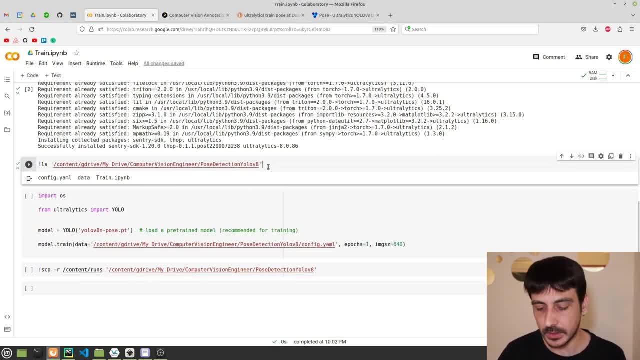 directory, which is where my data is located. so the only thing i need to do is something like this: and that's that's the content of my data directory, which contains the two folders, images and labels. now that you know where your data is located in your google drive. 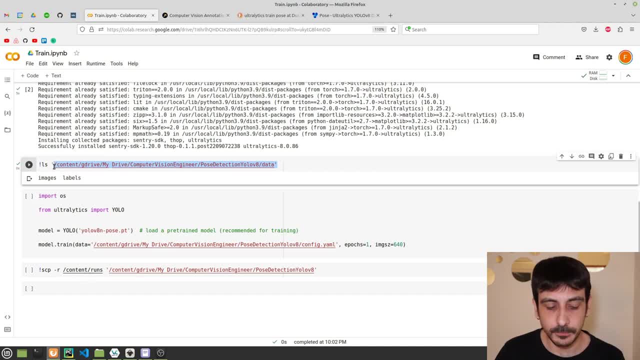 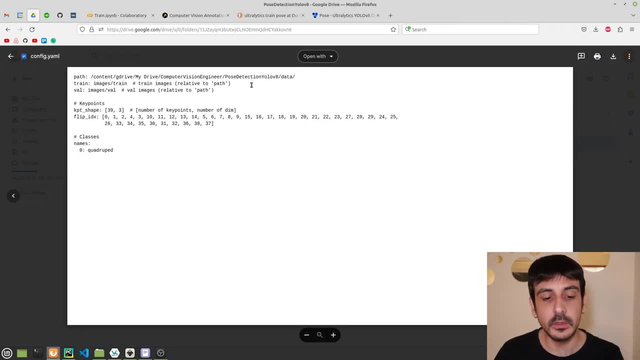 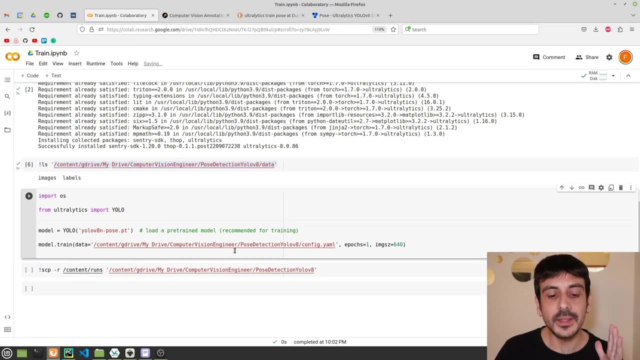 now you can just copy and paste this um, this path, in your config file. right now that you know exactly where your data is located, you can just come here and you can edit, you can edit, you can edit this field and you can just put wherever your data is located, and then you need to specify the. 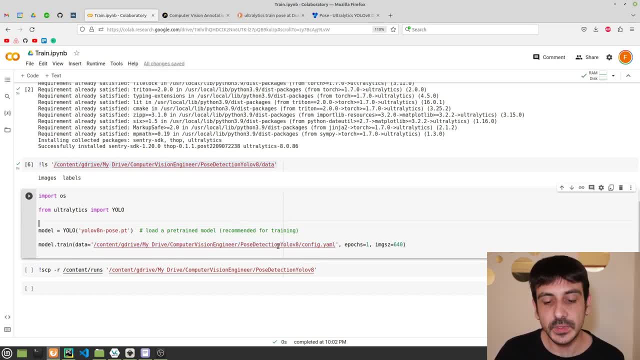 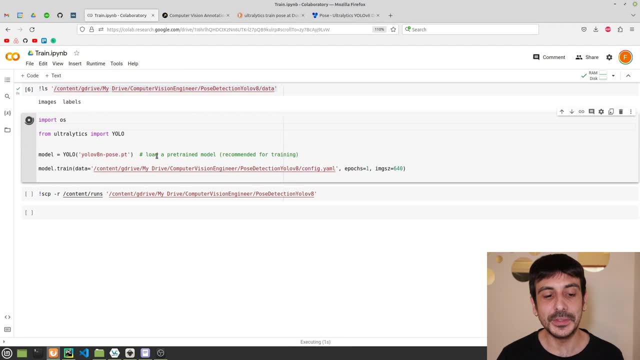 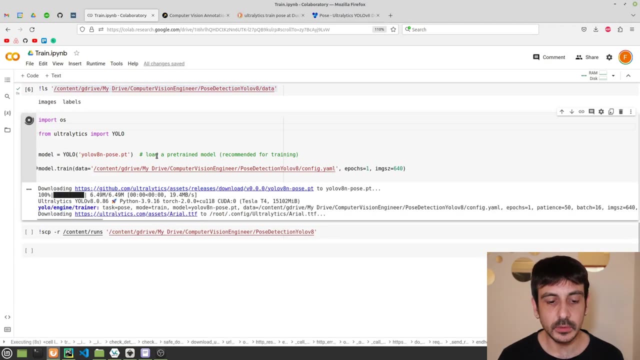 location of your configyaml file, and once you set this location over here, you are all set and the only thing you need to do is to click enter. right, you need to execute this cell, and that's going to be pretty much all now. everything is being executed. this is going to take some time. everything is 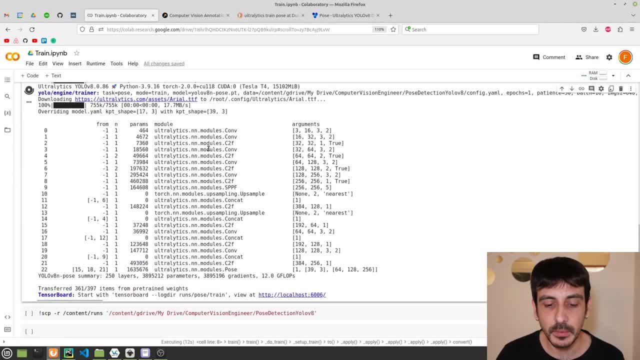 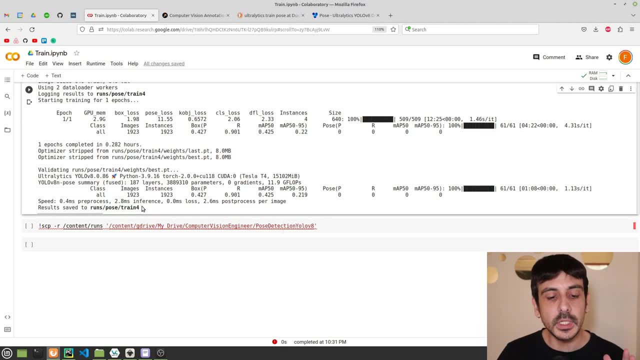 going to do is to download all the weights into this google call up environment and that's pretty much all. it's going to get all the data and then it's going to do the training. okay, now the training process has been completed and you can see that the results have been saved here. runs post train. 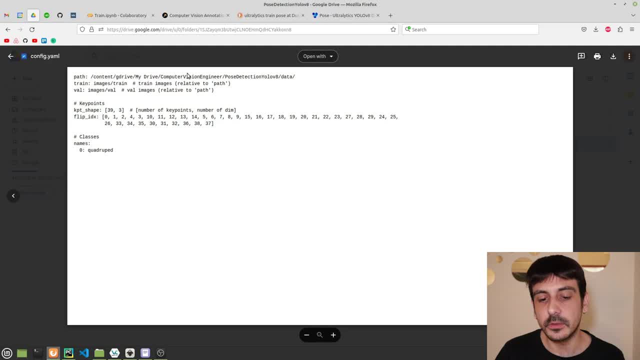 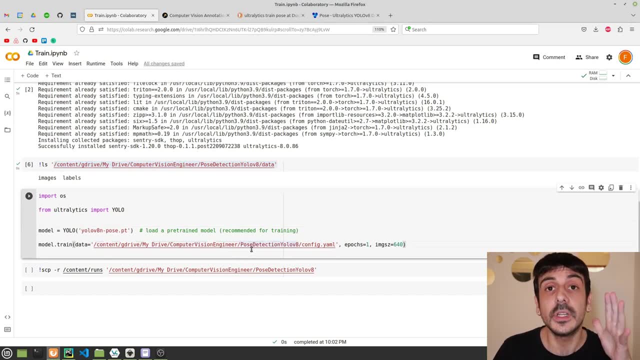 is located. you can just come here and you can edit this field and you can just put wherever your data is located, and then you need to specify the location of your config yum file and once you set this location over here, you are all set and the only thing you need to do 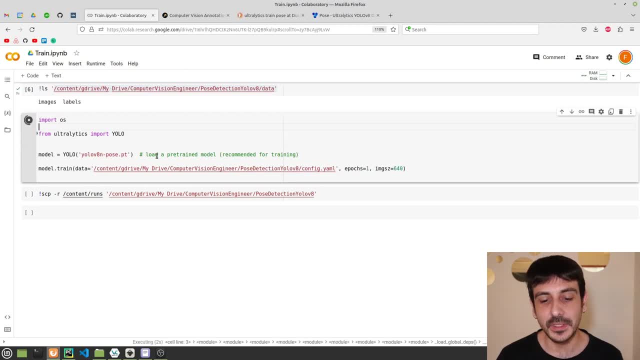 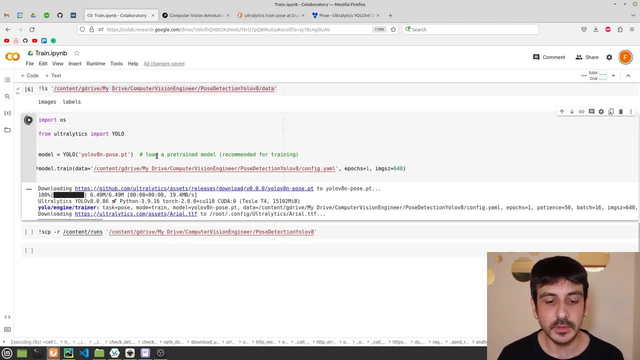 is to click enter. right, you need to execute this cell, and that's going to be pretty much all. now, everything is being executed. this is going to take some time. the first thing it's going to do is to download all the weights into this google call of environment, and that's pretty much all. 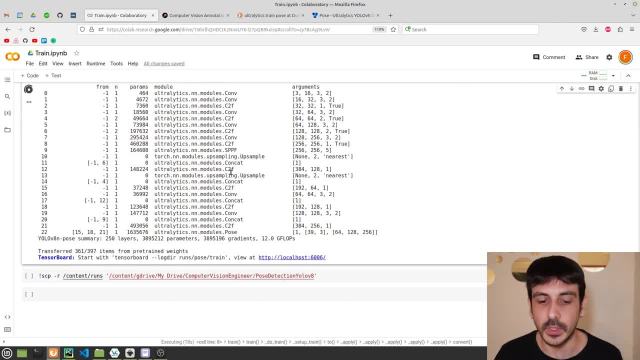 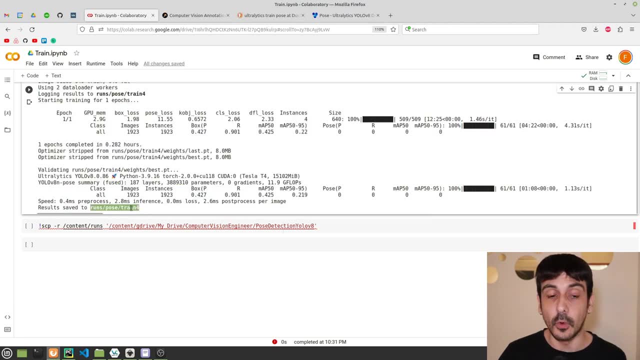 it's going to get all the data and then it's going to do the training. okay, now the training process has been completed and you can see that results have been saved here. runs post train 4.. so i'm going to show you how to execute this cell. 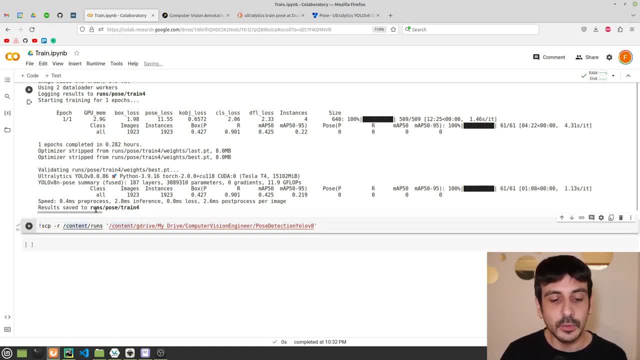 so we copy the entire content of the bronze directory into your google drive, right? remember that the idea of this training process is to download the results, to download the way to download the entire results which have been saved here and the way to do it, or one of the ways to do. 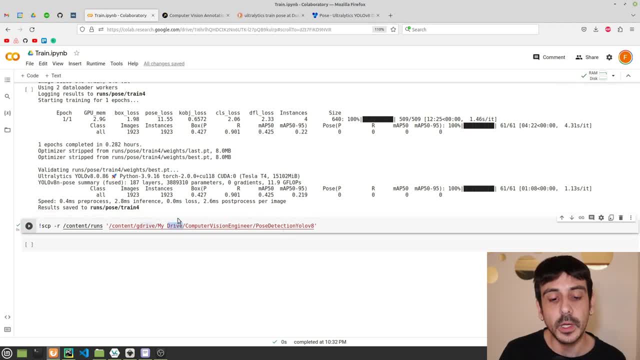 it. i would say the easiest way to do it is to copy everything into google drive and then just download everything from google drive. so this is this is the simplest way to do it, and please remember to edit this path to the path where you want everything to be copied when you execute this. 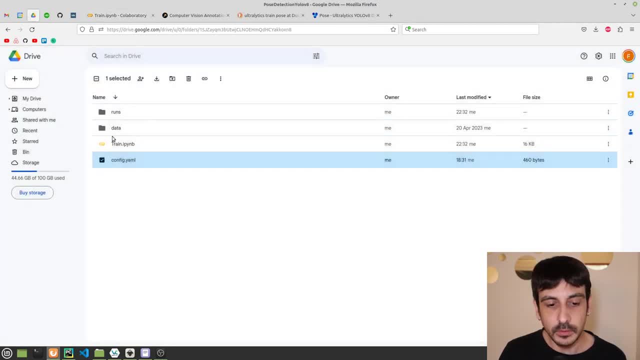 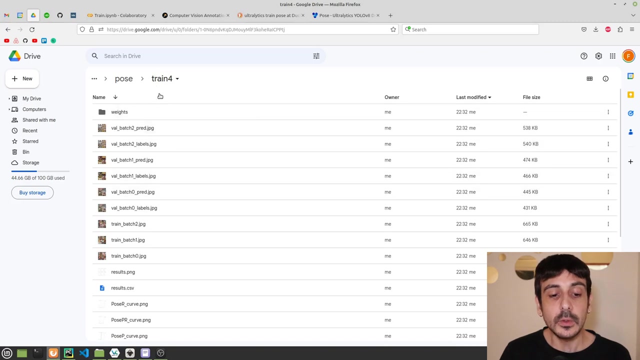 cell. so let me show you. if i go back to my google drive, you can see, this is the runs directory which was just generated, and within this directory is where we have this train 4, which is the result of the training process we have just executed. so everything seems to be okay and what we 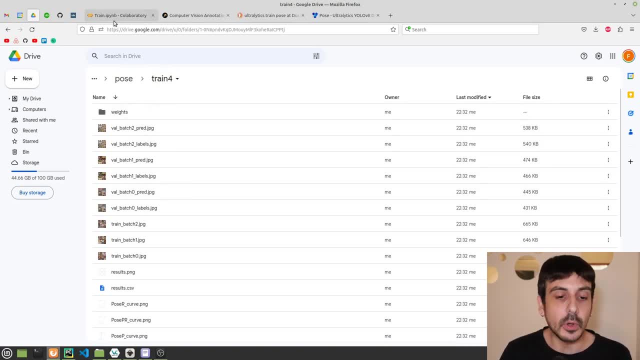 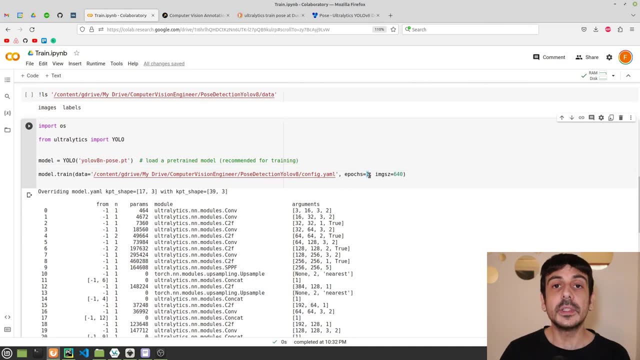 will need to do now is to download this directory into our local computer now. remember this was a very, very dummy training. this is a training we did for only one epoch. obviously you will need to do like a deeper training if you really want to train your pose. 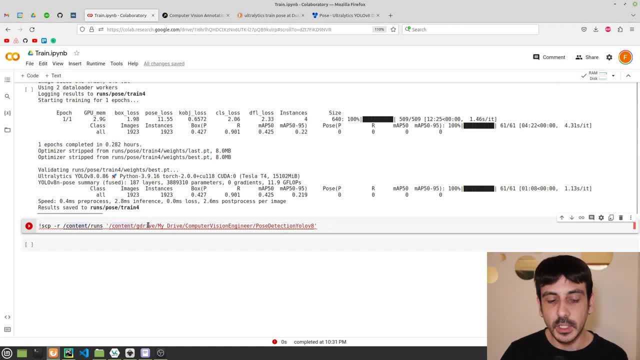 4, so i'm going to show you how to execute this cell so we copy the entire content of the runs directory into your google drive, right? remember that the idea of this training process is to download the results, to download the way to download the entire results which have been saved here and the way to do it, or? 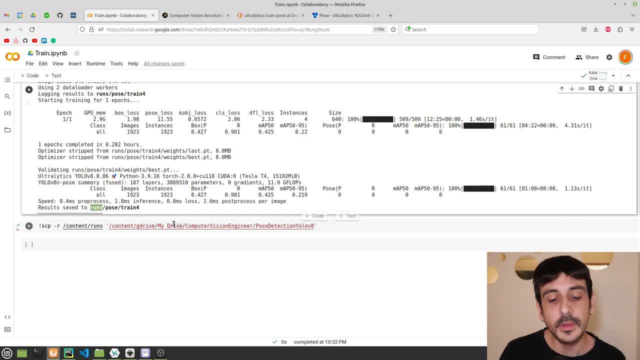 one of the ways to do it- i would say the easiest way to do it- is to copy everything into google drive and then just download everything from google drive. so this is this is the simplest way to do it, and please remember to edit this path to the path where you want everything to be copied. 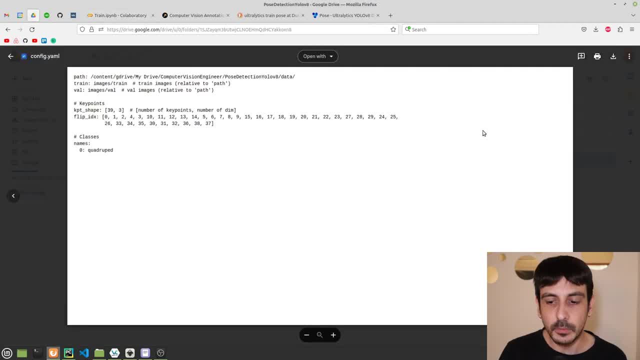 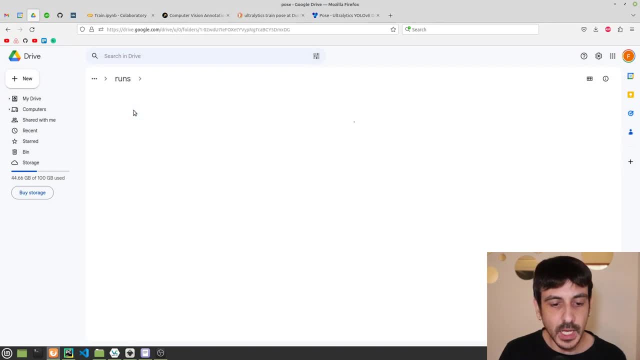 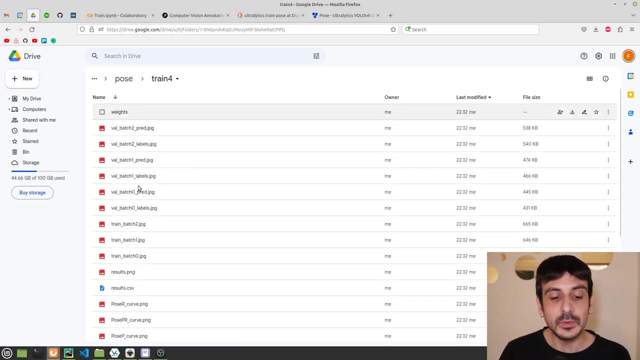 when you execute this cell. so let me show you. if i go back to my google drive, you can see. this is a runs directory which was just generated, and within this directory is where we have this train 4, which is the result of the training process we have just executed. so everything seems to be okay and what we will need. 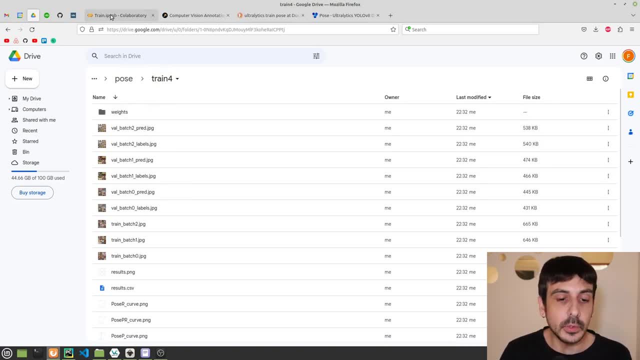 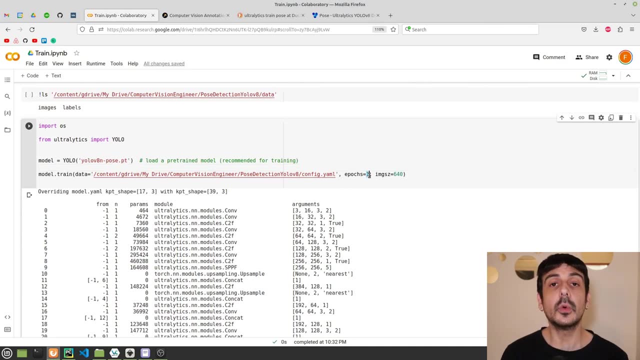 to do now is to download this directory into our local computer. now, remember this was a very, very dummy training. this is a training we did for only one epoch. obviously, you will need to do like a deeper training if you really want to train your post detector on your data. one epoch. 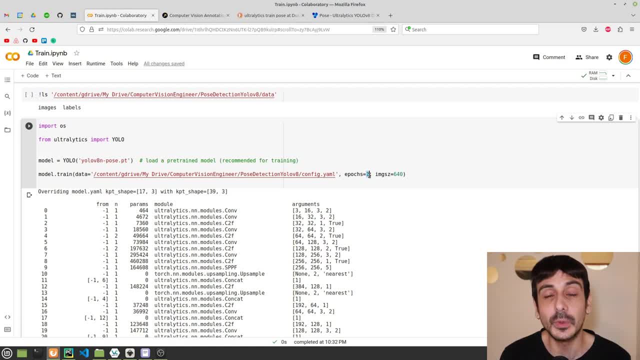 it's, it's very unlikely to be sufficient. you will need to do like a deeper training. in my case, i have already trained the model with my data and i did it for 100 epochs. right, i did it before starting this tutorial. so everything is already trained and we can just analyze the results. 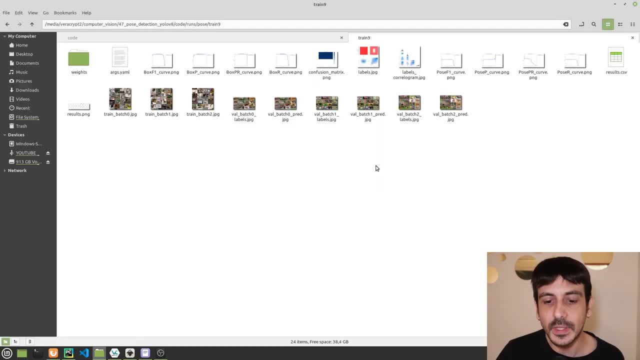 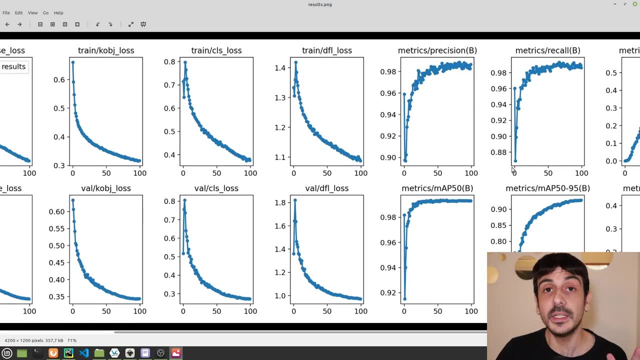 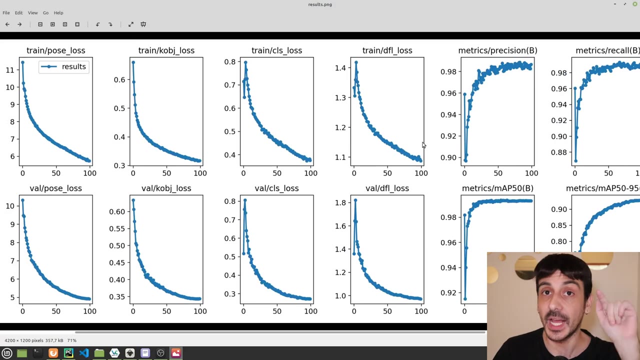 so now let's move to my local computer so i can show you exactly how to validate the model i trained using a yellow v8, and you can see that these are many, many, many different plots, many functions. we are uploading a lot of information, but we're going to focus in the loss function and 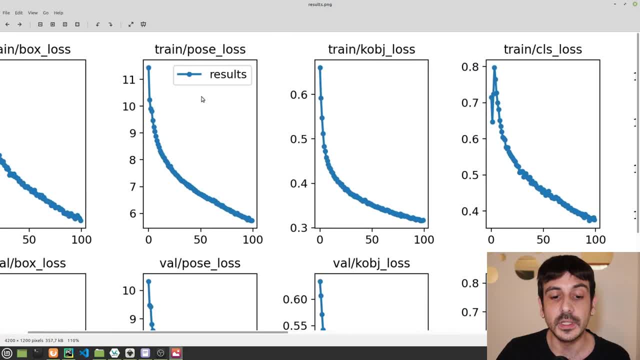 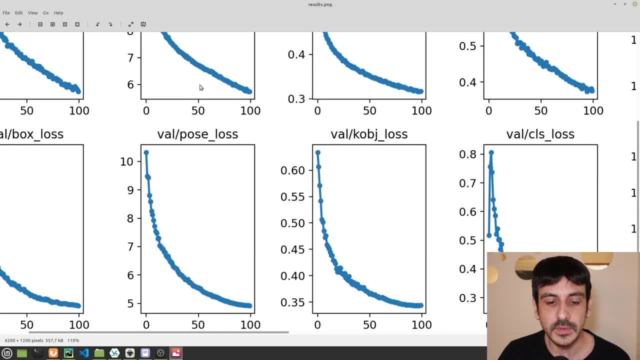 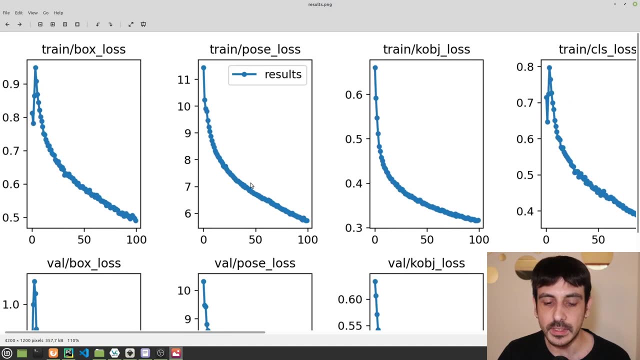 specifically, we are going to focus in this loss, which is the loss function related to the post. so we are going to focus on the post loss related to the training set and the post loss in the validation set and if we look at the training set, you can see that the loss is going down. 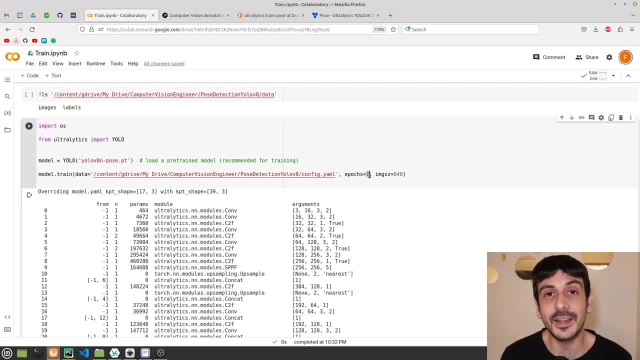 detector on your data. one epoch it's it's very unlikely to be sufficient. you will need to do like a deeper training. in my case, i have already trained the model with my data and i did it for starting this tutorial. so everything is already trained and we can just analyze the results. so now, 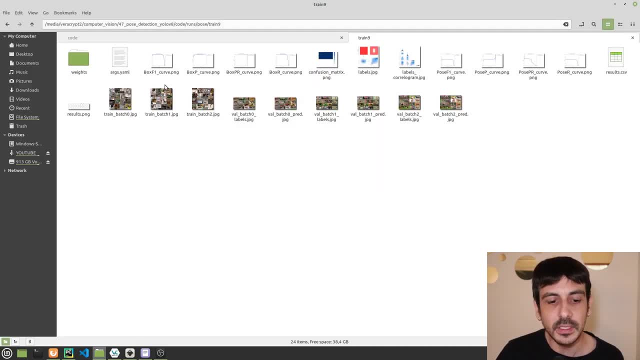 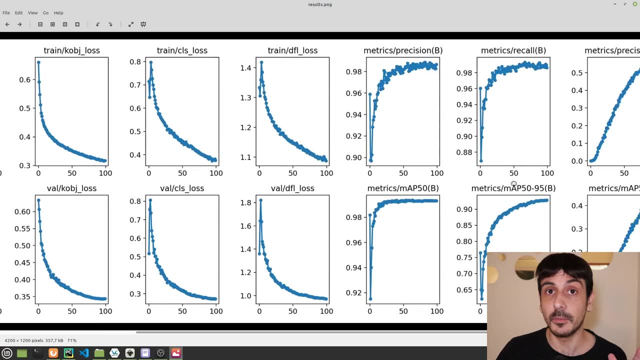 let's move to my local computer so i can show you exactly how to validate the model i trained using a yellow v8 and you can see that these are many, many, many different plots, many different functions. we are plotting a lot of information, but we're going to focus in the last function and 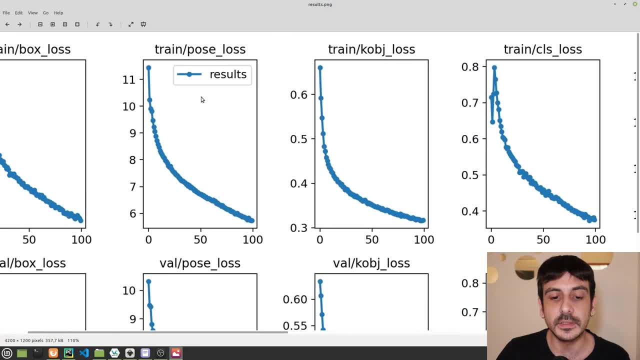 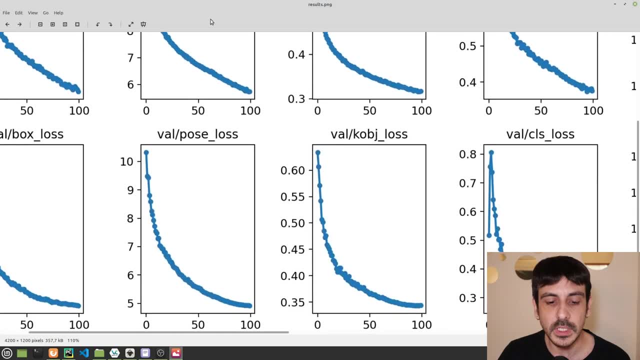 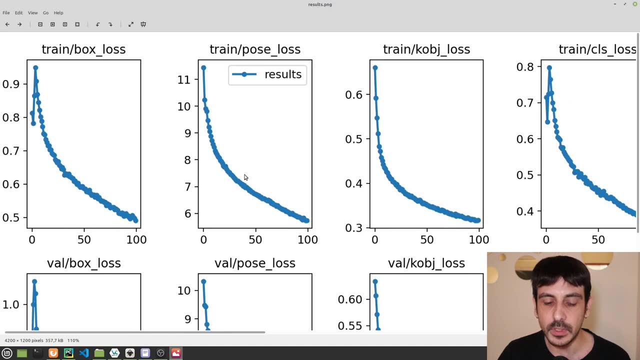 specifically, we are going to focus in this loss which is the last function related to the pose. so we are going to focus on the pose loss related to the training set and the pose laws in the validation set and if we look at the training set, you can see that the loss is going down. 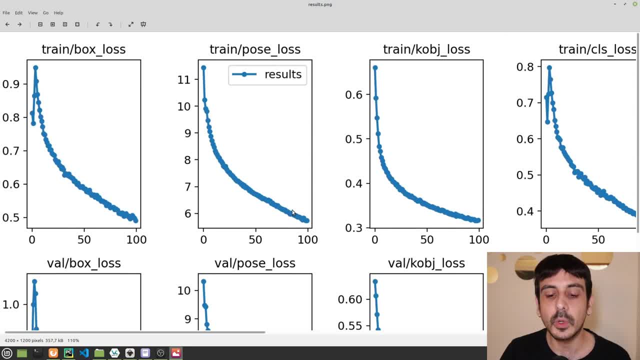 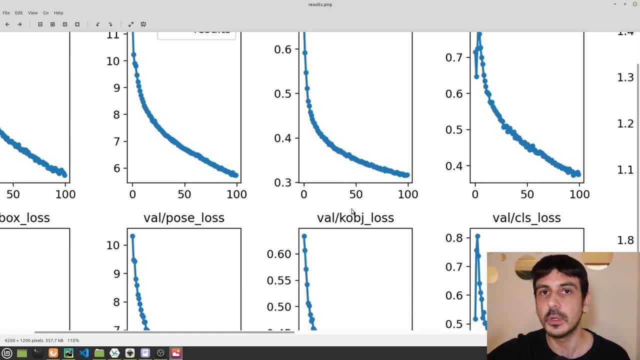 but not only is going down, but i would say that's going to continue going down for even more epochs. right, you can see that the trend is that it's going down and it's going to keep going down for more iterations, for more epochs. we haven't reached a plateau and i would say that. 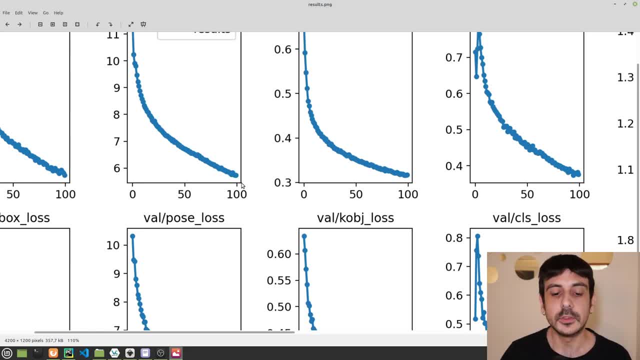 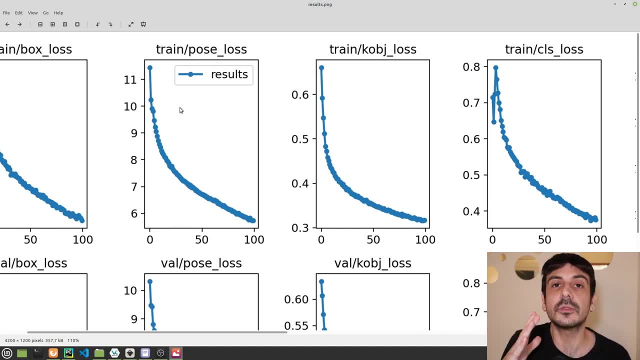 we are very far away of any plateau right, so this is a very good sign and it means the training process is going super well and it means that the the model has extra capacity. it has more capacity so we could continue training this model and it will continue learning more about this data. that's what i take by looking at. 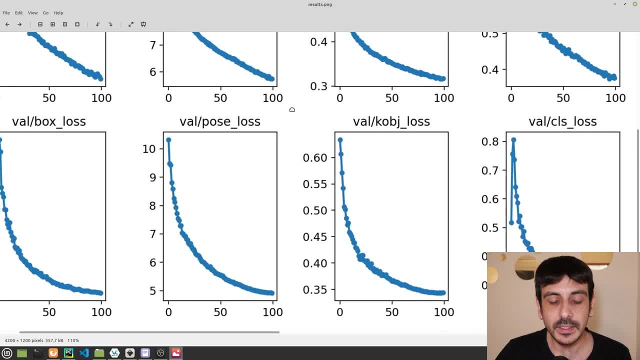 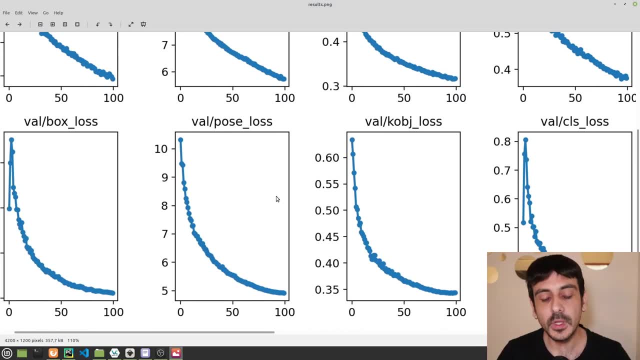 this post dose in the training set and if we look at exactly the same function but in the validation set, we can see that it's going down. so that's a good thing, but i have the impression that it's starting to be something like a plateau, right. it's not very clear because it's happening right in the 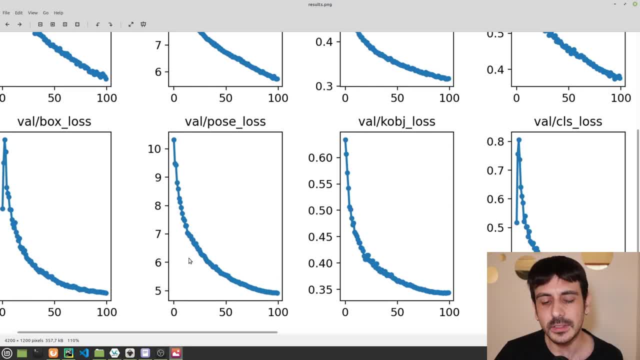 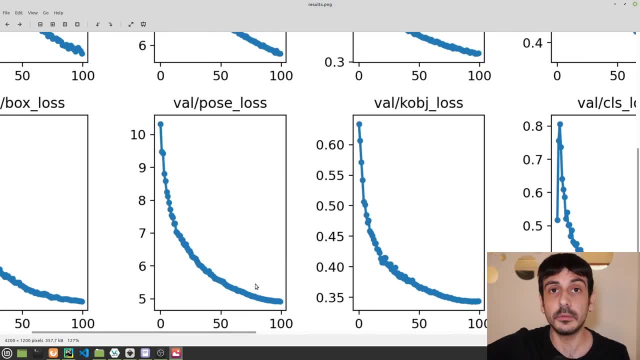 in writing the end of this training process. but you can see that it somehow seems like this is going to be a plateau from now on right. at the very least, we can see that it's going down there. that's absolutely and 100 clear. and then it's unclear what will happen from now on, or what. 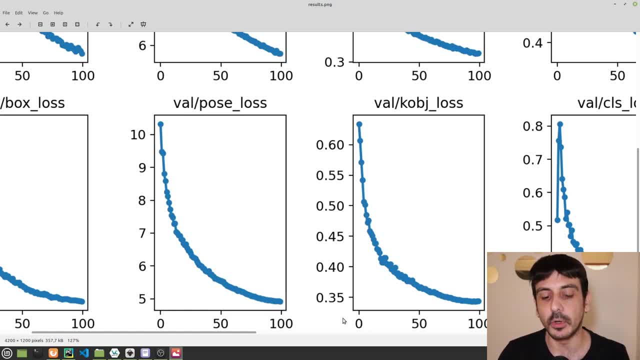 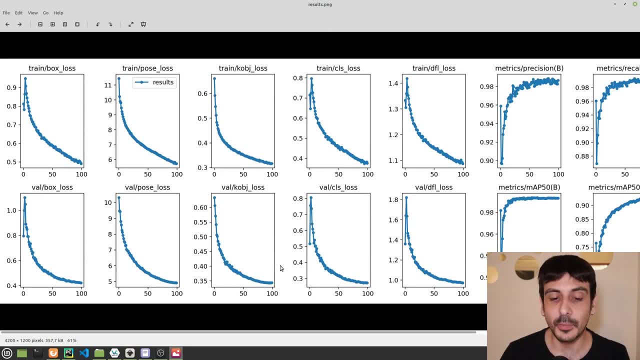 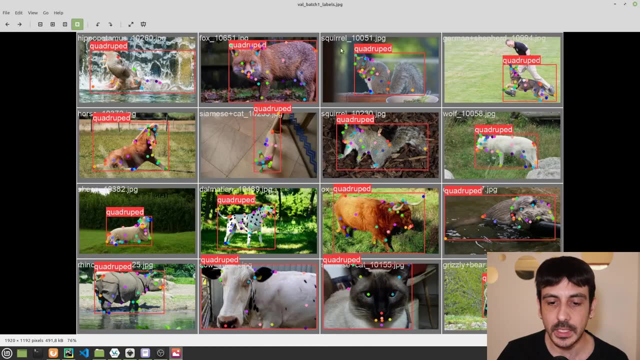 would have happened if i would have this model for more epochs, but it seems we may have reached a plateau, and that's something we need to keep in mind in this validation process. but now let's take a look at exactly how it's performing with some images. so the way i'm going to do it is like this: i am going to open this. 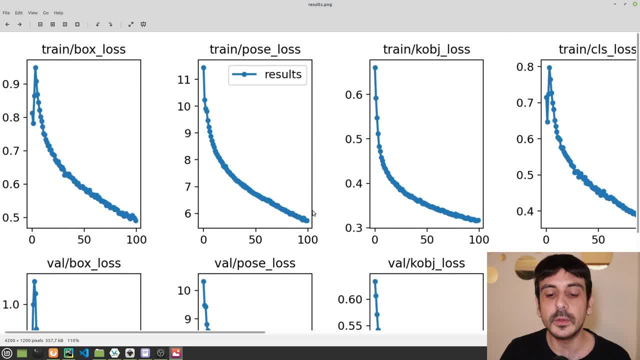 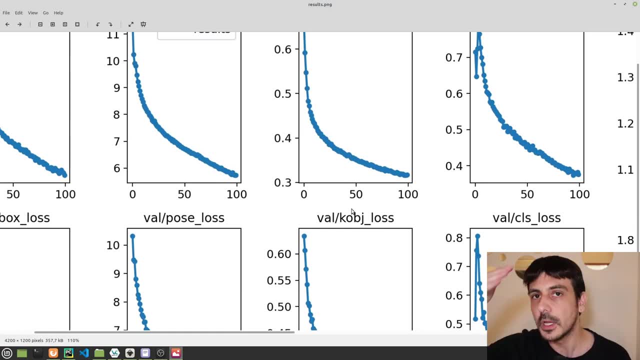 but not only is going down, but i will say that's going to continue going down for even more epochs. see that the trend is that it's going down and it's going to keep going down for more iterations, for more epochs. we haven't reached a plateau and i would say that we are very far away of any plateau. 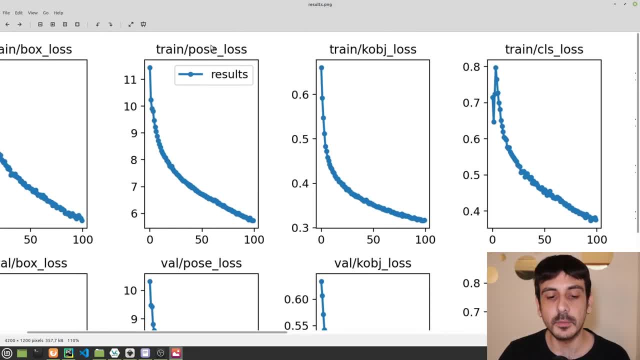 right. so this is a very good sign and it means the training process is going super well and it means that the the model has extra capacity. it has more capacity so we could continue training this model and it will continue learning more about this data. that's what i'm. 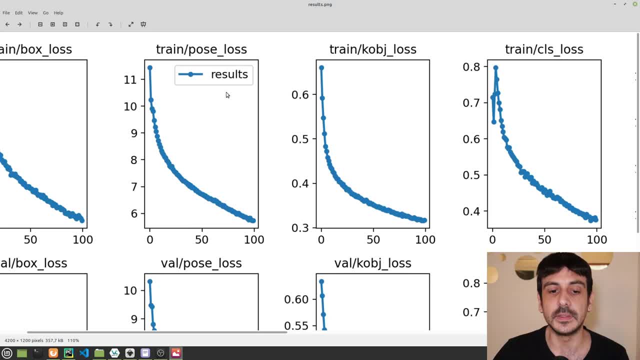 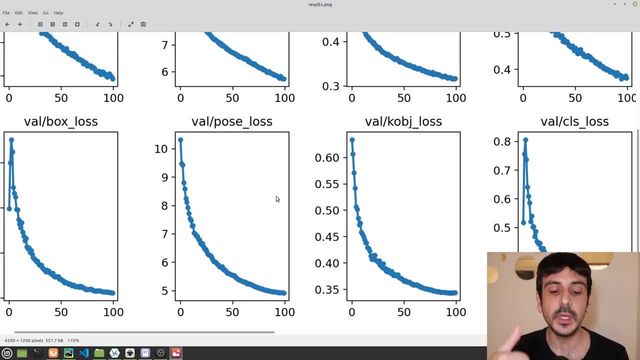 going to focus on. so let's see what i take by looking at this post dose in the training set. and if we look at the exactly the same function but in the validation set, we can see that it's going down. so that's a good thing, but i have the impression that it's starting to be something like 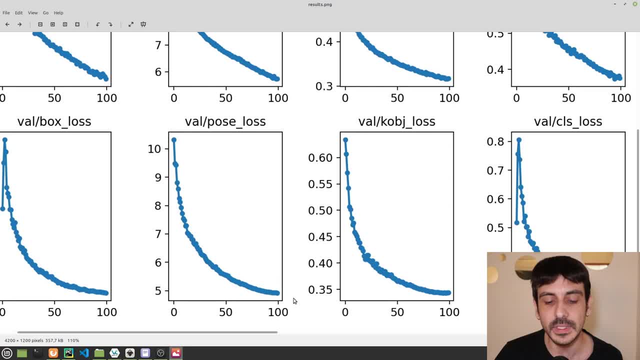 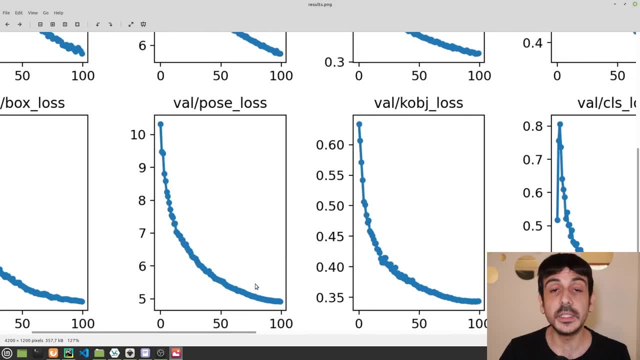 a plateau, right? it's not very clear because it's happening right in the in the end of this training process, but you can see that it somehow seems like this is going to be a plateau from now on. right at down there, that's absolutely and 100% clear. and then it's unclear what will happen from now on. 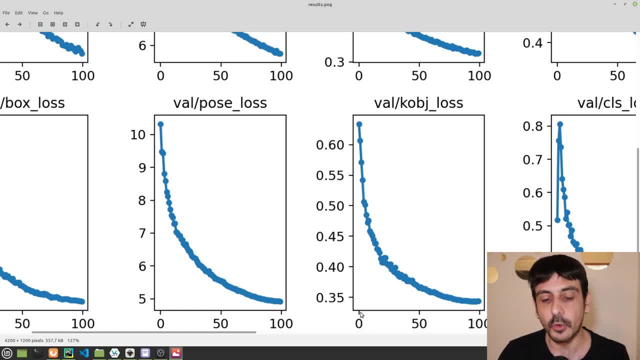 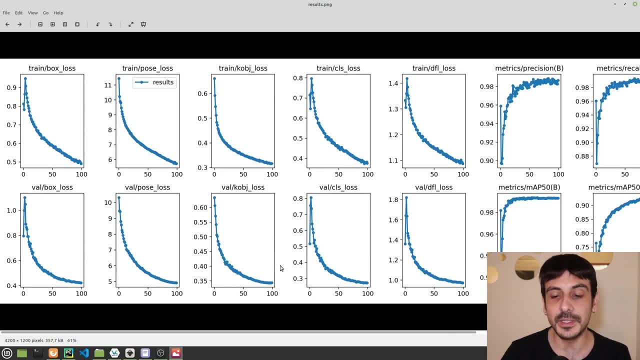 or what would have happened if I would have trained this model for more epochs. but it seems we may have reached a plateau, and that's something we need to keep in mind in this validation process. but now let's take a look at exactly how it's performing with some images. so the way I'm going- 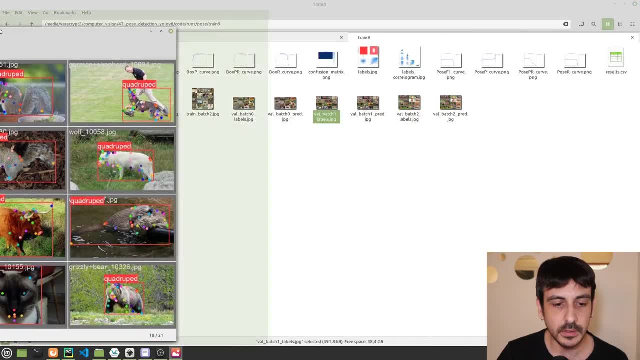 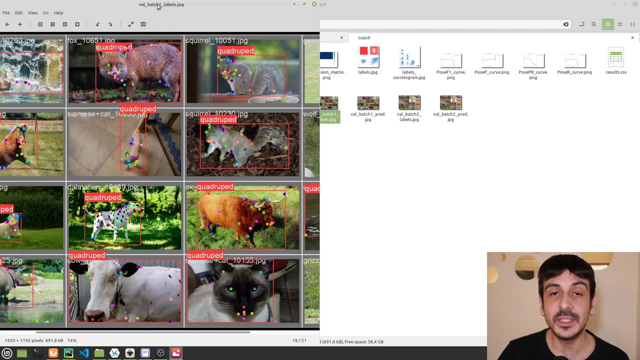 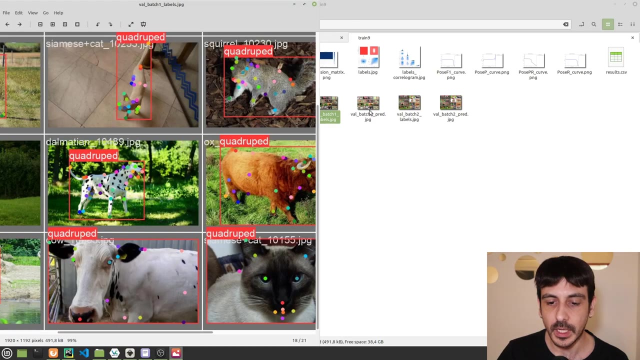 to do. it is like this: I am going to open this image, which is the is one of the batches in the validation set, and these are all labels. right, these are not all predictions, but these are the labels, the annotations. now I'm going to keep this open and I'm going to open exactly the same batch, but 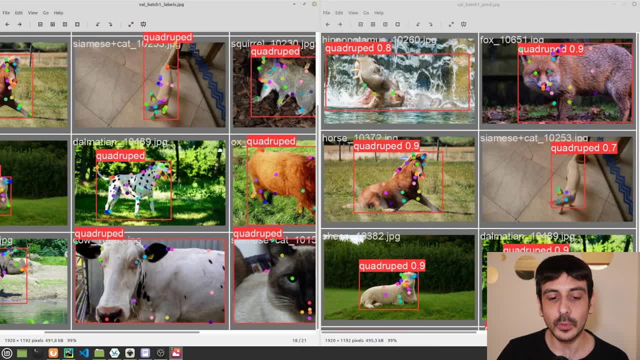 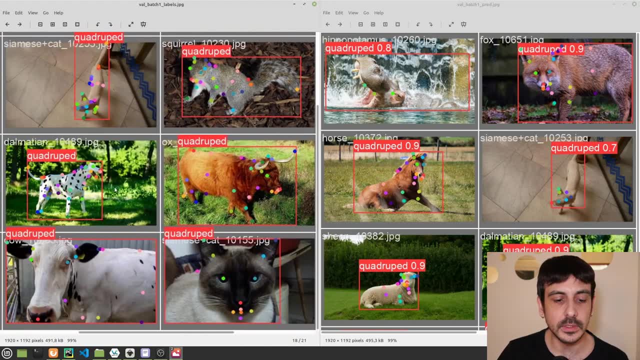 all predictions right. this is going to be a very good way to analyze the results, because now we have a lot of images and we need to keep them open. and we need to keep them open and we need to to make more conclusions. we need to make a take a look at more samples. we need to. this is a much 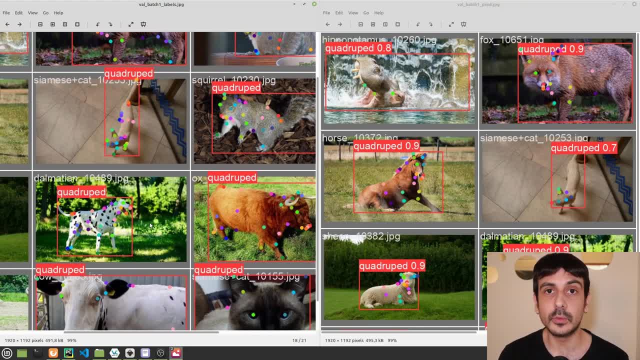 more complex problem. in my previous tutorials i show you how to train an image classifier using yellow v8, an object detector and an image segmentation model, and i will say that today's model, this key point detector, is much more complex than everything we did before. so this validation- 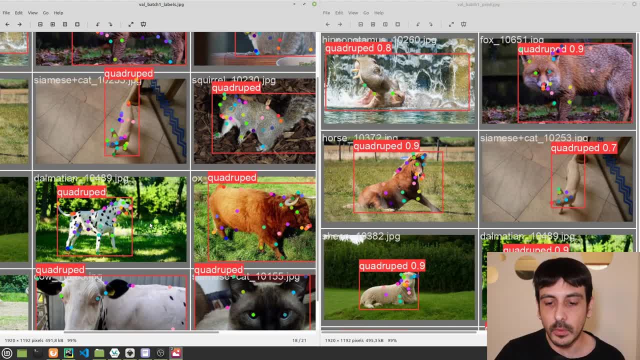 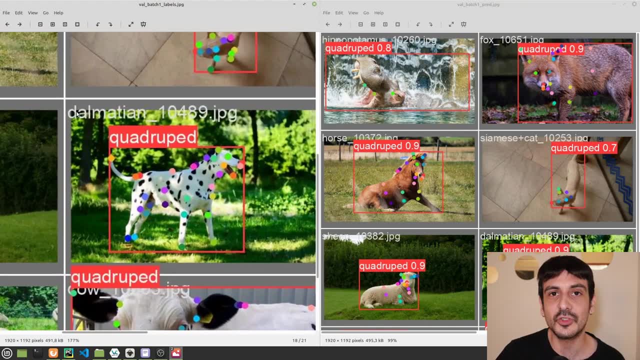 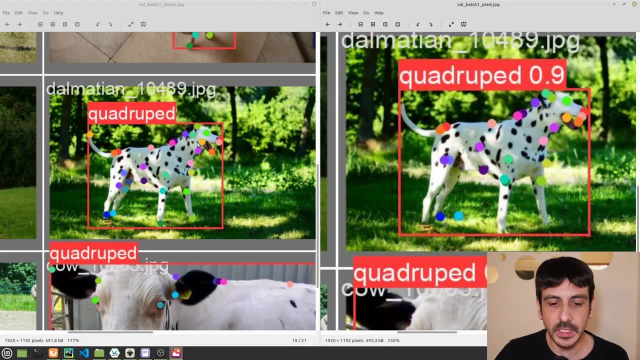 process will be more complex as well. now, if you look at all of these images, i'm going to focus on only one of them. i'm going to focus on this dog, on this dalmatian, and i'm going to show you exactly what's going on here. let's focus on this animal first and you can see that, basically, these are. 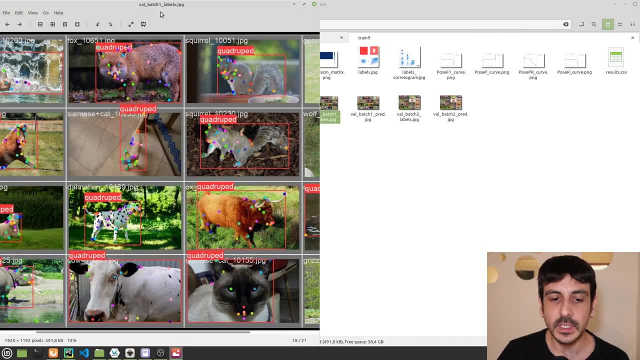 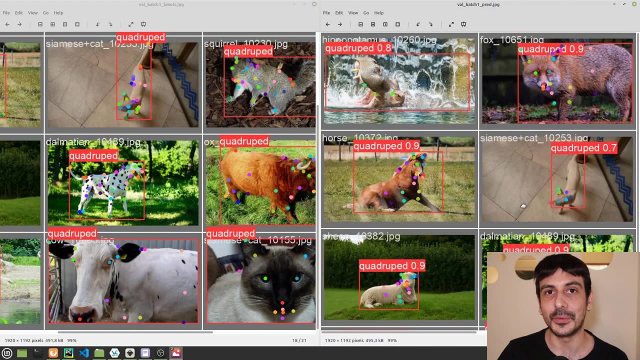 image, which is the, is one of the batches in the validation set, and these are all labels, right? these are not or predictions, but these are the labels, the annotations. now i'm going to keep this open and i'm going to open exactly the same batch, but or predictions. right, this is going to be a. 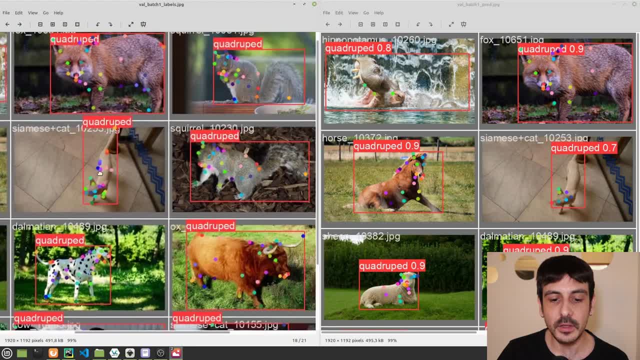 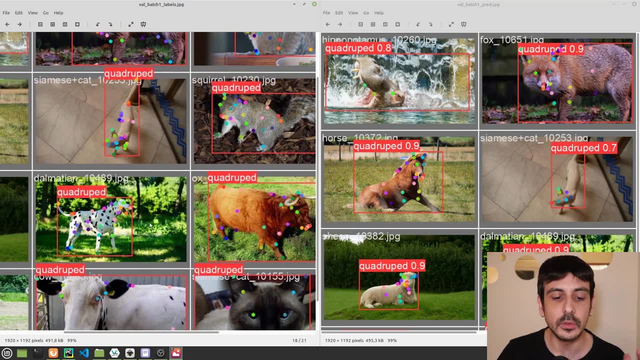 very good way to analyze the results, because now we have a lot of images and we need to make more conclusions. we need to make a take a look at more samples. we need to. this is a much more complex problem. in my previous tutorials, i show you how to train an image classifier using yellow v8. 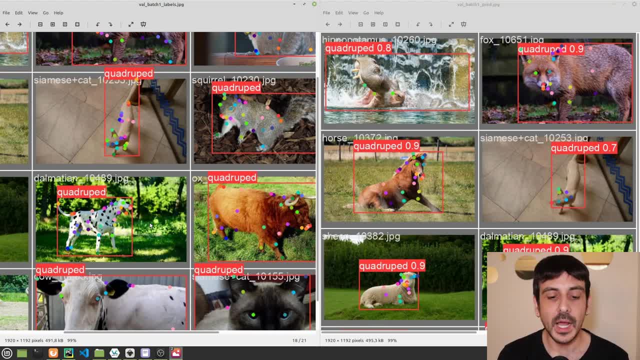 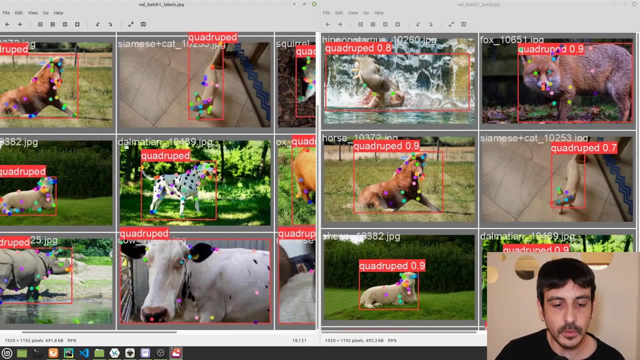 and i'm going to show you how to train an image classifier using yellow v8, an object detector and an image segmentation model. and i will say that today's model, this key point detector, is much more complex than everything we did before, so this validation process will be more complex as well. now, if you look at all of these images i'm going to focus on, 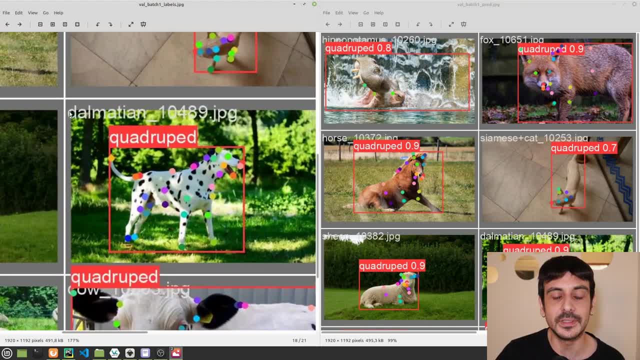 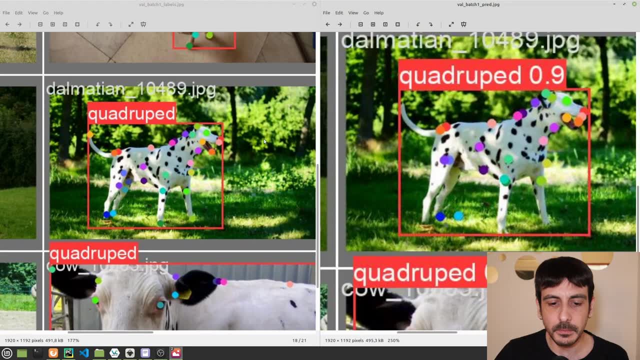 only one of them. i'm going to focus on this dog, on this dalmatian, and i'm going to show you exactly what's going on here. let's focus on this animal first and you can see that basically these are all of our key points. these are basically, these are ground truth. these are all of our annotations. 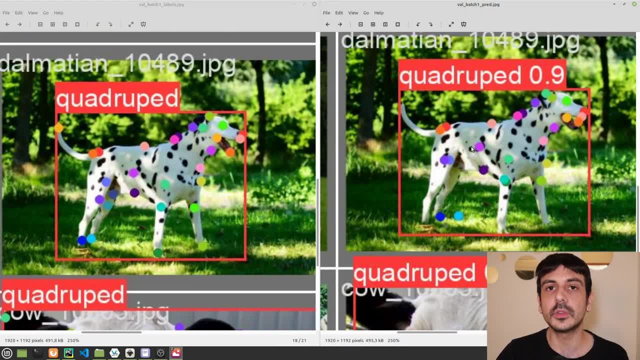 and these are all of our predictions and you can see that it looks pretty well. it looks very, very well. i would say that if we look at all of these key points which are around the face, i would say they are perfect. i would say they are very, very good. and then if we look at these key points over, 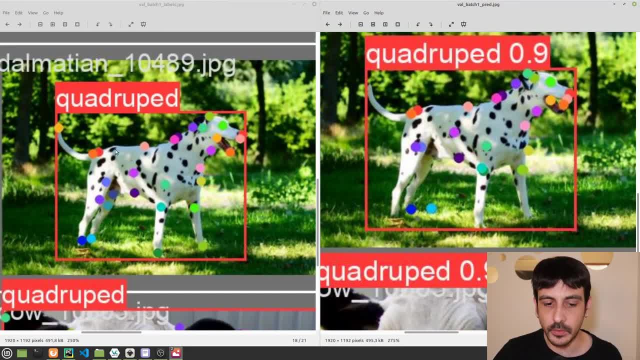 here. you can see that it's very good as well. if we look at these three key points. it's also very good, these two key points over here as well it's. it's very good too. and then if we look at the legs, i can see something is going on here, because i don't really 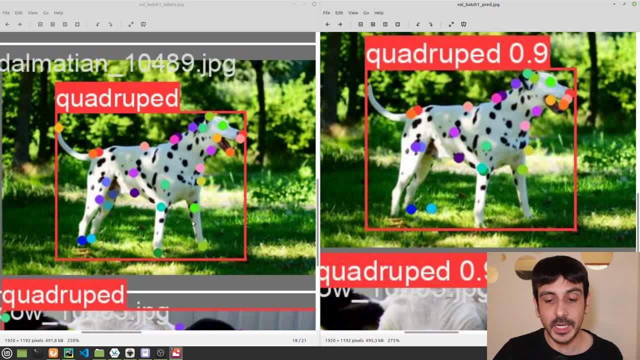 see these two key points. so we are not detecting the legs and if i look at the legs entirely, i will say something is going on, because i don't really see. i i think we have an issue in the legs and also you can see that this key point which is at the end of the tail, we are not detecting this. 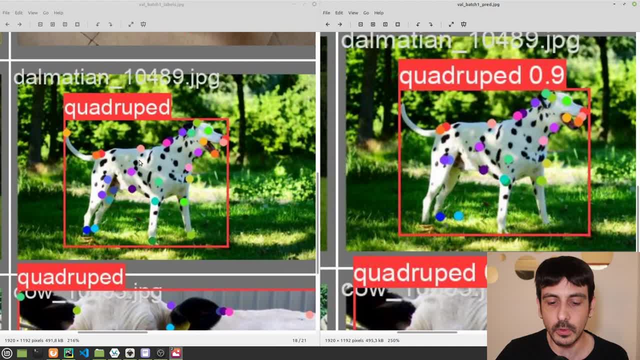 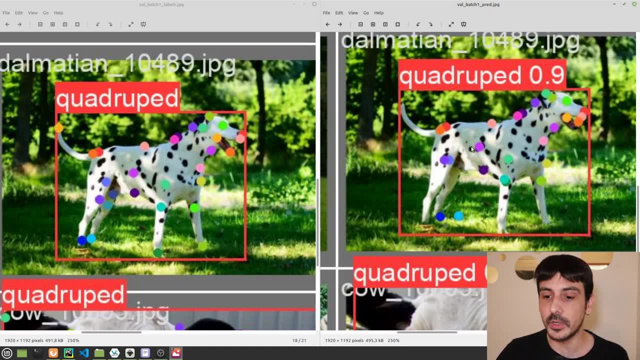 all of our key points. these are basically, these are ground truth. these are all of our annotations and these are all of our predictions and you can see that it looks pretty well. it looks very, very well. i will say that if we look at all of these key points which are around the face, i would say they are perfect. i 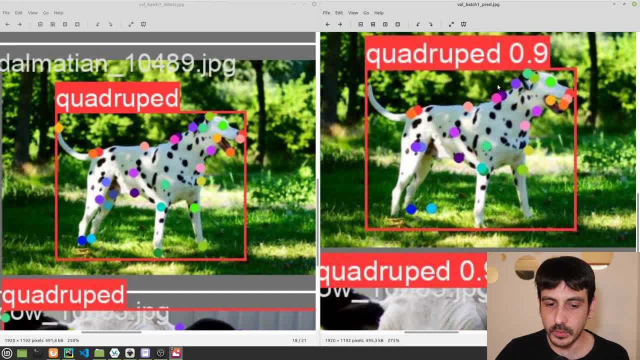 would say they are very, very good. and then if we look at these key points over here, you can see that it's very good as well. if we look at these three key points, it's also very good, these two key points over here as well, it's. it's very good too. and then if we look at the legs, i can see 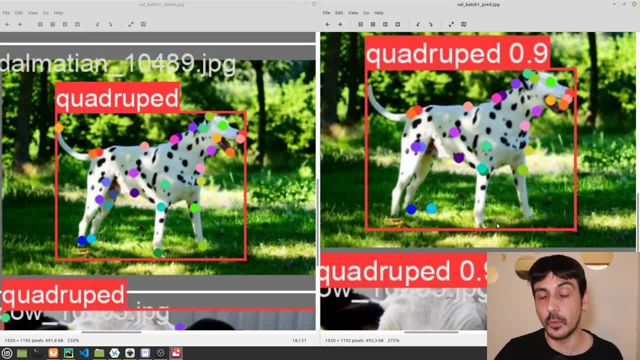 something is going on here, because i don't really see these two key points. so we are not detecting the legs. and if i look at the legs entirely, i will say something is going on here, because i don't on, because i don't really see. i i think we have an issue in the legs and also you can see that this. 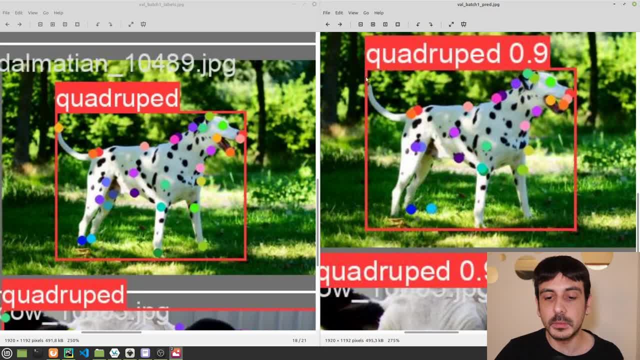 key point, which is at the end of the tail. we are not detecting this, this key point, either. so we have some issues. we have an issue in the tail and we have an issue around the legs, but everything else, i would say that is pretty good. i don't know what you think, but i think it's pretty pretty. 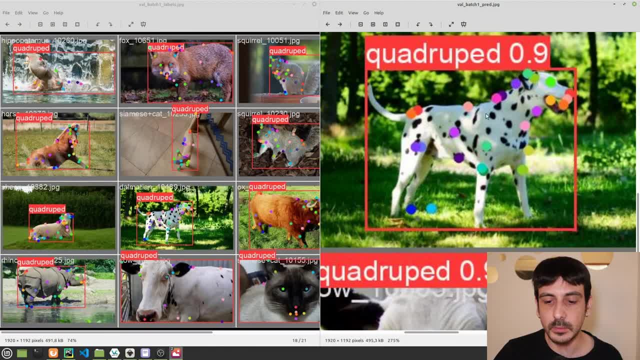 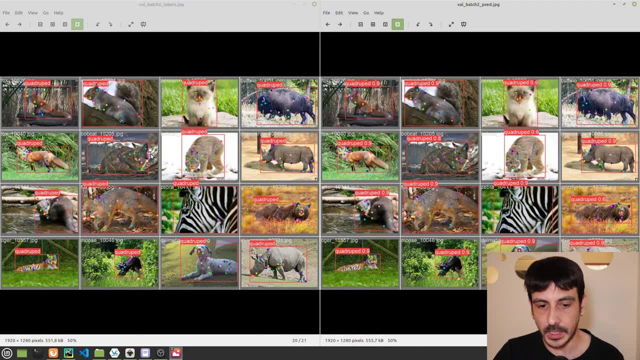 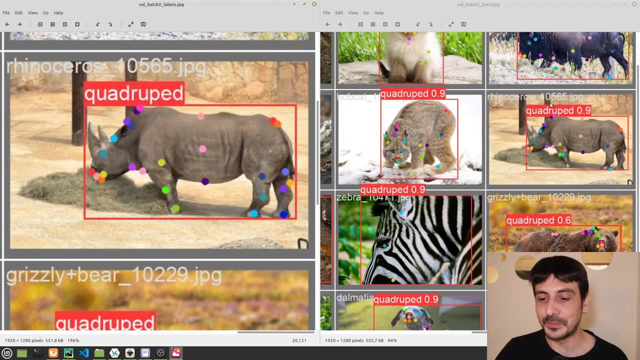 pretty good. so this is one of the examples, and now let me show you another one which is in the, in another batch. again, these are the annotations and these are the predictions. so let me show you what happens in this rhinoceros. let me show you what happens. these are our annotations. 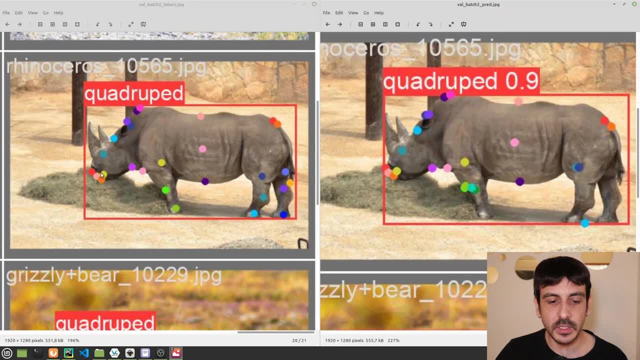 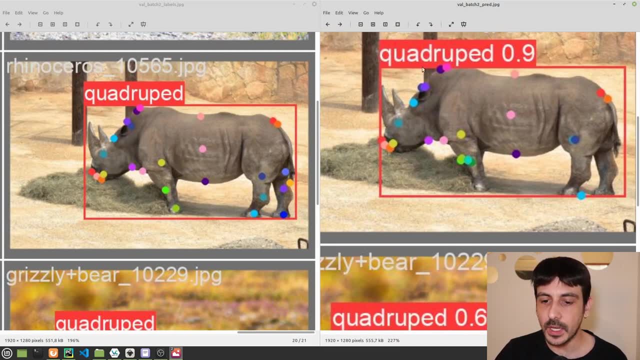 and these are our predictions, and you can see that we have a similar situation around the face. i would say: everything is just okay. we have like a very good detection. then over here, here, we have very good detection too. these three points are very well detected. then over here. 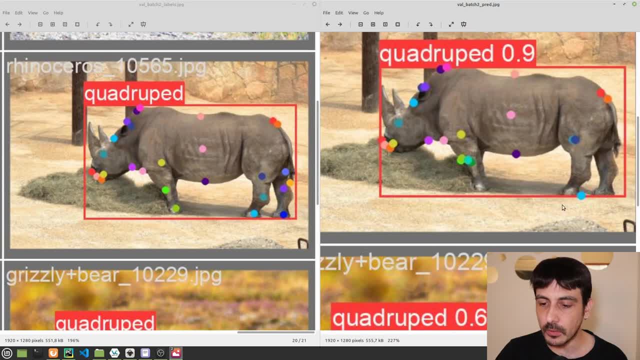 everything is okay. and then we also have an issue around the legs. right, we are not detecting all the key points in the legs properly. the same happens over here with this other leg, and the same happens in the tail, in the, in this key point which is the end tail, and then everything else. 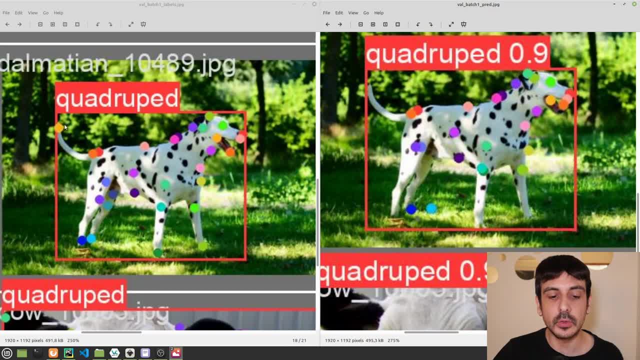 this key point either. so we have some issues. we have an issue in the tail and we have an issue in the legs, but everything else i would say that is pretty good. i don't know what you think, but i think it's pretty, pretty, pretty good. so this is one of the examples, and now let me show you another. 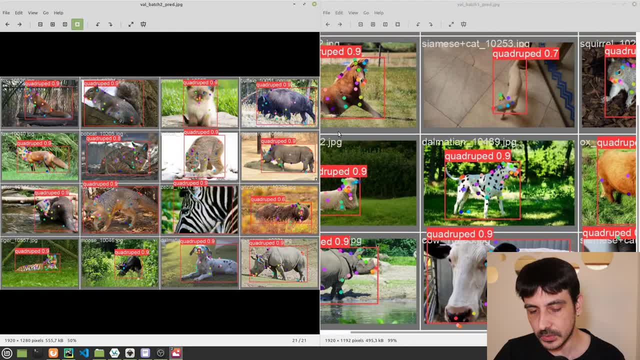 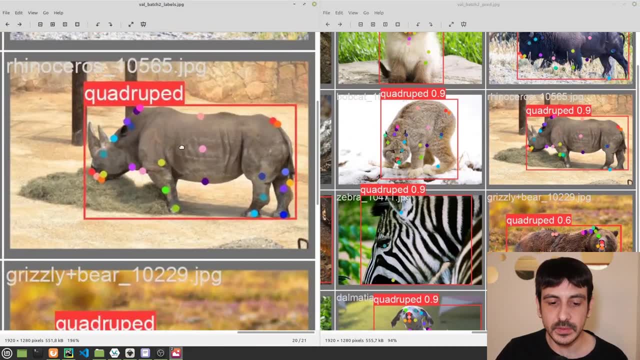 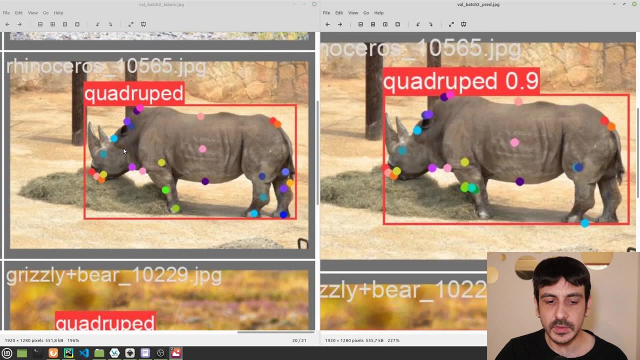 one which is in the in another batch. again, these are the annotations and these are the predictions. so let me show you what happens in this rhinoceros. let me show you what happens. these are our annotations and these are our predictions. and you can see that we have a similar. 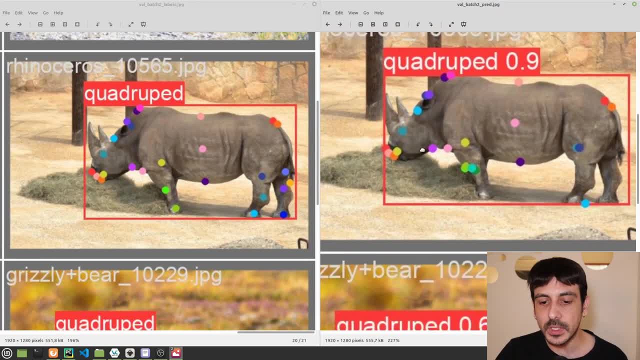 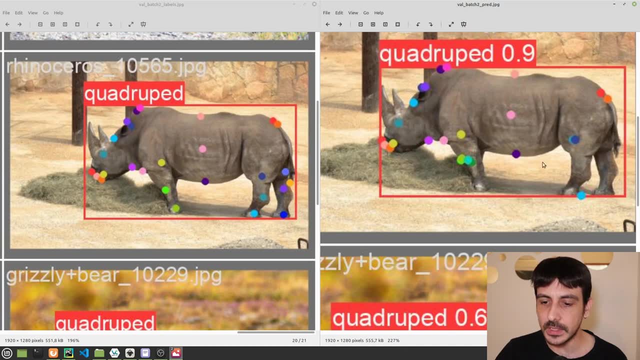 situation around the face, i would say everything is just okay. we have like a very good detection. then over here, we have very good detection too. these three points are very well detected. then over here, everything is okay. and then we also have an issue around the legs. right, we are not. 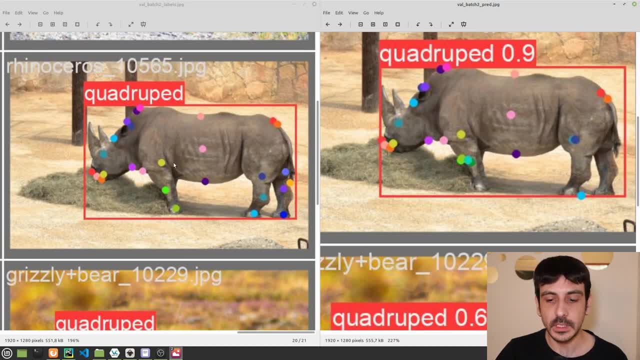 detecting all the key points in the legs properly. the same happens over here with this other leg, and the same happens in the tail, in the, in this key point, which is the tail, and then everything else seems to be working super properly. we are detecting all the key points. 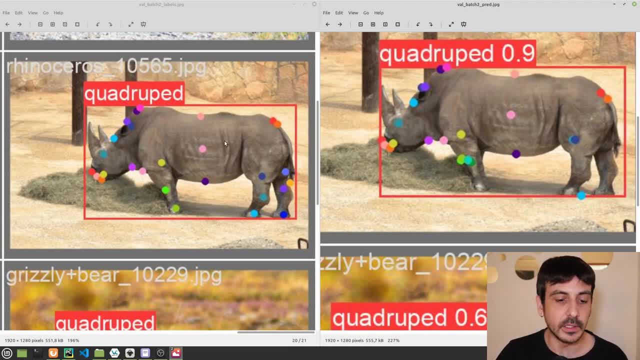 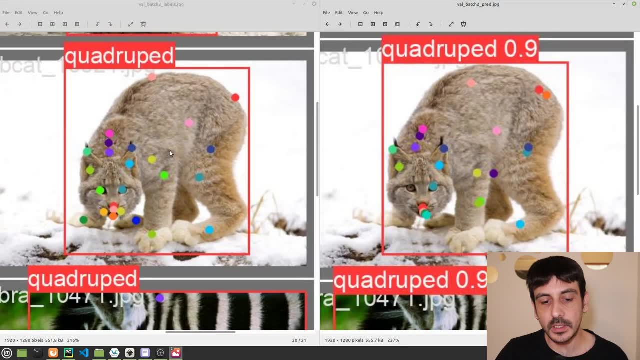 but we have an issue around the legs and around the tail. and now let me show you other examples, for example this one over here. you can see that in this case we, we have the animal in a different posture, so it's a little more challenging for them, for our model, and you can see that in this case. 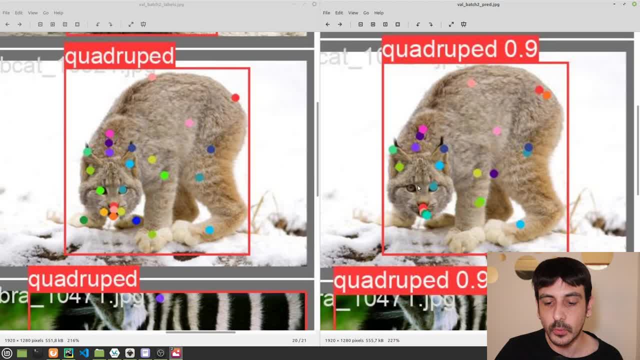 we are detecting the face very, very well. actually, we're not detecting this eye, but other than that, our key points around the face are very well detected, and you can see these three key points over here. everything is okay. this one is okay, this one too, and then you can see that we have. 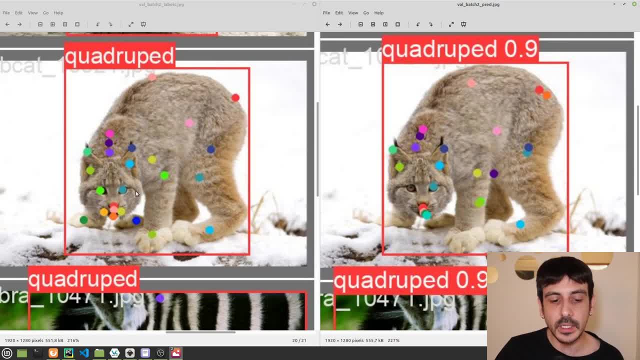 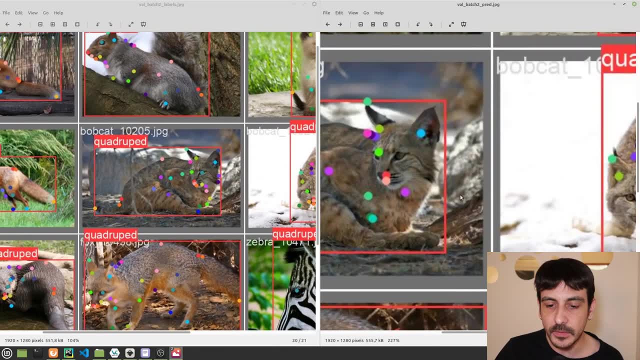 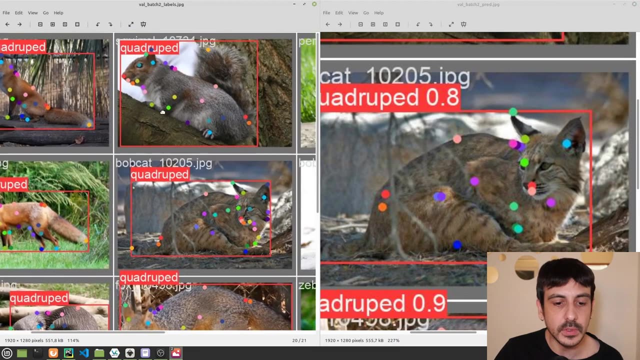 all key points which are also very well detected. but we have an issue again around the legs right and that's pretty much what i noticed by looking at many of these examples right. in many of these situations we have many different situations because there are different animals, they are in different postures, there are different shapes, different positions. that are very well. 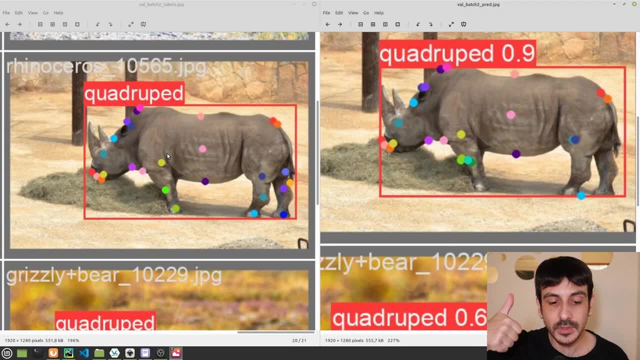 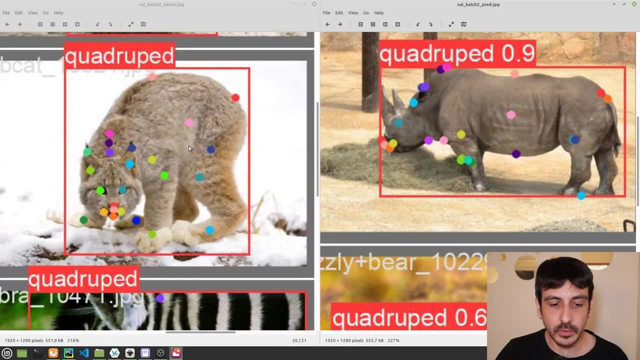 seems to be working super properly. we are detecting all the key points, but we have an issue around the legs and around the tail. and now let me show you other examples, for example this one over here. you can see that in this case we we have the animal in a different. 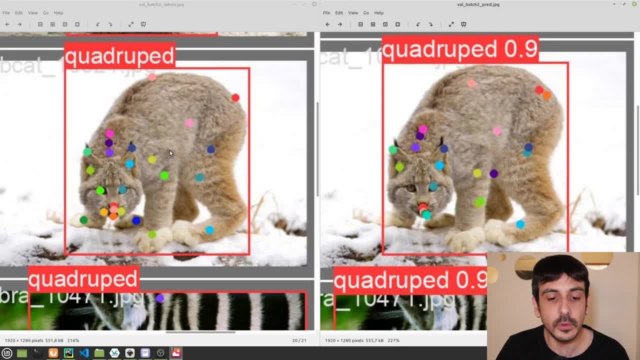 posture, so it's a little more challenging for them, for our model, and you can see that in this case we are detecting the face very, very well. actually, we're not detecting this eye, but other than that, all of the other key points around the face are very well detected and you can see these three. 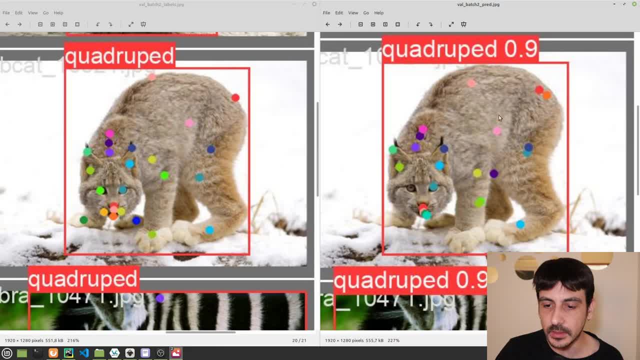 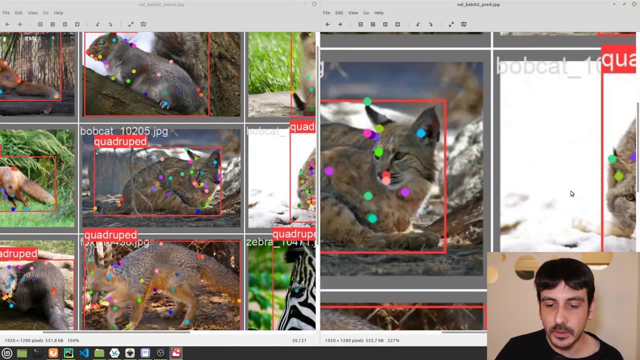 key points over here. everything is okay. this one is okay, this one too, and then you can see that we have all key points which are also very well detected. but we have an issue again around the legs right, and that's pretty much what i noticed by looking at many of these examples right in many of these situations, 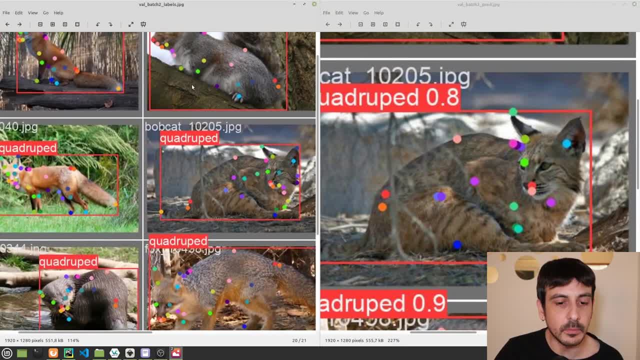 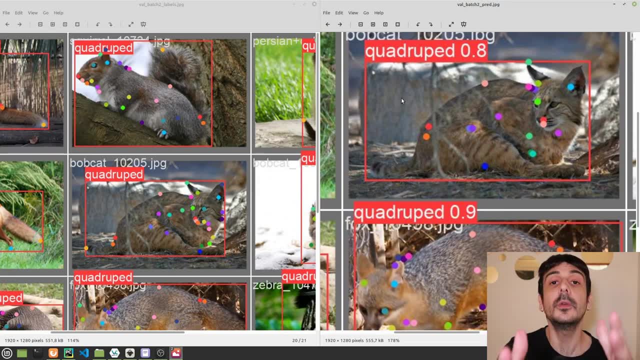 we have many different situations because there are different animals. they are in different postures, they are in different everything. so we are going to notice different situations, but after inspecting a few different animals in different positions, we are going to notice that the model is performing very, very, very well, but we may have an issue around the legs and 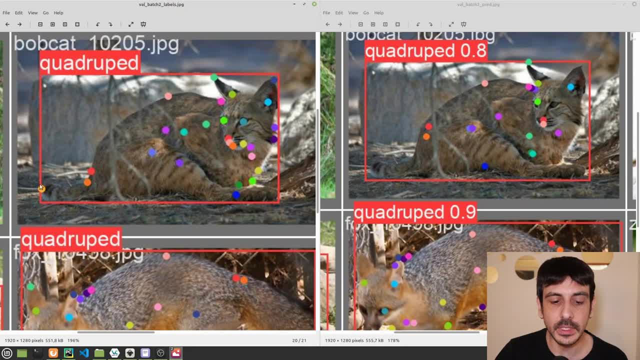 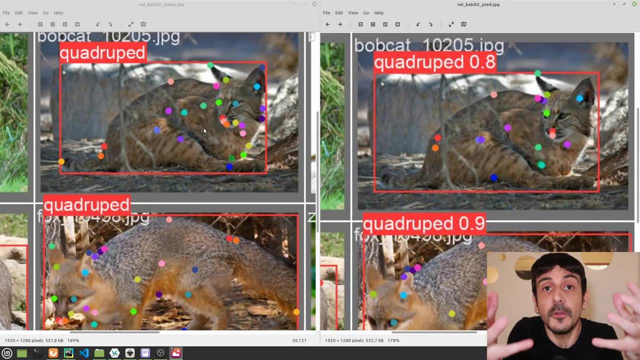 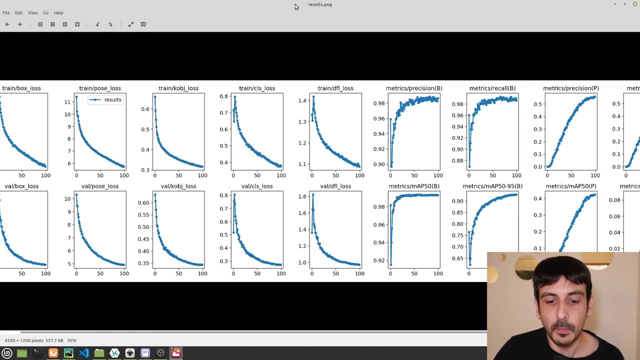 around the tail. that was my impression by analyzing many of these pictures. so, by combining this information, all the information we got by analyzing these images, all the key points, how were they were detected, and so on, and also combining everything with the loss function, with this plot regarding the loss function in the training set, and in the training set we can see: 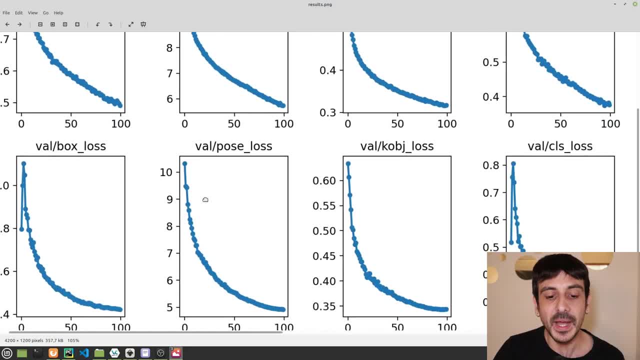 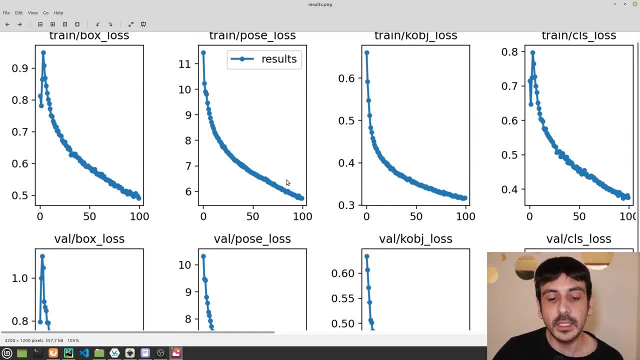 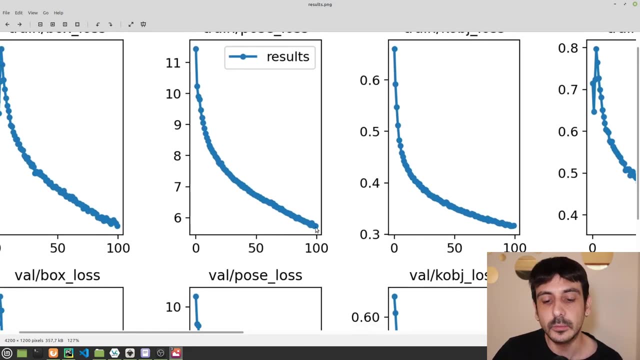 that the model is performing very, very, very well validation set. my conclusions from here will be to make a deeper training, to train this model for even more epochs, and i am curious to see what will happen in that situation because if i look at the training laws, i really like what i see. i i think this model have way more capacity. i think we could. 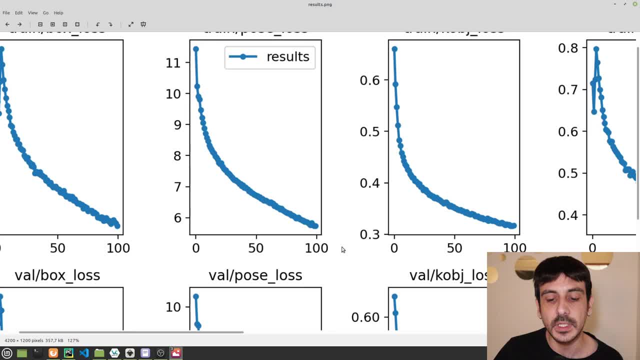 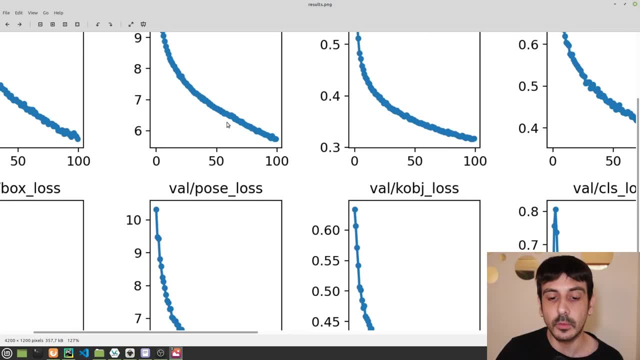 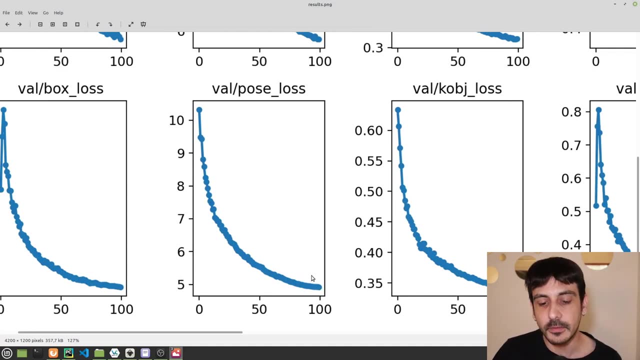 train for, i don't know, 50 more epochs, 100 more epochs, and i think we will be in a very good situation. the training laws will continue to go down and it will continue to go down in this way, very far away from the plateau. but if i look at the validation loss i have, i'm not completely. 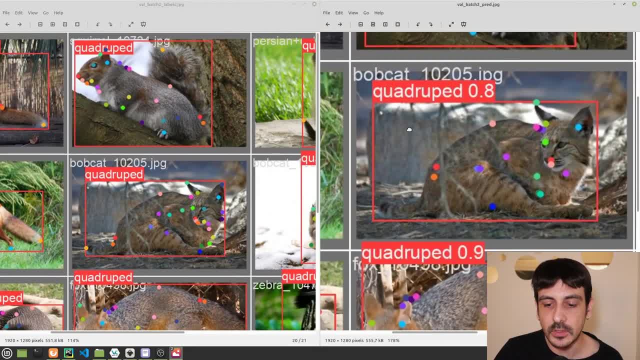 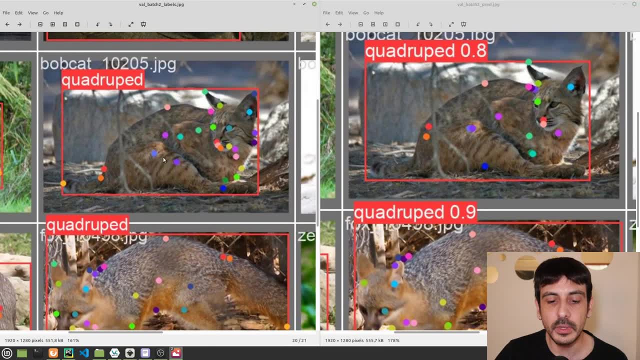 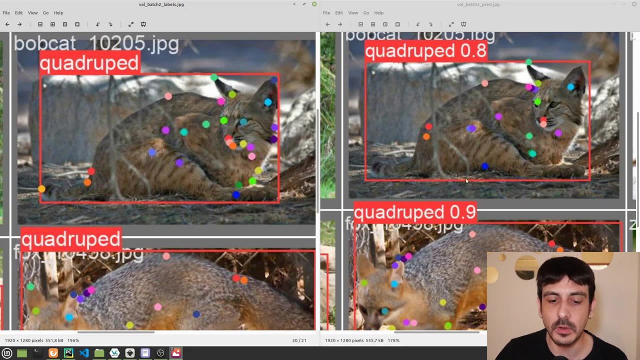 different everything, so we are going to notice different situations, but after inspecting a few of these images, i had the impression that the model is performing very, very, very well, but we may have an issue around the legs and around the tail. that was my impression by analyzing many of 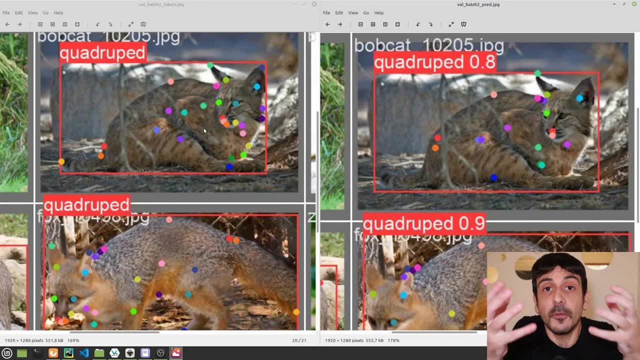 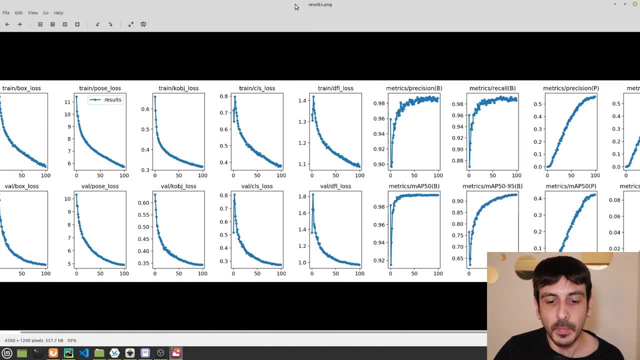 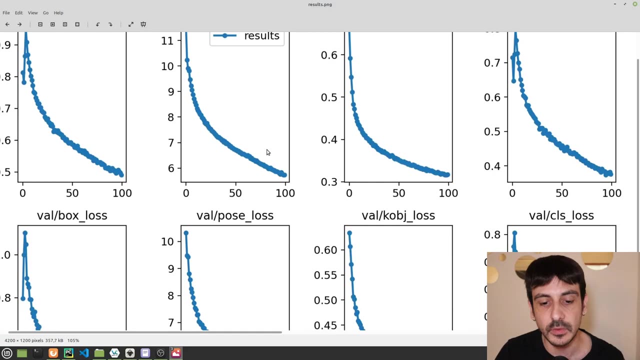 these pictures. so, by combining this information, all the information we got by analyzing these images, all the key points, how were they were detected, and so on, and also combining everything with the loss function, with this plot, regarding the loss function in the training set and in the validation set, my conclusions from here will be to make a deeper training, to train this model for 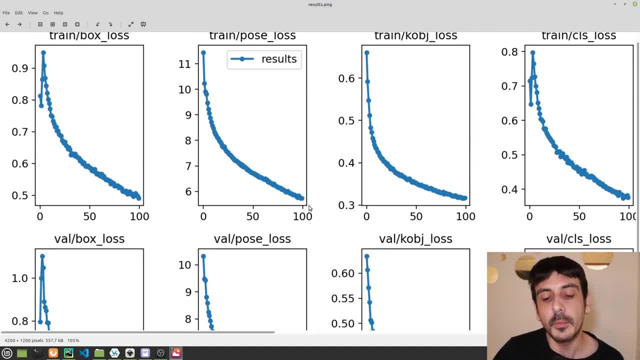 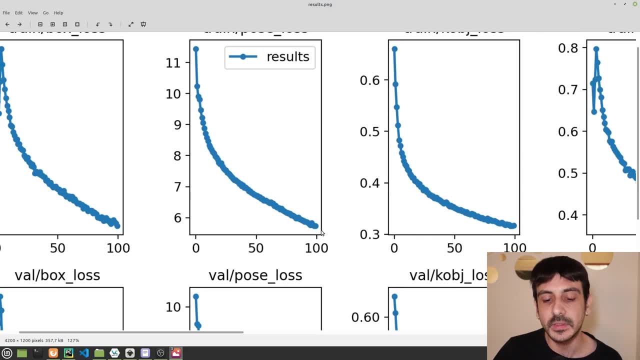 even more epochs, and i'm curious to see what will happen in that situation, because if i look at the training laws, i really like what i see. i i think this mode have way more capacity. i think we could- i don't know- 50 more epochs, 100 more epochs, and i think we will be in a very good situation. the 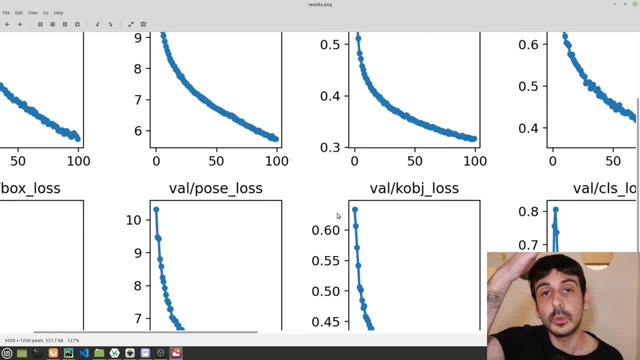 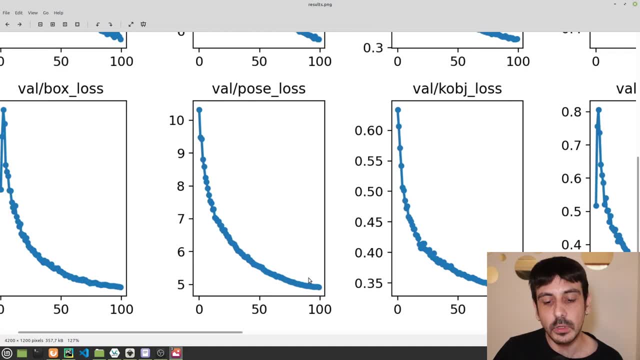 training loss will continue to go down, and it will continue to go down in this way. right, it seems we are very far away from the plateau, but if i look at the validation loss i have, i'm not completely and absolutely sure what happened from now on. so what i will do now in order to improve these. 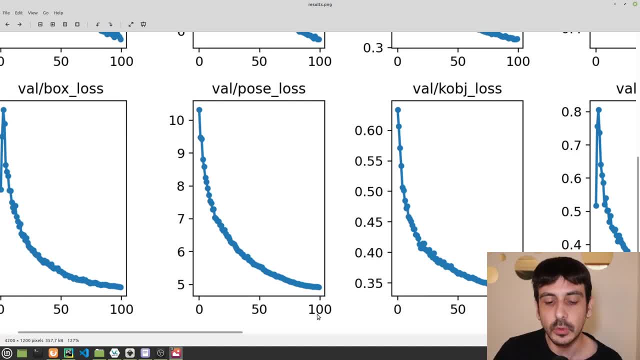 results, or in order to try to improve these results, will be to continue training for more epochs, and i will see what happens. next, i will see what happens with this loss, and then i will see what happens by analyzing these images again. right, that will be my next step, by analyzing all this information. so this is a very good 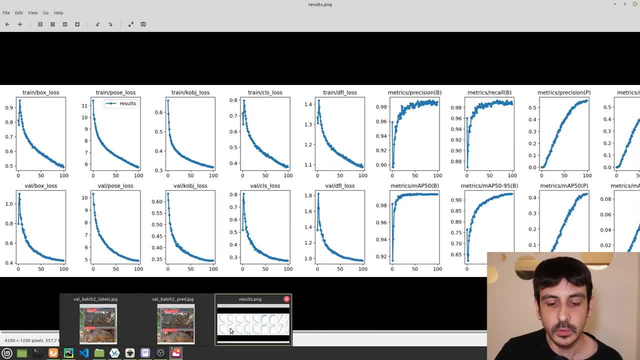 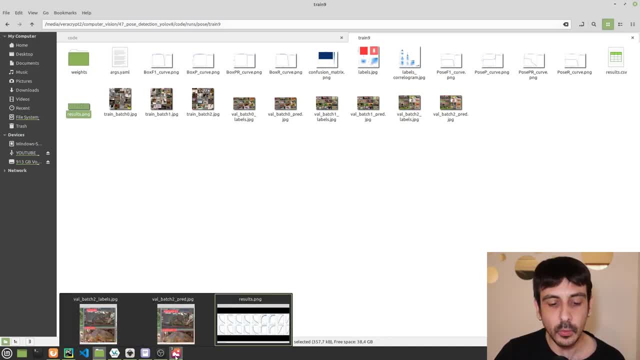 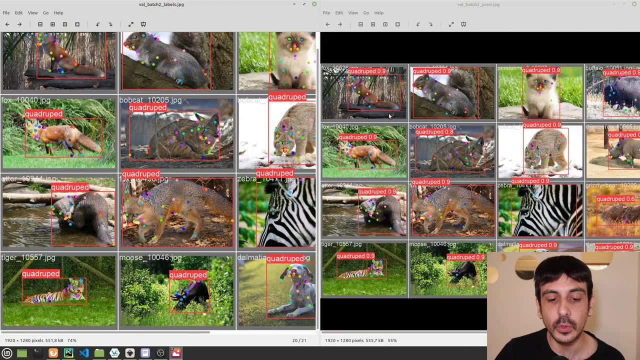 example of how to analyze your model, how to analyze your data and your plots, and so on, in a more complex example as this one, because remember that now we are trying to detect, now we are trying to learn something that's way more complex, as we did in our previous tutorials. now we are not trying to learn like a bounding box. 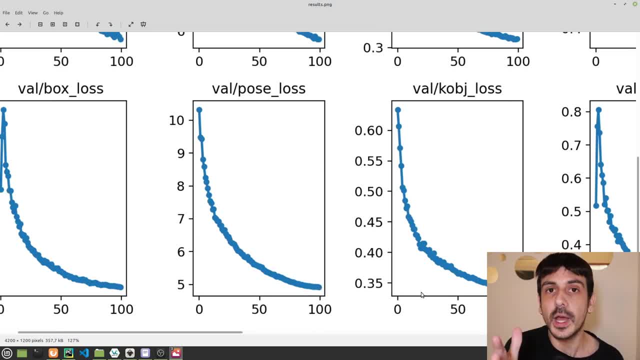 and absolutely sure what happened from now on. so what i will do now in order to improve these results, or in order to try to improve these results, will be to continue training for more epochs, and i will see what happens next. i will see what happens with this loss and then i will. 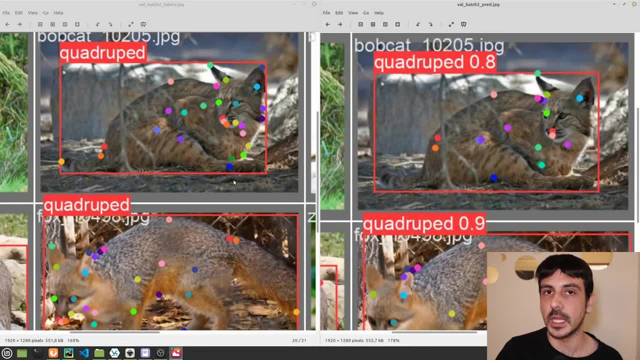 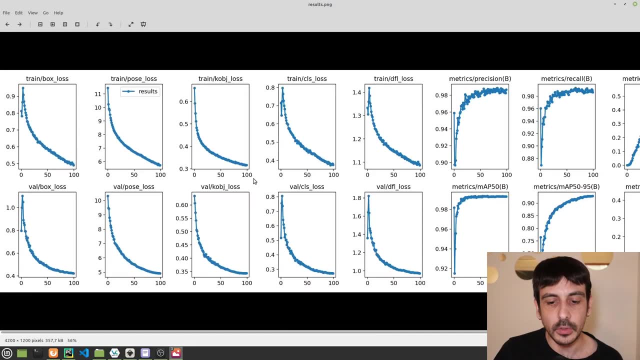 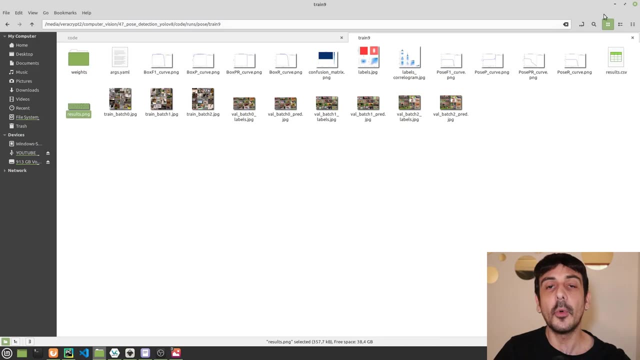 see what happens by analyzing these images again. right, that will be my next step, by analyzing all this information. so this is a very good example of how to analyze your model, how to analyze your data and your plots and so on, in a more complex example as this one, because remember- 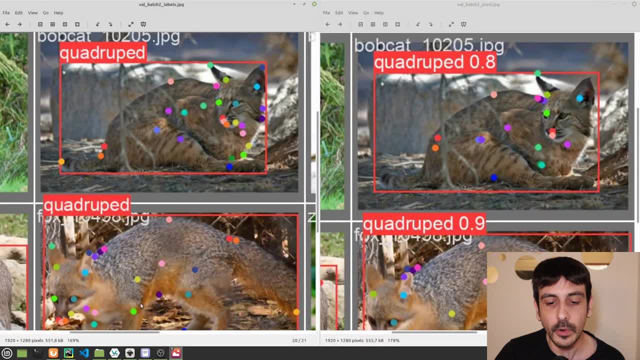 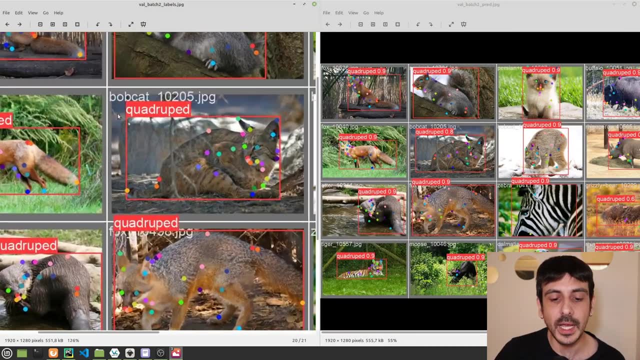 that now we are trying to detect. now we are trying to learn something that's way more complex, as we did in our previous tutorials. now we are not trying to learn like a bounding box or a mask, but we are trying to learn the entire structure of a model. 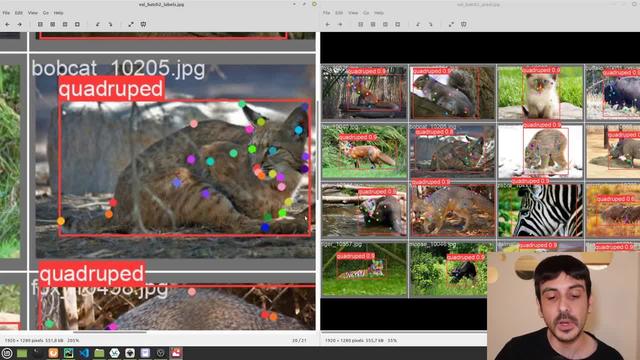 quadruple. so that's trust me. it's way more complex than everything we have made so far. so this is a very good example of how to validate a model when the problem is a little more complex. take a look at the last function. take a look what's going on. take a look in the training set. 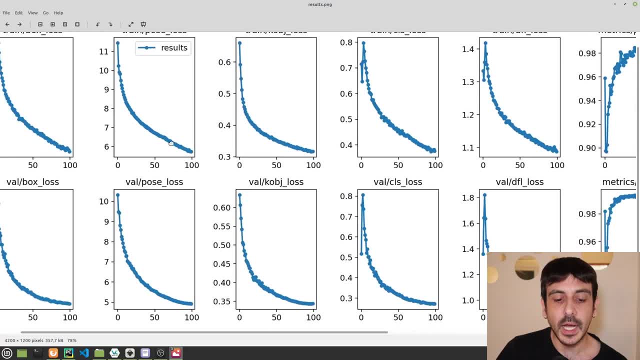 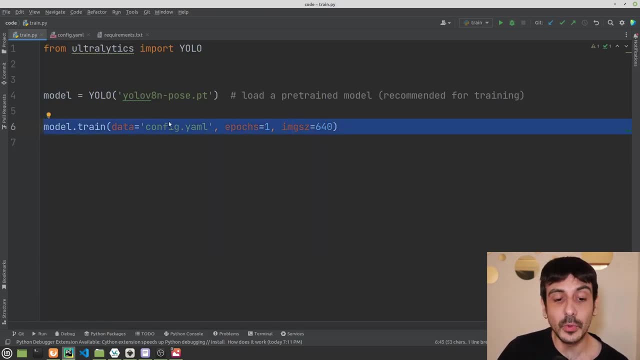 and the validation set and also take a look at some examples and then just make some conclusions. in my case, what i will do is to train for more epochs. and also, please remember that we are always using the default values of this model. uh training, right, we are training this model using all the default values, the only values we 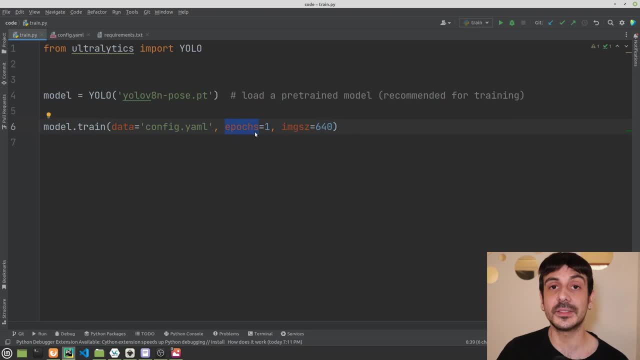 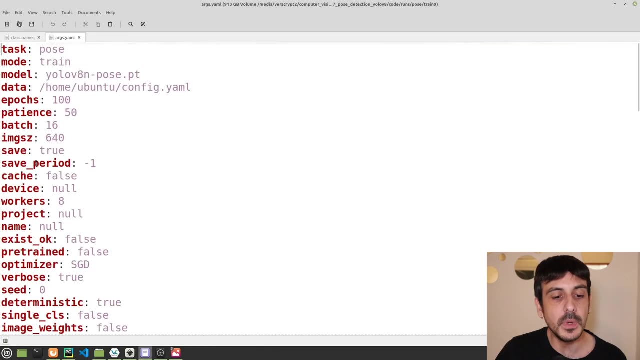 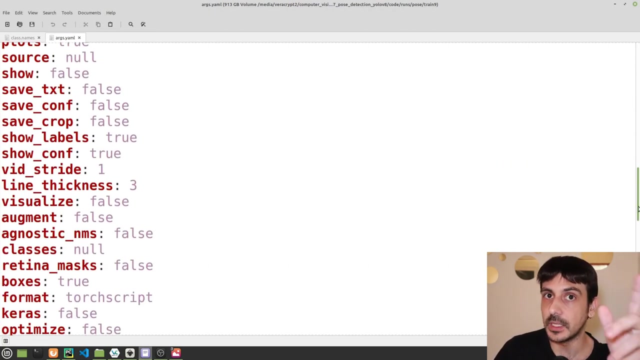 are specifying are the image size and the number of epochs, and that's it. and if i show you the entire configuration file we are using, is this one, and you can see that we have many, many, many, many, many hyper parameters. so another next step, in case a deeper training is not enough. 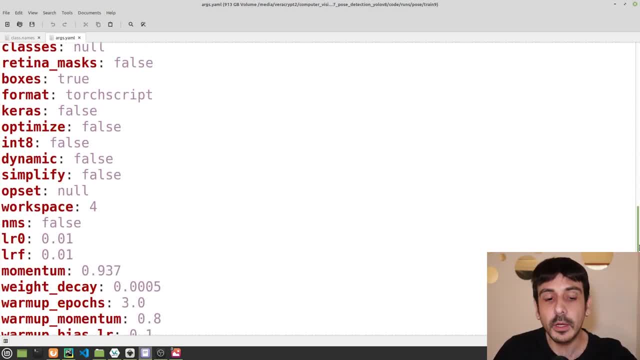 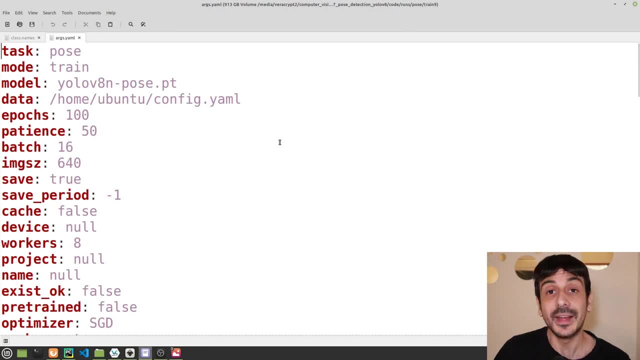 another next step will be to play around with the different deeper parameters and to find another combination of parameters which will be better for our use case. that's very important because if you are approaching a more complex problem like this one, like the one i am doing right now, i will say that it's not very realistic to expect everything goes super super. 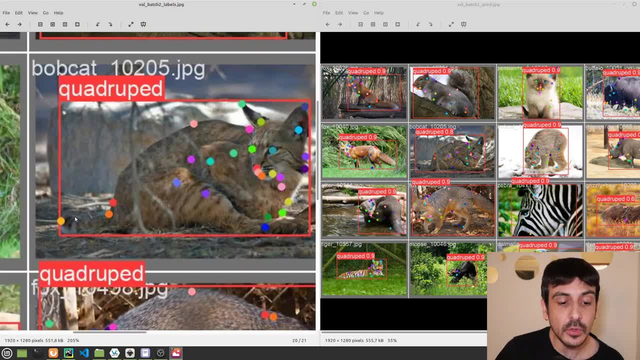 or a mask, but we are trying to learn the entire structure of a quadruple, so that's trust me. it's way more complex than everything we have made so far. so this is a very good example of how to validate a model when the problem is a little more complex. take a look at the last function. take a 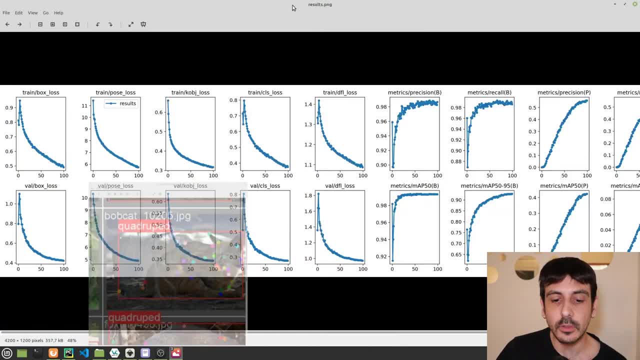 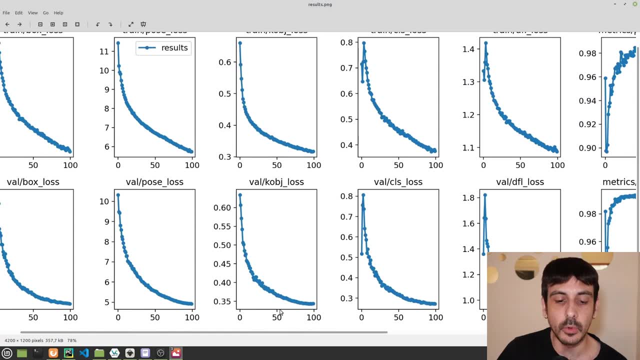 look what's going on, take a look in the training set and the validation set and also take a look at some examples and then show you how to do it in a more complex way. so i will see you in the next video. bye, bye, just make some conclusions. in my case, what i will do is to train for more epochs and also please. 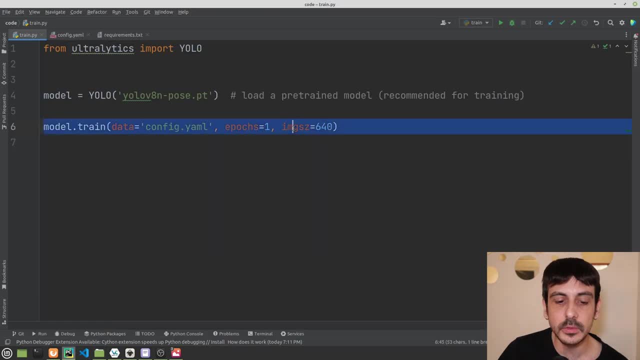 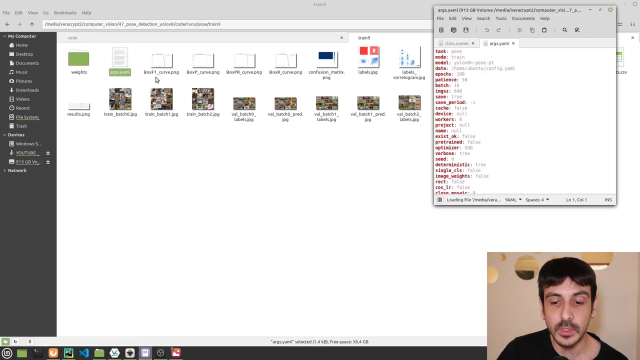 remember that we are always using the default values of this training right. we are training this model using all the default values. the only values we are specifying are the image size and the number of epochs, and that's it. and if i show you the entire configuration file, we are 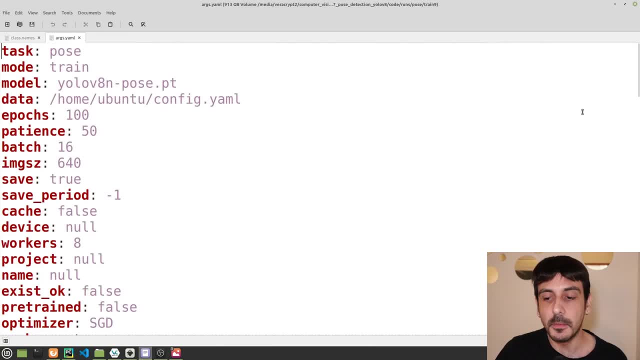 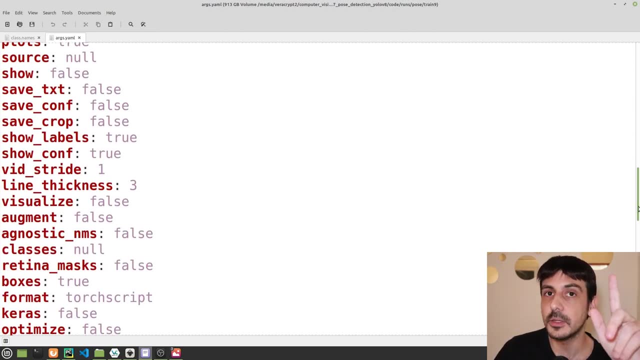 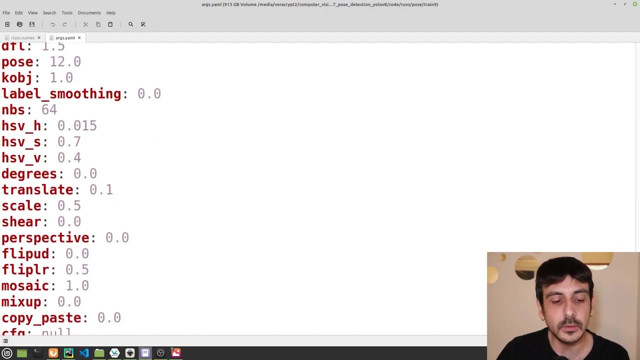 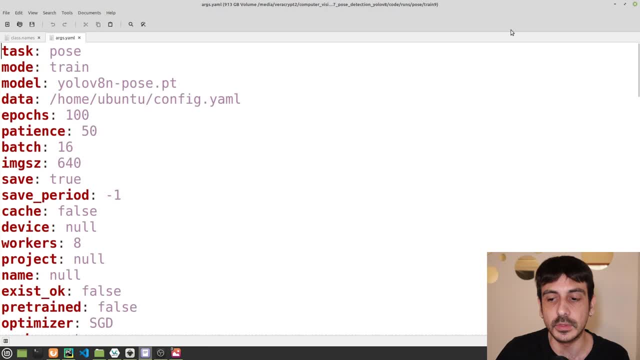 combination of parameters which will be better for our use case. that's very important because if you are approaching a more complex problem like this one, like the one i am doing right now, i will say that it's not very realistic to expect everything goes super, super well from the first. 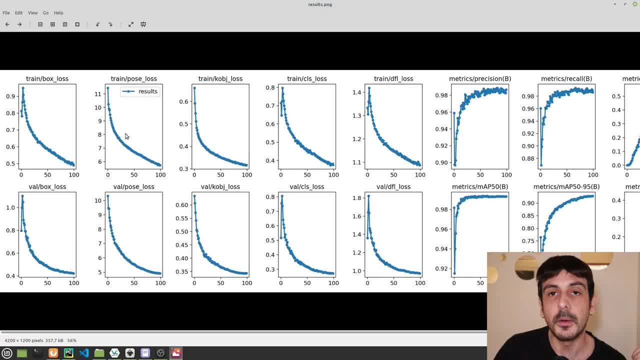 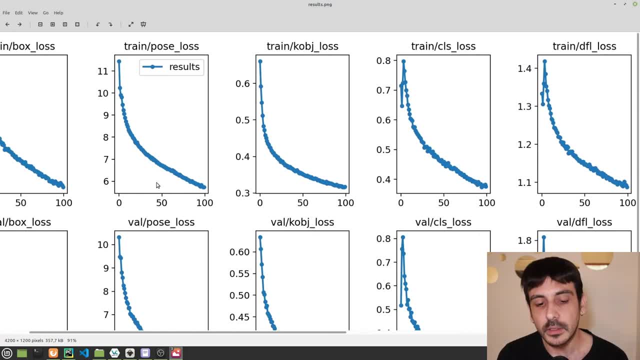 from the first attempt by using all the default values. right? i will say, if you're, if you, the problem you are trying to solve it's much more complex- then most likely you will need to play around with the different parameters and you will need to find a combination of parameters. 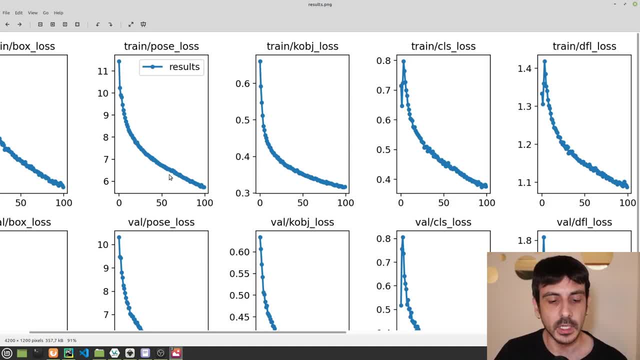 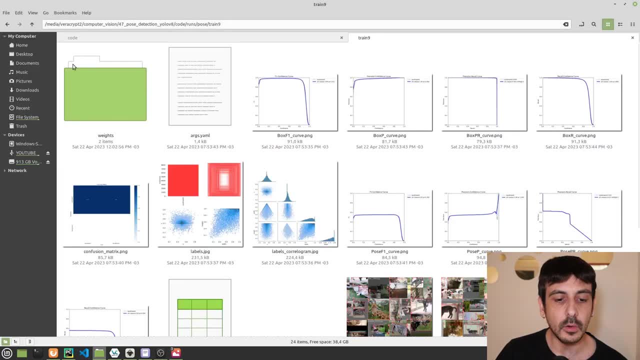 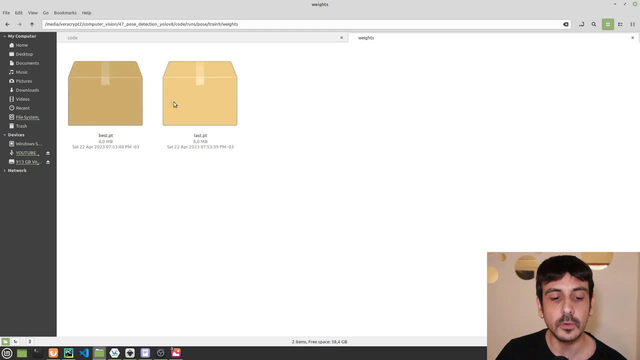 that suits well with your problem, with your project. so that's what i can say about this validation process. and now let me show you something else, which is where the weights are located. within this folder, you will see another folder which is called weights, and within weights you are going to see: 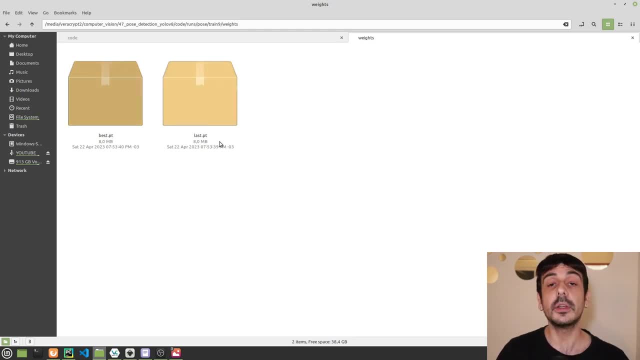 two files, which are bestpt and lastpt. these are the models you generated with this training process, and this is something that i have already mentioned in my previous tutorials, but i'm going to say it again: lastpt is the model you trained at the end of your training process, and bestpt 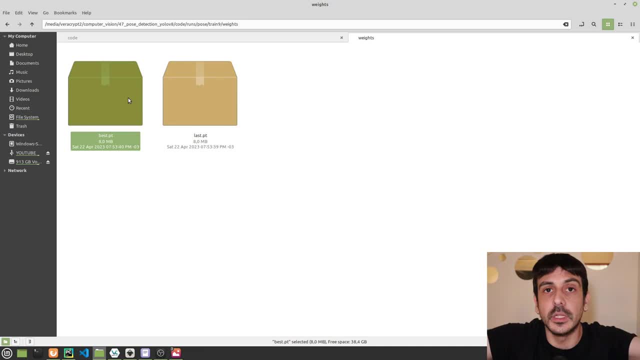 means that this is the best model you trained in the entire training process. so you have these two, the one you like the most, and what i usually do is taking lastpt. i consider that this is a much more robust model, so this is the one i usually consider when i'm making my predictions, and that's. 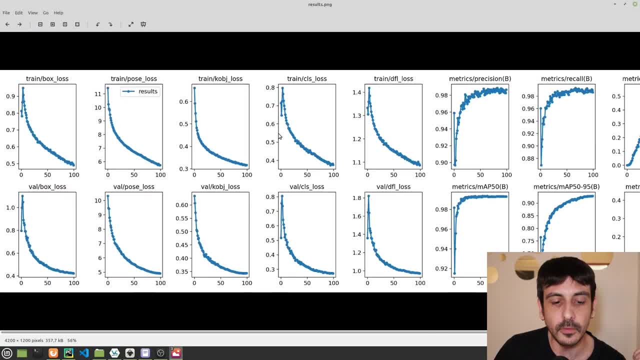 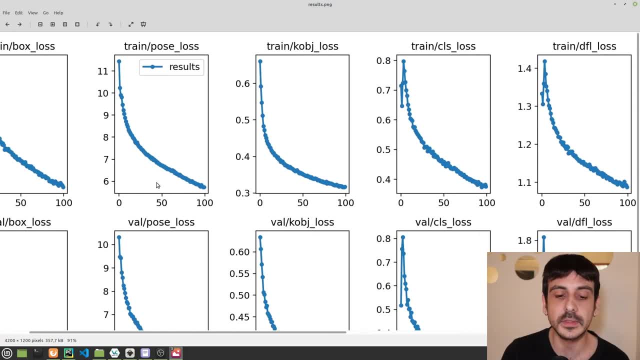 well, from the first attempt by using all the default values. right? i will say, if you're, if the problem you are trying to solve it's much more complex, then most likely you will need to play around with the different parameters and you will need to find a combination of parameters. 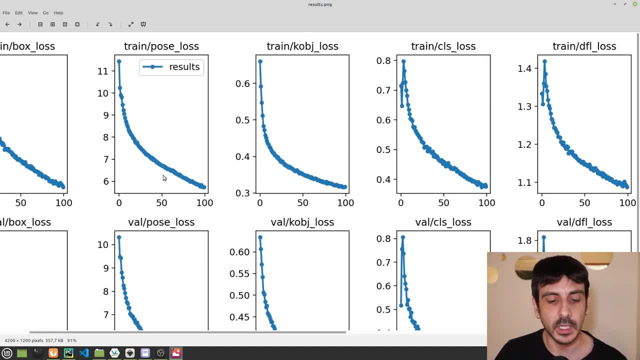 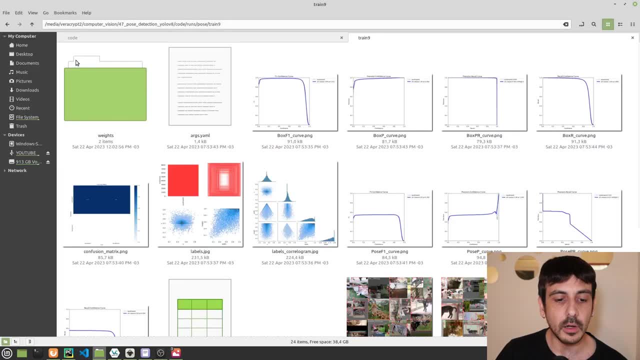 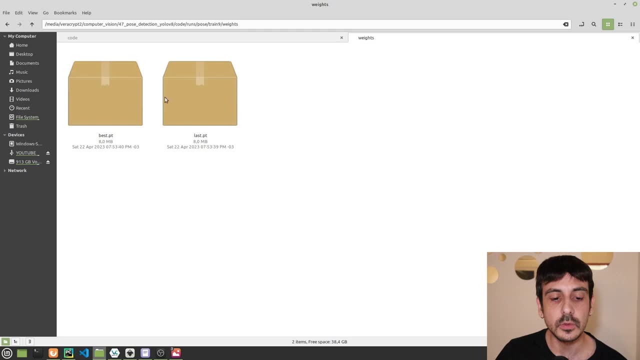 that suits well with your problem, with your project. so that's what you can say about this validation process. and now let me show you something else, which is where the weights are located. within this folder, you will see another folder which is called weights, and within weights you are going to see: 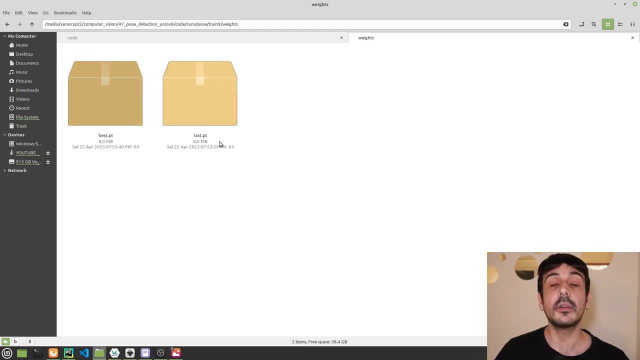 two files, which are bestpt and lastpt. these are the models you generated with this training process, and this is something that i have already mentioned in my previous tutorials, but i'm going to say it again: lastpt is the model you trained at the end of your training process, and bestpt 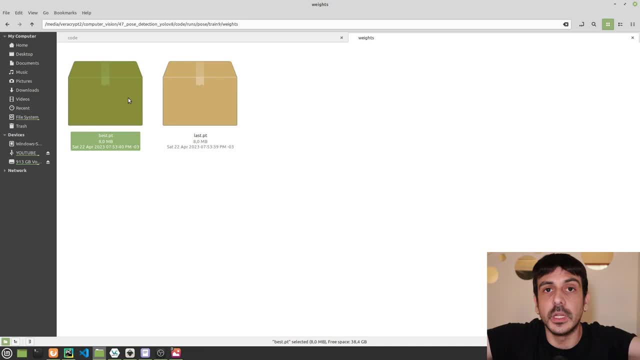 means that this is the best model you trained in the entire training process. so you have these two models and you can just choose the one you like the most, and what i usually do is take in lastpt. i consider that this is a much more robust model, so this is the one i usually consider when i'm 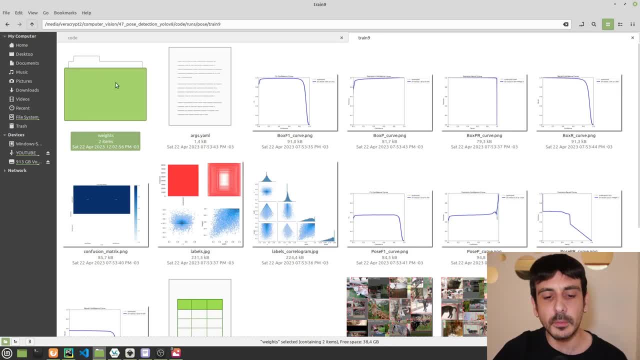 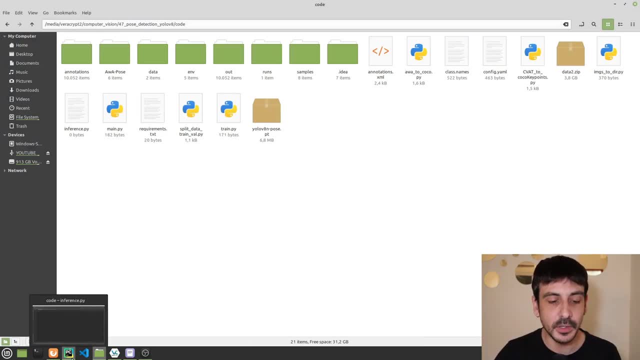 making my predictions. that's pretty much all i can say about this validation, about validating this model, and now it's time to make our predictions. so let's get back to pycharm and let me show you this file, which is called inferencepi. this is the file we are going to use in order to 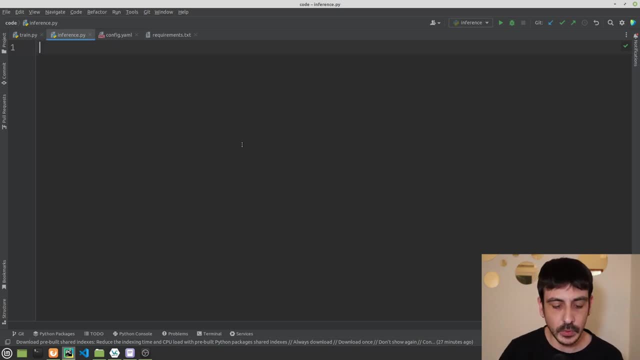 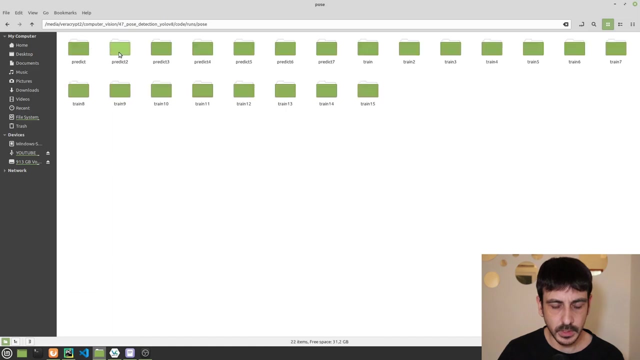 make predictions with the model we just trained. so let me show you how to do it. i'm going to start importing from ultralytics import yolo- ultralytics import yolo, and then i'm going to define my model path. i am going to specify the location of the model we just trained right, which is this one: 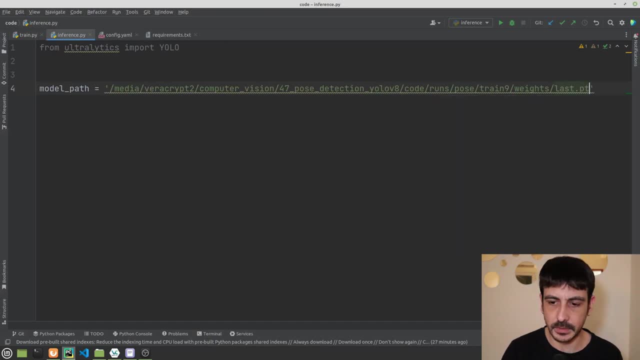 in my case, this is the location of my model. i'm going to select lastpt and i'm also going to set the path to an image, to an image i'm going to use in order to show you how to make predictions. my image will be located in samples- wolfjpg. let me show you super quickly the image i'm going to. 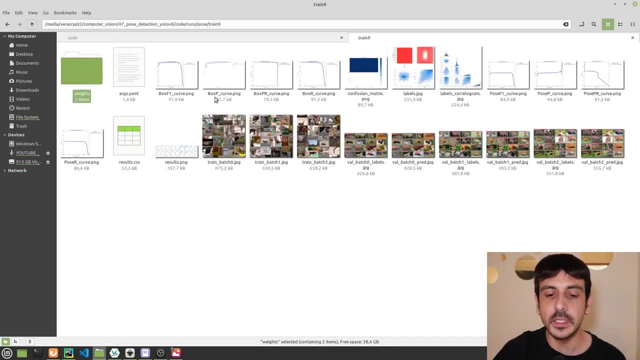 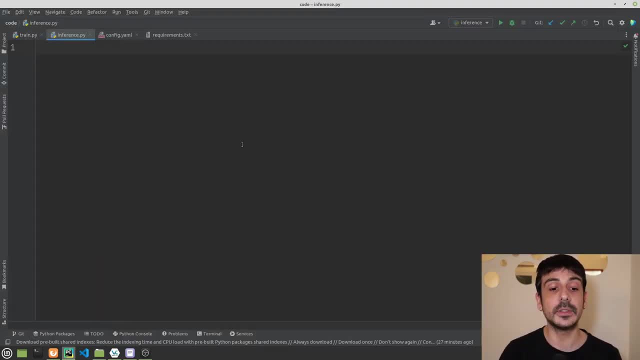 pretty much all i can say about this validation, about validating this model, and now it's time to make our predictions. so let's get back to pycharm and let me show you this file, which is called inferencepi. this is the file we are going to use in order to make predictions with. 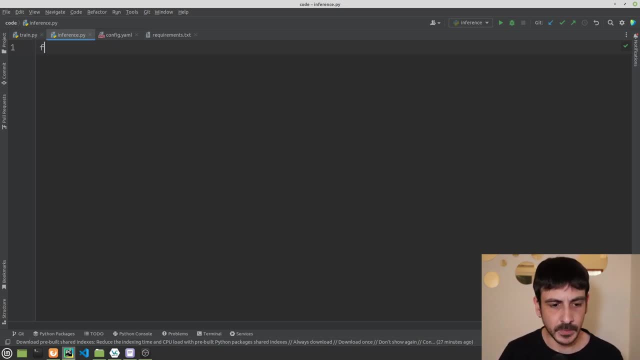 the model we just trained. so let me show you this, and these are the models that i have designed today: you how to do it. i'm going to start importing from ultralytics import yolo, ultralytics, import yolo, and then i'm going to define my model path, i am going to specify, 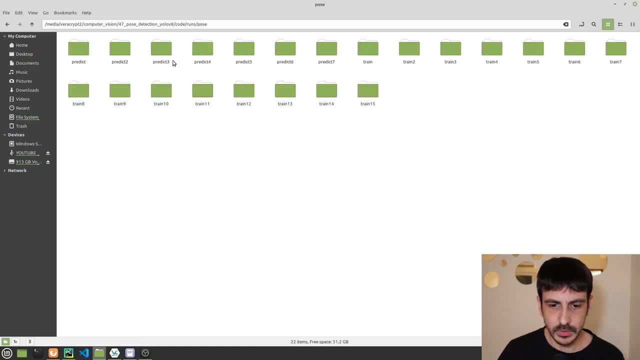 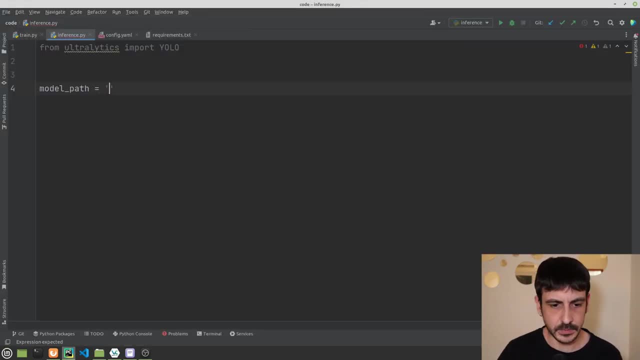 the location of the model we just trained right, which is this one in my case. this is the location of my model. i'm going to select lastpt and i'm also going to set the path to an image, to an image i'm going to use in order to show you how to make predictions. 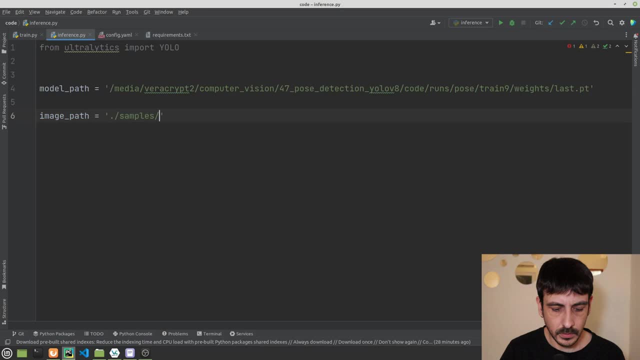 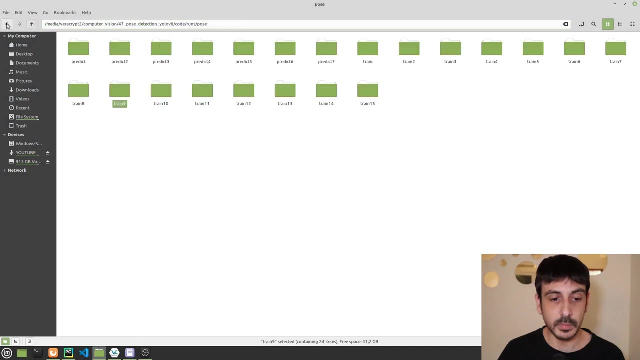 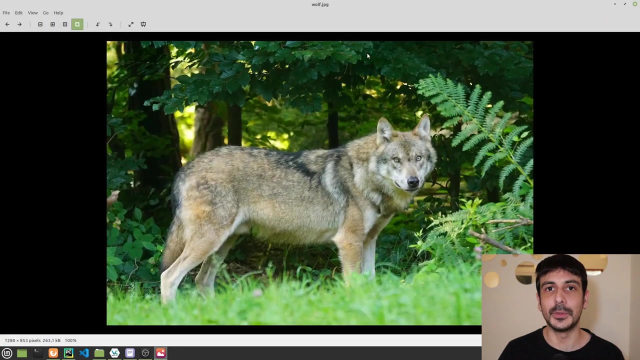 my image will be located in samples- wolfjpg. let me show you super quickly the image i'm going to use in order to show you how to make predictions with yellow v8. let's go to samples, and this is exactly the image i am going to use. you can see that this is the 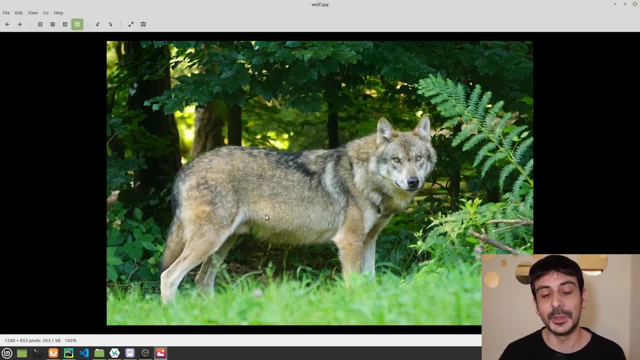 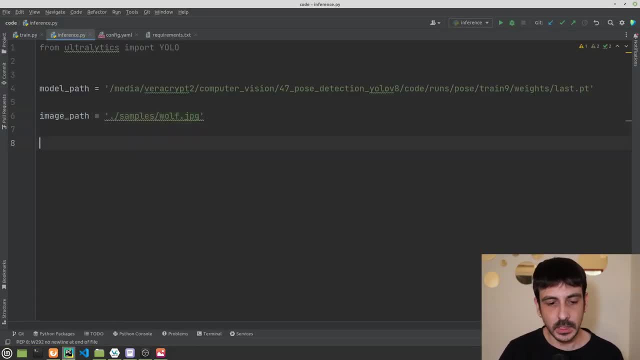 image of a wolf, which is obviously a quadruped, so it's going to be an amazing image. in order to show you how to use this model, now let's get back to pycharm and let's do something like this: i'm going to define my model like yolo model path, and then we're going to say something like results. 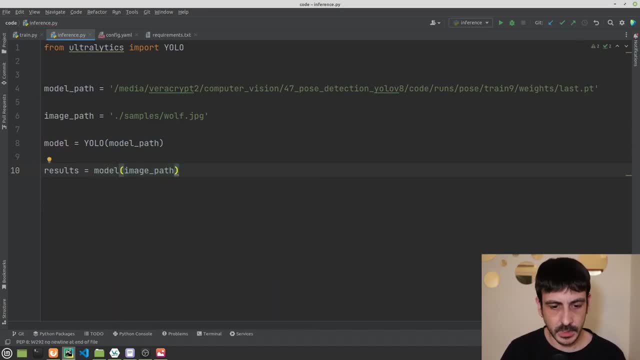 equal to model image path, and i'm going to select the first element because, as we are predicting only one image, the first element will be just fine, and then it's just about iterating for result in results, and this will be something like for keypoint in result: keypoints. 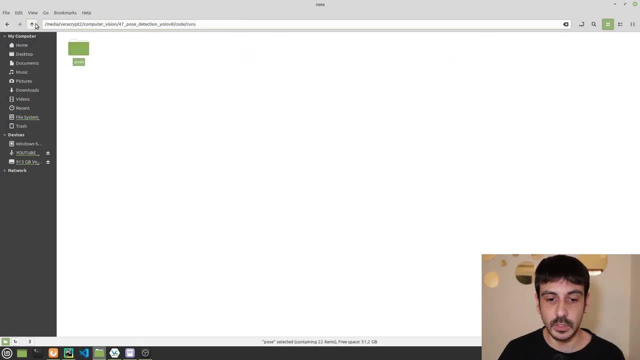 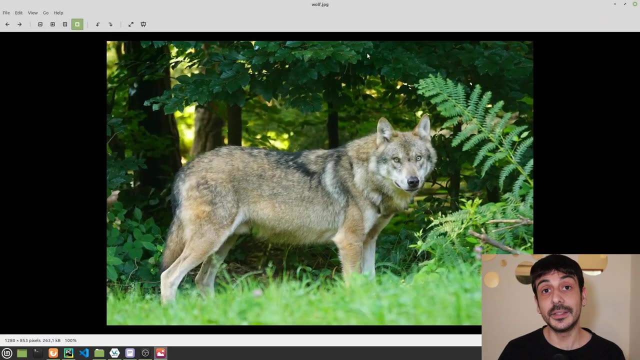 use. in order to show you how to make predictions with yolo v8, let's go to samples, and this is exactly the image i am going to use. you can see that this is the image of a wolf, which is obviously a quadruped, so it's going to be an amazing image. in order to show you how to use this model now, 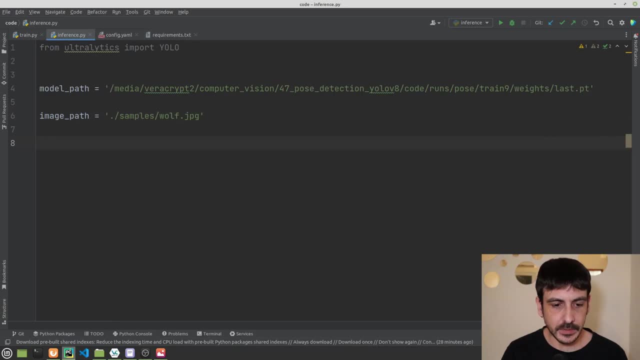 let's get back to pycharm, pycharm and let's do something like this: i'm going to define my model like yolo model path, and then we're going to say something like results equal to model image path. and i'm going to select the first element because, as we are predicting only one. 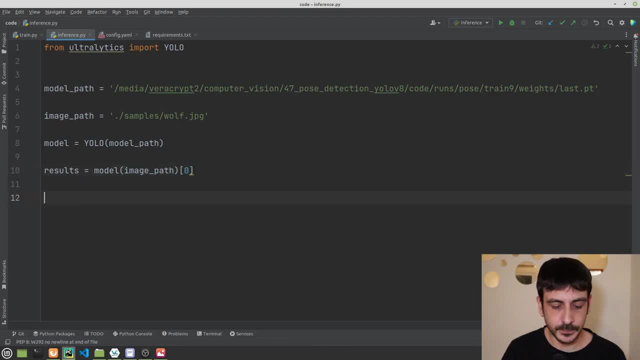 image. the first element will be just fine, and then it's just about iterating for result in results and this will be something like for keypoint in result, keypoints dot to list there. and for now the only thing i'm going to do is to print keypoint. so we make sure everything is okay and let's see what happens. 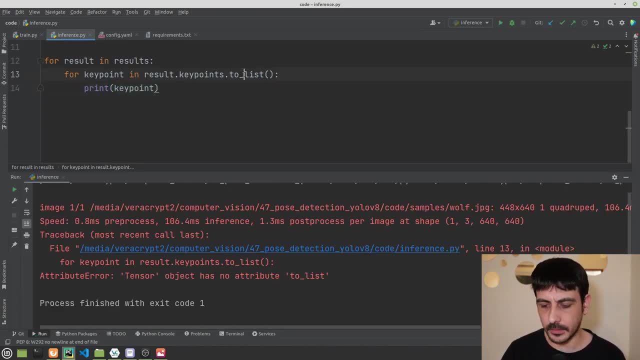 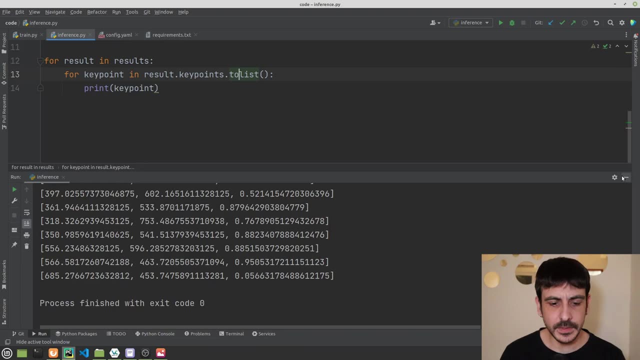 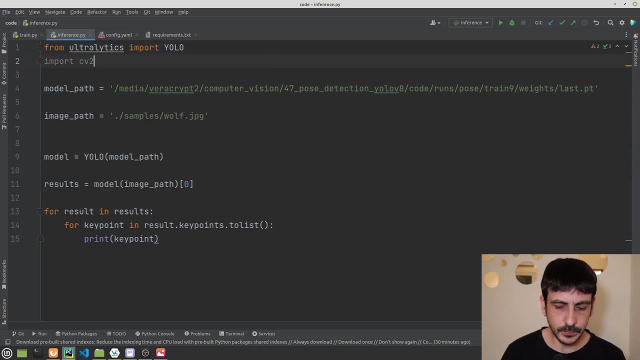 okay, it seems i have an error, and i think i know what's the error. to list goes with the without the underscore. so let's see now. okay, now everything seems to be okay, and what i'm going to do now is i'm going to import cv2, because i am going to read the image and i am going to plot all the 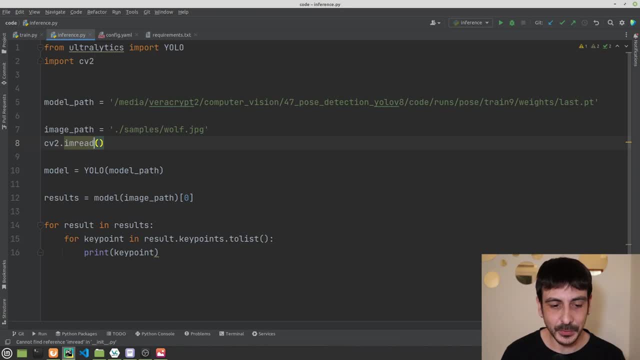 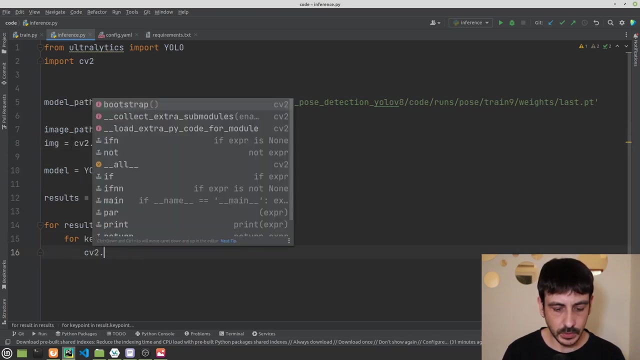 key points on top of this image. right, that's going to be a very good way to show you how to predict a keypoint, so i'm going to create all these key points. so cv2 in read image path. this is going to be image, and now i'm going to call cv2, dot put text. maybe it's a very good idea. 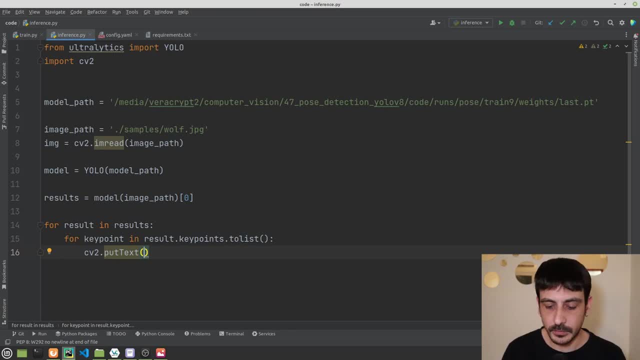 to put the text of each one of these key points, to put the key point number on top of each one of these key points. so this is going to be image. then the key point number will be. let's do it like this: key point index. key point in enumerate. 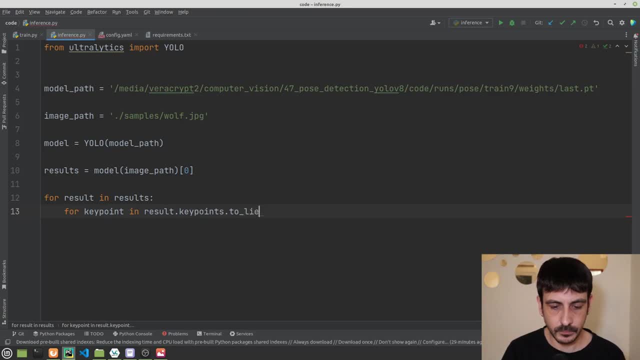 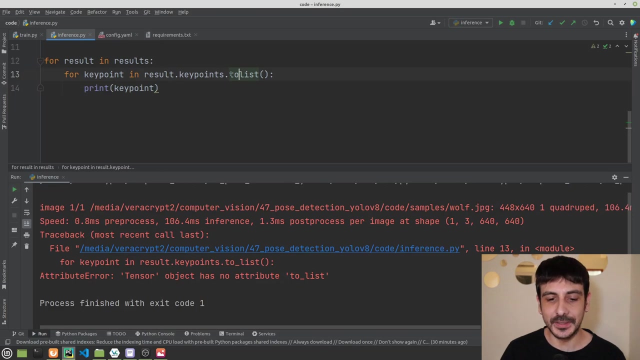 dot to list so that everything is okay. so let's see what happens there and for now, the only thing i'm going to do is to print key point so we make sure everything is okay and let's see what happens. okay, it seems i have an error and i think i know what's the error. to list goes with the without. 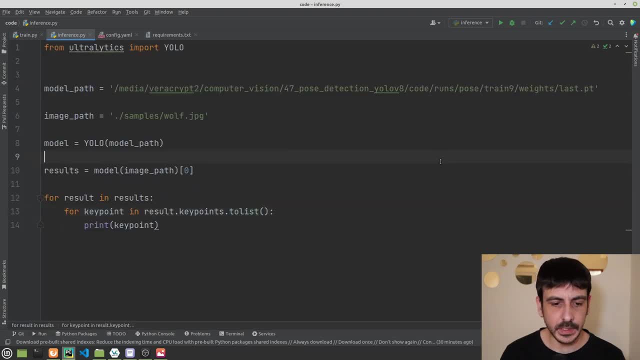 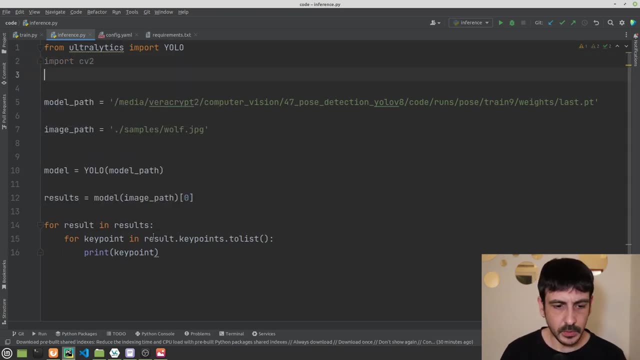 the underscore. so let's see now- okay, now everything seems to be okay- and what i'm going? I'm going to import cv2 because I am going to read the image and I'm going to plot all the key points on top of this image. right, that's going to be a very good way to show you how to predict. 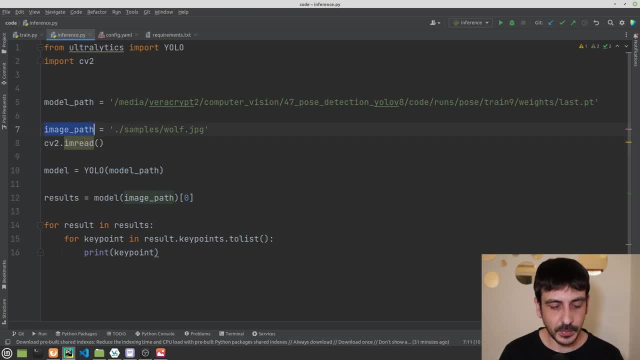 all these key points. so cv2 in read image path, this is going to be image. and now I'm going to call cv2 dot put text. maybe it's a very good idea to put the text of each one of these key points, to put the key point number on top of each one of these key points. so this is going to be image. 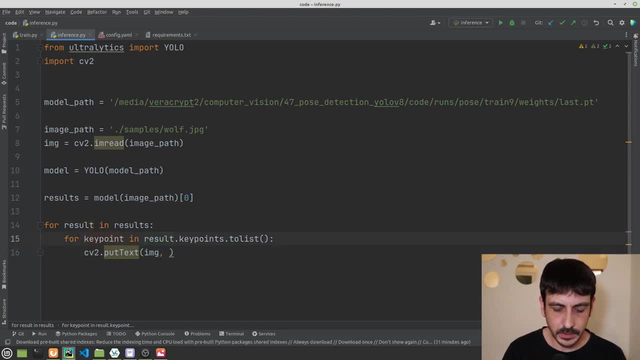 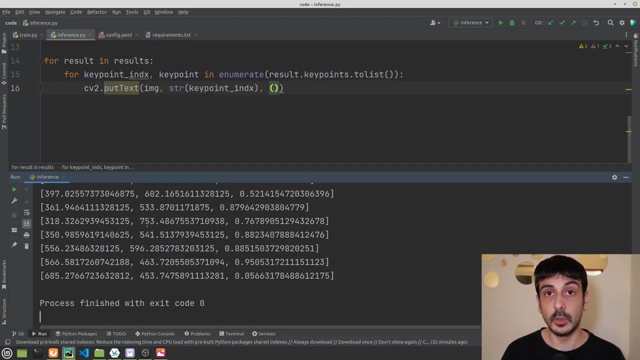 then the key point number will be. let's do it like this: key point index, key point in enumerate- okay, and then string: key point index. okay, now the location, and remember. this is how my key points look like. we have three values, and the values we care about in this moment are these two, because 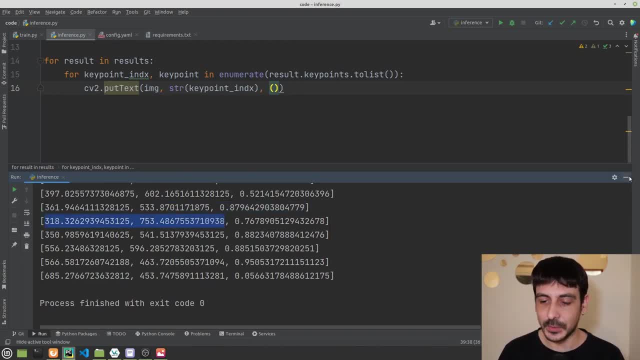 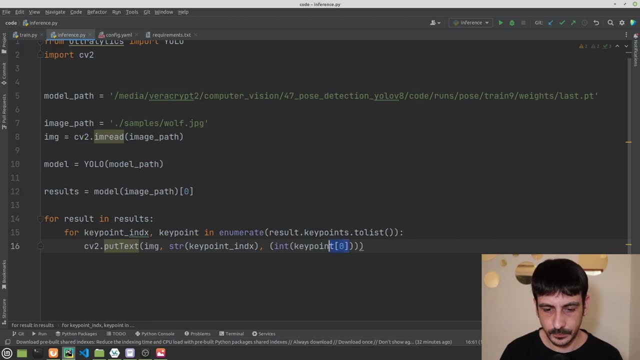 these are the XY position of the key point, so I'm just going to do something like int- key point zero and int- key point one. okay, now I have to select the font which I'm going to set in this one font- cursive, simplex, then the font size, which I'm going to set in one for now. 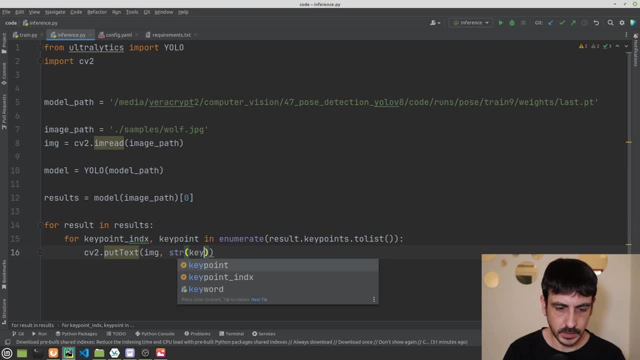 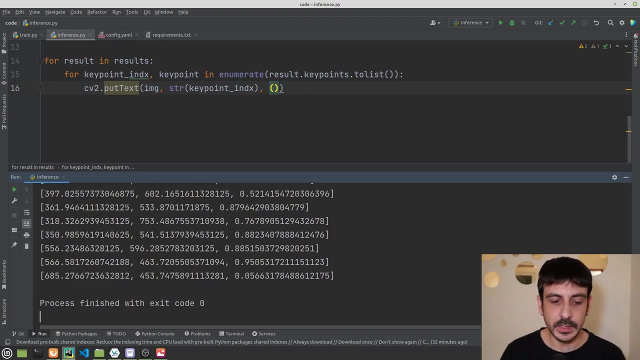 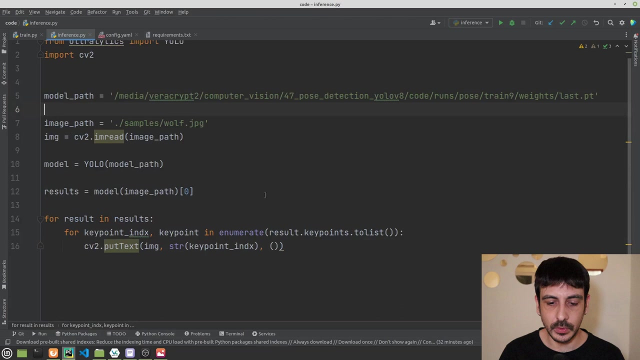 okay, and then string key point index. okay, now the location, and remember, this is how my key points look like. we have three values and the values we care about in this moment are these two, because these are the x, y position of the key point. so i'm just going to do something like int, keypoint 0. 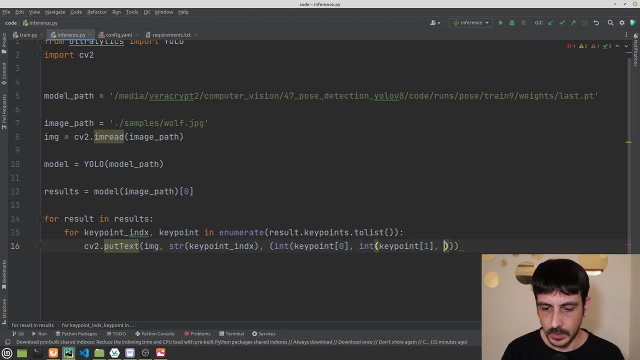 and int keypoint one. okay, now i have to select the font which i'm going to set in this one font, kershi simplex, then the font size, which i'm going to set in one front now, then the color. something is not right. let me see, i think i'm not closing these brackets. 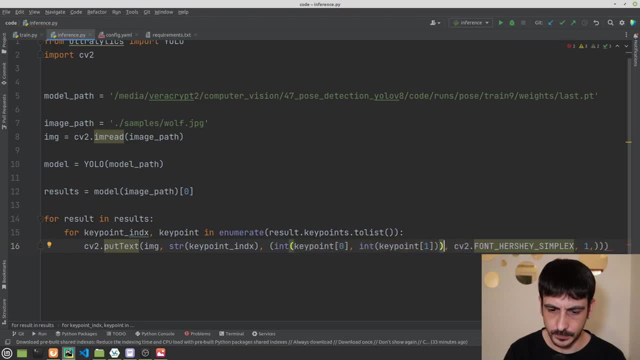 i think that's reason one. two: okay, there, let's see. now everything's okay, okay. okay. now the color, which i'm going to set in green, so this is something like this, and then the, the text width, which i'm going to set in two, and this is going to be all for now. now let's see. 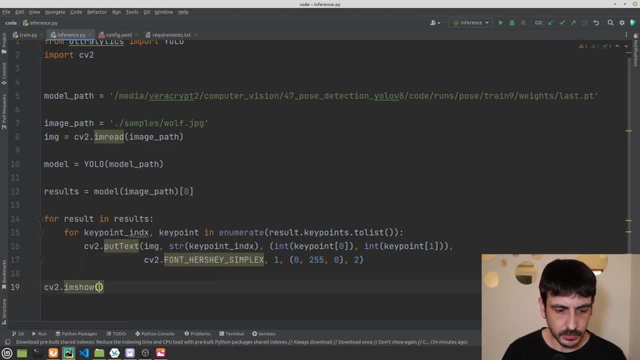 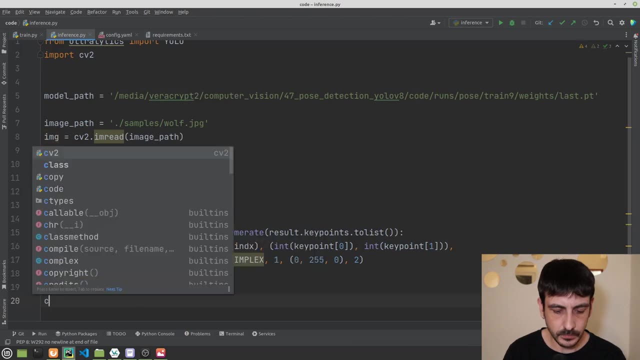 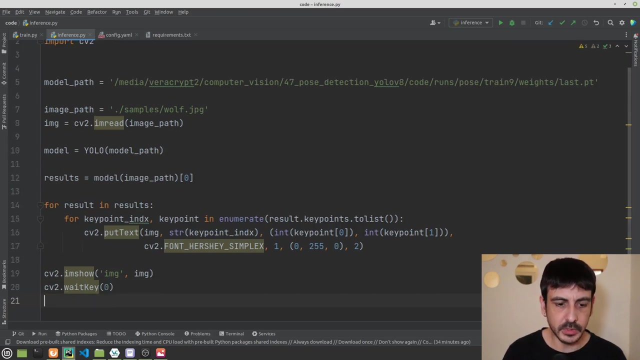 how it looks like. right, i'm going to call cv2 in show image and my image then cv2, white key. okay, zero, okay, and that's pretty much all what we are doing here is plotting the image and drawing all the key points on top of this image with the key point number on each key point. right, so it's going. 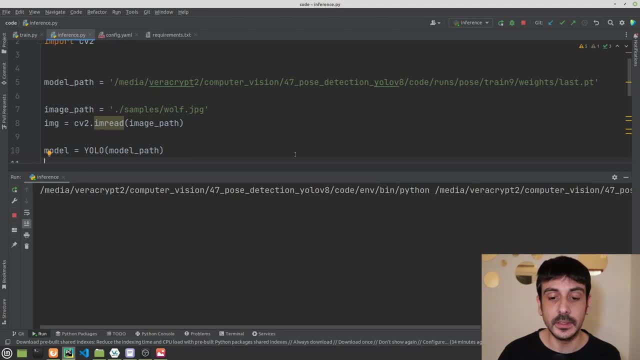 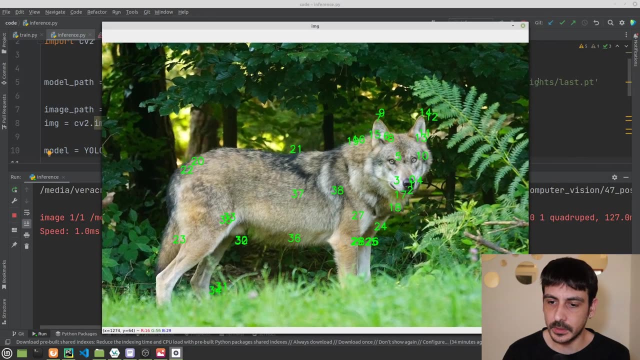 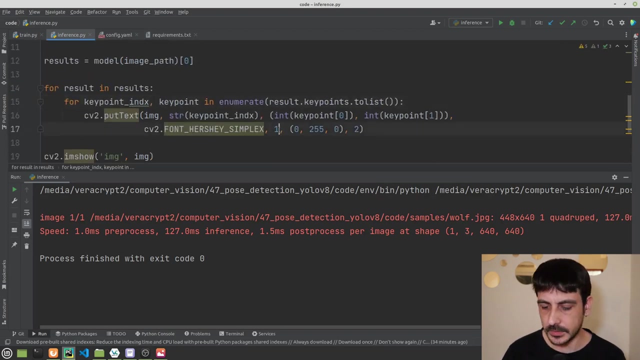 to be easier to know exactly what we are detecting in the entire image. and this result: everything looks pretty well. but i'm going to do something so i can improve the visualization. i am going to make the font size equal to 0.5 and i'm going to press play again. okay, now the visualization is a. 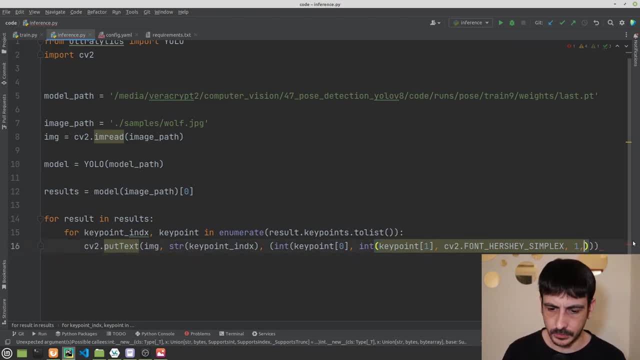 then the color. something is not right. let me see, I think I'm not closing these brackets. I think that's reason one to okay there. let's see, now everything's okay, okay, okay. now the color, which I'm going to set in green: so this is something like this. and then the it takes width, which I'm going to set in two. 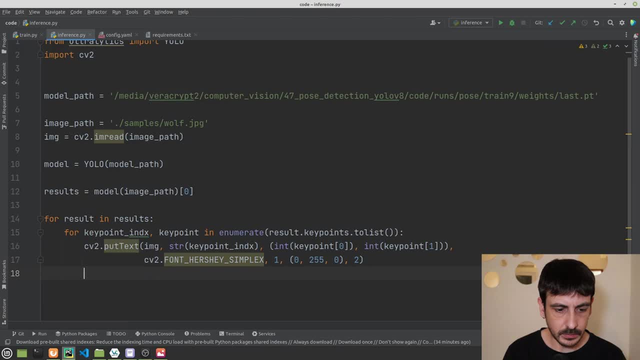 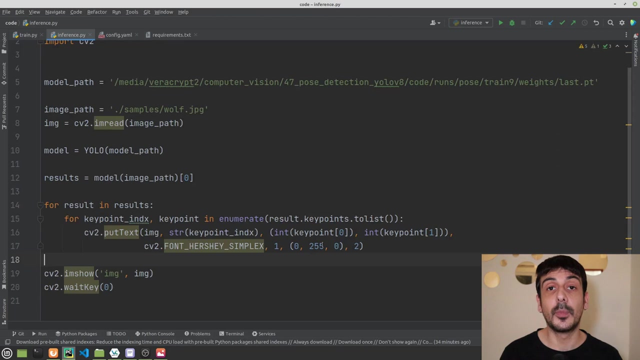 and this is going to be all for now. now let's see how it looks like, right? I'm going to call cv2- imshow image and my image, then cv2- weight key zero. okay, and that's pretty much all what we are doing here is plotting the image and drawing all the key points on top of this image with the key. 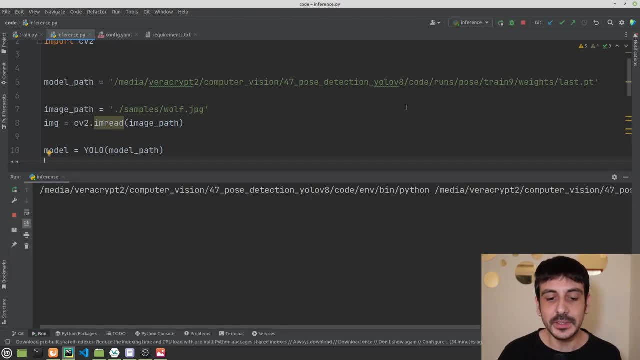 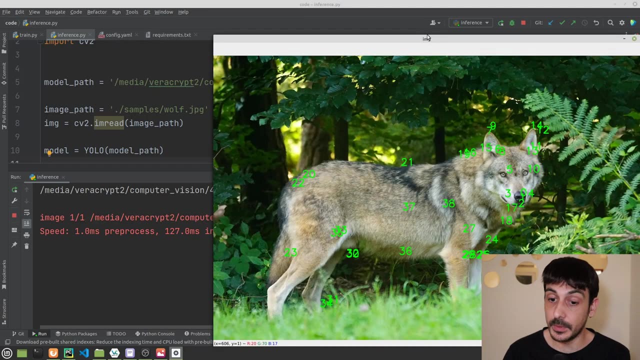 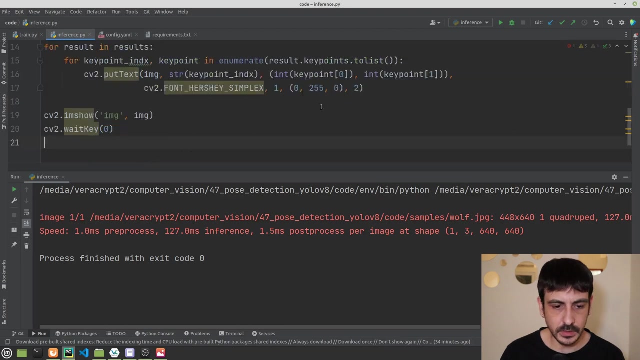 point number on each key point, right. so it's going to be easier to know exactly what we are detecting in the entire image. and this is the result. everything looks pretty well. but i'm going to do something so i can improve the visualization. i am going to make the font size equal to 0.5. 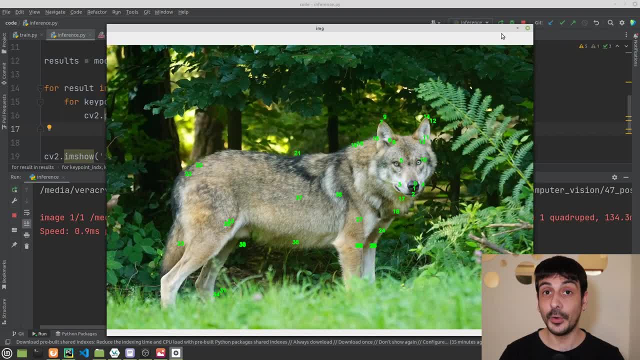 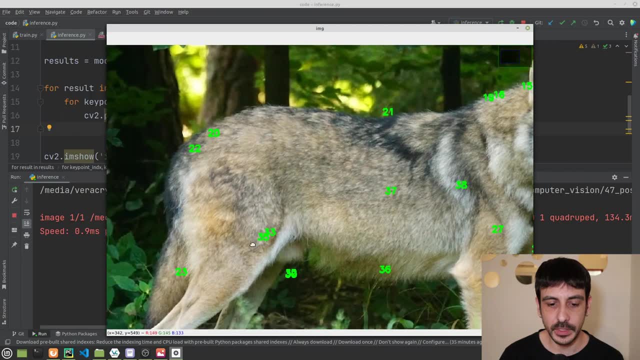 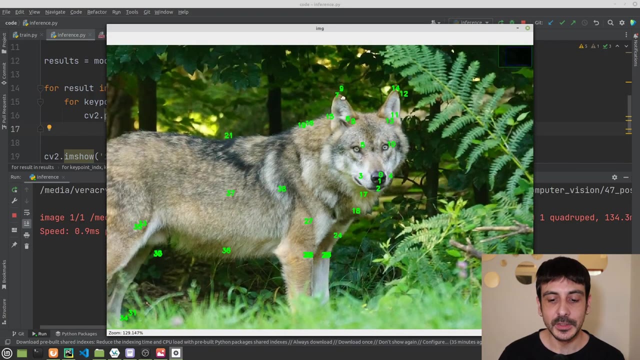 and i'm going to press play again. okay, now the visualization is a little better and you can see that everything looks pretty pretty well. right, we are plotting all the key points on top of our image, and this is exactly how you can make predictions using yellow v8. so the last thing i'm going to 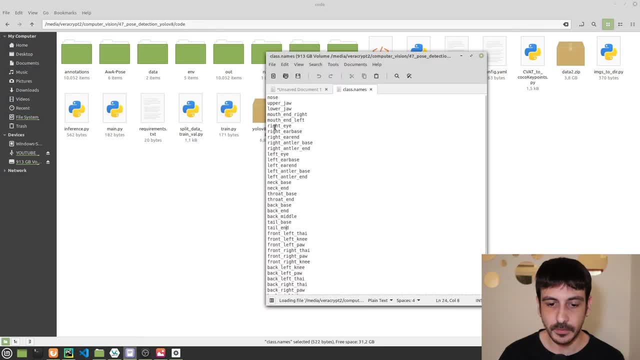 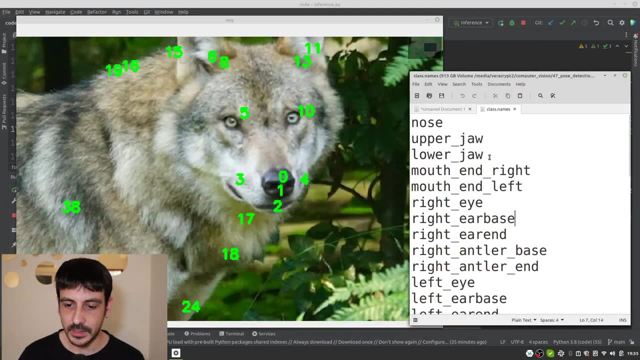 show you is to open this file, the class names and let's take a look at exactly what we are detecting. right, so you can see here, zero, we have the nose, then upper jaw, lower jaw, mouth and right mouth and left and so on. right, you can see that, for example, 21, we are somewhere around. 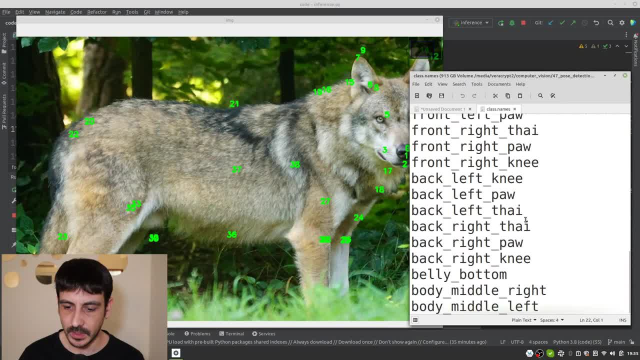 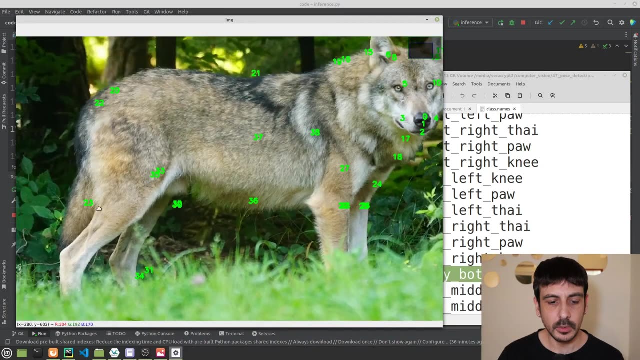 here, which is back middle, it makes sense- then 37- we are around here body middle, right, and then 36 belly bottom. so everything looks pretty, pretty well and you can see that we are still getting the issues we notice in the other pictures, which is, the legs are not very well detected and the